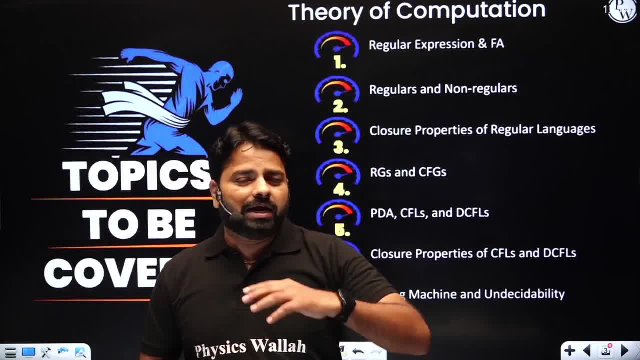 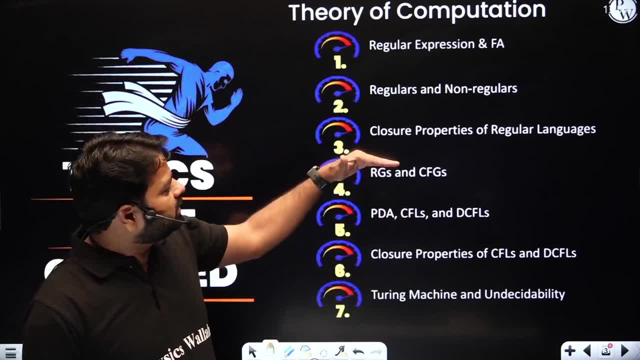 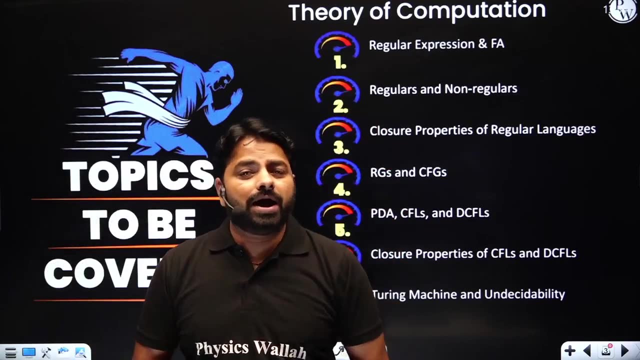 kinds of operations which are required to understand, like what is the union of two regular languages and intersection and so on. then we will go for the second. uh, you can think, as it's the second part, as the first part you will be covering with all the basics and all the important. 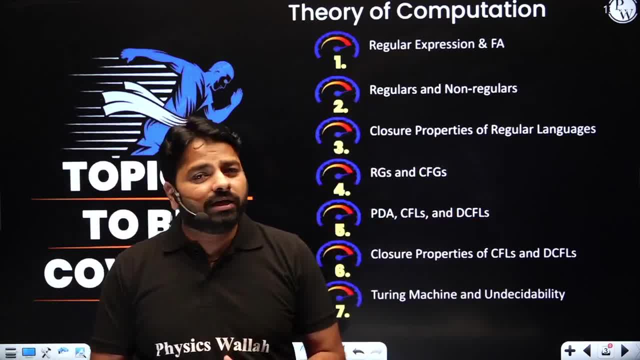 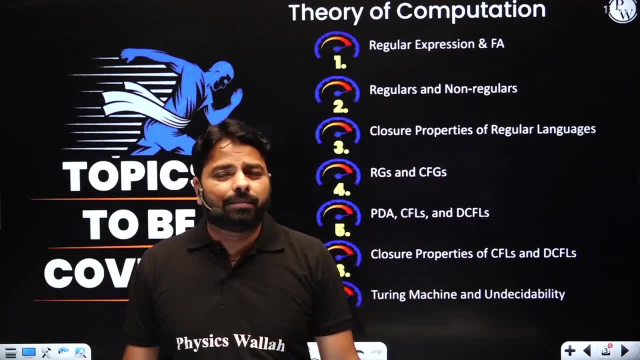 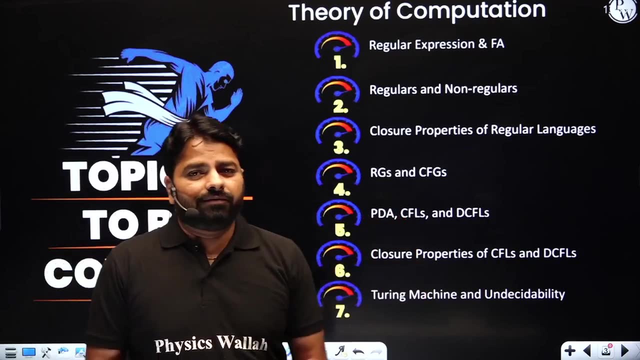 concepts. maybe you will have half of the weightage of the toc in this, the first three topics. sometimes then we will have the grammars, where regular grammar and context-free grammar- both- are discussed. then we have the pushdown automata, along with the various languages which are context-free. 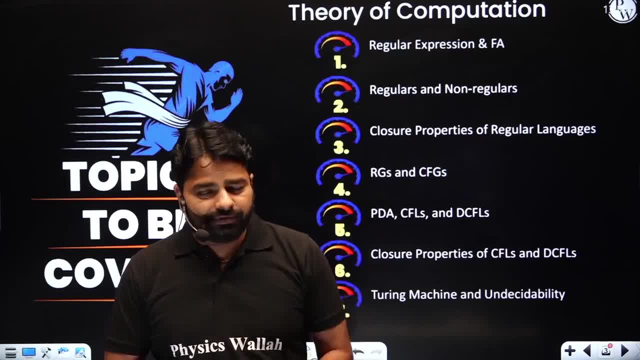 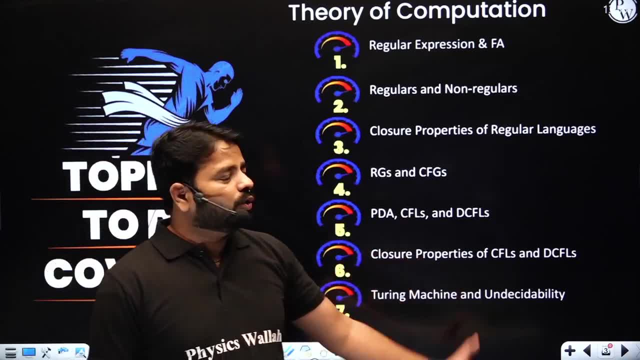 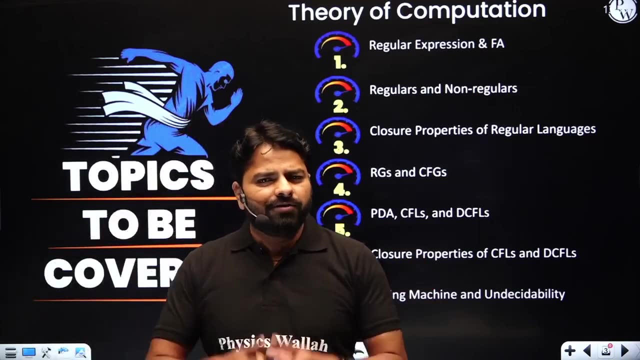 languages and also deterministic context-free languages. here we'll be learning how to identify cfl's and dcfl's. then we have the sixth video closure properties of cfl's and dcf's. okay, then finally, the theory of computation, motion and undecidability. if you look at the weightage of this theory of computation, then 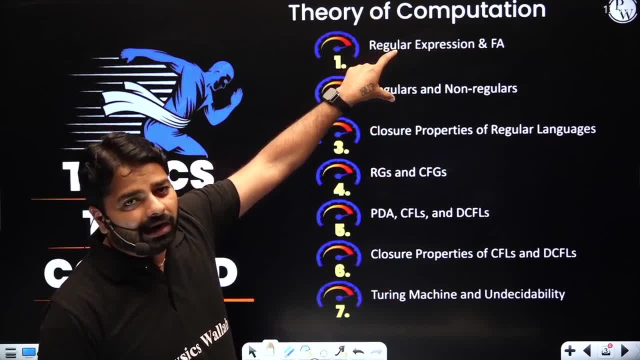 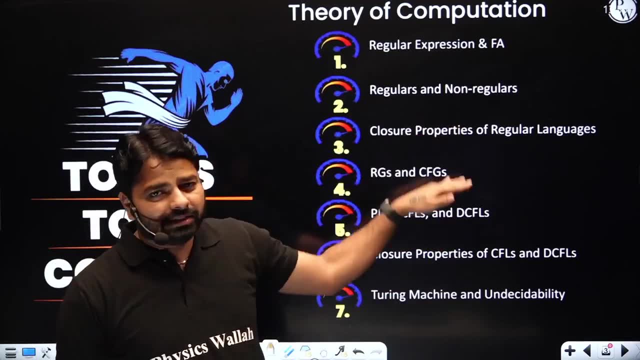 the first, the two topics will have at least two to three marks and the last topic you will be having around two marks and then remaining marks will lie somewhere in this, and closure properties are very important here: closure properties of regular languages and closure properties of cfl's and 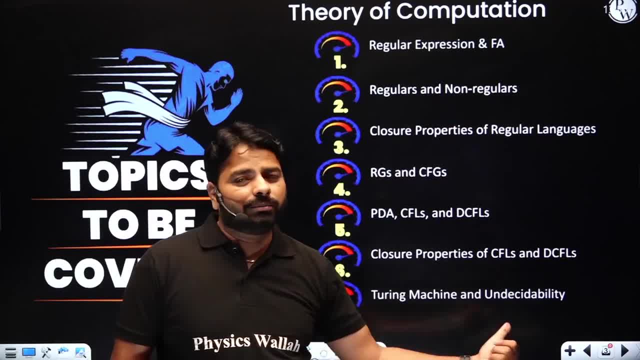 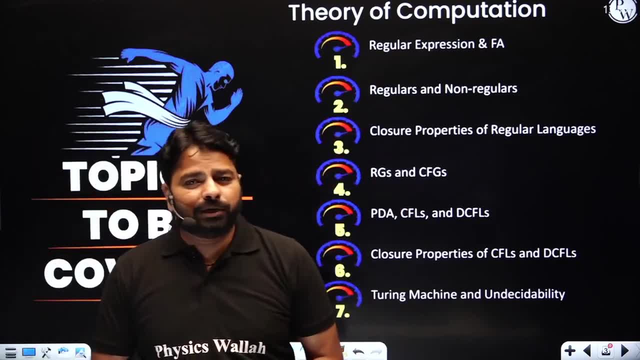 dcf's and one more closure properties i'll be covering in turing motion, which is for recursive languages and recursively enumerable languages. so this is the second part of the theory of computation. let's begin with the first topic: regular expressions and finite parameter. do you think that? 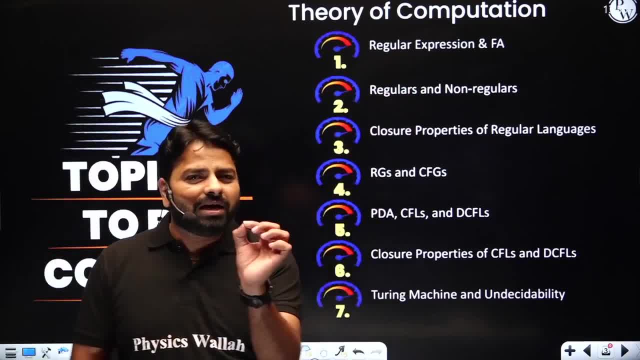 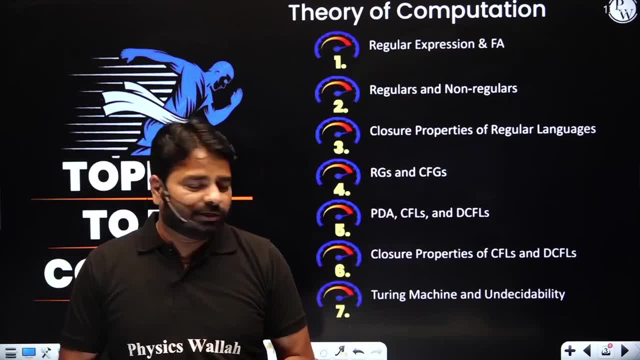 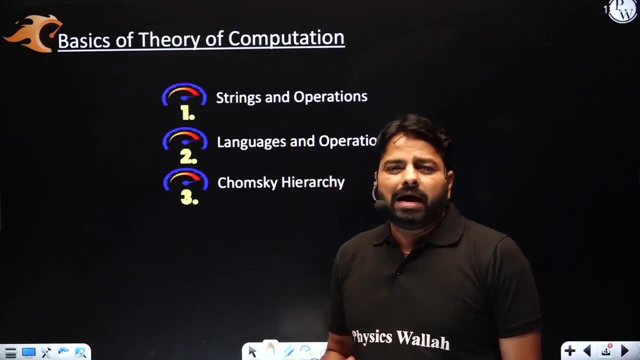 i can begin with this regular expression for an editor directly. no, so we'll have some basics before starting: regular expressions and finite parameter. then we will move to regular expressions. okay, this is what i want to explain as basics in theory of computation, where first you should know: 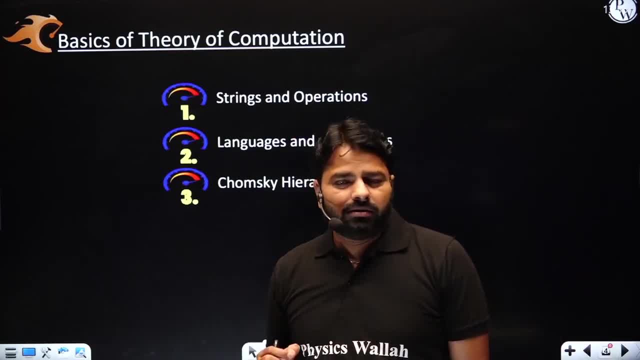 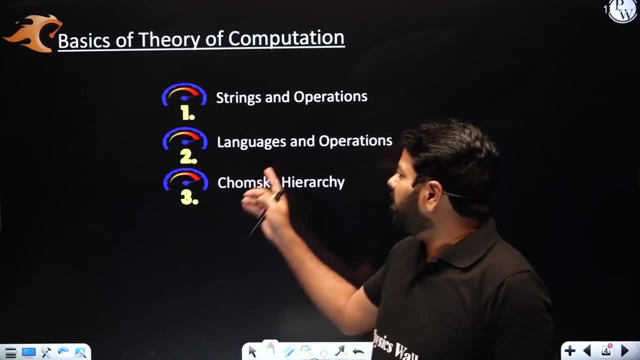 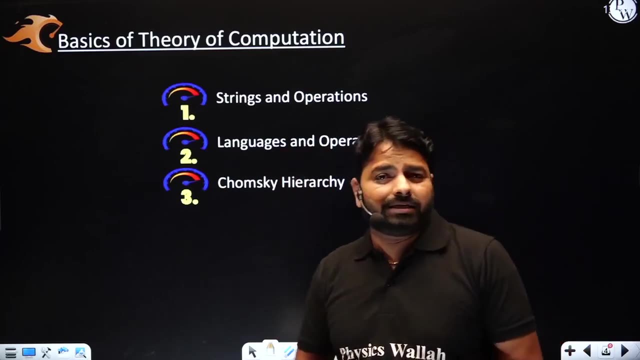 what is the string and how do you form a string for the given over the given alphabet, and what the various operations can be applied over the strings. and also what is language and what are the operations you can apply over the language. also, you know that language is called as a set right. the set synonym is here in: 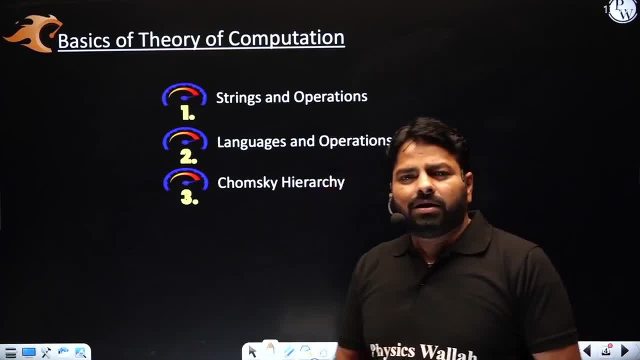 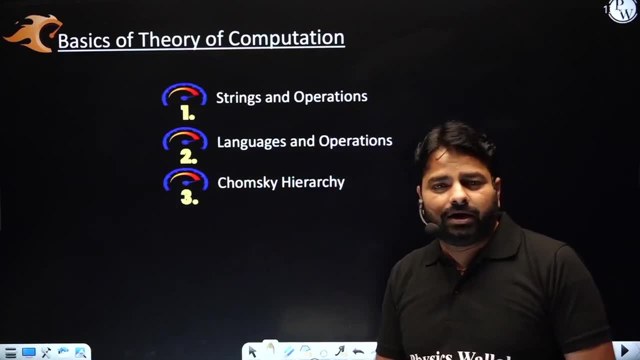 toc is a language, and then we will look at how this toc is, uh, the combined with various formal languages, with the help of chomsky hierarchy. so let's start with the first, very simple and basic to the theory of computation, that is, what is a string? 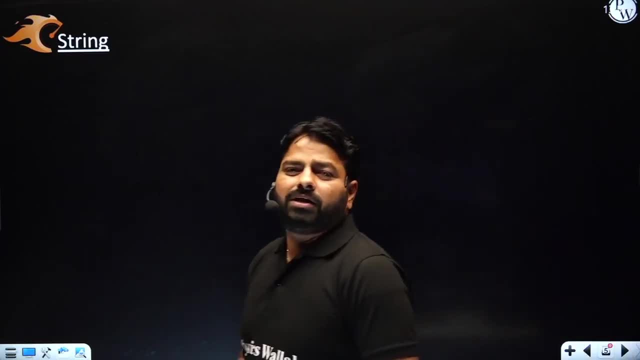 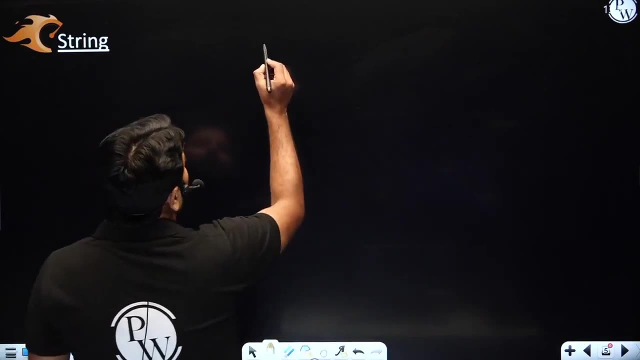 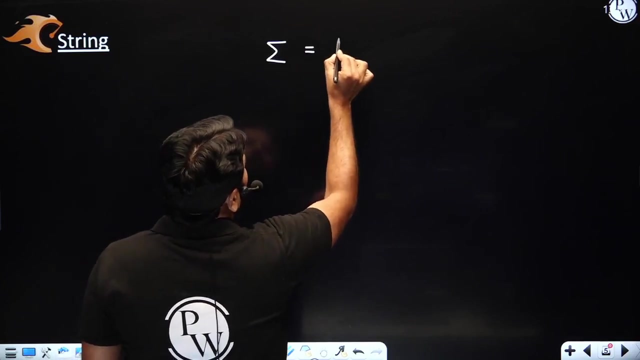 okay, yeah. so what do you need? if you want to form a string, what do you need? that is alpha bat. so first thing is you require alpha bad that you made denote with sigma where alphabet could be any set of symbols, like you may use 0 or 1, or sometimes you may use a comma b. it need not be binary alphabet, it could be even. 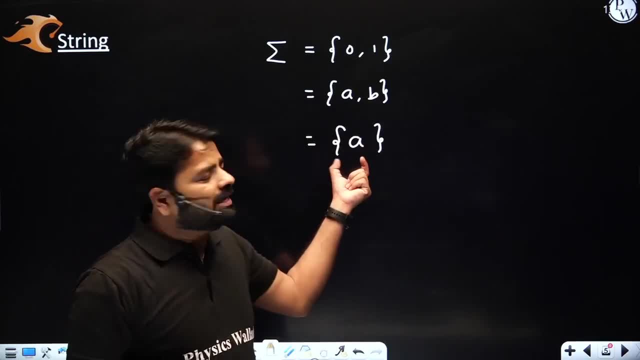 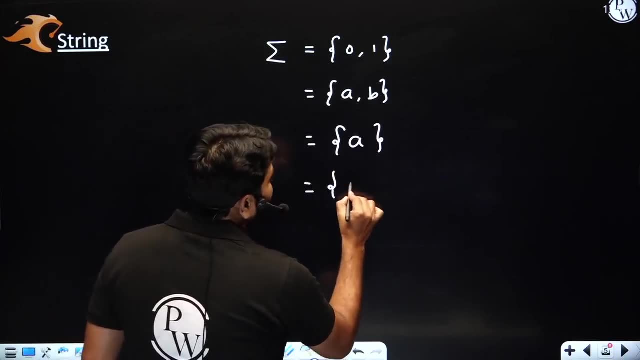 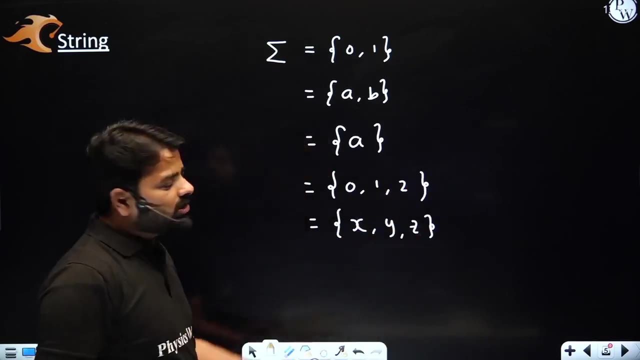 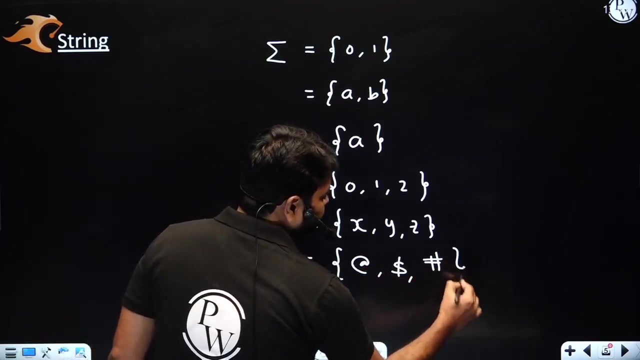 unary alphabet. unary alphabet in the sense it has only one symbol that is used to define the string or language. or you may use ternary alphabet, like 0, 1, 2, or you may use x, y, z- it need not be digits or alphabet letters. you may also use like symbols, depends on your requirement. likewise, every. 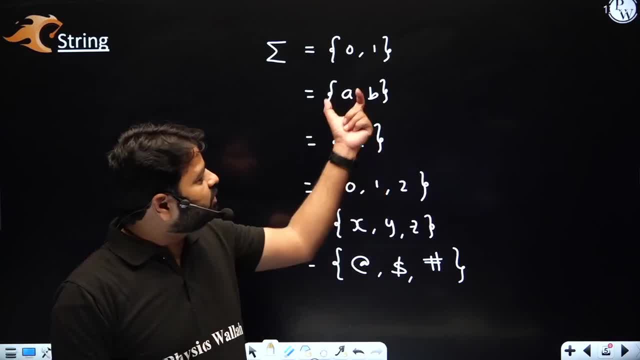 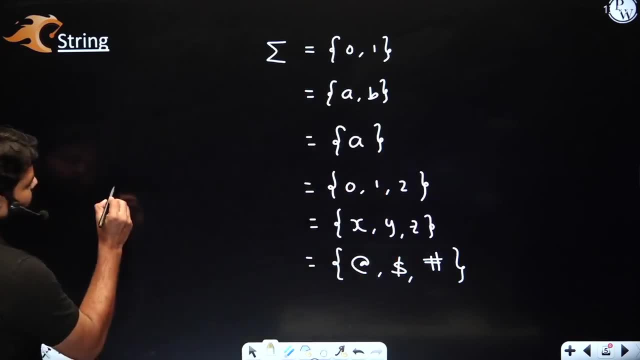 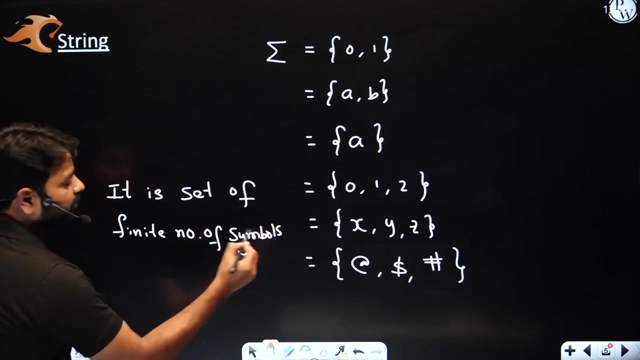 alphabet is set of symbols, but how many symbols? you can keep. finite number of symbols. if you want to know what is alphabet? it is set of finite number of symbols. it must be defined before writing any string. so first you should read what is alphabet is given in the problem. problem to problem it may. 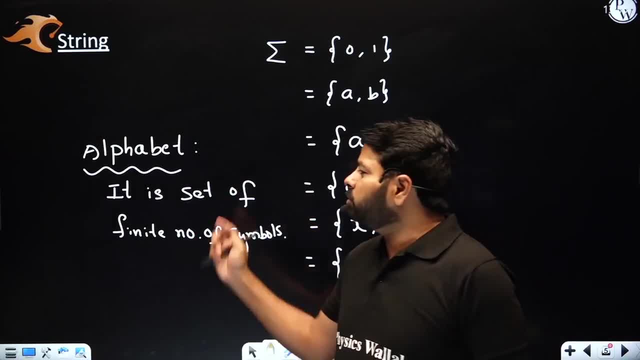 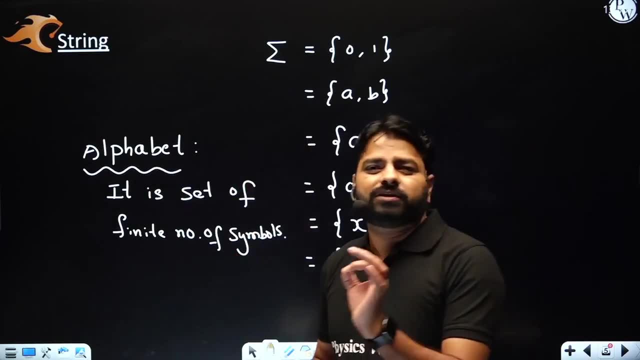 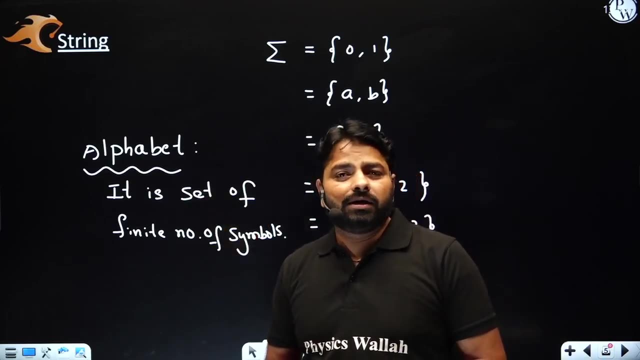 vary. so first you read what is an alphabet. using this alphabet, how you are going to form the strings of a language. so i understood. the alphabet is nothing but set of symbols, which must be finite number of symbols. as you know, if the set is infinite, it is impossible to learn the 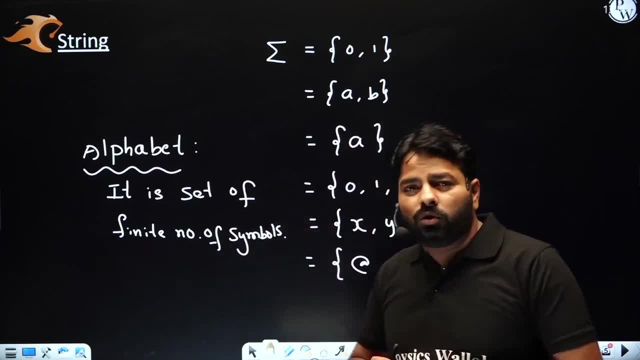 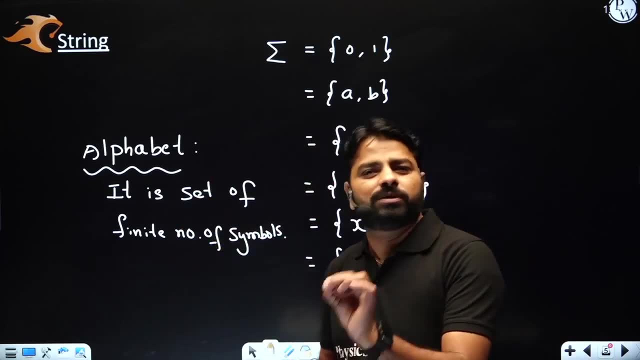 alphabet itself. so that is reason you require- like you go for english alphabet or in the alphabet or any language you take in the world- the alphabet always contain finite number of symbols. okay, so i believe what is alphabet everybody understood. now let's move to what is a string, okay? 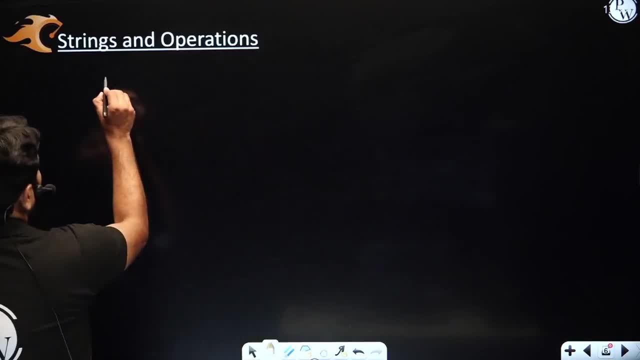 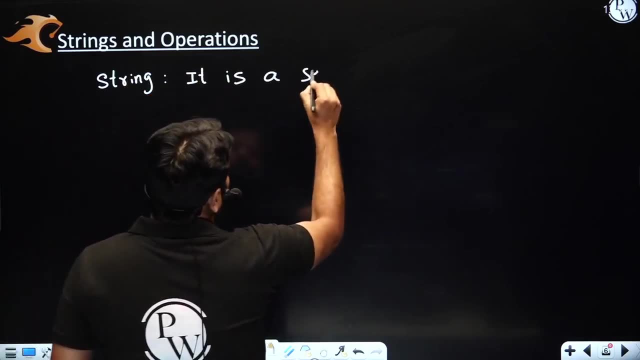 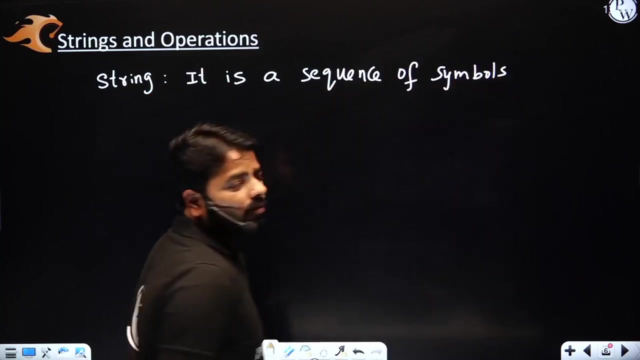 what is a string? string is a sequence. what is it? it is a sequence of the symbols, where you get the symbols defined over the sigma. so these symbols are defined over sigma. whatever the sigma has. you must take those symbols to form a string. you no need to take all the 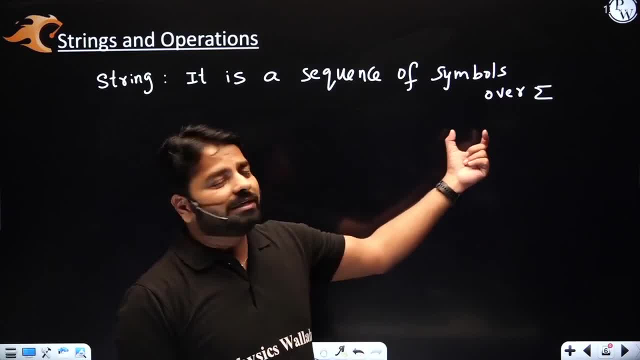 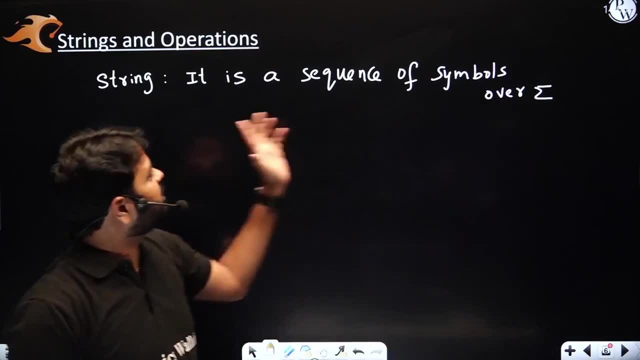 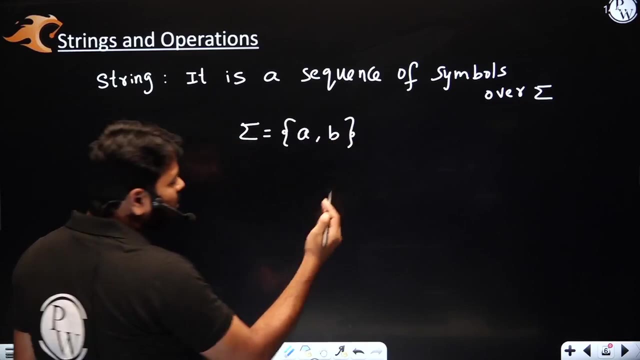 strings. but whatever the required symbols you have, you you required to form a string. what are the symbols you require to form a string you must take to form a string? let's talk about sigma, which is very famous in our subject: a comma b, or 0 comma 1 or x comma y. it's called as binary. 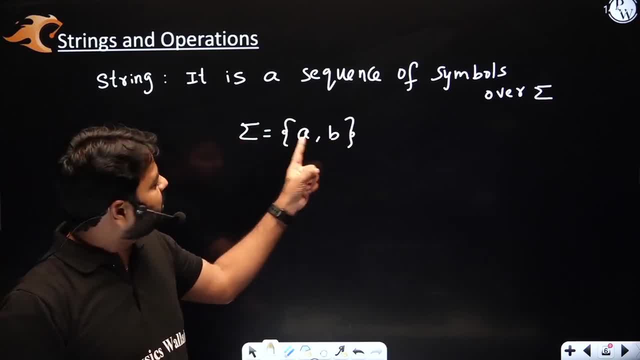 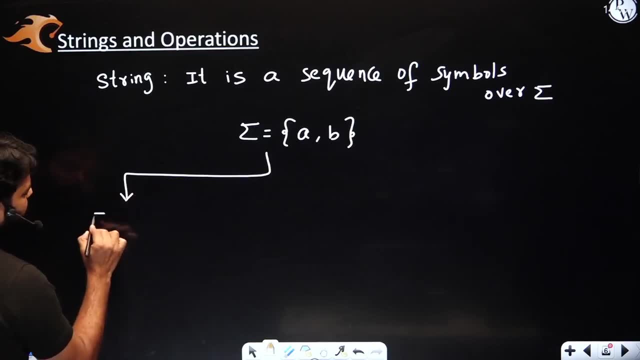 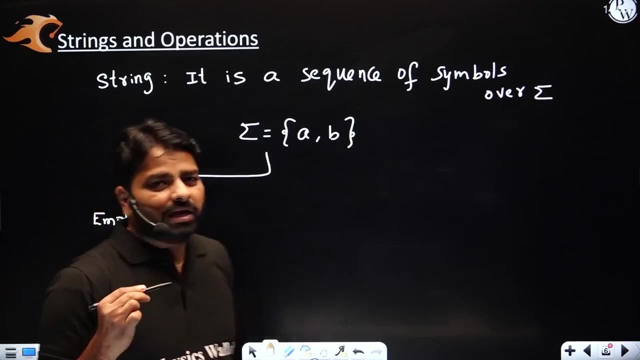 alphabet. what is it called as binary alphabet? because it has two symbols. let me take the very simple string which is called as empty string. oh, there is one word which required to understand empty, that is, empty string. empty word can be used in various places, but all the places it not be same like. empty set is. 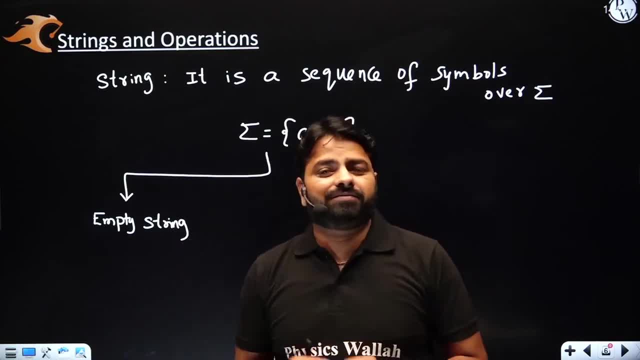 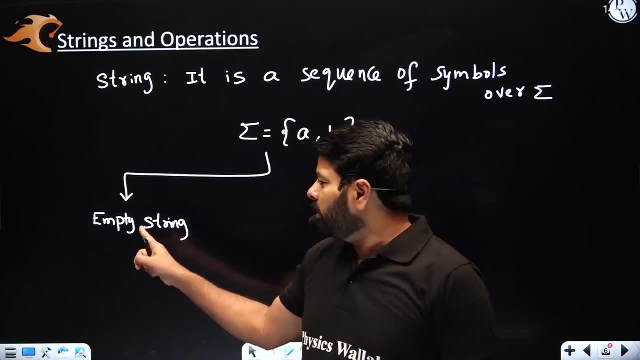 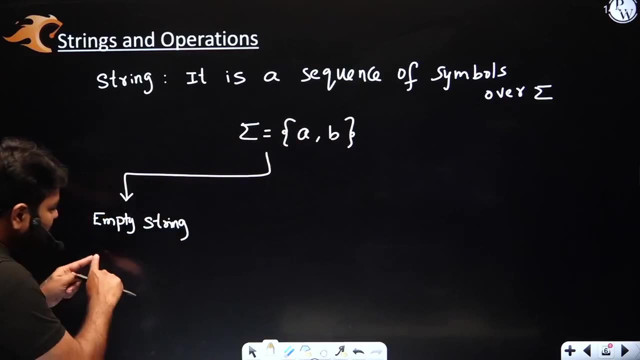 different. empty string is different, empty language is different. you must aware what are these different words we use along with the empty, so empty string- nothing. but it is a string which has zero sequence of symbols. so when i don't write any sequence here, that's called as empty string. to define it. i don't 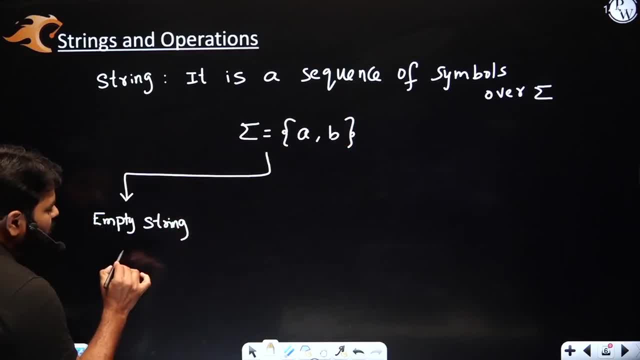 have a. i don't have a, b in this empty string, so we denote with epsilon. sometimes we represent with lambda, but remember epsilon lambda is a symbol from some other place, but here it is not a symbol. the symbol is a and b. remember, these are the only two things which are called as what. 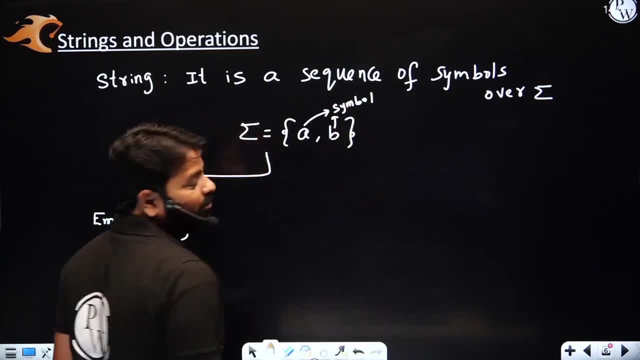 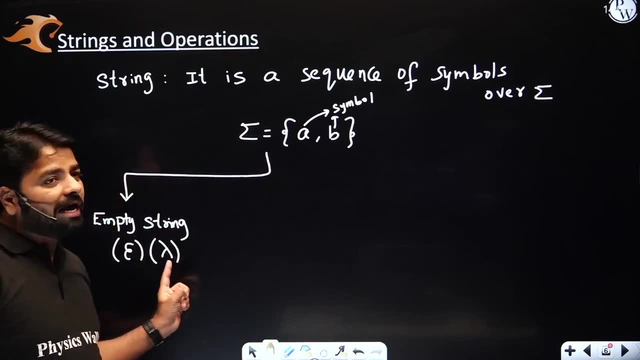 symbol. a is a symbol, b is a symbol, but this epsilon and or lambda denote empty string and never call this epsilon lambda is a symbol in alphabet, no, unless they mention it, but here the epsilon lambda is called as empty string. what is the meaning of empty string if i denote the string? 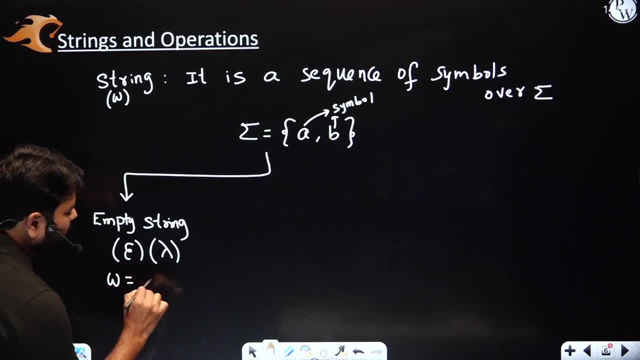 is with w and this w is epsilon length of w. if you try to find out it is 0, you should never say it is 1. remember this point. the length of the string is 0 because there are no symbols in the empty string. to denote there are no symbols, we have epsilon. so now onwards, whenever i take epsilon, 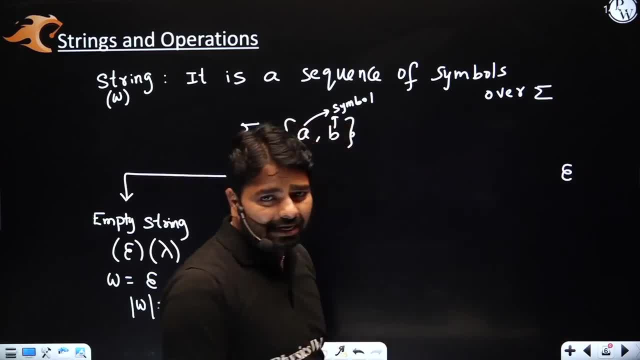 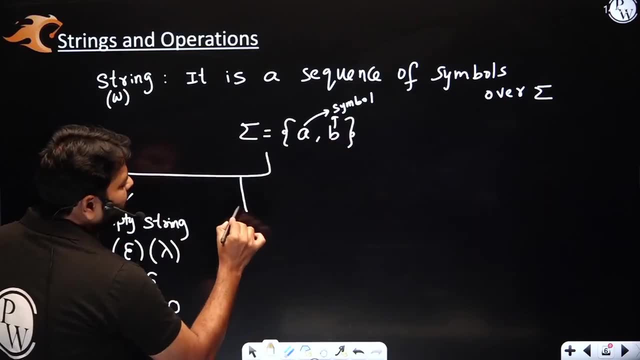 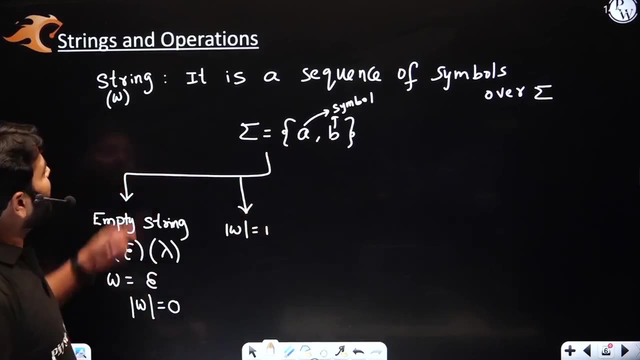 you must assume there is no symbol in that string. that is how you define epsilon. okay, next, what else? you have the strings over the a comma, b and if i take, length of the string is 1. if i have the string with one length, what are the strings you can form here? 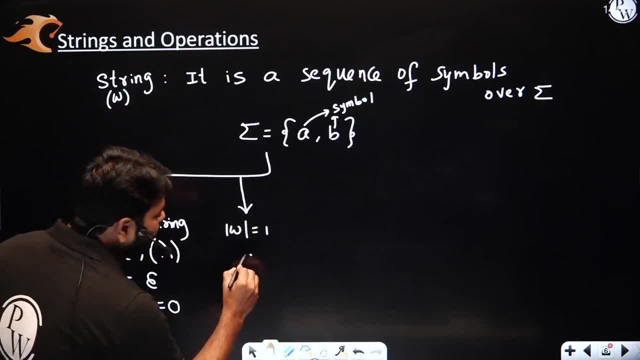 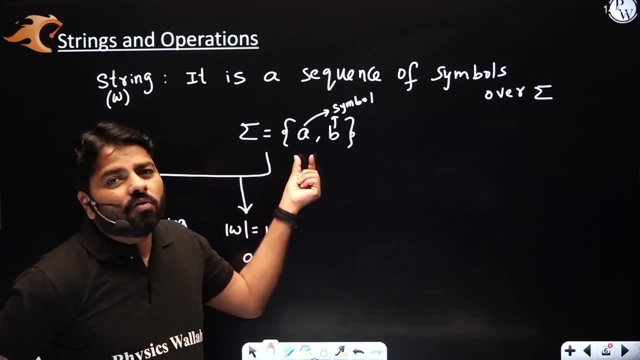 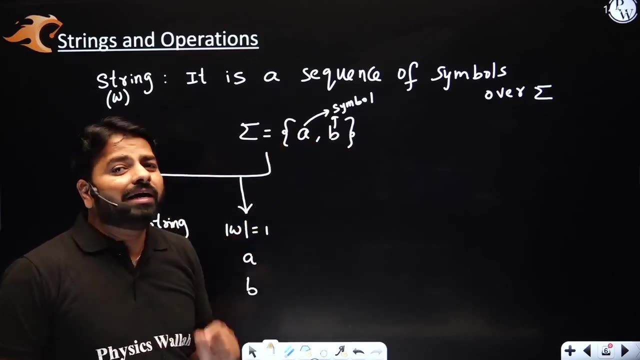 the a and b itself. they are one length. a and b, they are one length. and there is another definition of alphabet. alphabet is set of one length strings. i call it a set of symbols, right, but symbol is another definition. symbol has another definition. it is the one length string. anybody saying symbol, remember this point. symbol is. 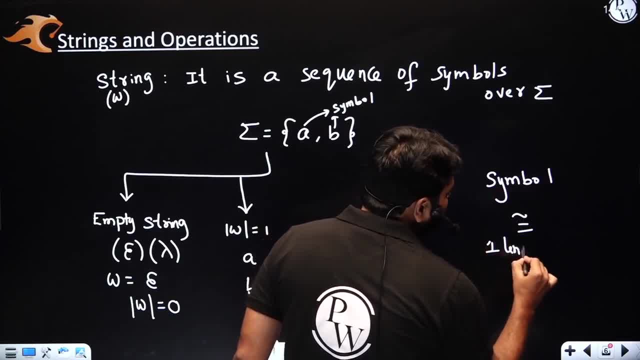 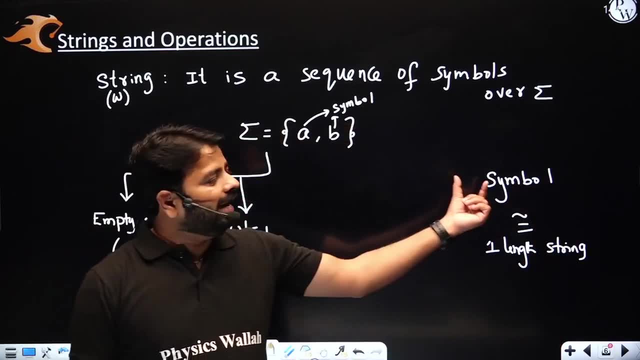 actually same as one length string. always. what are the symbol? you see, there has to be one length string, okay, so in the strings, whenever i write a symbol, that's called as one length string. fine, that's why i have written a and b. then i will move to. 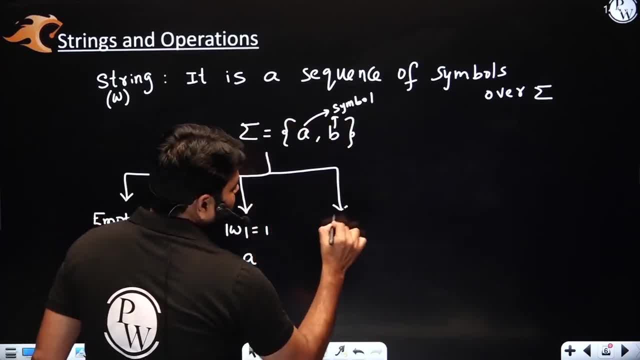 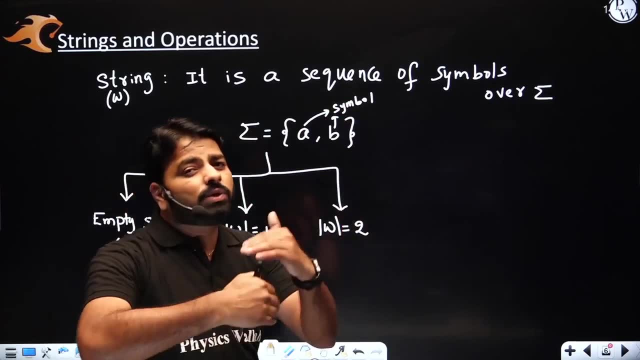 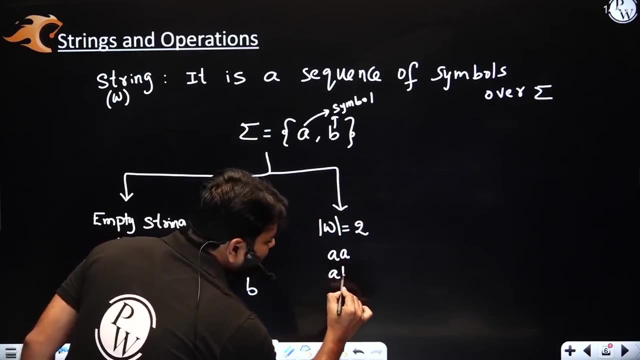 two length strings. tell me what are the two length strings? you know like what is the meaning of two length? it is a sequence of two symbols that means one after other. suppose a followed by a, it's a. two length, a followed by b. again two length, b followed by a, b followed by b. that's all you can. 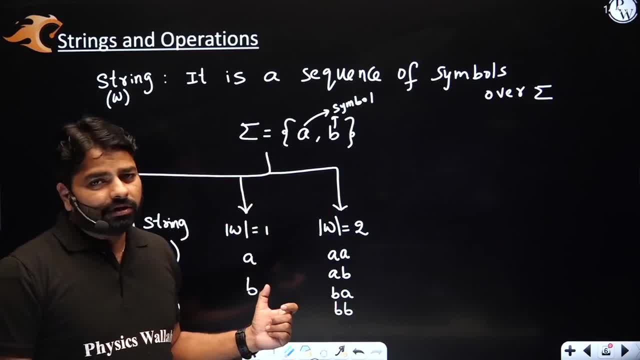 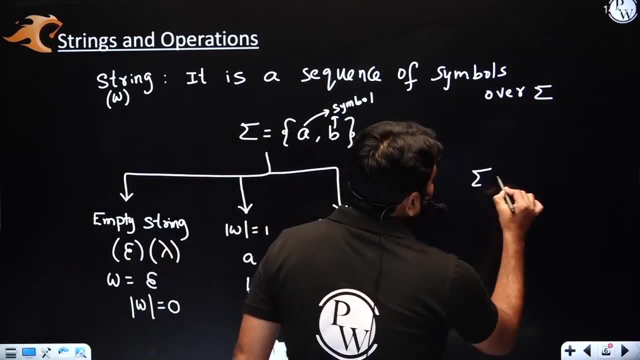 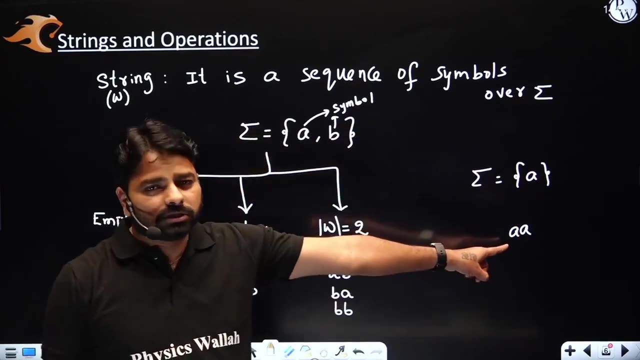 form using given sigma, sometimes more than these four strings possible. if the sigma has more symbols, right. if the sigma has only one symbol, let's say a, then how many two length strings you can form? only one, that is double a. there is no other two length possible here. if a, b, you can't write. 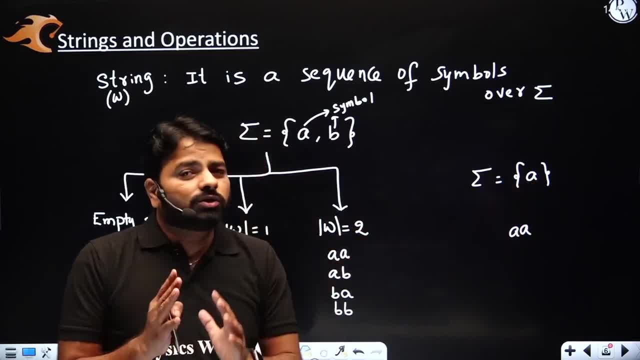 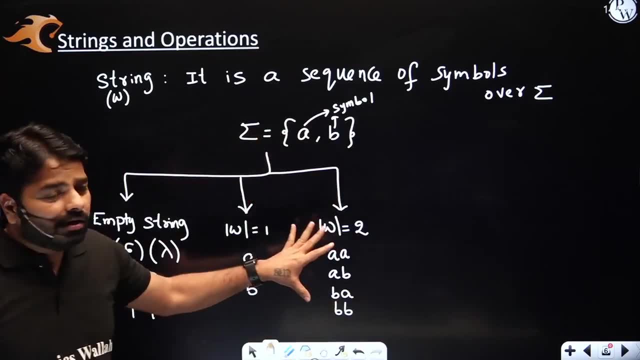 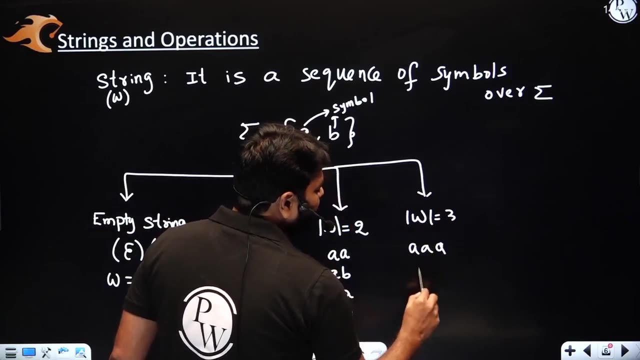 because sigma is not having a b. so this is all you require to learn: what is the sigma and how do you form the string from the given sigma. i hope you got a clarity with two length. similarly, you can form three length like a, a, a, a, a b, all possibilities, b, b, b. how many three? 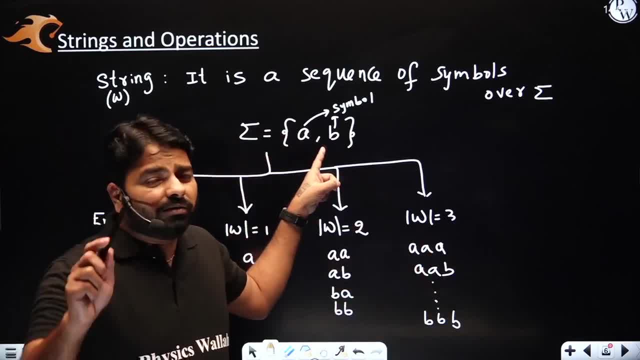 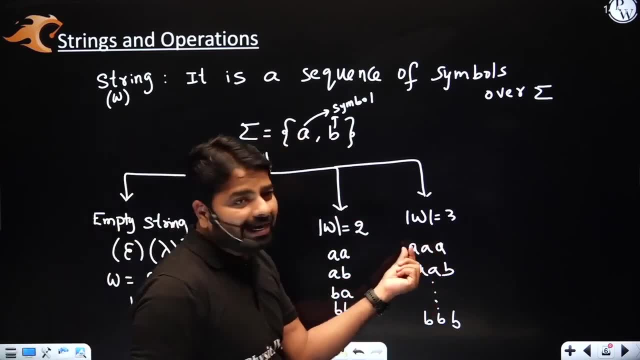 length strings are possible over the given sigma, which is having two symbols. remember what i am saying here. there are three positions you have to keep, and each position could be any symbol from the given sigma, like. if i want to find out how many strings here, then you should take like. 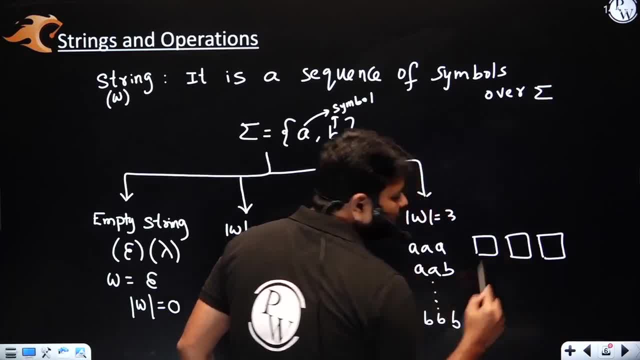 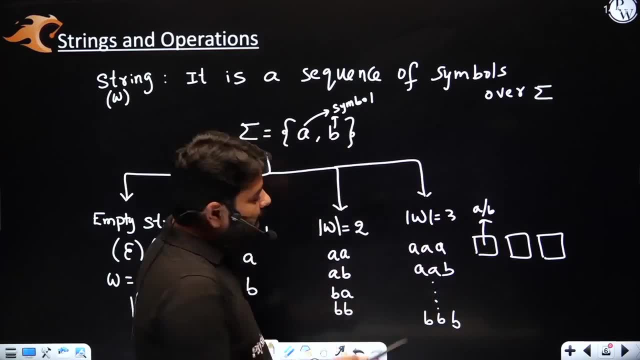 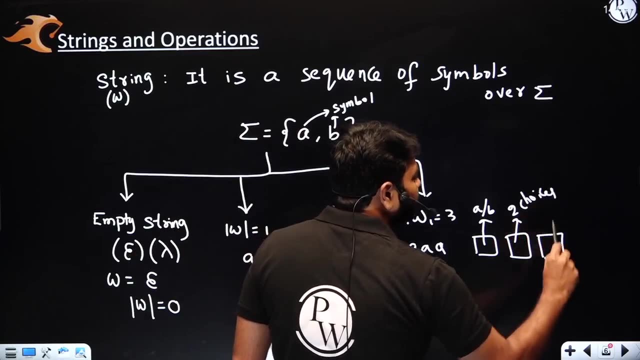 combinations. you have three positions and each position is having either a or b, but not both at a time. impossible, right? you can't keep both at a time either. you can keep a or b in the first position again. similarly, you have two choices: a or b. here also you have two choices if you try to form the number of three length strings. 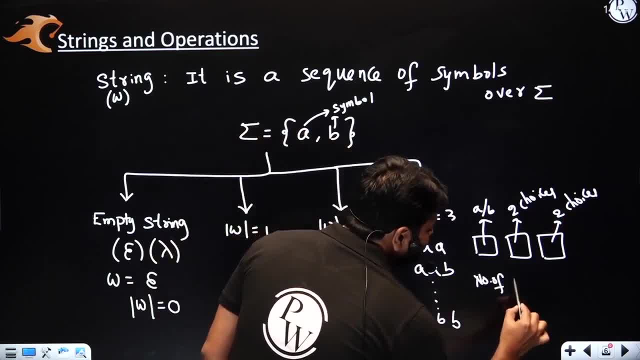 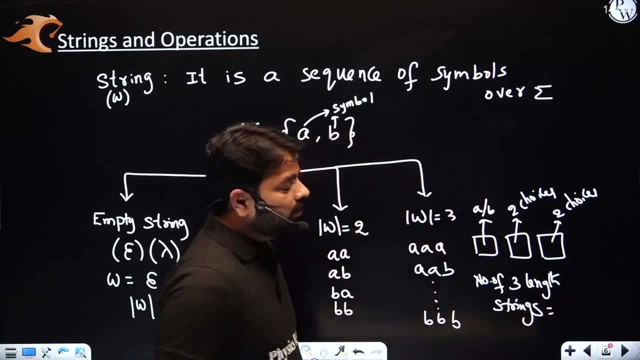 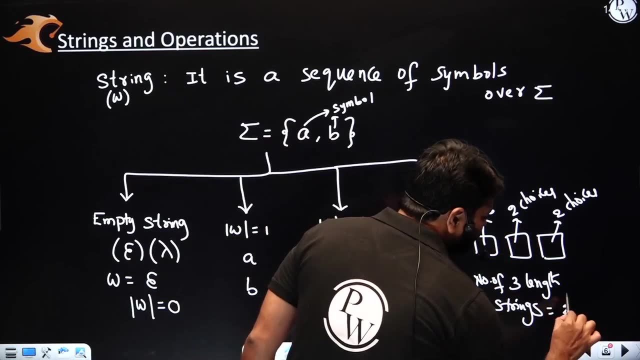 how many number of three length strings here possible number of three length strings, which is equal to two possibilities and multiply with two and two, you will get two power three, which is equal to eight. you got eight right in general. how do you form? anyhow, we will solve again in the questions. 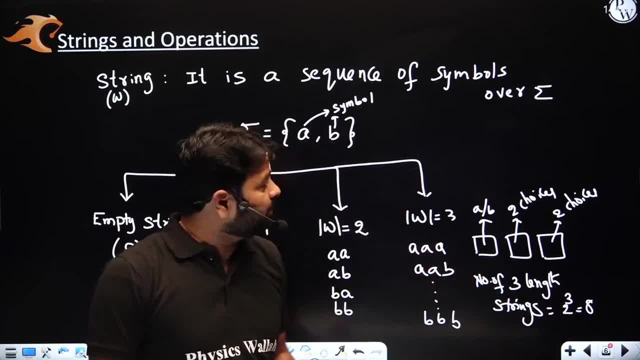 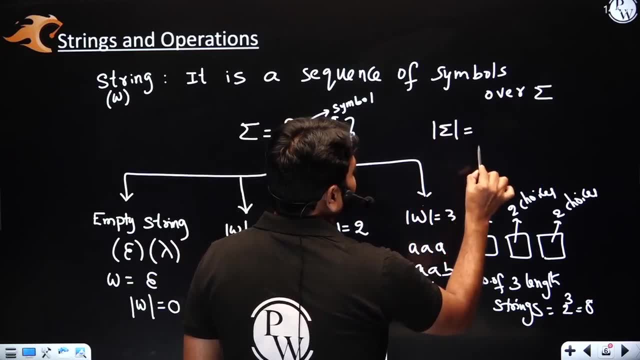 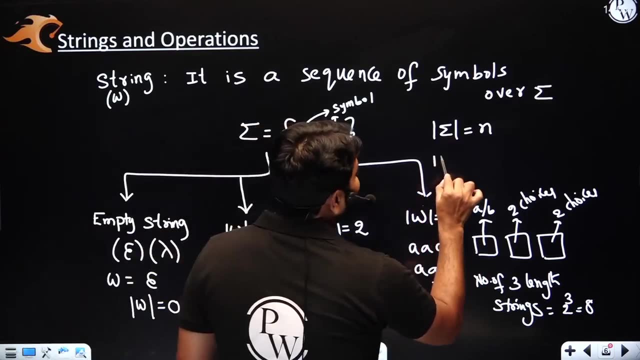 but i want to give you what kind of questions we can expect in the exam. so they will give you in general. i'm just forming it. length of sigma is equal, let's say n. so i have n symbols in the sigma. now i want to form length strings. how many k length strings are possible? i want to form k length strings. 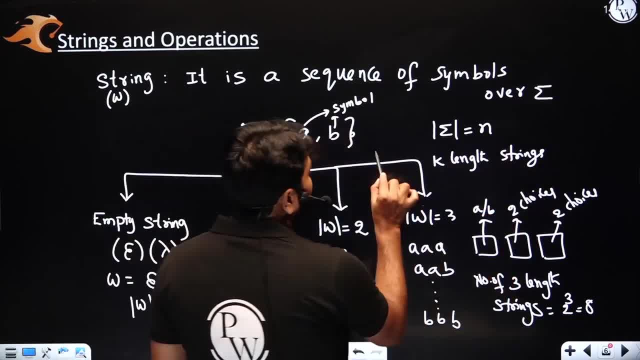 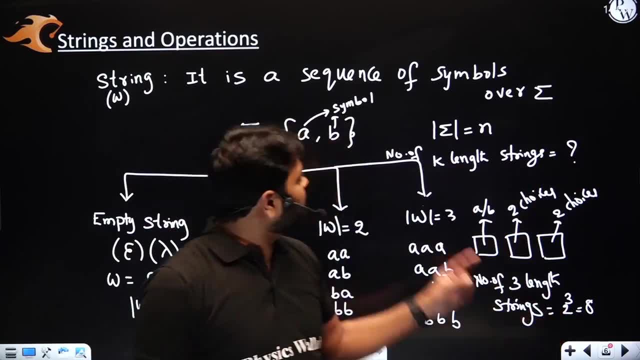 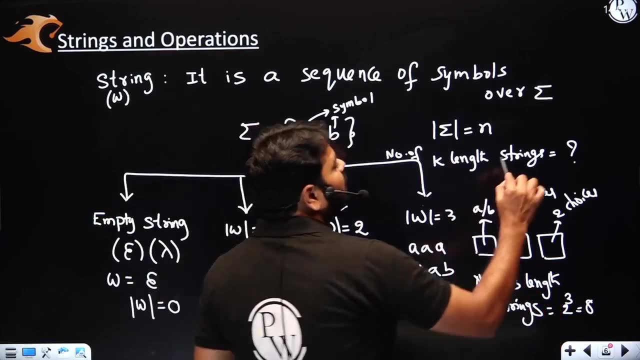 how many k length strings are possible. can you find out the number of k length strings? can use this formula here. what do you mean by two? two means two symbols in place of two. what you get, n and in place of three, you will get number of k length strings right. so it's equal to. 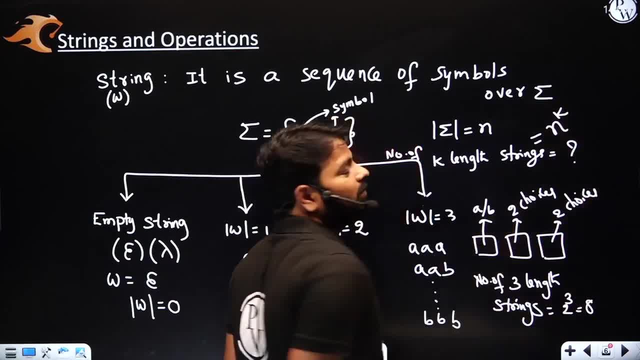 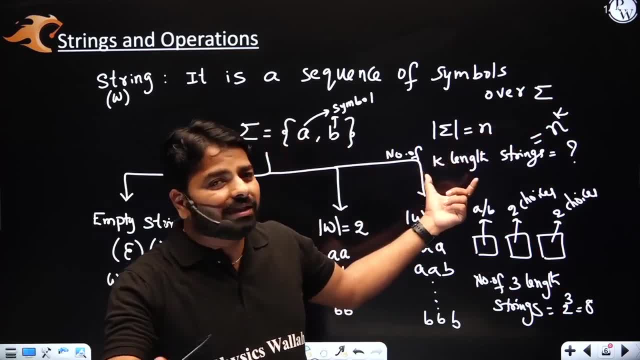 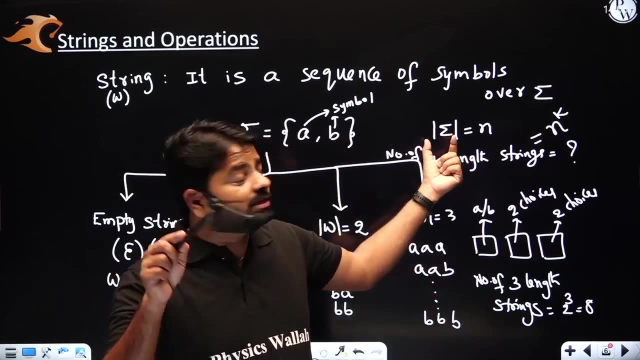 n power k. n power k. is that clear? n is the number of symbols in the sigma, k is the. what is the string length that you want to form and total number of k length strings possible over n length alphabet over n size, n, or you can say, or n number of symbols in the alphabet. 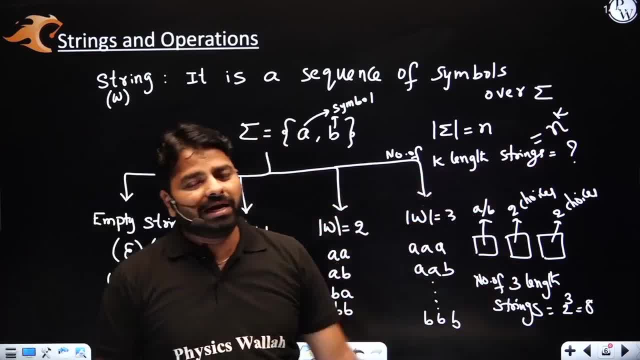 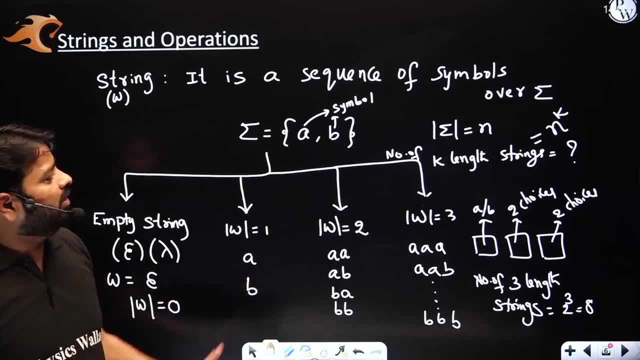 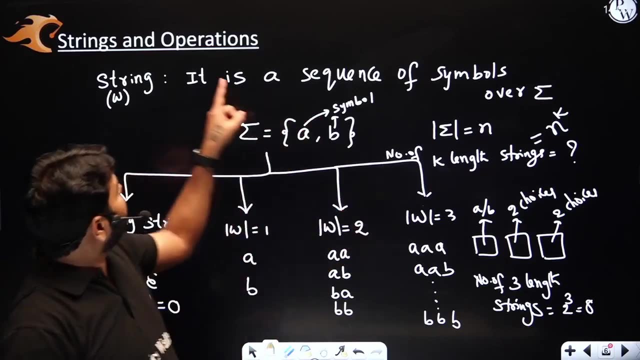 so there is n power k. so you may note down that how many k length strings possible over n symbols, which is equal to n power k. fine, so this is how you can find out the strings over the given sigma. now let's move to some of the questions which you require here. the questions are possible like operations you. 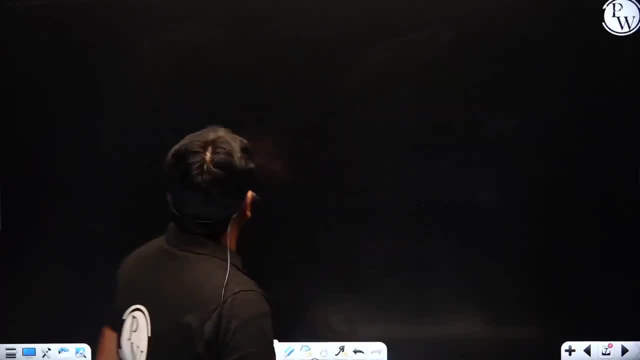 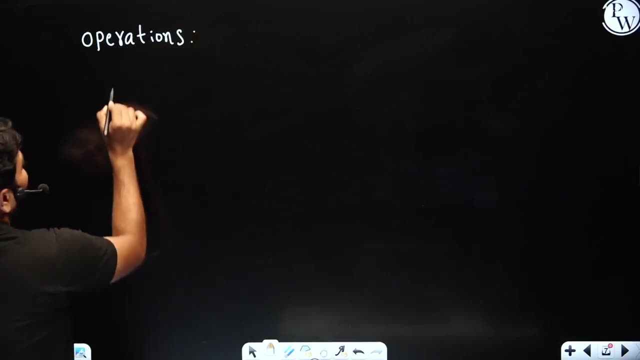 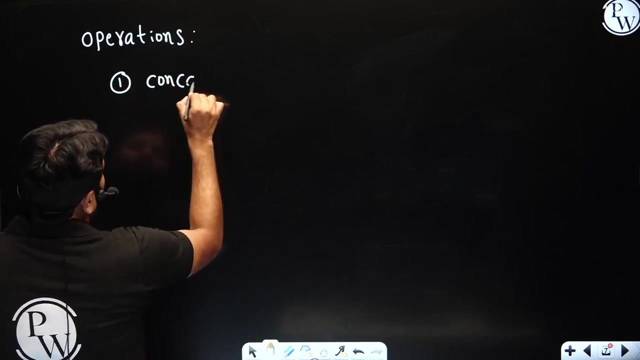 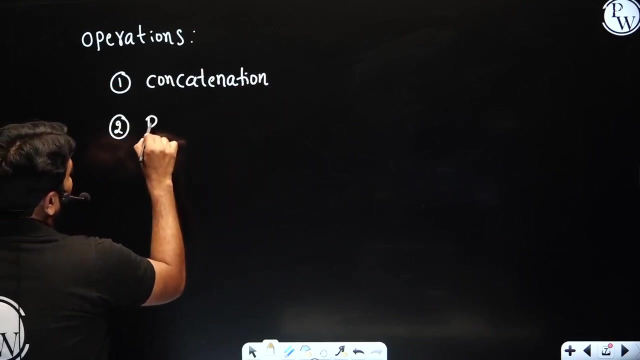 want to know some of the operations. let me write some of the operations over the strings. what kind of operations you may try, like the first one which is maybe important, that is, concatenation. second, sometimes you may come across a reversal of a string. of course, already i tried the length of the string. 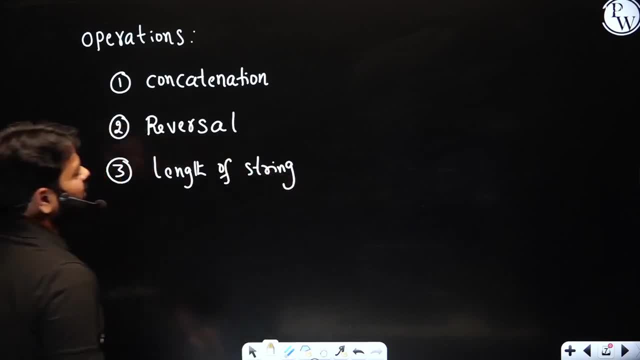 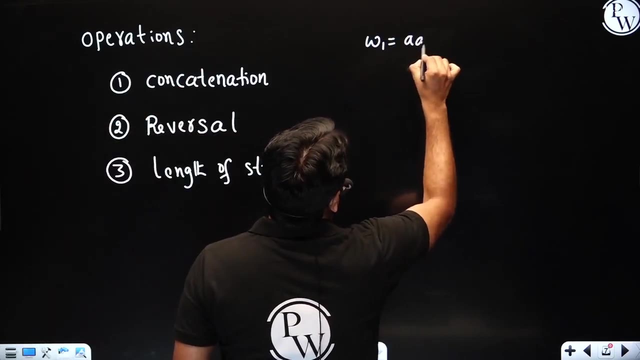 the number of symbols in the sequence. likewise, you may apply lot of different operations over the strings, but i have just taken the few operations. what is the concatenation? let me try. no, let me do a scale. no, let me do a scale. Suppose I have: w1 is a, a, b and w2 is, let's say, b, a. 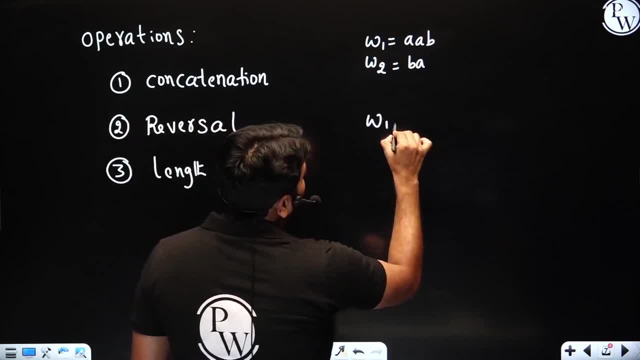 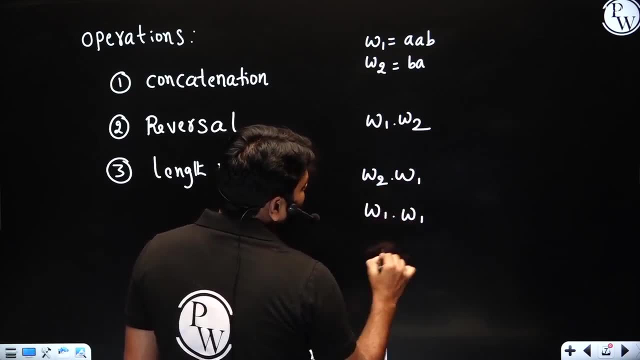 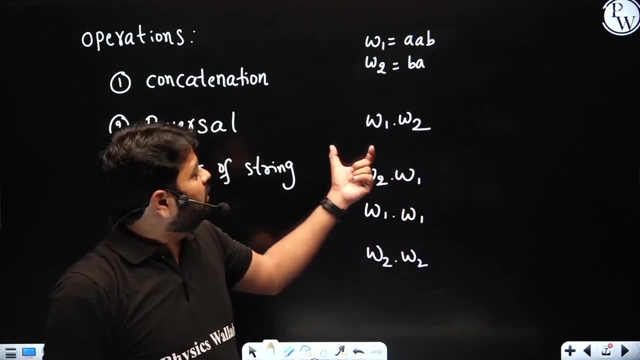 Then I may form the w1 followed by w2, or I may form w2 followed by w1, or I may form w1 followed by w1, or I may form w2 followed by w2.. There are various ways to perform the concatenation over the given two strings. 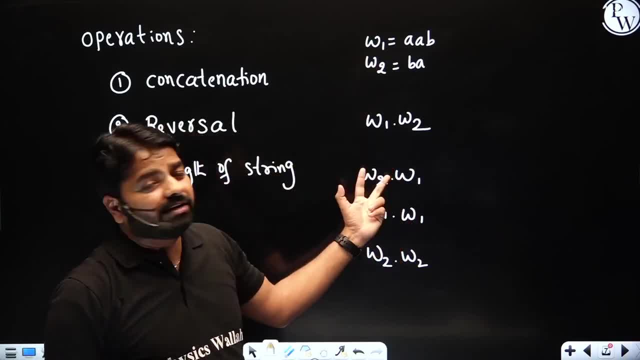 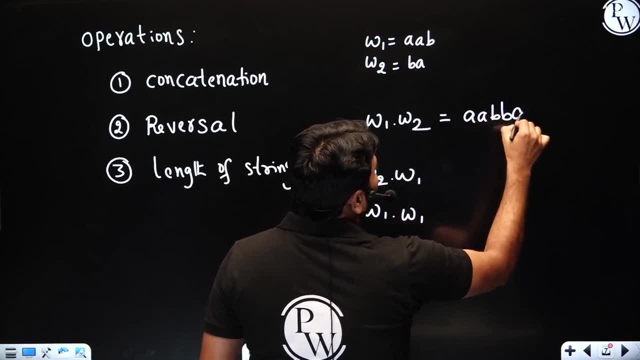 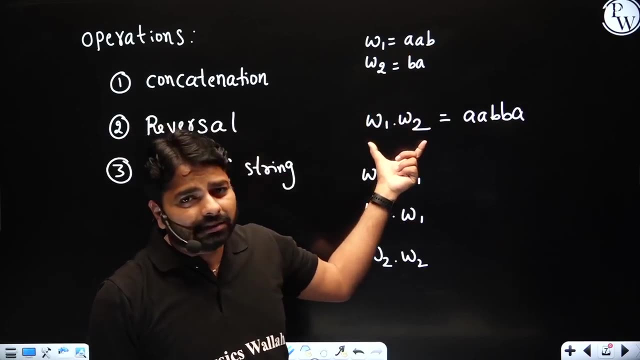 Like I may take the same string twice or different strings in different order. So if you say w1 followed by w2, it's just a sequence. First you take a w1 followed by w2 and you may wonder. so if the length of the w1 is 3, length of w2 is 2, then what is the total length, which has to be 5?? 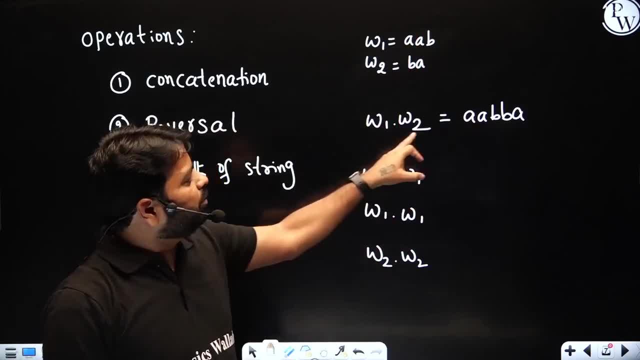 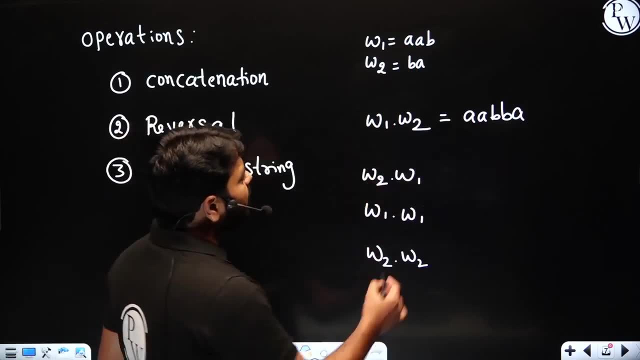 That means 3 plus 2, which is 5.. So this is a very important factor: length of w1 plus length of w2, which will be length of w1, w2.. And similarly, Length will be same: 2 length first, b, a and then followed by 3 length. 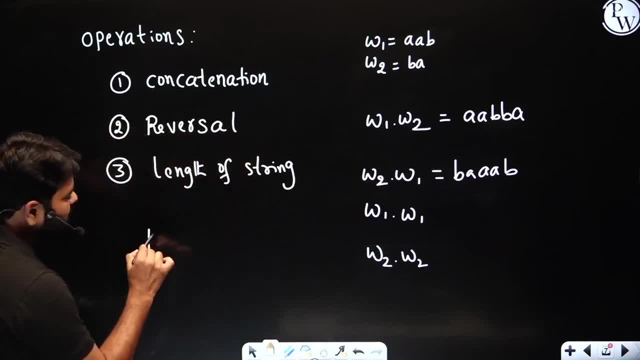 So again, you will get 5 length Here. you are going to ask: is it always length of w1, w2 equal to length of w2, w1?? Always, But w1, w2 need not be same as w2, w1.. 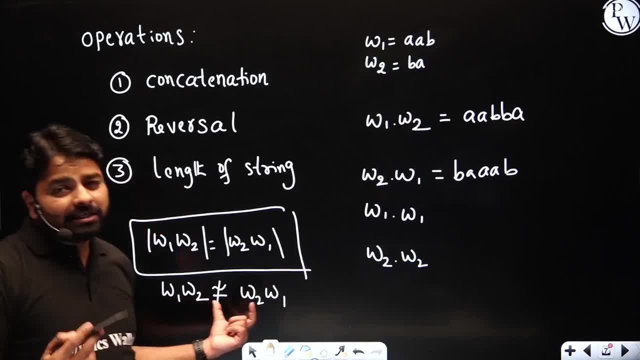 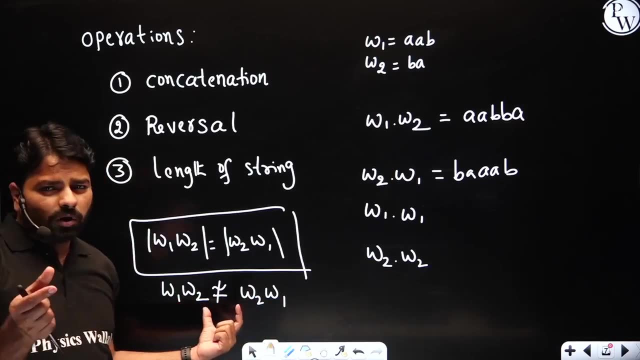 The strings need not be same. Remember that. Maybe same in some situations, but In general the w1, w2 need not be same as w2, w1.. This is called as commutative property over the concatenation. We will also discuss this point. 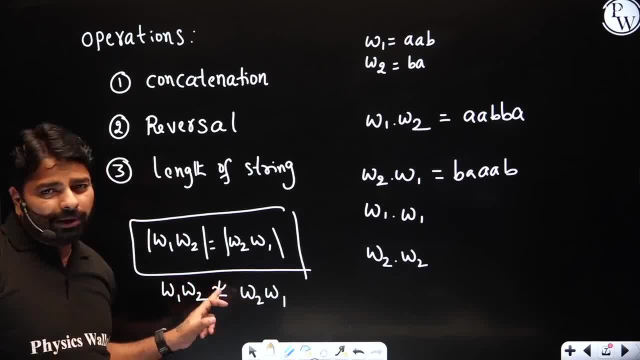 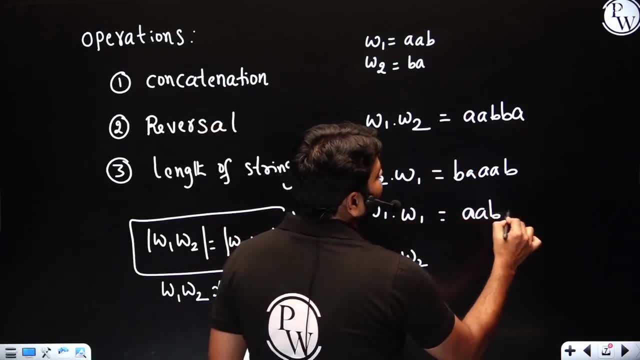 But remember this symbol is need not be equal, So remember this point too. w1, w1, which is 3 length, right 3 length, followed by 3 length, which will be 6 lengths. Some people may write this as: 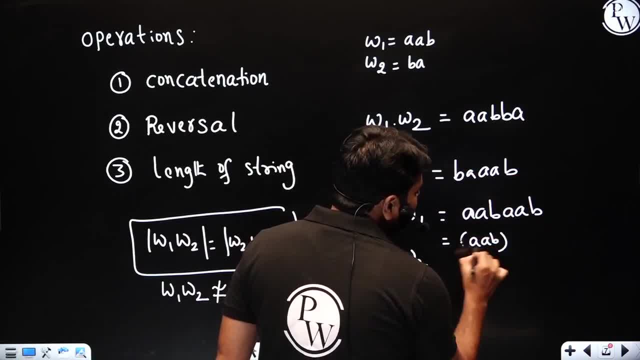 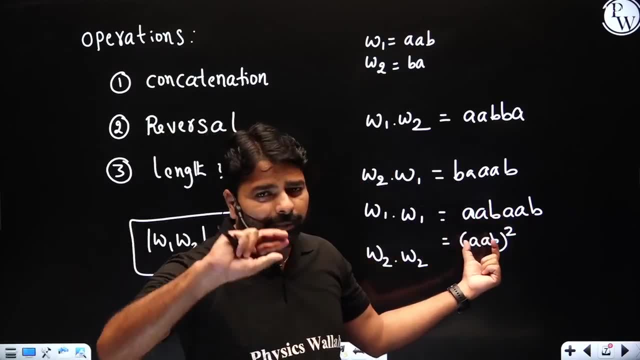 If you want to represent some other way, a, a, b square. So this square is not mathematical square. This square is over the strings, So it's a repetitive. So a, a, b, when you repeat twice, you can also write in the form of a, a, b, power 2.. 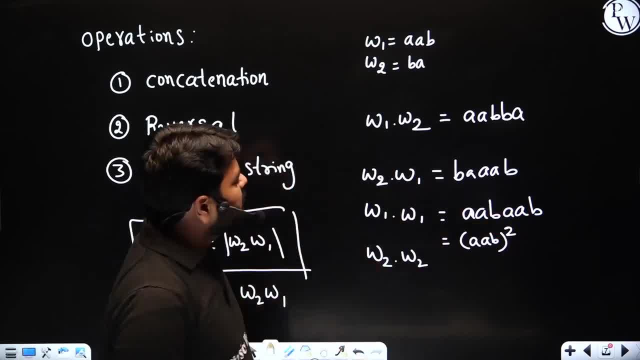 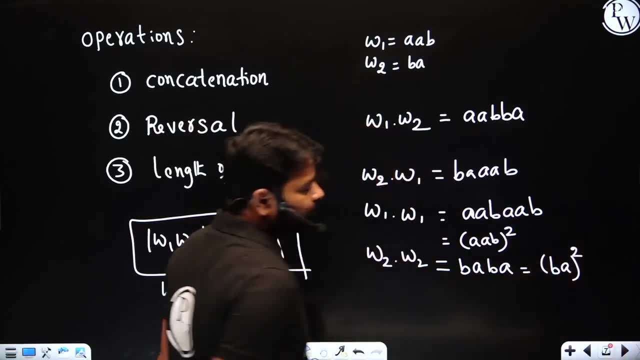 Which represents same as a a b followed by a a b, Now w2, w2, right, b a followed by b a. You can also represent as b a over 2.. So this is how you can do the concatenation over the strings. 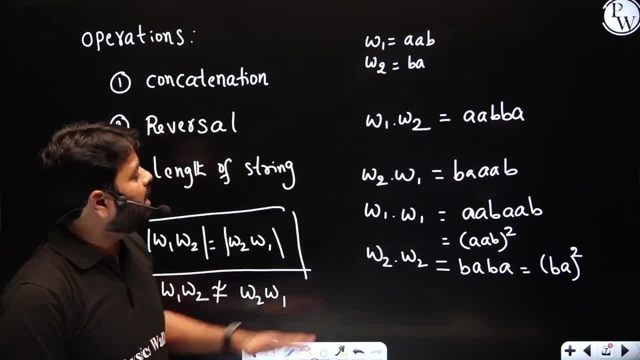 Similarly, let's talk about the reversal of a string. Here I am always taking- remember the sigma is a, b. When I change, I will definitely mention in the slide itself. Now let's come to the reversal. Reversal of a string. 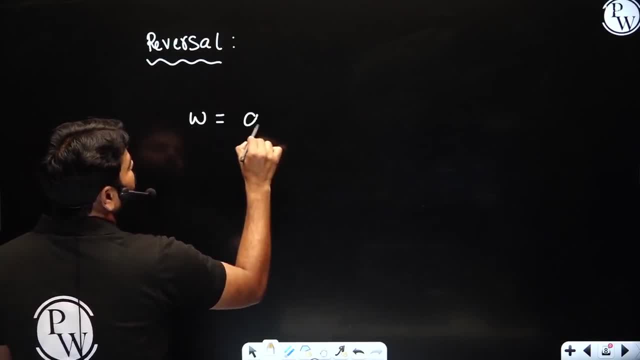 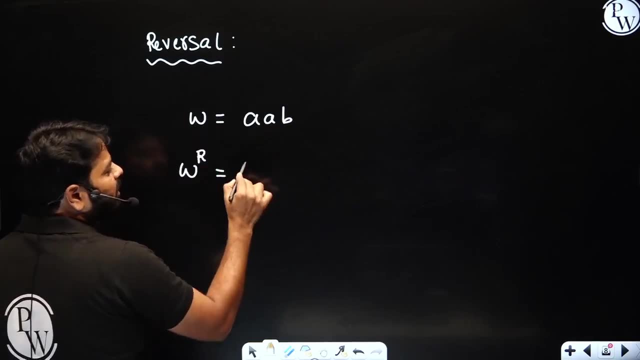 How do you perform the reversal of a string Which is straightforward? Suppose I have a, a, b, What should be the reversal? Reversal? you may write as w, power r, Which is same as reverse of w, which is b, a a. 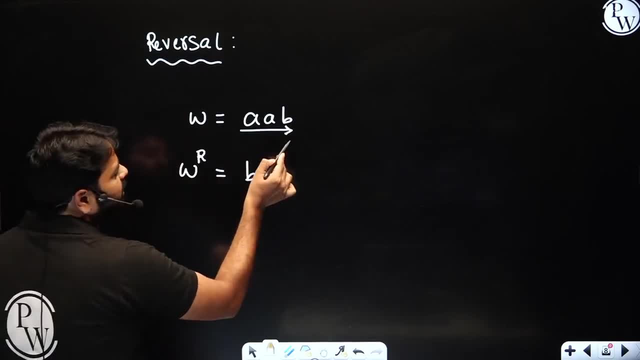 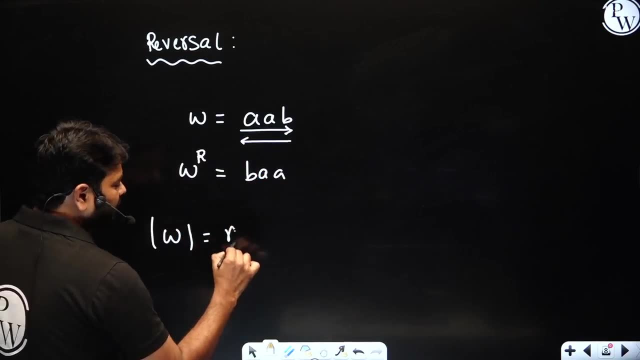 Instead of writing in this left right now, you will change the direction right left, So you will get b, a, a. In case. if w has length, let's say n or k, anything, Then what is the reversal of a, w? 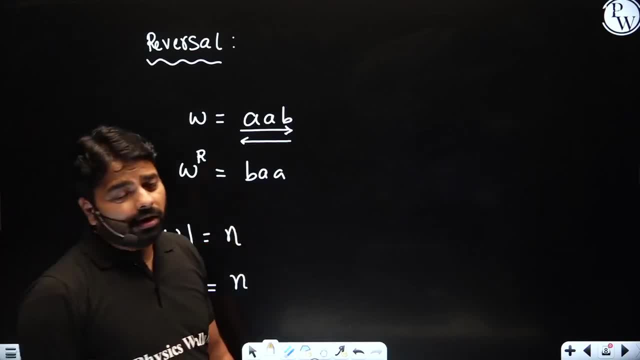 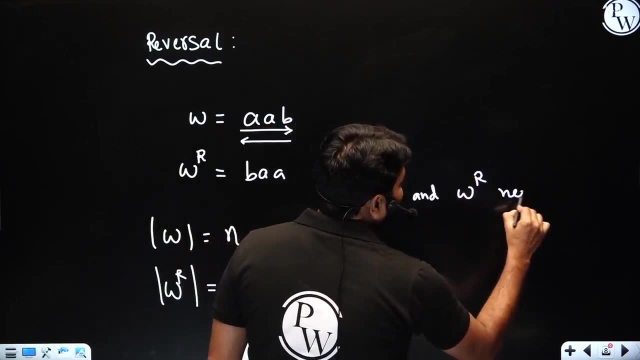 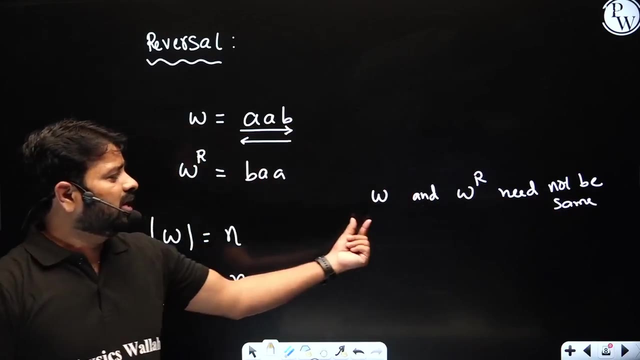 It is always: n. w and w power r need not be same. Remember that w and w power r may or may not be same. It depends on the sigma and it depends on the string. Now you may ask that in what situations these two are same. 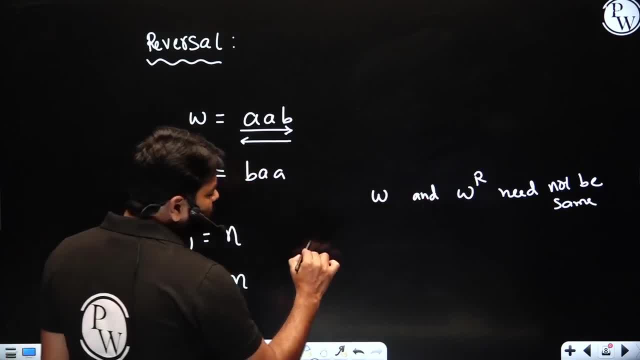 Yes, when I take a palindrome like w is a, b, a. Now do the reverse. you will get the same. When you write in the reverse order, you will have the same. When you have the concept of palindrome, w and w, power r will be same. 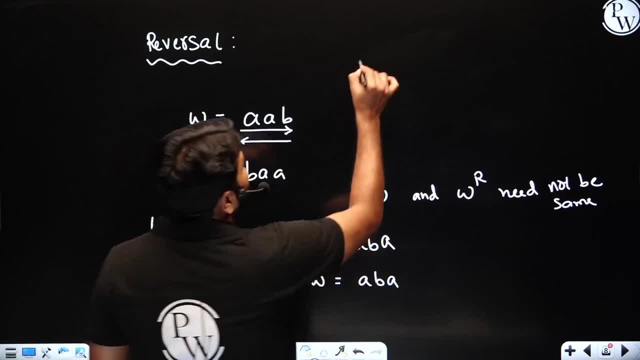 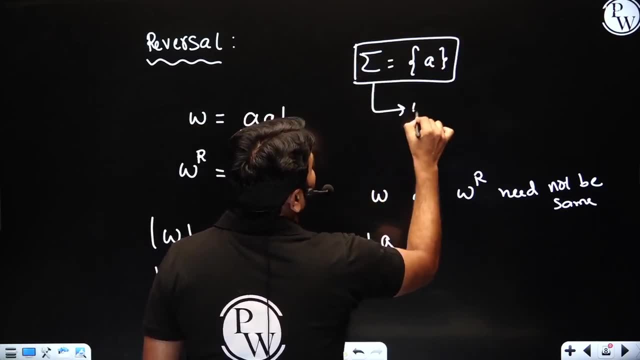 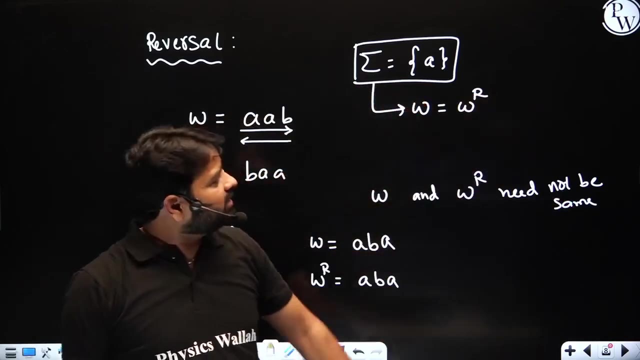 What are other situations you may face? it When the sigma is having only one symbol, let's say a. In this case write whatever the w is always same as reverse of the w. This is the one more important point: that w and w power r is always same when the sigma has only one symbol. 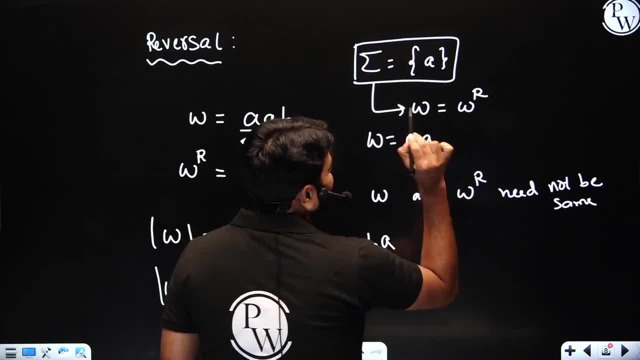 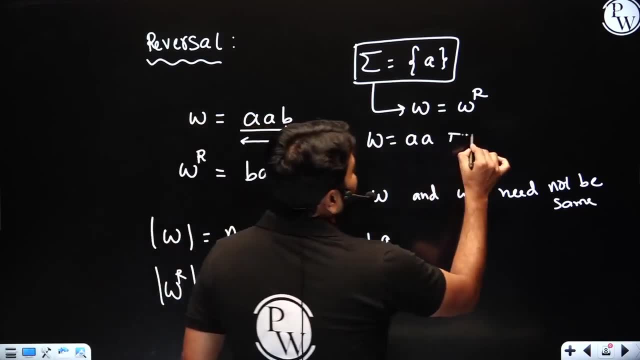 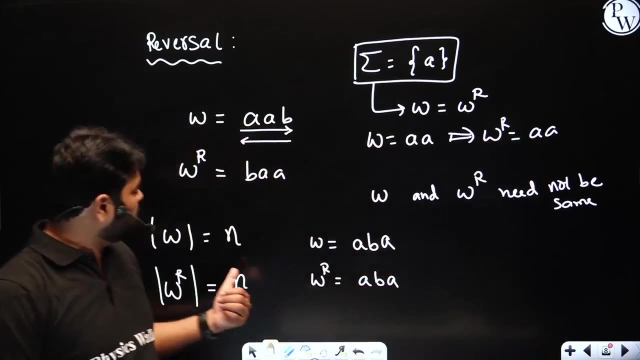 You may check. w is equal to, let's say, w. Now write in reverse order, because all the symbols are same. You write in any direction, you will have the same right, which is w, power, r, w. Here, when you have more than one symbol, there is a chance to have a different signal. 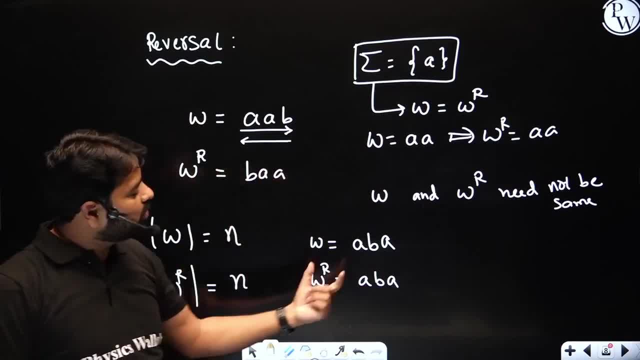 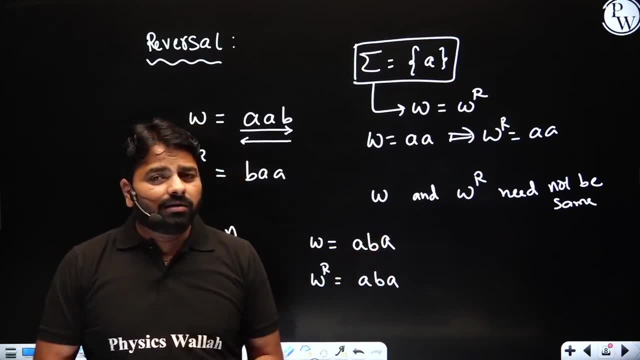 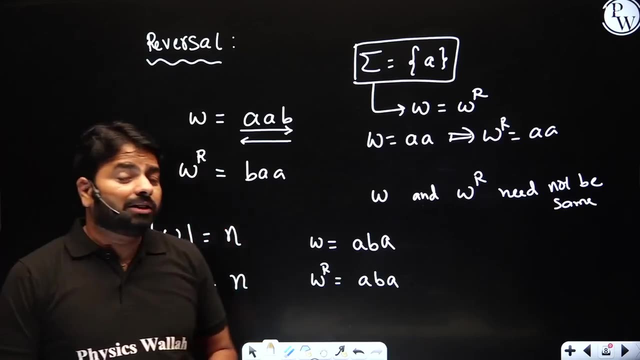 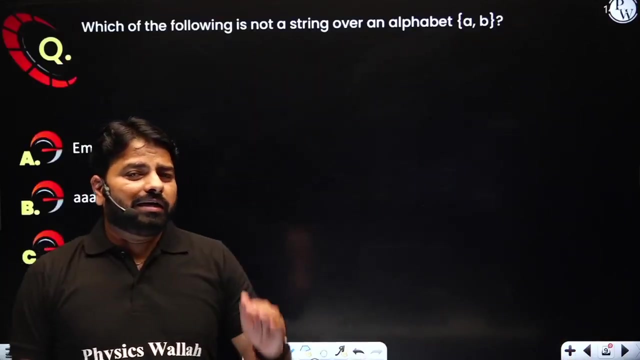 You will have a chance. but sometimes you may have the same sequence. if the string is a palindrome, Fine. so this is what: the reversal of a string, The length of the string is always same as length of the reversal of it. Now we have seen the concatenation and reversal. 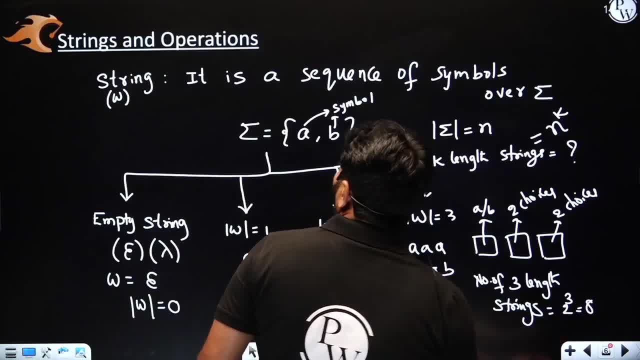 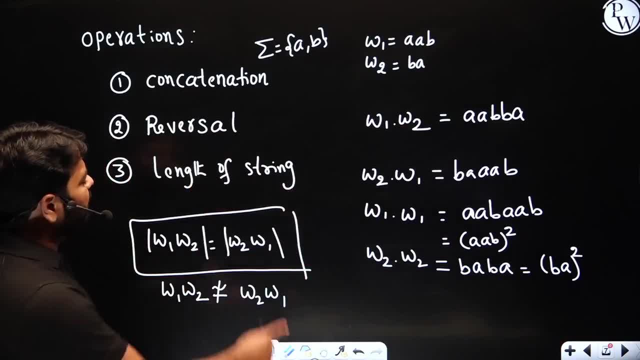 So what is the next one? we have to see The length of the string. I hope you don't need a special slide for that Length of the string. we have already seen. we were talking about it. The length of the string is nothing but the number of symbols in a sequence. 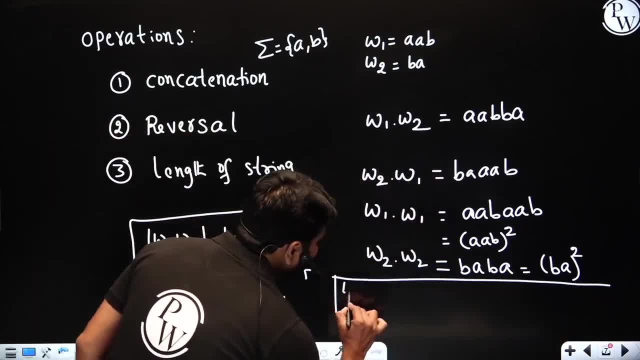 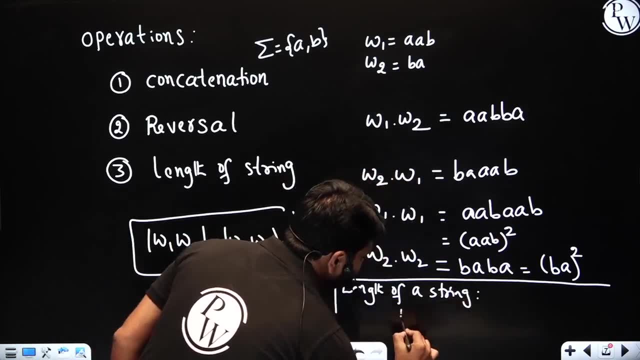 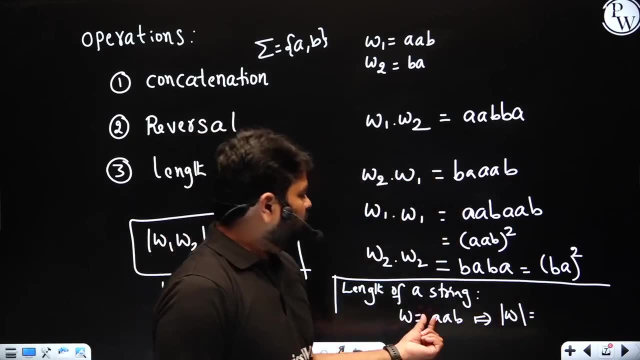 Let me take an example here. What is the length of a string? Suppose w is equal to a, a, b. What do you mean by length? Length is just Three symbols. in a sequence we will write just three. Length of the string is a, three. 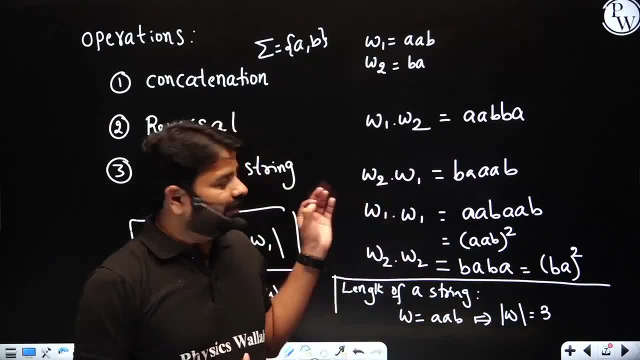 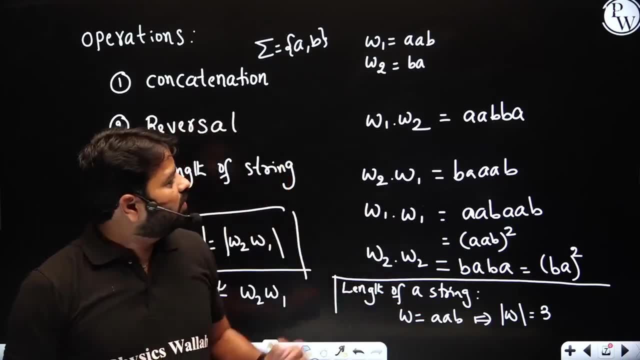 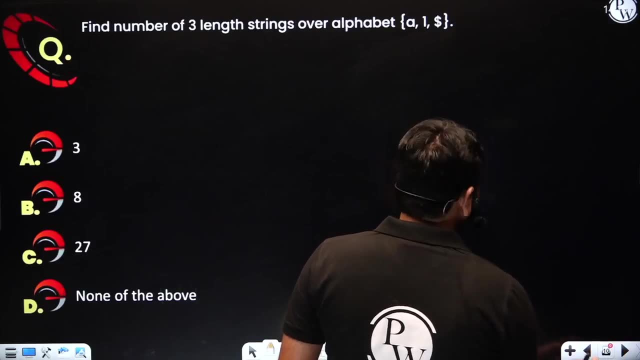 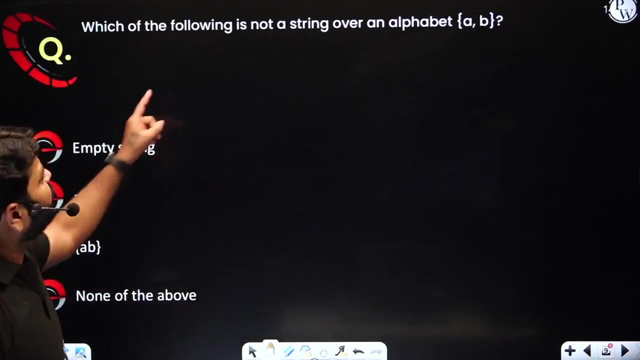 Fine, We have come across the definition of a string and a few operations over the string. Now it's time to learn some of the questions over the string. There are various operations that I will discuss through the questions. Okay, The first question is: which of the following is not a string over the alphabet a, b? 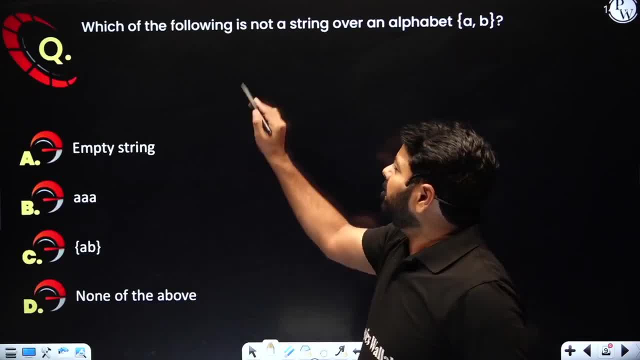 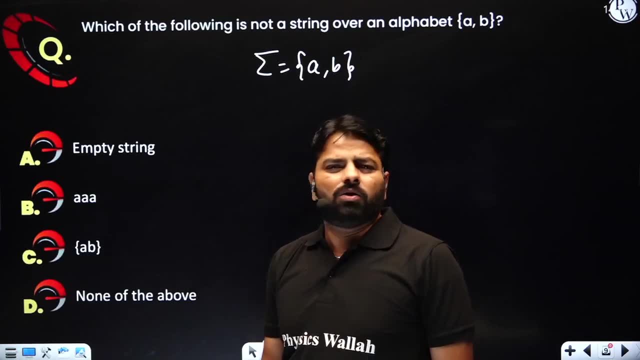 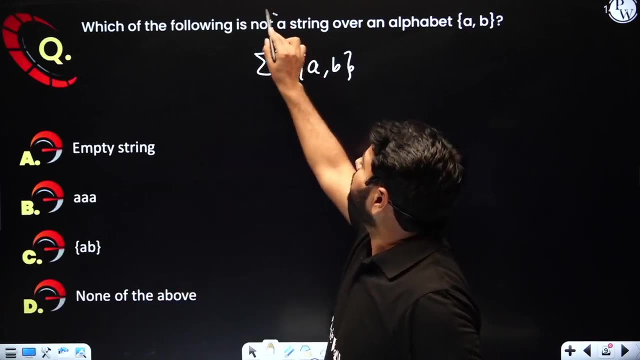 So we have two symbols in the alphabet, That is, sigma a, b- Empty string. Is it a string? Always, Over any sigma in the world, the empty string is always a string. Fine, Now the question is, which is not a string? but this is the string. 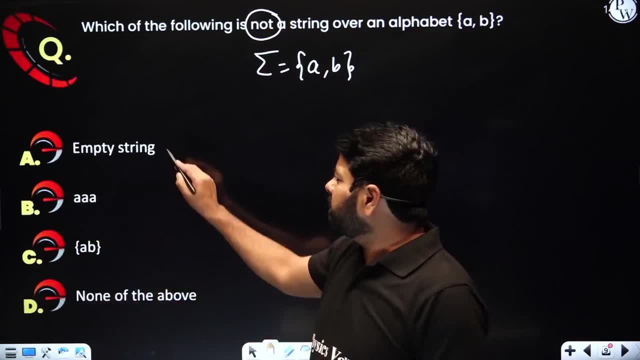 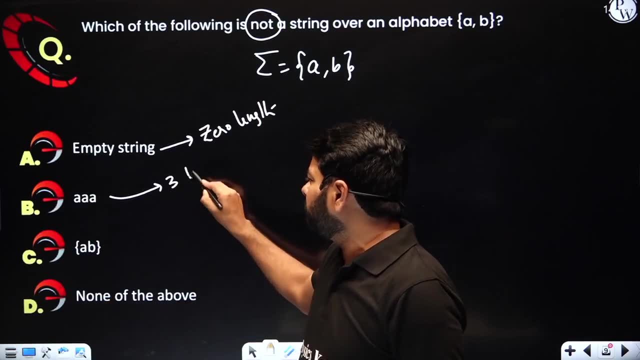 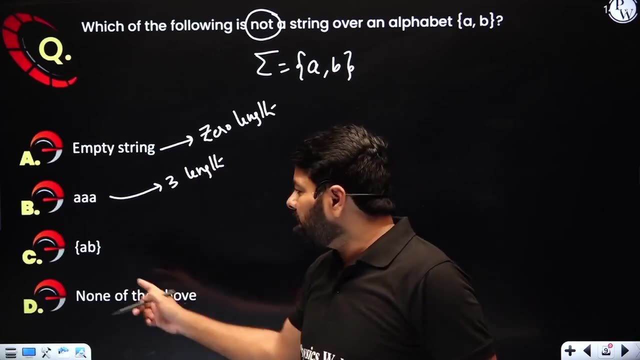 And a, a, a. Yes, it is a three Length string, right, This is a zero-length string. Fine, This is a three-length string which has a meaning, But this a, b in the square brackets, in the curly brackets, sorry. 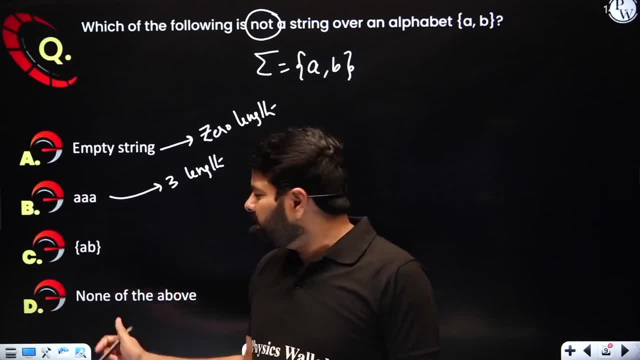 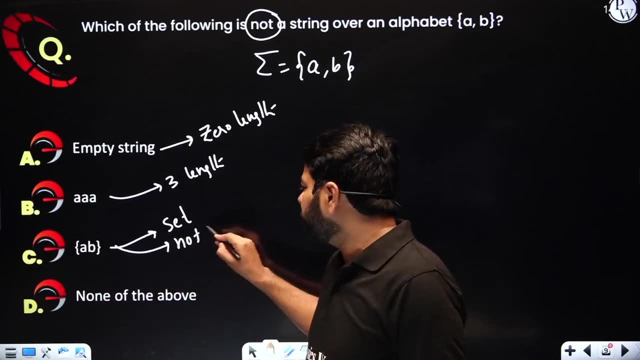 In the curly brackets or any brackets we mentioned here. that's not a string, right? It is a set here. This one is called as what It is: a set, not a string Set. It is not a string. How do you know it is not a string? 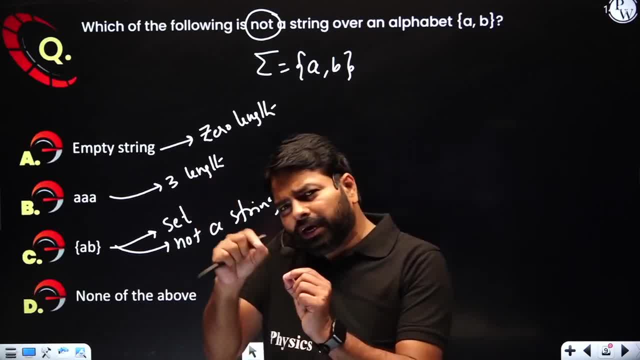 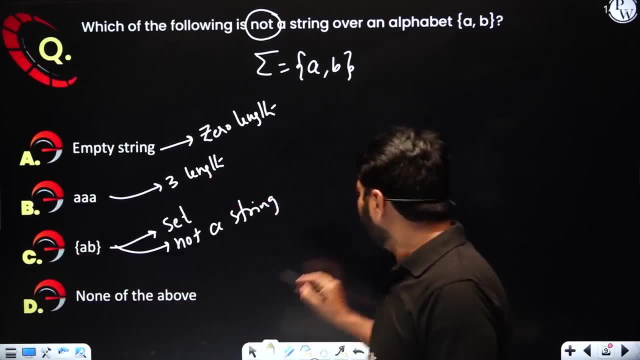 Because Because the a and b are only symbols. Anything you write in a sequence, it has to be a or b. This curly bracket should not come in a sequence. right, You can write a, b. This is a string, But this is not a string. 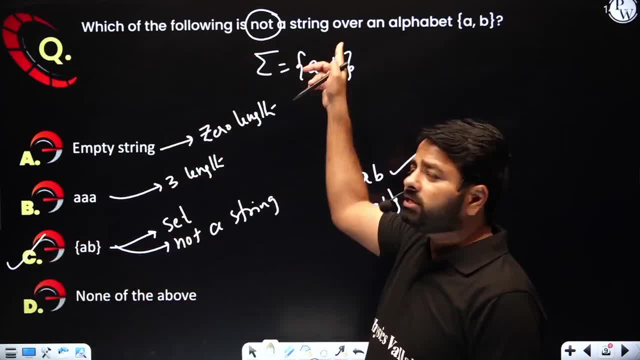 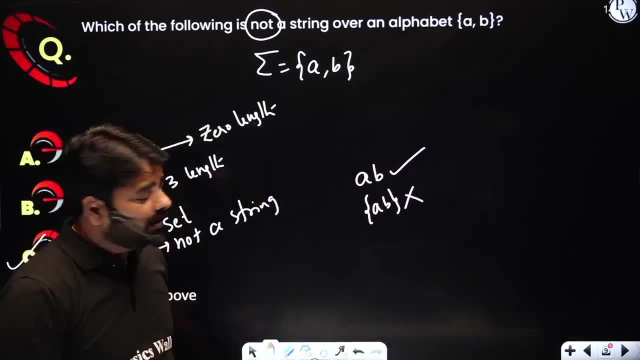 Okay, So this point we want to choose, not a string. So this is definitely not a string. Okay, You may ask. so what are the situations you may face? Not a string, Clear, Clear. So when you write a string, you always remember. 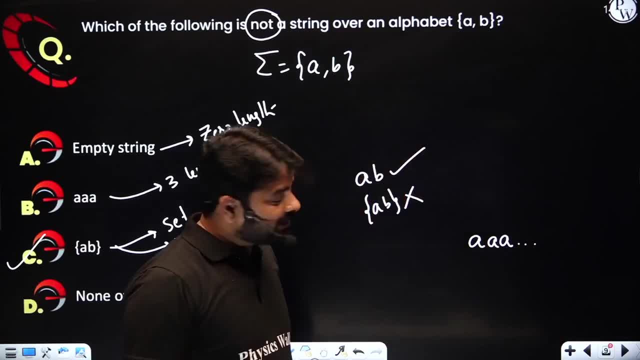 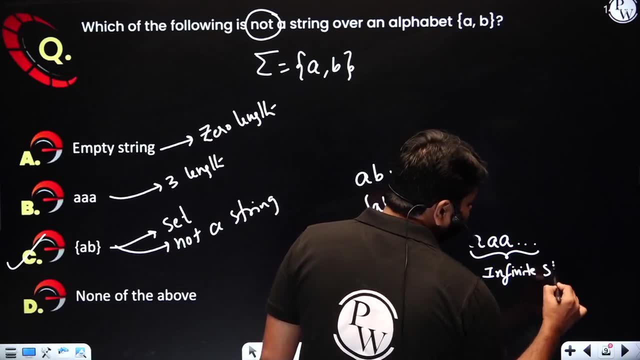 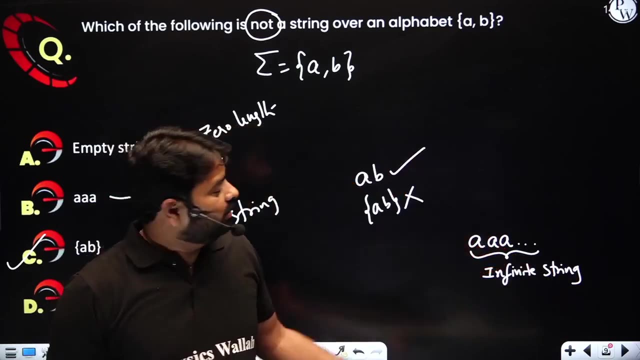 You can't keep something like this Infinite string- Especially, this should not come into the part, as a string is always a finite By definition- In. theoretically this is a string, infinite string- But you should never write in the computation, So this should not be considered as the computational string. 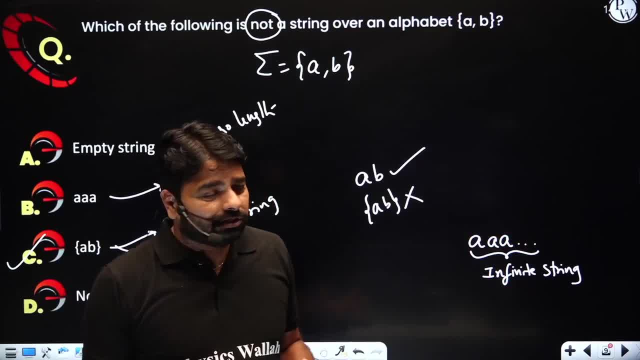 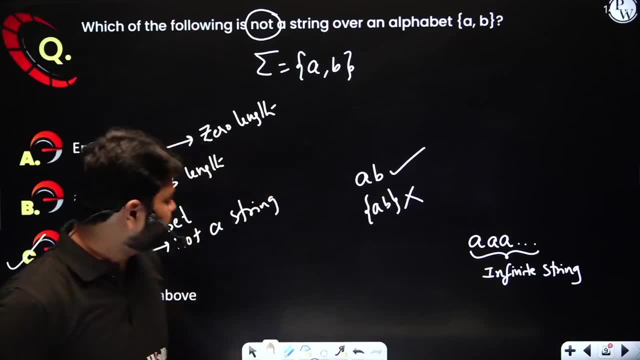 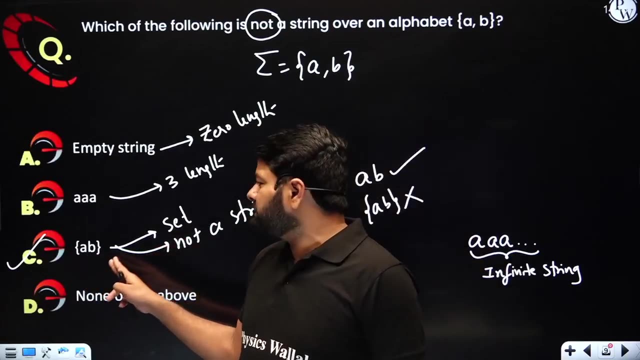 So this is very special. We don't write in any language. What we write, we'll see in the language definition How to form the string in the language. So we got the answer. that is, the c is not a string. it is actually a set which has a string. 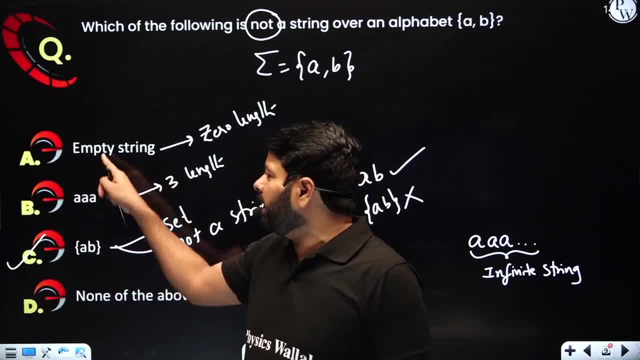 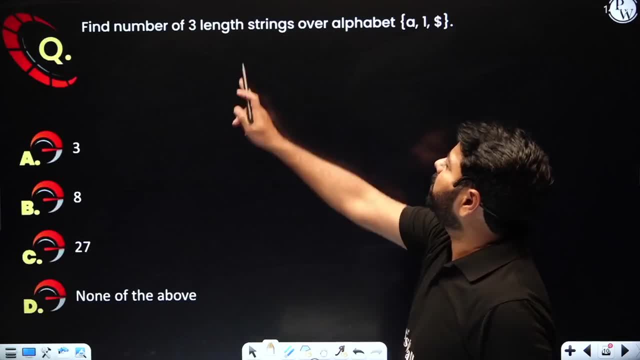 How do you speak? It is a set which has a string, But other two, a and b, are straight away. they are strings. Okay, Next question, Point: number of three length strings over the alphabet a1 dollar. Don't surprise. 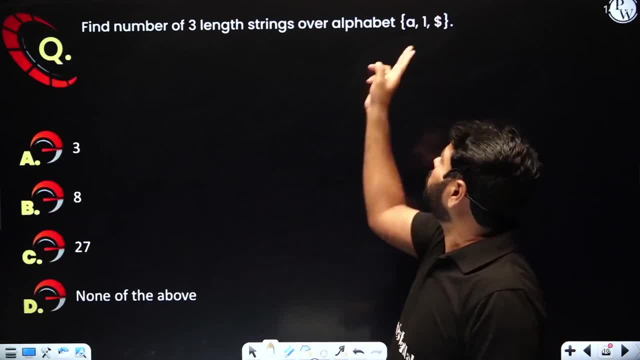 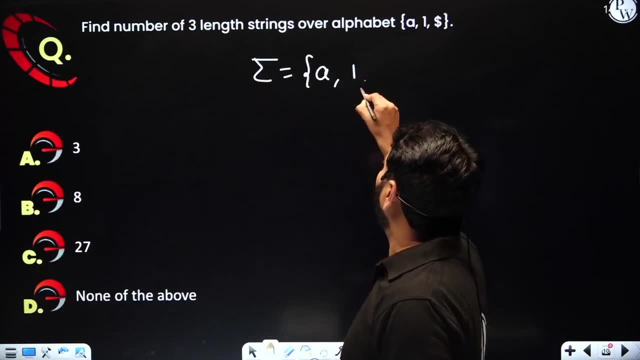 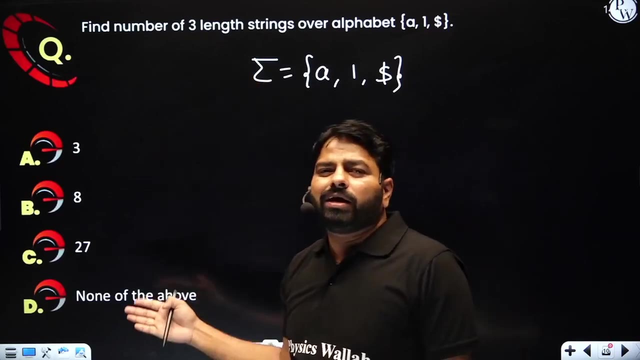 These are the three different symbols that I need in my language, So I have Formed the alphabet: a1 dollar. Here we have three different symbols: a1 dollar. Now you need to form the three length strings right. So you require a concept of formula that can give you a direct number. 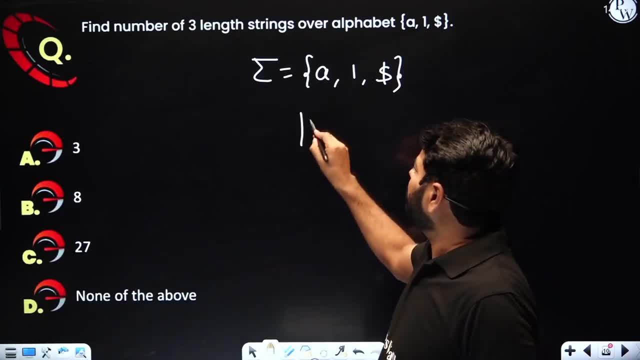 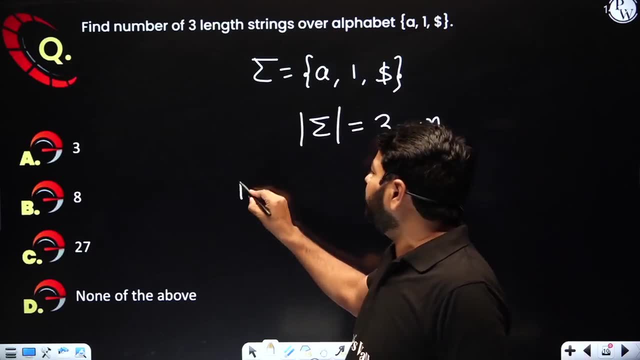 So I already explained how many symbols are there. The size of the sigma is three instead of n. So I already mentioned it is n. Now if you want to find the number of k length strings, you can use That if you have remembered it. otherwise you can form it. 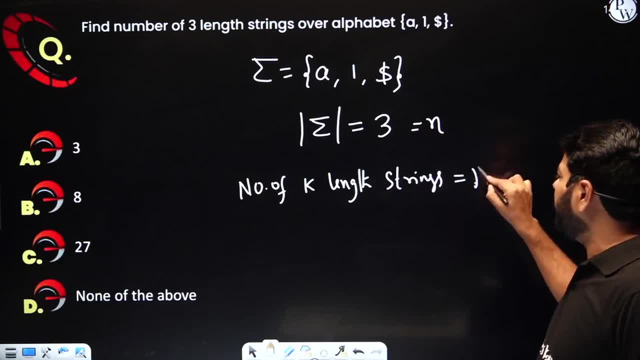 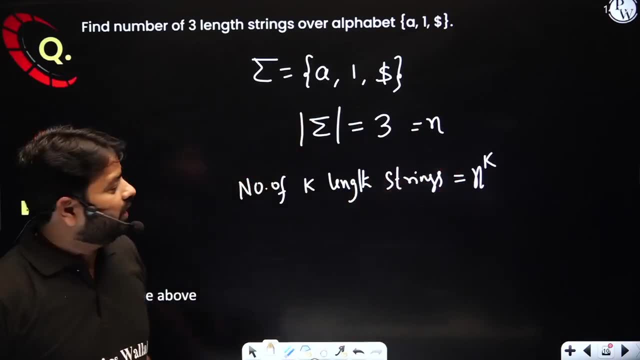 Number of k length strings is equal to what did I mention? n power k, because each position you will have n choices. There are k positions, total n power k. Now n is here three and k is here also three, So no confusion. 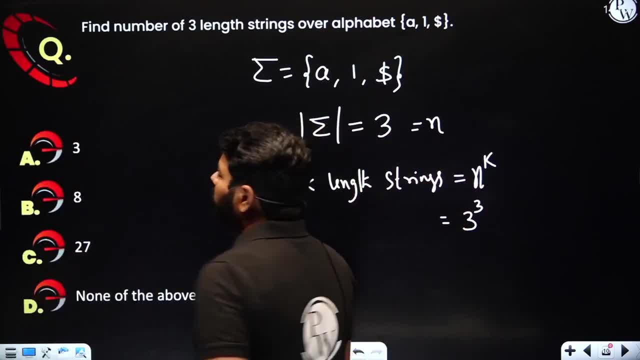 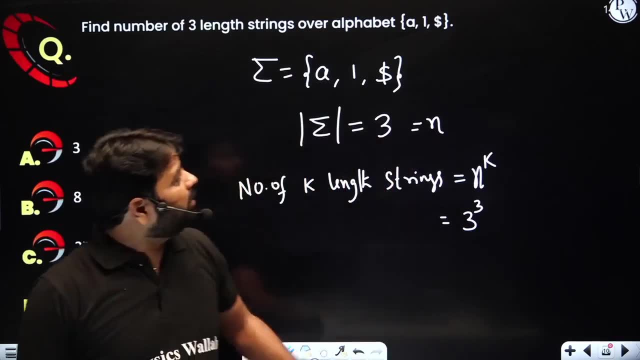 n is three, k is three, So three power three. So which is the right option for you? 27.. This is how you calculate number of a k length strings over n symbols: A number of three length strings over three symbols. Fine. 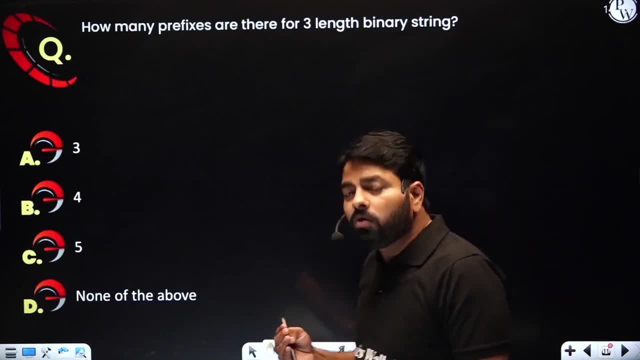 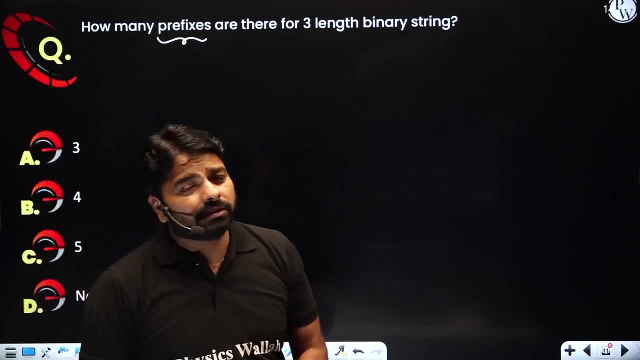 How many prefixes are there? Okay, this is another kind of operation over the string. So now, first you should know what is a prefix, Then only you can find how many prefixes are there for the three length binary string. Binary string, when they mention the alphabet, is given to you. 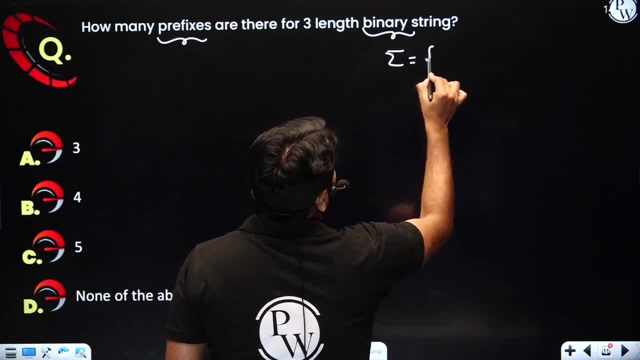 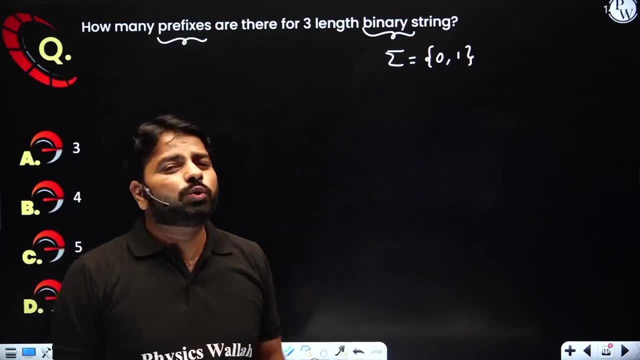 Binary. it mentioned that sigma is having two symbols. You may mention zero one, Or you may mention a comma b, or you may mention x comma y, but keep two symbols in the sigma. Now I'm assuming it's a very famous for us binary language digital right. 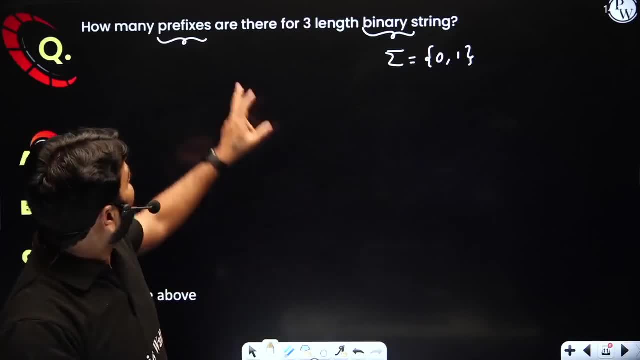 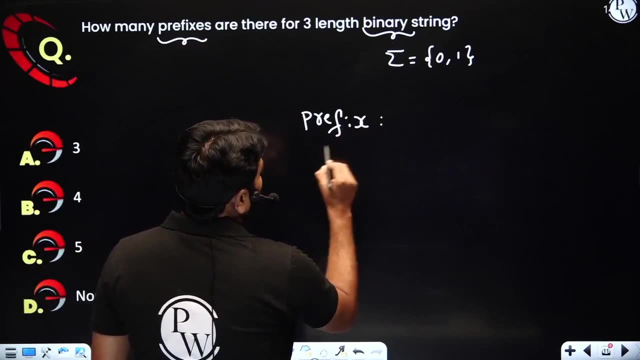 In the logic we use the two symbols zero or one. Now how many prefixes are there Before that? what is a prefix? What is the prefix of a string? Let's say string is 101.. I have taken three length string to understand easily. 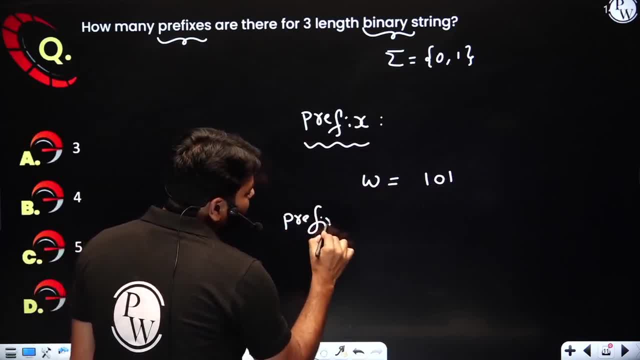 What are the various prefixes that you can write? What are the various prefixes that you can write? What are the various prefixes that you can write? How to write a prefix over the w Prefixes of w. What are the things you can write? 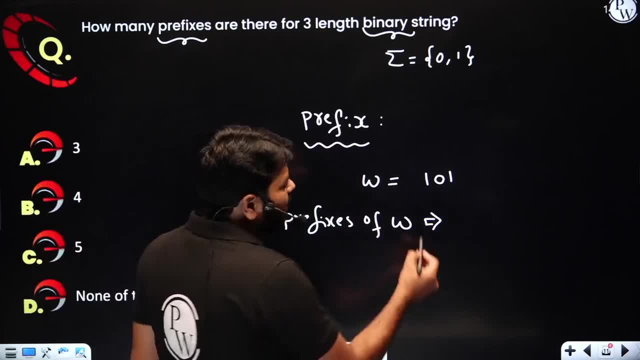 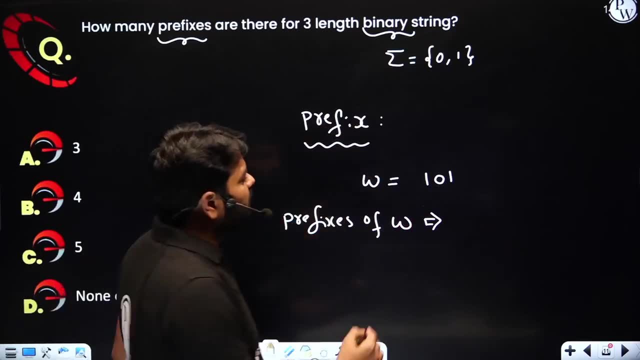 You know in this string, Whether you take prefix, suffix, substring, any kind of operation over the string, like sub sequence, anything, you always follow left, right. But where do you begin, Where do you end And what do you take? Three things are different. 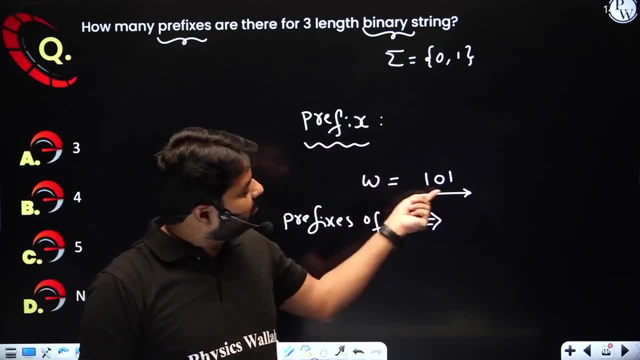 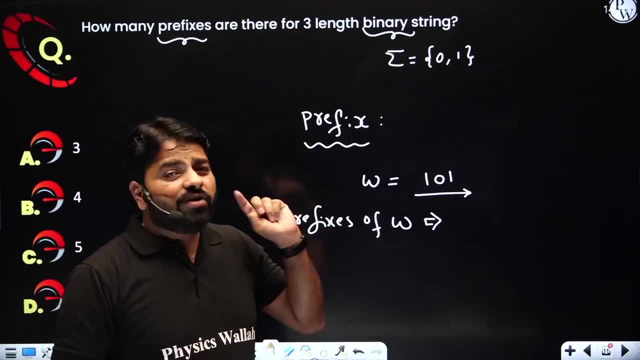 Where do you begin And where do you end And what symbols you consider in the sequence, sequence from left to right. remember, these are the three points are important. so in the prefix, where do you begin? begin is always in the first position, here, before the first position. 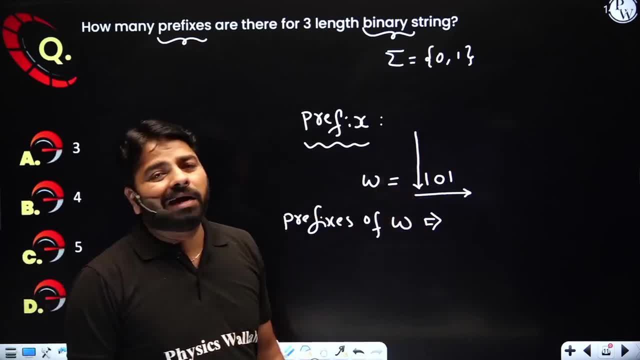 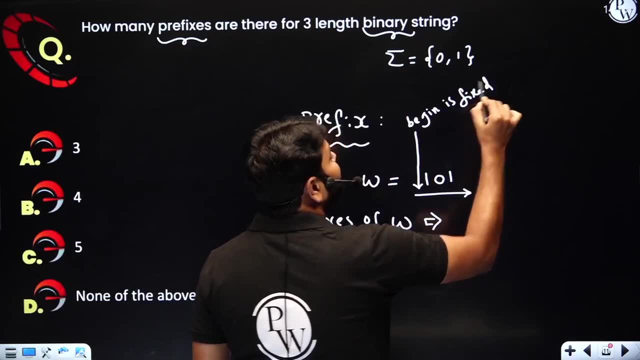 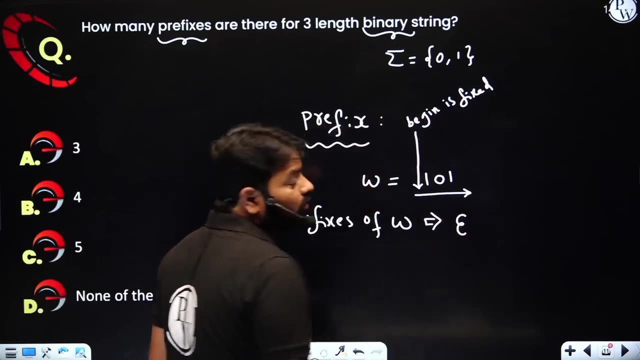 where do you end doesn't matter. so beginning is already fixed in prefix, end is anywhere. so i have the choices to end. if i begin here and end here, you will have epsilon. so epsilon is very special prefix of the any string. you take any string in the world, epsilon. 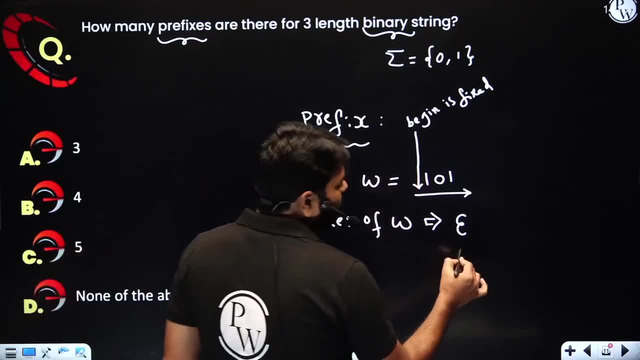 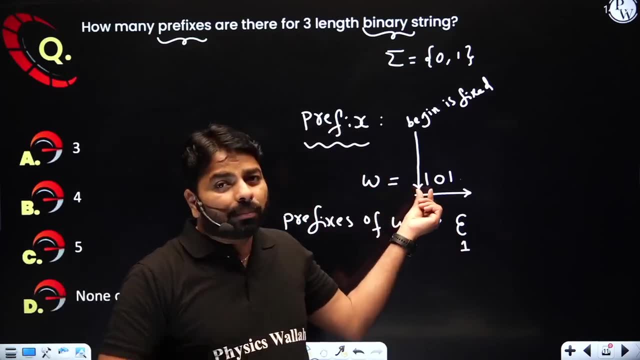 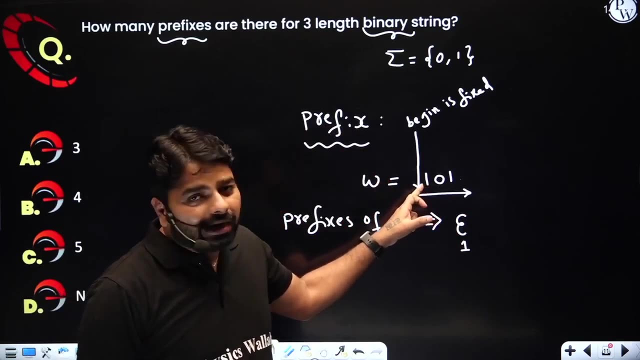 is always a prefix to that string. next, what else you can write. you can start before one, you can end after one. that is sequence of all the leading or beginning symbols of the string, the sequence of all the beginning. so here, epsilon is there, one is there, and after one you can have zero. see, i'm. 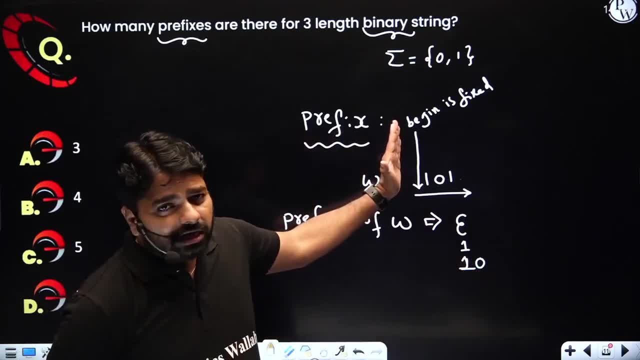 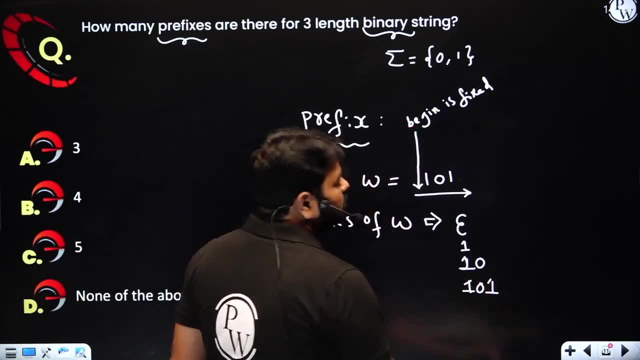 i cannot take zero directly. why? because beginning is fixed. if you want two, two symbols, you can go up to zero. if you want three symbols, you can go up to one, zero one. so these are the prefixes are possible for the given string. now you may have doubt, sir, i have. 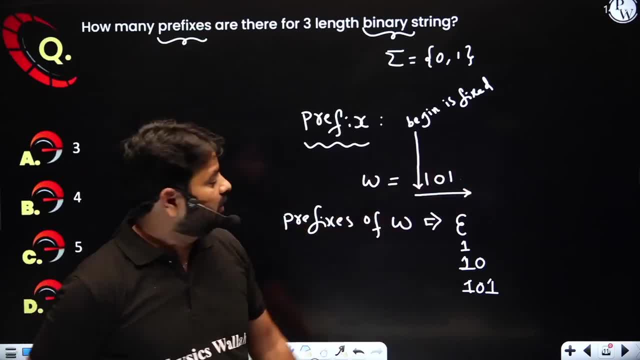 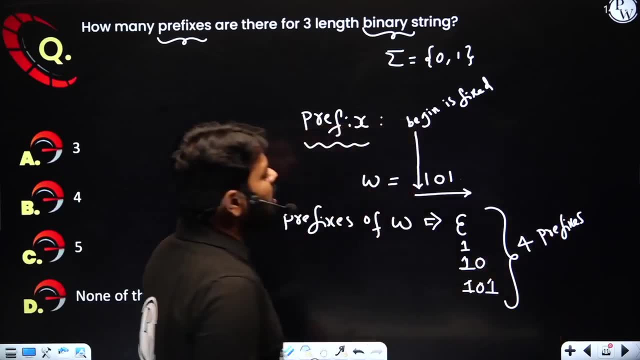 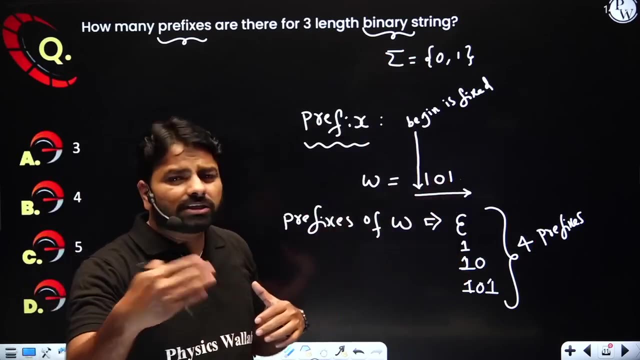 three length string. how many prefixes i can have? total four prefixes. these are how many. are there four prefixes? now it's very easy to answer. how many prefixes are there for three length string? it's not only one zero one. you can take any three length, three consecutive zeros or one one zero. anybody you take, you will have four prefixes, but prefixes. 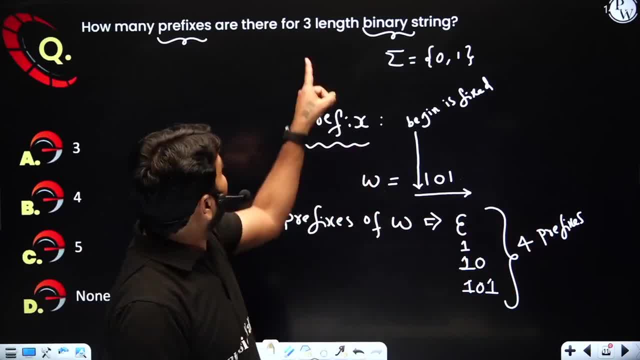 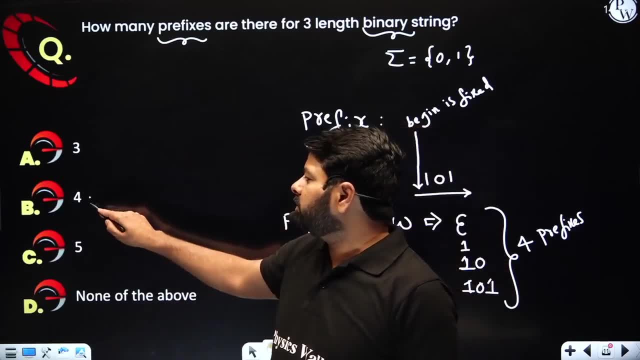 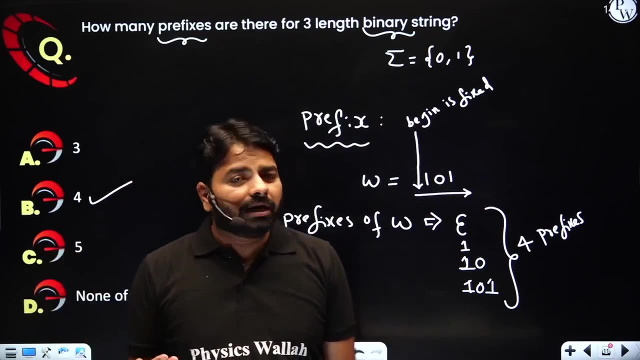 might differ, but number of prefixes will before always. so now you can answer easily for the three length binary string: how many prefixes are possible, how many prefix are possible. that is for okay. sometimes you may have answered three other thing. three: when will be that? that is in the 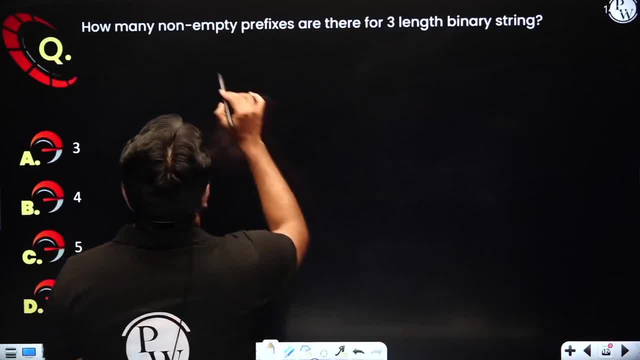 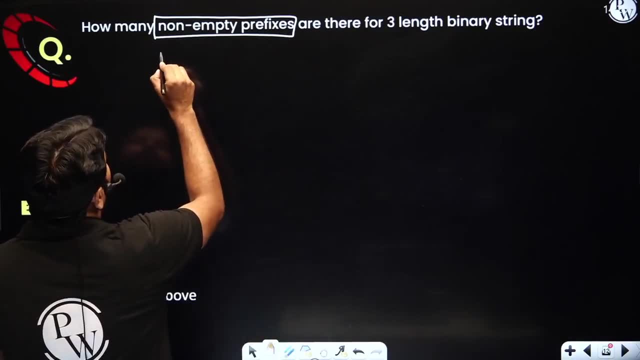 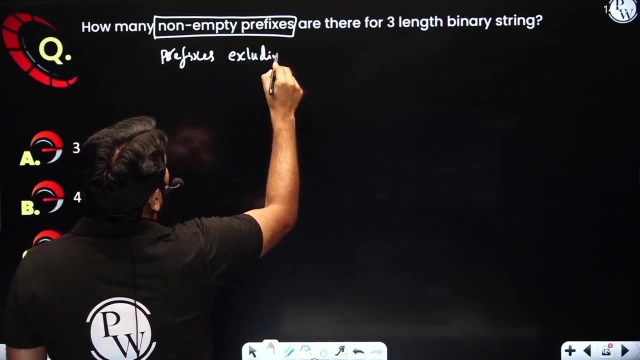 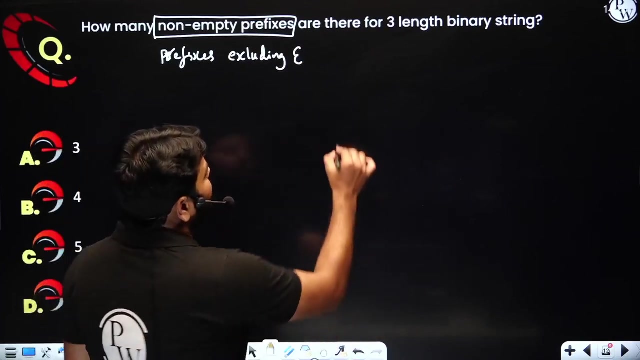 next question: how many non-empty? so remember this non-empty prefix. that means exclude epsilon. it means prefixes, prefixes excluding epsilon. you can't include epsilon now. previously, when I asked how many prefixes, epsilon was included. now you can't now I'm just taking again: W is equal any the length. 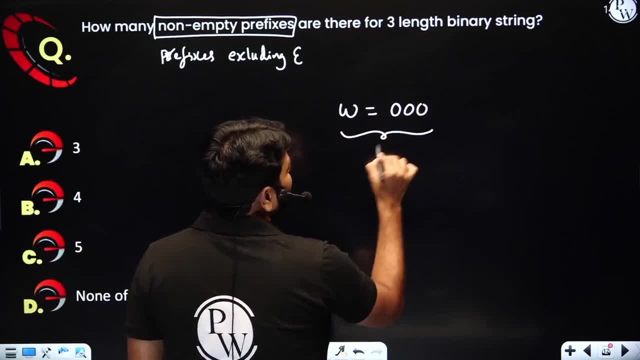 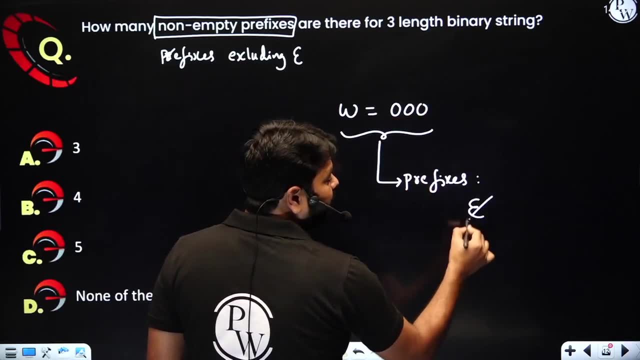 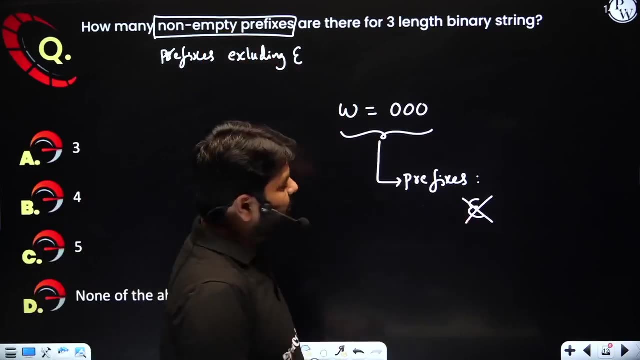 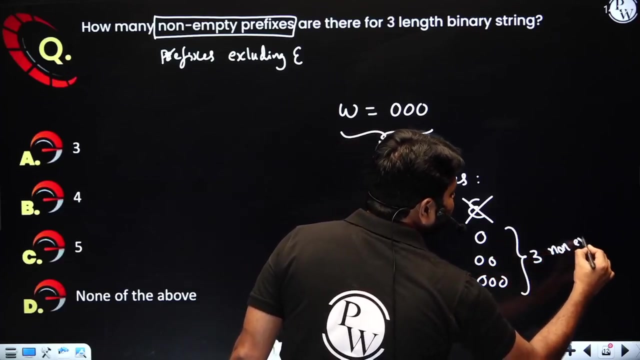 0, 0, 0. now what are the prefixes are possible prefixes? one is epsilon, but that you can't take now as non-empty prefix you require. this is empty. this is empty prefix or empty string. you can say now: 0, double 0, triple 0, how many? you got 3 non-empty prefixes. 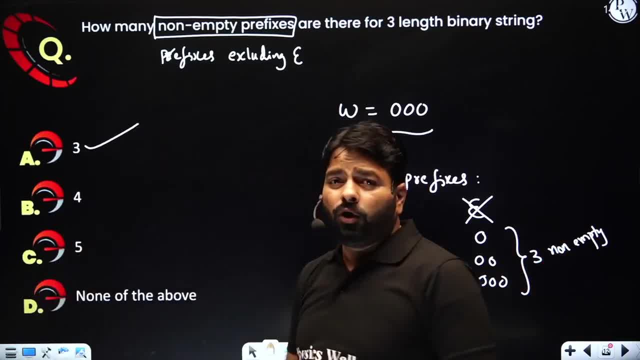 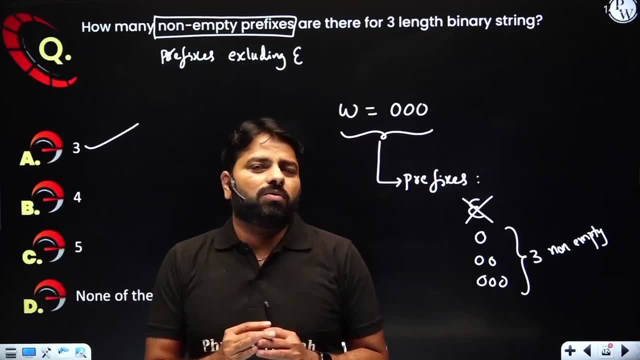 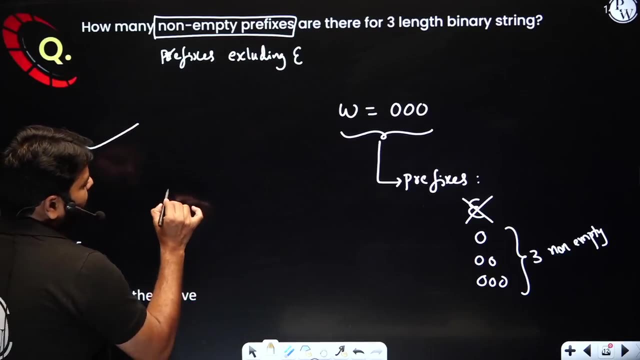 so you will answer now. 3: I hope you have a difference now. when they ask non-empty prefixes exclude epsilon. when they ask number of prefixes include epsilon in general. you can write a concept now when the length of the string is n or let's say K. 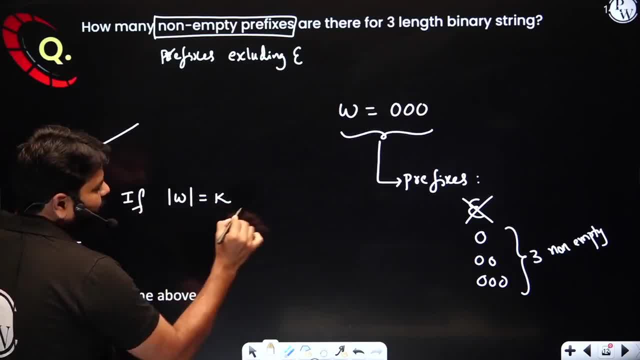 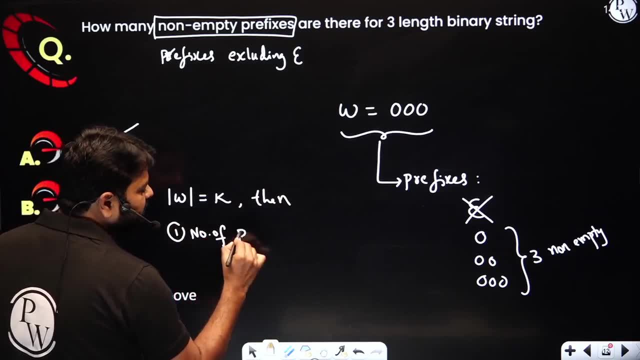 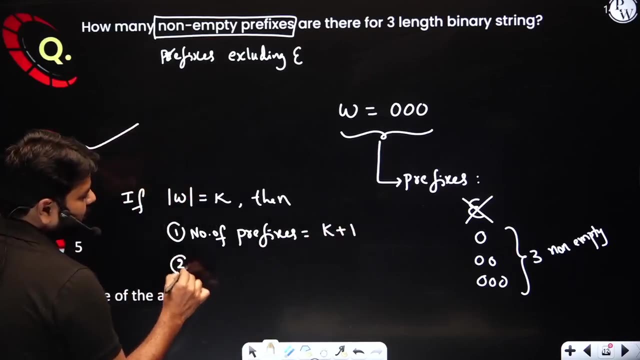 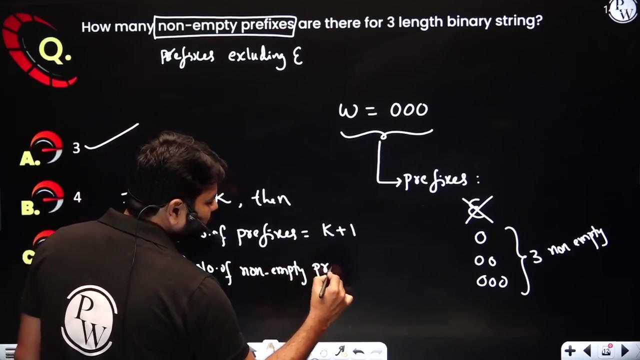 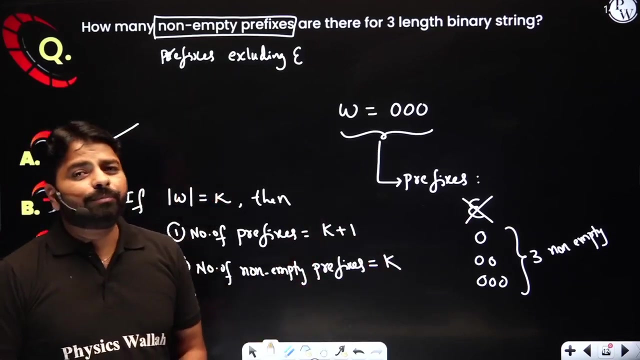 assume W is a string, then first point: number of prefixes is always K plus 1 number of non-empty prefixes. hey, where that one epsilon is deleted. so this is how you can form the prefixes. similarly you can also learn suffixes, substring. let's look at some of the 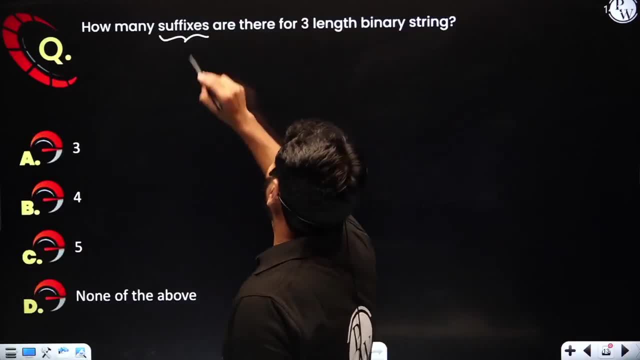 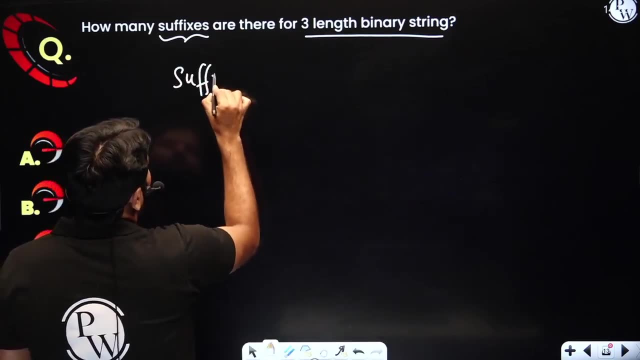 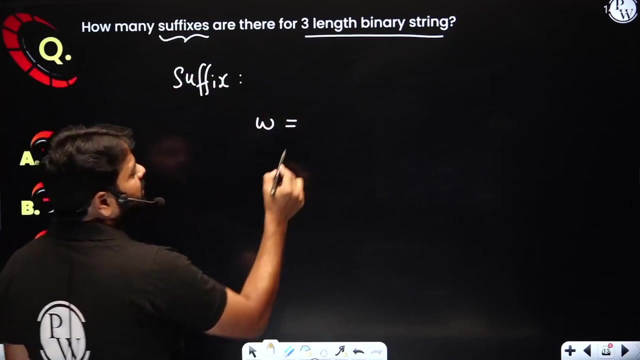 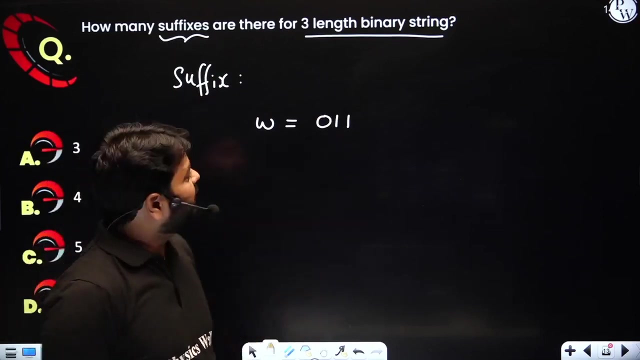 important operations. how many suffixes are there for three length minus string? now, what do you mean by suffix? as usual, let's take the string suffix of a string. let me take a first string, then I will find the suffix: 0, 1, 1. now what I told in prefix. the beginning was fixed here in. 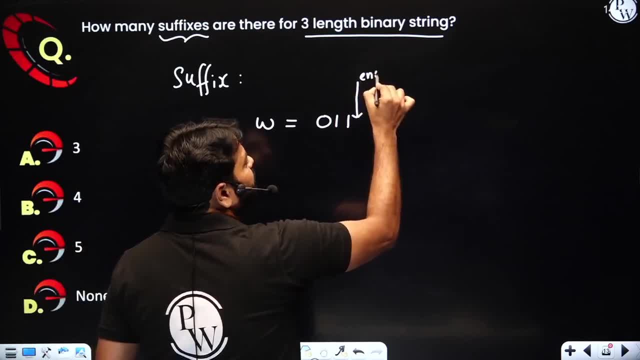 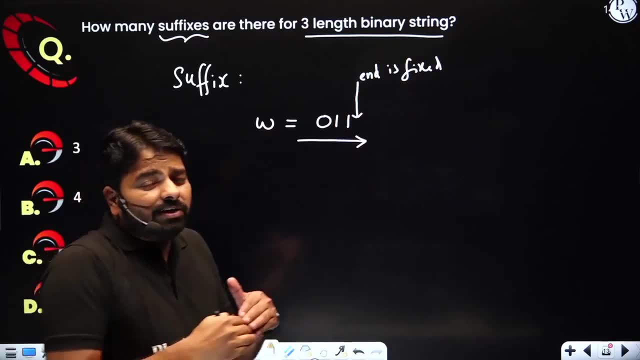 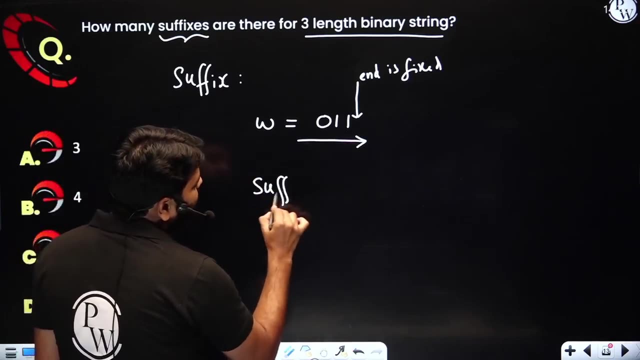 the suffix ending is fixed. now, where is the beginning? that's your choice, but sequence is always from left to right. it's the sequence of ending symbols, a trailing symbols. now, what do you get if your suffix is fixed? What are the suffixes you can form over this w? 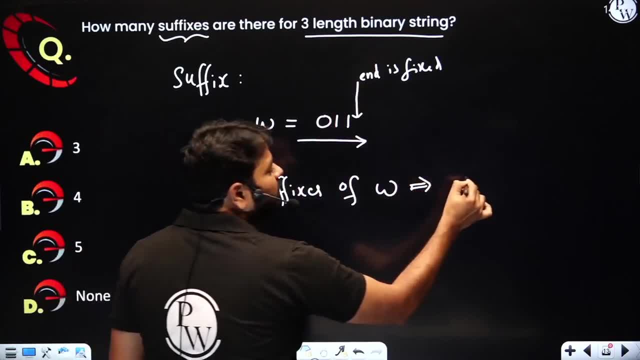 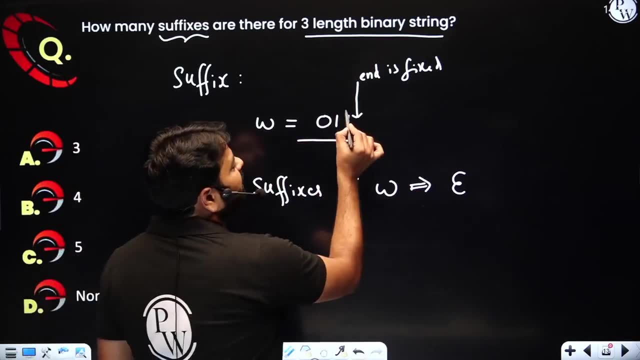 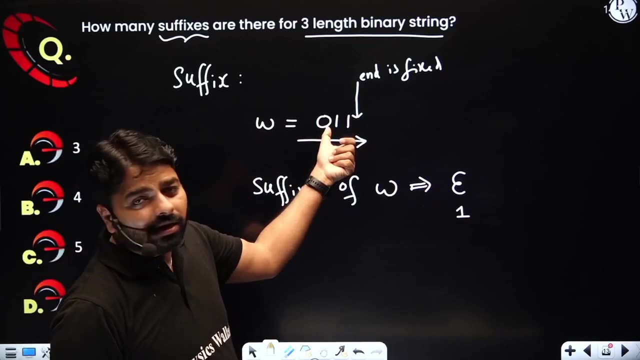 Now, if I start here itself and end here itself, you will have an epsilon. That means I have not considered even one symbol in the sequence. Then, if I consider one symbol in the sequence, that is only the last I can have. If I consider two symbols in the sequence, I have to end here so I can begin after 0,. 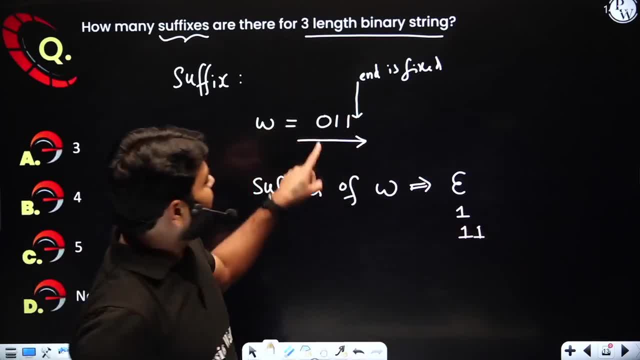 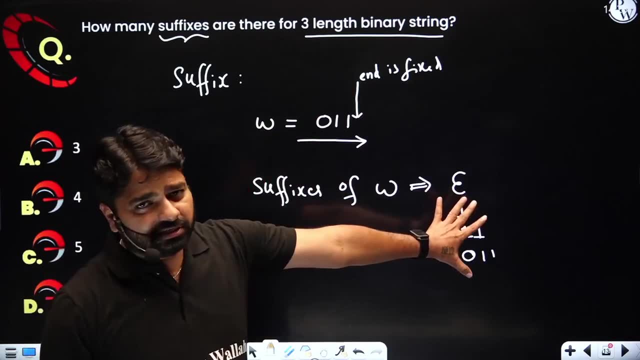 then you will have a double 1.. Then if I want to consider all the symbols that I want to begin in the beginning, then 0, double 1.. So these are the possible suffixes. These are the possible suffixes for the given string. 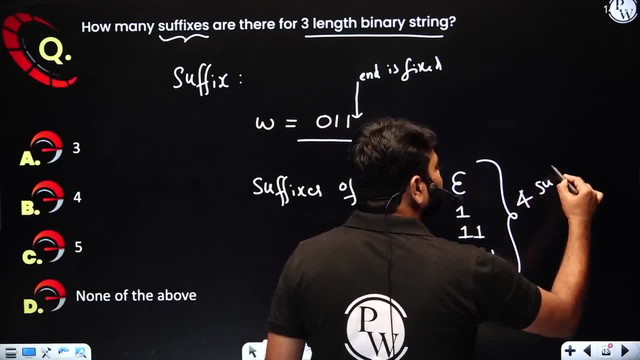 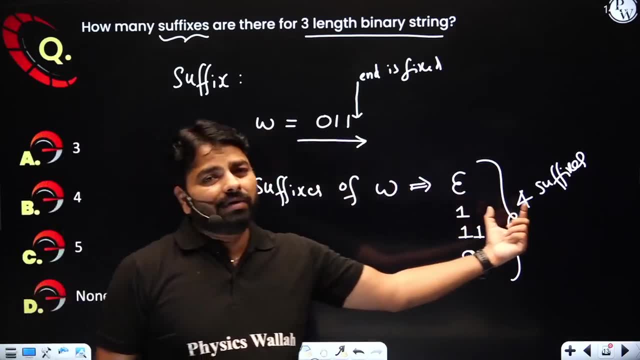 So again, how many suffixes? you have Four suffixes. When you have the three length string For the given three length string, you will have the four suffixes. This is how you can calculate Now onwards. you can easily answer it. How many suffixes For the given n length string: n plus 1.. How many prefixes: n plus 1.. So number of prefixes, number of suffixes will be same, But prefix suffix need not be same. Remember that point too. 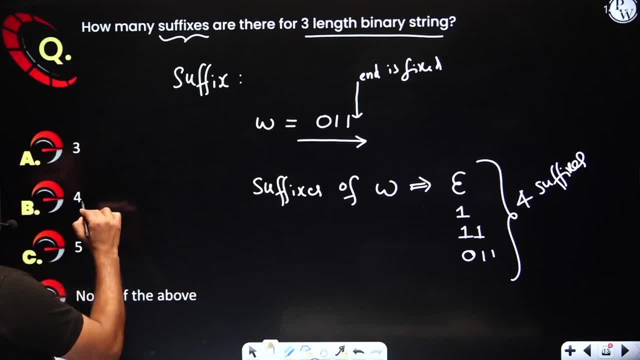 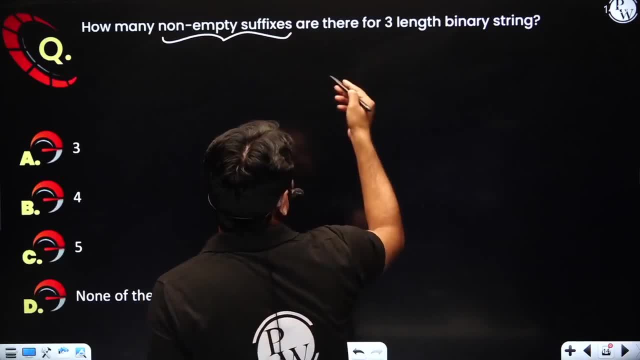 Now you can make a formula like: the answer is here: 4.. Similarly, if I ask non-empty, suffix same. Now I am not going to mention it. So total you have now 3 instead of 4.. Where epsilon is ignored. 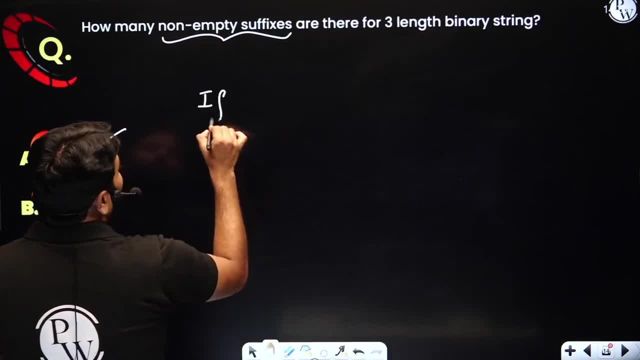 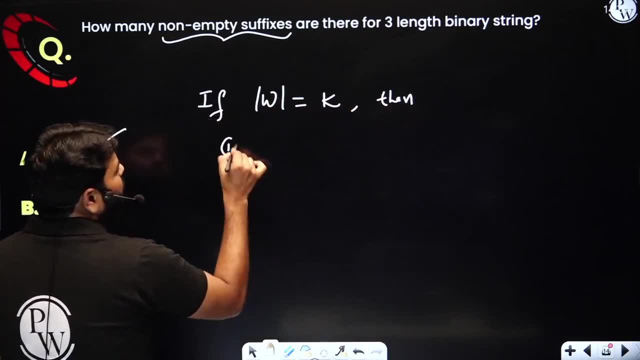 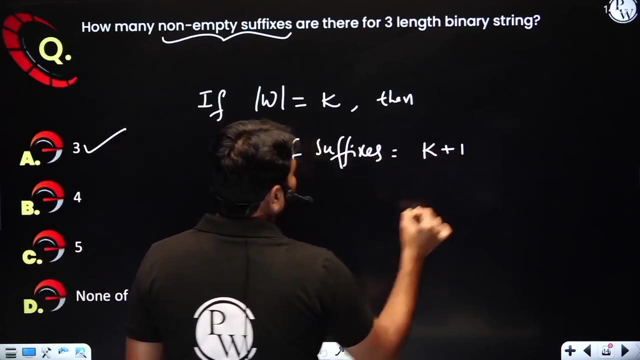 Where epsilon is ignored. So I am just writing: If the length of the string is k, then you may write the first point, the number of suffixes, Same like prefixes, which is equal to k plus 1.. And second, number of non-empty suffixes. 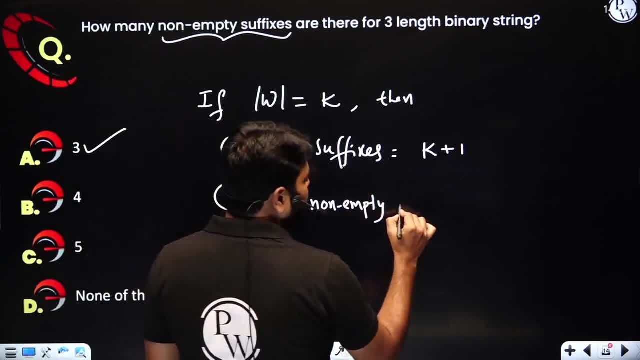 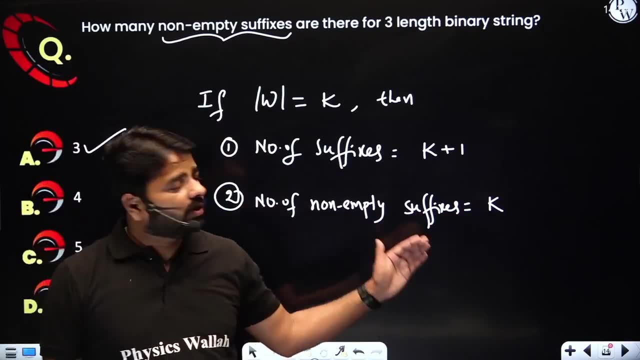 That means exclude epsilon, which is equal to k. I hope you got a clarity. What are the prefixes and what are the suffixes over the given string? And the count is always same when you are talking about number of prefixes and suffixes. 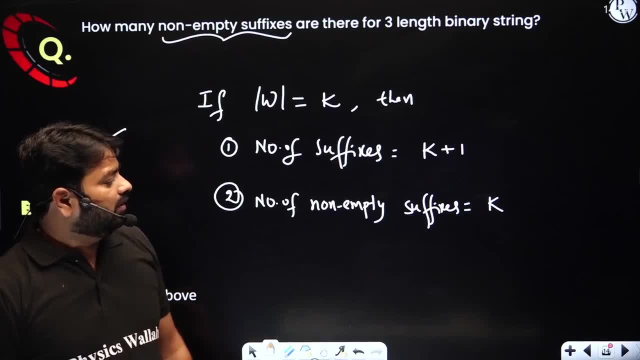 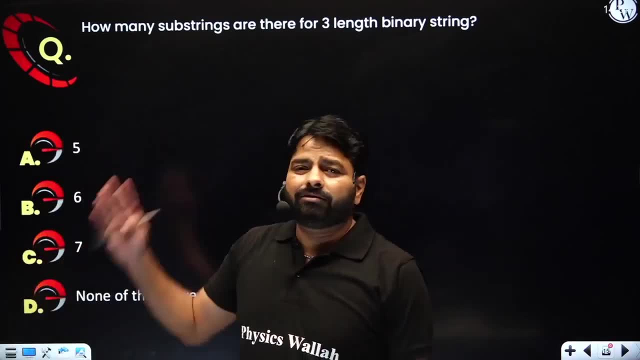 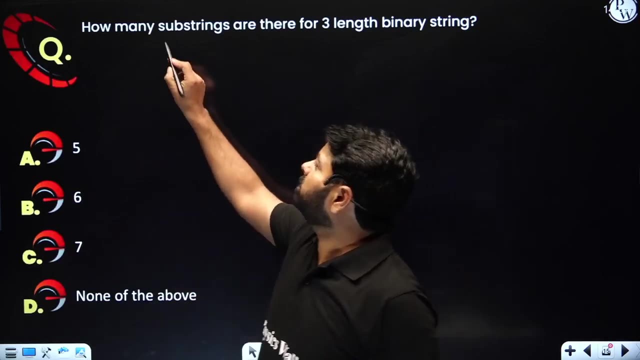 But only the strings may vary. Very interesting question. I have seen nearly 3 gate questions based on the substrings. Of course there are questions on prefix suffix too, But the majority questions are based on substrings. Why this is very important? 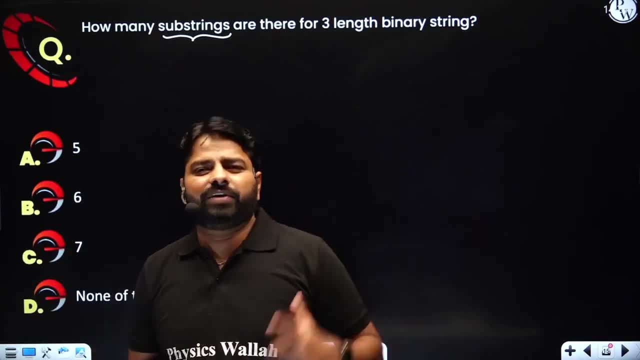 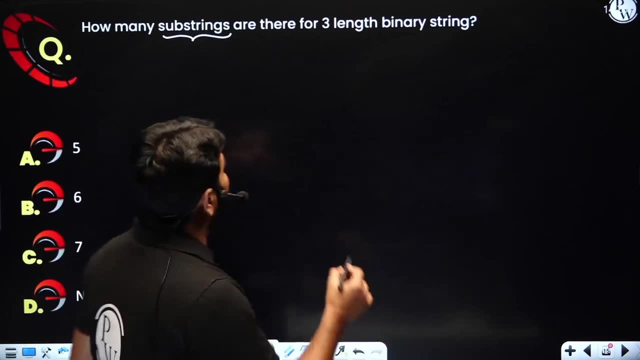 In prefix and suffix. it was so easy Because one thing was fixed And you always go from left to right in a sequence, So it is very easy to form. When it comes to substring, what is the substring first Before answering this question, what is the substring first? 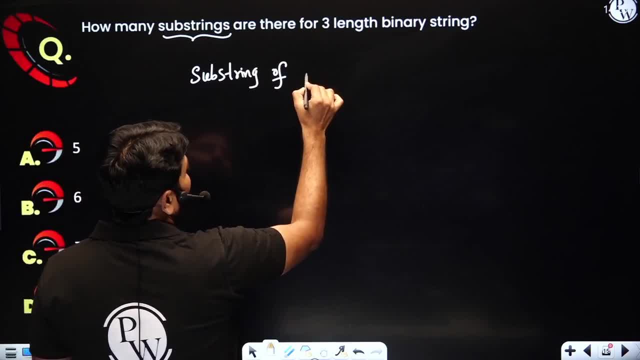 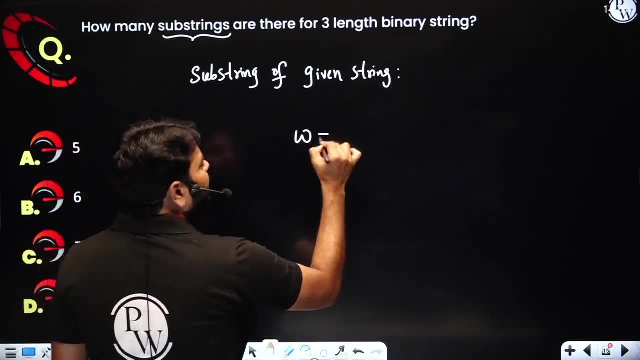 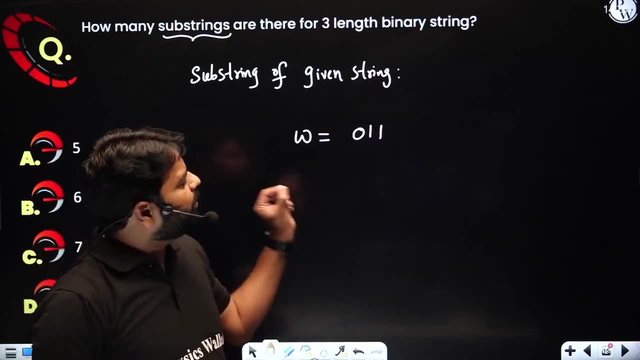 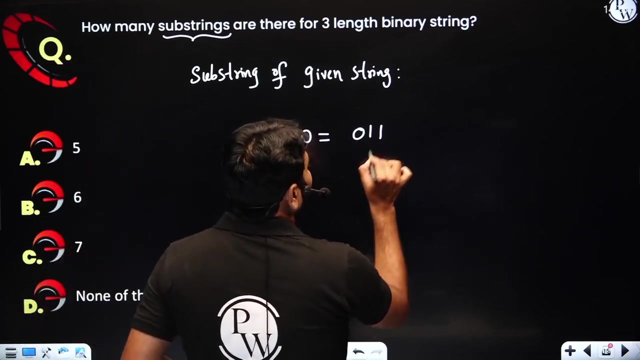 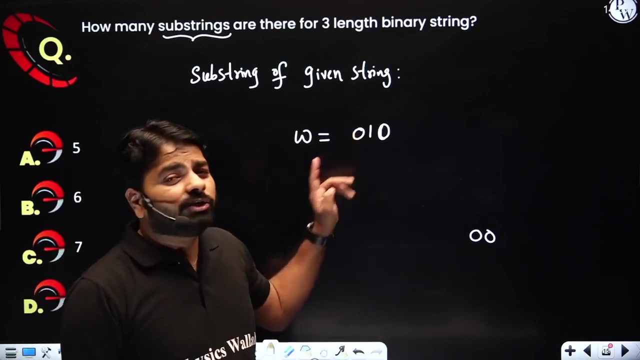 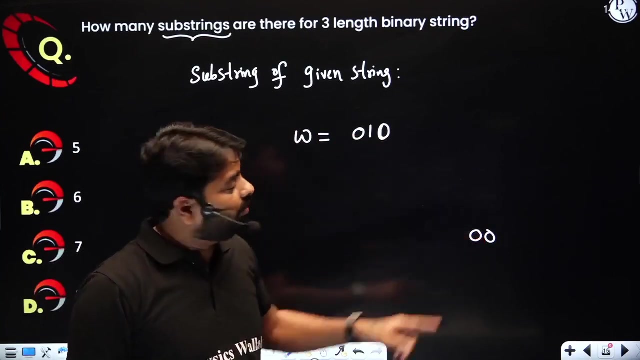 Substring of any given string, Right? So given string, let us say 011.. 011.. Now you can try to understand The substrings. it should be the part of the string somewhere, but part doesn't mean that. suppose I have here instead of 011, here you have a 010, 00. you can't write. it is not a part. part means it should be there somewhere and should maintain a sequence: 00, both symbols are there, but not in the same sequence. right after 0, another 0 is not coming. you can't take such a thing as a substring. 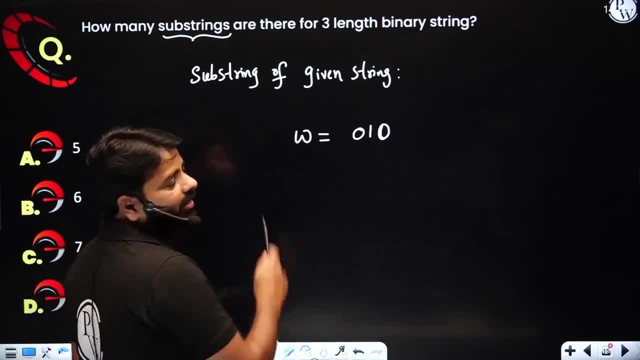 Now, what do you mean by substring? It should be the part of the string somewhere. So now what part you want to consider? Sequence has to be left to right and you can take any part. Let us try Substrings. What are the substrings possible? 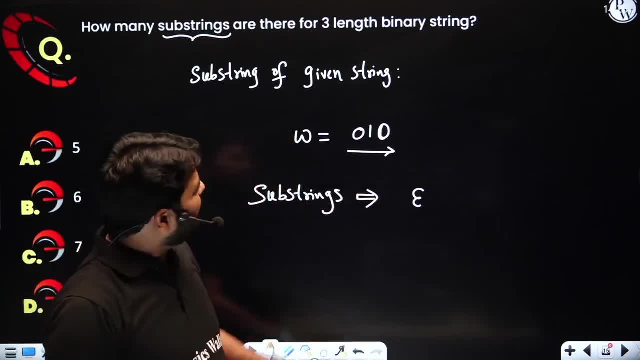 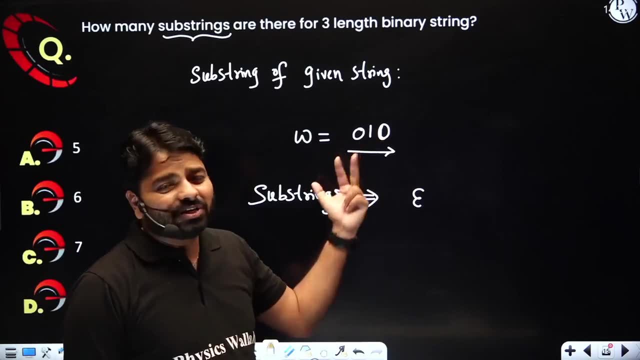 Epsilon. You may ask, sir, I can't see epsilon. but epsilon is there everywhere Right After 0,. so many epsilons are there In between 10,. so many epsilons are there In between 01.. 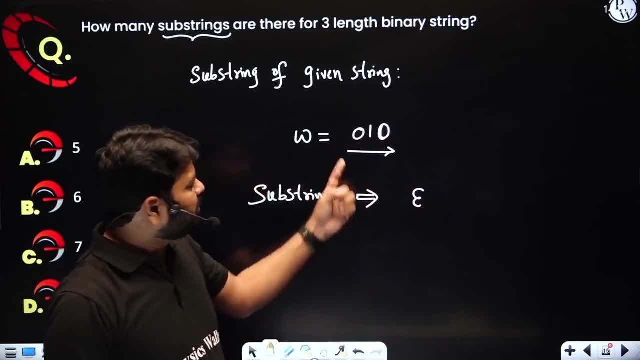 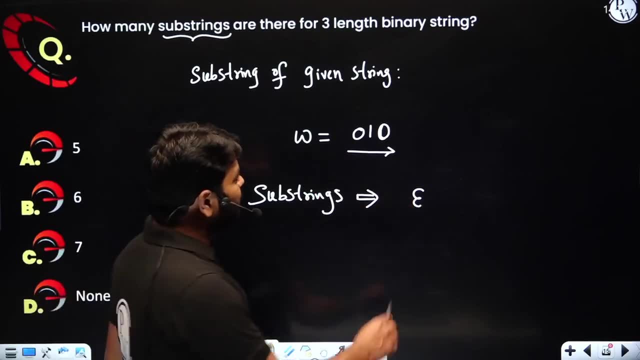 That is what the epsilon property and behavior that epsilon means. I am not considering any symbol That means epsilon. Epsilon is part of it, but it is 0 length string, Now 0,. how do you get 0 from this string? 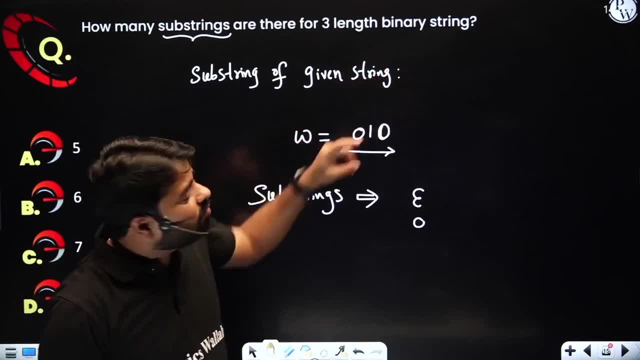 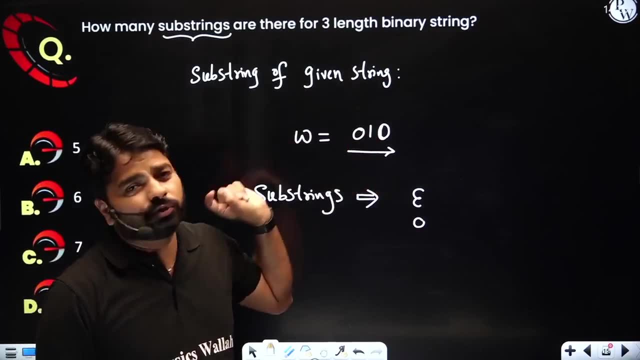 There in many places. You can take from here or you can take from here One length string. I can take it as a part of the string. So this 0 is a part of the string but appeared in various positions. That's fine. 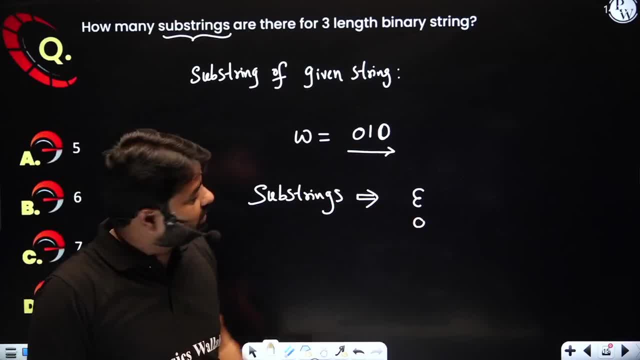 It could appear in more than one place. This string could present in more than one place, Right Next, 1.. Is it present? I am concentrating on one length first. First, 0 length. I focus, Yes, there, And 1 length is also there. 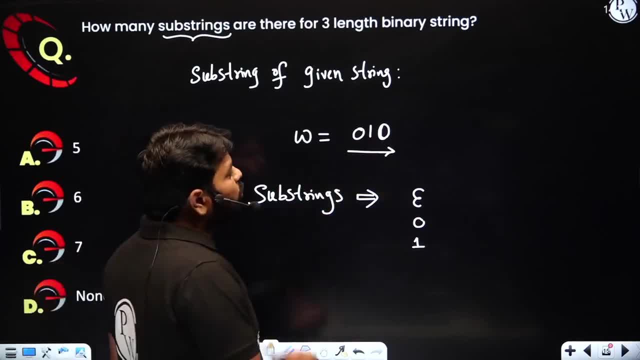 So this 1 is present at one place. That's fine. Now, 2 length. When you write 2 length, what do you write? 0, 1.. Because that's there, in this position, in this path, And 1, 0.. 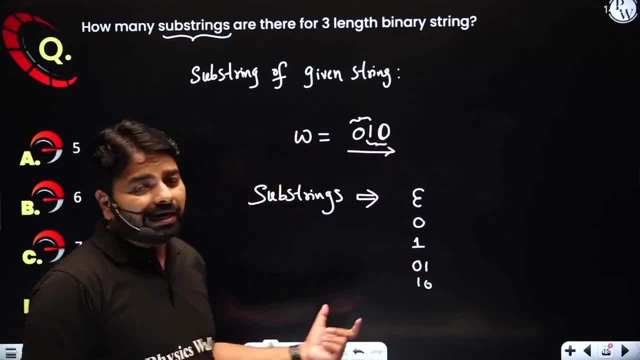 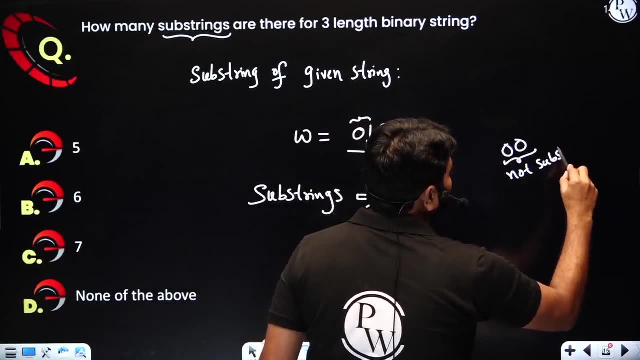 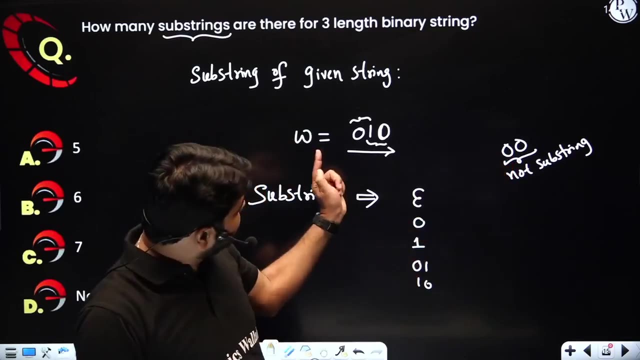 It is there here, But you can't write double 0.. That is what I am saying. 0, 0 is not a substring, But this comes under. if you study algorithms, this is called as a subsequence. You may skip some symbols to get this 0, 0. 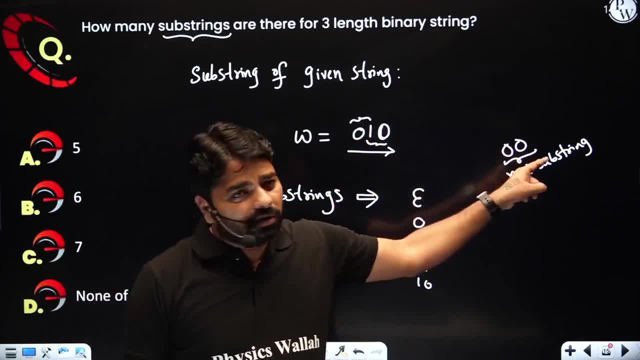 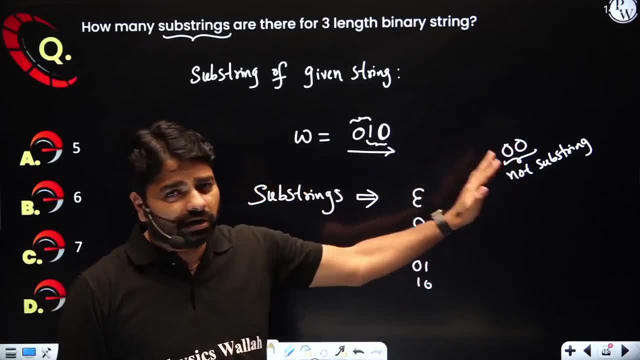 I am going from left to right. If I skip this one, I will get 0, 0.. So this is called a subsequence. So I am not talking about that. But right now it is not a substring. 0, 0 is not a substring. 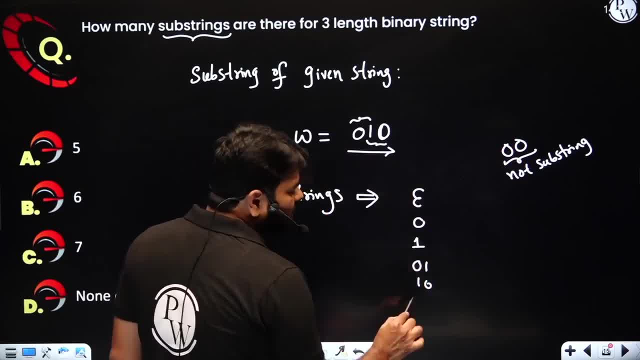 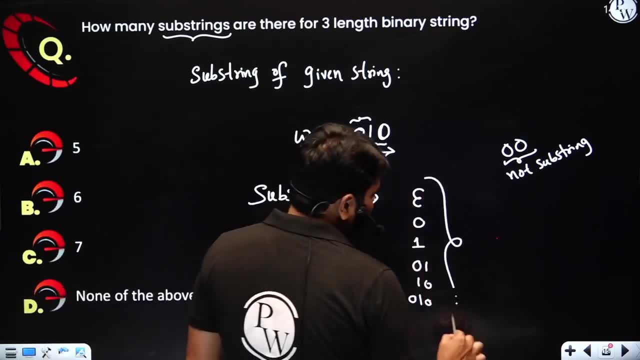 What else we have here? 2 length- I have considered all the possibilities- And then 0, 1, 0.. 0, 1, 0 is a 3 length substring. These are the possible substrings Right. 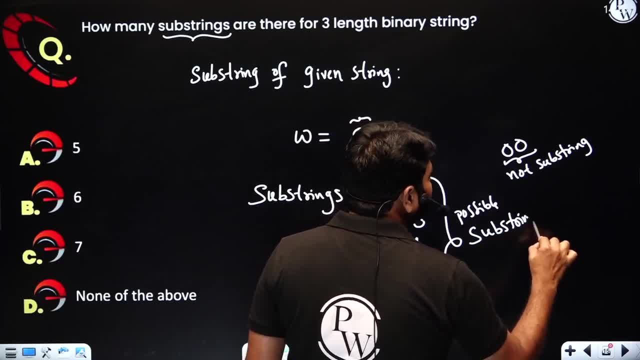 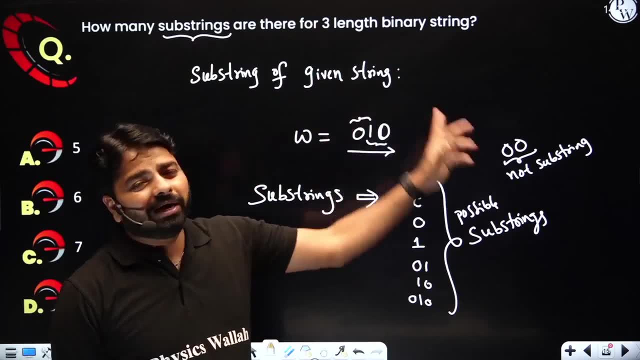 But you may wonder now, how many substrings? How do I find out? It's a very difficult, As you know. how many substrings are there for 3 length binders string It's not unique. Why it's not unique? 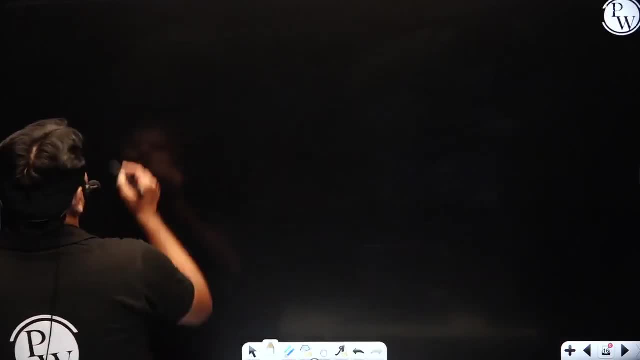 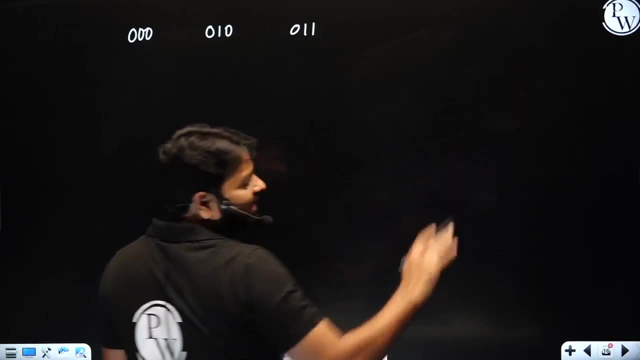 Let me take one example. Let me take 0, 0, 0.. And 0, 1, 0.. 0, 1, 1.. That's all enough. There are so many right, So I am just considering these 3.. 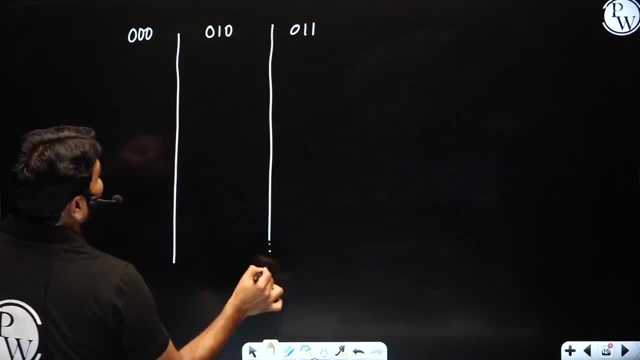 Let's say these are the 3 different strings we have. You are looking at a string. Now the question is here: find the number of substrings. You are trying to find here substrings. You are trying to find here substrings. 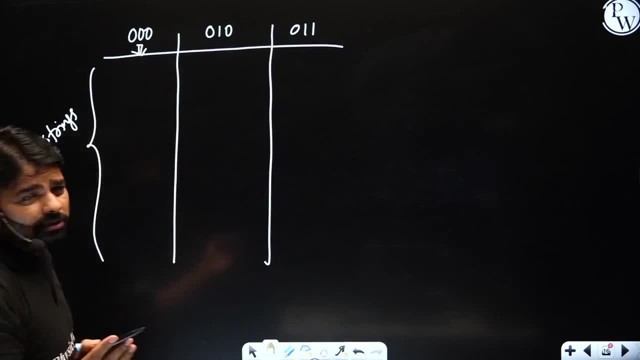 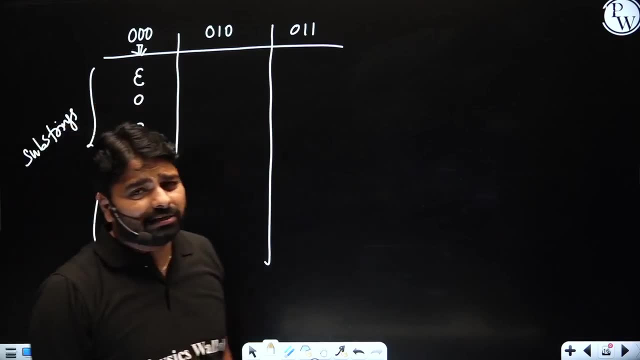 For these 3 consecutive zeros. what are the substrings possible? It should be a part of the string Epsilon 0, 00, 000.. That's it. You can't get more than these substrings. Now, when you take this: 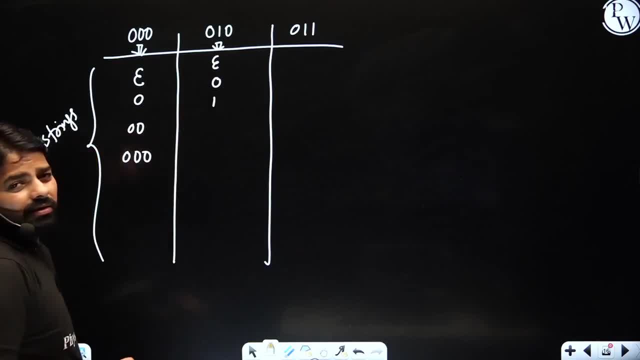 Epsilon: 0, 1, and 0, 1, 1, 0.. Just now we have tried right: 0, 1, 0.. Now, when you compare these 2, here, only 4 substrings are there. 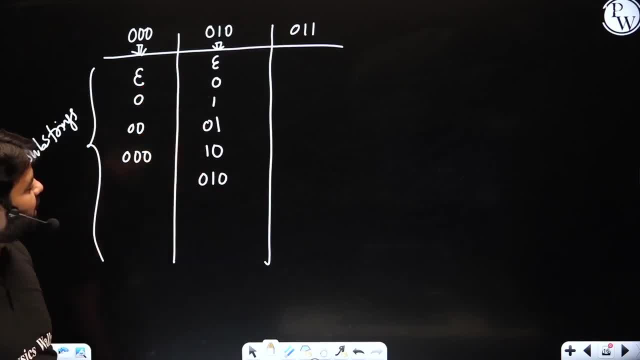 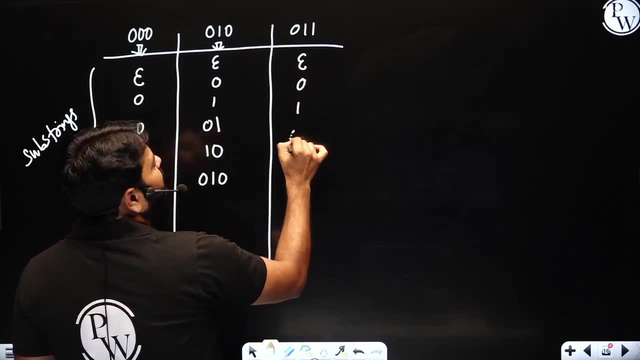 Here 1, 2,, 3,, 4,, 5,, 6.. Here 6 substrings are there. And what else here? You can see here Epsilon: 0, 1, 0, 1, 1, 1, and then 0, 1, 1.. 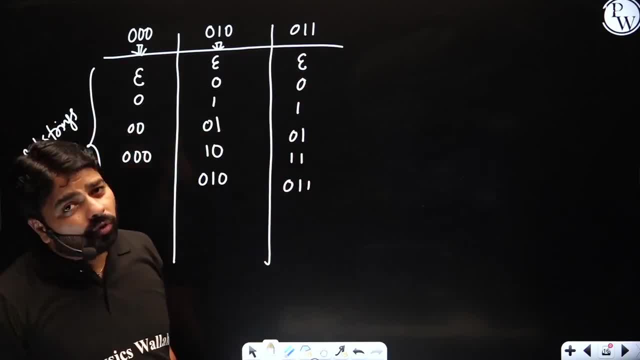 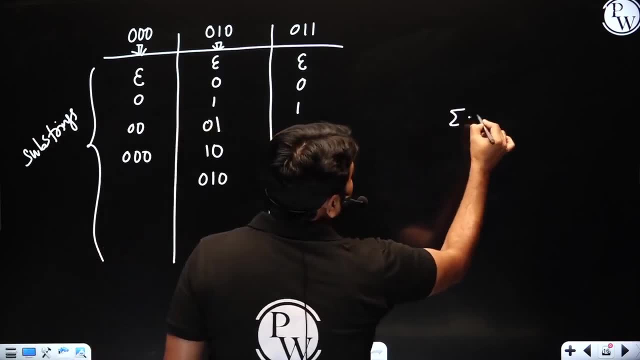 Here also you have 6. But sometimes you may have more too. Suppose, assume that your sigma is having 0,, 1, 2. Then what else? You know? I am just saying that sigma is, let's say, 0,, 1,, 2.. 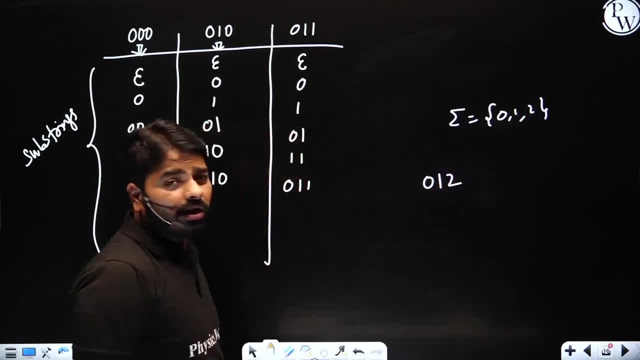 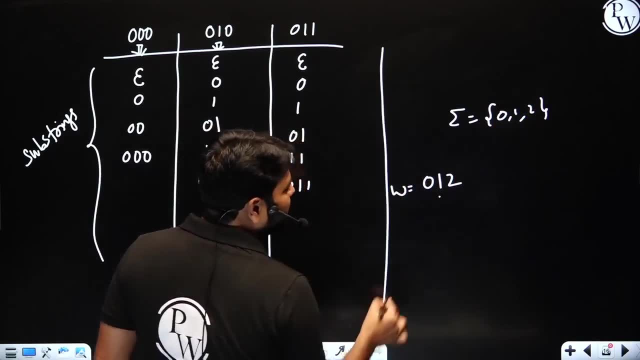 3 length. you may write 0, 1, 2 also, Or 2, 1, 0.. Or 1, 2, 0. All the 3 symbols are different. In that case, if this is W, this is a special example I am taking. 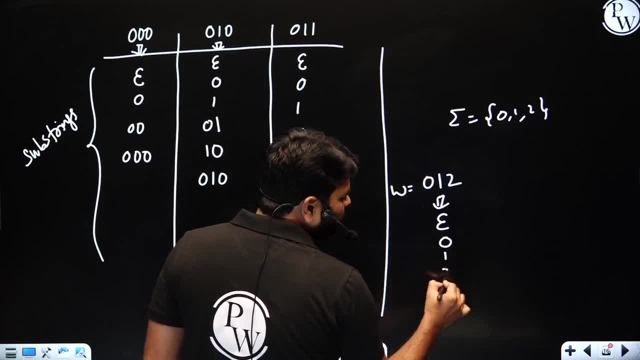 For this Epsilon: 0, 1, 2, and 0, 1, 1, 2, and then 0, 1, 2.. You look at now 1, 2,, 3,, 4,, 5,, 6, 7.. 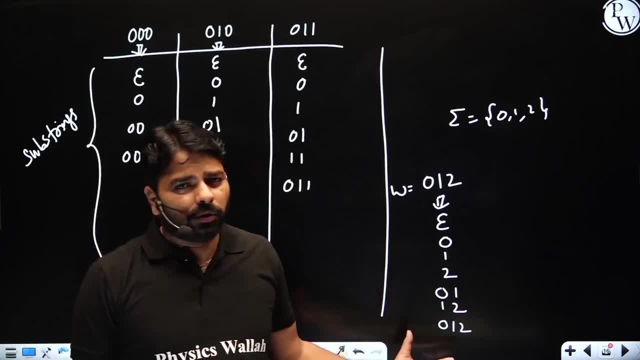 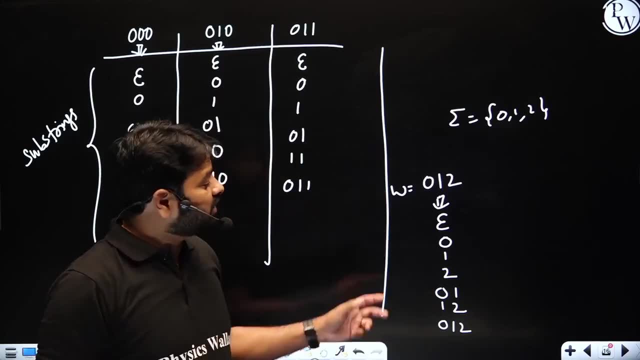 7 substrings are there Then how do you get this point Clear, what I am saying? So for a particular sigma, this number of substrings for any length is going to vary. See for the 3 length only you get different answers. 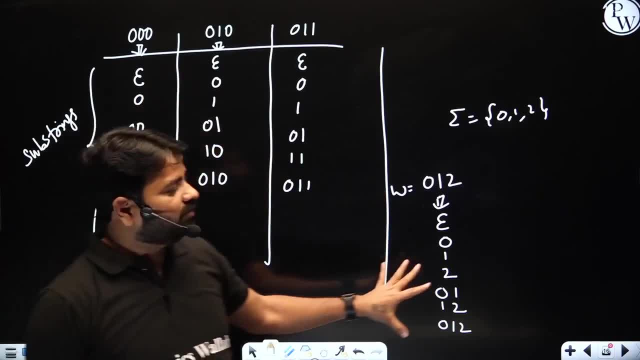 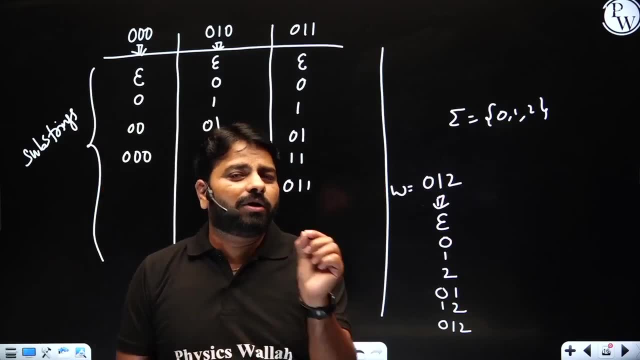 Like here you have 4.. Here you have 6.. Here you have 7.. It depends on the sigma. how many substrings are there. So what I say here, that depends on the string. the number of substrings will vary. 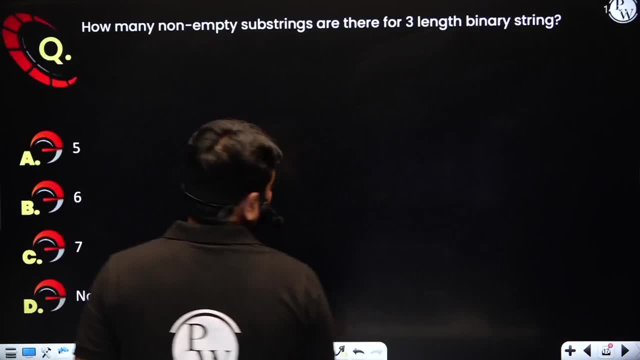 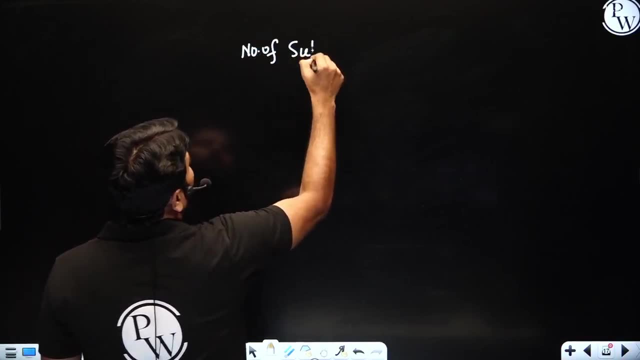 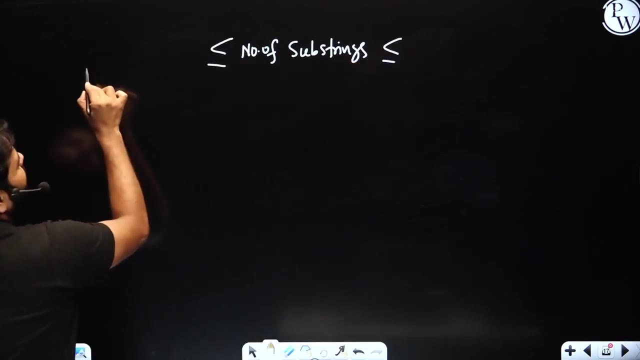 So I am going to make a formula for that. If you want to find the number of substrings, there must be lower bound and upper bound. The lower bound is always possible when all the symbols in the sequence are same, Like when you have: W is equal to 0, 0, 0.. 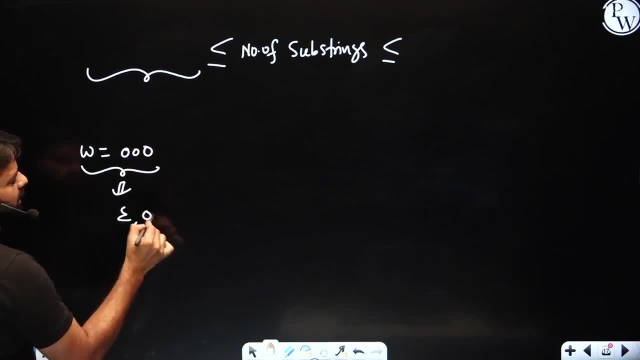 Then what are the substrings? are possible Epsilon 0, 00, 000.. How many? you got 4.. How did you get? If 3 length string is given, you have the 4 substrings. 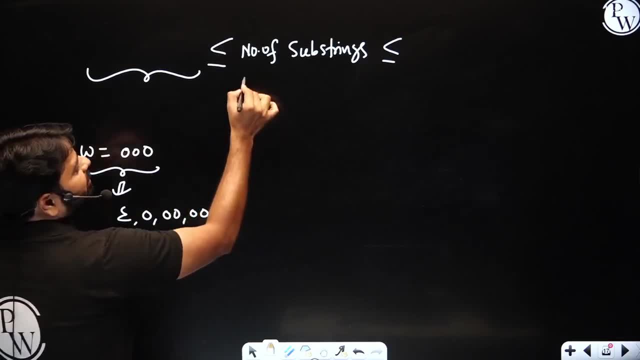 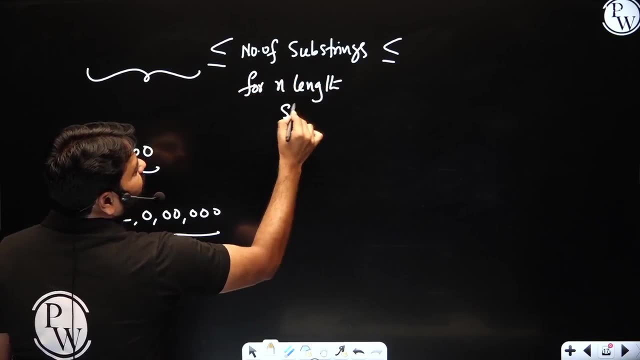 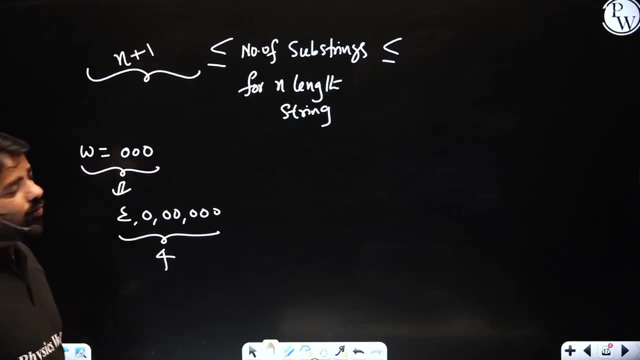 So if n length number of substrings for, let us say, n length string, Then you will have: for n length string, you will have n plus 1.. n plus 1.. But how do you form this? 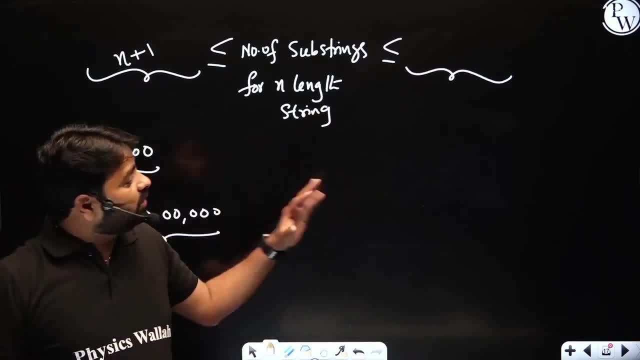 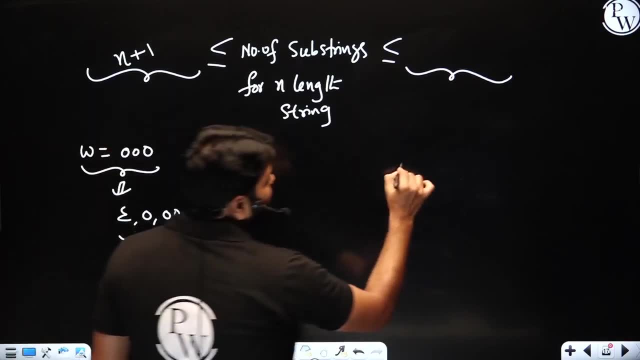 Let me take that example, Because I do not know what is the sigma given. So definitely I have to assume the sigma is in general could have different symbols in a sequence, So W. I am taking something like 0,, 1,, 2.. 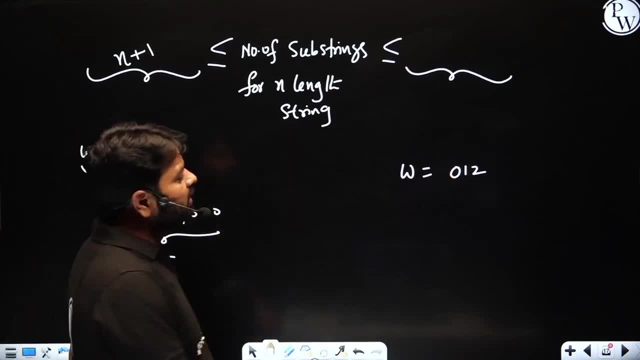 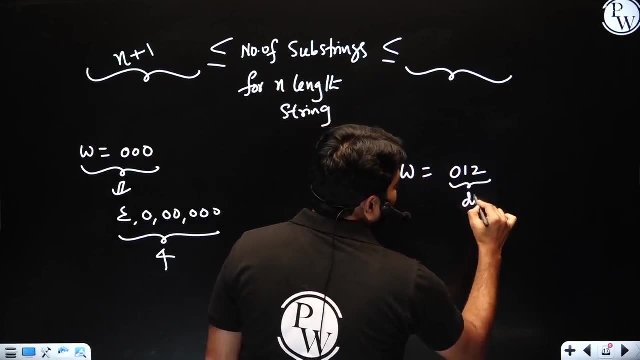 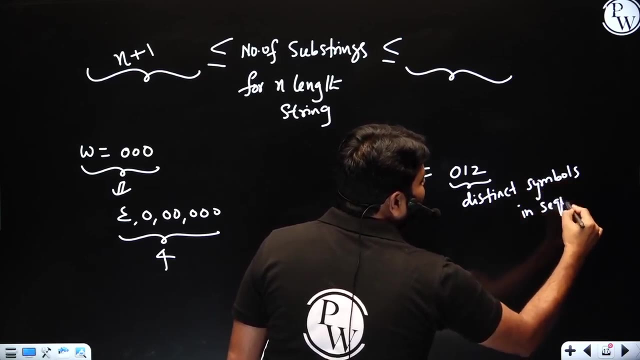 If the sigma is given, the formula is going to change, definitely. So here sigma is not mentioned. So I am just considering: all the symbols in a sequence are distinct, Distinct symbols in a sequence There is no repetitive symbol at all. 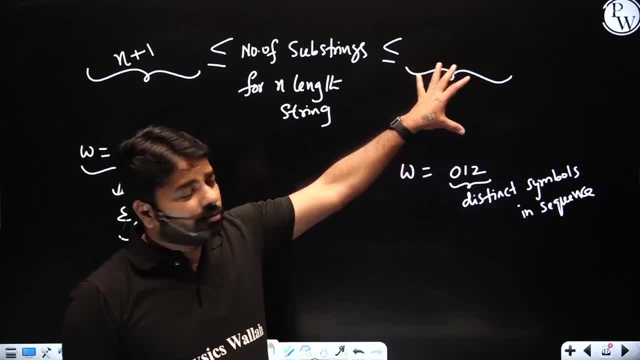 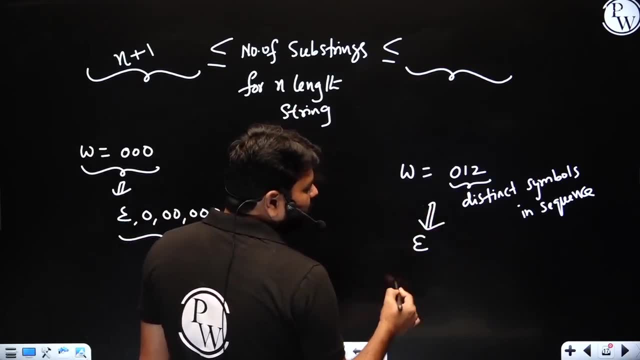 In that case you will get the maximum number of substrings possible for the given string. So how many you will get? So here, epsilon 0,, 1, 2.. It is a 1 length, right. 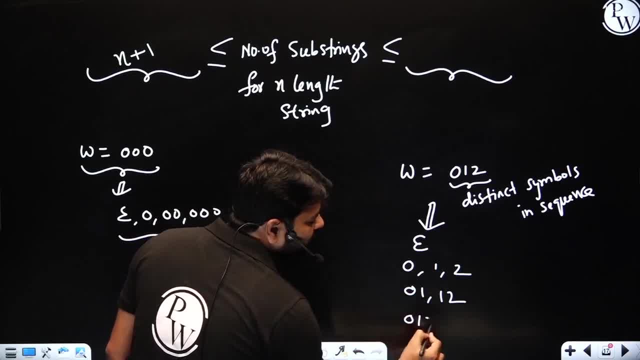 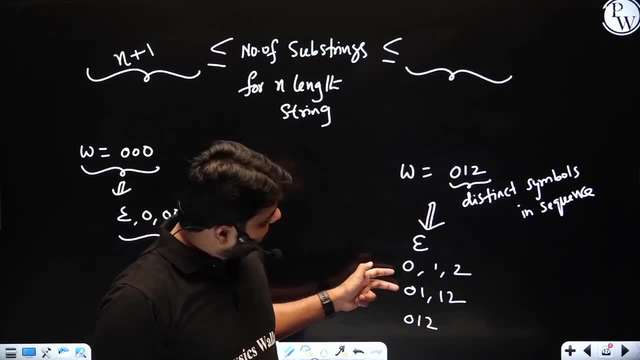 2 length. how many? you get 2. you get 3 length. how many you get? Only 1.. So I am just making a formula For 3 length string. you have total 7.. How do you get this 7?? 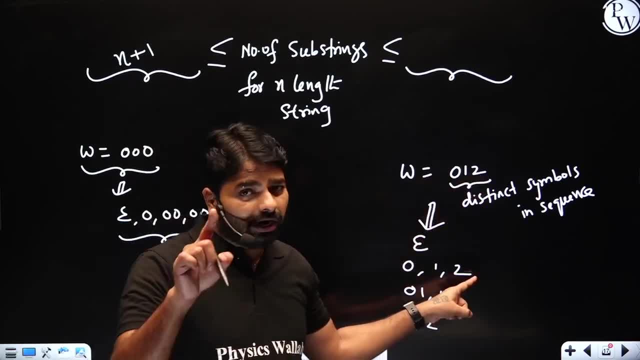 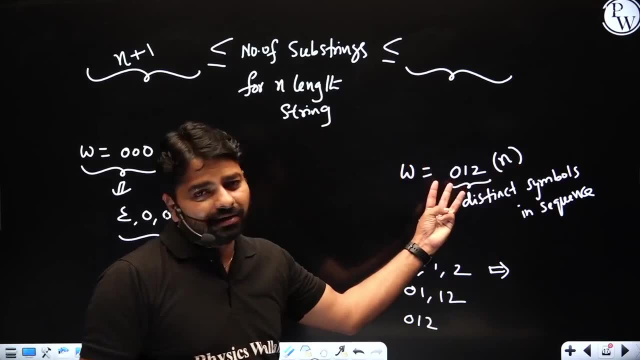 See, when you have 3 length, there are 3 substrings with 1 length. So this is in general. if this is n, Let us say n. n length means n is equal to 3 here. If there are n symbols which are distinct, you will have n substrings here. 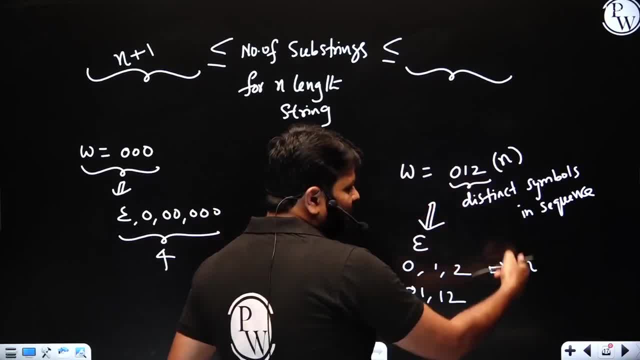 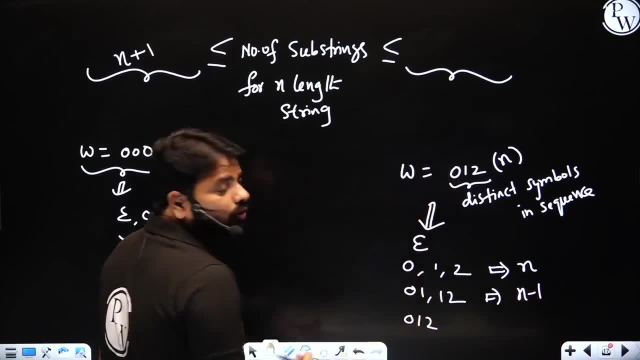 Right, 3 substrings here. 3.. n means 3 here. Remember that n means 3 here And here. how many you have n minus 1.. 3 minus 1, you have 2 substrings. 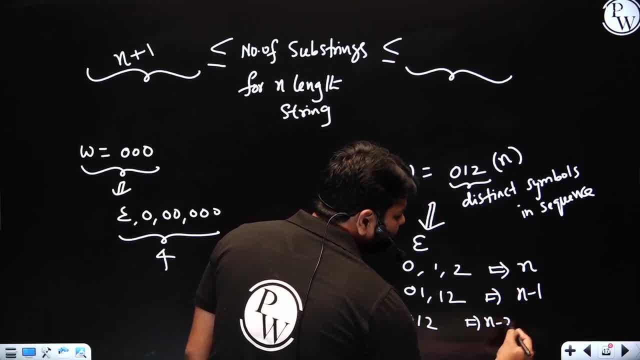 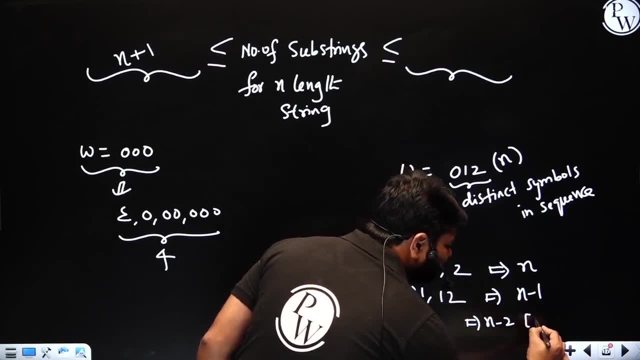 Here how many you have: n minus 2.. Keep on going till 1.. This 3 minus 2 is what 1.. Actually, it is what It is, 1.. So I am just mentioning in the square bracket: 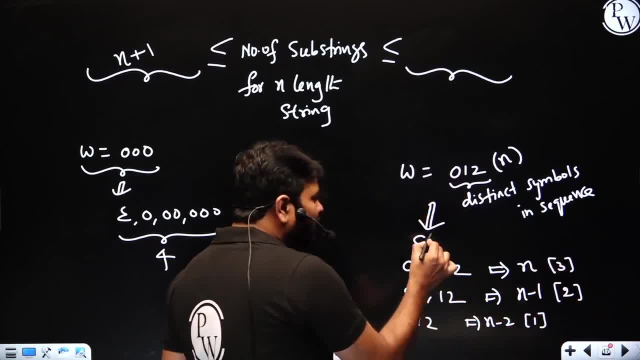 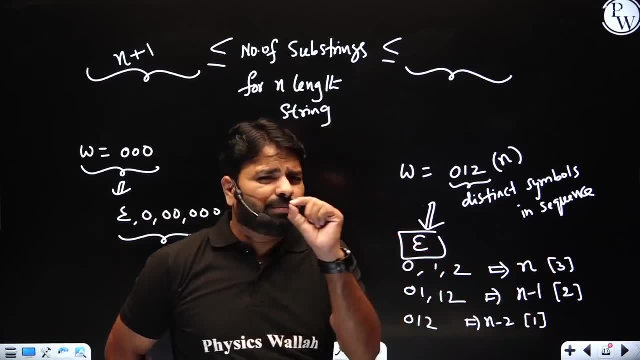 This is actually 2.. This is actually 3.. So additionally, you have epsilon. Epsilon is there for every string as a substring. Now, 1 plus 2 plus 3.. It is going to make a summation formula like 1 plus 2 plus 3.. 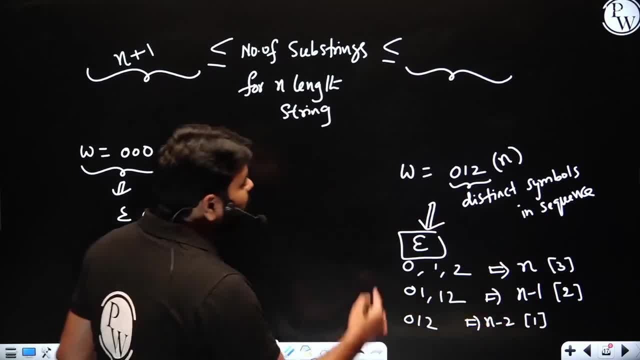 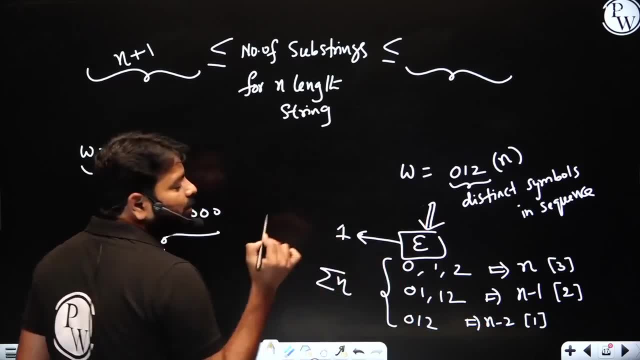 n into n plus 1 by 2.. If you remember this concept, sigma n concept, So in general, in general, this will form sigma n and additionally this will give you 1.. So sigma n plus 1, that is n into n plus 1 by 2, is a sigma n plus 1.. 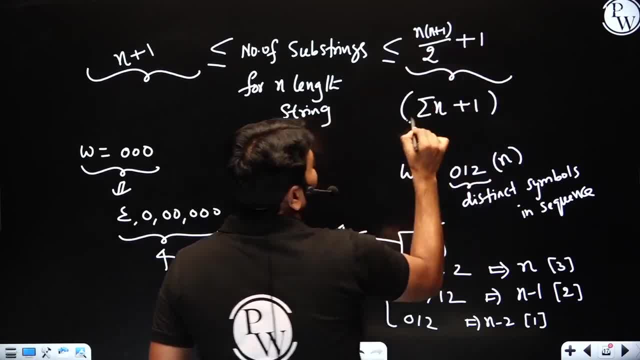 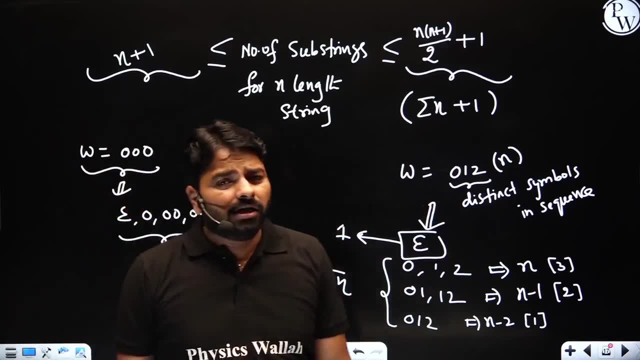 You can also write as sigma n plus 1.. When do you get When all the symbols in the string are distinct? That is the case. This is how you can calculate And remember. do not answer uniquely: always this one or always this one. 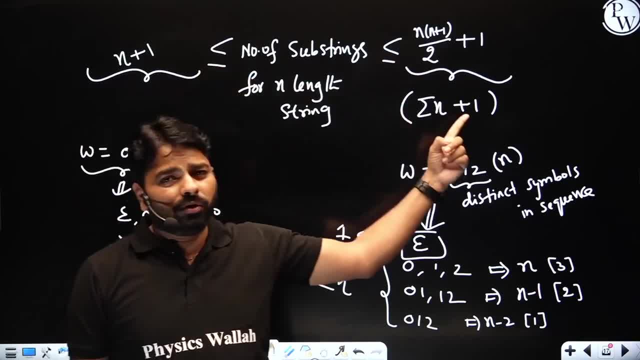 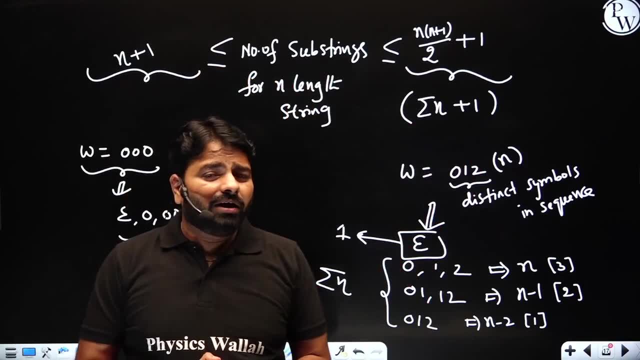 There are special conditions for lower bound and upper bound. If the condition is already given in the question- that number of substrings for the given number of n length string where all the symbols in a string are distinct, Then you just go to this answer. 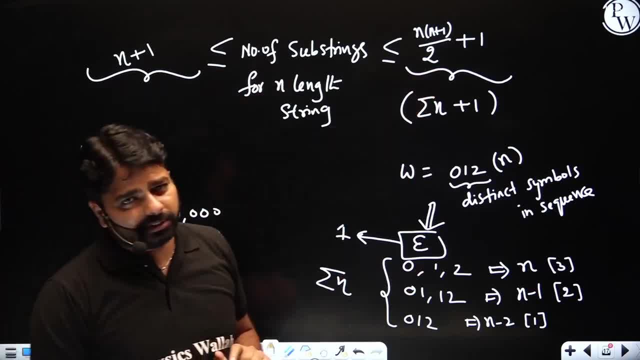 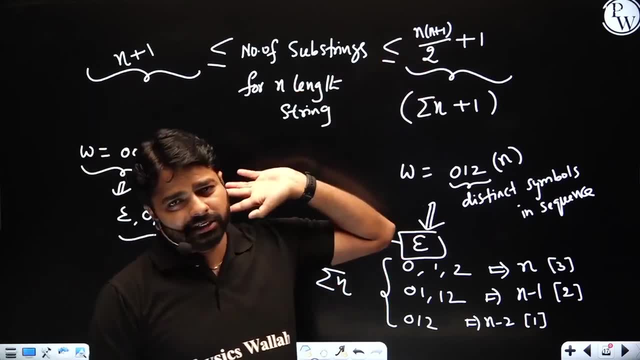 There is one more question. I am asking Number of non-empty substrings. When I ask non-empty substrings, just delete epsilon here, epsilon here. Here you will get n and you will get sigma n. That is it. So plus 1 will not be there when the question is number of non-empty substrings. 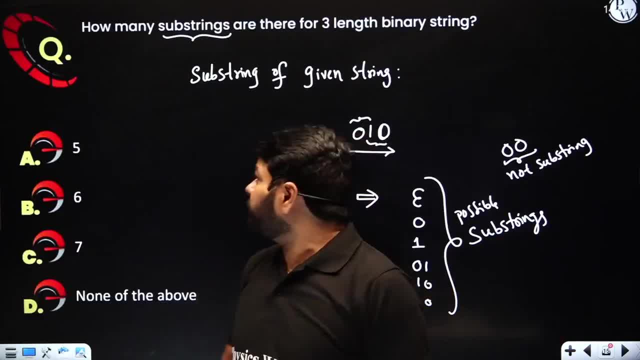 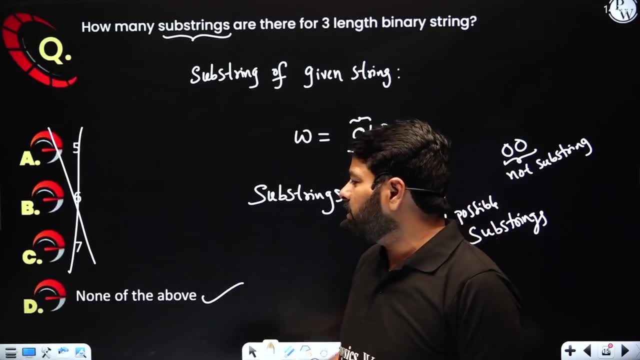 I hope you got a clarity. Let us come to this question. What do you have? How many substrings are there for 3 length binary string? Impossible to answer like this. So you will go for none of this, Because the question has two answers. 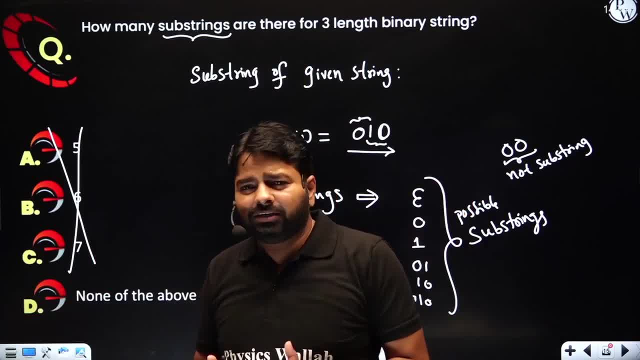 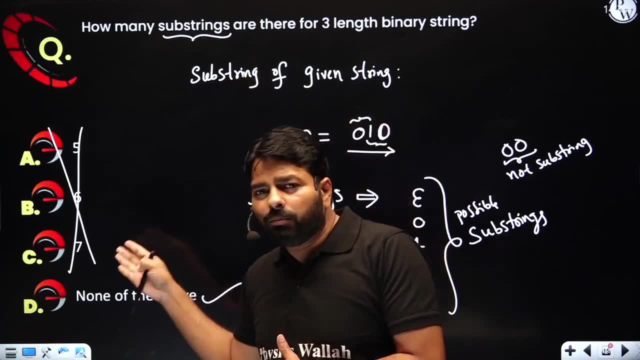 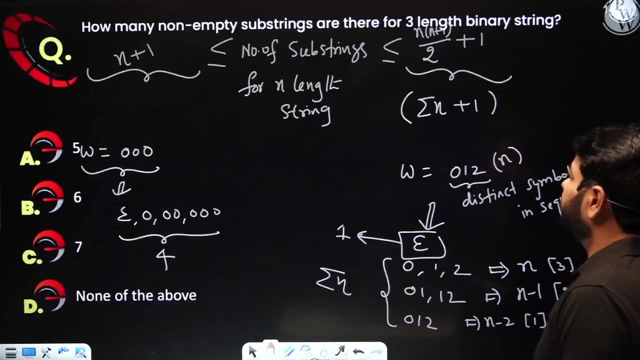 Lower bound and upper bound. The answer could be anywhere in between, Right? That is why you cannot answer uniquely. There is a range, Minimum answer and maximum answer will be there, But not like a particular number for this. Let us move to the another question. 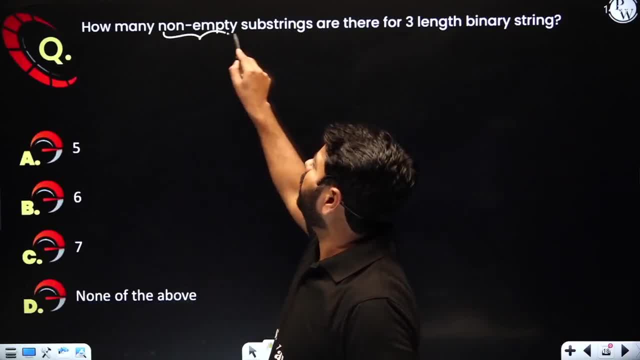 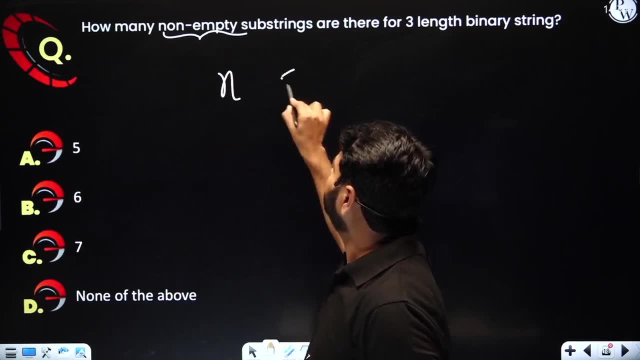 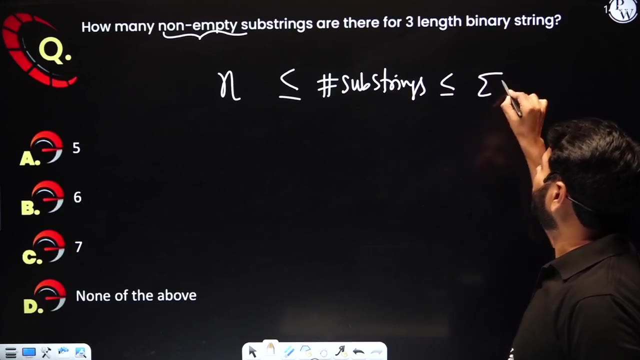 How many non-empty substrings? As usual, non-empty substrings, I just told. minimum, you will have n number of substrings. Maximum, you will have sigma n. So for this question, for 3 length binary string, you will have a 3 minimum. 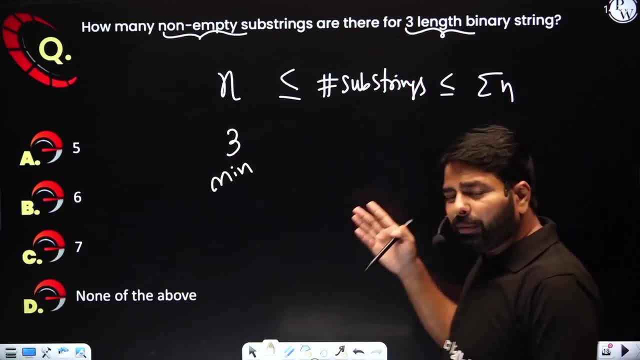 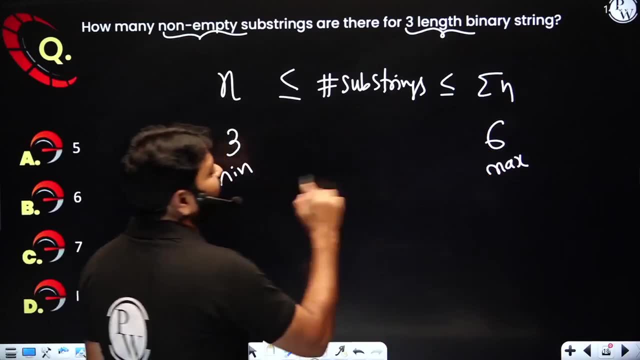 Maximum. that is 3 into 3 plus 1 by 2. That will be 6.. So this is the maximum. The answer should be somewhere in between 3 and 6 in between. That is why this options cannot be correct. 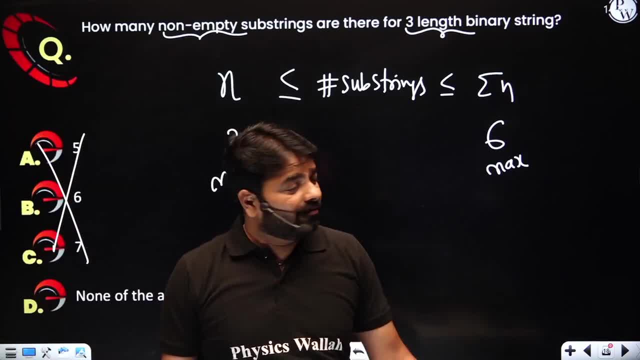 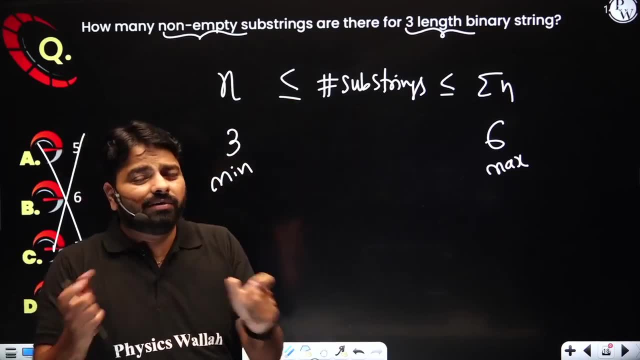 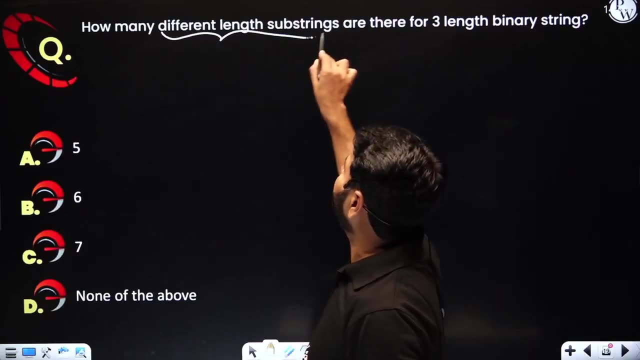 I hope you got a clarity why we answer none of the above. The reason is you cannot answer a unique number for finding number of substrings, as you have the different answers. How many different length? Oh, this is completely different question which was asked in the previous gate. 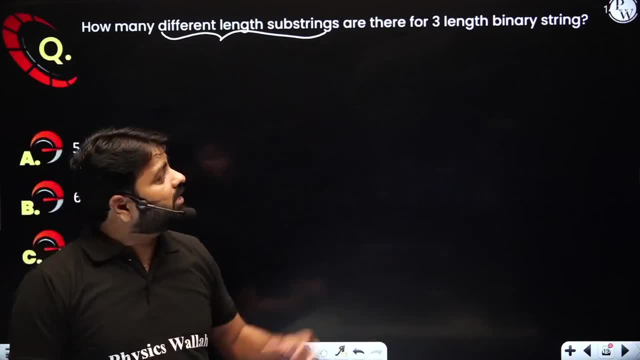 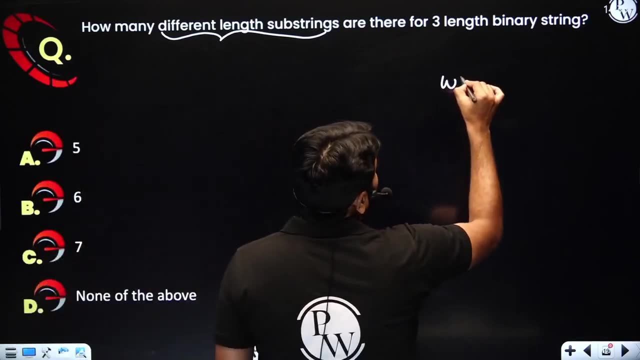 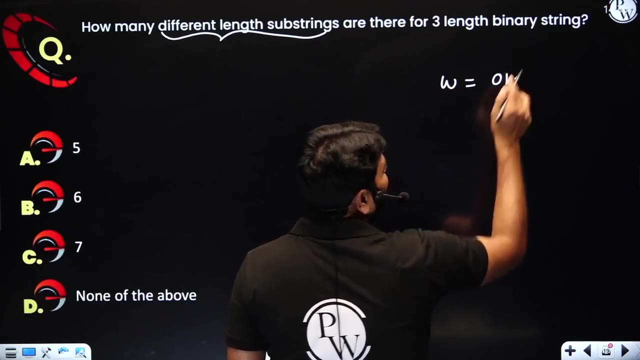 How many different length substrings are there for 3 length binary string? Now, what do you mean by different length? Let me ask the question again. Suppose w is, let me take 0,, 1,, 2.. Of course it is not binary string, right? 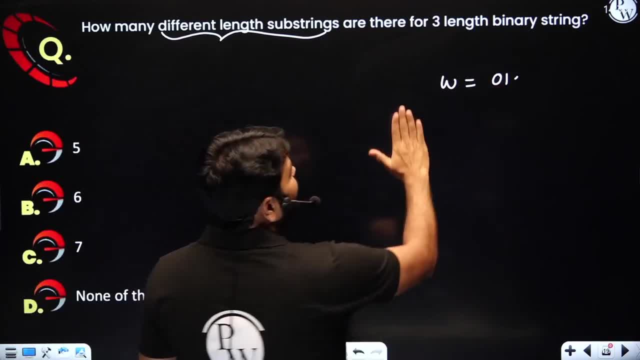 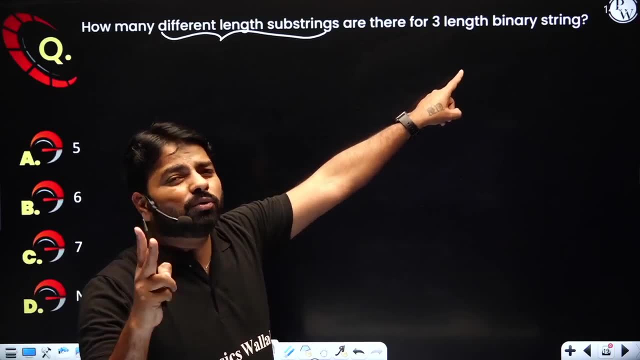 The question is very simple. If you are going for the previous questions, that is, about binary strings, You should be very careful. Binary strings: you have only maximum 2 symbols, Maximum 2 symbols. So this formula could change. Instead of sigma n could change. 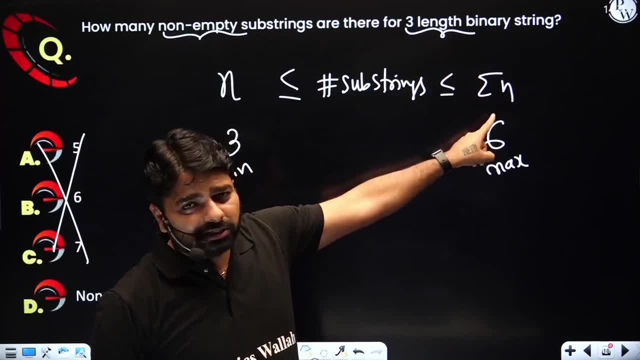 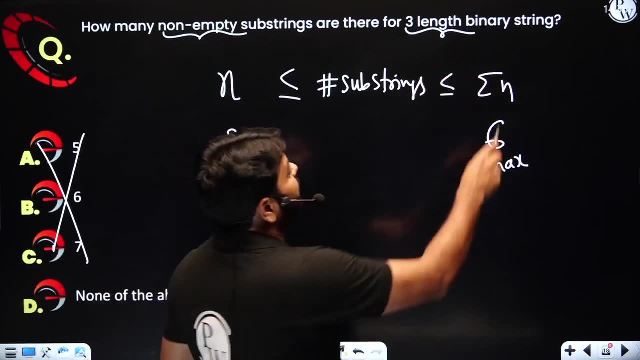 Because I mentioned the binary string. So symbols will repeat. Symbols definitely will repeat. So this is not the maximum answer at all. So in general I have taken 3 length string, But when it is binary the answer will change here. 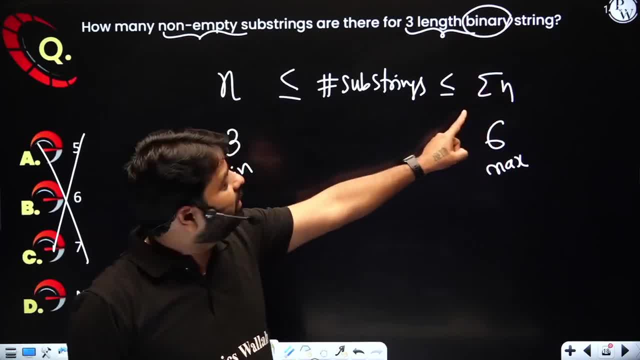 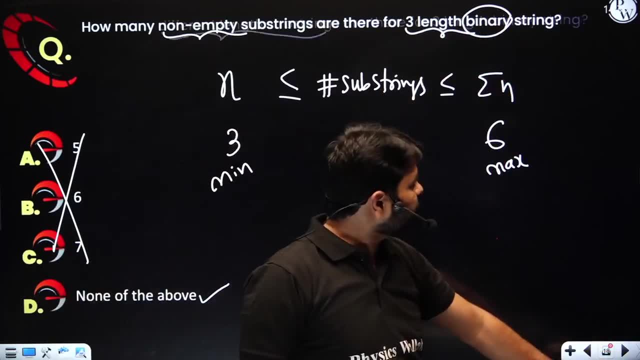 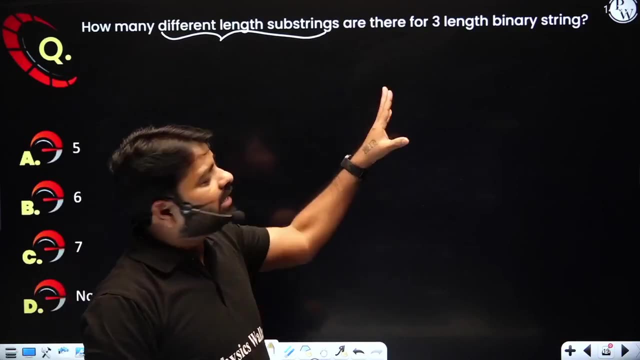 So I want you to calculate it, But be careful. In general, the question will be for 3 length string. I modified to 3 length binary string, So be careful about that formula. Okay now, How many different length substrings are possible for 3 length binary string? 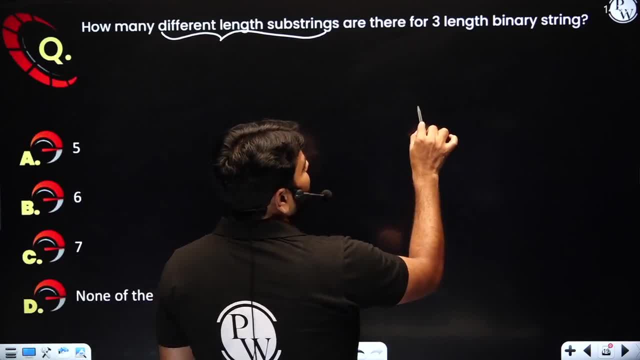 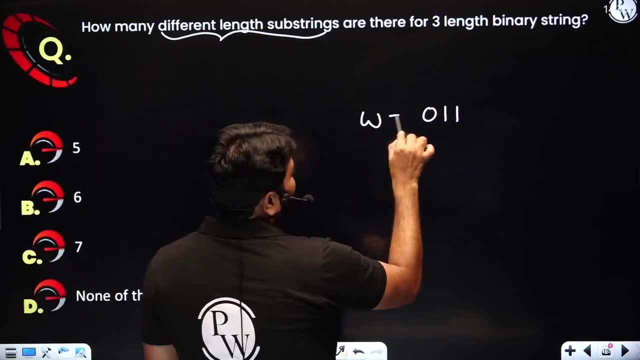 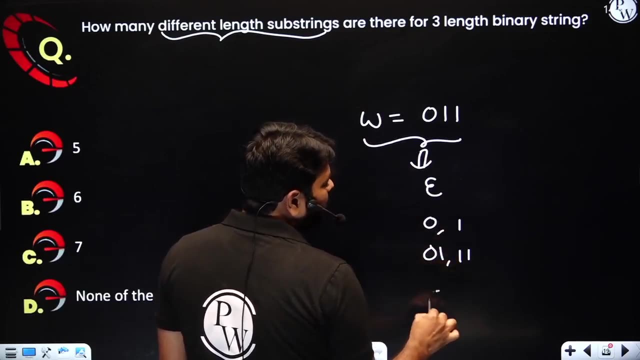 Now let me take 3 length binary string. Okay, So I am just taking 0, 1, 1.. Now, how many different lengths are there? This is w Epsilon: 0, 1 and 0, 1 and double 1 and 0, double 1.. 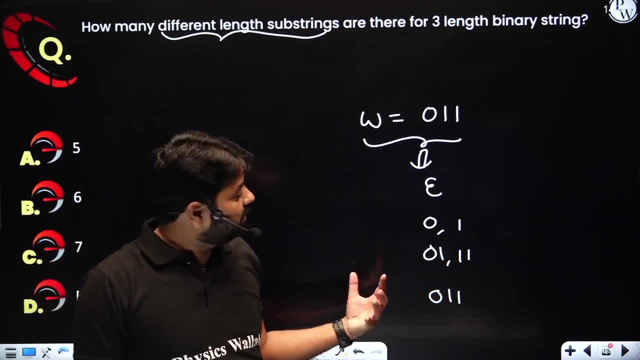 When you are talking about different lengths, I am not talking about different strings. If I ask different strings For this string, you have 7.. 1,, 2,, 3,, 4,, 5, 6.. You have 6 here. 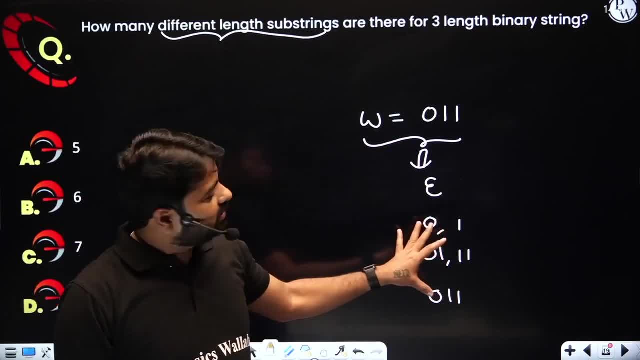 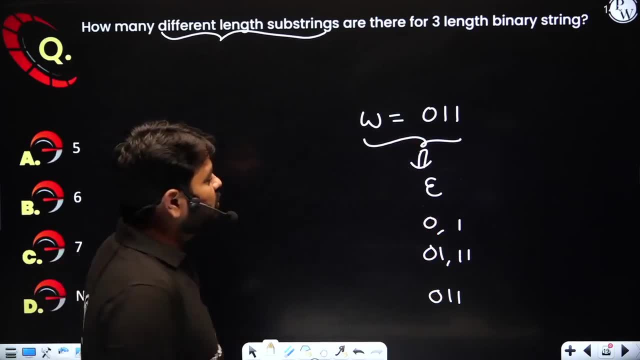 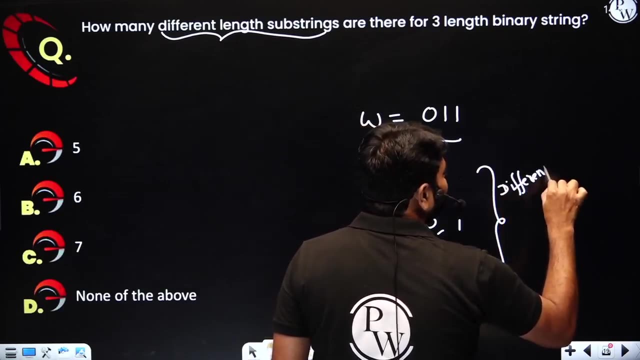 Right For this string. you have 6 substrings, Different lengths. You take any string from 3 lengths you will have different lengths are same Here. how many different lengths. Different lengths, Different lengths, How many different lengths. 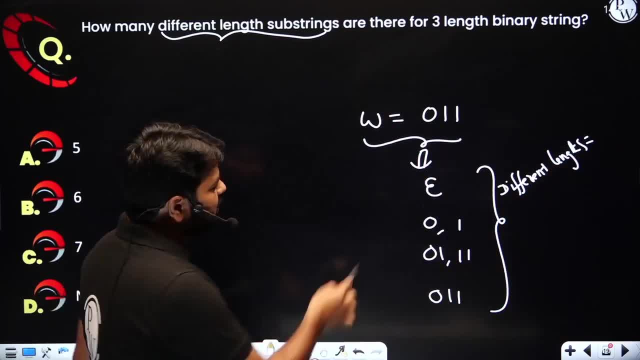 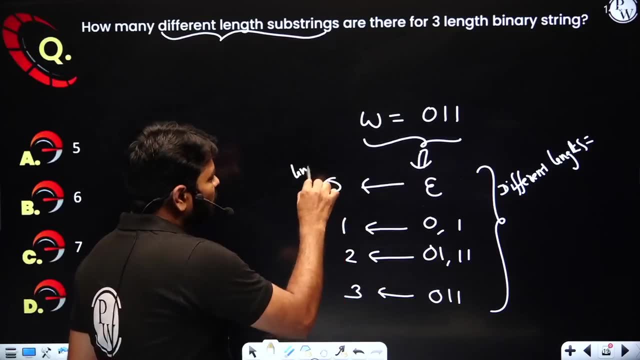 1, 2, 3, 4.. This is 0 length. These are 1 length. These are 2 length. These are 3 length. These are the lengths I am calling Length 0.. Length 1.. 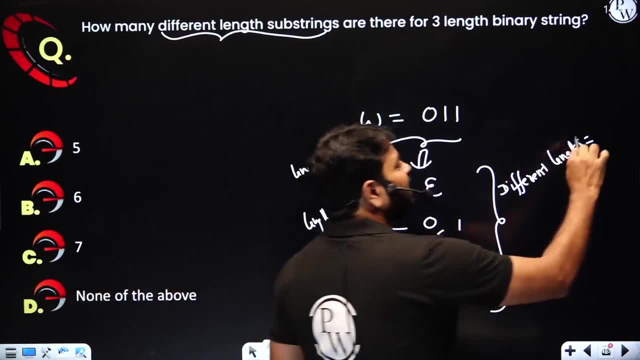 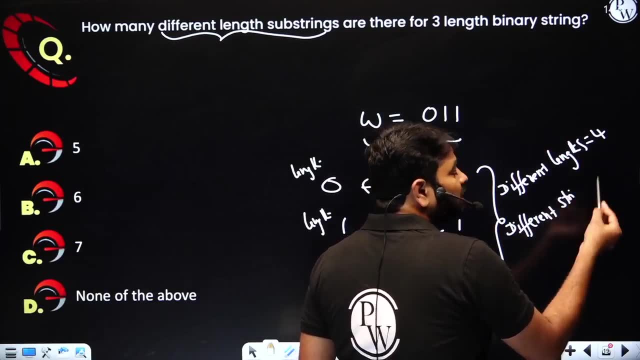 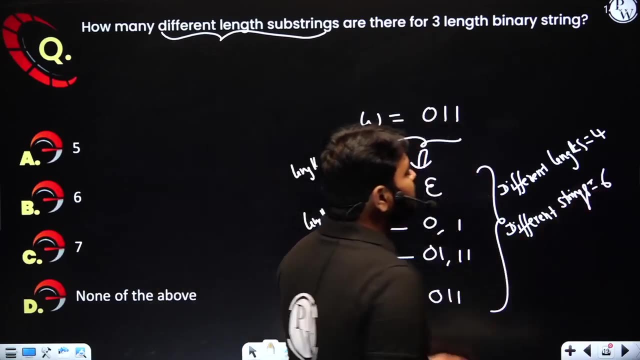 How many different lengths? 4 different lengths. So different lengths are 4.. Different strings: how many? for this Could change: Different string, different substrings: I am calling about Different substrings, How many? 6.. So my question is about different lengths, not number of substrings. 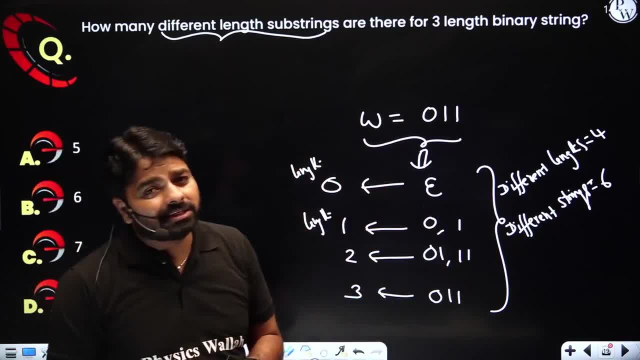 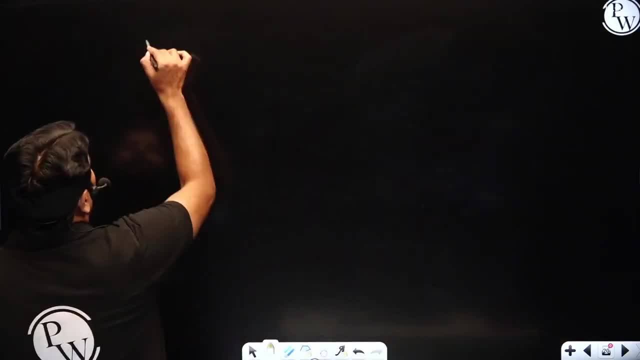 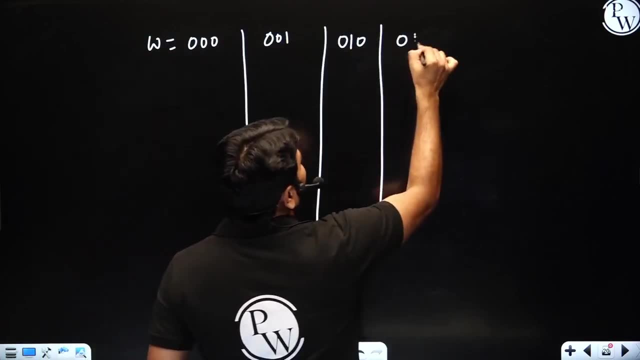 Number of different lengths. So here: number of different lengths or different length substrings, how many are there? 4. Now, my question is very simple. I will just take 000, 001, 010, various different 3 length strings I am taking here. 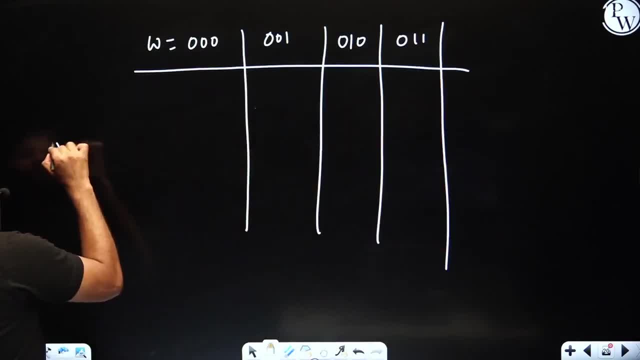 Now find different lengths. Different lengths: how many are there? Different lengths: substrings: Here, how many will be there? 4. Here, how many will be there? 4. Here, how many? But number of substrings may vary. 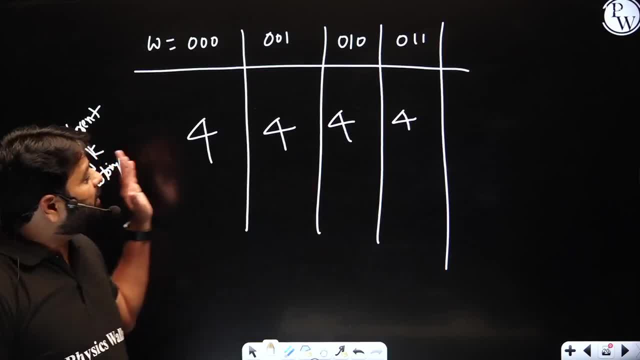 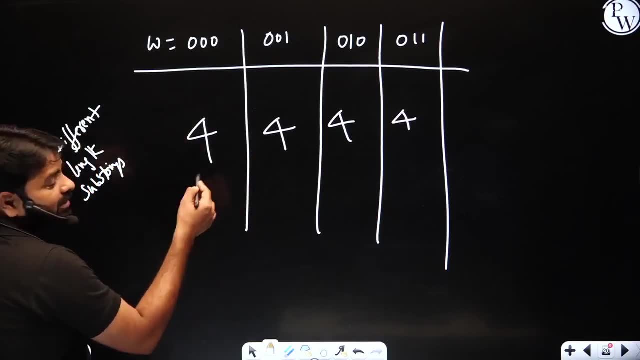 As it is told, number of substrings may vary, But number of different lengths are same for all: 4. only Here 0 length will be, there 1 length. The 4 does not mean that 4 strings. Remember that. 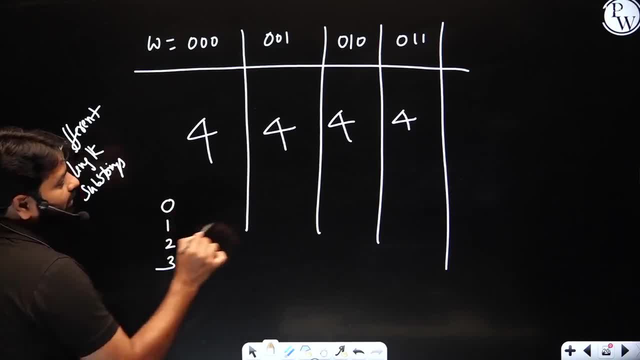 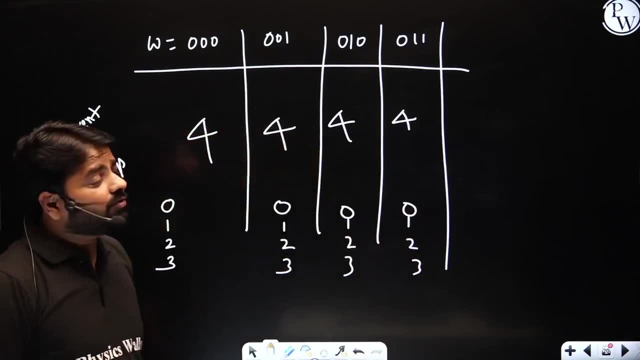 0 length, 1 length, 2 length, 3 length Here: 0 length, 1 length, 2 length, 3 length. Here also, you will have 4 different lengths, are there? That is why you get the answer 4.. 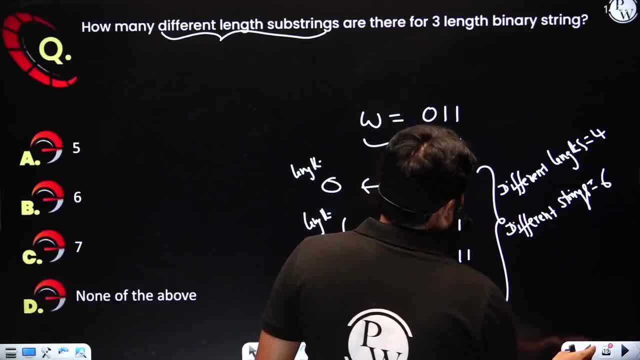 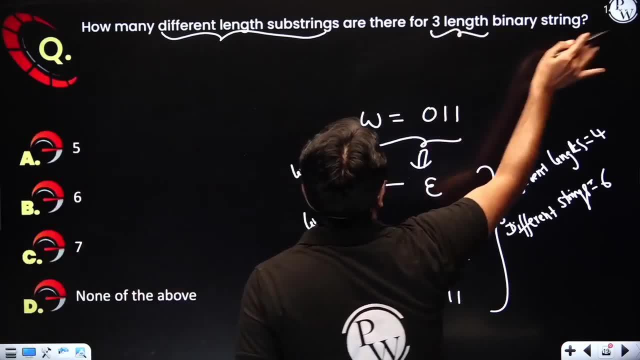 So how do you get the 4?? Just calculating different lengths, substrings. Now you answer it. for the 3 length Does not matter binary string or tanner string, any string, If it is 3 length, how many are there? 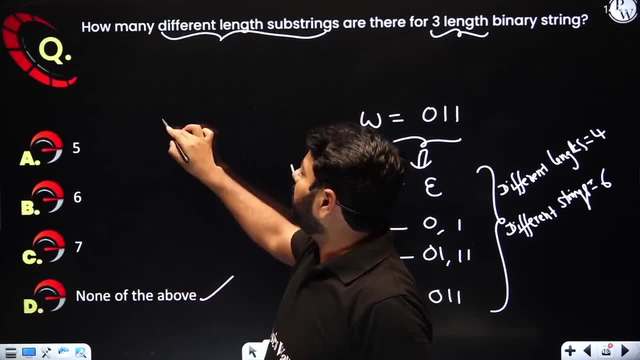 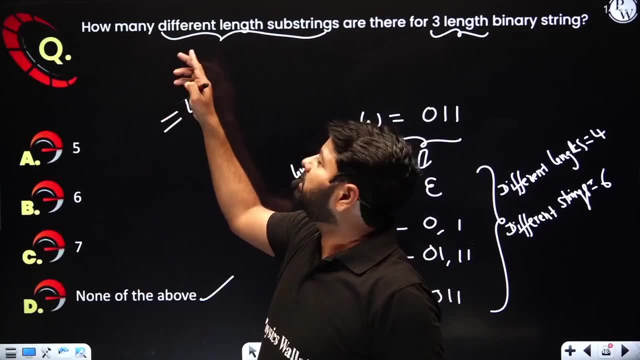 Oh, it is not there here. answer right. So none of the above you go, But answer is here 4.. Now one more question, which was actual gate question: How many non-empty that is other than the 0 length? 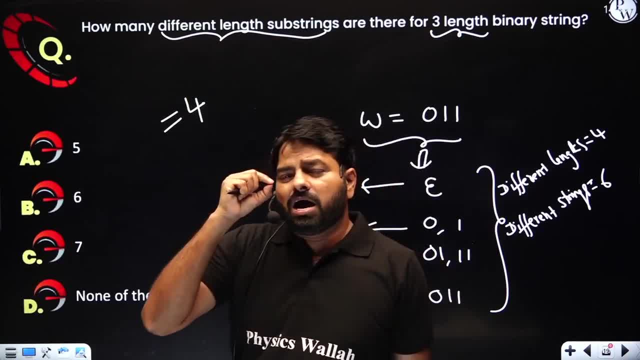 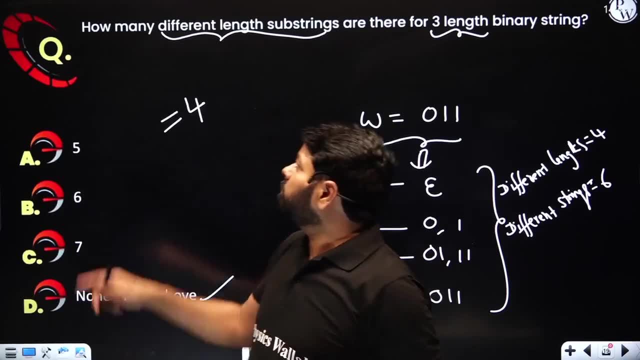 How many different lengths of strings Excluding 0 length? If I exclude 0 length, the answer will be, rather than 4, it will be 3.. That is it. If you include all the lengths, you will have a 4.. 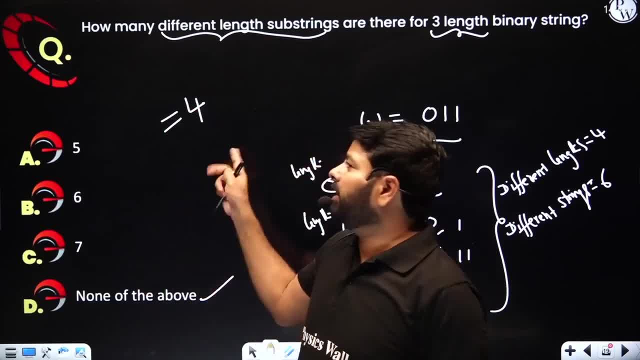 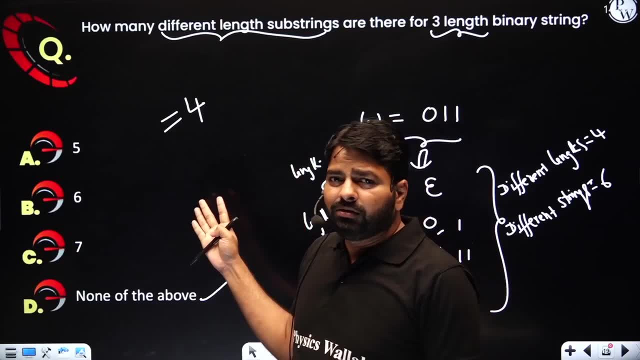 If you include other than the 0 length, you will get a 3.. If you exclude 0 length, you will get a 3.. If you include 0 length, you will get a 4.. This is one of the famous gate question which was asked. 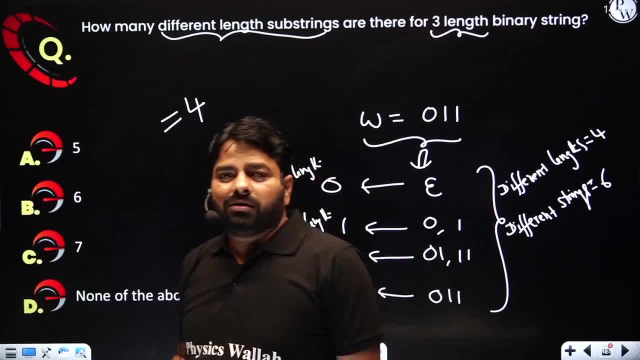 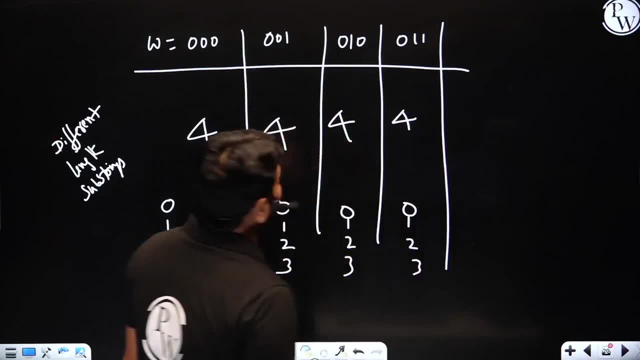 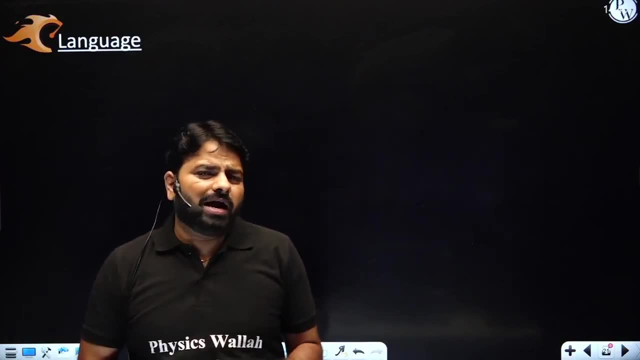 But that is not for the binary. That is, in general, string that could have any sequence of symbols. Fine, Now we will move to the language. So far I have explained what is a string, what are the operations of a string. 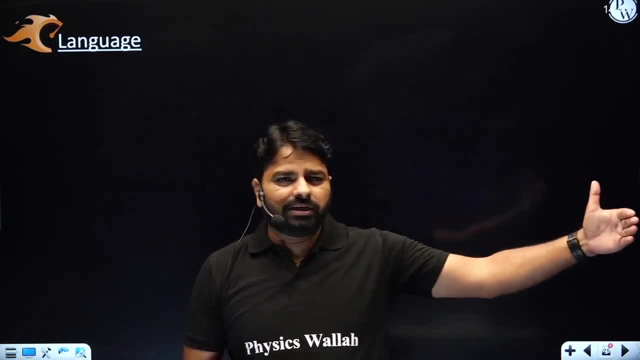 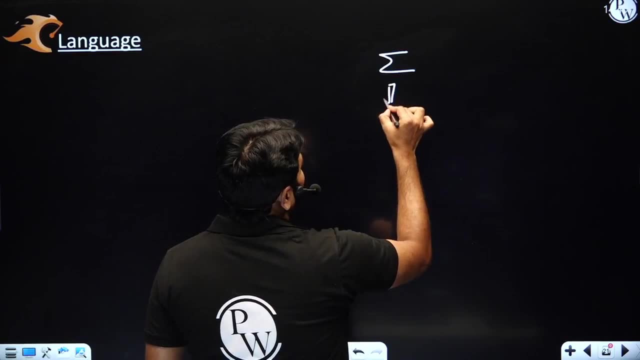 Now let us come to the language. You have an alphabet, then you have a string, then we will have a language. So, as I told, without a sigma, you cannot form a string. Without a string, forming a language is difficult. 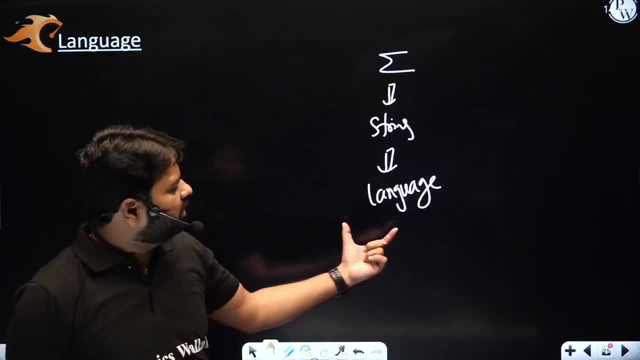 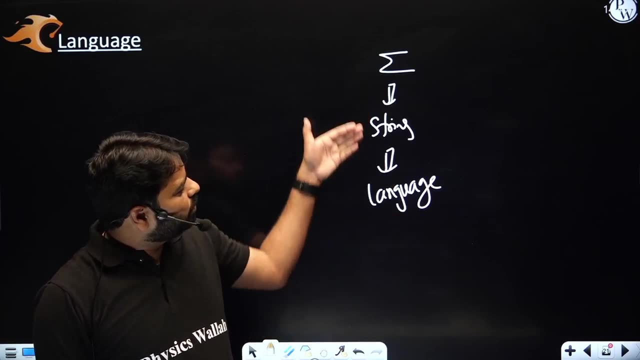 Then why do you want this language To specify or to represent the problems, All the problems we denote or represent with the languages? That is why you need to know the sequence. The sigma has a symbols. Using those symbols, you will form the strings. 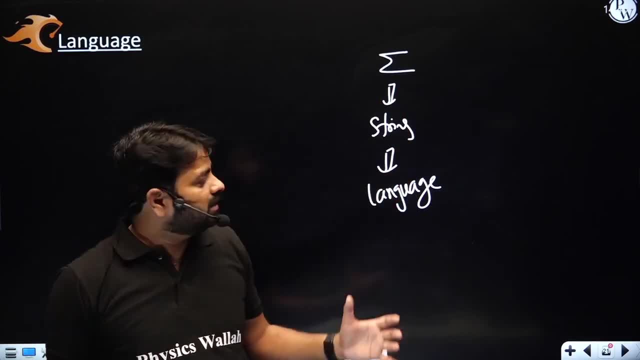 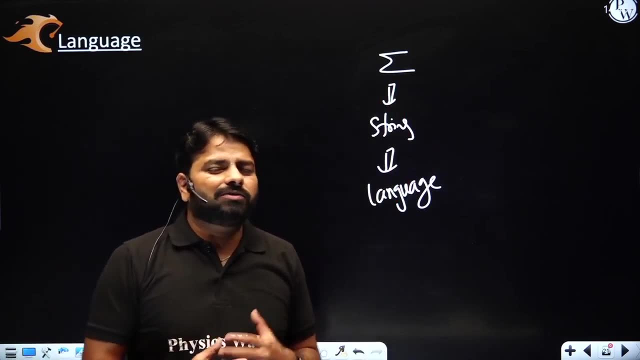 Using those strings you will form a language. So if I have the certain set of the strings in the language, you can represent a problem Like I want, a problem where I want to solve the length is divisible by 2. Then I will represent to the language. 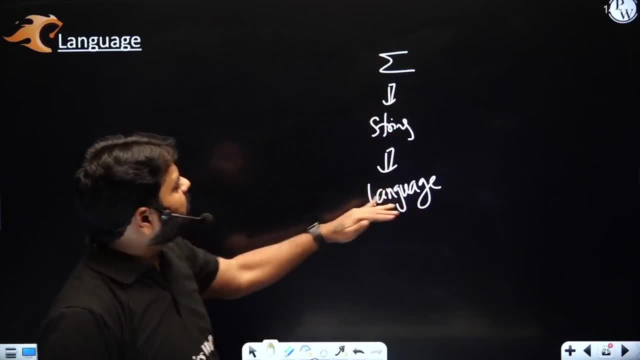 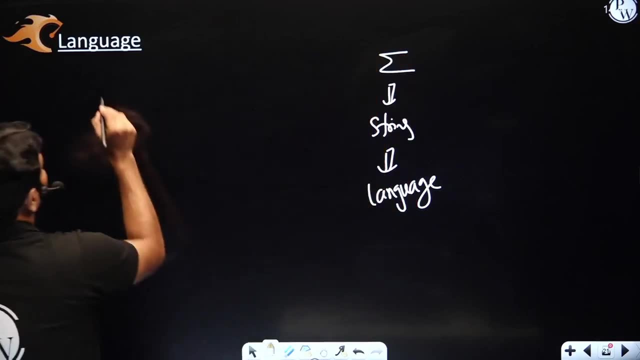 So we will get to know slowly. Now let us come to the language. What is a language? You see that language is a collection of the strings defined over the sigma. What is a language? It is a collection of the strings. 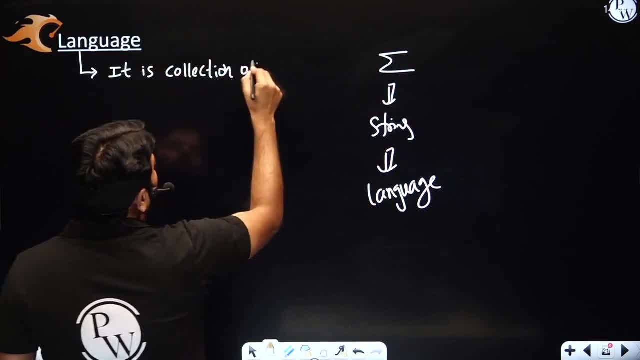 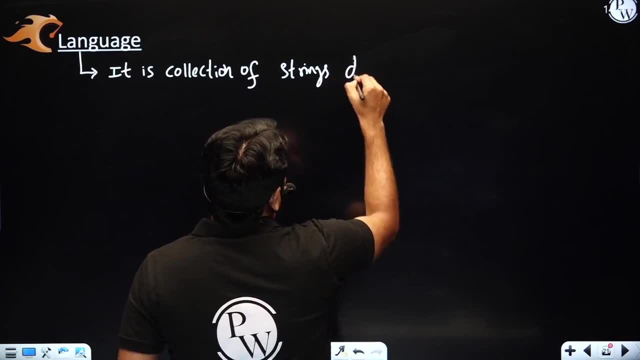 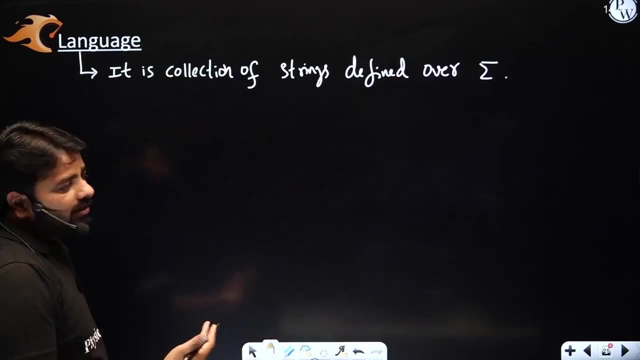 What are the strings? you have understood. You collect all those strings. Collection of the strings defined over the sigma. Sigma, here, alphabet. Now, what kind of languages you can form. Let us see: My sigma is a, b, The strings: how many strings are there? 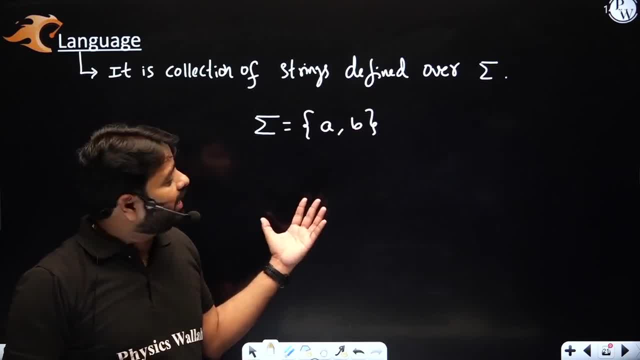 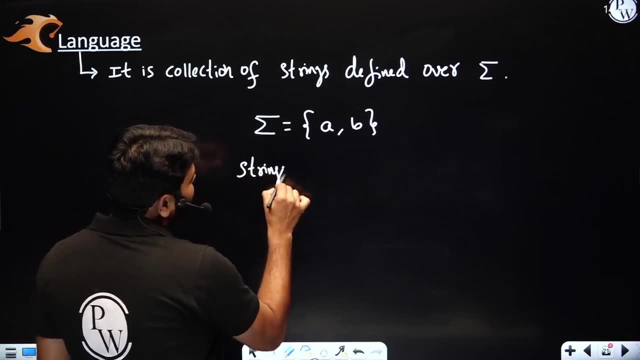 If you ask me how many strings, I cannot say 10, 100, 1000.. Infinite strings are there. Can you write some of them here? Yes, What are the strings are possible here? Strings Epsilon a, b, 2 length, 3 length, so on, right. 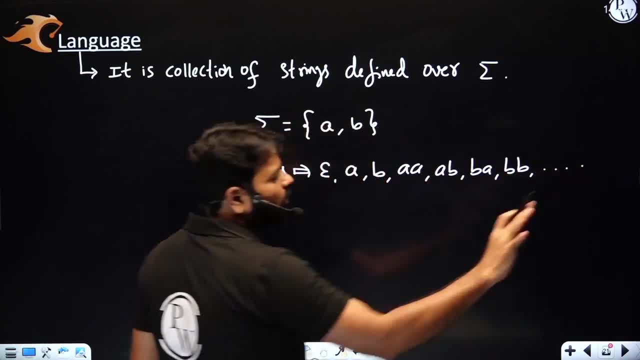 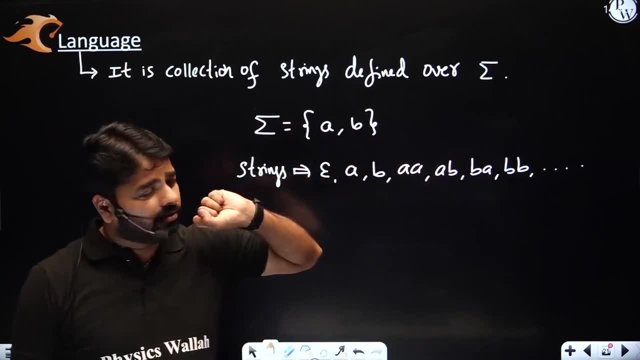 You keep on writing, you will never end up, But you cannot write all the strings. You cannot write all the strings in a sequence till infinite. These are the strings. There are infinite number of strings possible, But every string that you write has to be finite. 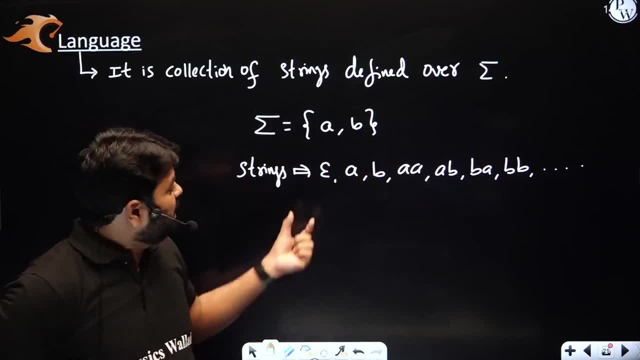 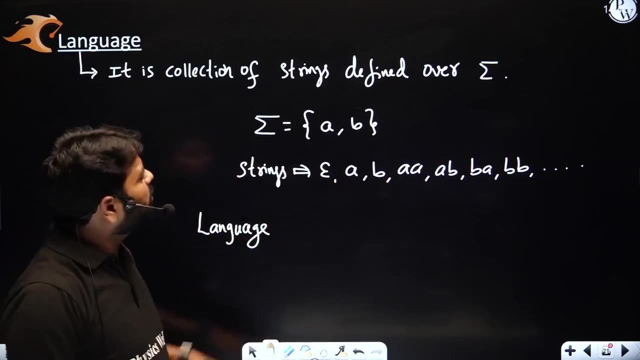 This is a very important terminology. in theory of computation, Every string should be finite, But such finite strings can be infinite. Remember that point. Now, what is the language? So many languages are possible over this sigma. What are those languages you can write? 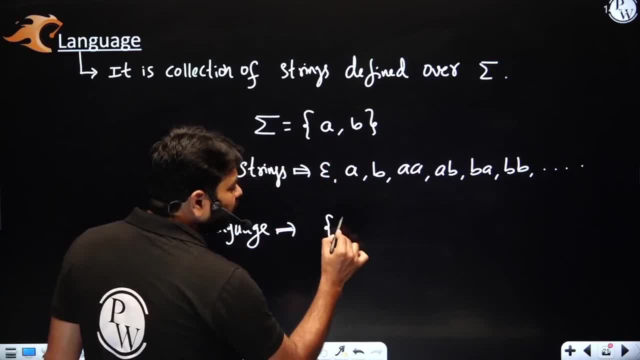 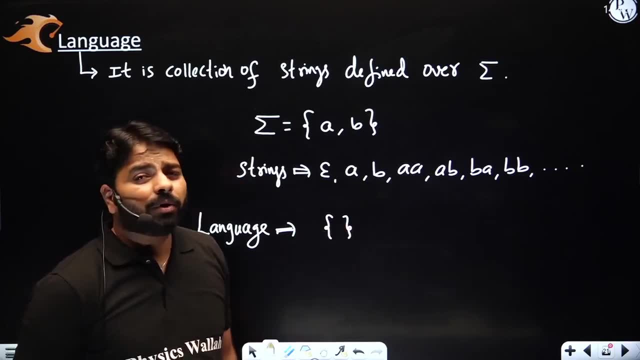 Here the one language could be empty language. What is this language? Speciality of this language is: I do not have any string to represent in my language. My problem specifies: I do not want anybody to present in the language. Then this is called as empty language. 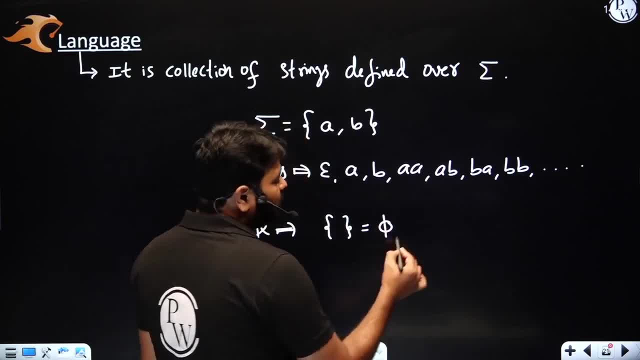 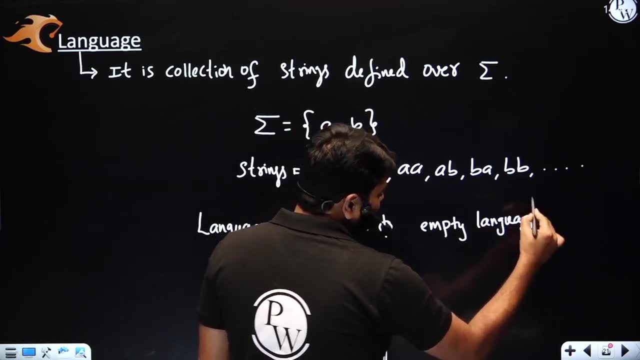 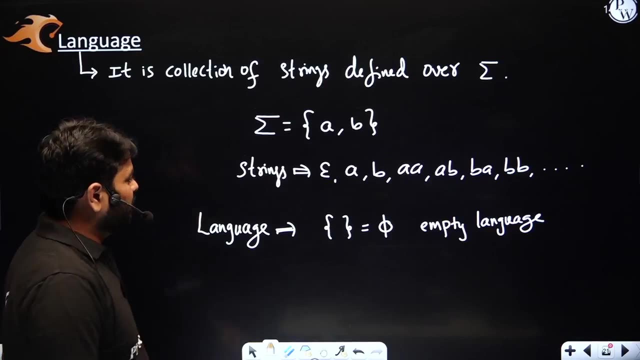 You may represent with empty set the pi. This is called as empty set or empty language. Represent there is no string present. Even epsilon is also not present in this set. Always, we represent the set with the curly brackets. Now, is there any other language? 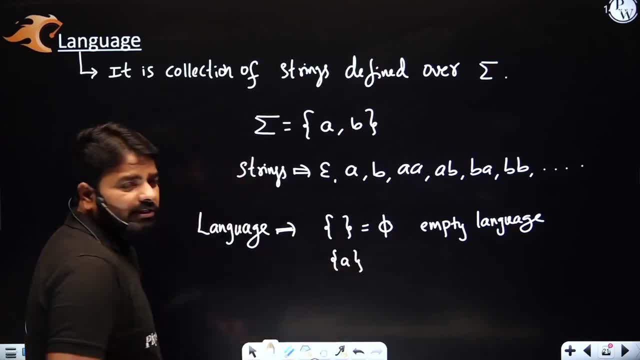 Yes, I may have only a singleton language. It is called as what? Singleton, where only one string present. I may have even epsilon. Oh, that is good, It is also singleton language. I may have only b. I may have only double a. 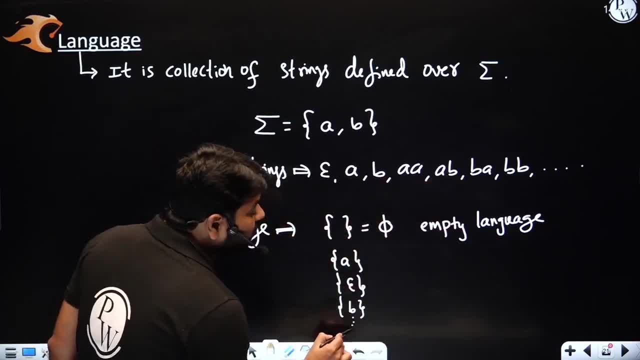 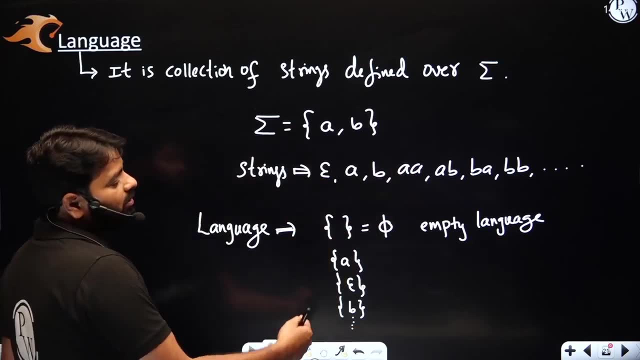 I may have only a, b. Such singleton languages are infinite. It is not 1,, 2,, 3.. You can write: this is only the string in the language. So let me mention some of the strings here. First, I have mentioned empty. 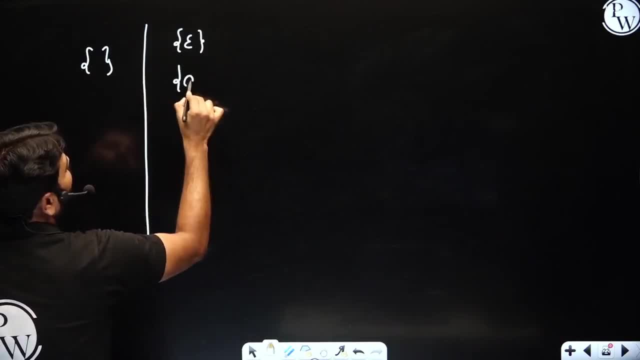 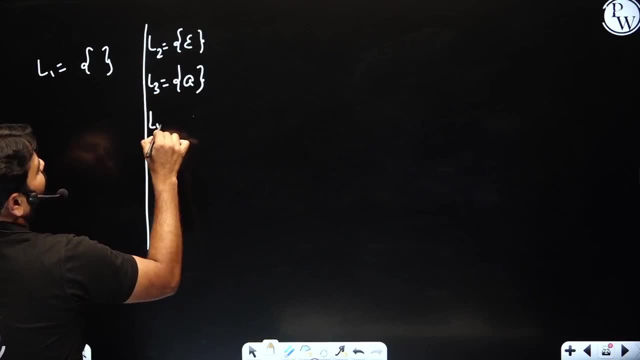 And then epsilon. These are all languages. You can mention L1.. This can be L2.. This can be L3, and so on, L4, V And L5, let us say double a, L6, a b. 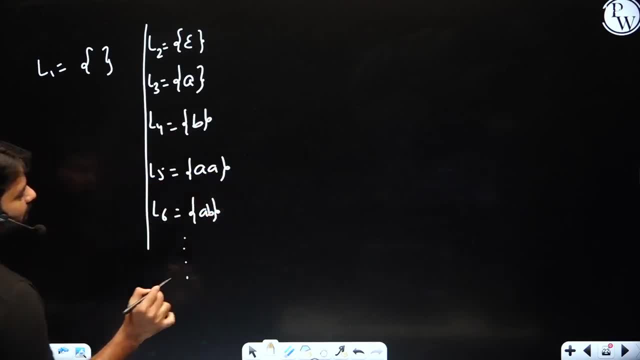 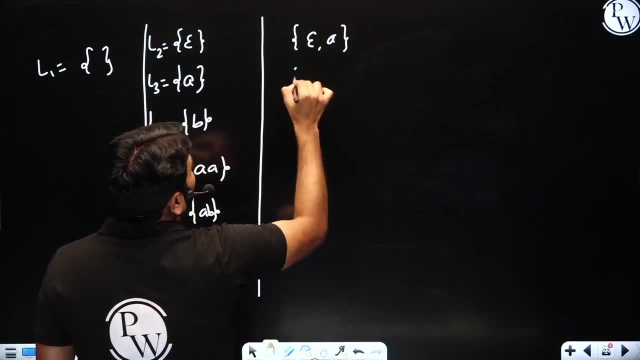 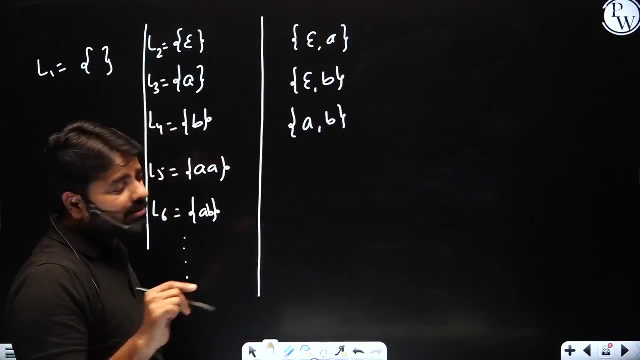 These are singleton languages, So many are there. Now I am going to write the languages which is going to have two strings, Like epsilon a or epsilon b or a- b. Oh, it looks like alphabet, but that is also a language, because that is a set. 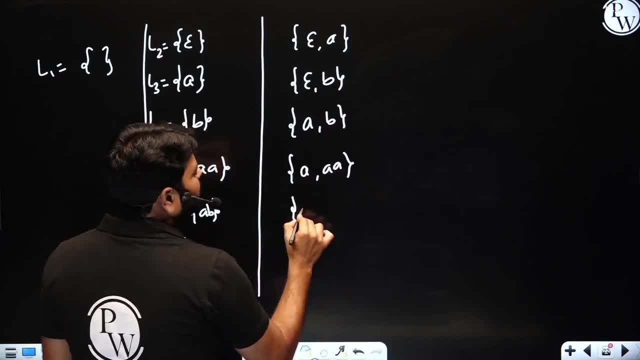 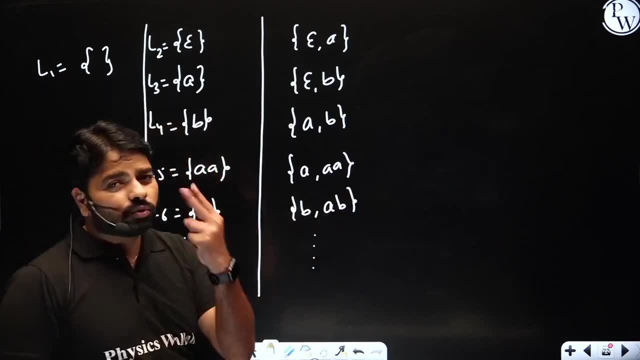 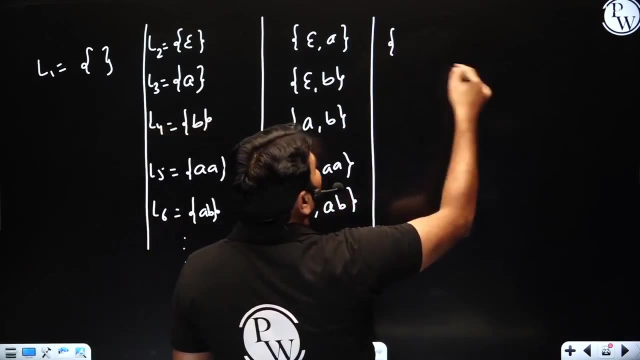 And a double a. Likewise, how many you can write? So many, right? So many infinite languages. you can write with two strings. What else you have? You can write 3 length, 4 length, 5 length. You can represent when you have more strings, right? 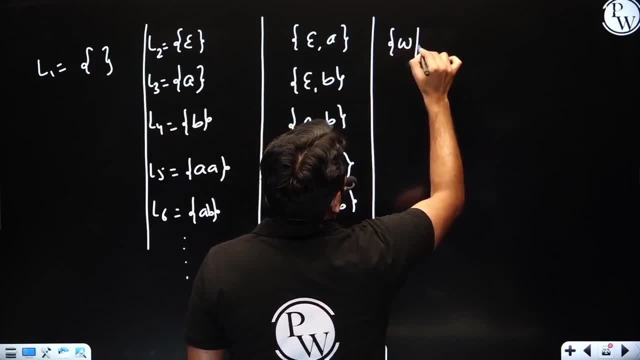 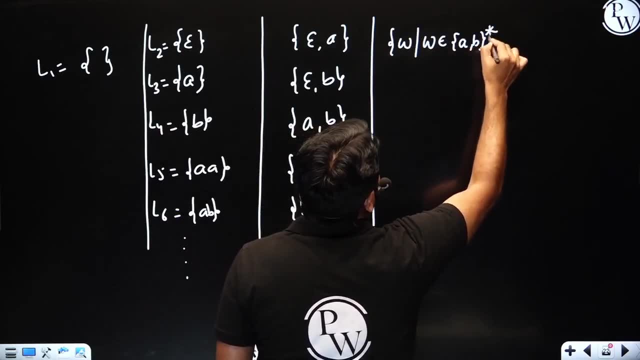 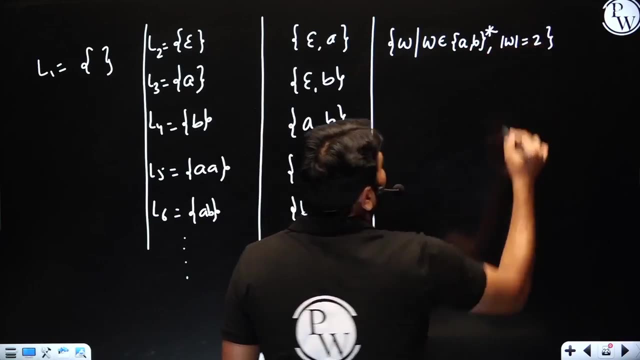 You can represent like I have a, w, such that the w belongs to a very special notation: a, b, whole star. Okay, that is not important right now, But I am just mentioning it. What is the meaning of this? Before this, I have mentioned something like a, b, whole star. 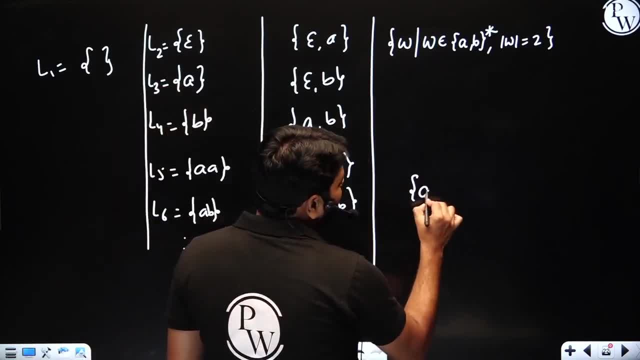 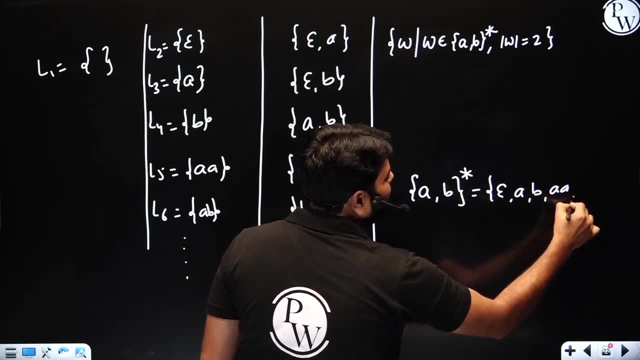 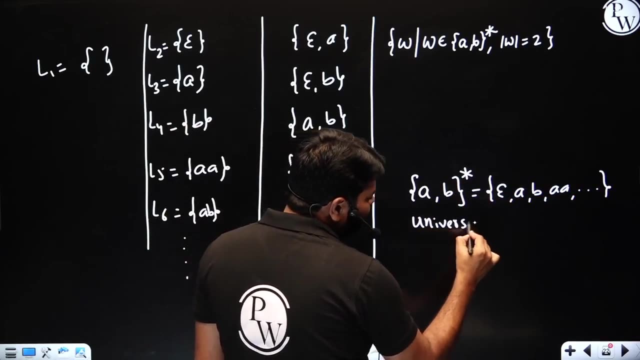 Here in this languages, the a- b whole star represent all the strings that you have, Like epsilon: a, b, double a, Every string present that is called as, basically, universal set. What is it Universal set, You may ask, sir? why do you represent this way? 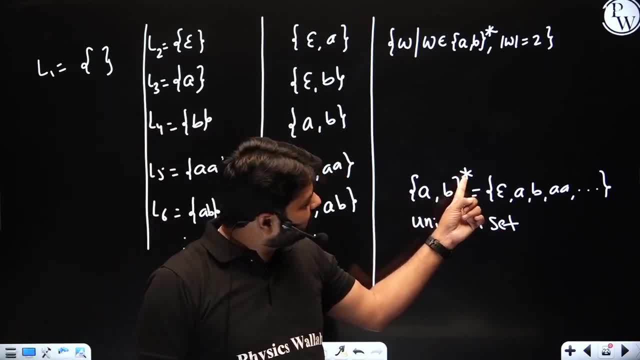 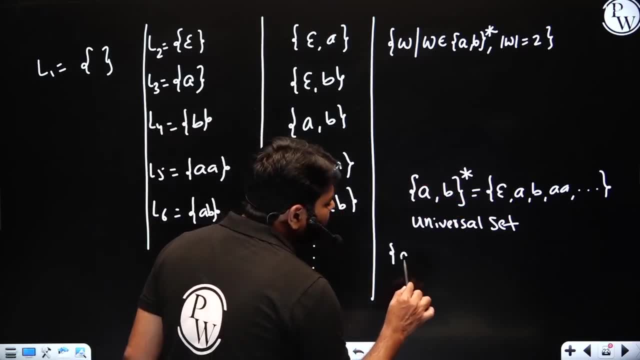 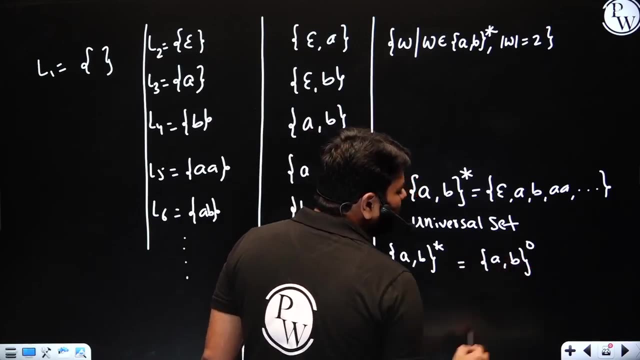 Because this set can be repetitive any number of times. It can be repetitive any number of times with the help of star. This star is basically called as clinic closure. You may ask, sir, how do you generate all the strings, This: a, b, whole star. it means a, b, power, 0 or union. you can say: 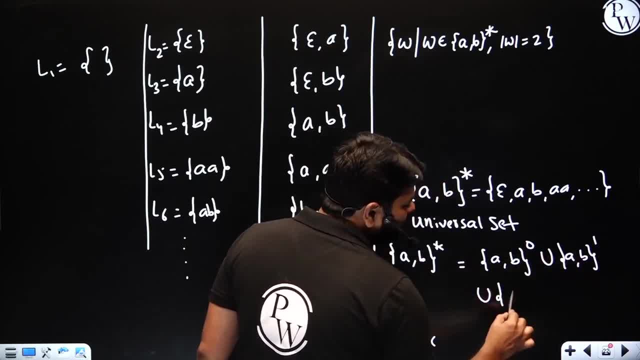 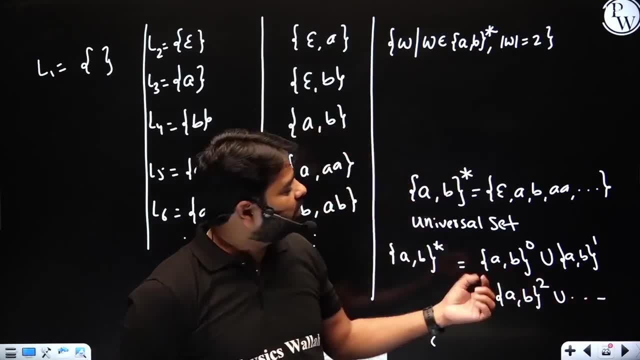 a- b power 1. union a- b power 2.. Which is going to give you all the length strings. Like a- b power 0 means take 0. length string Means epsilon: a- b power 1 means a- b only. 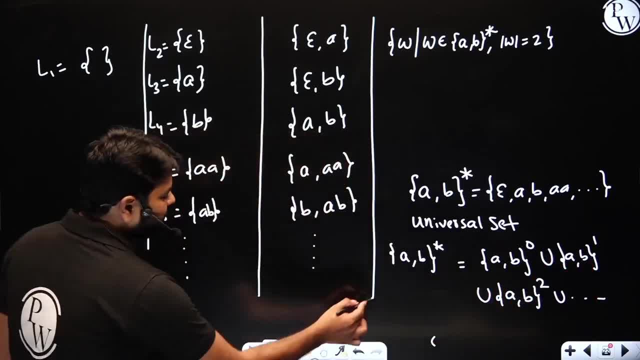 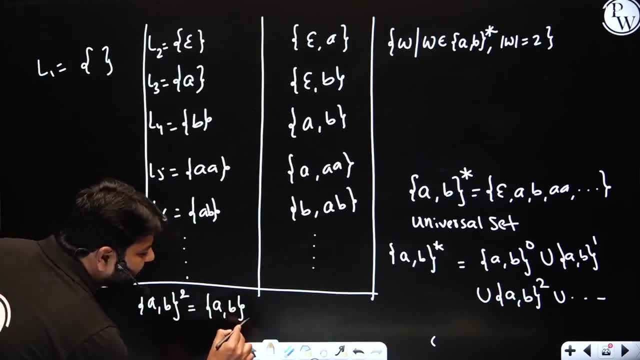 When you write a b power 2, you will have a different meaning here. So let me explain here: a b power 2 means repetitive Two times. you repeat with the concatenation Which gives you all the two length strings. 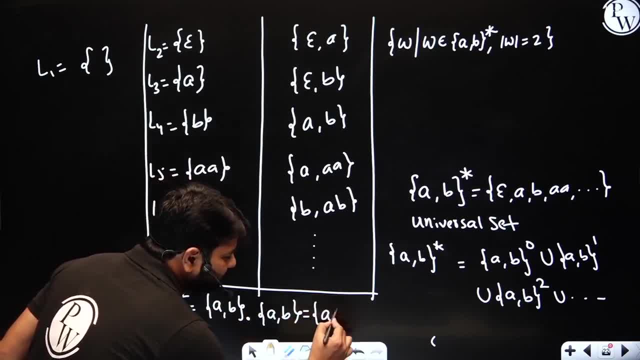 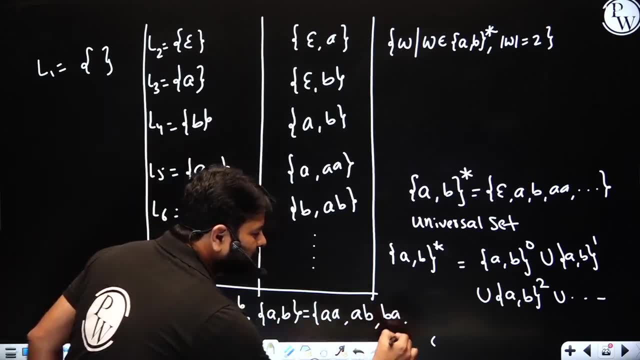 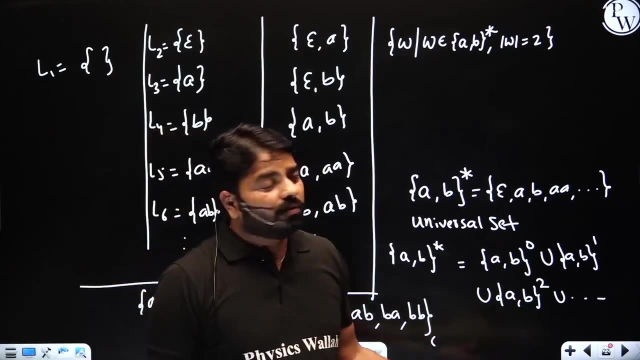 See that a dot a, Which is going to give double a, a dot b, b dot a, b a And b dot b, which is bb. This is how you get all the strings which are present over a b. Here all strings are present. 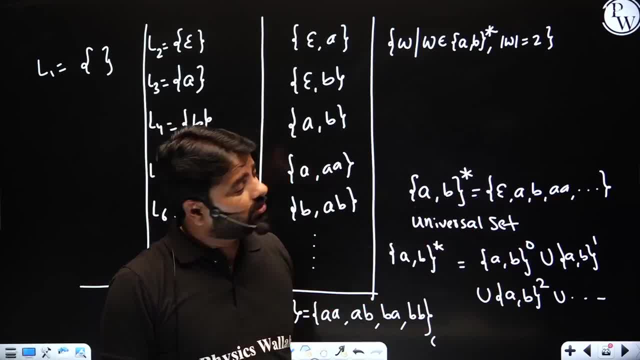 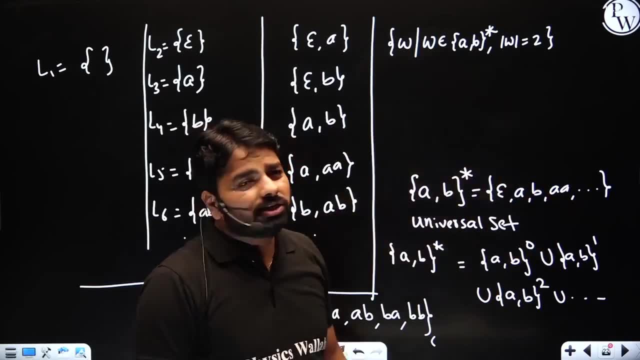 This set is called as universal set, also called as universal language. Now, what is the meaning of this? w belongs to a, b whole star means w is any string over a, b. Instead of saying w is anything we are writing. w belongs to a, b whole star. 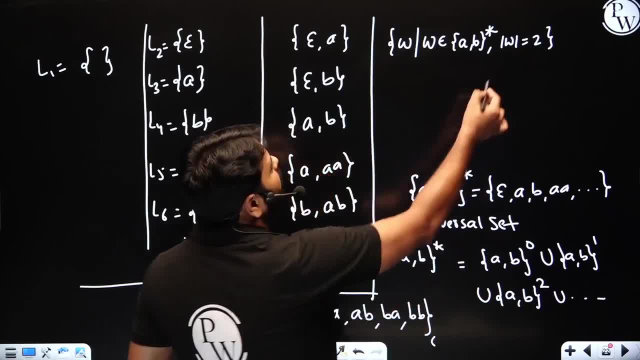 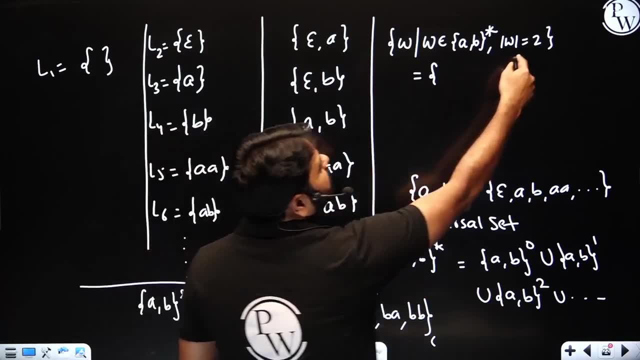 What is the meaning of this set notation? All the two length strings I require, which is exactly same as what I have written here: a, a, a, b, b, a, b b, Because I want two length only. So a a, a, b, b, a, b b. 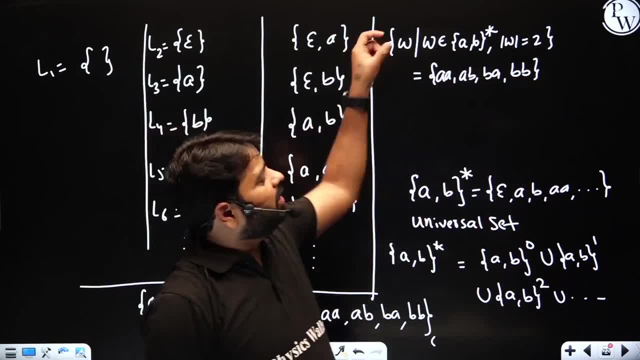 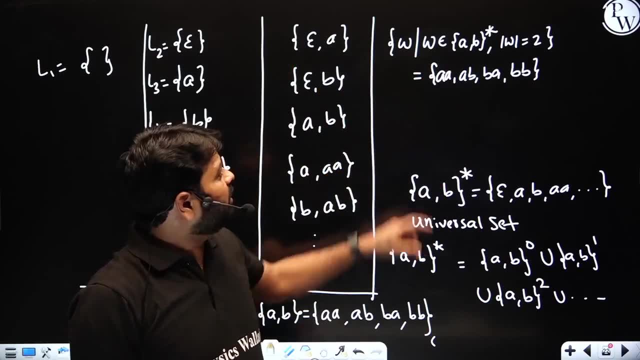 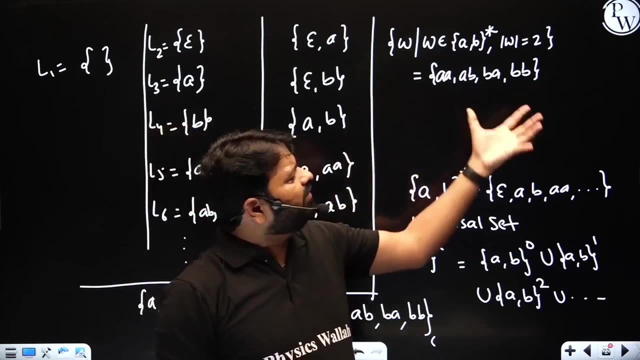 That's it. This notation I have taken from the set theory. Where set theory, you have set builder or set roaster, notation that can be used to form the strings or elements of the set Element is nothing but a string. There are various ways to denote the set. 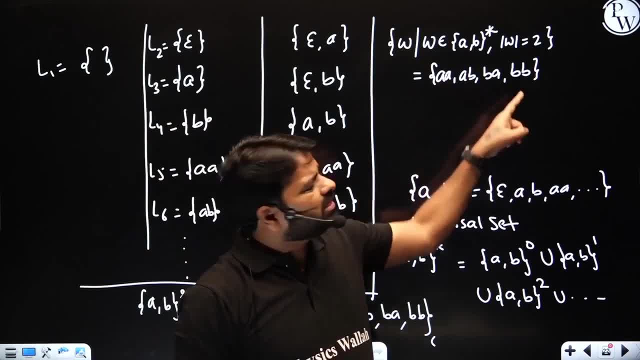 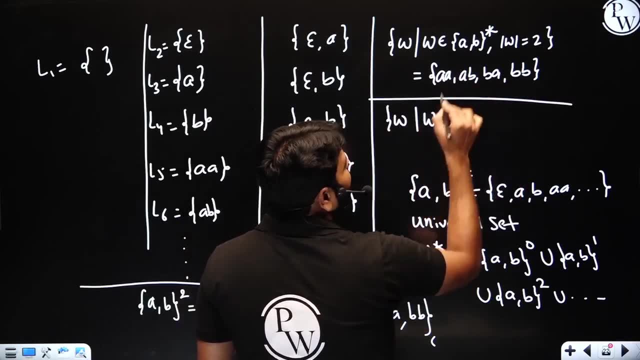 So I have used one way to denote Why I am using it, Because writing all these strings are very difficult. If I suppose length of w such that w is any string over a, b which is easy to write, Length of w is 100.. 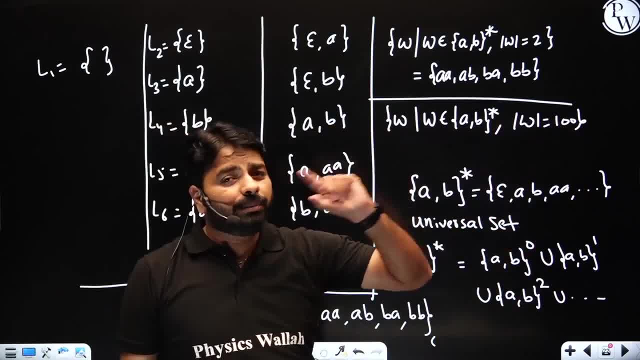 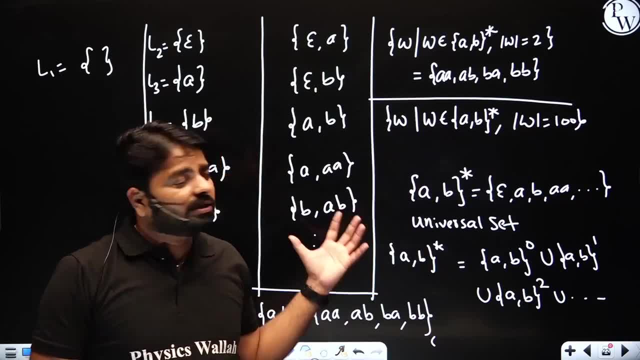 Can you write all the 100 length strings? Very, very difficult, But this notation will help you to denote. this language has all the 100 length strings But in case, if you want to write, maybe this board or this slide is not sufficient to write all the 100 length strings. 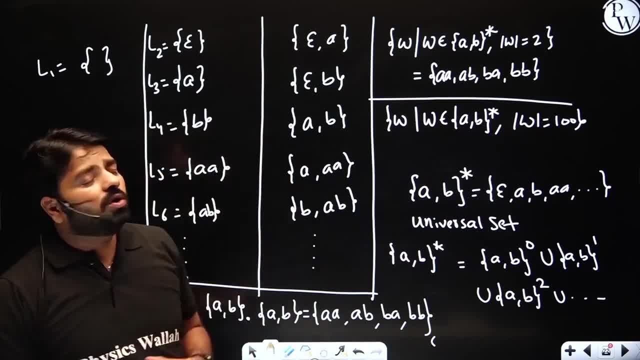 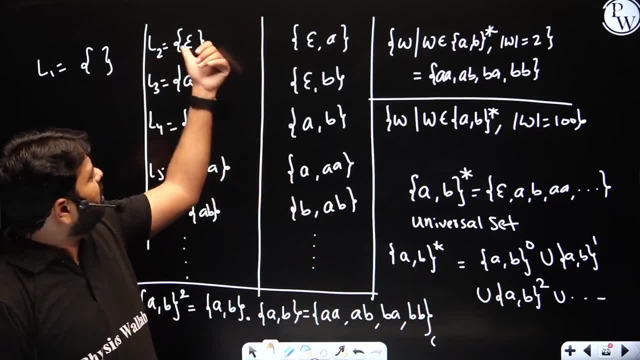 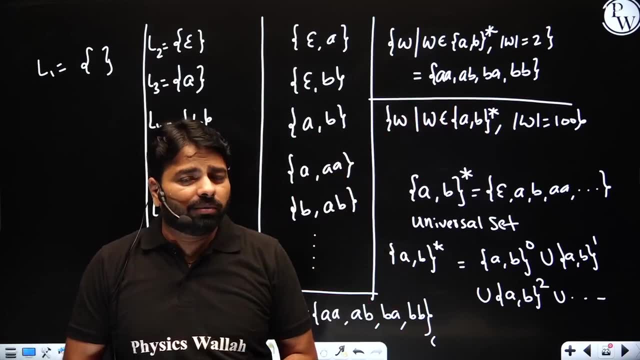 That is the beauty of this set notation. I hope you understood what is a language. Language is a collection of the strings. That strings may not present or may present only one, or may present only two strings or may present any number of strings. The language may present any number of strings. 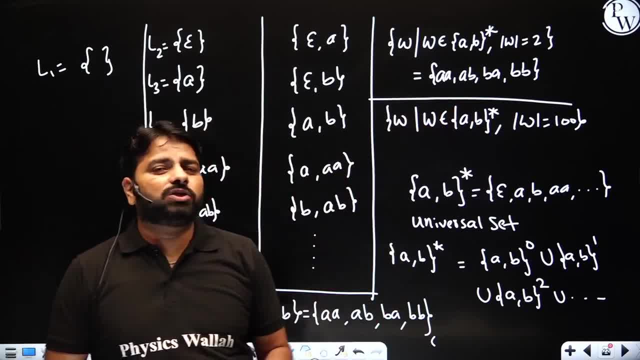 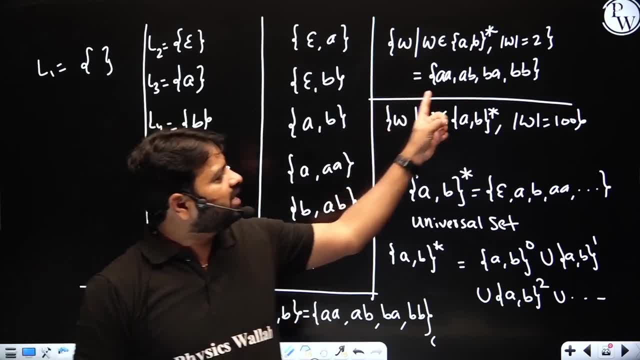 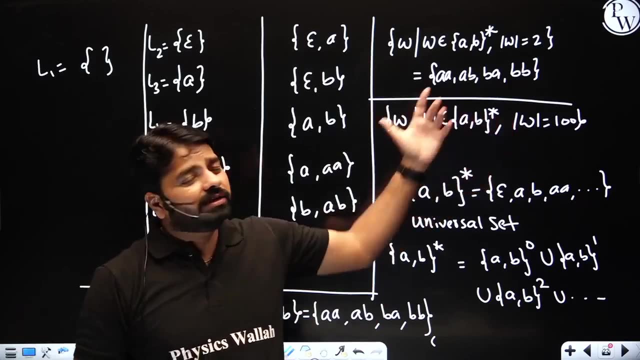 Based on this, I can tell you the language is two types. One is the finite language, Other one is infinite language. What do you mean by finite language? When the number of strings are finite, then the language is finite. If the number of strings in the language are infinite, then language is infinite. 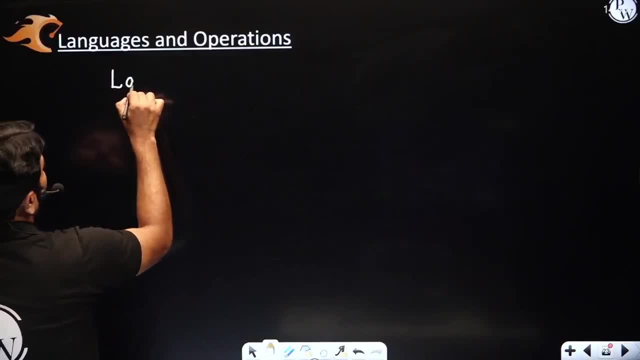 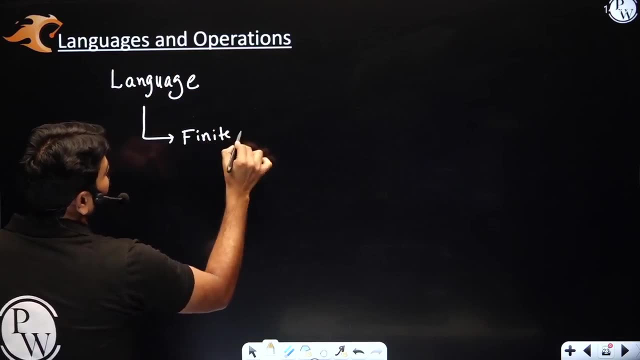 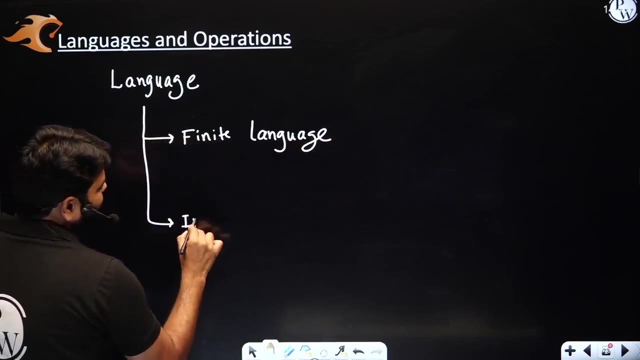 Let me just mention it. The language that I have defined so far is two types. One is the finite language, also called as finite set. Another one is infinite language. Very simple, We always use a finite string, but language can be two types. 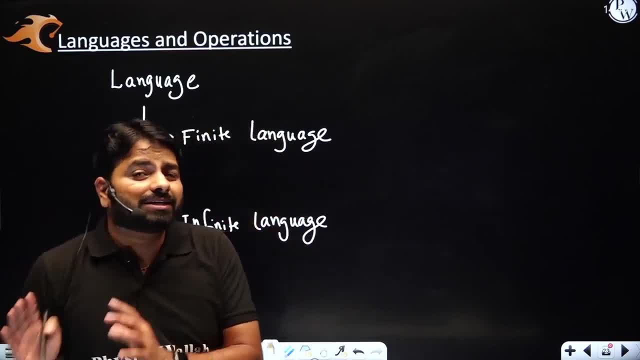 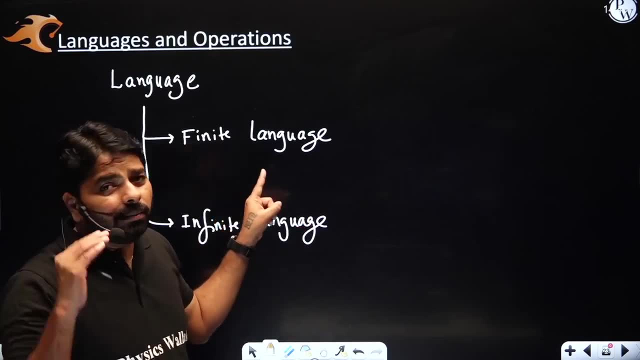 Remember this point: We can use only finite string. String has to be finite, but language can be finite or infinite. When the language is finite, it should contain. number of strings should be finite. When the language is infinite, the number of strings should be infinite. 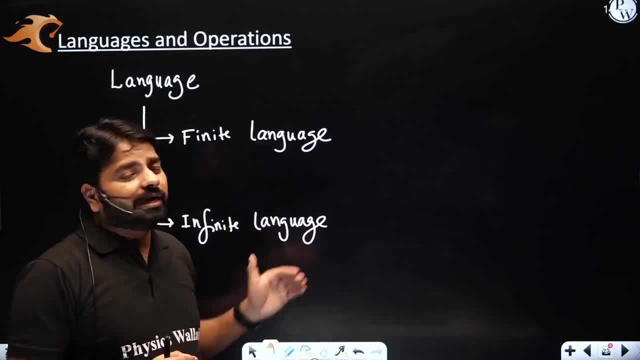 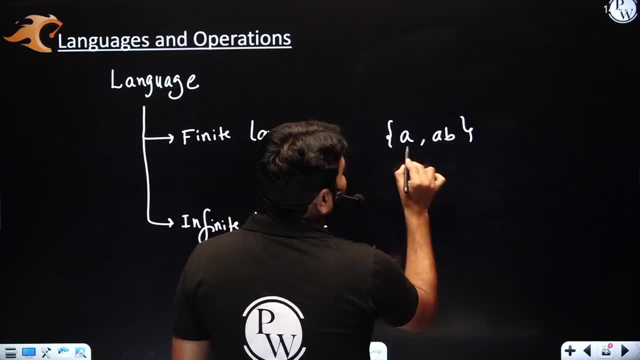 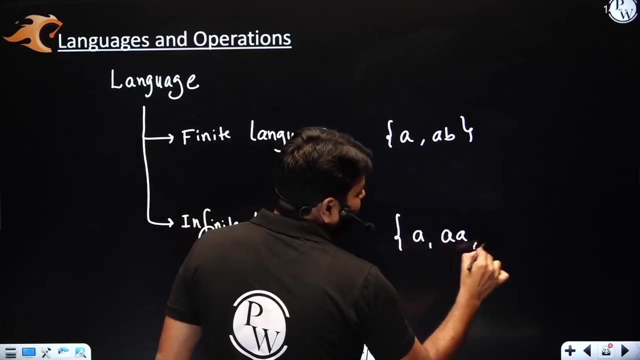 But in this language and in this language too, both should contain only finite string. type. Example: suppose I take A AB: Here each string is finite. but how many total strings? Two. So it is finite language Here. infinite language: A, AA, AAA and so on. 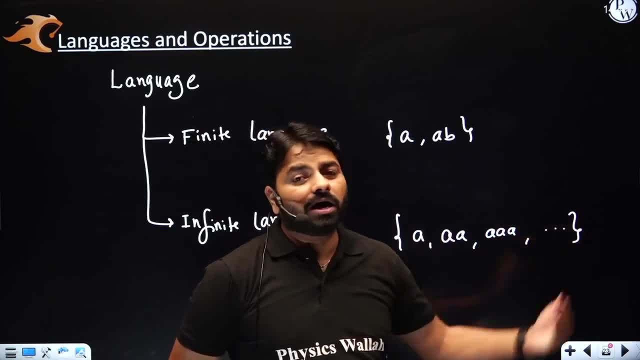 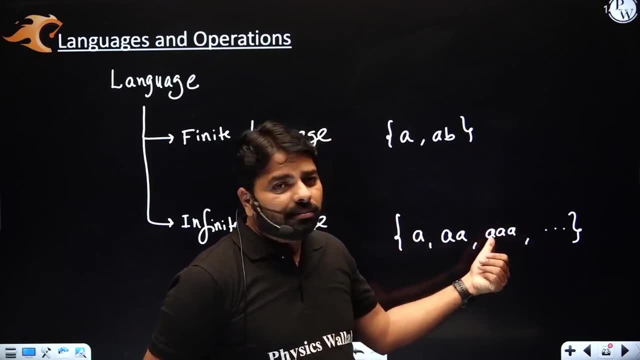 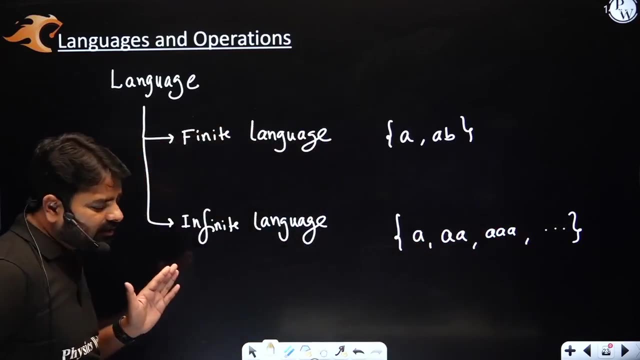 Here. see, every string is finite, but total strings are infinite. This is how you would say finite strings. only there Each string is finite, but such finite type you have infinite. This language is called as infinite language. I hope you got a clarity. what is the finite language and what is the infinite language? 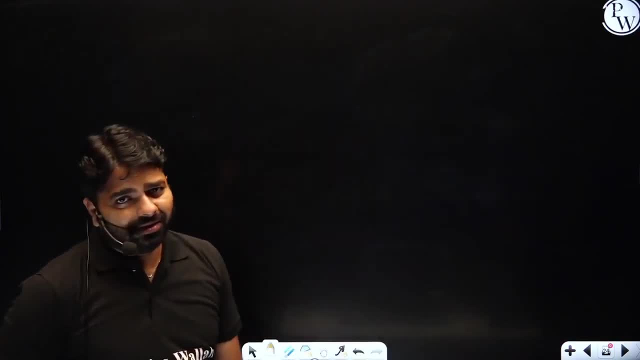 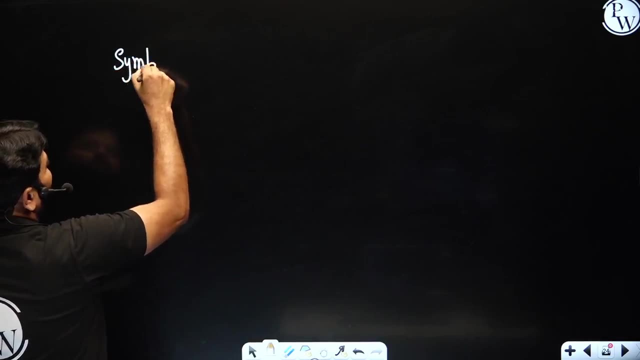 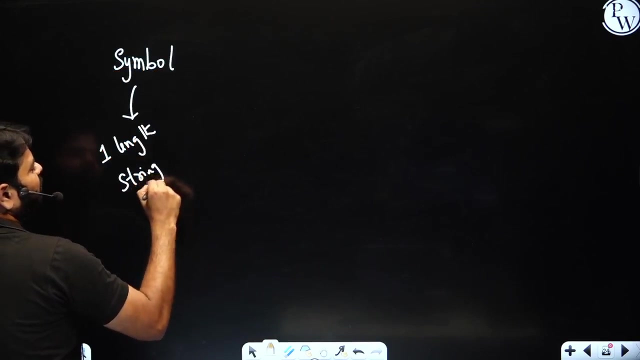 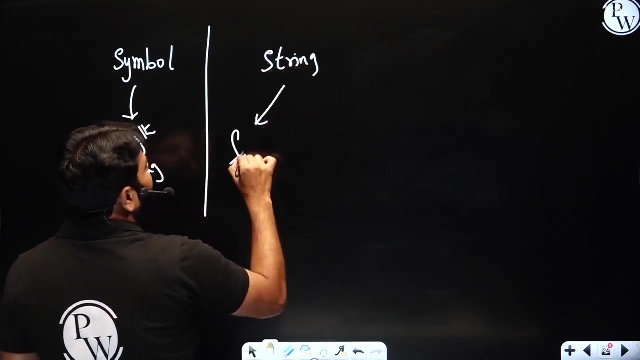 And let me give you clarity before going into the actual topic. So here, symbol is always one length string, No doubt about it. One length string. You will never have two length. Symbol means one length And string is actually two types in general. 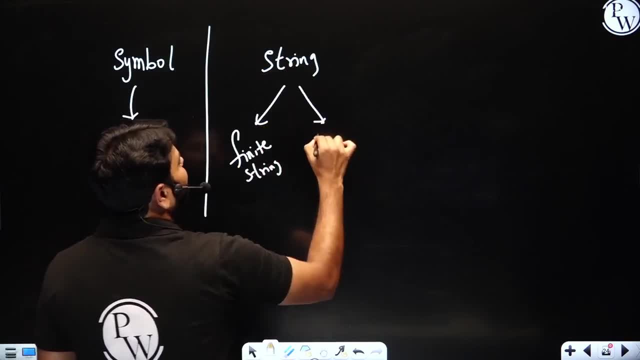 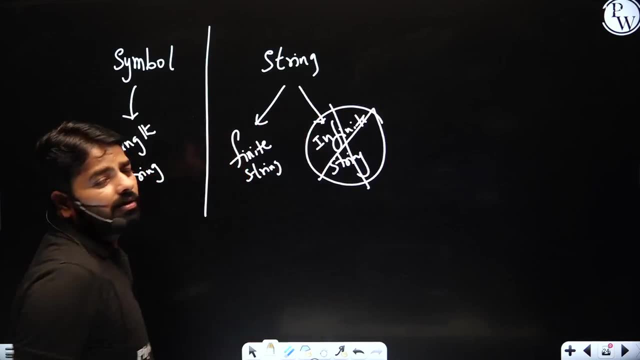 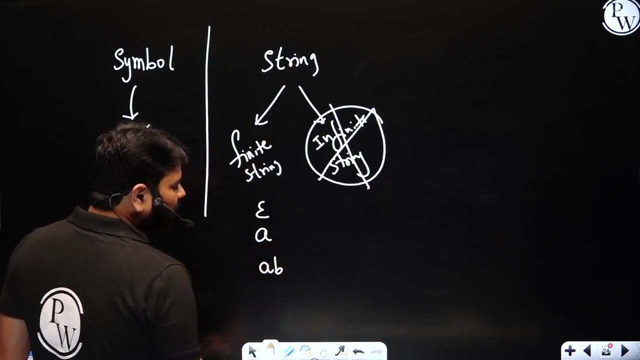 Finite string and infinite string, But in theory of computation we never use the word infinite string, So this is not possible. String means we always take finite string, We always write something- epsilon, A, AB- But you never write A, B, A, dot, dot, dot. 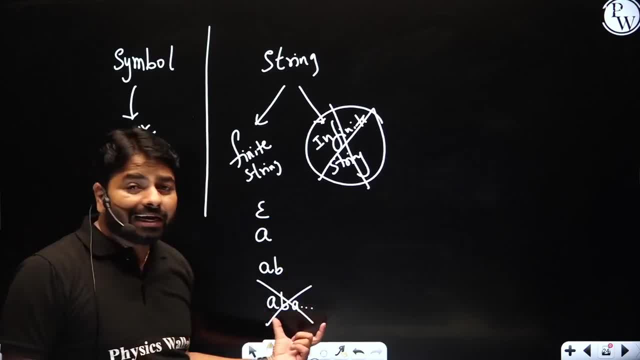 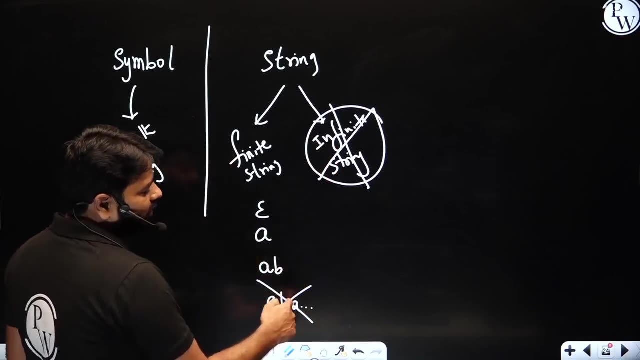 This is impossible. You must mention like a real number. Real number will never. sometimes you can represent infinite length, The number itself, But string itself you can't represent infinite. So we don't use in computation at all This string is infinite actually. 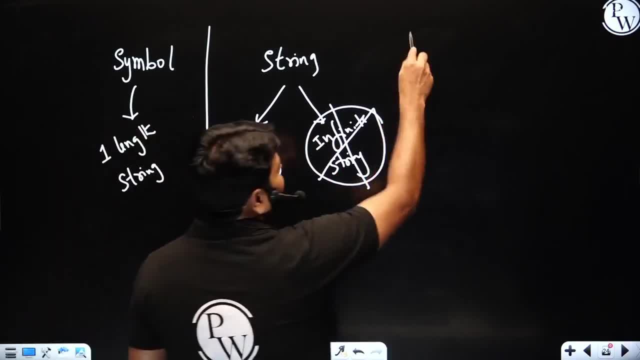 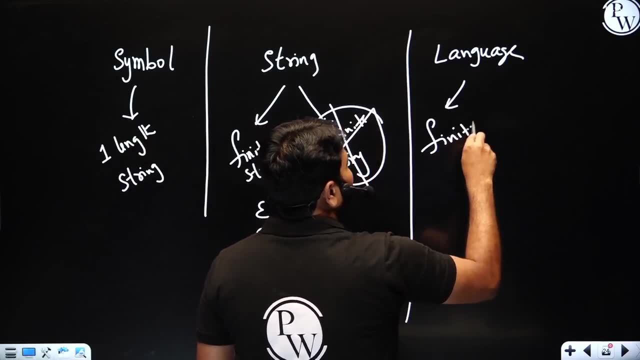 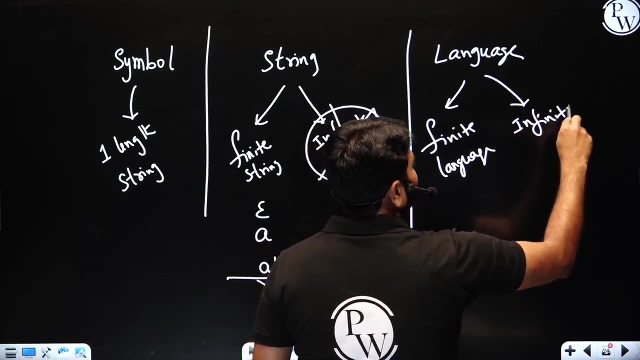 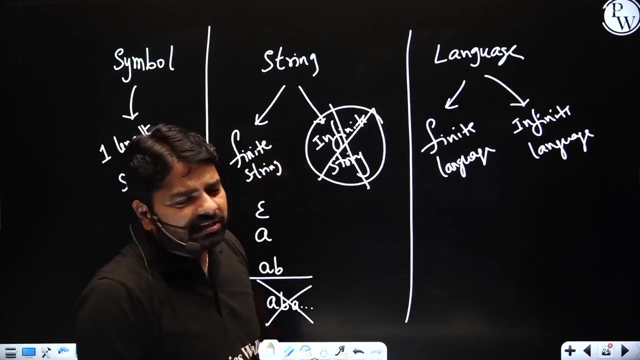 But we don't use in computation. And language is two types: Finite and infinite. That's possible. Finite language and infinite language, That's great. I have just shown that And, in case, if you want to represent infinite language, there are various examples. 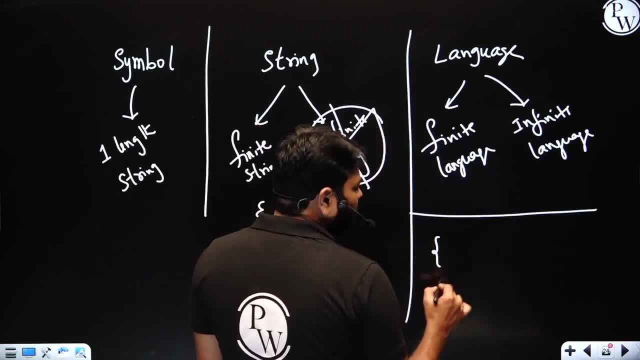 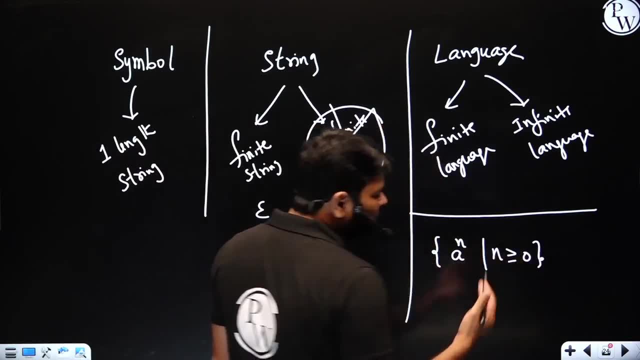 So let me show some of them. Like I want to represent A power n such that n greater than or equal to 0. It's going to represent infinite language. How do you know that? See A power 0, A power 1.. 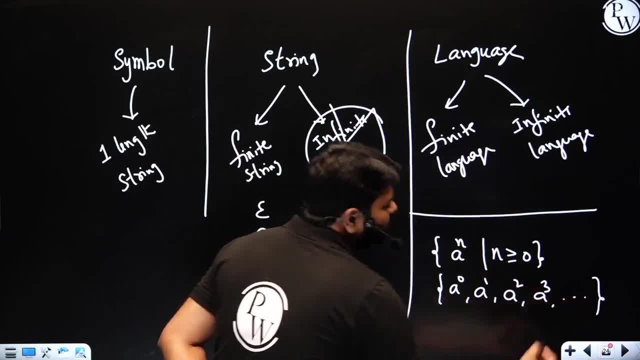 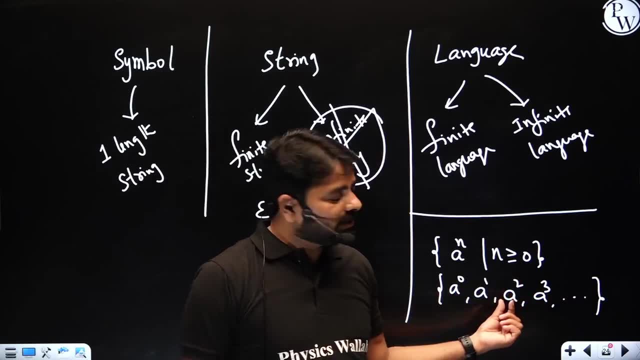 All the possibilities. when you write, It's going to form infinite number of strings. A power 0 means epsilon And A power 1 means 1A. A power 2 means 2As in consecutive And 3As in consecutive. 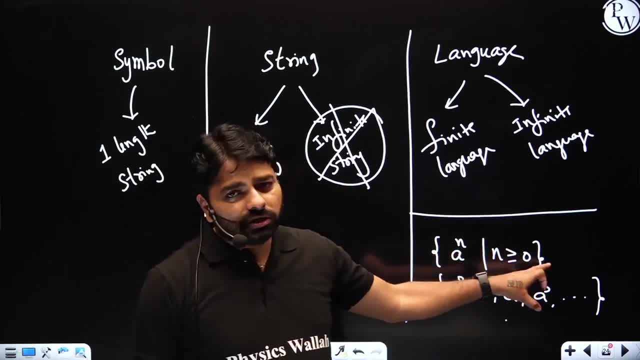 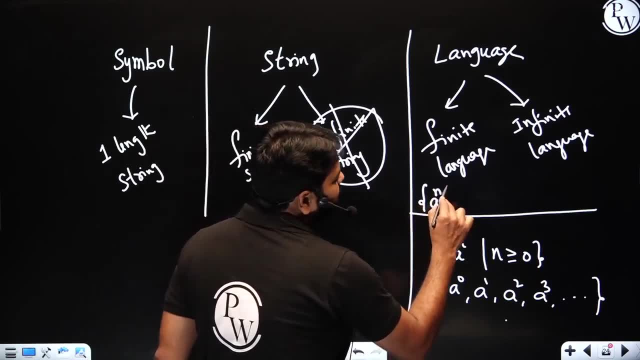 And so on, And this notation is going to represent infinite language. Similar notation also you can use for finite language, Like I mentioned, A power n such that n less than 3. Then up to 2 length you can keep in the language up to here. 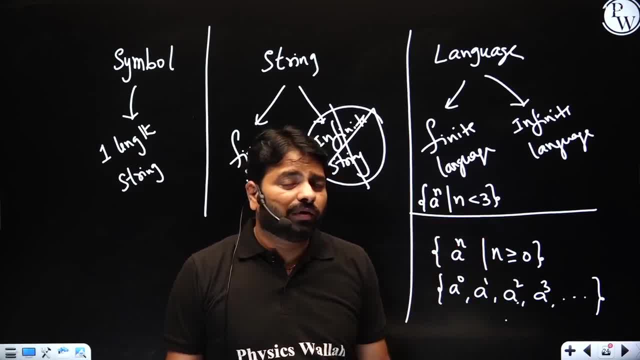 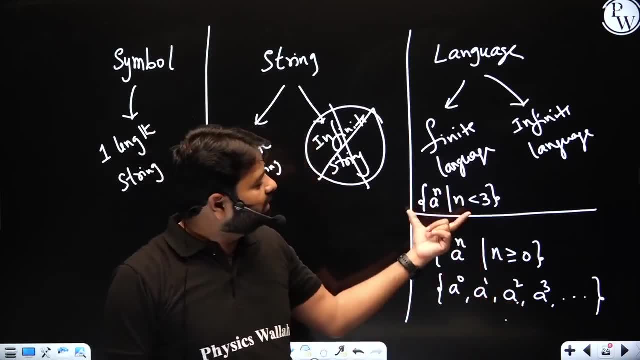 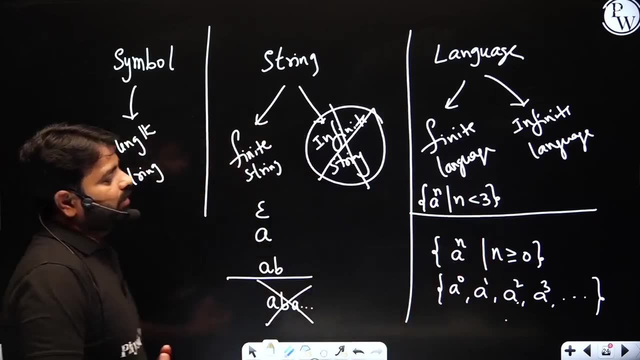 Then language will be finite. This notation can be used for both finite and infinite languages. Sometimes we write in sentence, Sometimes we represent the string, Sometimes we write in set notation. We all are actually equivalent to understand what is the language. Okay. 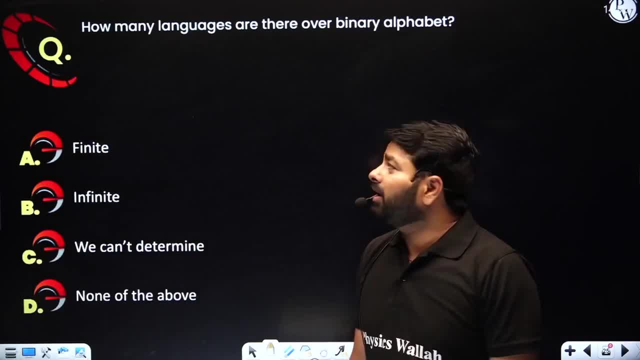 Now let's come to the point. So now we have understood, Understood what is the language. How many languages are there over binary alphabet? Binary alphabet in the sense sigma has two symbols. How many languages are there? Finite, Infinite, We can't determine. 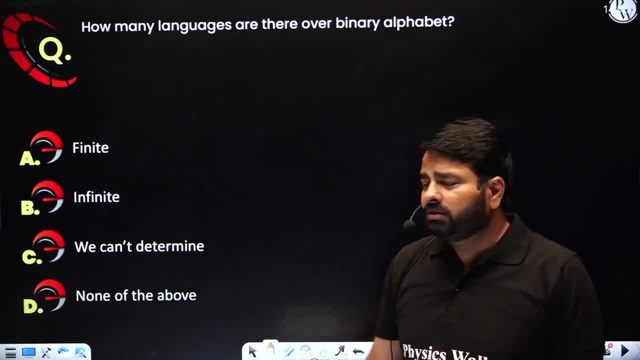 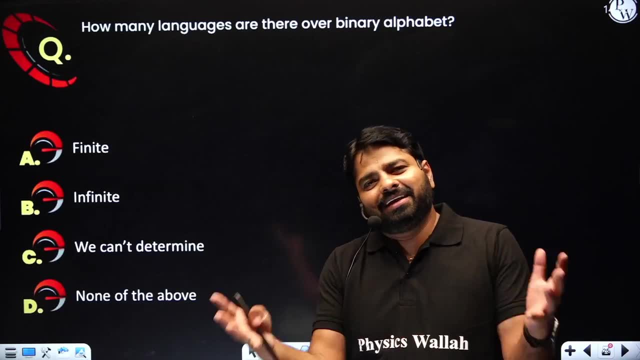 And none of this. So this: What is the right answer for this? If it is the finite number of languages, Then definitely. you can't write infinite number of strings In general for any given sigma. you have infinite number of strings. String is already infinitely possible. 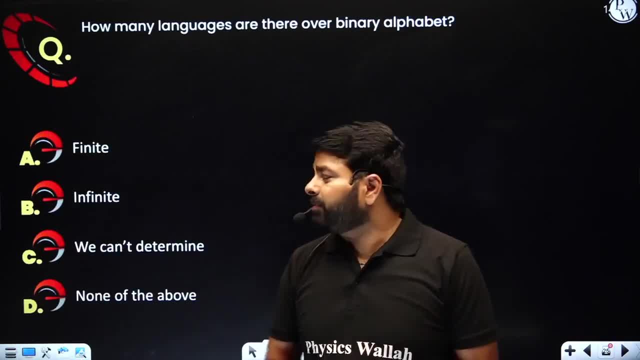 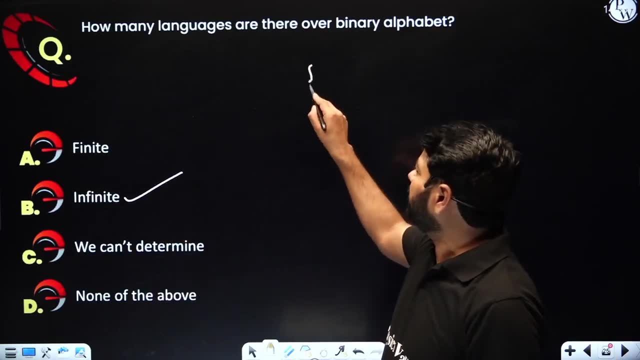 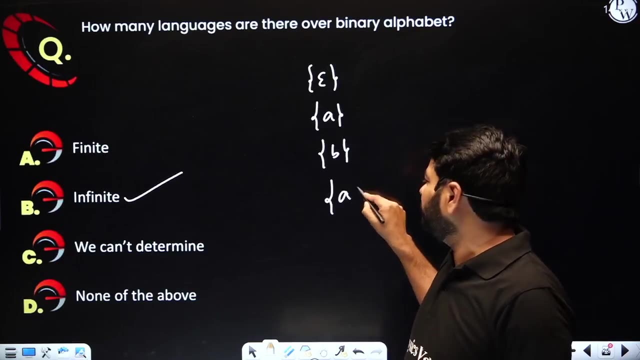 Right, Then language: definitely you can form infinite. So the answer is infinite. I have just shown with one length: only The language which has one string Like this, only you can form infinite. Why do you want different languages With one member? 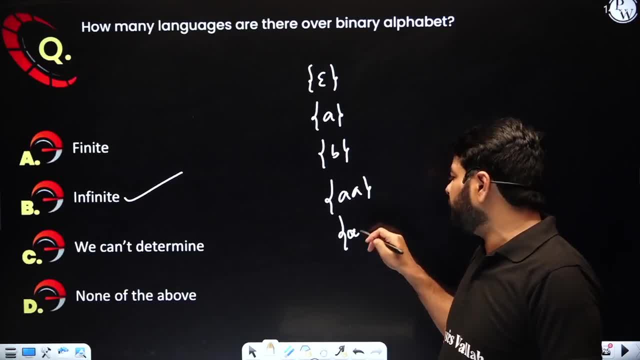 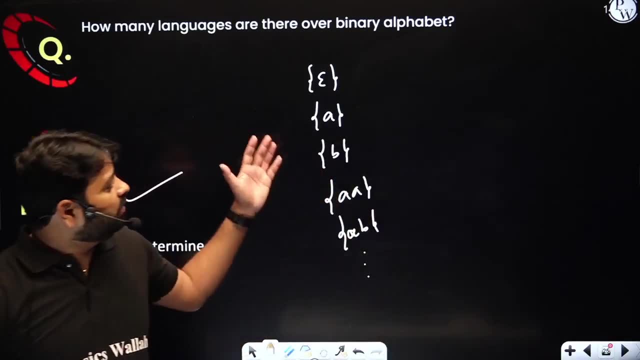 With one string. The language has only one string. You can form infinite languages, No need to worry about the size 2 or 3.. Okay, This is how you can say: Just understand how many strings are there? Infinite strings, Each string you put in a set. 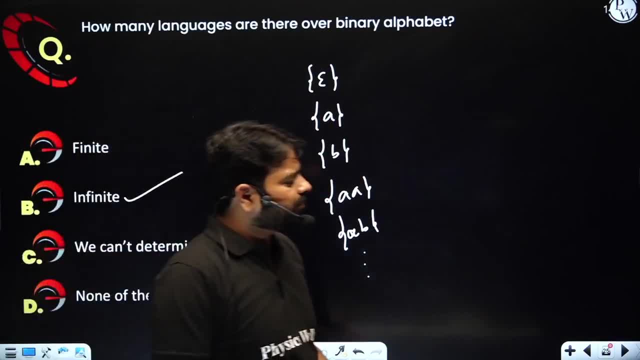 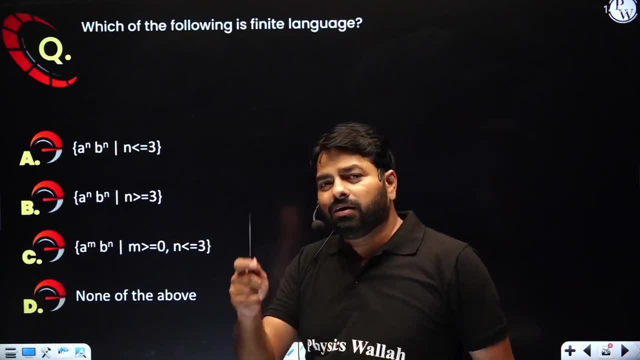 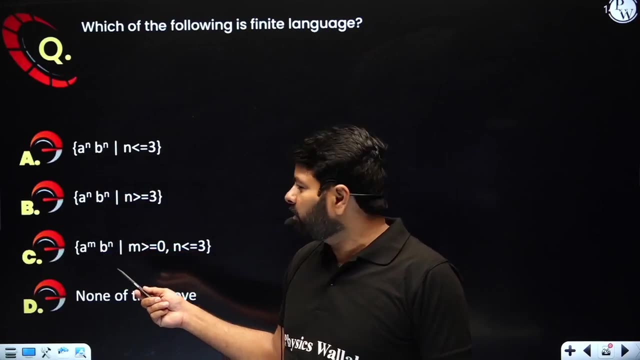 Singleton sets only, there are infinite. Okay, Very simple. Next, Which of the following is a finite language Can you identify using the mathematical set definition? Of course, we are going to come with these notations many times in future, But this time, which language is going to be finite here? 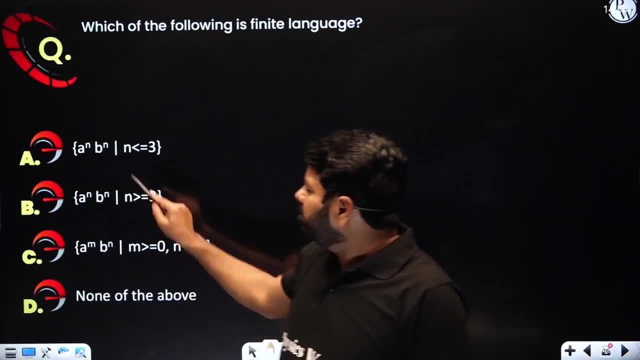 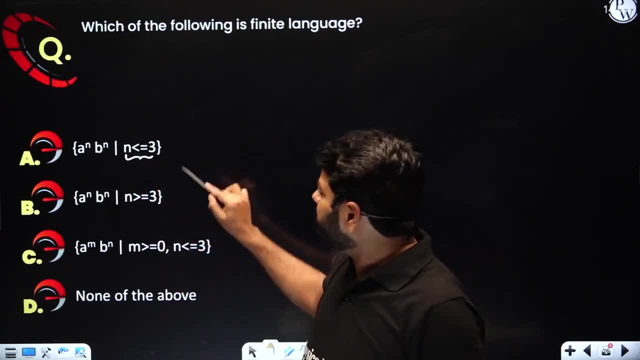 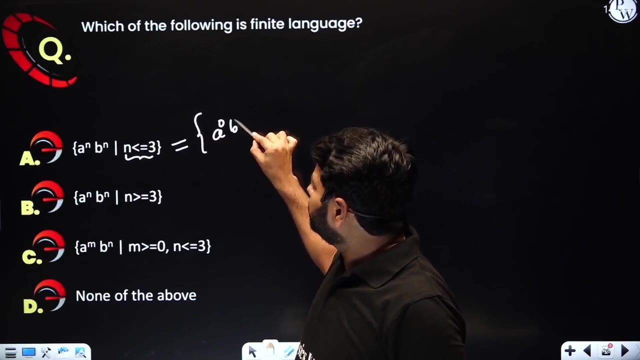 And which language can be infinite? Understand here n less than or equal to 3.. So here n value up to 3, you can substitute here. That means I can write here: a power 0, b power 0.. Because both are equal right nn only. 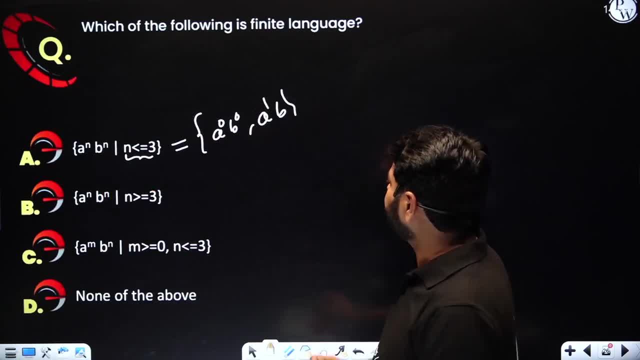 Another one: a power 1, b power 1.. Another one: a power 2, b power 2.. Can I write? Can I write a power 3, b power 3? Yes, But you can't write a power 4, b power 4.. 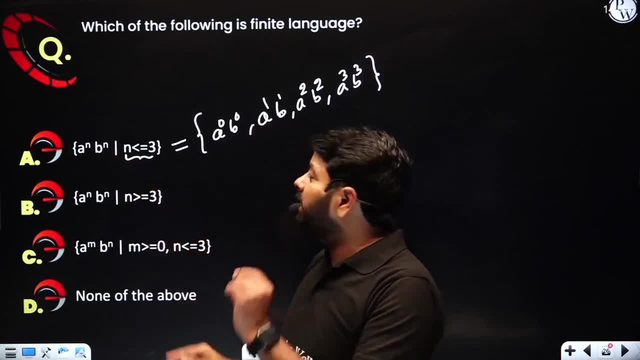 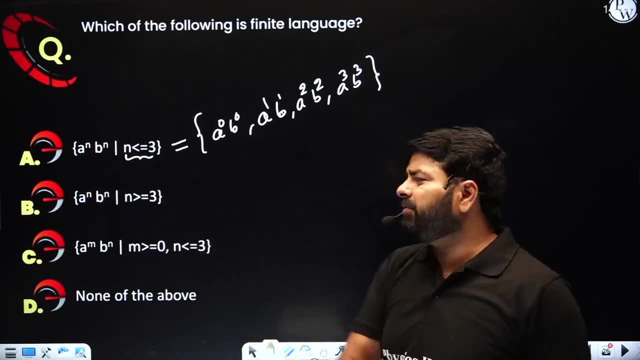 As you know this, both powers are same. That's why you can't write differently. Some people might write a power 0, b power 1.. That's wrong, Because both powers are representing the same variable. Now, how many strings are there? 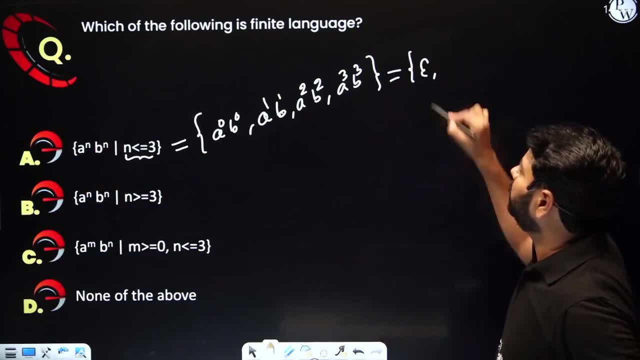 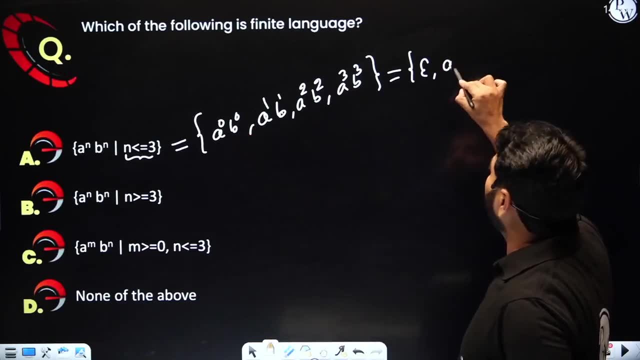 Only 4 strings. What are they actually? One is epsilon: a power 0 followed by b power 0. Means 0 symbols followed by 0 symbols. That is epsilon only. Next, ab Is a power 3, b power 3.. 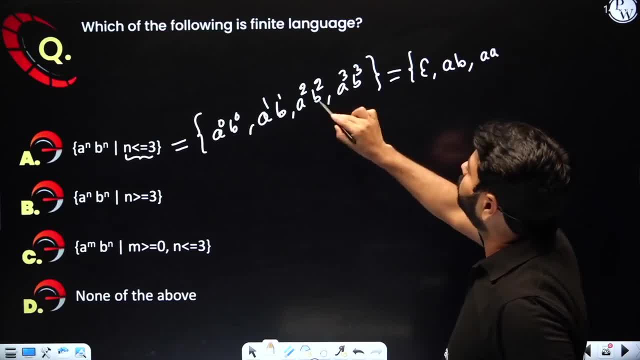 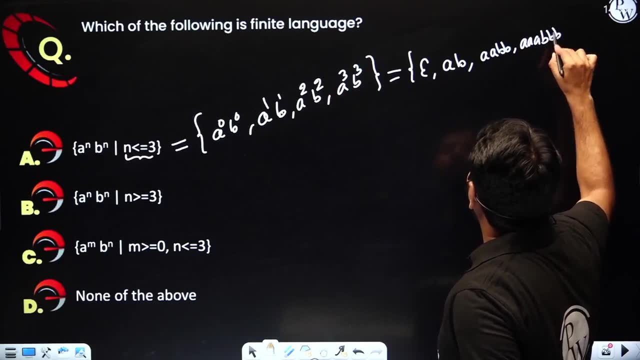 a, power 2 means aa, b. power 2 means bb in a sequence, And similarly, 3a is followed by 3b. That's it Definitely. this is what a finite language. As per the question, we got a finite language. 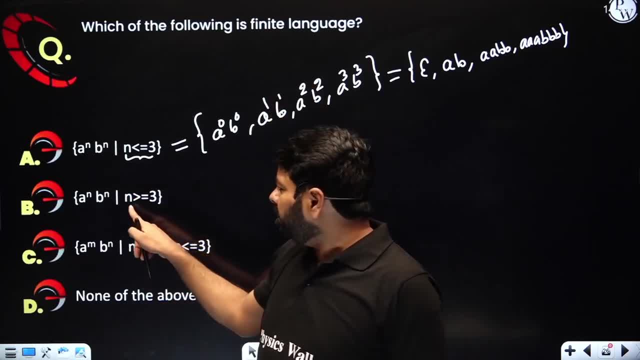 But you need to identify. it could be MSQ type, You don't know. right n, greater than or equal to 3.. It starts from the 3, but there is no end for it. Right 3, 4,, 5,, 6.. 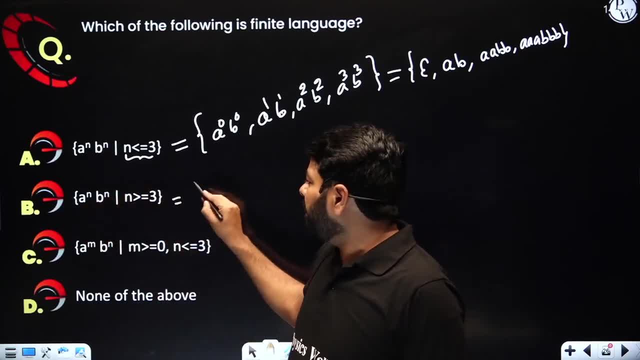 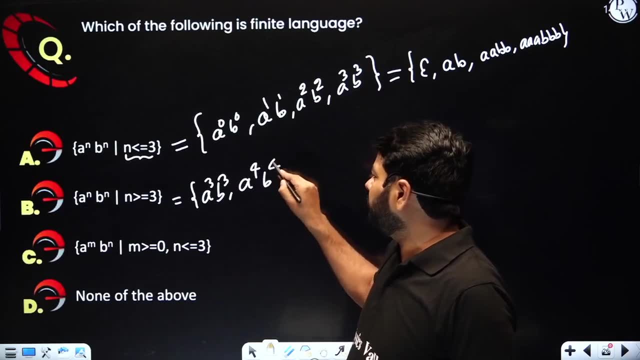 You keep on writing it. infinite strings possible Here. you will have a power 3, b power 3.. Is there any end for this language? No, You keep on writing. you will have possibly infinite strings: a power 6, b power 6, and so on. 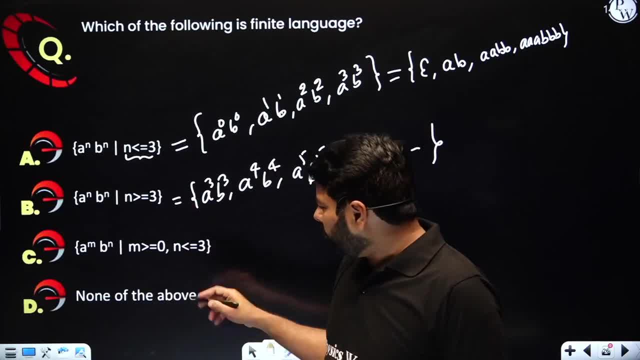 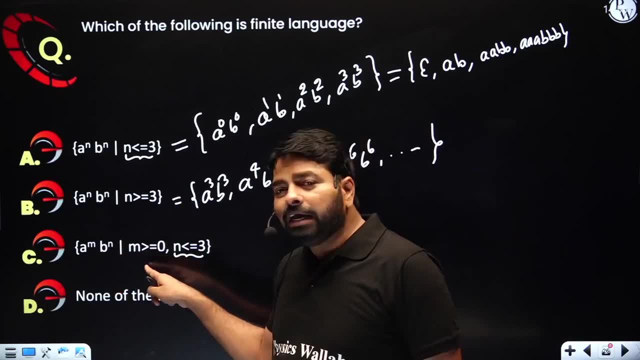 No end, Right, This is infinite language. And now n less than or equal to 3 is fine. That could form possibly finite number of b's, But the a's number of a's is already starting from 0. But it can have any. 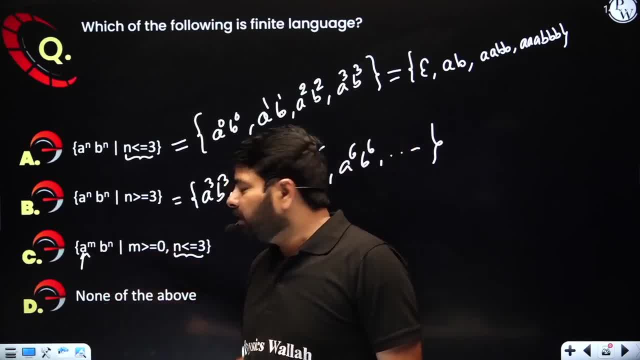 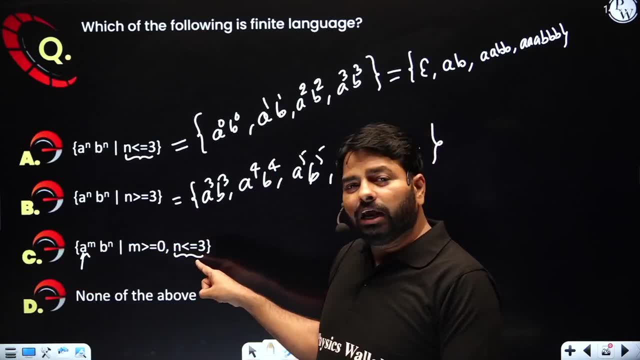 So this is the key. The a's here can have any number Like no a, 1a, 2a, 3a, 4a, 5a and so on, Even though b's can be 0,, 1 or 2,, 1, 2 or 3.. 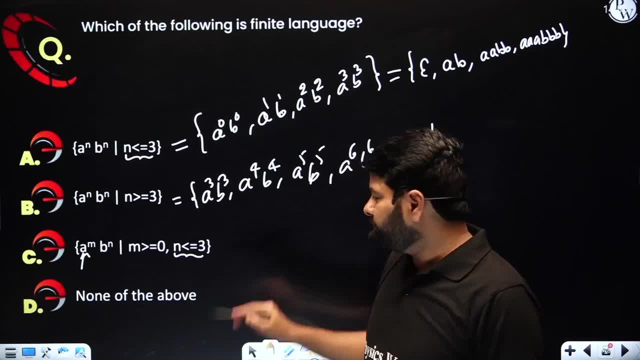 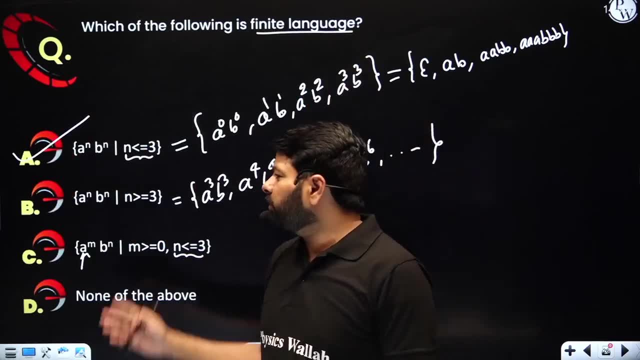 But a's are any, This could represent infinite set. So this b and c are infinite. a is only the finite language that you have. Fine, This is how you can identify. Of course, these questions are very easy And without this, the TOC you know could see. 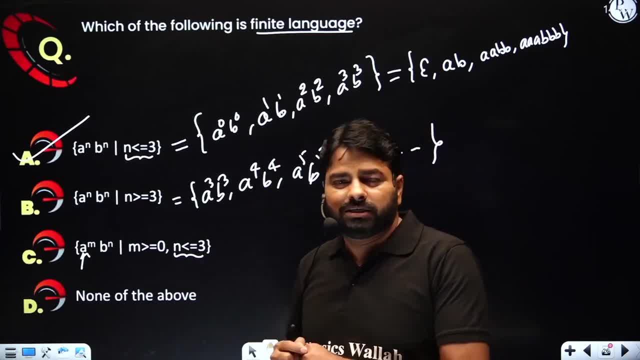 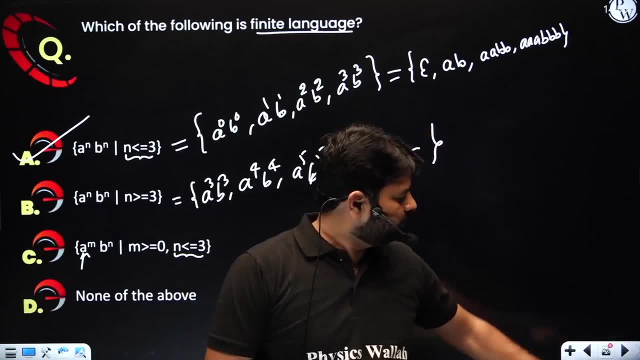 A different way. That's why I am trying to cover in the basics What is a language? How do you understand a finite language? So this can help you a lot. Now we know languages And if you want to know some of them, 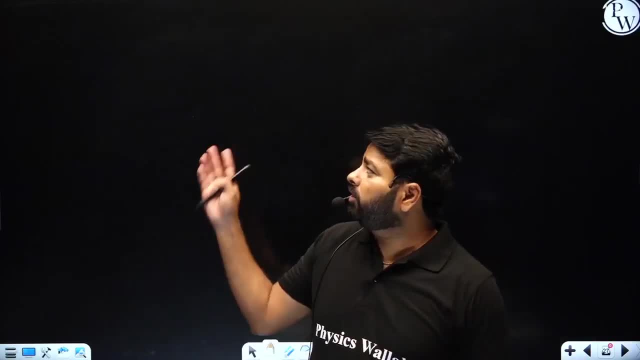 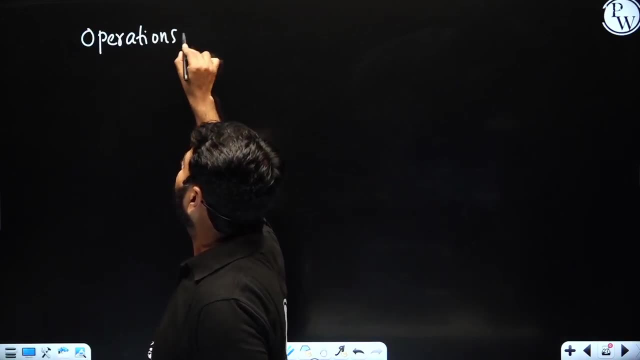 Okay, Like operations, I will just tell you, Before going to the Chomsky hierarchy, Some of the operations. Anyhow, The closure properties, We will talk about these operations. much Language operations. Suppose I have a one language, L1 is equal. let's say: 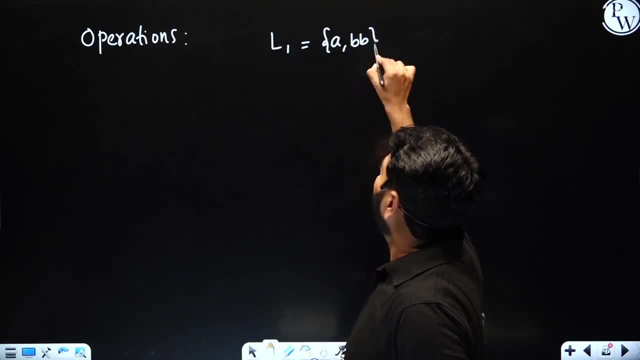 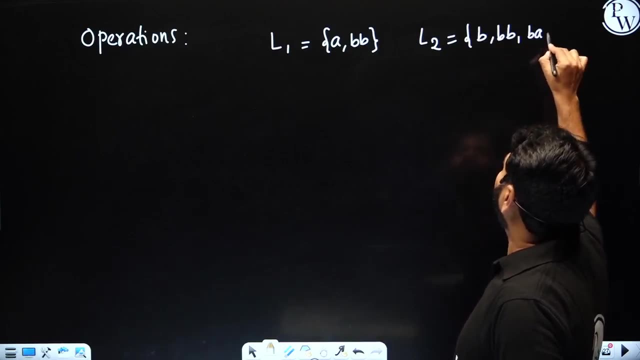 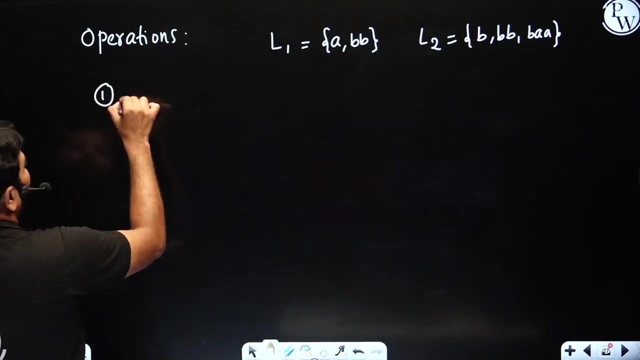 a comma b b And L2 is equal. let's say b comma b b comma b a a. So I have two languages. What are the operations you can do over these languages? One is, let's say, union, Very simple. What do you mean by union? 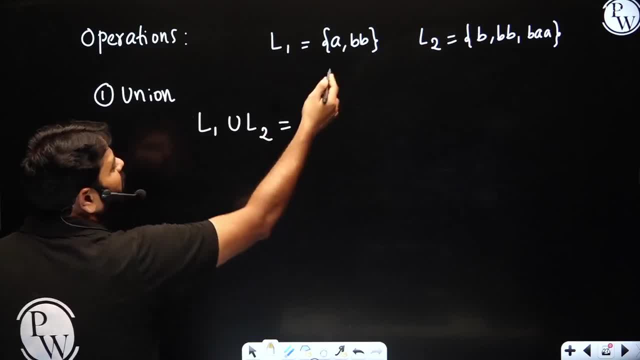 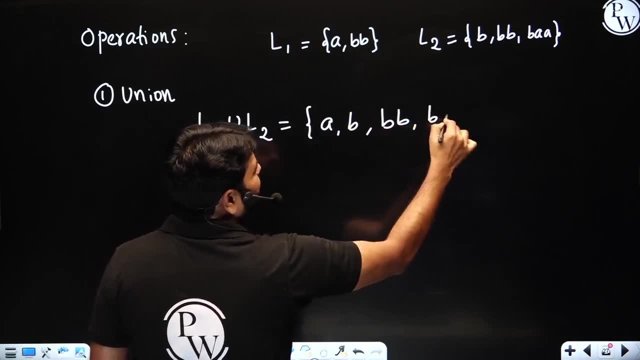 If I do L1 union, L2.. We will combine all those things from L1 and L2.. You may get like a, b. I am combining both Like set union. definitely Here double b is appeared twice, So you take only one. 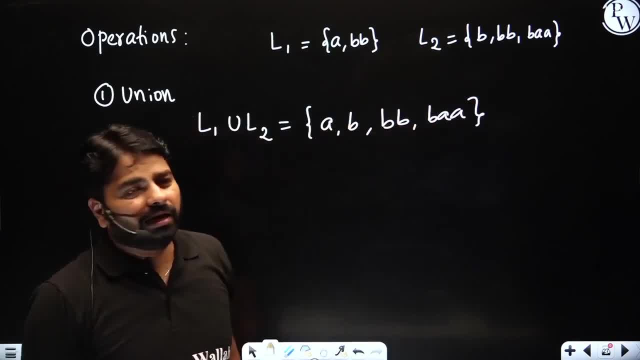 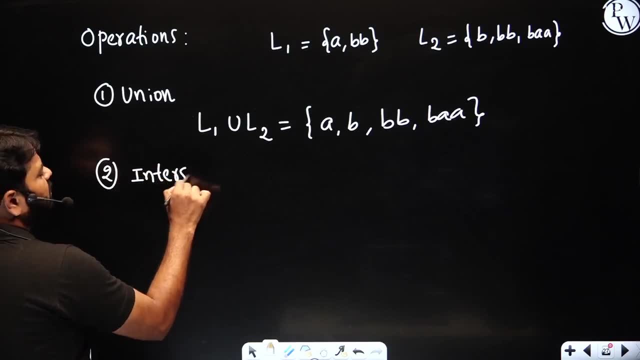 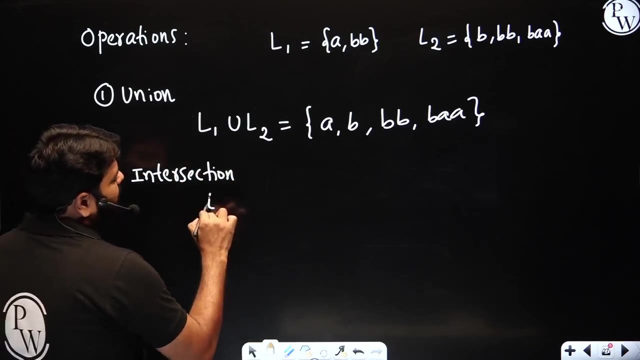 Because in the set This thing cannot be repeated in the language Right Now. Second Intersection: You will talk about these operations In detail In closure properties. Just I am defining What is union And what is intersection L1, intersection L2.. 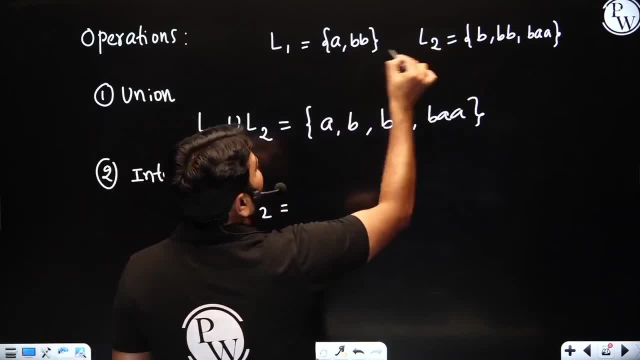 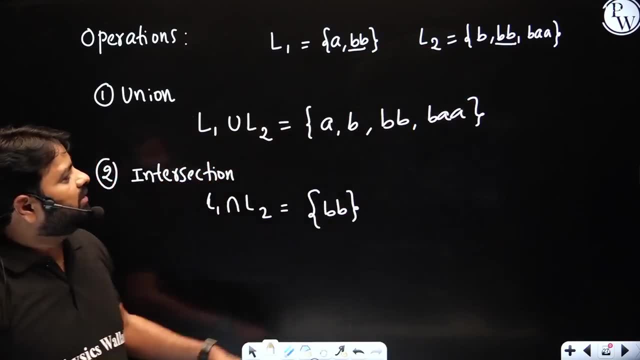 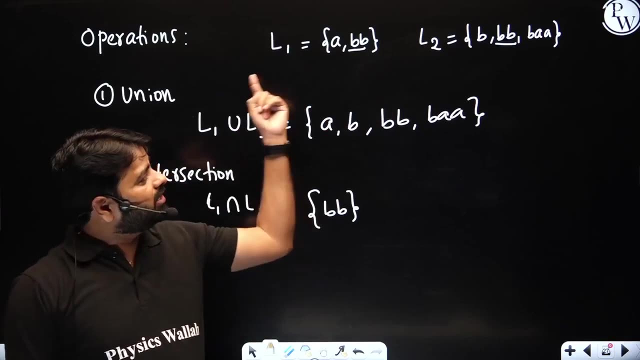 What is L1 intersection L2.. Which string is common? Double b is common in both of them, So you will get double b. The common strings of two languages is only double b. This is how you calculate intersection of two languages. Intersection of two languages. 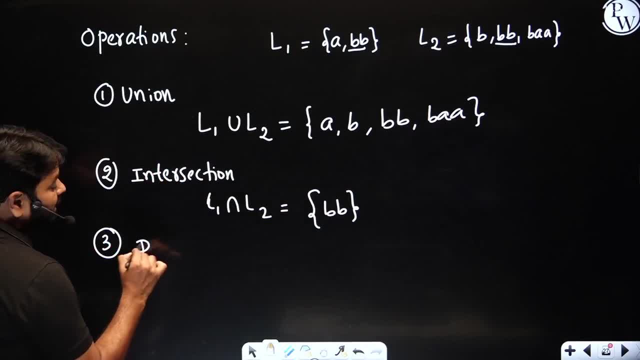 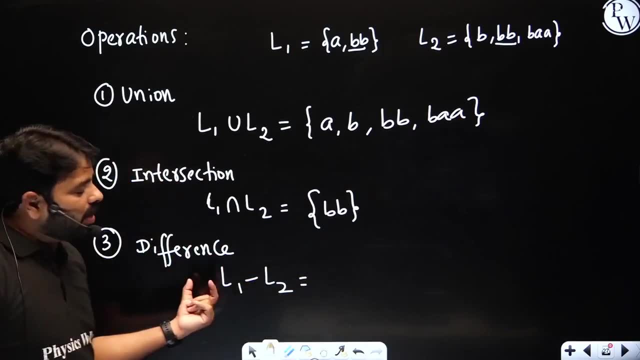 And what else you may have. You may have difference, Set difference or language difference. What do you mean by this? L1 minus L2.. From L1.. Delete the strings which are there in L2.. Again From L1.. 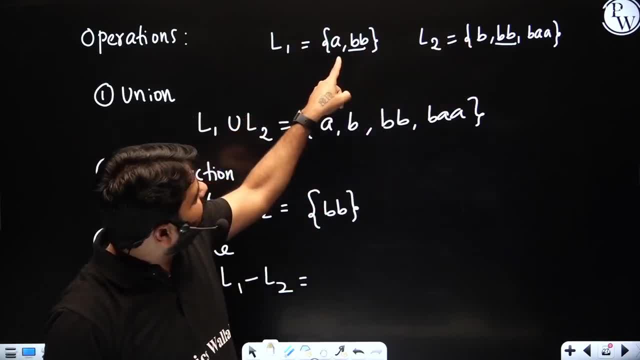 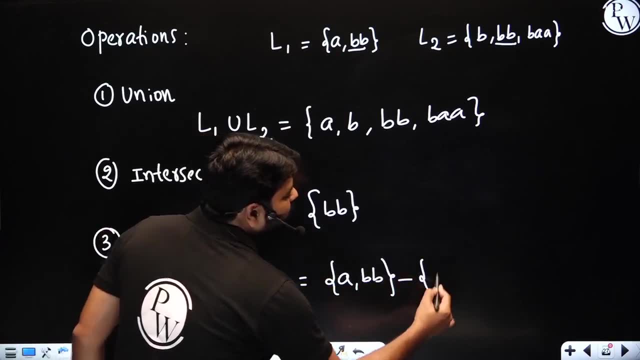 Delete the strings which are there in L2.. So which string is there in L2. Double b. So delete it. You will get a. See here: a comma double b minus b, comma double b, b, double a. Answer always depends on L1 only. 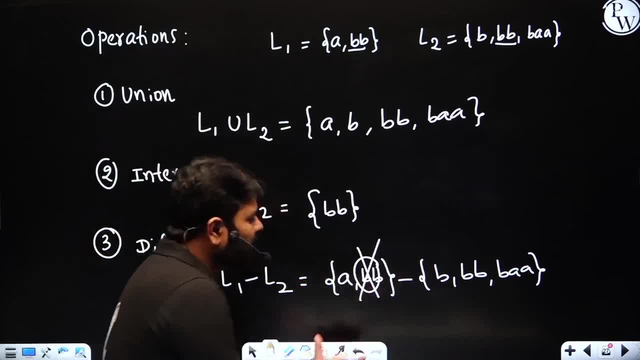 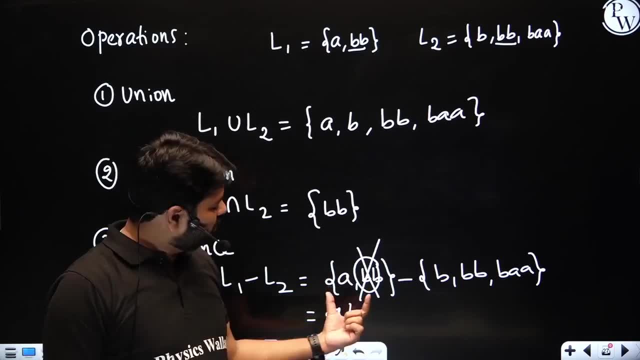 But those strings which are present in L2. Will be deleted. The answer will be only L1.. Ok, If a also present here, Then you will get empty set. Look at that. What is set difference? Similarly, You have lot of language operations. 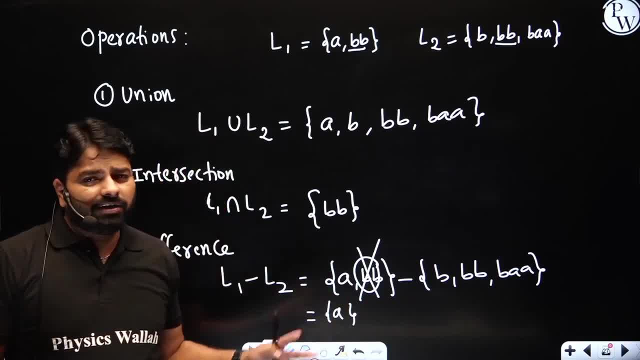 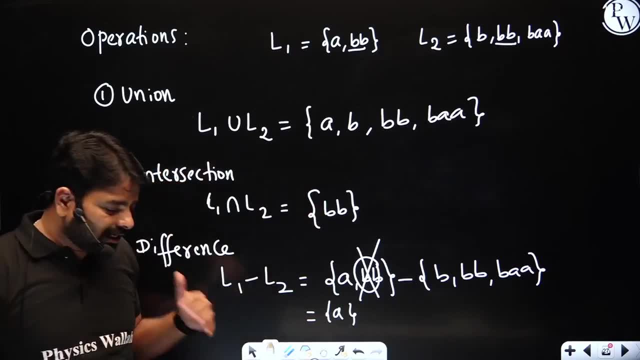 Like complement, You will have symmetric difference. All these properties or operations Will be covered in closure properties. I hope You have understood The strings and string operations, Language and language operations. All these are going to help in theory of computation. 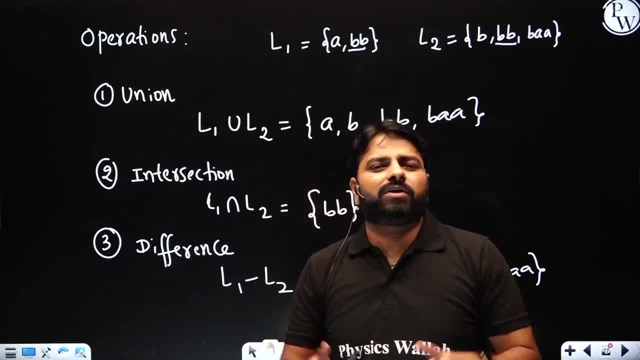 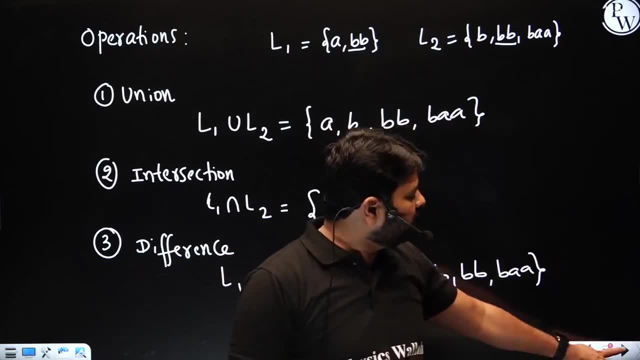 In various places To understand the behavior of the languages. To begin with This theory of computation. Let me begin with What is there in this theory of computation, That is, Chomsky hierarchy: In the beginning, In the end, At all the time. 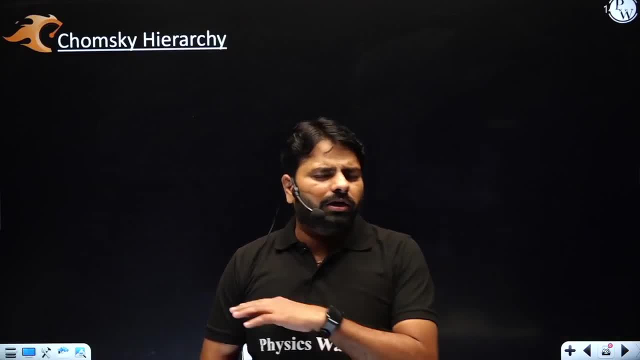 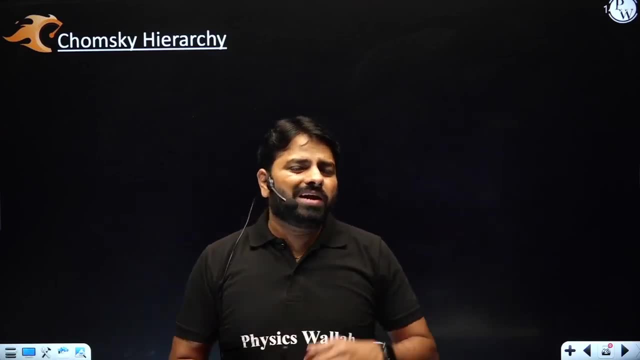 You are talking about the Chomsky hierarchy, only. In the Chomsky hierarchy All the languages are well classified And related, One language With other language. Clearly See here What are those. Classes Are present here, So 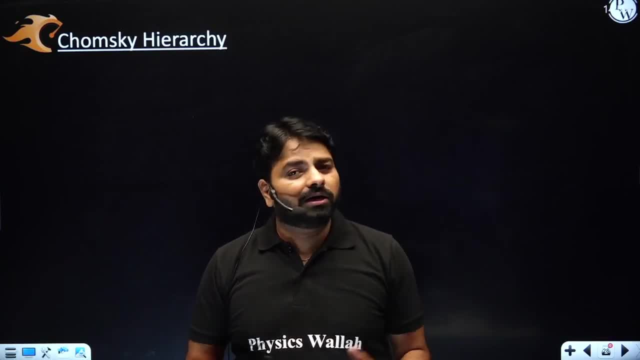 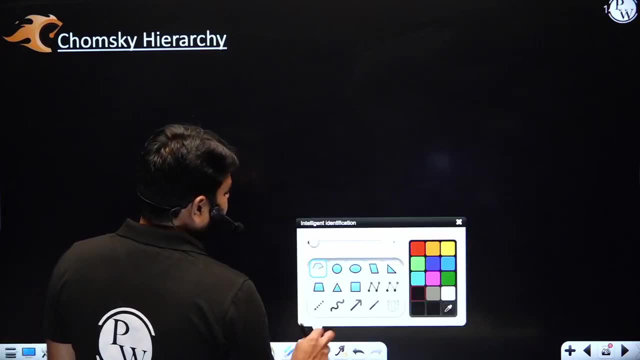 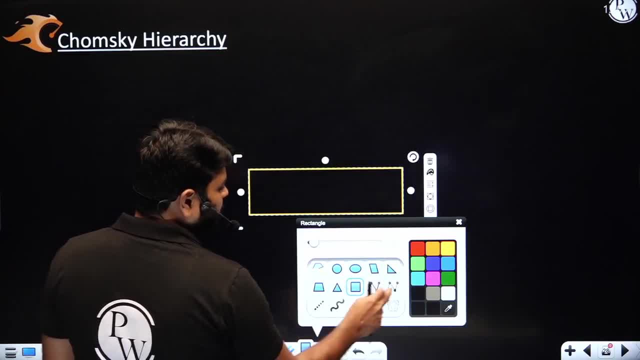 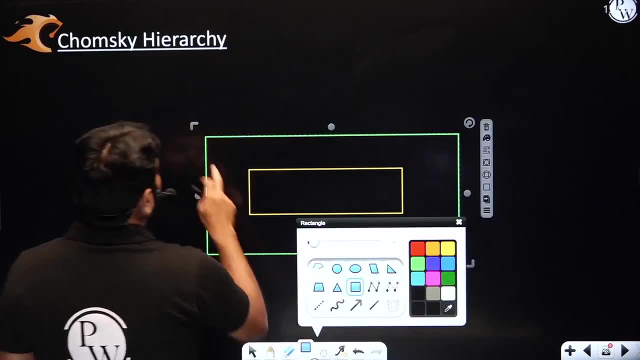 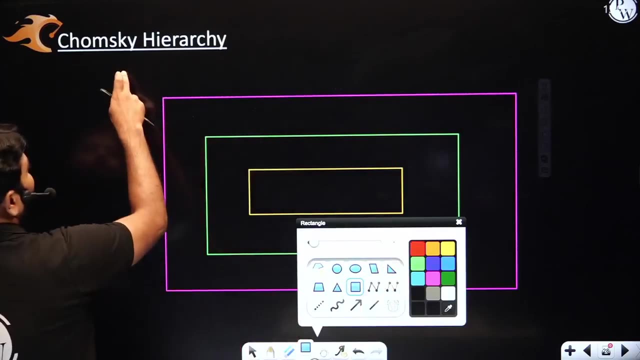 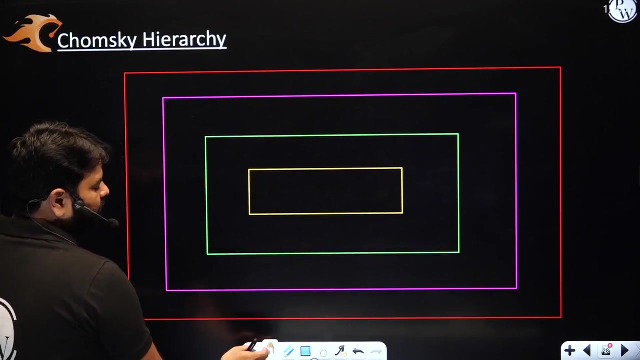 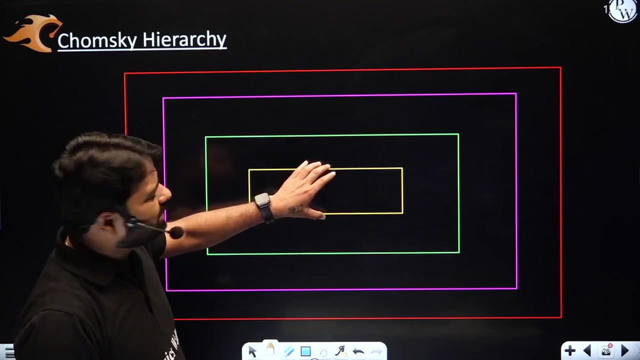 He has defined 4 classes: 1,, 2,, 3, 4.. 7,, 8,, 9,, 10,, 11,, 12, 13.. okay, one of those four classes, right class, you can say type three class and type two type one. 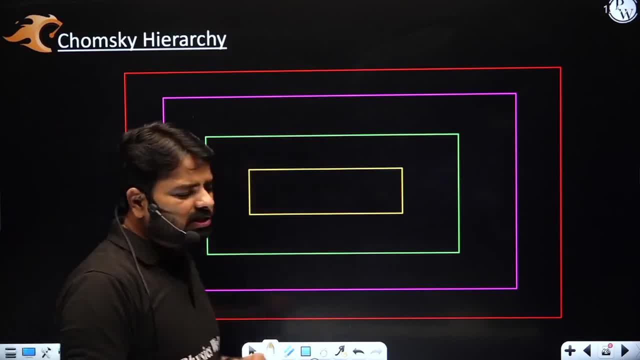 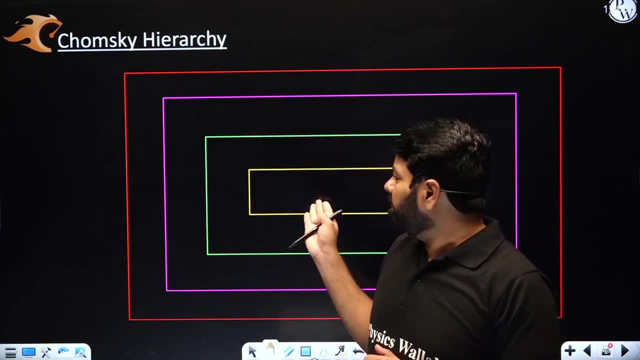 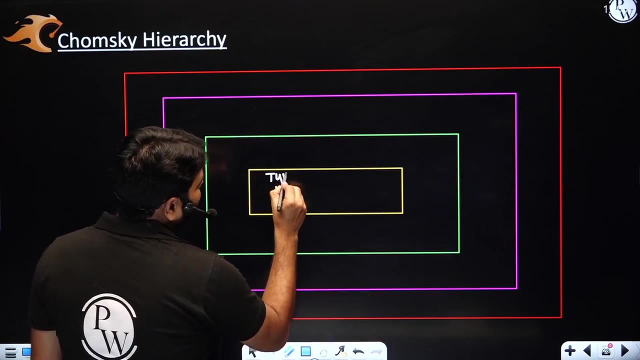 type zero. so we have a name for each box here. each box is not a one language, it is the set of languages. but all the type three languages are there here in one box. we call it as a one class. so i can say it is the type three class and the green one is the type two class- all the languages. 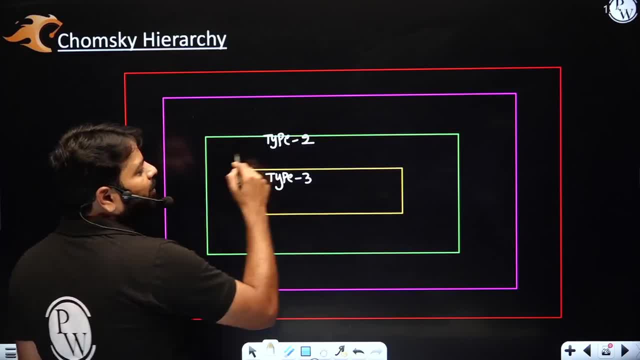 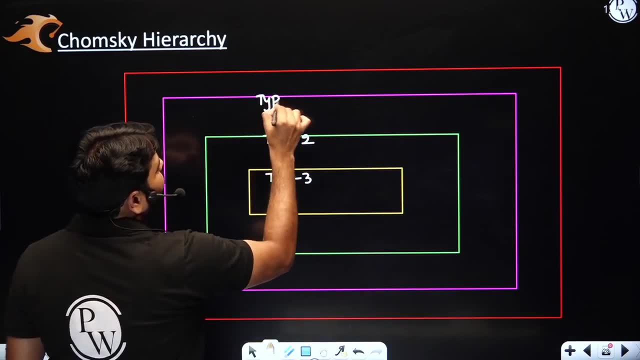 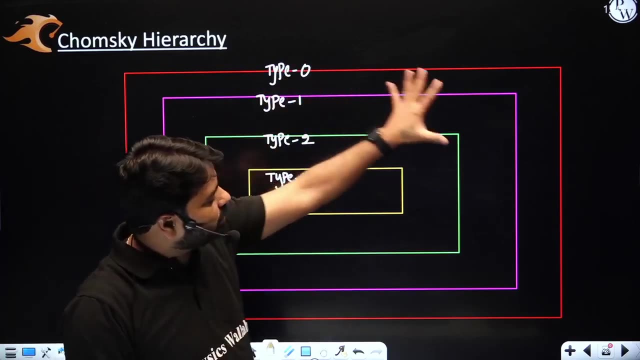 of one type will be placed in type two, but some of the all the type three also covered in type two somehow. and type one and type zero, the smallest number will represent biggest class. zero is going to represent biggest class guess one where it is going to cover all the other three types or three classes inside that. 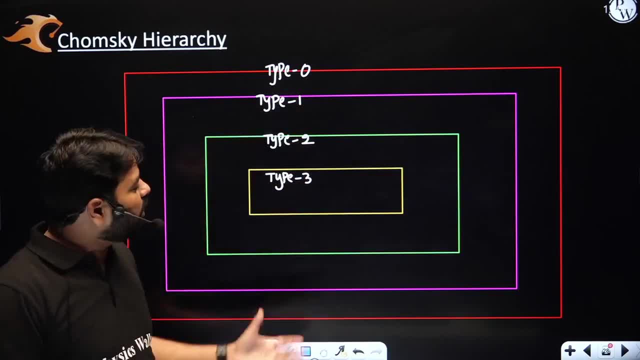 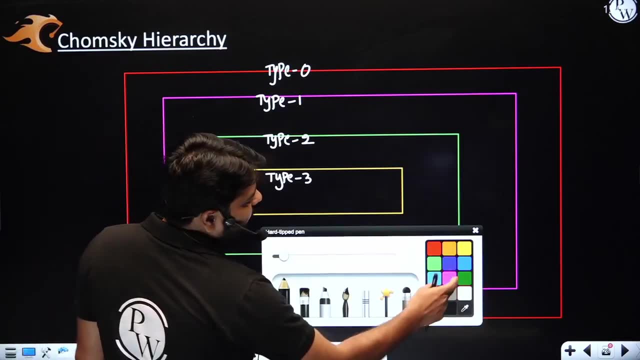 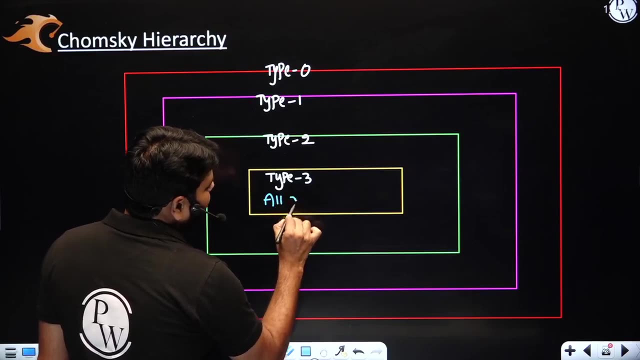 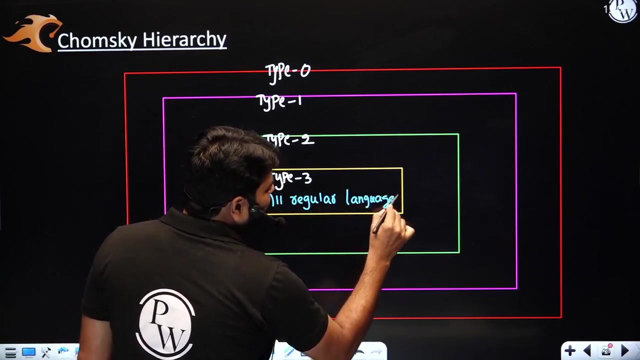 so what are the relations and what is this types? that is what chum's hierarchy is, the in the type three class, all the regular languages are covered here. here, all regular languages are covered here. what is the beauty of this regular language is that it is a one language, and it is a one language and it is a one language. 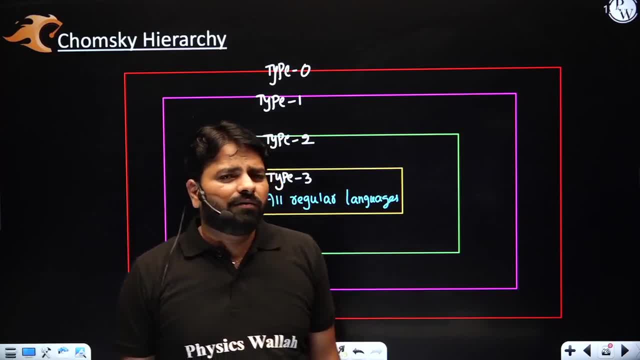 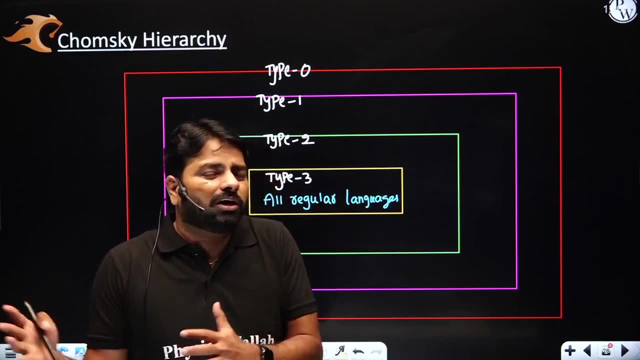 now, all the problems in the world which do not require a memory can be fit into here. that means to solve any problem. you don't require any additional data, such as like stack or queue can be placed here and you can solve with the help of this. representations like, whatever the models. 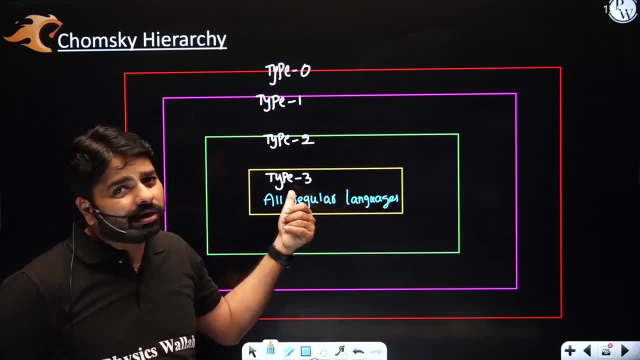 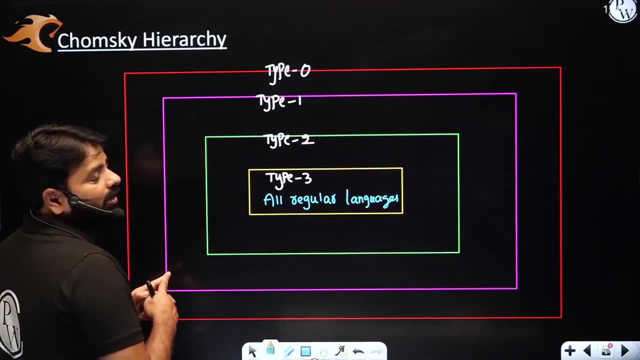 that you have here, like finite automata or any other model you have here. you can use them to solve. that is the beauty of every class here, and when i cover type two, the type two has a name: context-free languages, including the one language and the other language and the other language, and 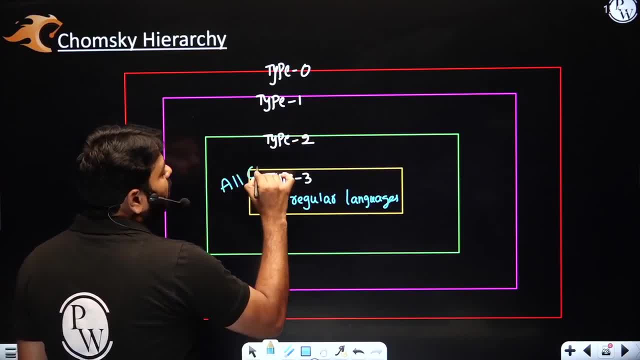 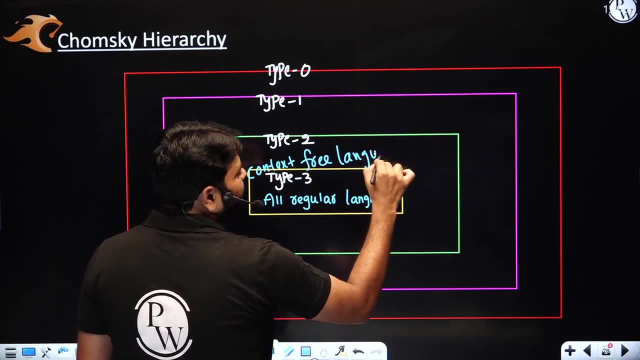 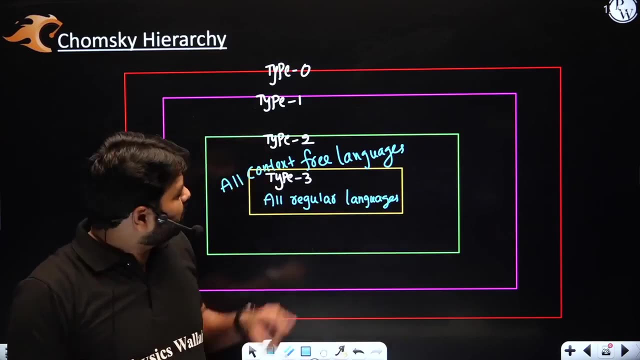 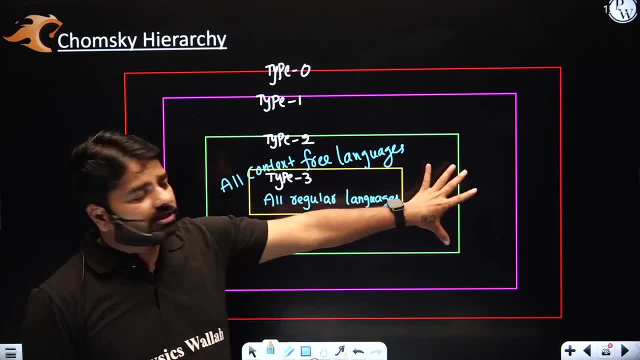 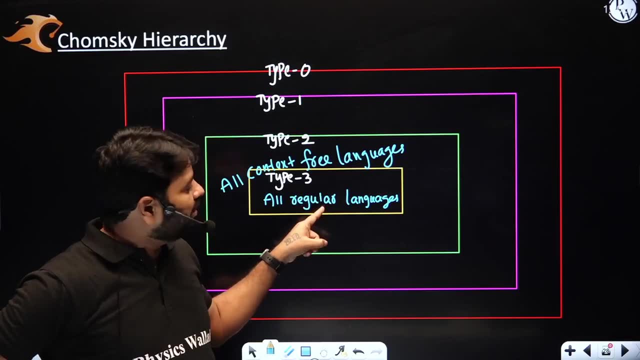 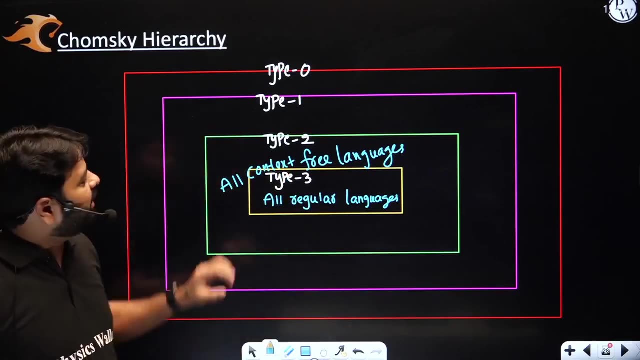 type three: ok, so all the context three languages are fit into this type two. so there is a relation: context-free- all regular languages are context-free languages. that relation is preserved here. okay, next type one: when type one comes, including these two languages, there are additional languages, all of them together called as context-sensitive languages. so here, all context-sensitive languages. 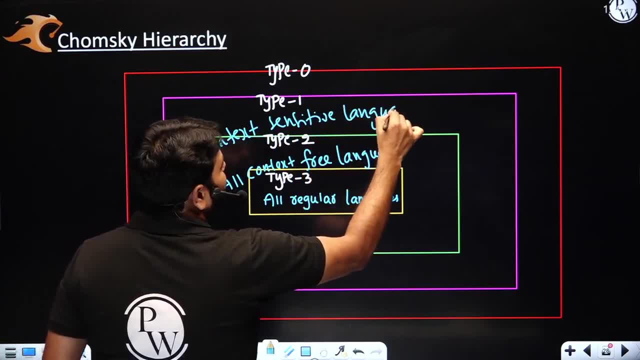 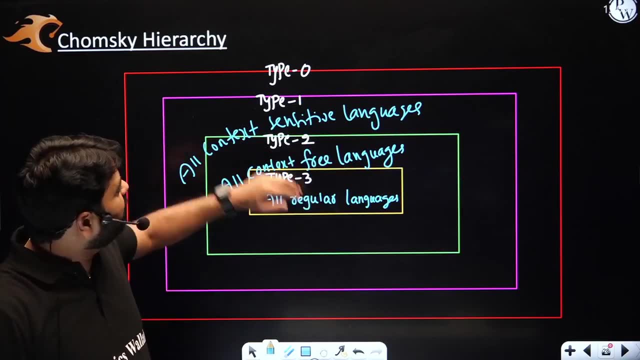 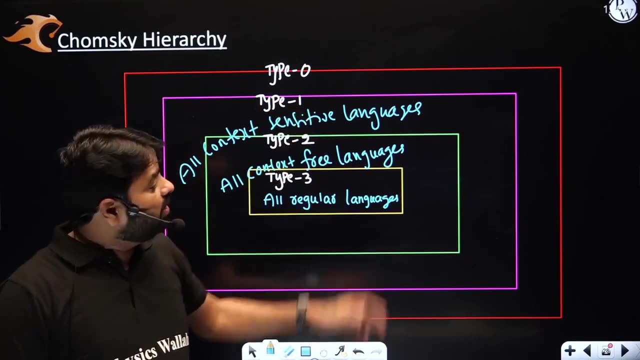 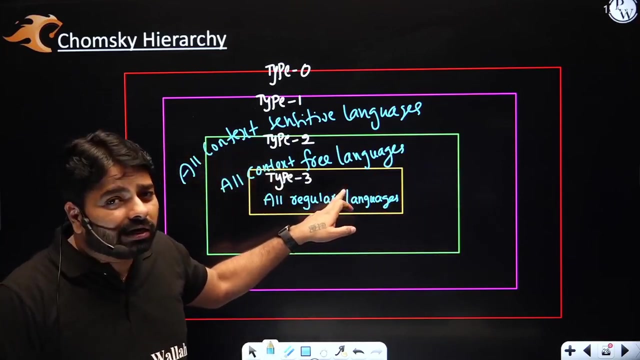 inside. remember, every regular language is context-sensitive and every context-free is also context-sensitive and everything inside type one is also context-sensitive. so this is what the difference between regular context-free and context-sensitive. but can i say every context-sensitive is context-free. context-sensitive can be here or here or here. so how can i say context-free if i 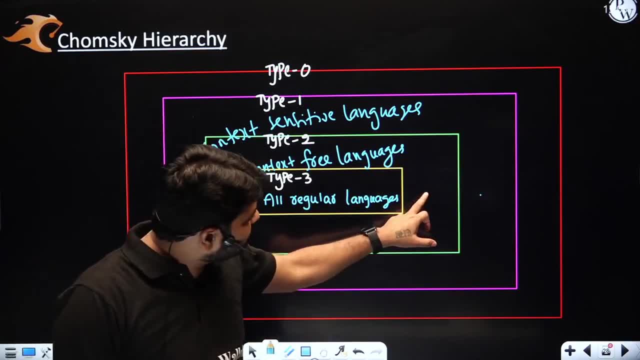 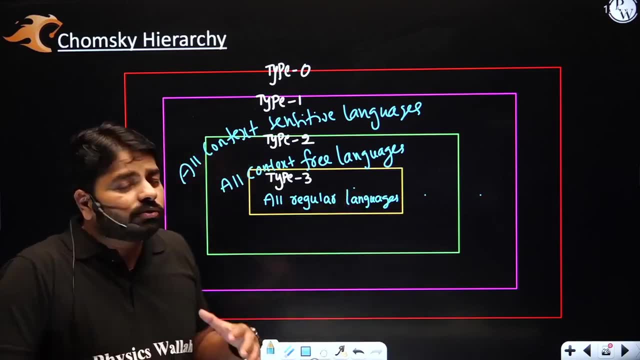 am going to be here, then that is not a context-free. but if context-sensitive is here, yes, that can be context-free. that is a context-free. if context-sensitive is here, that is a regular, also context-free. so you need to understand when i say context-sensitive language, don't 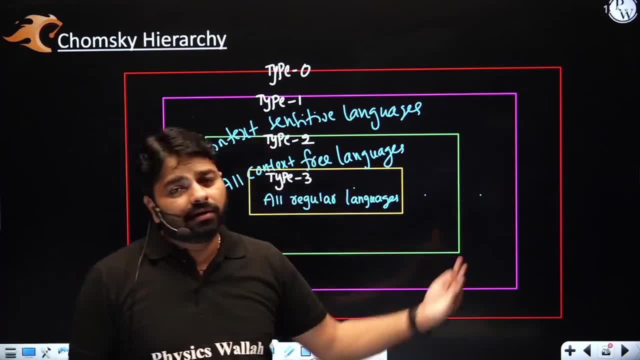 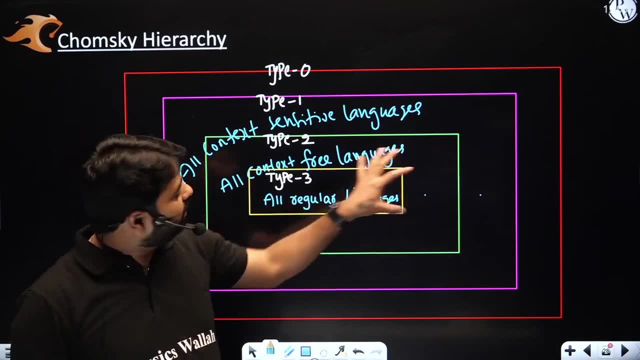 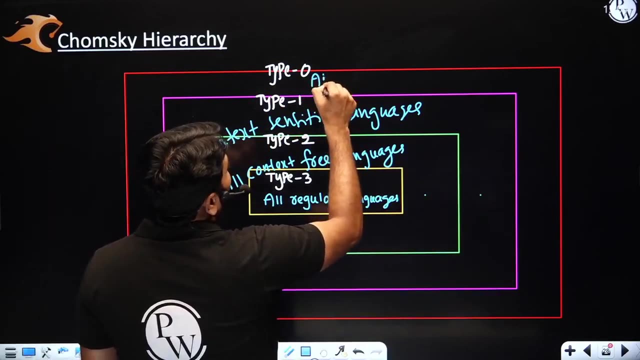 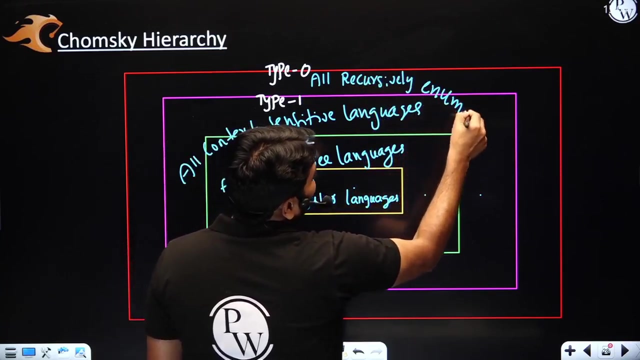 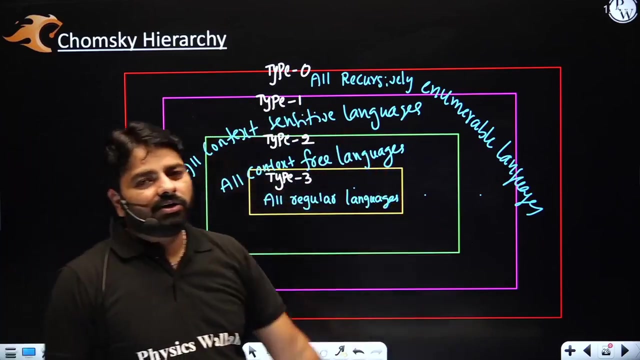 assume this one assume and every. everything inside the the pink color box is called as context-sensitive language. so all the context languages are here, including regular language and context-free. now type zero, the red color box, it is all recursively enumerable languages, all recursively enumerable languages here. that means everything i have written. you just say that recursively enumerable language are present. 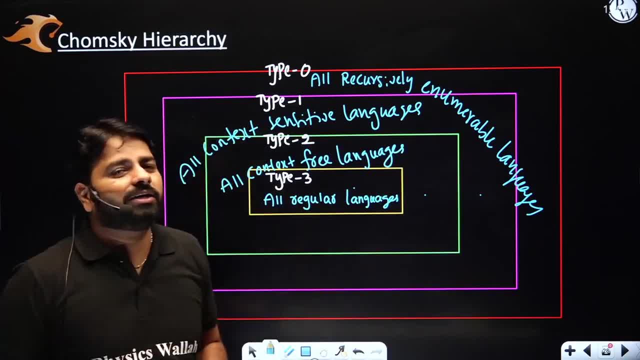 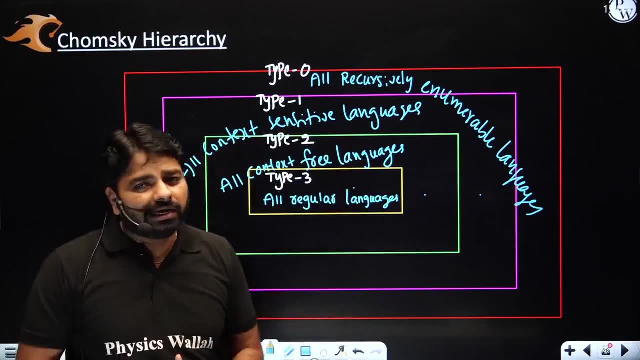 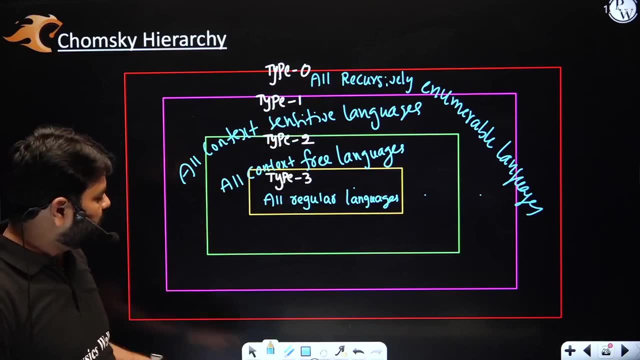 here this recursively enumerable languages are classified into here, four types, you can say. but we will learn later on, slowly. so all these languages are beautifully classified by chomsky hierarchy based on the computation behavior. we have a different models here, let us say here we me start with one by one quickly. as you know, i can't discuss all the chapters at a time right. 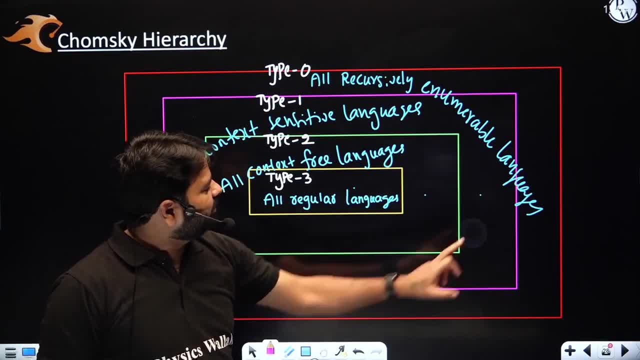 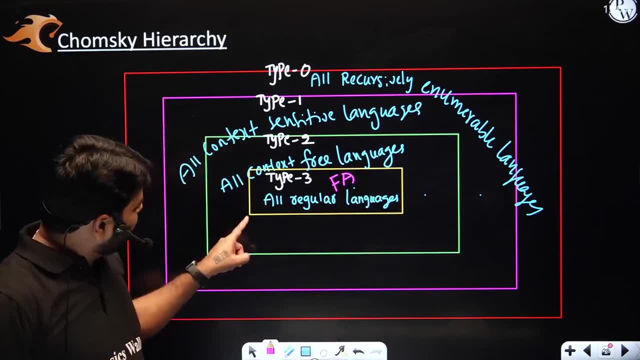 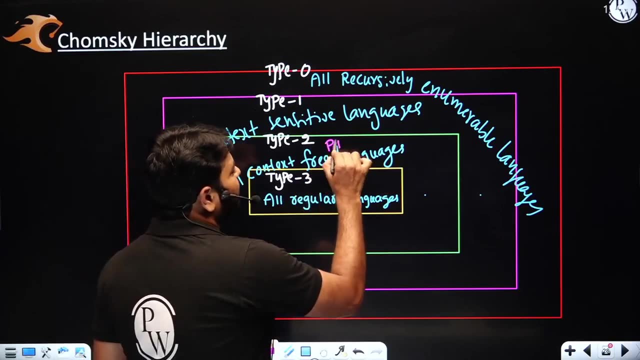 okay, so this regular languages. we have a model called as a finite automata. so anything you want to represent in these languages, you can use finite automata, or you can use pushdown automata, you can use linear bound automata or you can use turing machine. 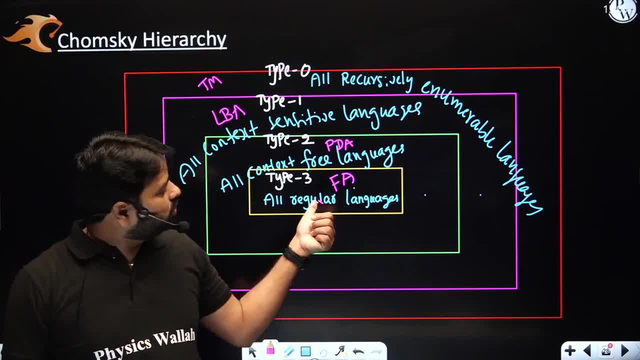 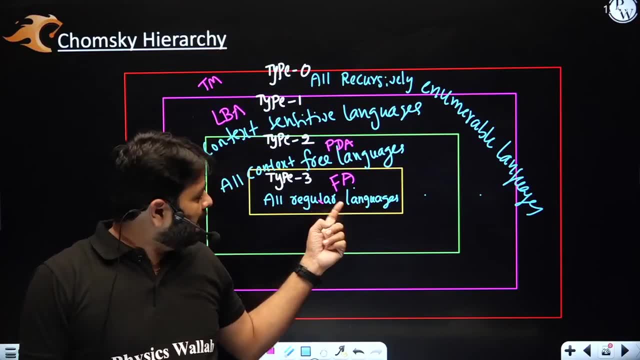 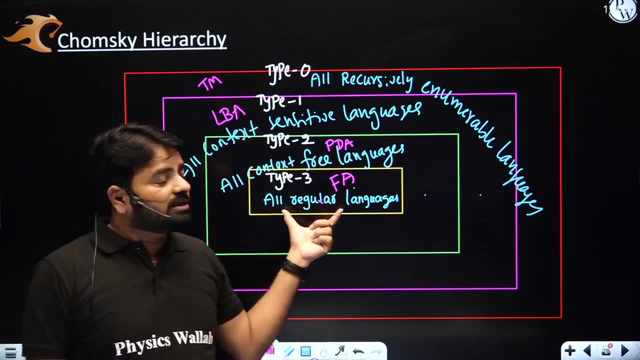 so for this language especially, you can use finite automata or pda, or lba, tm, because this language is covered in all the classes. every regular language can be accepted by finite automata, can be accepted by pda, can be accepted by lba, can be accepted by tm, because this is the 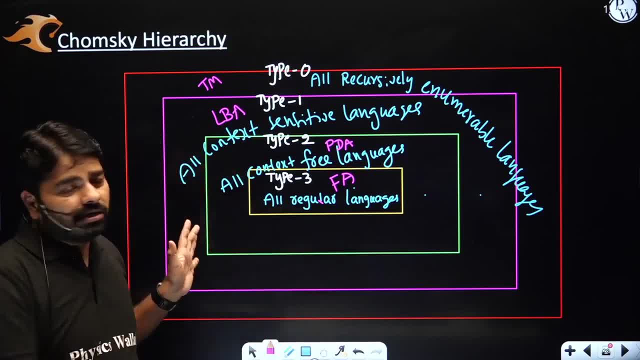 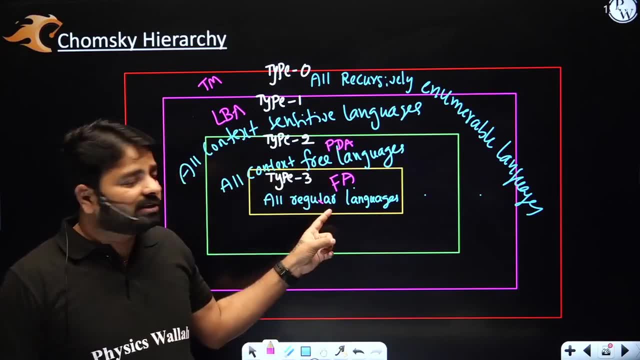 smallest class, which is included in all the classes. i hope you understood those people who are believing regular language is only possible by finite automata. that is wrong. regular language is possible by finite automata, as well as pda, lba, tm, but finite automata is equivalent to regular language because the every time you 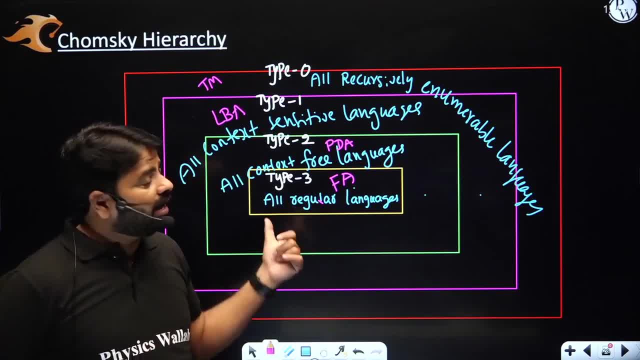 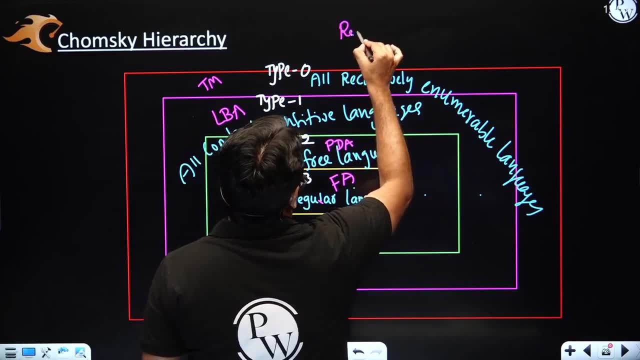 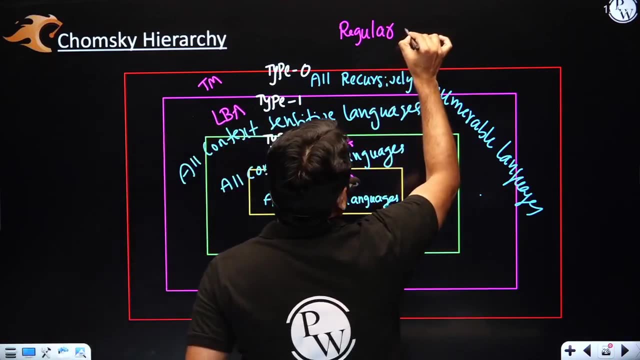 design finite automata. it only represents regular, but when you have a regular you no need to be finite. so there are two directions. remember, if i give you regular language, if i give you regular language, if i give you regular language, you can design any of this machine like i can design finite. 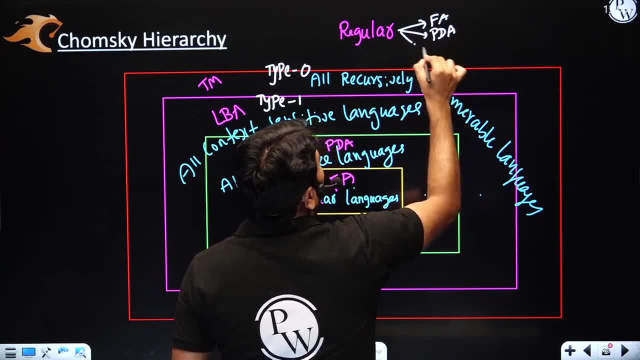 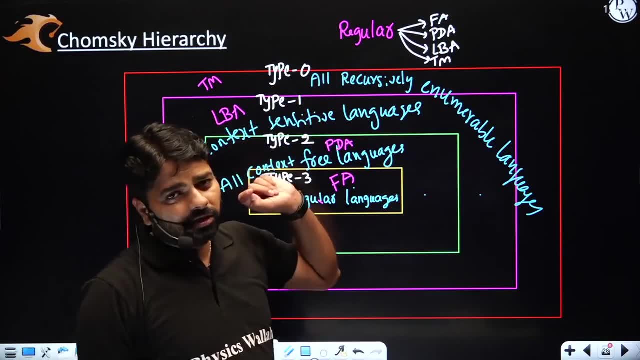 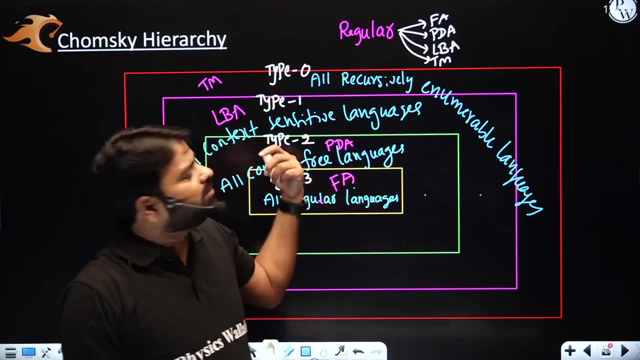 automata. i can design pda pushdown automata. i can design lba linear bound automata. i can design turing machine. if i have a regular language, but if i have a finite parameter that only represents the regular, that regular may be called as some context free or some csv, but not every cfl. so understand. 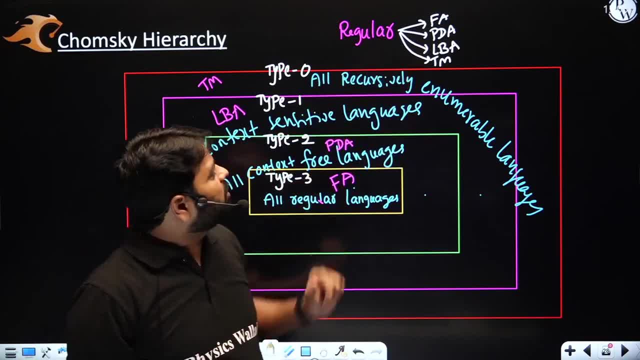 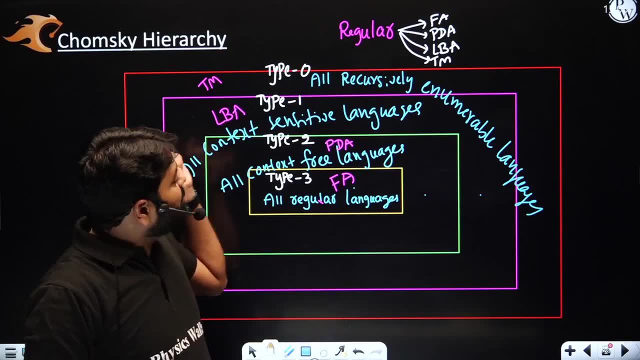 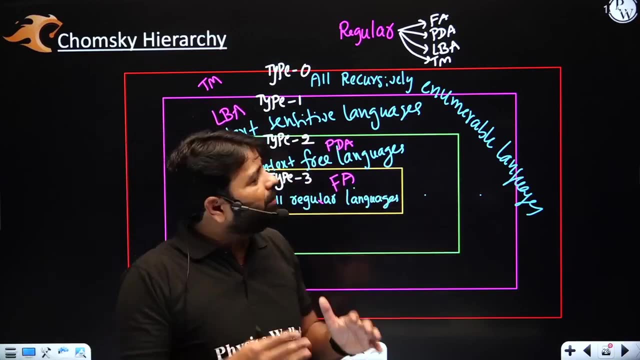 the directions how you need to interpret properly. so every regular you can design finite parameter, pda, lba, tm, but every turing machine you can't say regular, because some turing machines can do non-regular. that is what the behavior. every regular you can use any of this, but when i say tm, i can represent recursively. 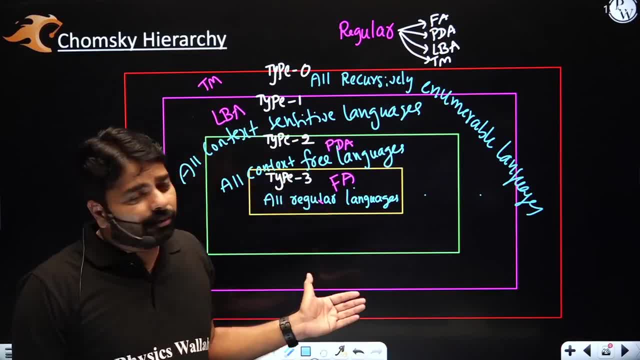 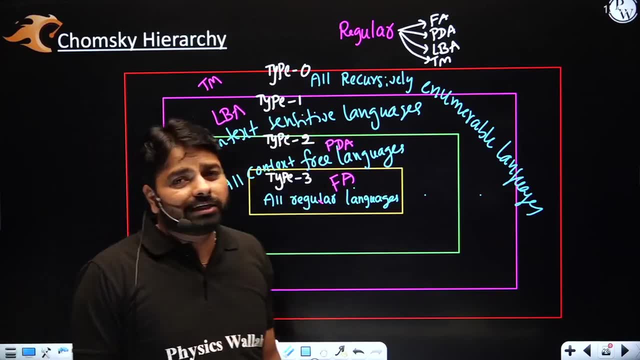 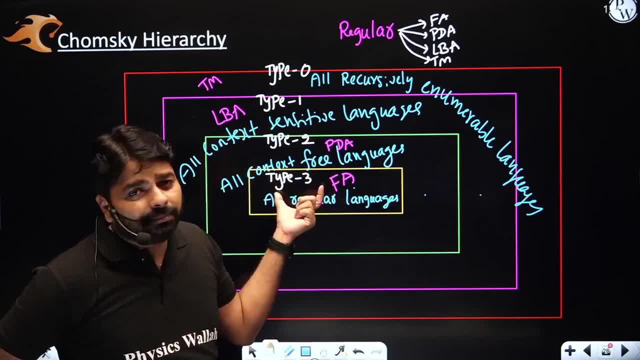 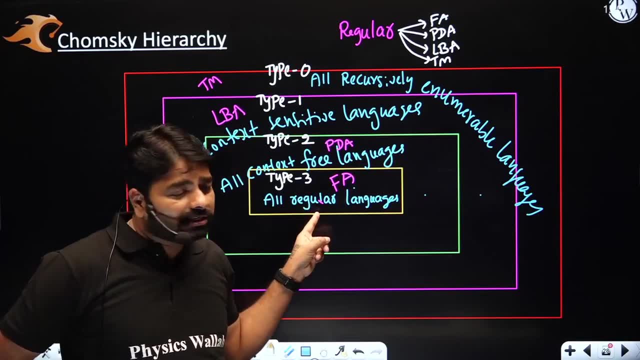 having infinite number of regular languages. if it is a type 3, if type 2 class, then you will have infinite number of context-free languages, which includes all the regular languages, no doubt because every regular language is already context free and all these relations are very important. 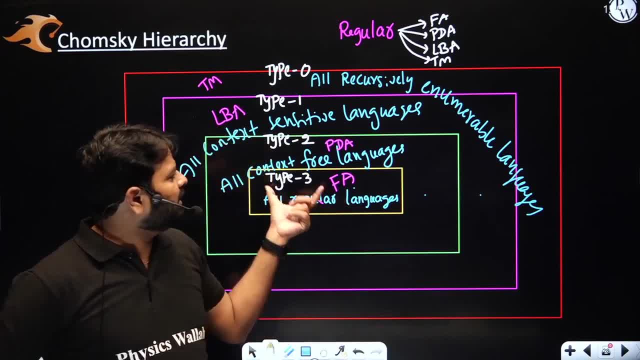 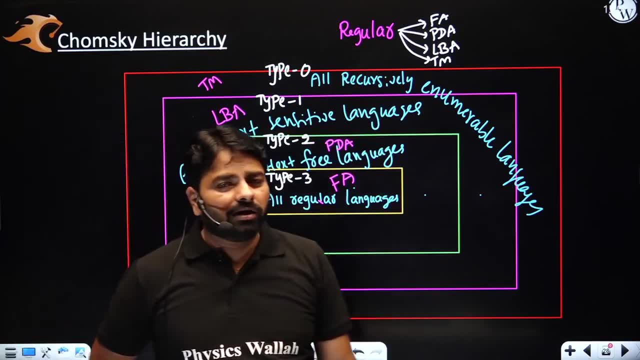 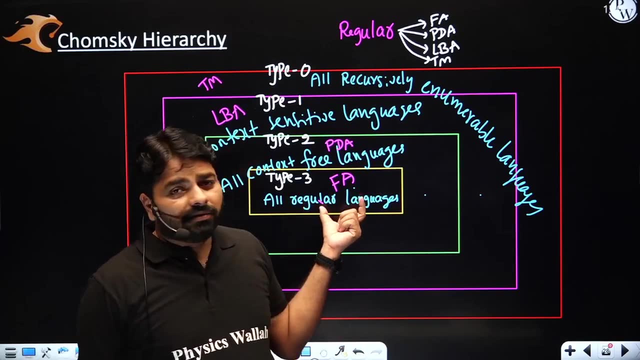 in the beginning. later on this will be our first topic, and then second topic- this box- and then third topic and fourth topic and so on we will be covering, i hope this. chomsky's hierarchy is going to talk about how the formal languages are classified to understand the various problems in the world, in the world. so that's what i told. if you are, 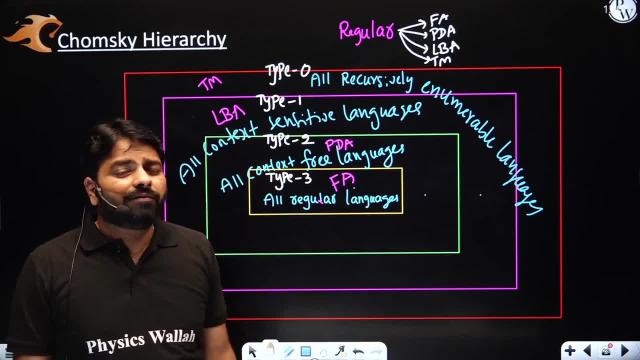 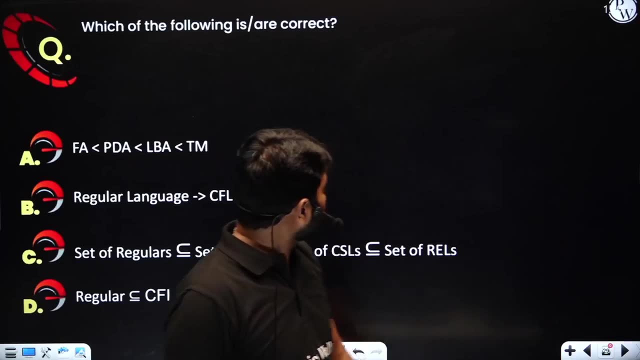 using regular languages. it can represent the problems where you do not require any additional data structure to solve. then all the problems can fit into here. so let's begin with this chapter- finite parameter and regular expression- as soon as possible. but before that let me start with some questions. okay, first question: which of the following is: are are correct, so this relations? 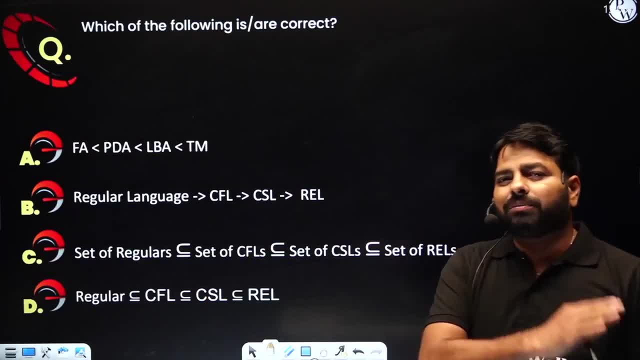 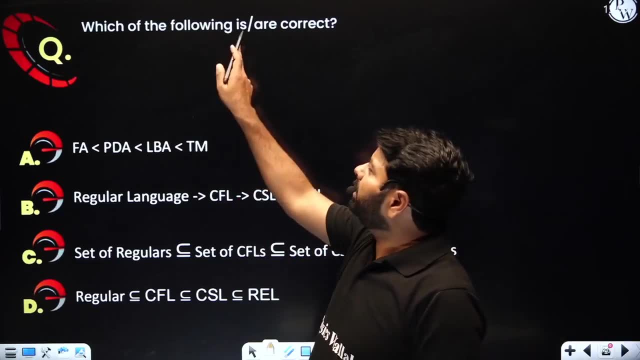 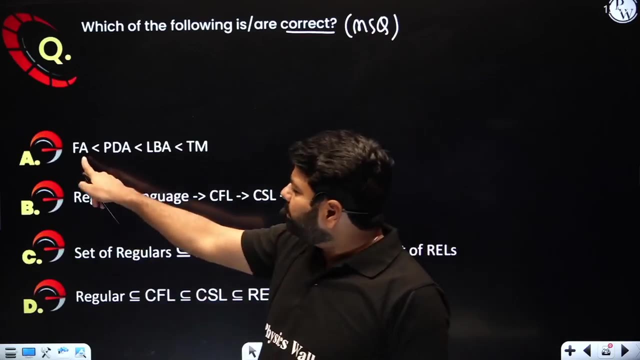 are preserved in chomsky hierarchy. if you understood chomsky hierarchy, this four points should have a clarity. which is right or which is wrong? okay, now, which of the following is are correct? so it could be msq. right, i've already. i'm mentioning it is msq, okay, what is the meaning of? 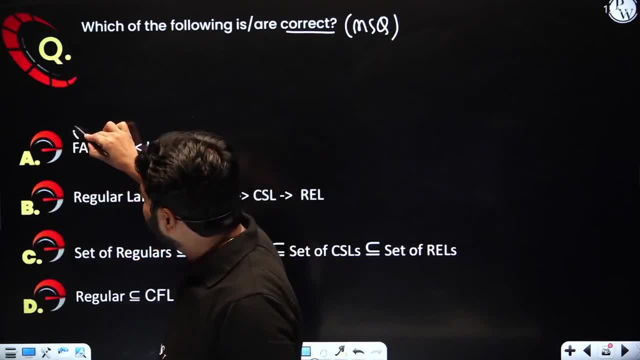 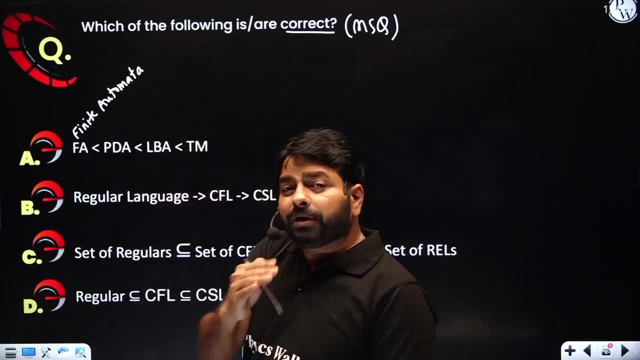 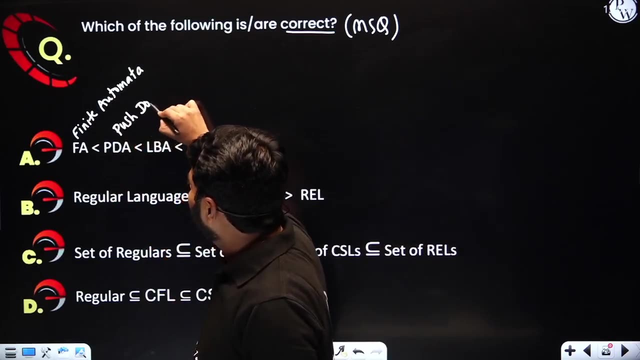 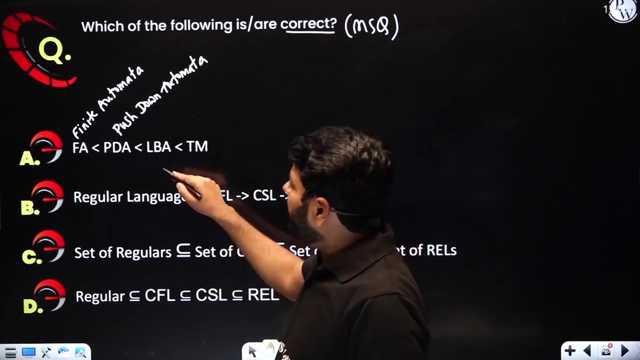 this. we have four machines right. fa means here finite automata. finite automata is used to represent- to represent the regular languages, pushdown automata. this is also a machine. we can design various pdas to represent context-free languages. we have a lot of linear bound automata. linear bound automata. 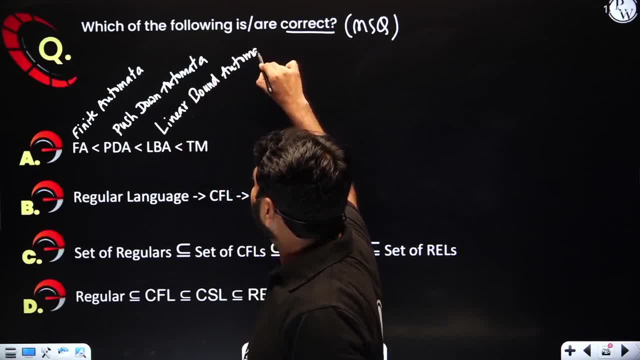 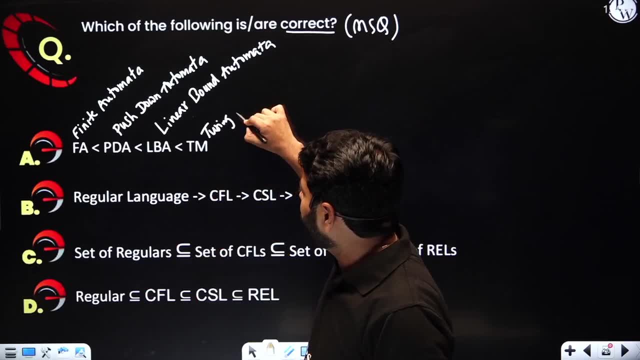 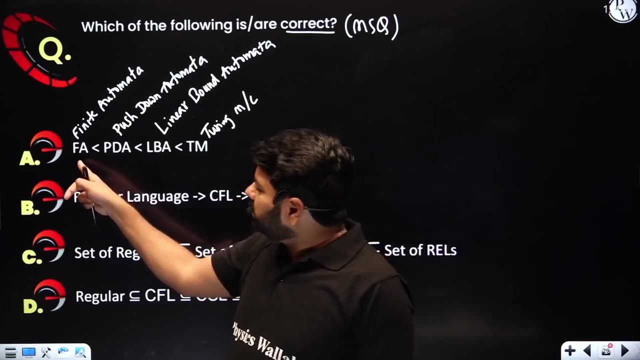 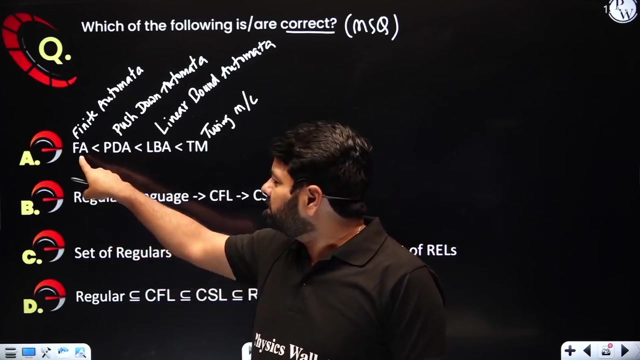 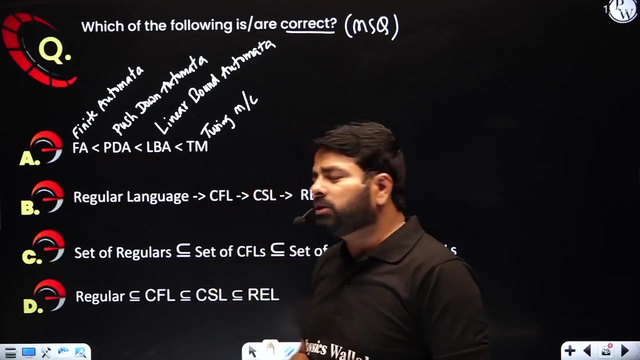 which is used to represent context-sensitive languages, turing machine, very famous in our toc turing machine to represent all the recursively enumerable languages. now this order is called as expressive power order. so what is the expressive power of the machines? the finite that can express very small class, even though you have infinite regulars, right, so that inner box, the small box, is. 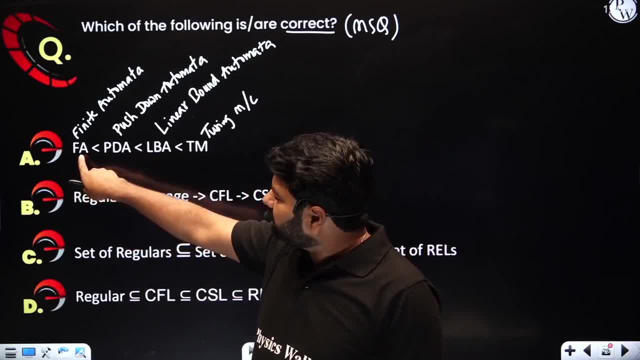 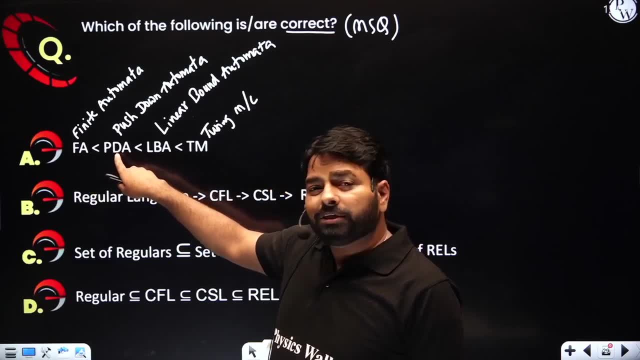 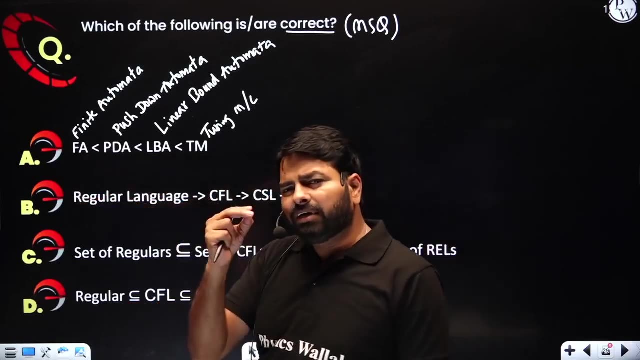 going to represent all regular languages, so rep the- all the languages are represented by finite beta- is smaller than pda expressive power, and all the languages that you represent with the pda is a smaller or subclass of lba languages. similarly so express for finite beta is having less expressive power than turing machine, so turing machine is. 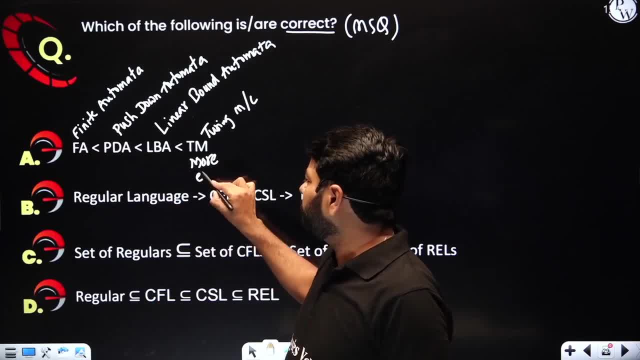 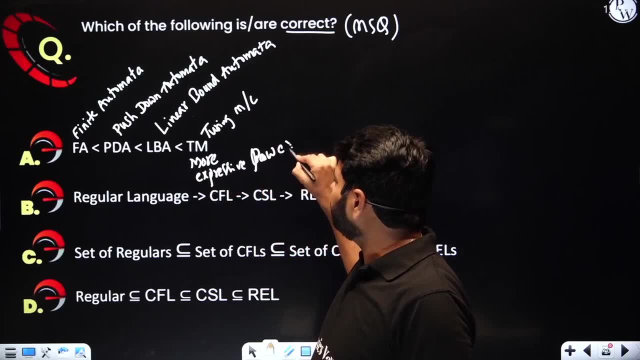 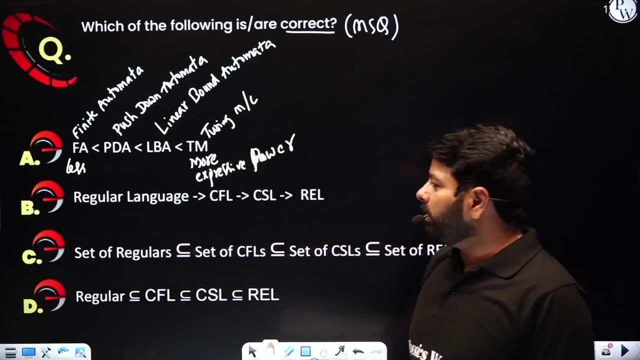 having more power, more expressive power because it can represent lot of languages. compared to any other expressive power, this one is a finite is less. okay, that's true, right, it's a correct. no doubt is correct. whatever would be regular language. oh, this arrow, you should understand mathematically. 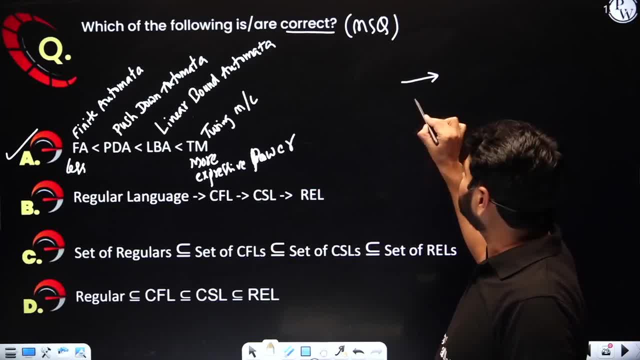 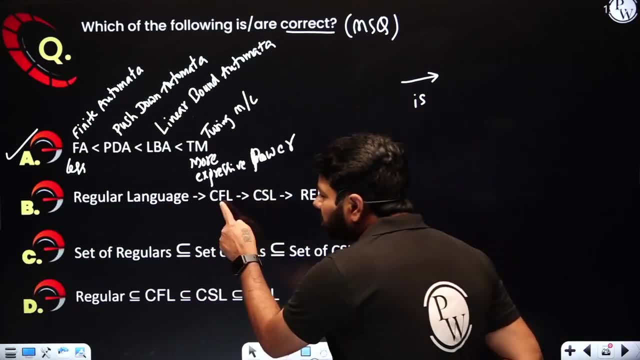 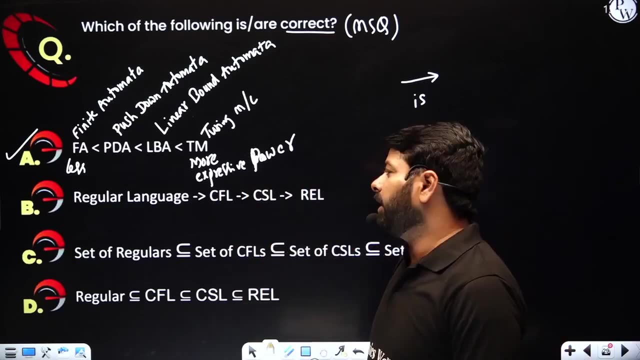 arrow basically represent implies basically represent employees or ease. can i say every regular language is context-free language? yes, every context-free language is context-sensitive language. every context-sensitive language is recursively enumerable language. okay, by transitively, regular language is also context sensitive. regular language is also recursively. 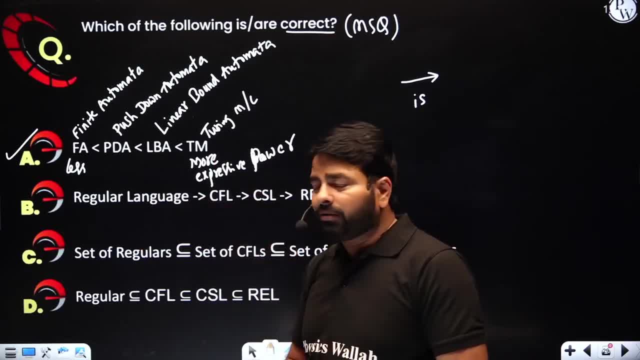 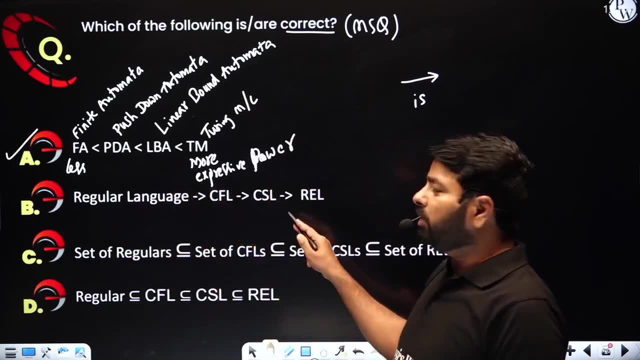 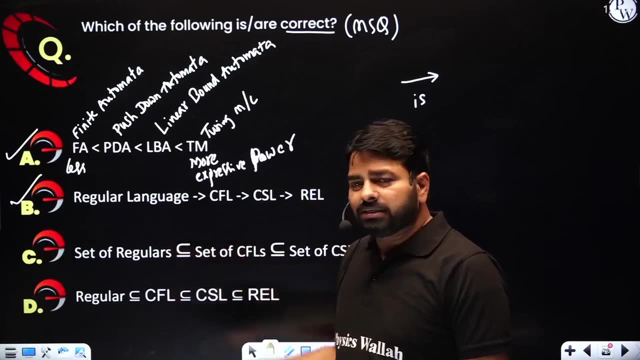 enumerable. but don't write in other direction. it will be wrong because in general that will not be correct. converse statements are wrong. so this side: regular language implies cfl implies csl employees are real, it is true. okay, now look at these two sentences. regular language means i'm. 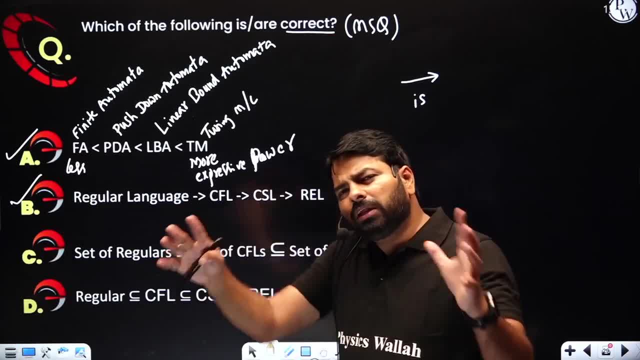 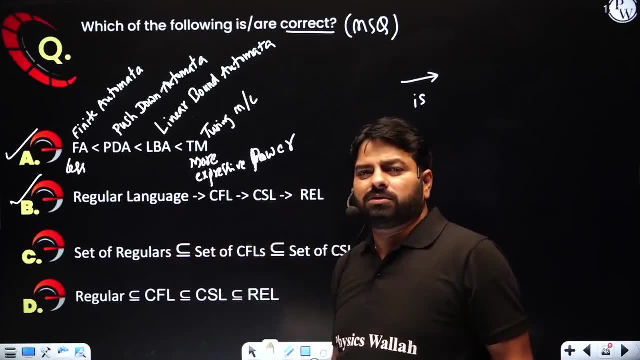 talking about one language. set of regulars means i'm talking about all the language in the class. both are different sentences. both are different sentences. it's like one person and set of persons. so this regular language is one language within the the type 3 class, but set of regulars. 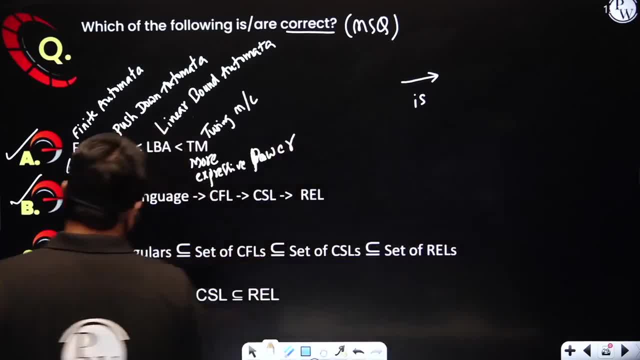 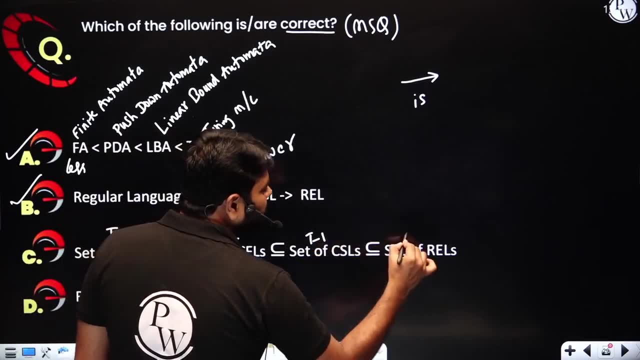 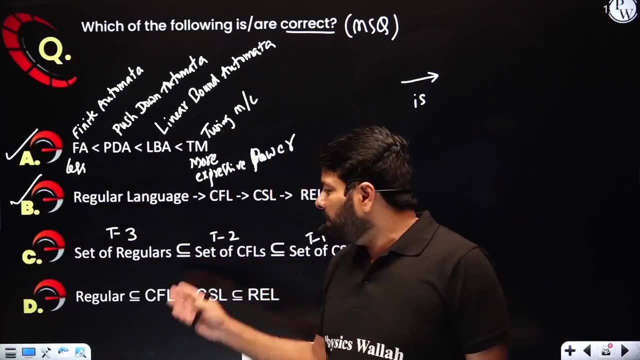 means type 3, whole class i'm talking about, so i can also represent like this: is the type 3 subset of type 2, subset of type 1 class subset of type 0? is it correct? of course it is strictly subset, we already know it. it's equal is just to denote. but it's actually. 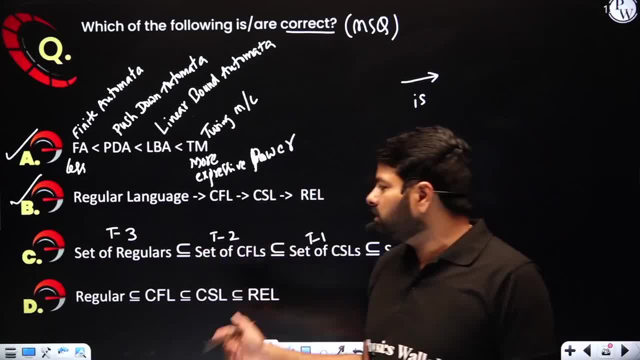 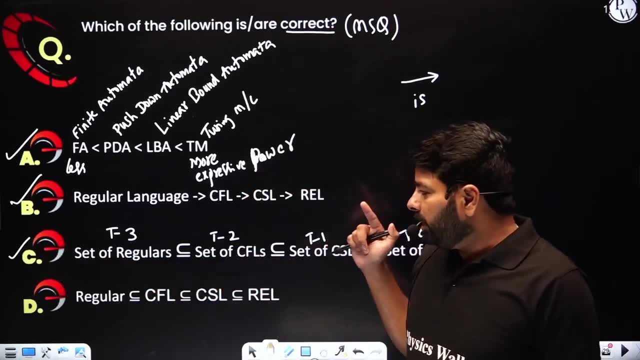 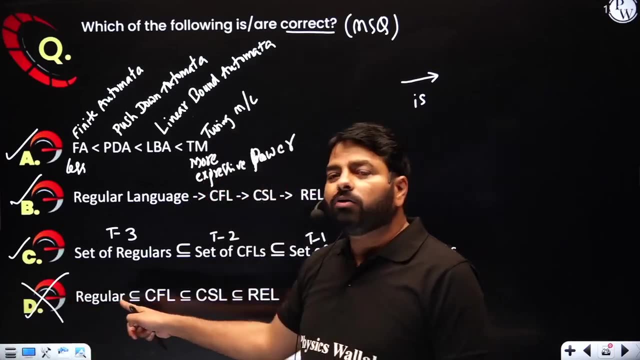 strictly subset. when it's already strictly subset, subset holds. so this is also true. okay, set of regulars is definitely subset of set of cfls. in case anybody using the sentences be careful, this is the wrong sentence. why regular need not be subset of cfl because one language, other language. 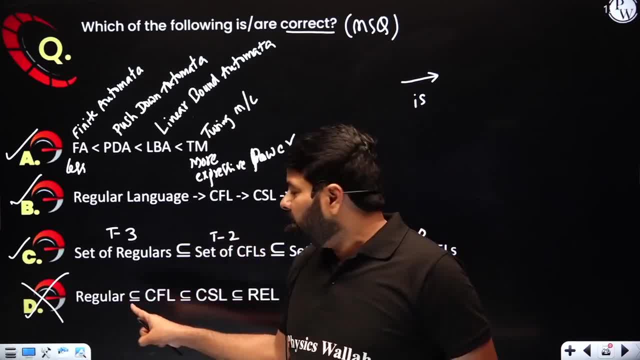 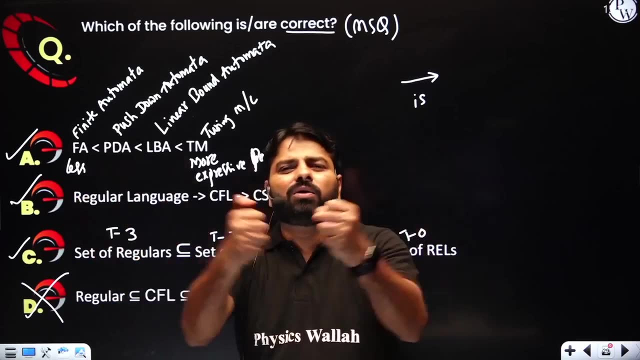 may or may not have relation. this is a very important factor. and in between these two, no relation is that's fine. there's a statement only, but regular, you cannot say it is a subset of a context free. these two languages may not have even single string relation. sometimes one regular, other, regular only, will not have a relation. forget. 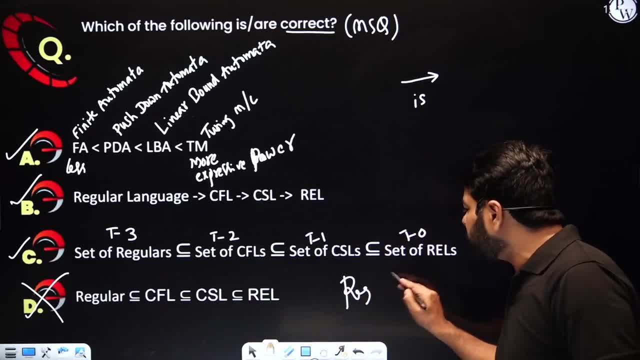 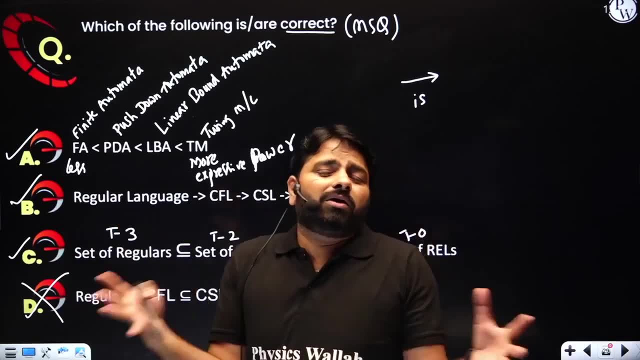 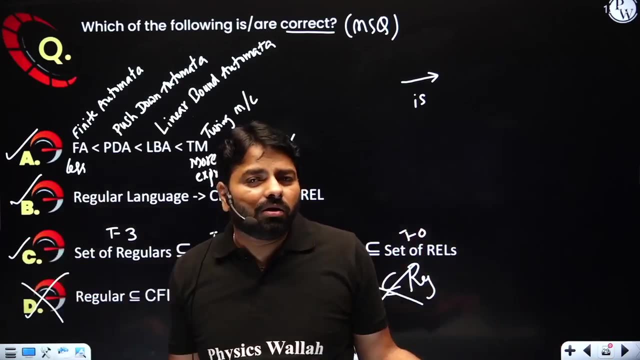 about regular and cfl. i cannot say regular subsets regular. that's also sometimes wrong. that's also sometimes wrong because one regular, other regular may not have a relation. one regular language may start, may ends with a other regular language, may ends with b when you try to relate. there is no relation at all. so understand regular, regular only some. 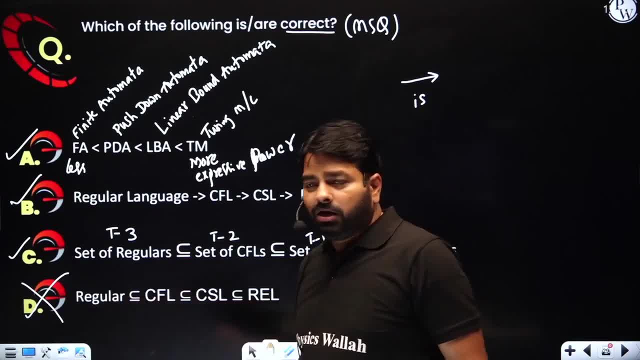 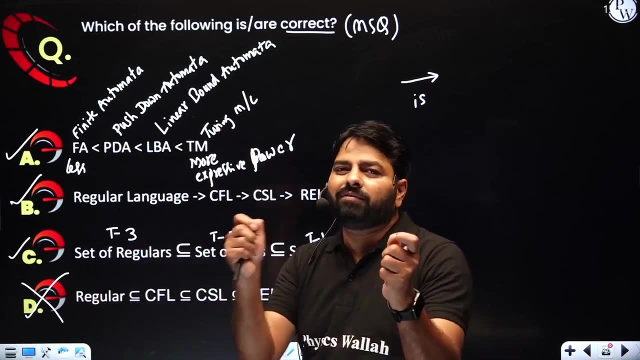 times. you may not relate sometimes, but these are in general statements. regular may or may not be subset of cfl, but the set of regulars means all the regulars. when you consider it is definitely inside all cfls but you take one regular from here. one cfl from here may not have a relation. 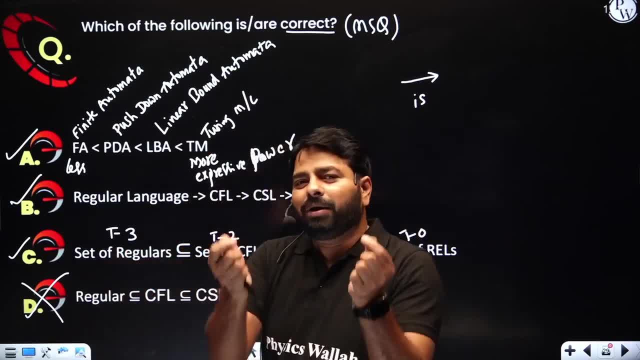 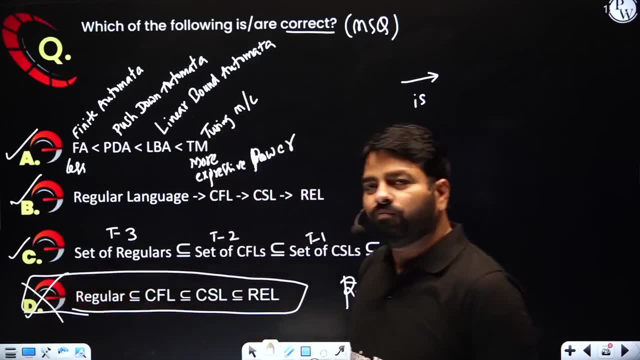 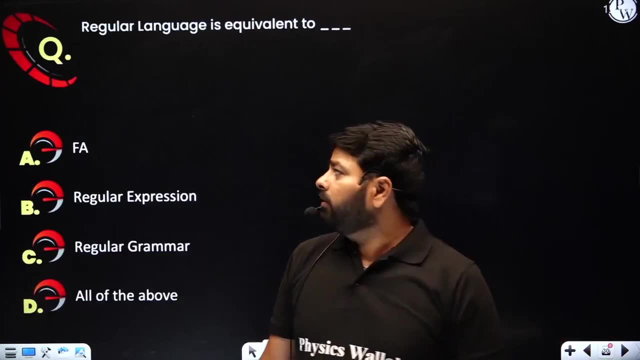 forget about others. take two languages from here only may not have a relation. okay, so this is very important. factor d is wrong statement to form. can you hope that you have understood this part? okay? the first three statements are correct now regular language is equivalent. you can't say context free language because context free. 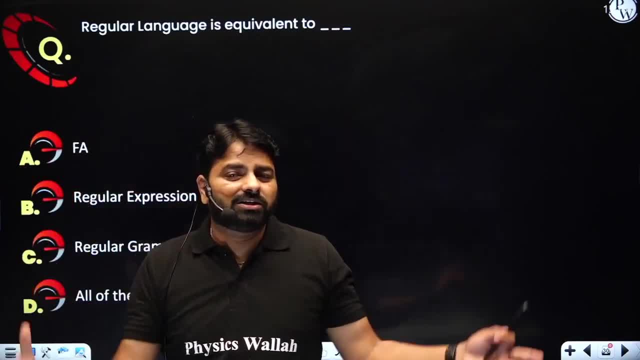 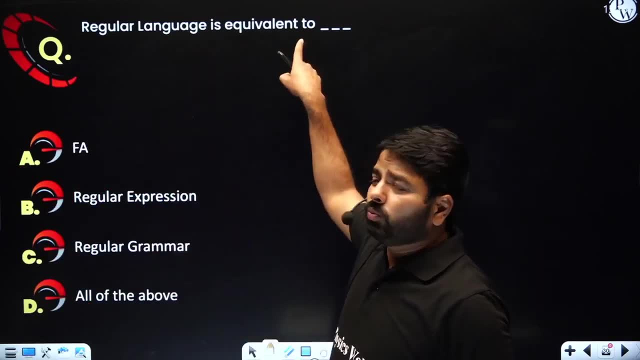 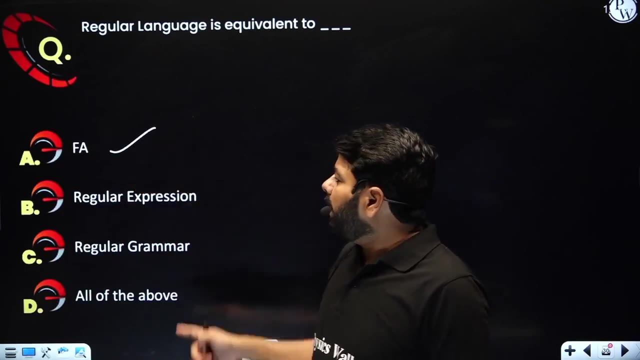 language could be non-regular also because the context free languages could be present within the type 3 class or within the type 2 class. now, regular language is equivalent to who is there to represent the regular language. one machine is a finite automata. that's true, and we have regular. 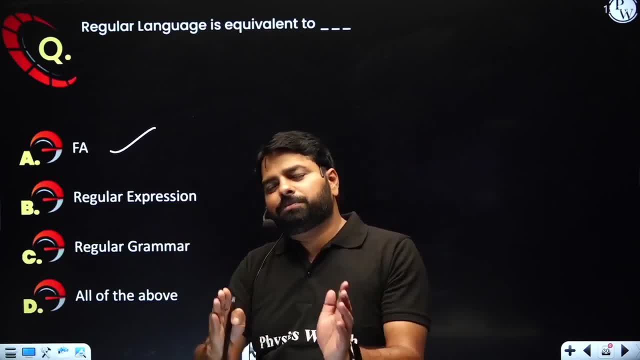 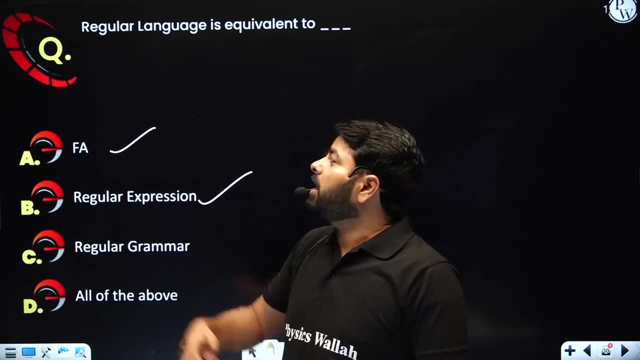 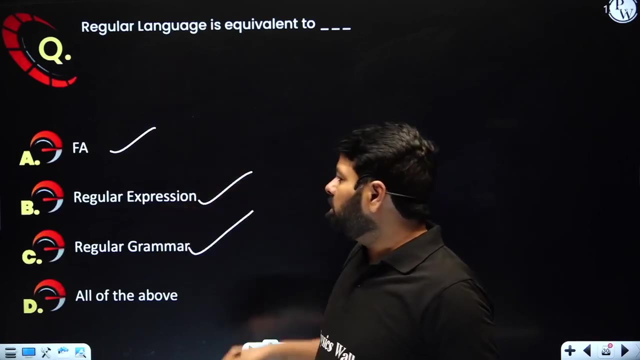 expression too. that's what we are going to learn in the first topic: regular expression and finite automata. so regular expression is another way to represent a regular language. if i have a regular expression, i can always represent a regular language. if i have a regular language, i can always represent, with a regular expression, regular grammar. so all these are 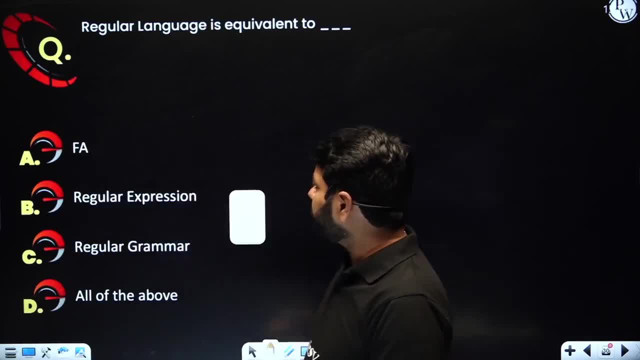 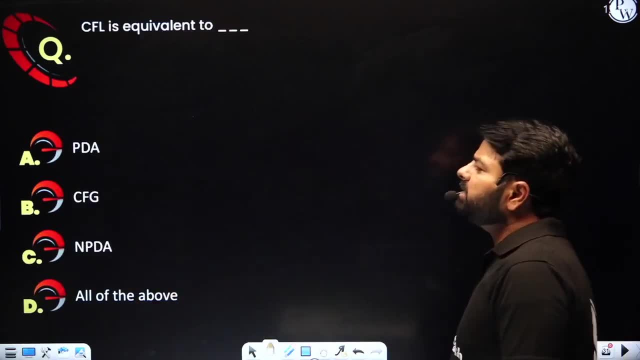 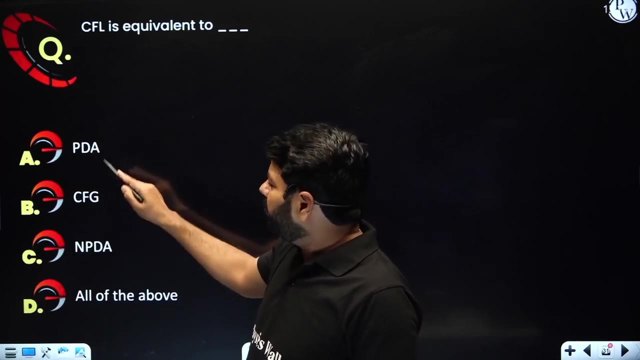 correct. so you can choose option d, correct. so this is how you can answer the questions: cfl, context, context-free language to represent this language. what are the various models you have? pda, context free grammar, npda. so what is this npda? that's what we learn in the later on in pushdown automata. 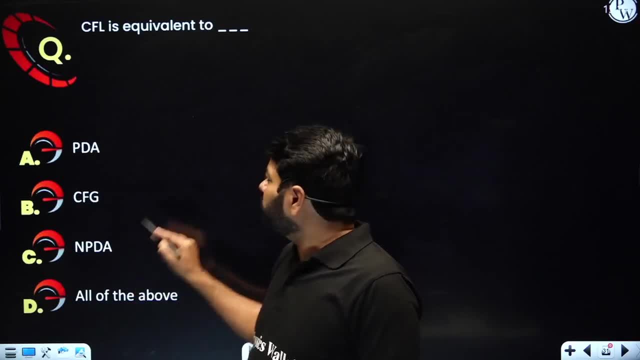 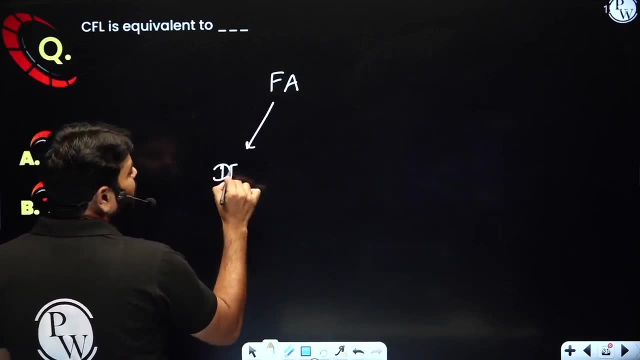 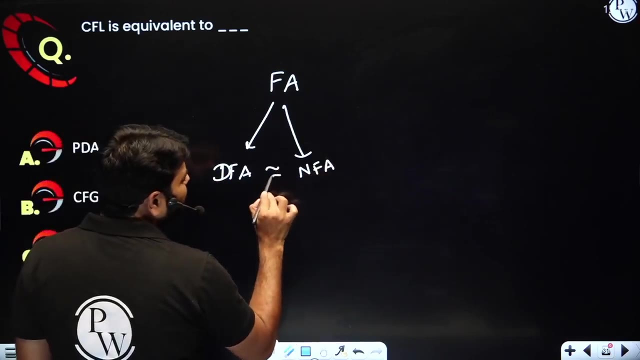 topic: pushdown automata by default- npda. so there are two types of pdas, like you know. if you talk about finite automata, let me write it. you have deterministic motion and you have non-deterministic motion. but do you really really need now? no, just i'm saying these two are equivalent because you 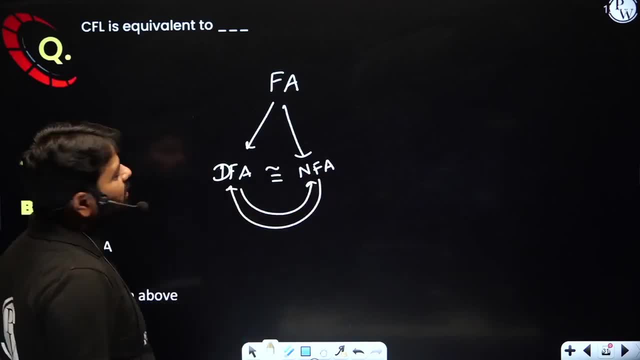 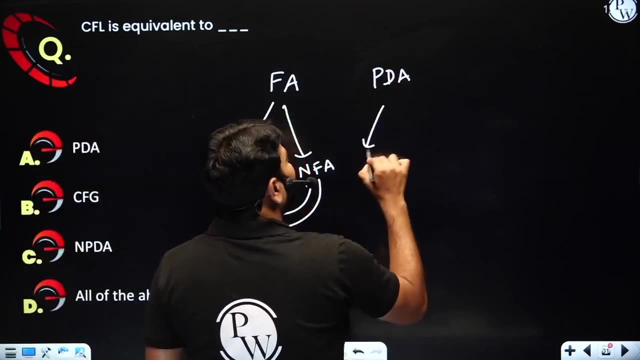 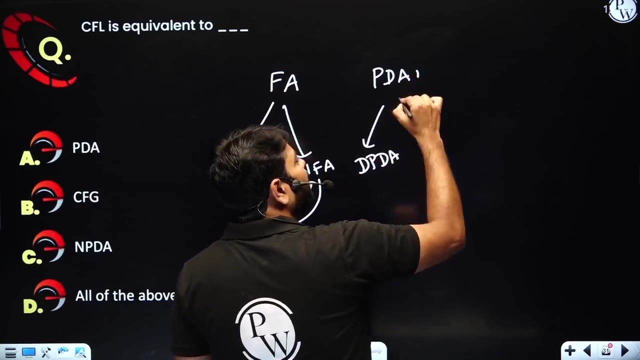 can convert one to other other to this. that's fine. that's why dfa and fa are equivalent in the finite automata. but when it comes to pushdown automata we have dpda, which is less restrictive than pda. here this pda only also called as npda. it's not another type, so here pda by default, npda. 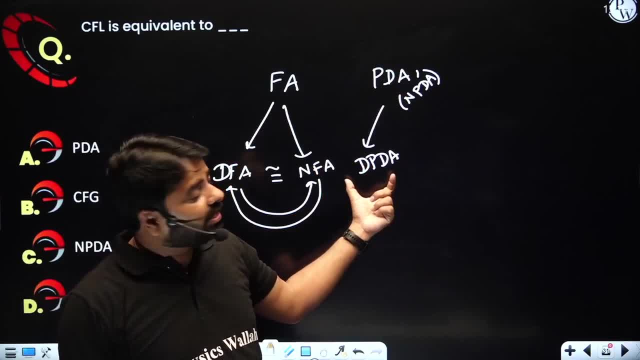 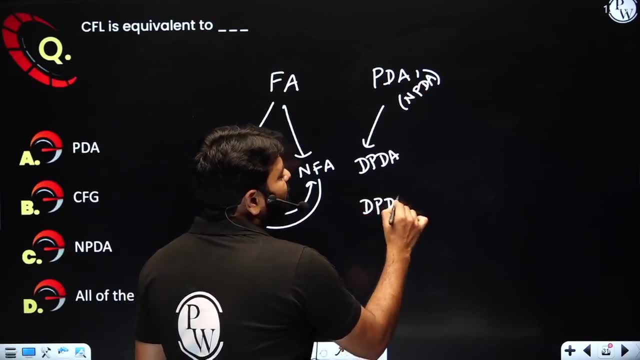 is a non-deterministic motion, but when it comes to pushdown automata, we have dpda, which is less powerful than pda, and you can also design dpda, which is restricted, a restricted format than npda and dpda here not equivalent to this one. here dpda is less powerful than npda, whereas dfa and fa. 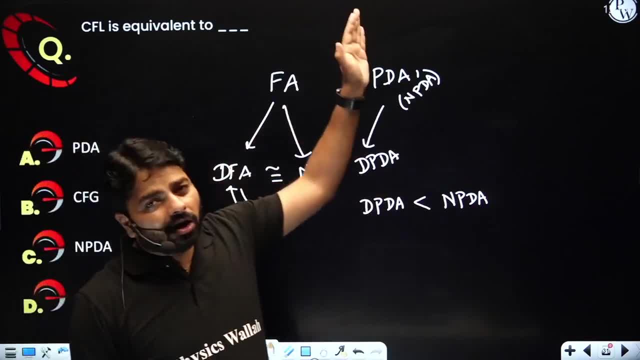 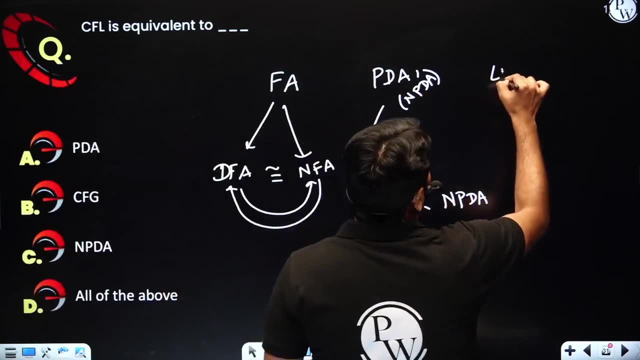 they are equivalent. so this is very important. pda also called as non-deterministic pda. pda also called as non-deterministic pda. and when you go for others like lba, you know relation is not known as non-deterministic pda. and when you go for others, like lba, you know relation is not known. 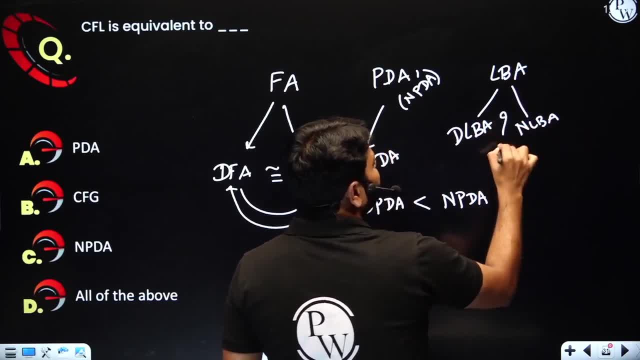 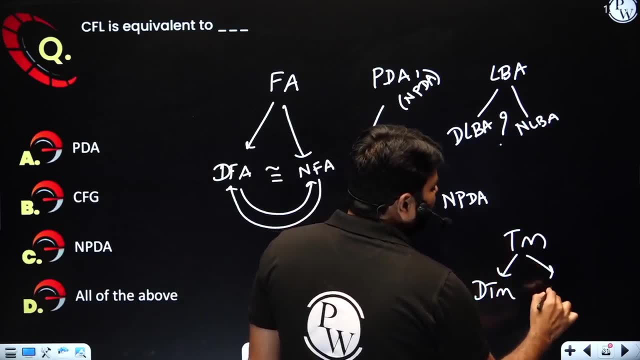 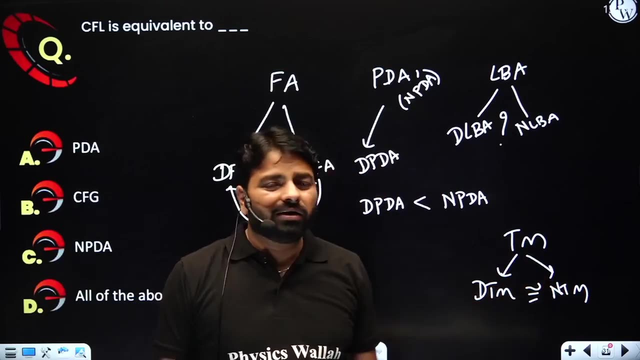 at non-deterministic lba. we don't know the relation at and turing motion. we have two types dtm: deterministic turing motion, non-deterministic turing motion. they are equivalent. again, you can convert one deterministic turing motion to non-deterministic turing motion or ntm to dtm. 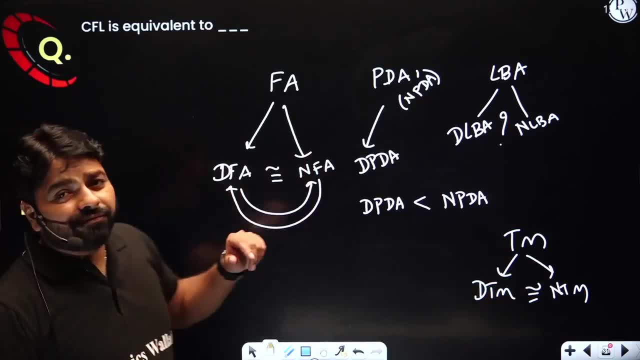 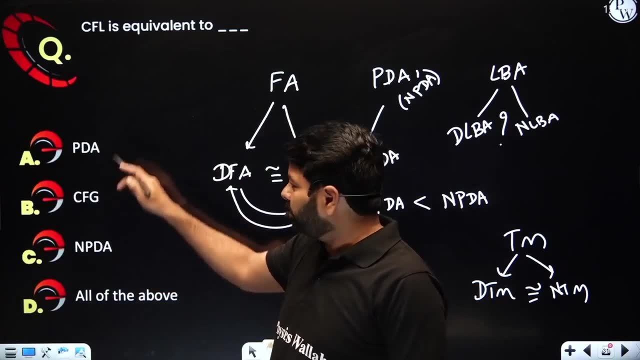 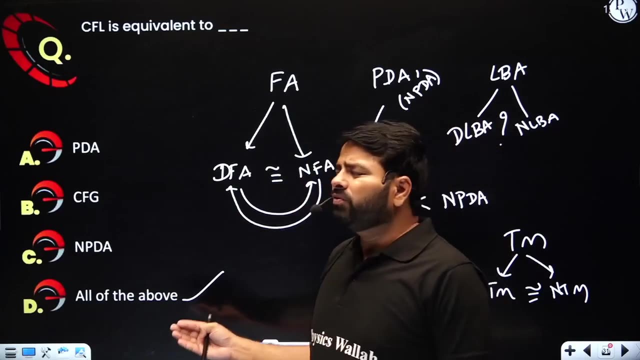 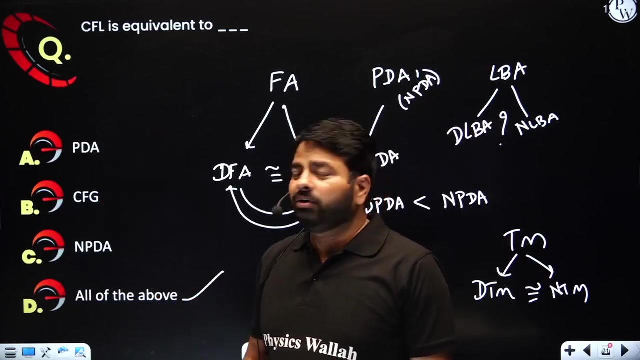 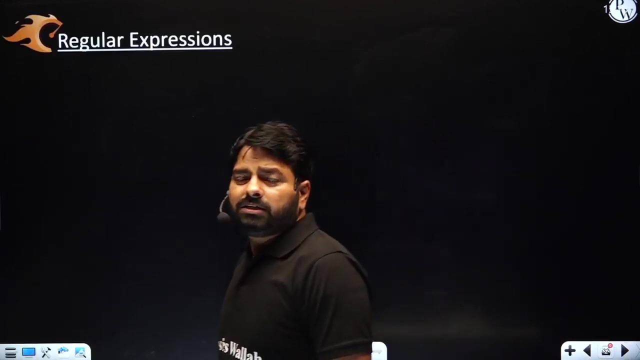 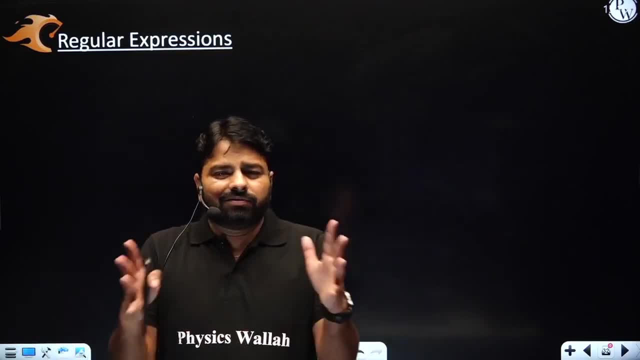 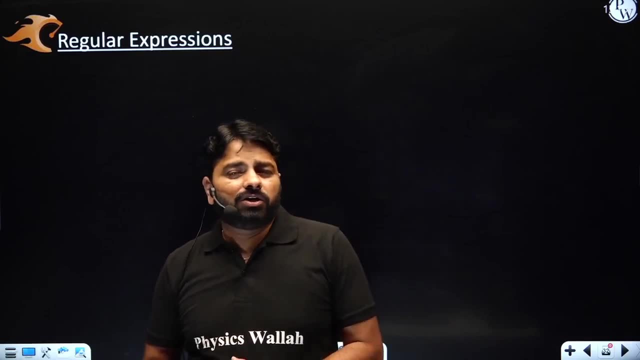 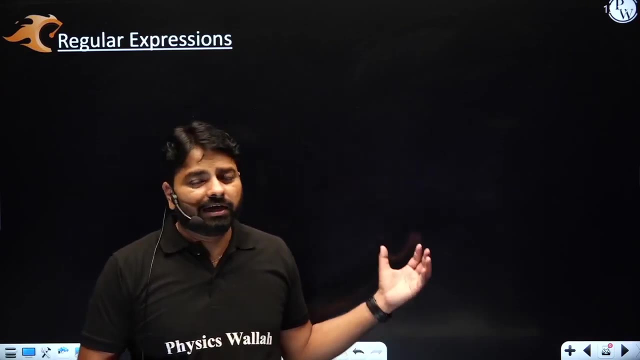 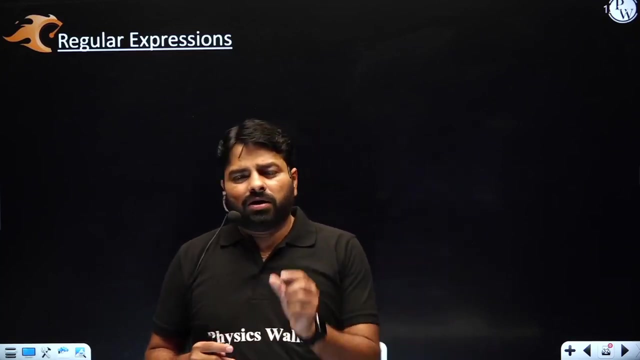 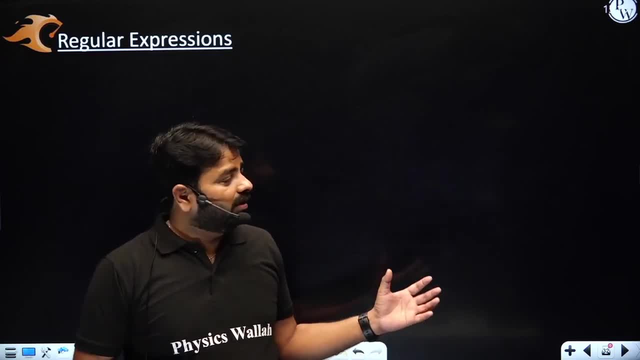 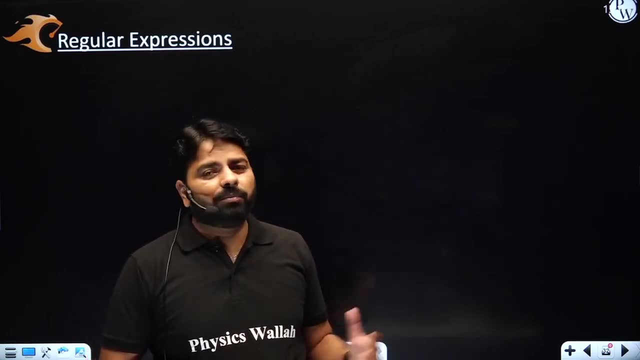 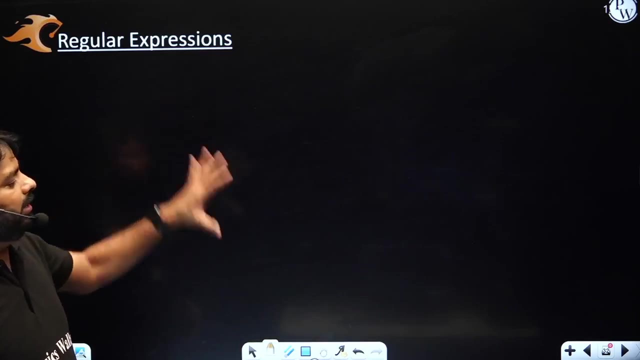 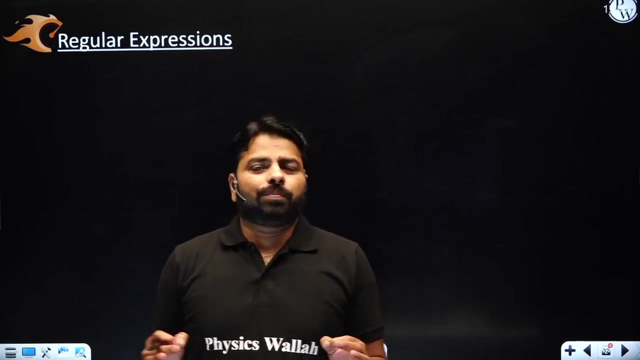 without you know any delay. so be prepare and ask doubts. if you have any from this video or any point which is related to the video, i'll be happy to help you. okay, in the next regular expressions. now we will see the regular expressions. you know, it is the first topic so far, what we have. 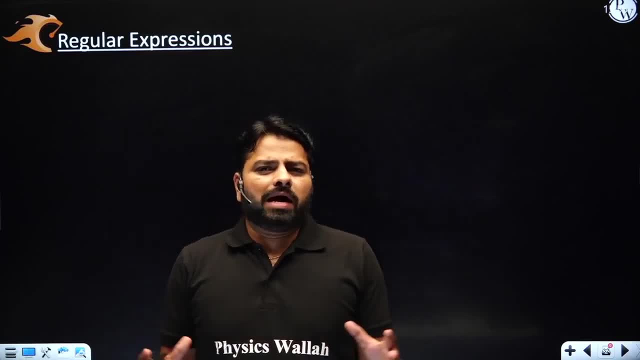 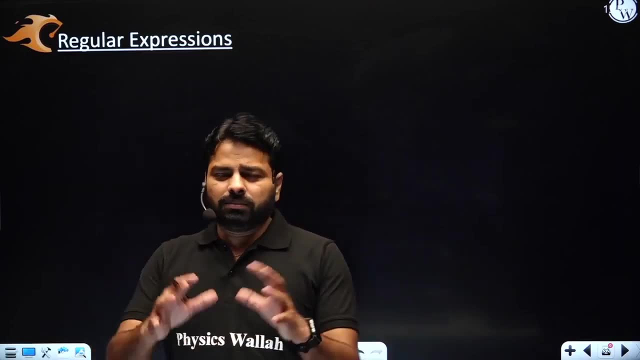 learned. it is just basics. some people who are having the basics, they can directly start from this topic. if you already know about the strings languages and the chomsky hierarchy, directly begin with the regular expression, then start practicing it and, as i told, whenever you have any doubt, just 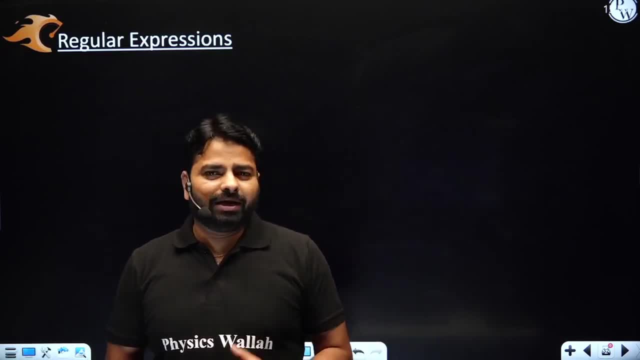 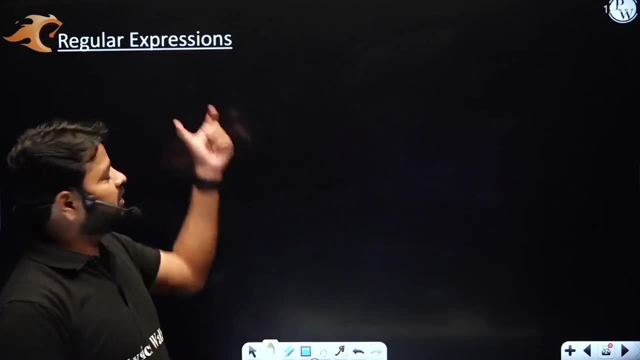 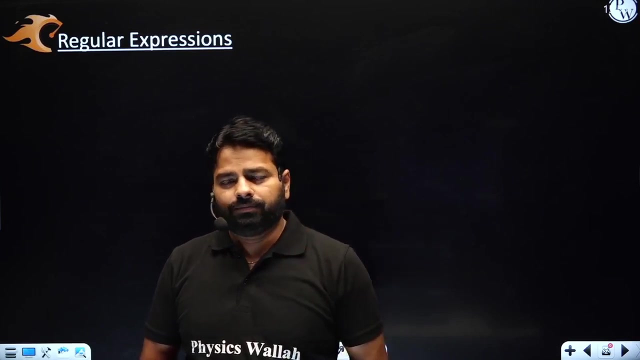 it is your responsibility to ask the doubts and my responsibility is to clear your doubts. let's begin with this topic: regular expressions. whenever you see expressions, you will see operators and operands. so we have here operators and operands. what kind of operators we have and how do we deal with them? that is the first step you should learn. then you will know how to. 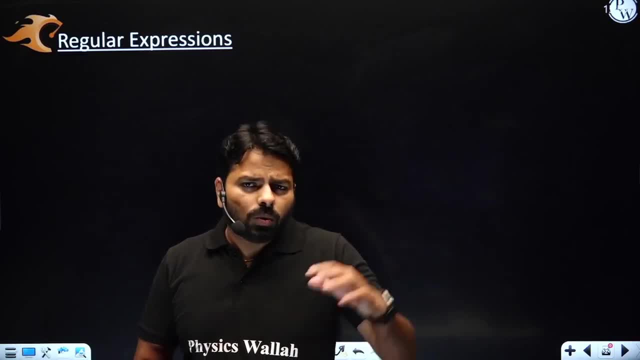 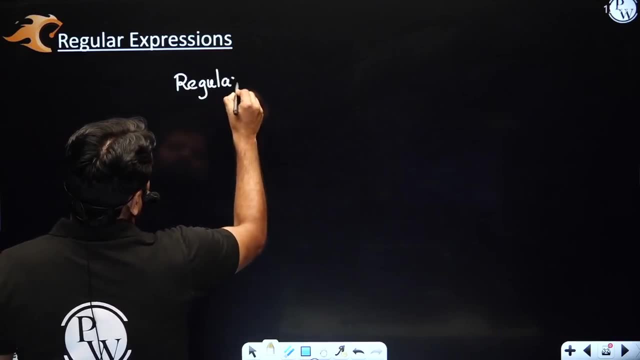 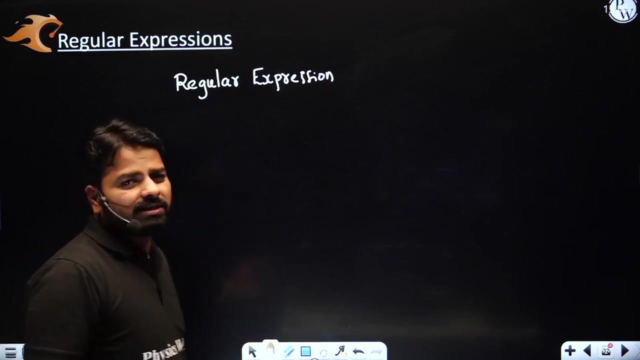 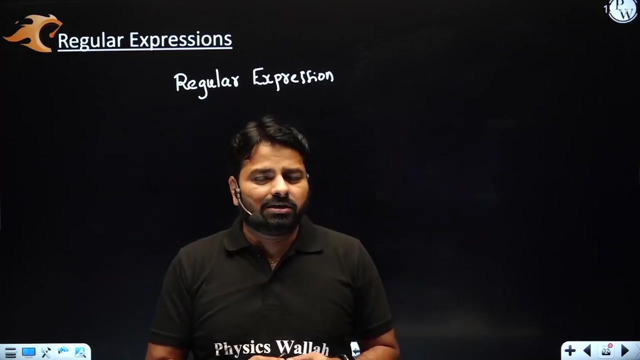 use the regular expressions or how to write the regular expressions. so what is the regular expression? regular expression is used to represent a regular language. if i have a regular expression, i can say that it represents some regular language. in that type 3 class there are infinite regular languages, so you can write. 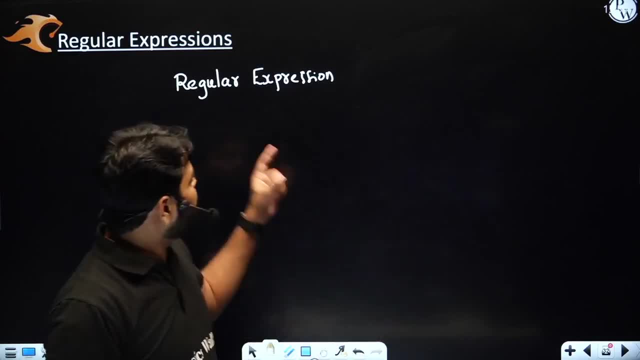 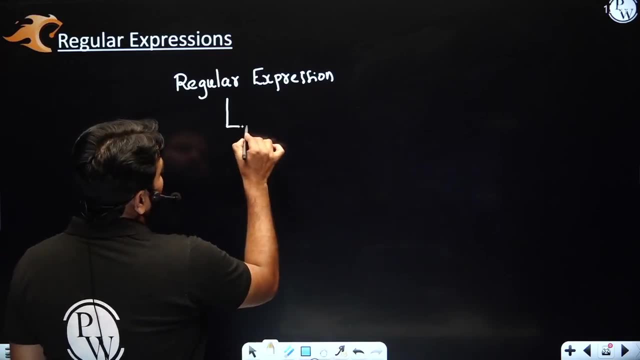 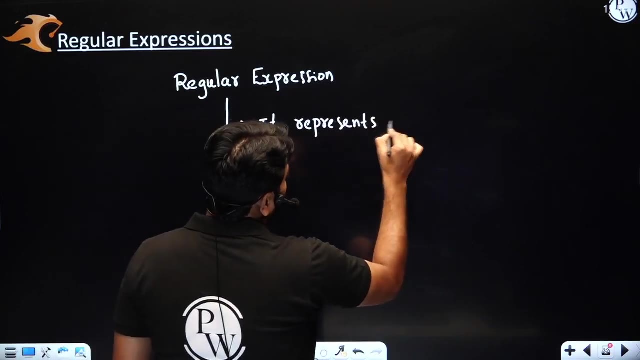 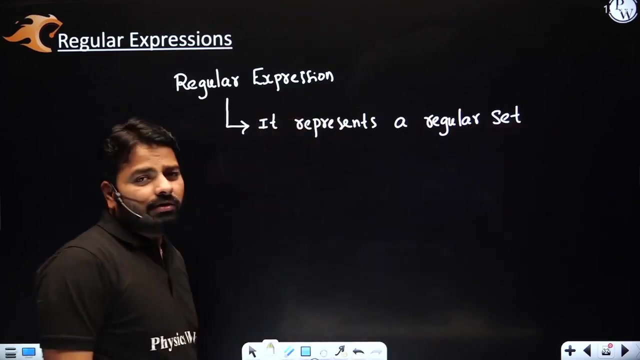 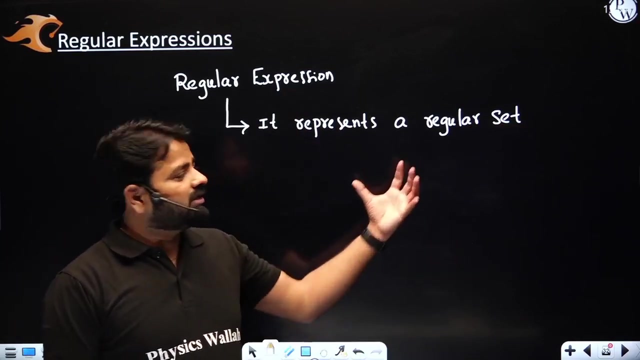 infinite regular expressions too, and if i have a regular expression then definitely it represents a regular language. so regular expression, it helps us to represent a regular language, a regular set. so how it represents using the operators, it has some declarative way that represents a regular set. so how to declare those operators? now we have four operators. 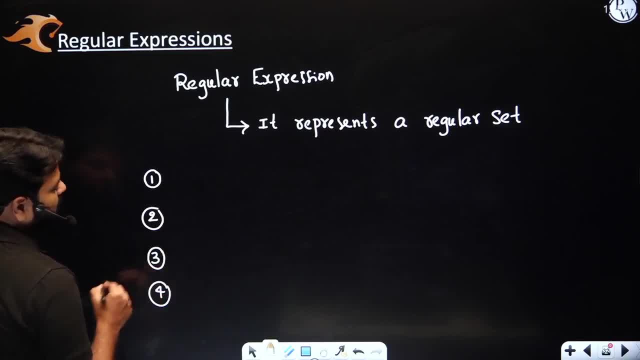 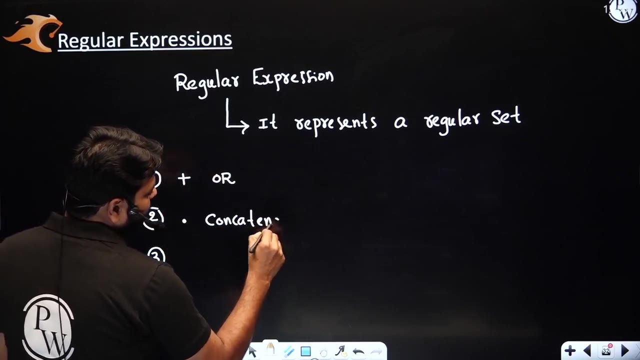 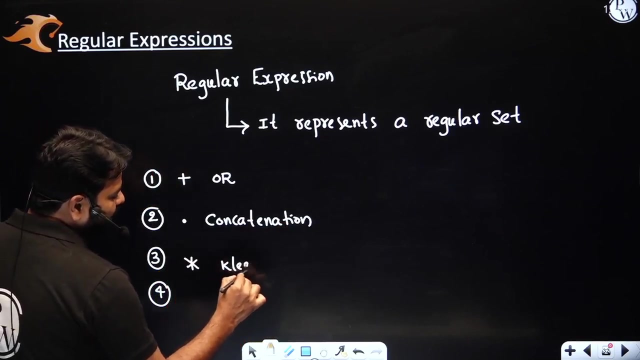 you can also say three, but i classified four as i have the two operators separately, like clinic closure and positive closure. one is the plus, which is called as r, and second is a concatenation, and other two are similar mostly. one is the clinic closure or clean star. 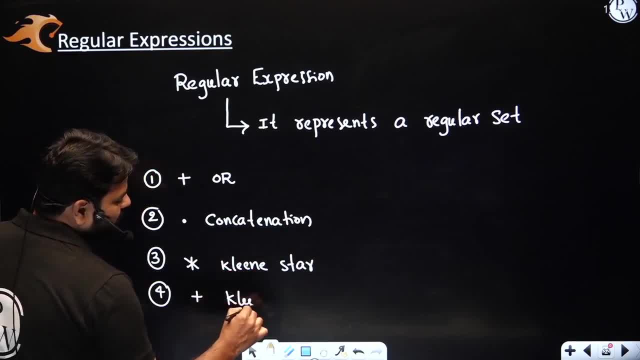 other one is clinic plus. again, do not confuse with the one and four, even though the plus is used in both the places, but their meaning is different. this plus is binary, this plus is unary, and the way we use both are different. the one and two are binary operators. three and four are unary operators. 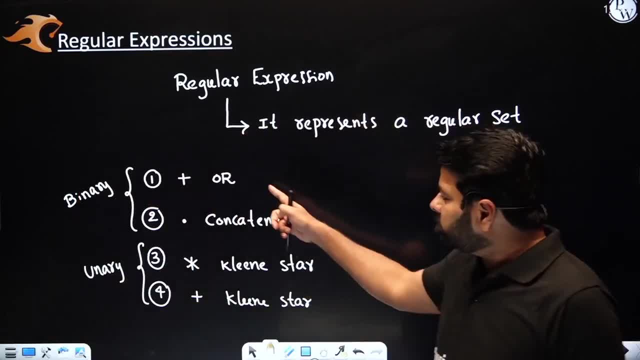 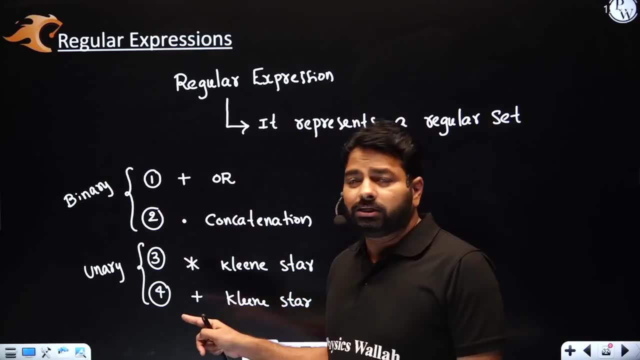 so how to use them, as i told, without learning this operators. if you try to write an expression, definitely you may fail in certain situations. so i also give you some examples of how to deliver an. always recommend to learn these properties of the operators. then you start writing the expressions. 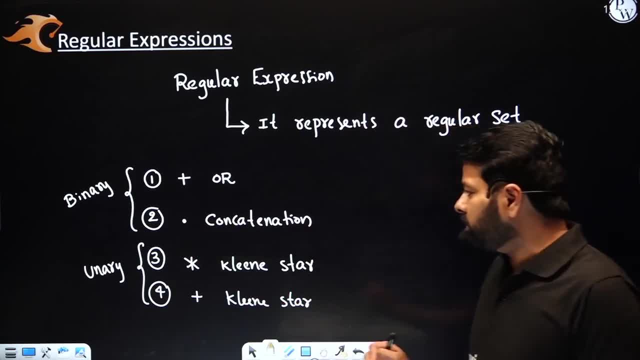 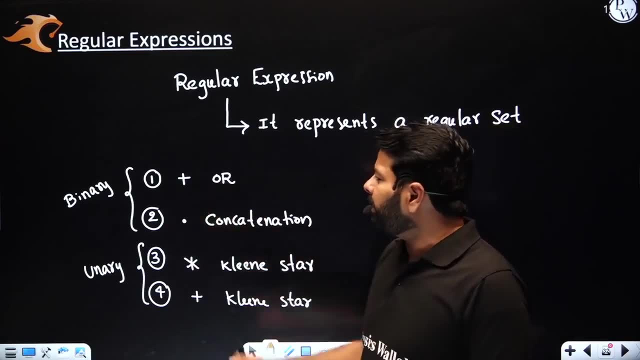 then you will get to know how to write an expressions and how to understand them. or, as i told, it's a binary operator, so you should have the two operands to represent this operator with the help of this operator. so one: if i say r1 is some expression, r2 is some other expression, 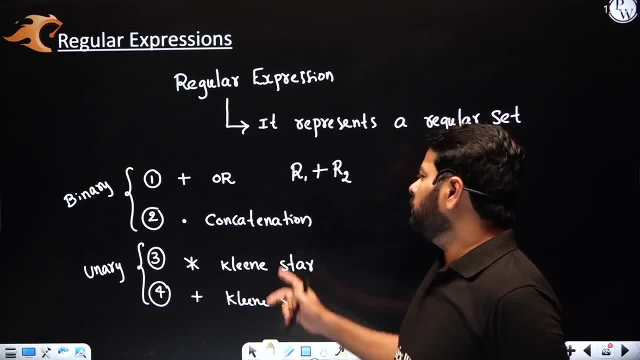 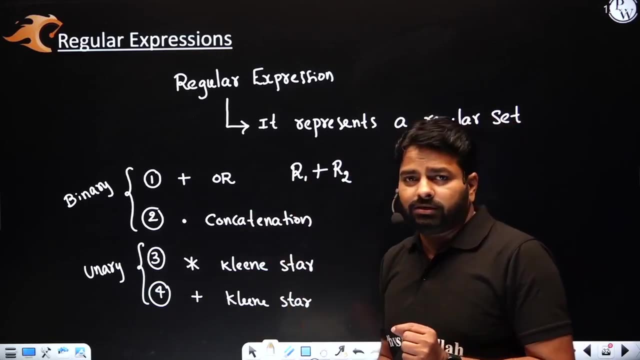 you can use the plus in between to denote r2. use this plus now if you want. denote the expression with the help of plus, you can write r1 plus r2. that what is the meaning of this? r1 plus r2 is either r1 or r2, but r1, r2 together you can't generate. you can generate r1 or r2 if you want. 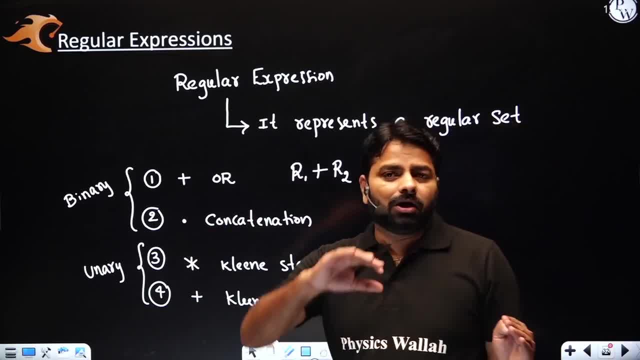 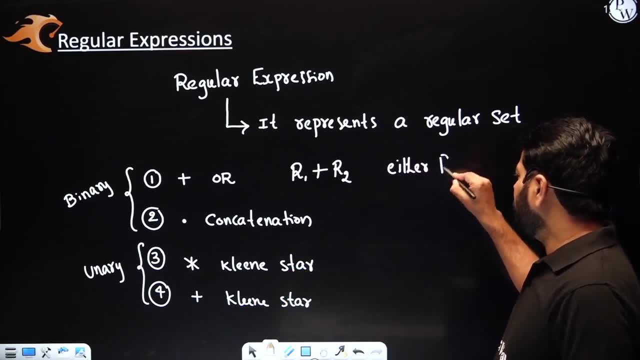 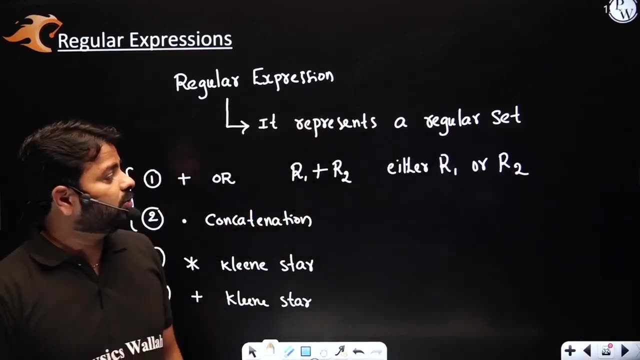 to represent the language, then that r1 will be there separately. r2 will be there separately. then what is the meaning of that? either r1 or r2. you can generate r1 as well as r2, but not together now, but not together, we'll see with. 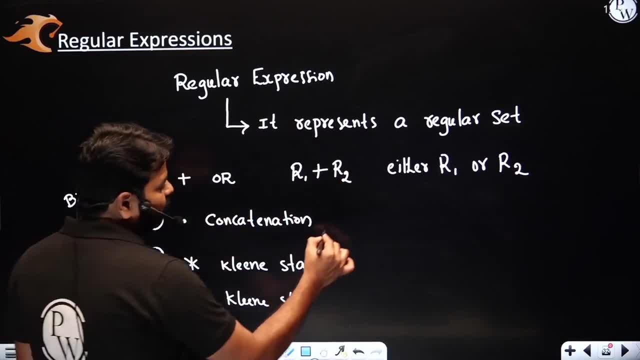 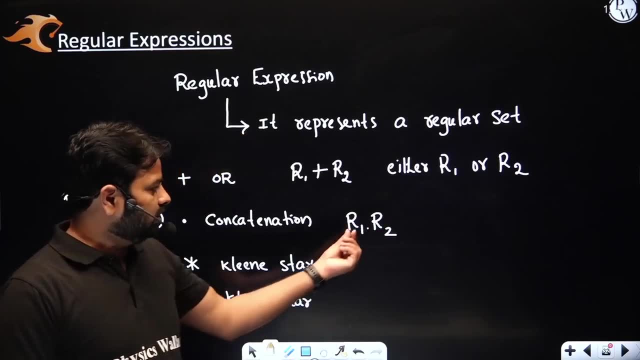 an example soon. and what is concatenation? if you want to write it- r1 followed by r2, either you may represent dot or you can omit it. dot is not compulsory to write. it means that r1 followed by r2, that followed by, you can represent with the dot. 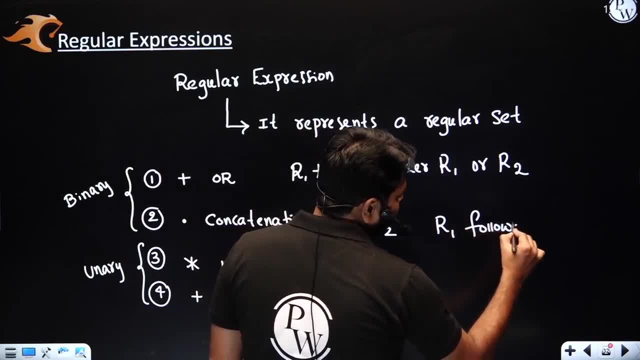 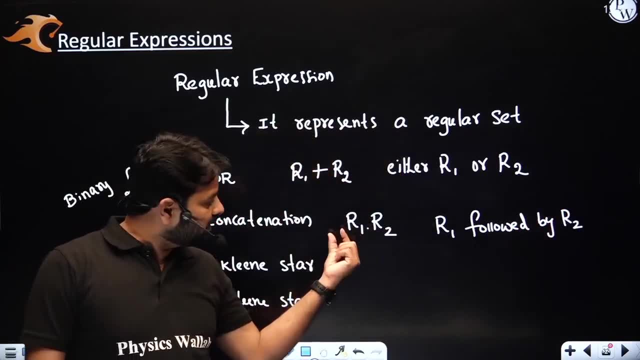 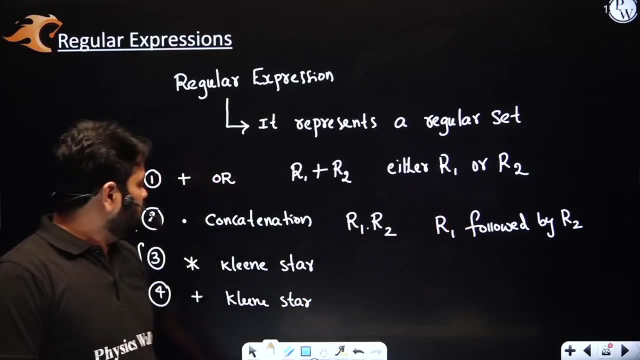 R1 followed by R2.. It means together always comes, but a sequence is maintained: R1 and R2.. Then the sequence is maintained: R1 followed by R2.. You cannot write R2 followed by R1. Remember that, By definition, R1 followed by R2.. Clean is star. It represents R, It is. 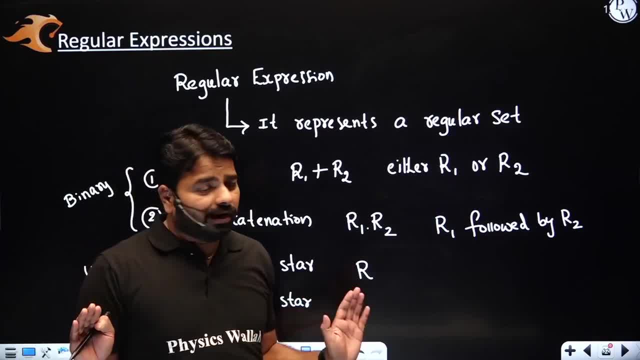 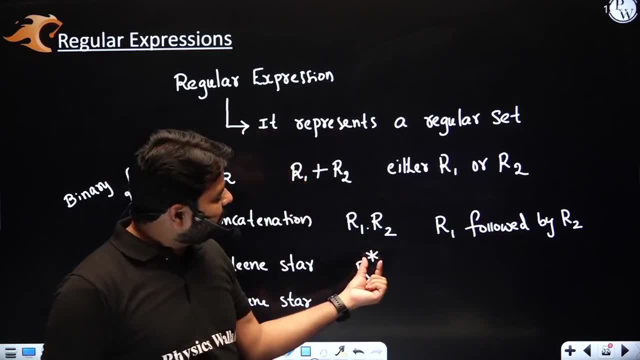 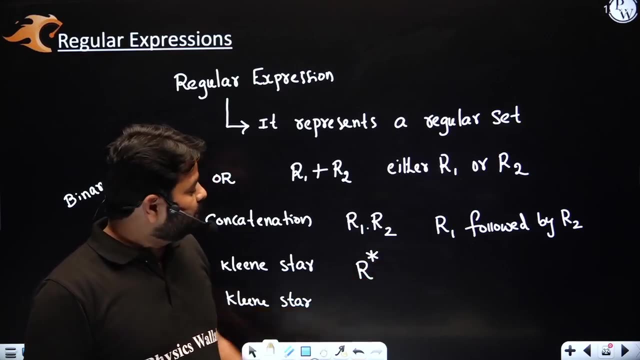 unilateral. You cannot write R1, R2 now. You can use only one expression or one operand, R. Then over you can write star. It is a cleanly star of R. You can also speak cleanly closure of R. Or you can say R, star, But all means same R can be repeated any number of. 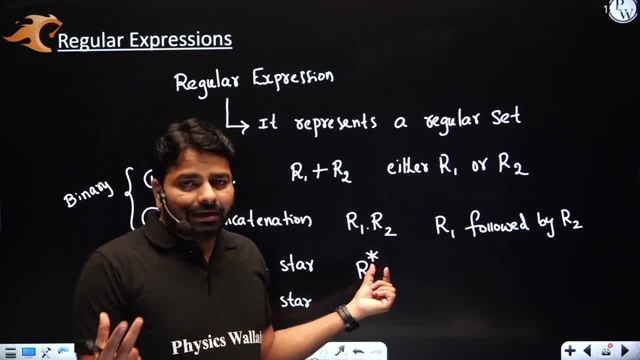 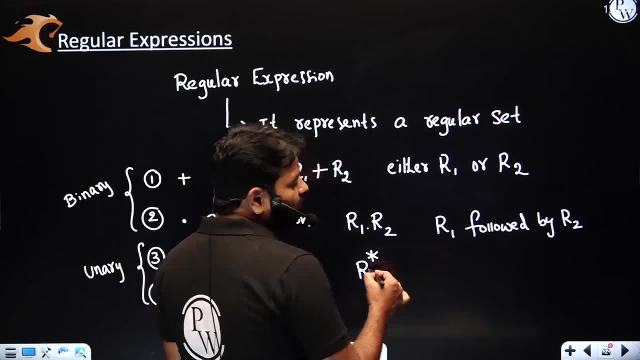 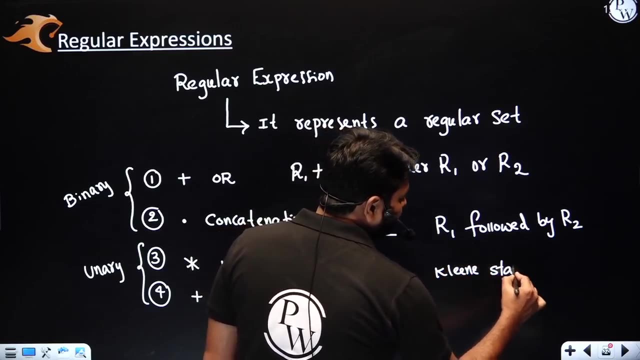 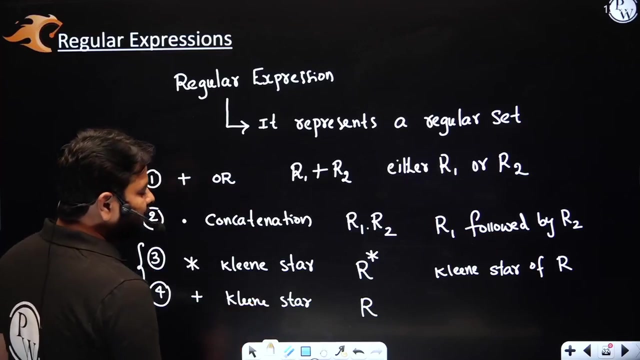 times. The star basically defines any greater than or equal to 0. So R can be repeated any number of times. So this is cleanly. closure of R. Clean is star Of R. Another one: cleanly plus. Sorry, Did I write cleanly star here. Okay, I just copied. 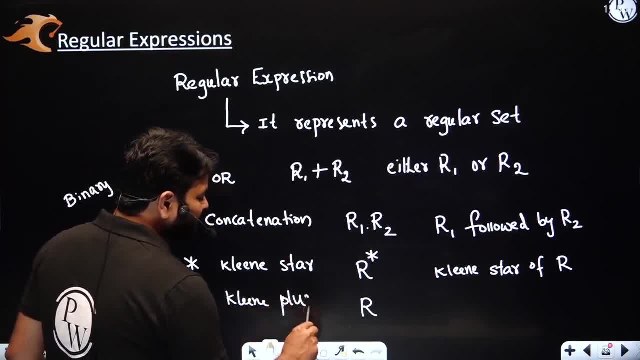 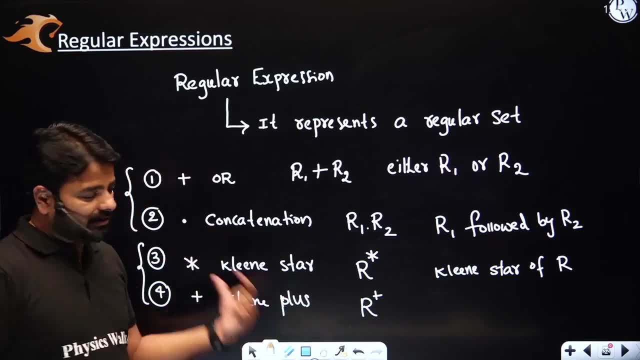 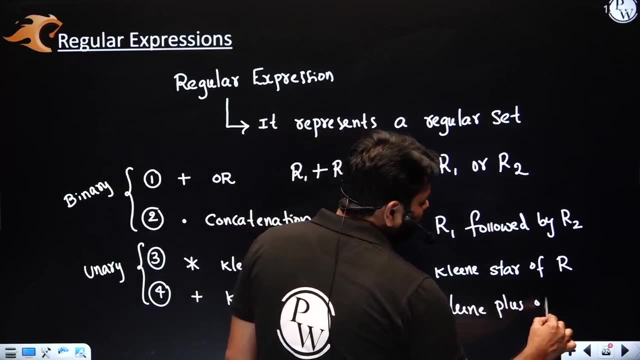 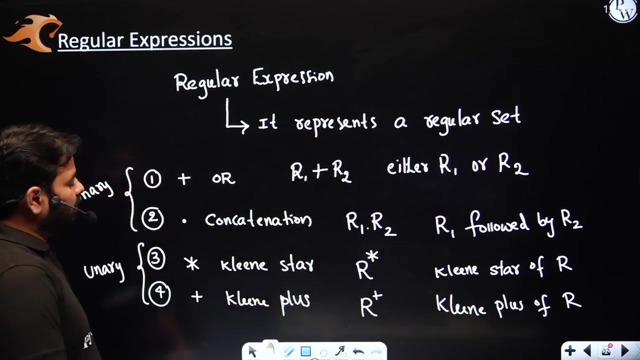 here. So what do you write here? Cleanly plus. What is R plus? So this is cleanly plus. R plus means you just speak like positive closure or cleanly plus of R. What is another name here? You have another name. You have another name here: Cleanly closure and positive closure. Or you can say: I am 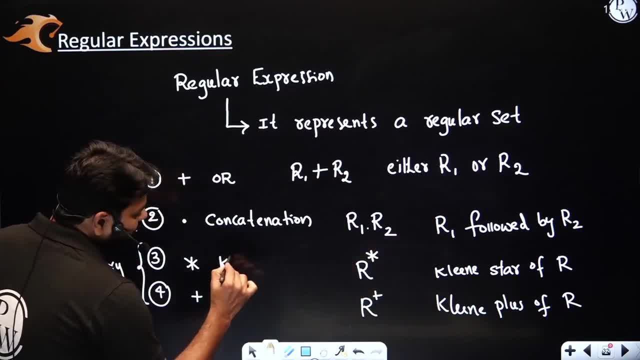 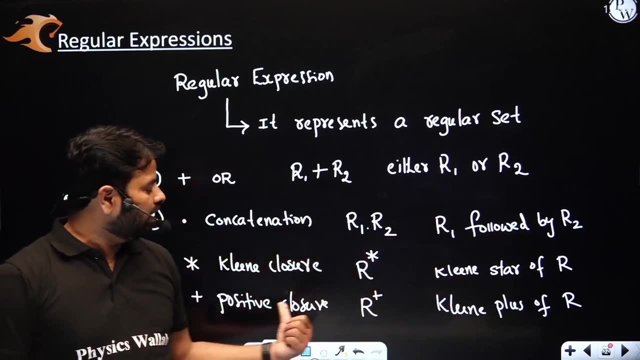 just writing another name here, But already I have written there. This is cleanly closure or cleanly star. Another one positive closure or cleanly plus. Other two names: Cleanly star, you can speak: or cleanly closure, Cleanly plus or positive closure. So what is the meaning? 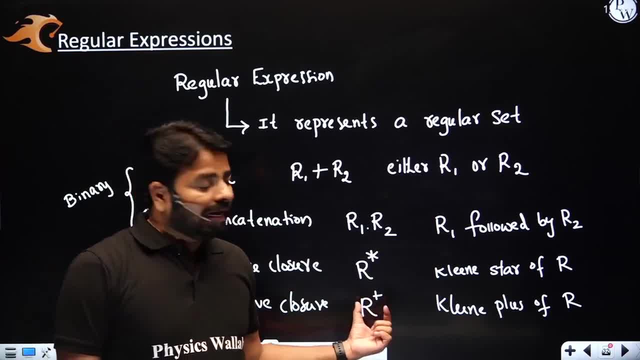 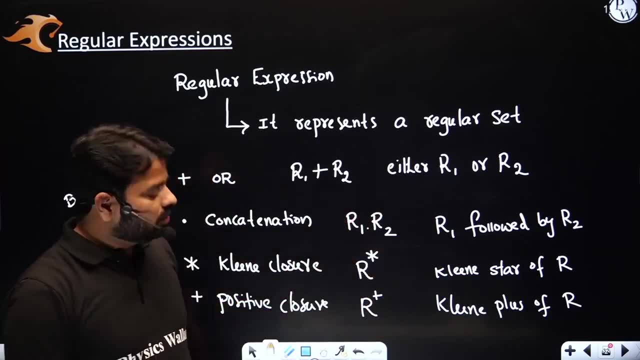 of the cleanly plus or positive closure. That is what this is, So it is small. You can say cleanly closure. You can also say code block. And what is R plus? R is two appearing numbers. It is three interesting things You. 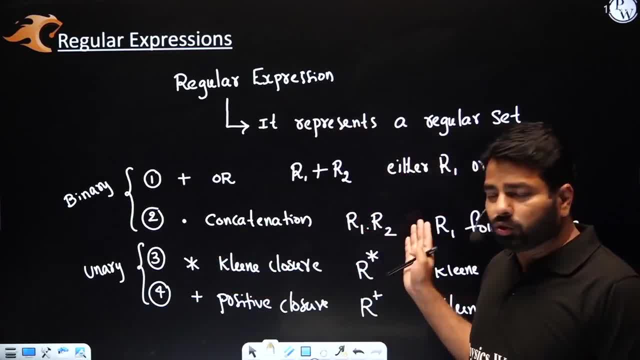 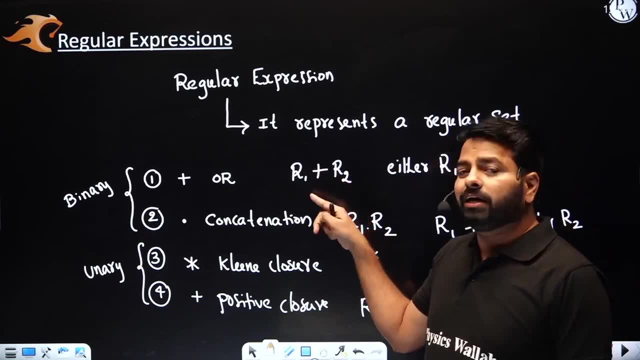 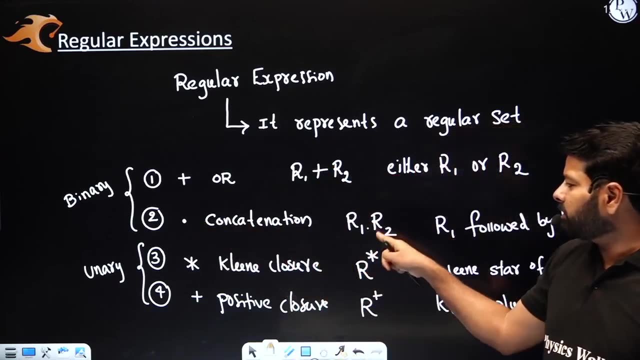 can use R for and R as in cleanly closure or cleanly closure. See, cleanly closure is the cleanly closure, But R plus is at least one time that R should exist. So to understand the meanings further, we will take each one separately. So I hope you understood at least the name of the operator. 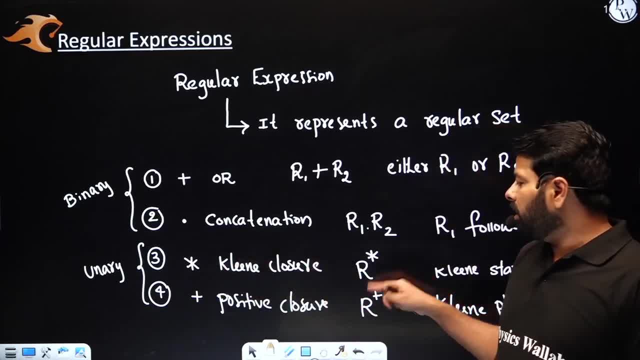 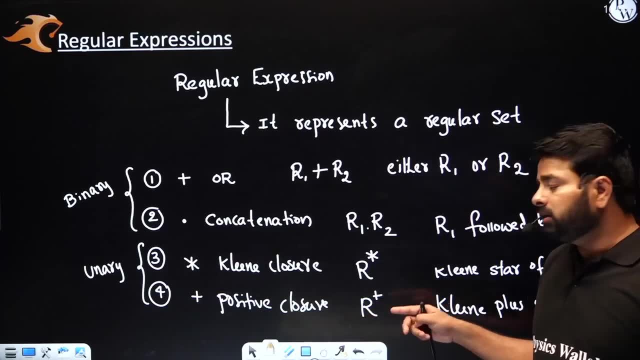 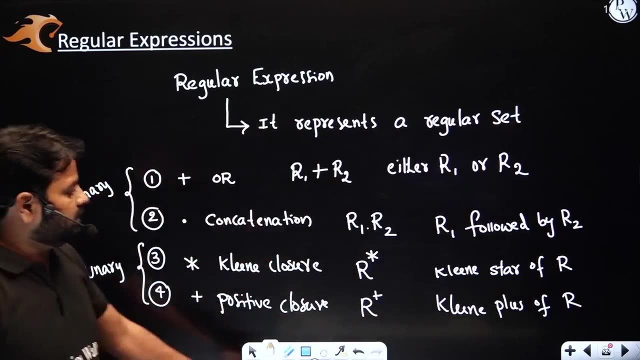 Kleene closure. you can write as Kleene star of r or r star. simply plus is the positive closure. it is nothing but r plus or positive closure of r, also called as Kleene plus of r. Let us begin with what is this plus? with an examples to understand all these four. we will see it. 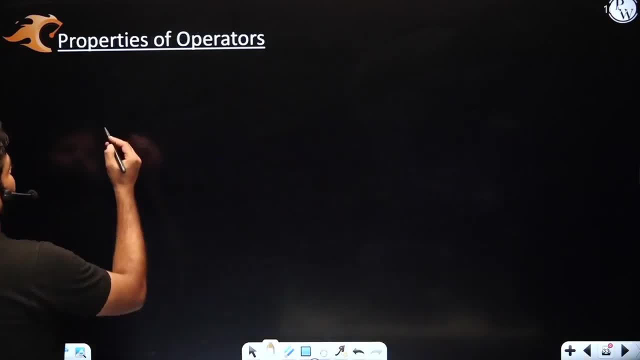 So, whenever I write a plus b, or whenever I write epsilon plus a, or whenever I write pi plus a, or whenever I write epsilon plus epsilon or a plus a or pi plus pi, you should know what is the meaning of this expression. as you know, everywhere I am using the binary operator plus. you should 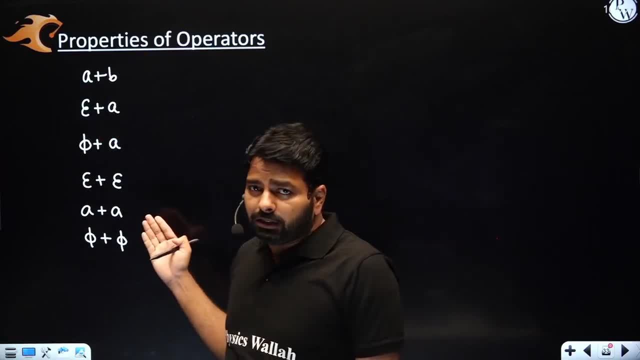 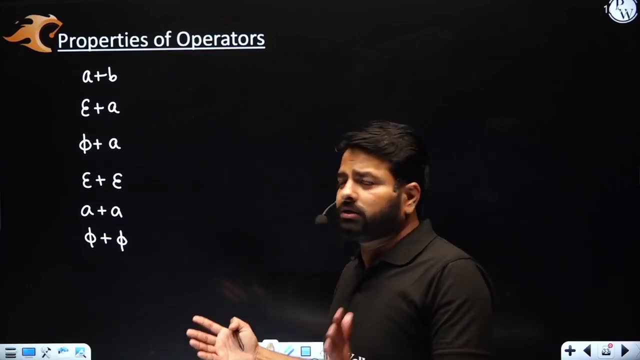 know outcome of this expression. So let us see what is the meaning of this expression, Because the meaning of the expression should be understood when you write it. Sometimes it can be simplified further, sometimes you may not. So whenever it is possible to simplify, just do it. 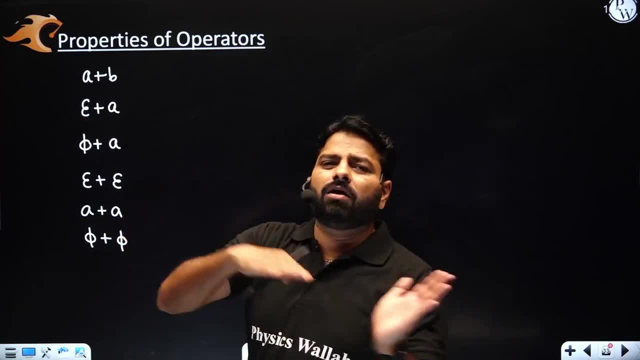 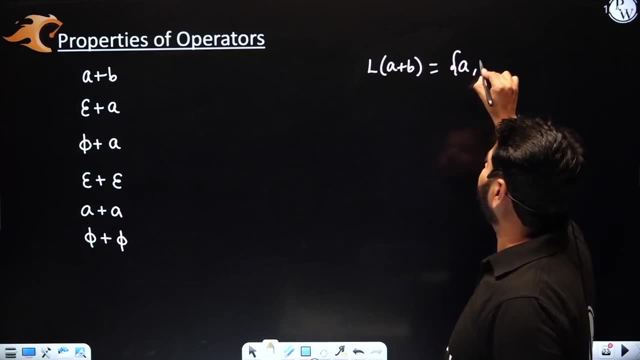 The first one. you cannot simplify because it has a or b. when you try to form a language, Language represented by a plus b, it is nothing but a comma b. Here, a plus b is an expression and what it generates is just set a comma b. How do you understand? 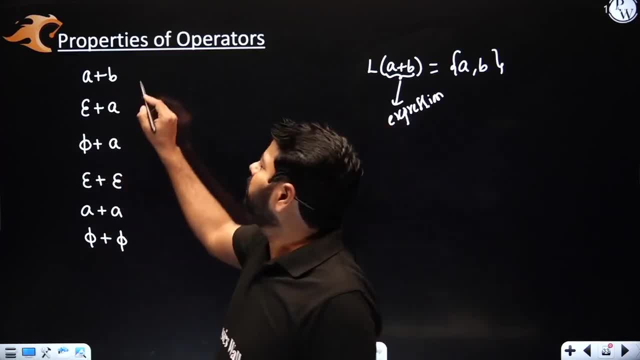 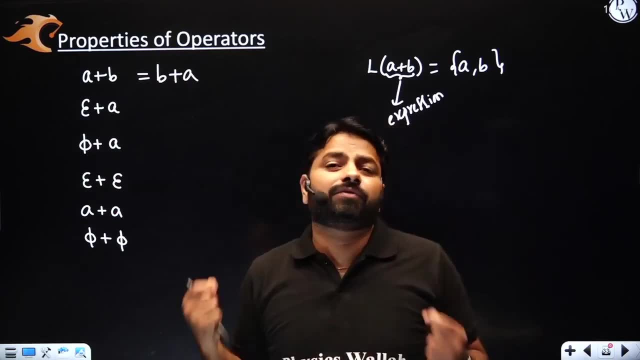 It is not possible to simplify further. Maybe if you want write, you can specify b or a, as it is commutative, The plus is here commutative, The operands you can switch if you want it, Like in the set, you can write a comma b or b comma a will get the same meaning. 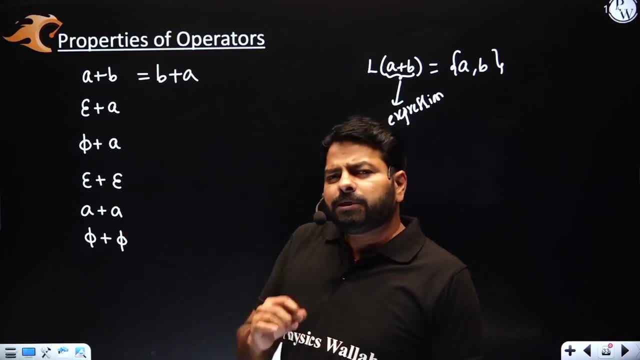 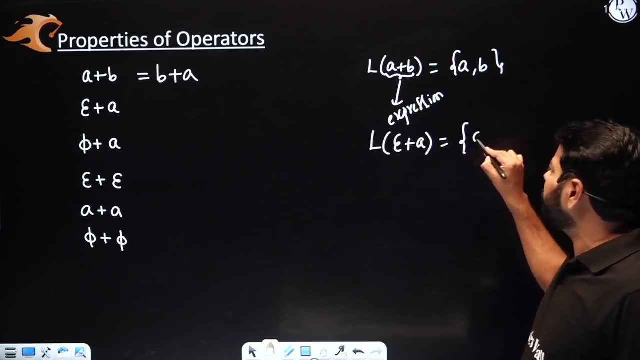 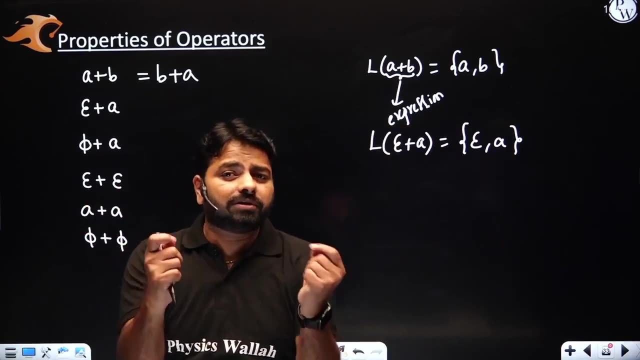 order does not matter. Next one: epsilon plus a. if I try to understand the language generated by epsilon plus a, you cannot reduce further. it is already epsilon special string and a is another string. You can't write only a because epsilon and a are both of different strings. Some people may write like: 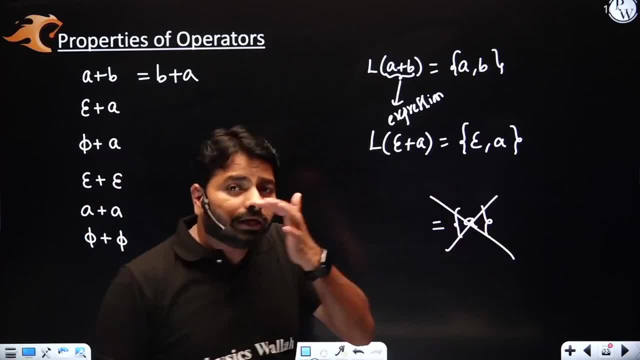 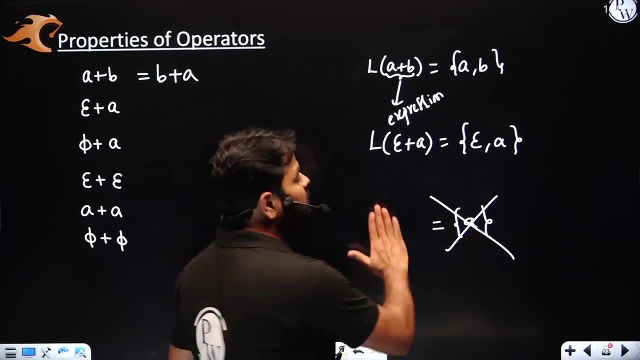 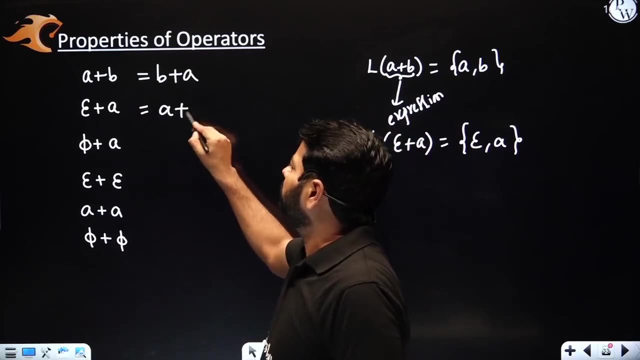 it's equal to a. that's wrong, because epsilon you can't ignore. Epsilon has to be there. It should be generated. When you don't write epsilon, that means you are losing that string. So please do not write this at all. Epsilon plus a. you may write, if you want it, a plus epsilon, but you can't. 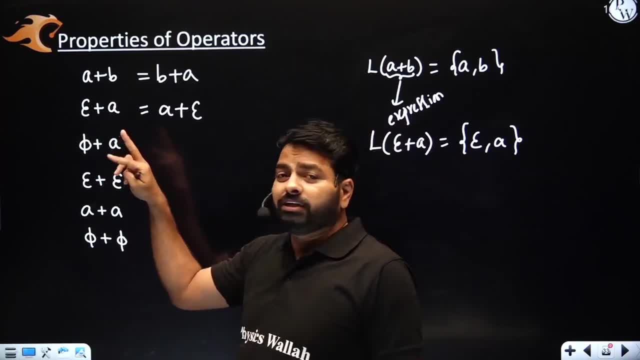 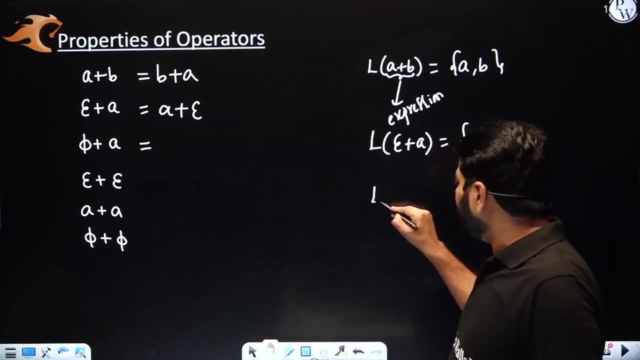 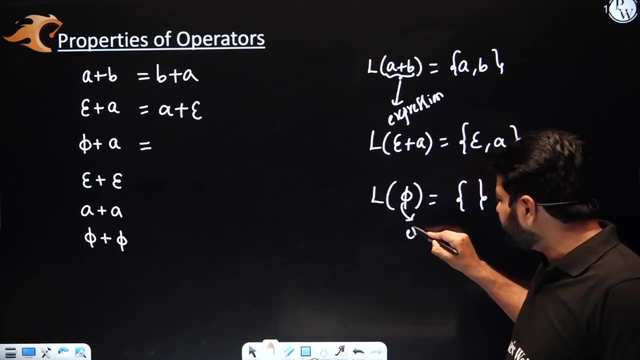 ignore any string. You can change the direction of, change the order of the operands, but you can't ignore anybody. Fine, pi plus a pi means what If anybody writing language generated by the pi is actually empty set? Okay, this pi is not empty set, It is an empty expression. 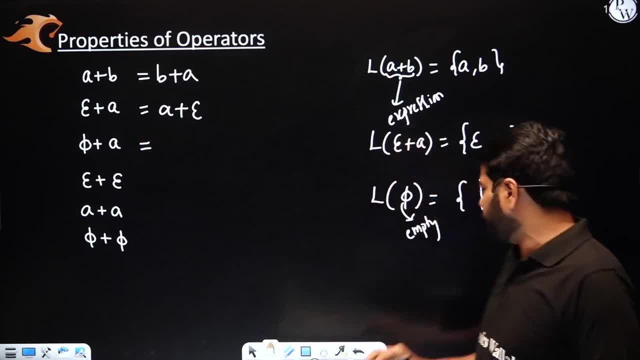 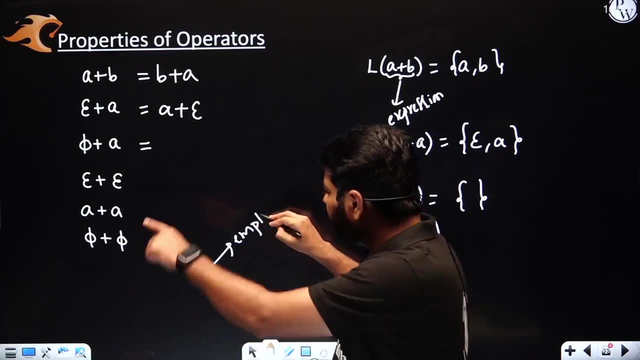 I'm using an expression, right, So don't call that as empty set. It is an empty expression Here. pi is used in different places with different names. Sometimes pi we call empty set. Oh, this is not empty set, It is an empty expression. Sometimes pi we call empty expression. But how do you know? 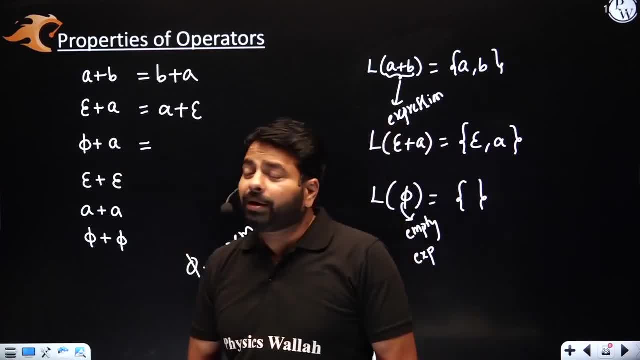 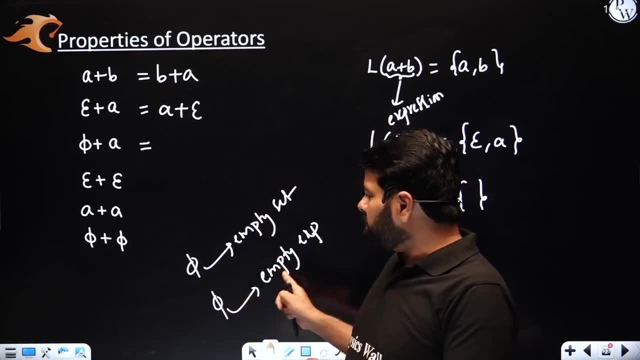 that? where do you write? i'm writing along with the operands operators, so it has. it is one of the operand in the expressions, so definitely empty expression. i hope you understood what i'm trying to say. in the set theory this pi represent empty set. in regular expression it is empty expression. 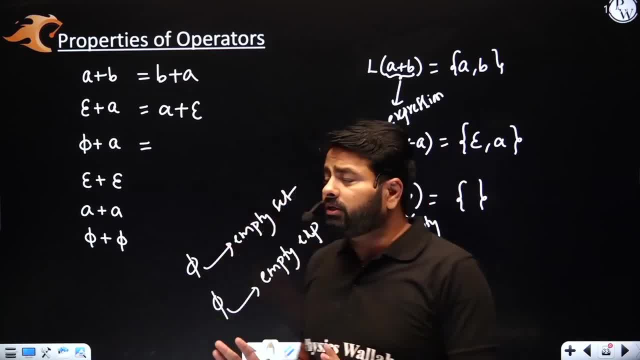 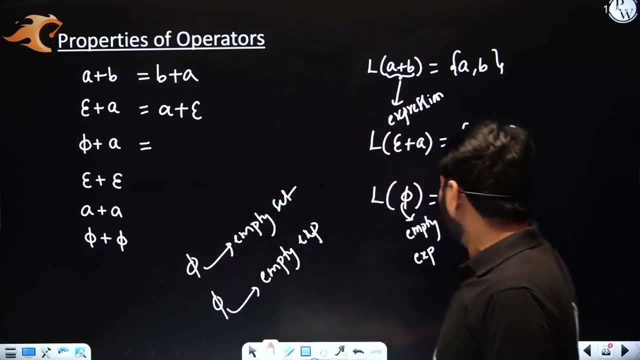 okay, in general we may use together, but be careful when you use it. the meaning should understood, right. so it's expression. so you call pi is empty expression. okay, so here you will get equal to pi, but this is empty set, even though i have right, i write pi, but that is not empty expression. this. 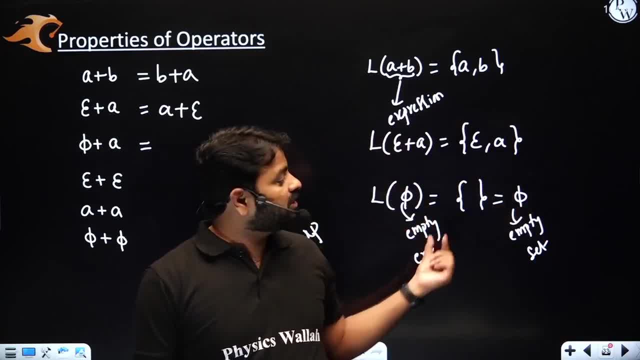 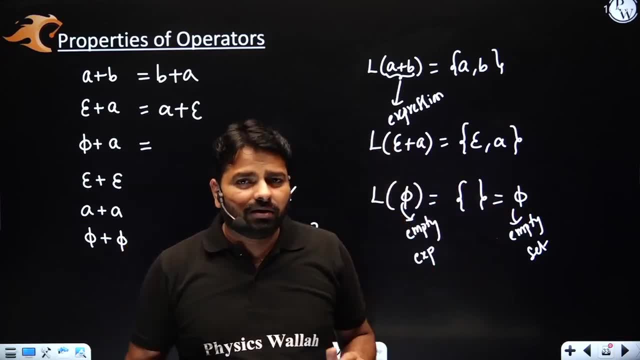 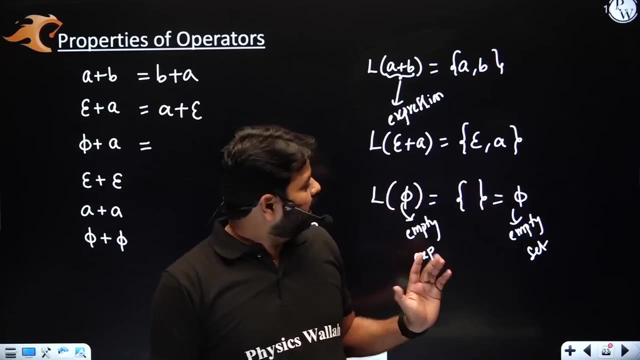 empty set. so language generated by empty expression is a empty set. that means l of pi is a pi, but this pi and that pi looks different, the meaning is different. okay, so that's what the problem with the these two pies. anyhow, the internally they are an, outside they are equivalent, and internally only. 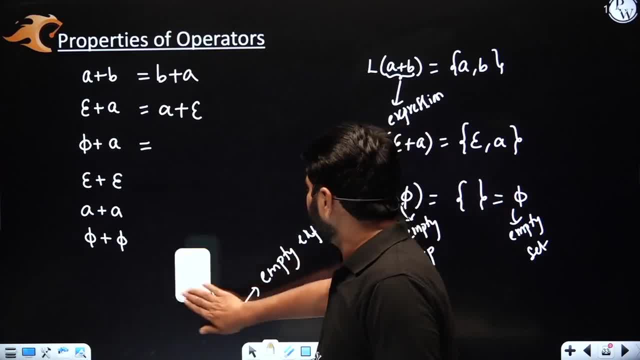 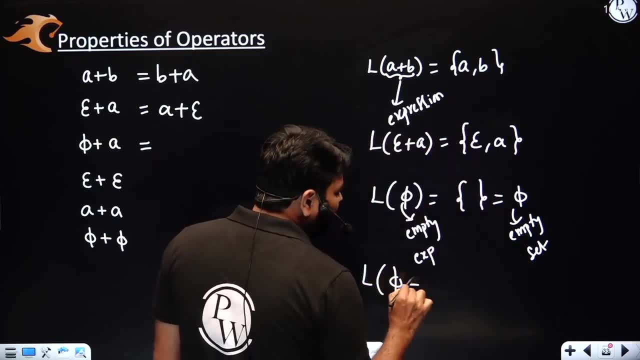 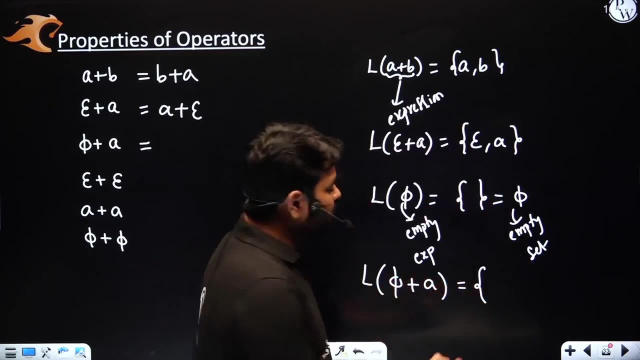 their names are different now, fine, so be careful with that. so pi plus a. what is the meaning? now? language generated by pi plus a. the pi will not generate even one string, so you don't get anything. a will generate one string, so a you will get. so when you get a language which has only a, you can write simply: 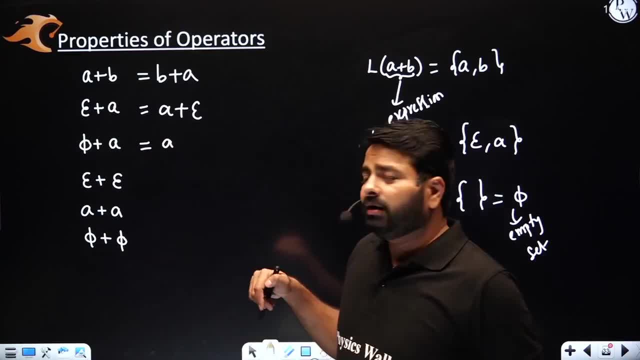 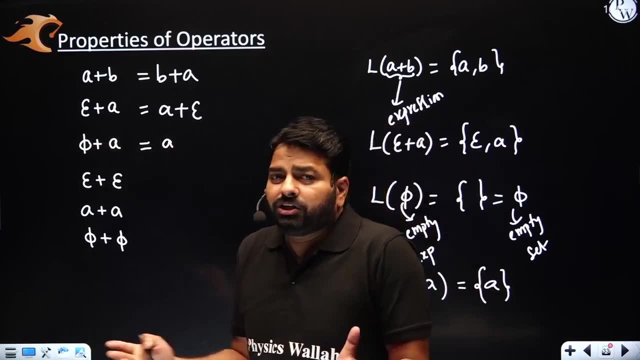 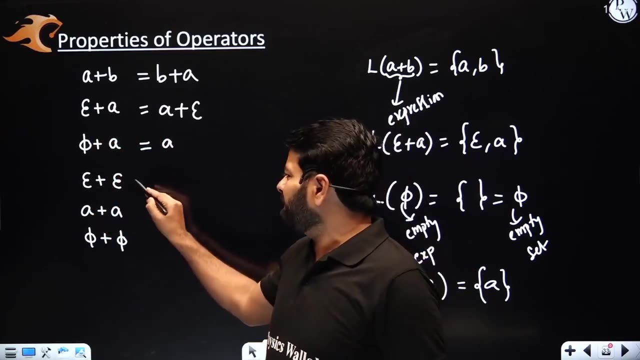 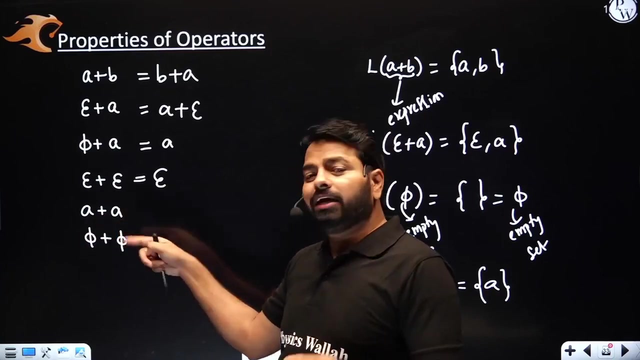 right, a plus pi, pi plus a. both are a only clear. so this is going to generate only one string, a. now pi has no participation in generating a. string comes to epsilon plus epsilon. both are same operands. right, you can simply write epsilon, both will generate same string, epsilon and a plus a. a is generating a, r, a is also generating a. 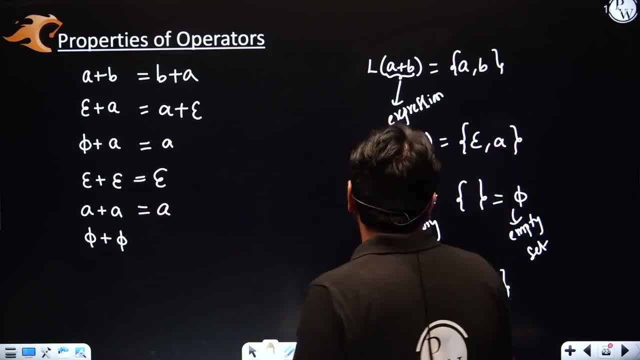 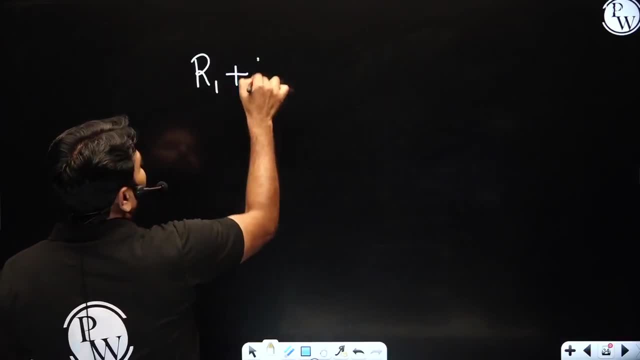 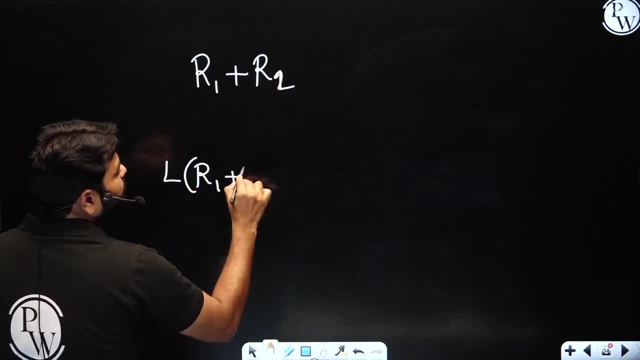 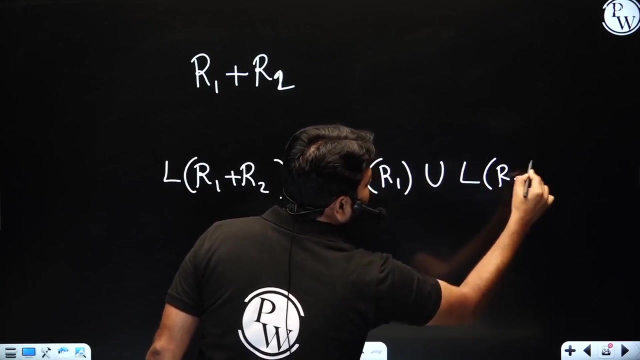 so both will generate a. what is the meaning of a plus a? let me write that too here. whenever you get a situation like r1 plus r2, remember the point. it's same as if i ask language generated by r1 plus r2. you just say: language generated by r1, union language generated by r2. you can. 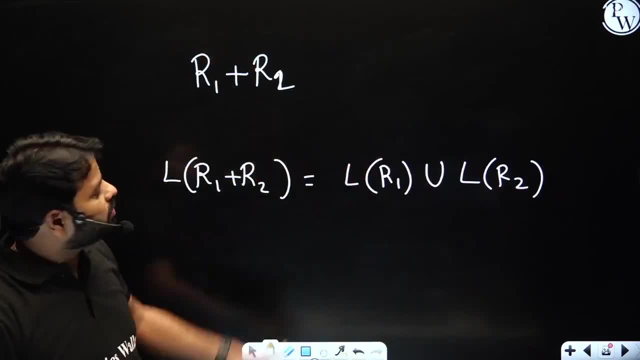 understand that way. if you want to understand what r1 plus r2 does, just do the union of two individual languages represented by them. so you want to understand r1 plus r2, just understand what is r1 generating and what is r2 generating, just do the union right. 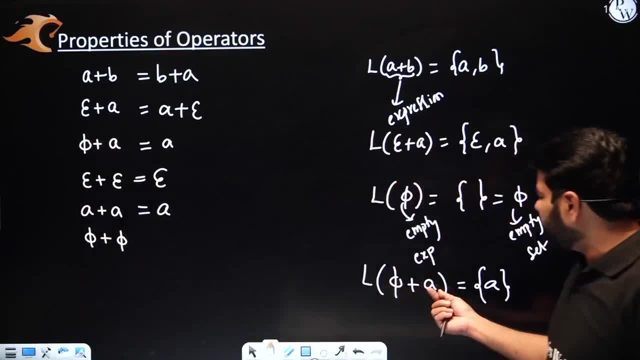 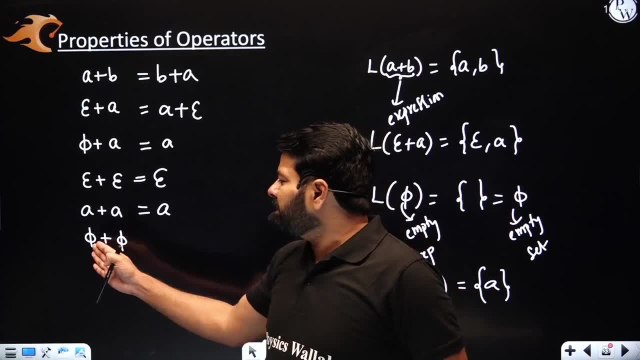 that's what i am doing all the time: what pi does nothing, what a does a. so i did the union. you got this. now pi plus pi see pi means it's generating nothing at all, so you will get empty set. union, empty set. you will get empty set. so it can't generate anything. so again pi here. this is how. 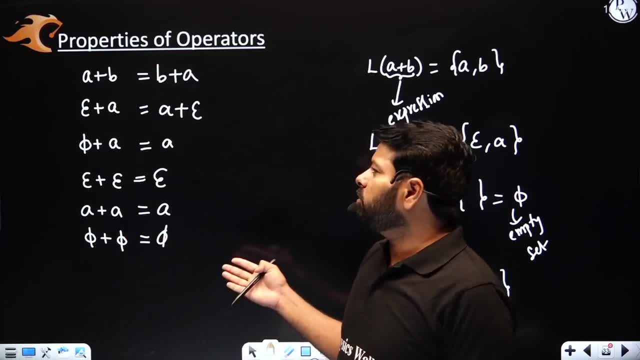 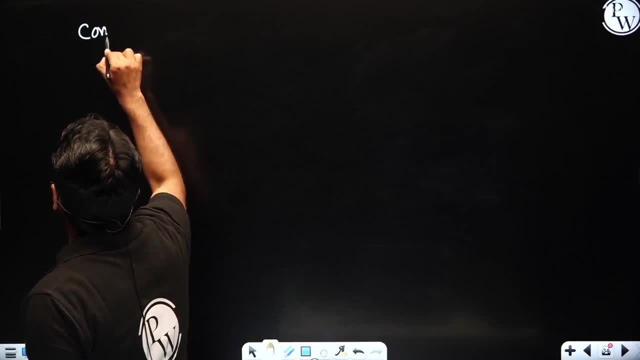 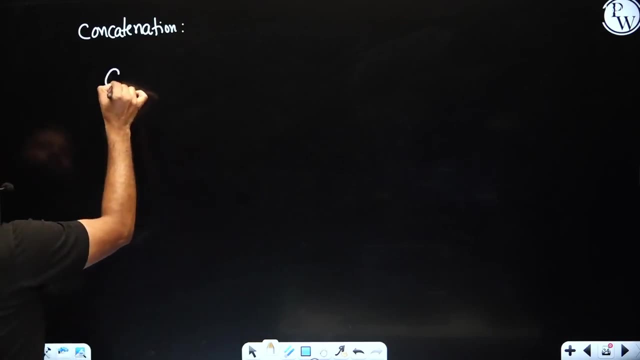 you use the r operator. now we will go to the concatenation. what is the concatenation responsibility? you have seen just now a plus a. you did, now i am doing a dot a. just think about what it does, like a dot, epsilon, a dot pi or epsilon, dot, epsilon, a dot a is done right: a dot, pi and pi. 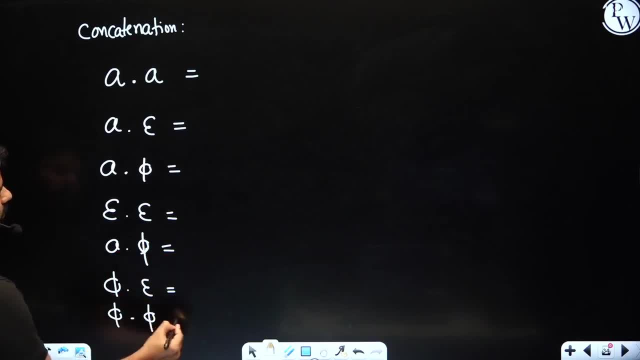 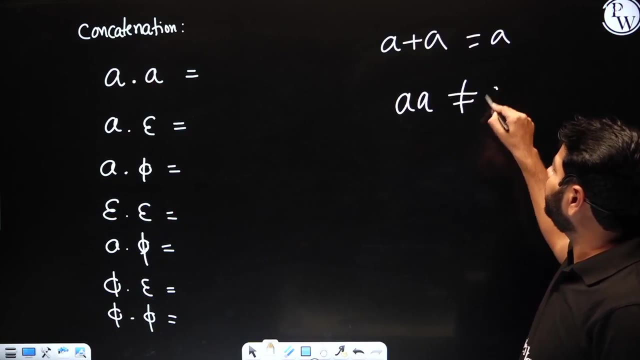 dot, epsilon, pi, dot, pi. so just try to understand this. few expressions which are using concatenation- a dot, a, see a plus a- means both are generating a. so you did, you said a. but when you say a followed by a, you can't say a. why? because it's a two length. it's going to be two length now. 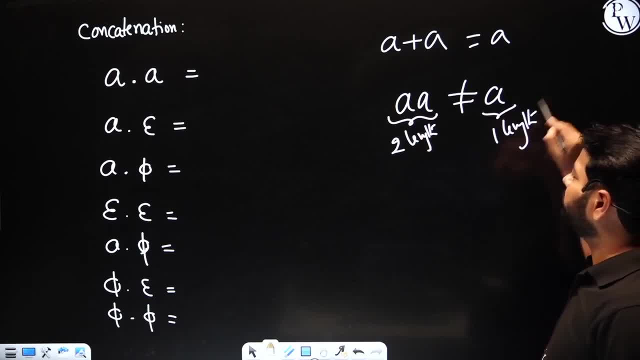 this is one length. how can be? they are equal, impossible, right. but here this side is generating a and that side is also generating a. you take any side, you always get a. so you have taken a. it's just like if else condition, if go this side or else go this side. but 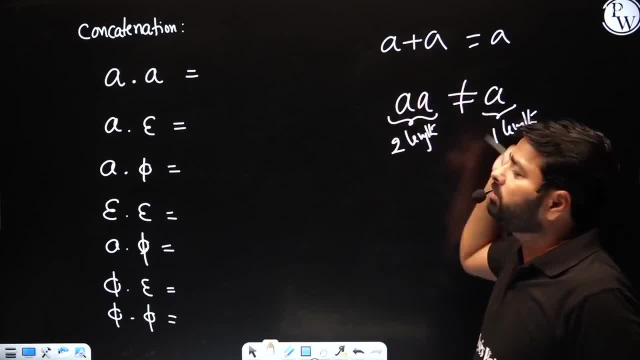 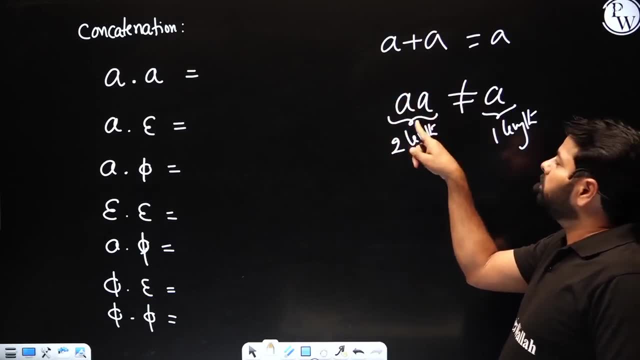 when you say a, you can't say a because it's a two length. it's going to be two length. now when you do the union, you got the same thing. then you don't need if else, directly you generate a. so that's, that's important for the plus. but dot means you must follow a, followed by a. you can't. 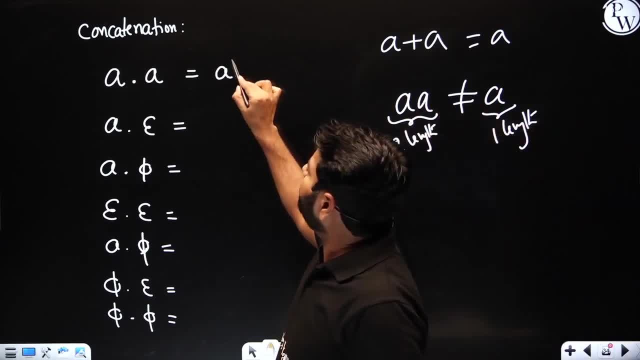 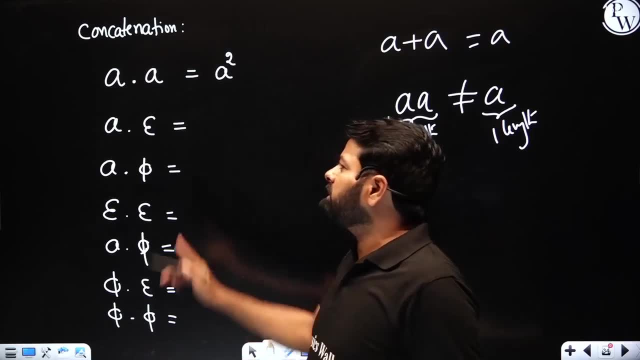 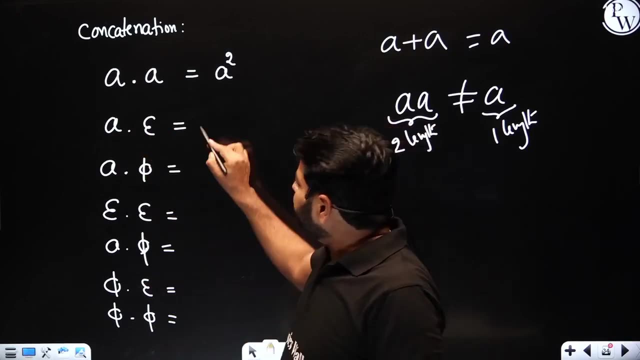 get a, you get w, so you may write as a power two. that's fine, because a is repeated twice. you may write a power two or you can keep as it is: w, that's fine. two consecutive ways, but a followed by zero symbols, a followed by epsilon means simply. 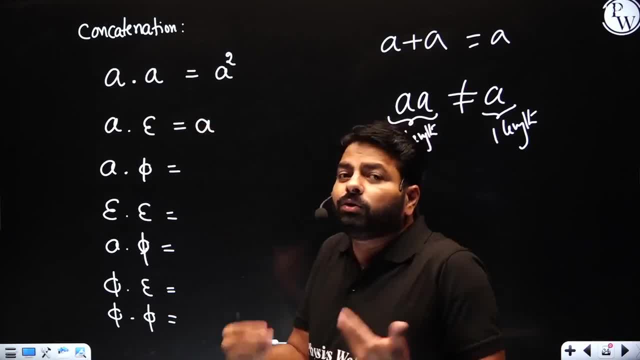 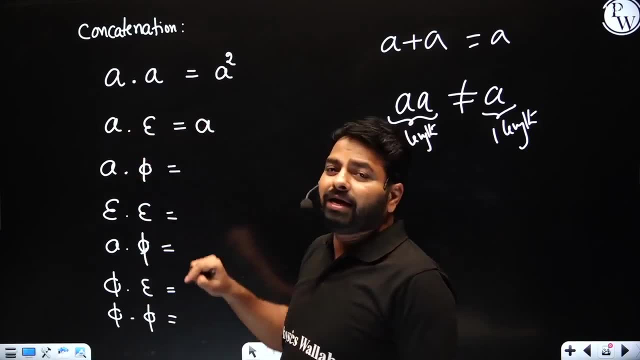 you can write a. see before a after a epsilon is there, that we don't write it all, because that is no importance for the epsilon when somebody else is present. so a followed by nobody is there, but that's empty string, basically. so one symbol followed by zero symbol, you will get one symbol. 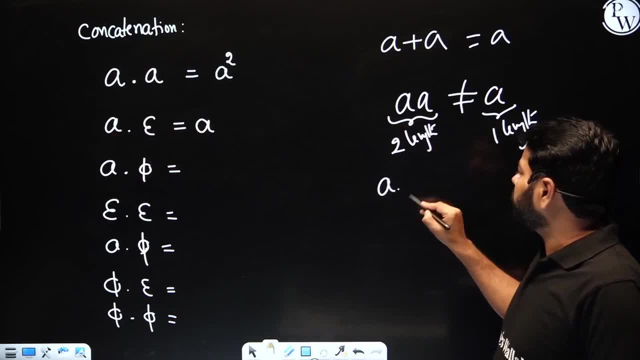 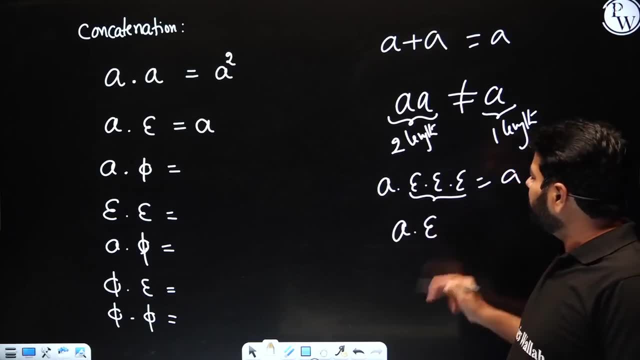 only that is a. so remember one more point: a dot epsilon, dot epsilon, dot. epsilon, it's just a, only because this is just zero symbols. let me simply: a dot epsilon is just a or epsilon a is a, only so we can write a before, a after a epsilon is there that we don't write it all, because there is no? 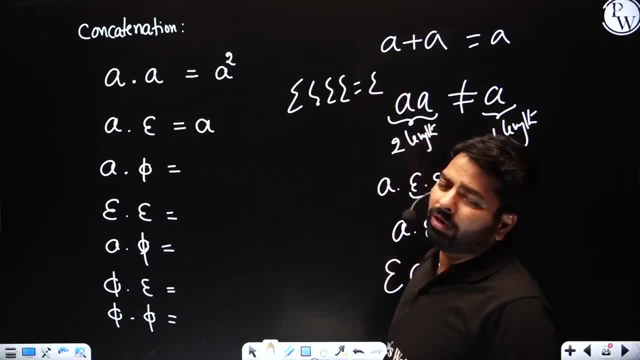 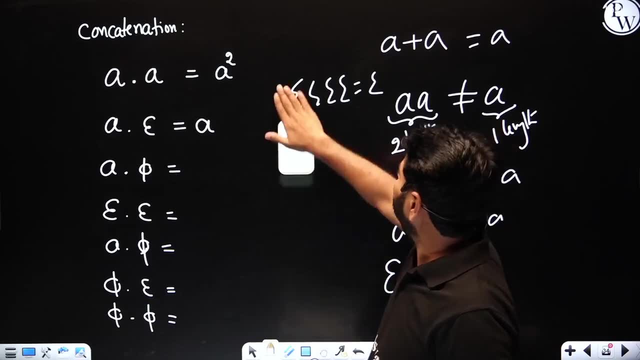 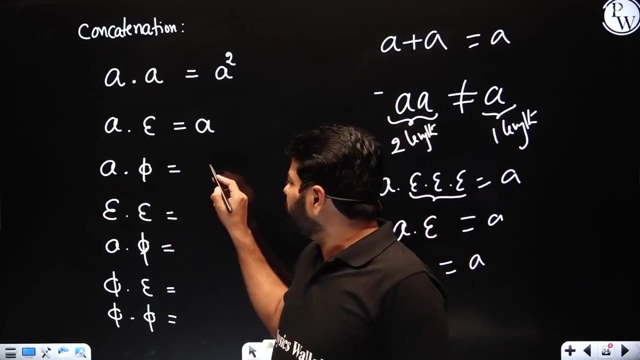 when you have so many epsilons like this, it just you can write one epsilon. two as this many epsilons has no importance writing. nobody is there right. fine, now a dot pi. here it is a problem: a will be generating a, but pi will generate nothing. how can i get some swing from here? 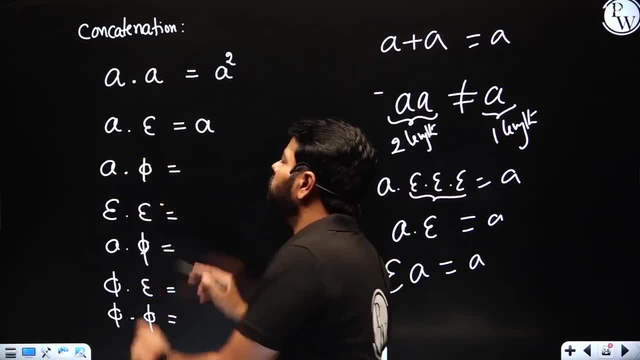 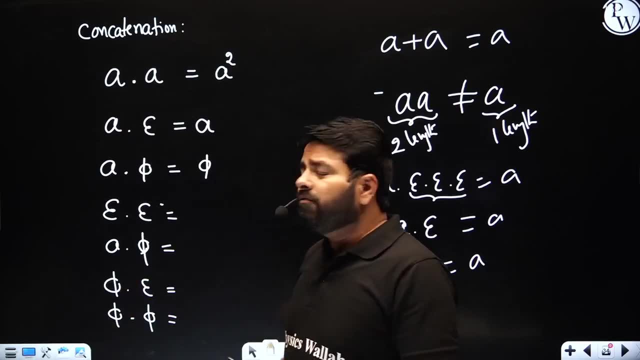 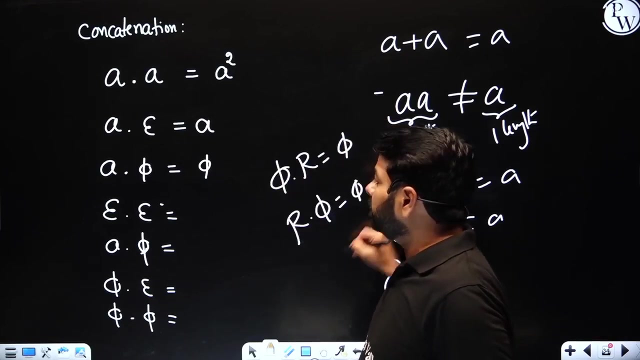 impossible, right? so this expression will never generate anything. so result is a pi, because pi, dominator in the concatenation. remember this point: whenever you see pi in the concatenation and whatever the expression that you are doing with, the pi is whole expression will become pi. so i say anything, pi dot, anything is pi r dot, pi is pi. but don't keep pi whole star, pi whole plus. 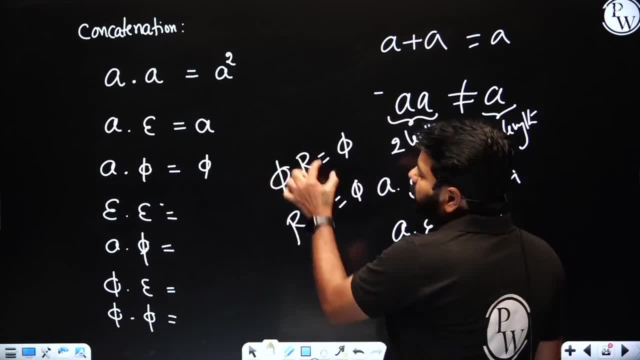 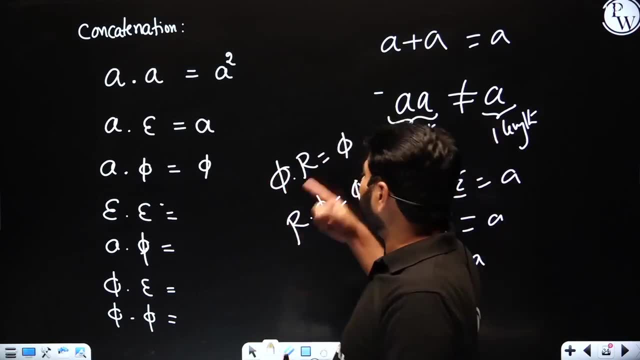 that's a different meaning. we'll talk about that. so pi dot, r r dot pi or pi dot, anything is always pi, because it can't generate even one string. so if you want to understand more about it, yes, we can come up with that. okay, let me take this. 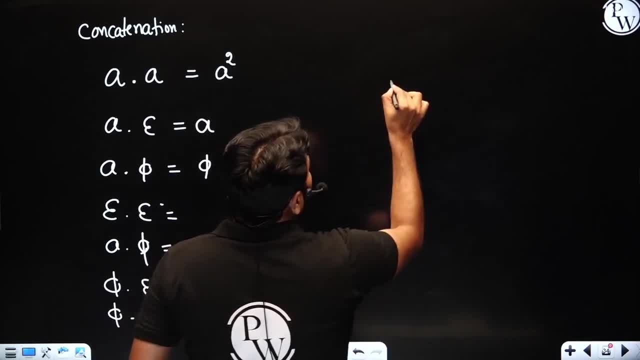 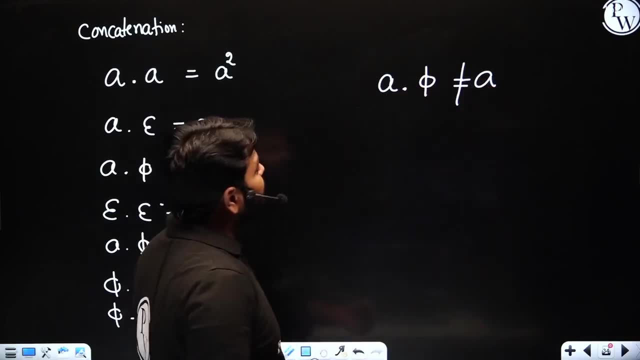 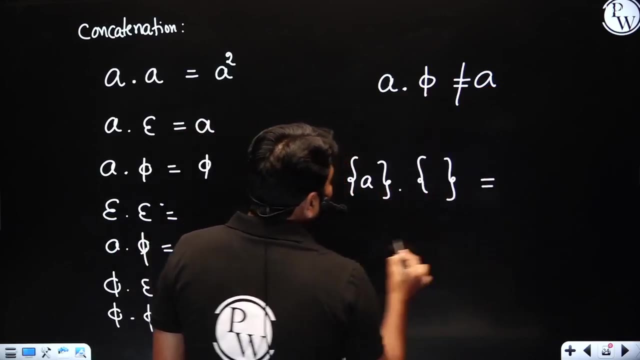 now some people, might you know, trying to understand. what is it? why can't i write a? why can't i write a right? the question is: a is going to generate only a, pi is going to generate nothing. then from here you can take a dot, from here you can't take anything. then how can i form? 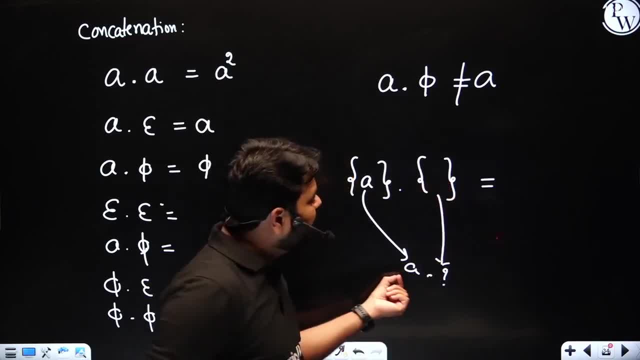 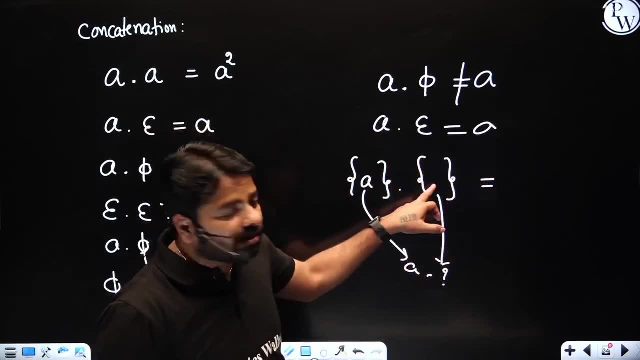 a string without taking anything. at least if you have epsilon here, a dot epsilon, you will get epsilon. so when i and somebody saying a dot epsilon, definitely will get a, no doubt, because here epsilon will be there. but this pi means empty set, and when you have empty set there is no string. 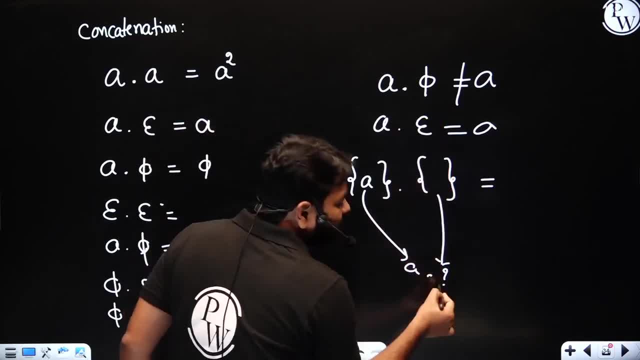 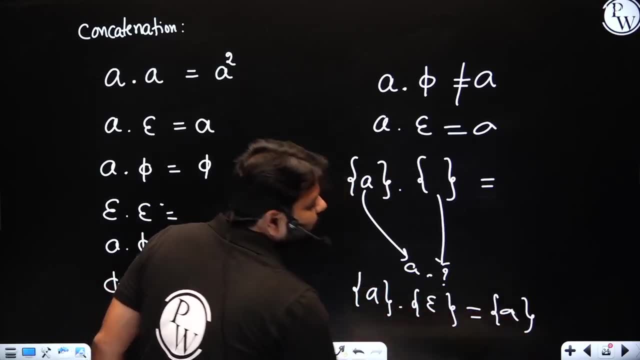 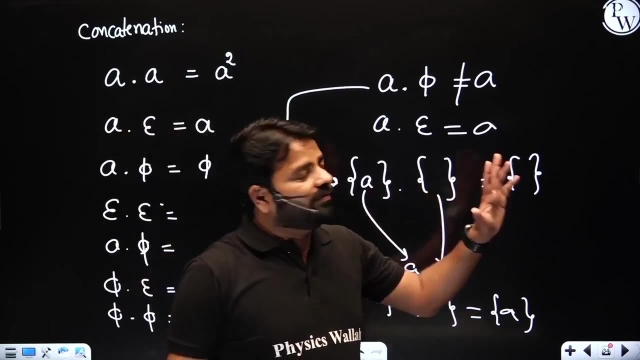 inside. in case, if you have a string here epsilon, then you can write epsilon. so in case, if i write a dot epsilon now a dot epsilon, you will get a, no doubt, but here you get empty set. so this means a followed by no one is always no one, but a followed by empty string is always a. 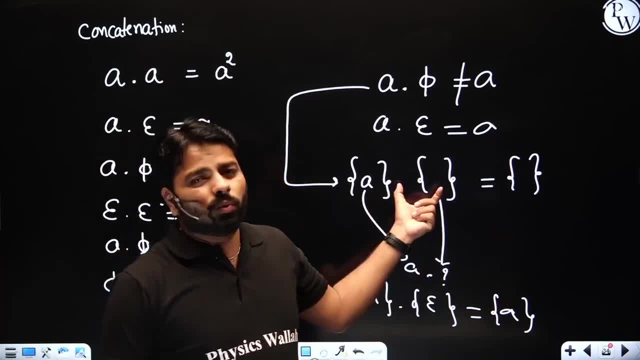 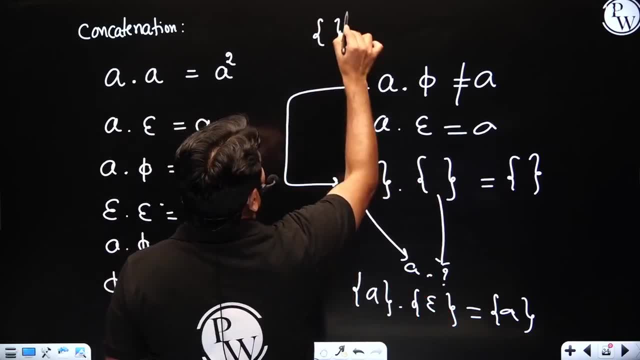 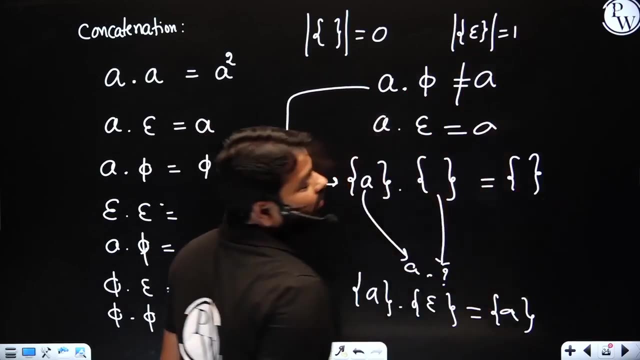 so understand the difference between these two. a set has no one set has empty string. both are different. why why both are different? if you take empty set, do the cardinality, you will get nothing. but you take set and ask the cardinality, you will get a one. and also remember epsilon length. 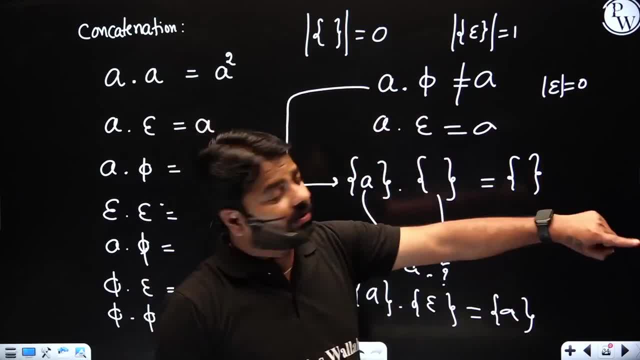 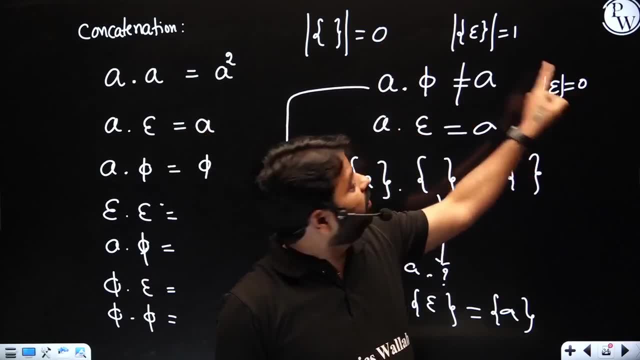 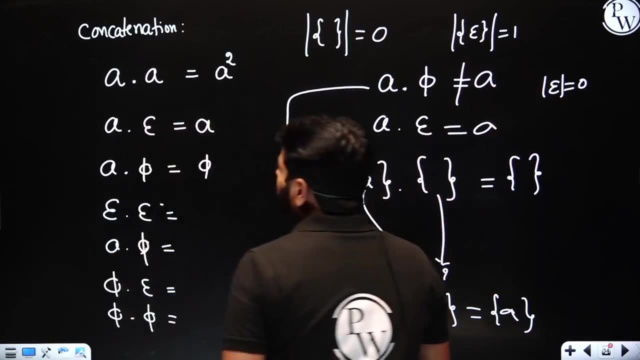 is zero doesn't mean that set which has epsilon is zero. remember: set which has epsilon means in this set, how many members are there? one member, but psi length of the epsilon is zero. both are completely different. so have the difference between these two. fine, now come to the point. 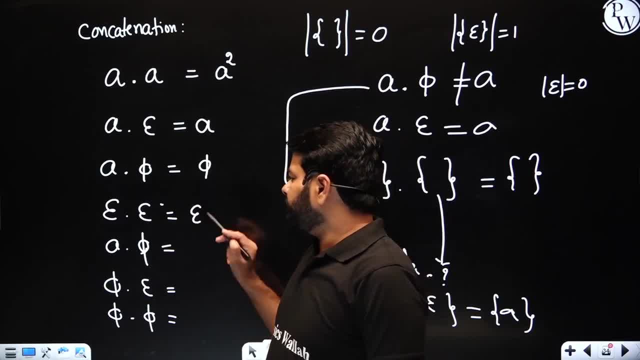 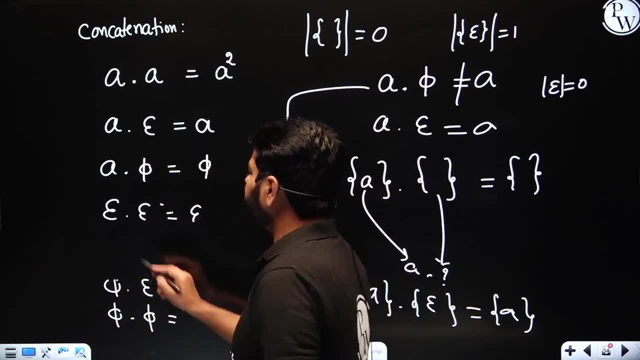 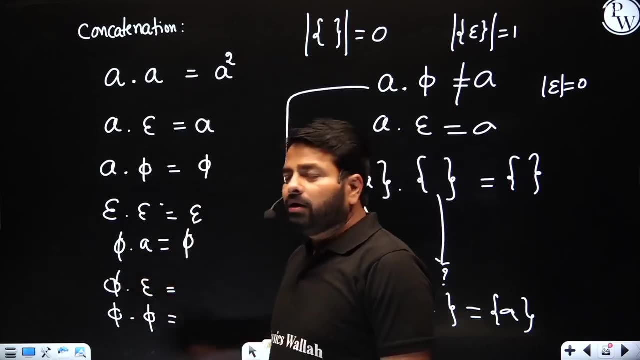 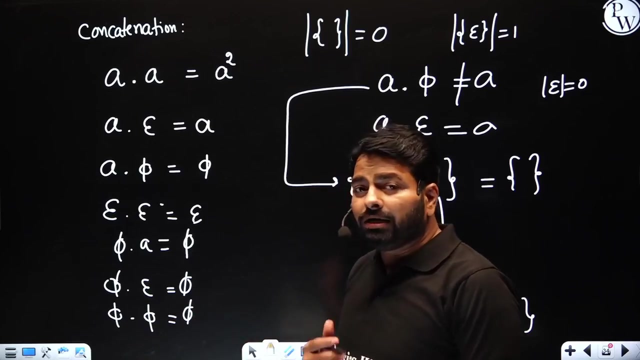 epsilon dot, epsilon. epsilon a dot, pi. oh, already asked here, so just change it if you want it. pi dot a, which is again pi, and pi dot epsilon. see, don't look at epsilon, look at pi. pi dominates whole expression. just write pi, pi dot. anything is always pi here. what do you understand? 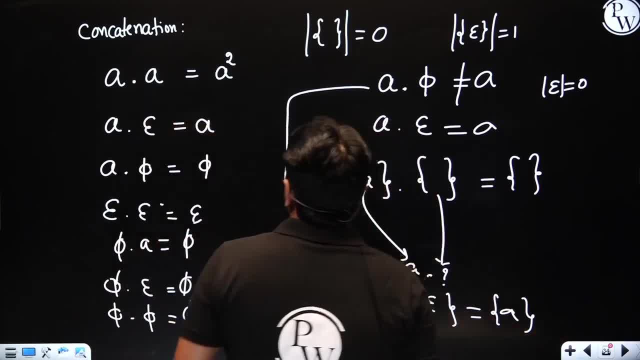 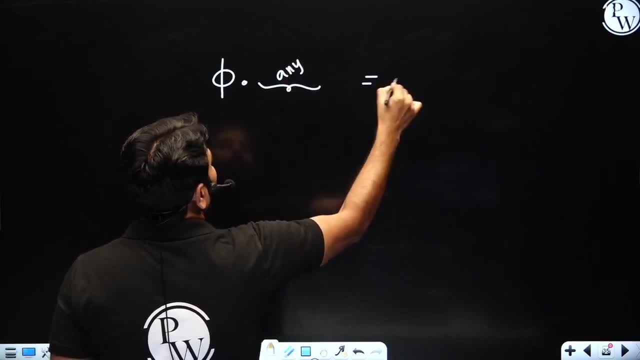 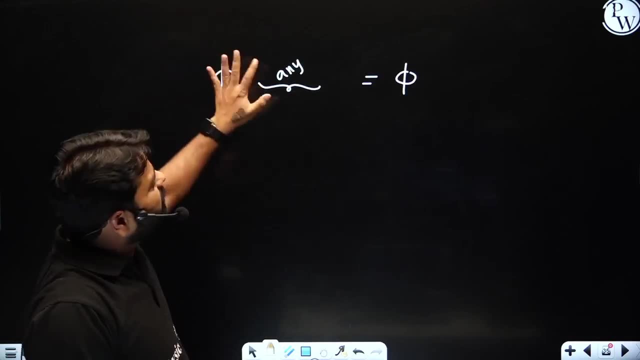 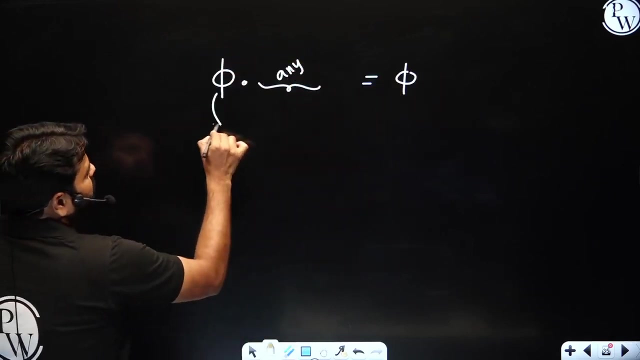 that there is one point which you require to remember: pi, dot any is always pi, but don't add anything to this. pi you know as a whole star or any other, so that gives you different meaning, but pi alone, dot anything is always pi, because pi acts as a dominator. but this is called as dominator along with the concatenation. 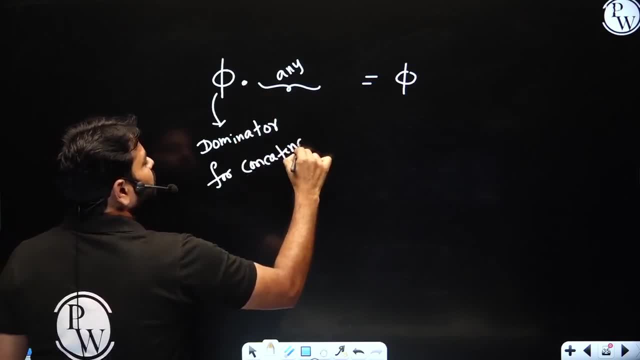 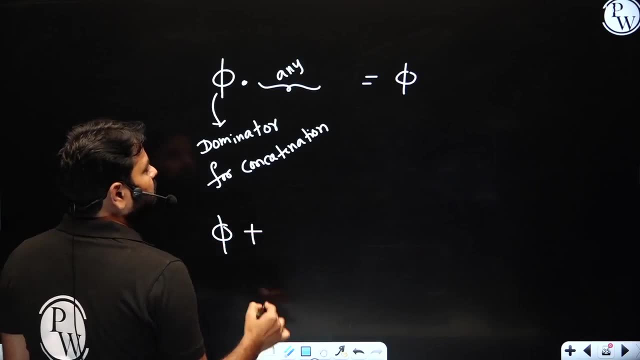 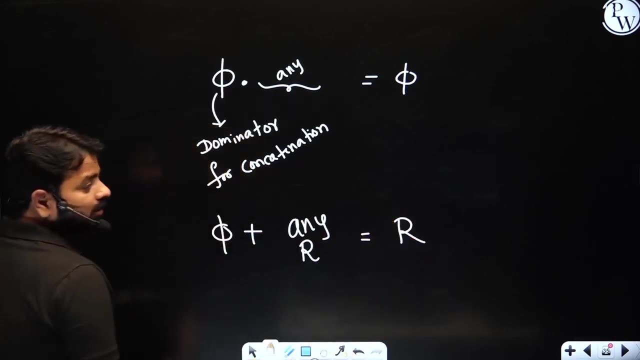 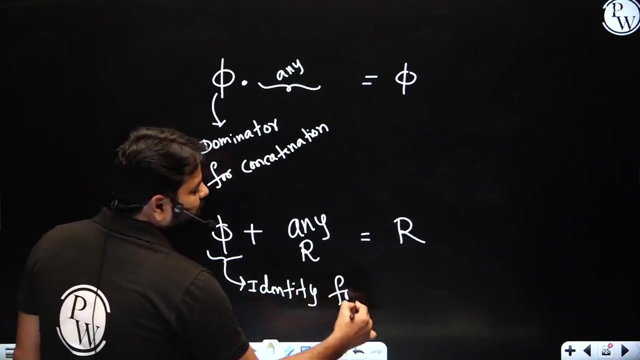 if you are doing concatenation, it acts as a dominator. that's why whole result will become pi. okay, but when you do along with the plus any expression- let's say it is r- the result will be r. why is that? because this acts as identity. it will not have an importance when somebody is there. identity for r operator. 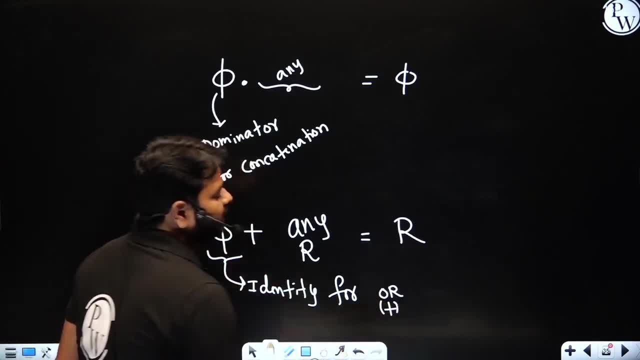 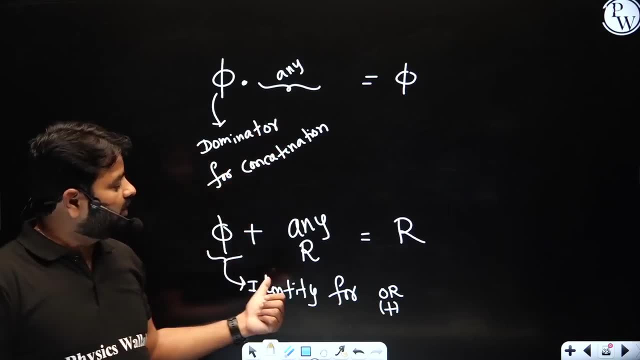 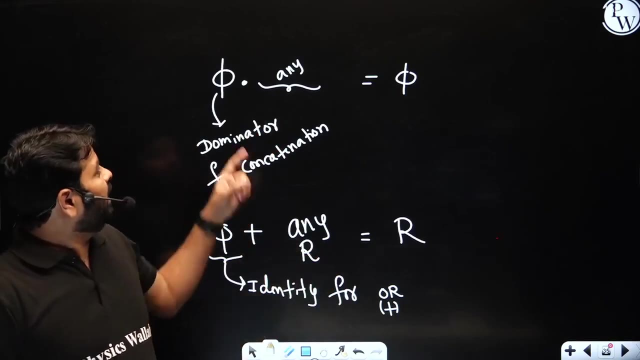 okay, so identifier r operator. so pi has two significances, along with the two different operators. for concatenation, it is a dominator. for r operator, it is identity. it has no importance when somebody else is there along with a plus, and pi has only importance when you do with the concatenation. So these two are completely 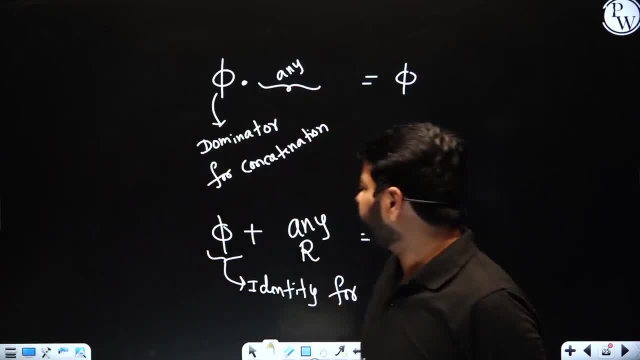 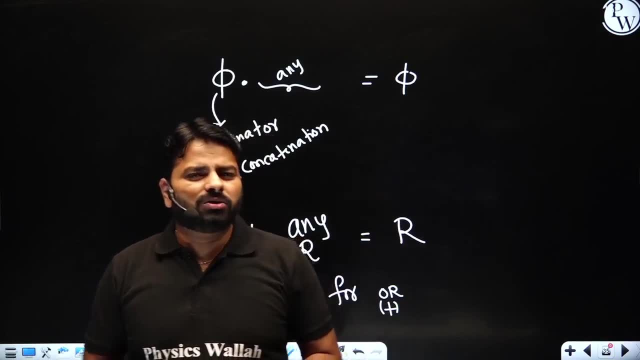 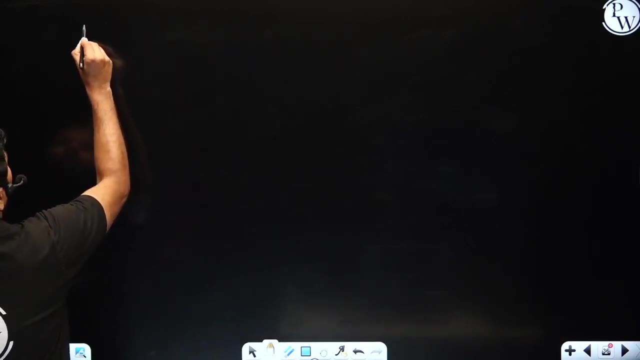 opposite direction, opposite ways. Fine, So far we have learned R and concatenation. Now it is time to learn what is this? cleanly closure and positive closure. Then we will begin with the regular expression as soon as possible: A star. what is the meaning of A star Actually? 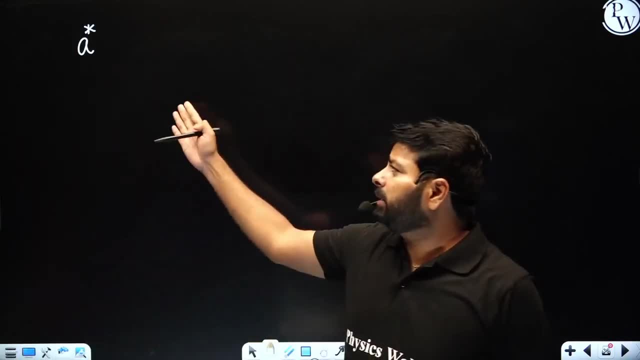 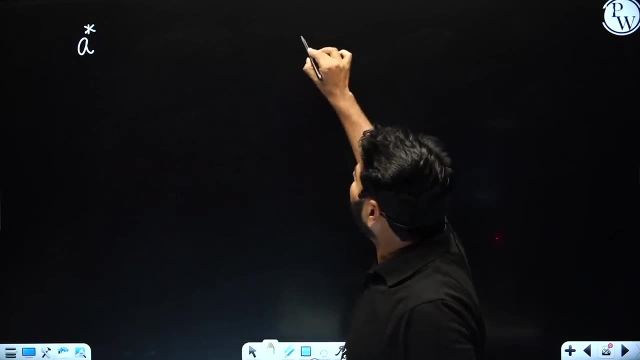 this is the simplest and best expression that represents cleanly closure of expression. right, You cannot simplify further. But what is the meaning of this one? Anybody ask what is the language generated by this A star? Then I can explain like now you can say A power. 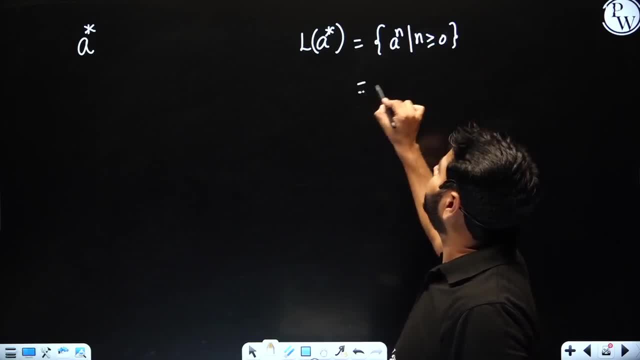 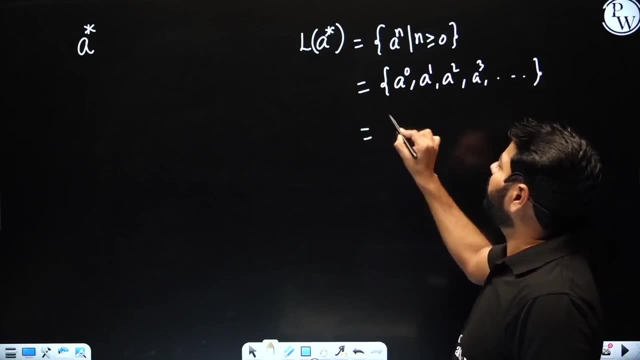 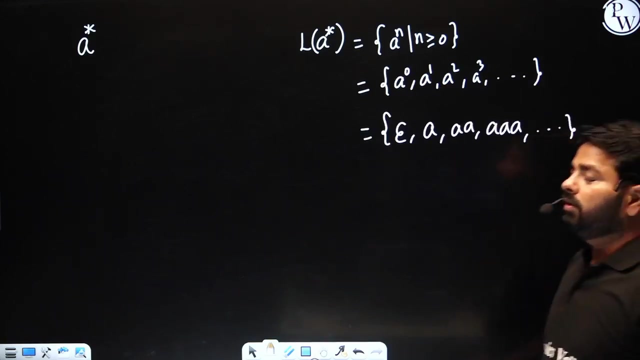 n, such that n greater than or equal to 0. or you can say: epsilon A power 0, A power 1, A power 2, A power 3, and so on, which will give you meaning of epsilon A power 0,, 1A, 2As, in a sequence, 3 consecutive As, and so on. Okay, So this is how you can understand. 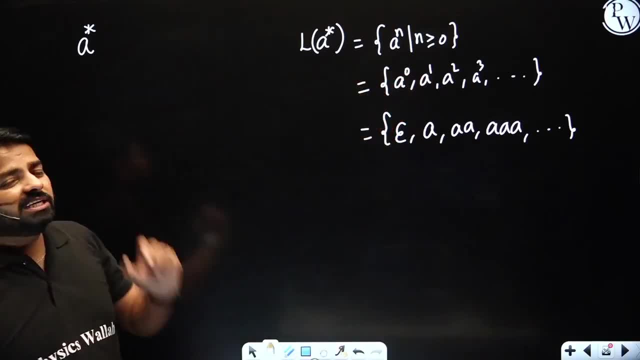 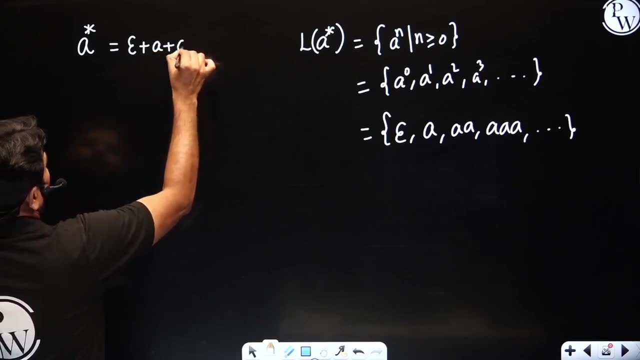 with the language notation, But in the expression it is the simplest. Some people may try to write it: A star is equal to epsilon plus A plus, double A plus and so on. But this is not an expression. It is just only to understand what it is right Expression, you know. 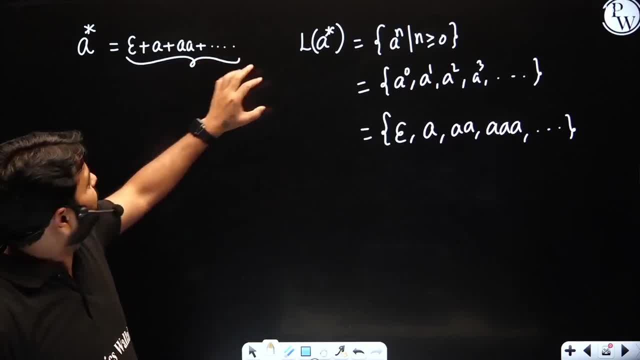 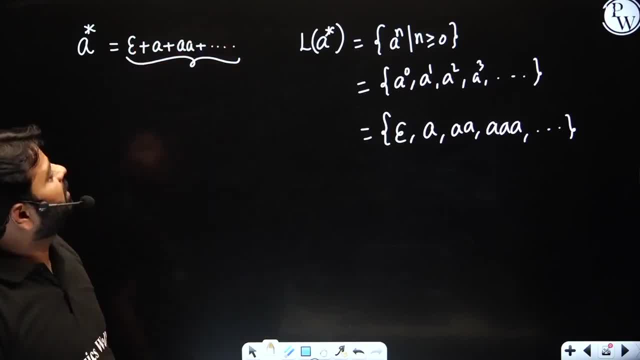 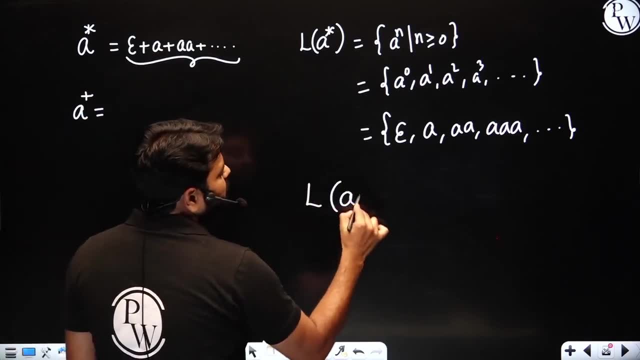 simple expression. It is a simple expression. It is a simple expression. It is a simple expression. This is a right way to understand, but not right way to express. Okay, A star means A plus. It means language generated by A plus. It means it is also A power n, but n begins from 1.. 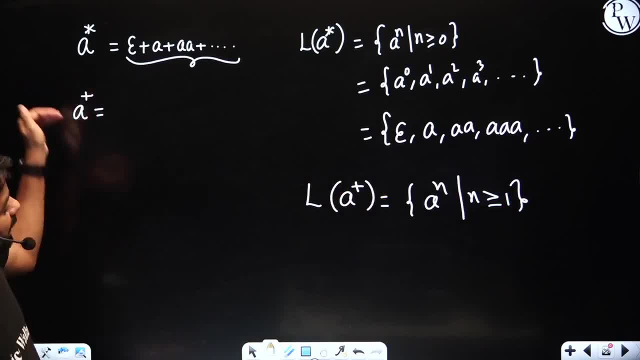 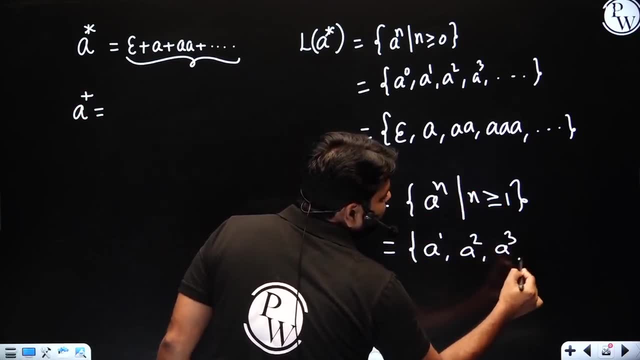 That means at least one A should present At least one time. it should repeat. So what do you mean by this? A power n such that n greater than or equal to 1? A power 1 or A power 2 or A power 3? 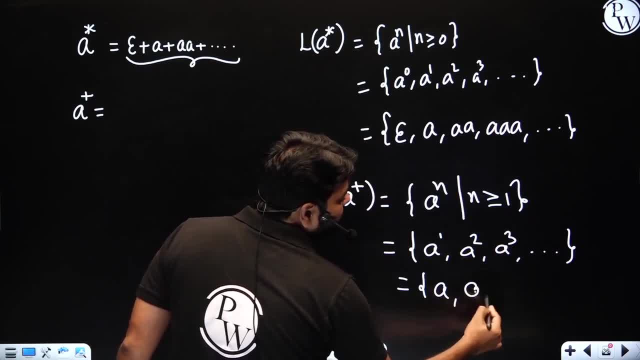 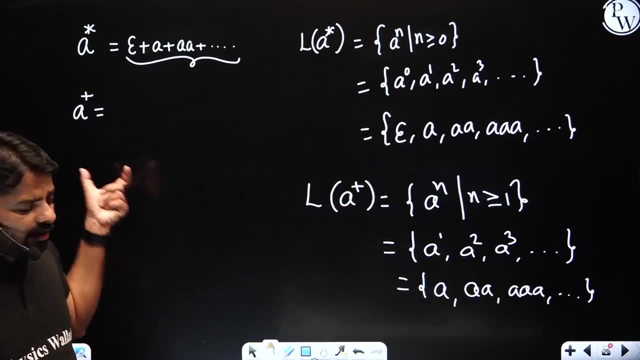 and so on, which will give you at least one A. Okay, Or you may have any sequence of A's if you want it. That is the meaning of A power plus. Whenever you write A plus or positive closure of A, the equivalent language is going to represent. 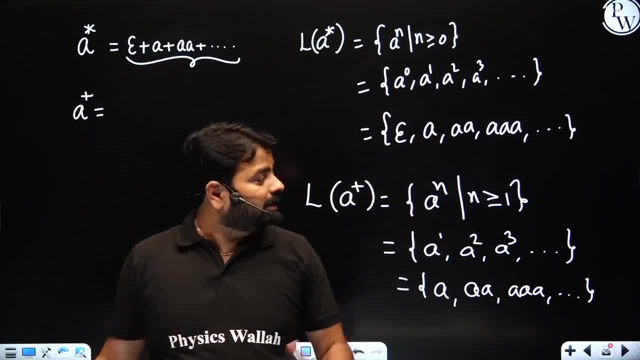 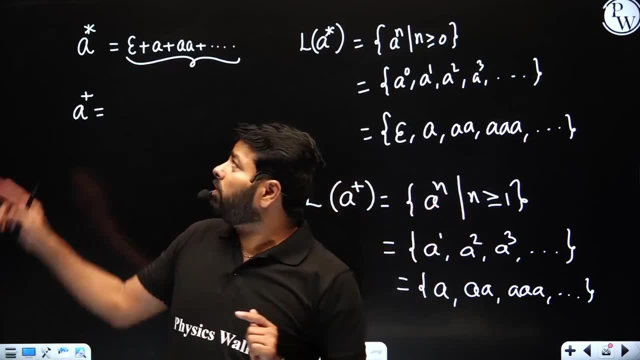 this one. So understand: you write expression but the meaning is here. As long as you do not convert your meaning into set, you might confuse a lot. That is what I am trying to express here with the expressions, but also I am explaining what is the meaning of that expression. 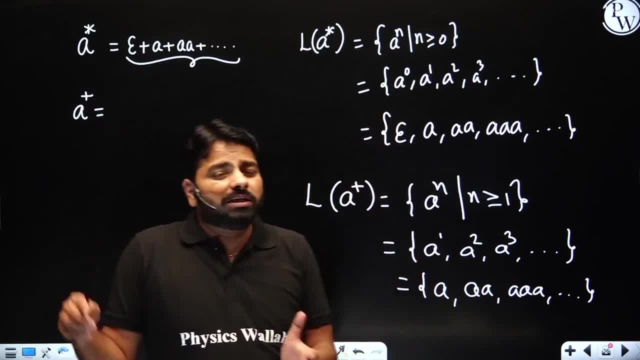 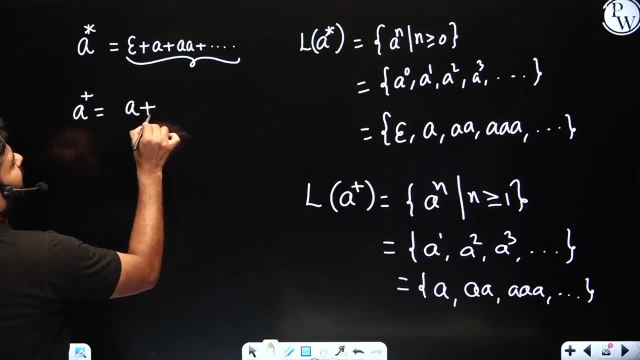 So always come to this language to understand what is the equivalent expression, What is the meaning of expression- Okay, I hope you got this- meaning Minimum A. or you may have 2 A's or you may have 3 A's, but writing this plus is not recommended, as you do not have finite number of. 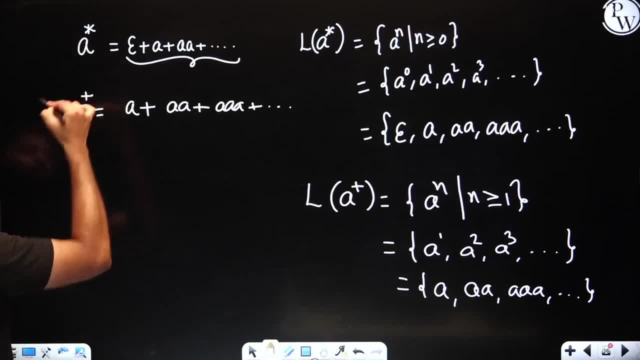 things to express. Okay, These are already simplest one. Now you got to know what is a clinic closure and what is the positive closure. Right, Clinic closure means it starts with the power 0 and it is a power 0.. Power 1, power 2 and so on. A power plus means it starts with the power 1.. So whenever you write, 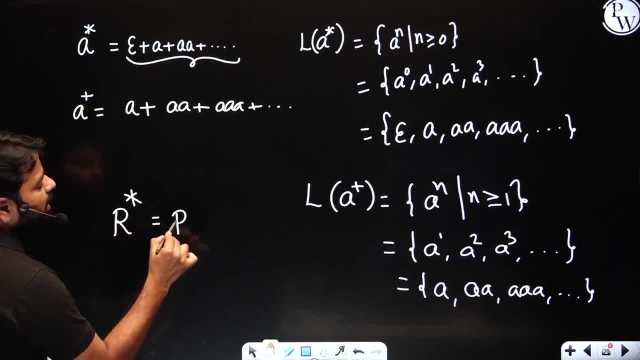 something r star you can understand- which is same as r power greater than or equal 0.. Whenever I write r plus the minimum, it should be beginning with 1 power. So this is how you interpret the clinic closure of r and positive closure of r. 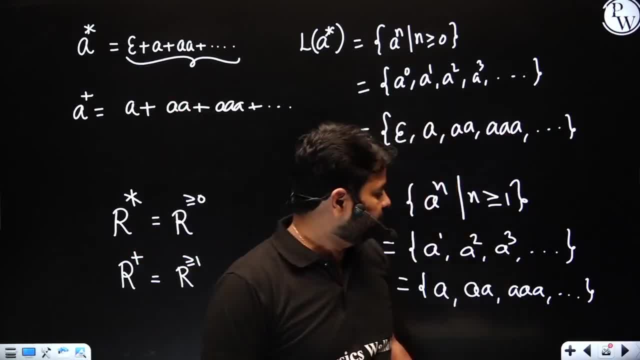 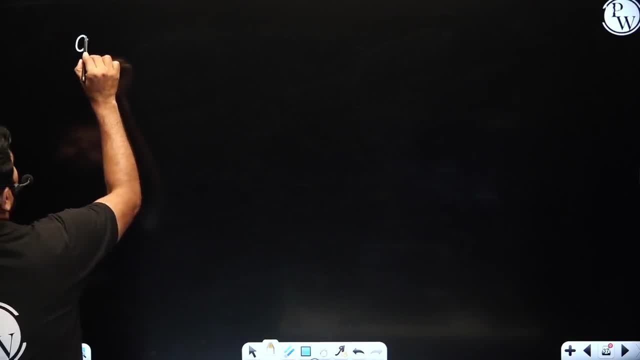 Let us begin with some examples to understand both of them. The first one: suppose somebody said A, followed by A star. What is the meaning of this? Can you simplify further? Yes, it is possible. Let me explain one regular expression when you write. 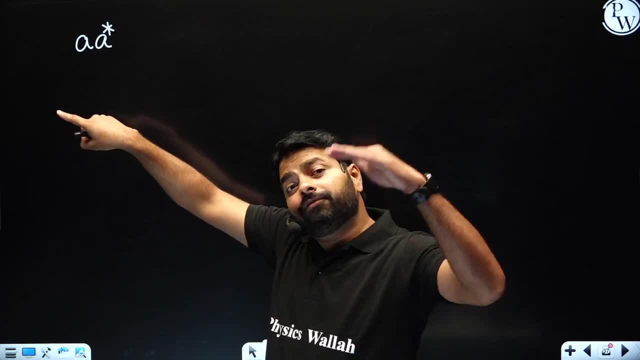 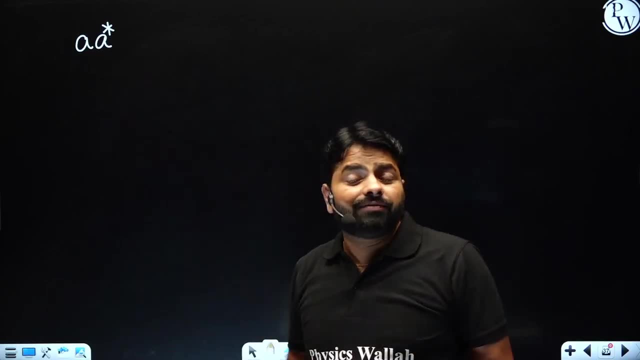 here and to represent the same meaning, you can write infinite equivalent expression. That is why it is asked most of the times in the gate. You know A, A star has infinite answers. Are you able to look at the four options which are given to you to find out which is equivalent here? Because 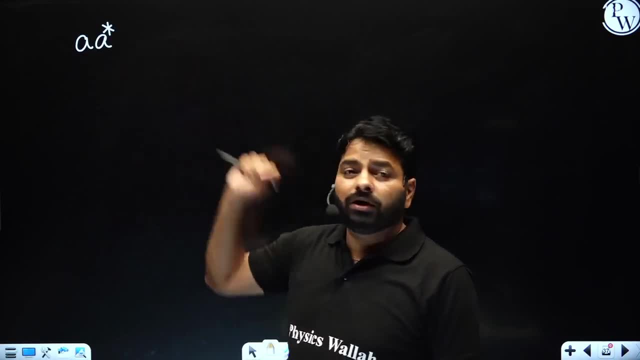 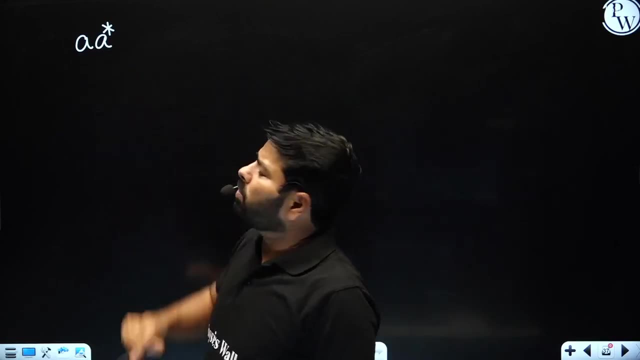 we will have four options in the gate and out of this four, how many are equivalent to this? As you know, there are infinite equivalent answers. are there A? A star? what is the meaning of A A star? Look at that. A is always there- A star. 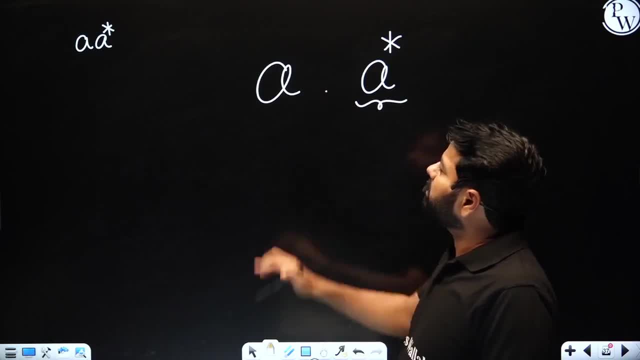 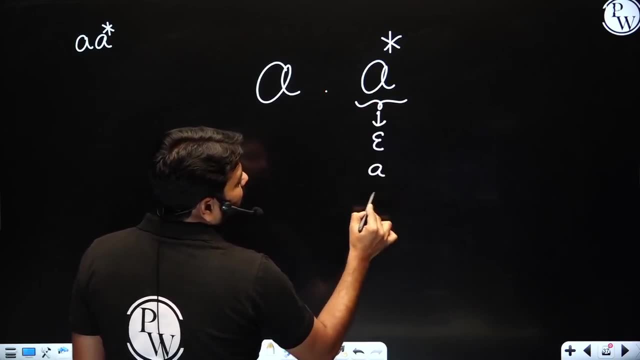 this: A star can generate anything, But there is a dot means compulsory. these two are there. This will always give A, But what it gives, It can give epsilon or A, or double A or triple A and so on. When this A is taken with epsilon, what do you get? You get A epsilon, which is A, When you take. 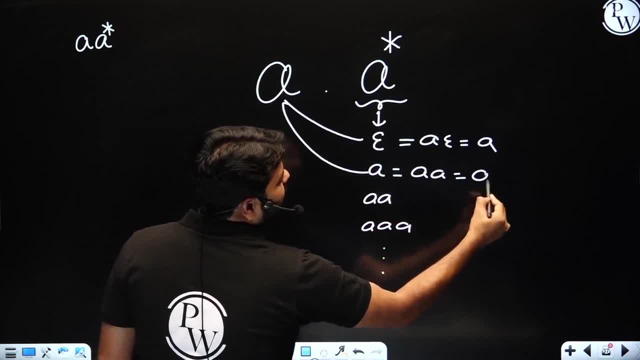 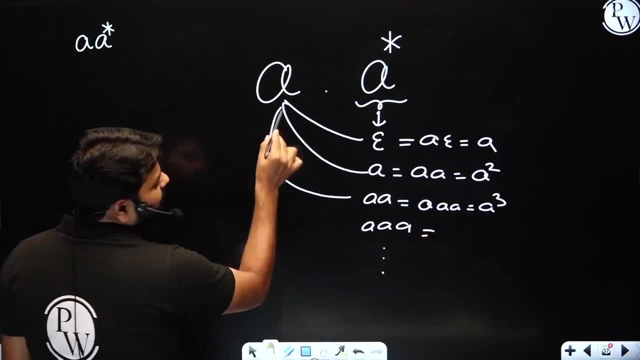 this A, followed by A, you get A, followed by A, which is A square, and when you take A, followed by double A, you will get A, followed by double A, which is A power 3, and definitely A, followed by triple A, because dot is there. That means you must take this A always, So A followed by 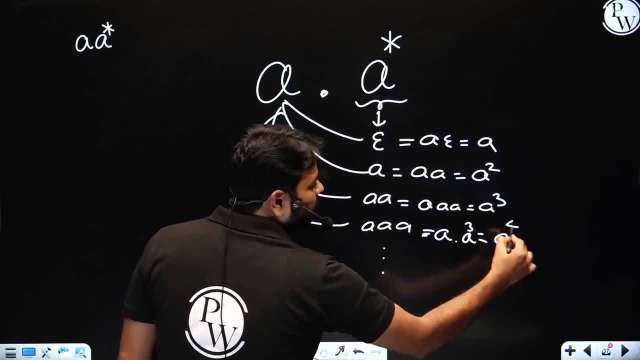 A power 3.. This is A power 3, right, A power 4. and what did you get? It is impossible to get epsilon. Epsilon is there only one side, but not both the sides. When you have both the sides. 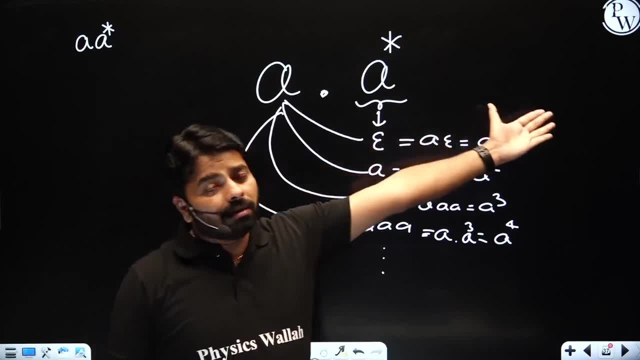 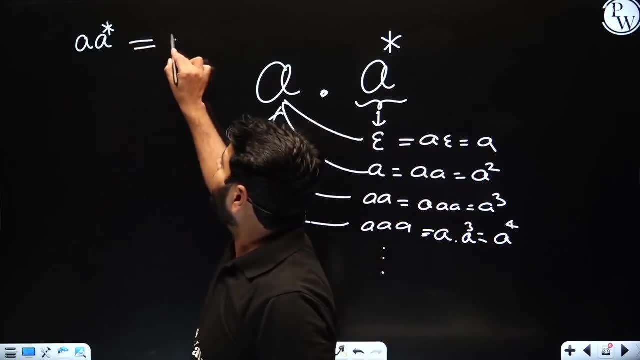 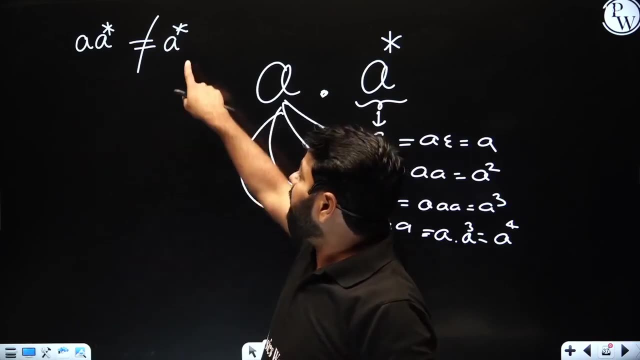 the result will become epsilon. See, epsilon will never come out, but minimum string is A, then followed by every string comes out. So whenever somebody thinking which is equal to A star, it is always wrong. Why? Because the A followed by A star will not be A star, A star. 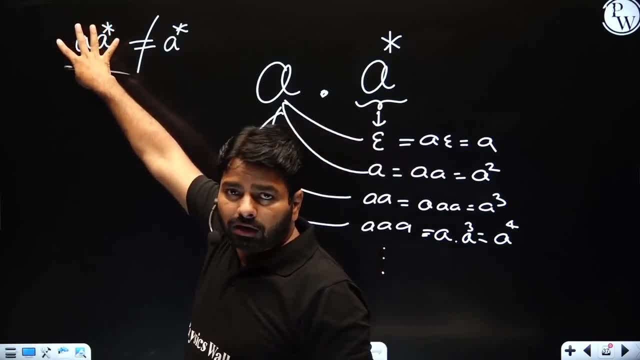 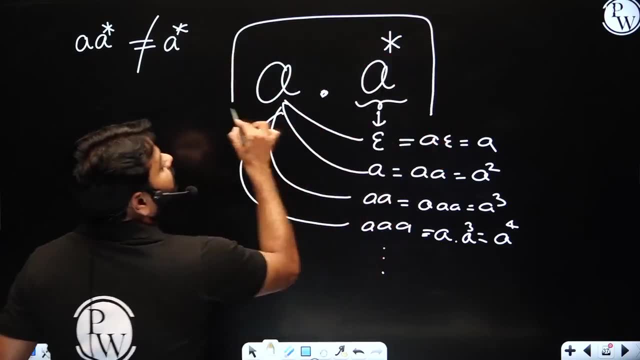 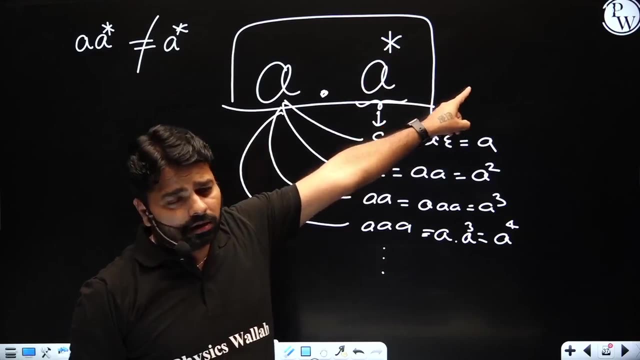 will have an epsilon, but A? A star will not have. Why, Even though A star has an epsilon, but A? A star has an epsilon. So when you think together, A epsilon become A. it is not epsilon. So it is very important, do you have an epsilon or not, except that everything is there. but 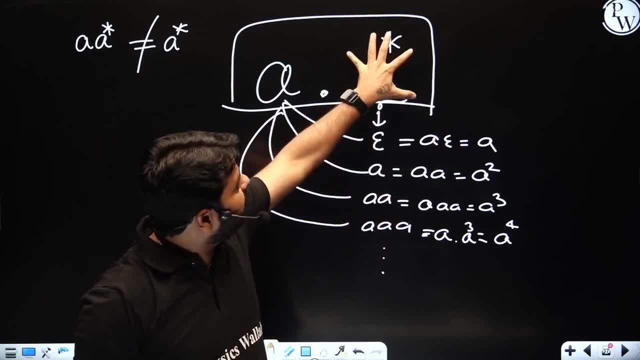 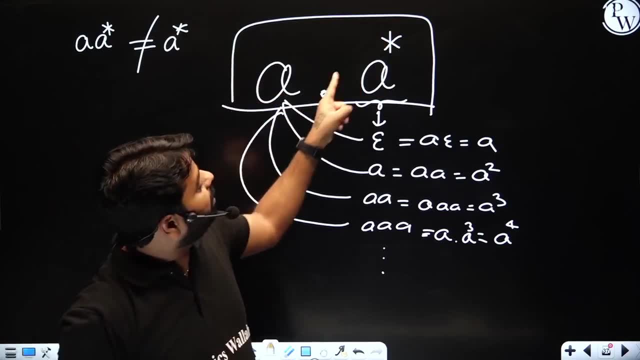 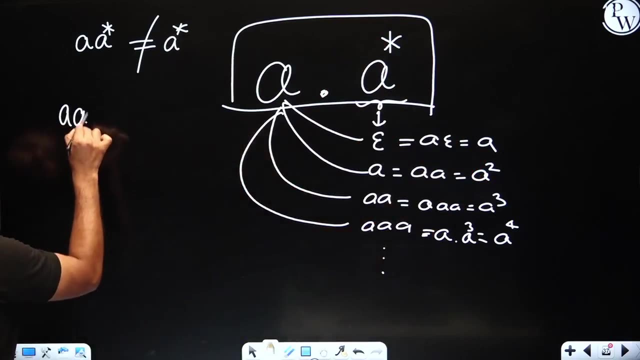 only epsilon is not there. Why it is not there Here? epsilon is there, but this is not only one in this expression, because other always there, Other always there. That is why A dot, epsilon, will get as A in one choice. Now, what did you understand from A, A star? What? 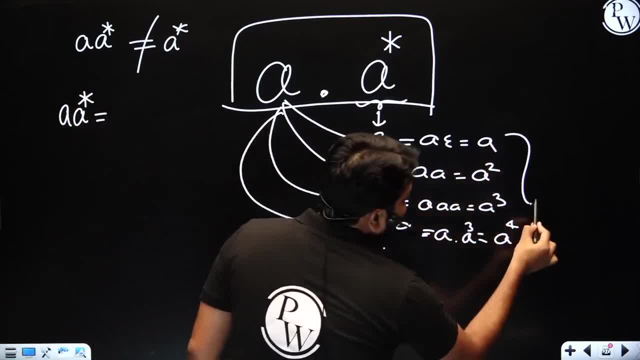 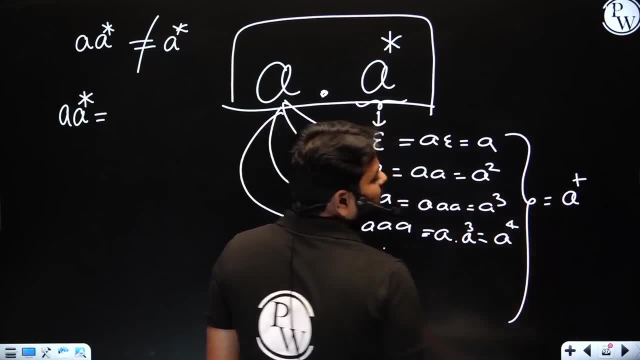 do you get? What is this conclusion? A plus A power plus 2, A power 3 plus so on. it is equal to A plus Yes or no. A plus Not only this. If I say A star followed by A Okay. 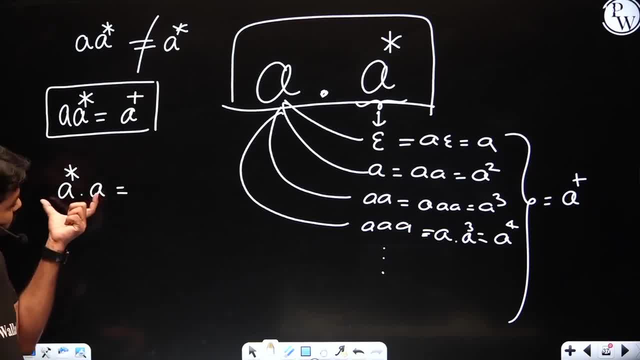 This time first epsilon, then followed by A, and together it will get minimum, A, Minimum A, Then A square. how do you get? Stop a, followed by a, a square, a square followed by a cube. so here you will have again a plus. now look. 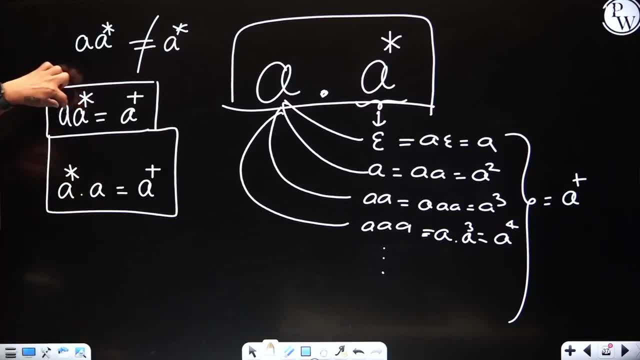 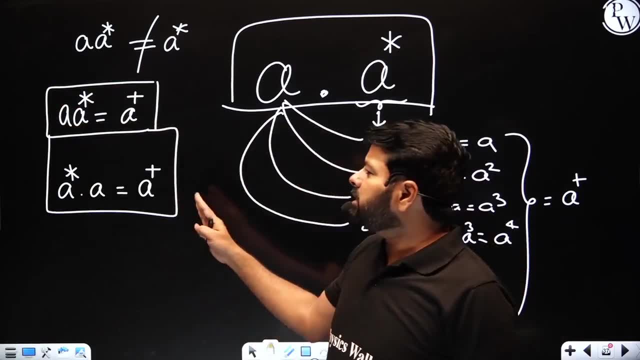 at these two expressions. even though you change the order- a star, a or a star- you get the same answer, at least one a in the language right now. this is the important point. now let's come to the another conclusion. when i use the dot, you got this meaning: right now, i'll go for a plus a star. 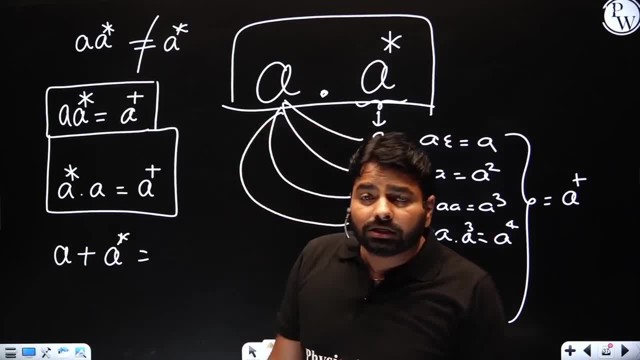 now something different. both are not compulsory all the time. see, i want to generate this thing. i can go to left of the plus, or left to the plus, right to the plus. you can go any direction. right, if i go here, i can generate a. if i go here, i can generate a star. now tell me, when you talk about 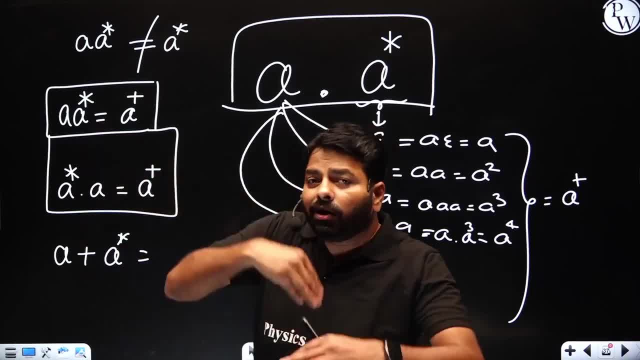 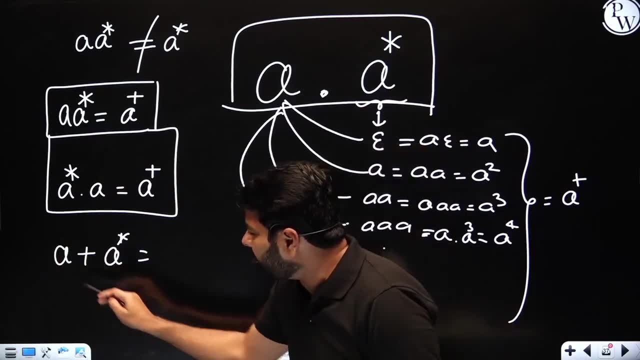 the plus, it's nothing but union. when you talk about the dot, it's a followed by. that's why you are not able to generate epsilon from here. but can i generate epsilon from here? you can go this side or this side. if i go this side, i can get epsilon. that means a union, a star. you. 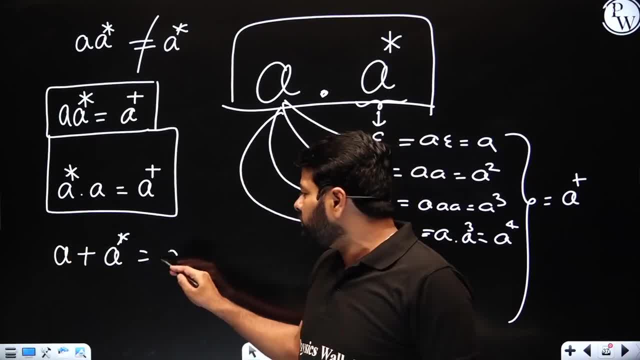 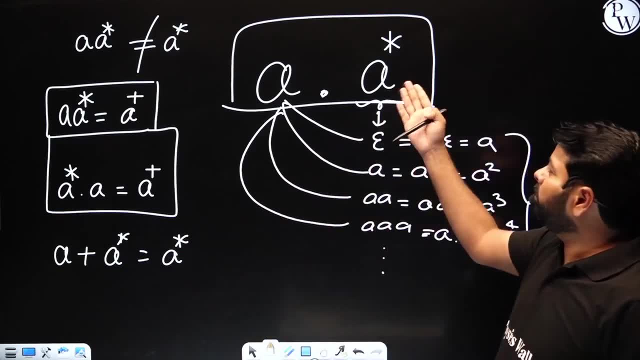 can see a star. why? because they are already present in a star, so you can write a star. now understand the difference. how did you get a star here, here? how did you get a plus? this is equal to a plus, but a plus a star is a star. where is the difference between these two? 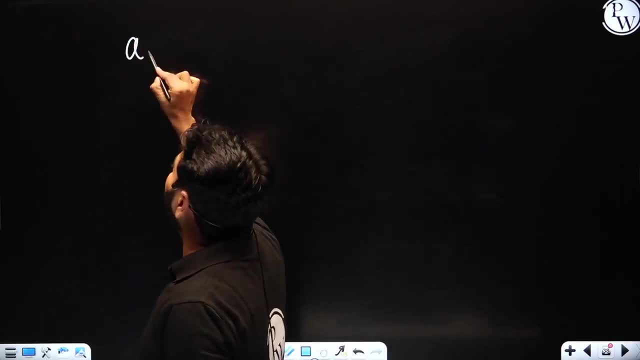 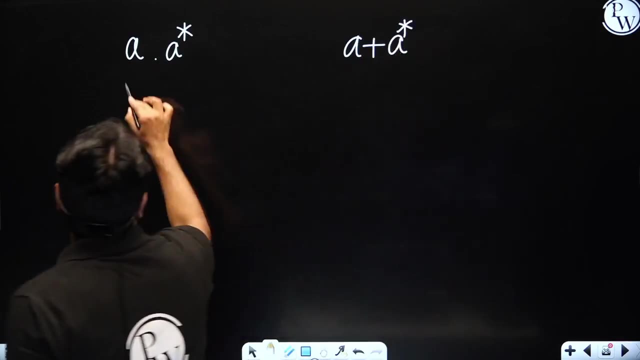 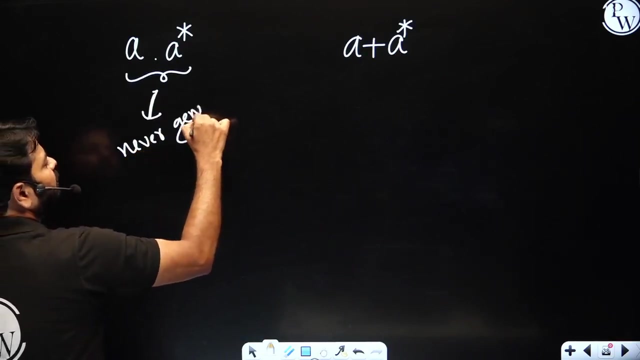 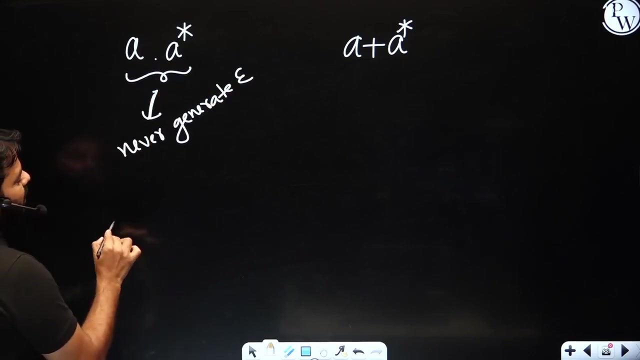 you need to analyze in the beginning, only later on you don't come to this right later on. you will never come to this. these are the very basic questions, and this will. it's impossible. never generates epsilon. how did you, how did you know that? because minimum string is a, a dot epsilon, minimum string is a, so which? 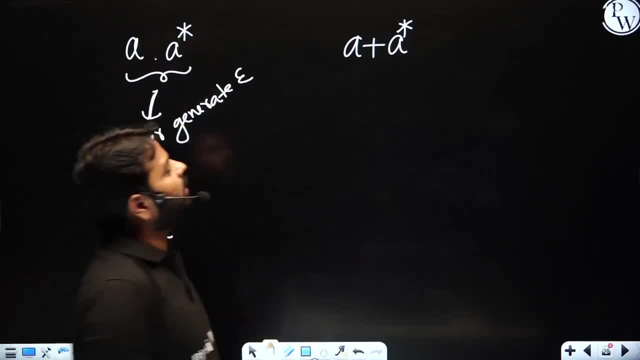 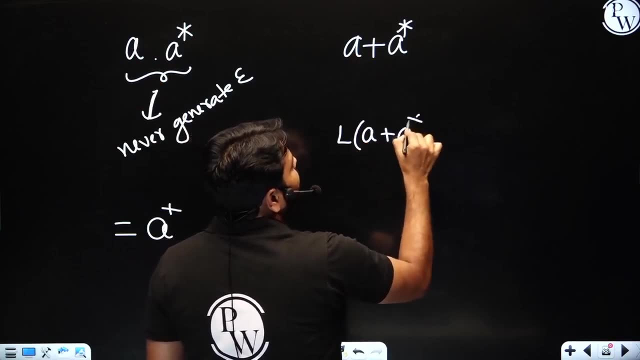 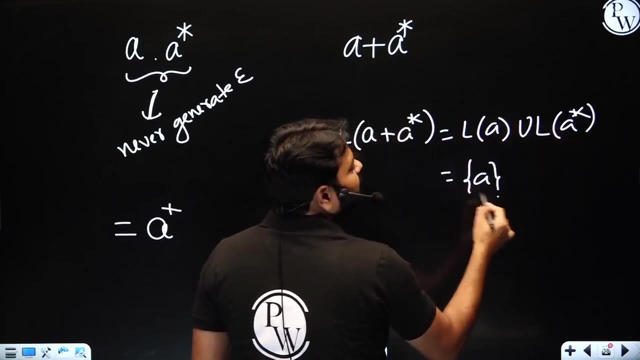 is equal to a plus, as you can generate a power, two power, three and so on, but here this is a plus, it's it's same as, like you know, even i ask l of a plus a star, which is same as language generated by a union, language generated by a star, even though this gives a but that's not. 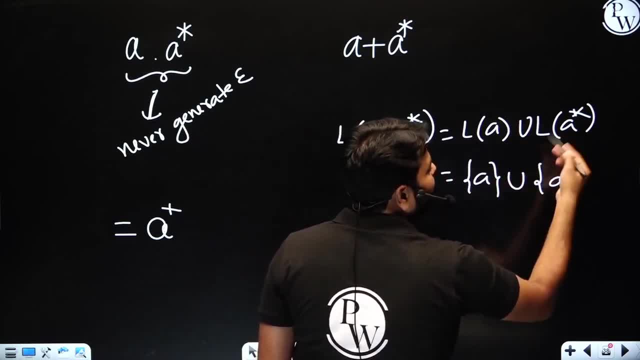 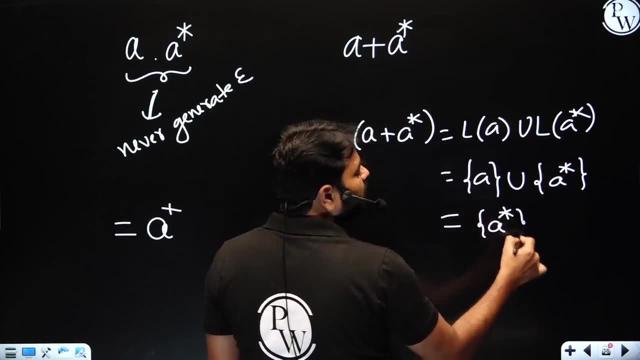 compulsory when i take a it's union. it's whatever a star generates. you know, whatever a star right together, what it generates a star, only all the strings which are generated by a star will be here. right, this is how you get it. a star means here you will have epsilon, you have a, a square. 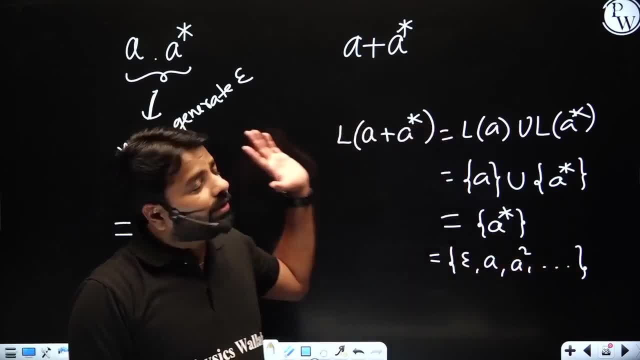 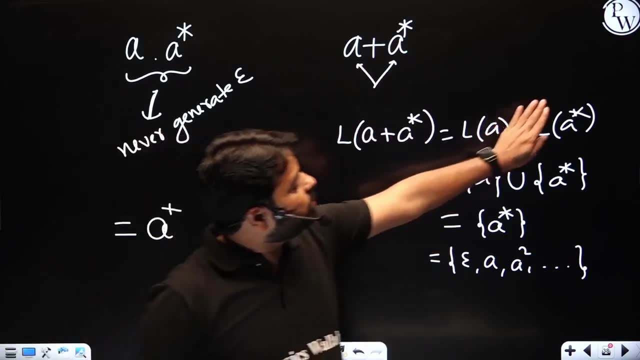 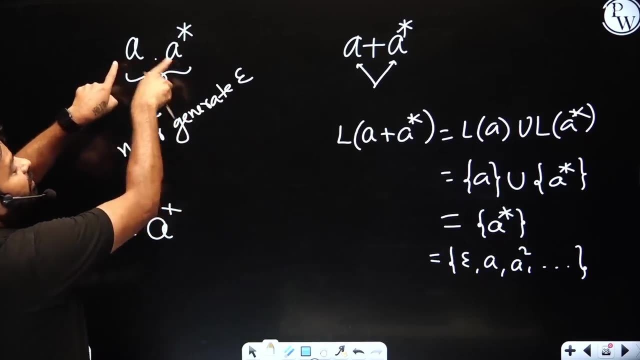 and so on. here only one doubt. so how did you get epsilon? because this is r, you can go this side or this side simultaneously. so these two are independent expressions. you are doing the union, but when you go here, they are not independent. they are dependent one after other. 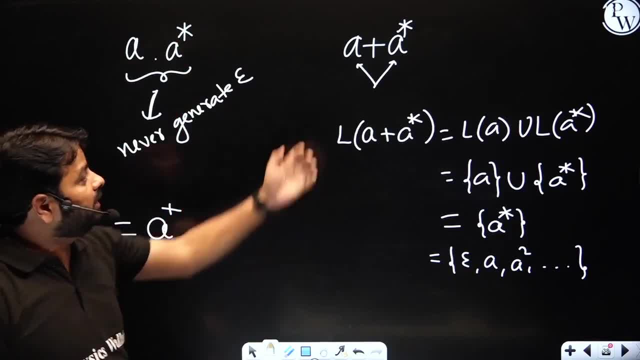 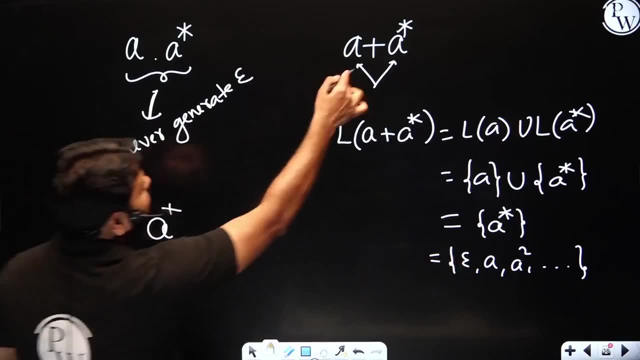 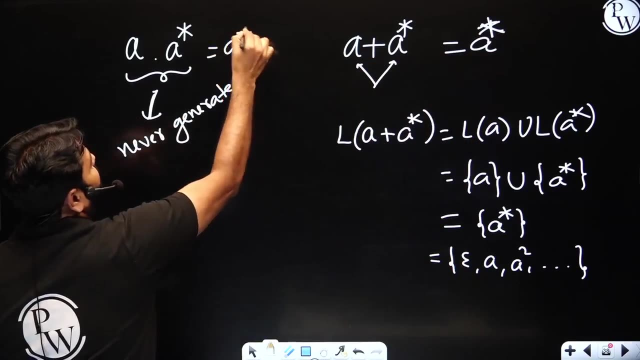 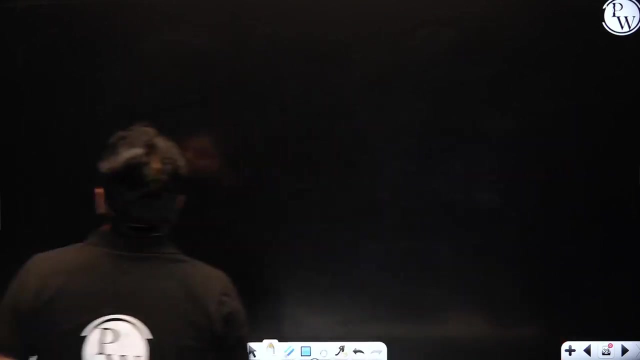 that's why this epsilon cannot be pulled separately, but here this epsilon cannot can be pulled. you can generate any point of time separately as a spring. so this is the difference, and that is the reason this is equal to a star. this is just equal to a plus. okay. similarly, you can think about various expressions. i'll just write some of them, you just 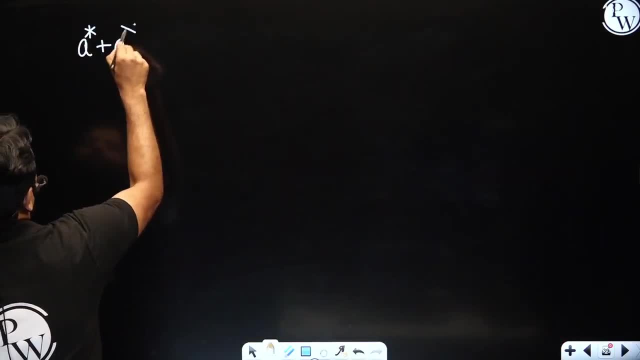 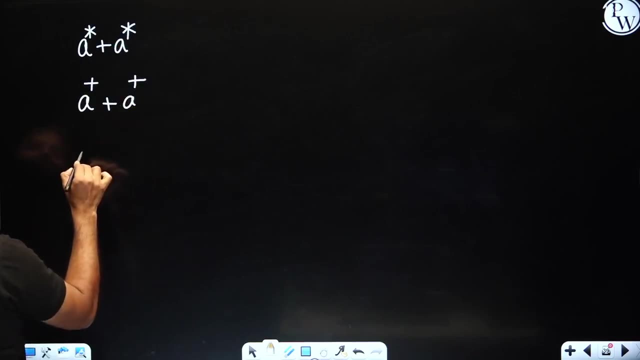 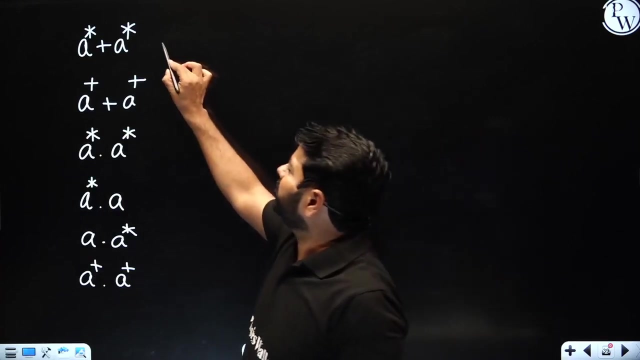 think about it: a star plus a star. just think about it: a plus plus a plus. no confusion. i may write many things here, but don't confuse any of them. i'm repeating them. okay, few things only. as you know, there are many questions to solve here. if these are the basics, 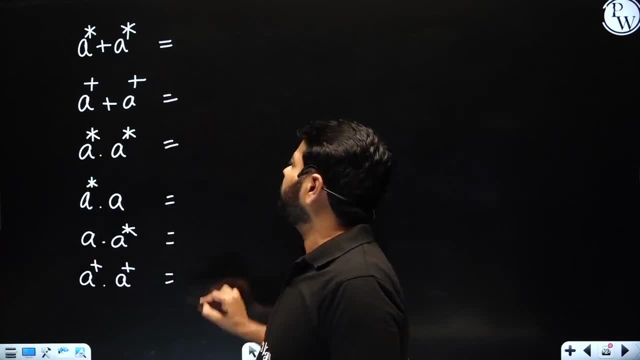 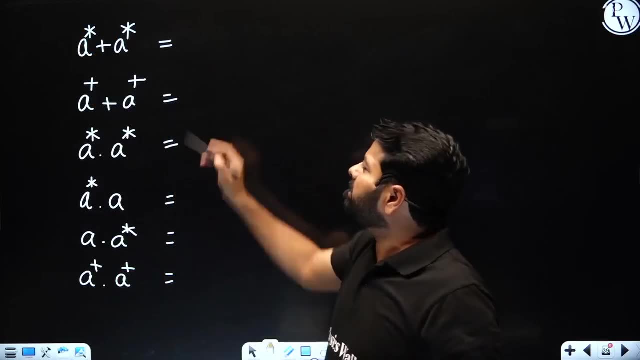 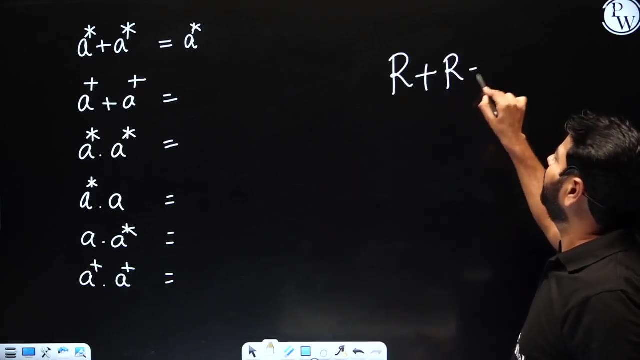 then we'll begin with the questions after this. okay, let's start with the first one. a star already generating every string over a union with again a star, you'll get the same, right you know for this, no, no difficulty. r plus r what it should be, r there's no doubt about it. right, you know you can. 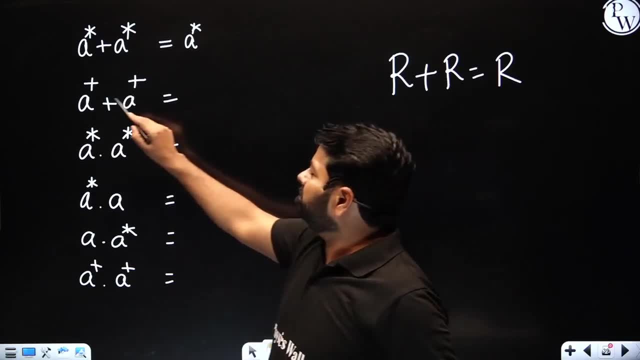 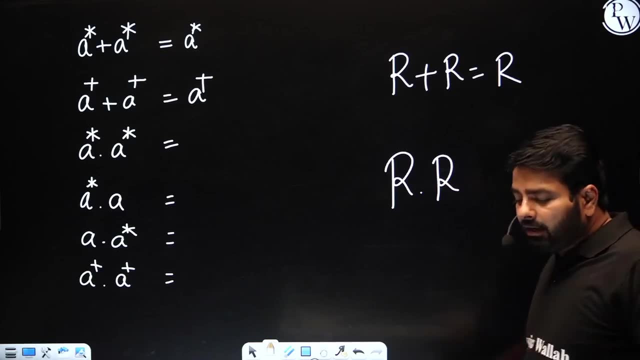 so whenever you have such situations, be careful. r plus r, r only, but only. the thing is, when you are saying r dot r, you may get r, you may not get r. that depends on what is inside. r, remember, need not be equal to r. it could be r square, but r square might get r, might not get r. 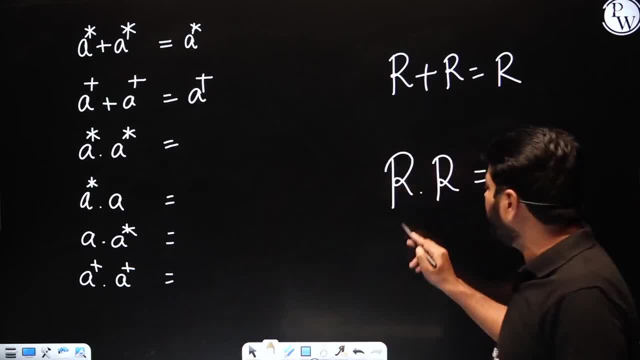 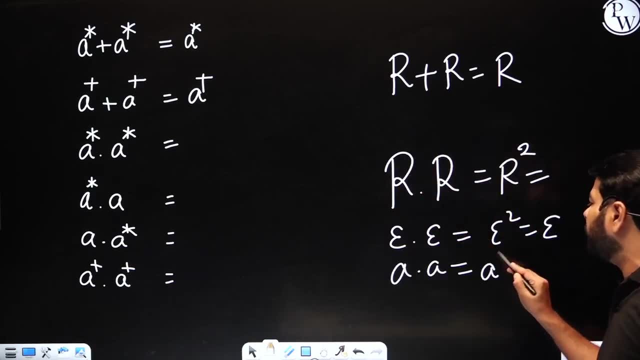 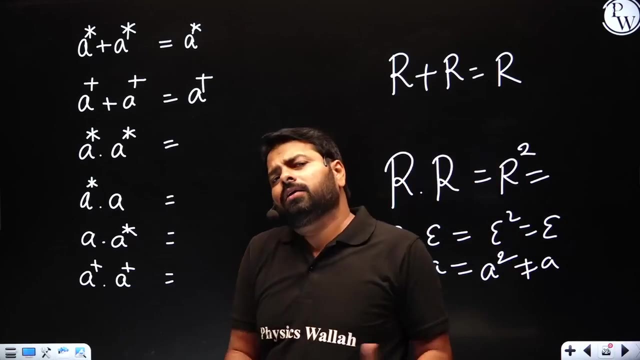 depends on what r is, what r is. suppose if i take r is epsilon, epsilon, dot epsilon, then epsilon square is again epsilon. if i take r is a, a dot, a, which is a square but not equal to a, understand what r is. if r is something which can give r again after r square, that would be special. 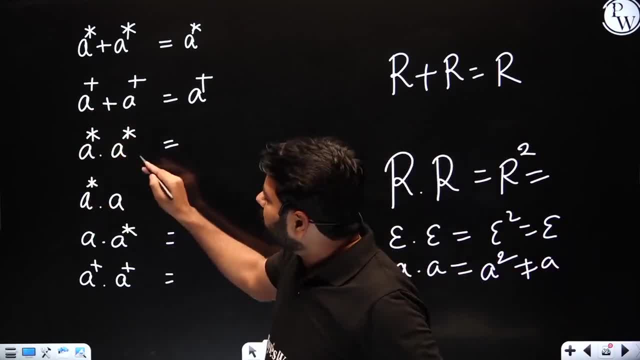 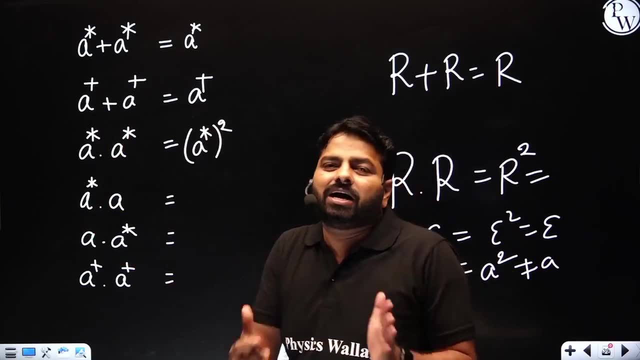 case. but here a star, a star dot. a star is what? a star square, let's say correct, because you are repeating twice. but when you are repeating a star again and again, what do you get? can i get epsilon from here? yes, both are having epsilon, so that you can get epsilon. 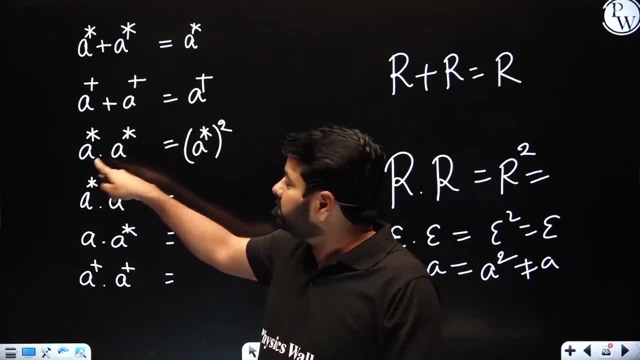 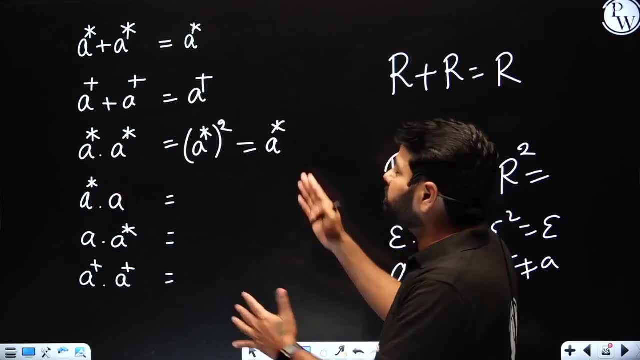 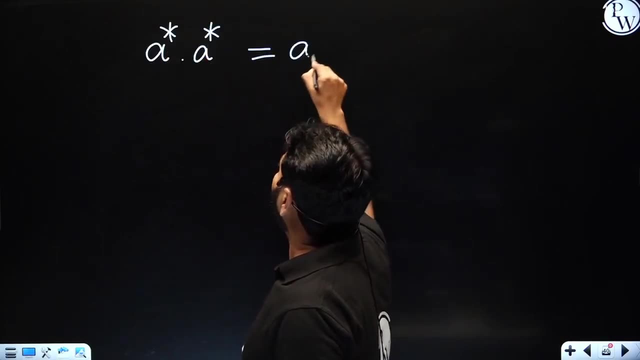 can you get one? yes, yes, yes, a yes. first one, i can put epsilon. second one: i can put a. so epsilon dot a is what a is again a star. so now i need to explain: how did you get a star, a star dot a star? why did you get a star? look at: 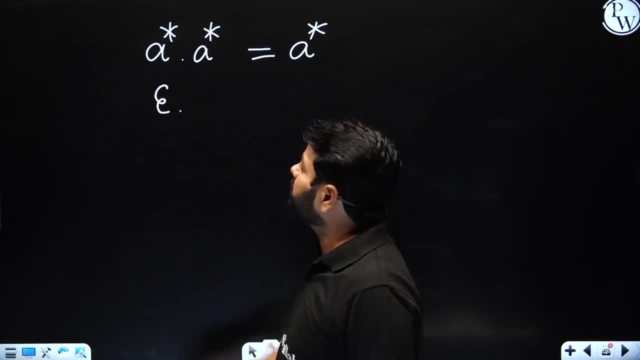 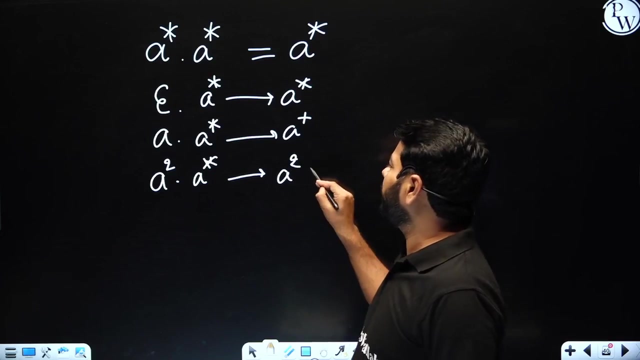 here i will put epsilon all the time. even though i have infinite choices, i put epsilon now. i'll just take a star. one case i have a star. other case, maybe this is a a star, this a plus, and this may be a square dot a star. it's something like a square dot a star. but whatever, you get all when 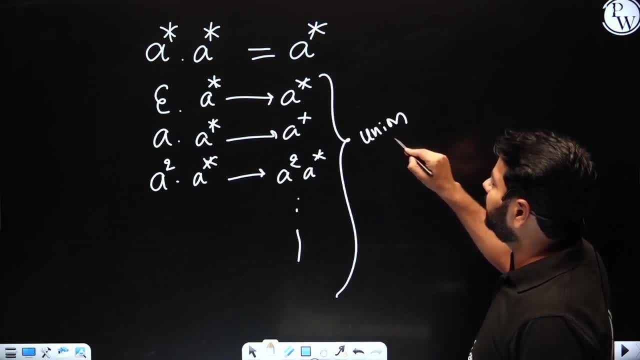 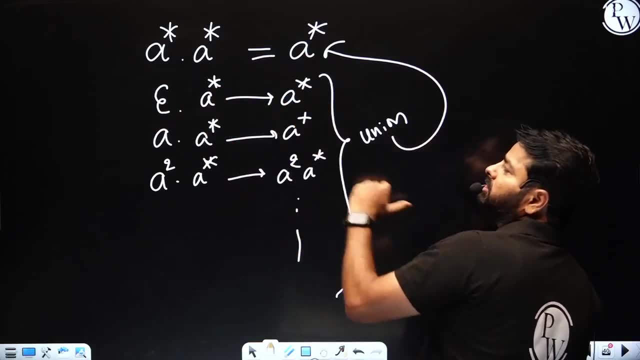 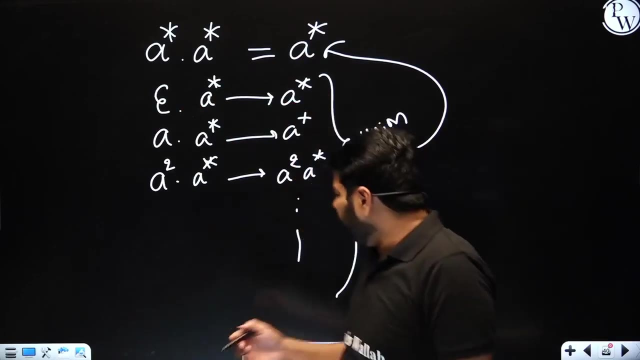 you do the union union. combine them. you will get a star only because a star will have all of them. a star is also part and remaining all are recovered in a star. together it will become a star. i hope you got the point right. it's just like union when somebody is having all union, some, some, some, some. 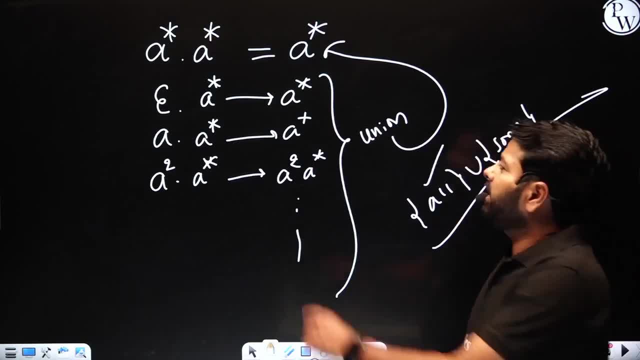 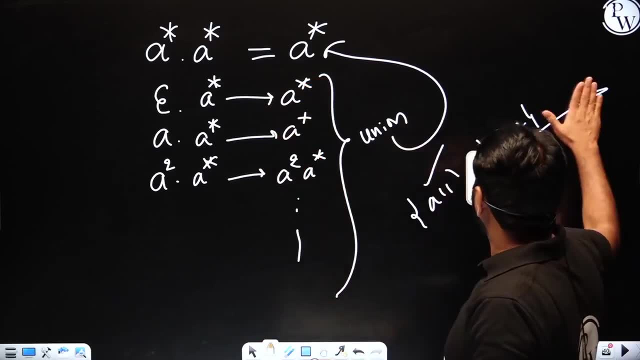 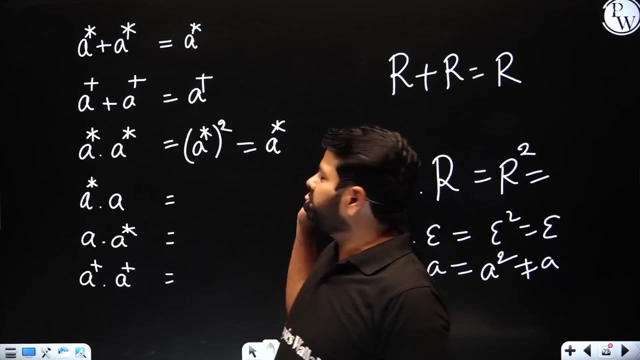 right. the result has to be all right. the same way, here a star is having all the strings. you are doing the union with the you know some subsets only. so this is the important point for you now: a star dot a star is a star. you can also write a star whole square, but don't write a square whole. 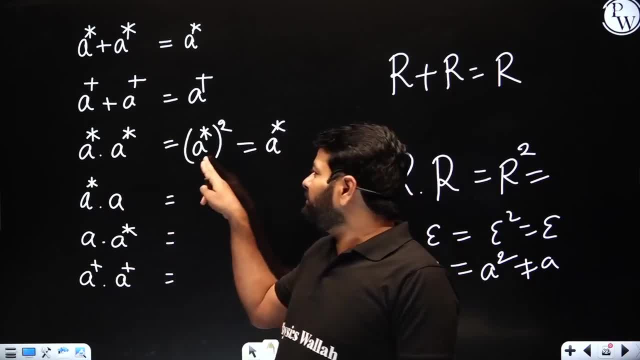 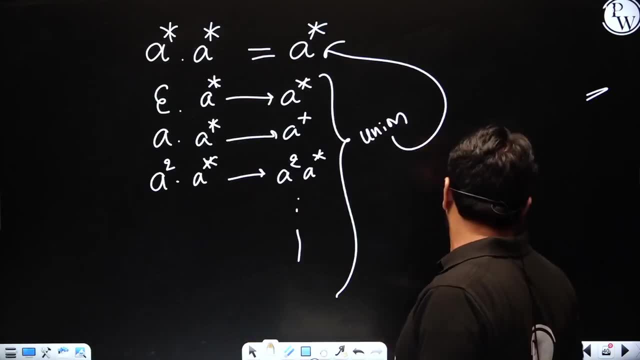 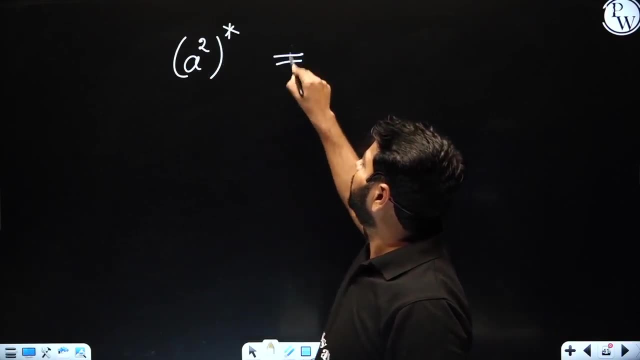 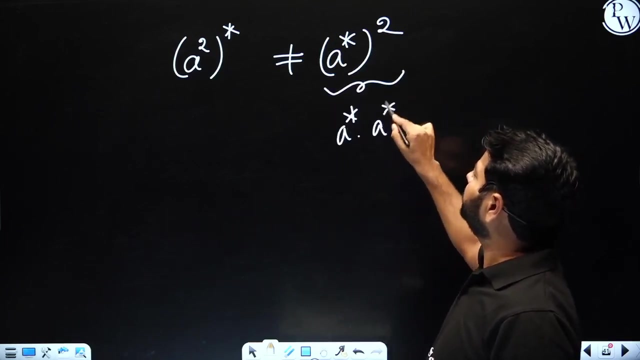 star. it's not just mathematics, right? so be careful. a star whole square is different from a square whole. you may ask me, sir, can you explain a little bit about it, okay, a square whole star, why it's not equal to a star whole square? this is just now. we understood a star dot, a star which is equal to. 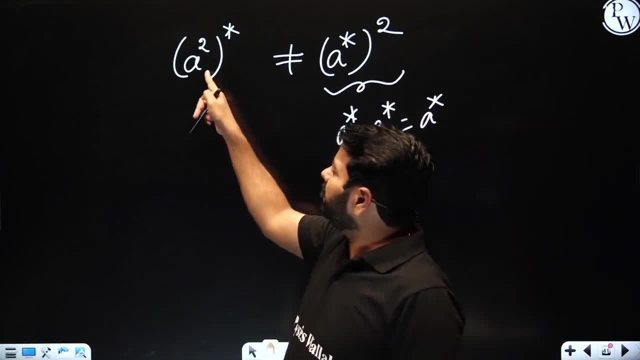 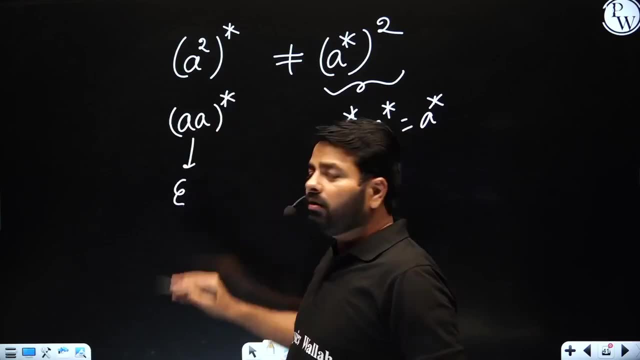 what a star this one and the first one, this a square, whole star is. it's actually represent double, the whole star means which will generate epsilon when you put double. this a power zero, and it can generate a square, how it can generate when you put double a power one. 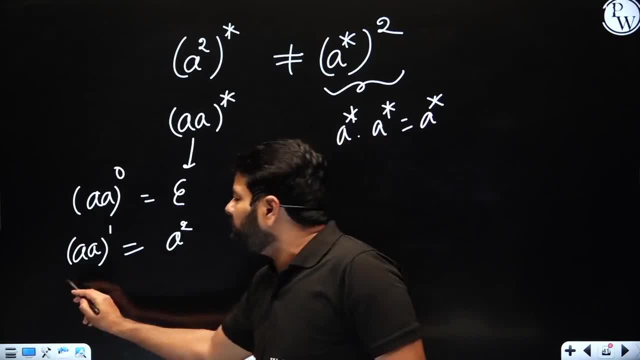 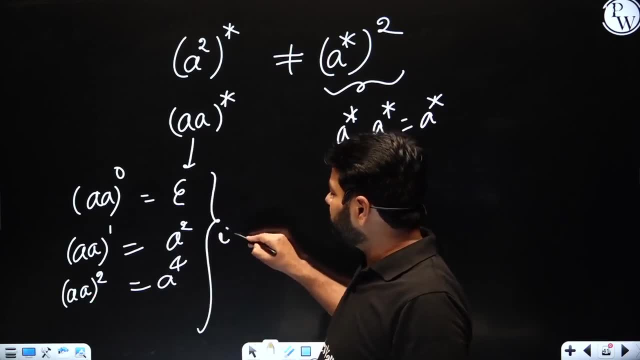 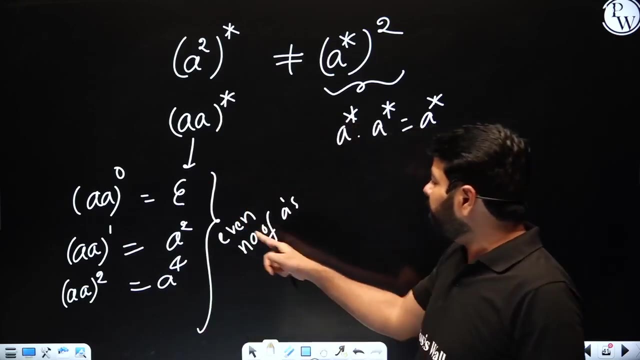 which is double a, double a- nothing but a square. next, double a power two means two a's. you write twice, you'll get a power four and you will basically get even number of a's, even number of a's in every string that generated by the expression okay, even number of a's here. this: 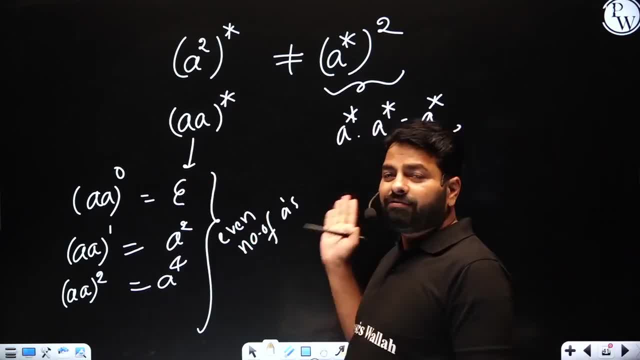 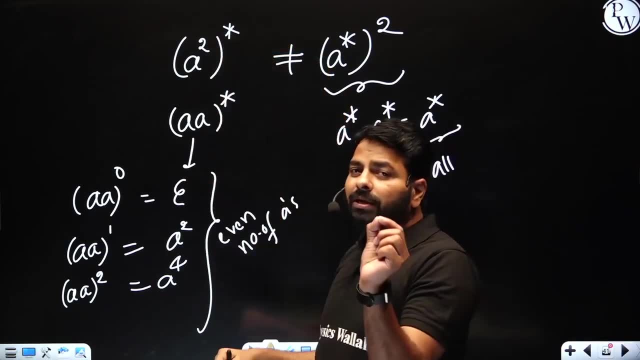 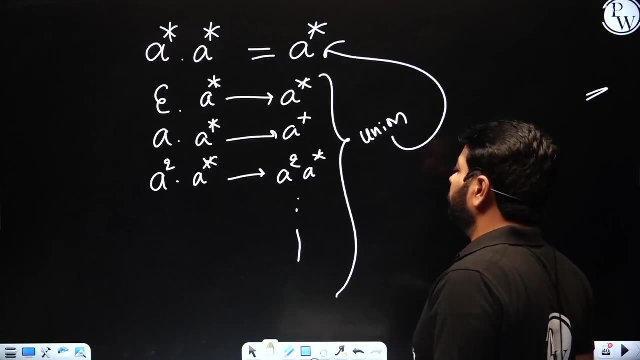 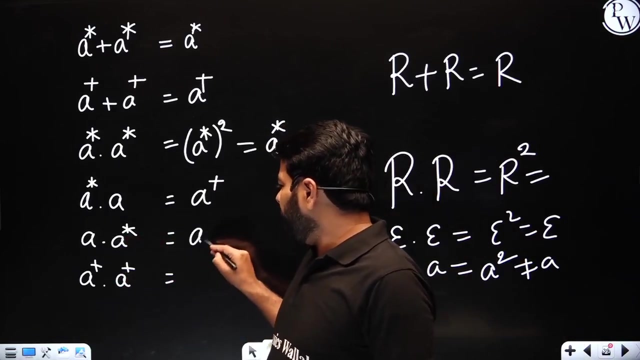 represent all a's. okay, that's the main difference. relation is like: this expression, whatever it generates, the language entered by this expression will be strictly subset of the language generated by this one, so that subset relation exists. come to the point: a star, dot, a. just now i explained a plus a dot, a star, a plus. 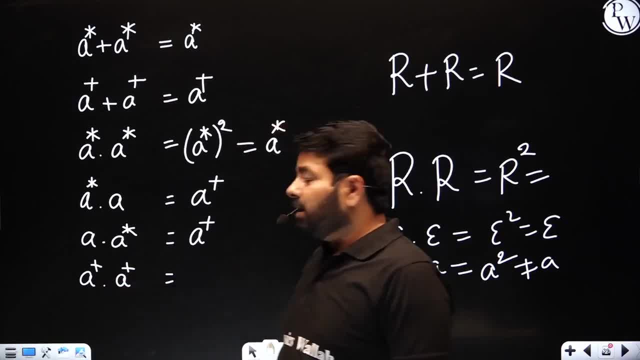 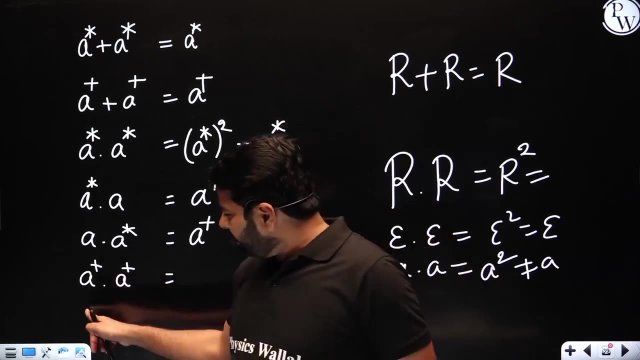 a plus, a plus, very interesting. can i write a plus? think about it. a plus, dot a plus. can i write a plus? if i write a plus, that means you are trying to say i can generate one a. can you generate one a here? see minimum one a here, followed by minimum one a. one a, followed by one a. is it one a? no, right, two a's. 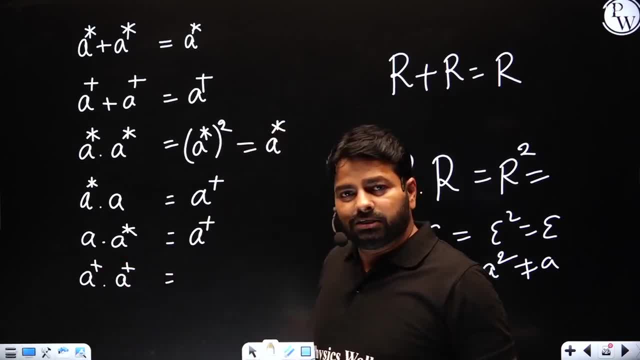 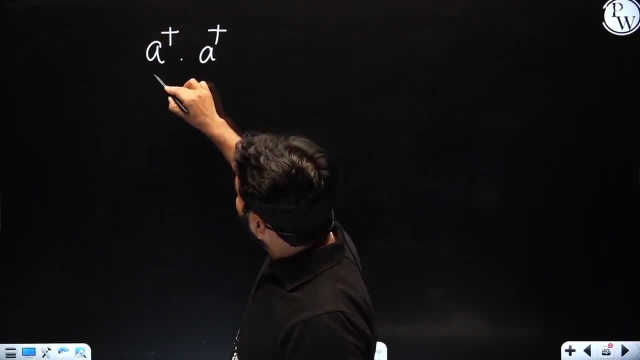 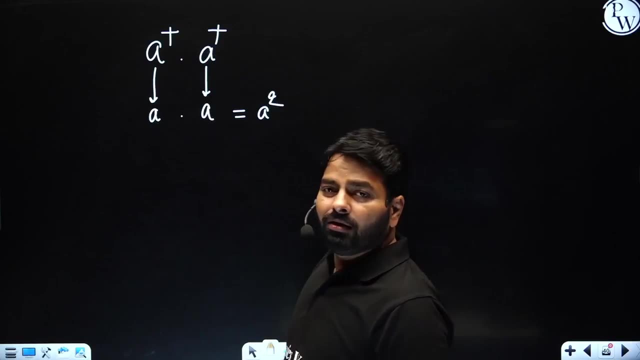 so here it's impossible to say a plus, okay. just conclusion: a plus, dot, a plus. understand, what is the minimum here, a. what is the minimum here, a. so what do you get when i concatenate a square? okay, later there are many choices. i can take a here, here i can take a square. next minimum: 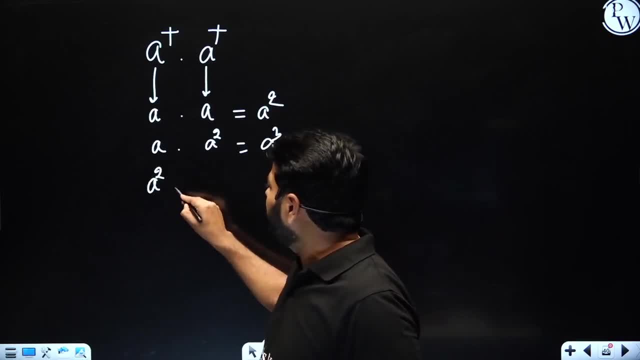 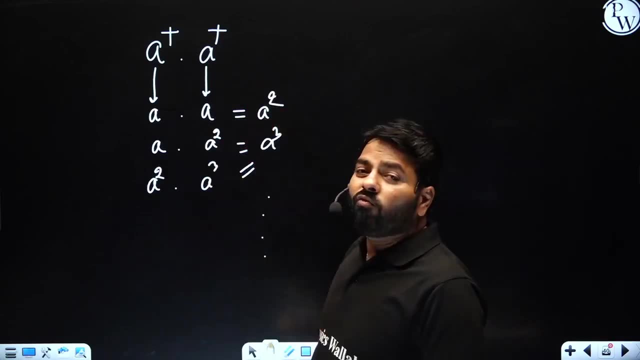 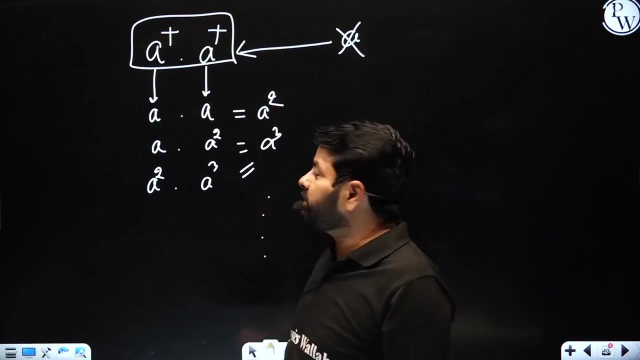 to get a power three, or i can take a power two here or a here. you will get the same: a power three. like this: you can get every possible string after this, but here one a not exist. here here a not exist in the whole expression. i am talking about not a part of the expression. 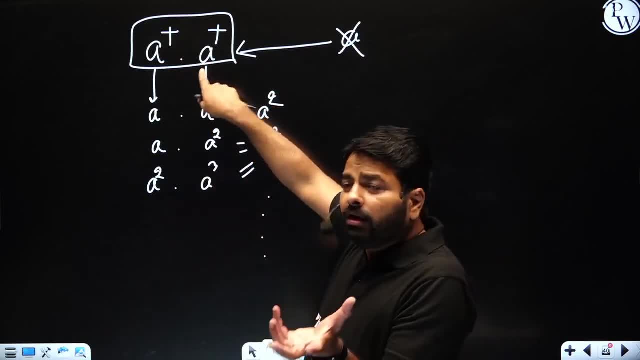 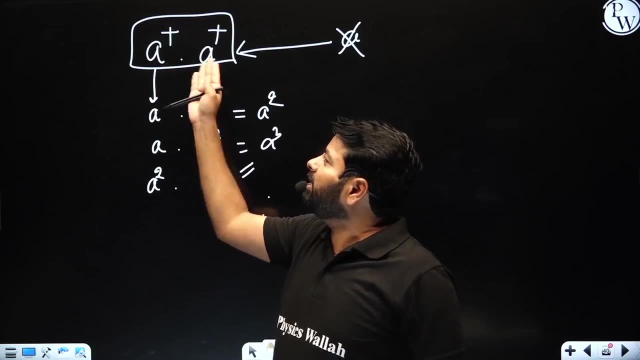 because it's a concatenation in the part, it may generate a, but all together it can't generate a a part of the expression because it's a concatenation in the part it may generate a epsilon impossible as minimum one length of in each sub expression. fine, now what is this means? 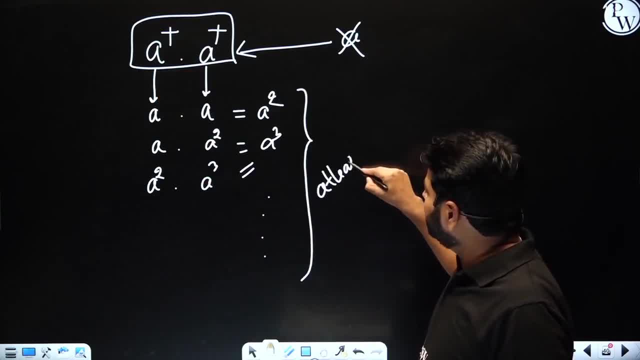 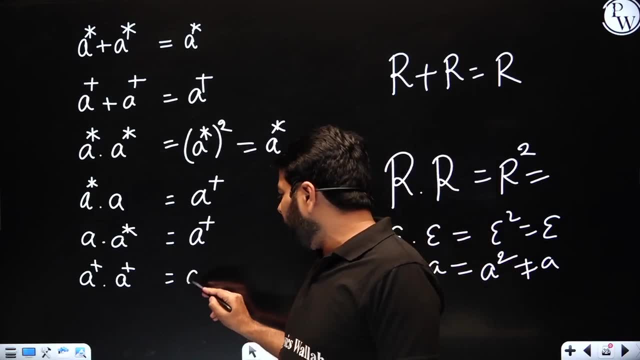 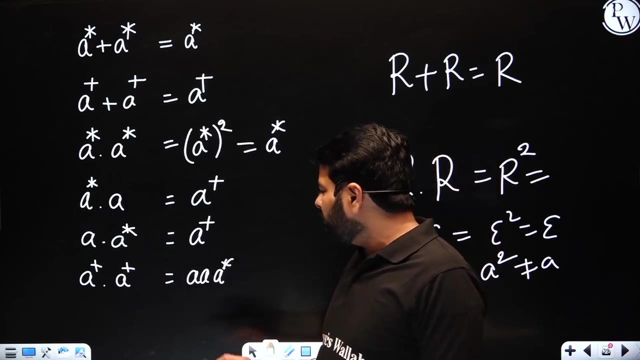 at least two a's. the meaning of this result is: at least two a's you can generate from the expression. how do you represent this? two a's you can generate remaining any number of a's you can generate. either you can write a star separately here or you can write a a plus. 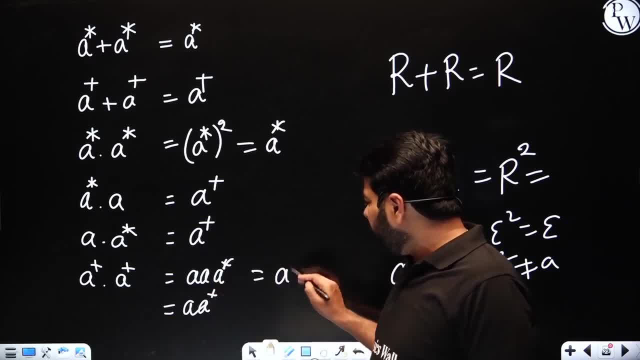 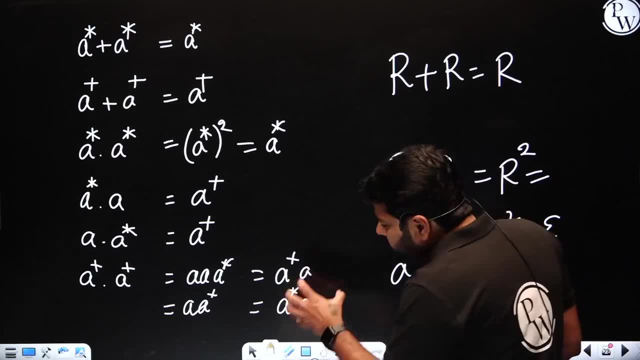 this: a, a star. you can also write a plus, or you can write a plus a or what else? you can write a star, double a. so many ways to represent. but each of this expression is trying to say i will generate at least two a's. but how do i generate that? depends on how do i express using clinic. 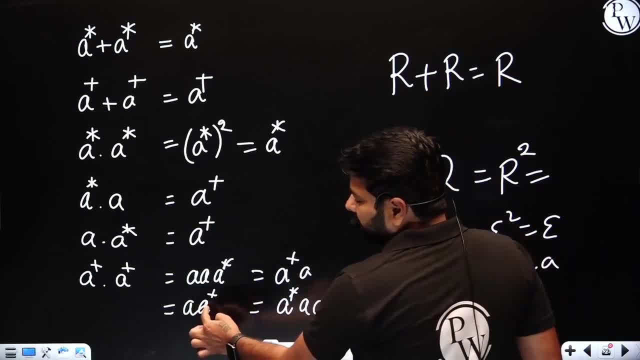 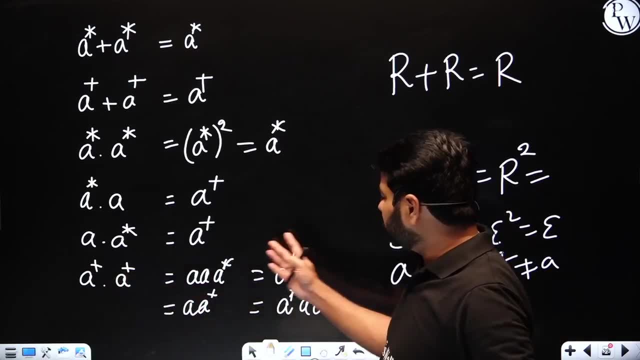 closure and positive closure, right. so try to analyze a- a plus- how is same? how is it same as a plus a plus, right? try to understand this too, you'll get to know. all the things are very easy, fine, just it is homework for you. just try to cross check now. with this, you got to know. 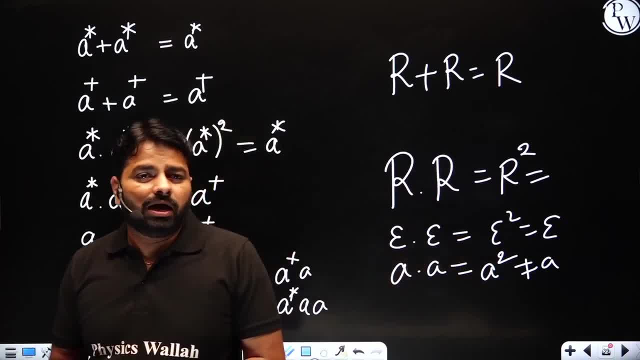 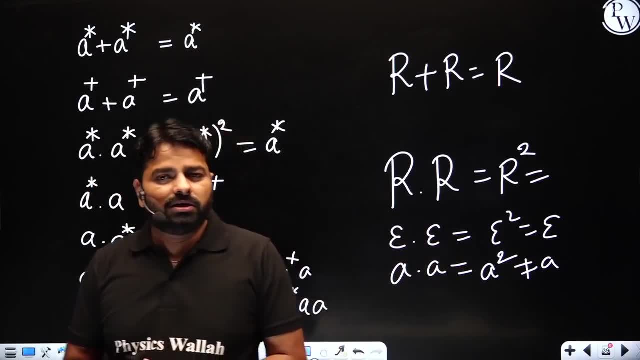 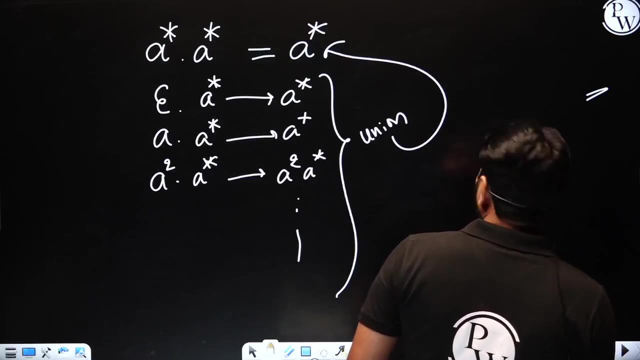 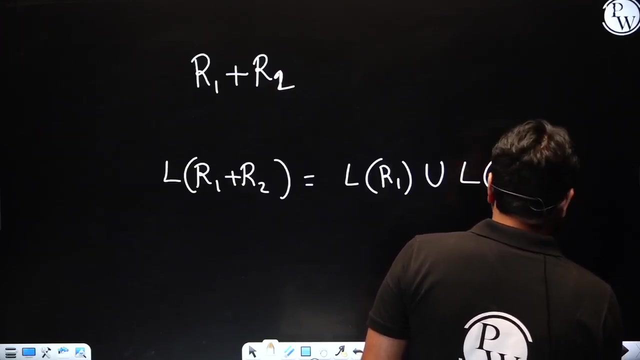 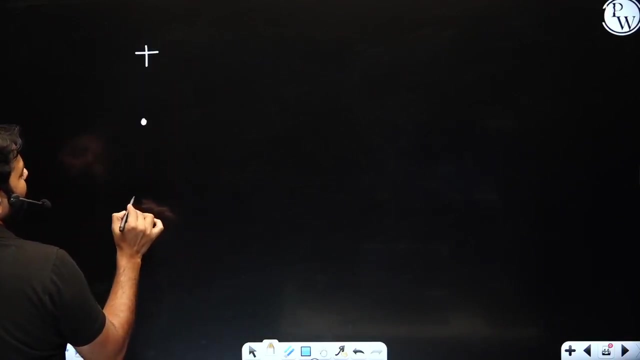 how to use our concatenation, clinic closure and positive closure. but is this enough? no, still, there is a lot to know about regular expressions like. first thing is, let me explain some properties before going to the questions. okay, here we have plus, we have dot and we have 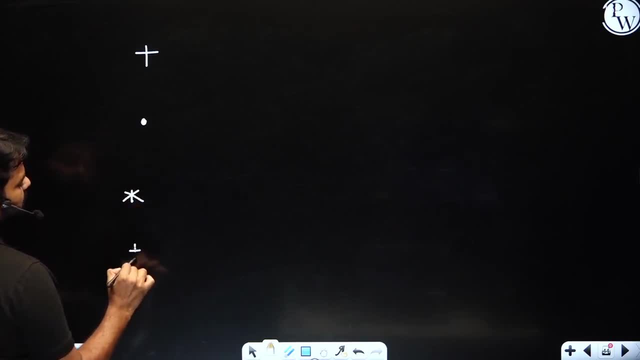 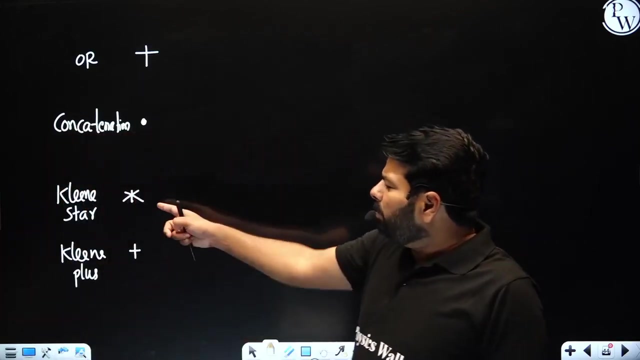 clinic closure that star. another one is plus right, because there are two plus right. should know what are you trying to say? or concatenation clean is star and clinic plus. now let's see. try to understand. what did you learn? the unary operators are so simple, only the definition could. 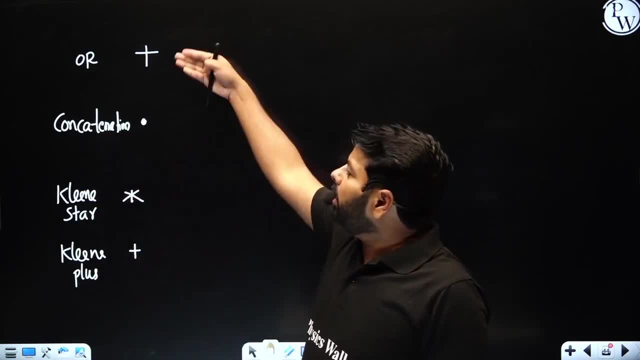 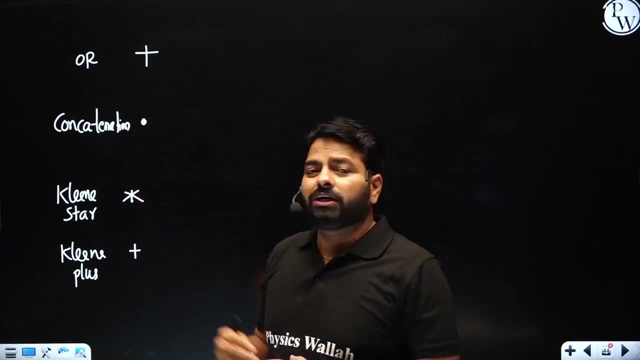 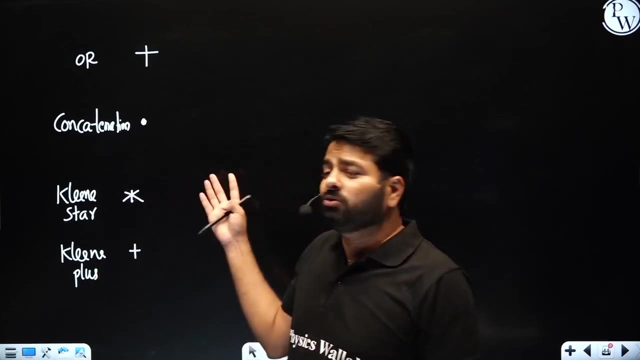 be difficult, but later properties are very easy. but r and concatenation properties are many, many means because they are binary operators. when you are learning with the binary operators, you should know about properties like associativity, commutativity and identity and dominator. there are many things to know about them. so the first two operators will have lot of properties like 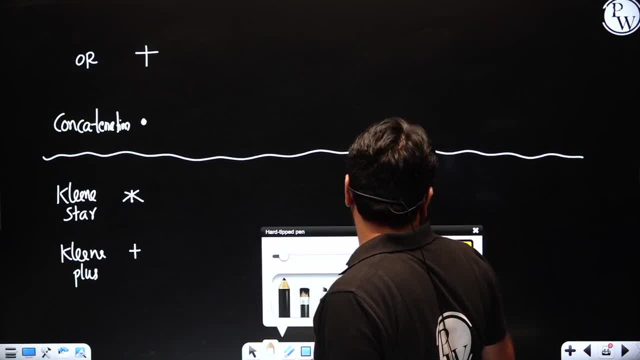 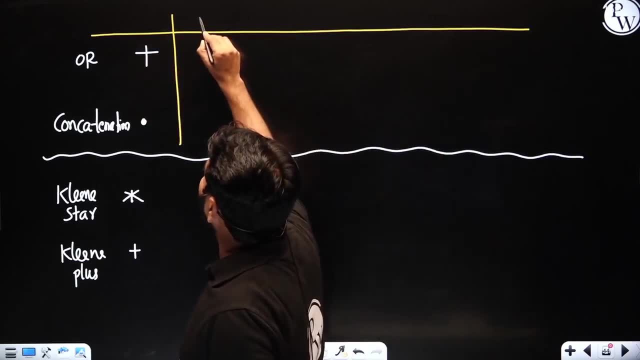 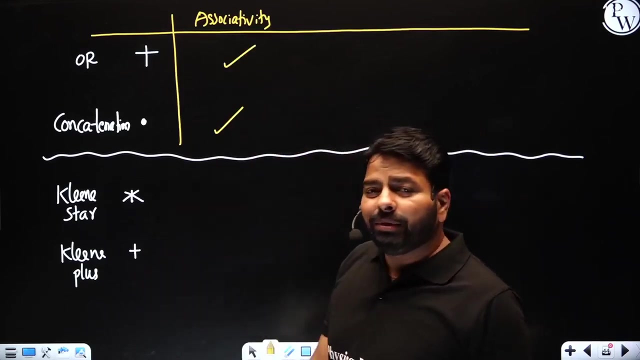 let me talk about some properties here: r and concatenation. let's talk about associativity. if you have studied in other subjects, it's fine. the same definition: associativity, plus and concatenation. do they satisfy associativity? yes, they satisfy associativity. what is the meaning of associativity? let's talk about the plus. like you have r1 plus, r2 plus. 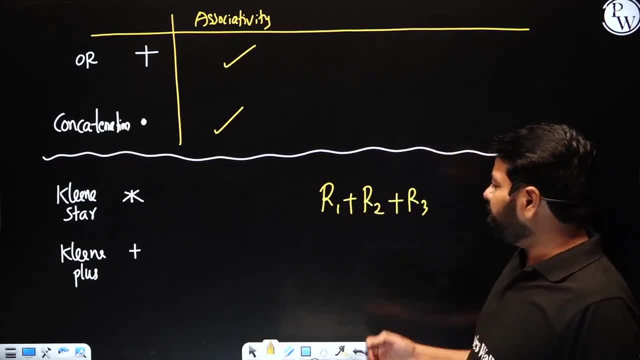 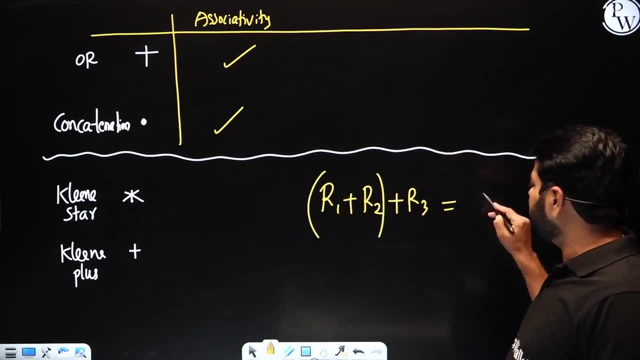 r3. whether you take the left or right associativity, it should have the same meaning. like i take r, this is a left associativity is: is it same as right associativity, without changing the order of operands- left plus you do first or right plus you do first? if you get the same meaning. 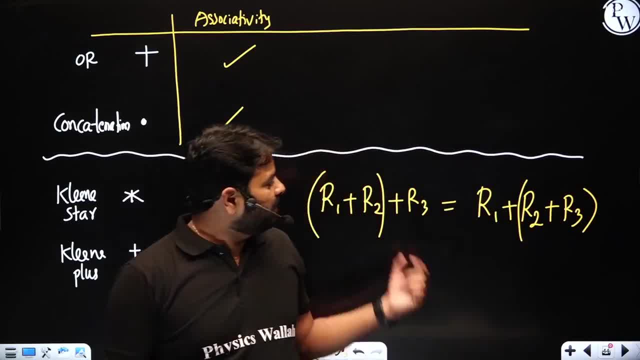 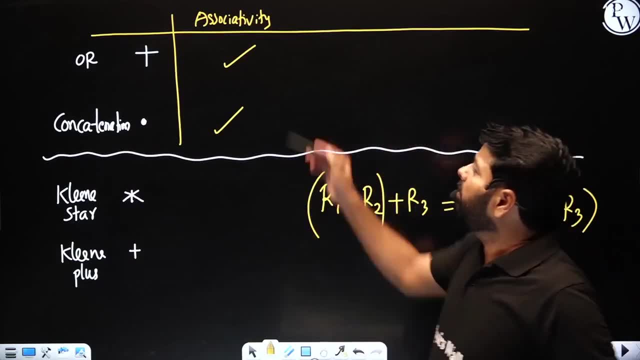 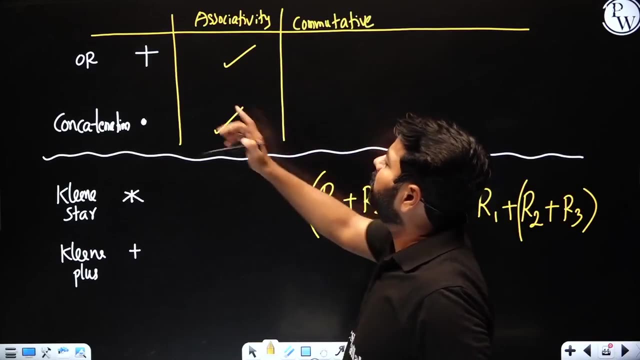 result. if you get the same, then we say that, plus, that r operator satisfies associativity, so it satisfies similarly, concatenation also does the same, but when it comes to commutative, so it is important topic for you- you should know how it behaves for r, you don't have any issue. 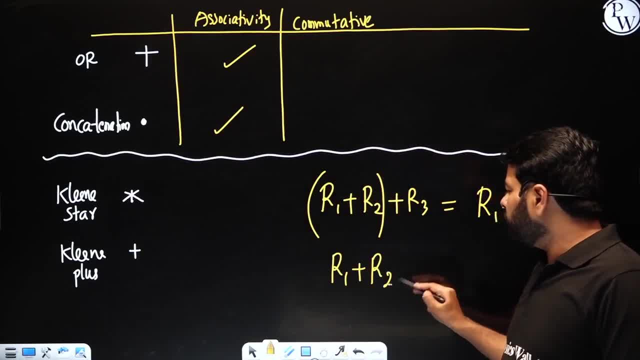 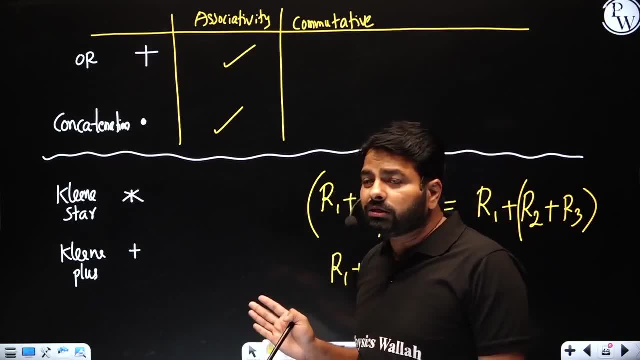 commutative means r1 plus r2. you can also write r2 plus r1 by switching left and right operands will get the same meaning unconditioned, not same. see if i have a dot b. if i change to b, dot a will not get the same meaning. 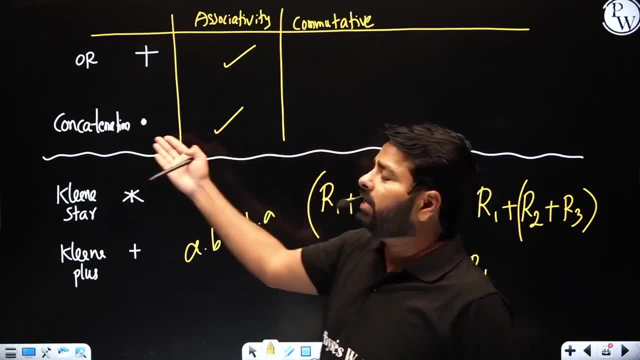 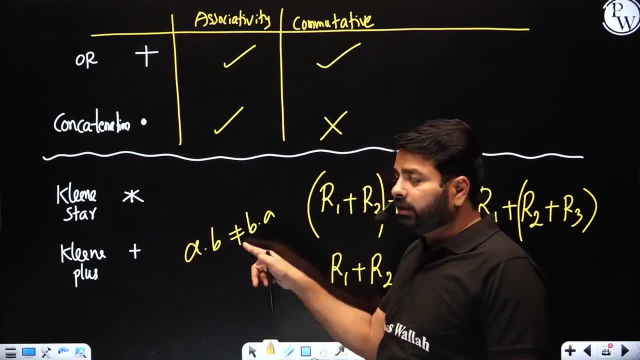 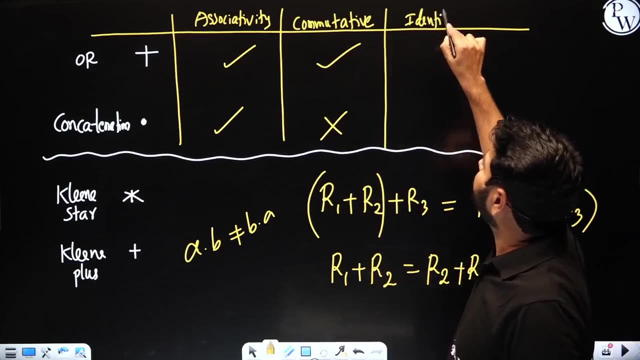 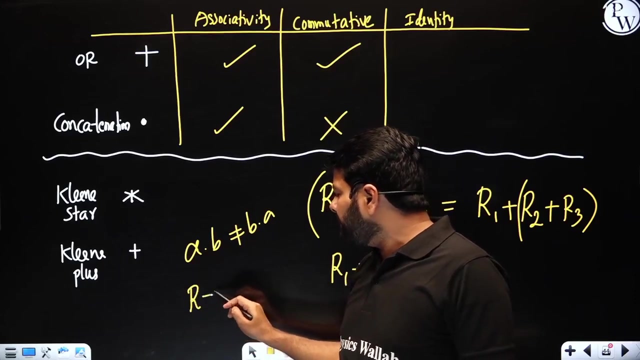 that's why commutative will not be satisfied for concatenation. so even though it satisfies for r but it will not for concatenation, that's very important here. similarly, you think about what is the identity for r, identity in the sense: suppose you have r plus somebody should write, so the result should: 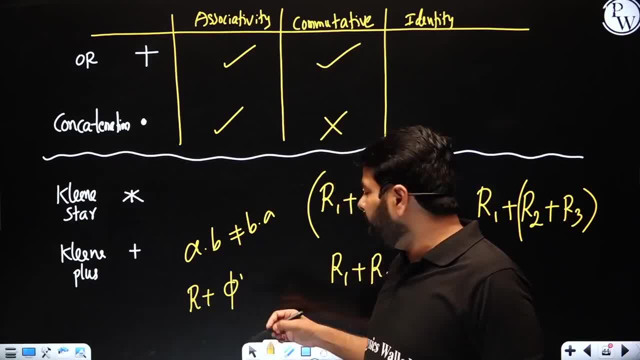 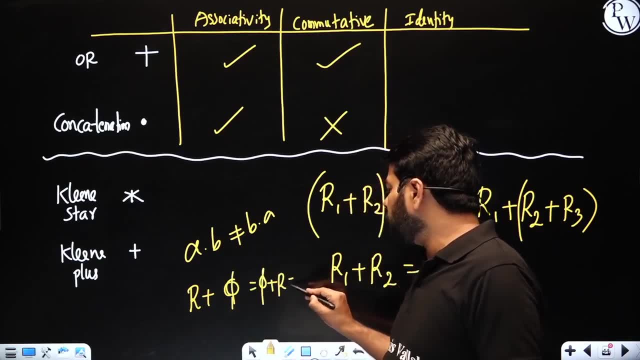 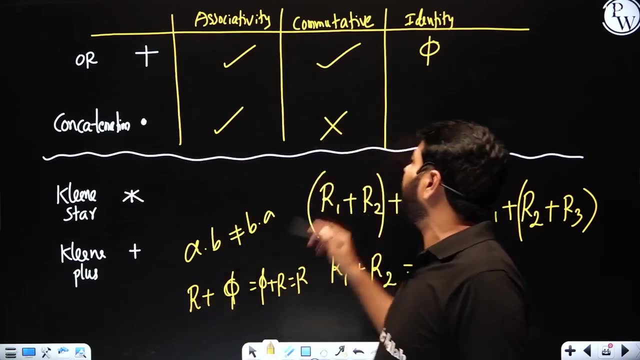 be r. you know that pi acts as what r identity. pi acts as identity. you can also write pi plus r, which is equal to r. so here pi is an identity for r, for concatenation, r, dot, epsilon, so epsilon will act as identity. these are the three important properties. you know there are so many other properties like distributive. 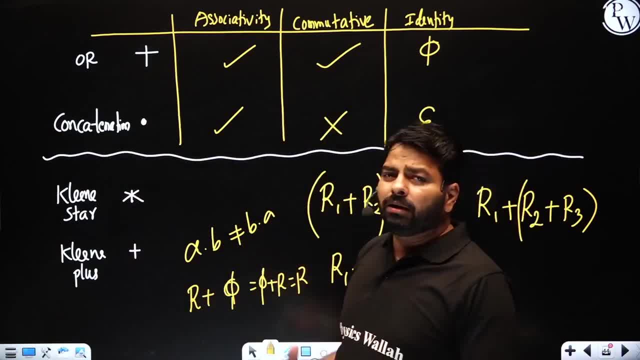 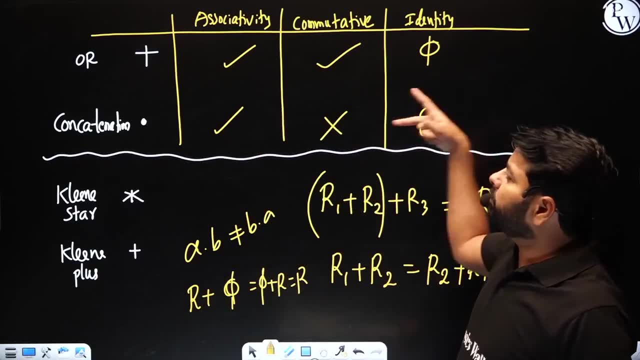 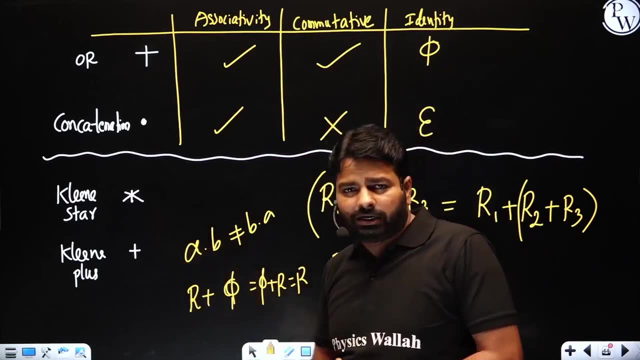 dominator. there are so many and if you are interested you can learn about them, but this would be sufficient for the exam point of view. and associative commutative and identity. so identity exists for both the operators. so these operators, these properties, these properties will not be there for clean star and clean plus, as they are unary operators, right? so all of them, you. 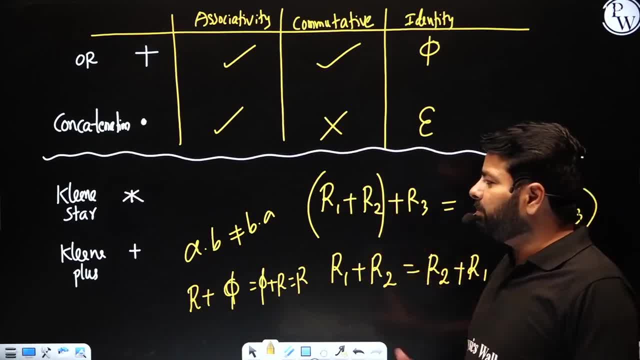 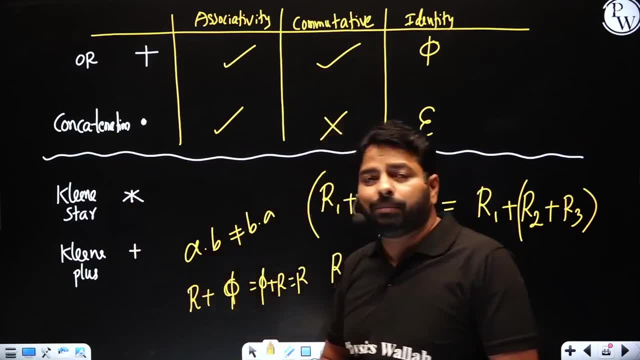 look at, you have the many operands with the same operator but you can't have here, remember. that's why this properties will not be reserved, will not be exist for this clean star and clean plus. that's why they are very simple. once you learn the definition of these two, you don't need much. 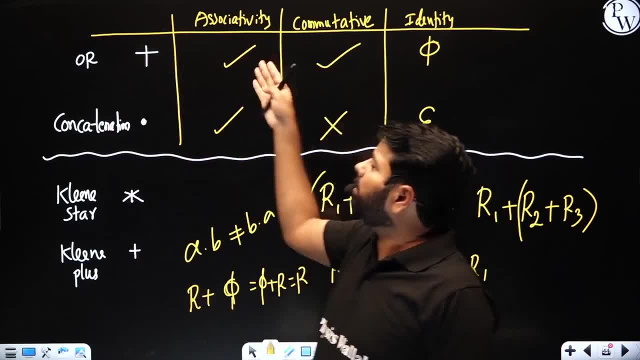 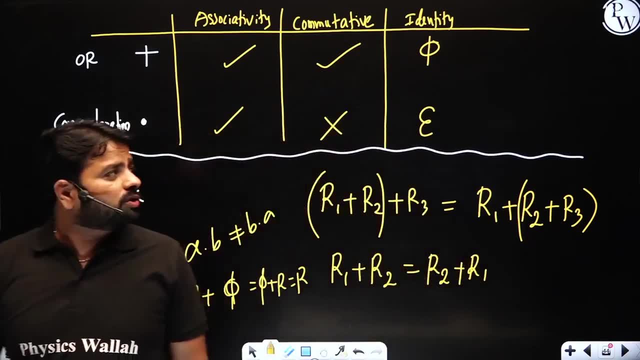 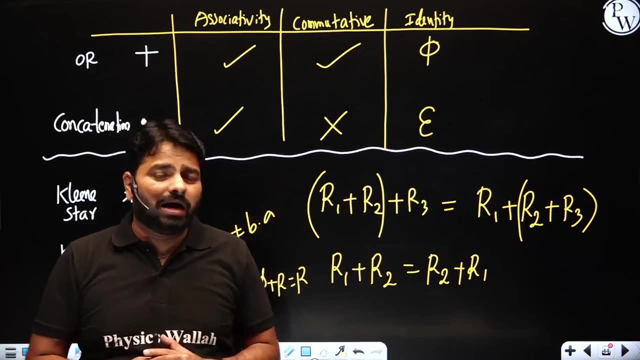 to learn. but here their definitions are so easy but they are applied in different ways in different times. you should be having clarity with this. we got to know what are those operators and what are the properties of the operators and how you simplify when you have the multiple. 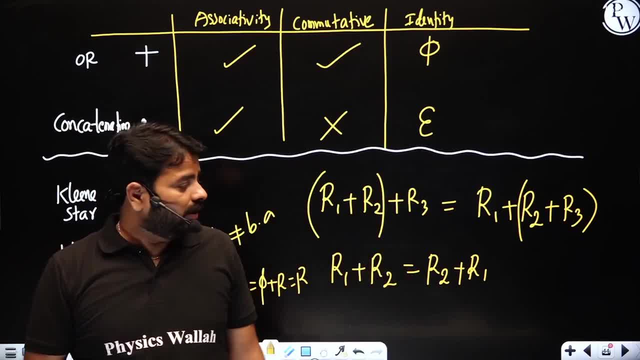 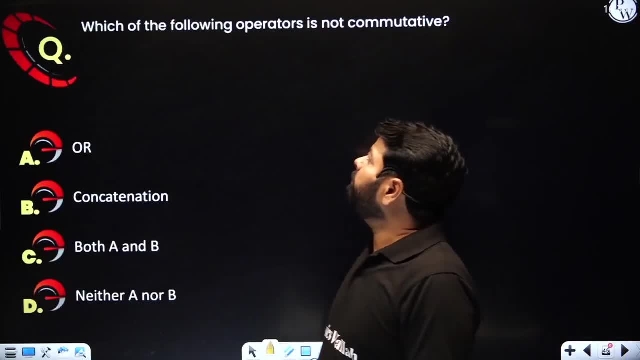 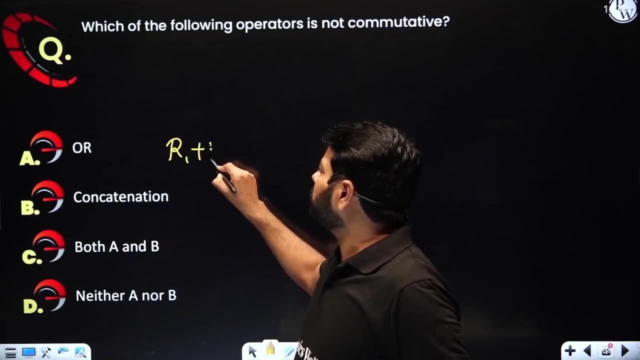 times the different kinds of operands. now. now we'll start with some questions. which of the following operators is not commutative? where is it? commutative means i told the r will check r1 plus r2 is it same as r2 plus r1? to understand it, just take any. 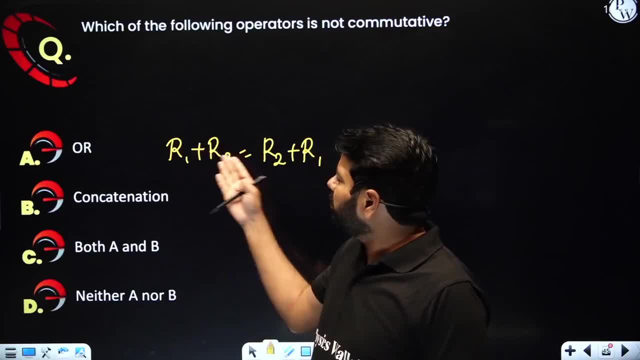 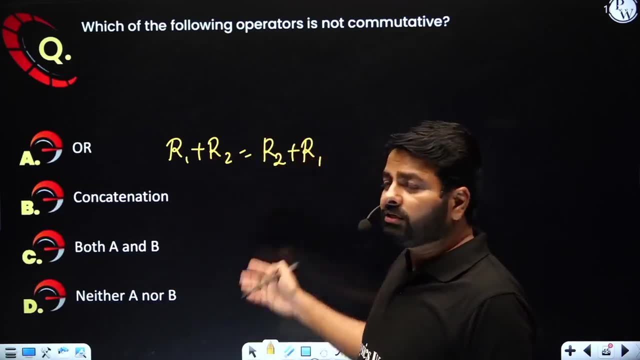 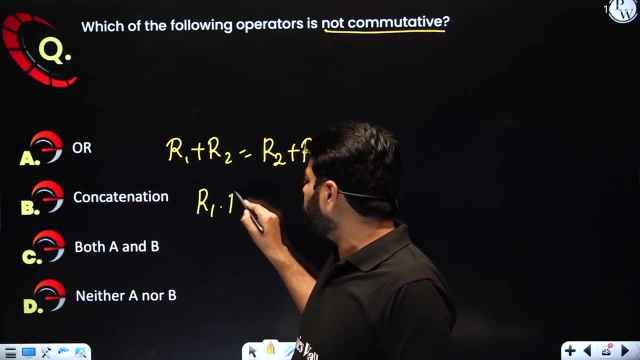 example, or take: understand the definitions: r1, union r2 has to be same as r2 union r1 when you convert into the languages. so it's, it's going to satisfy what commutative. but we want not commutative. okay, concatenation: r1, dot, r2. if two expressions are concatenated and if you switch. 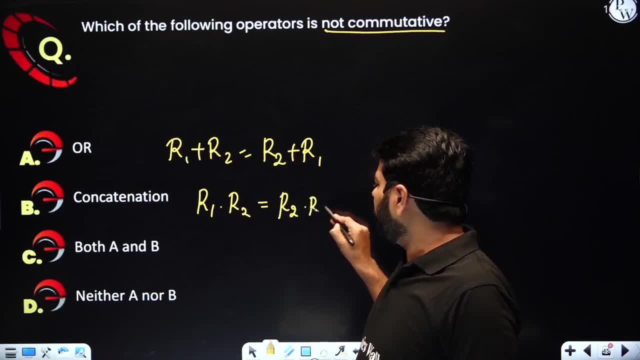 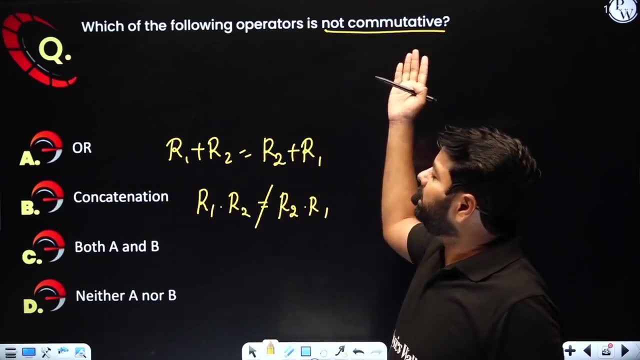 left and right, you will get r1 dot r2, and if you switch left and right you will get r1 dot r2. and right operand, like r2 dot r1, will not be equivalent. sometimes, sometimes, sometimes, maybe equivalent doesn't mean that it holds right if we say that it operator is commutative all the time. 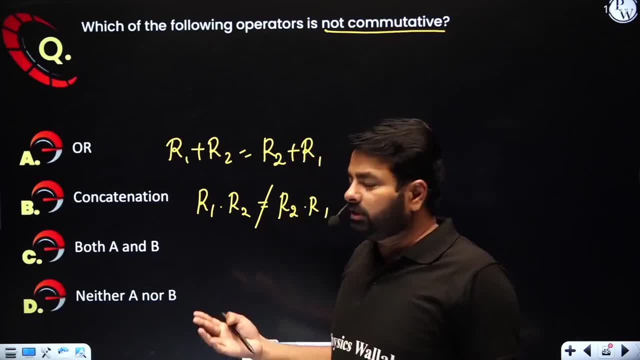 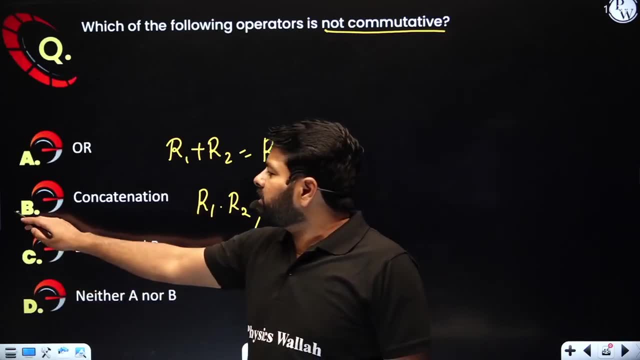 it should hold. then one time it is not holding, we say it's not commutative. so concatenation is in general not commutative. fine, so b is not commutative. that's the right answer for this question. okay, sometimes you may be facing the question. 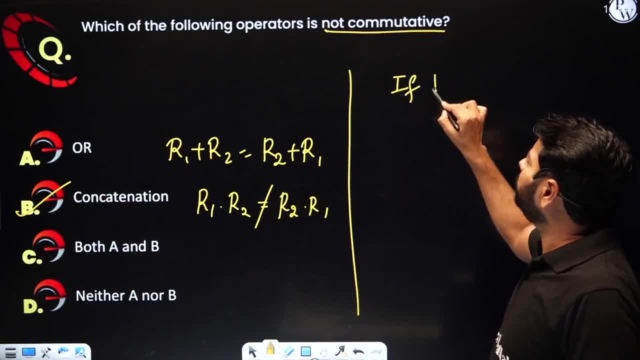 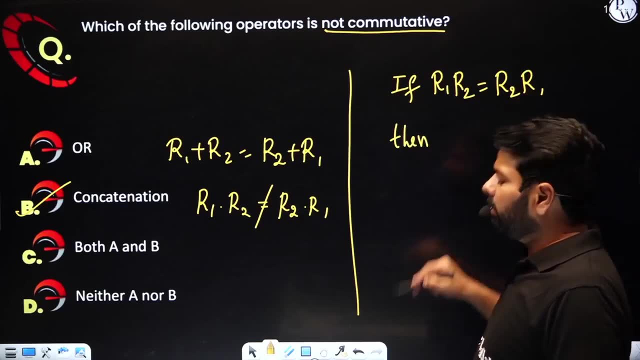 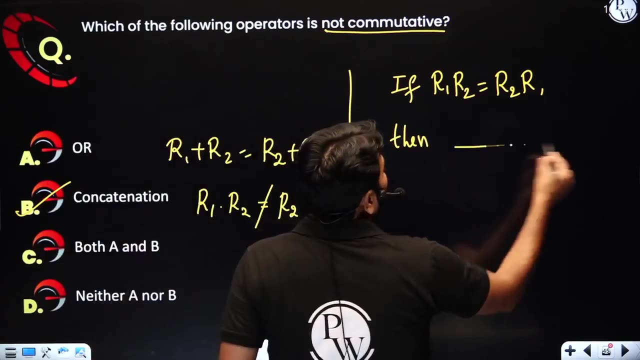 if r1 dot r2 is equal to. that could be possible sometimes. if r1 dot r2 is equal to r2, r1, then find the right choices for r1 and r2. yes, it could be possible, sometimes, only not all the times. then what are the possibility then? choose the right statement. can you think about in which situations? 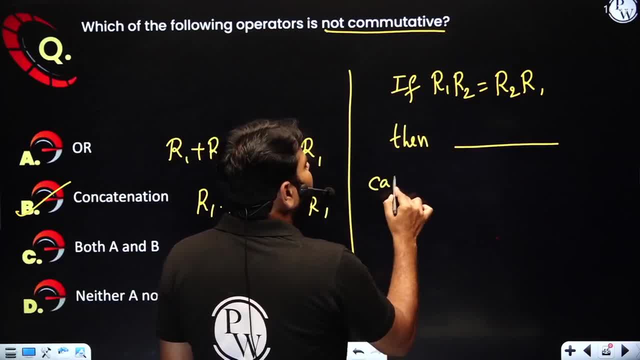 this: r1- r2 is equal to r2- r1. there are many infinite cases might be there. case one: it could be possible. if r1, dot, r2 is equal to r2, r1, then find the right choices for r1 and r2. yes, it could be. possible. if r1 dot r2 is equal to r2, then find the right choices for r1 and r2. yes, it could be possible. if r1 dot r2 is equal to r2- r1, then find the right choices for r1 and r2. yes, it could be. 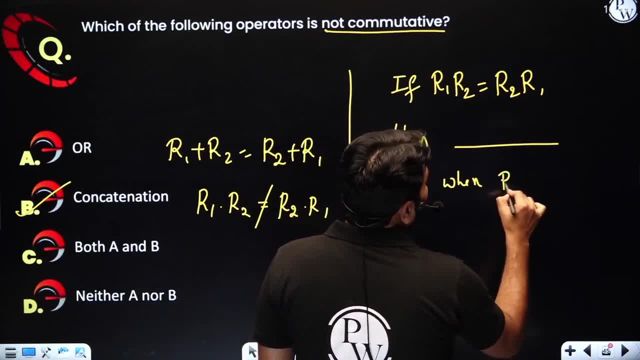 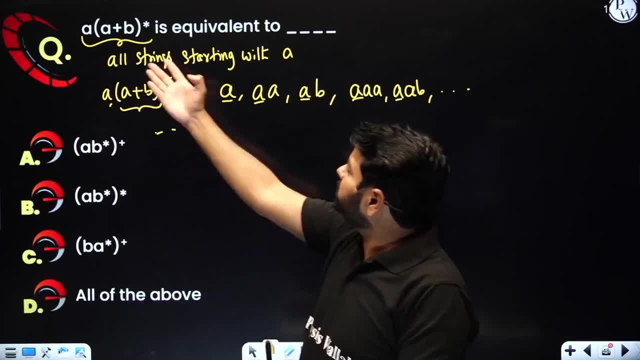 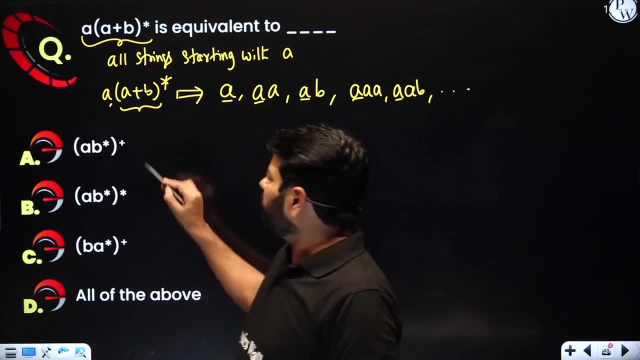 possible if r1, dot, r2 is equal to r1 and r2? yes, it could be, and what option is giving? so what question is asking? is that i want the strings? what option is giving? just you need to match. okay. okay, first one: what is the minimum string? if you can do this? 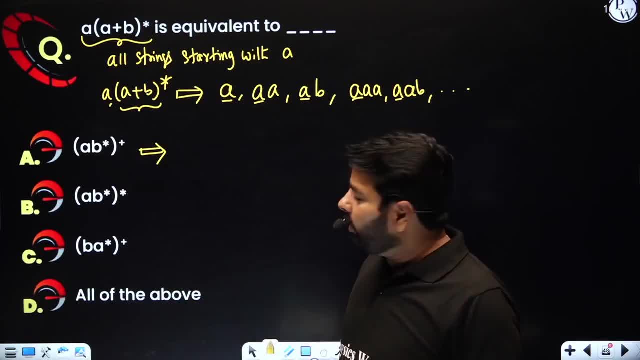 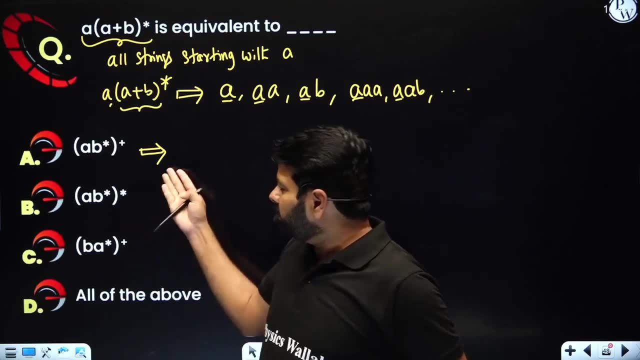 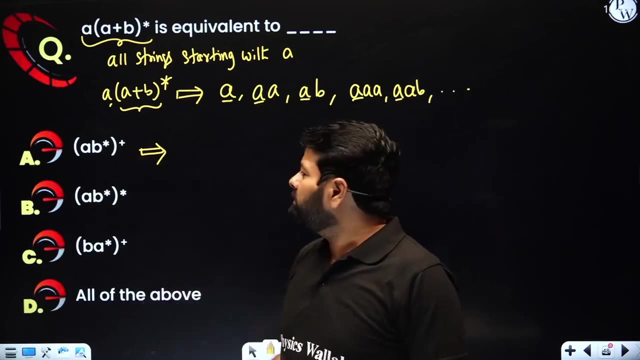 minimum string. nobody will stop to answer this question, only the difficulty that you may face writing the strings in in order according to lengthwise, if you can do that. so first, how do you do that? think always like zero length first. is there any zero length? no, because power zero. 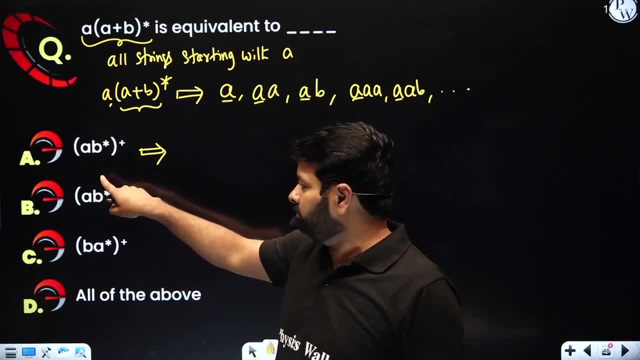 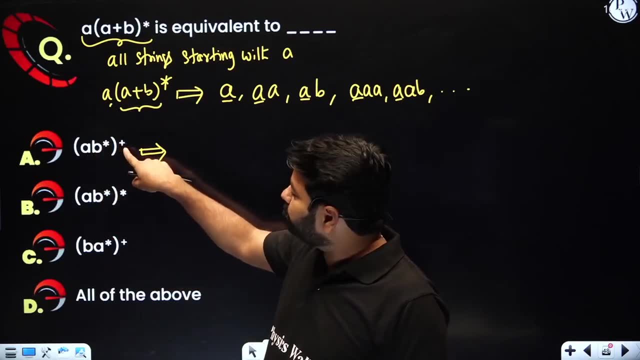 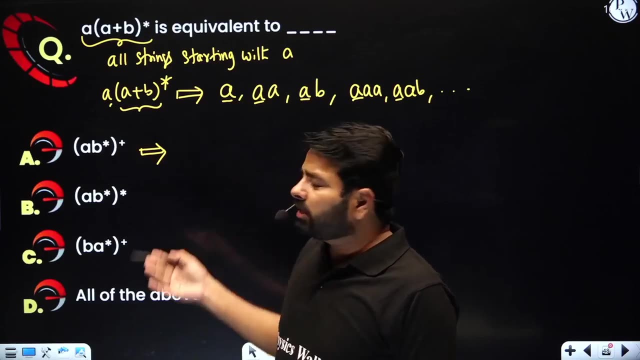 impossible. right, you inside, epsilon is not there. epsilon impossible because if i go inside, a always comes. if i am outside, there is no star. it's a plus. okay, can you think about it? what is the minimum string? you get one, a, because take a power one and 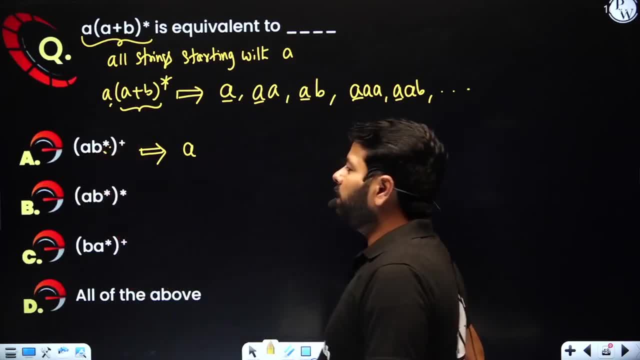 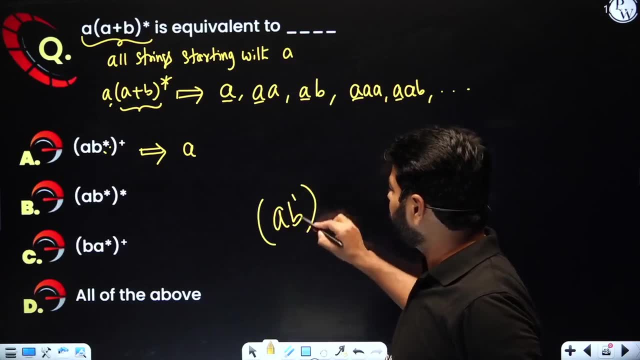 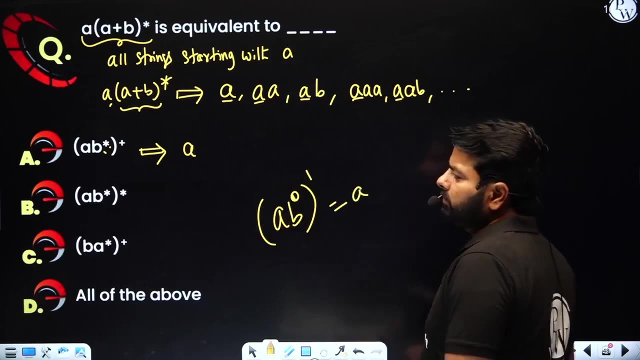 here. put a b power zero and take a, so a b power one, whole power one. so you got a, a b power one, whole power. sorry, b power zero, sorry, whole power one. a b power zero, whole power one. what is it a next? can i get a b? think about it, because if you get a b, that's the wrong option, right? 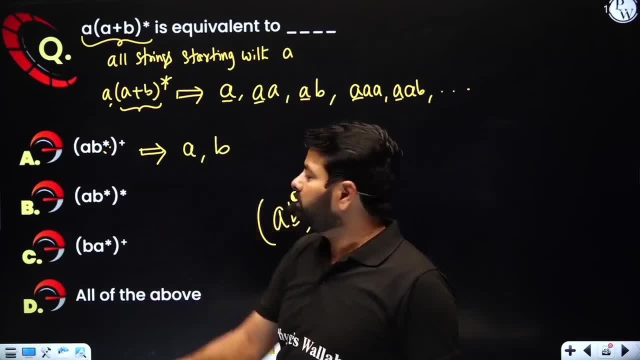 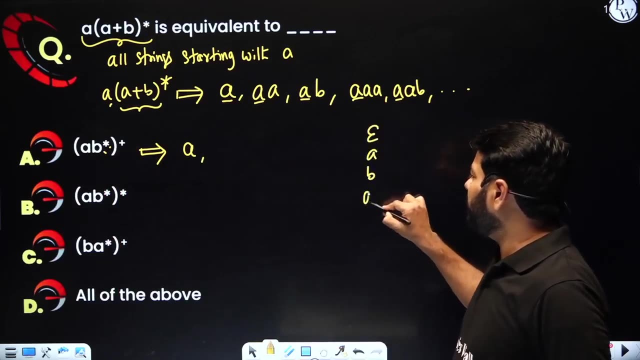 so you want, you don't want a b. if it gives a b, leave it. now what is needed here? b is it possible? no, why when i am trying to take a b, a always comes. so b is not possible. very simple. so here in the order, just look at epsilon a, b, like a plus b, whole star strings. just cross, check them. you will get the 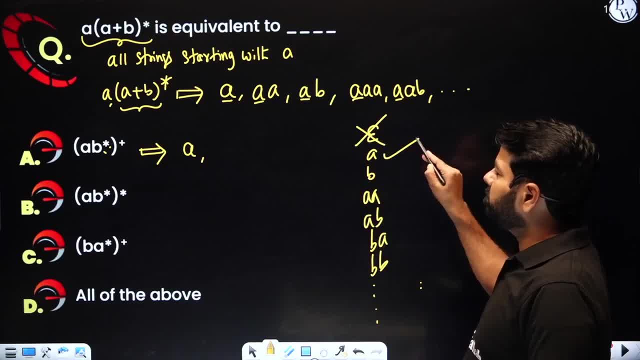 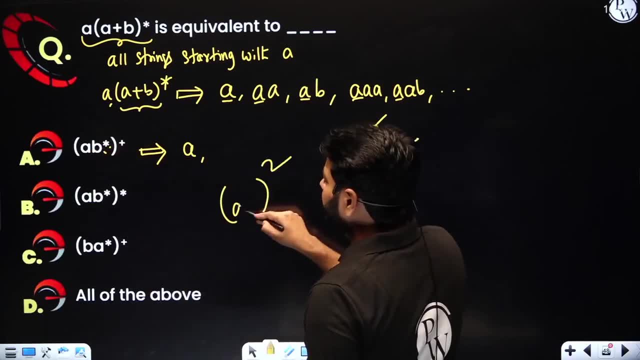 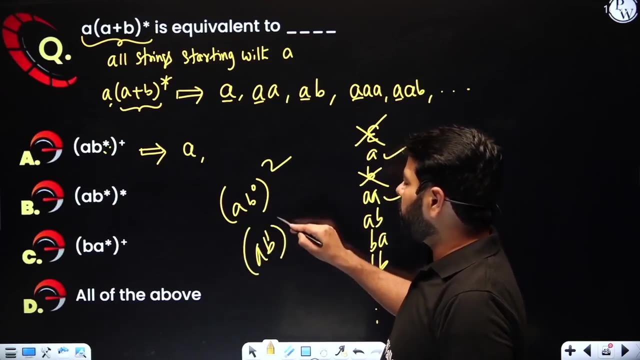 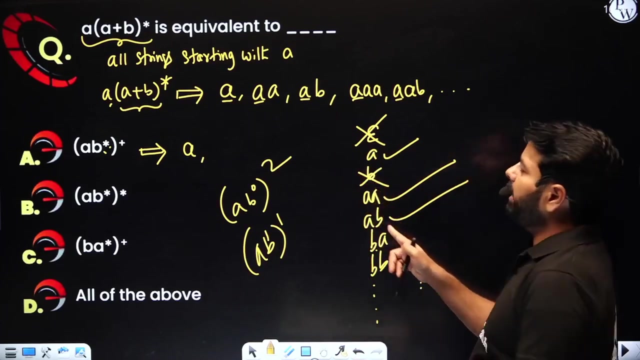 right answer: epsilon not possible. a possible and b not possible. and double: a you take twice power two and take a b, power zero, yes, it's possible. a b: you take a b power one, power one, yes, possible. b a: how do you get this b a? see so far, a a, a, a b, all three are matching. 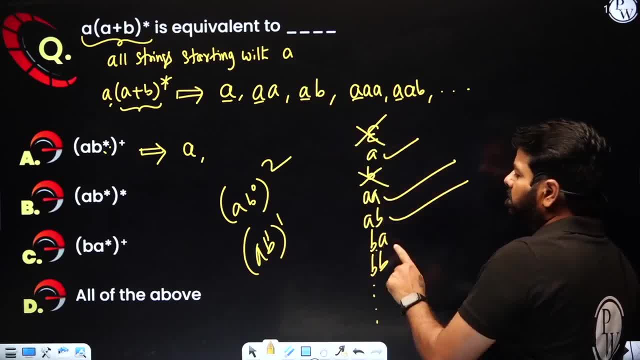 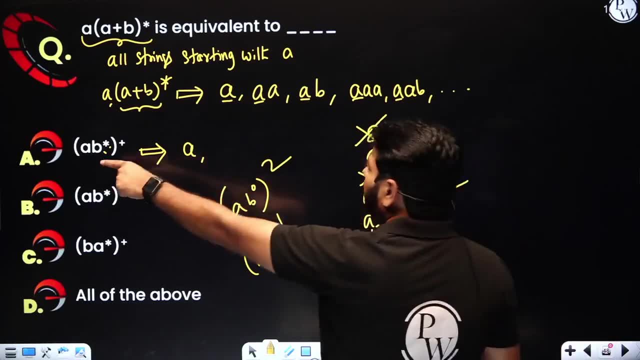 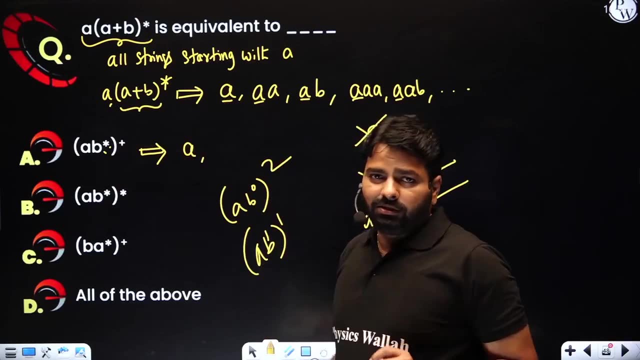 as per the order from the question. right next b a: is it possible directly be impossible without a? so this is anyhow not possible. double b: impossible without a. and up to two length. both are matching. so there is 99 possibility. both could be equivalent, but by looking at the options only you have to. 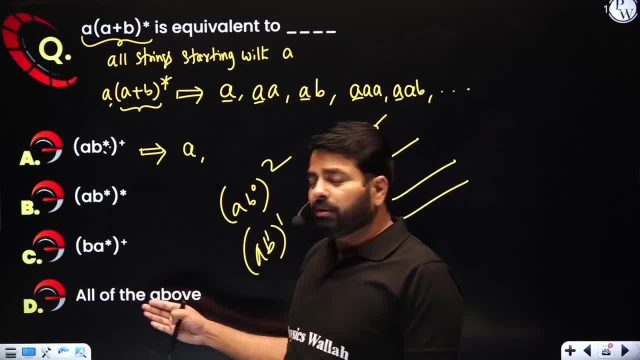 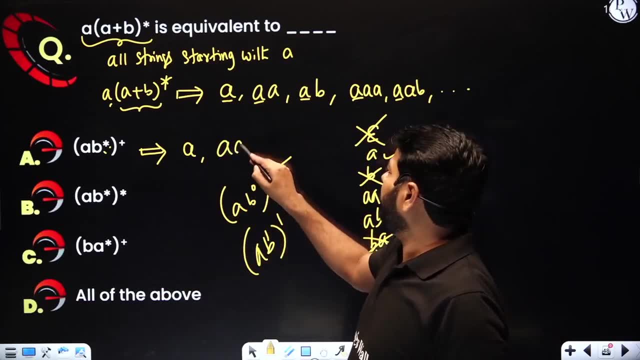 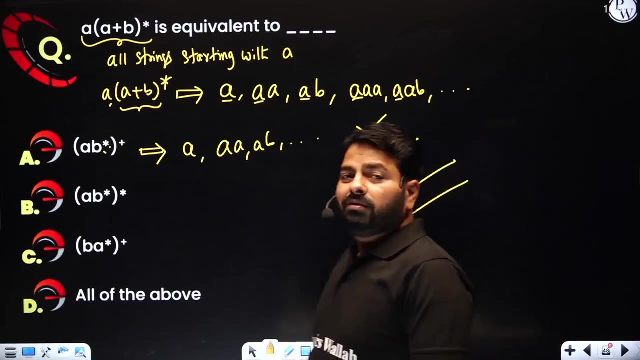 answer it later. okay, if none of this above is there, just go for three length and cross check two, so up to two length. both are exactly matching a and then double a, a, b and later. i did not check because to save my time in the exam time is very important- rather than finding the right answer. 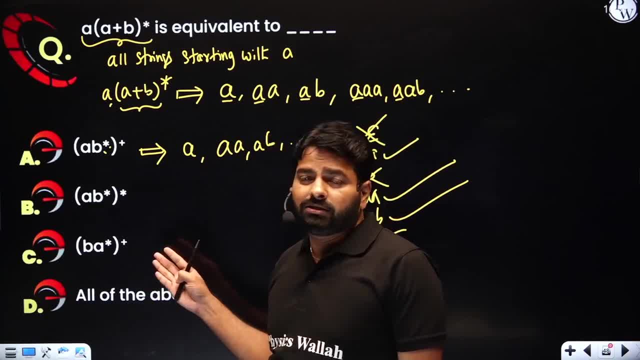 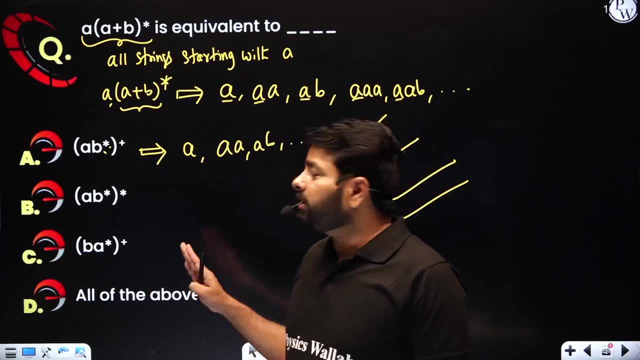 sometimes some people find this right answer after 15 minutes, and some people will answer this within one or two minutes. so which is more important? take less time and answer it correctly. if not, you can postpone it to the end because, uh, you know you are spending more than 10 minutes for. 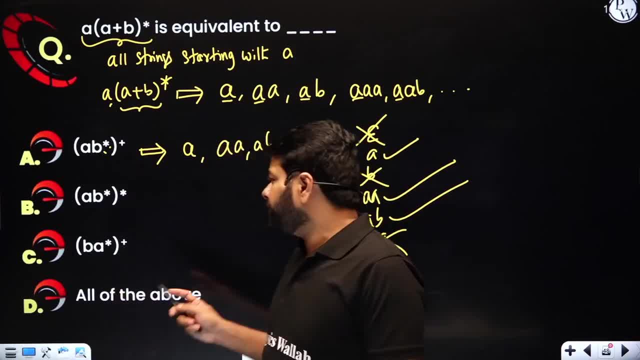 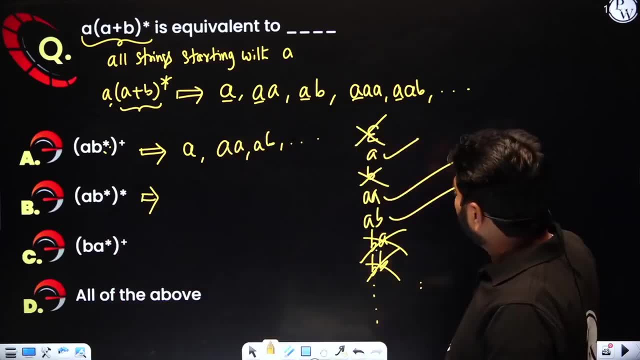 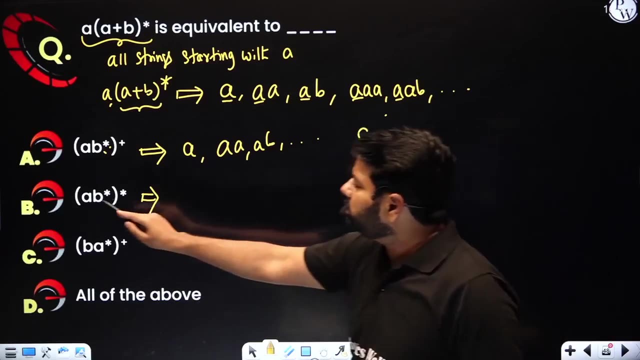 a question means you are losing a lot of questions in the exam. okay, next this one. what is the first thing you can generate? again, start from the beginning: epsilon a, b and so on you have this is generating epsilon. i don't want epsilon in the question, so epsilon is generated, so straight away. 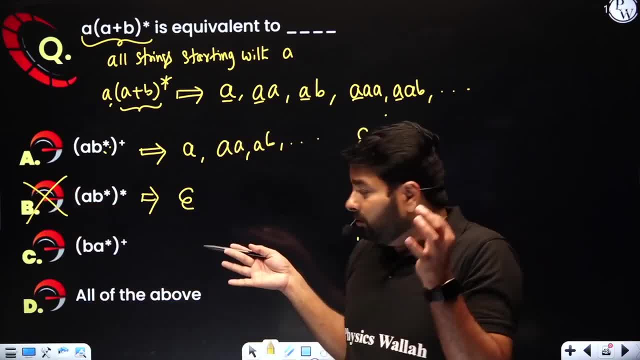 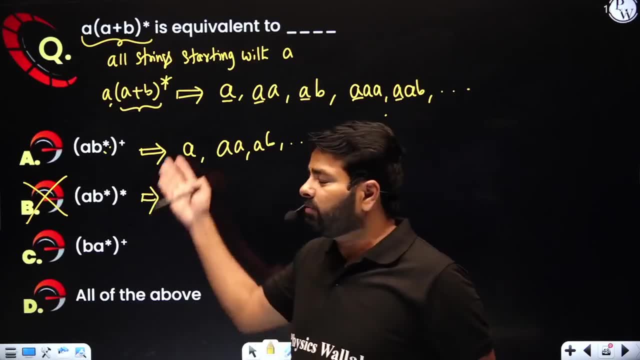 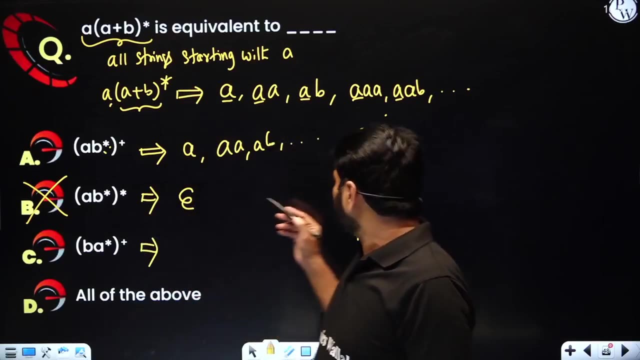 it is not equivalent, no need to go for any other string. so sometimes first time you try for the minimum string you may get the answer that is not equivalent. so you ignore it. not equivalent is very easy to answer the next one anyhow. epsilon is not possible. that's correct. we don't want it. 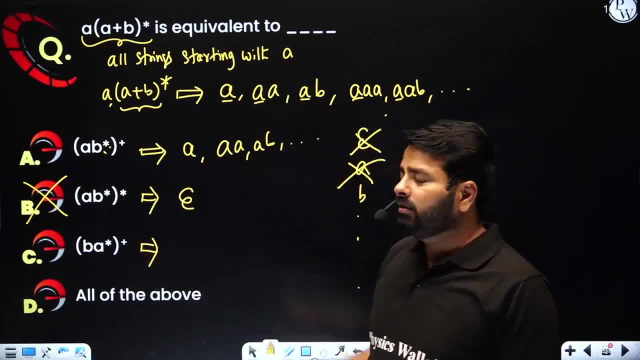 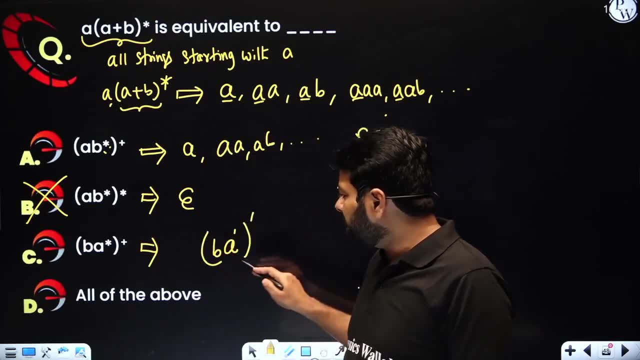 but single a. can you get? it impossible. but we want a. so this one is not giving a y, because whenever you want to take a, then be always there along with it. see that you want a. but without b you can't be. b followed by a star, so only a you can't take. when: 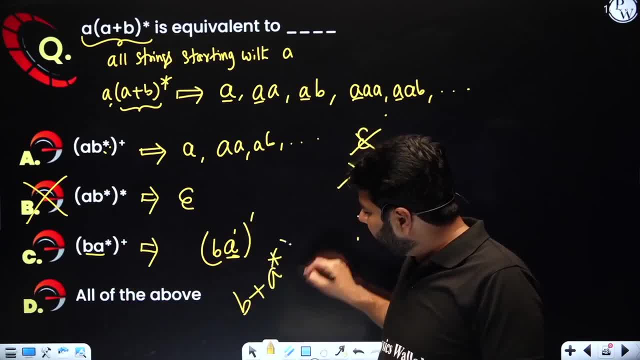 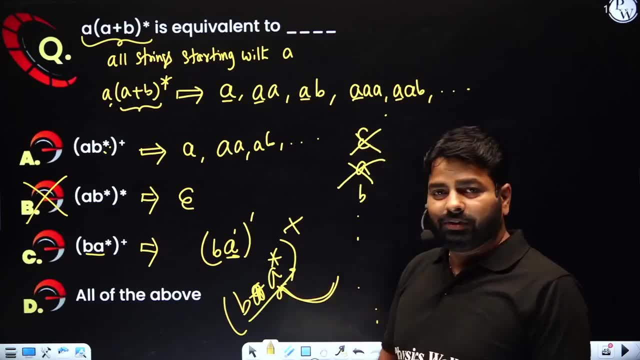 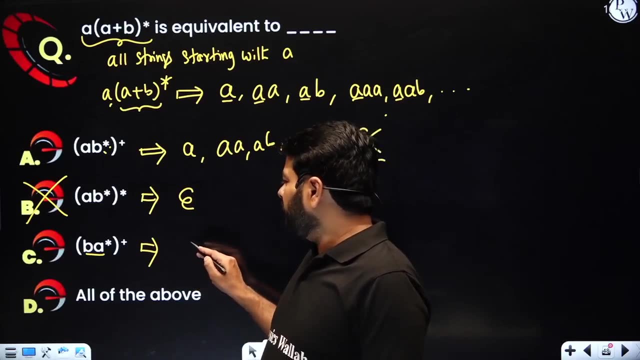 will you take, suppose b plus a star is there, oh, then only a you can take. but here dot is there, then only you can't take both. you have to take right. so understand, why you can't take only a. so here, here a not possible, but we want a. that is the reason. c also we 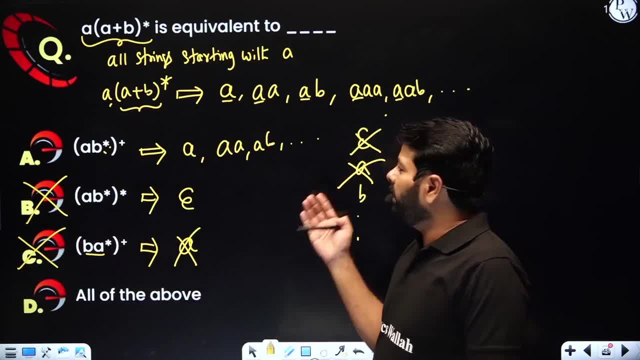 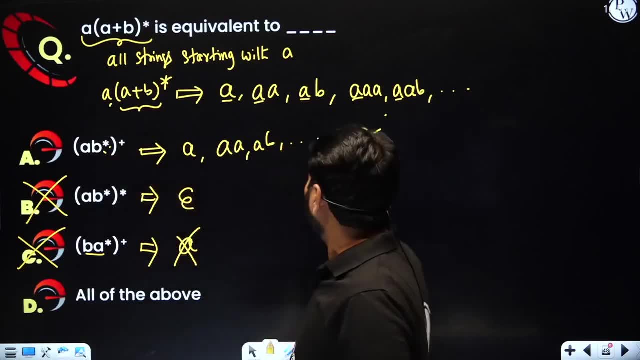 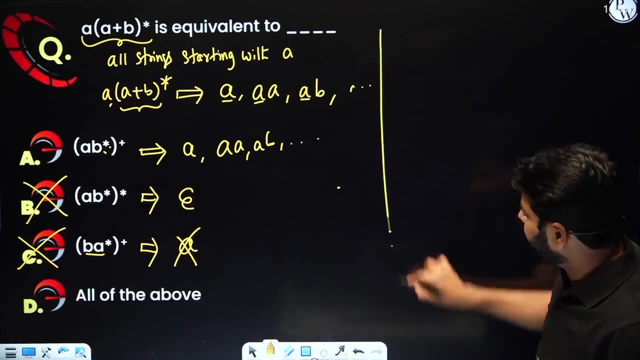 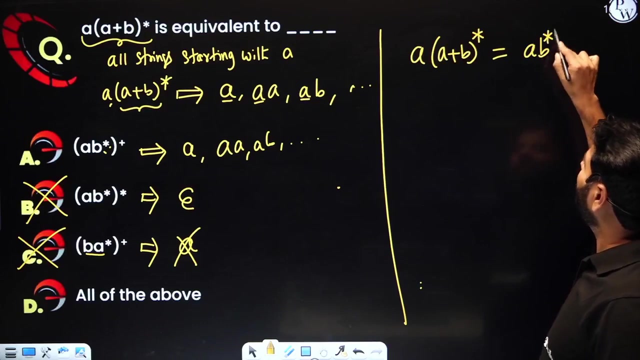 eliminate, only a is left. that has to be correct and verify. if you want, you can understand. this is the one of the famous expression to say: starts with a. okay, i'll just show some of the expressions which could help you for future. starts with a. what expression you have here? a b, star, whole, plus. okay, you should believe now that. 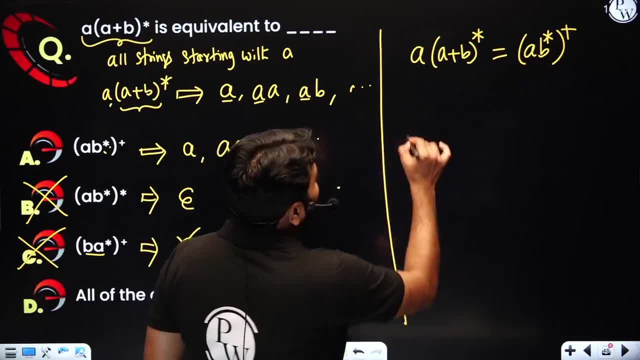 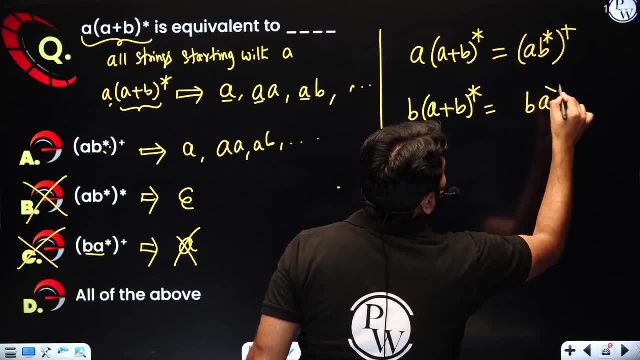 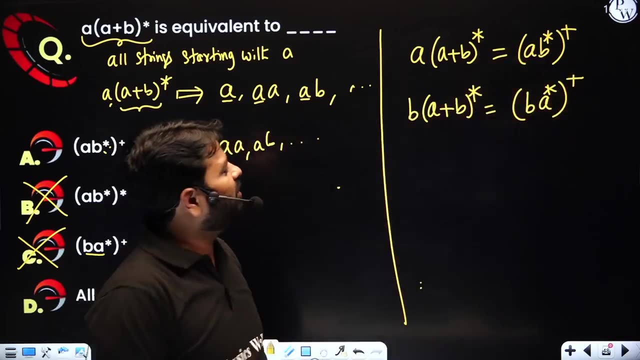 expression is also starts with a. in case you want to have starts with b, slight change here, that's it. you just switch b here, a star, whole plus very simple expressions. okay, there are many other equivalent answers i'm not talking about right. similarly, you just think about ends with a. okay, in case. next question is there you should answer. 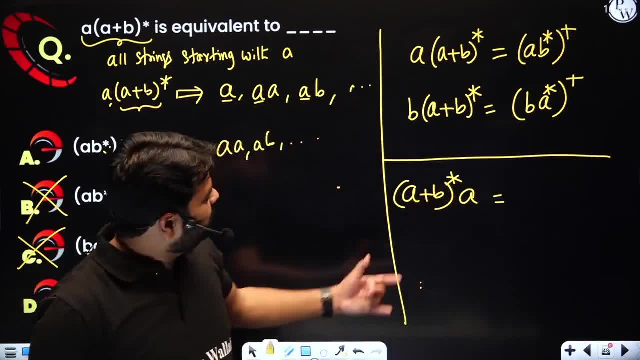 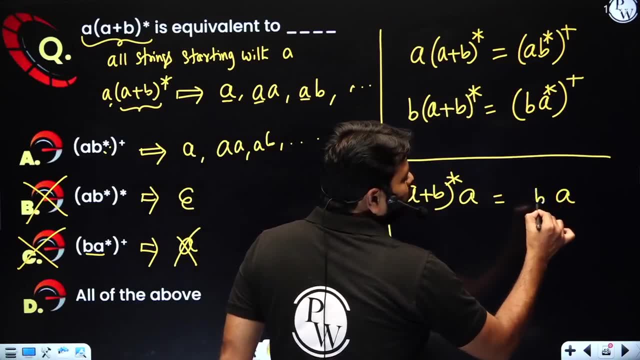 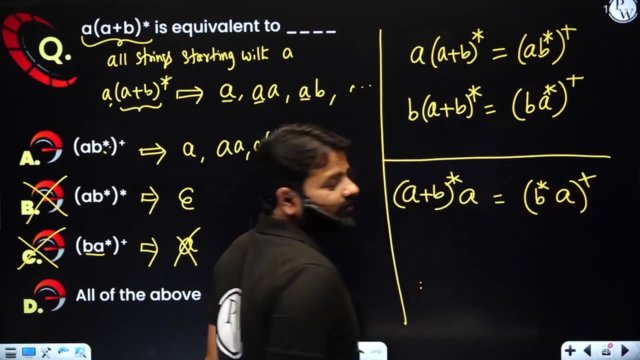 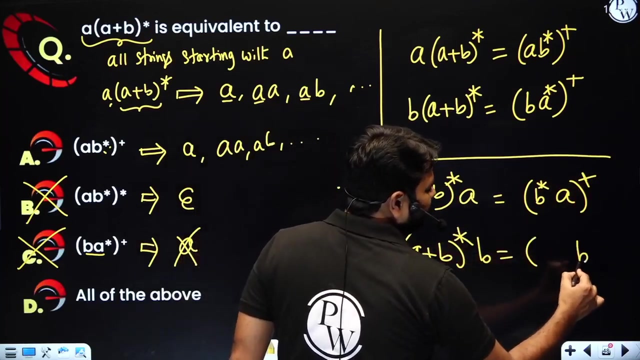 very quickly now. when you have starts with, your focus is on a in the beginning. now ends with a, your focus is at the end. a and b is optional every time and repeat any number of times almost same right. see that now. if it is ends with b, b is at the end and a could be repeated any number of. 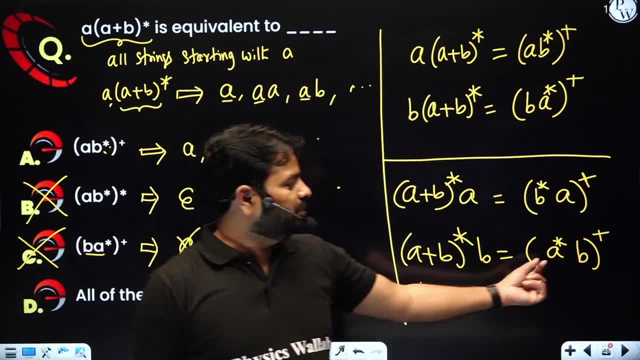 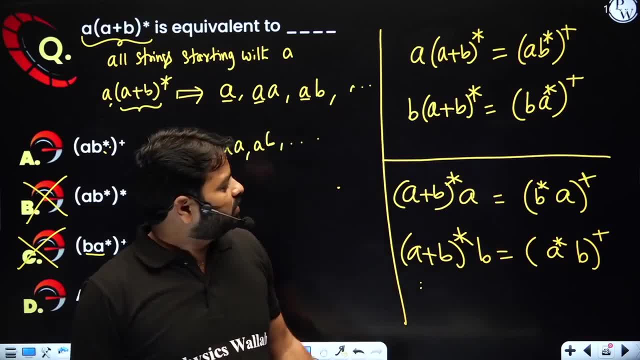 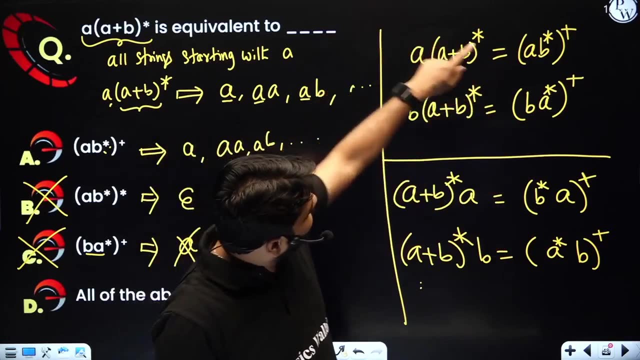 times, but at least one string should end with b, so that's why we have a plus over now. these are the very famous and important expressions for the exam you could remember. sometimes you face it, but understand the how to place those a's. if you are starting with a place a first, if you are starting 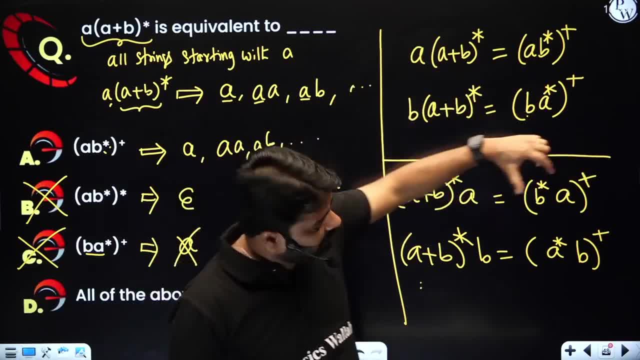 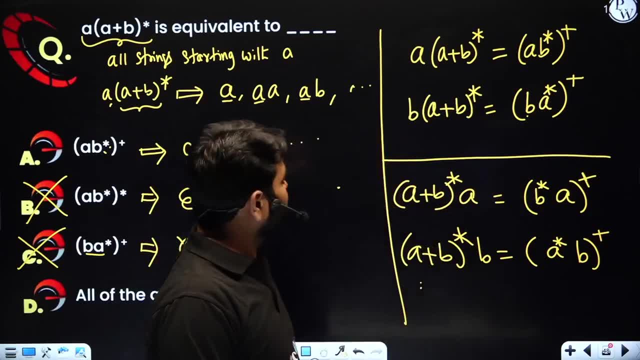 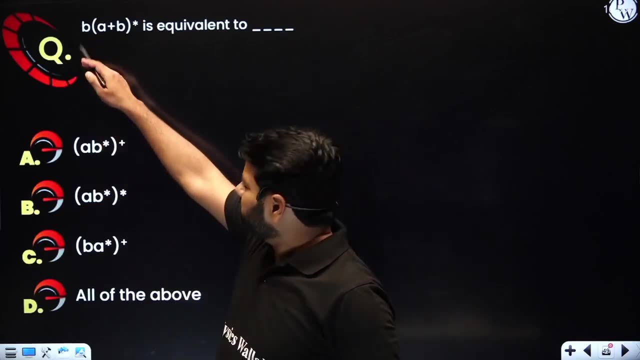 with b, place b first. if you are ending with a place a at the end, if you are ending with b, place b at the end, within that posture closure, within that posture closure. okay, next question. oh, now you may answer it very easily. starting with b. so look at where is the b first. b is here and don't believe that answer is right right now. 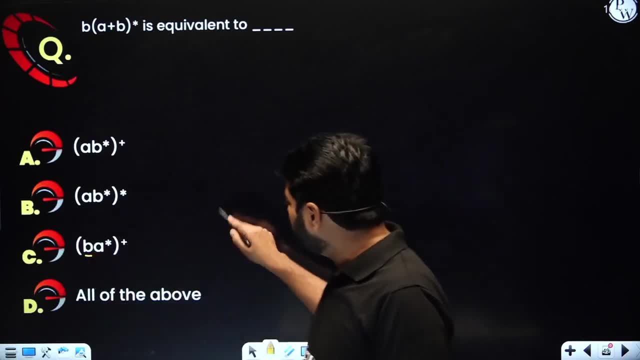 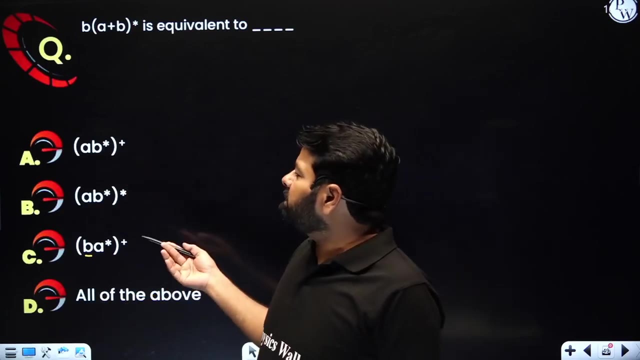 but identify b, a is the whole plus sometimes whole star will be there, so you should be very careful. that is the wrong answer, because epsilon might be generated okay, so this is absolutely right answer. sometimes could be possible. other might be equivalent. you don't know right, you never tried maybe, so now you should cross check. they might be wrong you. 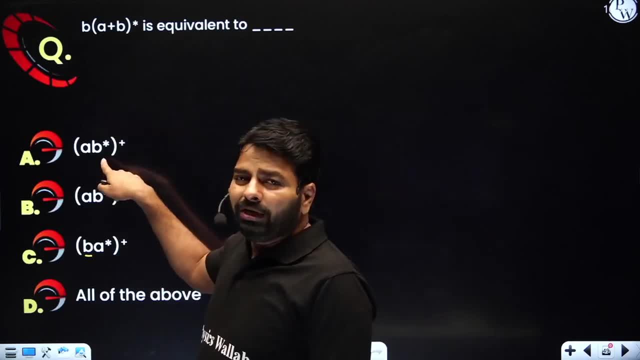 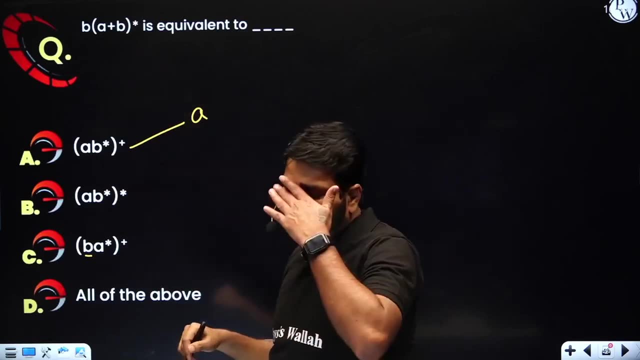 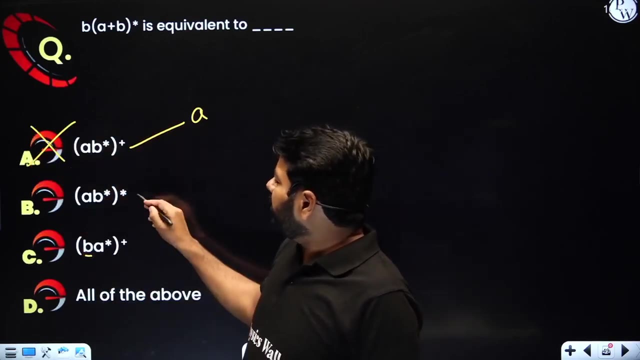 should eliminate it. why this is not end with b? because here only one year i can generate, so when one year i can generate, so how can be equivalent to starting with b? sorry, starting with v, right? so this cannot be starting with b. this cannot be starting with b. so eliminate now. here epsilon, we can generate, but here epsilon, not there all. 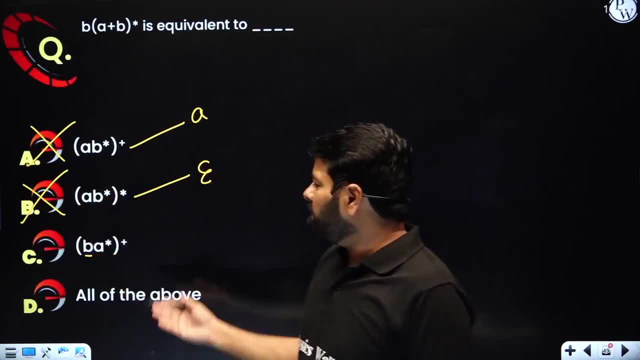 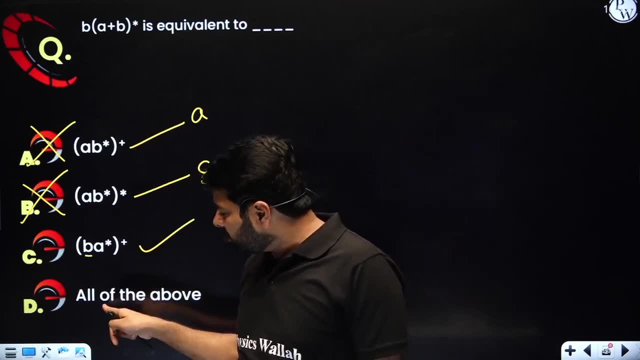 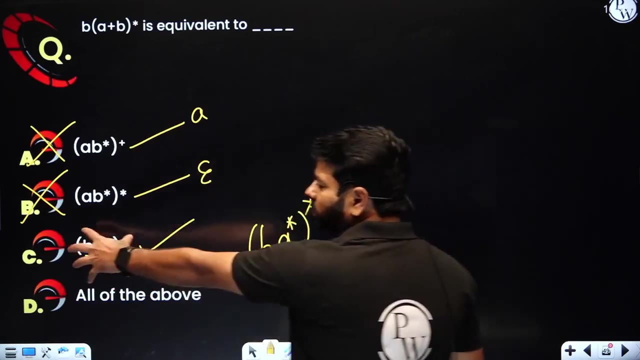 the string starting with b, so we eliminate it. now i just told: right, this is only the equivalent to this one. so c is the right answer. but to confirm this, because here none of this might be there, if i have one option, let's say b: whole star, old star. if this is the c option, then definitely you. 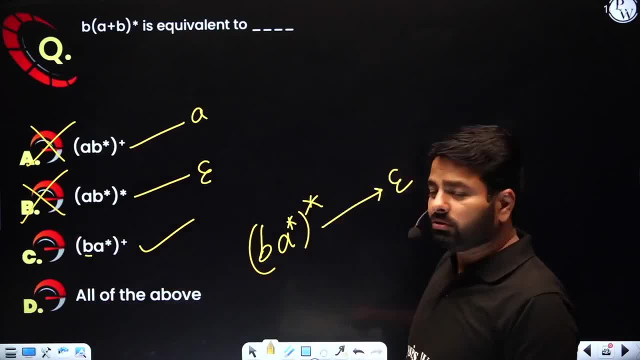 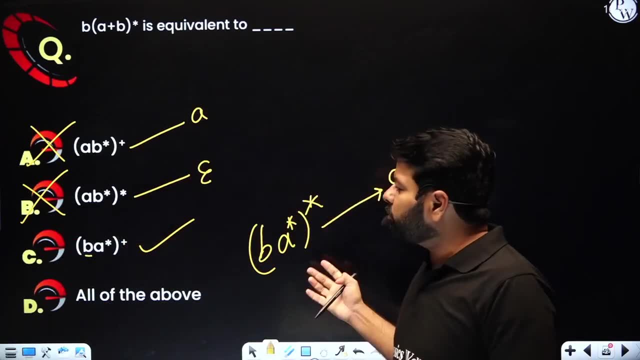 can't choose a c also why here epsilon is coming out, but here that whole star is not there. here plus is there. that is the reason. this is the right answer for the given question. so sometimes you should be very careful while choosing the option right? so c definitely the right answer i've. 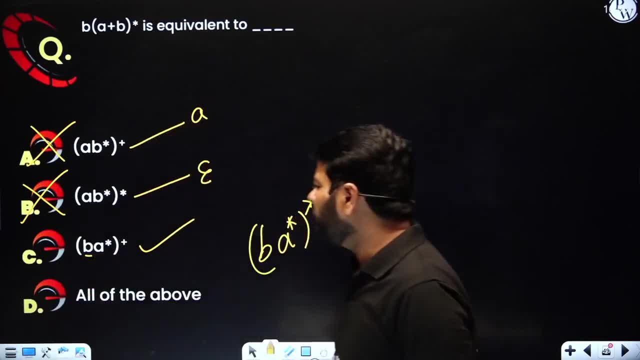 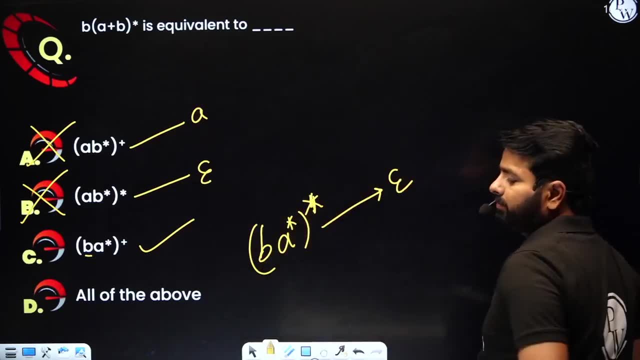 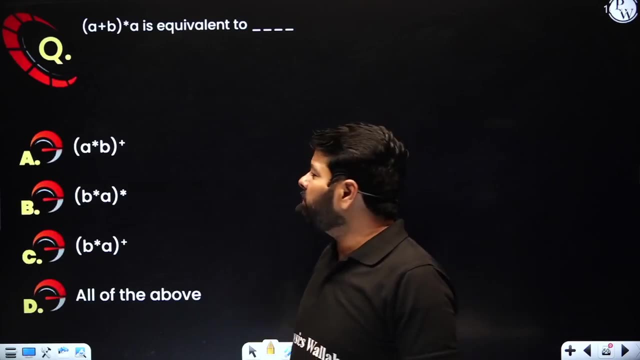 explained all the forms in the previous slide too. okay, but when you have this, definitely this is not equivalent to the given one. because this is not equivalent to the given one. so because of old star, only because of this star, okay, yeah, now you choose it, i don't spend much time for you, uh, now. 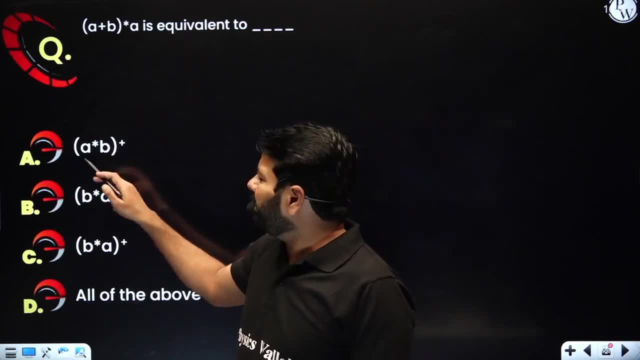 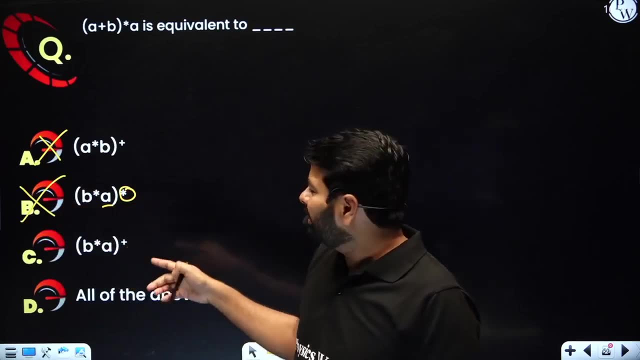 ends with a. no guarantee of ends with a. so eliminate ends with a looks like. but here, what is there, star? that's why i deleted epsilon coming out right, you can't generate epsilon here now. this one we require as ends with a and your positive closure is there. 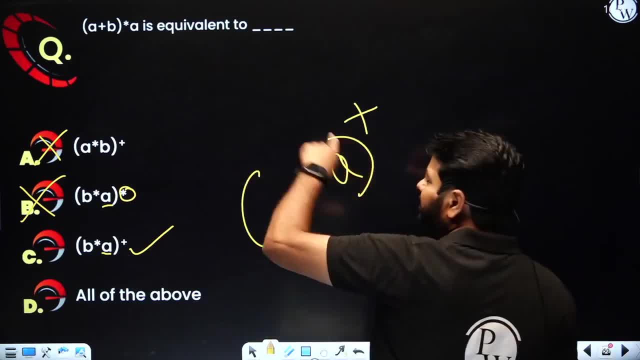 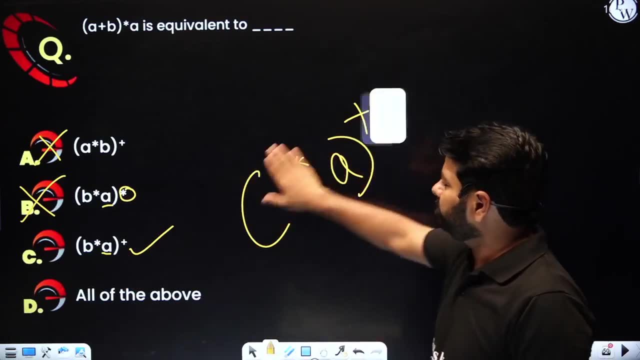 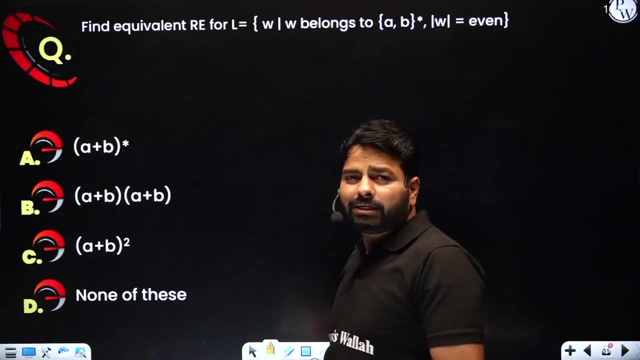 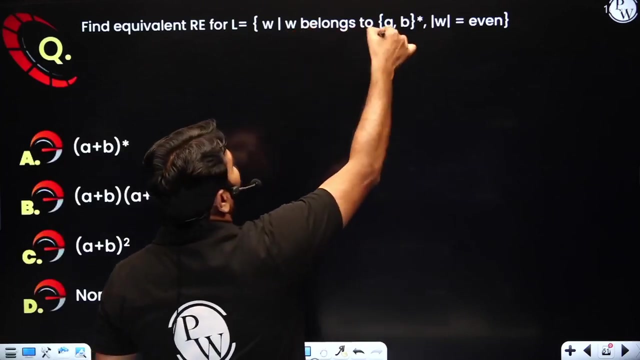 so positive closure, and a should be there as ending with a, and here b star should be there. so this will shoot our given expression. fine, let's move to the next one quickly. okay, find the equivalent regular expression for the language which has even length strings: w belongs to a comma, b, whole star and every string. 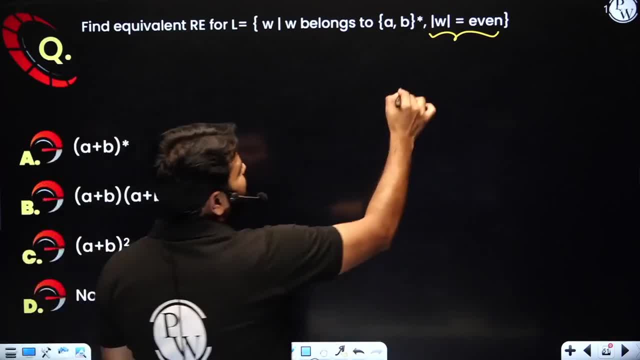 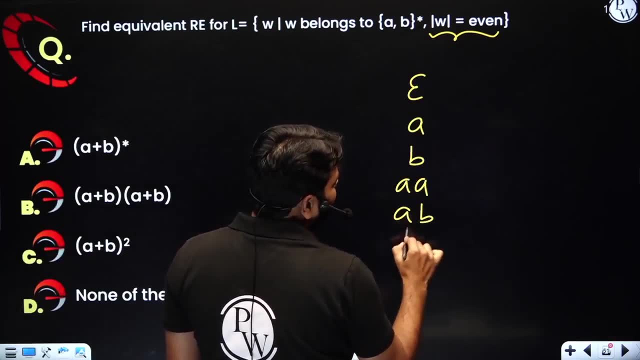 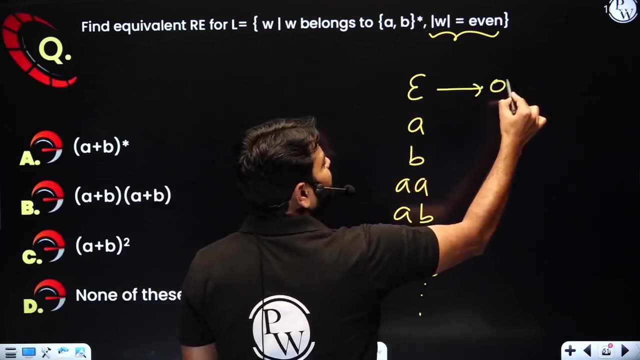 is even length. what do you mean by even length whenever i say length of the string is even what could be even length? suppose i have epsilon a, b, double a. these are the strings in the particular order right who are going to be even length. epsilon 0 length. this is right length i am talking about. 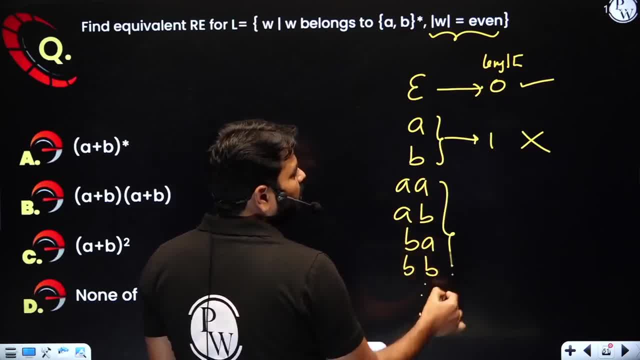 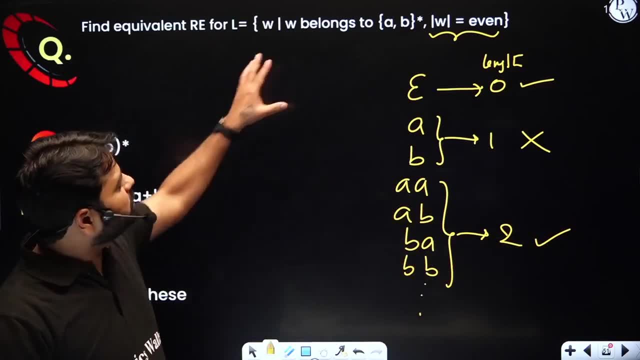 one length. we don't want this are our two length. yes, we want them. so this kind of strings: zero length, two length, four length, six, eight, nine, ten zero length i am talking about, and so on, those strings should be there in the language. i hope you got the problem. first, the 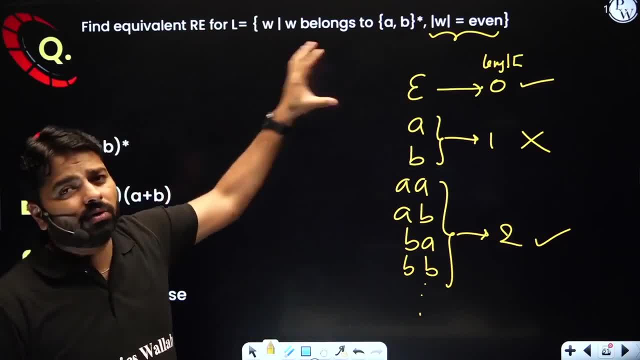 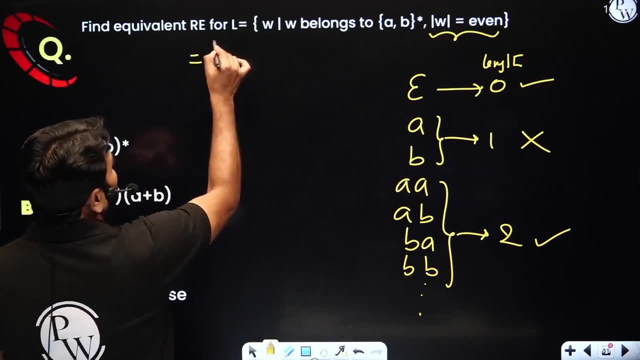 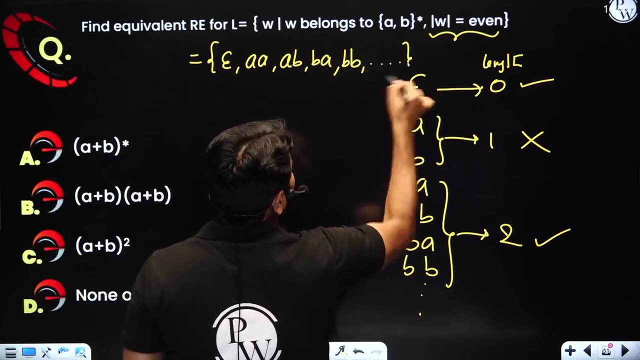 language which has all the even length strings, language which has all even length strings. those are nothing but epsilon w, a, b, b, a, b, b and so on. so i'm writing those strings here: epsilon a, a, a, b. writing all those even length strings are difficult in in listing format. so 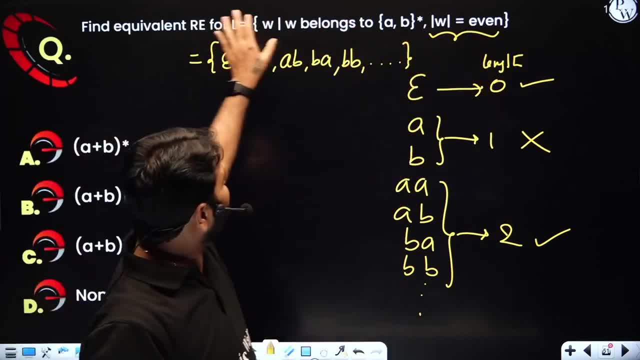 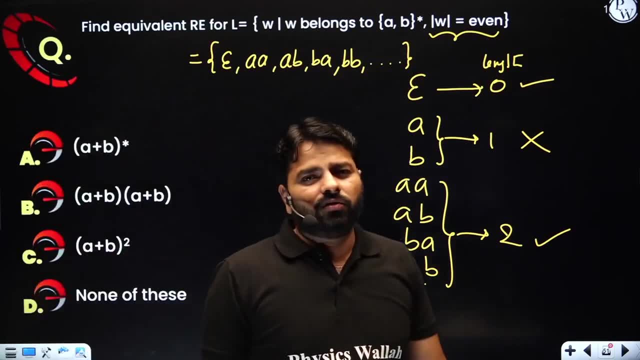 we have written a conditional set format right. so i mentioned all the conditions in the set and that will give you all the strings which are having even length. so now we got a clarity. we have a language which generates all even length strings and we have an expression. we want an. 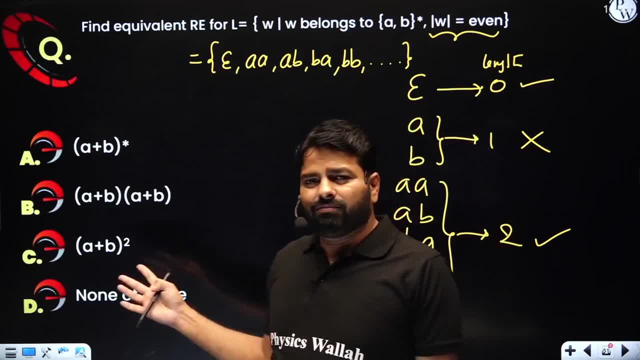 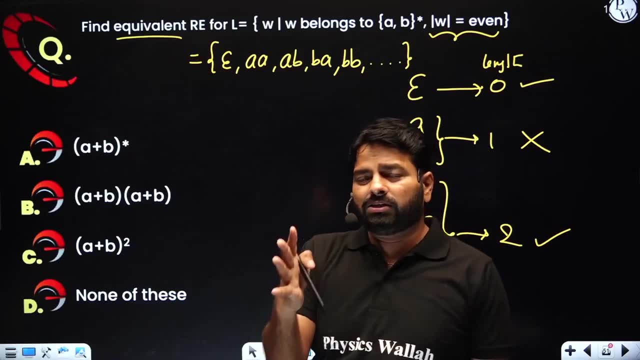 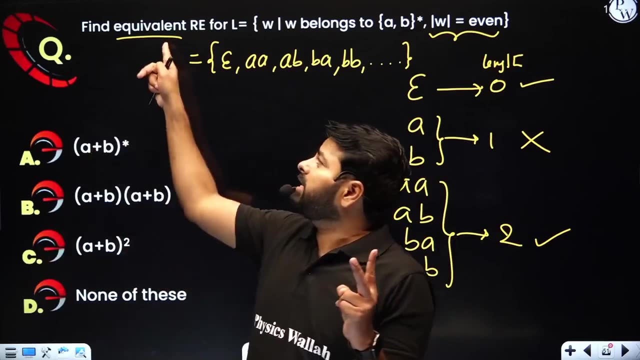 expression for that. okay, you may have, may not have, but you should understand what each one does. okay, so we want equal length. remember, we want equal length. that should only generate, and it should generate all even length strings. remember, two words are very important when somebody is saying equal. 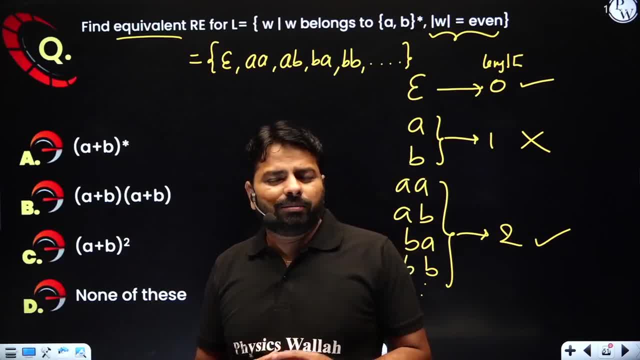 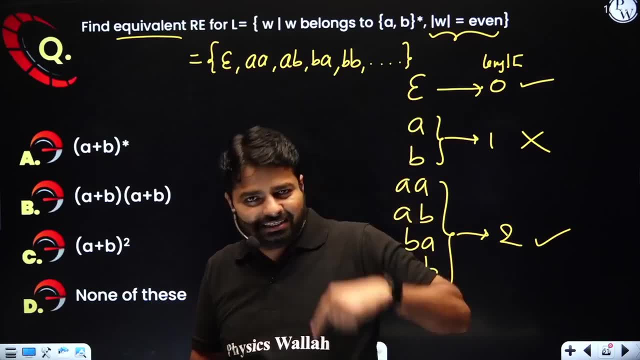 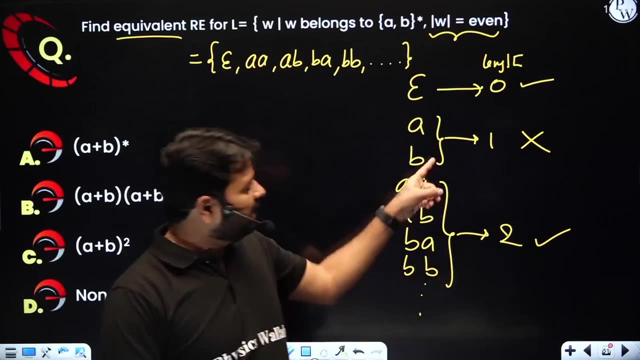 length are denotes. remember, it should generate all what you need and it should generate only what you need. it can't generate even one extra, one less. okay, a plus b, whole star. you know already. it generates everything, including one length, so that we don't want, right? so what is the relation? 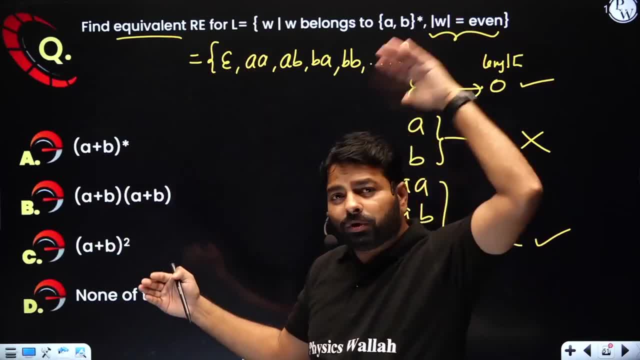 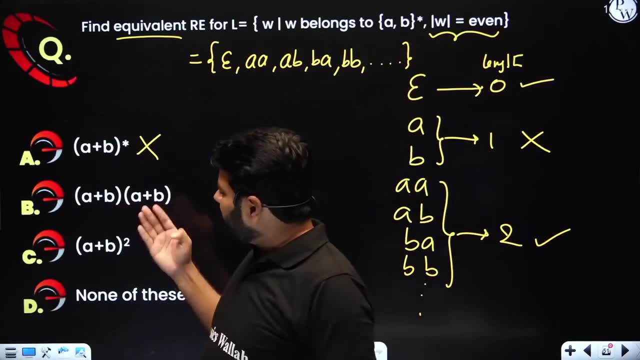 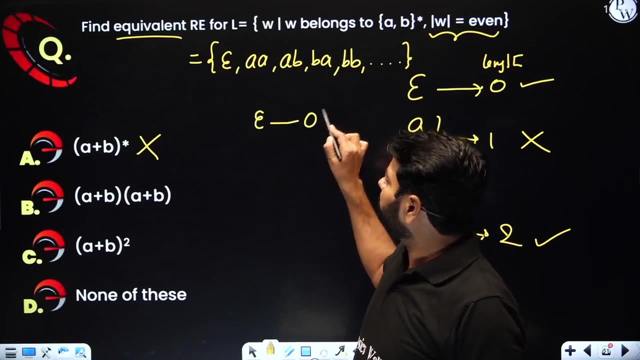 it is a superset, it's not equivalent. it is a superset, so definitely we don't choose it. okay and oh, what is this? and how do you understand this? this form, especially now? remember when i write epsilon. what is meaning? the zero length when i write a or b? oh, one length. now you may have a doubt, sir, only when i write a is also one length. 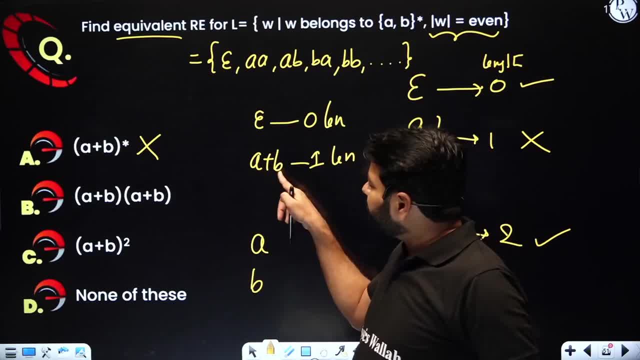 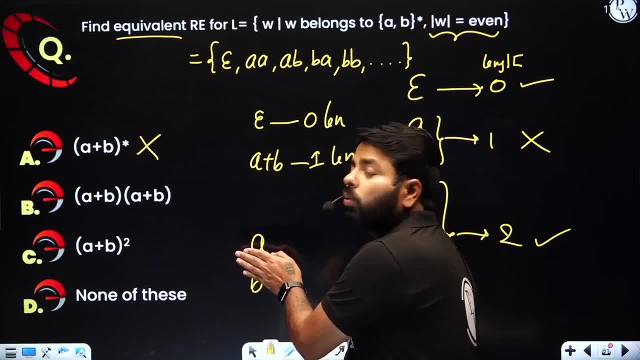 and only when i write b is also one length, then a plus b also one length. what is the difference between these three? when i write a, one length, but not all one length, it's only a- a. when i write a- b, it is also one length, but not all one length. but when i write a plus b, 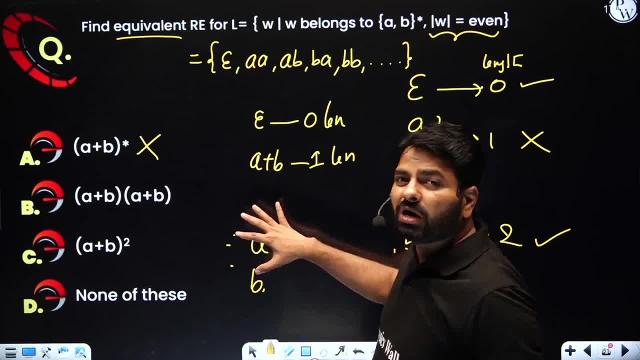 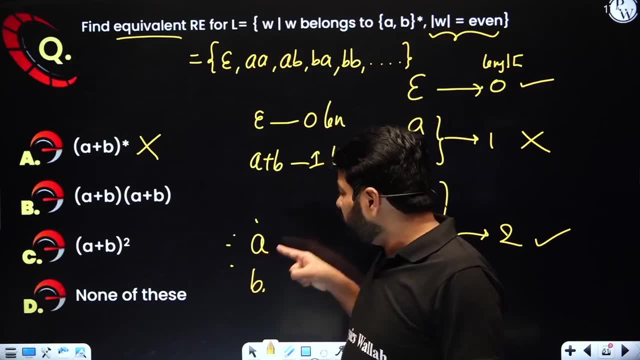 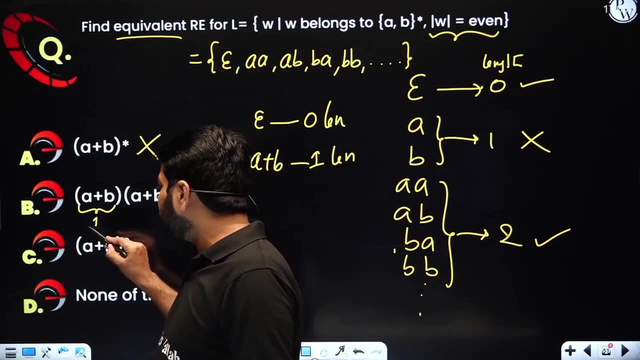 it represents all one length. you can't miss even one one length. that is the difference. even though a is one length, but it can't generate a, b, it's a specific one length. remember, specific one length. now, this will generate one length, this will generate one length and overall it will generate. 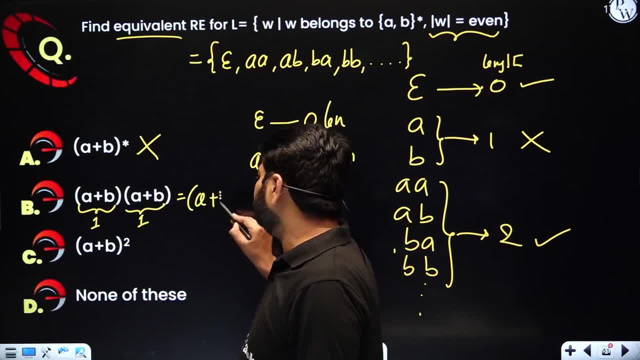 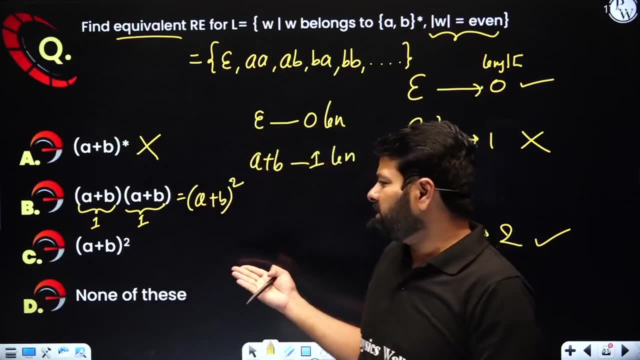 just two length. this can be written as a plus b. power 2 means it is generating only these two length. it is not generating zero length. four length, six length. so this is very specific case and it's obviously same as a, c, b and c. both are same. there is no difference, right. 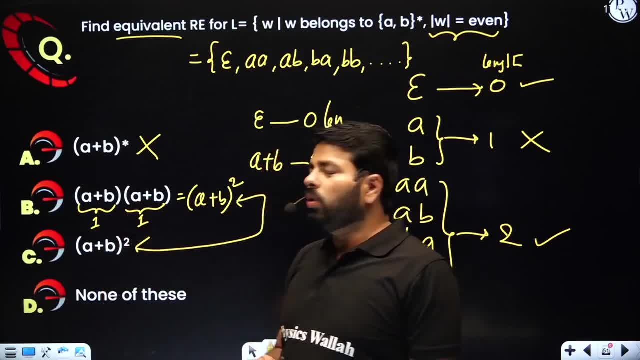 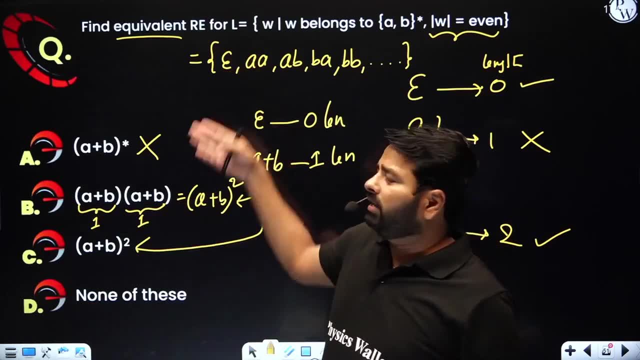 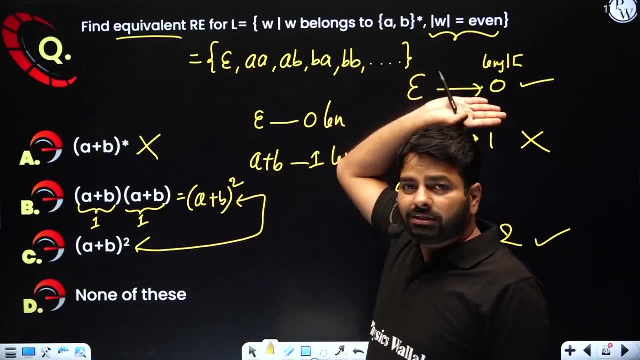 correct. so these two are generating only two length, but we want all even length. so b and c also not correct. it's not equivalent, even though it is even length. even though it is even length, 2 is even length, but it's not all even lengths. we want equivalent. remember the word? 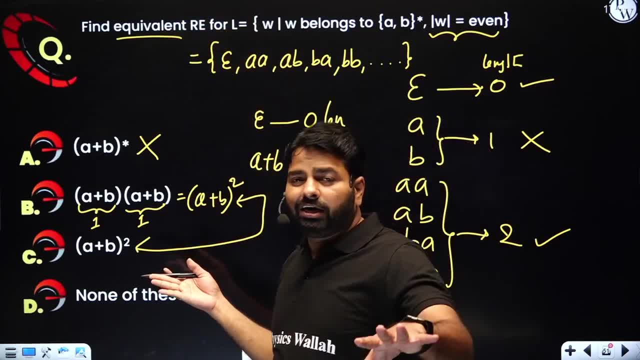 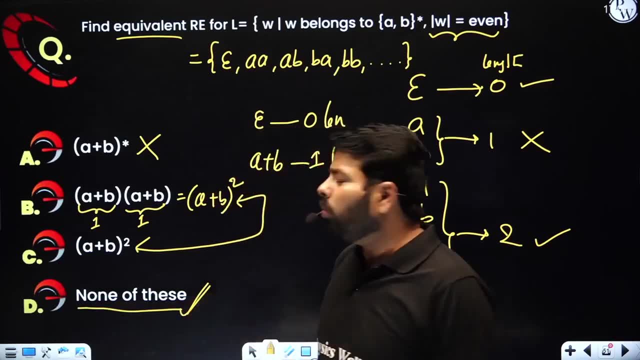 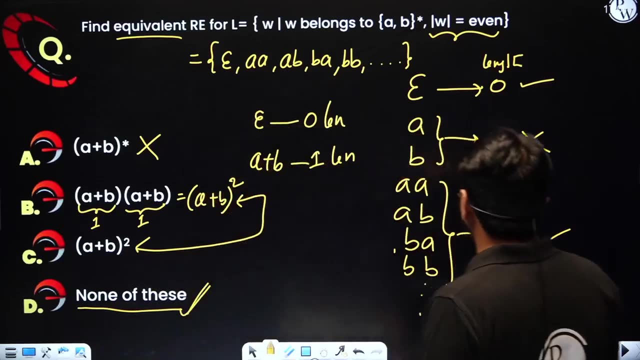 so here we don't have an expression that generates all even length, so we choose option c, option d, sorry, option d, none of this. what is the actual expression? now you may get it out. so how do i write an expression that generates all even length strings? so let's do that. the answer is here only. 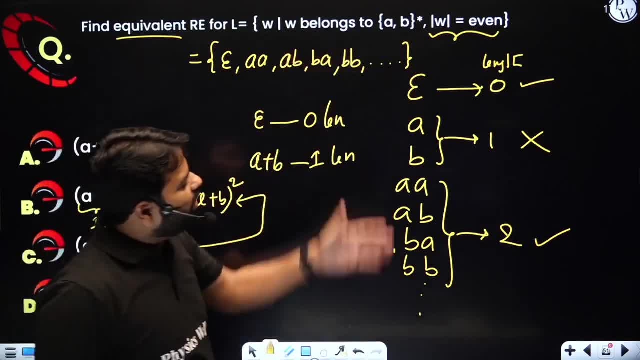 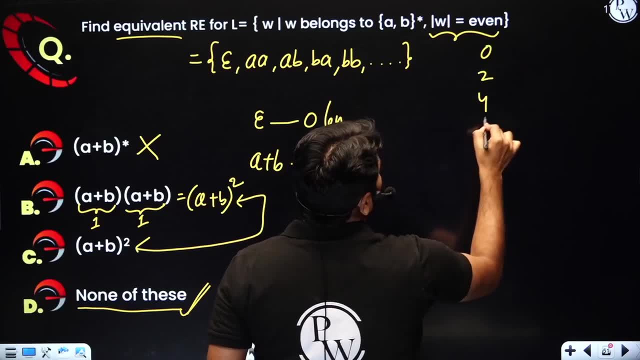 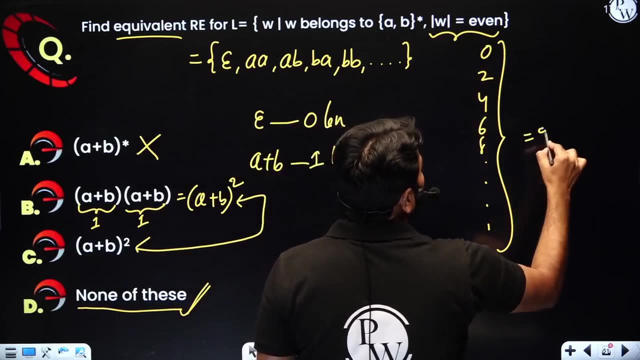 here also there. see, if you want to generate all even length, okay, just let me write here what is even length: 0, 2, 4, 6, 8 and so on, right, how do you do that? basically, for this, just you need to have some variable, right? somebody should say: uh, 2k, where k greater than or equal to 0. so if 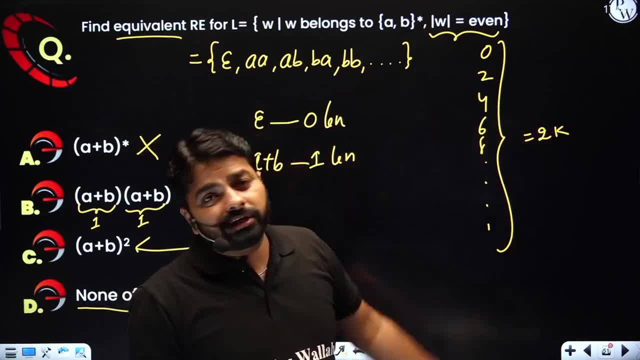 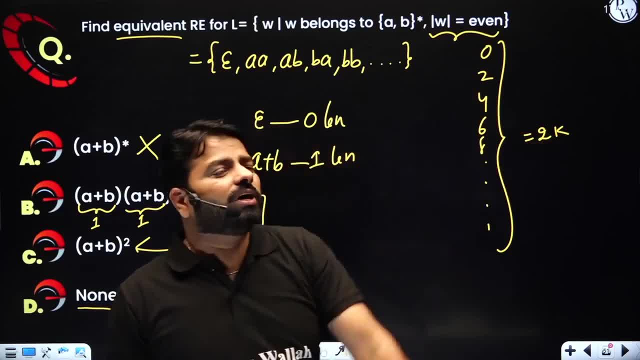 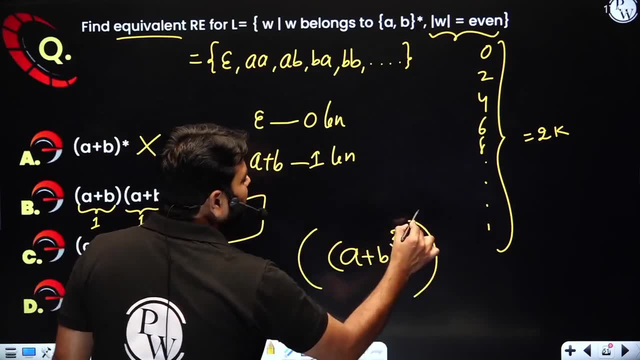 2, 2, 4, 2, 3. so that means, if you should know 2 length. so already you know the 2 length. right a plus b, whole square is a 2 length. this 2 length you repeat as many times you want, you will get. 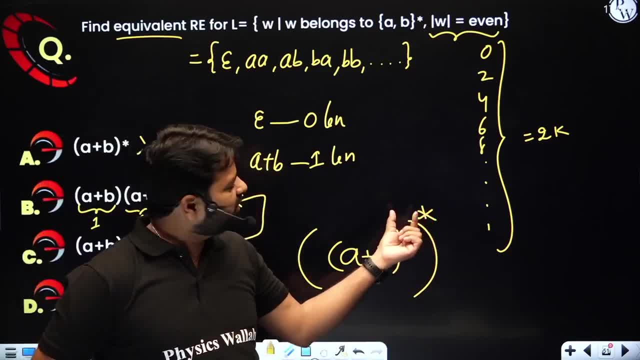 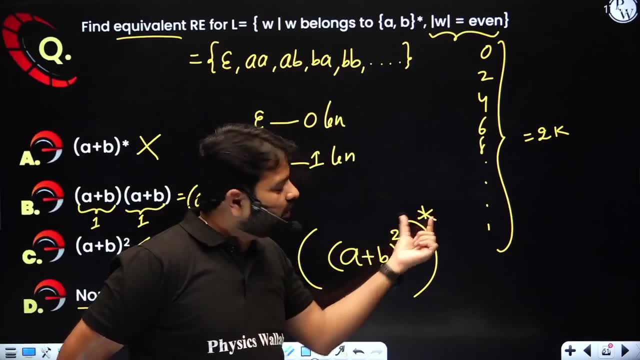 even length. c star means any number of times you repeat 0 power. 0 means you will get epsilon power. 1 means you will get all the 2 length here. you put it 2, then this a, this 2 length. you repeat twice, you will get 4 length. so this form you will have. 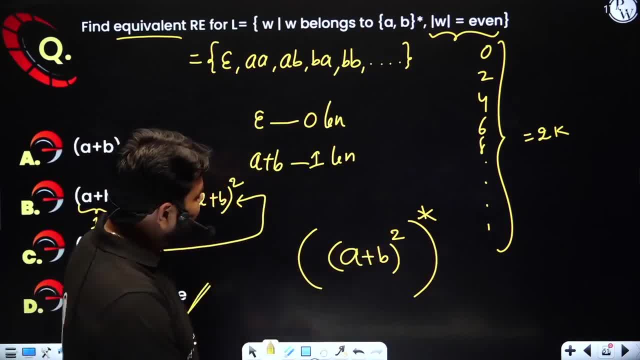 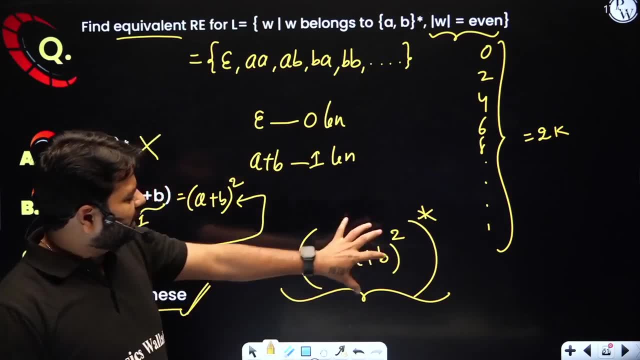 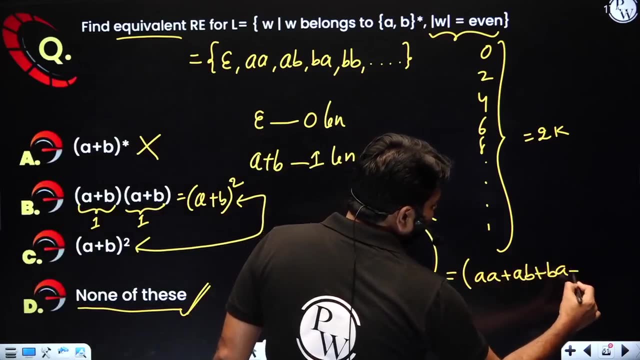 all even length. so this is the right expression for this answer. okay, a plus b, whole square, whole star. maybe you can simplify this. if you want it, there is another way to write, like double a or a, b or b a or double b, whole star, and you will get all the even length strings. 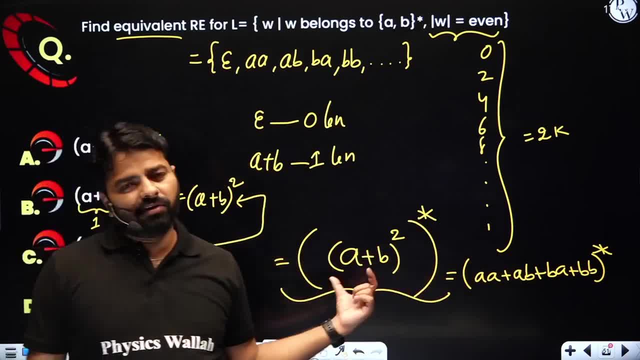 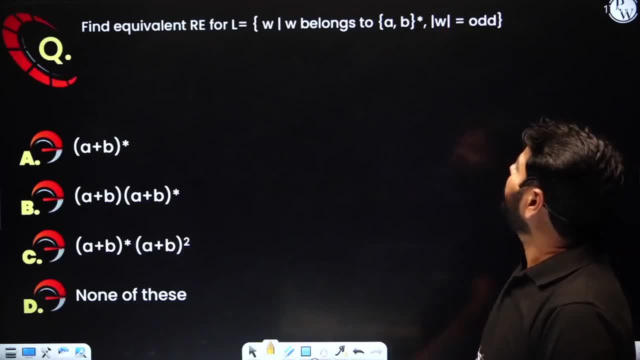 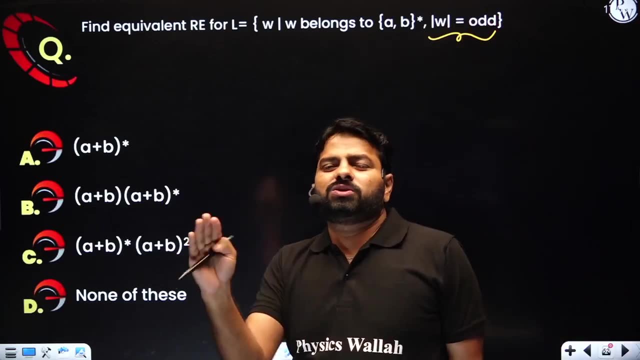 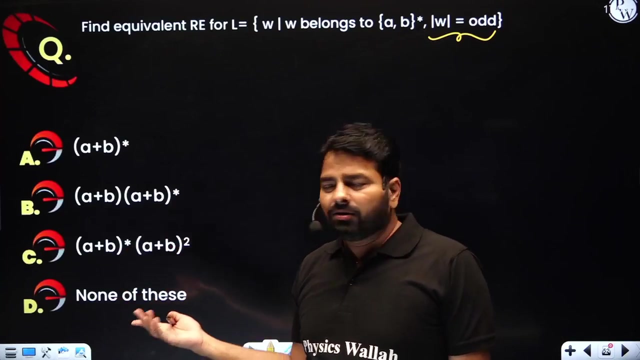 you will get all the even length strings. you can represent any form, okay. next one: all odd length strings. oh, what's the difference between even and odd? for even, you just do one more length, extra concatenation, you will get odd length, okay. in mathematics, even plus one is always odd, okay. so this is going to generate all we don't. 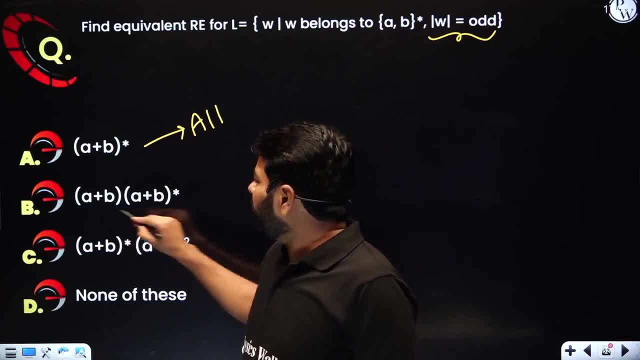 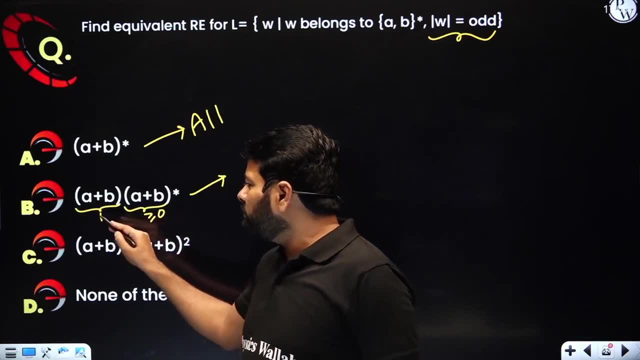 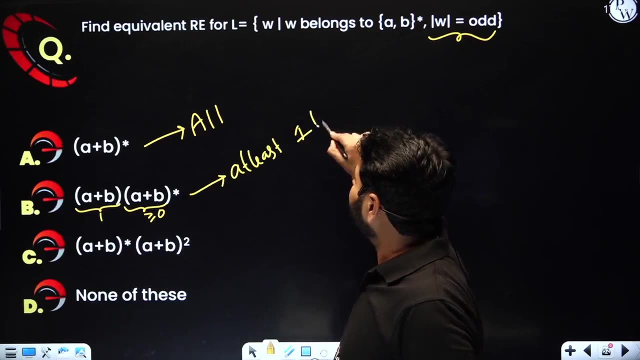 want all here. now you know at least one, because this a plus b is one length. this will be any length overall. when you do one followed by any will be at least one. so here at least one length comes, here at least one length. i'll just represent length of w greater than or equal to one. all means length. 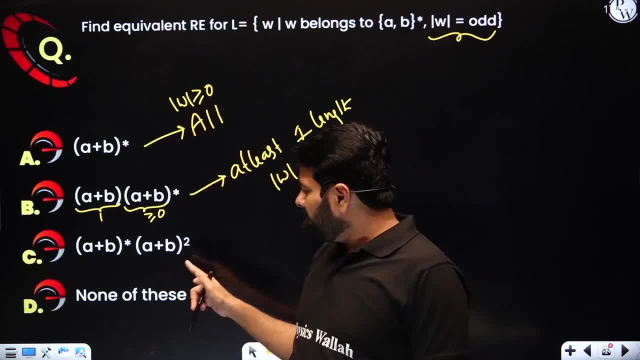 of w greater than or equal to zero, and this one is just now discussed, right? uh, it's even length, oh not even at least two lengths. sorry, it's not whole star. this is equal to two. this is greater than or equal to zero. what do you get? this is equal to two. this is greater than or equal to zero. 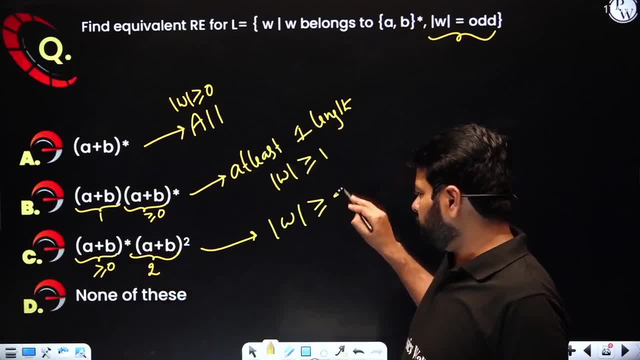 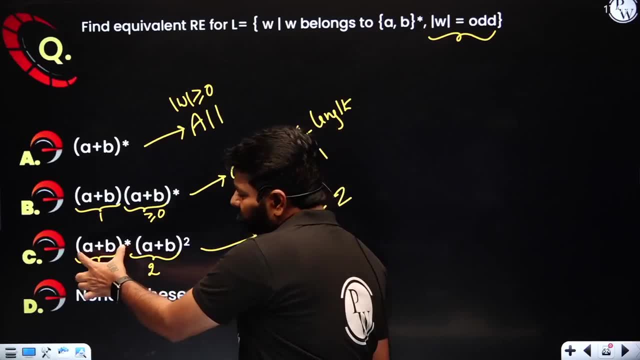 so what? you get length of w greater than or equal to two. from two onwards three length extra one. you take already. two is there. if you take power one, you will get a three length. if you take power two here, you'll get two to four, and from two onwards every length can be generated here. then what is? 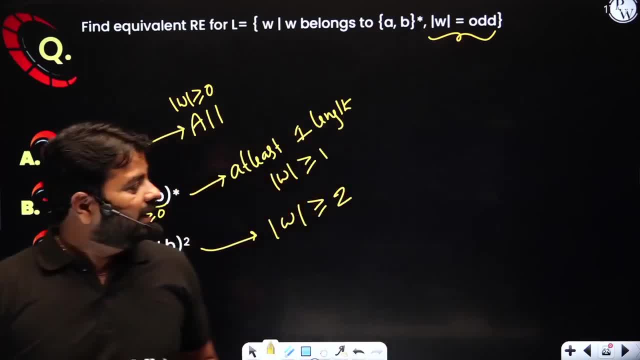 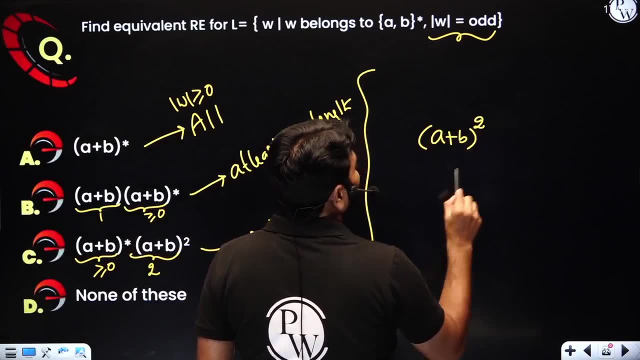 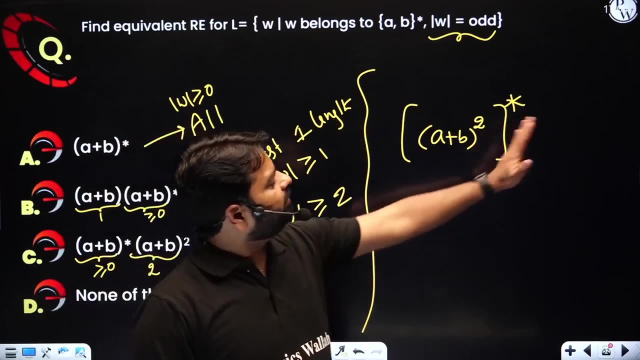 the question: you want odd length. how to do that? even length already. you have it. take that: what is even length? a plus b over two, that is two length. you repeat any number of times: this is even now one length. you concatenate after or before, you get odd length, already even length. 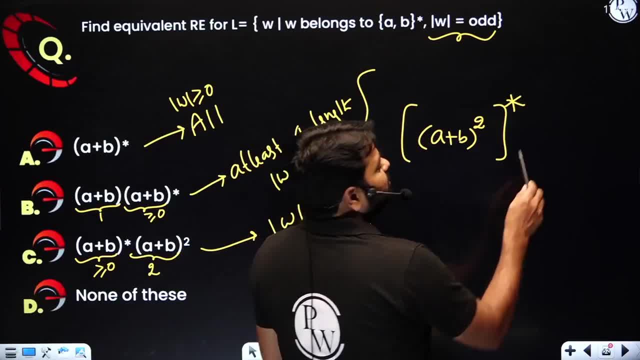 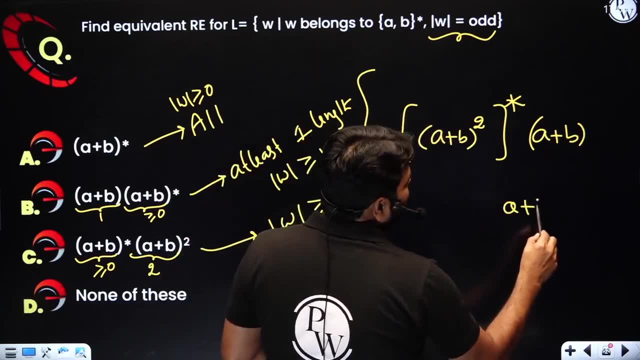 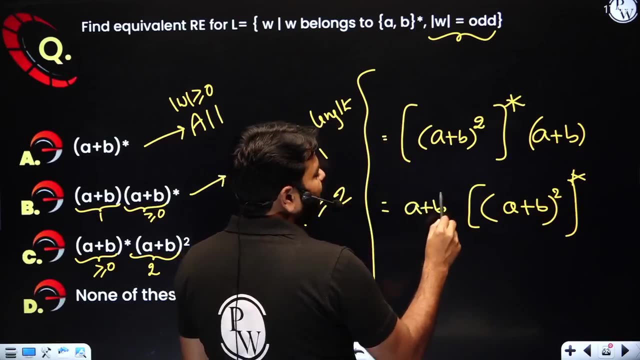 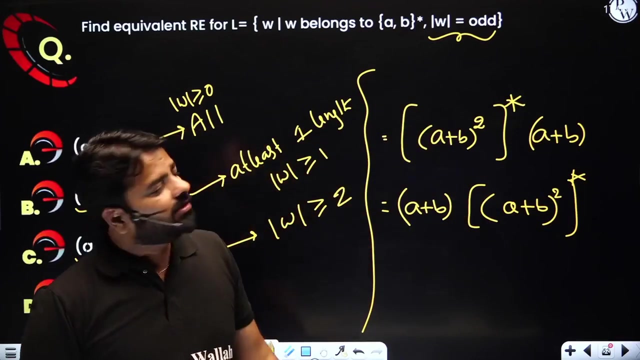 epsilon is generating, but odd length will not have an epsilon. you take just a plus b at the end. or you can take a plus b, whole square, whole star. you can take one length before. also we'll get the same meaning. you'll get the same meaning. both will generate odd lengths, all odd lengths. now you just try it. what do you mean by? 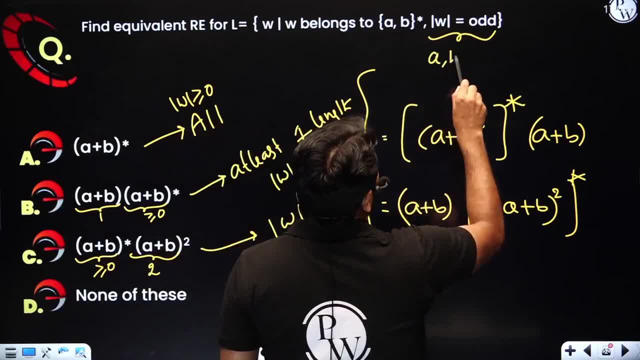 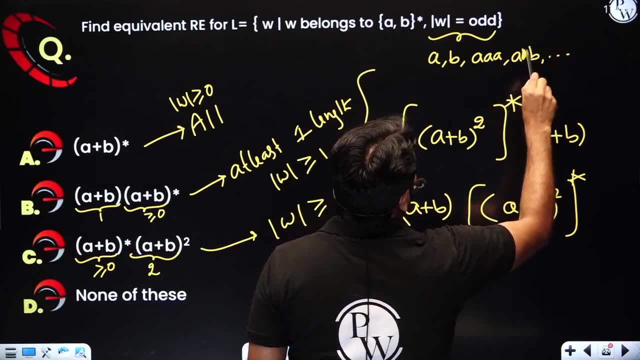 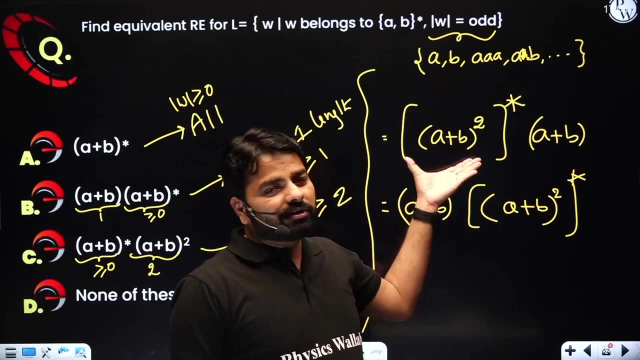 odd length. odd length is first a or b, then three length, oh, three length. there are many strings. the writing will take time, so i'll just keep like this. okay, you are guarantee that a comma b here. put power zero- you're already there- and three length. how do you get? take a power one here, so two. 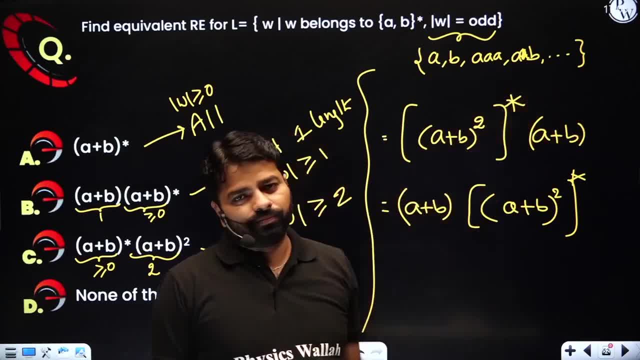 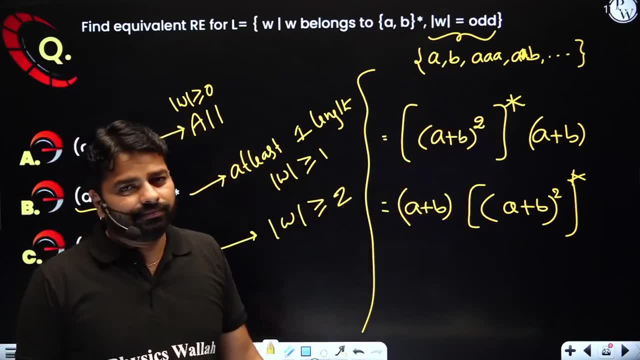 length followed by one length, you'll get all the three length. you'll get all the three length. similarly here also: okay, once you have even length, odd length is also almost same. but add extra one length to the even length, you will get odd length. okay, whenever you see the difficulty with the expression, just convert into very nice form like: 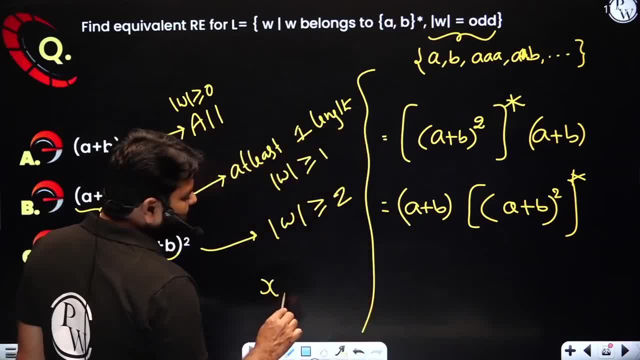 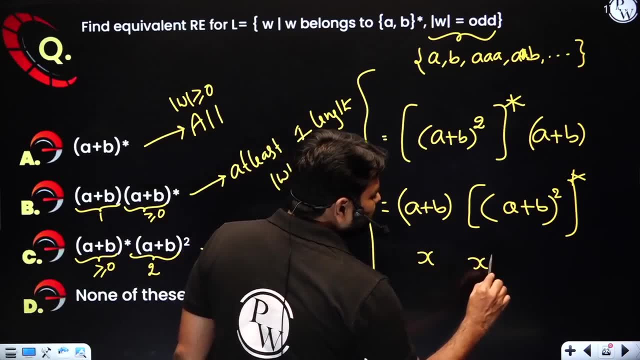 you know when, when somebody says like this: you know x is nothing but a or b, assume this then how it looks like x, x, square, whole star. how simple it is to understand. right, x is already. i know why it is so simple. i know why it is so simple. i know why it is so simple. i know why it is so. 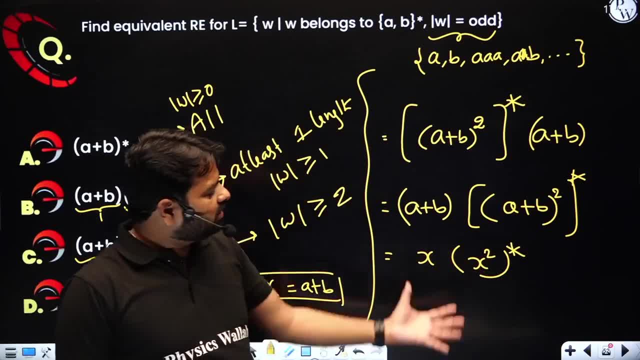 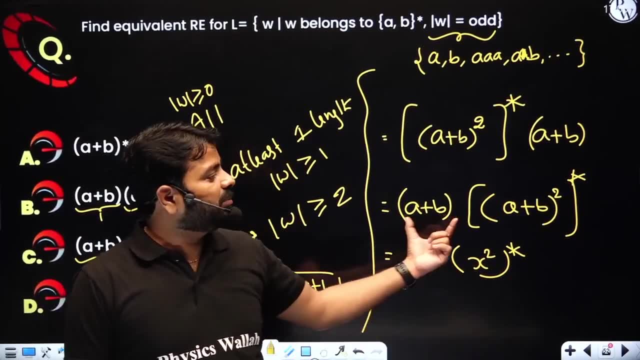 length, so x, followed by x, square, whole star. this looks so nice, right? and when the language is over one symbol, we always write this way. but when the language is more than one symbol, you need to represent properly. okay, but same one. you can denote for the two symbols also. but as 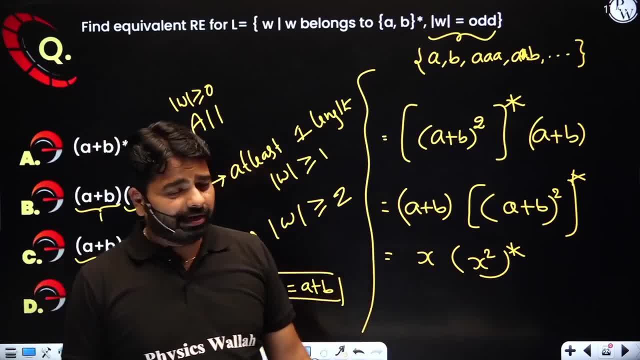 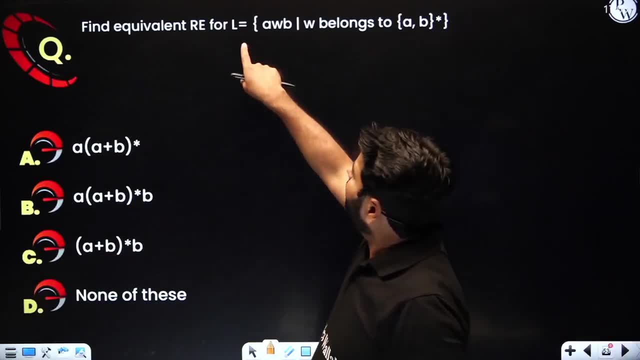 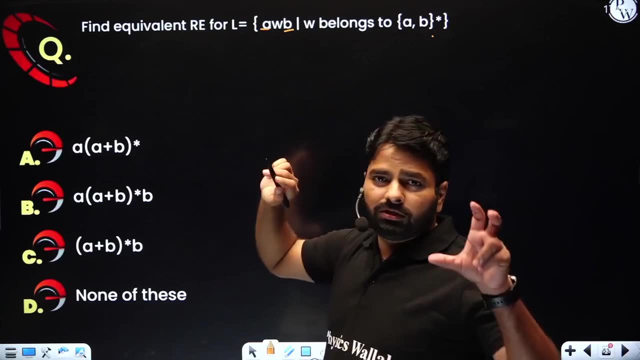 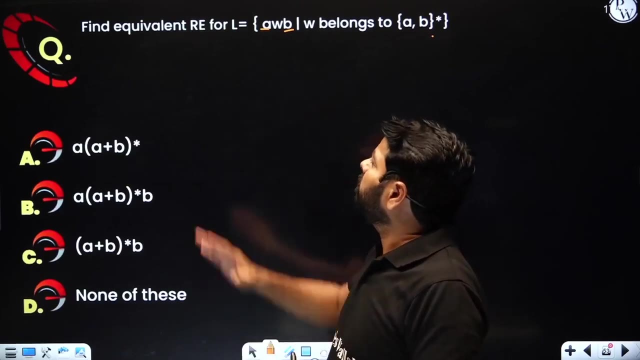 if x is equal to a plus b, then you can write this way: okay, we have the next question, which is um, having a language starting with a and ending with vc. w is anything starting with a ending with b. here important concept is you should know what actually language has. the language has strings. 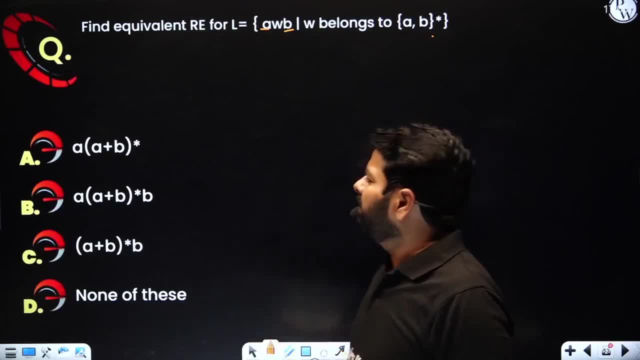 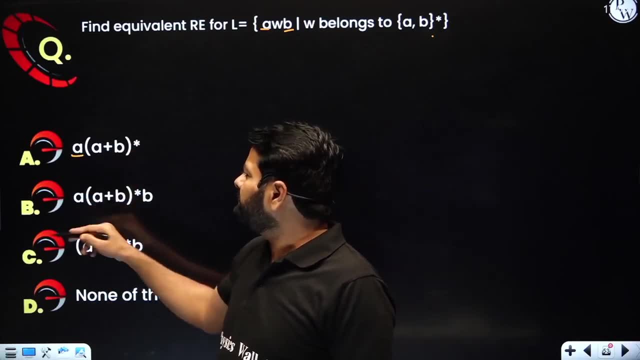 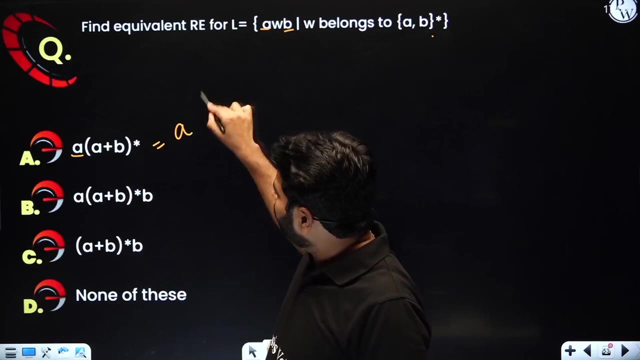 starting with the ending with b, then expression would become very easy. right in this four or three options, which of them is doing that? starting with the ending with b is only having starting with a. there is no restriction on ending. so this, this is starting with a problem you may just represent as a, followed by something. 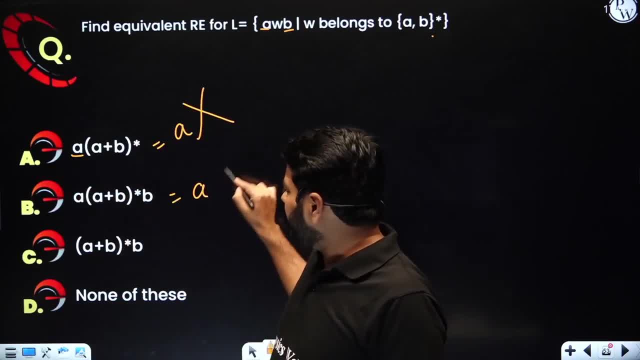 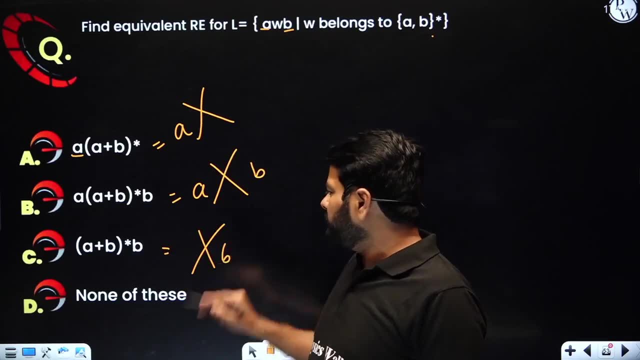 that's it. and this one- yes, it has a and anything definitely ends with b. this is what we are looking, and this one- anything is there- followed by b. this is for ending with b. in this, there are three problems: starting with a, starting with the, ending with b and ending with b. the question is very 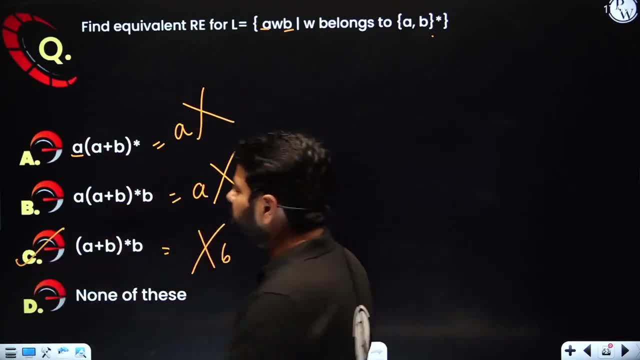 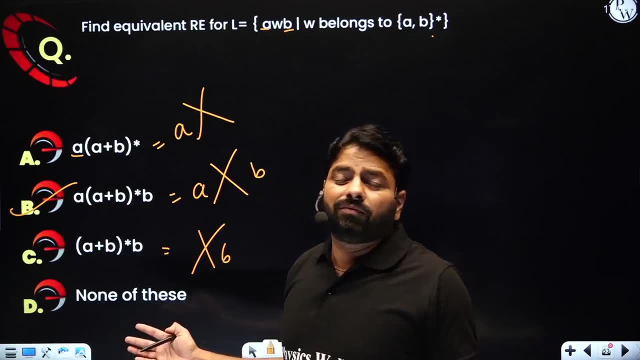 clear, starting with the ending with b. so we'll choose options. sorry, option b, option b, starting with the ending with b. so this is how you unless see how much time it took once you know about the expressions. hardly it will take, sometimes even seconds, five seconds, ten seconds, but it all depends on the 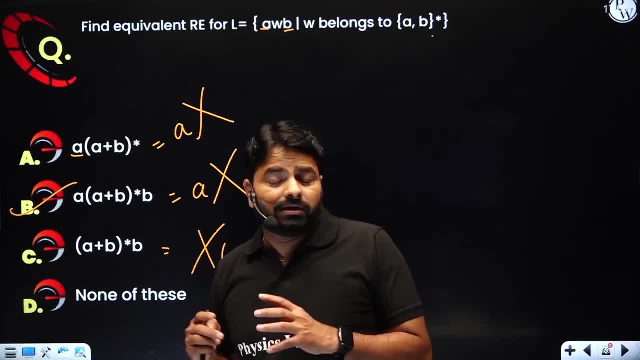 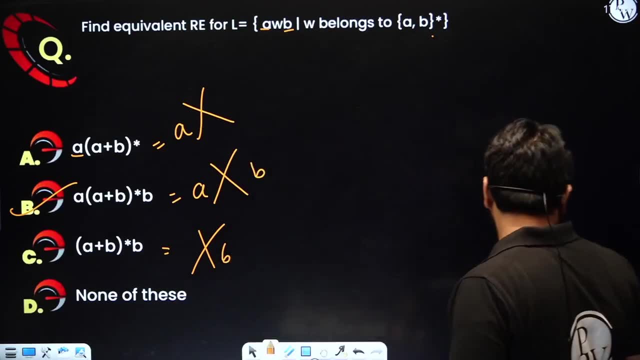 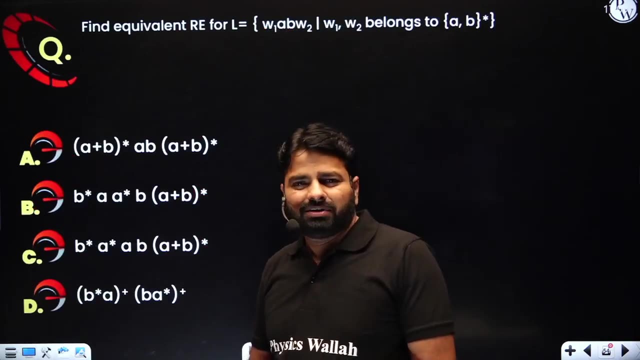 problem right, how good at your practice, how good at uh understanding and how you are practiced and how many questions are practiced. all matters at the end. next, sometimes, even though you practice lot and you may come with the wrong options or you come with the right options, but that's not enough. see, if this is msq question and you might. 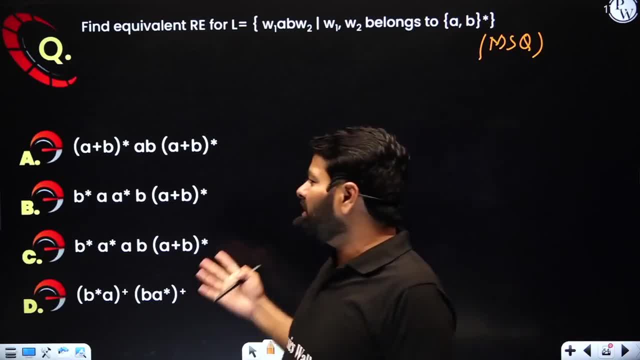 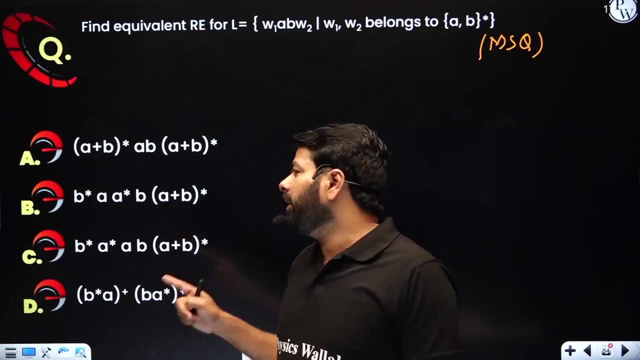 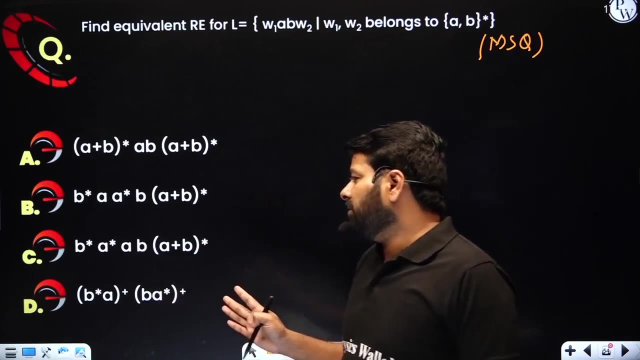 be worried about how many answers are correct. is it all or one or two? so here the challenging comes. so i'm saying it is msq and it's your job is to identify how many equivalent answers are there. so i may not be, you know, 100 percent. uh, explaining correctly right now, because you need a dfa to. 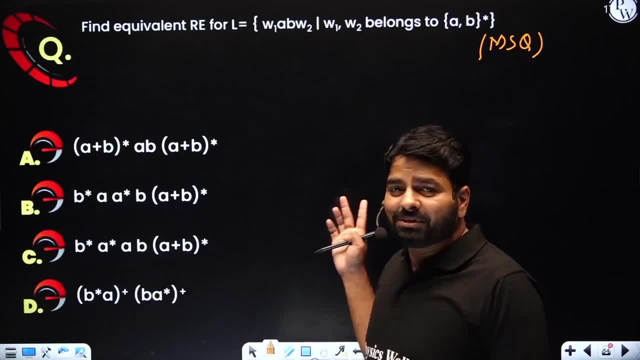 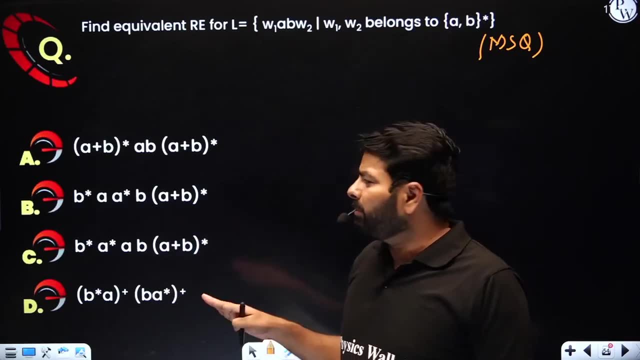 understand this behavior when you construct dfa for this deterministic motion. for that you will get to know why we are writing this. so spending much time on this question right now is not recommended. but i'll come to this question again. but let me discuss in my way first. 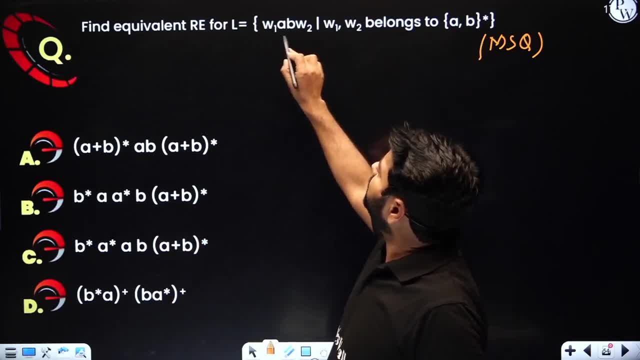 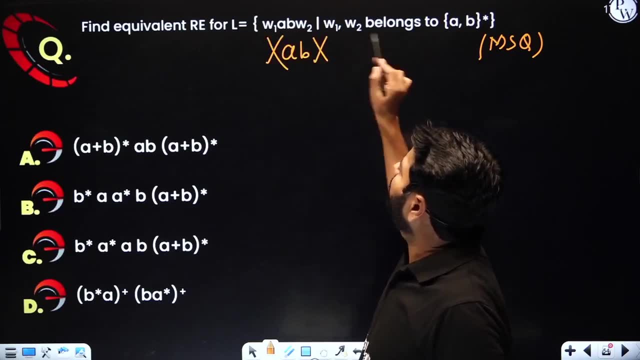 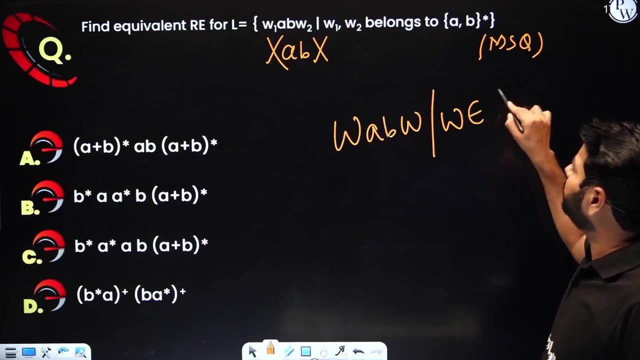 okay, what is the language for? language is it is having many strings, all strings, where contains a, b and before, after anything: w1 and w2. okay, you may have a problem if you write a, b, w such that w belongs to a comma, b, whole star, anybody. is this right way to write? 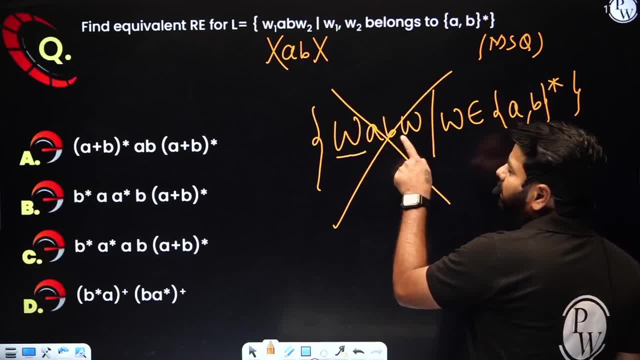 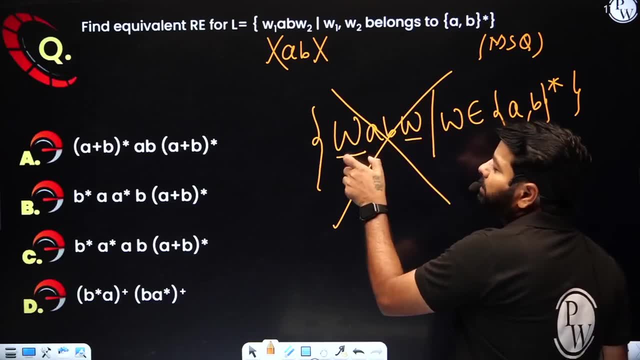 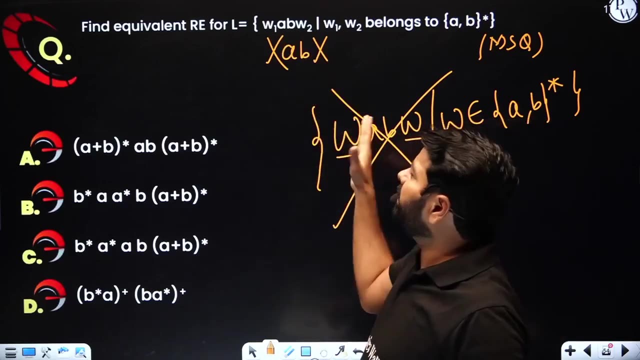 no, if you do this, you are saying: whatever is there, it is also here. but we don't containing a b before, after anything, not the same thing before a b. suppose triple a is there, after a b, also triple a. no need to be so. that's why we require w1, w2. the question is very clear: containing a b? containing a b. 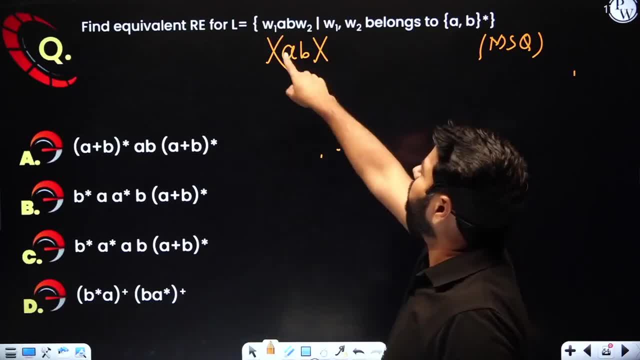 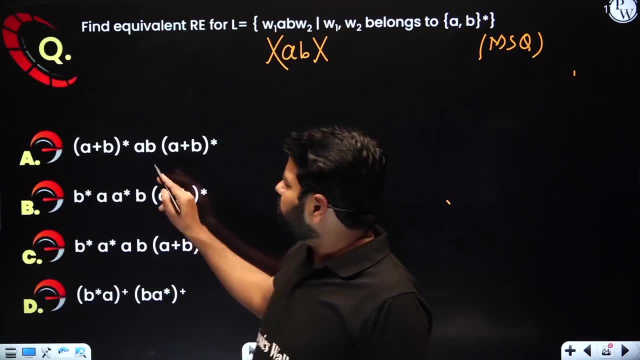 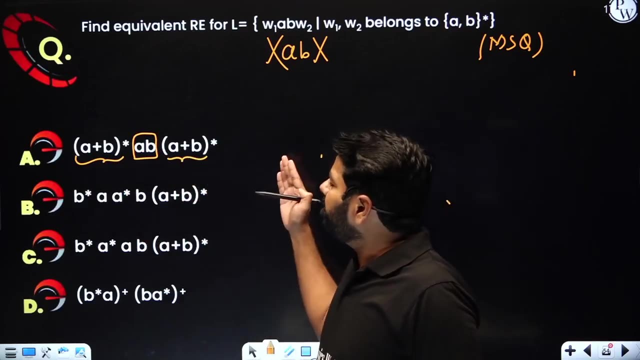 as a substring. okay, that's why we need to write two different variables to represent: before a b, after a b. okay, now in this, when you look at the first option, oh you are great. a, b is there and anything before and after, also anything. definitely a is correct, no doubt a is correct. 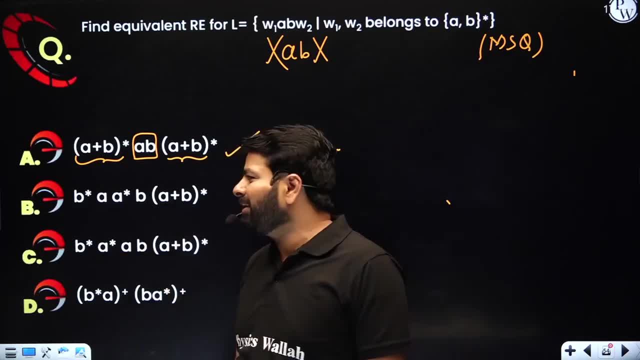 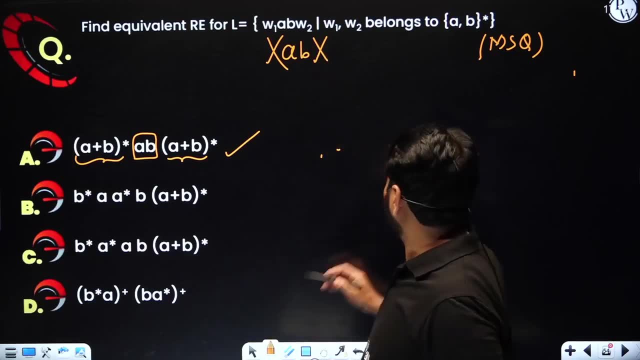 that doesn't mean that others are wrong. right, you should know about the properties of these expressions too. okay, what kind of property you look? now you know containing a b, so now let's behave it like containing a b is there if you want to see the first time a b here. no need to be if there are two a b's inside the string. 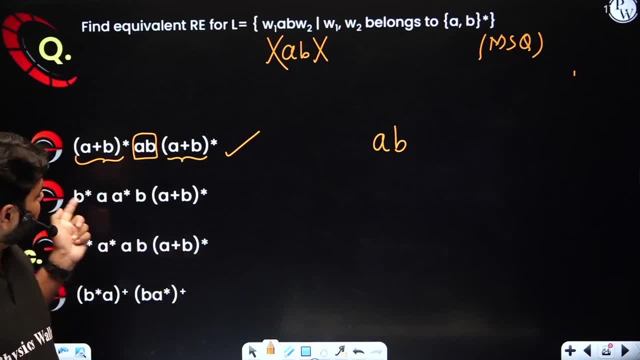 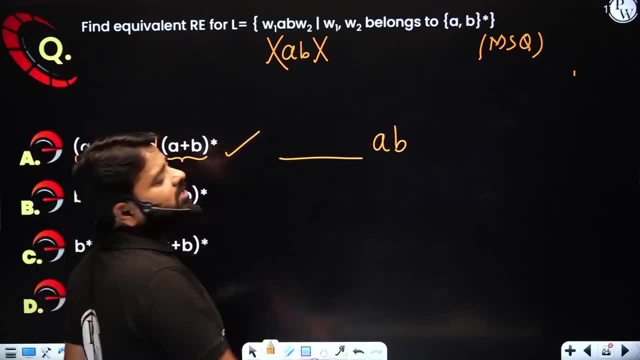 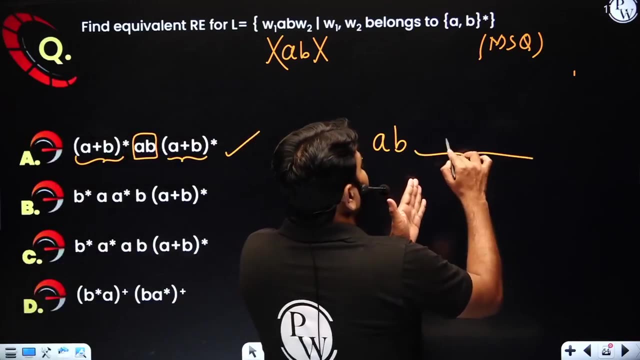 this: a b could represent any a b right, but there are some other ways to represent a b. suppose first time a b comes, first time before that, what possible sequence may come that never contain a b, because you are looking for a b right after that. anything is fine, after that any, but this is the first time a b, first time a b appeared. 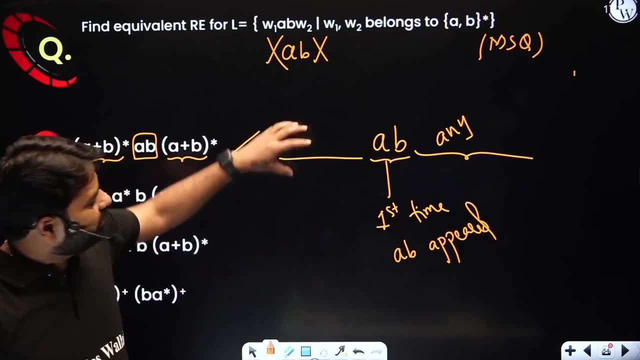 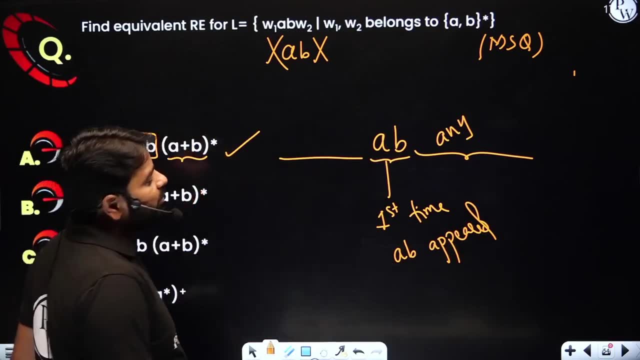 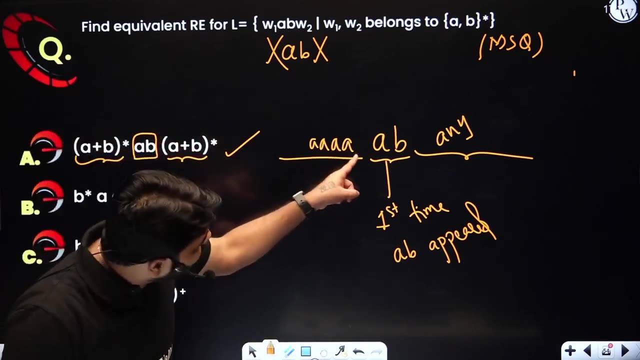 then what is the possible sequence you have here and i never will. i will never have a b here, right? so can i have any number of years? yes, you can have any number of is, any number of is. can i have any number of b's, but not after before that. any number of b's i can. 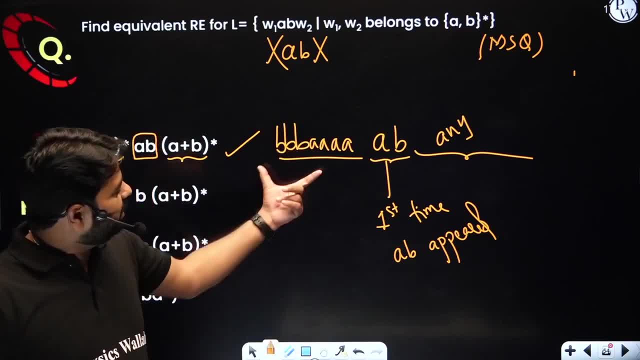 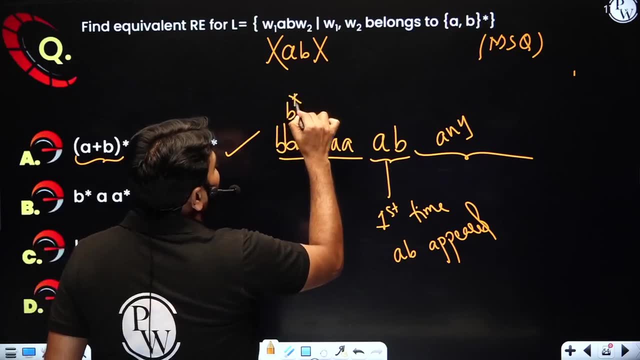 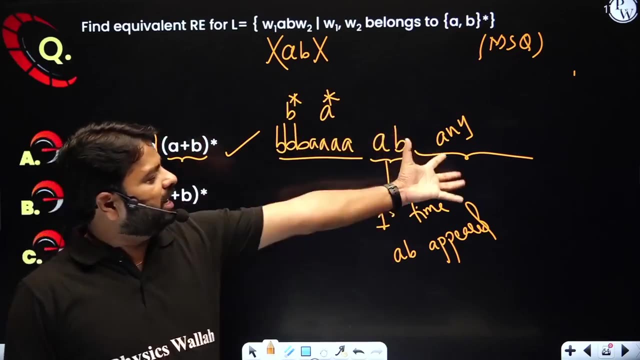 have. still i don't have what a b. so there are two choices: b and a's. any can come, but b is followed by a's. see here something like b star, a star can happen before having a b, before first a b. once you have a b doesn't matter. so this kind of form can also generate the same language. that is very 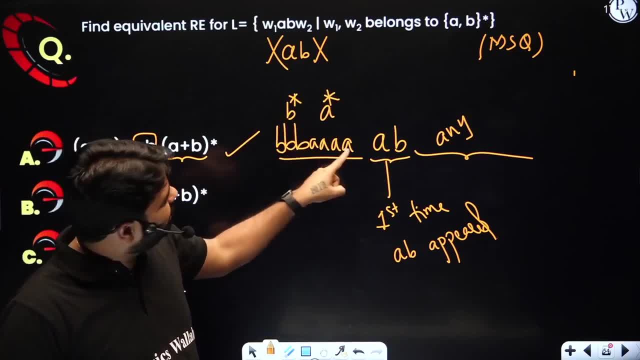 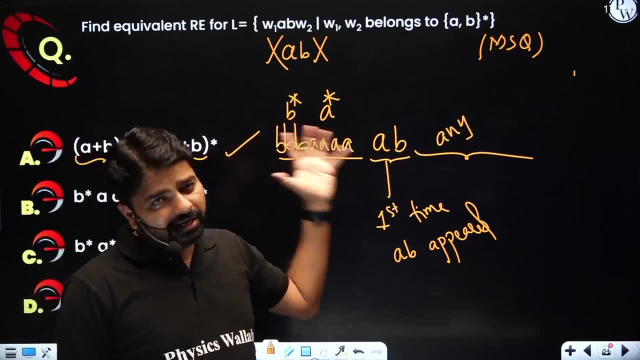 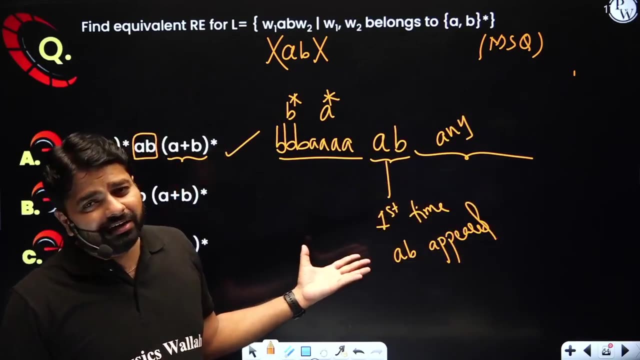 important- see b is still a is not appeared from this a b, so we are waiting for that. once a's comes, any number of a's doesn't matter, but followed by b will give you containing a b. so one of the difficult only when you don't know dfa, when you know the dfa, because to design a dfa 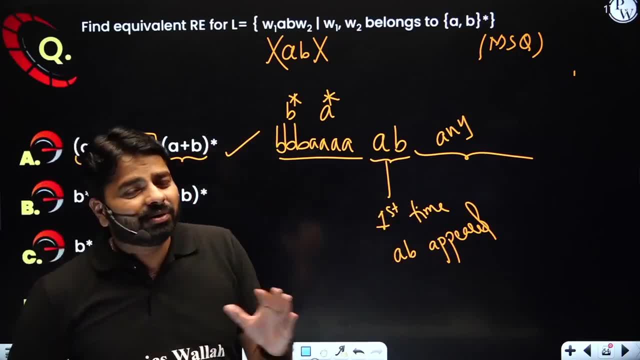 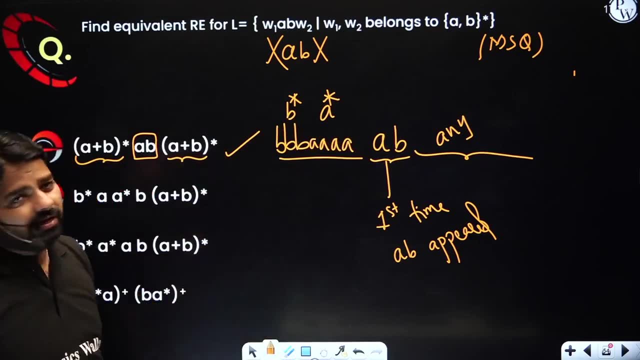 you have to think this way. there is no other way. there is no other way that you can construct dfa for this, okay. now, if you want to construct dfa directly, you have to think this way, right. but there is a technique. we have techniques to concern the dfa by taking the minimum string. 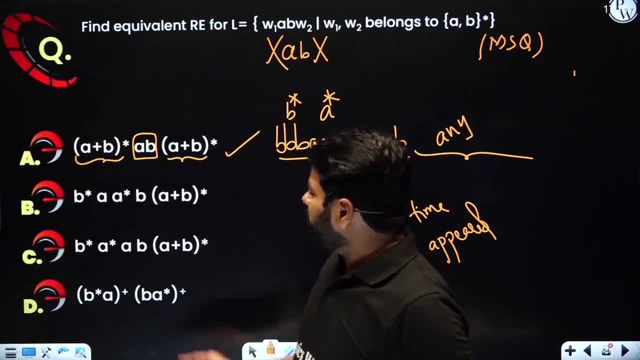 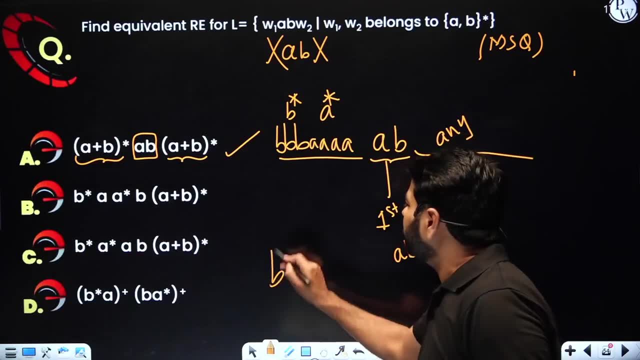 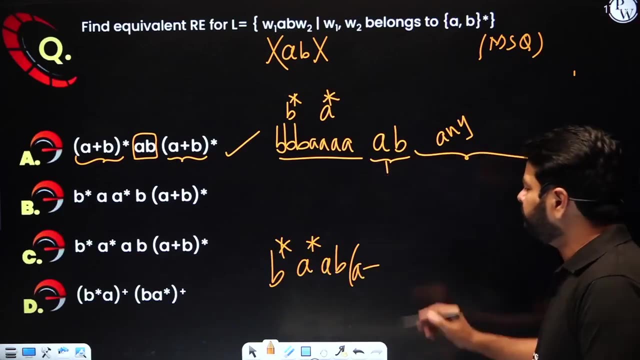 here. okay now look at this. here: a star a. oh, no need to write in this in this way. look at that. i'm just writing here: b star a, star a, b, followed by a plus b. this is the expression i have explained, but you can this. two are together, right. 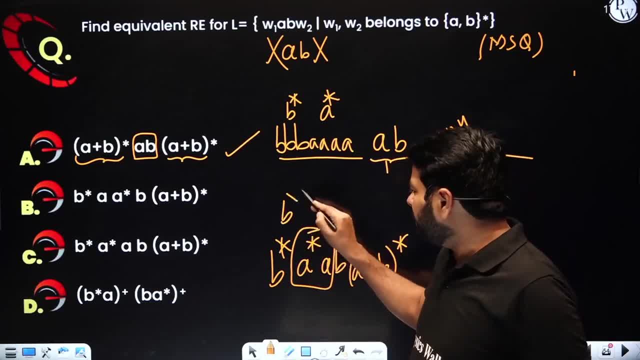 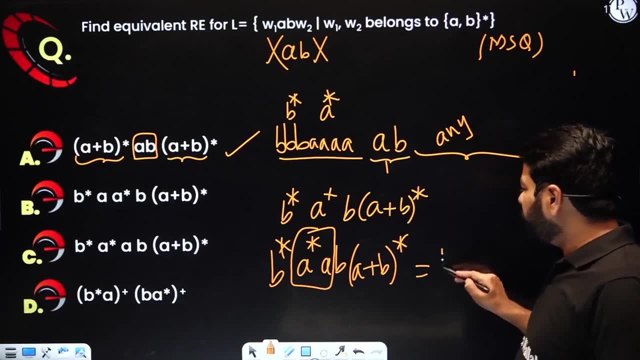 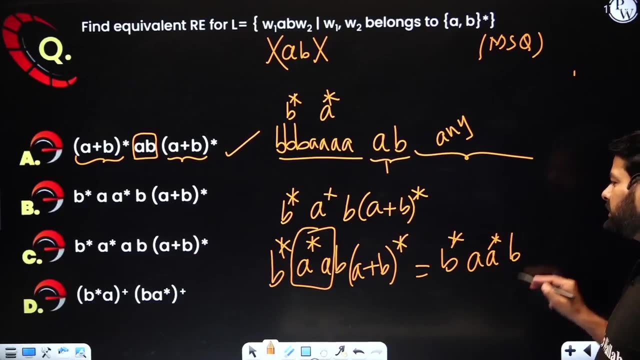 you can also replace with a plus right b star, a plus. this is another way you can write. or you may write b star, a star. you can also switch like a a star, a star, a a star. you can switch any, because both are same. see that how many ways you can write. these two are actually same: a star you. 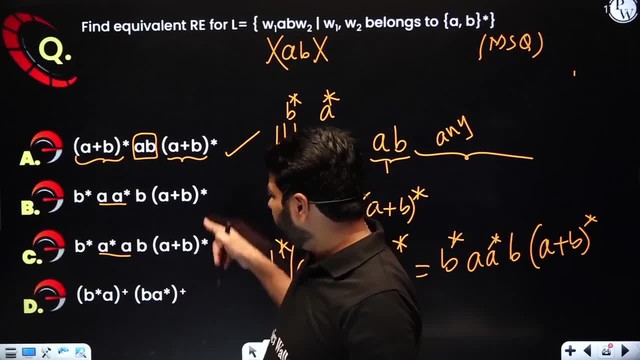 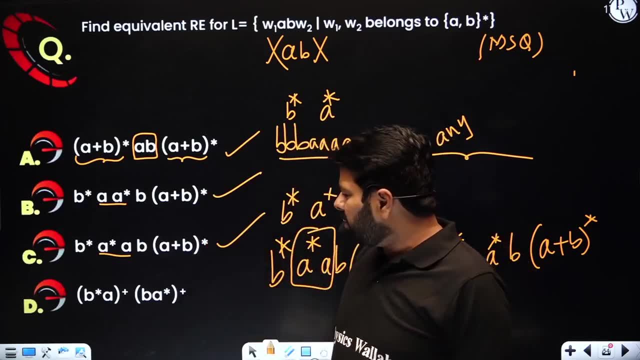 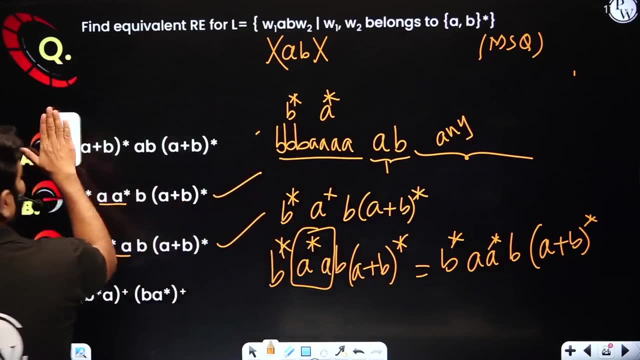 can write a star, you can write. you will get the same answer. right, these two are also equivalent and again have a doubt how this is written. how can i understand this? sometimes you don't need too much, because already the question is very clear. look at the option a. look at the option a. this one is: 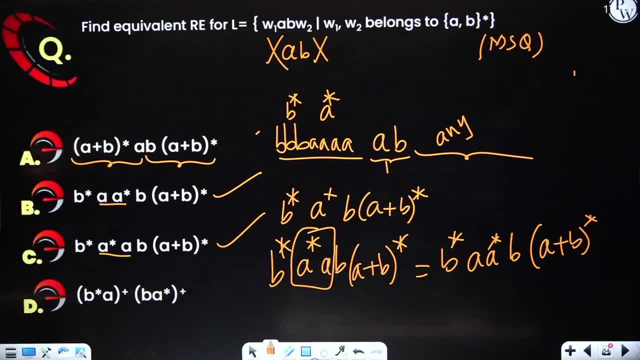 looking like ends with a. this one you. it's looking like starts with b. just this expression, this one- somebody has it in some other way- like this ends with a and this looks like star. of course, don't say that, but it is expression, right, this one i can replace with this: 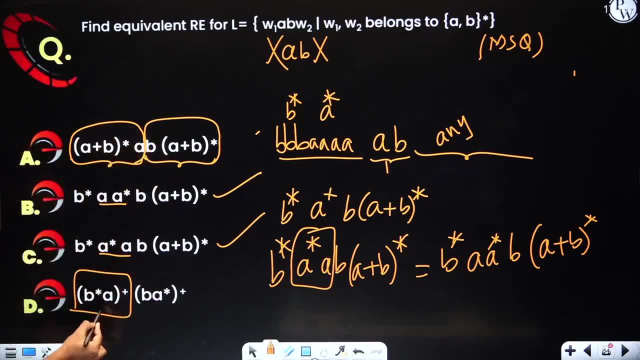 form, because ends with a form i can replace with this expression i just explained: ends with a and starts with b, how to write it. this is another form. starts with b and just replaced it. this one replaced with b- star, a whole plus. and this one replaced with b- a whole star, whole plus. that's it. 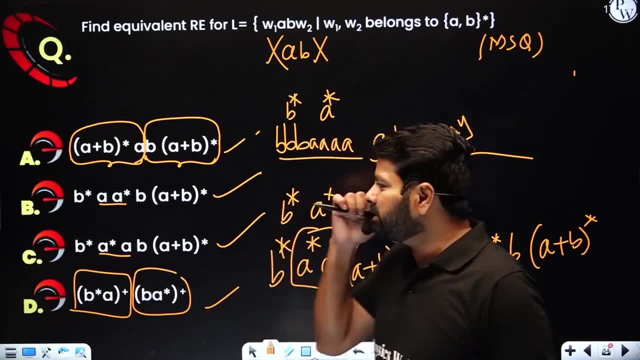 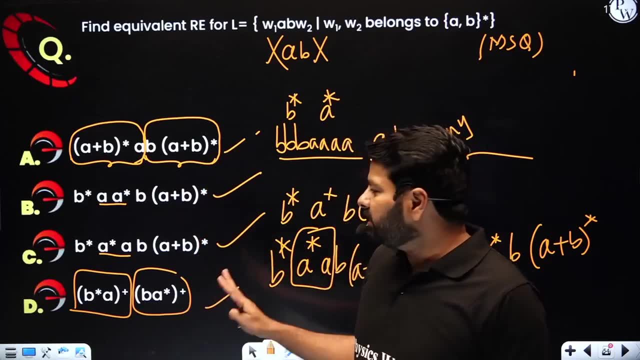 this is also going to be equivalent. the only thing is you, we must have much practice to know about all the different forms and which are important- as i said, everything is not important in the world, the world- but which are minimal and required for the exam. i have covered in the options itself. okay, 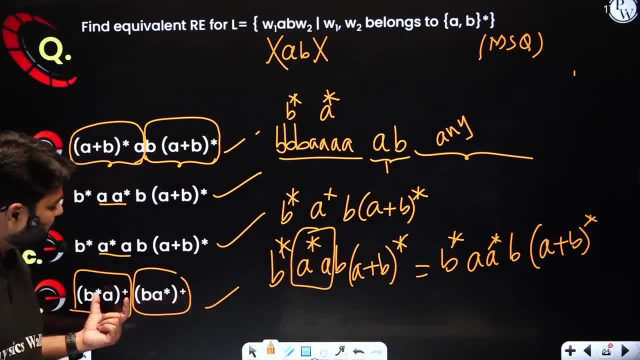 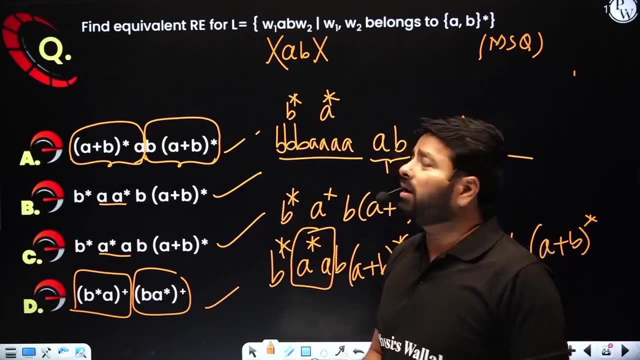 these are created by me, but these options were already asked in the gate, like: what is this, what is this? in future, they might give this and they put this in the options. you should think about their way. okay, fine, so all the options are correct. all the options are giving somehow, uh, containing. 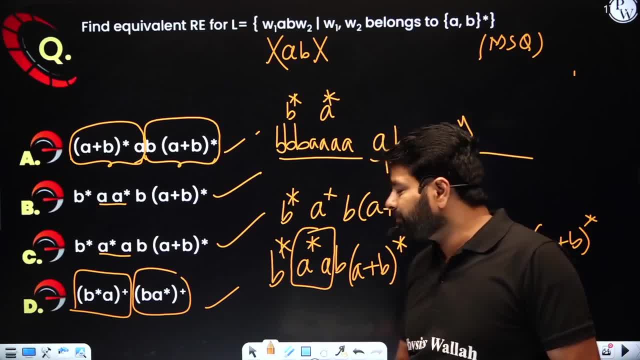 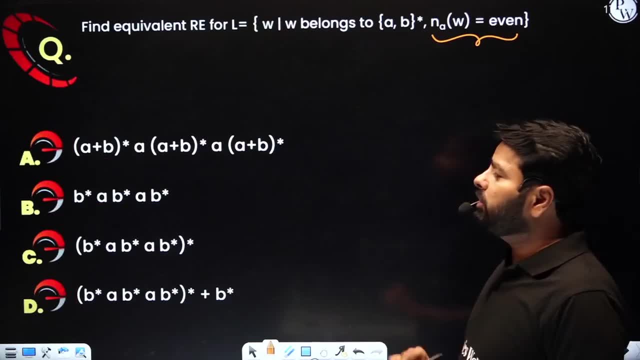 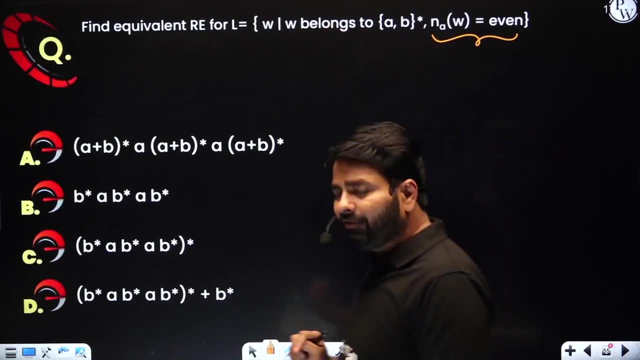 a b as a substance, containing a b as a substance. um, number of a's is even and no condition over the b. look at that. i want all the strings which are over a's and b's and number of ac is even here number of b's. we don't have any restriction. 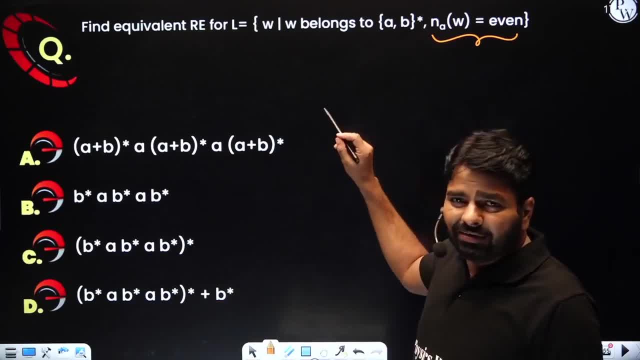 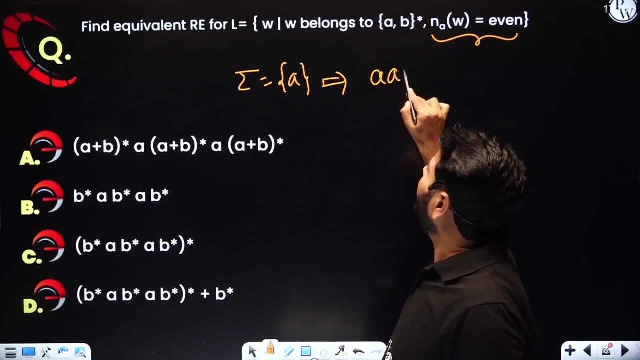 now look at all the options. think about what each one is doing. now. your focus on number of a's is even right. suppose sigma is only over a instead of a comma b. answer is straight away that even write w a whole- sorry, whole star, w a whole star, but here b is there a comma b, right? so now? 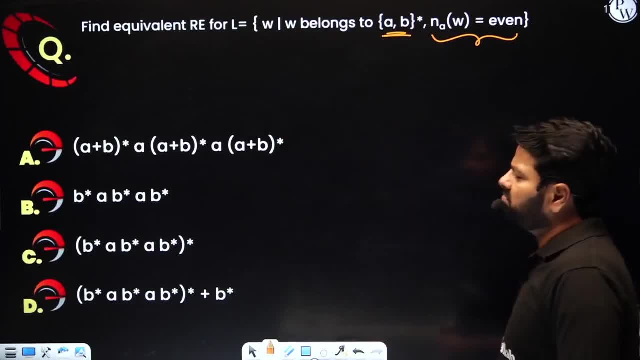 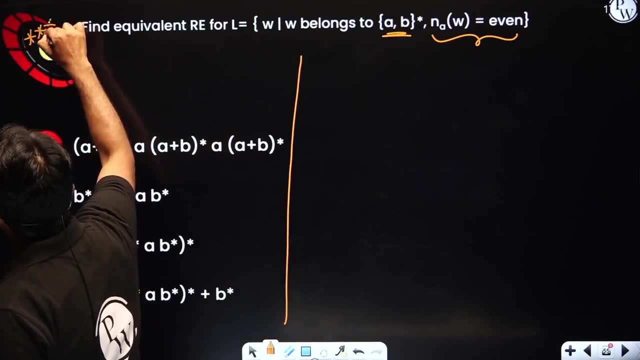 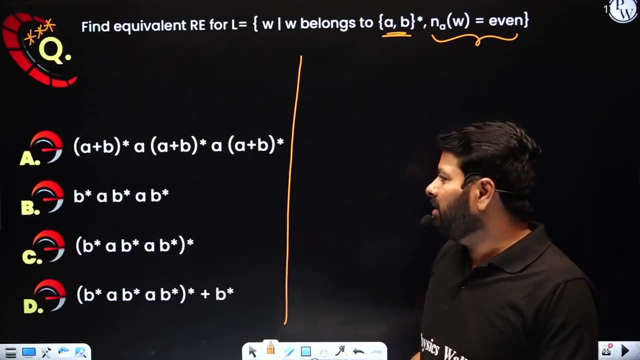 you should think some other way now what way it can solve. multiple answers are there and no doubt it is important for exam and asked multiple times so far. why? because very easy to confuse you with a lot of variations. okay, first i'll explain which are not correct so that you can conclude what is. 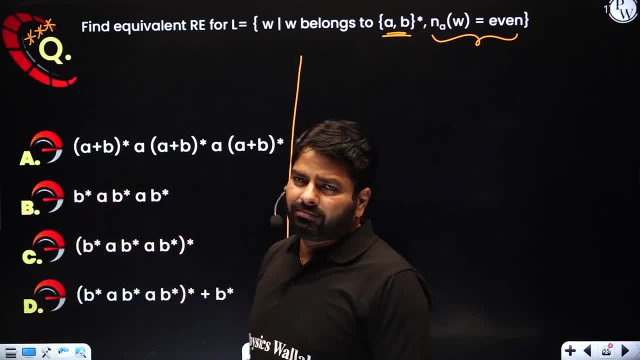 left at the end why this option is not correct. you just think about it. first, is number of aces even, and where is the condition here? one a, here second a and third a. i can generate from anywhere. that means three a's. also i can generate from here, right, one a, a, a remaining, i put epsilon, so this: 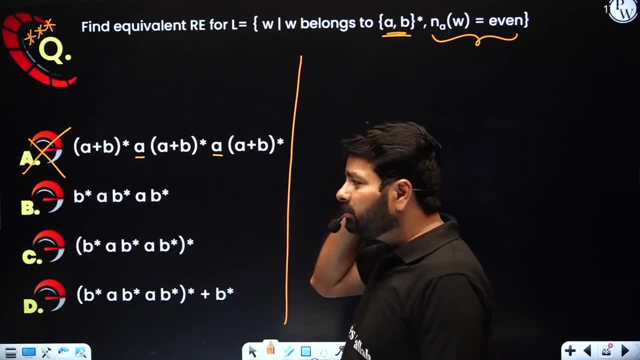 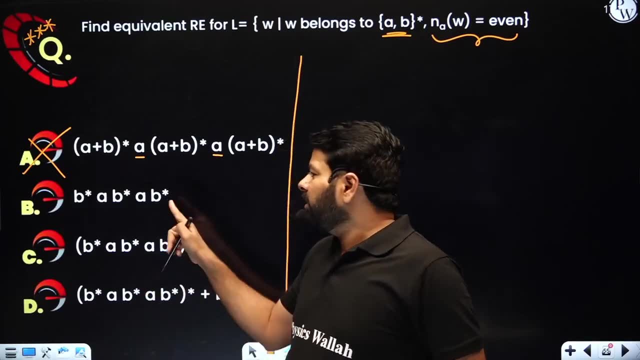 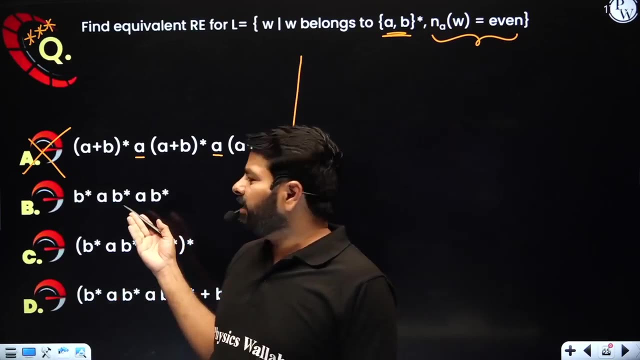 definitely wrong. it cannot guarantee even number of a's. maybe it will generate all possible, all even yes, but also it will generate- not even yes to this one- exactly two a's. my question is not about exactly two a's, it's exactly even yes. so this will generate exactly two a's. what is this? how do you write? 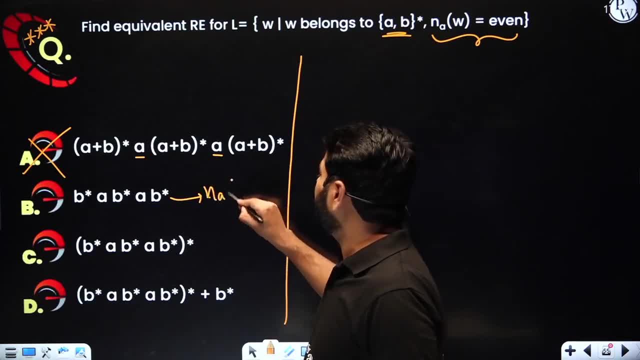 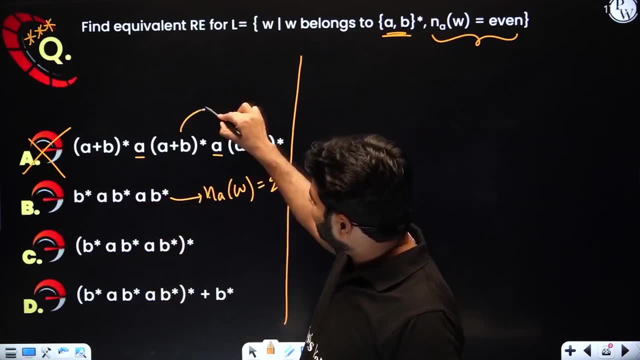 condition here, instead of even if you have equal to two, definitely this could be the right answer. then what is this, sir? what is the right answer for this? i have two a's and remaining places. anything is there. this will guarantee number of a's will be at least two. look at that. the question is if it is. 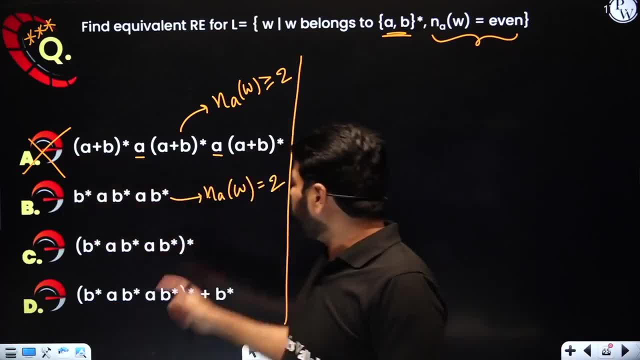 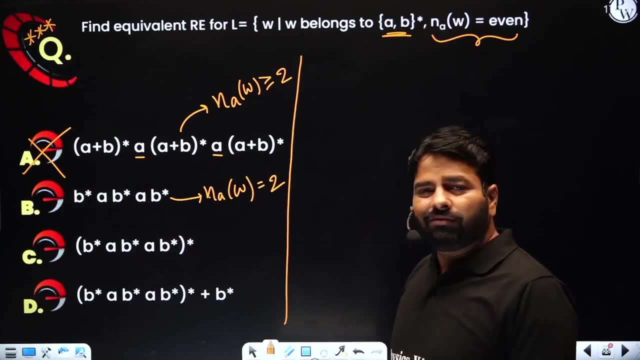 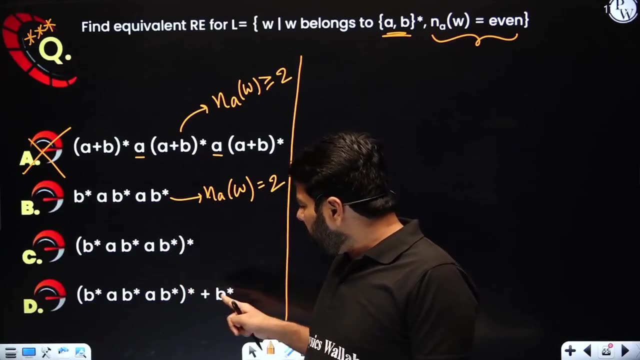 greater than or equal to, you should choose option a. if the number of a is equal to, then you should choose option b. what is option c options is somewhat difficult to say why. because the option c and d: almost same, but here only b's you can generate. in this option d there are only b's you. 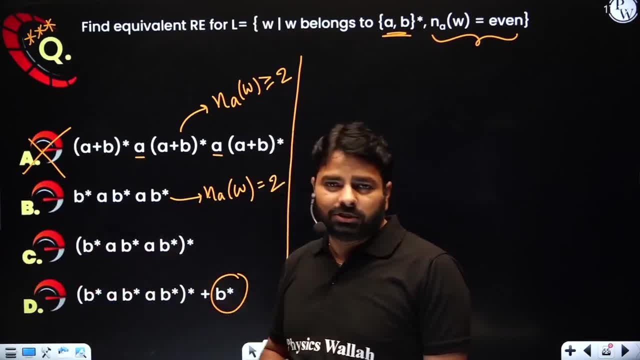 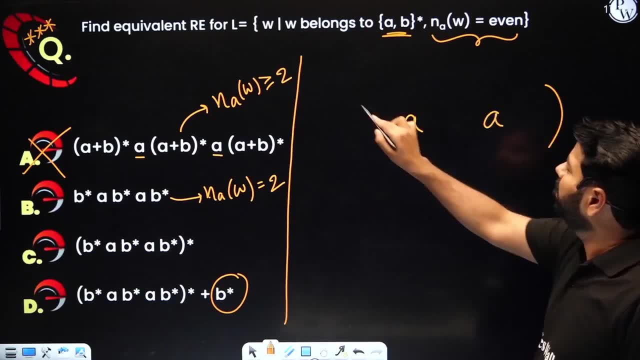 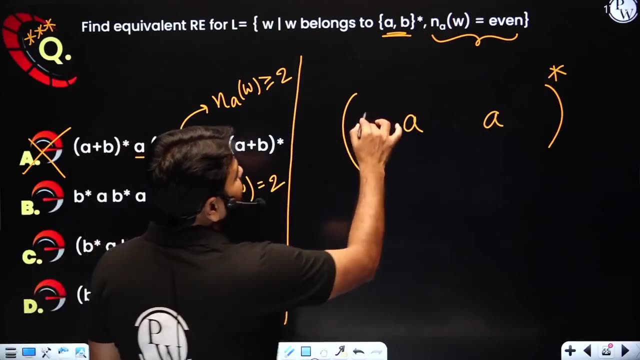 can't generate because if you go inside, when you take a b, a also comes. so in between these two, whenever you want, s is even definitely double. a whole star could generate even yes, but b's can come any point of time. this can come here. any number of b's, this can come here. 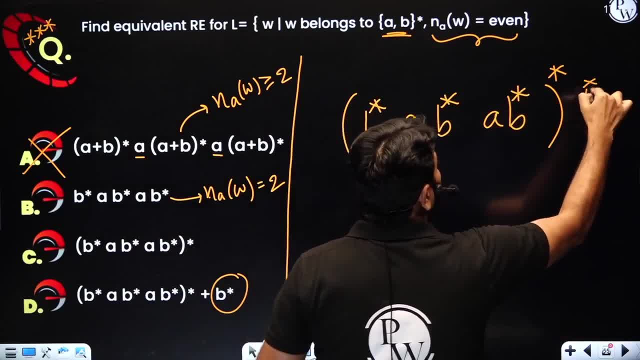 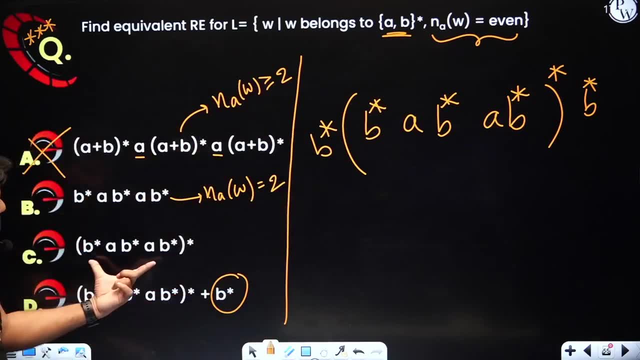 b's can come here, but that's not enough. b's can come here also, or here also the actual answer for the question. but this is not given anywhere. and look at this: here only b's you can't generate because zero number of a's also right answer, but here epsilon you can generate, here what is not. 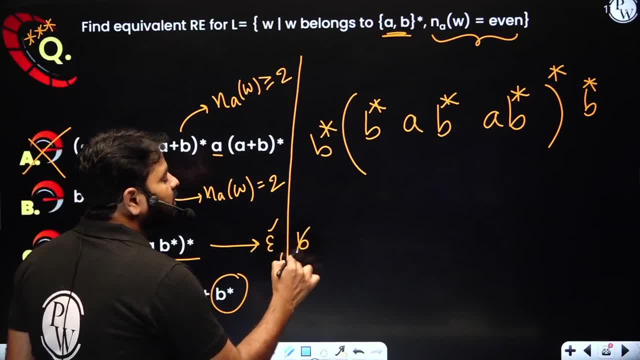 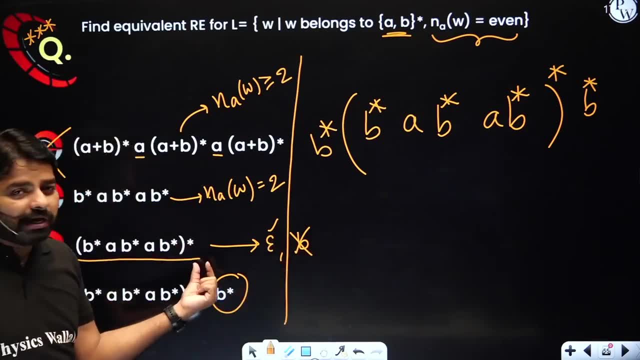 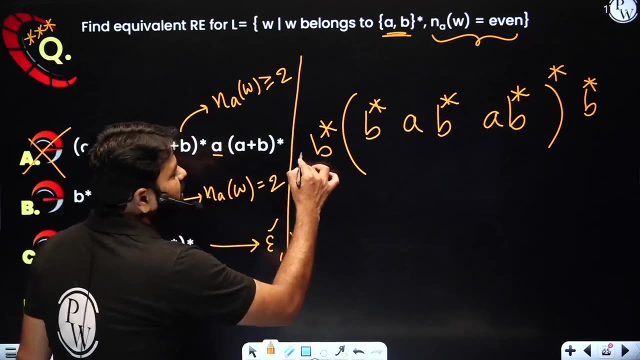 possible. epsilon okay, but b you can't generate. but b is having even number of a's, zero a's means even right, but here impossible. so to cover up that you need additional b star, or keep the b star here or here. answer will be sufficient. so you can choose this answer or you can choose. 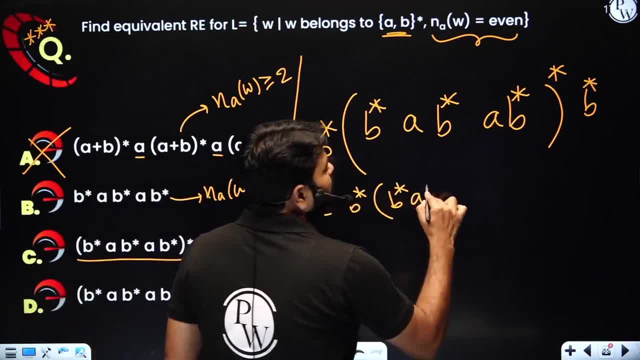 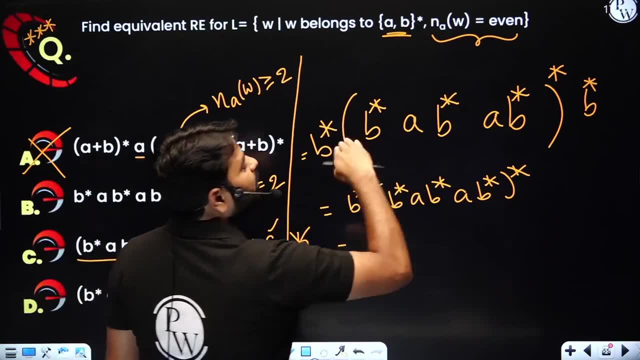 only b star here and you can try as homework. you don't need these two b stars. you can keep only one, that's fine, or you can keep only that b star, that is also fine. that's why this question is very, very important for the exam point of view. 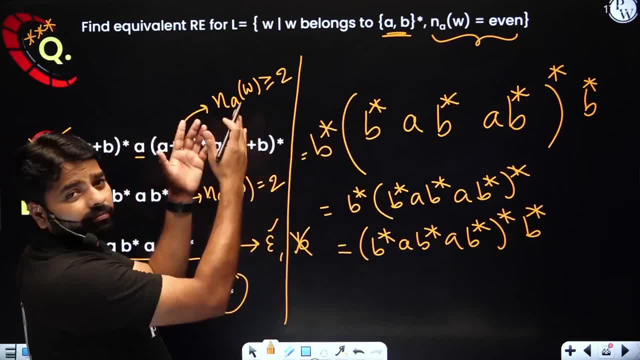 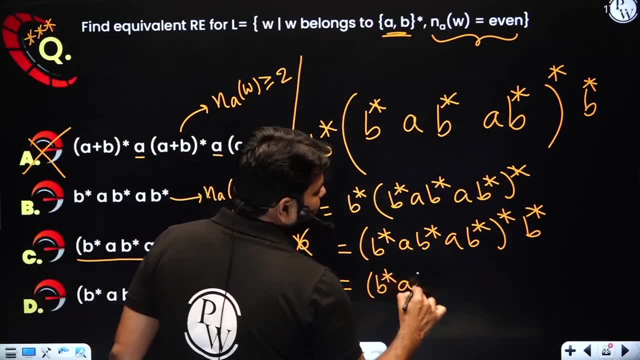 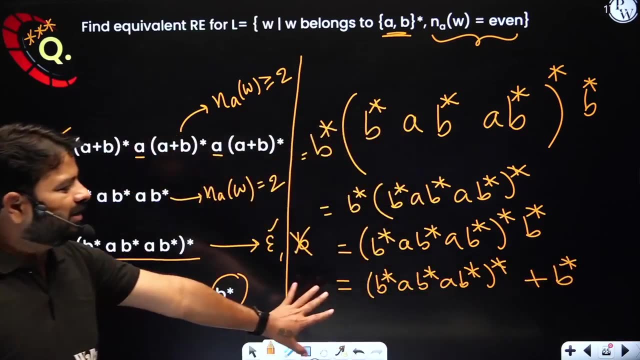 how do you write this many ways to say the same thing? and otherwise, why do you write b star here or there? keep outside also, that would be fine, till the language you get same. additionally, b star. how many other i am not writing here? you know, if i try to discuss this i may take half an hour. 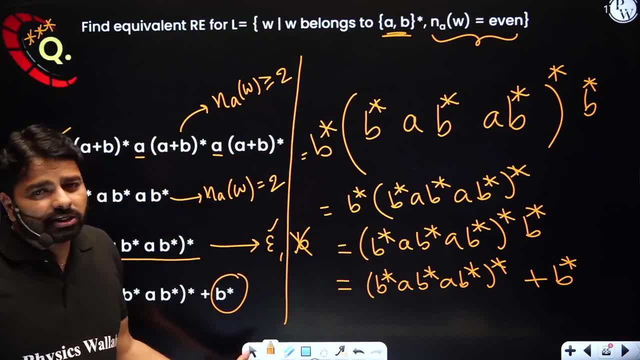 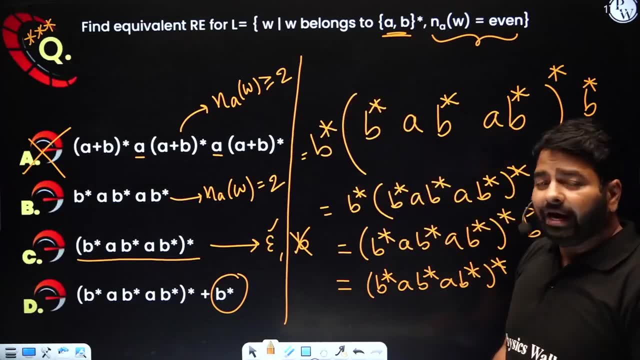 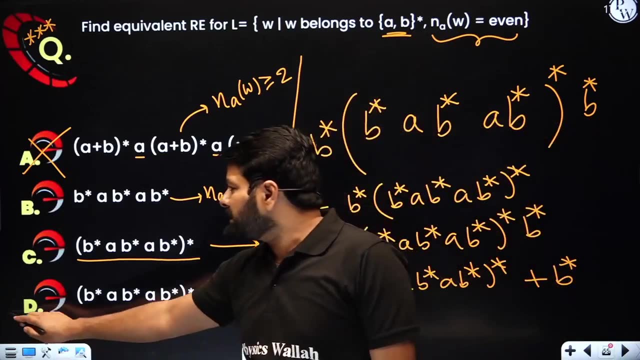 sometimes for the only this problem right as it crash course. so you have to understand why this many expressions are there to say this is a right or right language, or all these expressions are equivalent to this language. okay, so now d is the right answer and b, c. 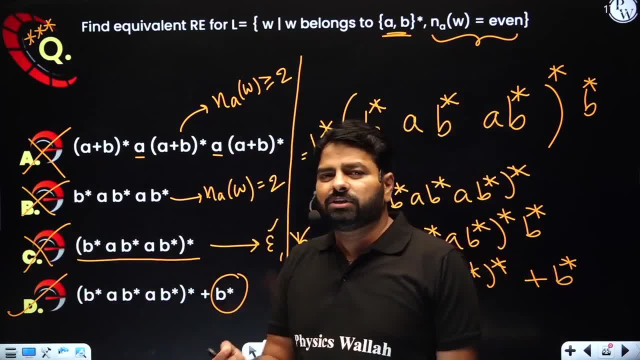 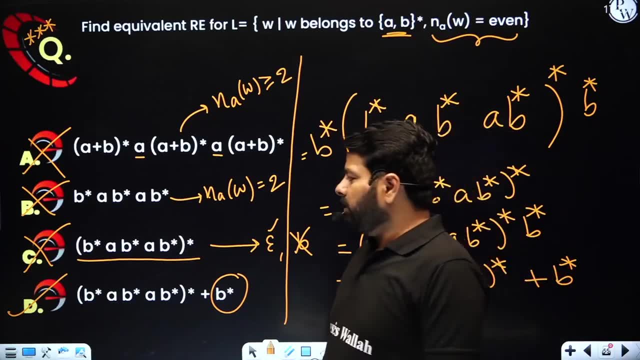 are also wrong. but c is only the one thing which is missing. only b is. i am not able to generate. that is the reason i am going for the option d, right option c is there? option d: none of this is there. you must go to none of this because this can't generate all string. 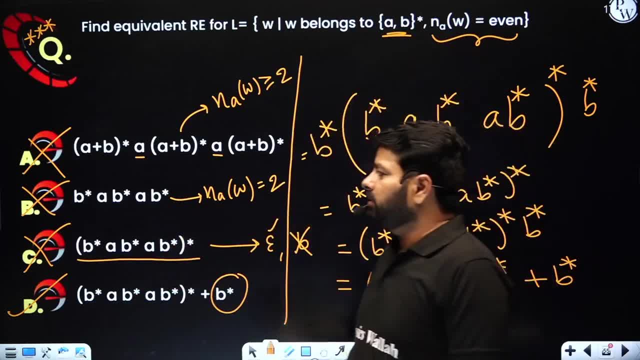 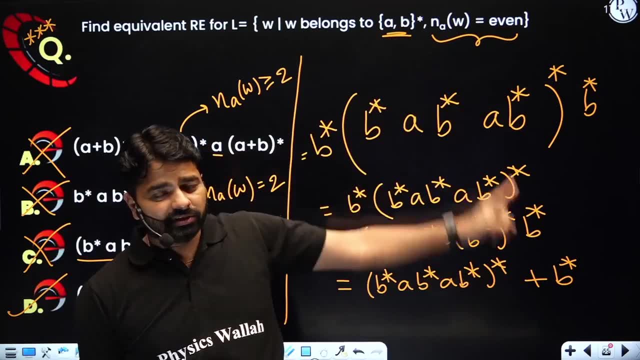 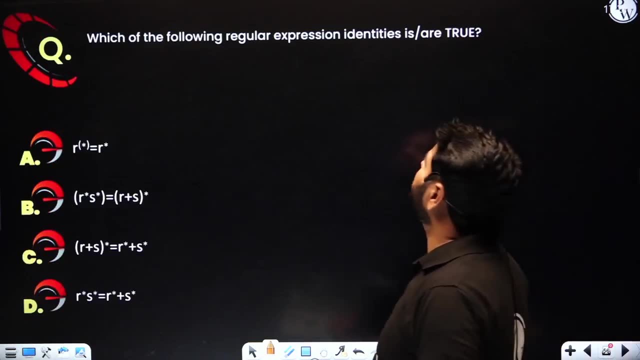 they are having even number of a's. okay, keep this as very important and practice all these expressions- and these are all are same and that is solving the given question only. okay, which of the following regular expression identity is true? it was a p by q and you should. 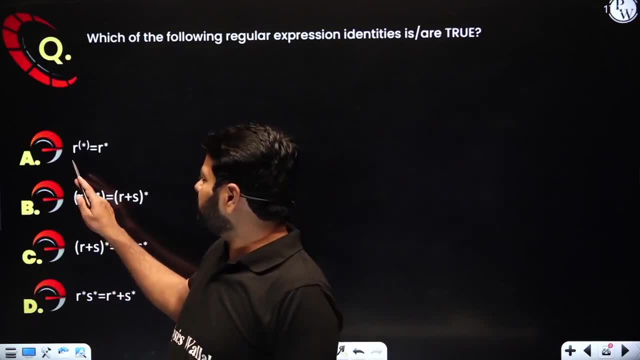 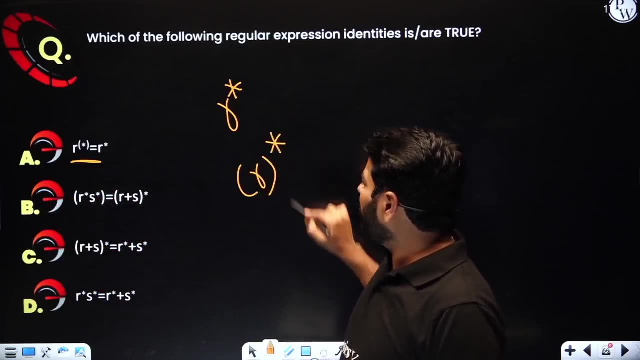 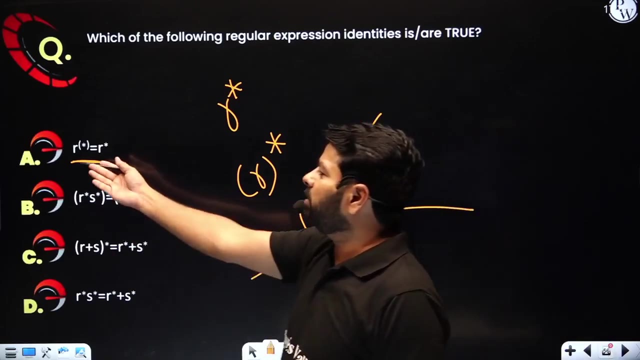 know what is well formed formula. see here, somebody is written some different way: r star, you know, r star, you can write like this: or r star, you can write like this: what is this? r star? it's not well formed at all, so ignore this option. this never be correct, because that's not well formed, as you know. operand. 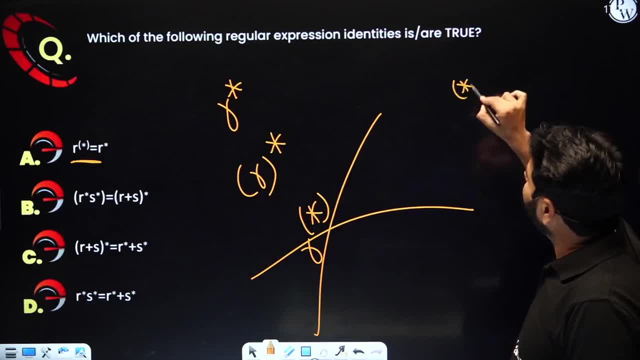 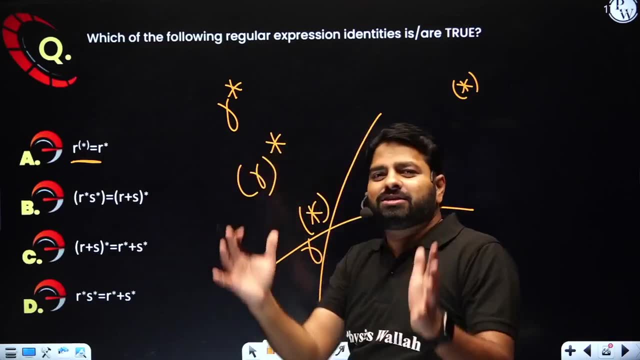 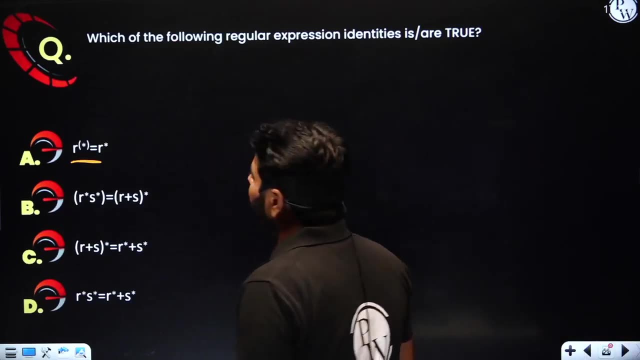 you can take parenthesis, but if you put a star for the operator, then whom you are applying, right. so operator should be applied for operands. when you close this operator, you are not mentioning any operand for it. it's not well formed first thing, so don't think about it. it's always wrong, okay, next. 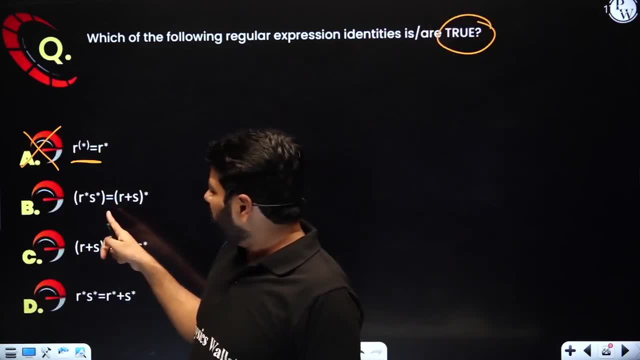 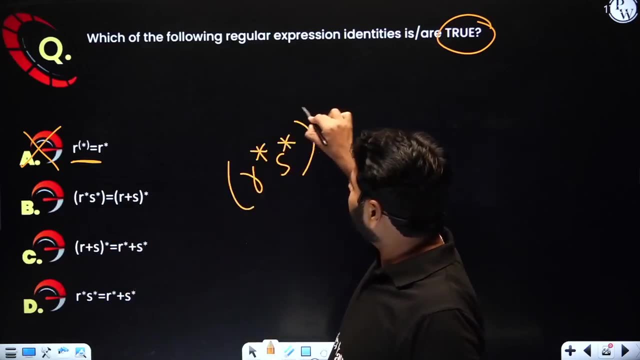 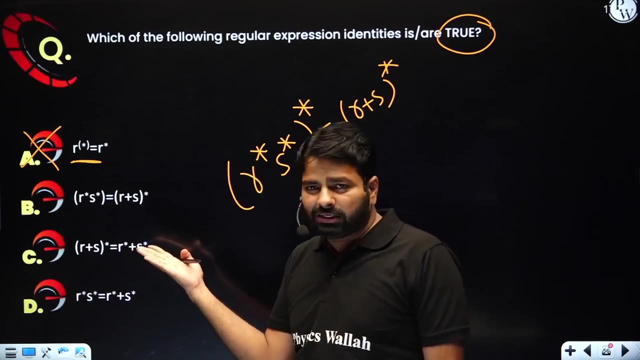 true, we want to choose true right. you already know about it. is this true? as you know, r star, a star, whole star. that is equivalent to. but what is given in the option? we have tried a star b star, right in place of ab we have r. that's it. here, star is missing, and are they? 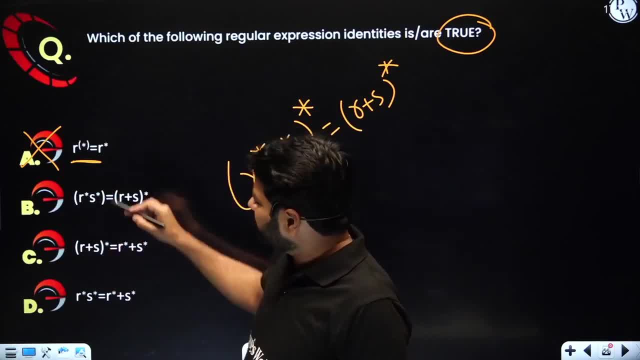 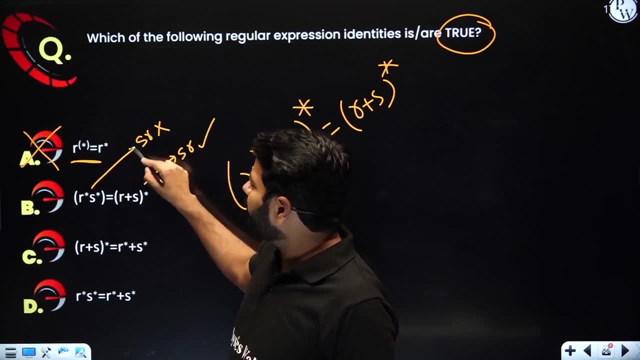 equivalent? no, how do you know that it is not? so what is the problem? we have to do is to you know they are not equivalent. very simple question: from here s? r you can't generate, but from here i can generate s? r. that's all enough. why they are not equivalent? if they are equivalent, 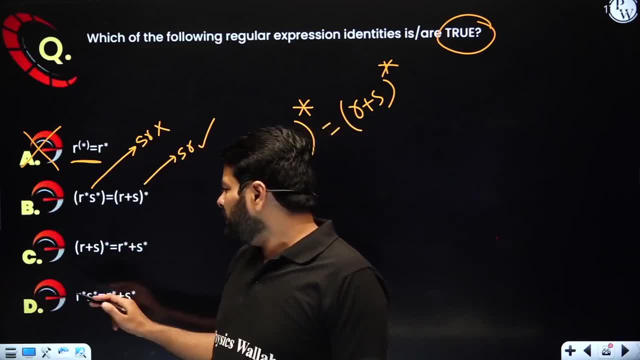 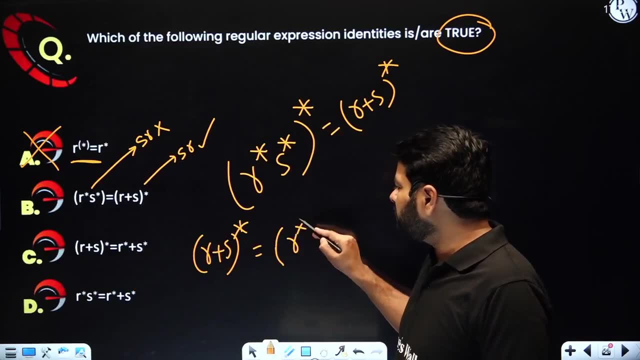 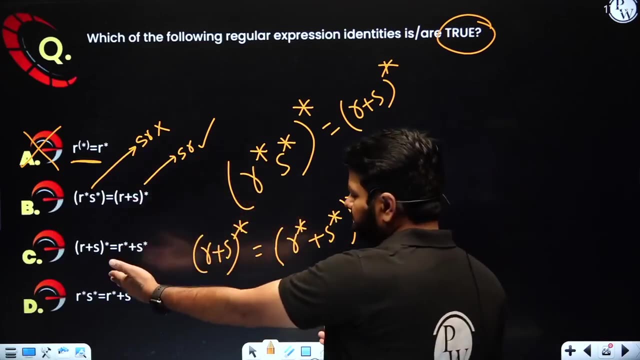 they should generate same set. what about this one? this one r plus s old star, equivalent to: if you have r star plus s star old star, then this two will be equivalent. we have tried in the previous in a previous year, previous questions: a star plus b star, whole star. there was a first option for this. 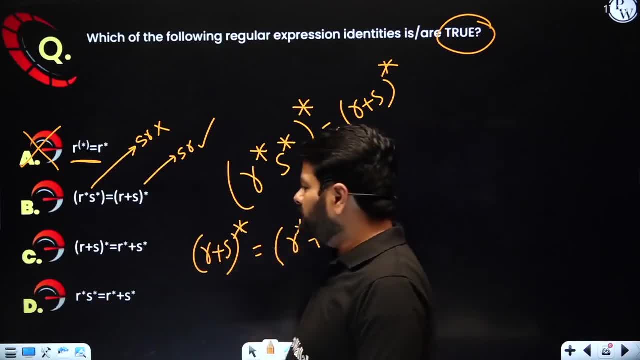 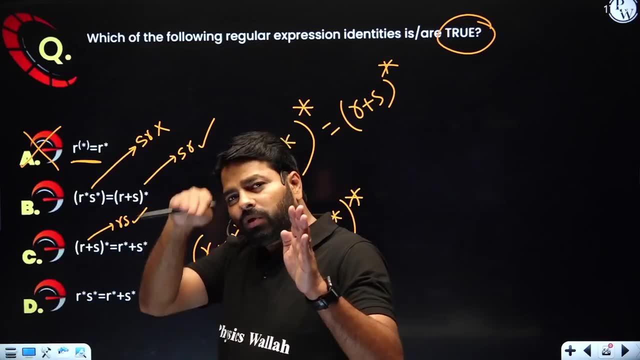 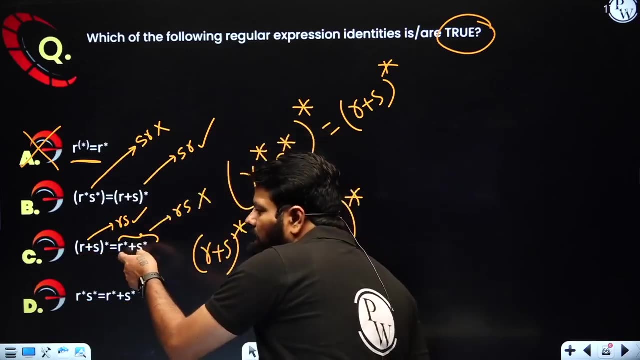 question. right, this was the question. this was the first option. fine, now here what is missing. you can see from here r s i can generate, how i can repeat twice. first time i take r, second time s, but from this r s is not possible, because only r or only s. how can i do r s together? not possible. 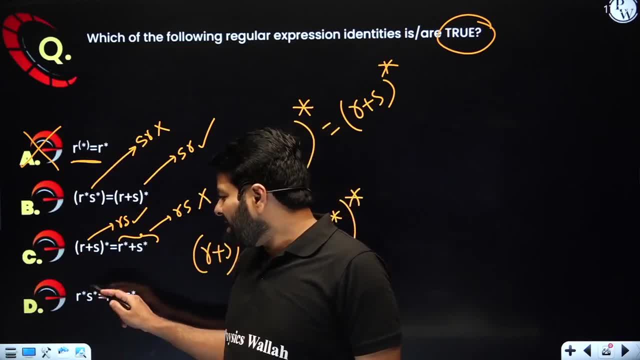 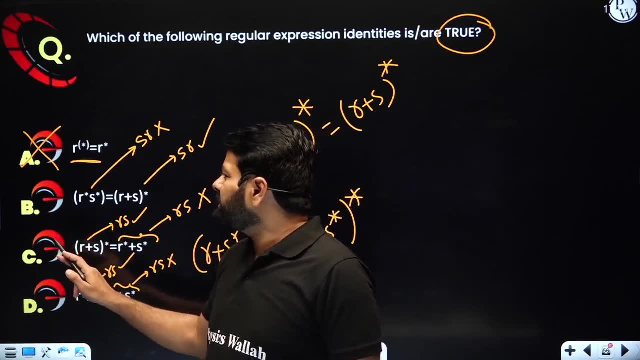 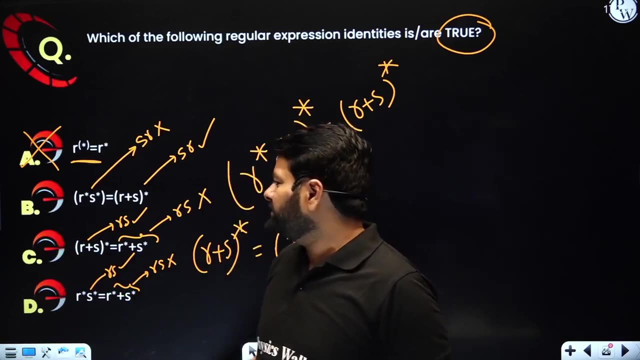 okay, this one is very simple again, here r s you can generate, but here r? s you can't generate. that's why uh, which is equivalent here, you can see right, anybody is true here. no one is true. oh, that's great, all are wrong. there's a. 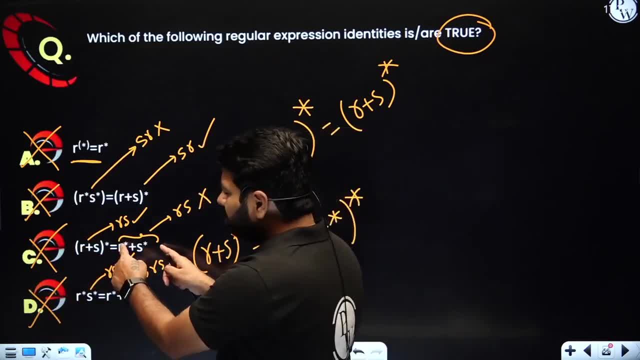 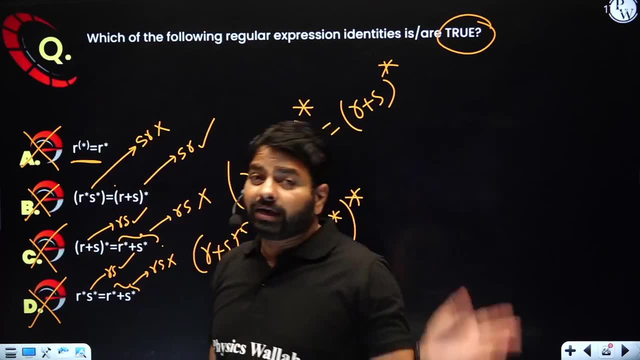 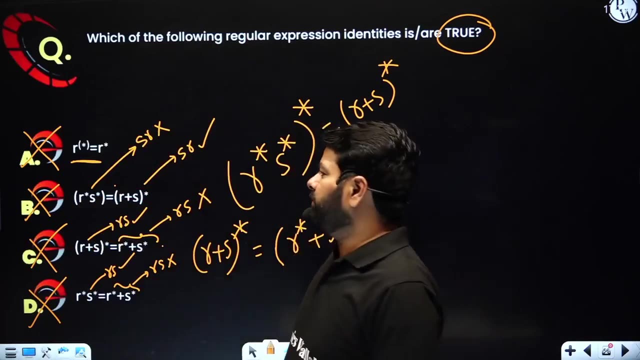 possibility to make it equal when either you put whole star here or you put here already parenthesis there. maybe in the actual gate question you might have a star here. so this could be possible. right answer in the gate question. but here, you know, i slightly change the question. so here all of them are wrong. all of them are wrong. such questions are: 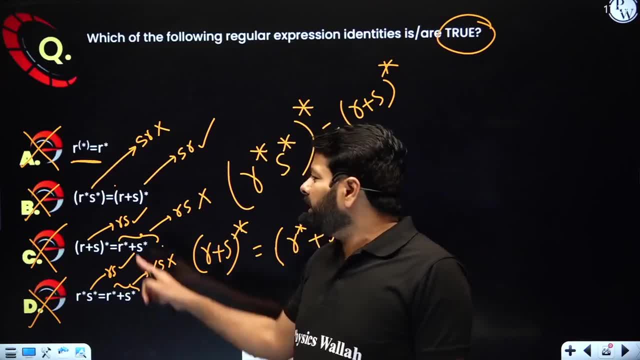 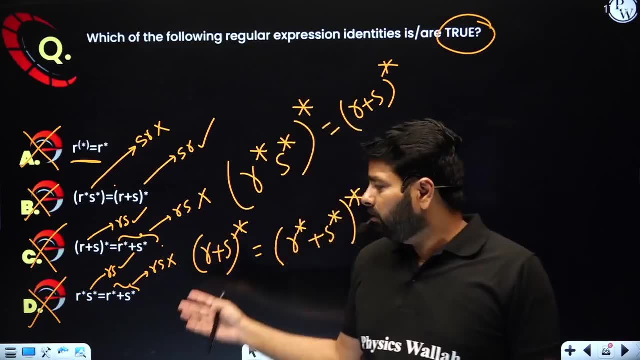 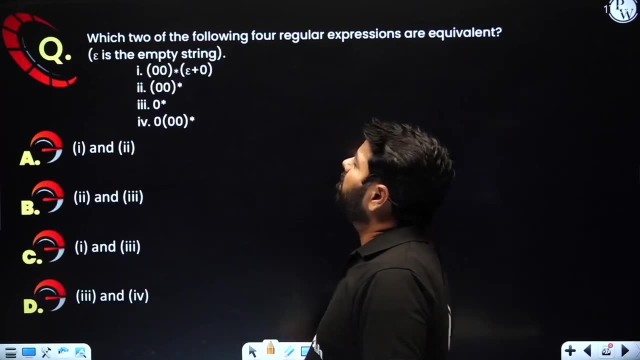 not possible. the exam at least one option should be correct, so in case this one: if it is given whole star, then definitely this option could be correct. okay, try to look at the possibilities. oh, next question: which two of the following four expressions are equivalent? so we have four. 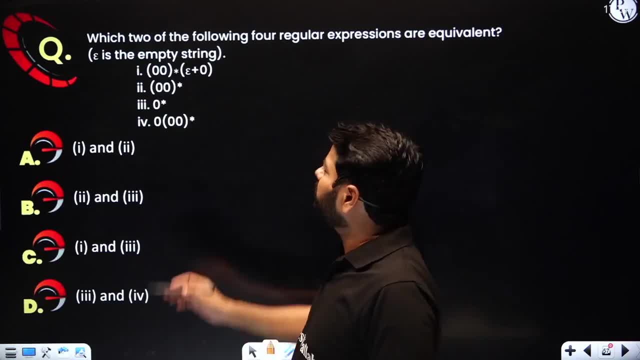 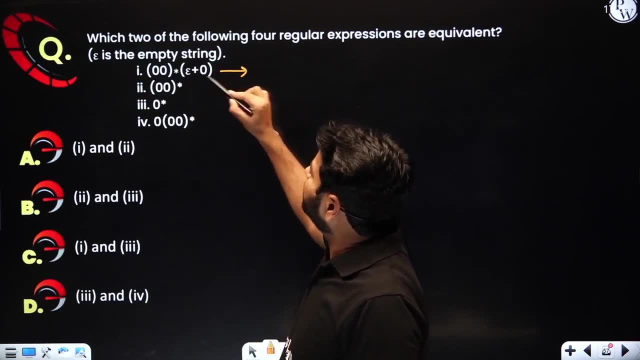 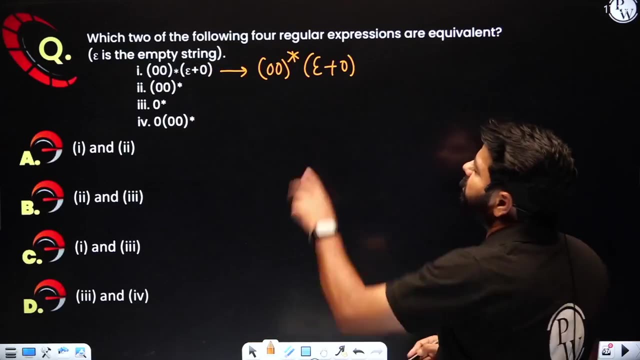 expressions here and which two are equivalent. now for simplicity. let's try to understand very quickly. and what is the meaning of this? okay, just write the star evo, zero, zero, star, epsilon plus zero. can you simplify very quickly? yes, just, you know. distribute it properly: zero, zero, whole star. 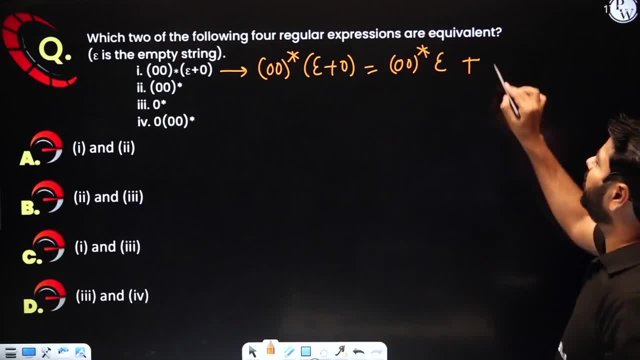 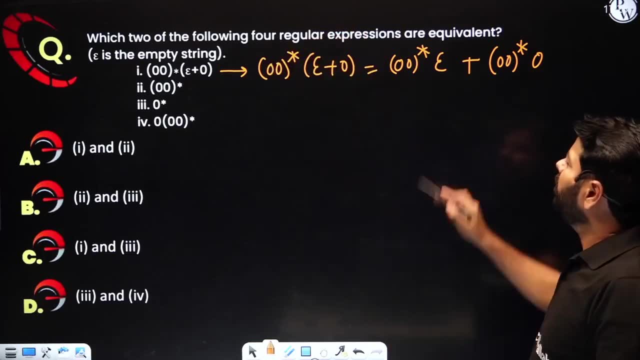 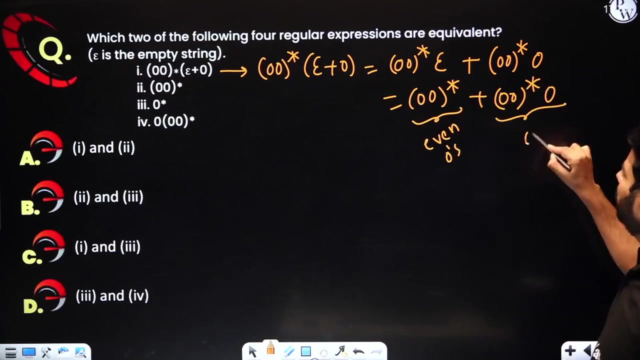 epsilon plus, and then for this you apply zero, zero, whole star. you got distributive right, you applied to now: this one is zero, zero, whole star plus. this one is zero, zero, whole star, zero. these are the very simple things, you know. this is having all even zeros, this is having all odd zeros when you have union. 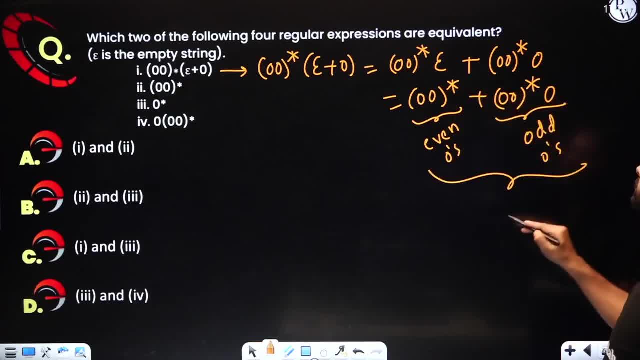 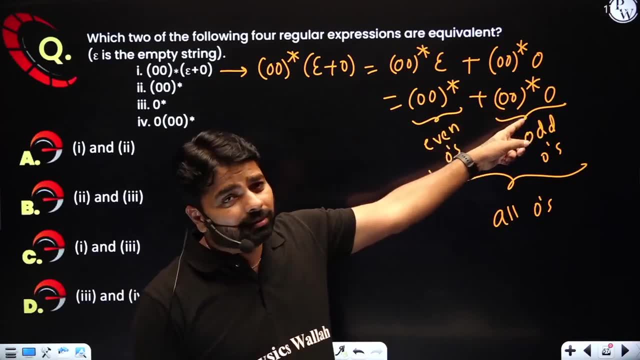 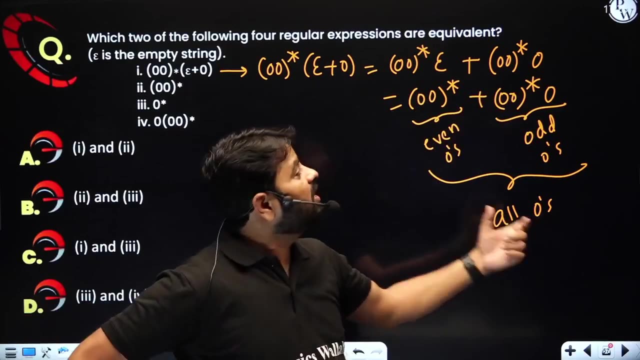 even zeros, union odd zeros, you will get all right. all zeros you have. you did not miss anybody. you want epsilon, you have here. you want zero, you have here. you want double zero, you have here triple zero. four zeros, five zeros, six zeros: you have covered all the strings over the zeros, that's all zeros. 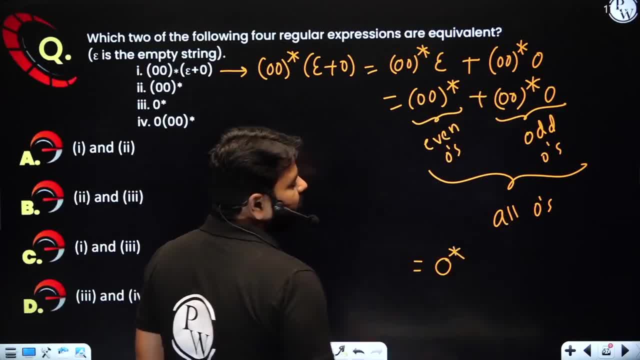 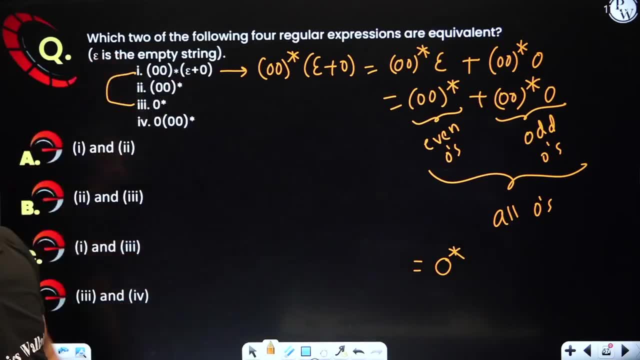 which can be written as equal to zero. star. how beautiful it is. now, when i write this, you got to know that, yes, one and three, definitely equivalent, just classic others. the two is even zeros, four is odd zeros. so one and three. one and three, where is it? this is the right answer, okay. 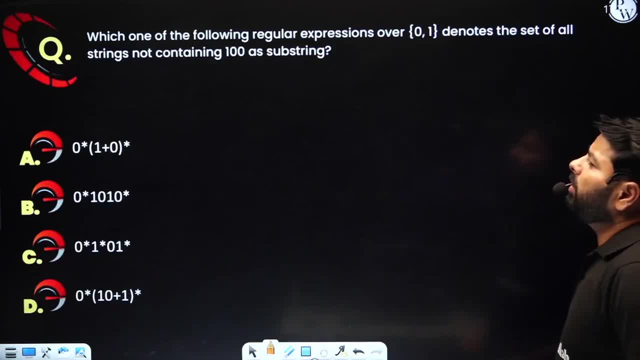 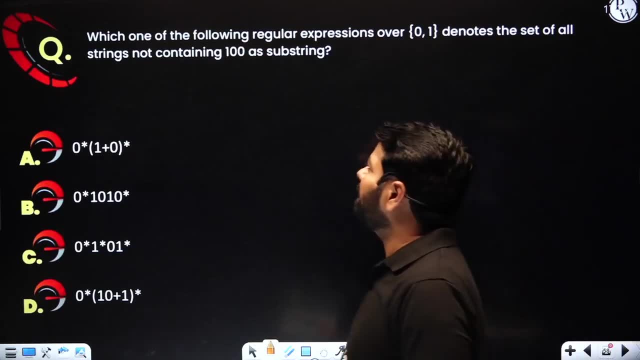 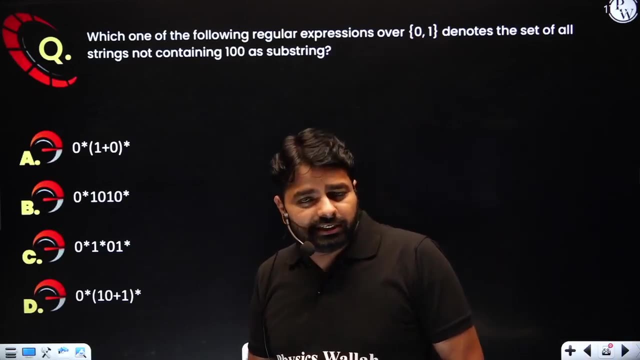 which one of the following regular expressions denote the set of all strings not containing one zero zero as sub string. really, i'm saying directly identifying such questions not easy. okay, i always say truth that, as per my knowledge, whenever it is easy i say easy, whenever it's difficult i try to. 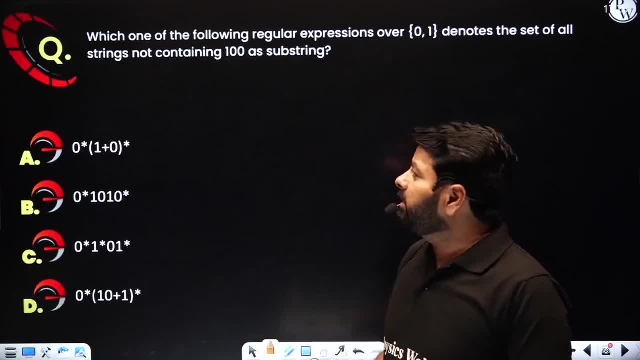 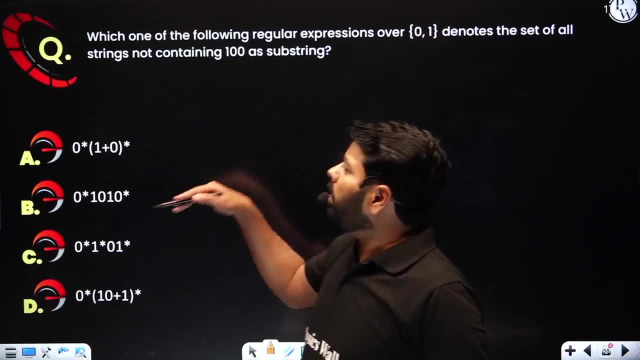 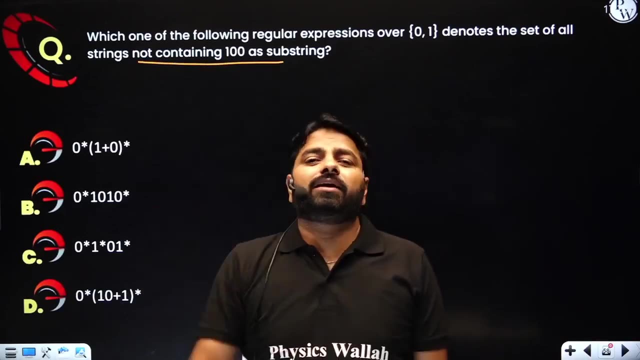 say it because you can challenge yourself to learn much. this kind of questions might not be easy, but it might waste our time, so you should have well strategy to practice. why it's not? you know easy to answer because not containing one zero zero is different from containing one zero zero containing. 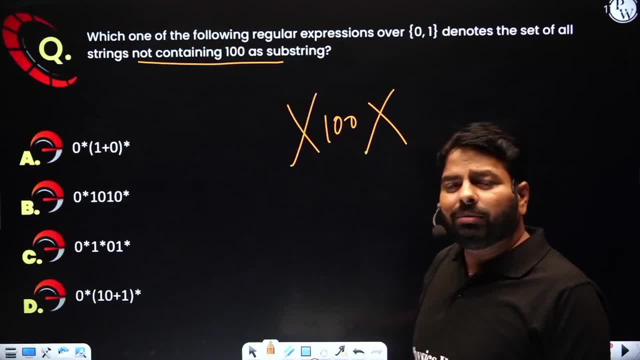 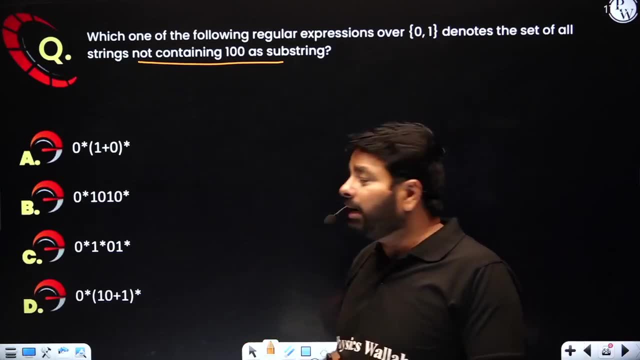 one zero zero. you can say one zero zero before, after anything, one plus zero star before, after. that would be fine. when i say not containing one zero zero, you can practice a lot how to write that expression. or you try to eliminate from the options that would be sufficient always. 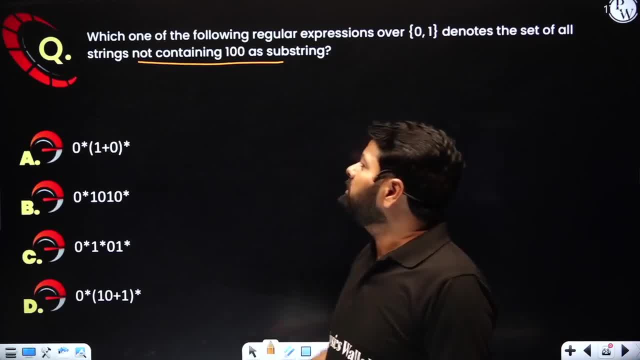 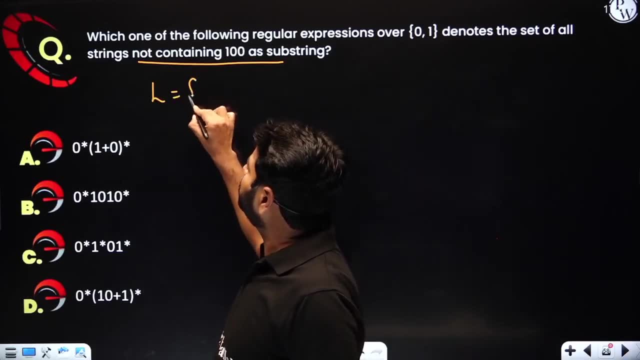 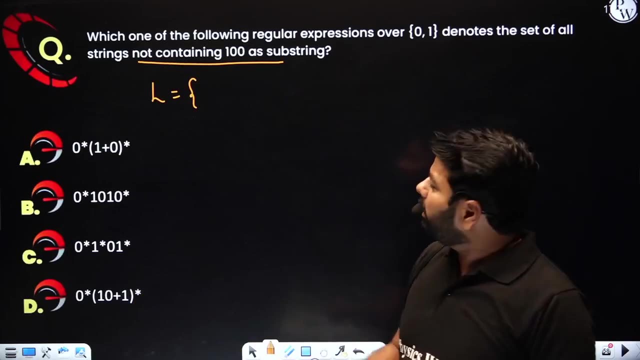 choose in the regular expressions elimination technique. so now let's try. what is the question in the language? not containing one zero zero means who? whoever not contains one zero zero. that should be there in the language. let's say epsilon. is it containing one zero zero? no, that is a valid string. 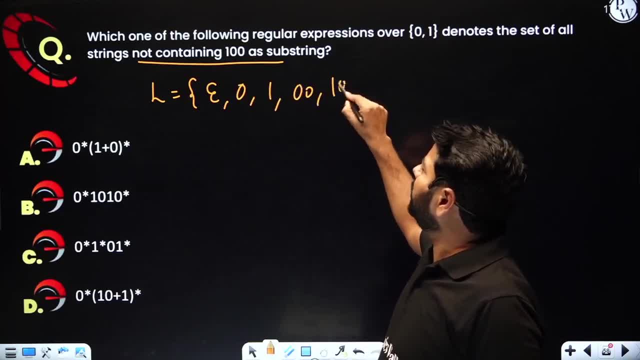 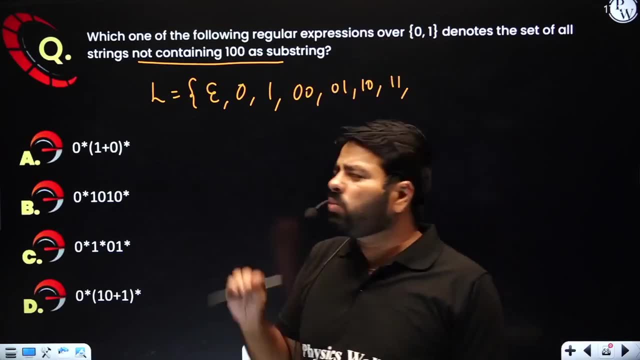 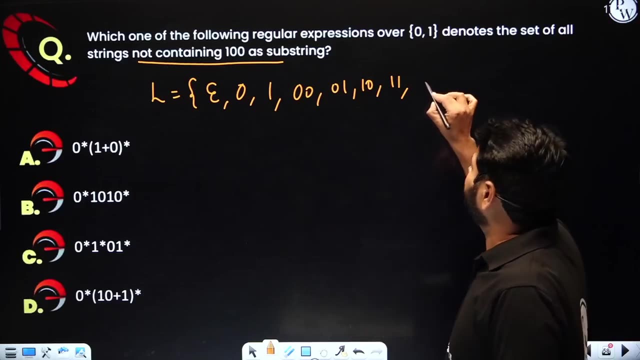 zero. one zero, zero. up to two length. everybody will not have yes or no. up to here there is no one zero, zero, no problem. but after that, whenever you see one zero, zero as a part of the string, should not be there triple zero. known it right. just try to understand what. 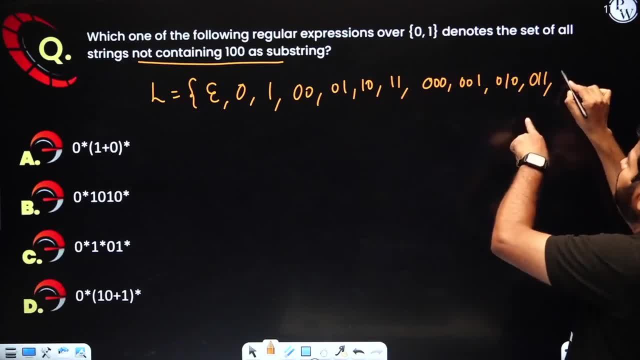 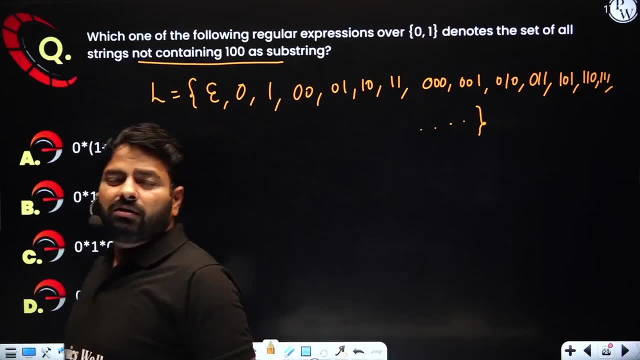 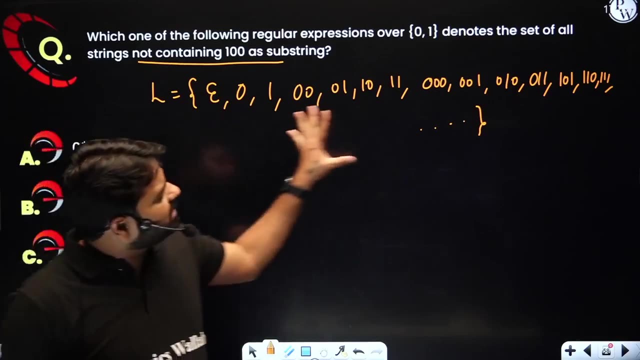 i'm saying right, a one zero, zero. you should not write so: one zero, one, one, one zero, one one, one, and so on in four length. never try to have a string one zero, zero as a substring. if any string has one zero, zero, don't keep in the language now. all the strings will never have one zero, zero, right. 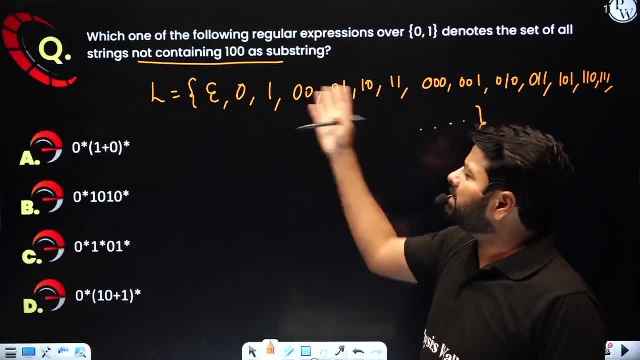 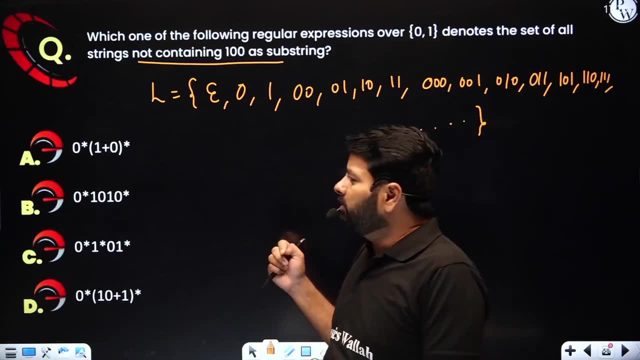 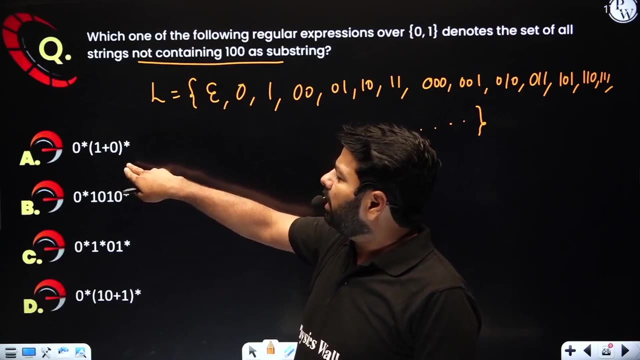 now come to the options. you don't need all this just for explanation, for understanding the problem. i keep on writing it, but actually it can be answered within a minute, sometimes even with few seconds also, you can answer it. okay, let me explain my way. option a: is it not containing one zero, zero? sometimes you need to think two ways. 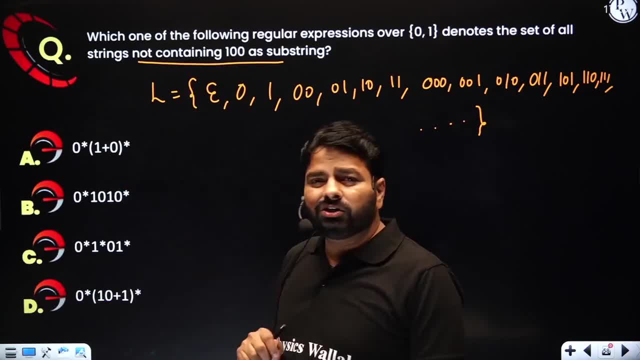 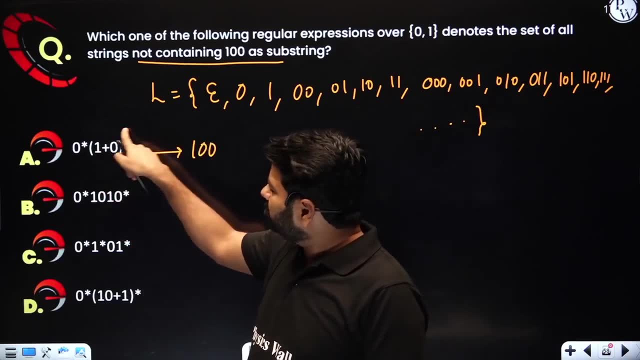 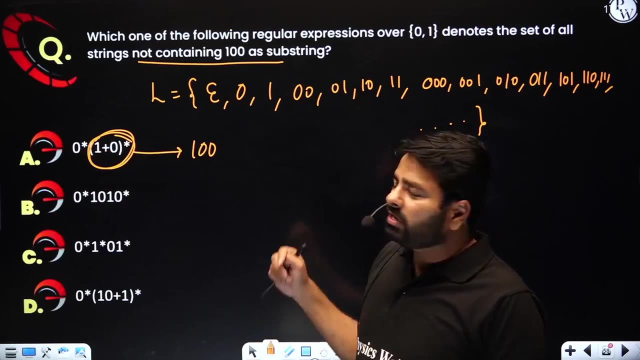 is it containing one zero zero, eliminate. is it containing one zero zero, eliminate it. one zero zero. see, here do you have a one zero zero, right? one zero zero. you can have it right this, everything is possible here, right, everything is possible. so one zero zero here. but we don't. 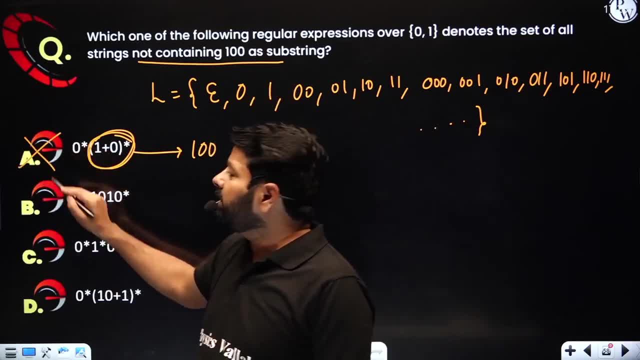 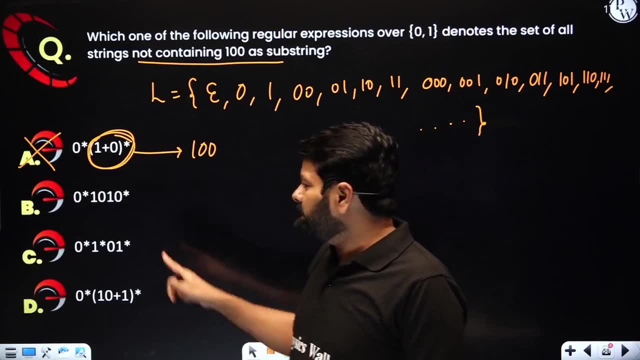 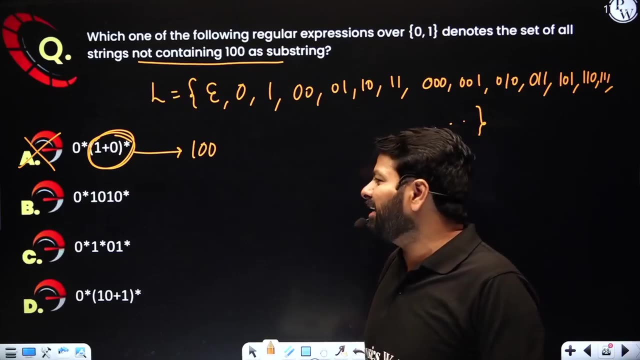 want it, we don't want it, so option: eliminated. see, this is what i am saying. you apply the elimination technique when you are not able to interpret directly. now look at this. is it containing every string? who is not having one zero zero? see, there are two ways to think about. definitely, you look at it. there is no one zero zero. there is. 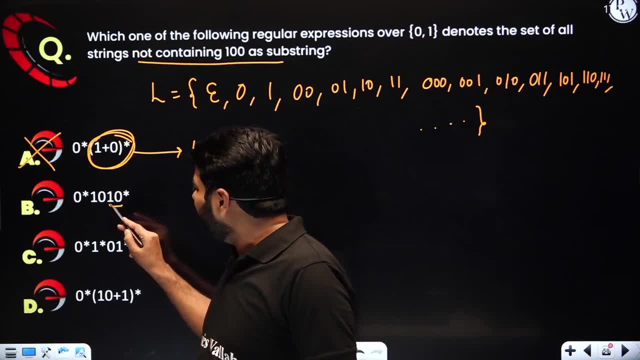 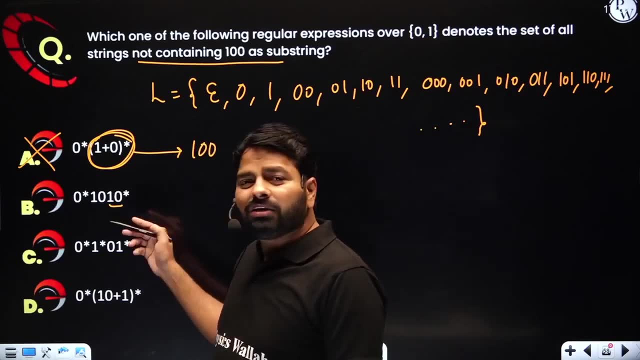 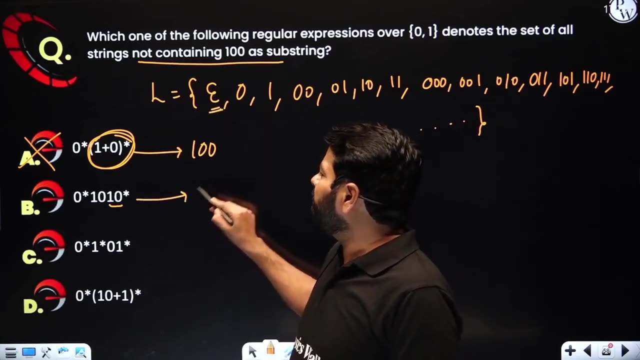 no one zero zero, you have it right. oh here, one zero zero, one zero zero. okay, let me come to this later. you have one zero zero, right? definitely it is a wrong sprinkle, but no need to think about that way. see, my language is epsilon. this is not giving epsilon enough right. sometimes you look at your 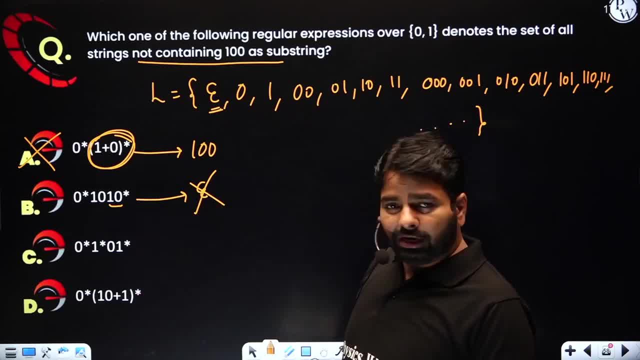 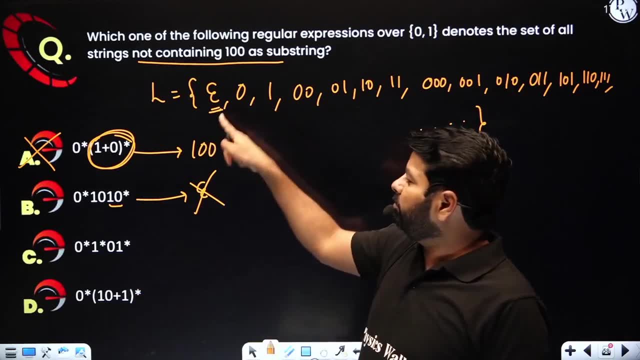 whatever i have, i should have from the options to say they are equivalent. now epsilon is there in my language and the option also should generate the whatever i have. epsilon i have, but option is not having epsilon, so delete it. that's one way. another way: one: zero, zero it's. 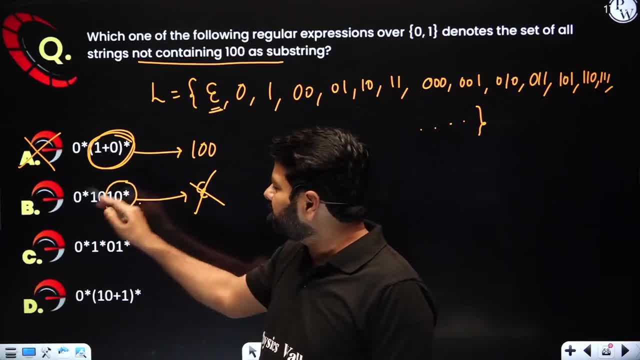 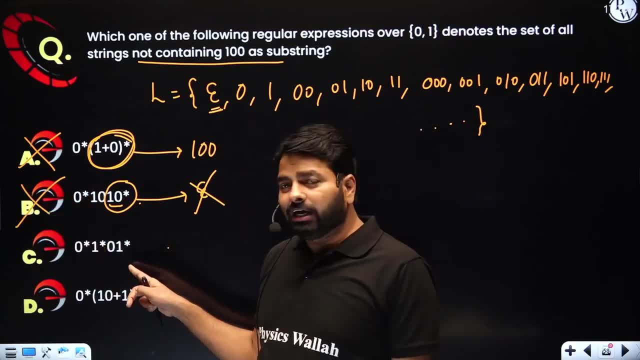 generating. but i don't want it here. see one zero zero. it's generating here. okay, next option b is deleted. option c: here. when you look at- actually i was trying to explain b, but now i'll explain definitely, when you look at here: 1 0, 0, impossible. that doesn't mean that both are same. 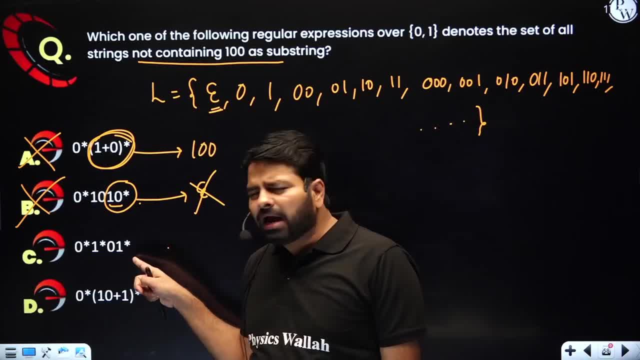 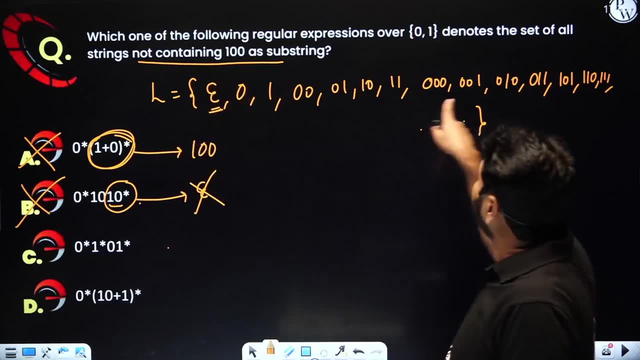 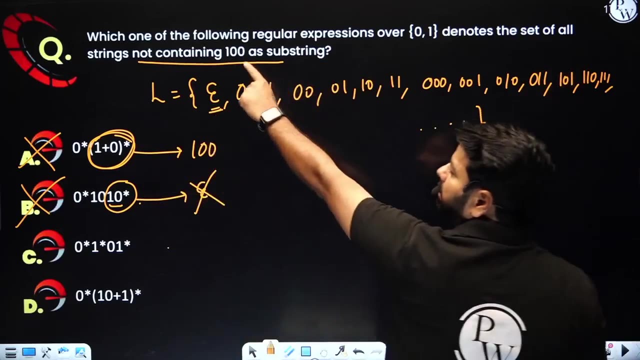 right, i'm trying. i'm trying to say again: it will never have one jio jio. but it is not equivalent to the given question, it is subset. but i want all the strings, not just few strings here. what i'm trying to say, i want every string in the world who is not having 1 jio jio? is that clear? but this: 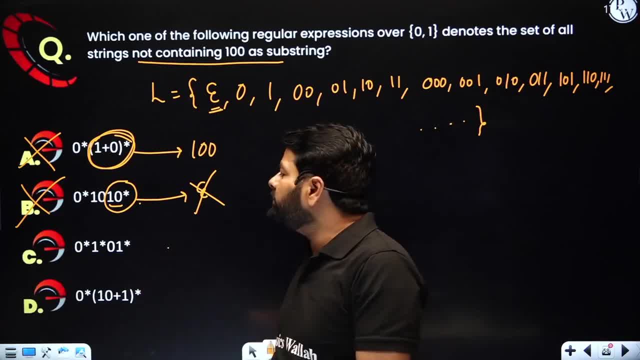 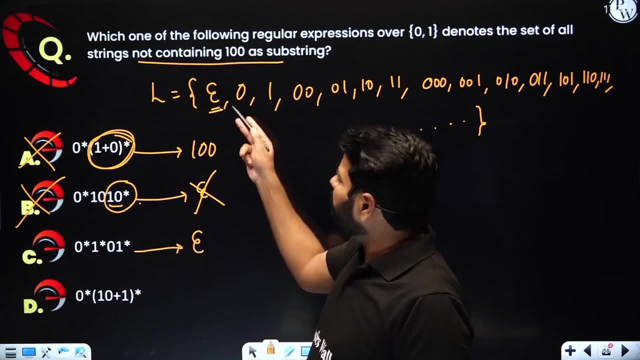 is not giving Entre 하나. giving all the strings is giving only some strings. that is the reason. how do you know that here? just look at our epsilon. I want epsilon, but this is not giving an epsilon, even though it is giving some strings only. it's, it's there. 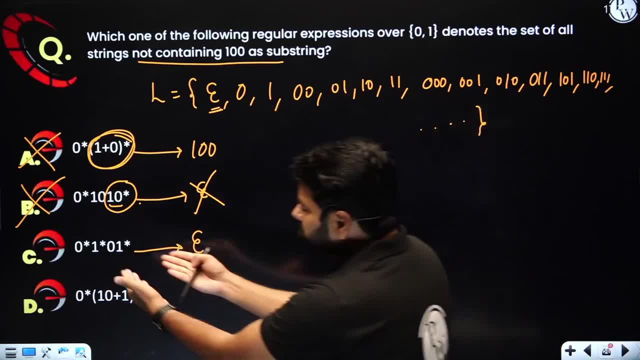 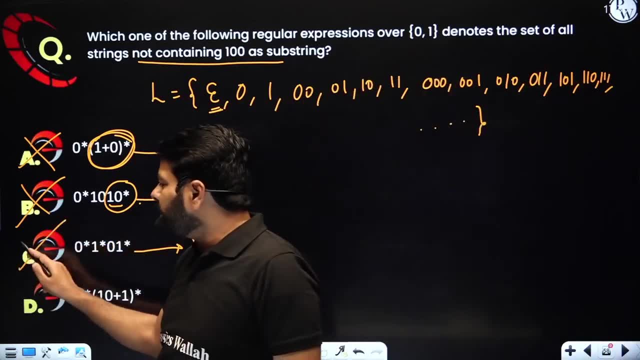 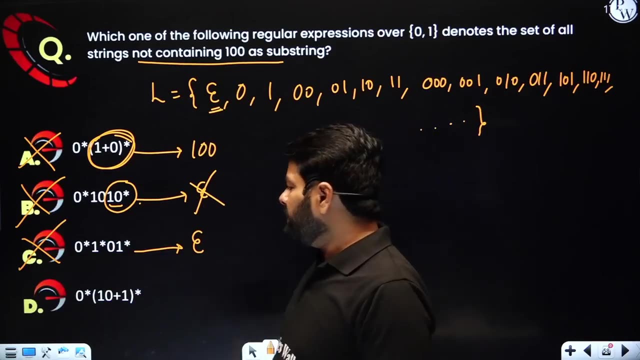 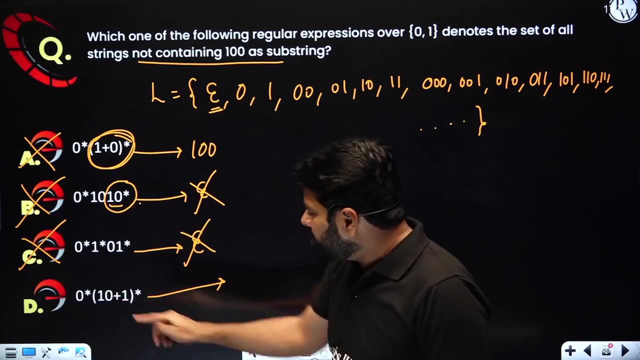 in the language, but not all the strings. okay, all the strings present somewhere here, but I want whole this language, right. so option C eliminated. only the reason is: C is a subset of our language not equal to our language. okay, next option D. now look at, is epsilon was not giving right here? here epsilon possible? 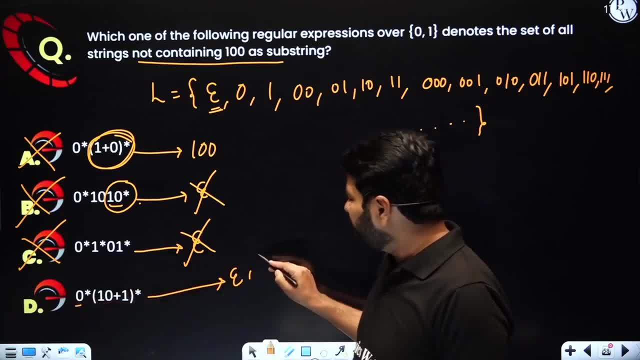 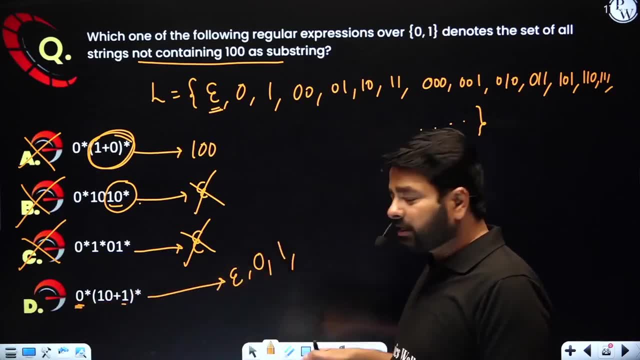 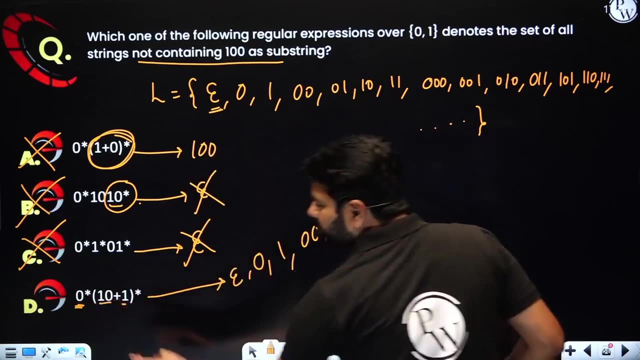 look at that matching next: 0 possible here, 1. possible here: 0, 0. you can take from here itself by putting epsilon second: one: 0, 0, 0, 1, 0 here and 1 here 1, 0. you can generate from here: 1, 0, 1, 1. you can repeat this twice. 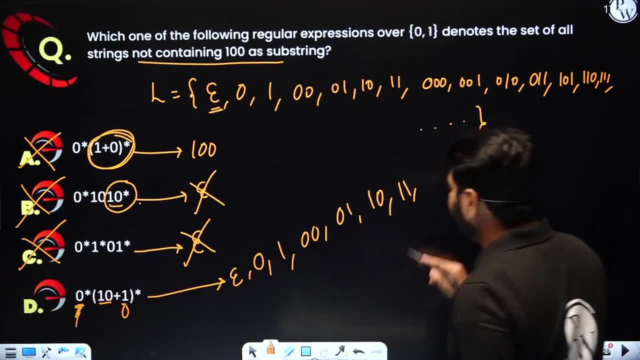 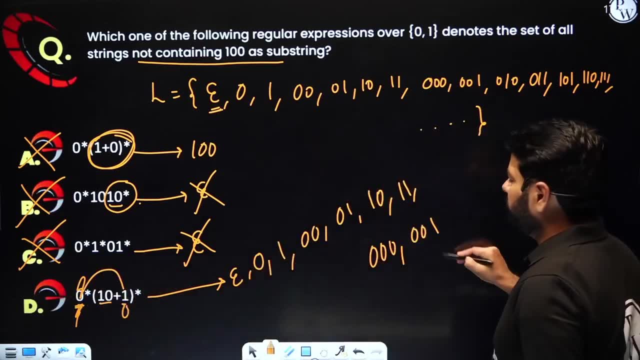 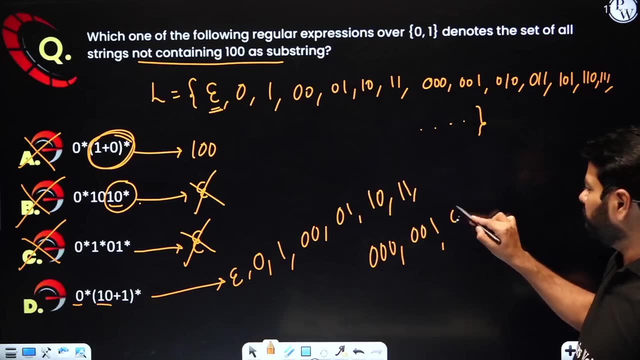 and triple 0 s you can generate triple 0 here itself. look at, are you getting everyone 0, 0 and 1 here? okay, try to understand how to get a string and 0, 1, 0, 0, 1 0 here, 0, 1, 0, and then 0, 1, 1, 1 0 here, and. 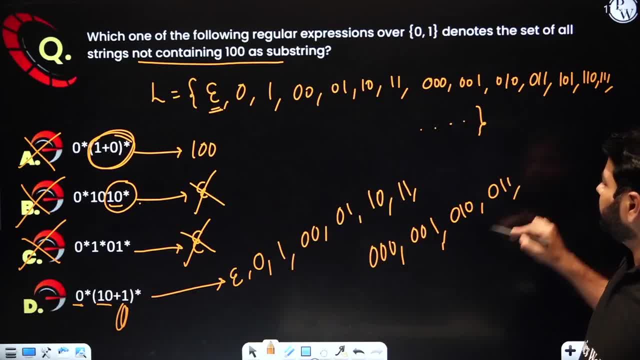 two ones here and similarly one zero one. you have one zero and then one and one one zero. so you have uh one here and then one zero you can get here, and then triple one you can get. but why you don't get one double zero here? you try here. why i'm not getting this one double zero? i? 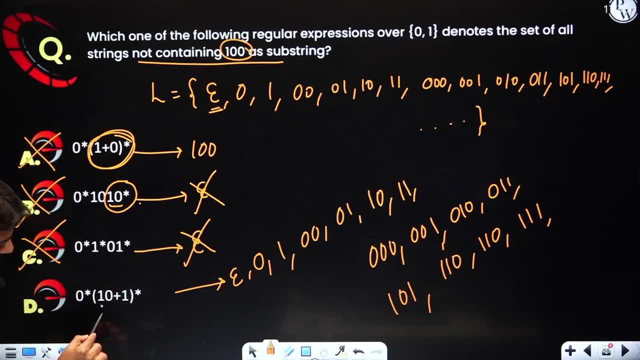 don't want it right. i'm not getting two. see one here if i take zero. other zero impossible here, because you can't come to this if you don't have all star here. if you have all star, you can come back and you can get the zero, but you don't have it once you have one zero, other zero immediately. 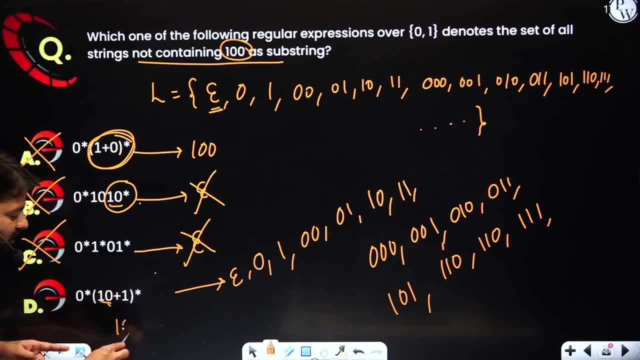 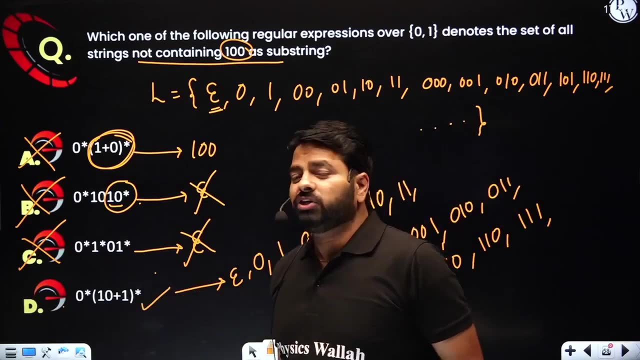 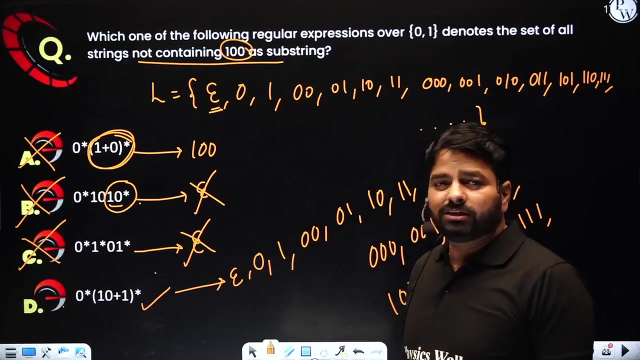 not possible, right, you can come back, but one zero. one zero comes, but not one double zero. so here, except one double zero, except the strings who are having one double zero, all the strings are possible here. so this is a very well known expression for the language, that is, not having one double zero as a substring in every string. okay, 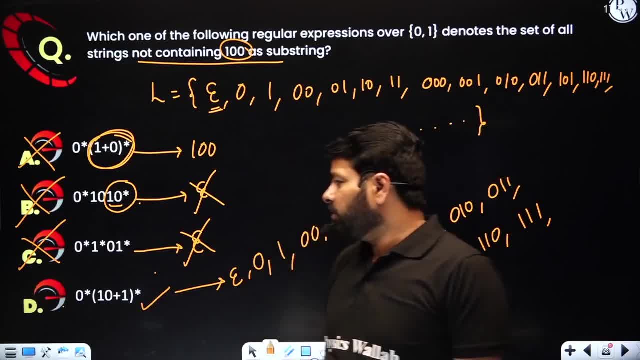 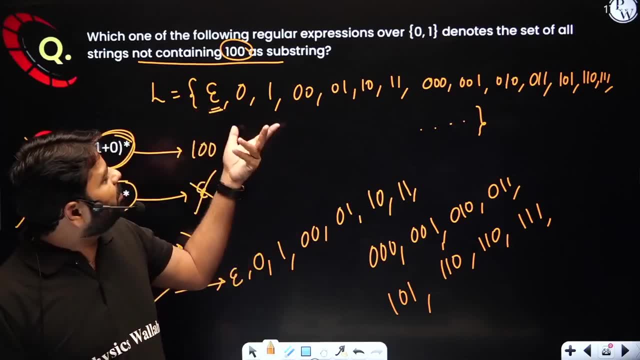 so this is a very well known expression. look at that: when we want to eliminate, definitely you should have the technique. what are the minimum strings? who are present in the language, who are not present in the language? that would be sufficient to eliminate it. maybe i have taken. 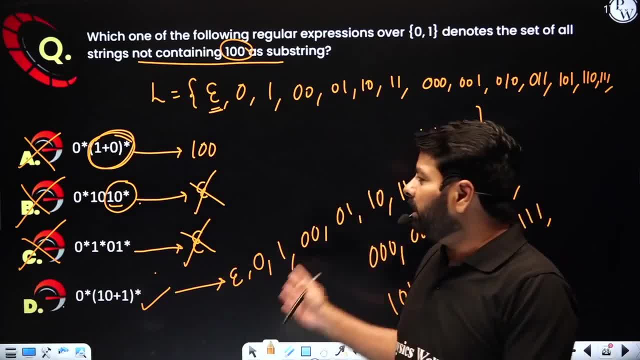 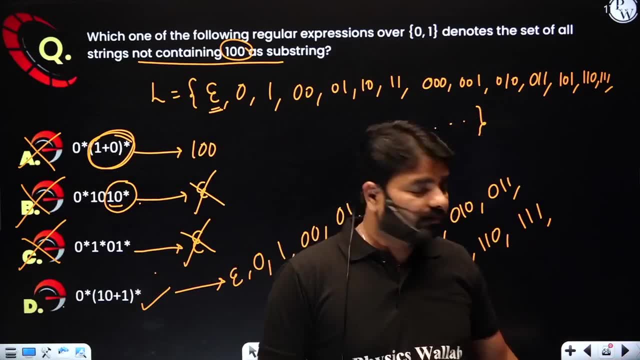 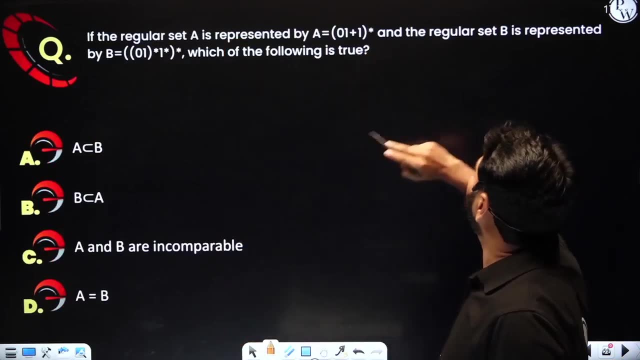 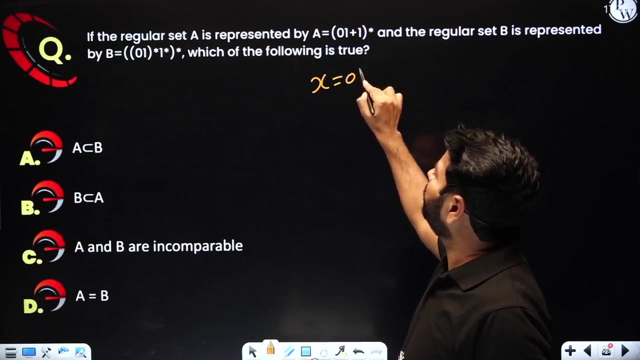 lot of things to make you to understand, but this could be answered within a minute if you know the okay, okay, very easy question. again, if the regular set a is represented by a is equal 0, 1 plus 1 whole star. b is represented 0, 1 whole star, 1 star. it's very simple, like you may assume. just x is 0, 1. 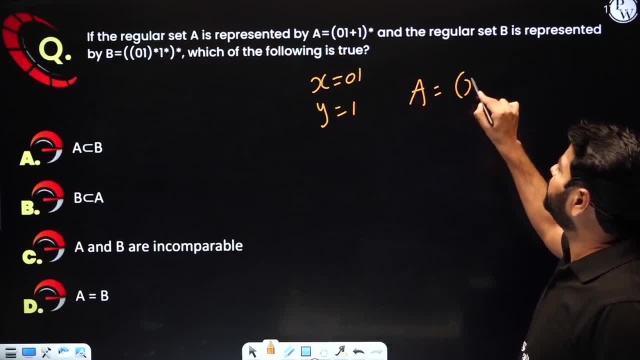 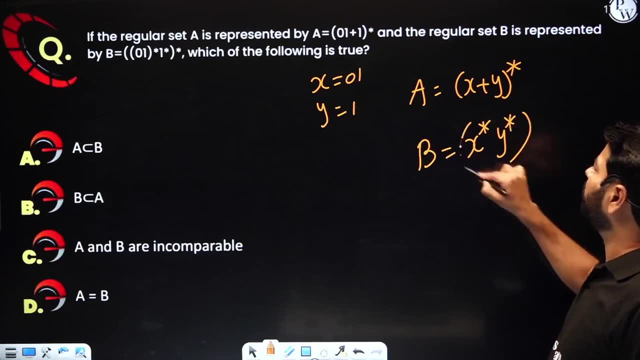 y is 1, so a looks like x plus y whole star. b looks like x star y star, whole star a. very simple, okay, x, y, you may assume a, b, that you already solved it. we know all these two are already equivalent. right, these two are already equivalent, so you can simply go for option d when you are. 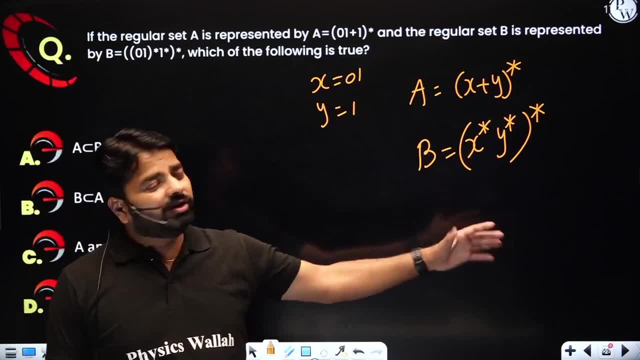 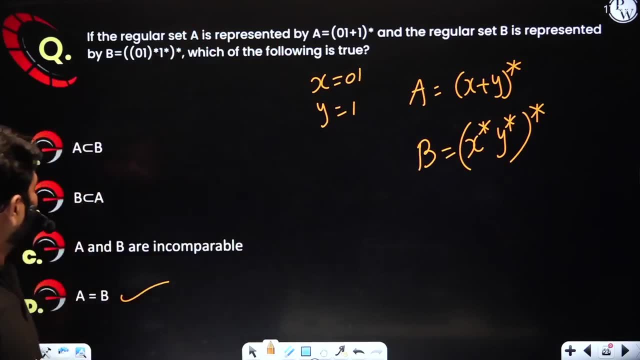 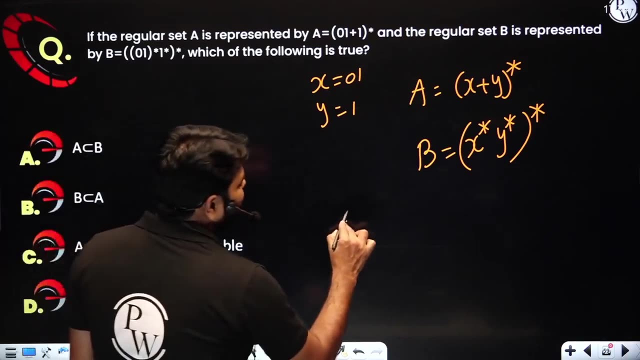 able to interpret it properly. this can be done quickly. when you are not able to do, just try to check. are they doing the same things? okay, of course. uh, these things are wrong. only the reason is if, instead of this, a subset, p, if the, if the right a subset are equal to b, this is right and b. 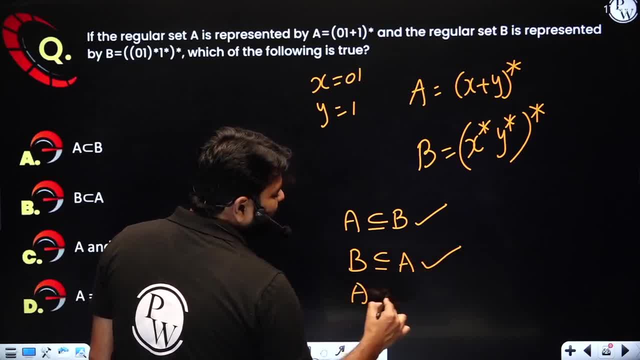 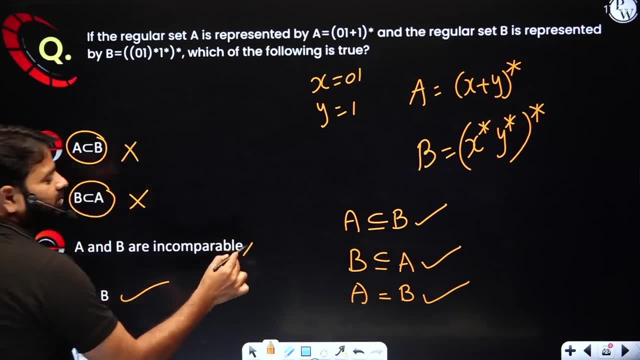 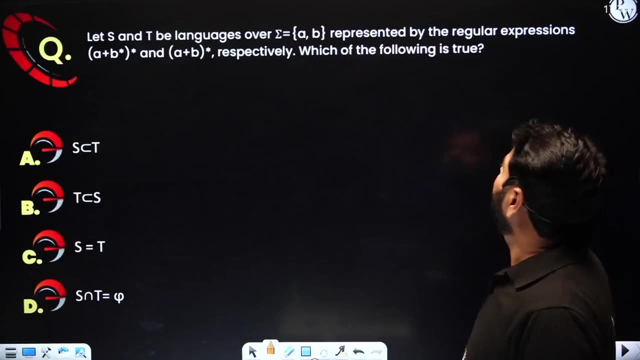 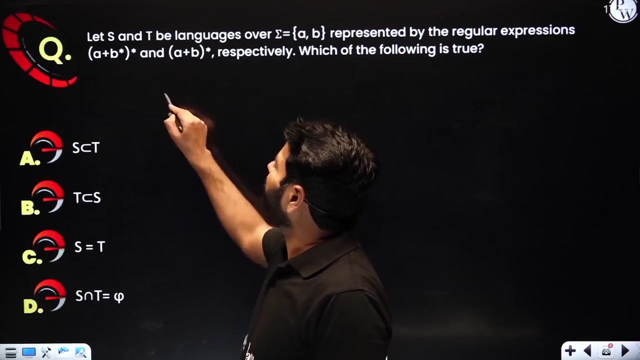 subset or a, it is also right. and a equal to b, it is also right. but here they have mentioned clearly, strictly, subset. that's why we don't choose it. okay, fine, again we have similar question. which of the following is true? you know, that's what the question is about. s is mentioned a plus b. once you know about a plus b, 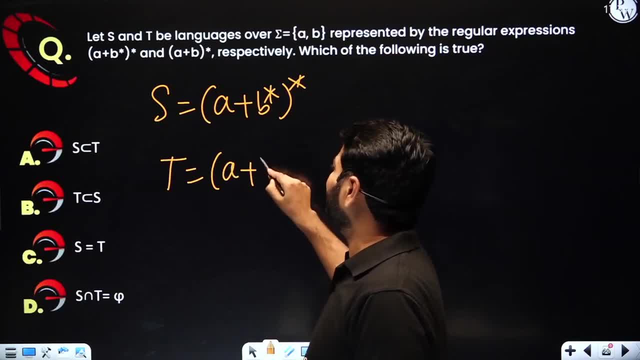 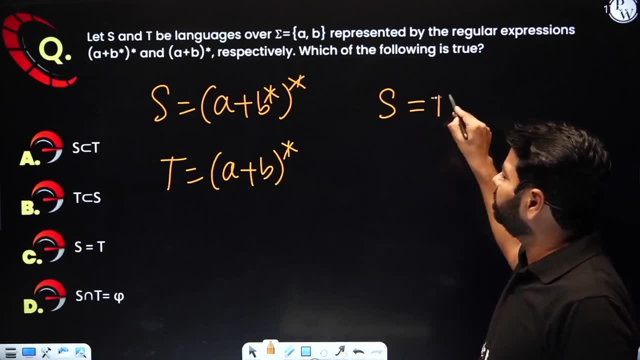 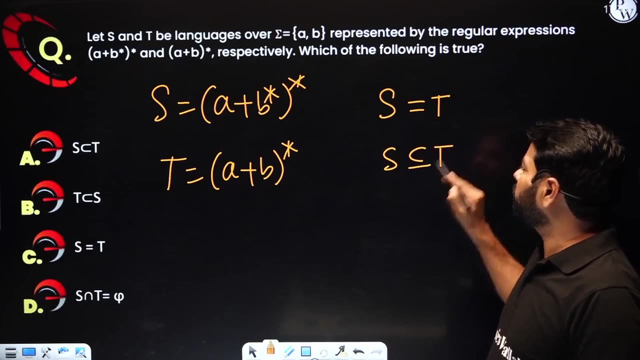 whole star. many things look so easy and i don't need to say: are they equivalent or not? what is the relation between these two? i just told s is equal to t because these two are going to generate the same set of strings and when these two are equal, you can write s subset are equal to t, or? 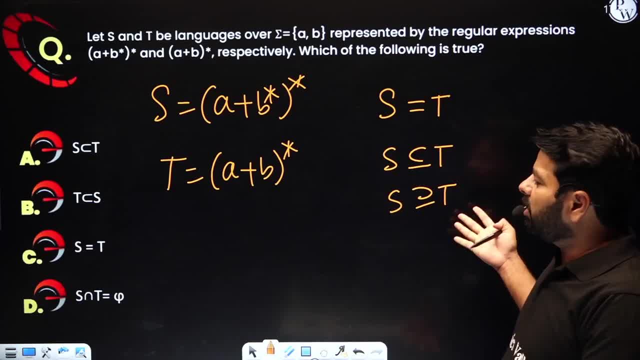 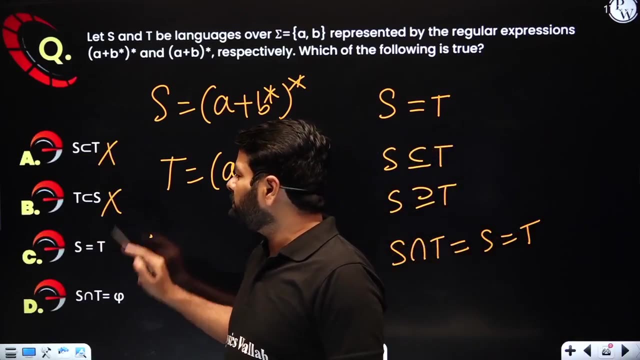 s superset are equal to t, and these options are obviously true. and what else you can say? s intersection: t has to be s or has to be t, because both are same. actually, right now you are strictly subset wrong. strictly subset wrong and equal to correct. and here 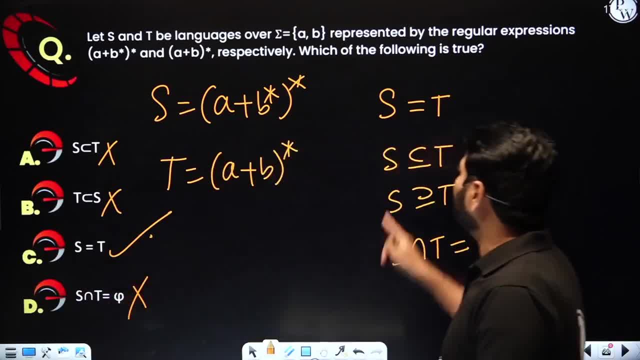 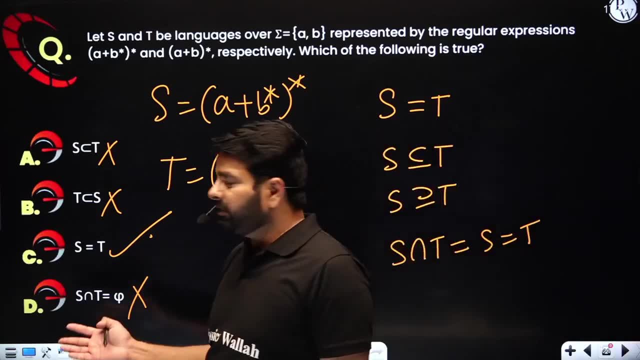 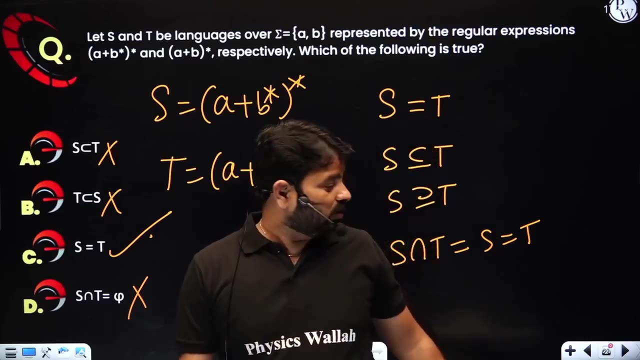 equal to pi. pi is means there is no common string, but we know s and equal. s and t are same, so s intersection: t has to be s or has to be t. definitely it has to be. you can't say this: equal to mt, right? how easy now to compare the two languages. 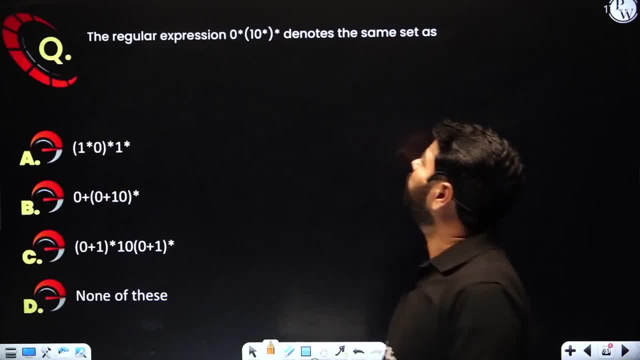 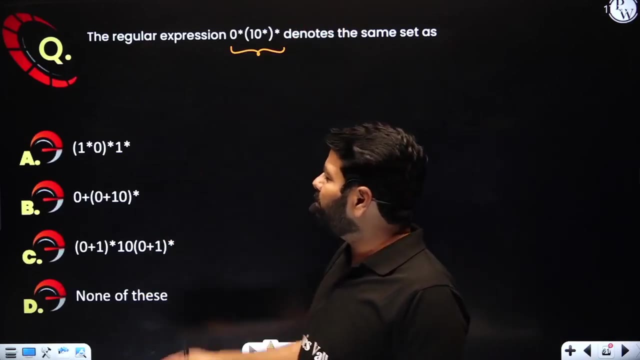 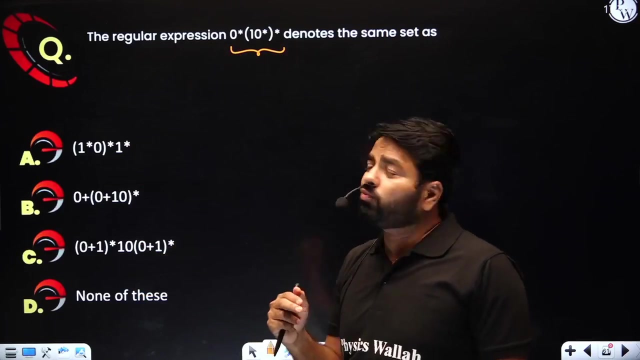 okay, can you do it now? i just explained it in the beginning, but you know we are doing continuously. definitely you might be missed somewhere here, somewhere. this expression, which one is equivalent to there are so many right think about. it's one of the uh again, important form for zero plus one whole star. zero plus one whole star, or a plus b whole star. 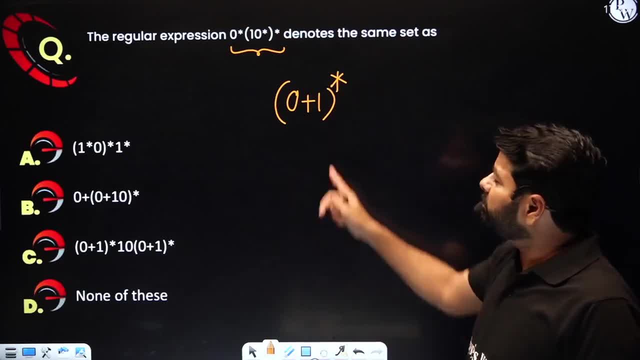 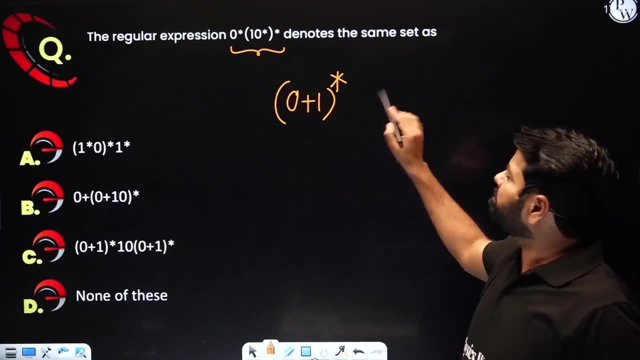 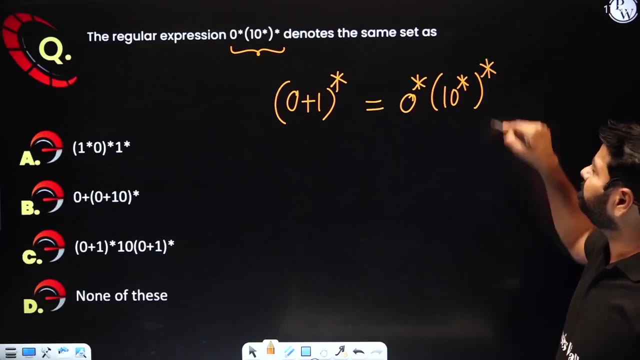 you have a lot of forms. you know this form you did not see so far, but if you see somewhere one of the option you might have been seen. now let me explain again why. this is equivalent to zero star, one zero star, whole star. okay, think about it. uh, various ways to explain. 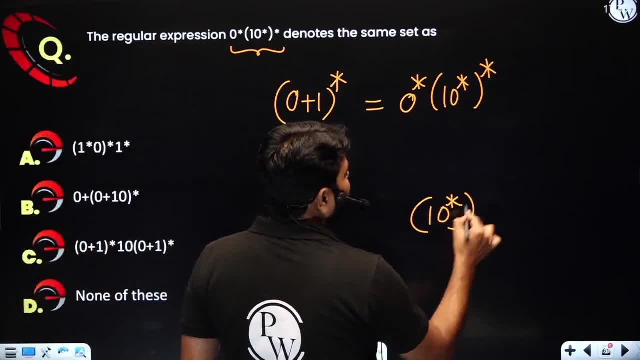 x is equivalent to 0 one-zero-star whole plus per child. so it is equivalent to x times a whole plus a whole plus one off, like four plus like there is a whole boss by flying would be cast into one s or two-zero-star unit one and so on. so that is again like this. you could makezeniexp events both from a n level at those twoếms, when you would have already explained, and thus, if you have something like just, you have more than one. so that is 1, which would be like one zeroo skills. that is the one, old bulls, and then it's encouraging. 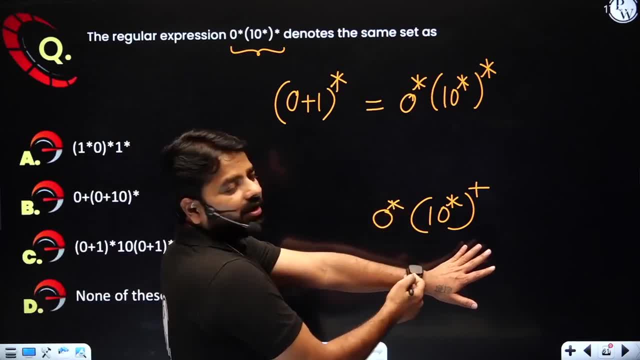 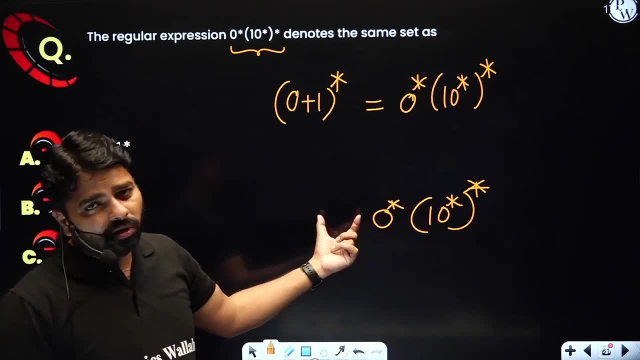 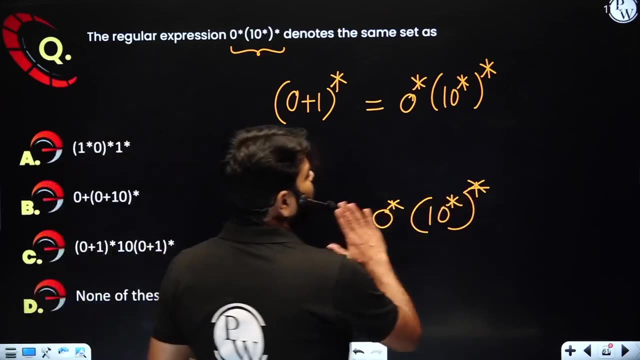 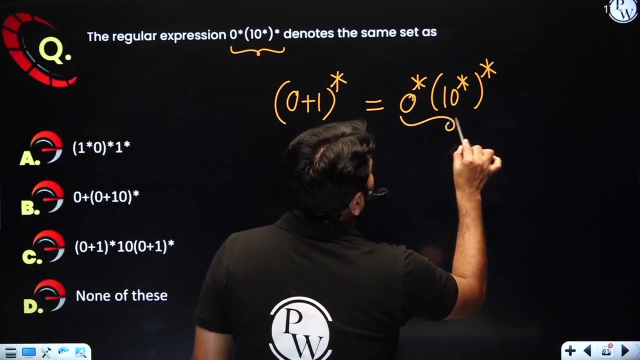 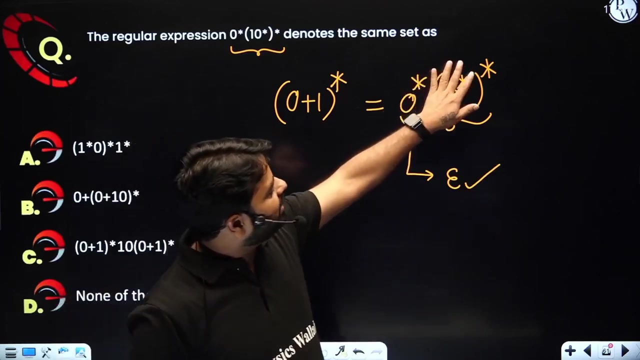 your job so the next little character can start. if it is after the valuation at there, okay. when you consider it as only cast and say that everything else okay, so he's coming, is already, is facing a little. He or into明 is equivalent to 0 plus 1 whole star y epsilon. can you generate? yes, how. 0 power 0 and this power 0. 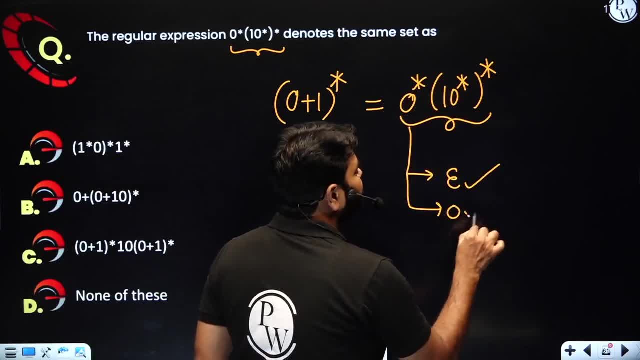 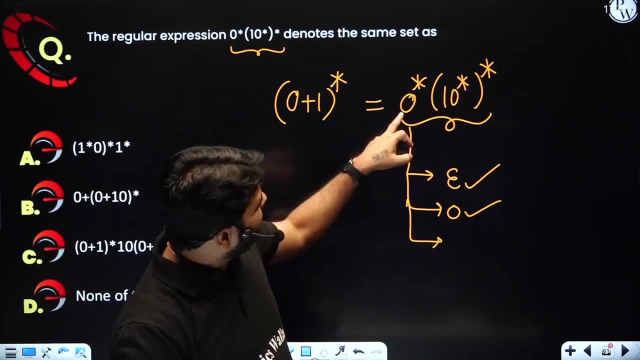 you will have epsilon. can you have 0? yes, here you have 0 power 1, put power 0 and whenever string starts with 0, take this 0 into consideration. whenever it starts with 1, don't take this and it you will have everything here. okay, remember everything here. it's very simple once you started. 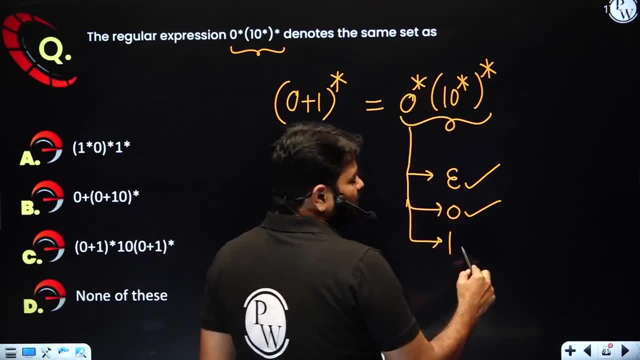 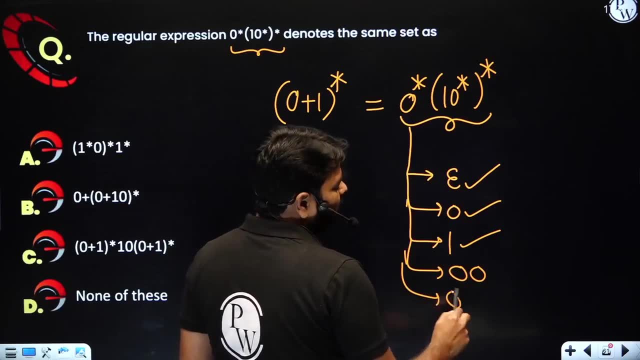 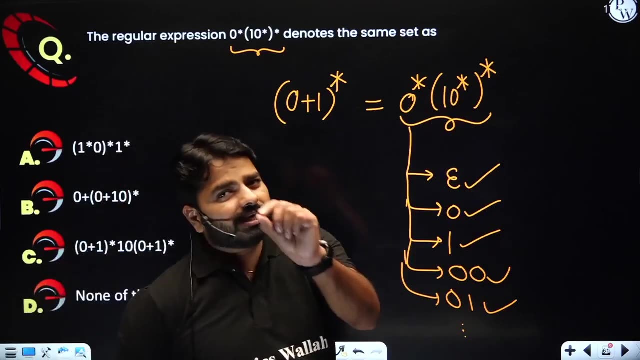 you go inside by ignoring this, by putting power 0, and whenever the string starts with 0, then take this 0, other 0 you can get from here and 0- 1. take one 0, another one from here, and so on. everything is possible from this expression. i'm saying: when the string starts with 0, take this 0 into. 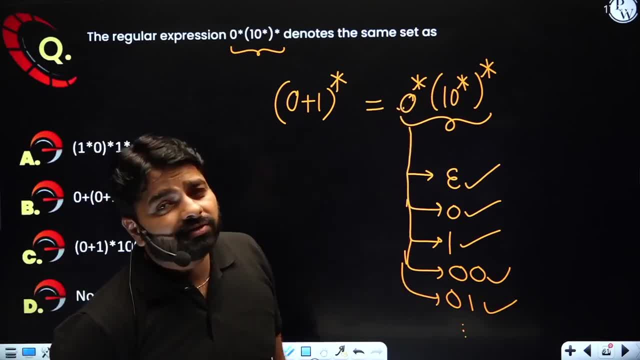 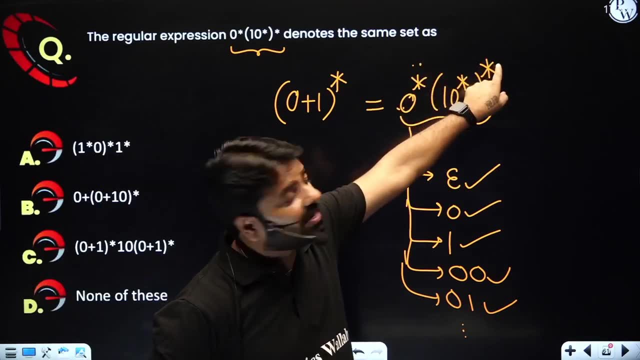 consideration to generate the first 0 and whenever the string starts with 1, take power 0 and starts with 1. already you know it is possible to generate it from here, because whole plus we have seen now it is just whole, sir. additional epsilon: epsilon. epsilon is there? okay, now come to. 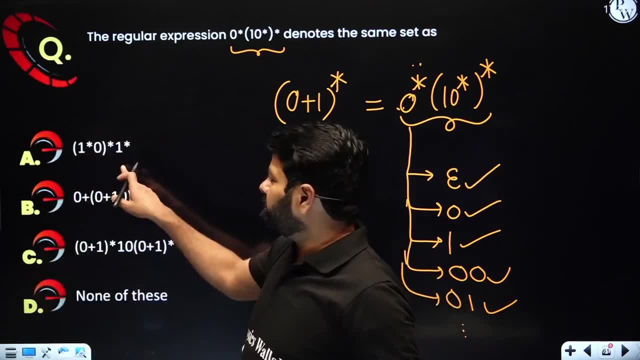 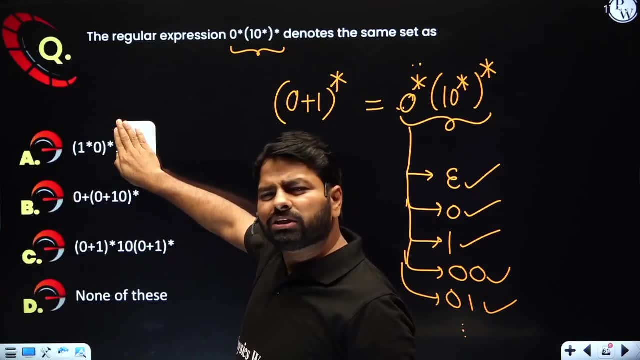 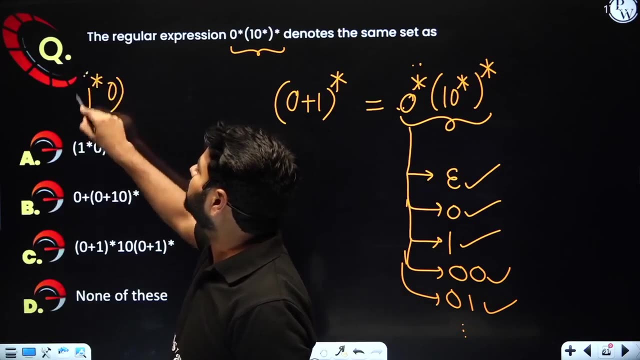 this one which one can generate all okay. now look at here: 1 star, 0, if you don't have this, and that's almost generating ends with 0. all strings, not almost all, but additionally epsilon. additionally, let me explain that: to 1 star, 0, whole, plus you know it ends with 0, right? 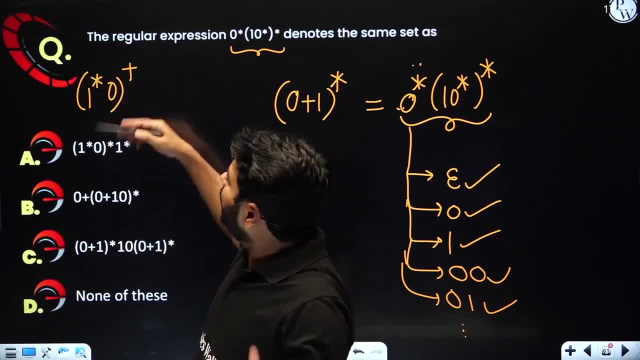 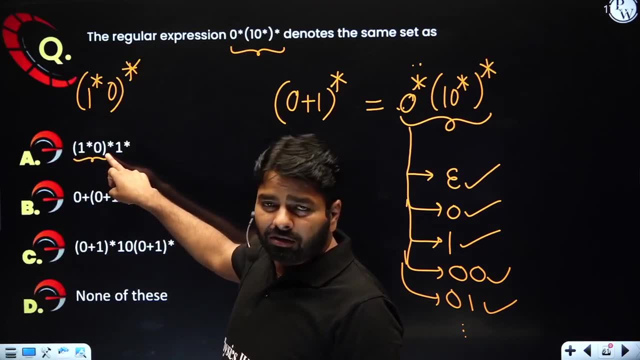 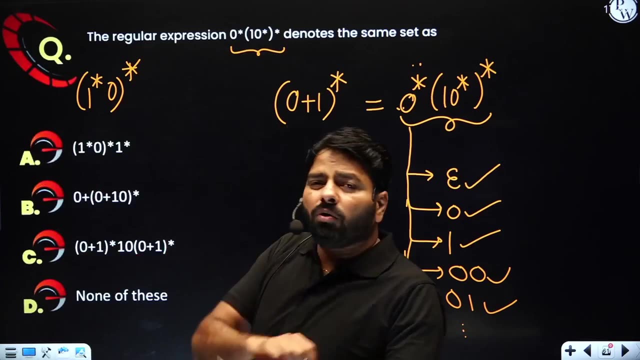 it's a form for ends with 0. now what do you have? additionally, epsilon also means power. 0 is added. now here ends with 0 or epsilon, and this one will guarantee ends with 1 or epsilon. so somehow here ends with 0 and ends with 1. all the strings are. 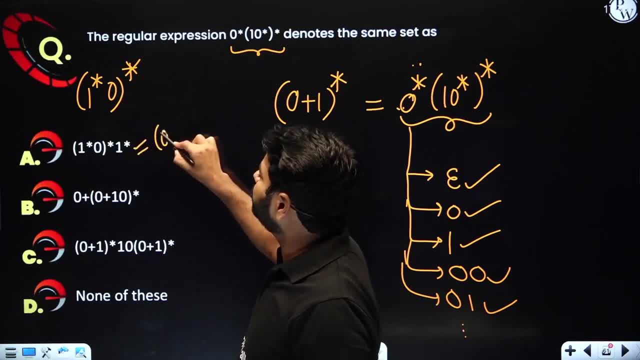 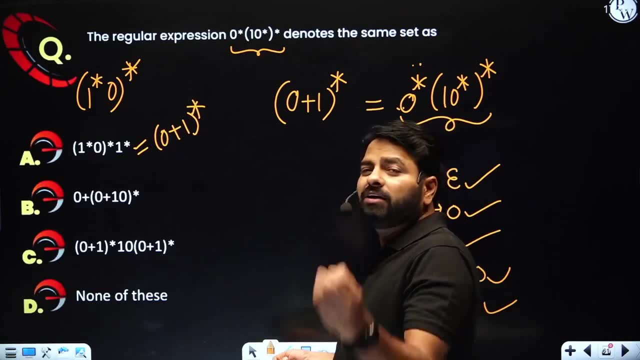 covered. so definitely this is equivalent to 0 plus 1 whole star. and here you want to know much. just try to generate one string, every string. you will see every string which is present in 0 plus 1 whole star. and now elimination is so easy. 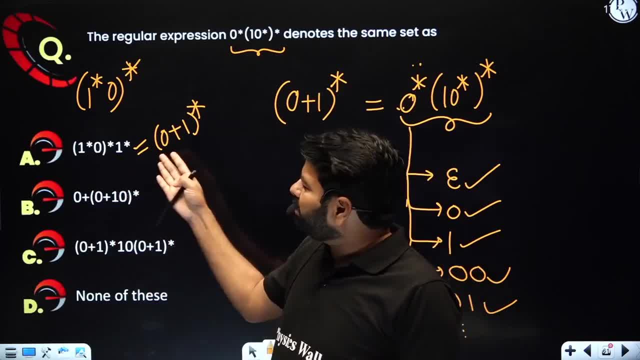 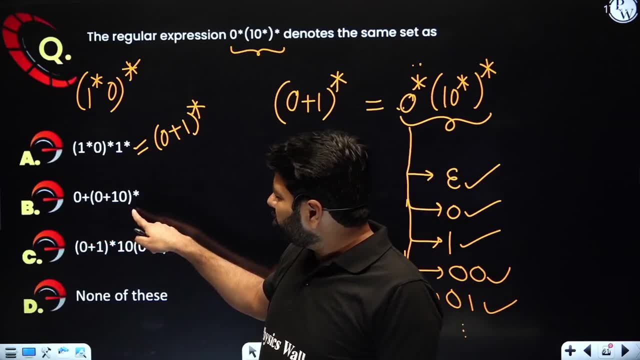 here again rather than finding the right answer. but i could explain much about it, but, as you know, we need to cover many things again now. 0 plus 0 plus 1, 0. also, what is missing here can you find out? can you generate epsilon? yes. can you generate 0 s. can you generate 1? no, that's enough. why it's? 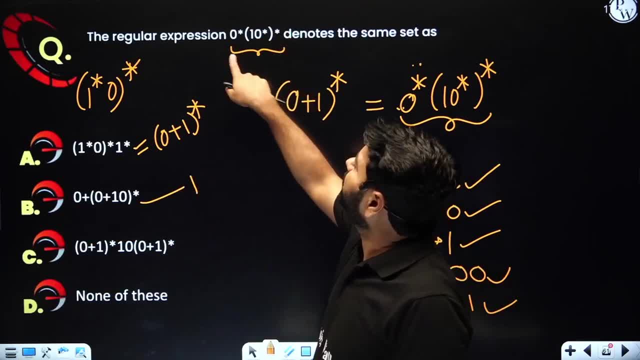 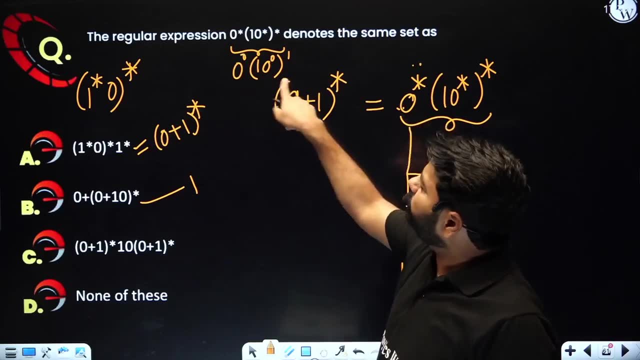 not equivalent to 0 plus 1 whole star. see here, can you generate 1 here, yes, how 1 here 0 power, 0, whole power 1 and 0 power 0. so this could give you 1, but here 1 impossible when you generate 1 whole star. 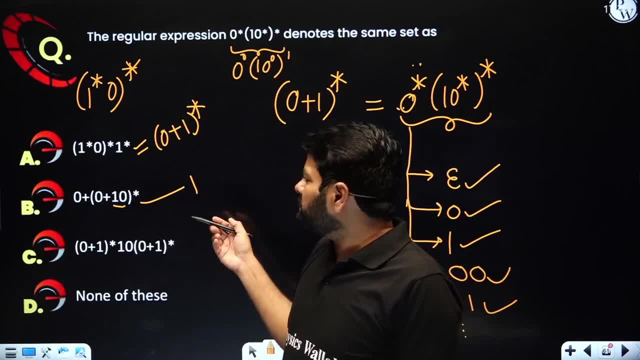 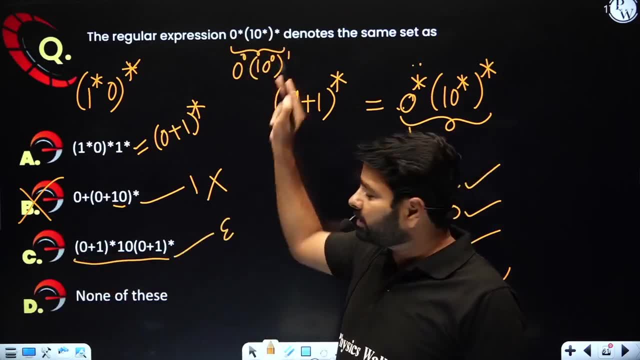 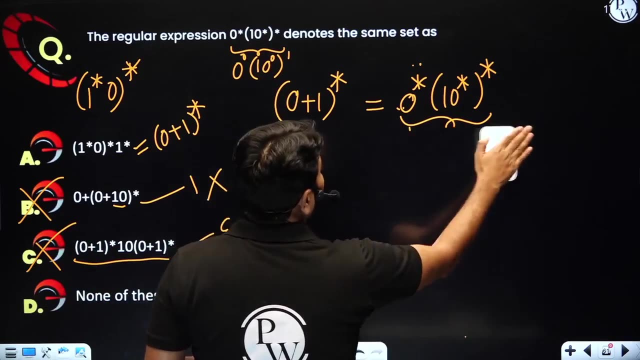 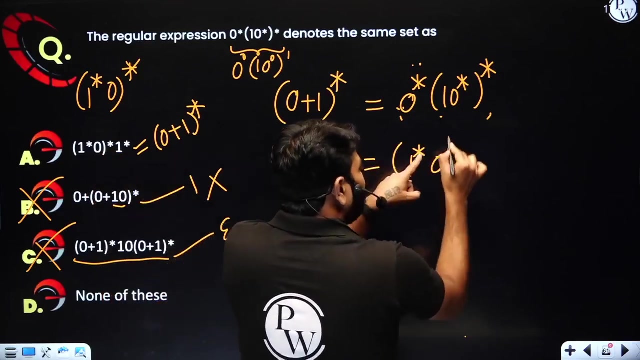 you could take 1. 0 also comes here. 1 is not possible very straight away, so be eliminated. and here epsilon is not there, but we need epsilon. epsilon is possible in the given expression right, c is wrong, a is equivalent. so here the expression that ends with a 0, right ends with 0, the old plus. 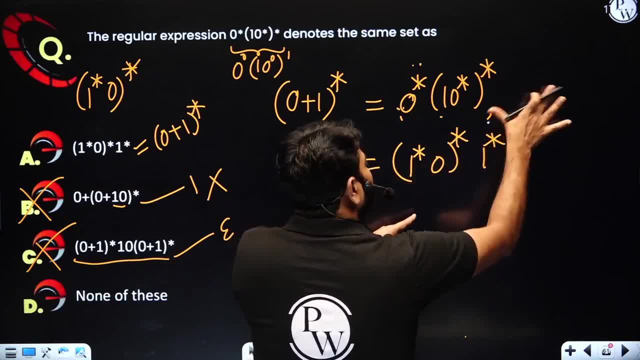 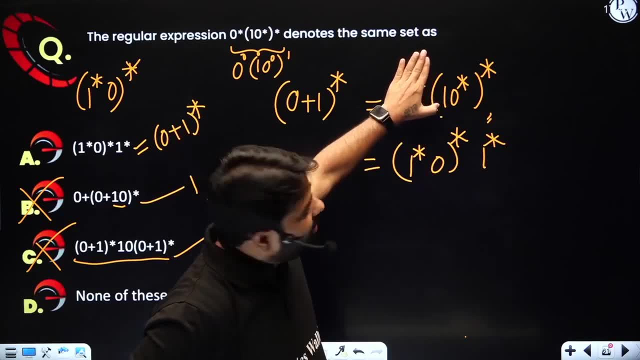 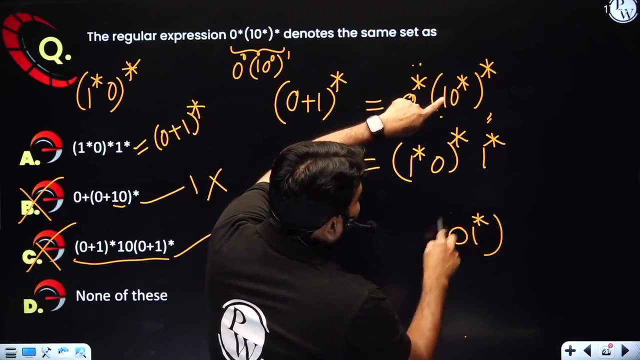 now you have whole star and 1 star. you want to write many other expressions. yes, you can write lot other, but i'll just give you a hint. when you take stars with 1 and you consider 0 star, when you take starts with 0 here, if you put 0 here, i'll write here 0, 1 star, whole star, whole. plus is. 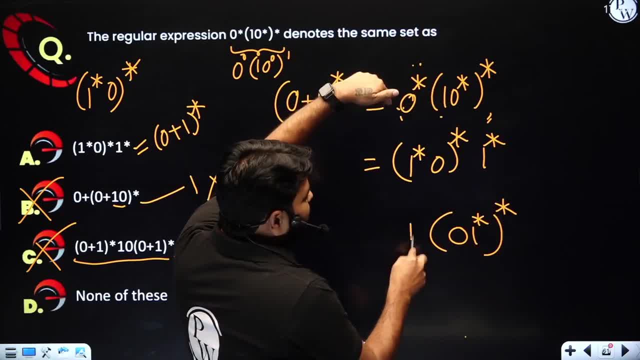 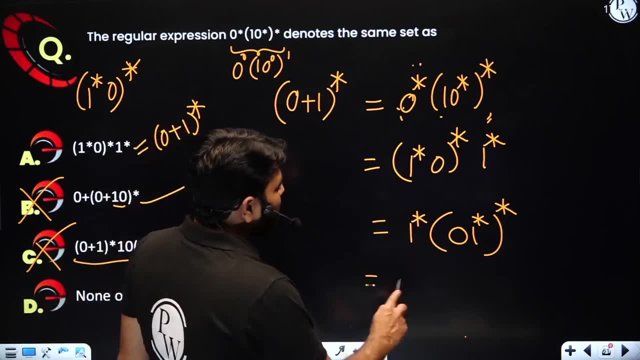 there actually whole star now to have an epsilon. but here you just write 1 star. you try on your own, will it give all the springs over? 0 plus 1 whole star. not only this. this ends with 0 concept right now i'll keep. ends with one concept: 0 star, 1. 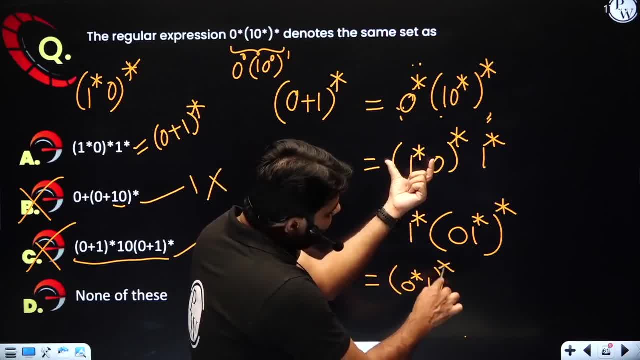 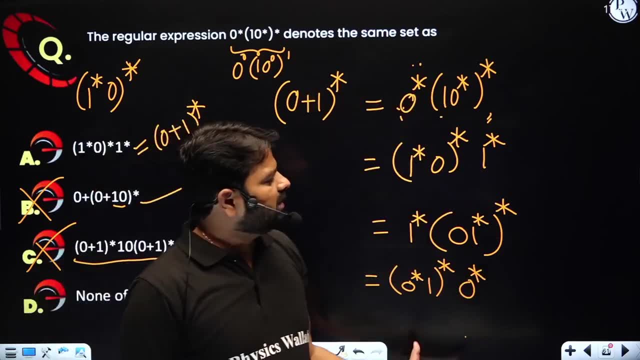 whole plus was there actually ends with 1? we have whole star ends with 1. if not ends with 1, ends with 0, 0 star. look at all these four expressions and try to do on your own. this should generate 0 plus 1 whole star. if not, comment below the video and if you miss any string, how to. 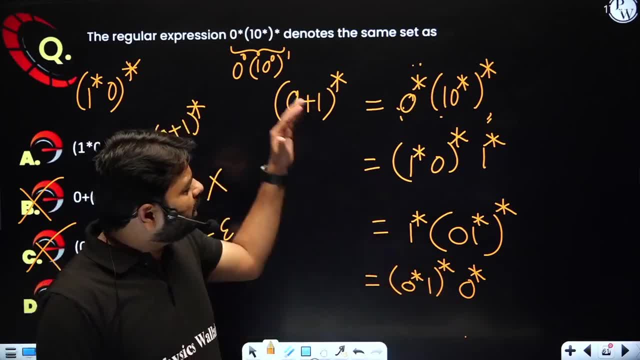 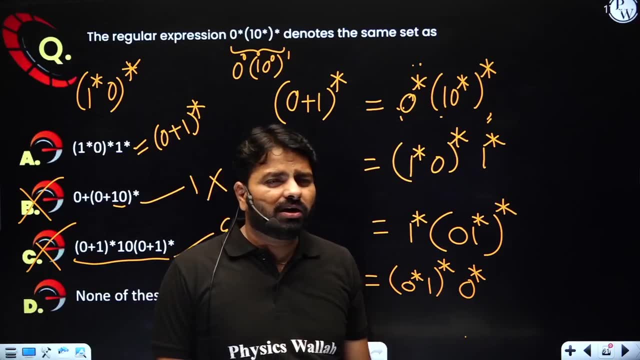 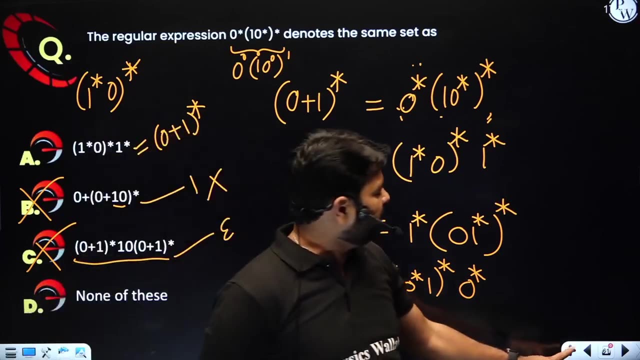 generate from that. i will, i will help you. so you keep on trying it. you keep on trying it. there are various expressions which are equivalent to 0 plus 1 whole star, a plus b whole star, and all of them are very, very important. in case, if you would want to know about various expressions, let me write many forms now. 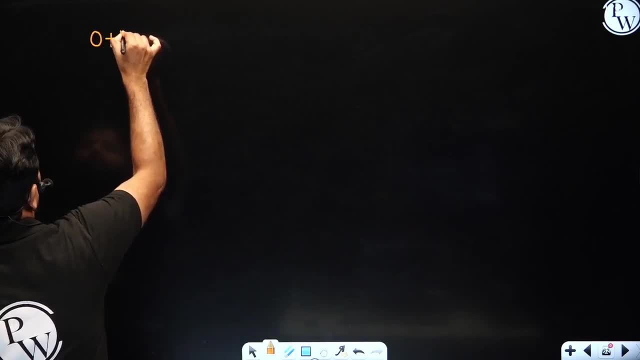 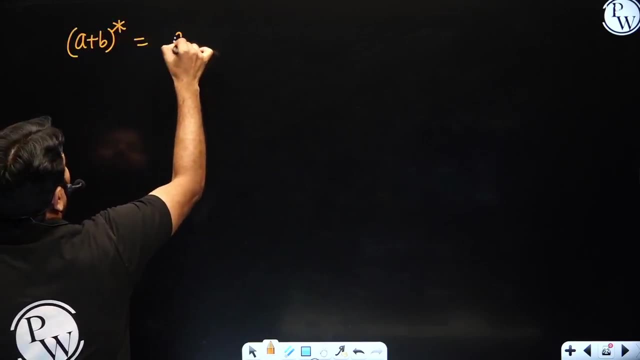 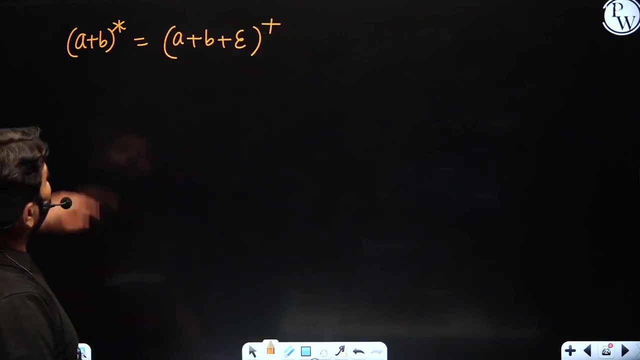 0 plus 1 whole star, or you can take a plus b whole star, both are same right. one thing you know you may are a plus b plus epsilon whole plus very important form equivalent to this one, because epsilon outside you can generate, now here inside. that's all everything. 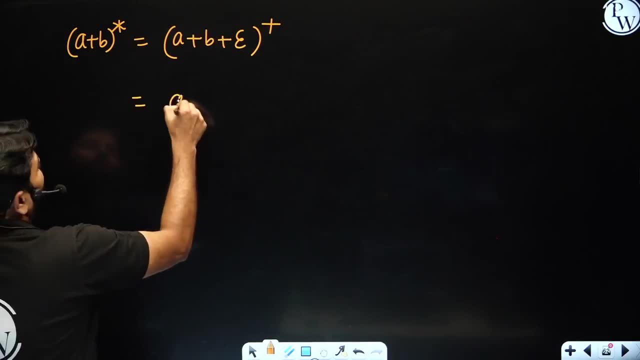 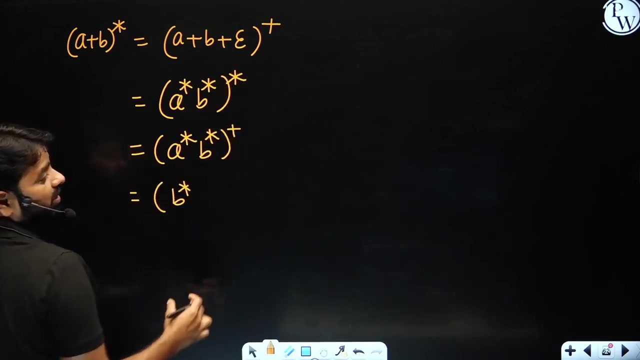 is same and you can generate a plus, b plus epsilon, whole plus, and you can generate a plus b plus and you can write a star, b star, whole star. and i'm just writing rather than explaining all these things. please work on each one: whole plus and whole star, even though looks different, but generate 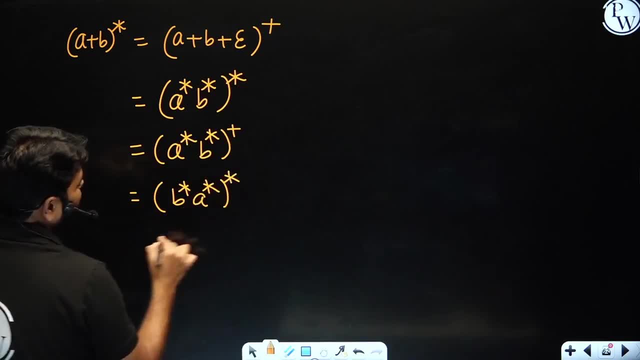 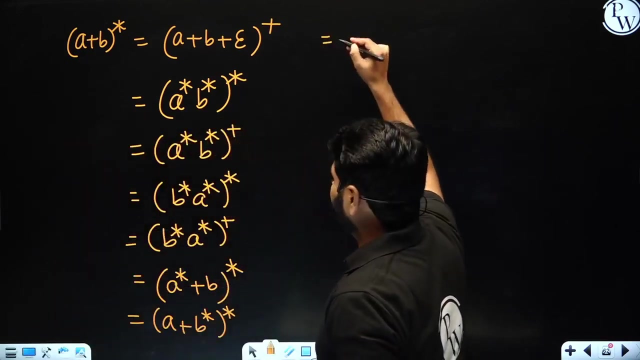 the same set and each one equally important for you. please work on each expression to understand very, very important expressions only. i'm writing here. you see directly them in the gate questions. you can easily identify it later on. a star plus b star, whole star. did i miss anything else which are important so far? 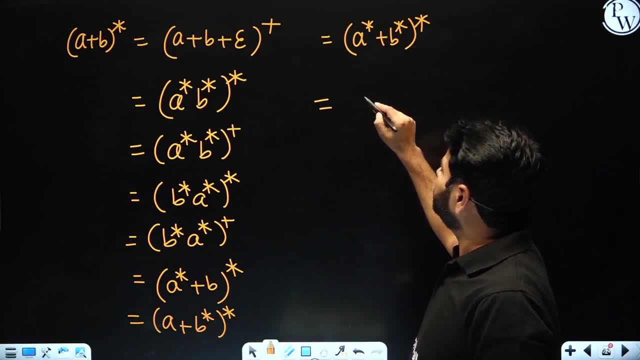 okay, uh, just now we have seen right. um starts with a, is there? suppose? so you want to start with b? then b star, is there? suppose? so you want to start with b, then b star, is there? so how you do that is- there is a starting picture here and then you have all the stars. 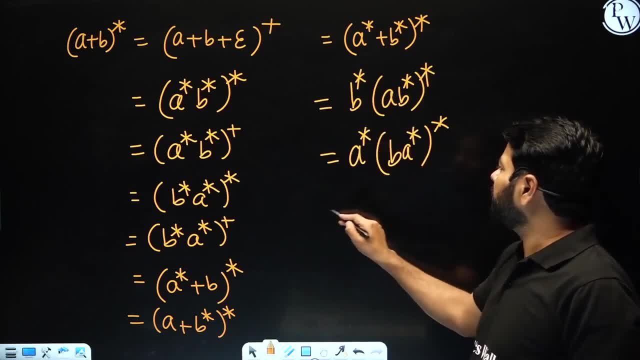 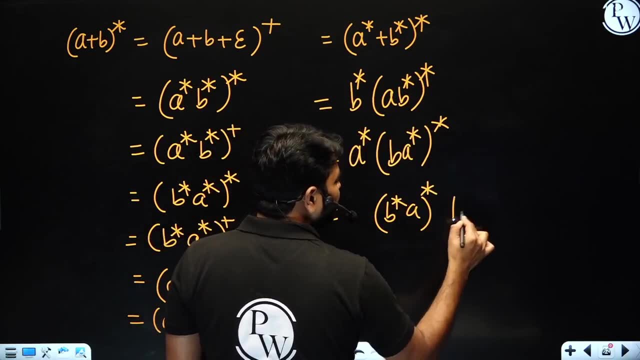 you have all the stars that will follow you. so you will know how to start with b and what you should have now. suppose start with b- you have here- and starts with a, you should have a star. suppose ends with a, then b star, a whole star. if you want to end with b, you need to have this one. 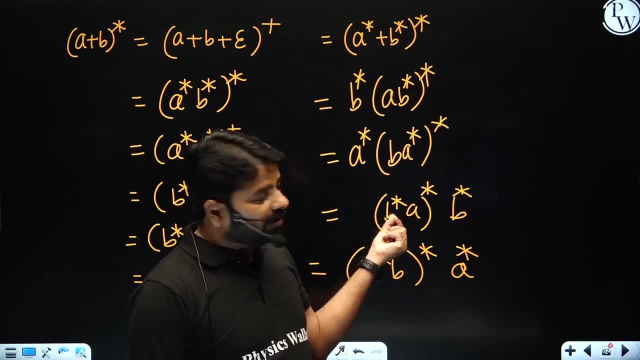 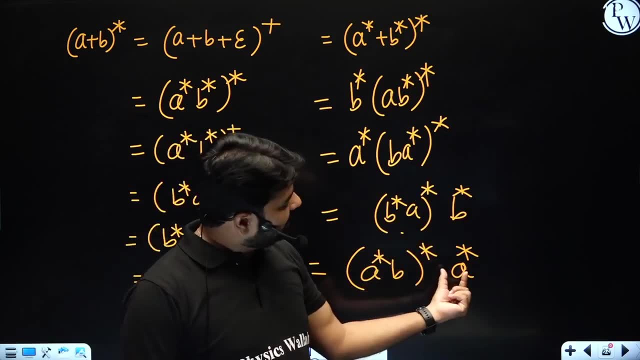 ends with b. so there is a concept that i am following which will help you when you practice. so when this is covering ends with a, then b is here. so ends with a to make it a star. i kept it. similarly, starts with b: i took first, then to 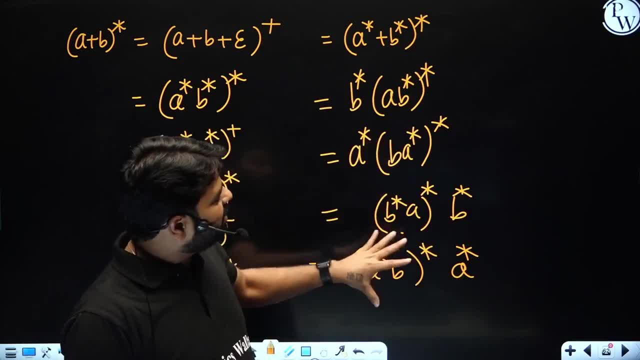 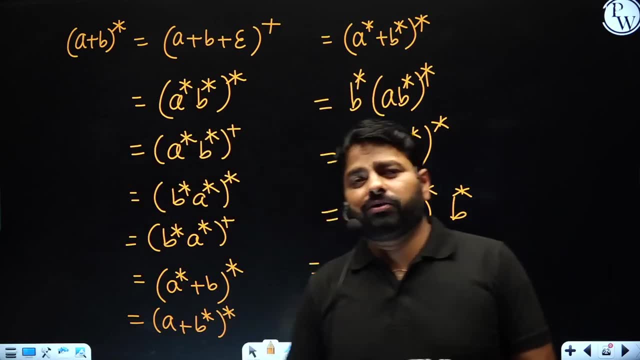 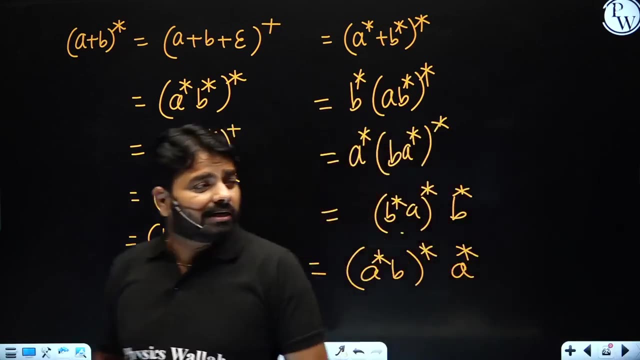 have the starts with the a star i have written, so there is a logic why i am writing this to make a plus b whole star. all these expressions are really important for exam point of view. okay, in case, if you are able to remember all this easily, that would be fantastic. in case you are still having 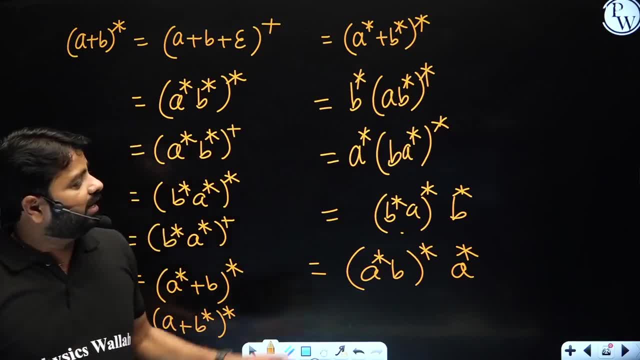 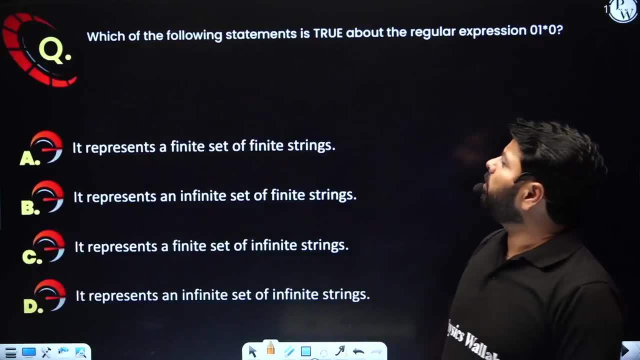 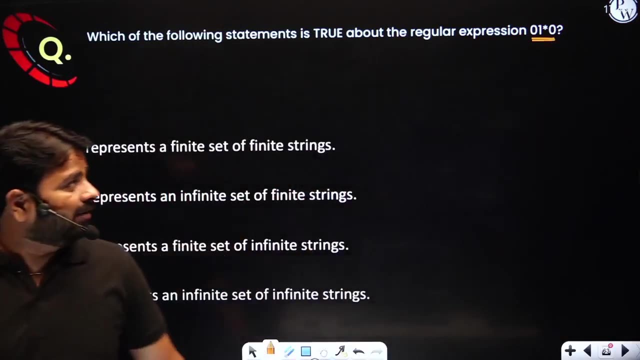 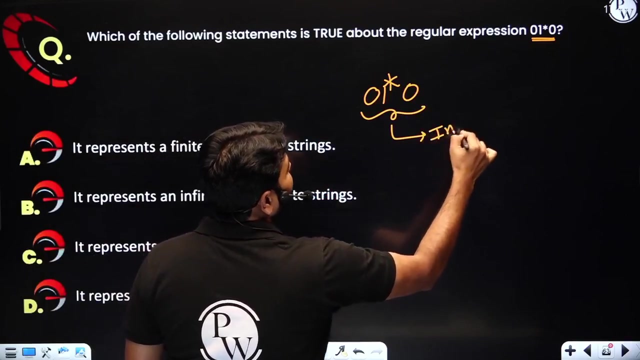 any difficulty. you can have a discussion. you will learn a lot from this expressions. which of the following statements is true about the regular expression? so 0, 1 star 0. okay, i was talking about the language right r set. is it finite language or infinite language? it's definitely going to represent infinite set, correct? so now look at. 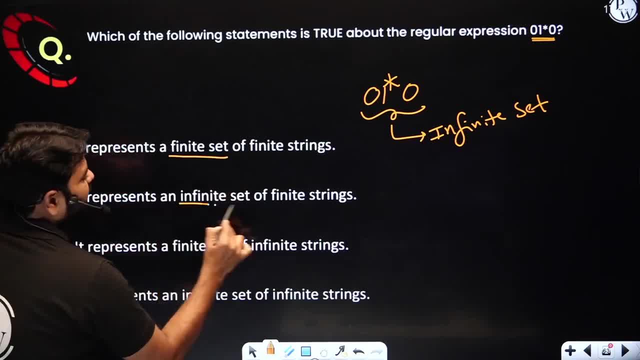 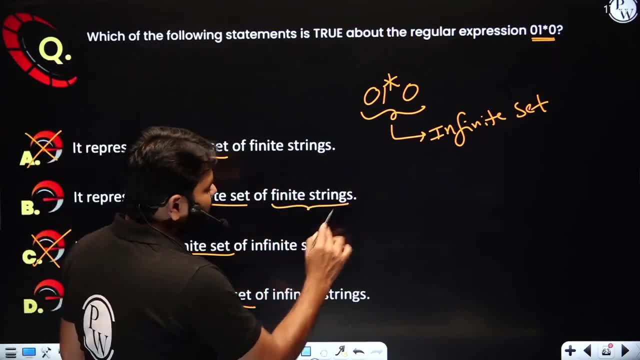 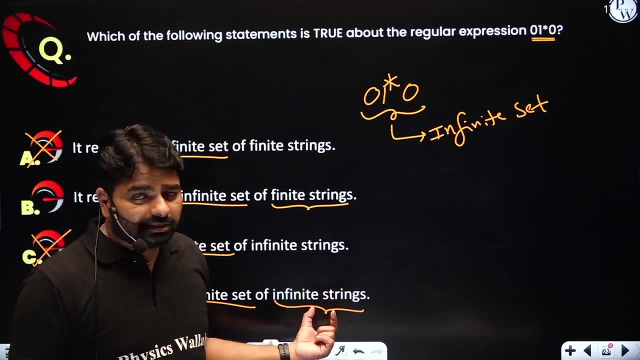 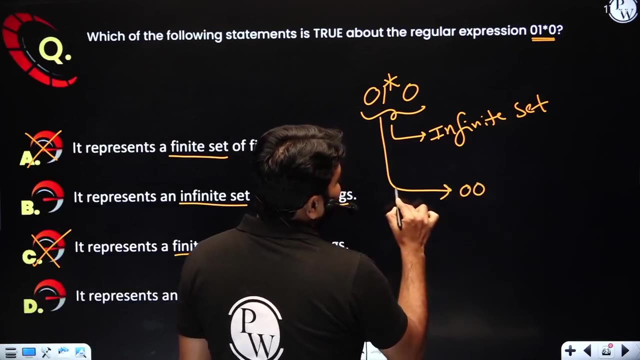 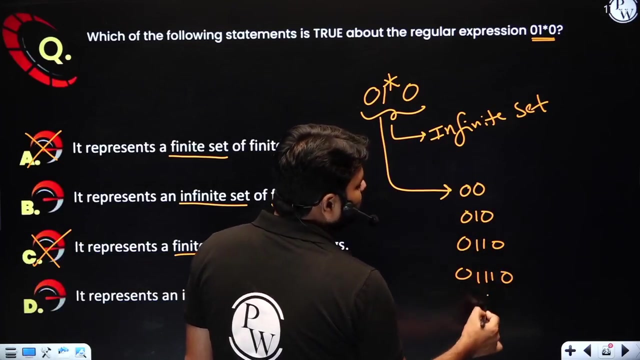 strings. is it having finite strings? is it having infinite strings? I told language never contain infinite type strings. it will only contain every string views finite. now look at when you write here: minimum string is double zero. next string is what? 0, 1, 0, 0, double 1, 0, 0, triple 1, 0 and so on. every string is finite. can you see that such 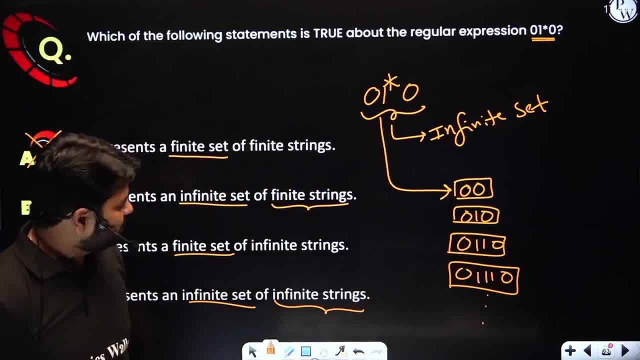 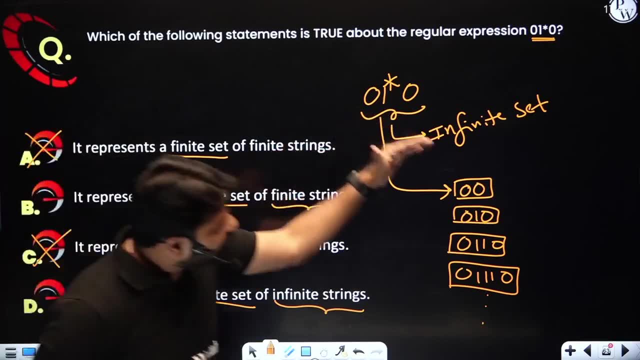 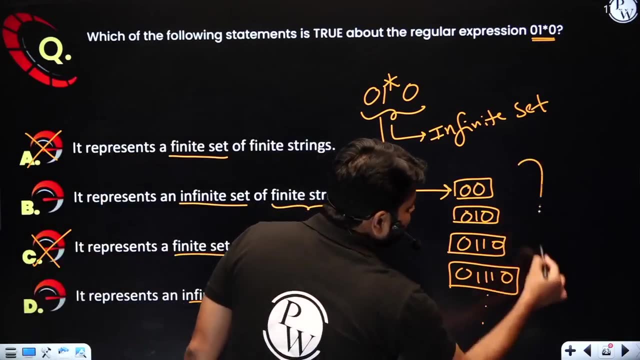 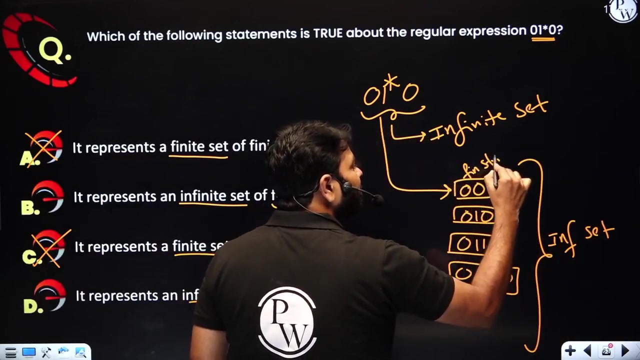 finite strings are infinite, but every string is finite, so it is infinite set. having finite strings, infinite set means already infinite number of strings. i have infinite number of strings, but every string is finite. only you can see here how many strings are there. this is infinite set, but each, each string is what finite string? this is also finite string. 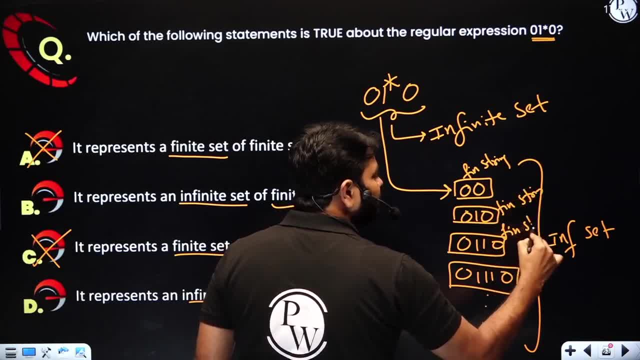 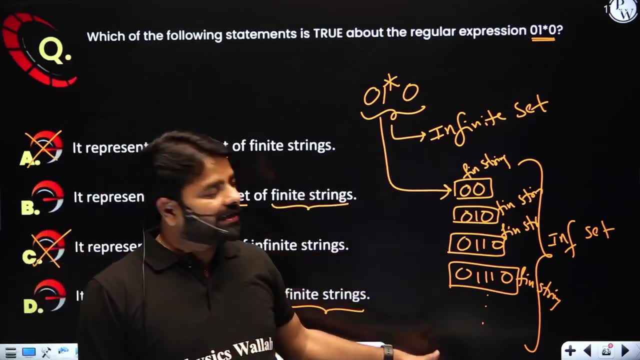 this is also finite string. every string is finite, but those strings are considered infinite times, so we call it is infinite set. it is infinite set. it means there are infinite number of strings, but every string is finite. only you can see here how many strings are there. this is infinite set. 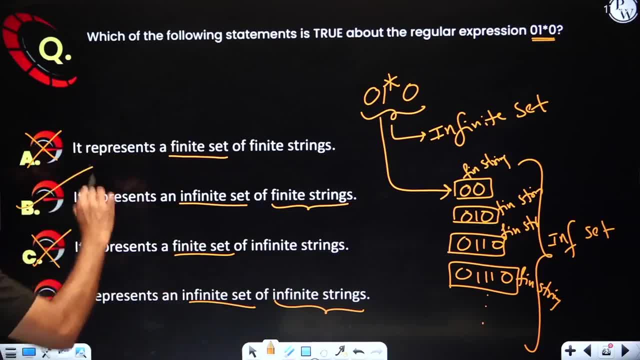 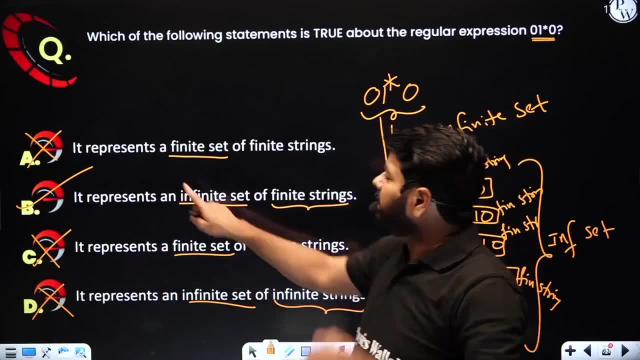 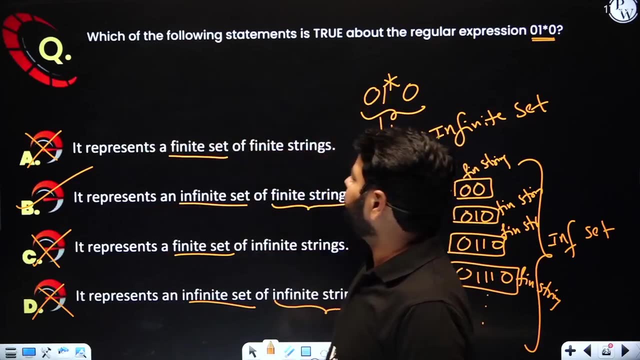 is infinite type. so this option b is right and d is definitely wrong. in case, if you want an example for each one, let's see it represents a finite set of final strings. example: if you want an expression, the expression i'll take: finite set final strings. let me take 0: 1 right. double 0, triple 1. 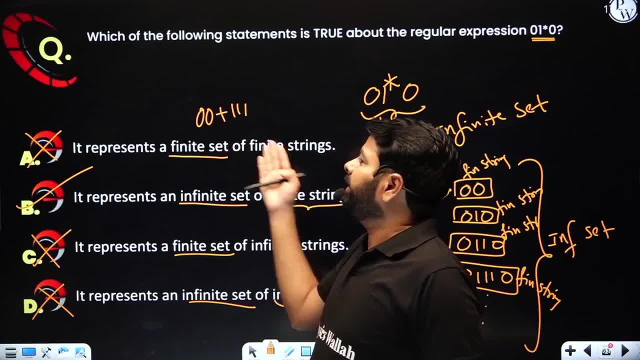 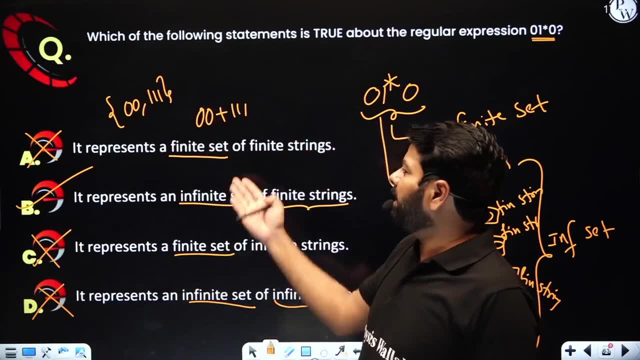 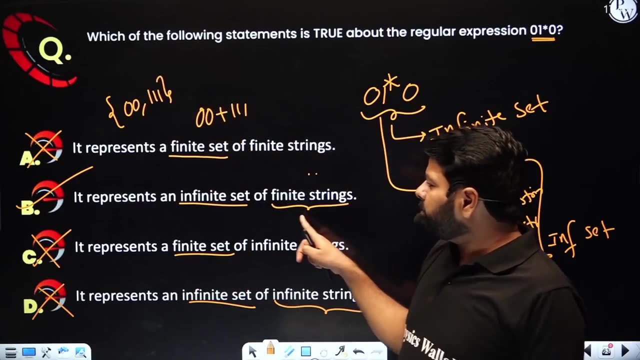 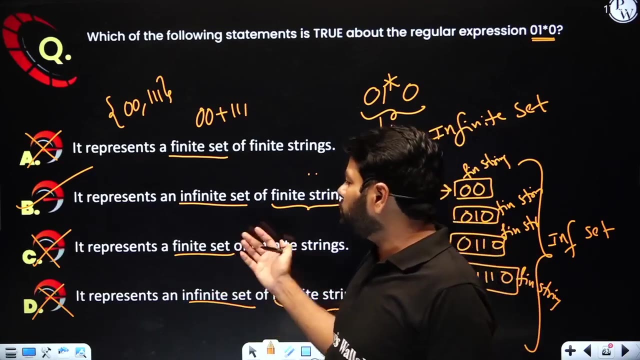 have how many strings? two each string. finite. that means, uh, equivalently the languages: double, zero, comma, triple one. so two strings. finite language. how many strings? two strings, each one is a finite type. this is the finite, this is also finite. and option c: finite set, but infinite strings. oh, we can't write, but still i'm writing is to explain for this finite set. okay. 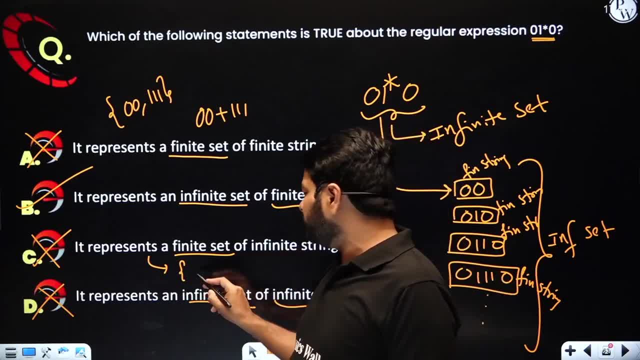 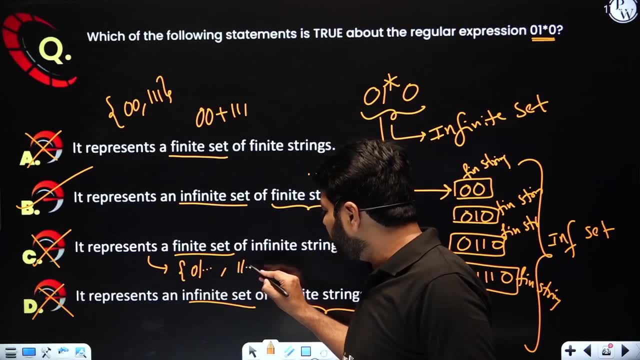 i'll keep only two. but having infinite type strings like zero, one triple dot, one string itself infinite, another one, one, one triple dot, that means see here the string. i can't complete it because the string is already infinite. when the string is infinite, how can you complete one? 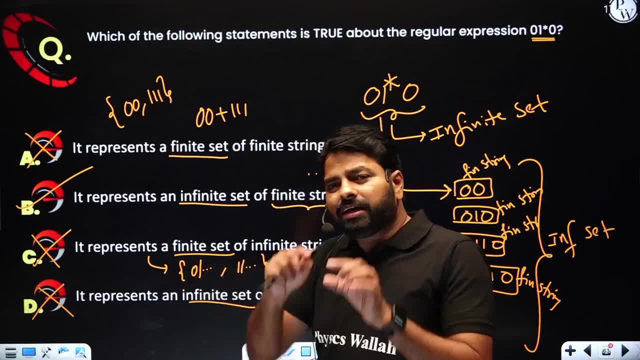 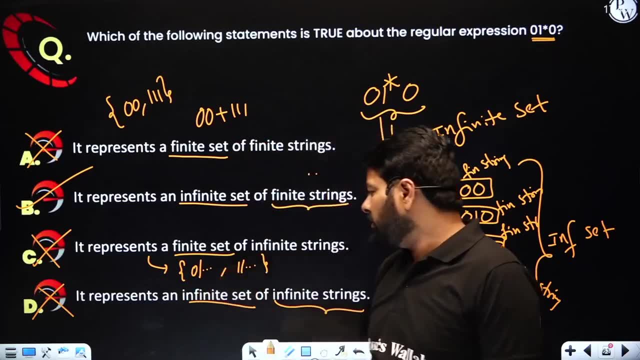 string. very difficult. what is there after? no, you know, at least in real number. you have a bar to represent if it is repetitive. here we are done denoting any such things, because they are not used in computation. another one, infinite set of infinite strings. oh, what is it see? zero, one zero. 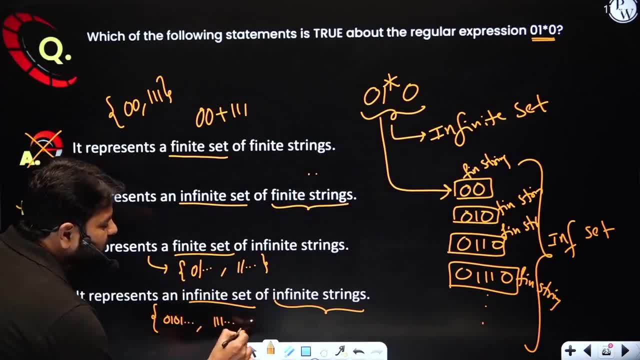 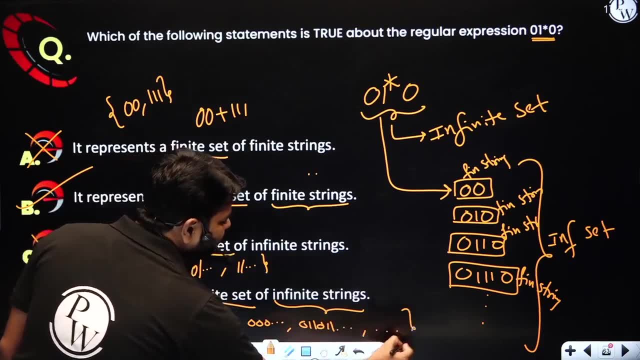 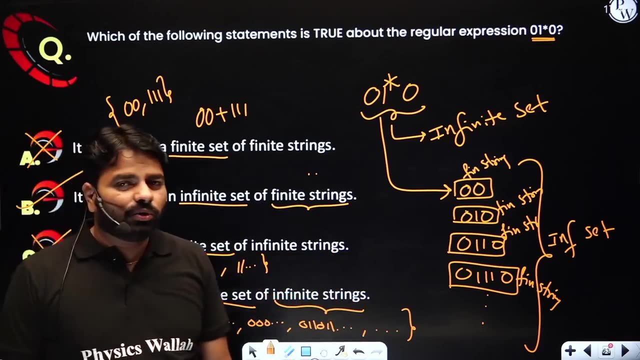 one, three dots. one, one, one, three dots. zero, zero, zero, three dots. zero, one, one, zero, double one, three dots. likewise, you have infinite. every string is infinite and such strings are infinite. okay, in general i already told you that can be infinite, but thing has to be finite. every string has to be. 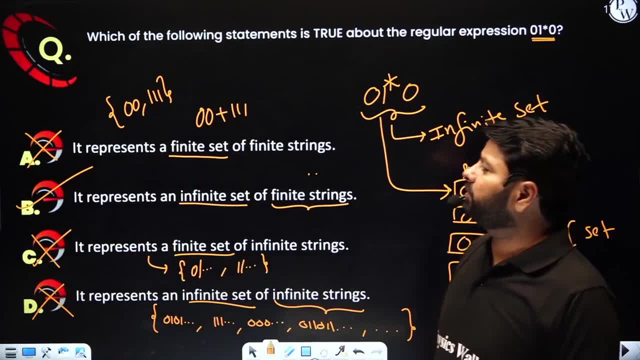 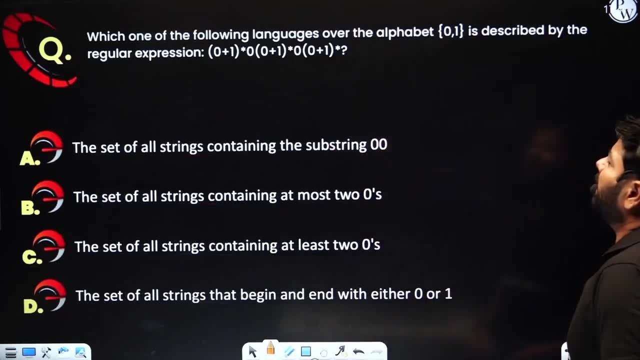 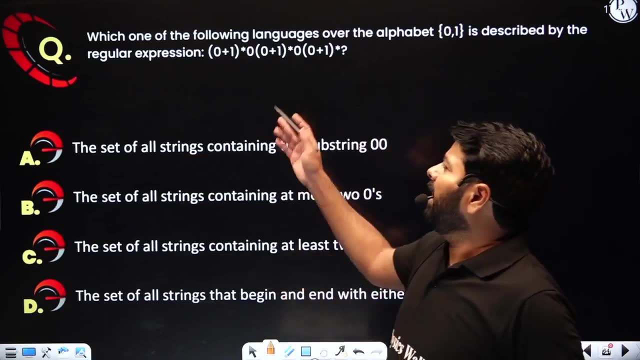 finite in the computation. you know it was a very beautiful question in the exam. so far, okay, which one of the following languages over the alphabet is described by the regular expression? identify quickly. i told you right already. no need to, you know, spend much time. one zero compulsory. 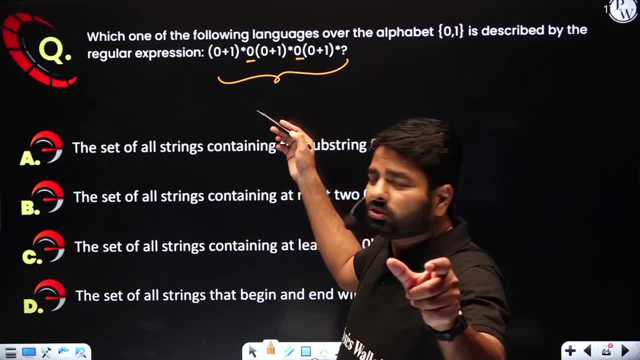 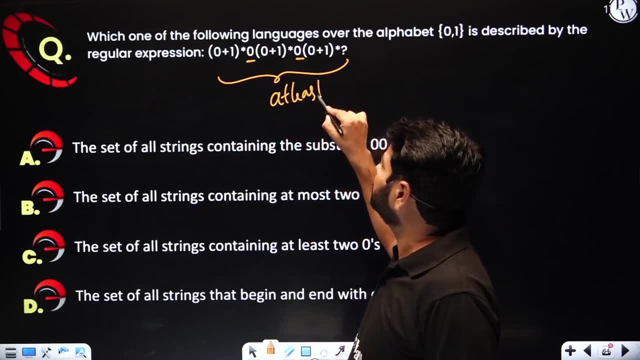 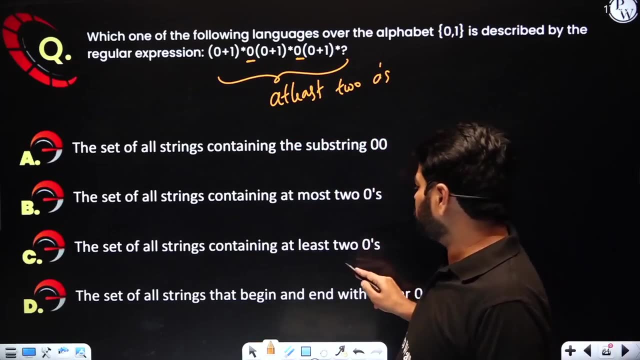 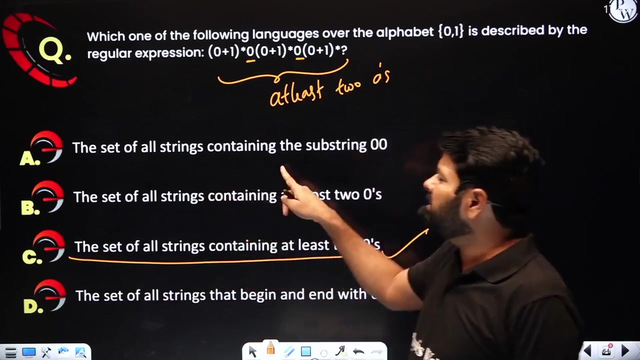 other zero compulsory, which will give you at least two zeros, two zeros guaranteed. third, fourth, anything you want you can cover from other other places. at least two zeros, at least two zeros. okay, where is that containing at most, containing at least this one. okay, in case you want to know all the expressions set of all strings containing the substring zero, zero. 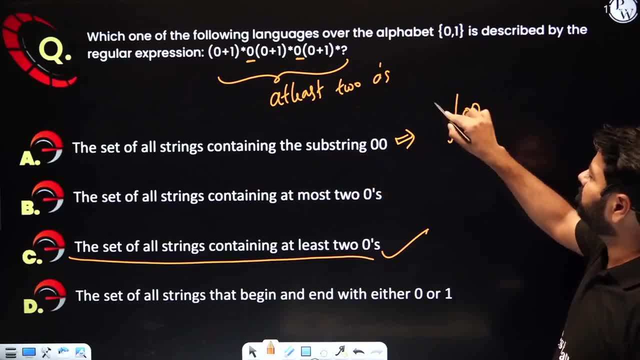 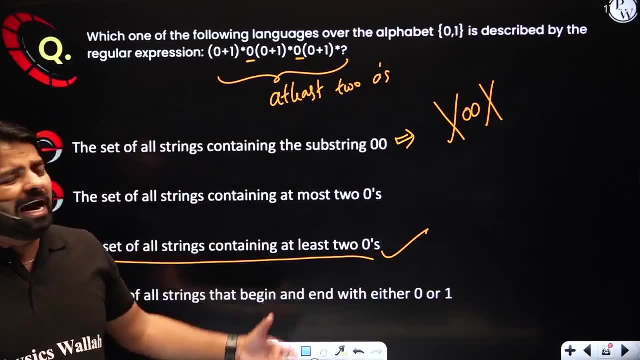 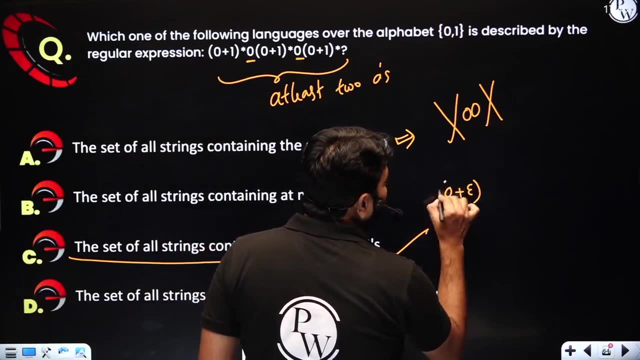 can you write it quickly: zero, zero before, after, anything, right? zero plus one whole star. zero plus one whole star. when i write capital x, understand it is zero plus one whole star, containing at most two zeros at most. you know, you should know how to write it. zero plus epsilon means at most one. 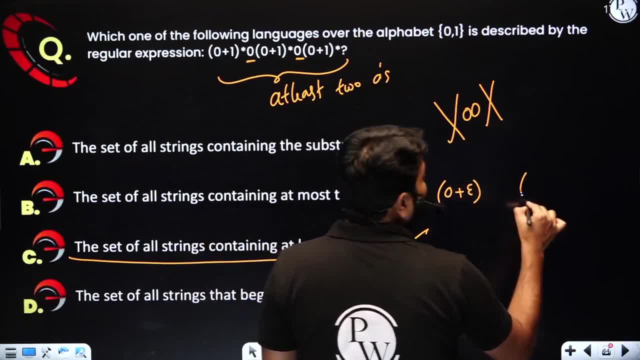 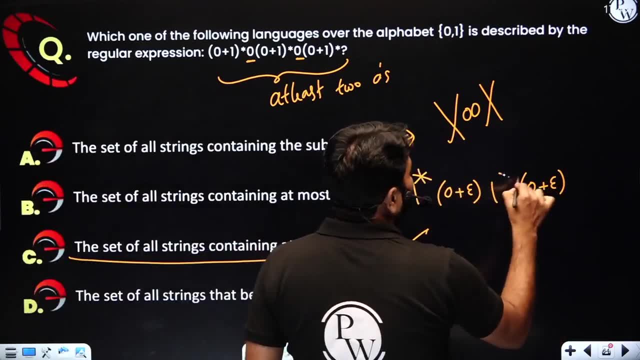 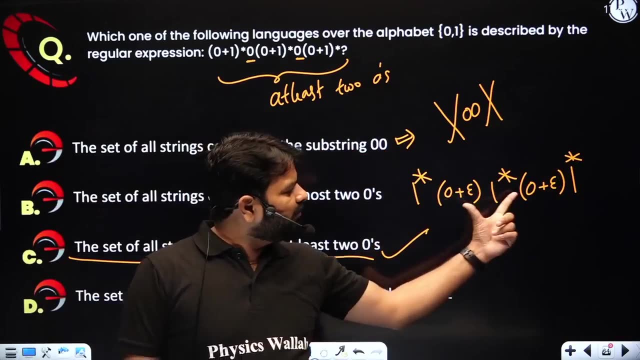 zero. so i'm going to keep at most one zero here, another zero here, at most one zero. so one can come any place. so i may write one star here, one star here, one star here. this will guarantee no zero. if you want to take epsilon, if you want one zero, any one of them, take one zero, other is epsilon you want. 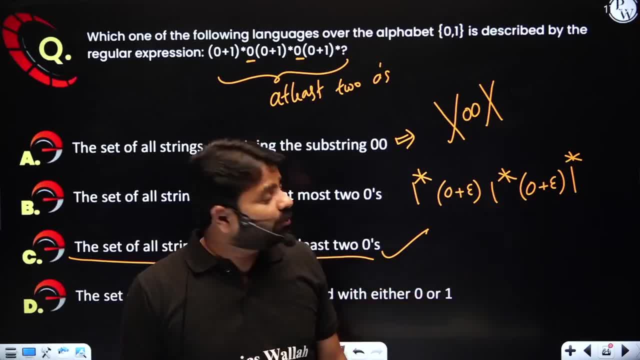 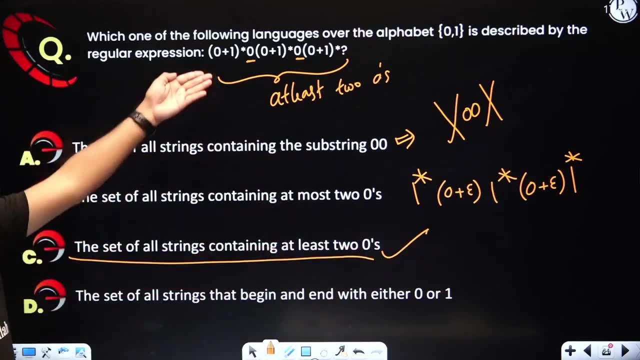 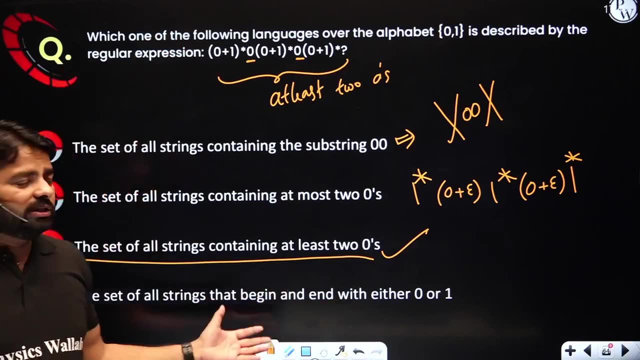 two zeros take, both of them are zeros. you want three zeros. impossible here, because maximum one zero, maximum one zero, it will guarantee at most two zeros. okay, containing at least two zeros is already covered. all since that begin and end with either zero or one. so this question, uh, you might think about it. begin with either zero or one and end with either. 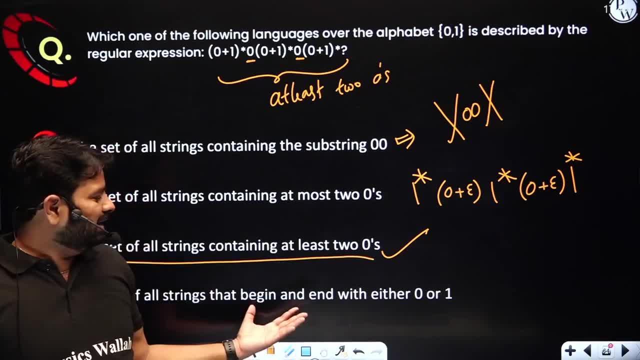 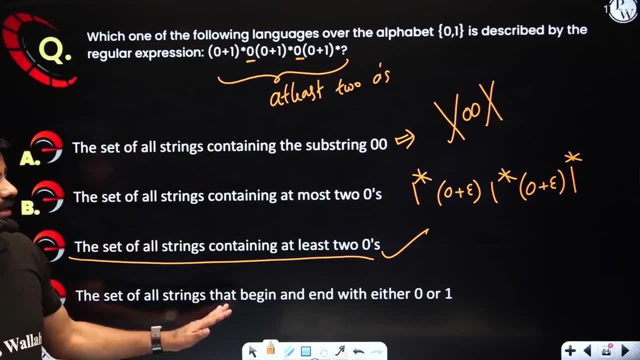 zero or one, which is: everything is possible, right there. is there any condition here: begin and end with either zero or one? anything is possible, right, except epsilon. everything is possible here, like zero plus one, whole plus. if you take, it will begin with zero or one or end with zero or one. 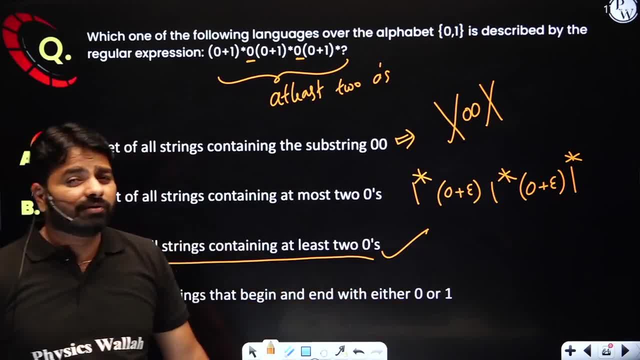 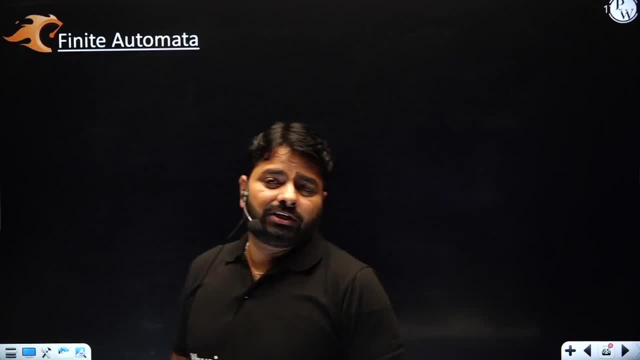 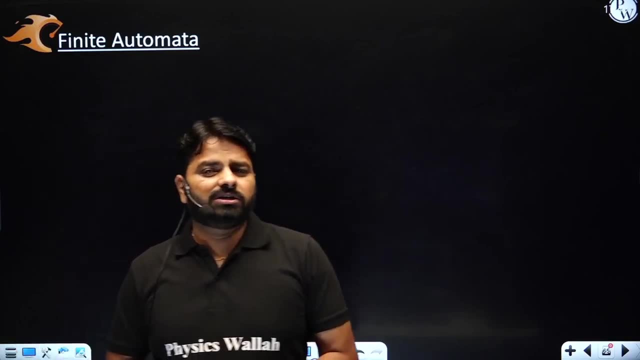 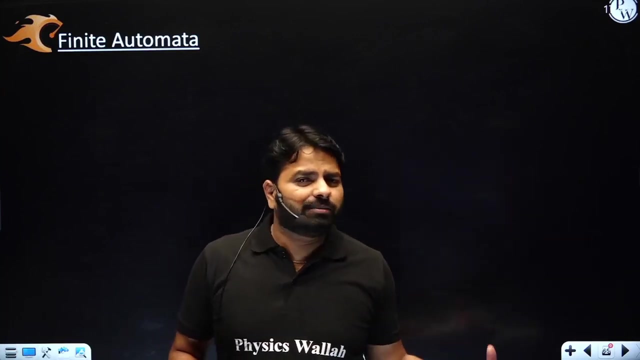 always except epsilon. everything is here, fine. zero plus one whole plus. okay. next topic is finite automata. in previous topic, regular expressions. i think almost all important questions are covered. uh, really, now you can go for the gate questions and try to practice it, because i've taken a lot of. 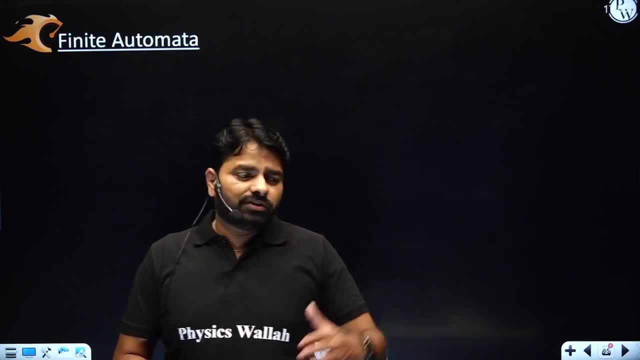 gate questions and a lot of new questions and a lot of questions which will help you to understand the all the concepts and the questions which will help you to understand the all the concepts, the all the concepts. now i hope you have understood various types of regular expressions. 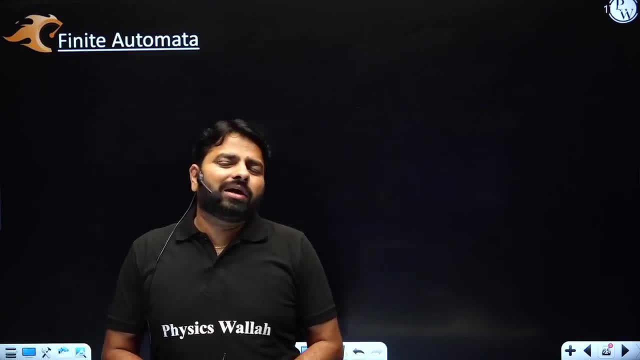 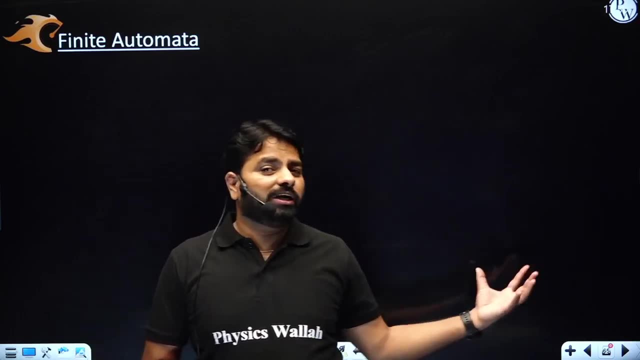 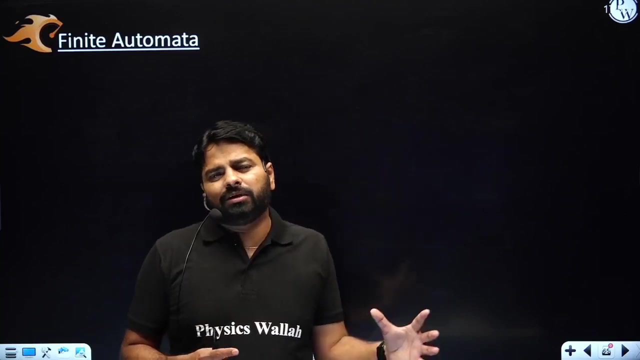 now, with this you will get an idea. what is a regular language? that means when i say the language is starting with a: oh, i have a regular expression, so it is a regular language. you should have that kind of opinion now. what is a regular language? have you understood them? have you seen them? 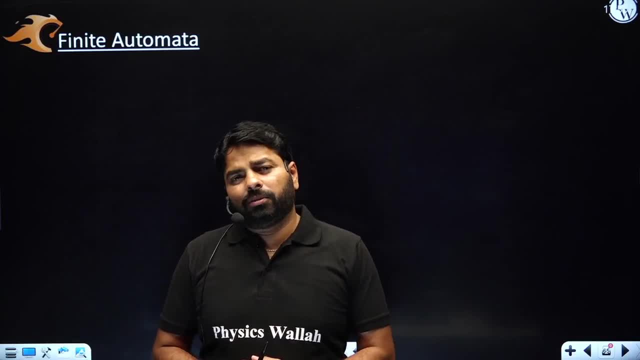 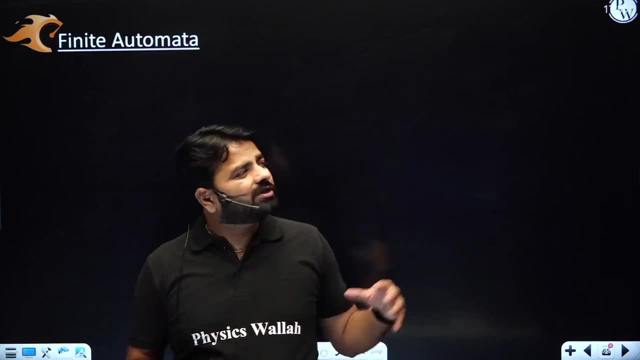 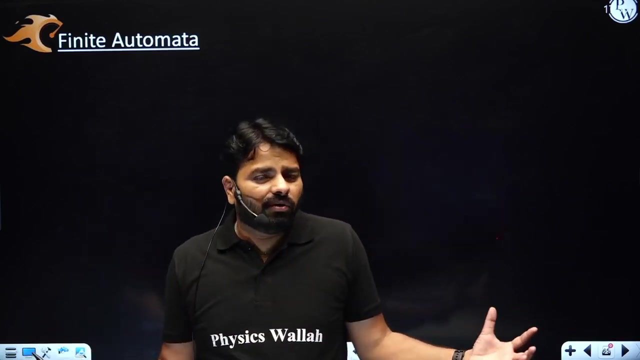 right. have you written them? yes, so many. but what you have not understood so far is: what is non-regular language? we can come up them after completing finite automata. what is non-regular language? because what is there if you know? what is regular language? if you know? 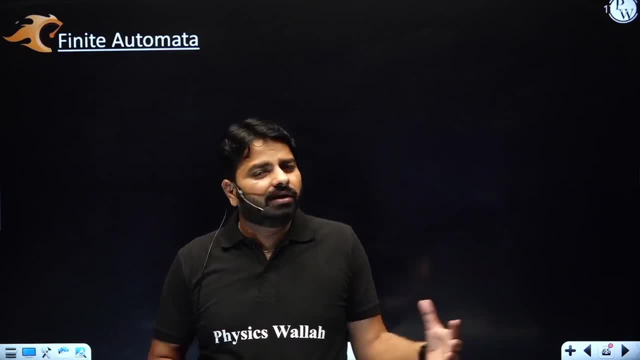 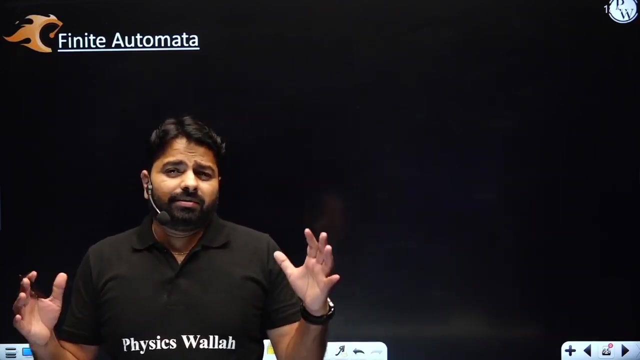 you can clearly understand later what is non-regular. okay, we are only try to learn right now what is regular, how better we can understand with various representations like regular expression, finite automata and, in future, regular grammar and so on. let's begin with finite automata. you know, the regular expression is the simplest. 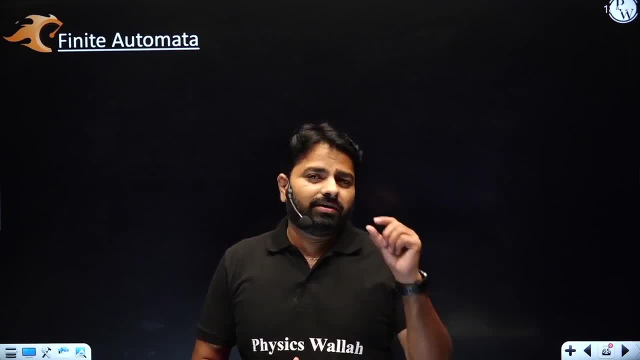 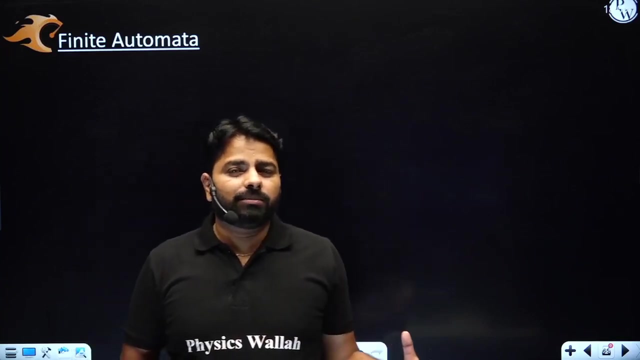 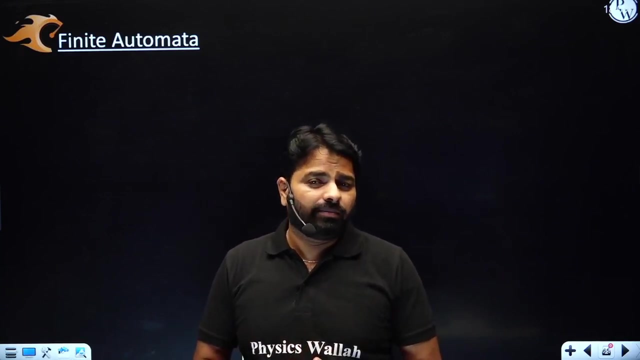 representation for representing a regular language. now we have another model to represent a regular language, which is finite automata. here you should have the models like deterministic and non-deterministic motions who are going to represent a regular language. you, to begin with. first you should know what is the automata, right first time we are dealing with. 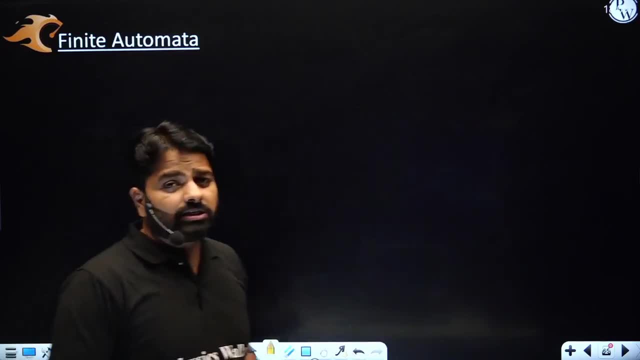 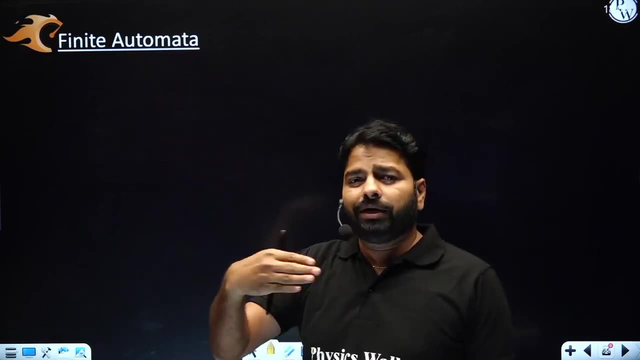 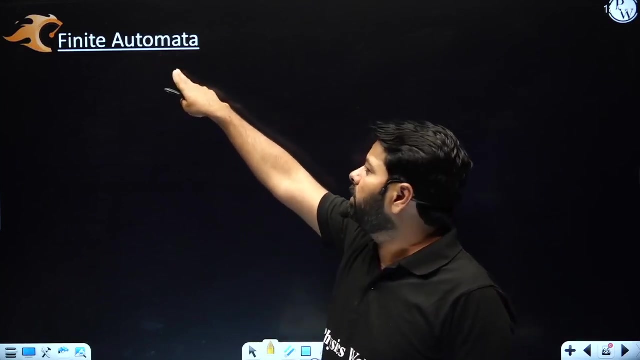 finite automata. so what is this? automata, which is a greek letter to represent the machines, like automata is a greek word which to represent machines. automaton is a single, uh, singular word to represent one machine, but automata can represent a singular or plural. where this automata? 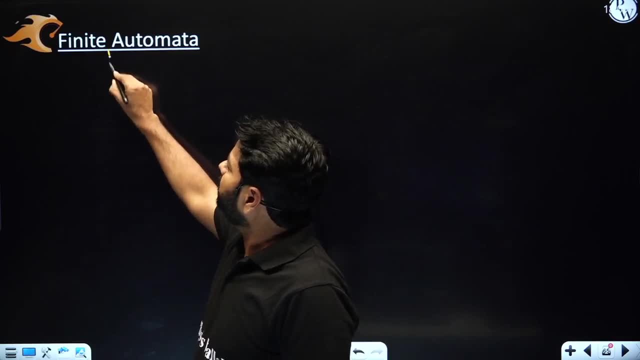 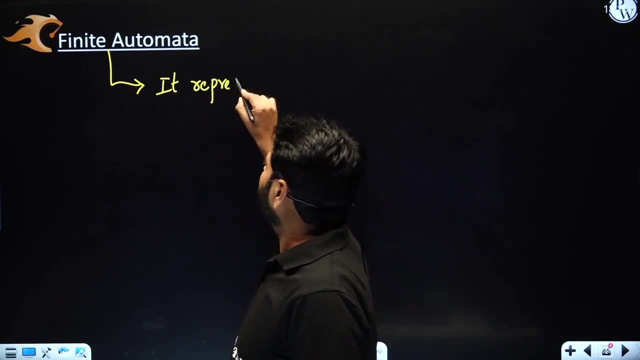 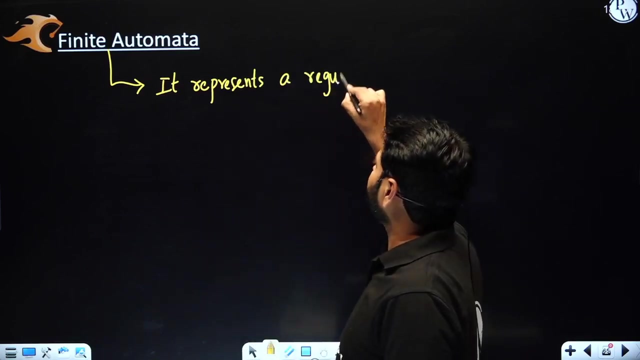 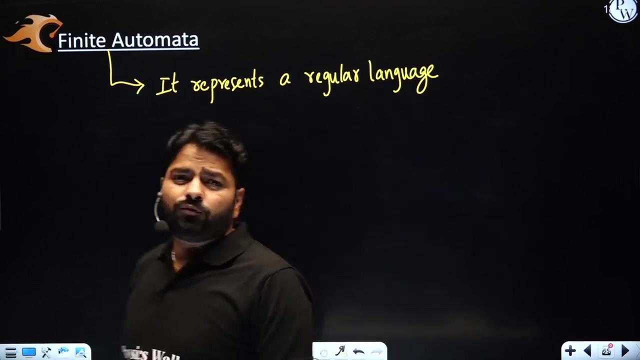 is a machine to represent a language. the finite automata is also a machine to represent a regular language. if you have a finite automata, that means you have a regular language, but how it represents a regular language, it's going to follow a definition and configuration which helps you to understand the various parameters, like whenever i say finite automata. 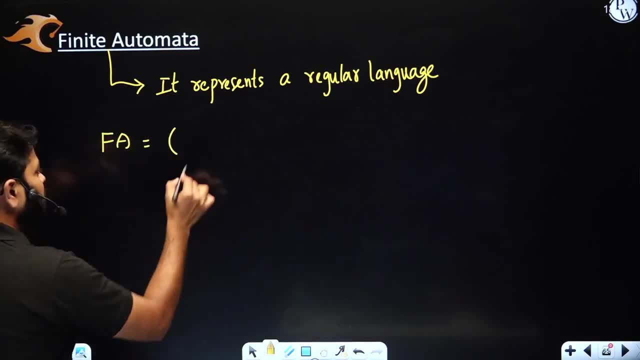 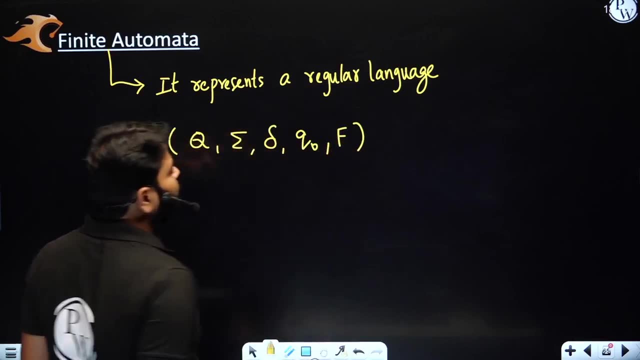 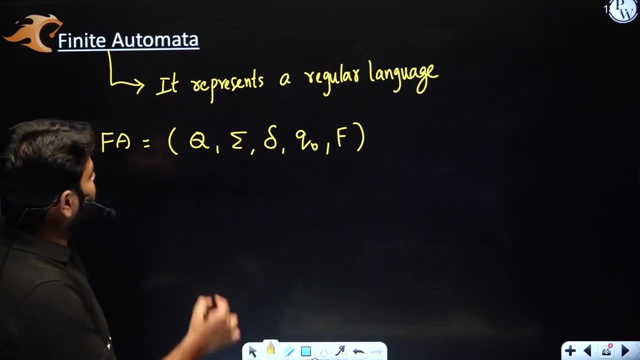 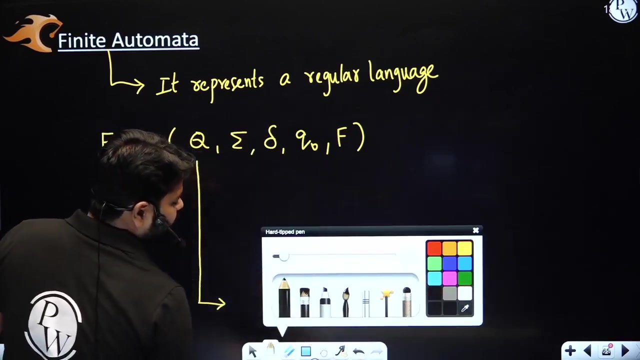 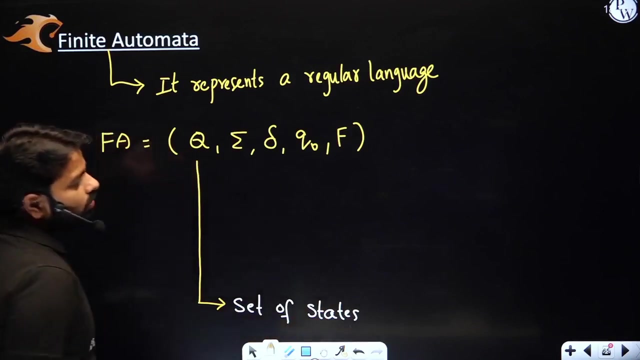 you will have set of parameters: q, sigma, delta, q, not f. these parameters will help you to understand the model. this model will represent a regular language. how it represents the q is basically what set of states. so you will have the states you want to know a particular machine? you can see i'm just drawing a machine here. 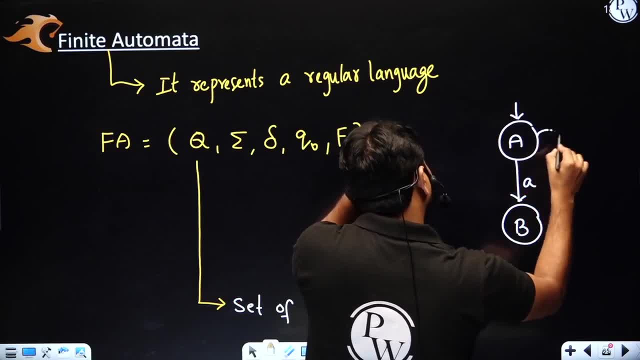 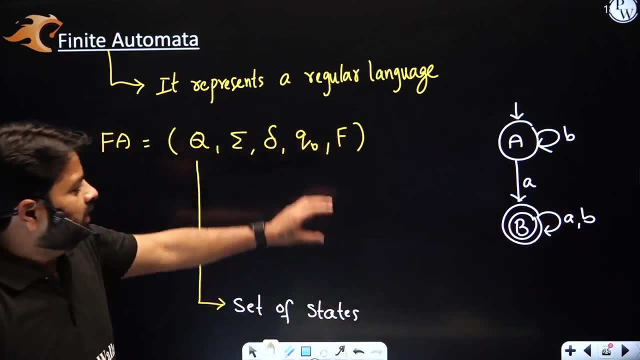 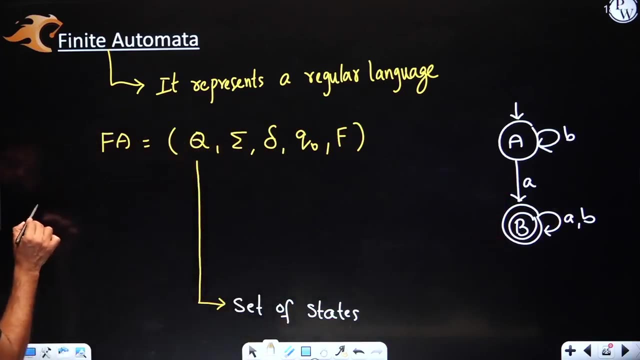 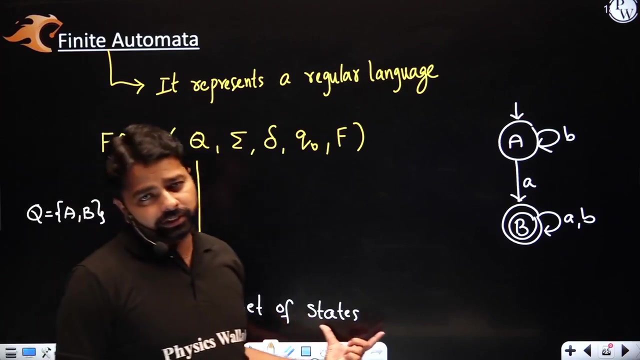 don't worry. what is it? you don't need to worry about it. okay, some machine here. every circle represent a state. how many states are there? two states? so somebody can say q is nothing but two states. set of states. right, this set will have two states. so set of states. how many states must be finite? you can't have infinite number of states. 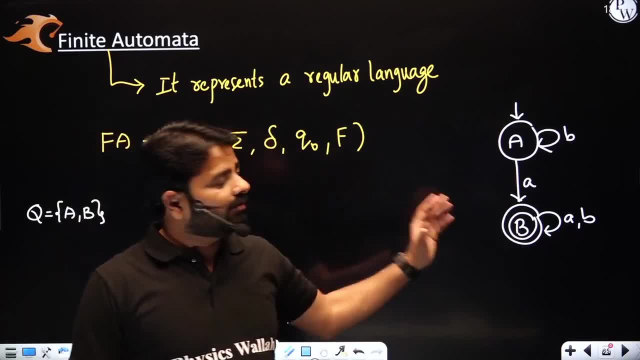 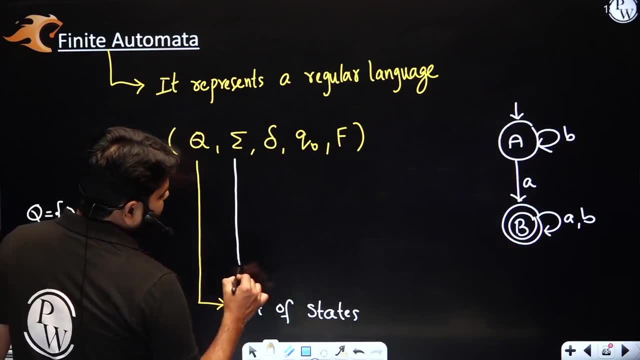 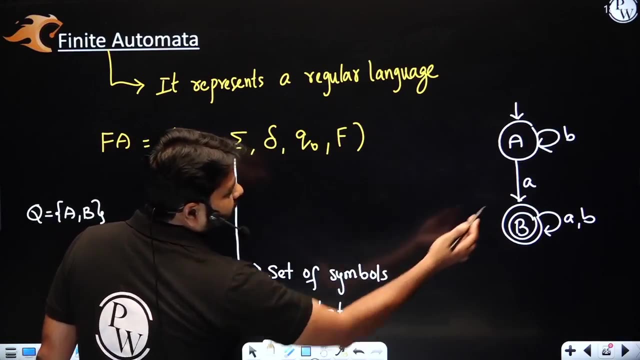 in the diagram, right in the graph or in the diagram. you can't have infinite number of circles. you should have definite number of circles to understand the problem. but sigma, this is that of symbols. it's nothing but alphabet. then what are the symbols here? small a and small b. that sigma is alphabet. it's nothing but a comma b. 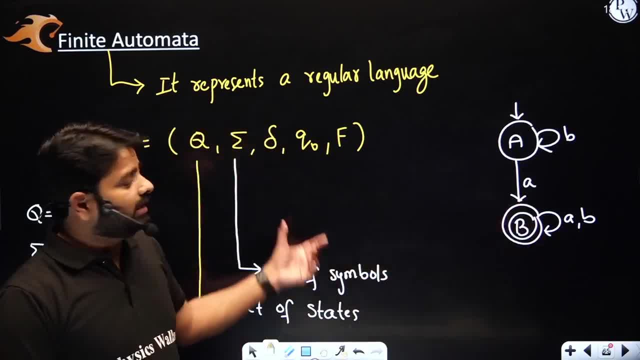 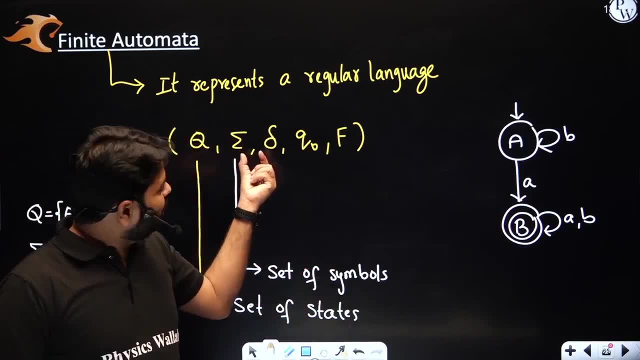 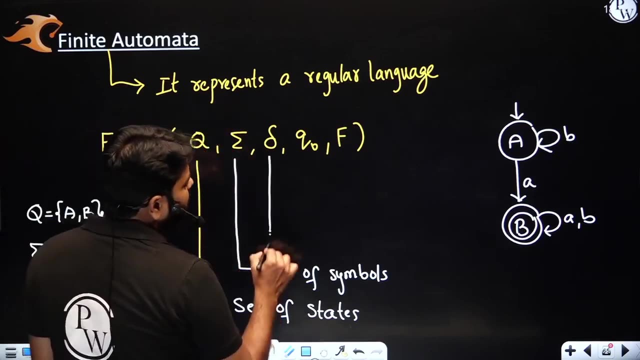 and what is delta? that's what you require to understand this. delta takes time to know the definition of a dfa, nfa, and this is going to help us to know about the different types of machines in finite automata. so it's just now. i can call it as transition function. 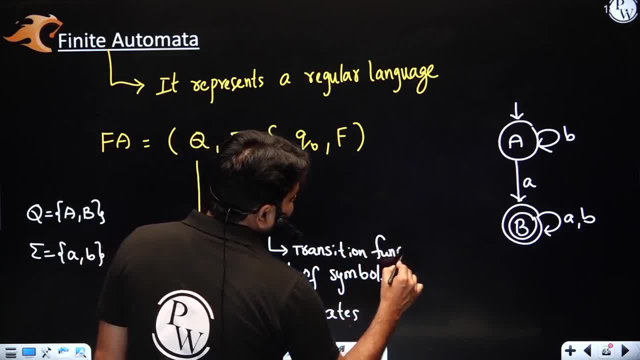 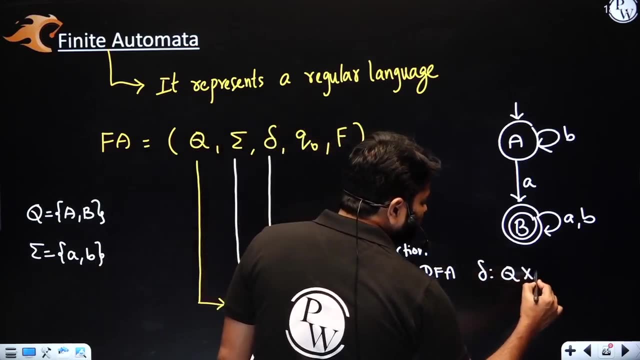 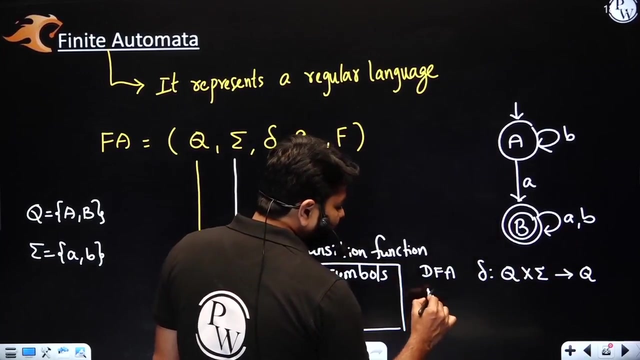 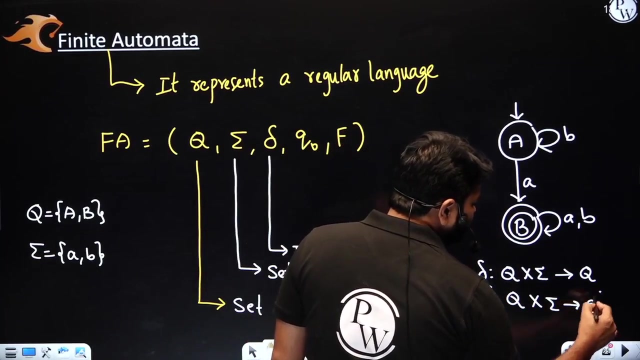 but what is the transition function? what is the transition function here? delta for dfa. for dfa delta is q sigma, which is a contingent product of q sigma, well mapped to q, whereas nfa delta is two cross sigma that maps to 2 power q. this is without epsilon. there is another nfa with epsilon, that will be: 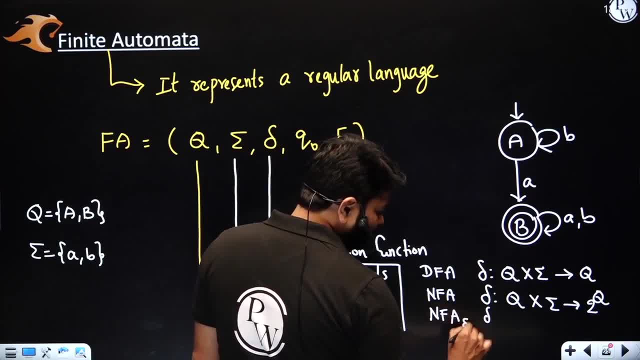 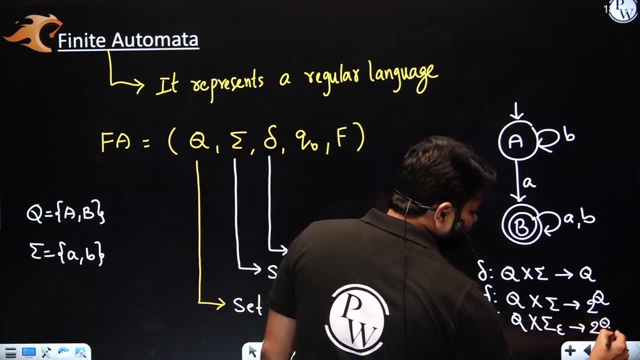 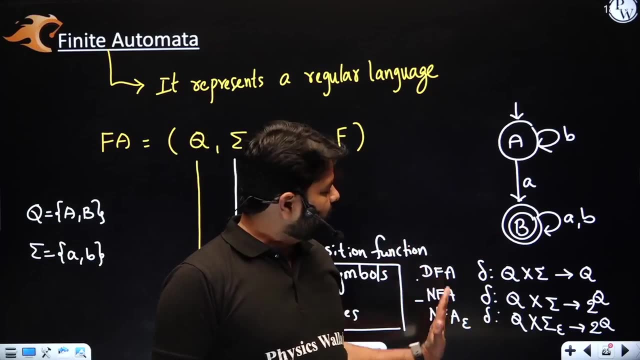 i'll just write nfa again, but with epsilon moves. q cross sigma. along with epsilon it maps to 2 power q. there is no much difference between nfa without epsilon. with epsilon moves and the various types of machines in finite automata. each one mapping will be different, like the first one is. 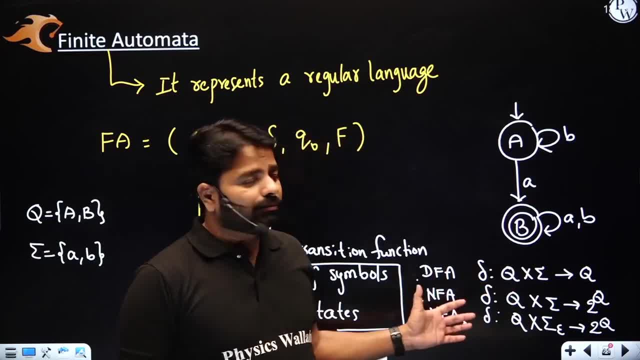 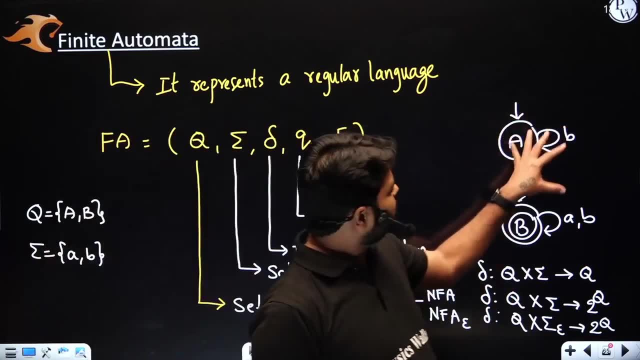 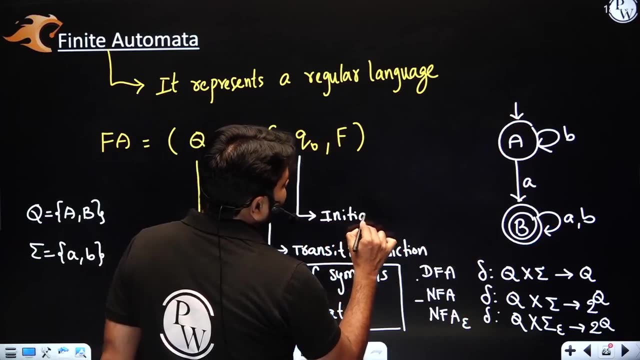 deterministic mapping. the two are non-deterministic, so we'll see them slowly. okay, q naught is every motion. every motion has the initial state. every dfa has initial state, every nfa has initial state. okay, so q naught is initial state or starting state, and remember that this q naught is here a. 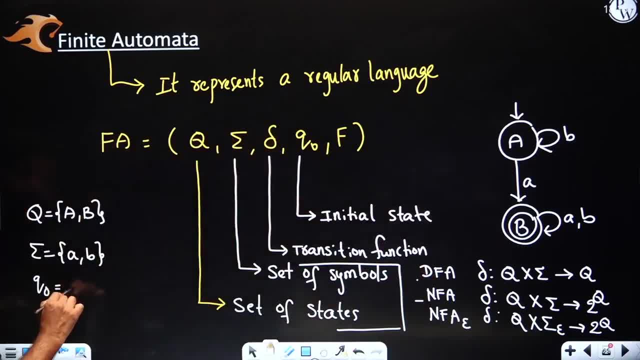 q naught is what a and this must belongs to one of the state in the q. okay, only if you ask me: what is q naught? q naught is belongs to q only is one of the state in the. q is acts as initial state. and what is f? don't suggest final state. it could be zero or more. 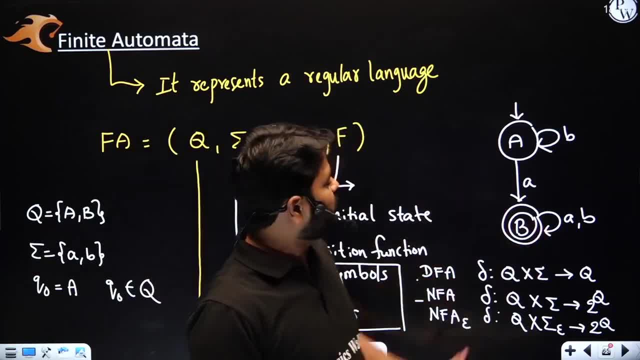 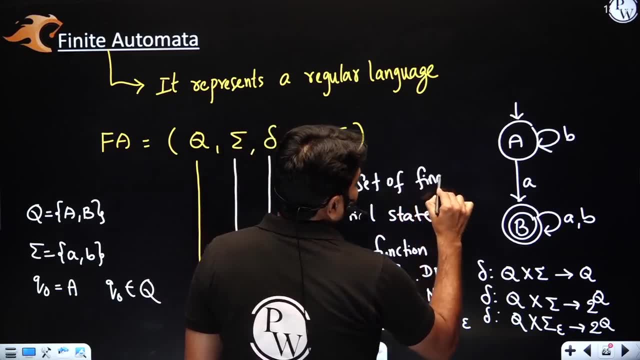 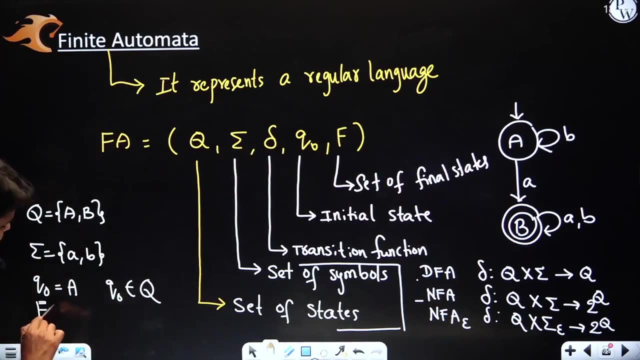 final state. sometimes no final state might present in the machine right, so set of final states could be zero or more. that is the meaning set of final states here. how many final states are there? only one. so you may say that f is here, what is it? b? that's why you'll represent in the set, because 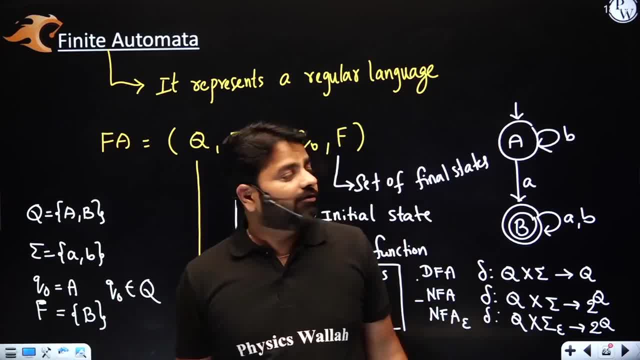 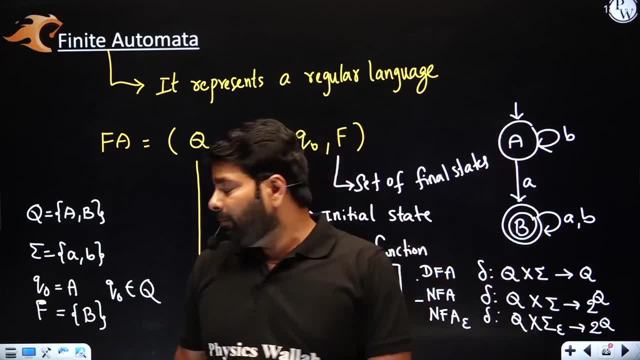 sometimes no final state. you must represent empty set here. if you have more than one, let's say a and b, both are final- then you have to write a comma b here. so depends on how many finals are there in the machine and that many states you must write in the set. fine, this is how you write, or you? 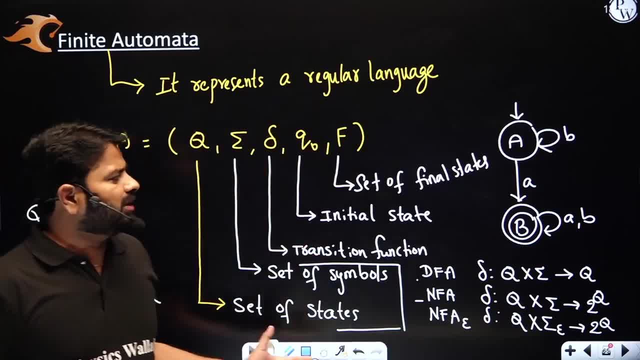 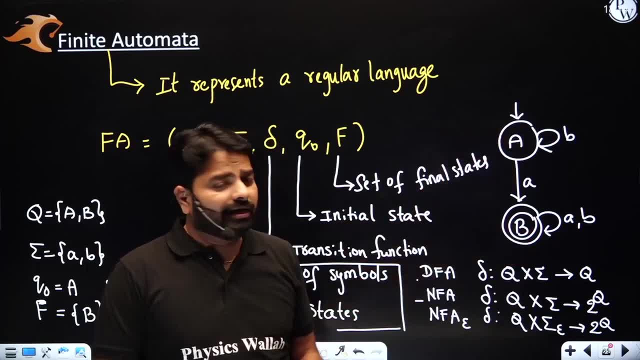 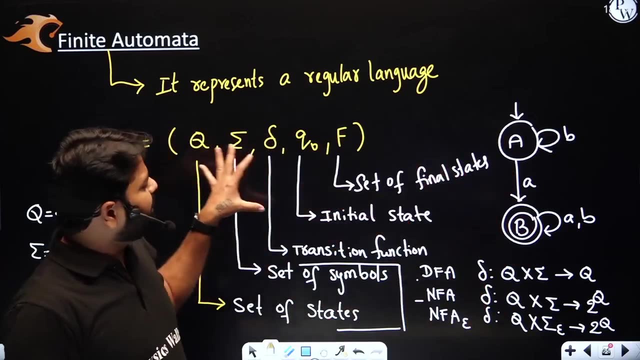 represent the finite automata and how this machine reads basically, right, i have just drawn the diagram but maybe you don't understand now as i have not explained clearly how to read the strings in the machine. to understand this first, how this is configured with this: five parameters. okay, how? 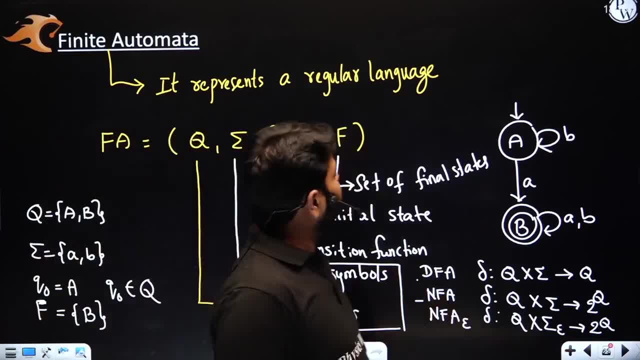 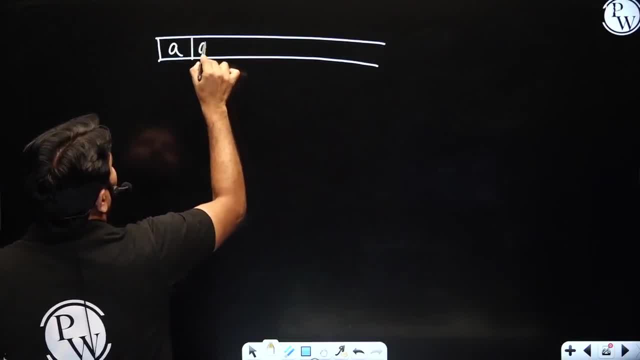 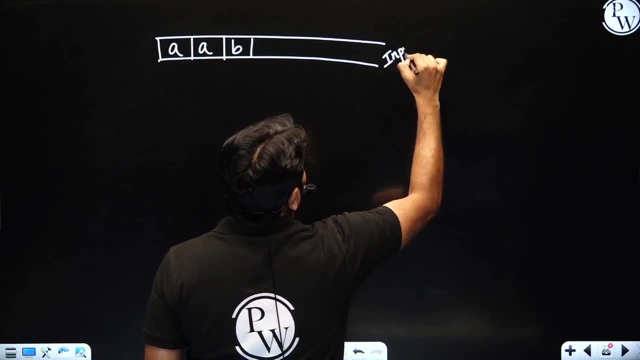 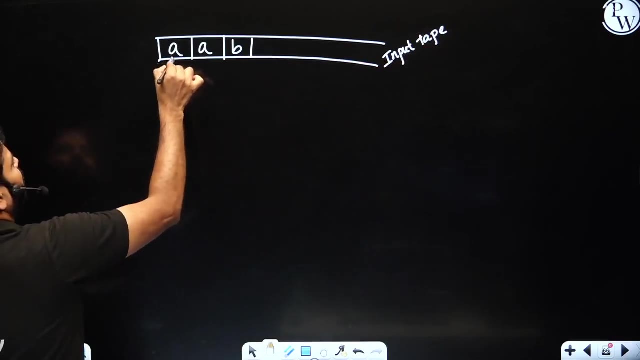 this is configured. let me explain with some diagram configuration. now your input will be here somehow, like i'm just reading, let's say a, a, b is a string and this is called as input a. as you are reading input symbols, you may call it as input tape. now you will be having some pointer or head to read. 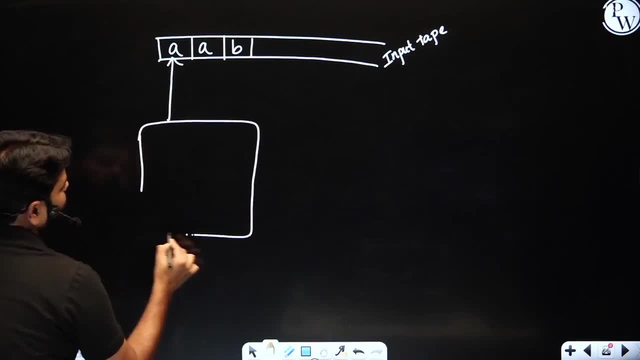 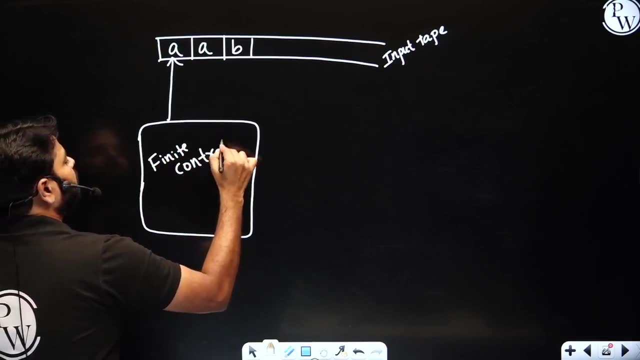 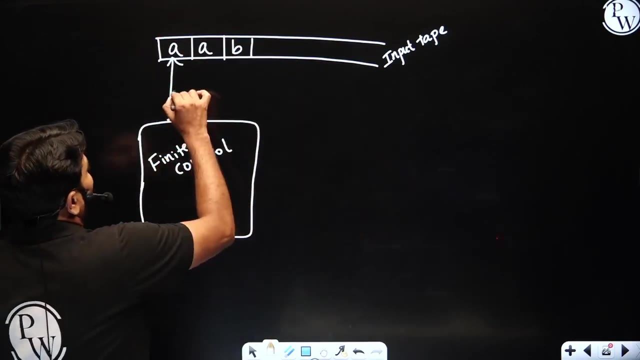 the symbol every time and your control is here. this is, you may call it as finite control. where have all algorithm or program here? now, what is the job of one? this whole thing represents a finite automata. well, you just call it as read pointer or read head. 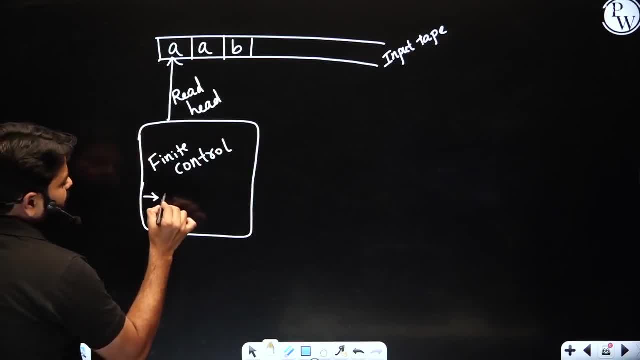 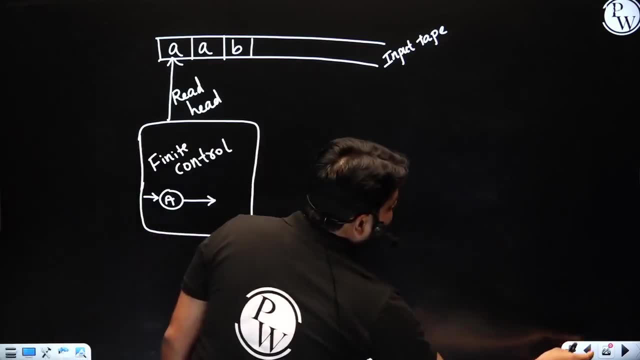 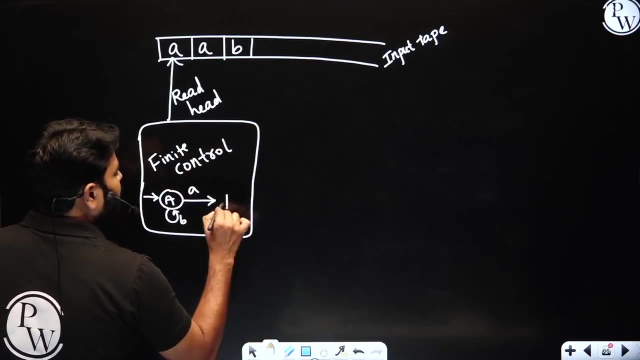 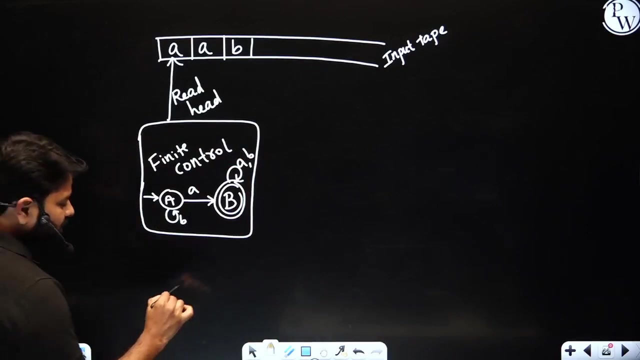 okay, now you may have you know machine here. let's say a, let me see the diagram, what you have, b, a, some diagram you have here. so what happens in this initial state is a and what is the current input symbol that you have under the head a. so in this motion you are going to run each input symbol at a time: a on a, you will move to b. 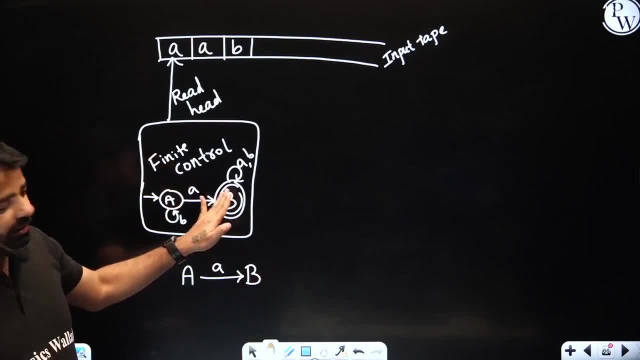 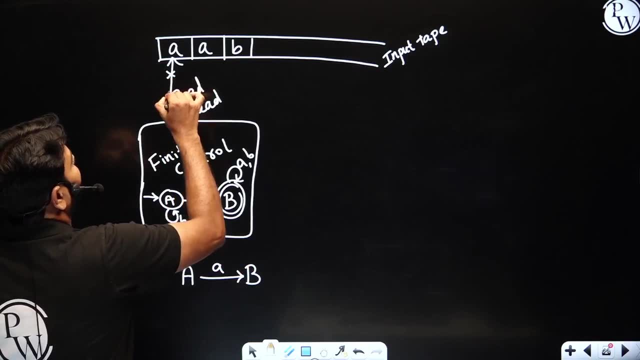 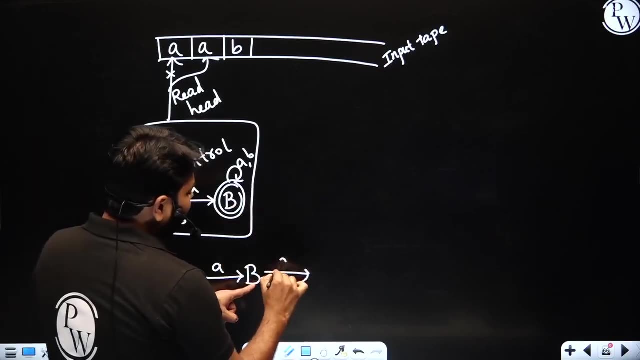 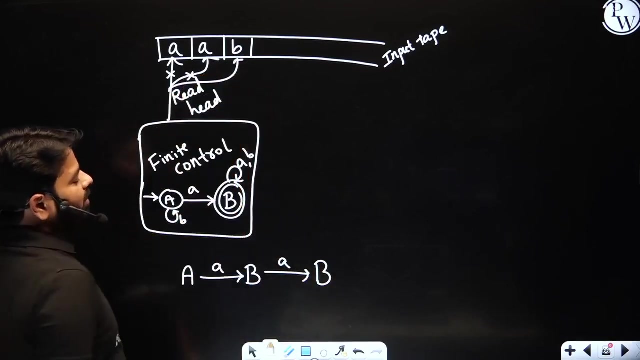 now current state is here. b current state is what b now. now a is already read, so the head pointer, it will move here. then next symbol is also a. now current state is b. from b. by reading a it will be in the same state b and after that this head will move here and from b again you will read b. 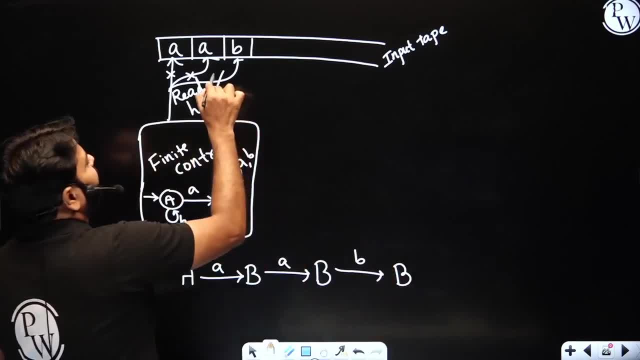 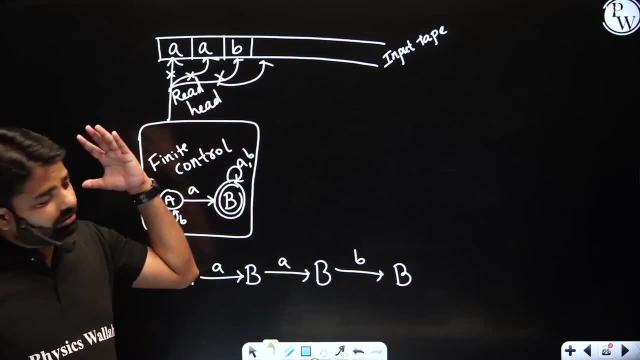 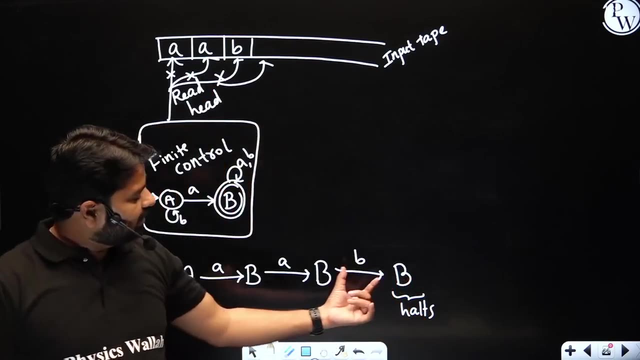 and you will be at b and its head is completed reading it right now. what happens? the machine halts, has nothing to read. next it halts. it halts at this state. whatever it is, doesn't matter, it halts now. this state is b is. is this b final or non-final? that depends on what circle you have. 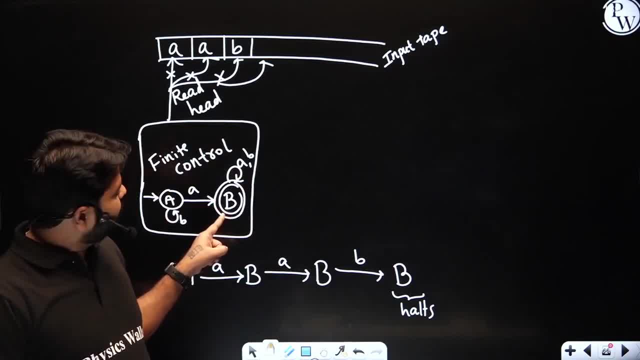 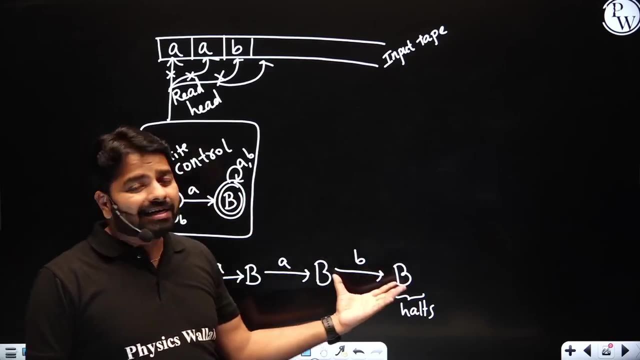 single circle or double circle. if you have double circles then you will say final state: as mentioned in the previous one, f is having only b because b is the final state. so double circles represents the final state. and if you halted double circle- one of the double circle- in the machine, then that string is valid. 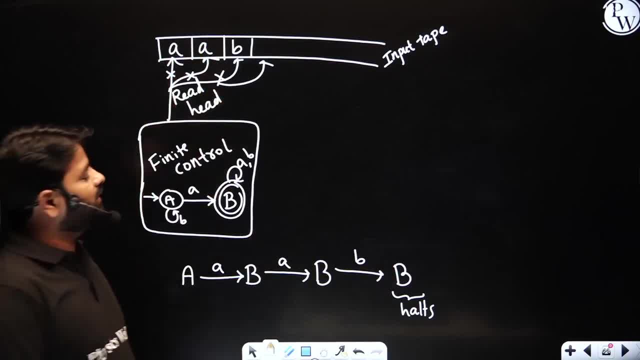 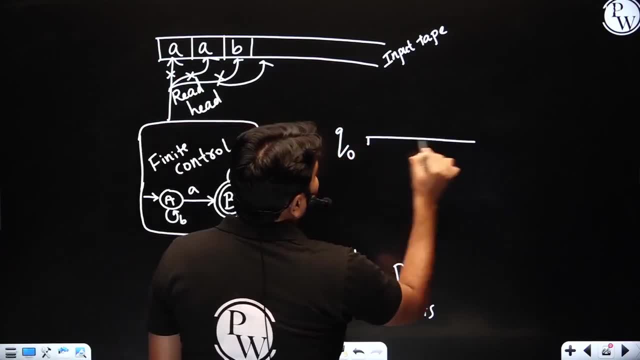 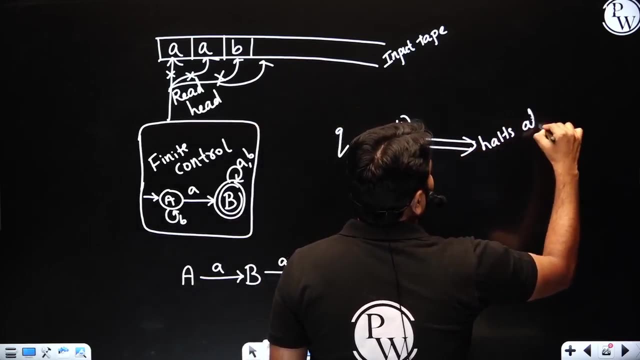 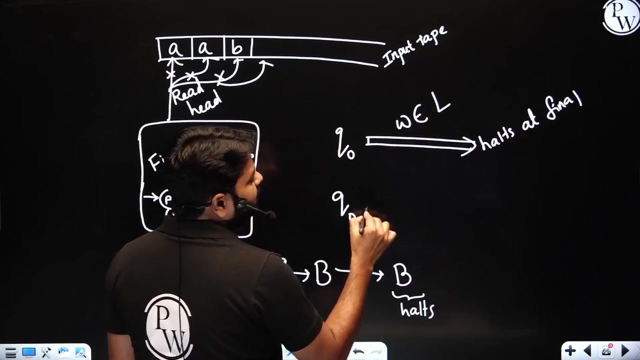 so this a, a, b is valid string. that is the reason. from initial state, from initial state, let's say: a is initial state. right, q naught. q naught after reading the string, after reading the w, if you halt at final, halts at final, that means w is belongs to, l suppose by reading the string. if you don't. 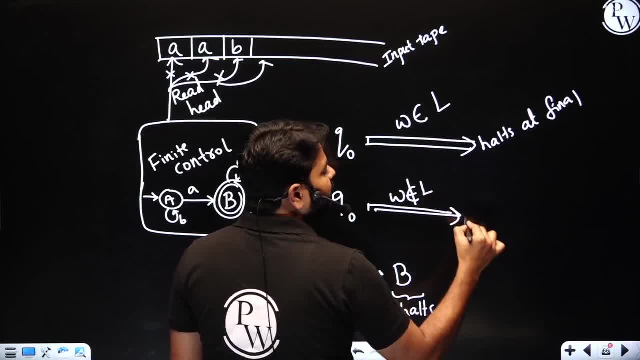 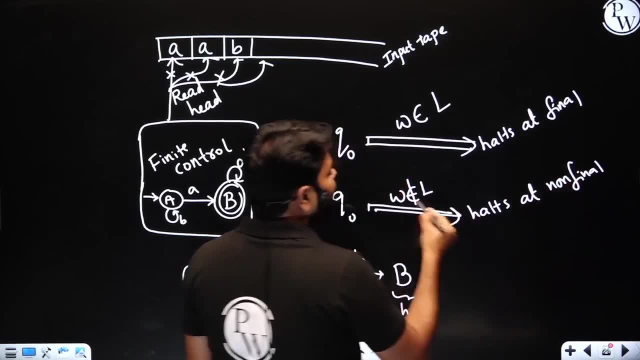 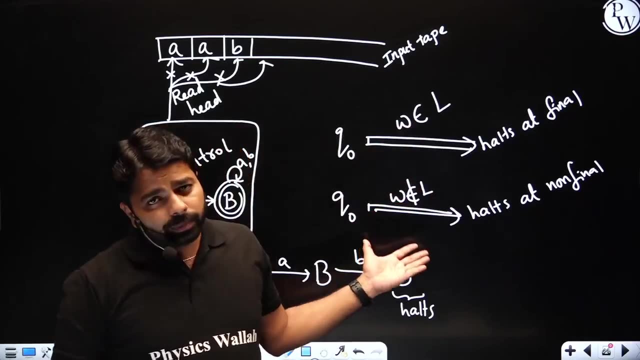 halt at final. if you don't halt at final, that means halting at non-final, halts at non-final, then the string is invalid. so there are two types of strings in the world. one might present in the language, one might not present in the language. if it is present in your language, it must halt at final. if it is not present, 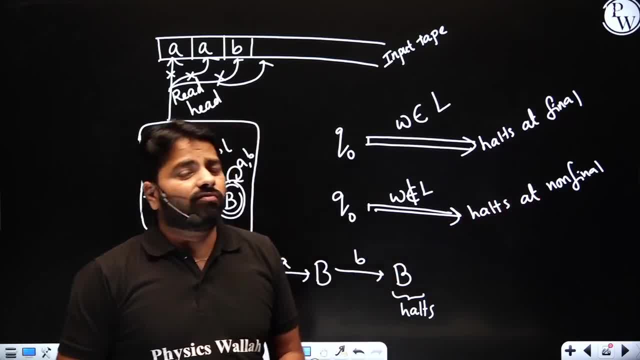 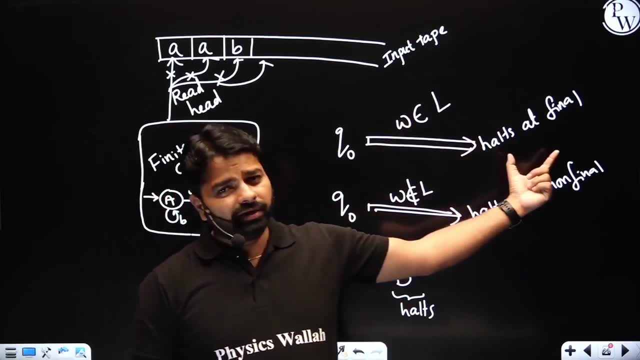 in the language, it should halt at non-final. so this is the behavior of finite automata. so finite automata either accepts the string or rejects the string. if it accepts, it should halt at final. if it is not accepting, it should halt at non-final. so when you design a machine like 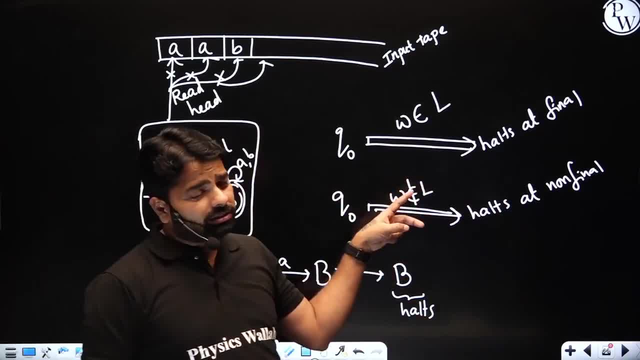 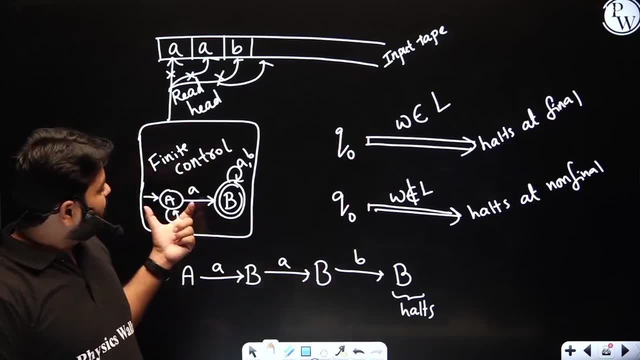 deterministic machines. you must think about these two possibilities. are you halting at a final state for your valid strings? then you should design such a way that you first design such a way that you, for every valid string, you should halt at final if the string is invalid. you should try to ensure. 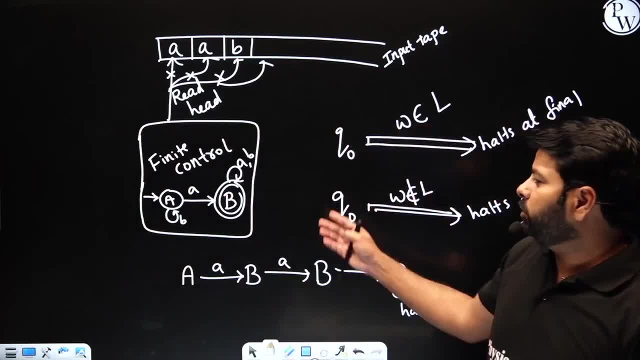 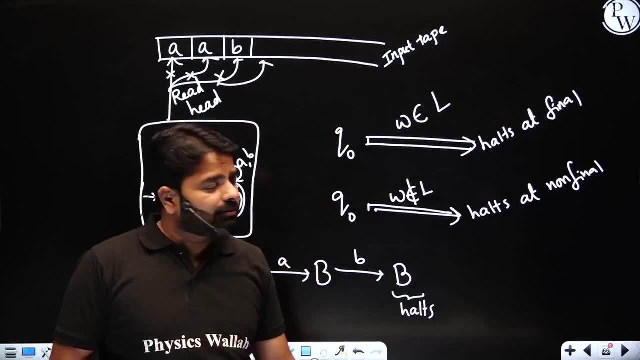 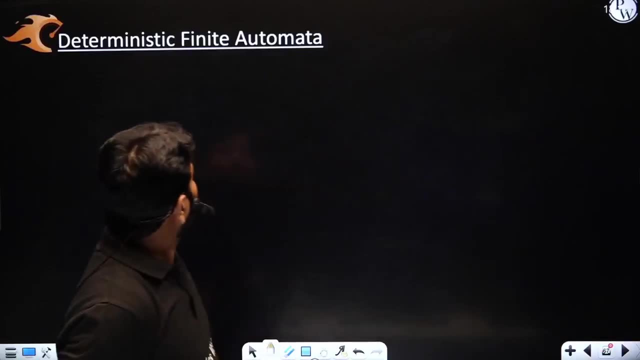 that you will halt at non-final right. so this is how you check about deterministic finite automata. now fine, uh, we have uh deterministic and non-deterministic types. let's move on to to understand the behavior of these machines. deterministic finite automata: first, we will focus on dfa rather than nfa- other things. 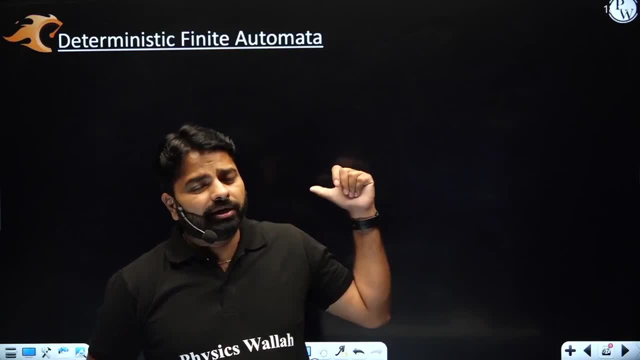 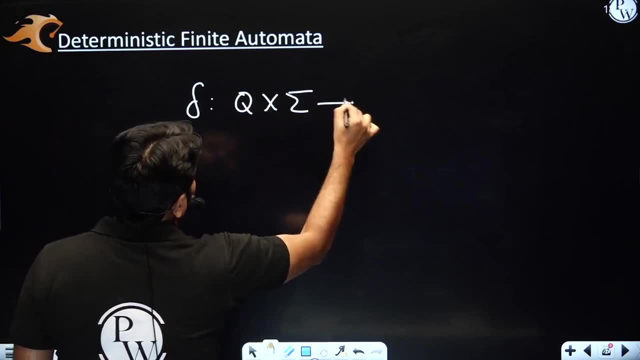 we have two types of machines: dfa and nfa in the finite automata. what is deterministic finite automata when you have dfa? so look at here. this is the main important transition function which will help you to understand what is dfa. dfa says that whenever you design a machine, 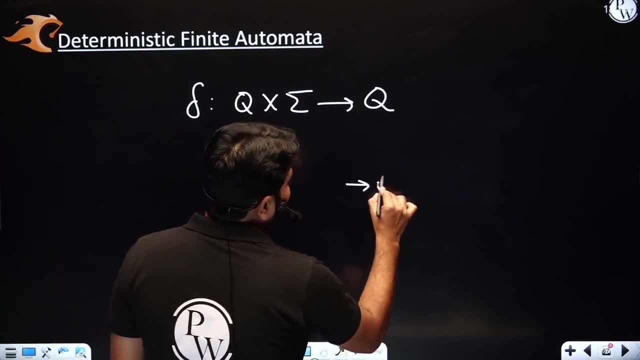 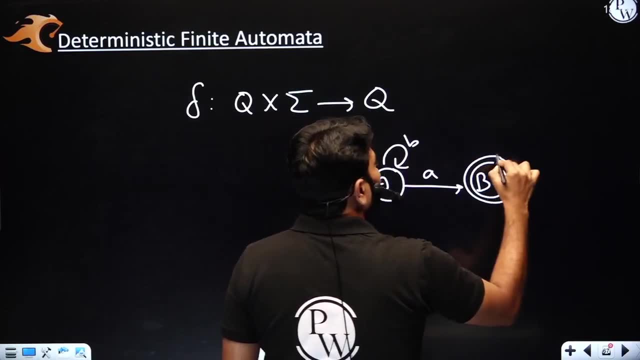 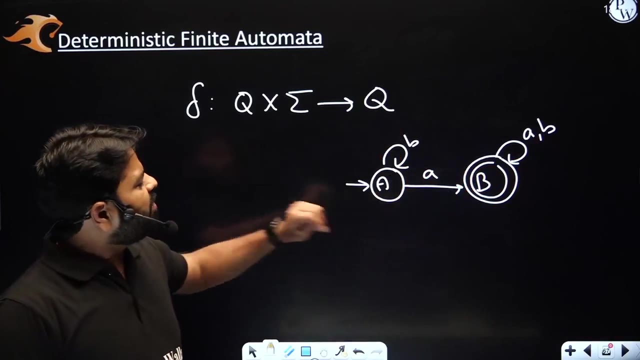 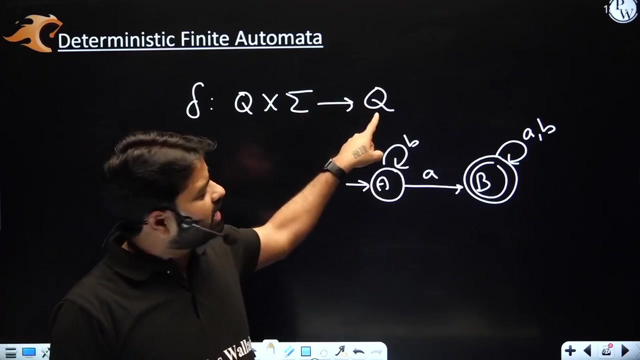 look at that previous example that i have taken right. okay, don't worry if i draw a different machine. that's okay, i have some motion here, right? how do i know it is deterministic or not? if it is deterministic, machine from every state, like this is every state in the queue, every symbol in the sigma you must have. 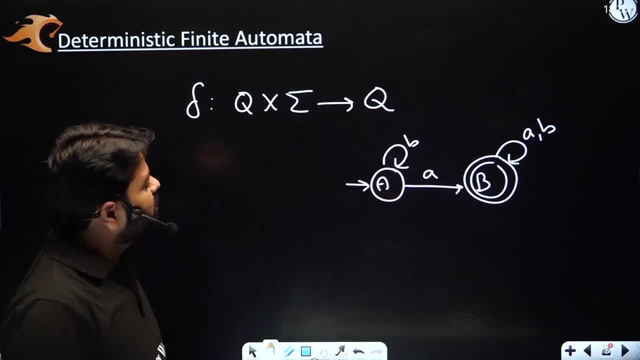 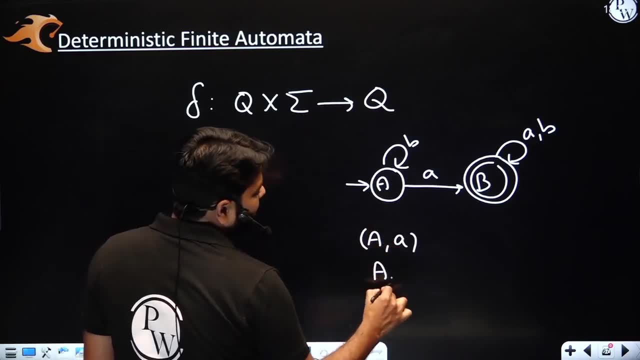 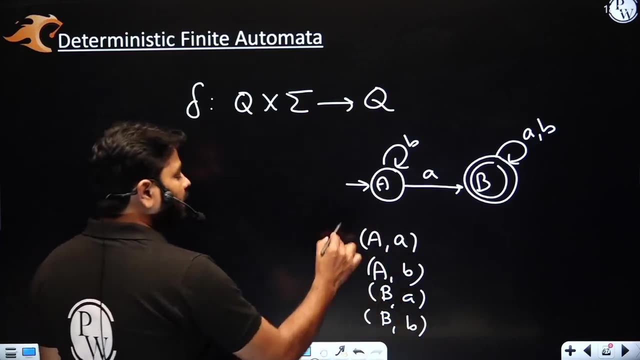 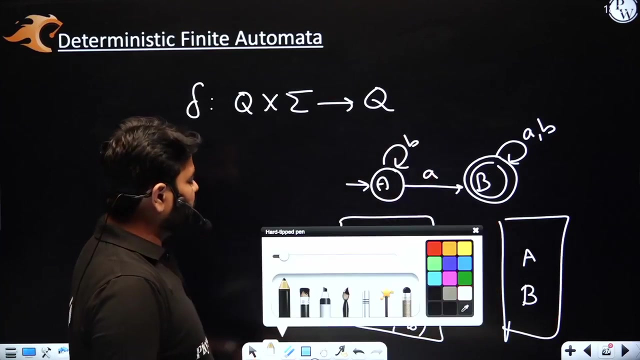 a transition in the queue: mapping: mapping. so here you can see q cross sigma means from a comma a, that's one combination, and a comma b, b comma a, b comma b. this is your domain, the q cross sigma, and from here you should map to q. what is q here? a and b. now you think about what are the mappings. 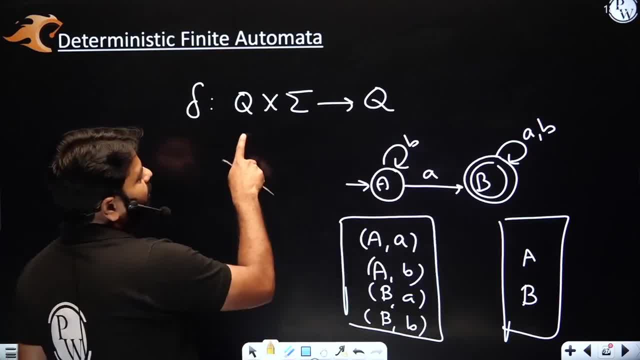 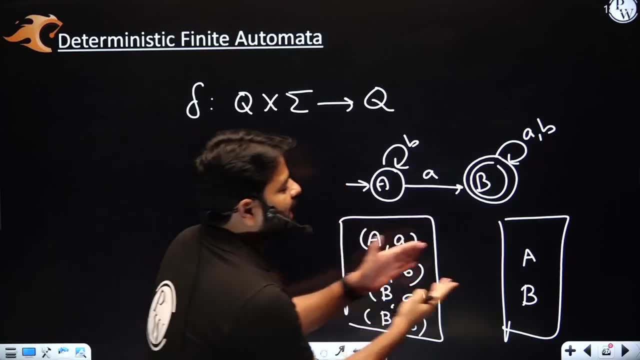 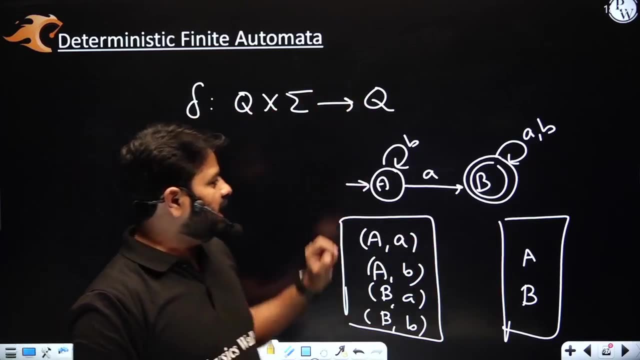 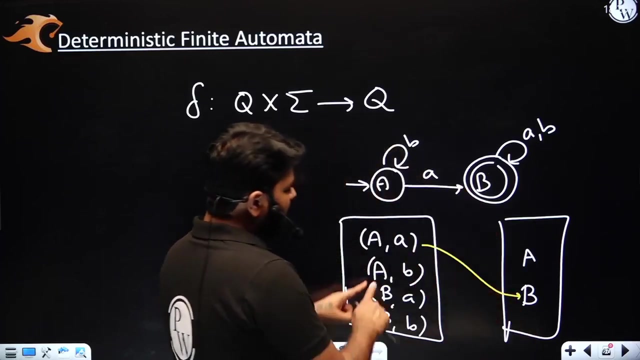 you have from q, every state in the q and every symbol in the sigma. you should have exactly one mapping, one transition here as per the this definition. exactly one mapping as per this diagram. exactly one transition now. see: a comma a: it goes to b, so it goes to b. a comma b: it goes to a. see that you have exactly one mapping, also exactly one. 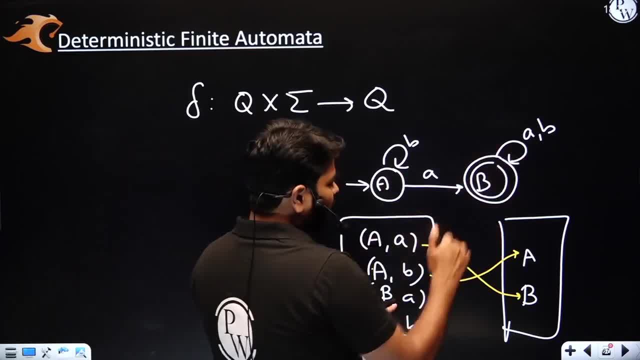 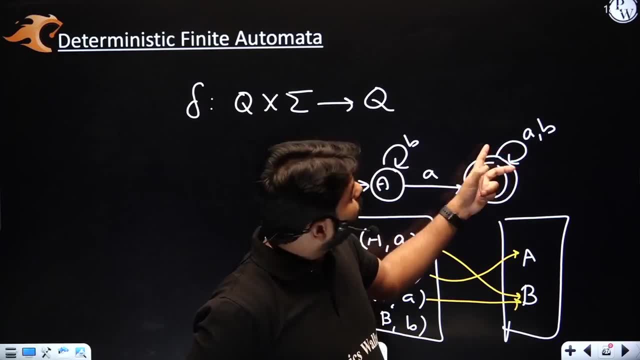 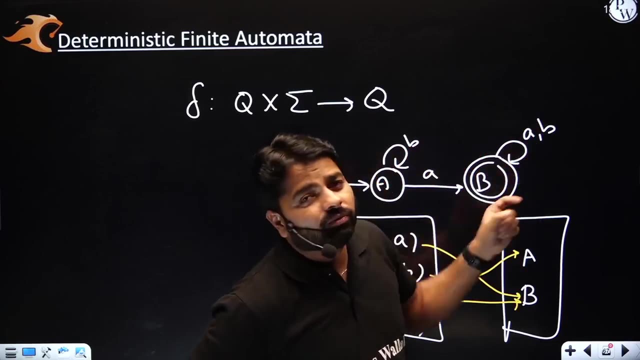 transition somehow, b comma a, exactly one transition. and b comma b. oh, here i might pretend, the one edge, but it's two transitions. remember, it's not one transition: a, you have one, b, you have one. two transitions. we have represented in short form with one edge. so here, if anybody ask how many, 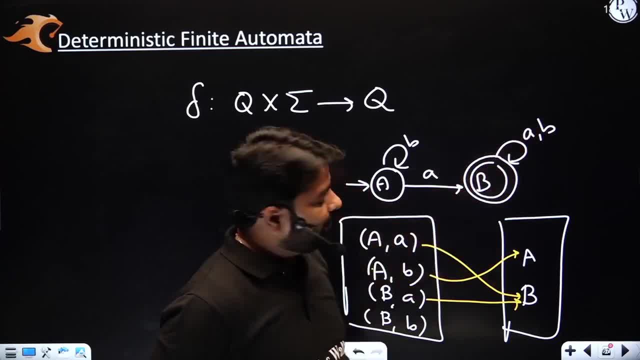 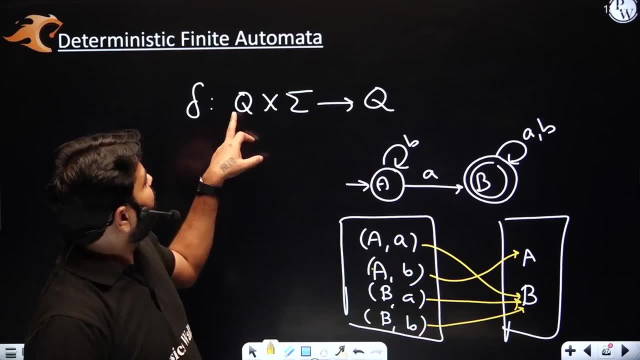 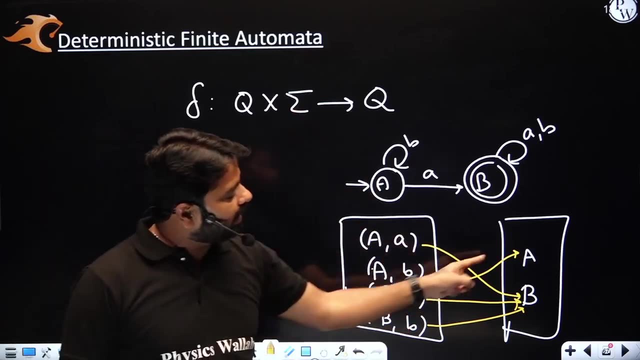 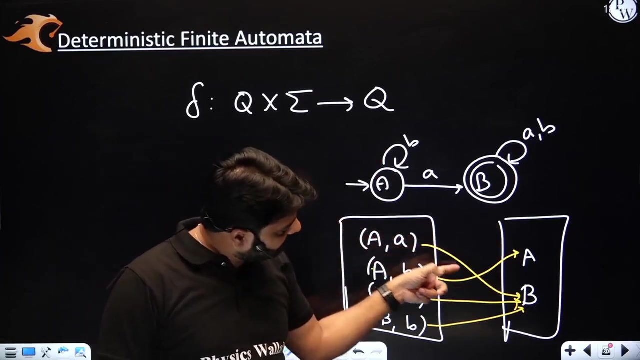 transitions here, not one, it's two, one for a, one for b. okay, and b comma. b is goes to b. only now look at, is the definition very clear. from every state, for every input symbol, there is exactly one mapping that goes to one of the state in the queue. right, exactly one. from this you have exactly one transition, right. 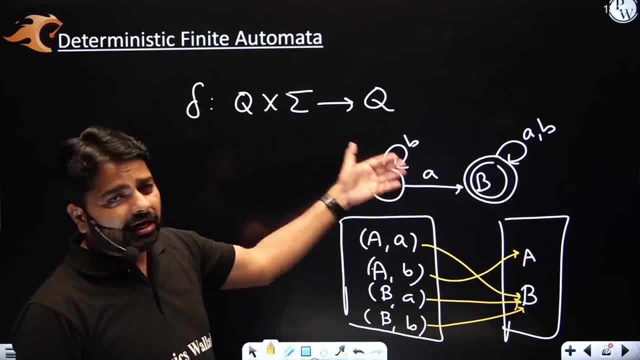 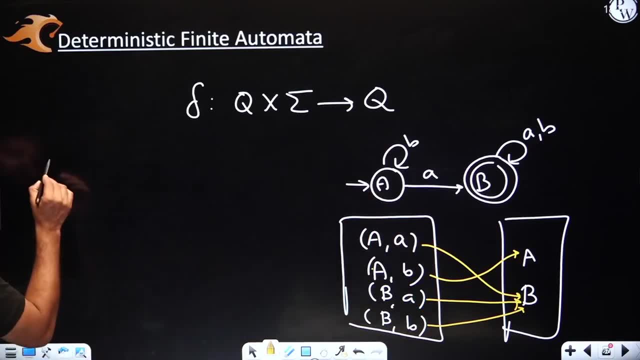 and the two exactly one mapping in the diagram- one transition in the function, one mapping. and the two exactly one mapping in the diagram- one transition in the function, one mapping. somehow they are correlated here. now, what is the definition of this dfa? very simple, if you, if you want to find the definition, just remember this from each state: 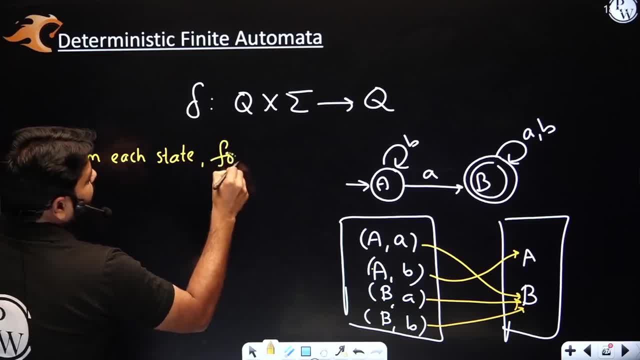 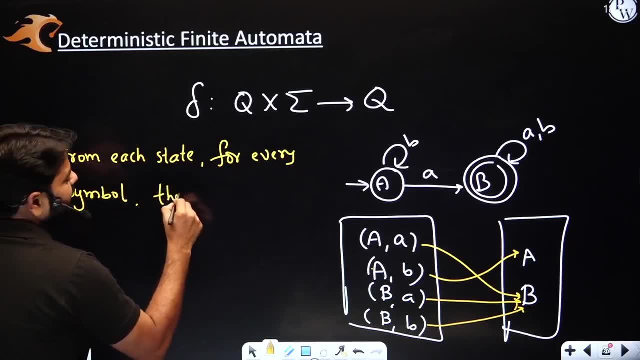 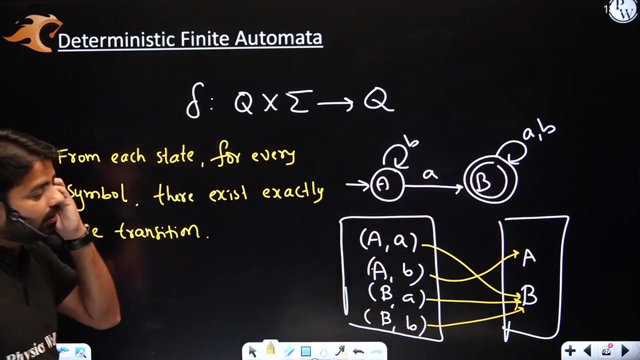 in the dfa for every transition or for every symbol. for every symbol, there exists exactly one transition, there exists exactly one transition. there exists exactly transition, there is exactly transition, exactly one transition. exactly one transition goes to the next state. this is complete definition of dfa as per the delta. 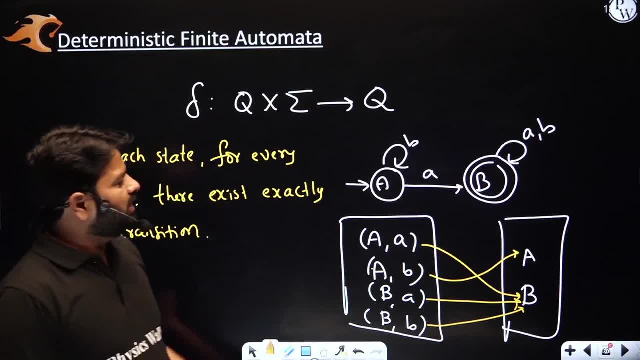 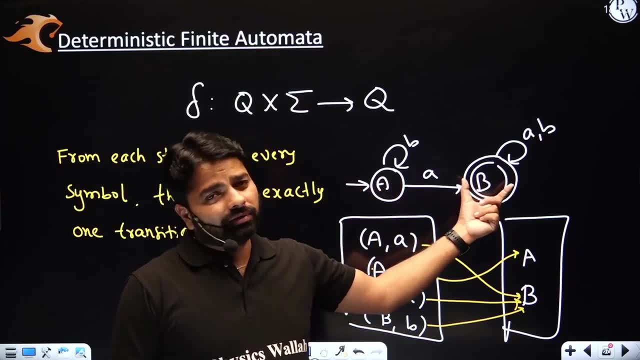 representation. once you remember this, everything will be easy. suppose you have two states, how many transitions for this state? you have two transitions for this state. you have two transactions. total four transactions. will see, that's why you got four here. the number of transitions always same as q cross sigma. 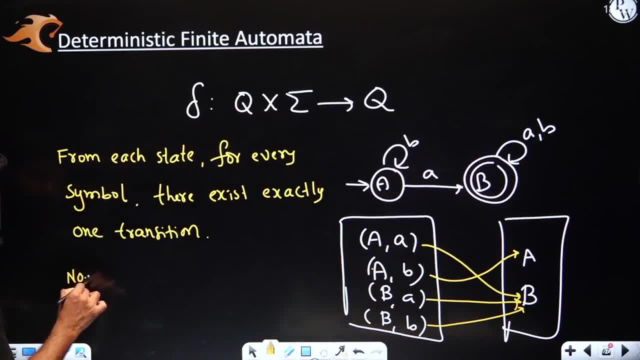 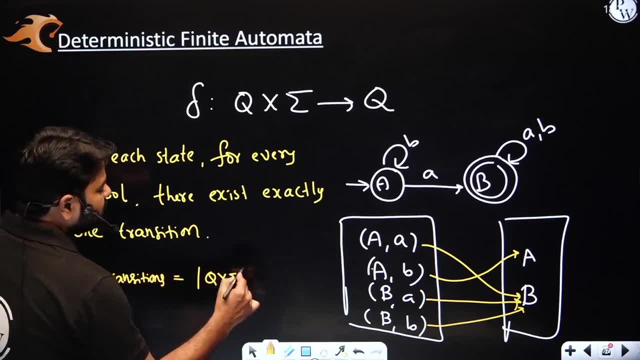 if anybody asks how many transitions in dfa, number of transitions that you see is definitely equal to size of q cross sigma, which is same as delta. right, that's? size of the function is same as size of domain, if you aware of it. okay, number of transitions always matches with this. 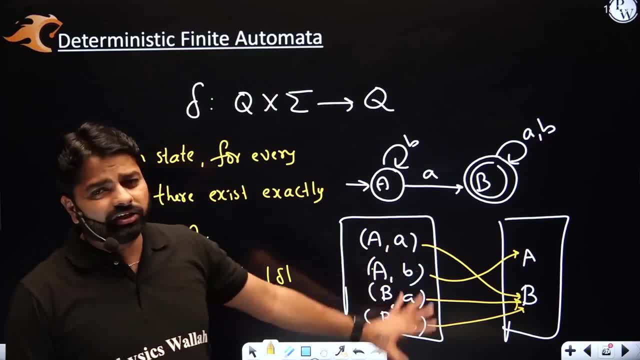 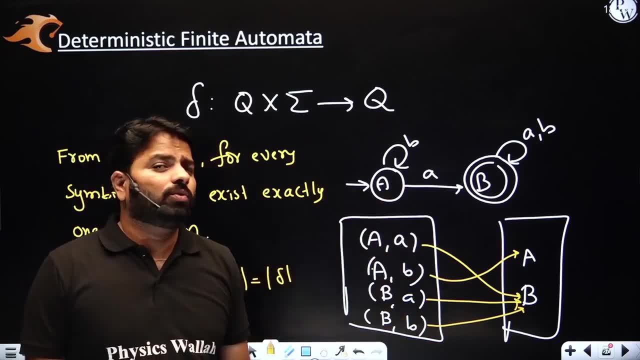 so let's come to this. you have now dfa definition, some of the important points. how many initial states must be there in dfa? only one. how many final states must be there in dfa? don't know, zero or more. so few points. you can remember in the beginning itself, one initial state you draw. 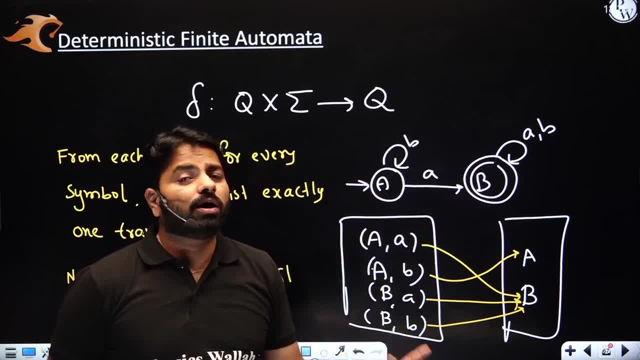 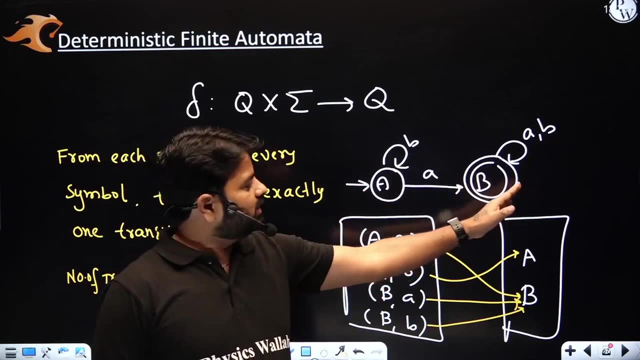 any dfa. how many final states don't know? zero or more. never say that at least one is wrong. okay, at least one is wrong, either zero or more final states will be there in the machine. okay, and always remember, if there are two states from each state, you should have a transition for. 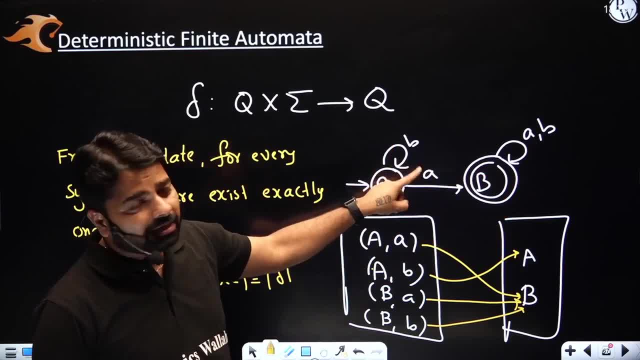 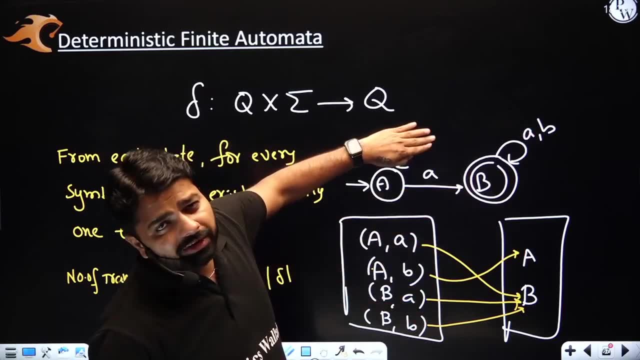 every symbol. see from this state: a is you have exactly one, b, also you have exactly one from here: a, exactly one, b, exactly one you can't miss. if i miss this one, that's not a df anymore. that's not a df anymore. okay, let's start with the problems. if you've already practiced, then 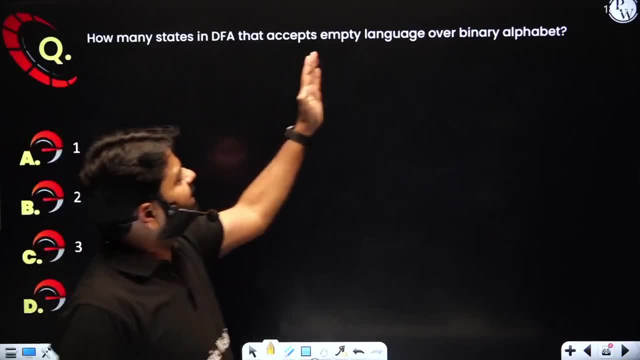 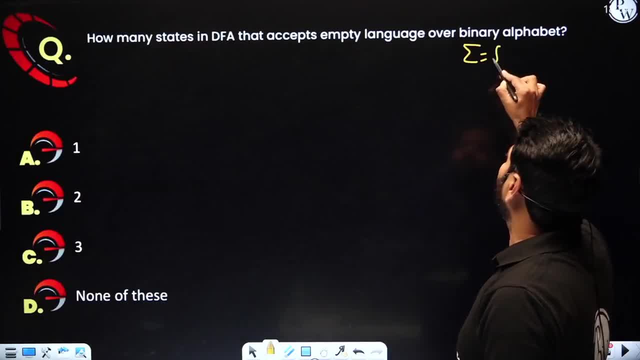 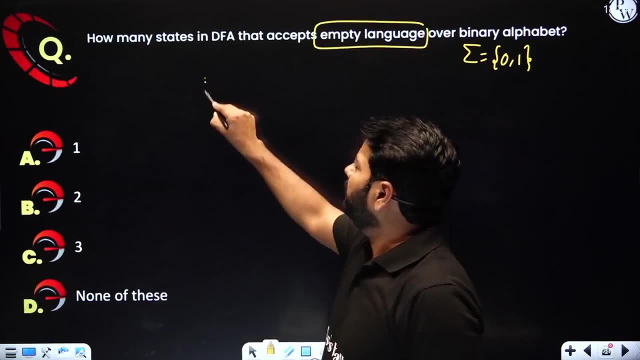 binary alphabet, so binary i'm taking here. sigma is equal, let's say zero comma one. i want to represent what empty language? what is empty language? l is they called empty set? that means i don't have a string to accept. then you should have a special state. 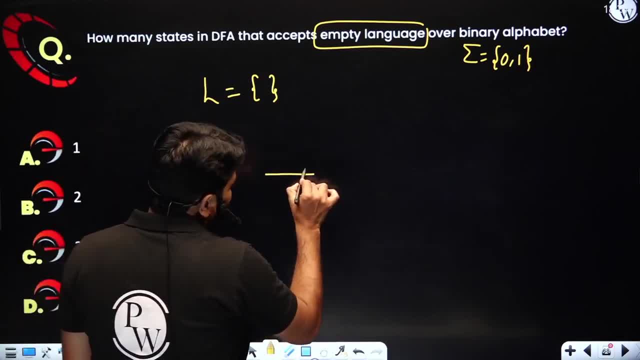 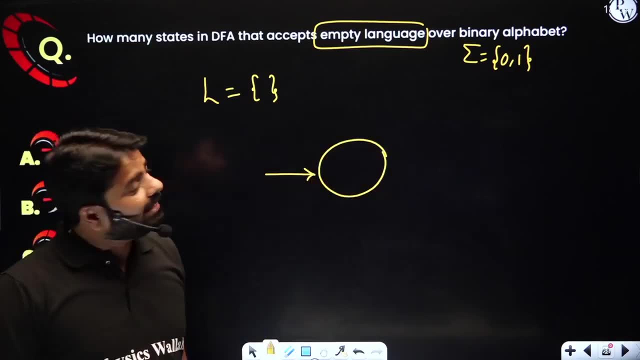 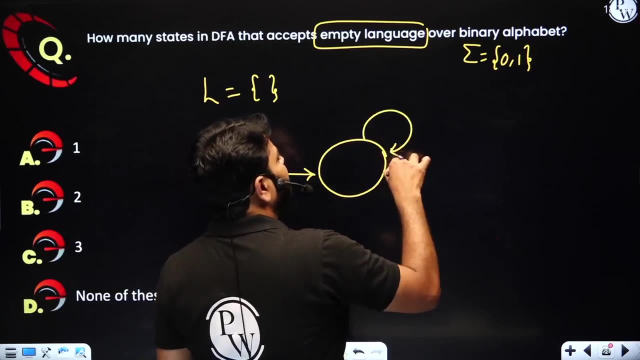 in the machine by beginning. only this arrow represents what initial state that goes right. when you begin the machine, you should go to dead state. dead state means you don't accept any state string from there onwards. so once you go here, you read anything, you stay here. zero or one, you always. 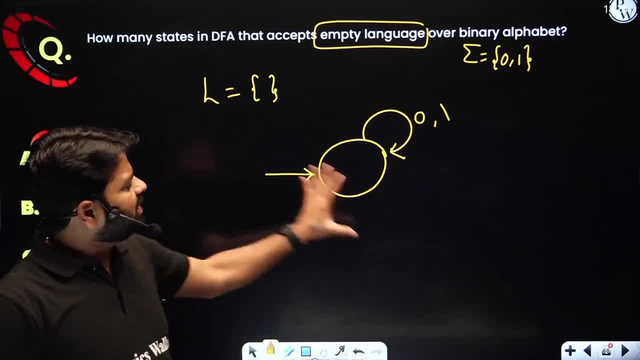 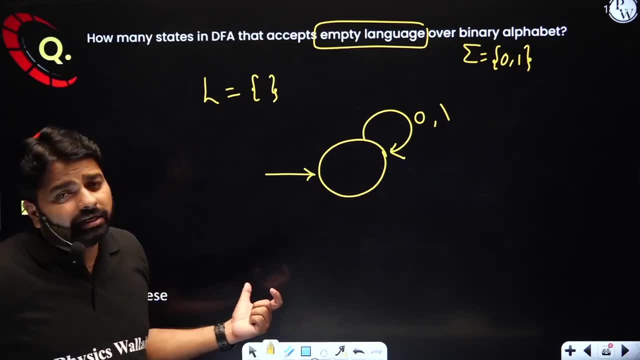 stay here because i don't want to accept anything. so initial state itself is dead state. i don't have a final in the machine. of course, here in the diagram you may design more than one dead state if you want. but if you want to design number of minimum number of states in dfa and somebody. 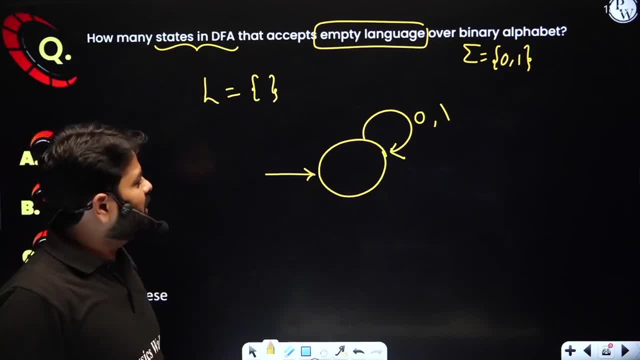 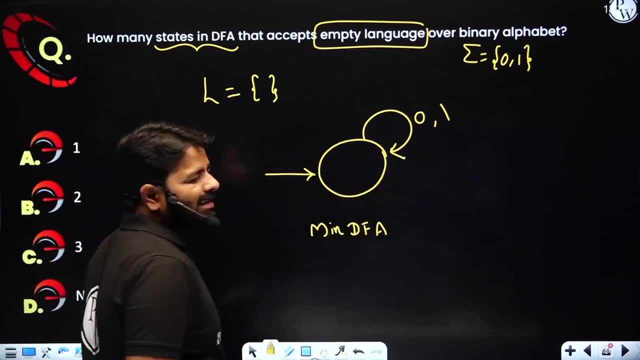 asking number of states. that means you must take only minimum dfa. so this is the minimum dfa. how do you know that? because i have only one state, less than one state impossible to design. now, how do i know this is empty language, because i have. do i don't have a final state here. do you have any final? 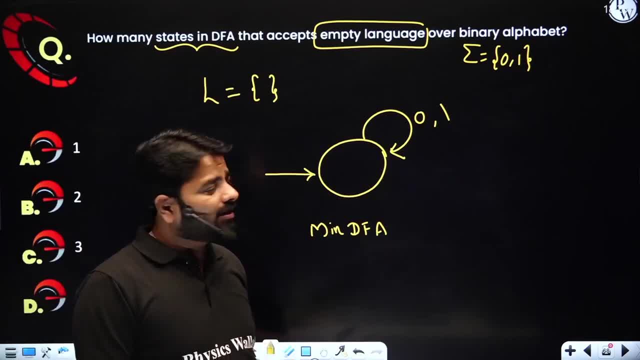 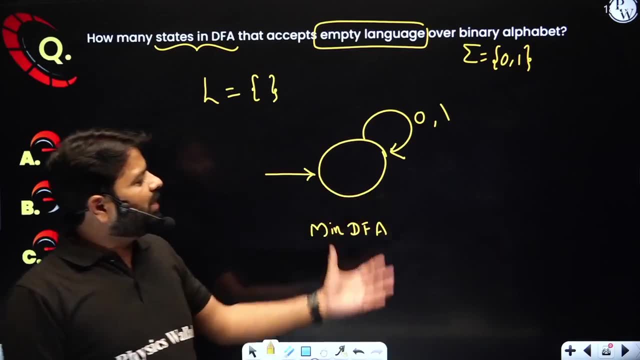 when you don't have a final, you can't accept even one string. is that clear. i don't have a final means. i accept nothing. if i want to accept something, i should have at least one final right. so very simple. when dfa has no final, means that definitely accepting empty language. 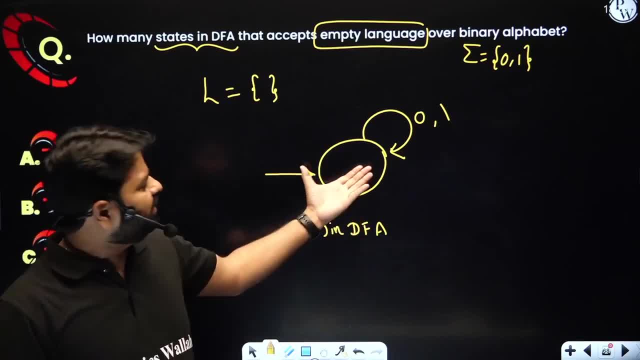 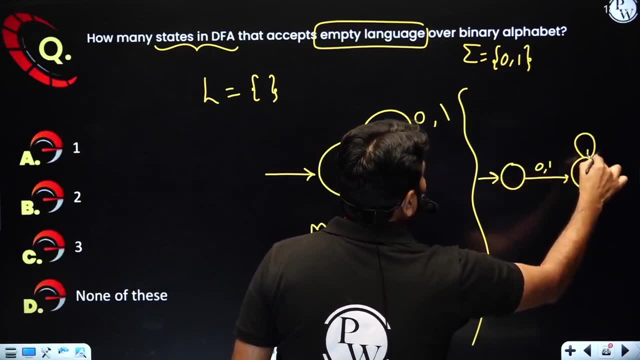 it's not necessary to design with one state because of minimum dfa. i design with one state. you may design with two states here, zero comma one, zero comma one. they're also accepting nothing. but it is also dfa, but it's not minimum dfa, even though. 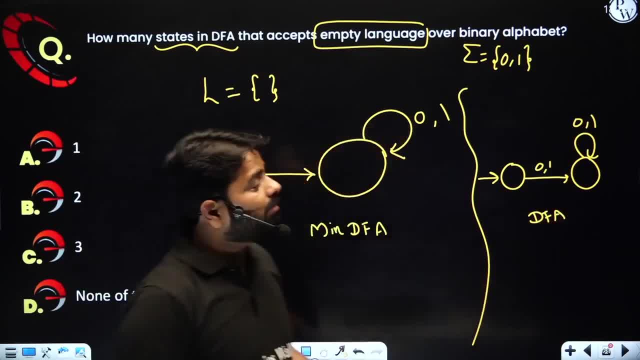 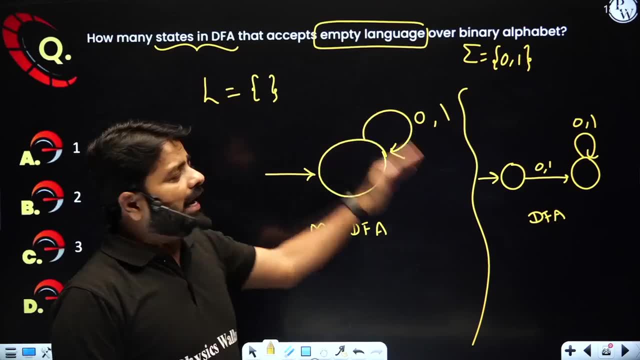 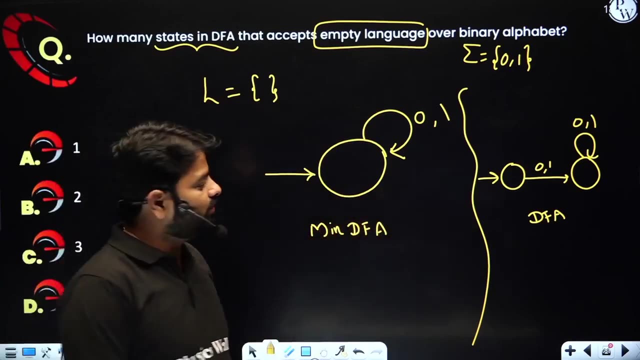 it is dfa. but when somebody is asking number of states you can't consider it. you have to consider minimum dfa. clear this point. okay for any regular language: how many dfs are there? very important question. you tell me now. i just shown two. can you draw one more? just try. 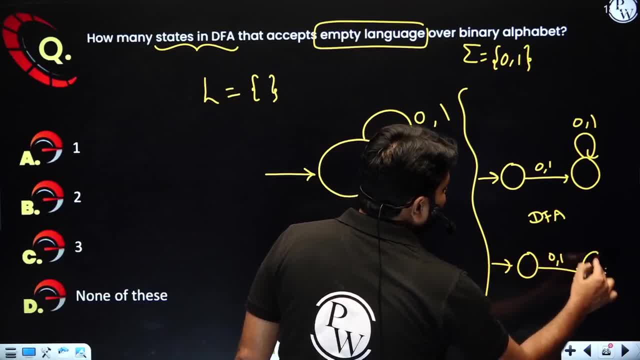 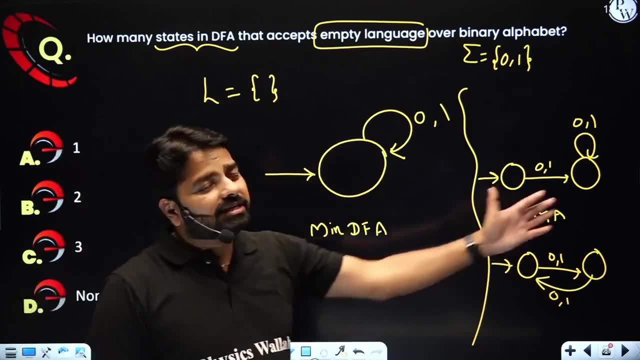 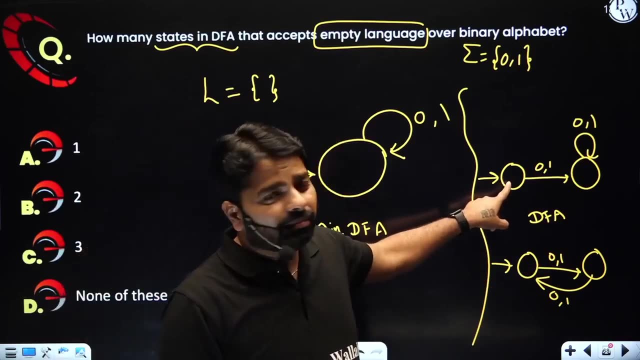 don't ask me, sir, why are you designing this way? only your choice. how do you design another dfa? likewise, with three states, i can design four states. i can design, but don't keep any final. but you must satisfy dfa. you can't miss any simple transition from every state, from every state. do 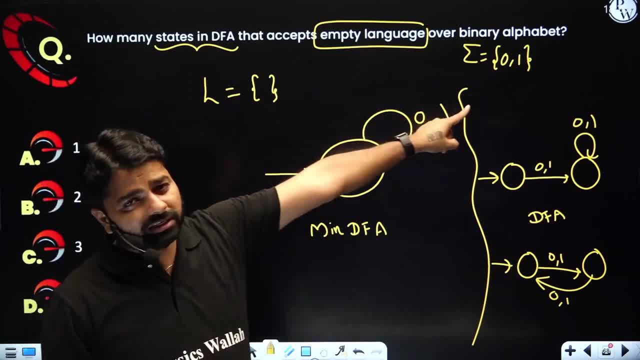 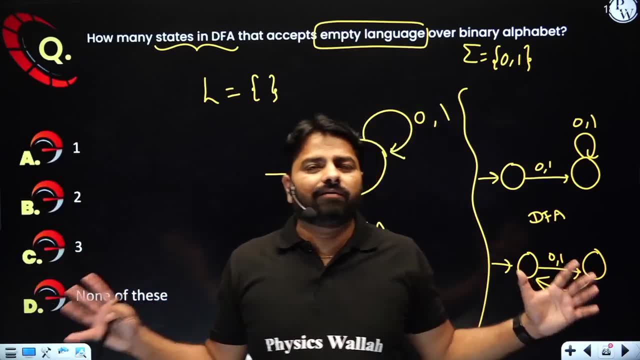 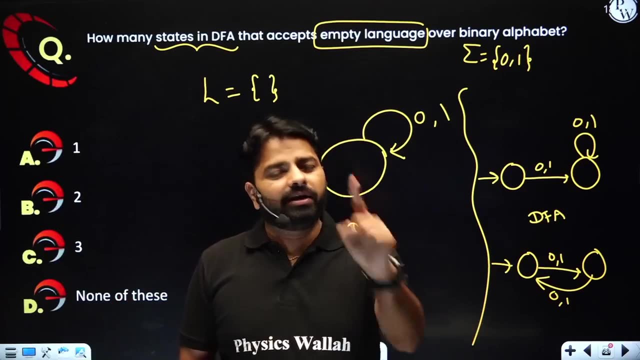 you have two transitions, exactly as you have two input symbols in your sigma clear. so the first point is: for any regular language, or every regular language, you will have infinite equivalent dfs, but only one minimum dfa. i'm just keeping a note for you. you can write yourself for every. 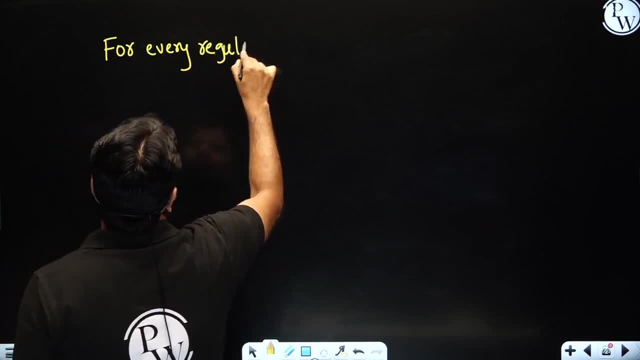 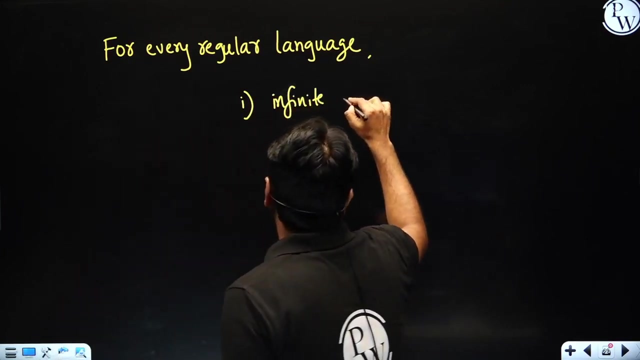 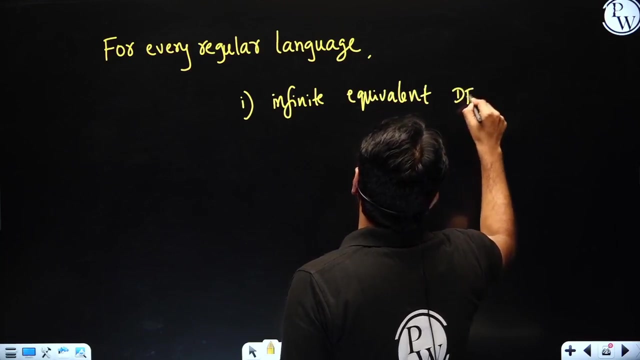 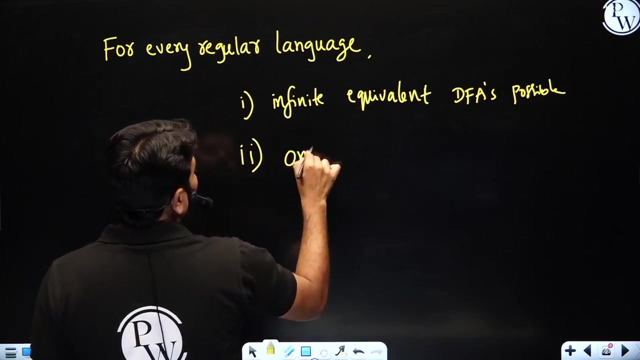 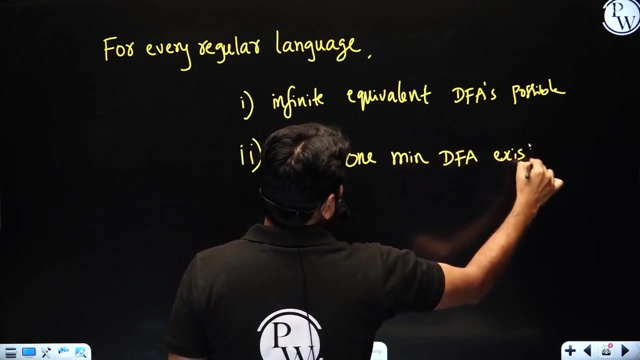 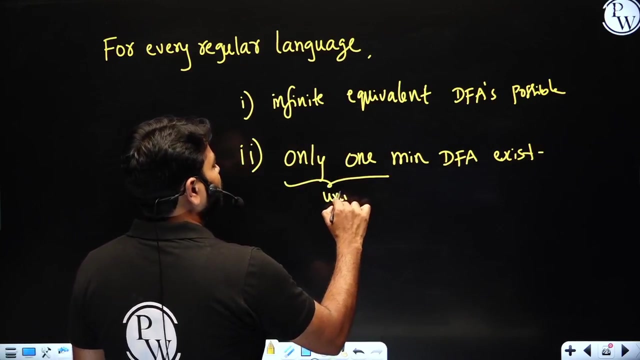 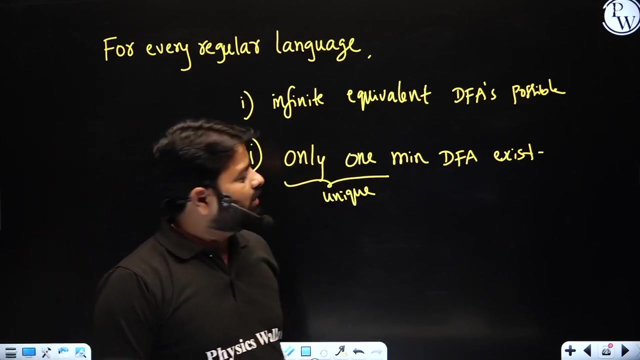 regular language or every regular set will have infinite equivalent dfa is possible, but remember, only one minimum dfa exists. you can't have more than one minimum dfa, unique minimum dfa. only one means unique. you can't have more than one. fine, but this are important points for every regular language. 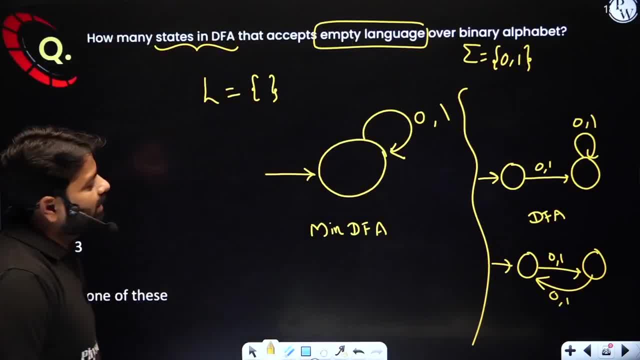 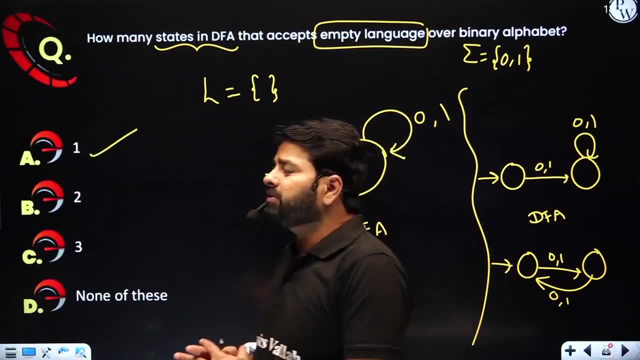 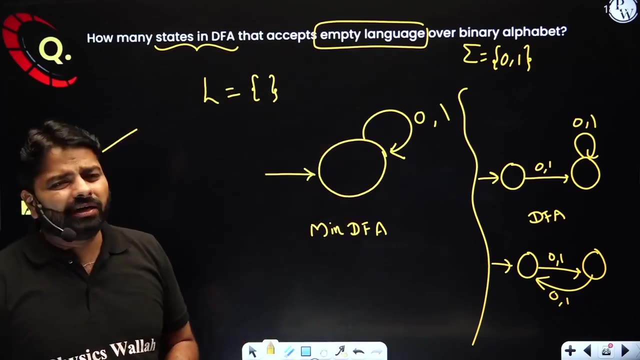 okay, now what is the right answer? how many states? you answer two, one, three, four, five. so which one is right answer? one state is once. it would be sufficient to accept the empty language over any alphabet. you may ask question, sir. that sigma is binary if it is turned. 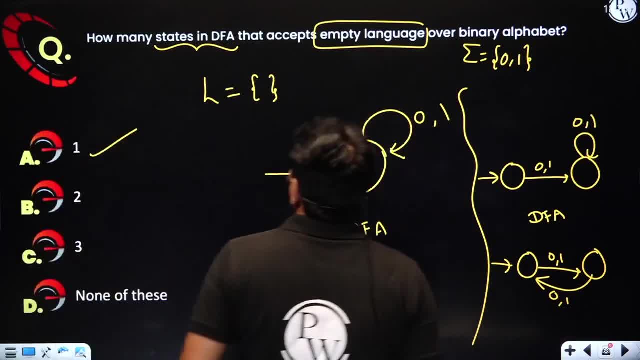 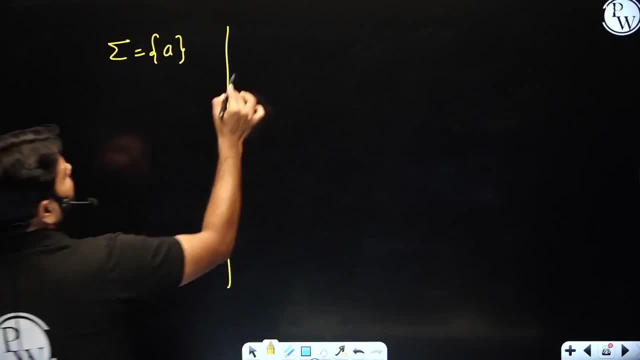 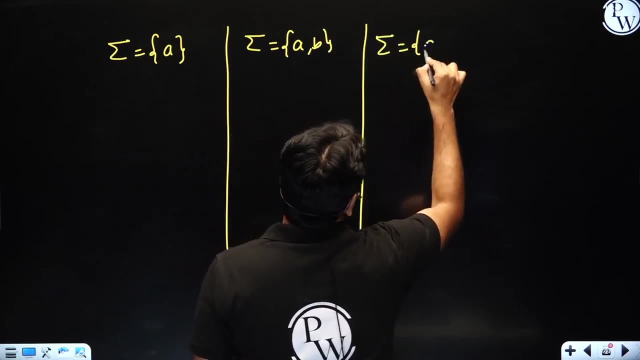 binary, what do you say? if it is unary, what do you say? so let me explain you. sigma is equal. let's say: a, how the dfa looks like. i want minimum dfa, only a comma b, how it looks like a comma b, comma c, how it looks like, and so on. you can design as many you want it i want to represent. what empty language. 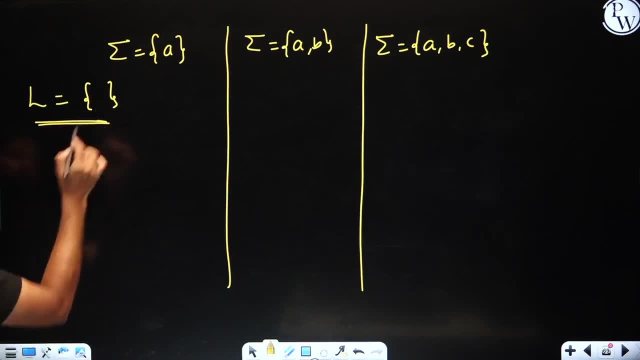 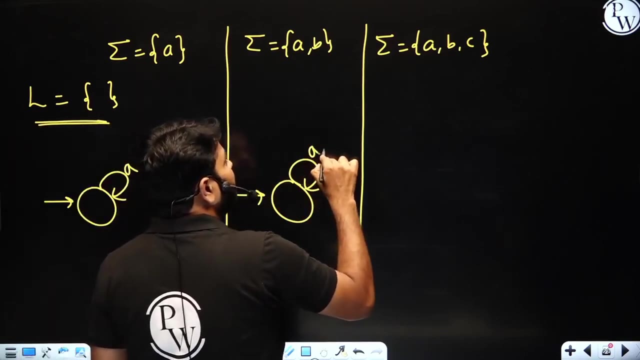 right for all of them. what empty language you want here? empty language, how it looks like? initial state is not final, because if it is the final, it will accept epsilon, but it is non-final as you don't have any string. just keep a here here, what do you do? empty language? keep a comma b. 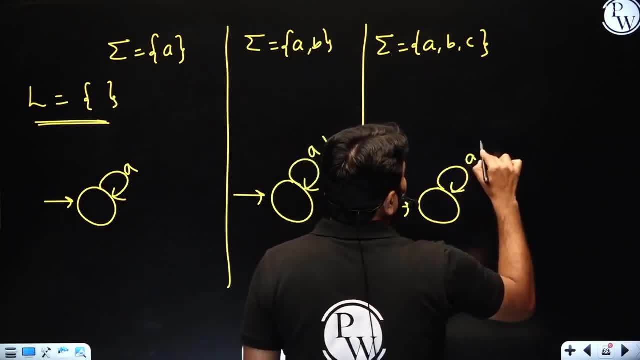 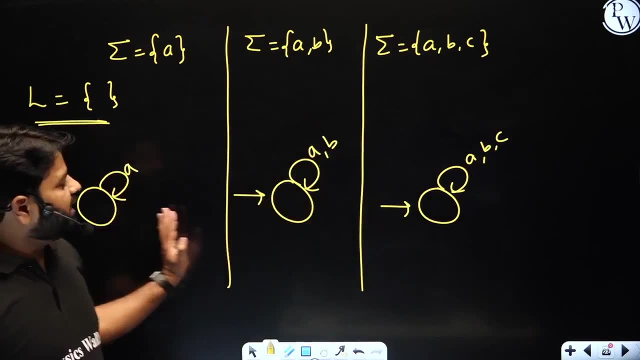 here. what do you do? number of transitions may vary, but number of states will not vary for the same language over different sigma. is it clear? the number of states are one, but sigma sorry. number of transitions would vary depends on how many symbols we have in the sigma. okay, number of. 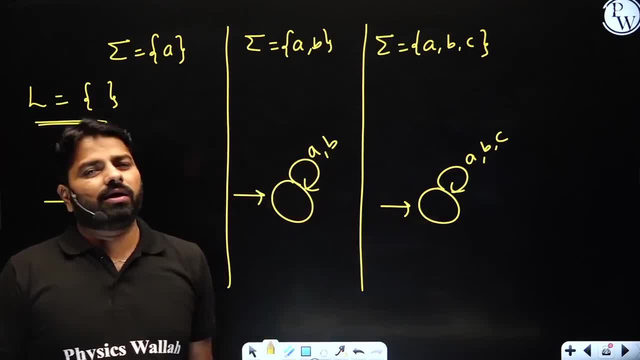 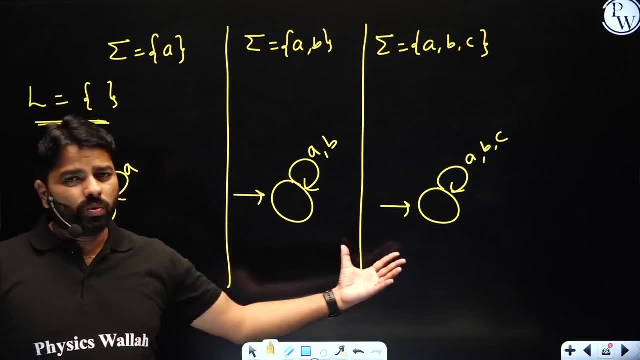 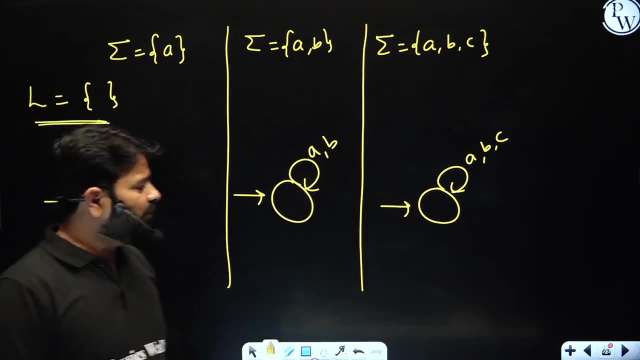 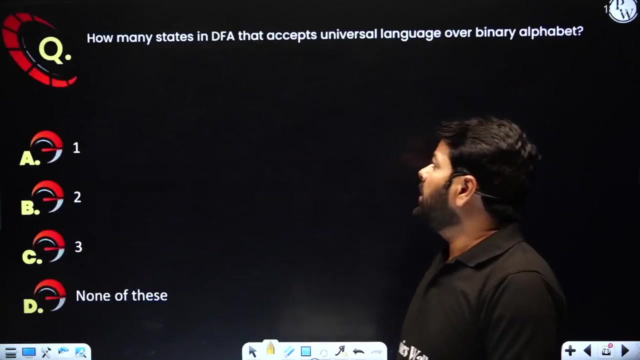 states in all the cases. you have one here. minimum dfa will have only one state, okay. and is there any final state? no, how many non-finals? only one, okay. so everything that i ask, you should know how to answer it. fine, let me go to another question now. can you answer it now: how many states in dfa that? 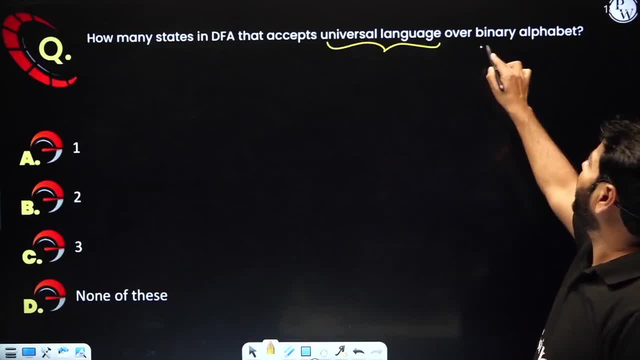 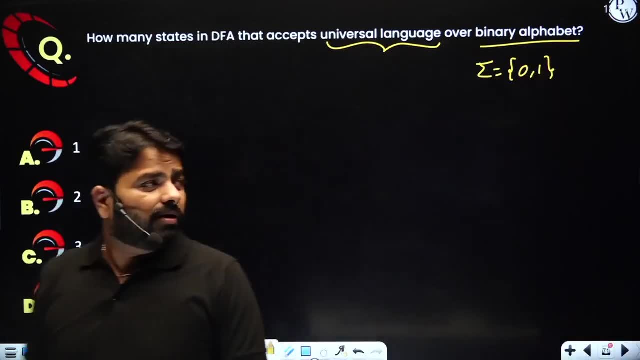 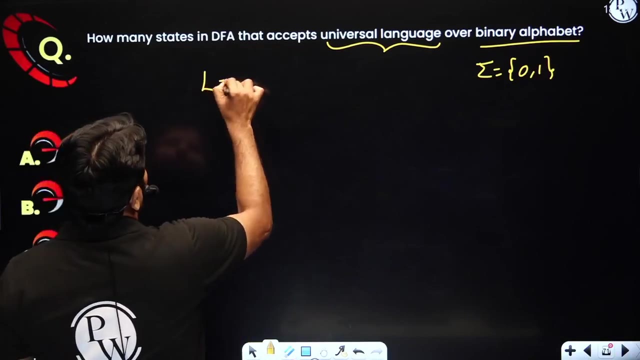 accepts universal language, very famous right over binary alphabetics. binary alphabet is what? sigma 0 comma 1 or a comma b. you can take any choice. now what is universal language? you know that in the regular expression you have written a plus b, whole star, so that a plus b whole star is going to represent universal language somehow. 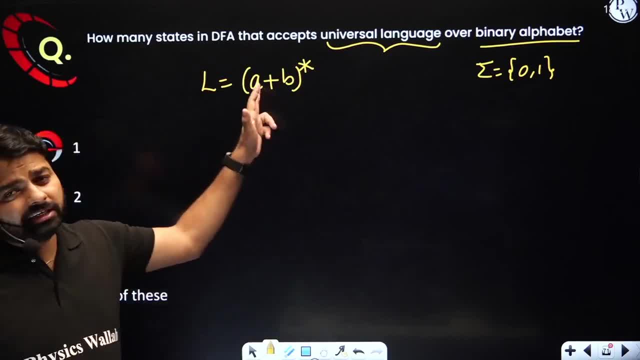 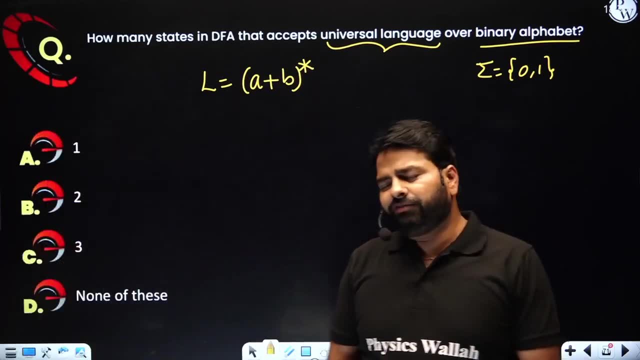 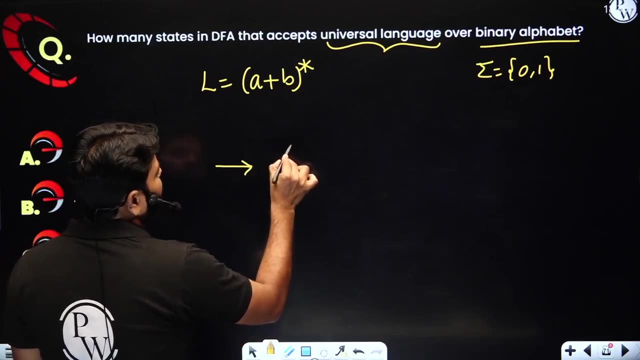 every string is present in the l generated by the a plus b whole star. now everything is accepted. there is nothing to be rejected. that means your dfa just keep finals only don't keep non-finals. like if i have initial state, first point, initial state, i am keeping final. what do you mean by that? 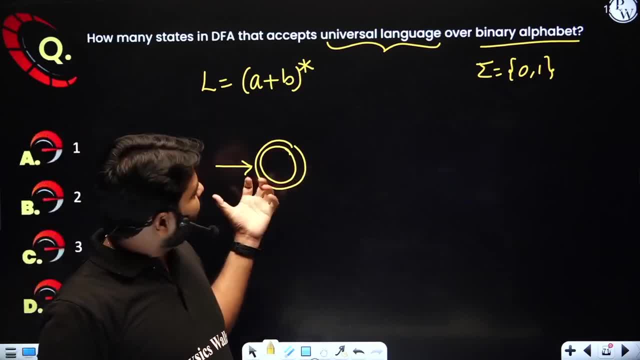 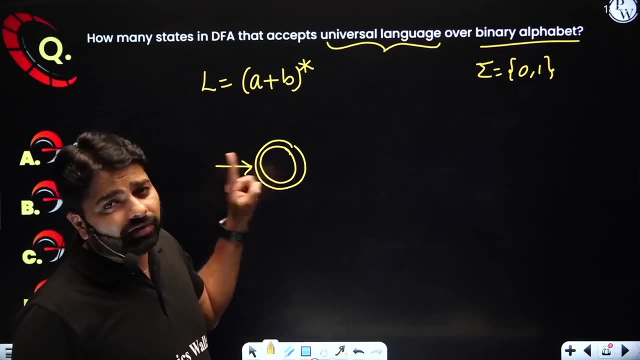 when the initial state is the final. it always accepts epsilon, because when you begin, you are reading epsilon by default when i don't read anything else. right? if the string is epsilon, you will always halt at final. you will always halt at initial. if the initial is final, then 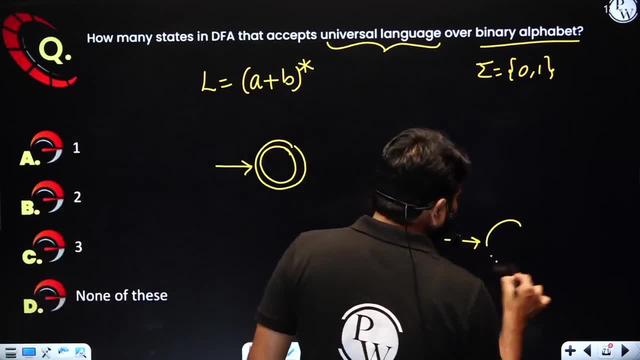 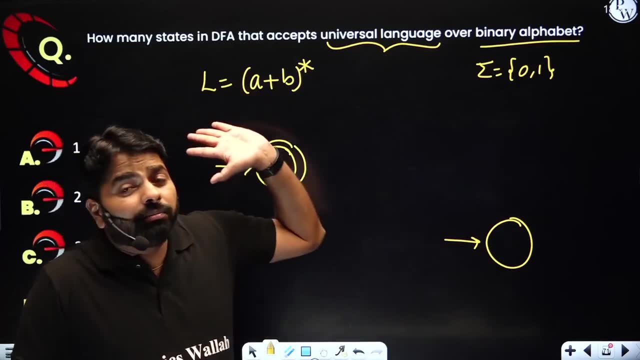 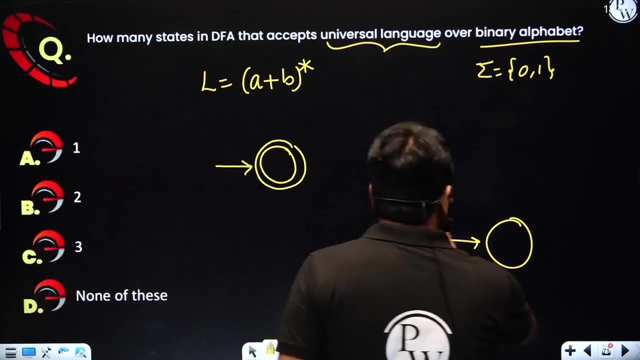 epsilon is accepted. so if the initial is non-final, epsilon is not accepted in deterministic machines. very simple: if initial is non-final, that means epsilon may not be. epsilon is not in your language. when the epsilon is in language, you must keep initial as final. try to understand this difference now. after that, is there anything to reject? no, 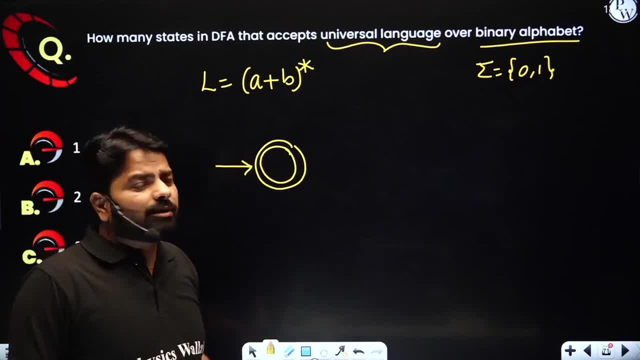 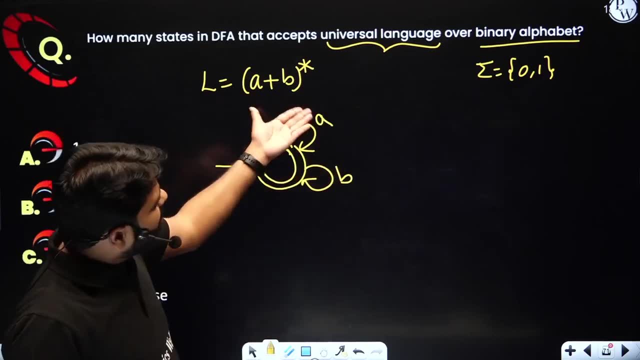 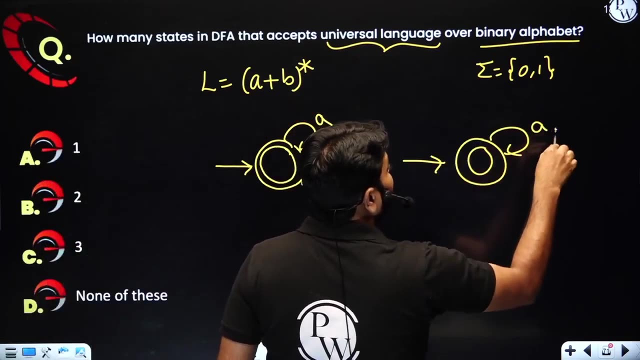 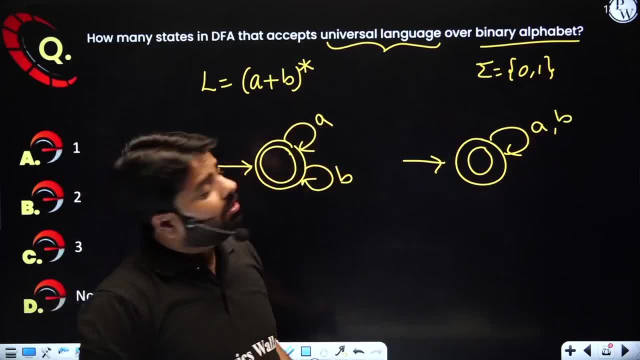 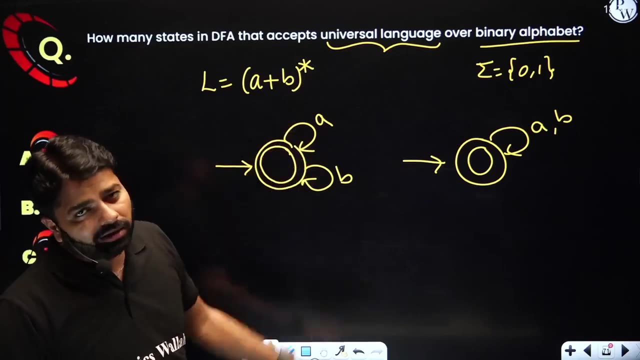 when you are writing a comma. b doesn't mean that after a b comes, maybe b will come first, or again b may come, or three a's may come, one after other, doesn't matter. this two means two independent transitions. two independent transitions. they can appear in any order, so any sequence over a's and 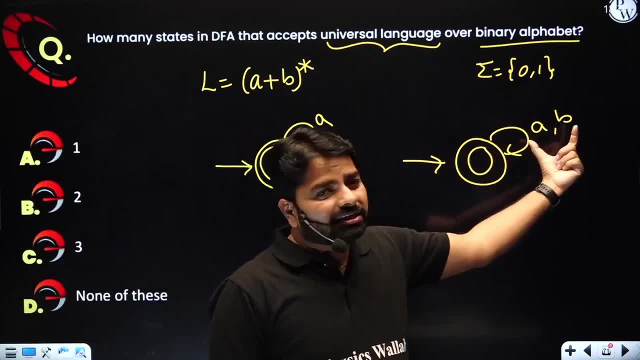 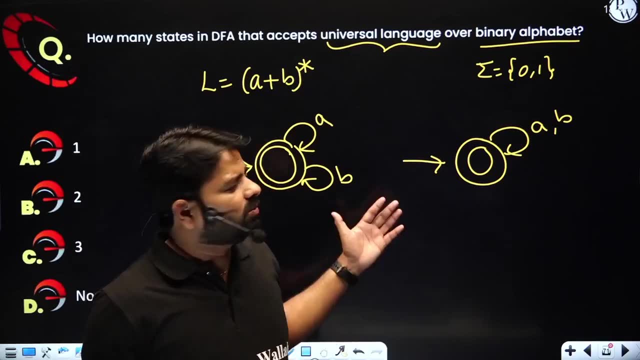 b's. when we write this, it means any sequence over a's and b's. when we write this, it means any sequence. it could be a comma b, b, comma a, or you may have three a's are consecutive, consecutively coming or doesn't matter what you think. so any a's and b's, that is a meaning. now, anyhow, both are. 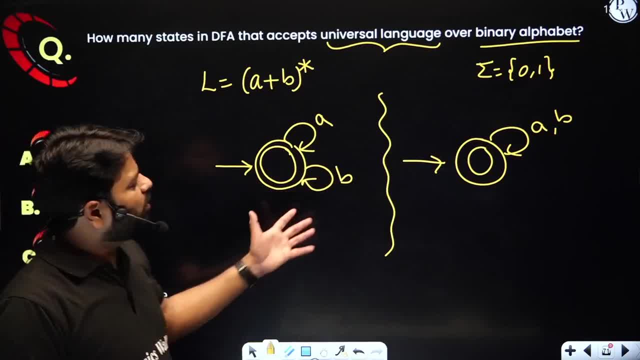 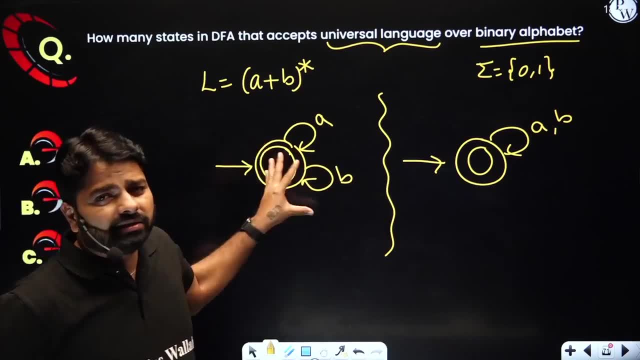 same how many states you require, one or more. just one very important point: if every state is the final in the dfa, if every state is final in the dfa, what is the language accepted by that machine? okay, dfa. i'm talking about if every state is the final in the dfa. if every state is the final in 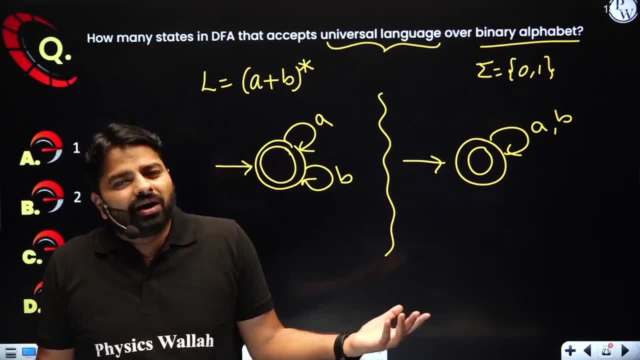 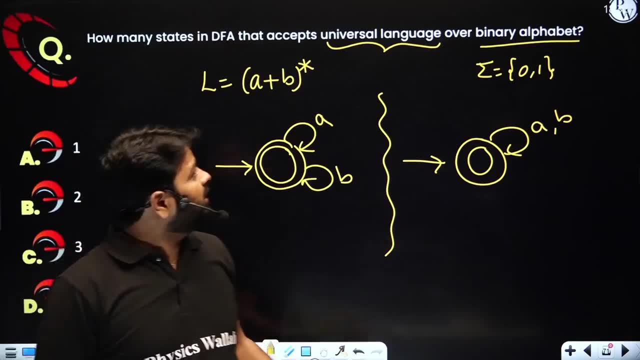 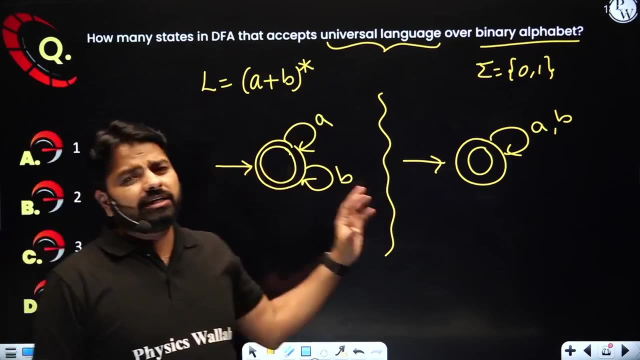 the dfa. if every state is the final there is: wherever you halt, you are alting at final. if i'm alting at final, the string is valid means every string is valid. when every string is valid, it has to be universal language. is that? is that my point here? okay, i'm repeating again: if every state in 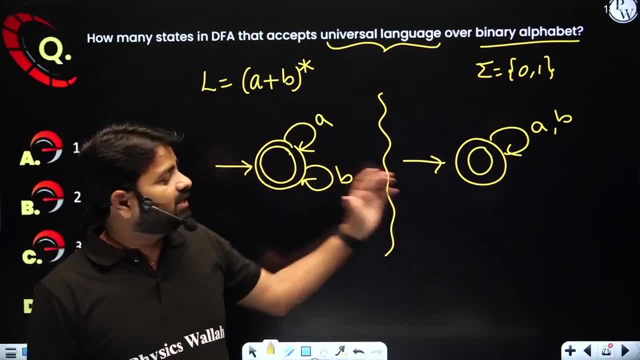 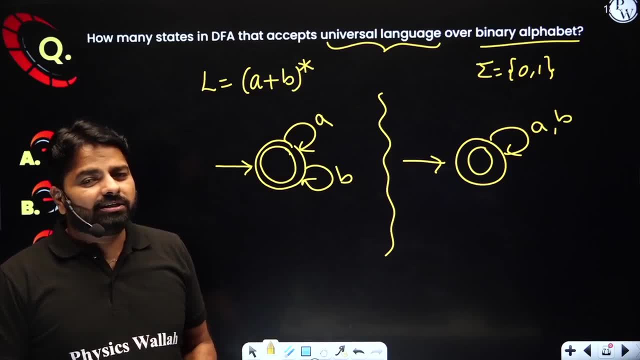 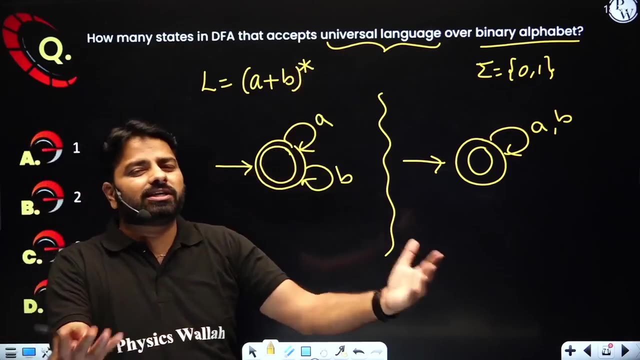 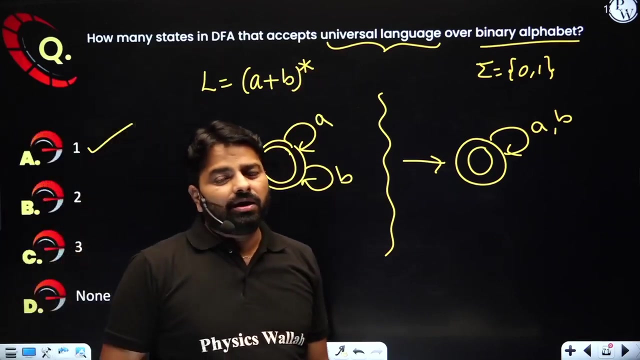 the dfa is final, if every state in the dfa is final, if every state in the dfa is final, it means for every string you will halt at final. it means your language is universal because you are not rejecting any string. okay, so how many states? one one. okay, if every state is non-final, empty language accepted. if every state. 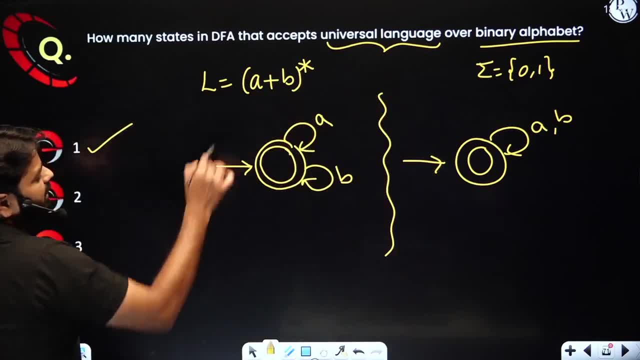 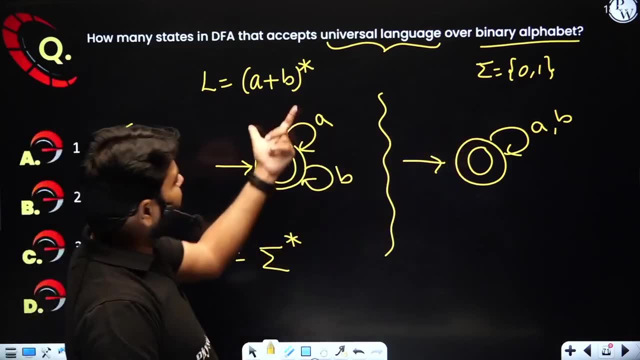 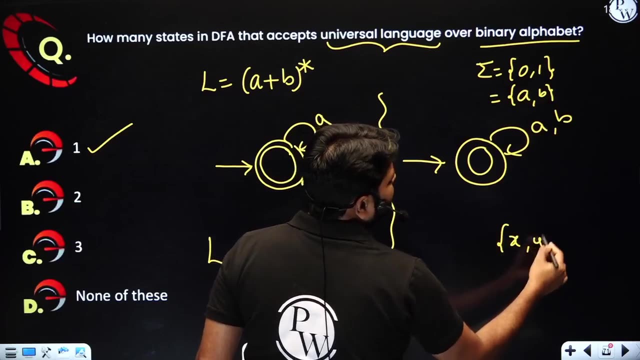 is final sigma star is accepted. you may call it as this: l is equal to a plus b, whole star. you can also call it as sigma star, because sigma is zero comma one or a comma b, that doesn't matter. you know, some times you may draw with a comma b, or you may draw with x comma y. all are same as if they are binary. 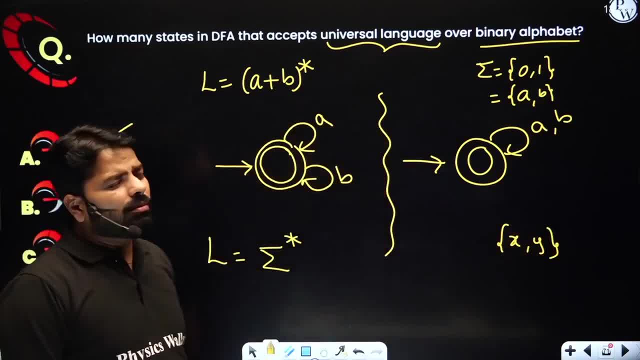 symbols. right, two symbols are there. in the language we mostly use a comma b, but as per the question, binary alphabet, nothing mentioned. you can take zero comma one, a comma b, x comma y, all are same. okay, don't worry much about it. the options you don't worry about: a, b, zero one, x, y, so doesn't. 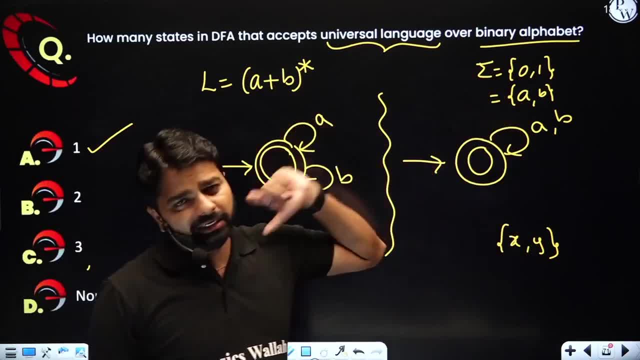 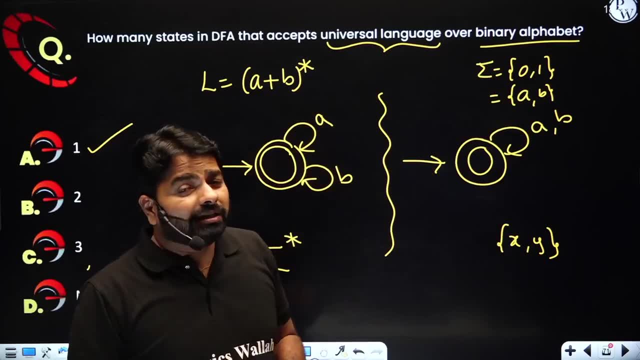 matter, just number of states only matters. you just take as per your practice. if you are practicing always with zero comma one, just take zero comma one. but if you practice a comma one, you can take a comma b, because always important what your mind thinks, how it, how quickly it thinks if you. 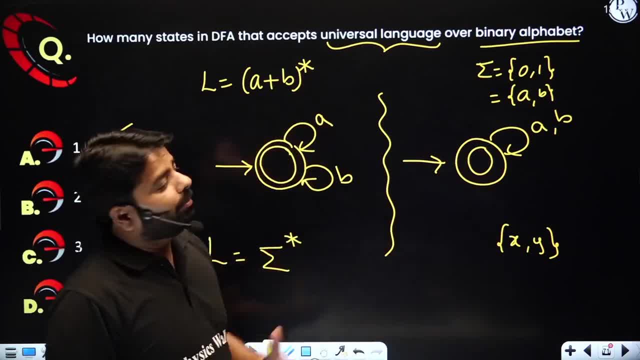 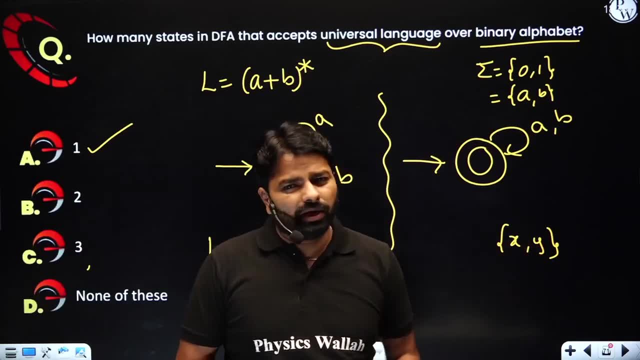 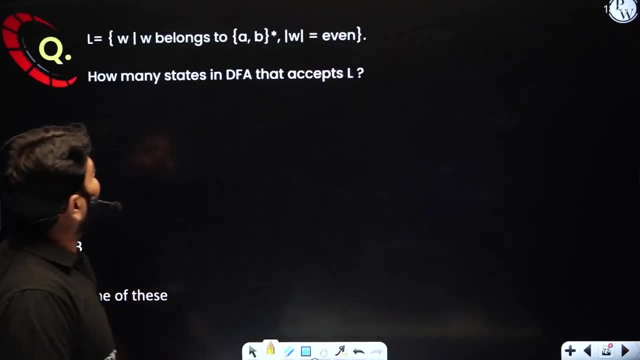 practice a comma b all the time. you can very well design with a comma b's, because always i practice with a comma b, sometimes zero comma one. i usually do very less with x comma y. that's fine. let's go to the next question. okay, how many states in dfa that accepts l, where every string is having even? 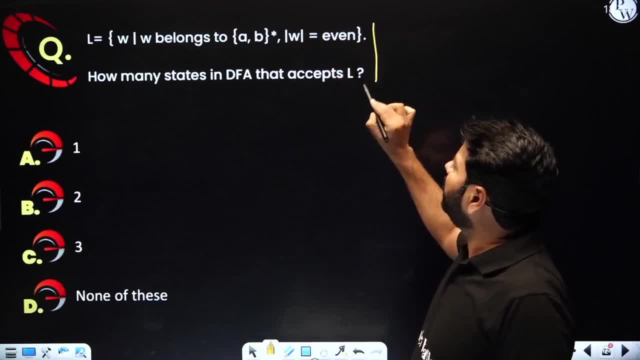 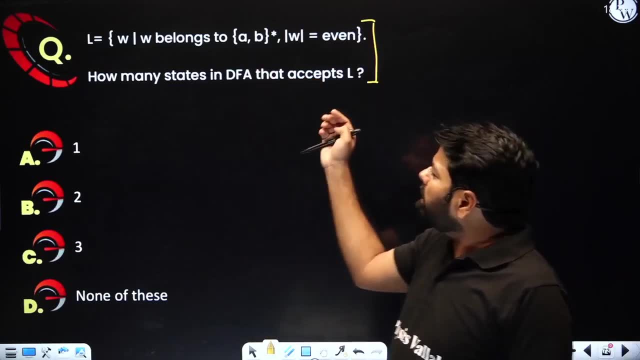 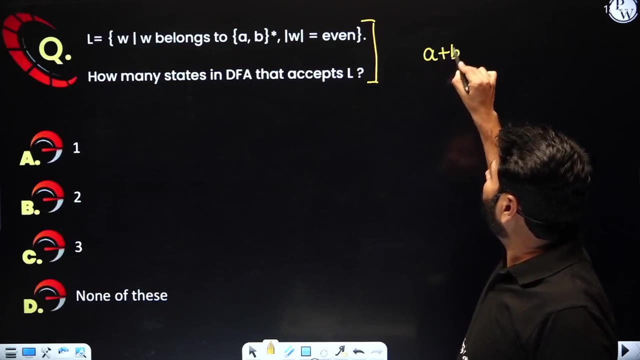 length. i hope you know the regular expression right. can you write that now? let's see who will write. okay, just think about it. stop the video and pause. pause the video now. just think about what is the regular expression to represent even length strings. did you remember that a plus b, whole square, whole star, that will represent every. 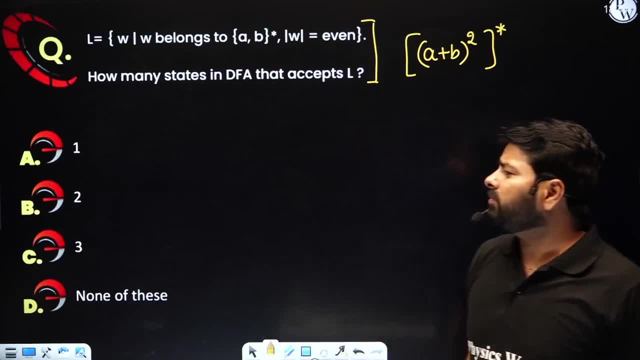 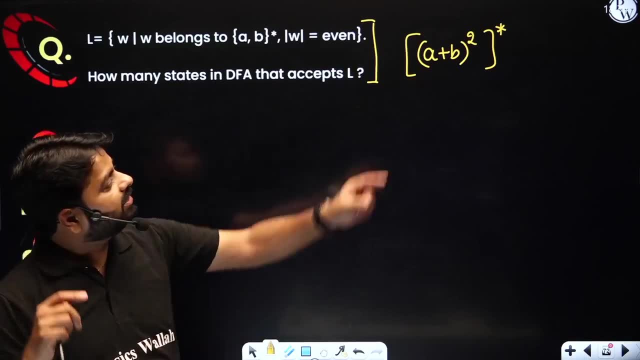 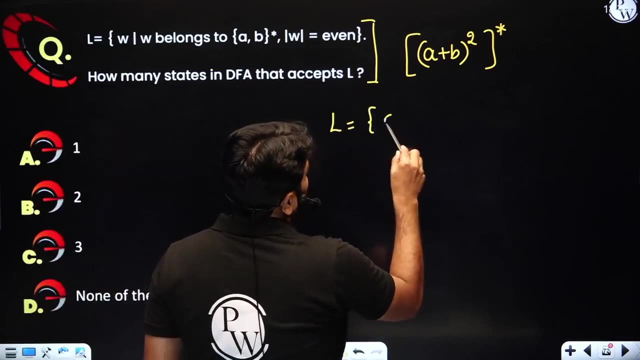 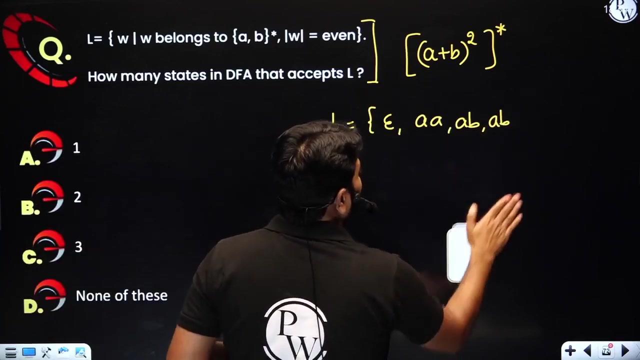 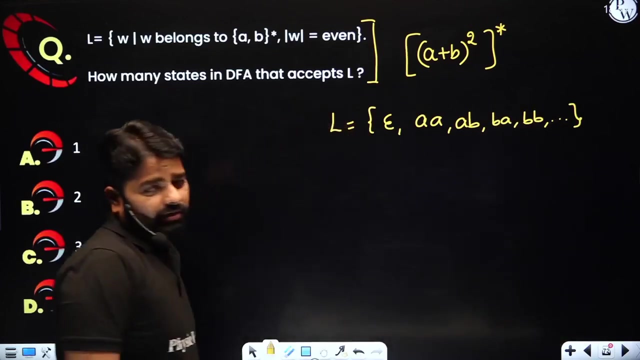 even length string over a comma b right now, how many states required to accept this language or to accept the language generated by this expression? think about it. okay. what is the language? epsilon then? one length, not possible. two length. fine, now look at your language in dfa. mostly always consider most of the problems. 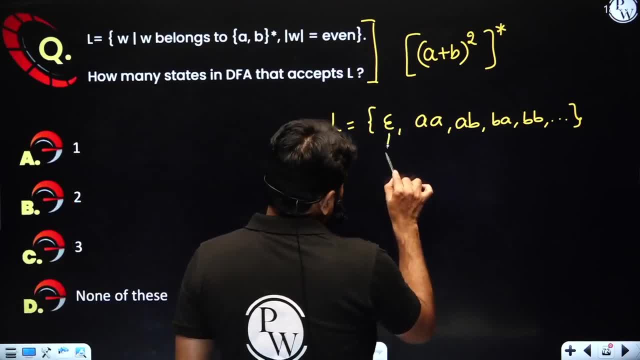 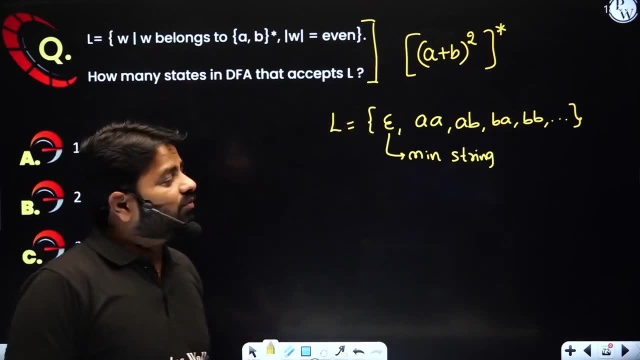 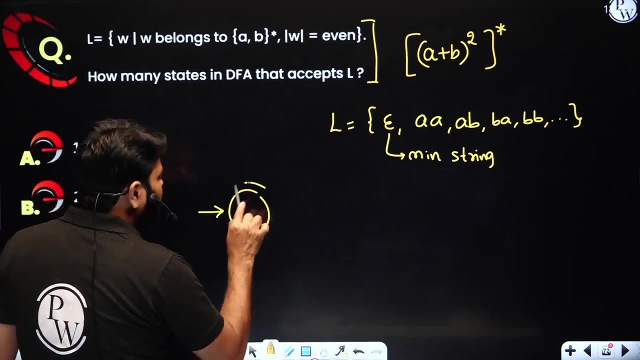 focus on the language and not on the language, and not on the language and not on the language. a minimum string. what is epsilon here? minimum string that will give you the beginning. once you know the beginning, you can slowly expand the machine. but When you have epsilon, then how do you design your machine? this is how you design now. i have accepted. 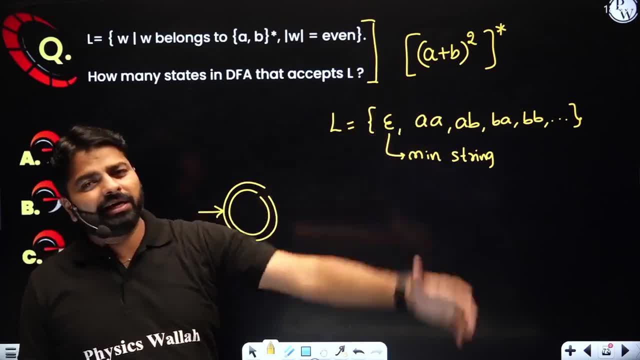 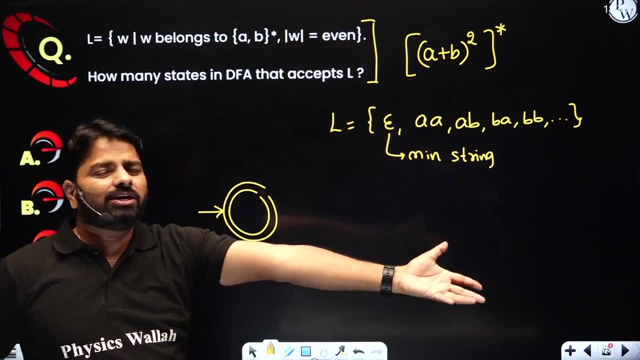 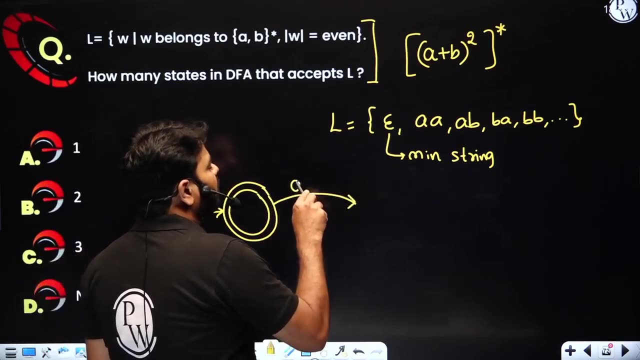 epsilon. how do i expand this state to accept the remaining strings? now you focus. the problem is even length. right means every second symbol, whatever it is, whatever it is, you should come back to final. that means just take the axillary state. one length, either a or b, doesn't matter. two different transitions, either a or b. you go to non-final. 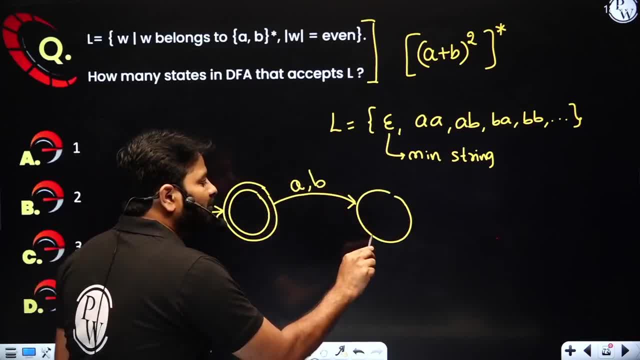 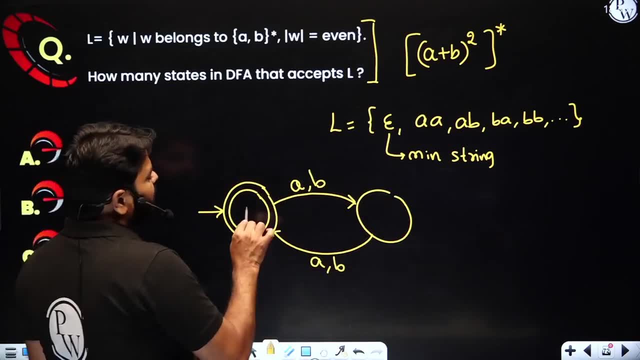 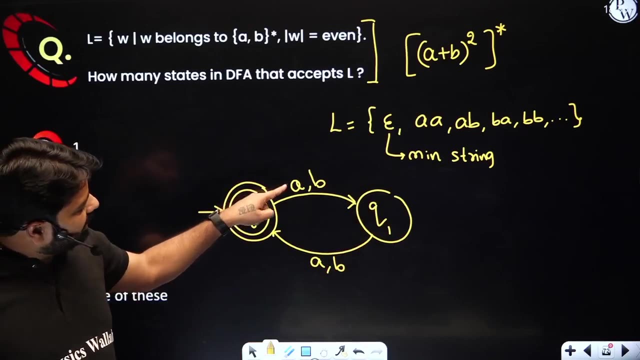 because it should not be accepted. after one length, you get one more length. you come back to final. now see, is it dfa? how do you know it is dfa? how do you know it is dfa? from q0: one transition for a. one transition for b. from q1: one transition for a. one transition for b. 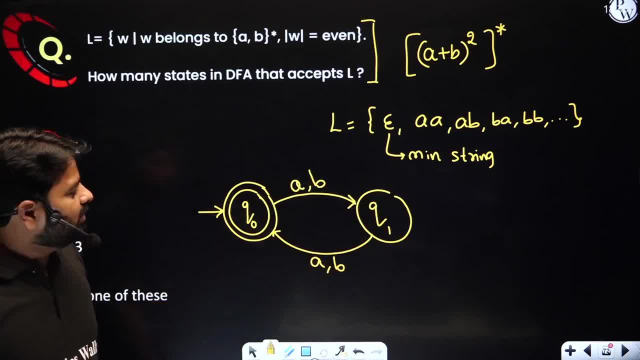 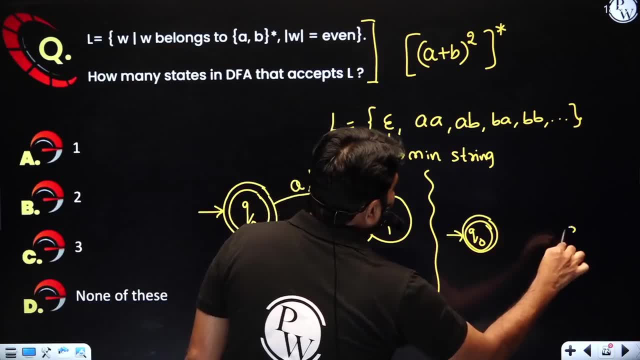 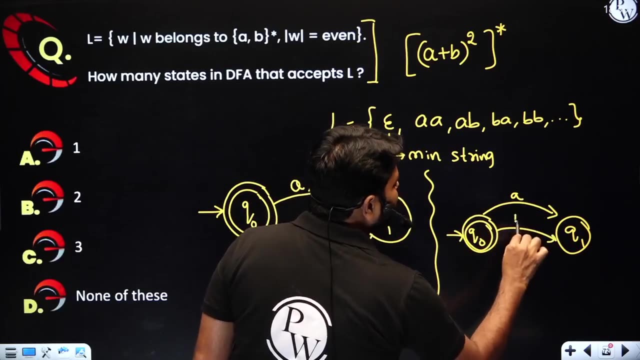 if you want to see exactly how transitions are there, you can see here. you may draw like this, but sometimes it would be appropriate in the beginning. you draw different way. it's actually a is here and one more transition b. instead of drawing two different edges, you can draw one transition for a and one transition for b and one transition for b. 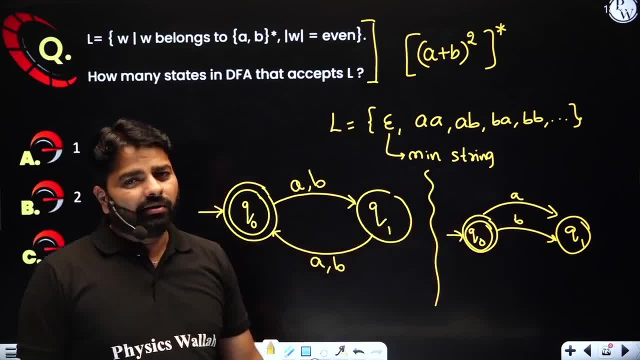 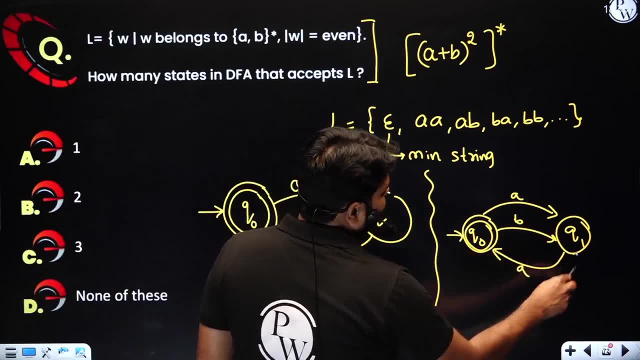 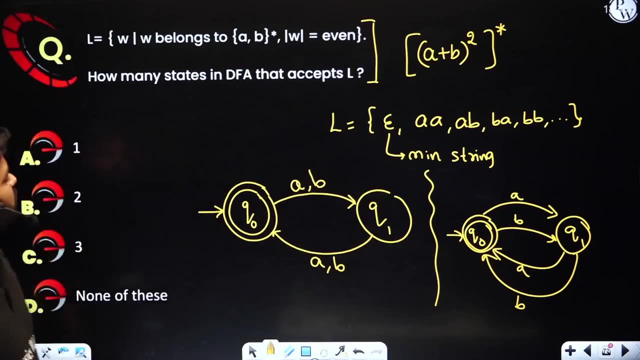 you can represent with one edge anyhow, two transitions. are there a short form to understand two transitions with one edge? okay. similarly, a, b, that's okay, that can be, you know, represent short form with one edge. so how many states? we have two, one, three, you can see simply two. 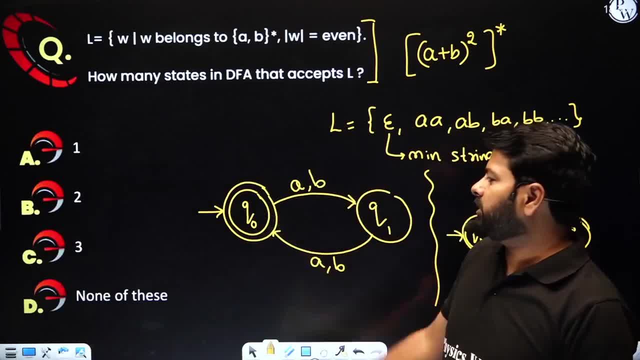 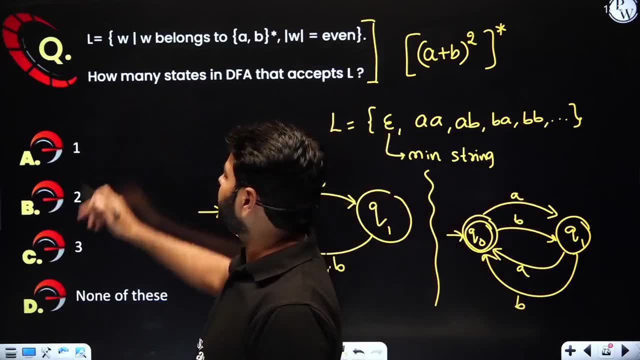 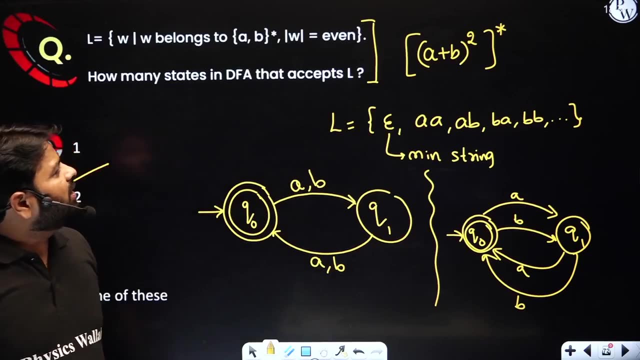 how many states? how many states are there? two states, how many transitions? if i ask here how many transitions? one, two, three, four, four transitions. but question is about how many states? two states, okay. so now if i ask um, how many states in dfa that accepts odd length strings? 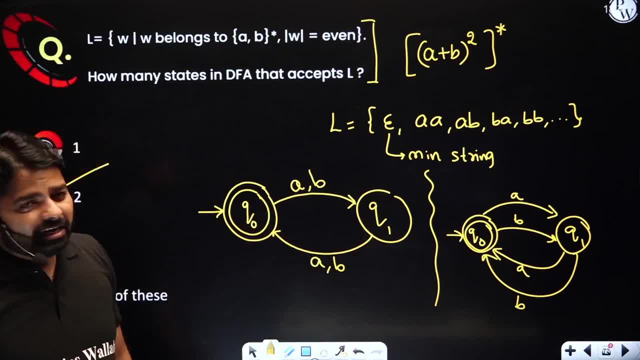 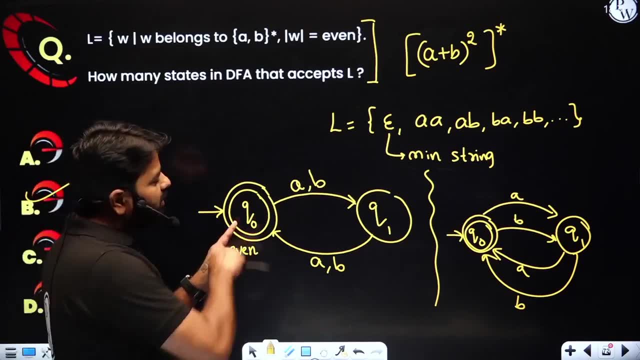 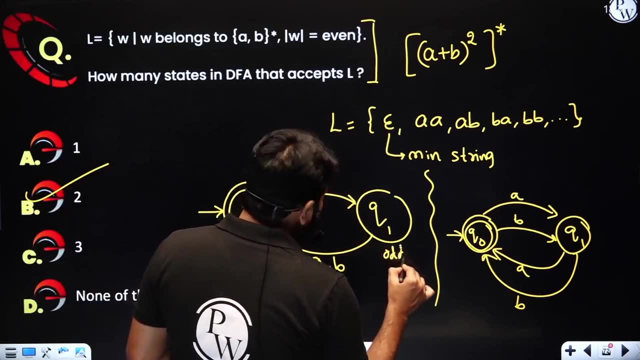 even length strings to write odd length. how do you design think about here? this q naught actually represent what? even whenever even length comes, that you always stay here. if there is no more symbol, you will stop here. if it is odd length, you will stop here. now you can easily understand. if even length strings 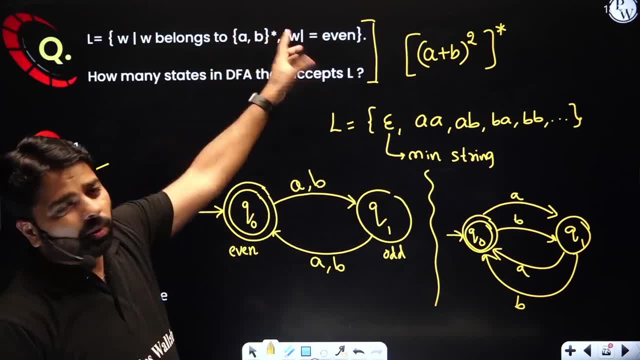 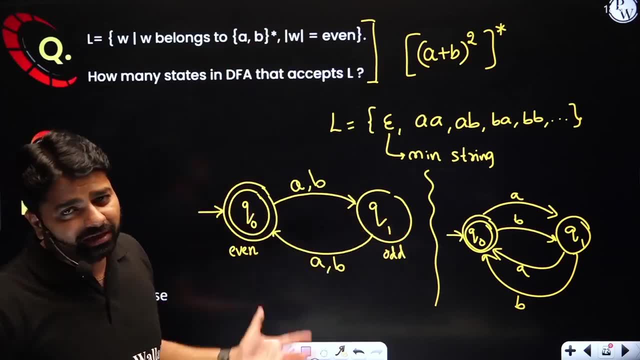 you want, you made even state is the final. if odd length strings, i want, i'll make q one as the final. if anybody makes both are final. every string, every string will accept. but anyhow, we have a better mission for that. okay, let's focus on odd length strings. how to design. 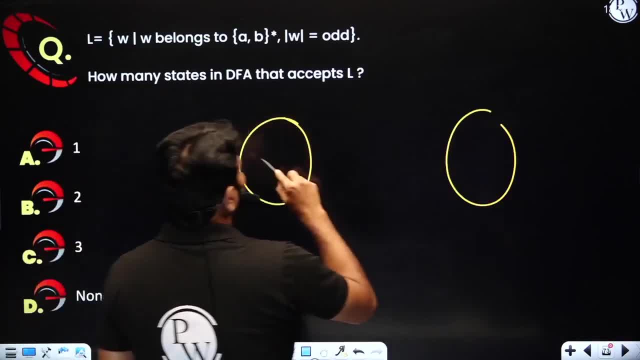 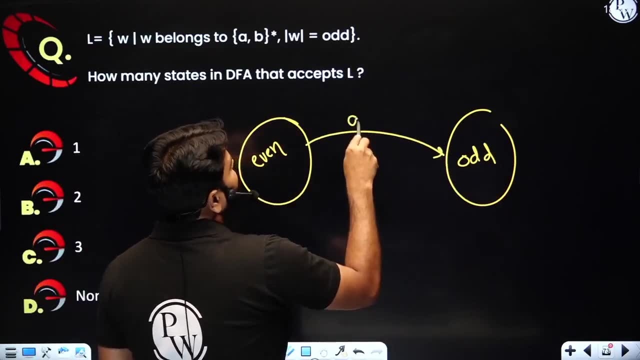 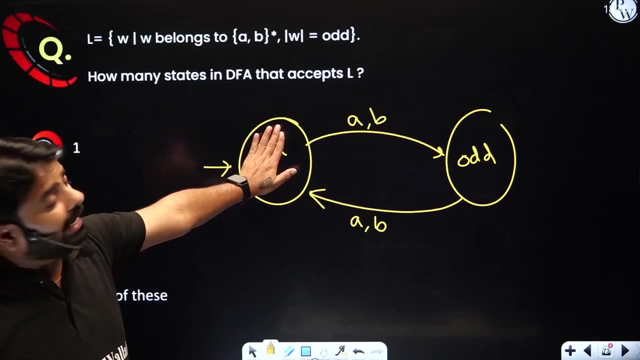 very simple. we have two states. this is the even state, this is the odd state. every odd length. you will go there. or b every even length you come back now. you decide which one you want to make final. so make this state is a final. i will accept all even length strings. 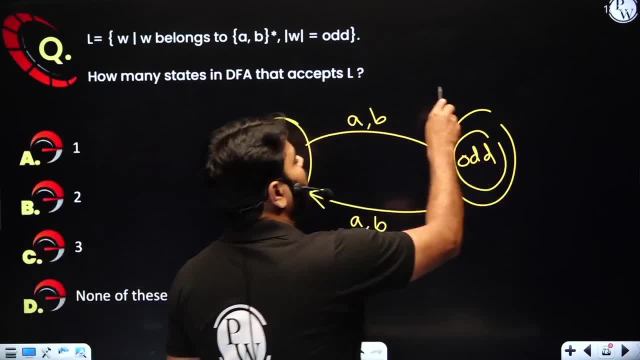 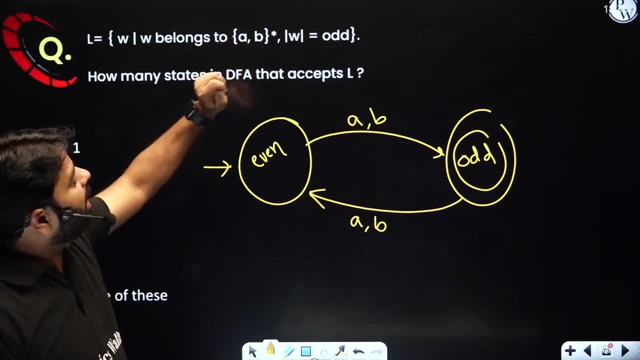 if i'll make this state is our final, i'll accept all odd length strings. as per the question you want all odd length strings. w belongs to a plus b, whole star, and the length of w is odd. it means every order lasts string should be there in the language. you should not miss even one or length. 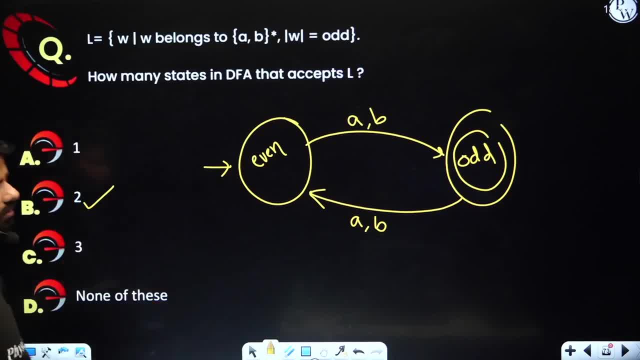 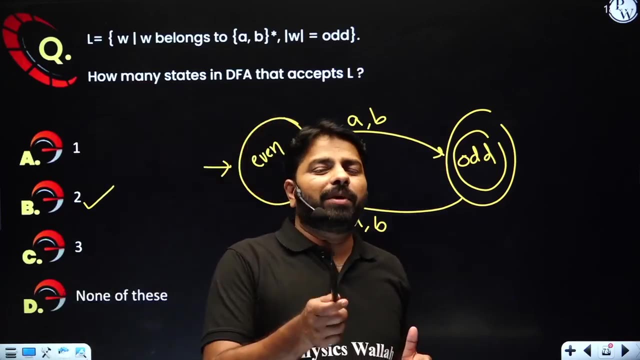 or length string, again two states. that means whether you find even length strings or odd length strings, the machine will have two states. only the final state will vary. i have one more relation between these two. okay, so first time i'm introducing that- the complement of a language. do you believe that? 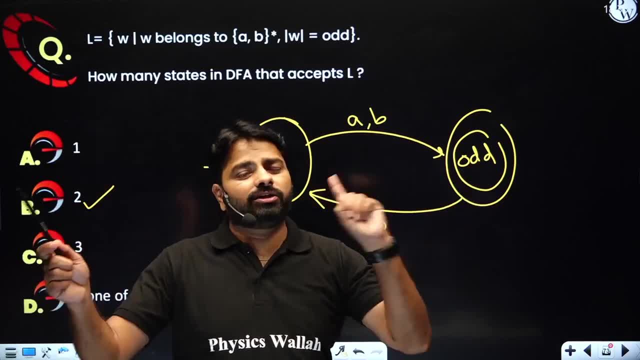 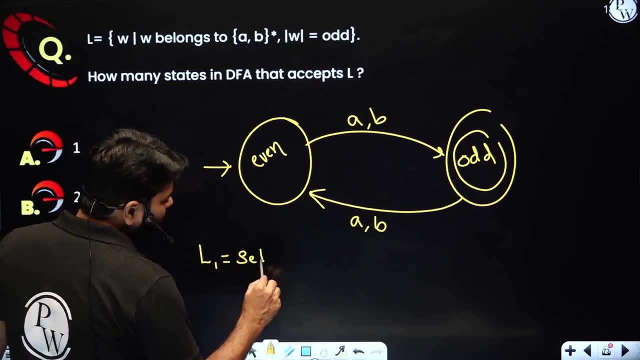 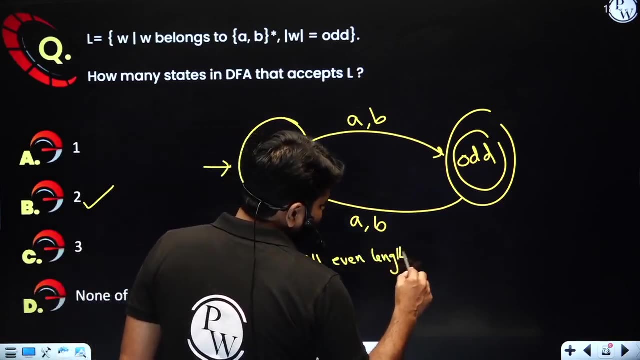 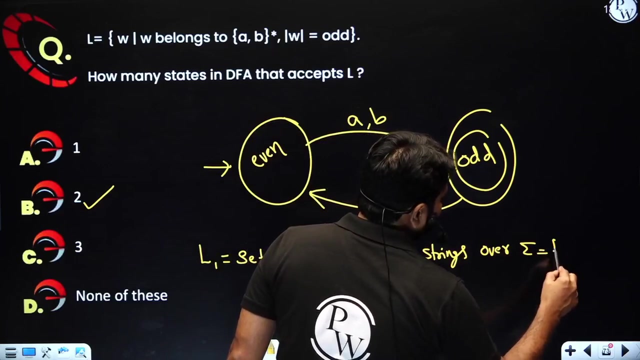 this uh question and previous question are complement to each other. okay, so let me explain the relation. suppose l1 is set of all even length strings over the same sigma. right, even length strings over the same sigma. what is that? a, comma, b. now this problem is our length strings, that is, let's say, l2. 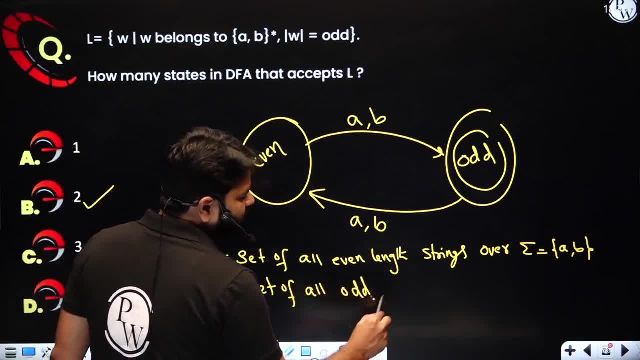 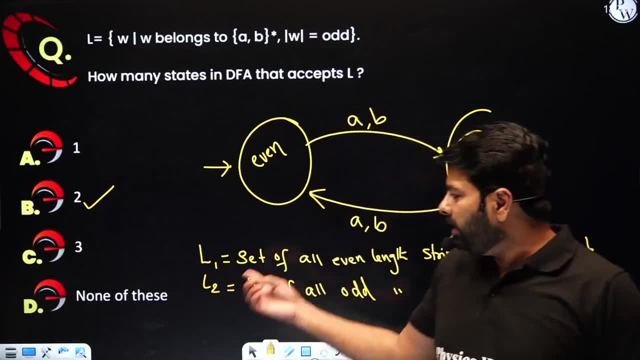 set of all odd length strings over same sigma. now what is the relation between l1 and l2? they are complement to each other. if i do the l1 complement, i'll get l2. if i do the l2 complement, i'll get l1. then what is the? 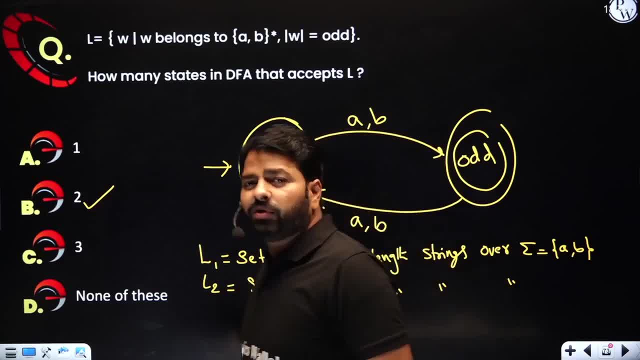 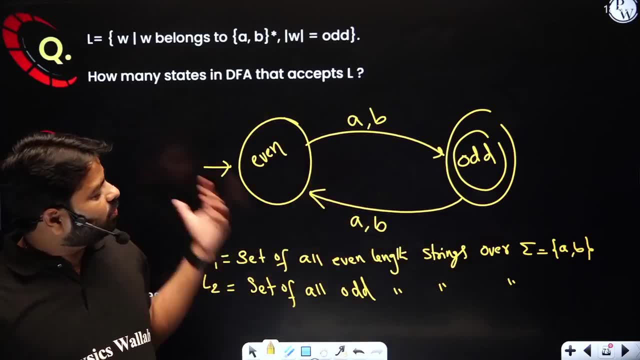 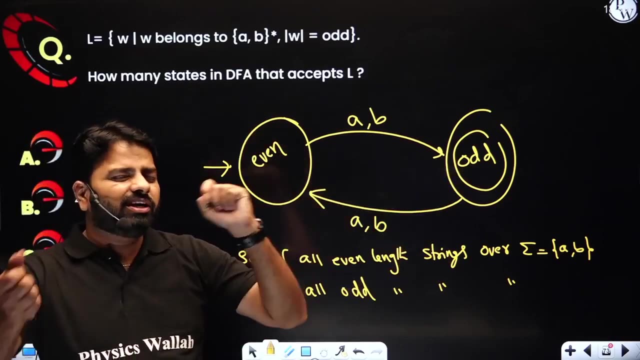 beauty of this concept is, if you know dfa for one language, that means you already know the dfa for another language. how is that possible? so look at the previous one, l1. when you want even length strings, this was the final and this was now final. just if you interchange, all the finals, you make non-final. all the non-finals, you make a final. 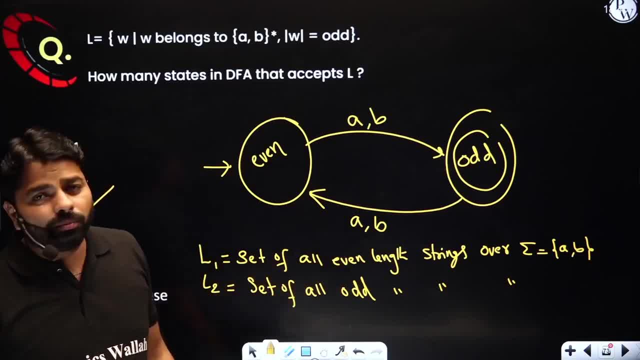 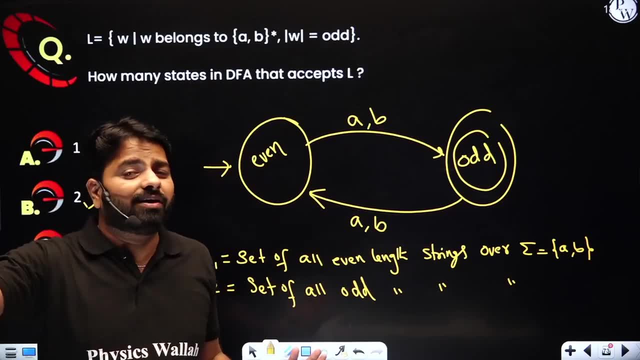 you will get the complement of the language accepted by the new motion. okay, so it's very important. it is applicable only for deterministic finite parameter. this concept please don't apply for non-deterministic machines. okay, will not work. so in deterministic machines, the complement of the 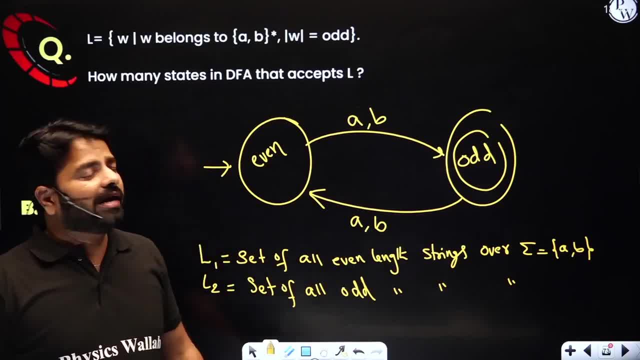 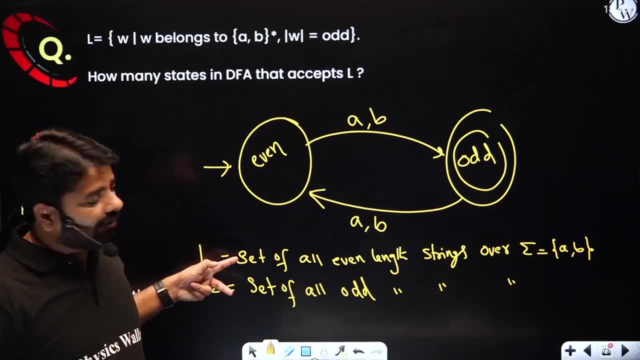 languages would be so easy. if you know the dfa for any one of the language, okay, these two languages are complement to each other. if you know dfa for any of these languages, you will get easily for the d for other language, dfa construction. so now you can just apply. what is the definition of? 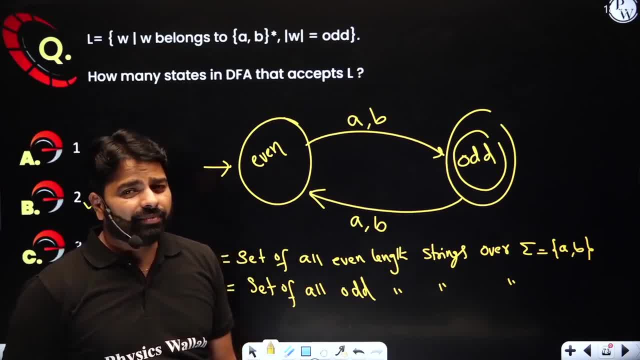 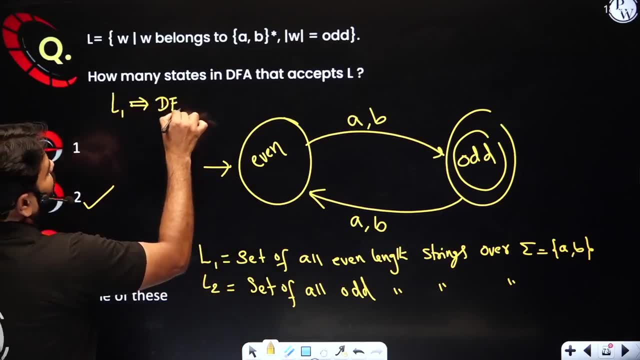 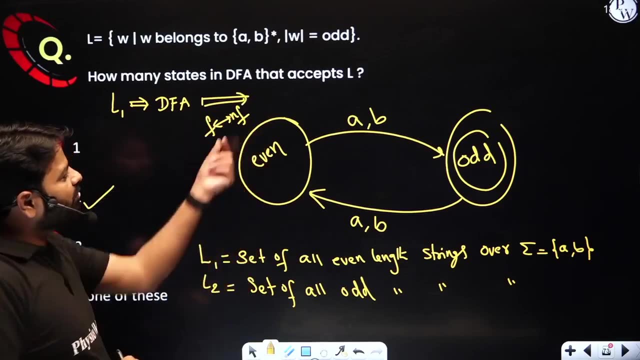 the complement of a regular language to design a dfa. if you know dfa for l1, i'm just saying for l1, if you know the dfa. what you do is just interchange finals and non-finals. f- nf means nf means non-final. 5, f means final. all the finals you make non-final, here only two. 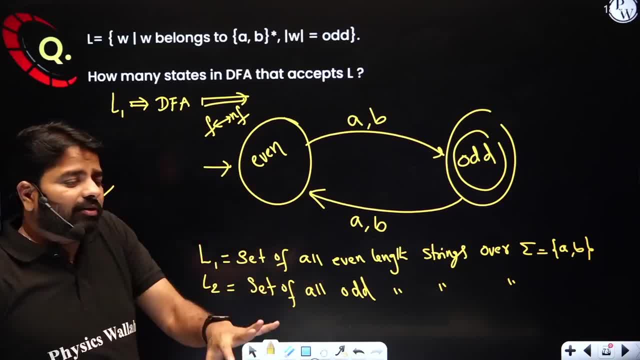 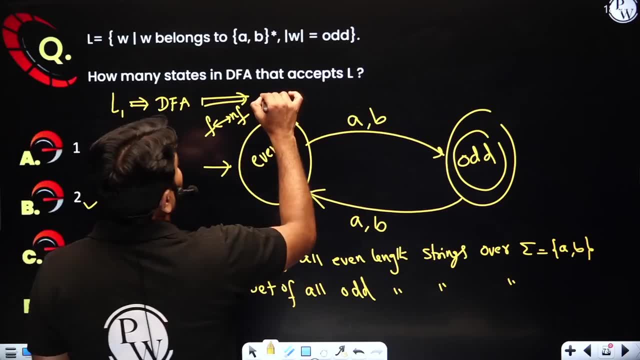 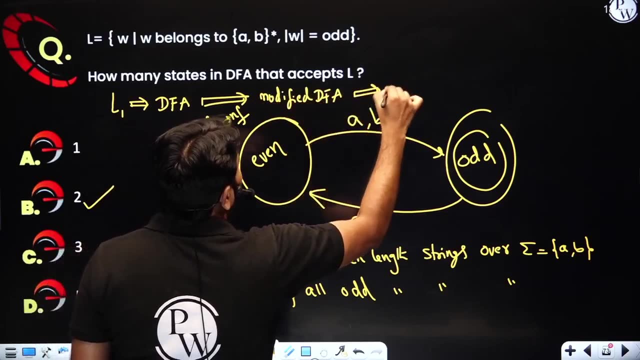 states are there, but you may have five states sometimes. whoever the final make non-final, whoever there is a non-final make final in the this dfa. so what do you get? you get some modified dfa. modified dfa: this dfa will accept l complement. okay, i've seen some people saying that complement. of a motion. we don't do the complement function of number five or seven. we don't find an infinite dfa in the commitment function. we find a complete complement thing in that dfa. we long after starter elbow of a step. we don't find a complete flological function. we welcome it. you see that at the bottom of the 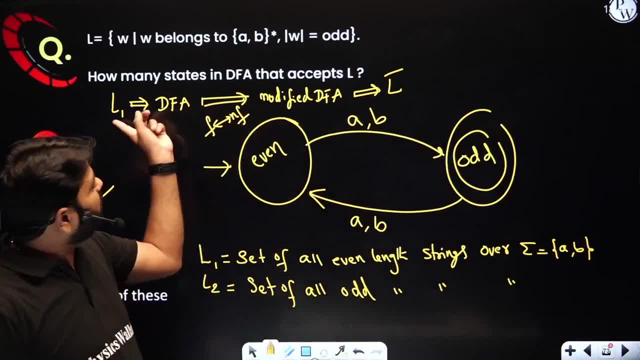 standard. we have schlicht level. we have step three to two, as we that standard type date. well, we'll create that dfa. so earlier we were now at the basic primary in this computer here in heavensbury we are using the for a machine. remember that there is no meaning for that. we do the complement for the languages. 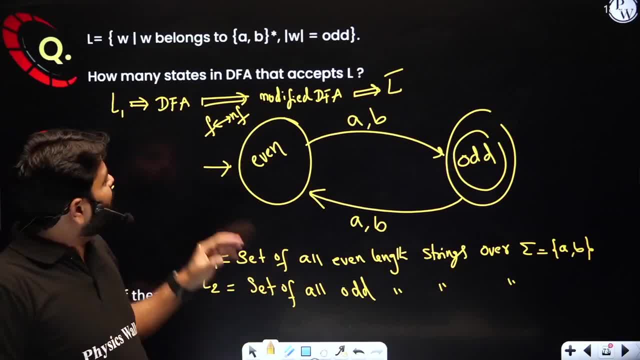 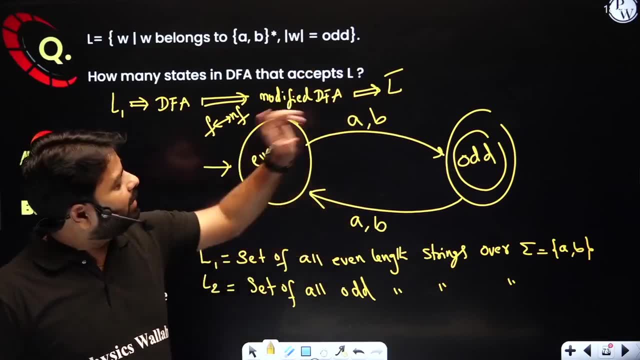 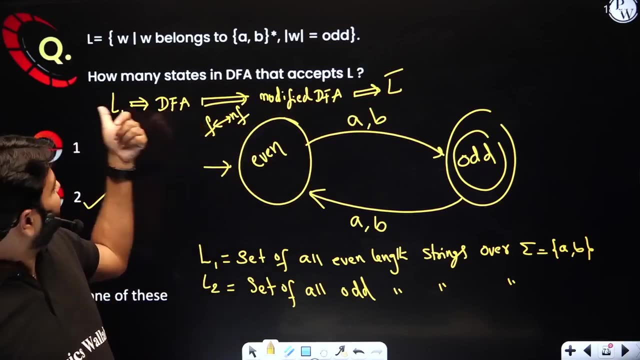 for that there is an algorithm to design a dfa. we take a dfa- interchange- final, non-final, we'll get another dfa that dfa accepts l complement- okay. similarly, if you have a machine for l complement, same approach: design a dfa- interchange, final, non-final, you'll get some modified dfa that. 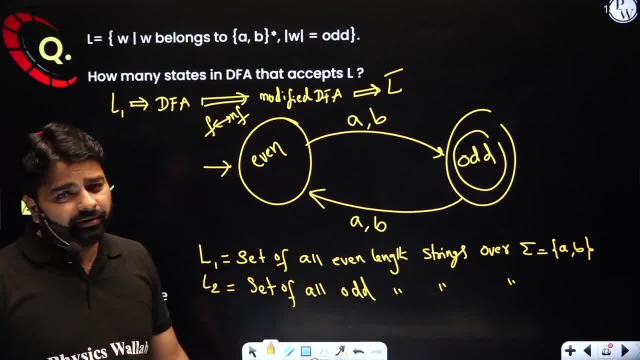 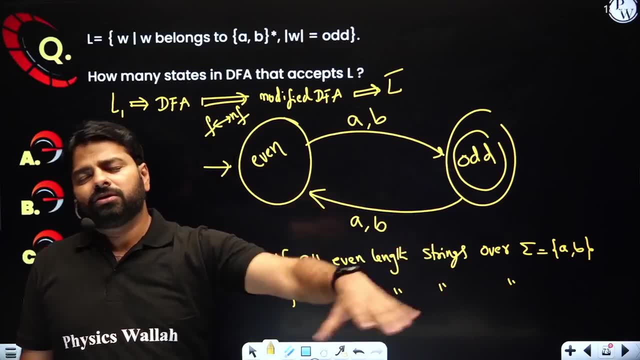 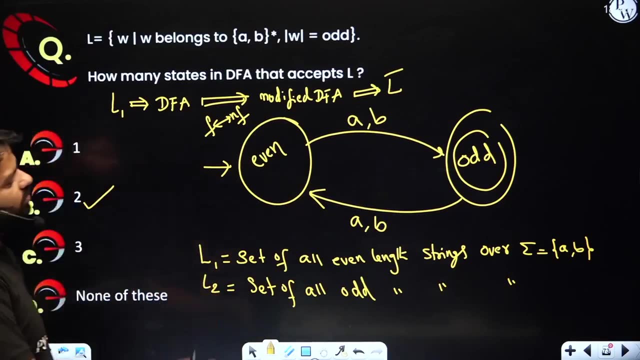 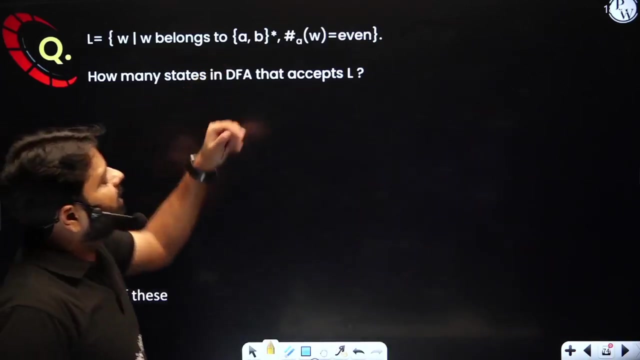 will accept l1, so conversely also it holds fine. that means, can i say that l is a regular language, then l complement has to be regular language. so many relations are there okay in this topic? fine, you have two states right, let's move how many states in dfa that accepts l, where now the number of, as is even not the length of the. 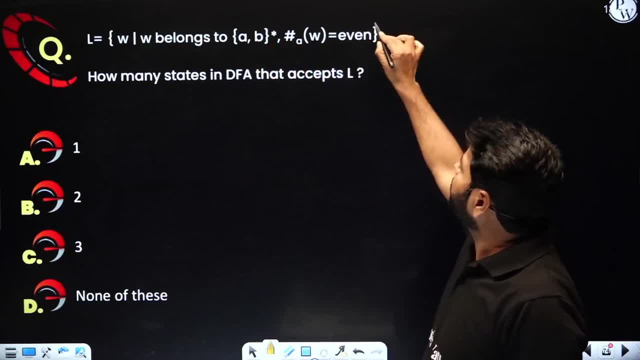 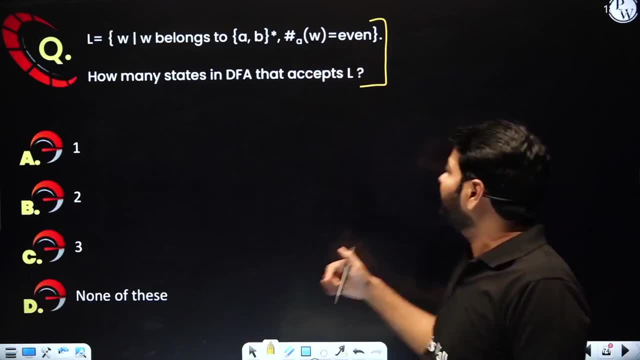 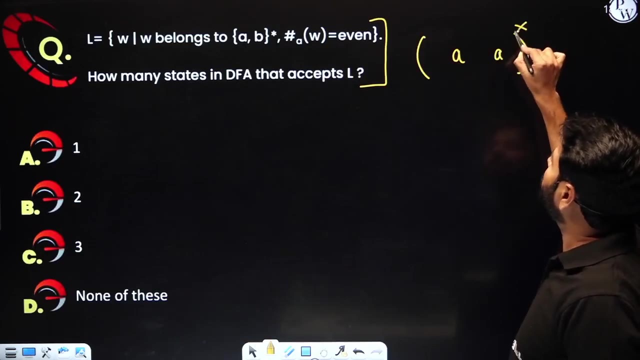 string. both are different. right number of as is even. can you write expression for this number of as is even. did you remember that? you know? you know many expressions i have written. right number of aces, even like a, a. this can be repeated any number of times. right, whole star, but b's can come any point of time here. 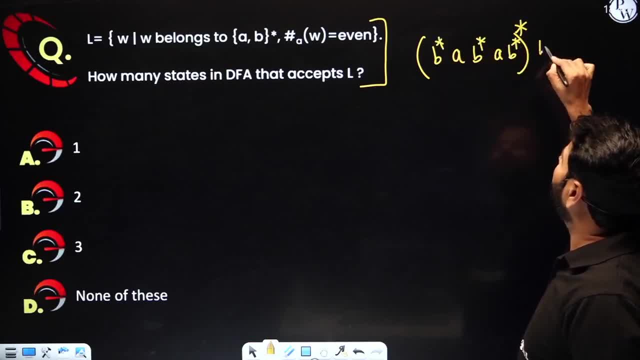 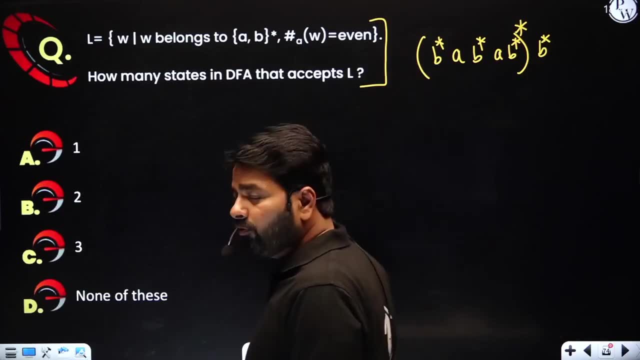 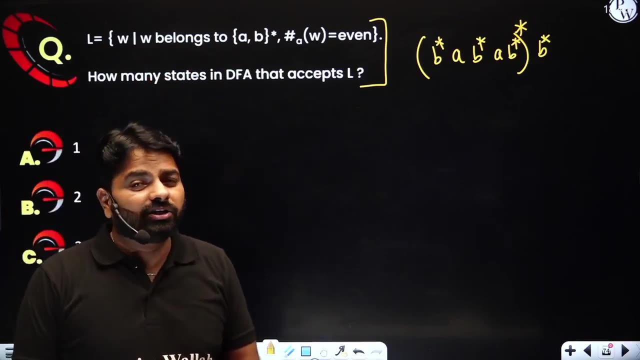 but obviously, uh, this would take much time to understand, no doubt right? so that b star you can write as a plus b star or b star. you can append here one more if you want it. so many equivalent expressions for this problem anyhow. but df is so easy, rather than expression sometimes. 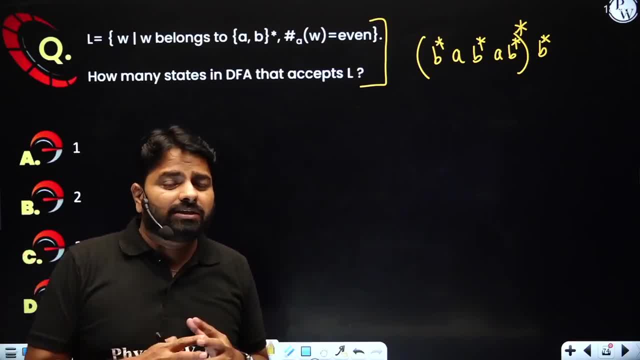 regular expression might be easy for you. as you know, you don't take much time to write, but sometimes dfs could be easy to design, sometimes even nfa, sometimes grammars. you know it all depends on how you practice, how you understand the approach. now come to the point, this problem. i feel dfa, so 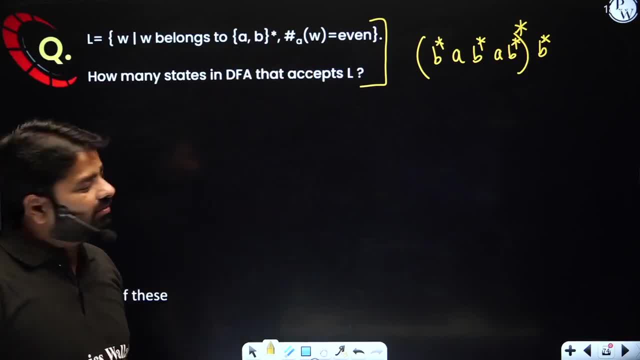 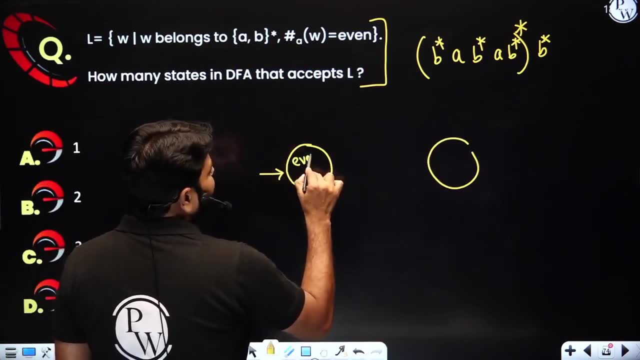 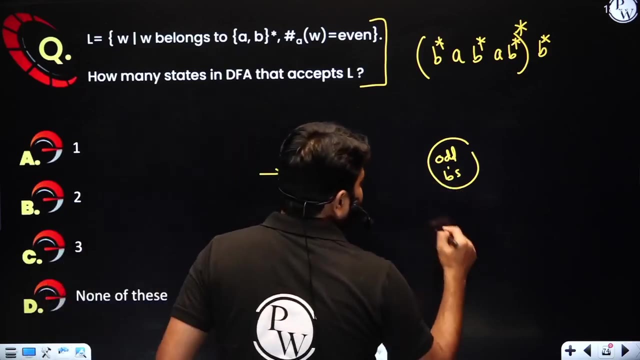 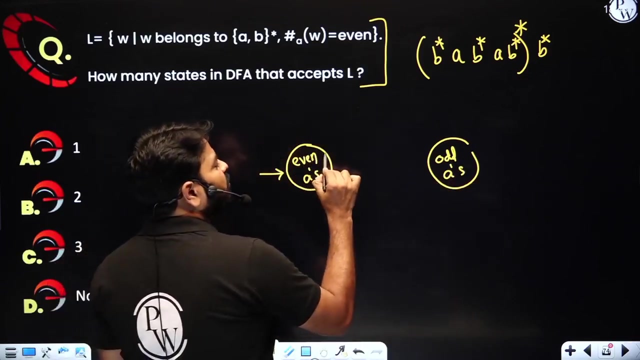 easy. why? see here number of aces. even now your focus is on number of aces, only right. this is uh for even yes a's only now. b's doesn't matter for me, sorry. odd a's now. when one a comes from here, i'll go to odd a. one more a comes, i'll come here. see here the. 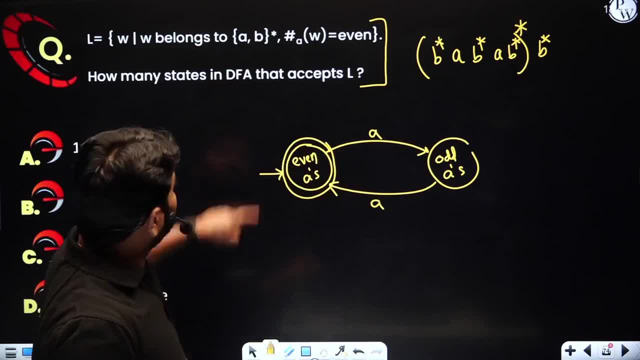 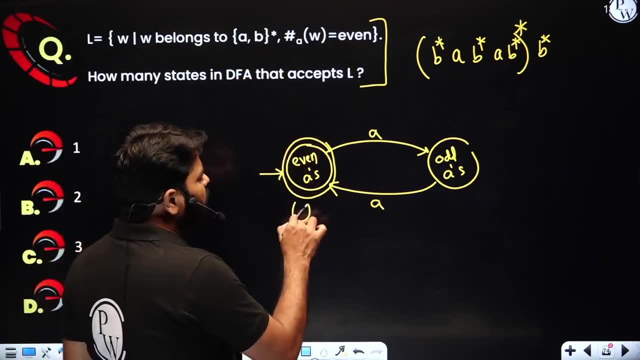 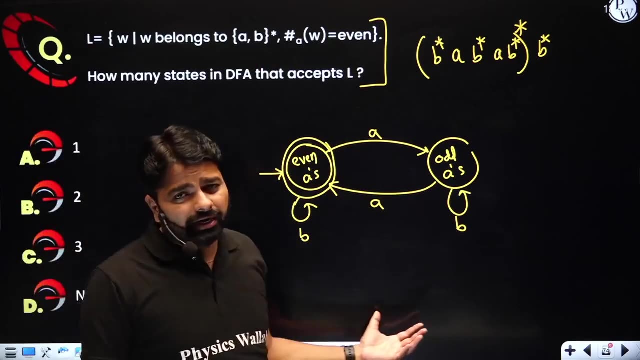 problem almost solved, but not complete. why? because b's also may come in our problem. b's may also come in our string. and what do you do from this? any number of b's we don't count from this, any number of b's we don't count. see that the problem is solved or not. i did not take much time to think about it, right? i should? 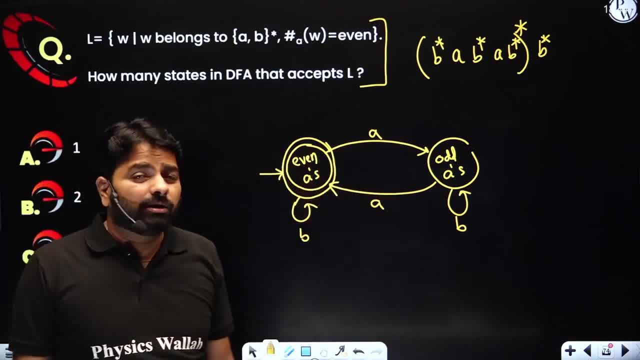 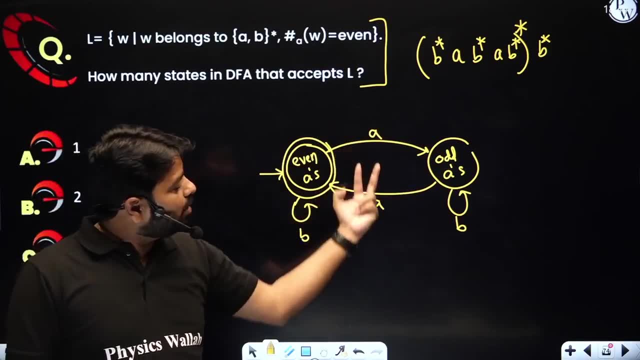 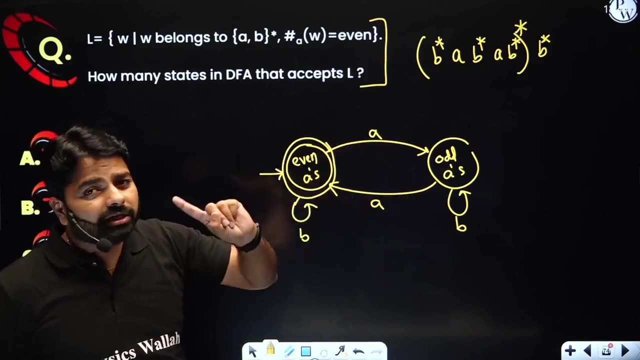 know how to you know, uh, understand the even number of a's, like i understood even length strings. now i'm understanding even years. if it is even length, i will write a comma b, a comma b here if it is even years only. yes, i will do. i will take a transition because i have to remember a is not the b's, b's can. 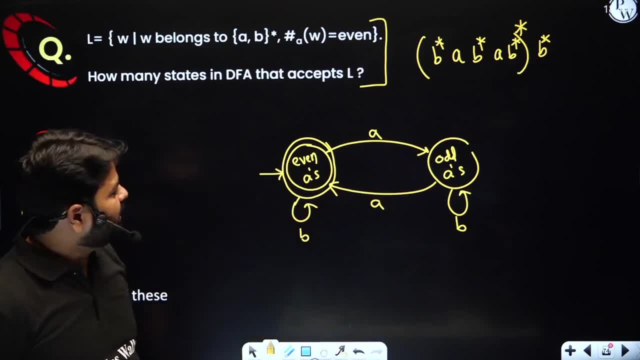 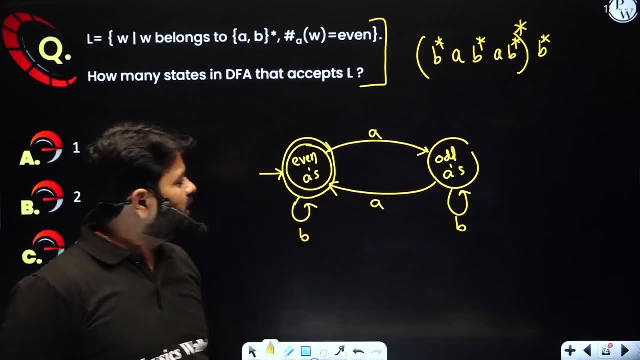 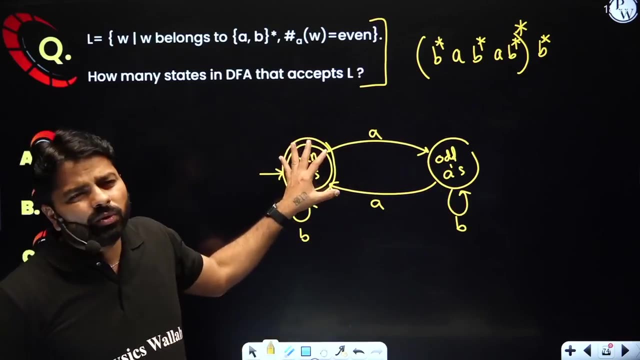 come any number of b's any time, right. that's why b's, we keep self loop and we don't have any condition over the base. that's why we have self loop everywhere. okay now, is it satisfying or is it accepting all the strings? who are having even number of a's? just see that when there is no a, 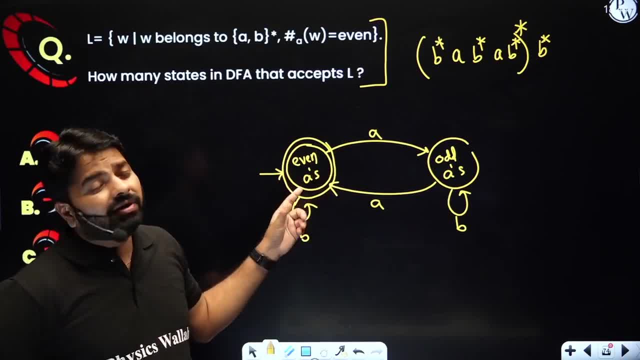 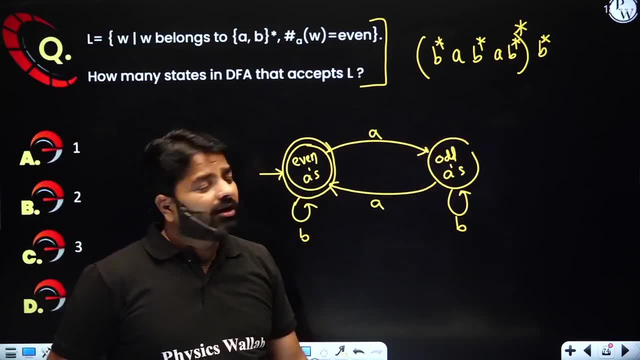 it might be epsilon, it might be only b's when there is a odd a. if one more a comes, then only it comes final. otherwise it will always here. okay, so this will definitely accept all the strings. who are having even number of a's? how many states? you need just two states again. 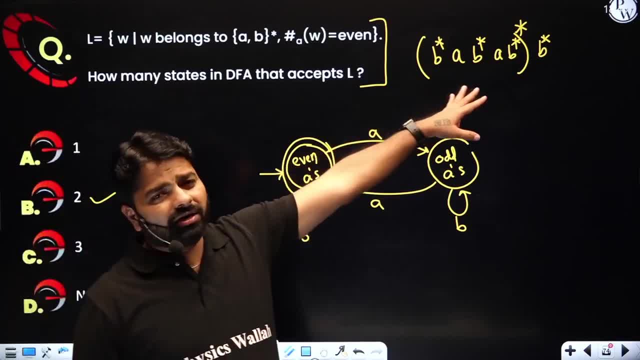 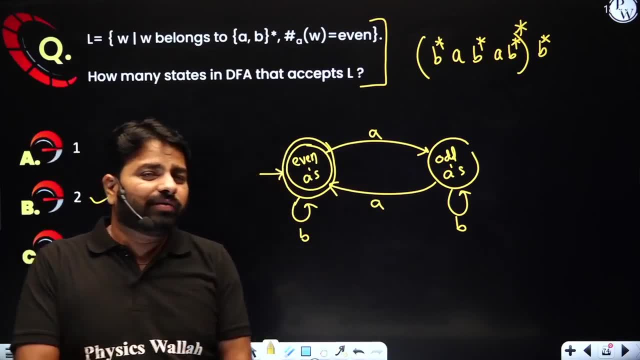 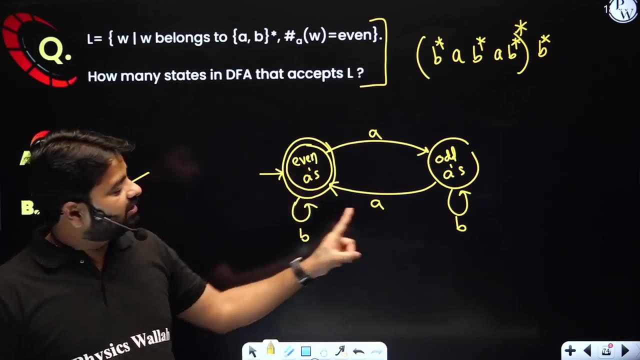 okay, would be easy. you know, compared to this expression, this motion would so easy for you because you have understood even length, strings, even number of a's and obviously similar, except this self loop concept, because b's have no condition. that's why we have a self loop. we are not looking for the b's at all. okay, how many states in dfa that accepts the all strings where each string is having at most three length. at the most three length. okay, i did not write an expression, but let's try. what is at most three is- did you remember this one? uh, sorry, it must be sorry- the at most three length, right? 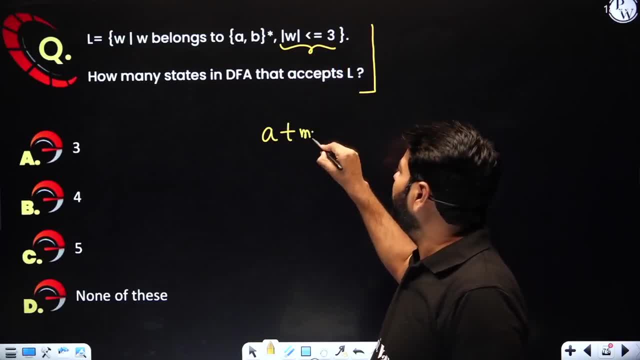 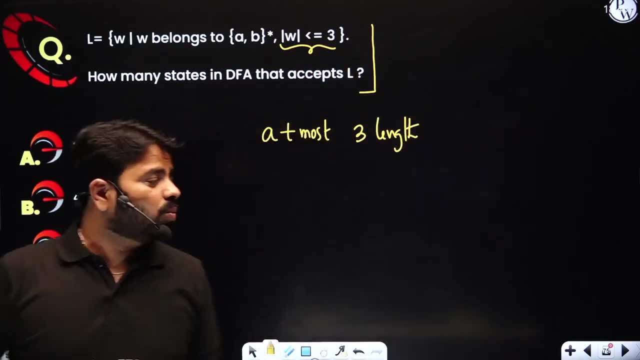 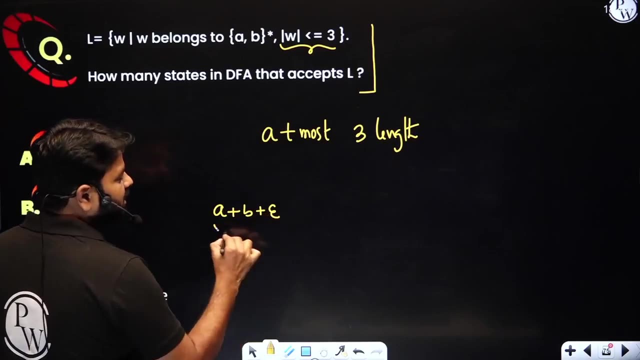 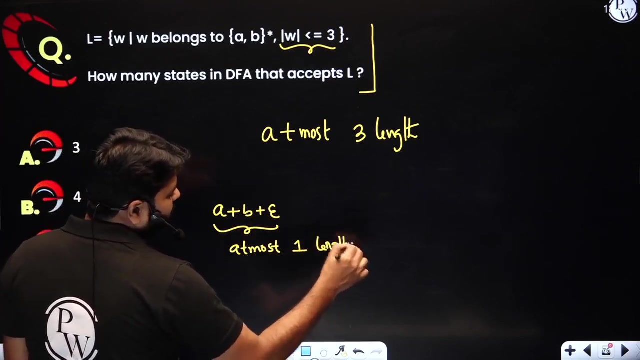 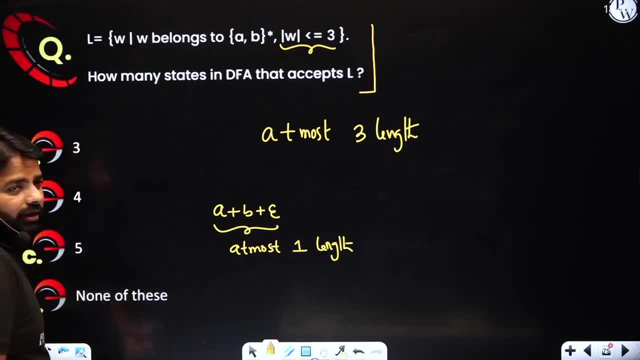 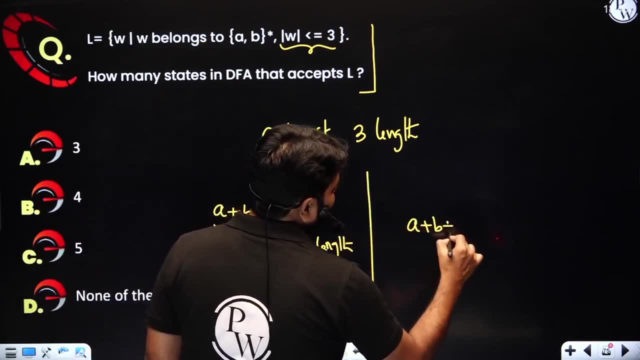 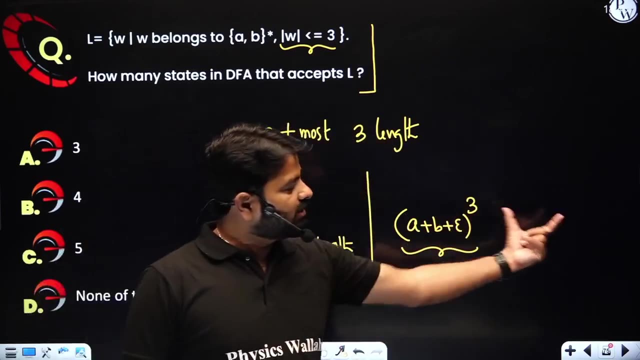 one means either a or b. now you want at most three length. how do you do that? this one only, you take three times in a sequence, that is a plus b plus epsilon. three times, that means power three, which will represent at most three length. when you write three times in concatenation, we'll get a plus. 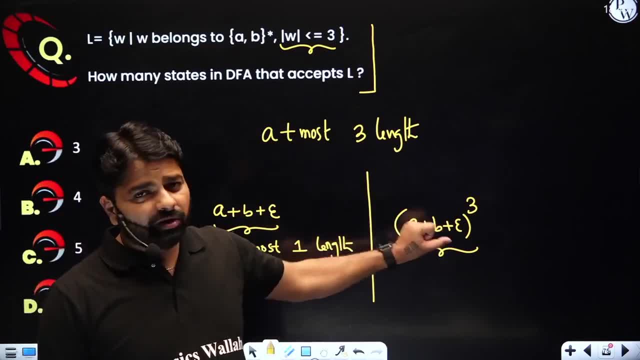 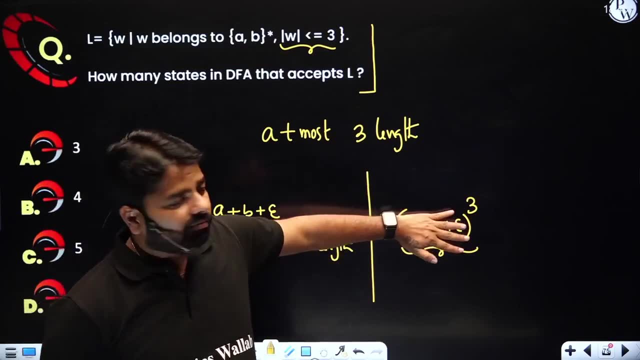 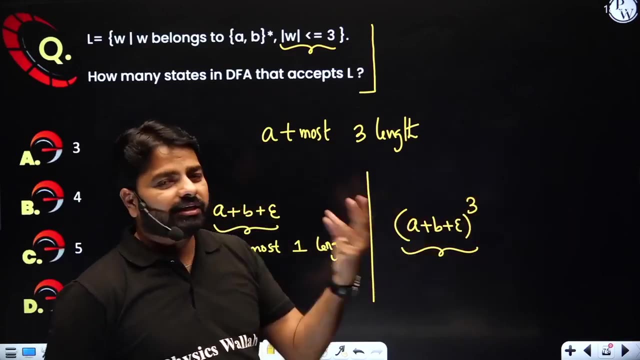 b plus epsilon, whole through all power three, which will be at most three length. in case, if you try to generate four length impossible, why a in power one and other power one. you can take a or b or epsilon, whatever it is. at most you can generate three length, minimum zero. how, everywhere you take. 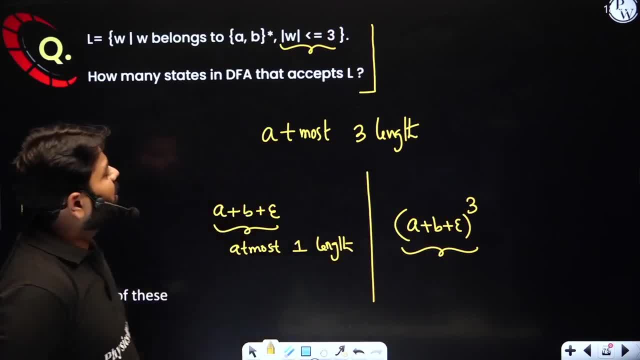 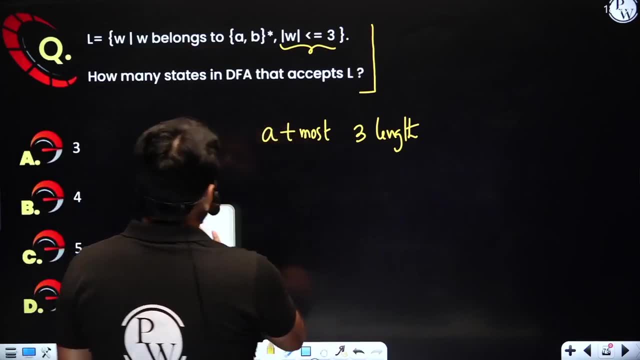 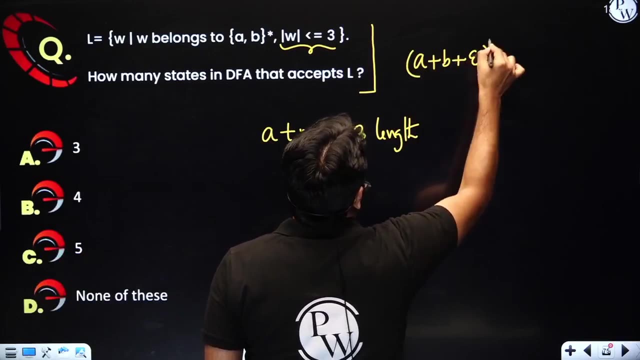 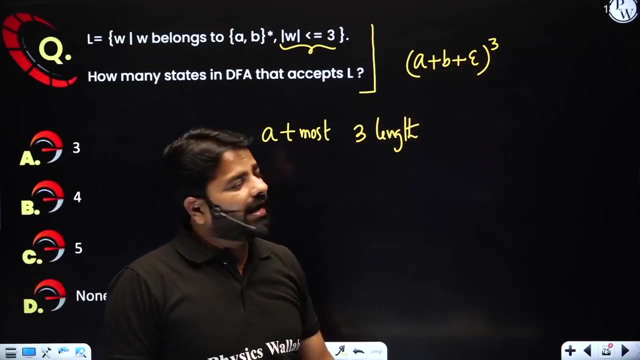 epsilon, you get epsilon, okay, so this is how what you can write of uh as an expression. now what is your problem? your problem is how many states in dfa? okay? concept is very simple. you have to track till three length. after that, anyhow, you don't have acceptance. the first, zero length is it accepted? yes, this will represent zero length. 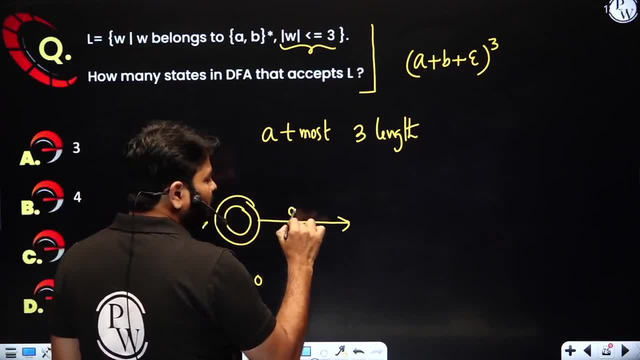 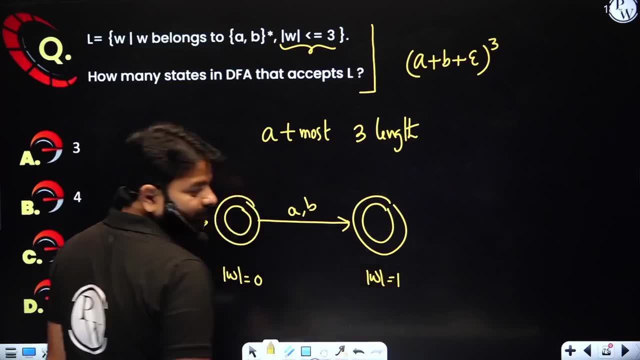 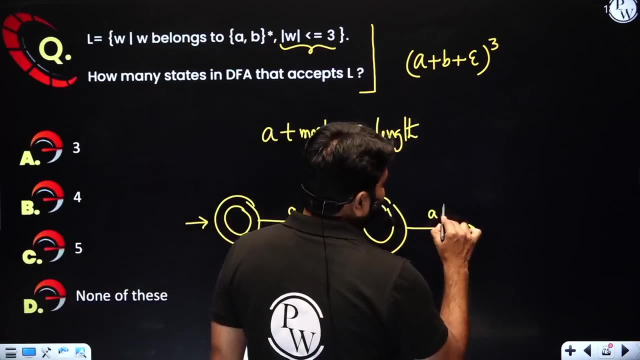 and one length. so you have to move it to remember that one length right, either a or b, you must go to the another final, but this one will guarantee one length. so if you have zero length string, halt here. if you have one length string, you halt here. two length string, you halt at third state. 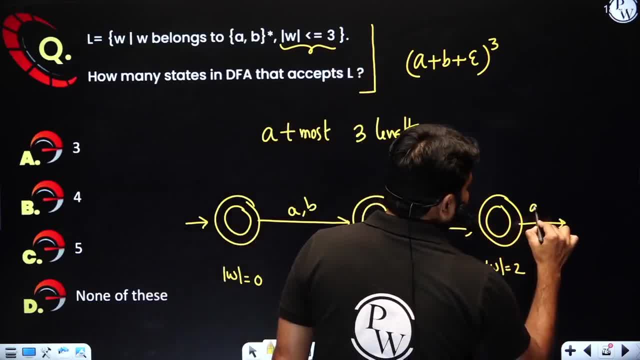 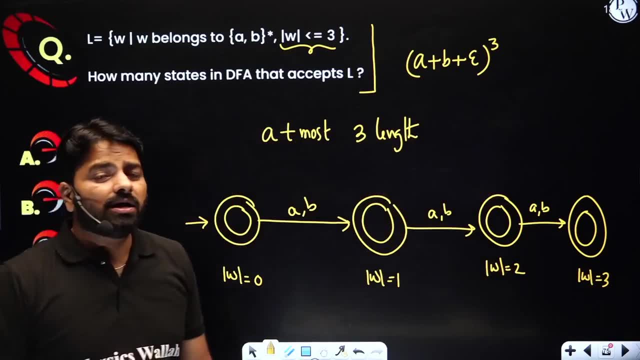 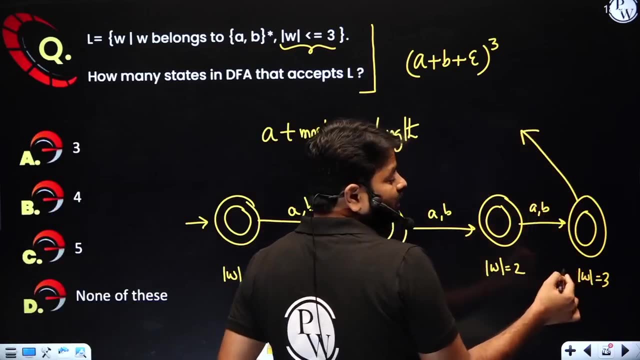 and three length you won't accept. yes, so three length. you go here and accept that too, but after that you can't accept it. so we have a special state called as dead state or reject state. now, any string or any length that is beyond three, you go to dead state and stay there itself. 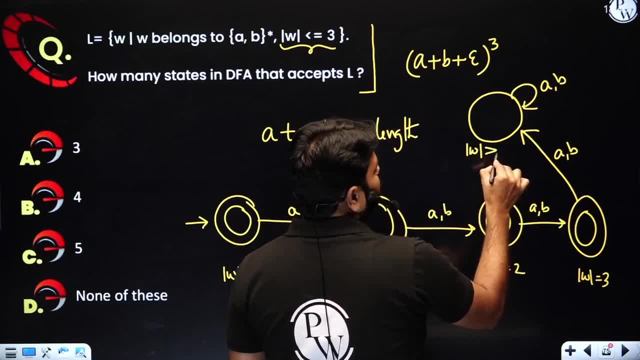 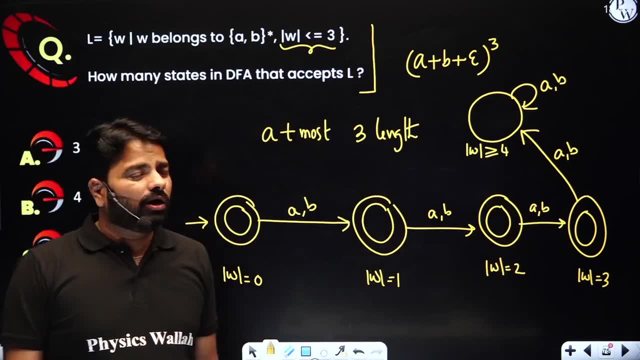 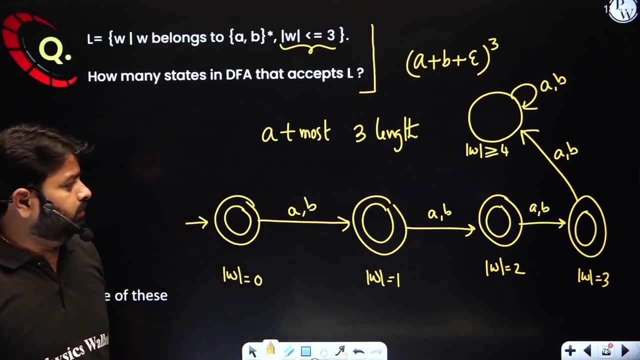 so this is length of w greater than or equal to four or get than three. you'd give any string in the world. i'll definitely have a path. how many paths you will have exactly one path. that's why you call deterministic motion fine. so at most three. length, so till three. length zero: one, two, three, you will accept. 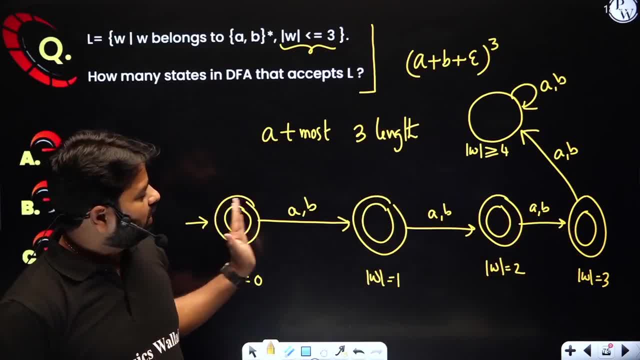 after three length you will reject how many states. you need one, two, three, four, five state and always you cross check after designing. did you made deterministic transitions from here: a, exactly one. b, exactly one, exactly one, being from every state, every symbol, exactly one transition should exist, not zero, not more than one. it should be equal to one, exactly one transition for every. 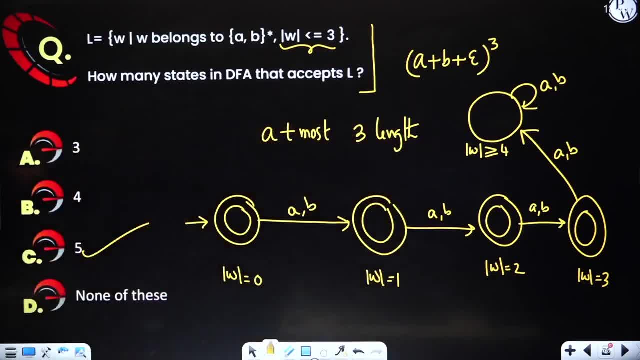 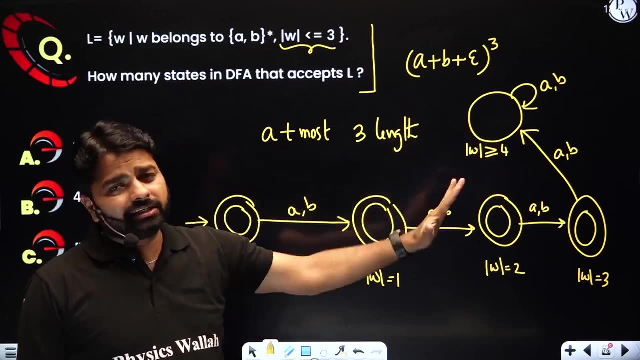 input symbol. so you will have five states. five is the right answer. right, and this dead state should be involved or counted in dfa. you can't ignore any state, any state, whether it is dead state or not, doesn't matter. if the dead state exists, you must count in the number of states as it is. 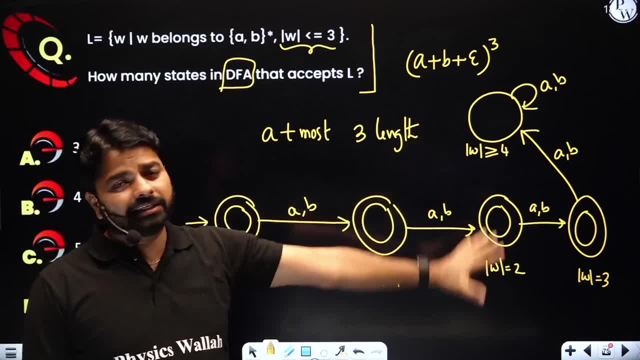 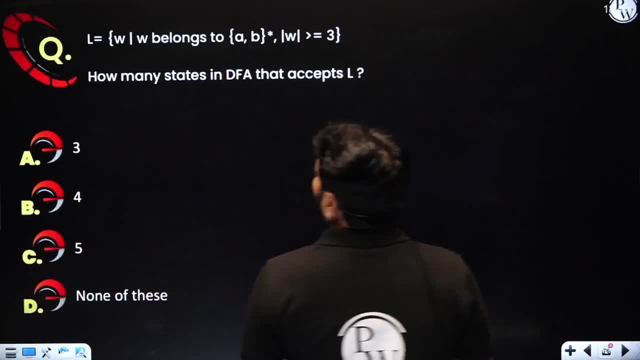 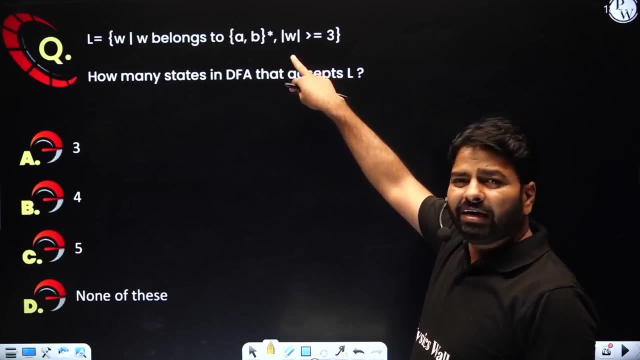 deterministic motion. it will always count if dead state exists. if not exists, you should not count. please try the next one. how many states in dfa that accepts l, where l is having all the strings, who are having at least three length, which is so easy? right, at least three length? how do you? 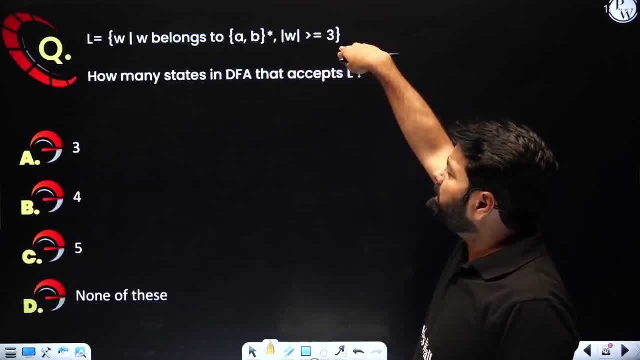 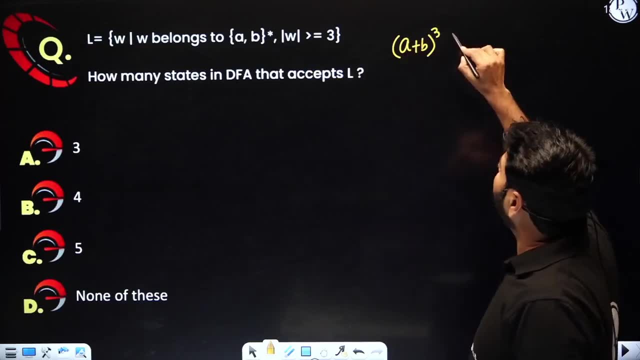 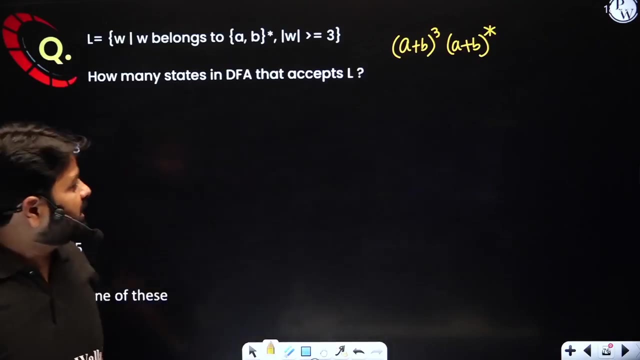 do that at most three. i have explained now at least three. how do you do that? a plus b, three length: you should guarantee minimum three, but after three length, length should be okay. so guarantee three length is there because there are many other expressions to represent this language, just very simple one: this will guarantee at least three. this will be 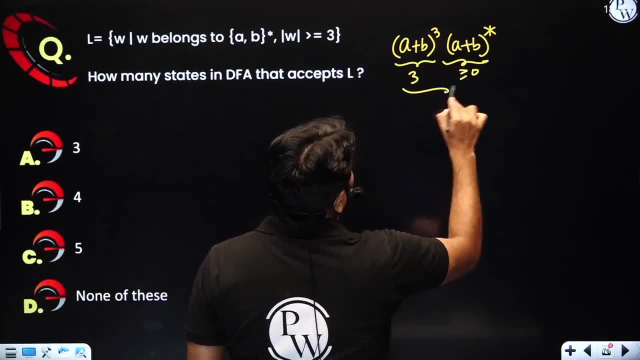 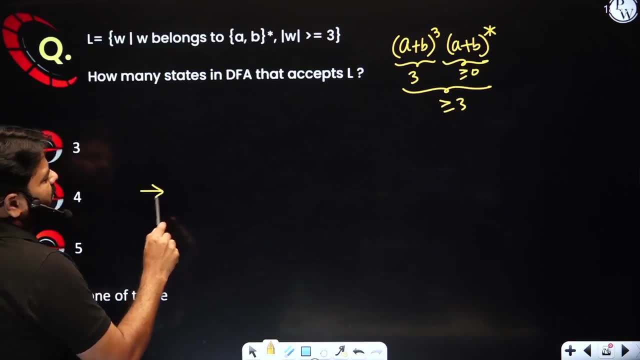 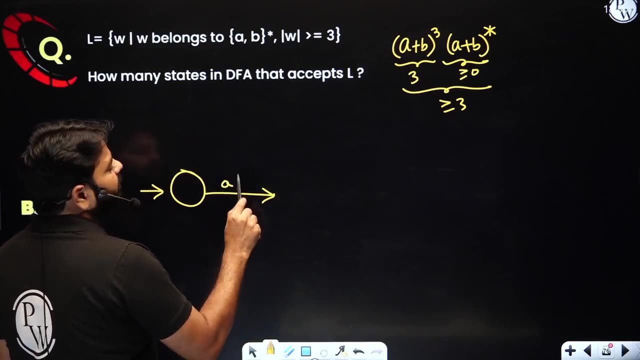 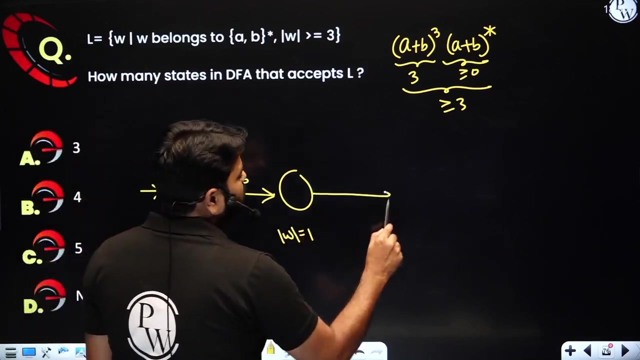 three. this will be greater than or equal zero will definitely guarantee greater than or equal three. fine, and now how to design dfa. already have designed, not takes much time, now at least three. so first go for the three length: a or b, one length, now zero length. i am not accepting one length. also, i am not accepting two length should not be accepted. 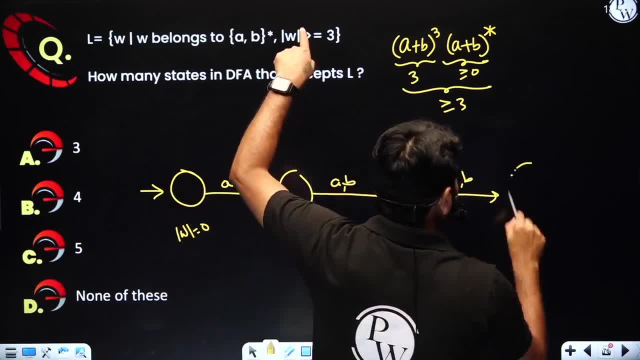 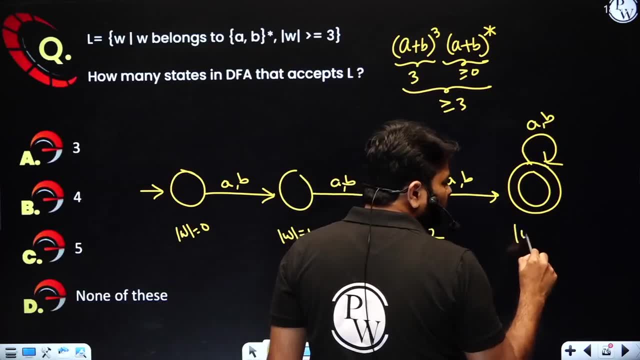 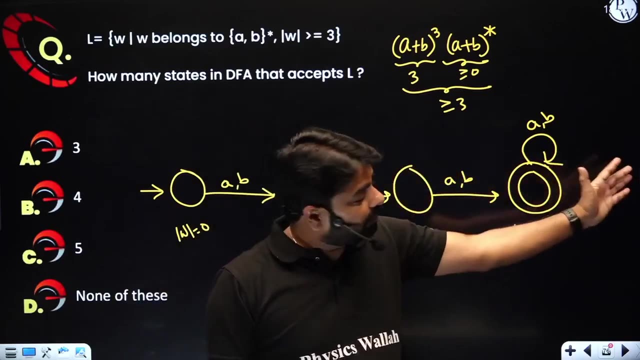 three length should be accepted because minimum three length should be, but after that every length or every sequence should be accepted. so this state is going to be greater than or equal to three should not go to the new state. why? because if you go for another state you are increasing the number of states, but we always design minimum number of states. 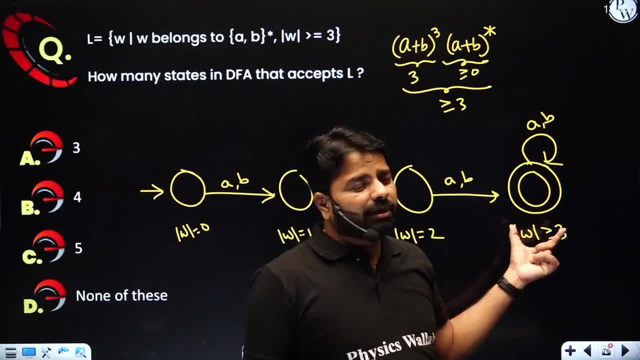 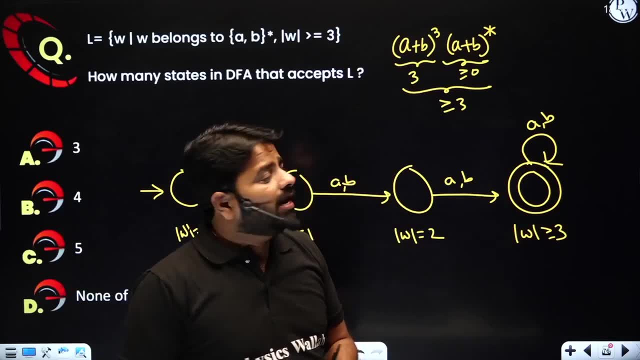 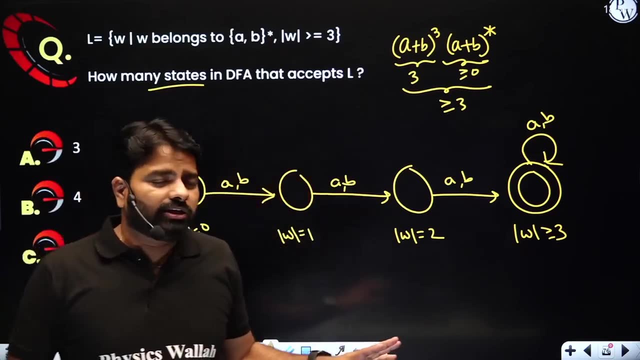 of states in dfa. that's why this dfa is minimum. in case anybody going for a new state, that is also correct dfa, but not minimum dfa. remember, in case you want to find the number of states, you should think minimum dfa, not just dfa, right, designing dfa is one challenge. the second challenging is: 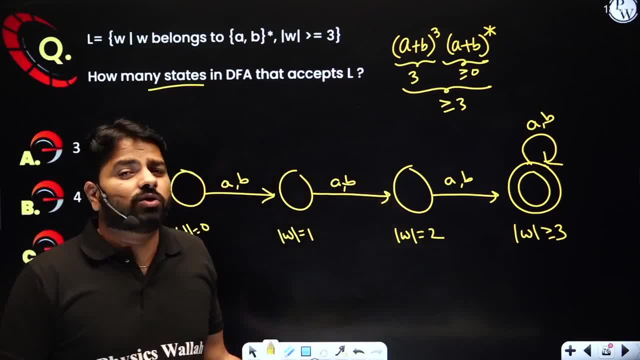 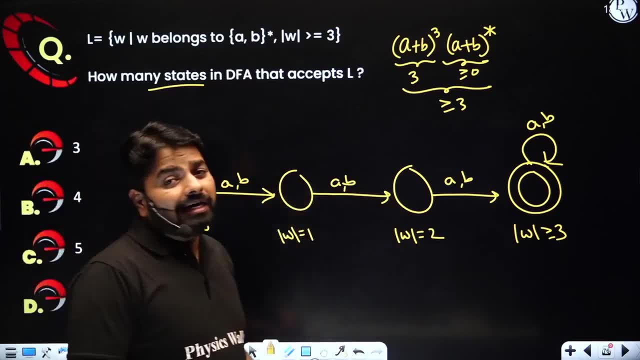 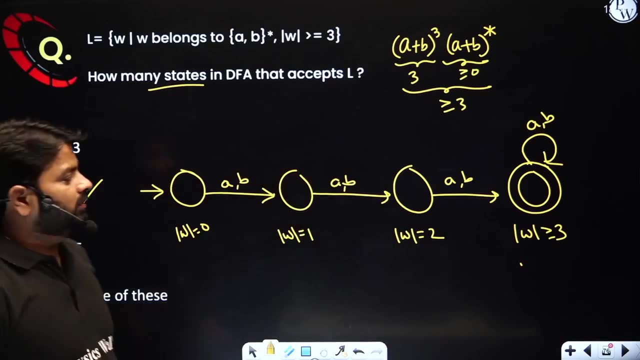 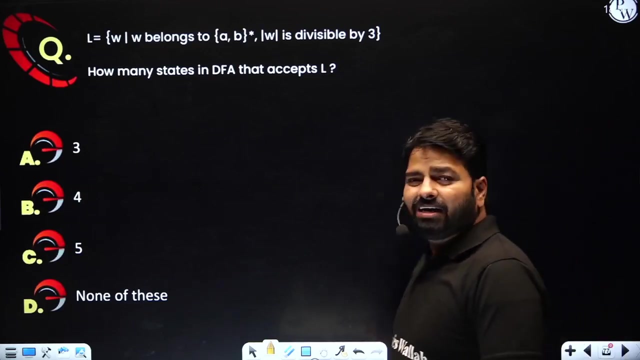 the i will design minimum dfa because your dfa is also accepting the same language. but that may not be minimum dfa sometimes. but how many four states where here dead state is not needed, dead state is not needed, so here four. okay now, uh, yeah, very interesting question where in the exam you don't need to design anything. 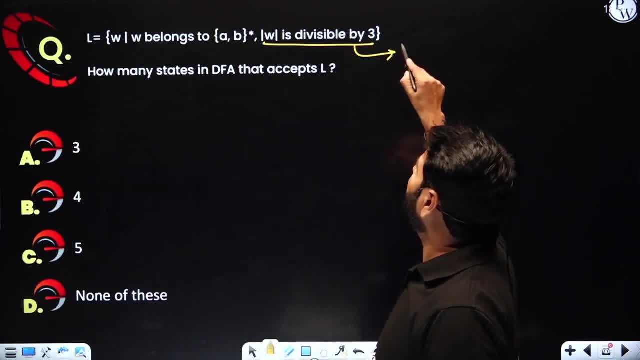 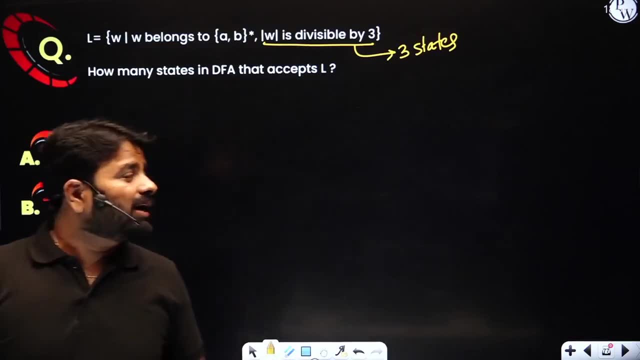 length of the string is divisible by three, then there are three reminders. so three states that's it. but anyhow, we should know how to design it right. length of the string is divisible by three. how do you design it? you know, when the string length is divisible by three, what are its remainders lengths? 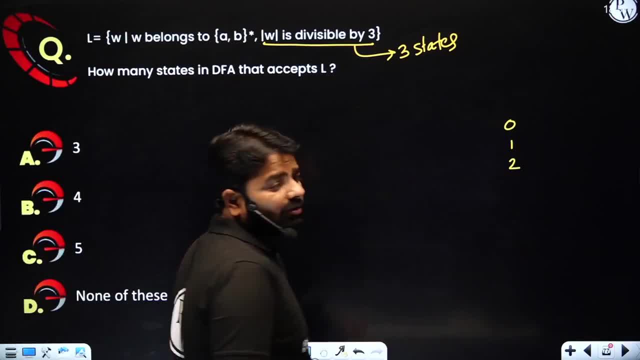 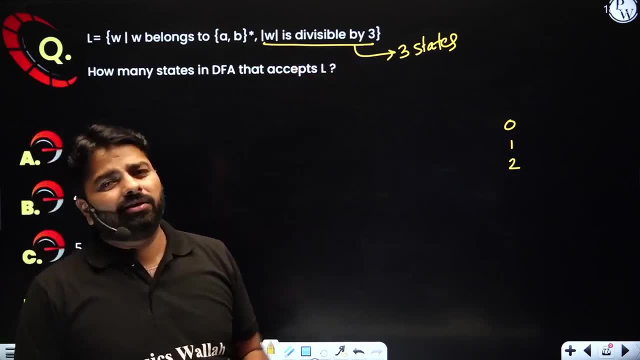 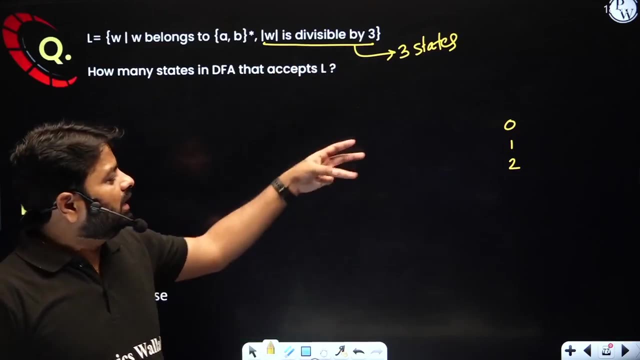 zero one, two. these are only three remainders right. when you divide any length with three: zero one, two. zero one, two, that's all. you take hundred length, hundred length divided by three, you definitely get the remainder one right. so somehow the remainders are three remainders possible. zero one, two. so there are three. 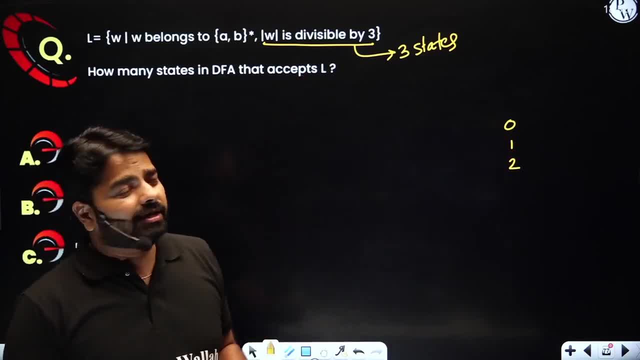 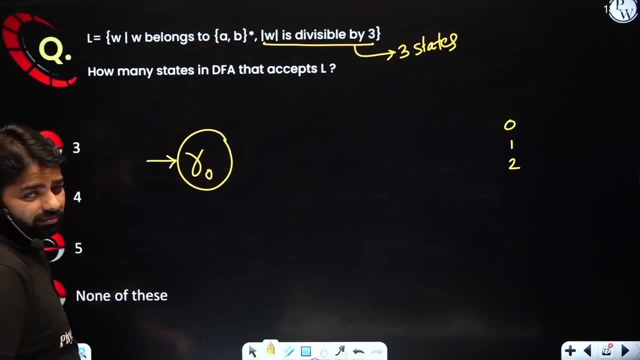 states maintained to understand that the length is divisible by three. so one remainder is for zero. let me say r0, which is initially epsilon, our initial state, r1 and r2. that's all now. these three states would be sufficient to understand the length of the string is divisible by three. 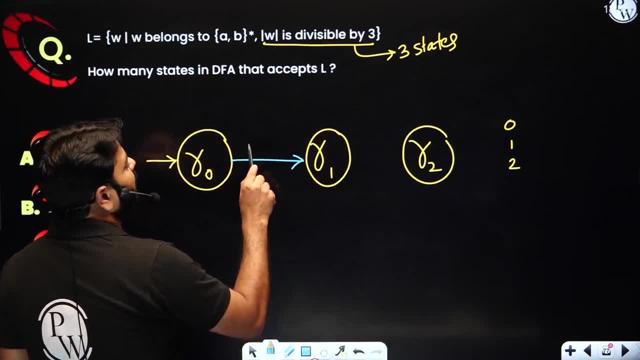 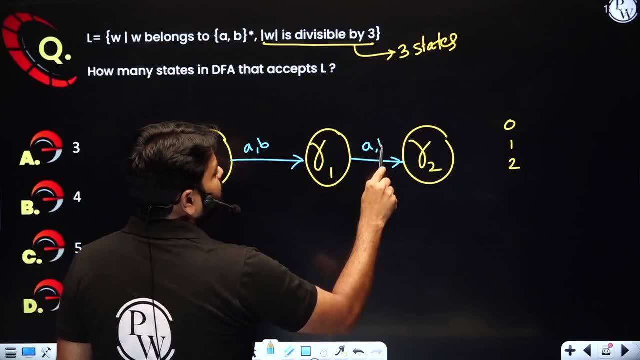 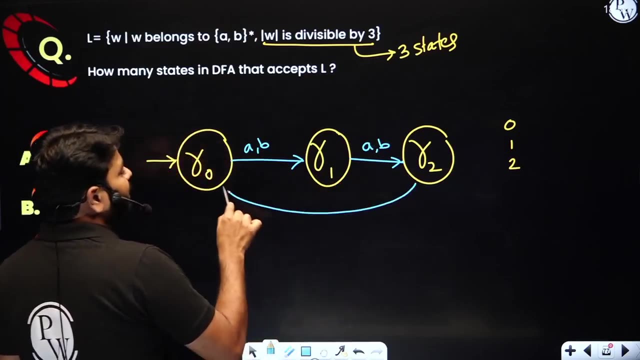 now see. this transition will cover the one length. So remainder 1 comes when you divide with 3, the remainder 2 length or remainder 2 when you divide with 3, now when multiple of 3 comes, you will get remainder 0 always, because 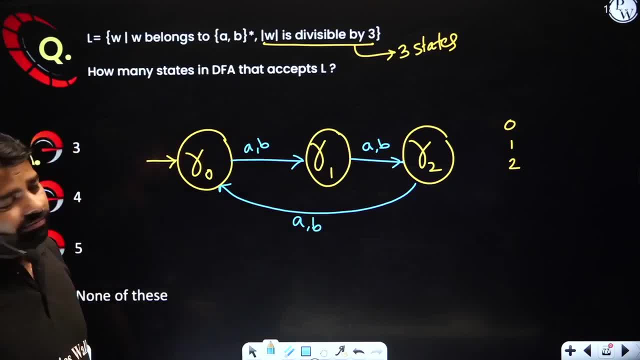 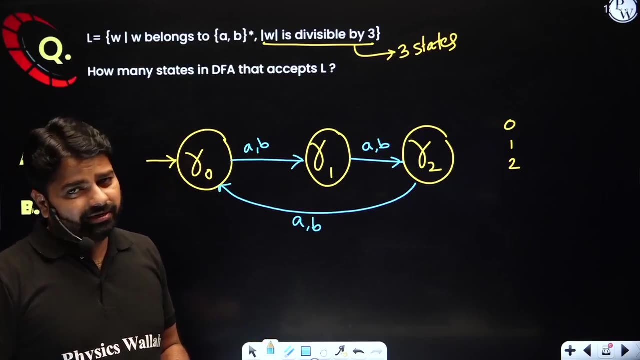 you are dividing with 3 and your problem is divisible by 3, any string length which is divisible by 3 must halted. finally, now tell me who is which state represents. which state represents? the string length is divisible by 3, so whenever the string comes here, that 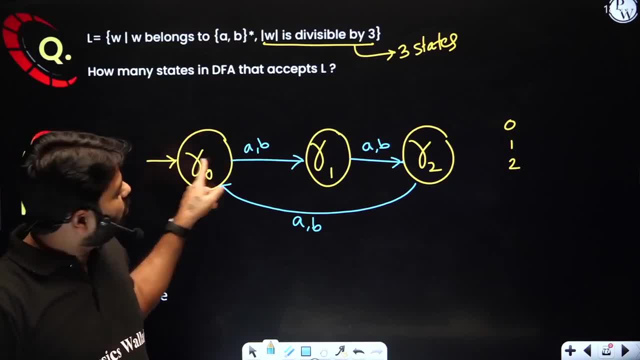 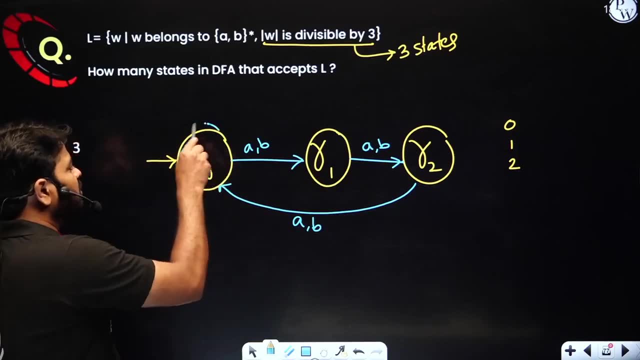 string length is divisible by 3, because the remainder is 0,, 1,, 2,, 3,, 4,, 5,, 6, every time is a multiple of 3, then you will halt here. so this r0 will be final. what is it? r0 will? 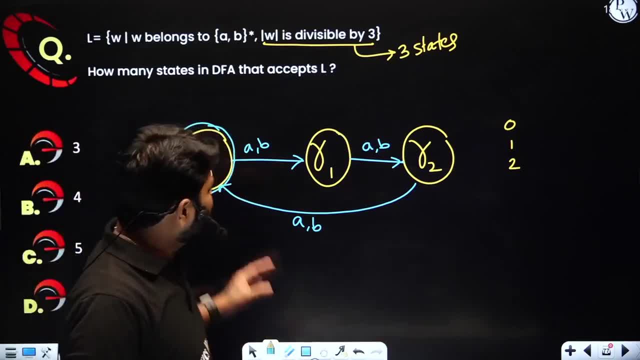 be final. here every state has a meaning. in case if you make r0 is a final, that is divisible by 3,. in case if I make r1, r2- both are final- then that is not divisible by 3,. 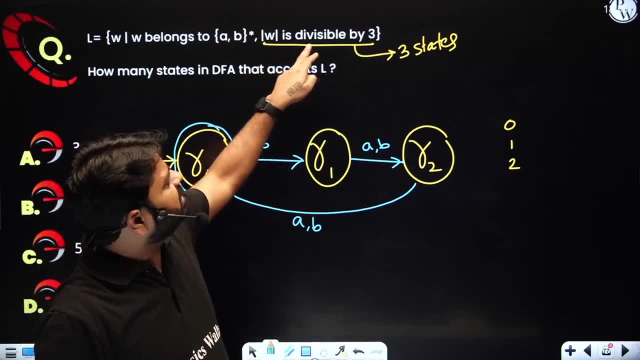 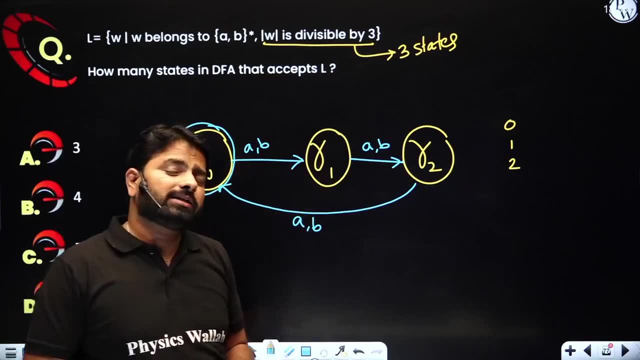 it is a compliment of this, no doubt. if I say length of the string is not divisible by 3, then you will make this: 2 are final. you may ask, sir, if I make only r1 is the final. what is the language? yes, so everyone has a different case, like: let us decide who. 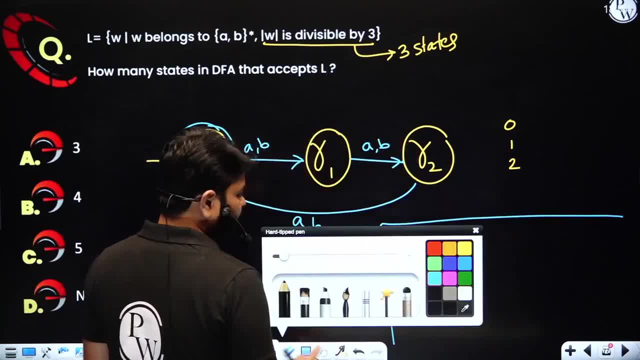 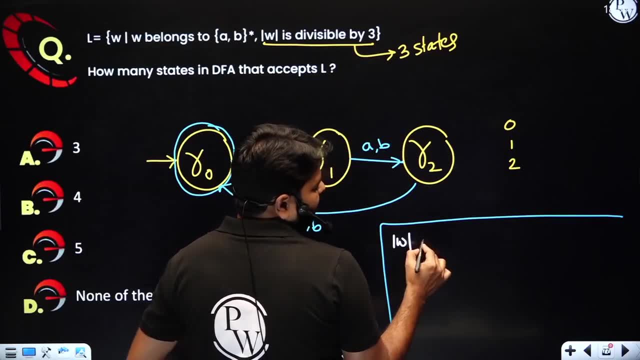 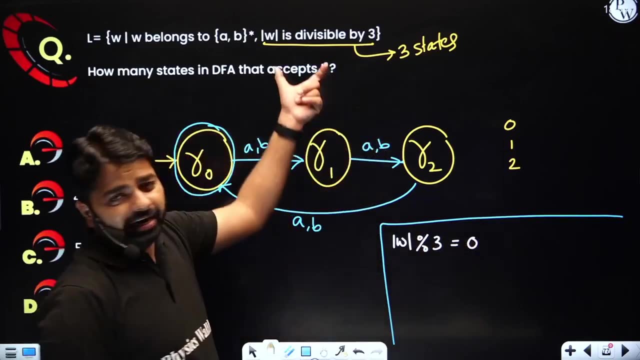 is going to be the final. for what situation, suppose you want to know? length of the w is divisible by 3, that is length of w. What is the difference? 3 is equal to 0. that is the situation, right. divisible by 3 means remainder 0. 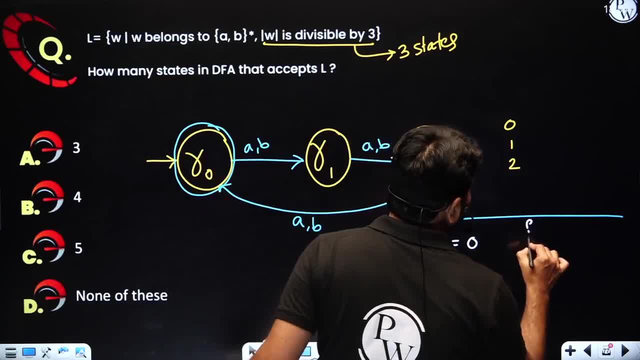 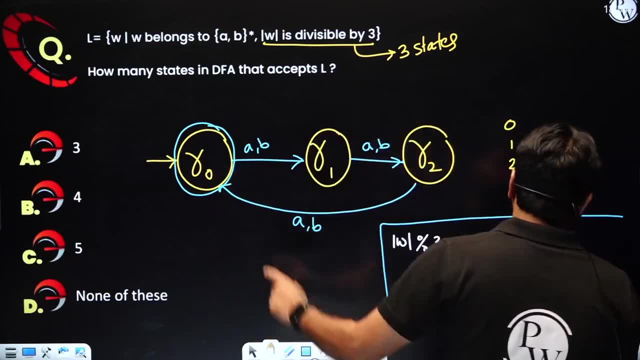 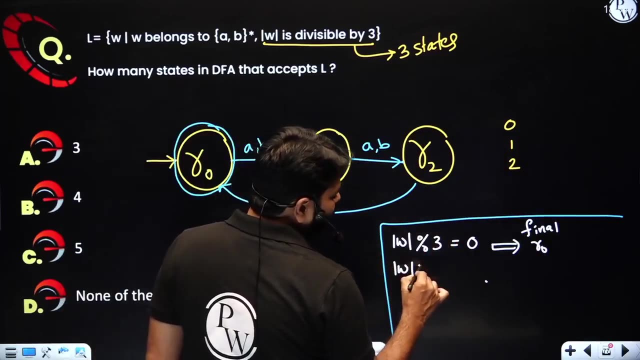 then in that case, who is the final? who is the final here? who is the final r0? okay, so i'm just designing only final states, because the motion is same. you suppose length of the w mod 3 not equal to 0. who is the final? r1 and r2. r1 and r2. 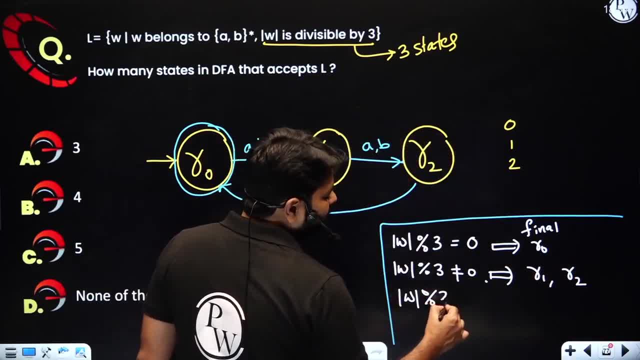 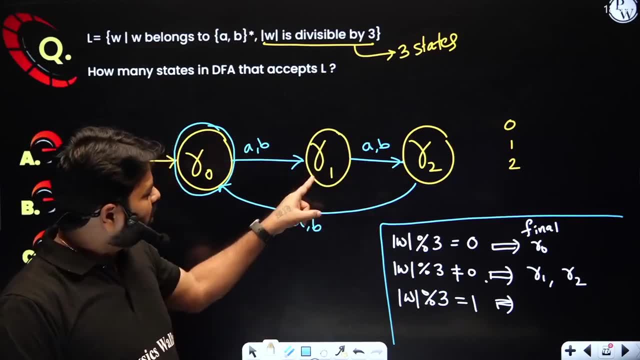 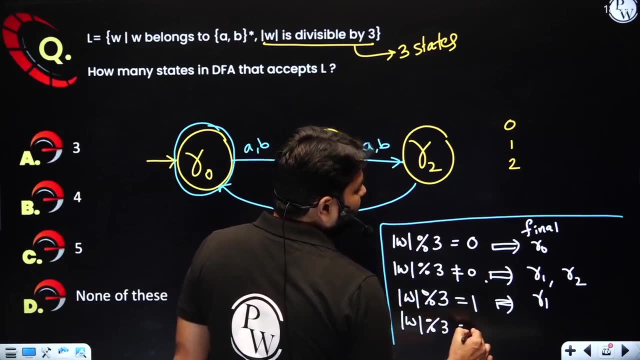 in case length of mod, the length of the string. mod 3 equal to 1 means remainder 1. in out of this 3, who is going to represent remainder 1? r1 will make r1 is a final length of the string divided with 3. you got remainder 2. then you will make r2 is a final. it's also simple to design a. 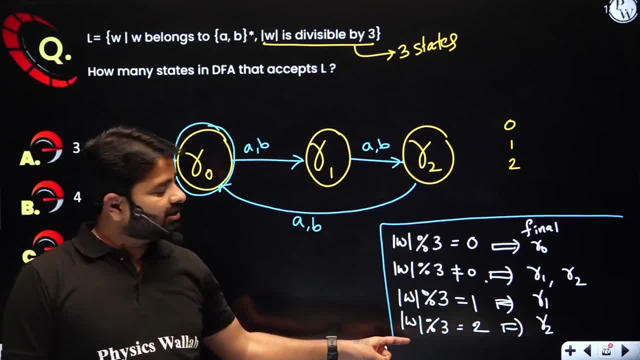 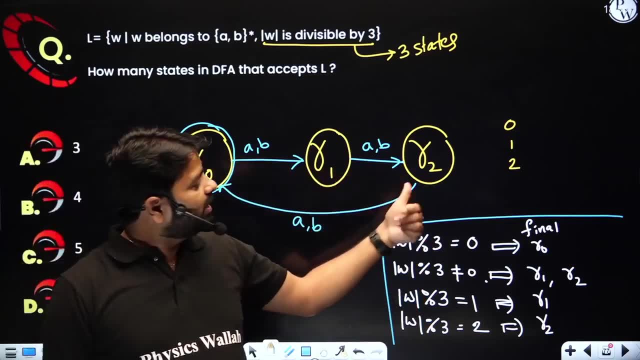 dfa, which is going to accept different strings based on the modulus condition condition. with the remainder of the string, you will get the length of the string, which is equal to 1 remainder 0. make the 0 is final remainder 1. make 1 is the final remainder 2. 2 is the. 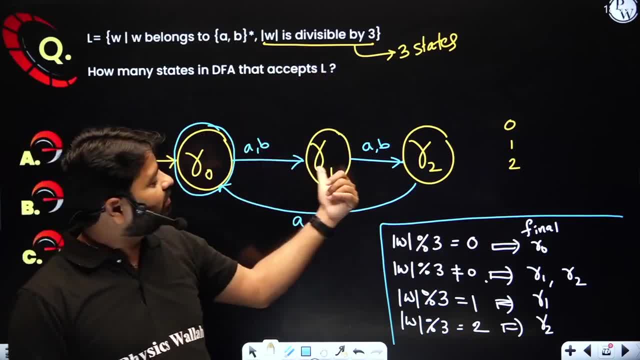 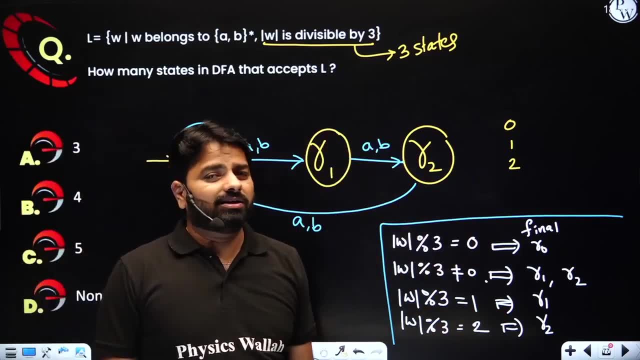 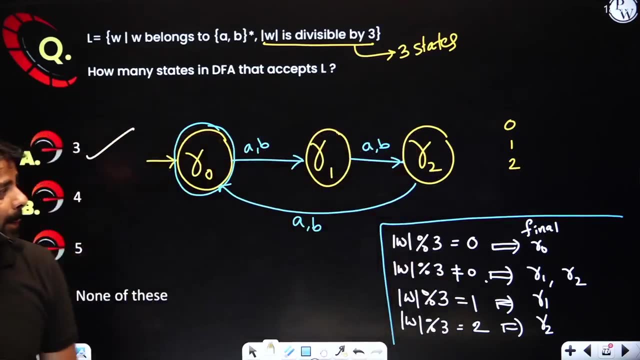 final. if remainder is not equal to 0 means not divisible by 3, means 1, 2 are final. so so simple to design such dfas. but over all of them, the number of states are. number of states will be 3. number of states is 3. easy, okay, let's move on. how many states in dfa that? 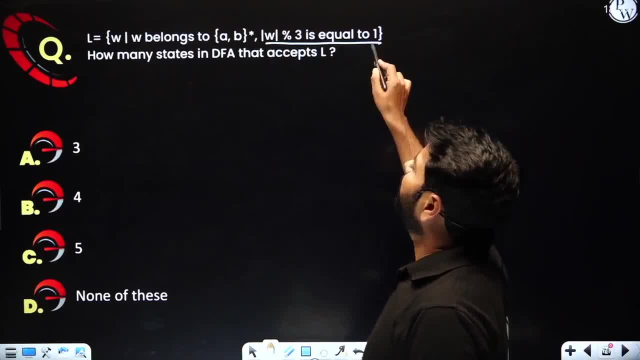 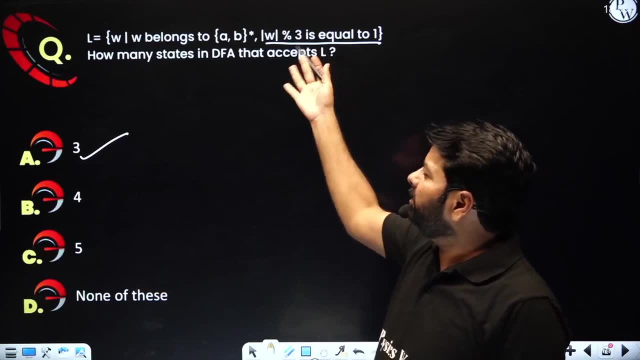 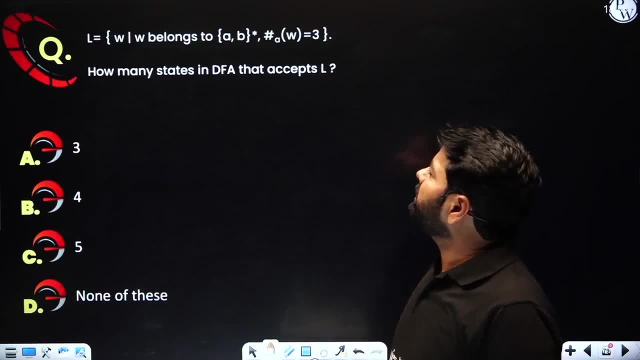 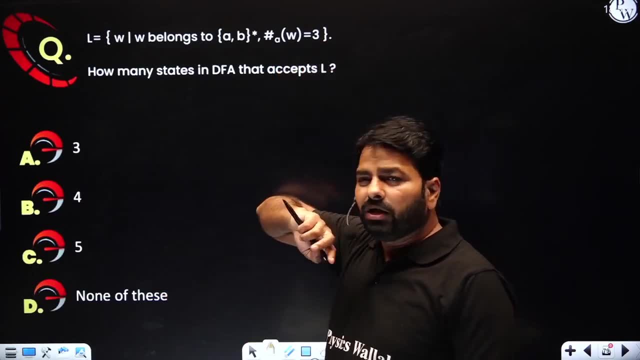 okay, this is a different question. it's not about the length of the string, it's about number of a's. so slightly change. the problem is: number of a's in a string is equal to three. now what would be the regular expression for this? what would be the regular expression for them? how many a's? 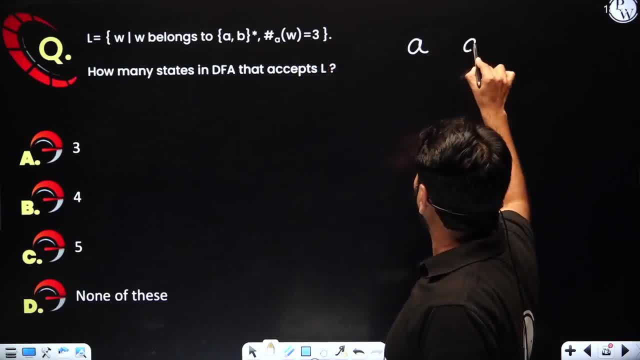 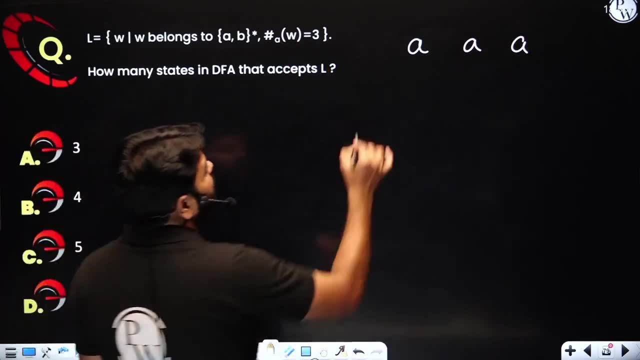 is exactly 3, so 1a, 2a, 3a, 3a is exactly, but how many b's? don't know. any number of b's can come, so you just write b star could come. any number of b's can come before first a or in between the. 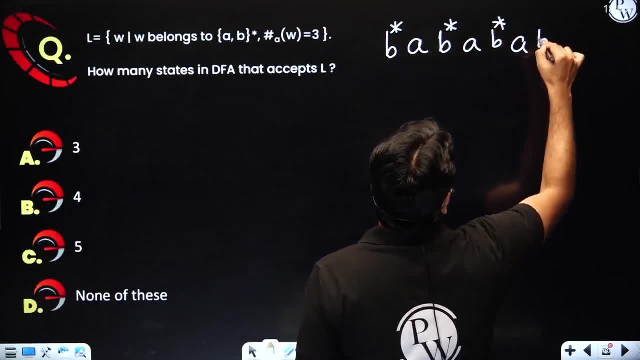 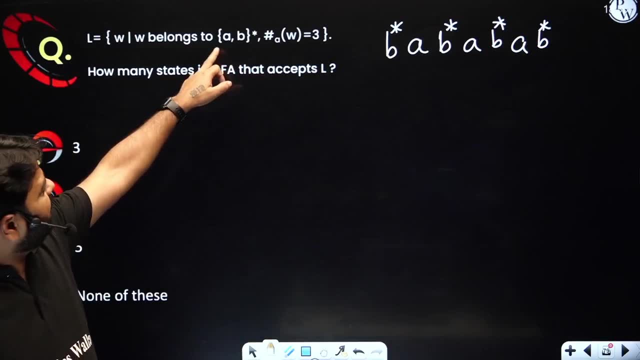 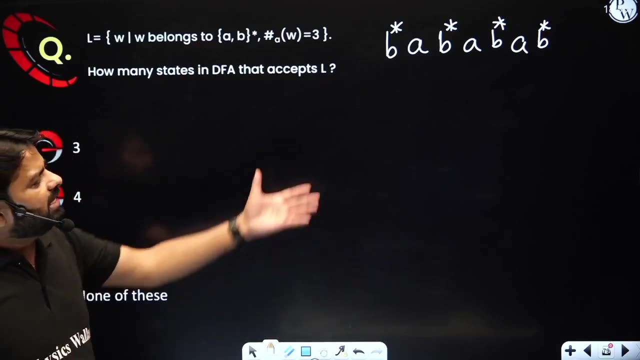 first two a's and in between the last two a's or at the last. so this is an expression to accept or to generate the language. where the language is, number of a's is exactly 3, but over a's and b's. now how do you design? very simple, you know the concept right: exactly 3a's, who is the minimum? 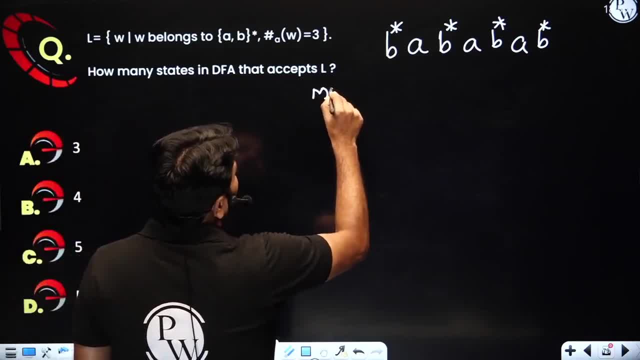 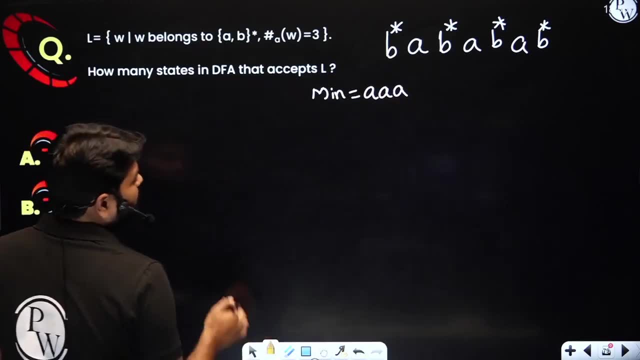 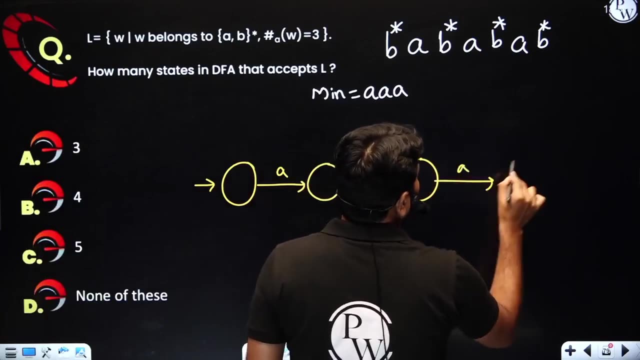 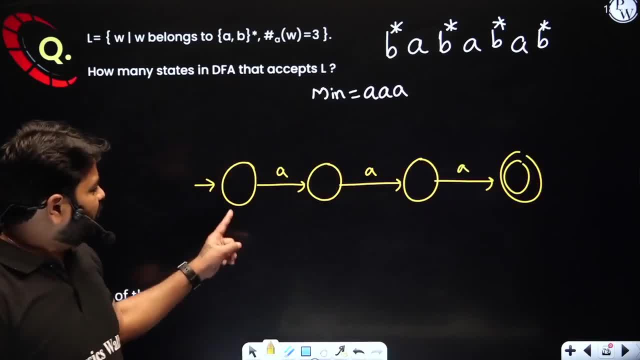 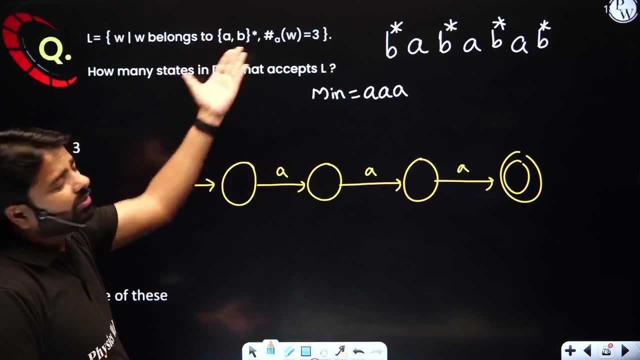 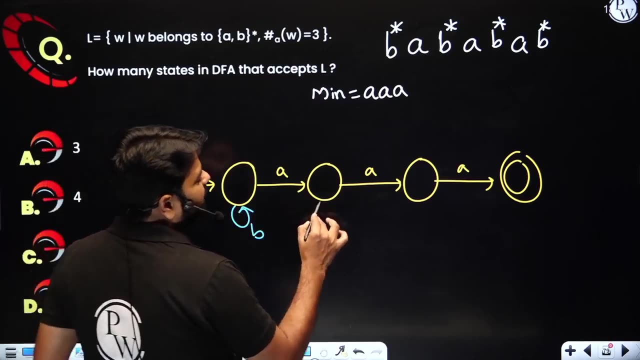 if you get any more, you go to net state now from here. if b comes, should i accept. yes, b's can come, any. i don't have any condition over the b's right. only a's should be 3, but b's have no restriction. any number of b's after a, any number of b's, see that formation of b star a, b star a and again b. 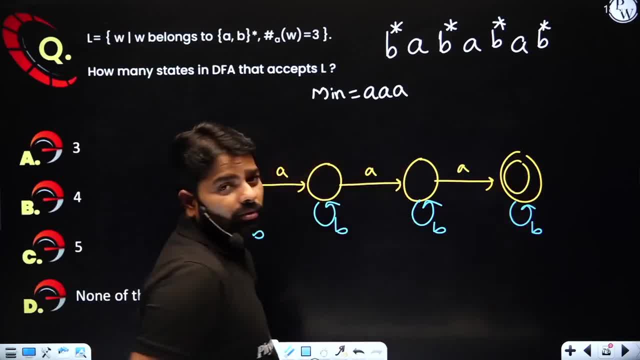 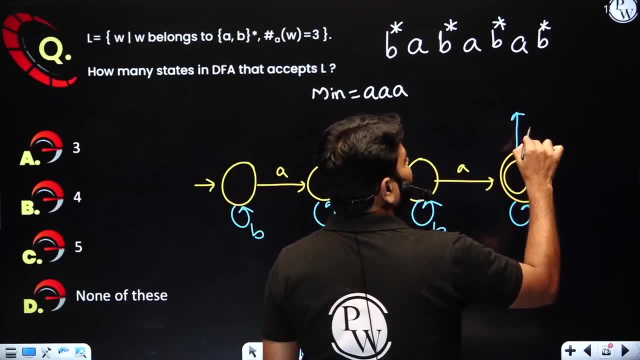 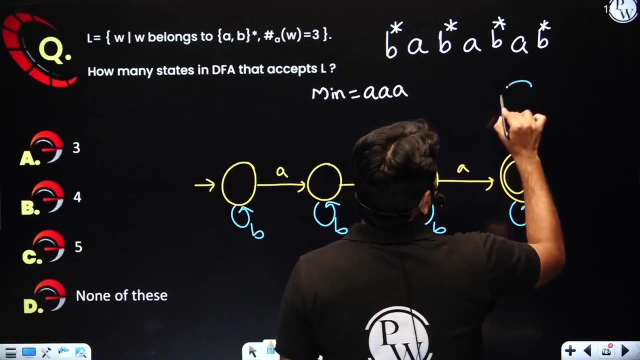 star. any number of b's after any number of b's, fine, but after this third a, if you get one more a you should not accept. so what do you do from here? if you get any more a here, because fourth a might come, might be possible to never stay in this path and you should go to dead state and stay there. 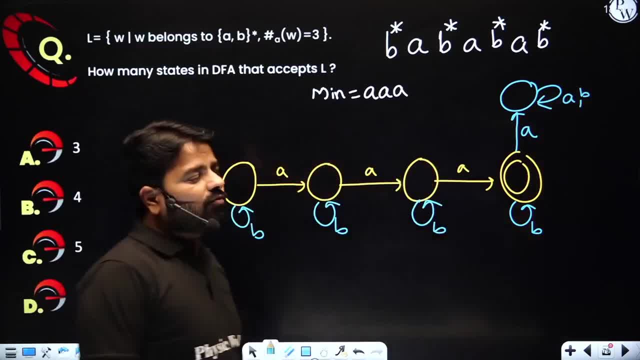 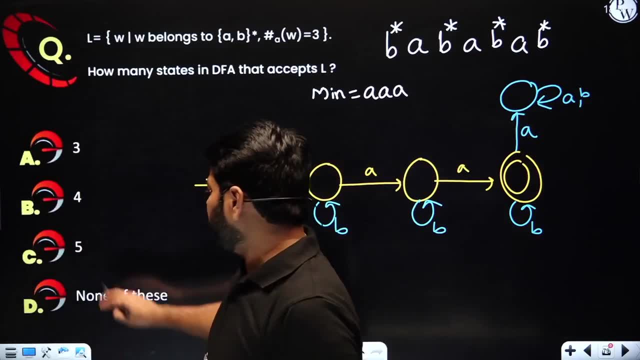 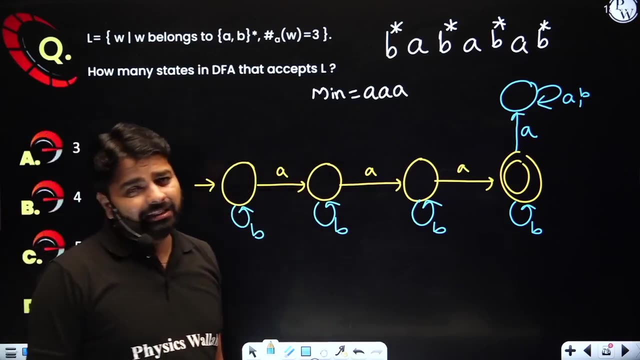 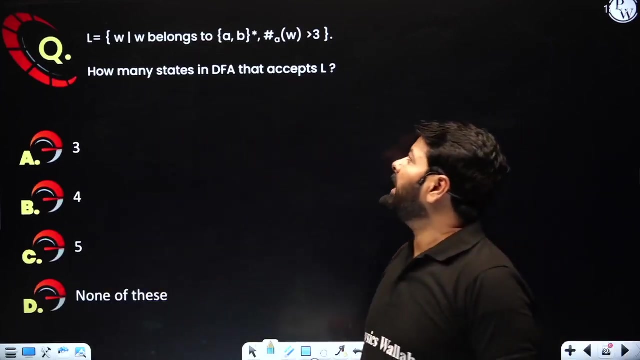 and any sequence after that should reject. fourth a should never come in case, if it comes, go to dead state. how many states are there now? five state? the answer will be here. this is how you design a dfa: to accept exactly 3a's. okay, now more than 3a's. more than 3a's means at least four a's right. more than three means at. 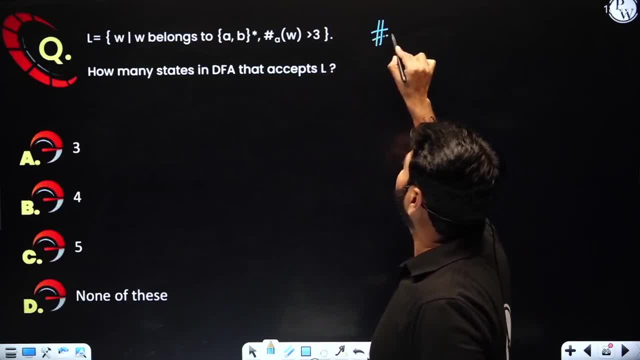 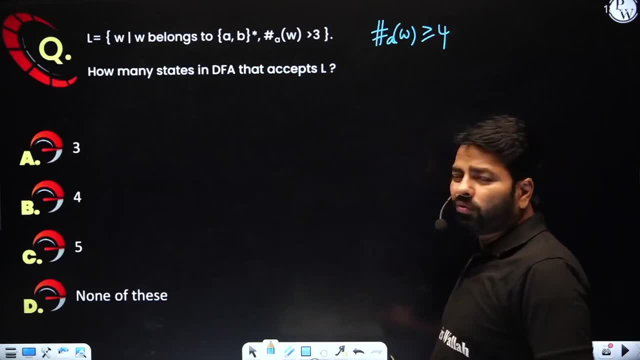 least four. now the question is number of a's of w greater than or equal to four. that is the meaning. greater than three means now greater than or equal four. how many a's you should guarantee first four a's: one, two, three, four. then after that you should guarantee first four a's, one, two, three, four. 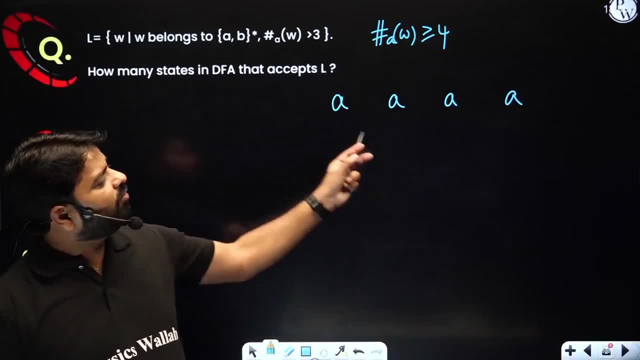 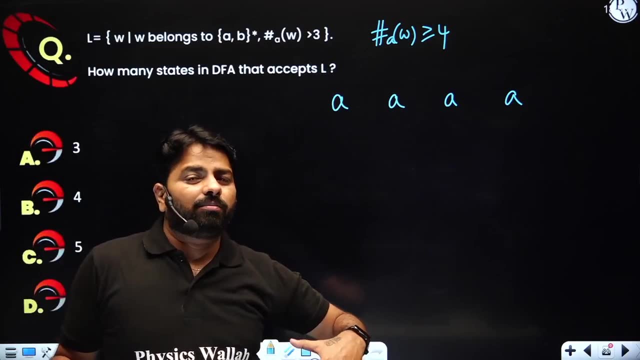 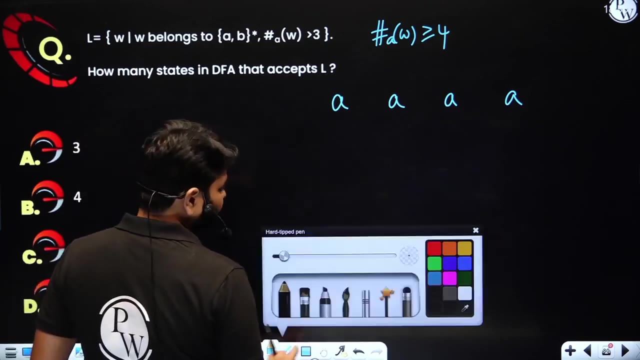 this. do you have any condition? no, i have satisfied minimum four years. now i can have five years, six years, seven years, because minimum four years but number of years could be beyond for any count. so now here it can be a's or b's, no restriction. if you want write an expression, expression only. 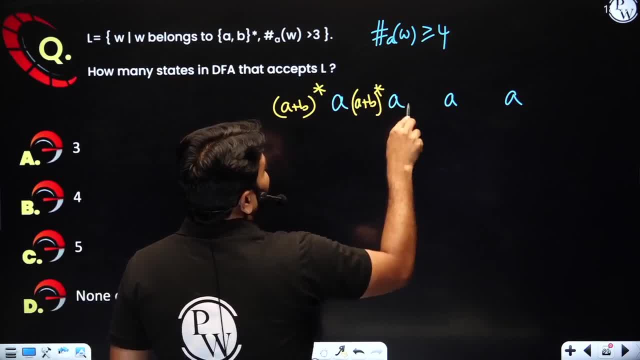 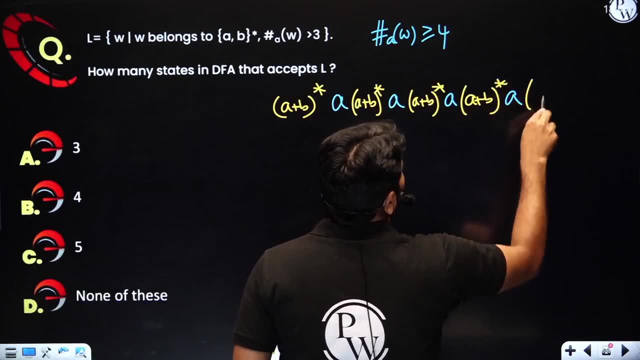 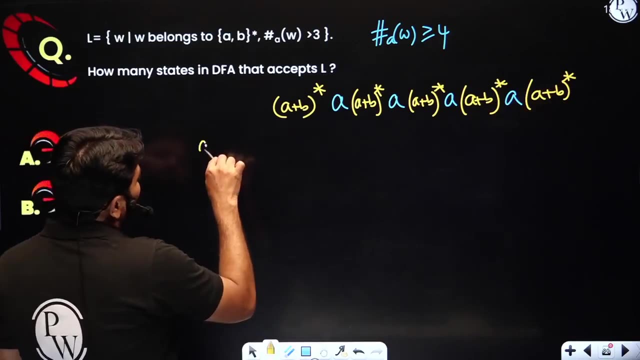 i'm talking about. you can have any sequence of a's and b's, very simple expression to represent at least four years. okay, i hope you know how to write an expression now. now i want to design the dfa, who is the minimum string four a's. that will give you an idea how to understand the problem. 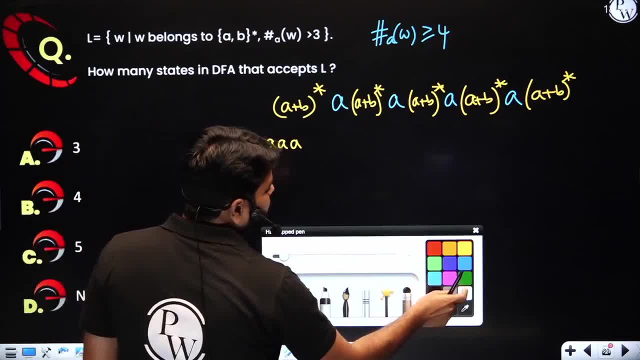 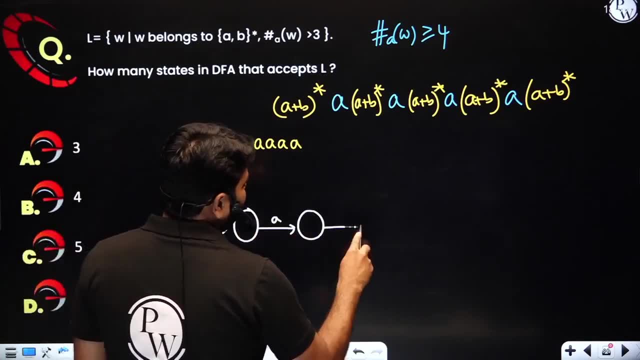 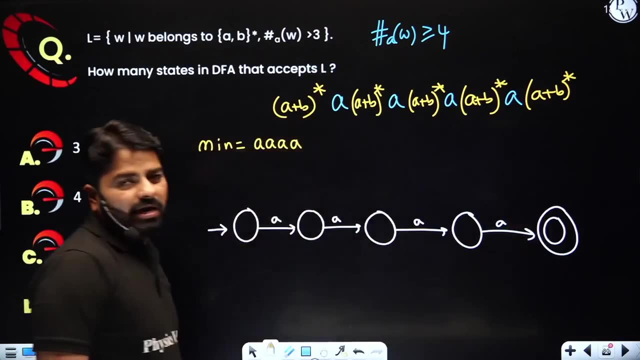 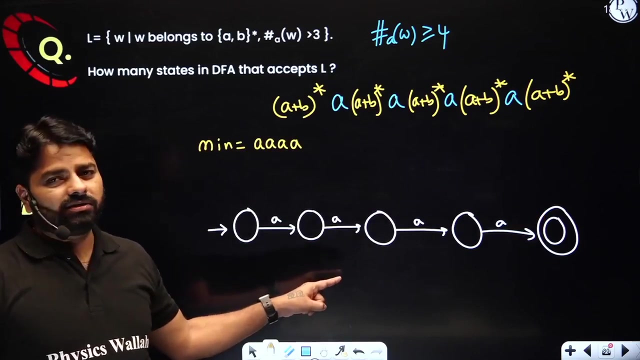 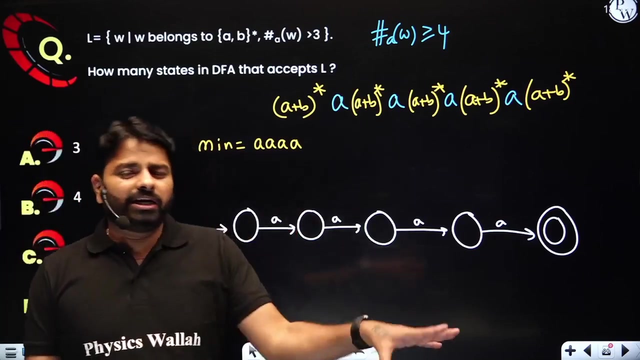 four a's, one a. you should know first four years how to accept. that's the minimum condition. have satisfied, fine. now you need to guarantee that all the strings, all the strings in the world, should have a path here, otherwise your motion is wrong. dfa means deterministic. you give me any. 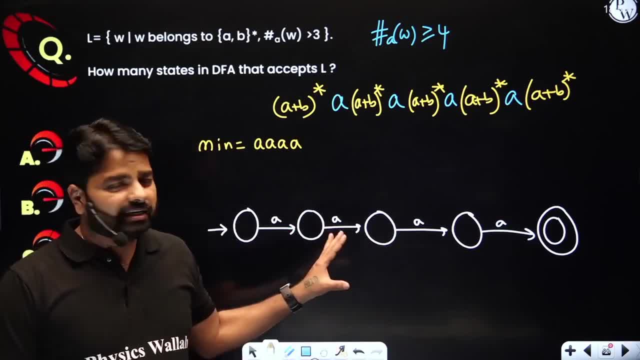 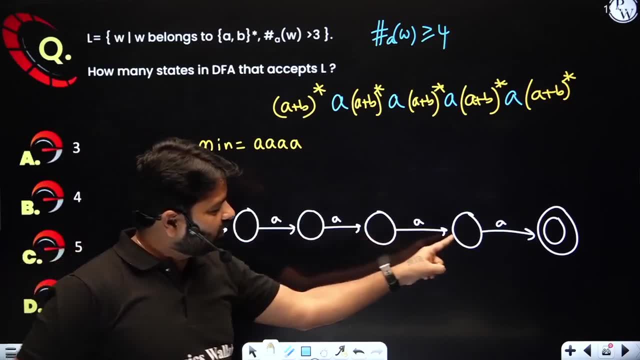 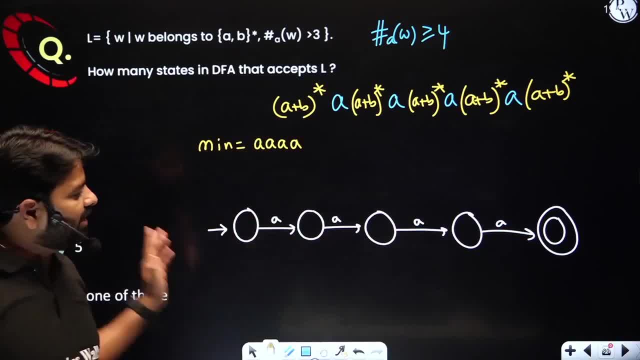 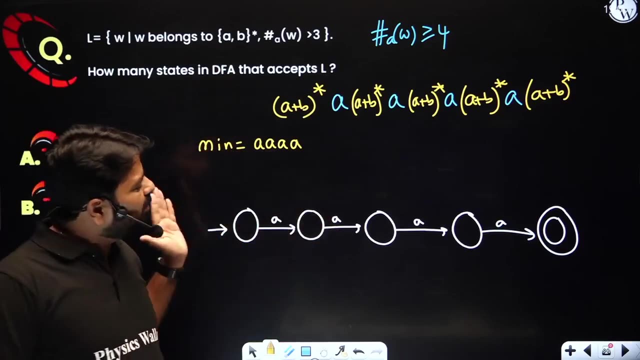 b when you cover them, then only this machine is dfa. never leave in the middle of the construction. okay, let's focus on what is here. b now, here you can see before this: a: are you counting any b's here? no right, i can keep blindly b cell flow. i don't have any issue with the b's right, any number. 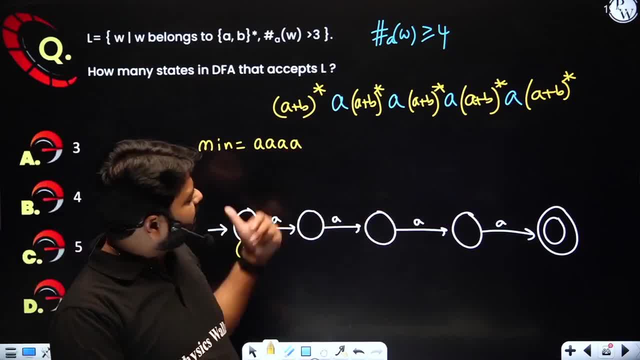 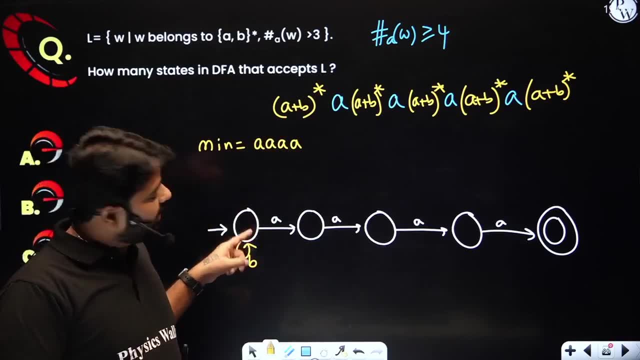 of b's can come, but somewhat. this expression and this diagram may not match directly, but internally, the same meaning. okay, because only b's we are thinking here, not a's. a is already covered here, a is covered b's already. one year is covered b's. i can stay here because i did not say four. 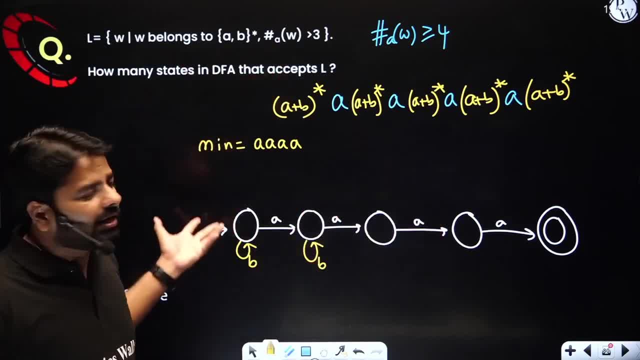 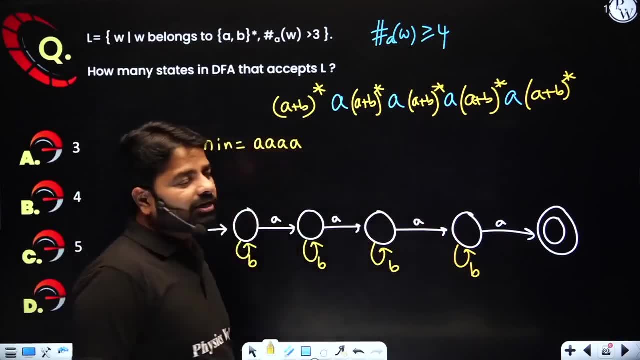 consecutive years. i said i want at least four years that can come in any sequence: right and after second year, any number of b's after third year, any number of b's after fourth year, because four years guaranteed. after fourth year a's or b's doesn't matter, because minimum four 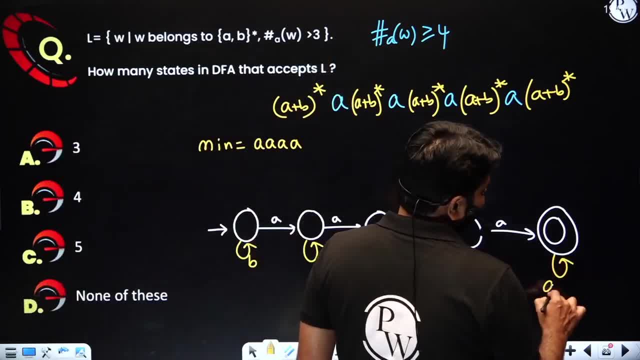 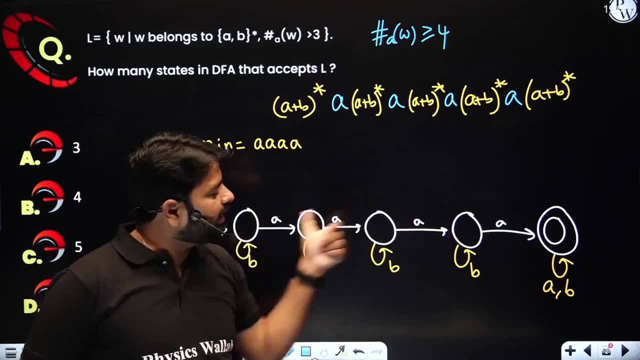 years satisfied. here you will have a or b you here. why didn't? why didn't you keep a cell flow? because a already i have covered. i keep on counting a's whenever i want to remember. i change on a right after this. i don't want to change on a. 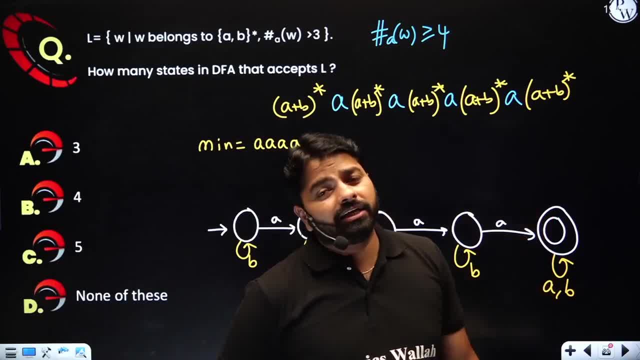 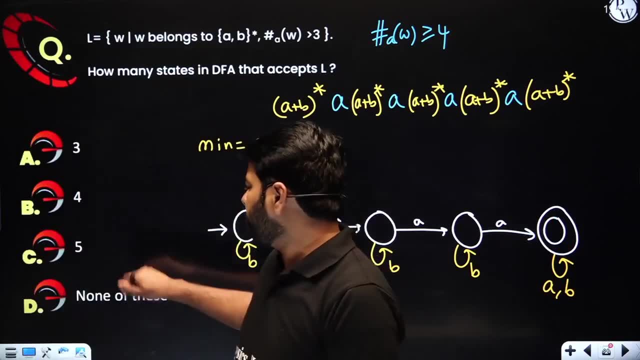 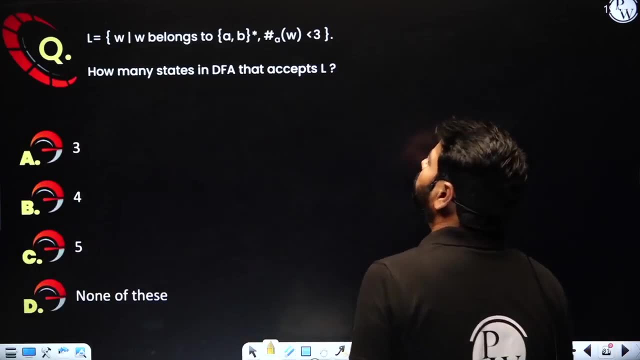 because i have satisfied my condition. now, a or b, i can stay in this final. so this is a dfe. how many states? now, five states, okay, okay, i'll give uh the next problem, as you know, challenging that you should design. now just take time, pause the video and try to design this. i've explained. 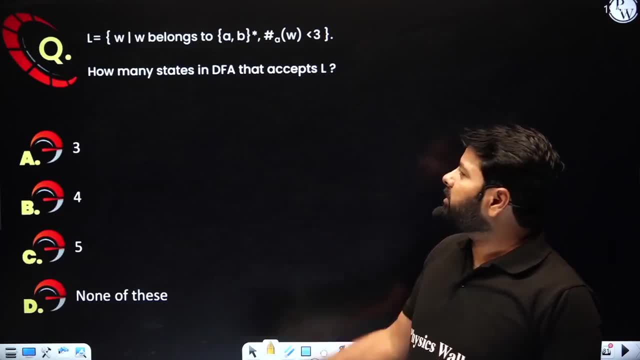 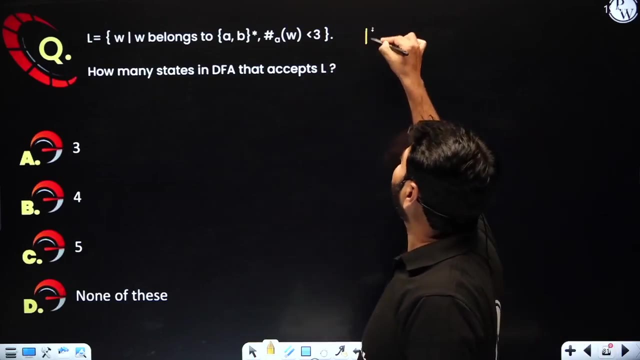 greater than or equal to 3, greater than or equal to 4, and just think about it, how to design it. okay, question is: number of is is at most two, two, not at most three. less than three means first. i have a clarity: at most two, at most two a's. you can приготов u s two a's time respectively. 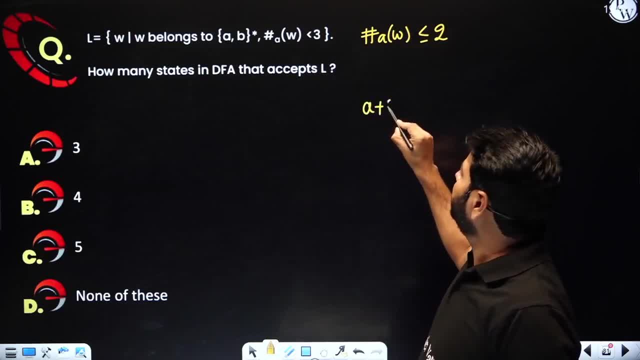 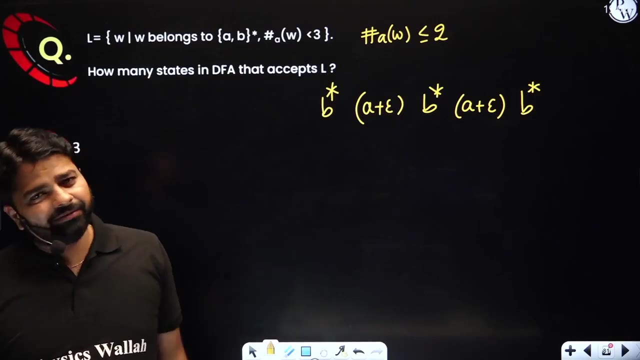 at most two ways. you can write an expression something like this: a plus epsilon, a plus epsilon. I'm just writing an expression to have a practice. this will give you at most two ways. anyhow, we don't need this expression to design a DFA. it's another. you know practice currently that you can write regular. 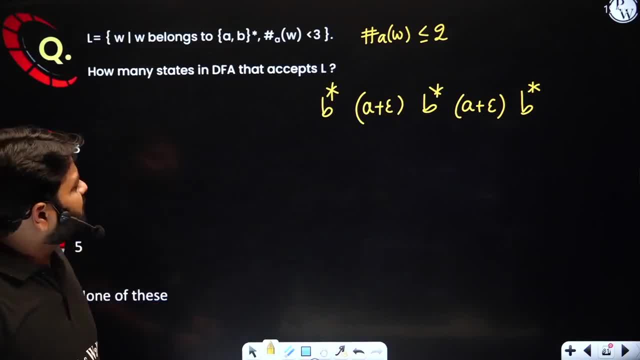 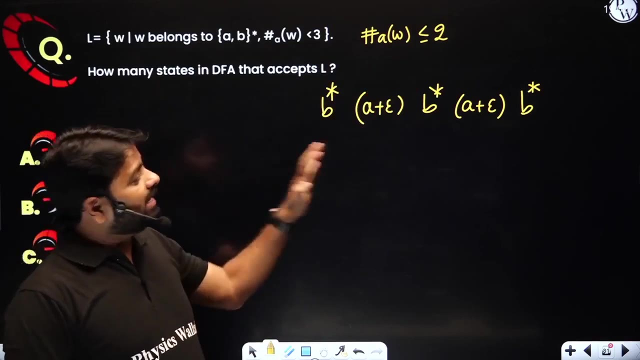 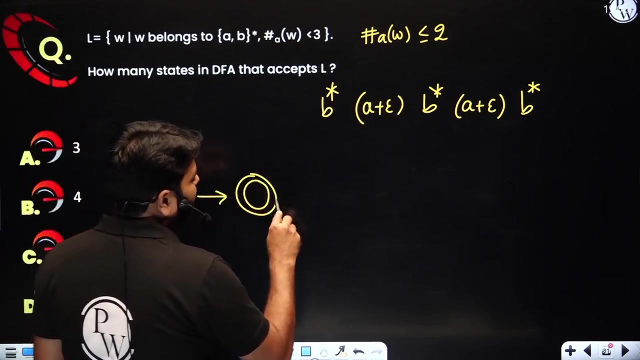 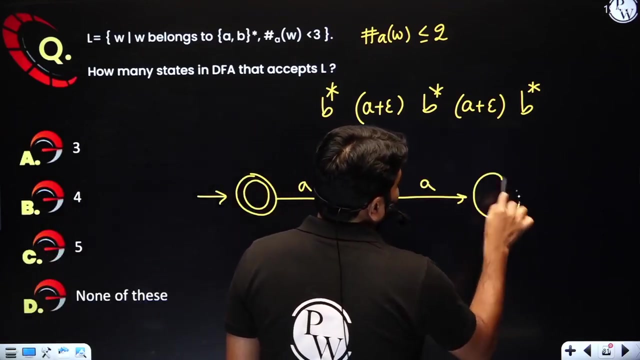 expressions along with the DFA. look how many states in DFA that accepts L. then now focus again. zero is accepted. one year is accepted. who is accepted, but third a should be rejected straight away. I will do that. no a accepted fine. one a accepted fine, please don't worry right now. two is accepted, but third a: what should be done? 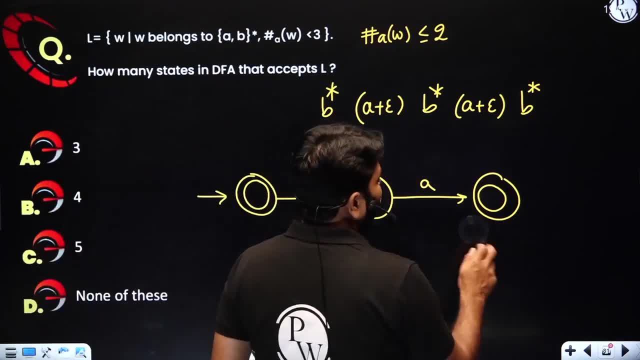 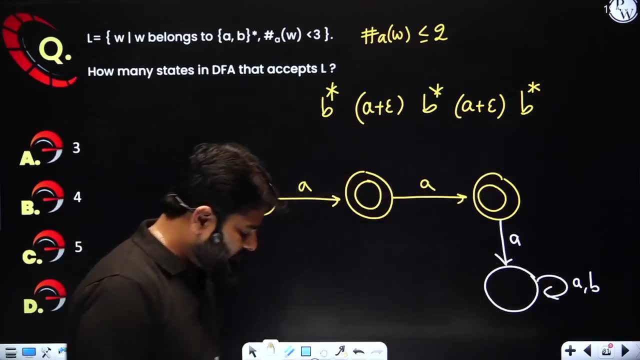 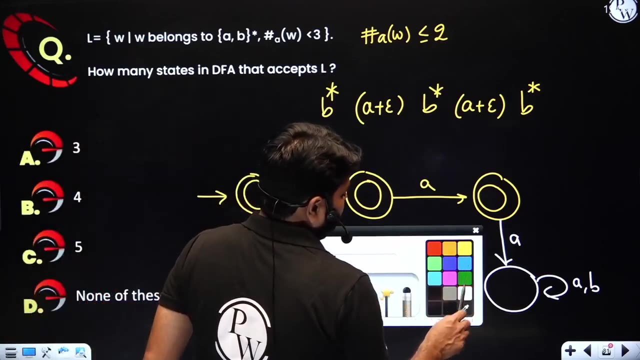 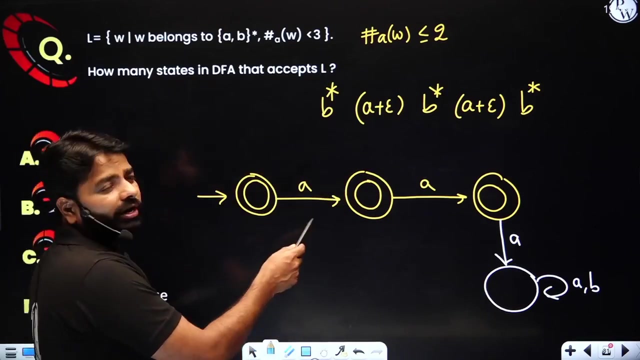 reject, rejected and after this we will make a DFA properly. we'll go to DFA, doesn't matter of that. anything comes, we'll stay there. it's not at over right now. so many transactions are missing. you should try to cover them. so can I have a B before here? yes, any number of B's can come, so I can wait for a after one year. 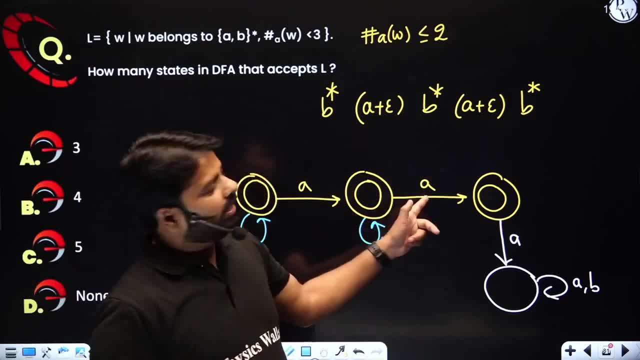 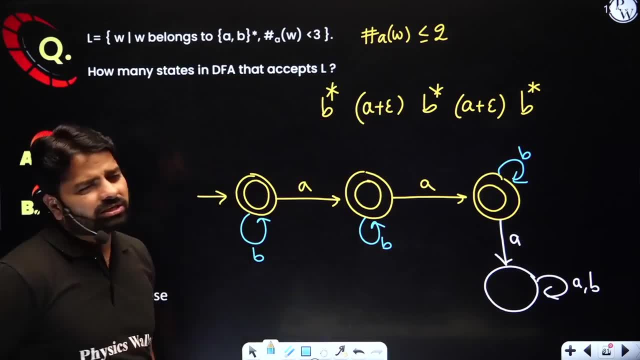 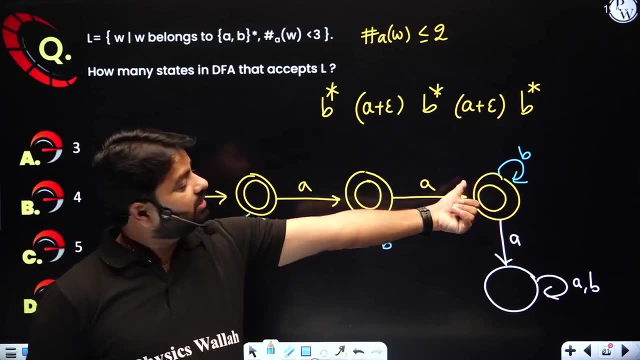 any number of B's can come after two. is any number of B's can come now? is it accepting all the strings who are having, at most ways, the till here? at most ways, anything you do, it's accepted because still you didn't cause a number of. is that too? once you cross two, is now you got a 30. everything is rejected. 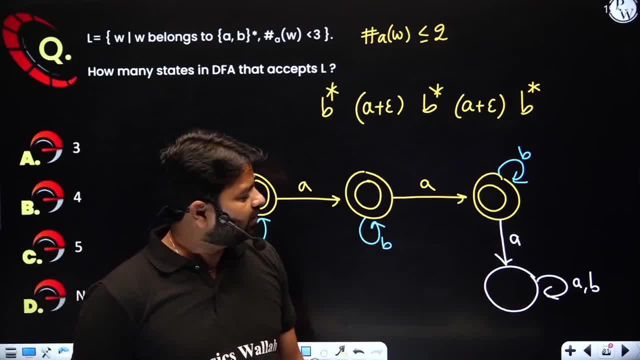 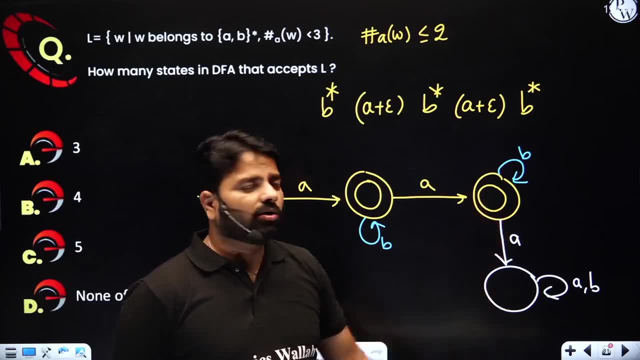 had. as you are going to get straight, what is the deficit definition? once you reach the dead state, impossible to reach a final, there is no path from this dead state to final, but this state is called as dead state. remember the definition of dead state. if that state has no path to the final, then it is called as the dead. 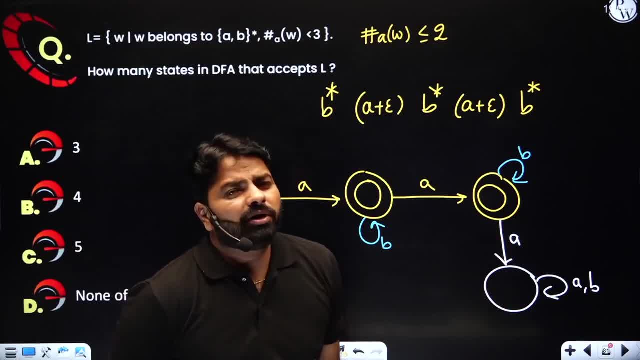 state: okay, a DFA. you may have multiple dead states, but no use in the minimum DF. II just have one dead. remember that you can design more than one DF. we use in the minimum. if I just have one dead, remember that you can design more than one DF, a or several, one or several presence at the DFA and remaining will be. 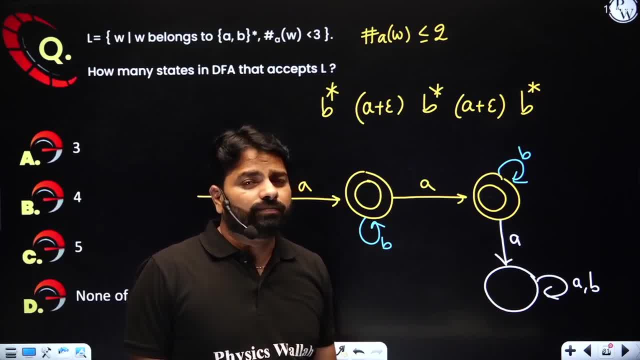 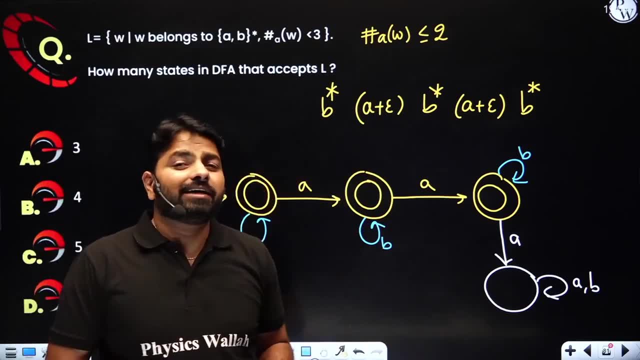 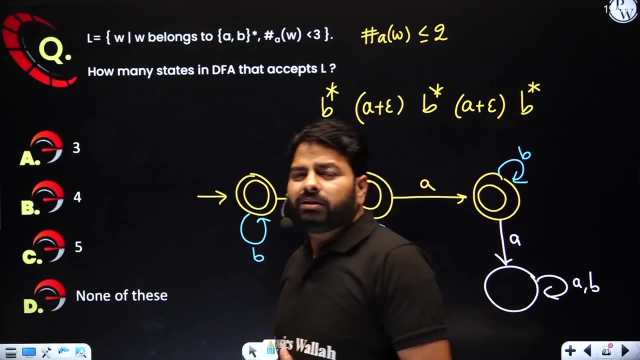 more than one dead state in the dfa, but no use, right, even though it is correct dfa. but if you want to design minimum dfa, then always keep one dead state if needed, if needed. but if anybody is keeping more than one dead state, that's okay. don't say that is wrong dfa. that's the correct dfa. but 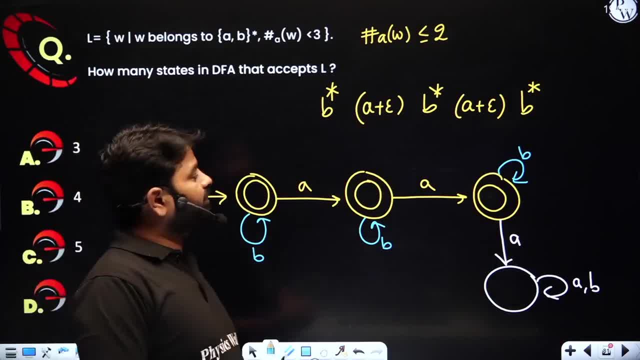 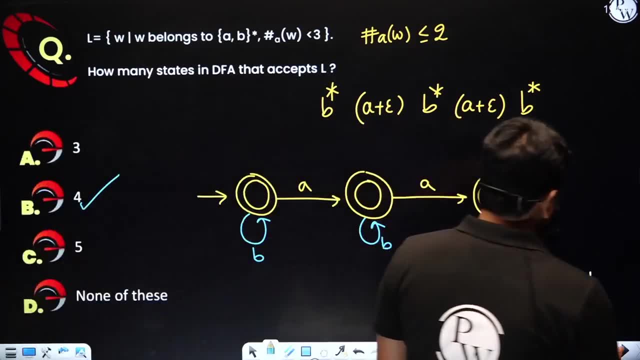 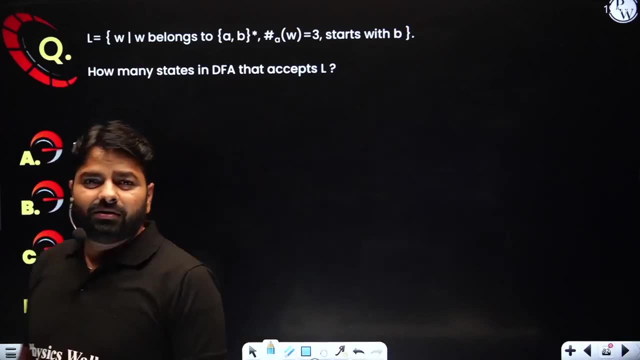 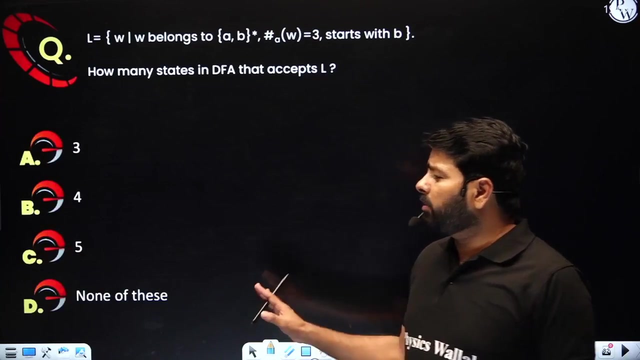 that is not a minimum dfa. fine, okay, how many states? four states, okay, yeah, very nice question, i feel. take time and pause the video again and please, uh, try to design find the number of states very quickly. it would take maximum one or two minutes, not beyond that. 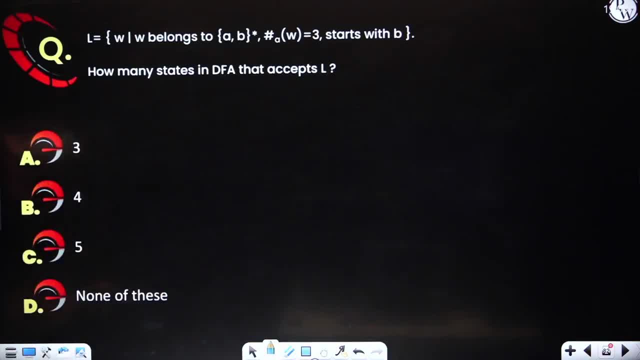 one. in any case, let's try that back and work together. okay, number of a's is exactly three, but starts with b. that's a very interesting question, right, you must start with b, you can't start with a, so be always there in the beginning. first position: that: 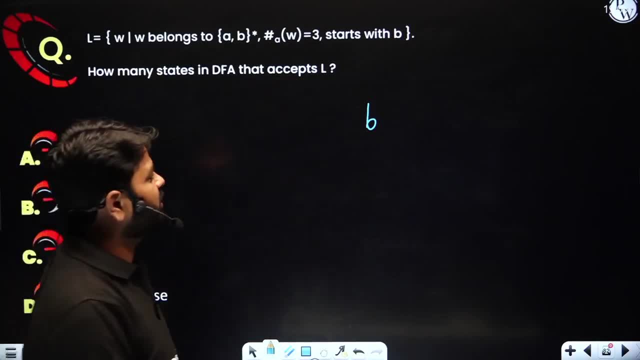 too, but after that you will have exactly three as and be is scattered, so one shall be. currently, finally, we are always there. so now, if you want to has a load of b, there must be someone. if you want, have no restriction, b's have no restriction. so somewhere you have three a's, exactly three a's. 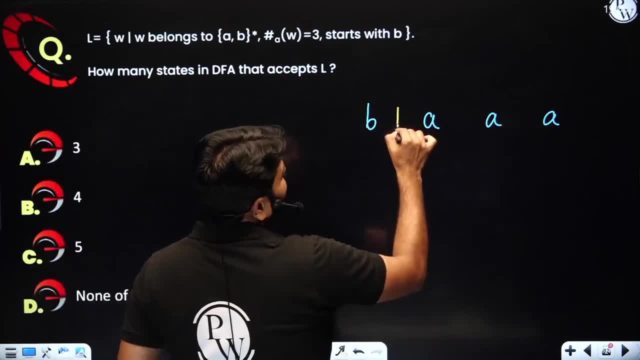 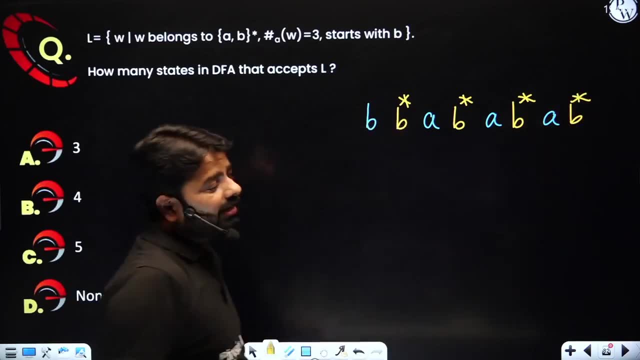 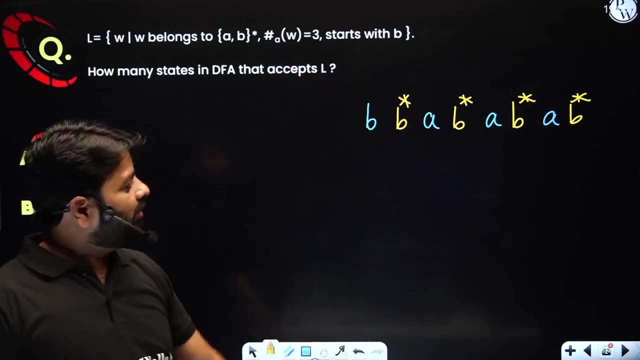 how many b's any number of b's might be here, we don't care, any number of b's here, any number of b's here, any number of b's here, but condition is very clear: the string should start with b and it should contain exactly three a's. and fourth year never happens. you will never start with a. 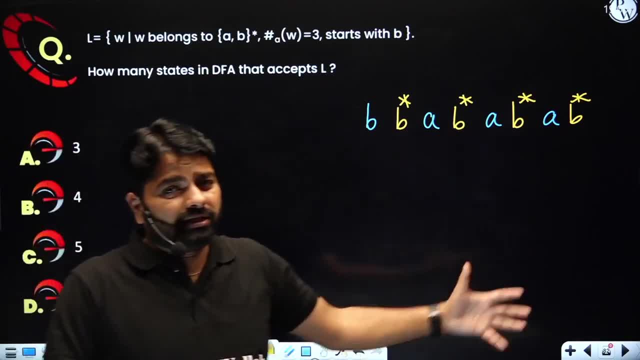 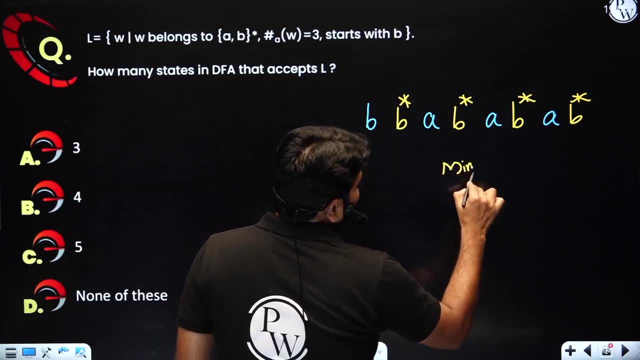 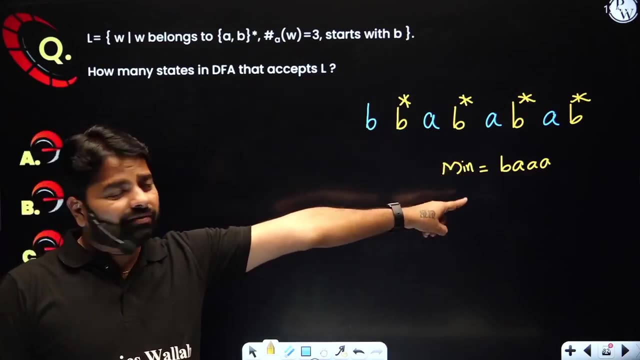 and any number of b's would be fine. how many things are there? so what is the minimum string? we look at this expression. the minimum string is b, followed by three consecutive ways because other b's are optional. right, there's only the string which is having the minimum number of. 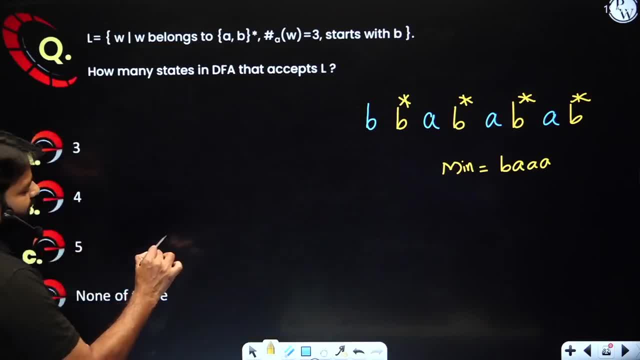 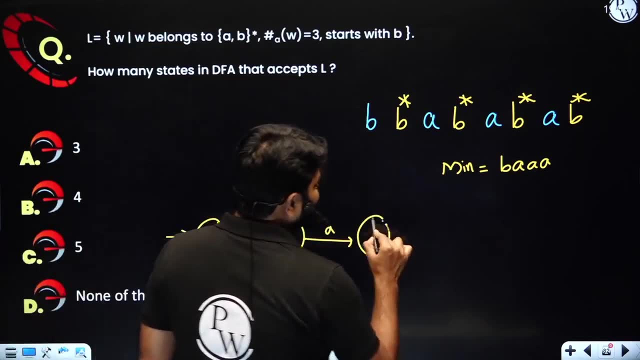 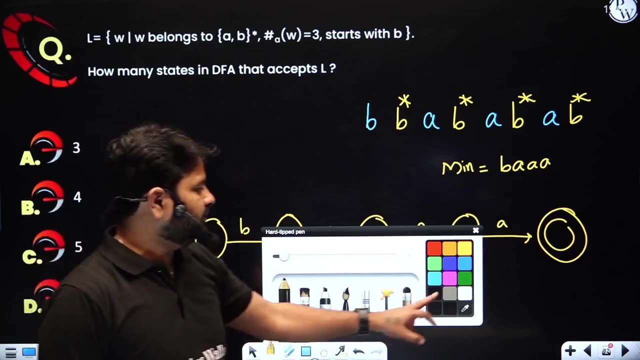 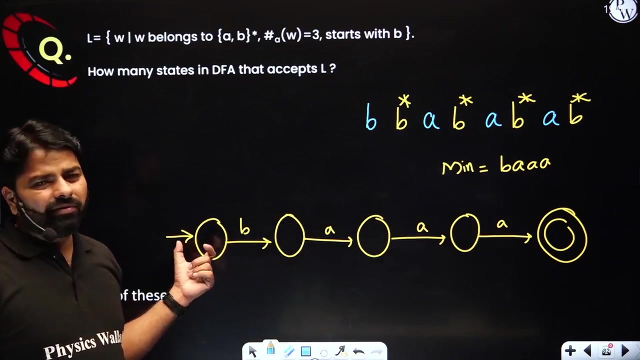 symbols, four symbols. okay, let's design the dfa with the help of the minimum string. b is must and then three a's overall. by looking at the minimum string, you always design this motion. now try to cover the missing transitions here. can i have a? can i start with the impossible right? 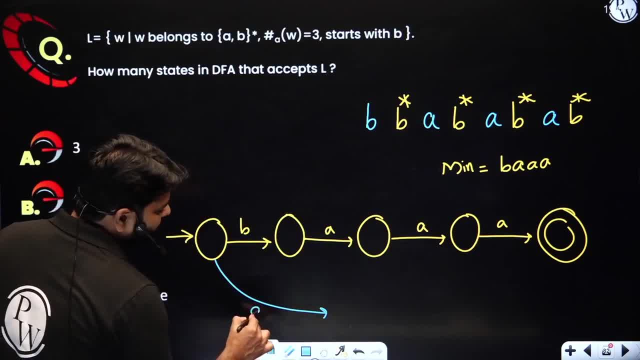 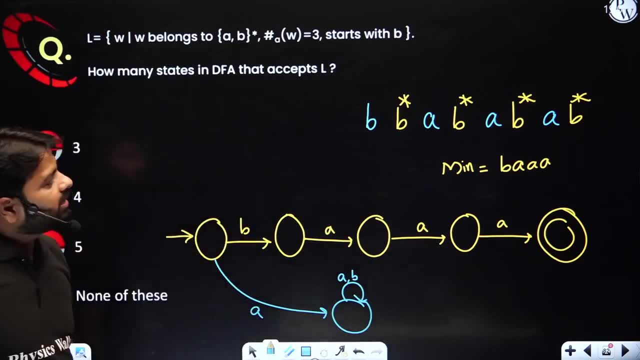 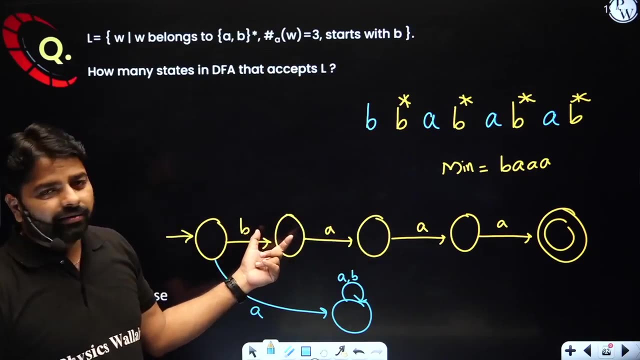 so what do you? do you go to dead state? go to dead state, yes or no? why do you go to dead state? because string never starts with a. it's clearly given that starts with b. now, from here, any number of b's can come, because i'm looking for the three a's after. 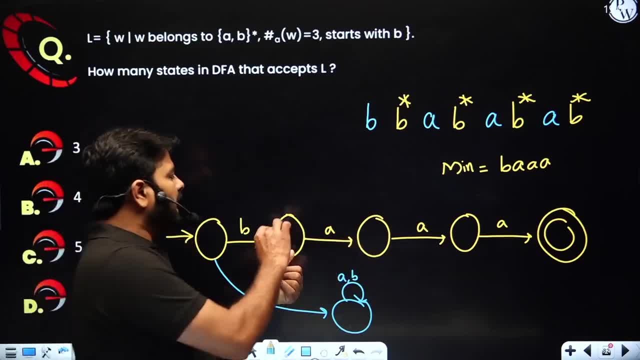 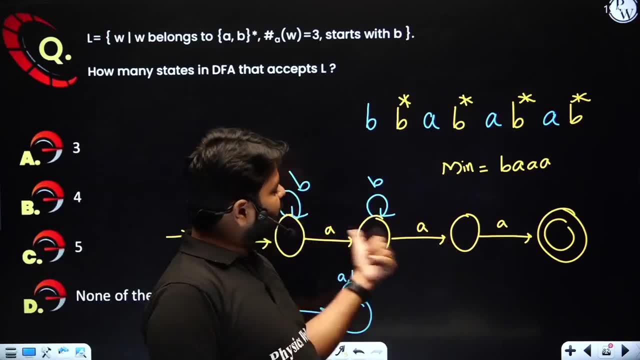 i start with b in the process. if i get any number of b's, i'll wait for the years after one a. if i get any b, i'll wait for the two more a's after two a's, after two a's. if i get any more beats, i'll wait for the third year once i get. 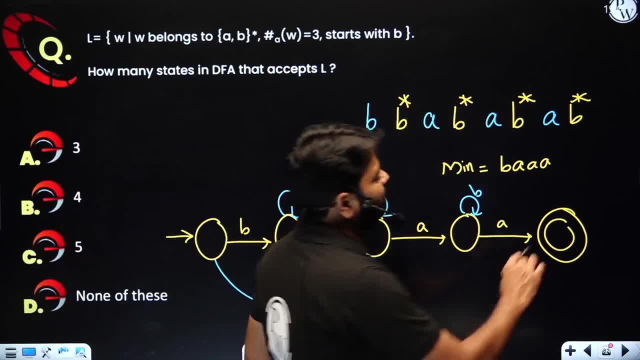 the three a's. i don't care for the bees. i can have any number of b's, but i should never have the fourth a. so after three years, if i get a fourth a, the number of the b's 줄 the. the number a should ever give to that three a sounds Ç, in order to Just do that. 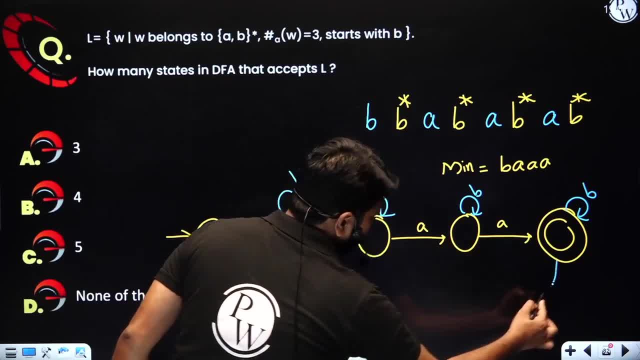 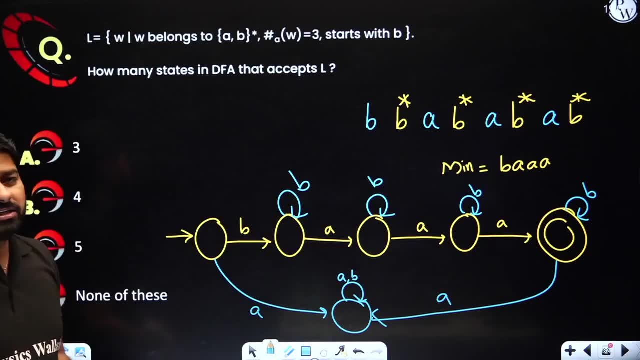 after three is if i get a fourth a, then i will come to that state. i hope it's very clear. if you know the pattern, if you know the sequence, it will be very easy to design. okay, so it almost looks like what i have written here. b, b. 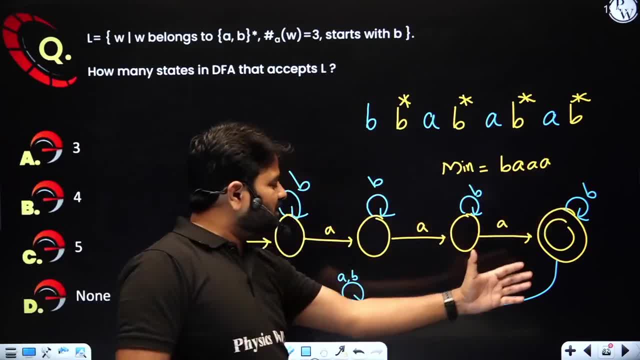 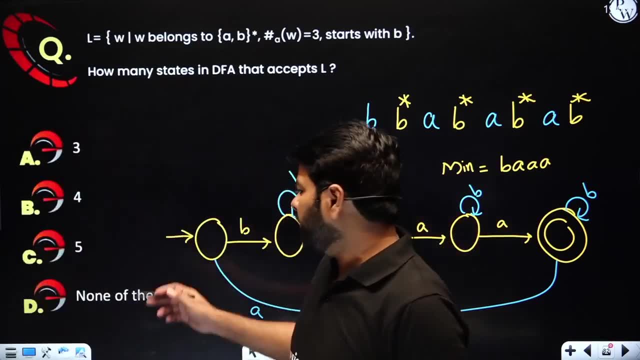 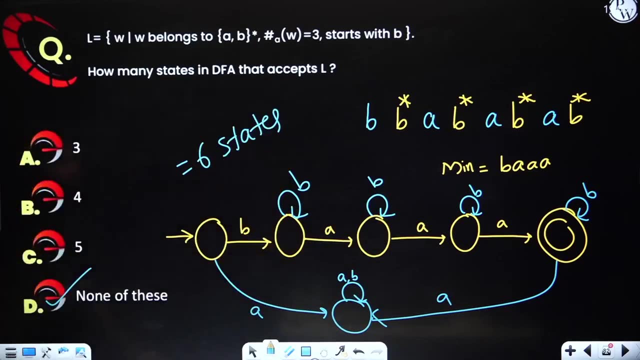 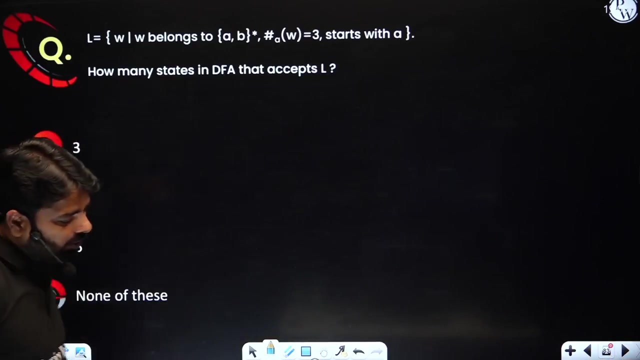 star, a b star, a b star, a, b star, those paths which are going red, said we don't care. okay, how many states, three, four, five, six, you have the six. no right, we'll go for none of this. so six states you have here. okay, it's more interest. interesting than the previous one, which looks similar to the. 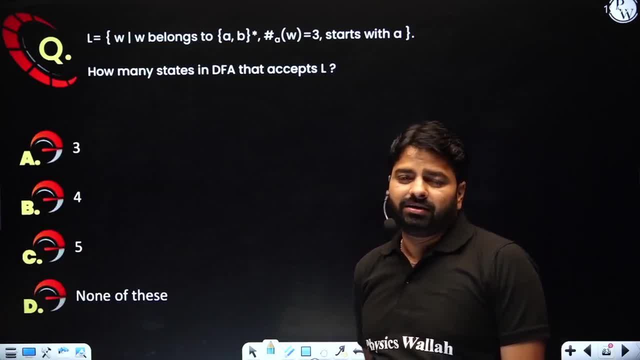 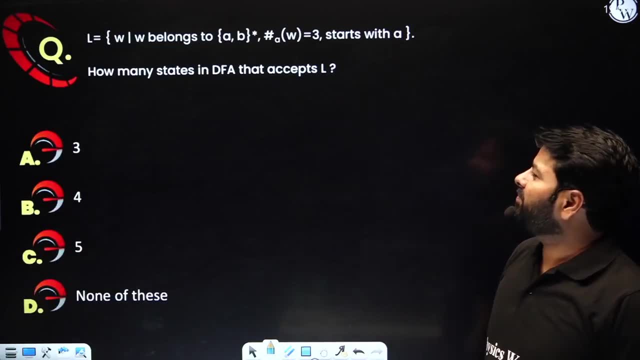 previous. but have a trick, or have a you know some you know interesting uh parameter that you need to observe. let's see can do that. so when you watch this video, please pause the video and click the subscribe button so that you can watch all the videos we have in the channel and then, as always, thank you very much. 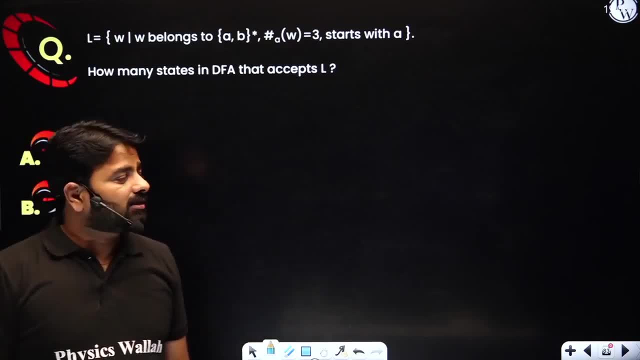 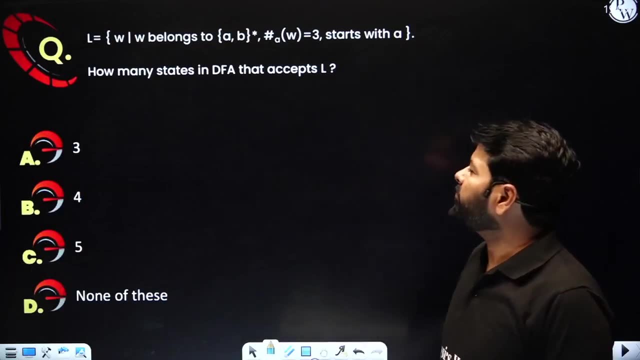 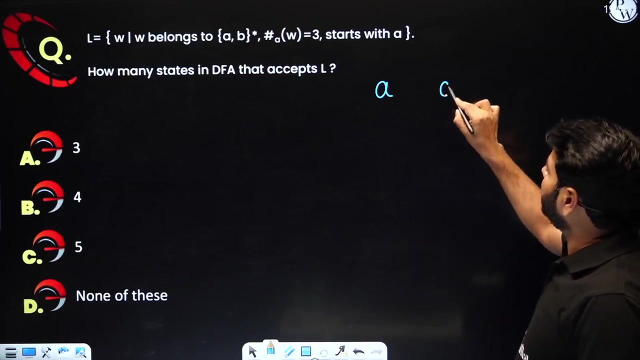 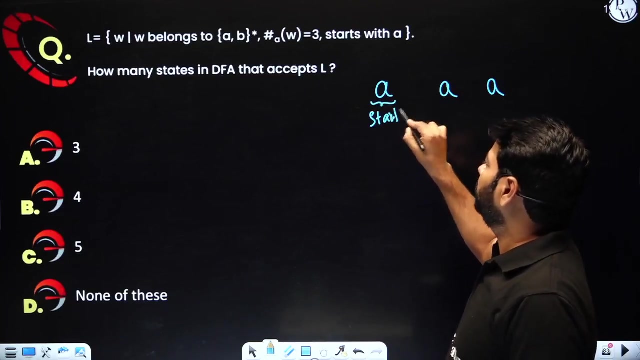 for few seconds and practice this as, rather than watching you always practice while watching it. okay, starts with a, but having exactly three s. what is the meaning? the string should start with a, but having exactly three s. so starts with a, but exactly three s somewhere this other two s, but start. this has to be start, but overall this is. 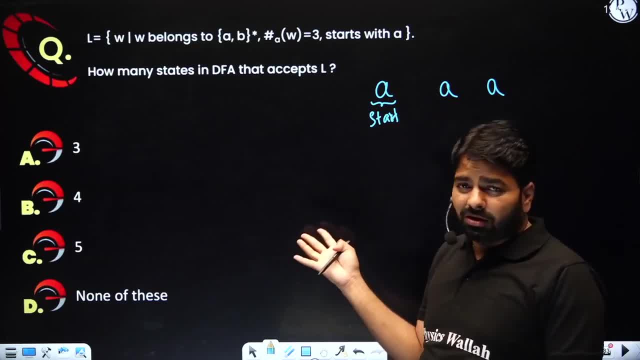 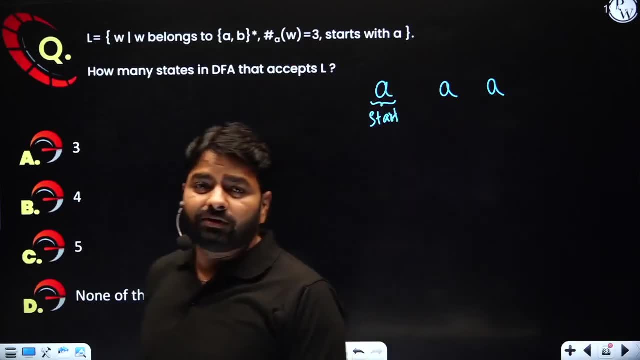 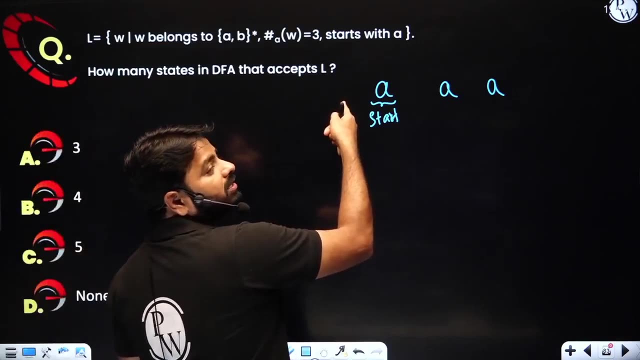 also counted in the three s. don't assume there are four a's wrong. the total number of a's should be three. but string should start with a. okay, the W should start. W should start with a. now, can I have the B star here? no, because I can't. 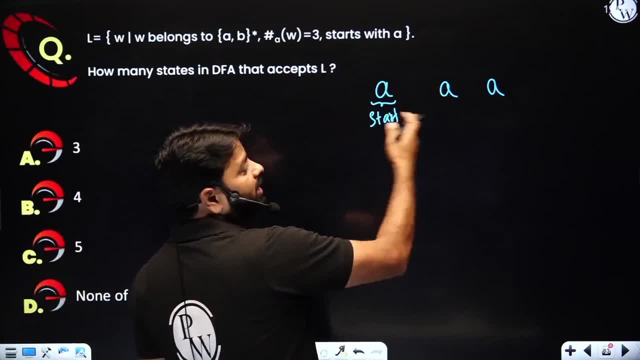 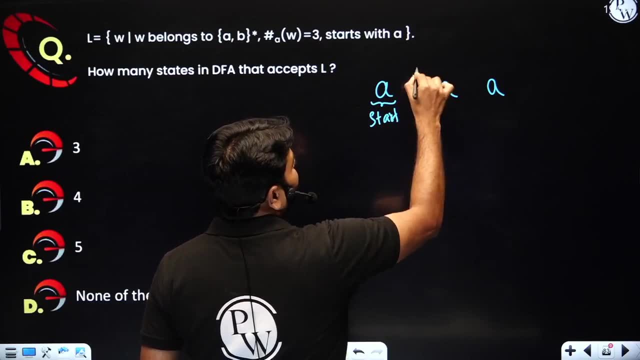 start with B. can I have a star? impossible, because maximum three a's and you can't start with a and you can't start with a and you can't start with a and you can have B star. here you can have a B star. here you can have a B star, because we don't count the B's. 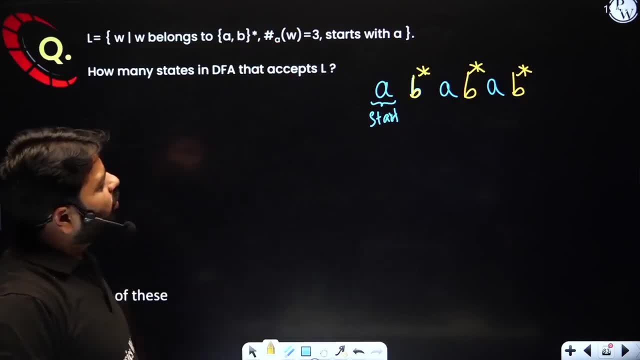 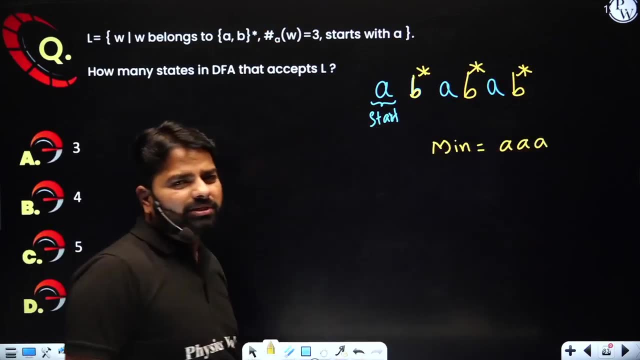 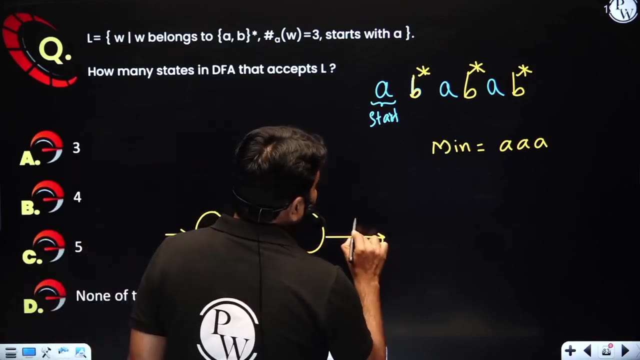 at all. that's all you have an expression by looking at this. what is the minimum string? you have a, a, a. once you have the minimum string, things will go very easily. three a's, but need not be consecutive. only the minimum string will go very easily will have the consecutive. 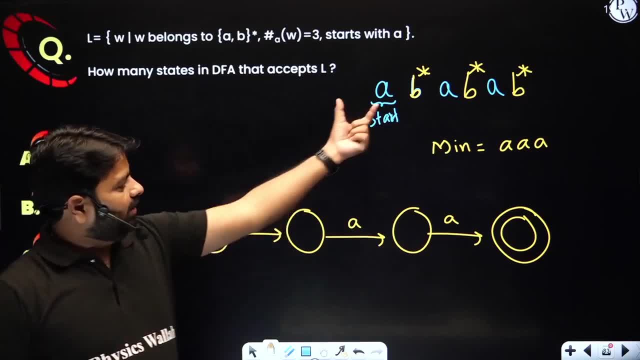 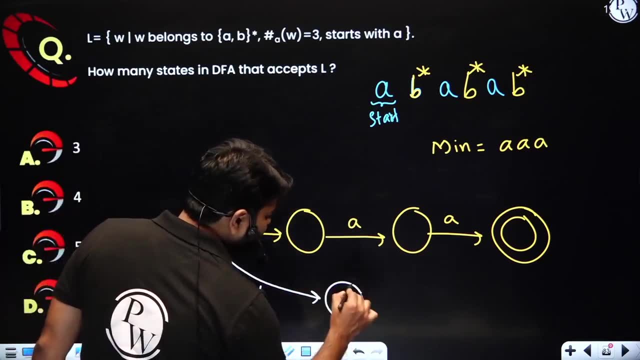 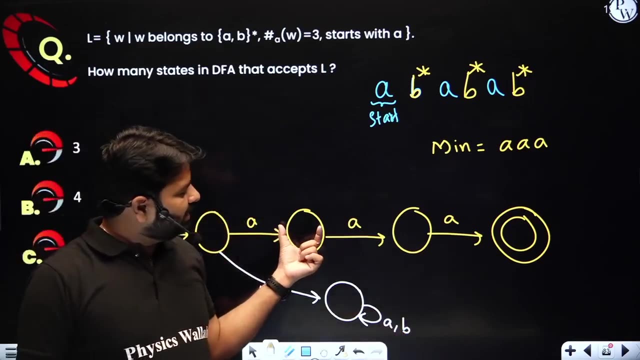 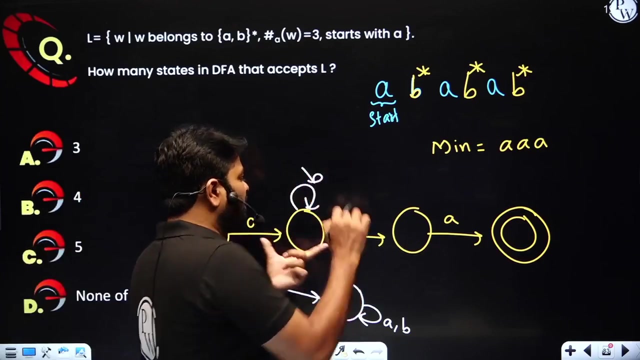 okay, now you should start with a, in case if the string starting with B, what do you do? you go to dead state. you can't start with the B. okay, that's missing. transition from the initial state. what is missing here? B. as I told, after starting with a, doesn't matter how many B's comes, just keep a self-loop after having two A's. 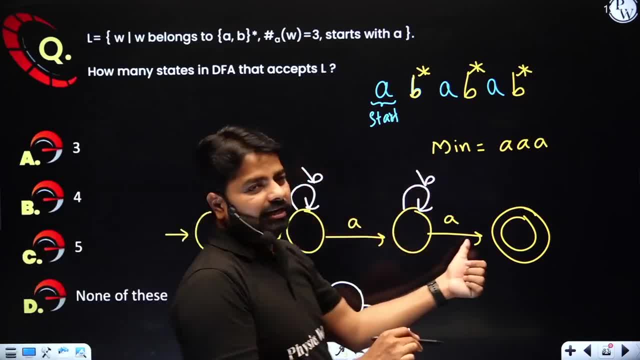 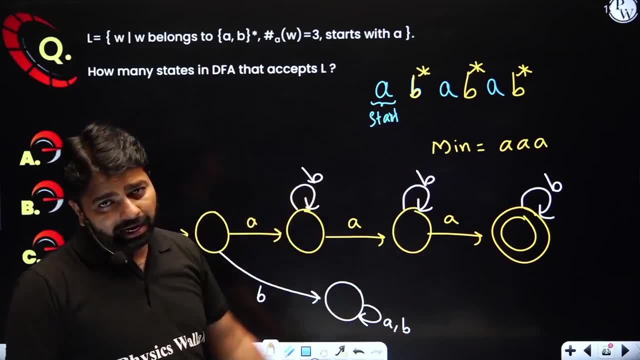 having two a's, any number of b's fine. after having three a's, any number of b's would be fine. but if a comes after the three a's then it should not be in word language, right? the string is crossing the three a's, so the fourth a should go to dead state will be invalid string. okay, how? 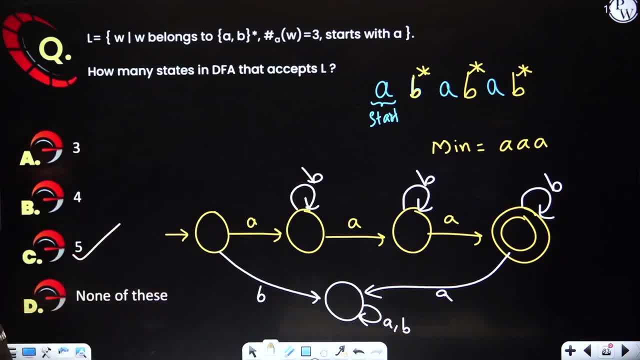 many states again. uh, i think this time is the five states. okay, including dead state. total. five states are there in case if i miss any transition, any motion. so please take care of this, but more fully: 99, i will not miss any transition as i am looking at every time, every state, see in all the machines. 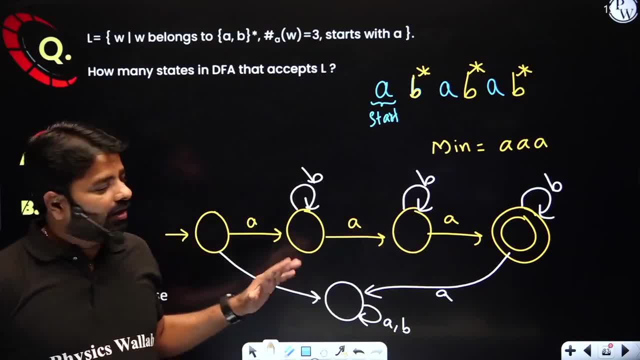 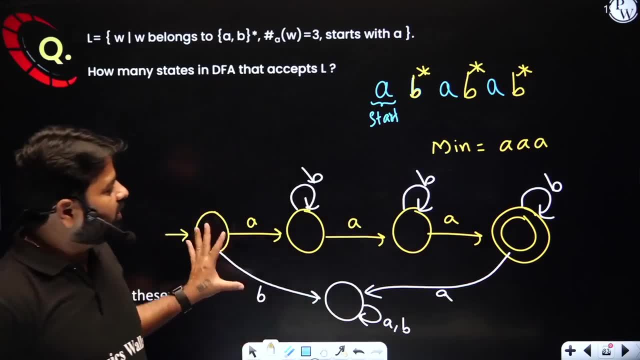 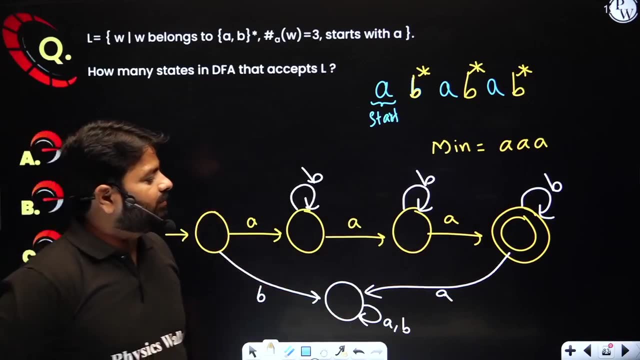 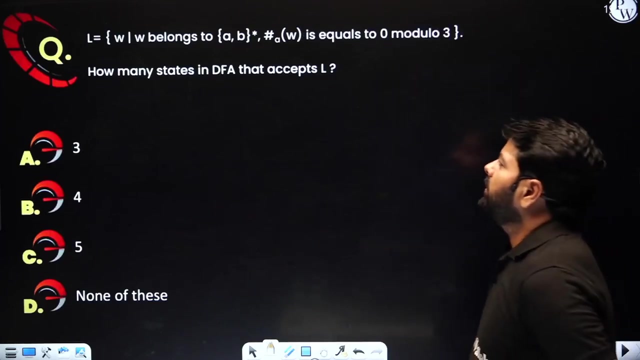 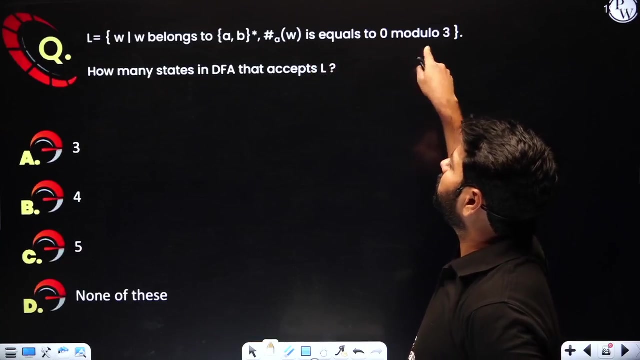 i design in such a way that i don't design randomly. i take the minimum string. i always start from here and go next, next, next, so that my whole motion is perfect in that process. if i miss any transition, please take care of that. okay, how many states in dfa that accepts l where number of a's is equals to 0 mod 3? what is the meaning of? 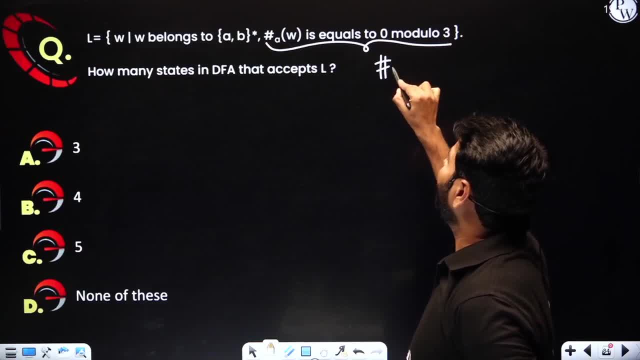 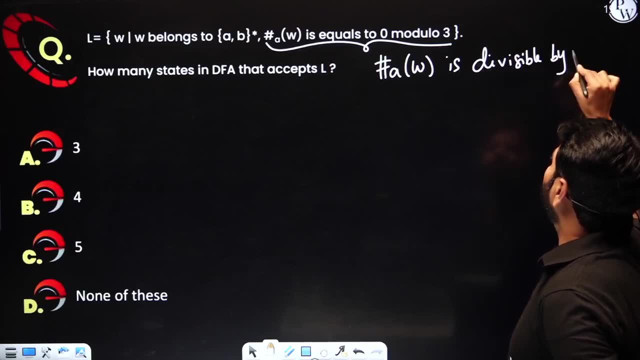 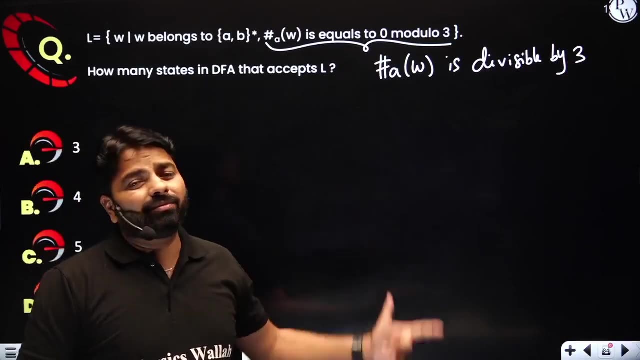 this, don't confuse much. it is nothing but number of a's of w is divisible by 3. very simple, right 0 modulo 3 means what divisible by 3? you already know. right, length is divisible by 3, three states. number of a's is divisible by 3 will also be three states. but where is the difference? 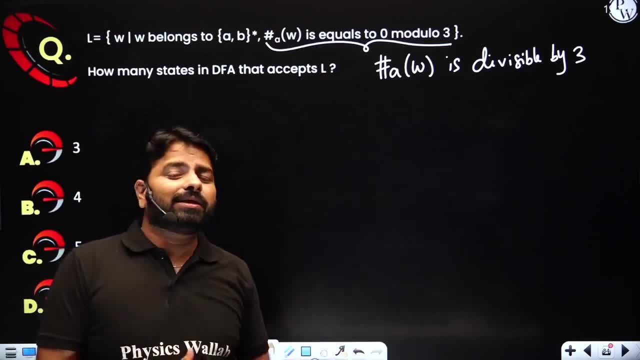 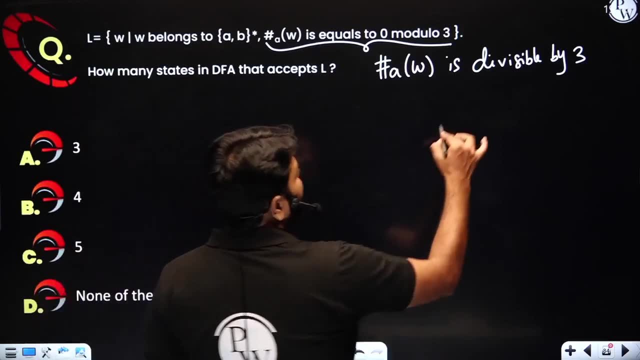 think about it. where is the difference? length of the string is visual by three- three states. number of a's is also divisible by three. number of a's in a string is divisible by three is also three states. but where is the difference? in the exam you can answer within two seconds. 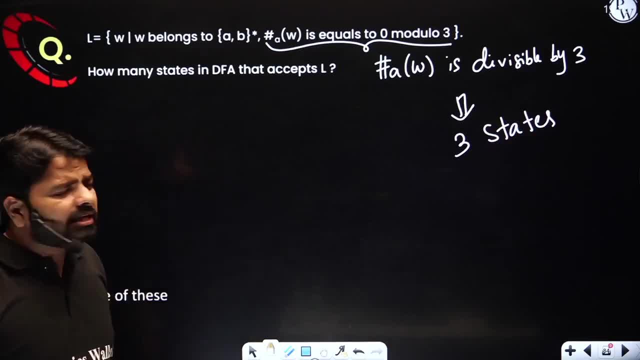 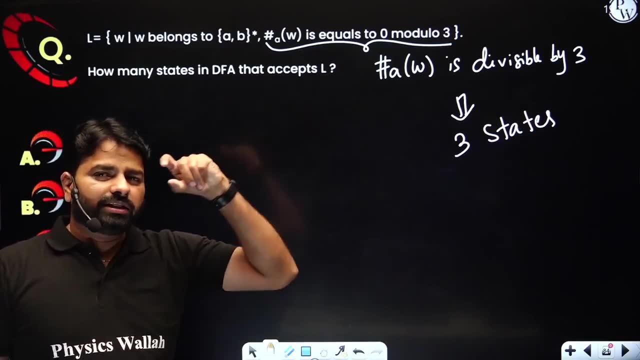 right difference is when you say the length erb, you change the state, but here only a's, you change the state. for b's you put a self loop that's. that's where the difference between length of the string and number of a's- number of a's- means focus is on a's. so 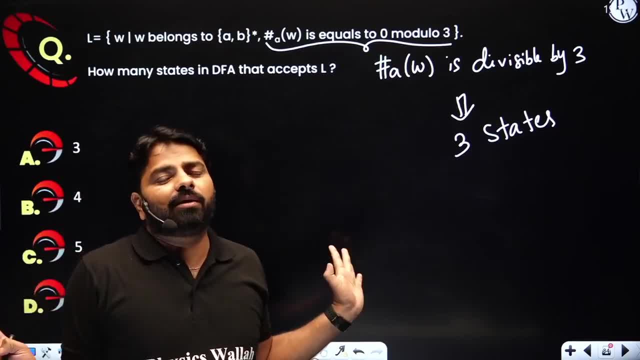 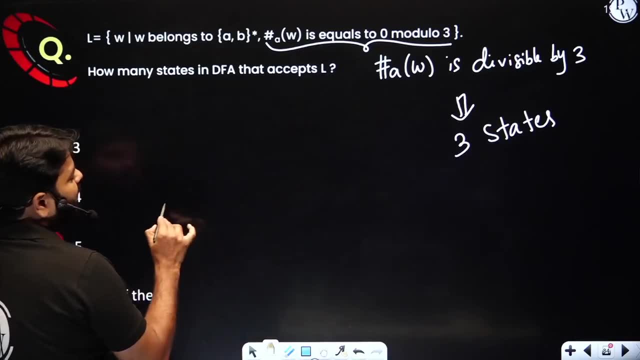 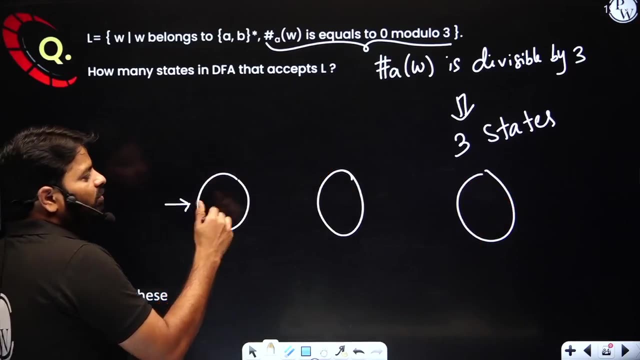 remember: the a's, not the b's. length means either a or b, it's length only right. so you will change the state anyhow. let's look at now how many reminders we will have. three reminders: zero, one, two, no a. if you get one a, go to the remainder one. 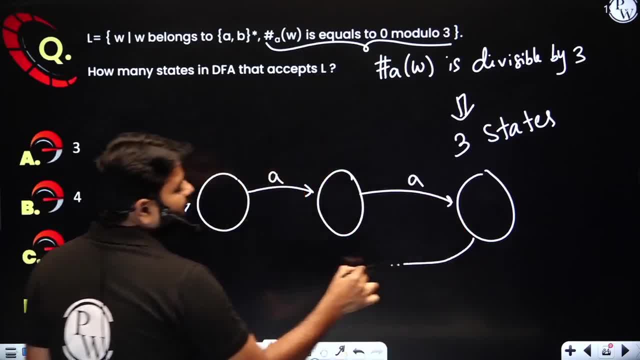 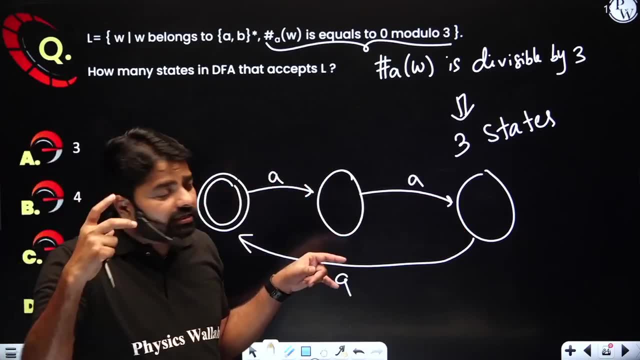 when you get the second a, go to the remainder two. when you go to the, when you get the third a come to the remainder zero and this state is the final. and where is the difference between the length? in the length a or b, you change the state a comma, b, a. 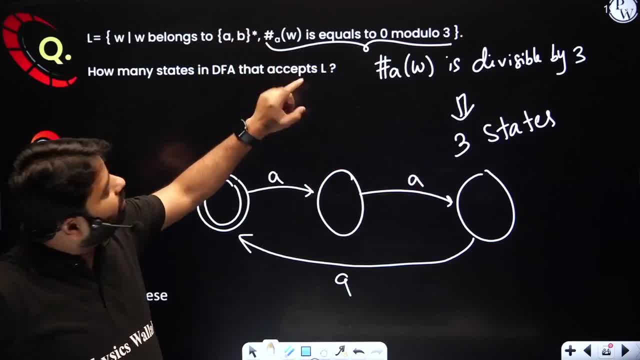 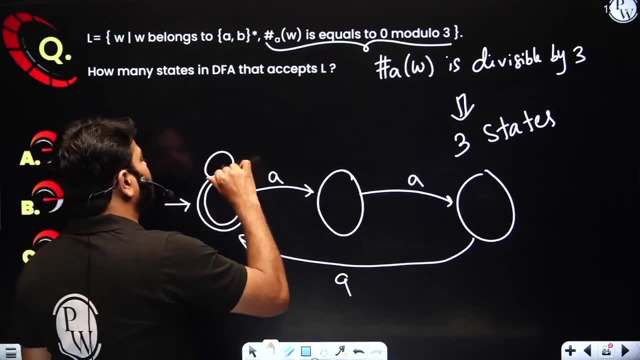 comma b: a comma b, but here b's we don't care, only a's we are counting. so every a you are changing the state. b is what you should do. you don't count because that is the: not going to count the number of a's, to put a self loop. 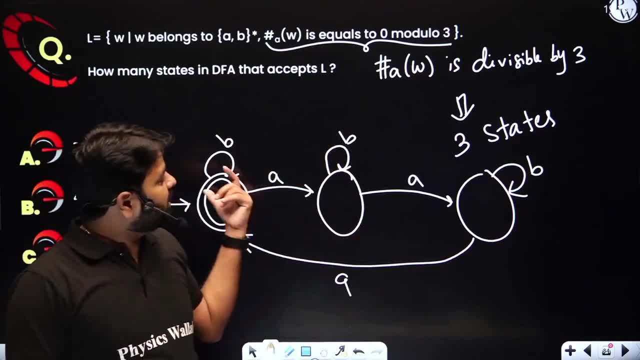 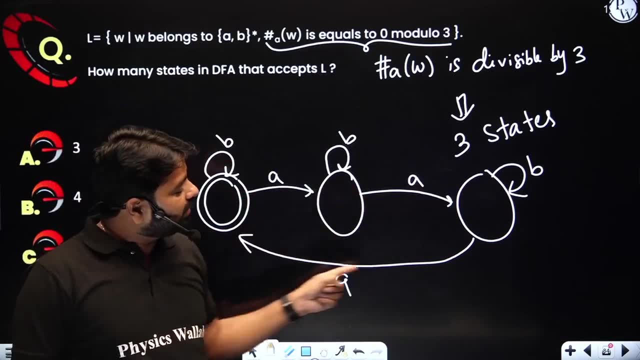 number of states, three here and there, but there b self loop you don't have, as you are counting a's and b's. a or b will consider as one length, but here a is only counted to check this condition, where a is divisible by three or not. 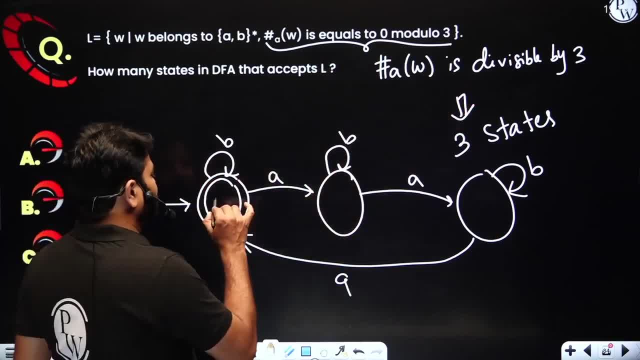 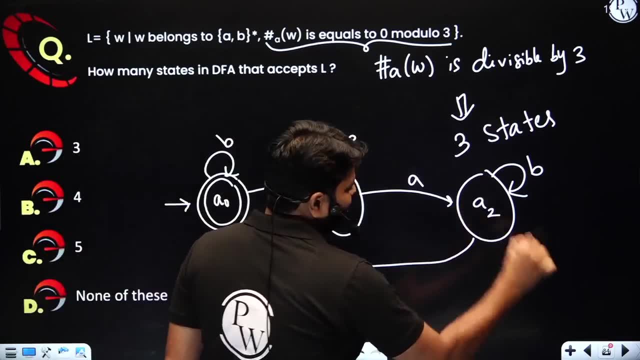 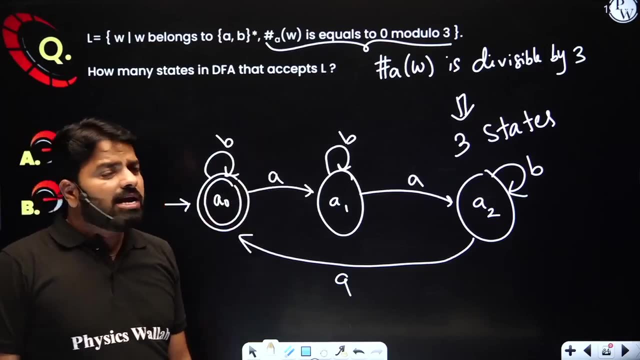 now, a is divisible by three. okay, let me write: uh, this state is a zero, a one, because, as i am counting the remainder, okay now, if i make the state a zero as a final, you got the number of a's is divisible by three. if i make a zero as a non-final, but a1, a2, both are final. 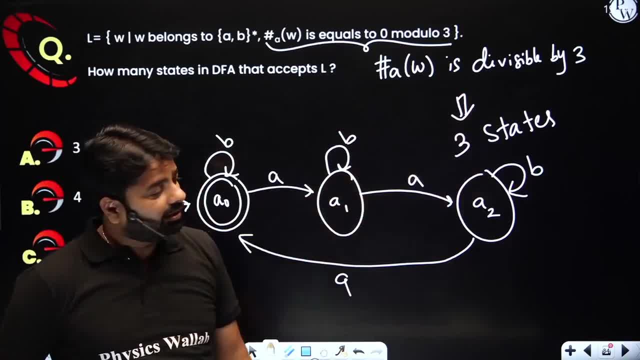 then number of a's is not divisible by three, it's a complement. if i make this, two are final, this is non-final, then obviously it's a complement of this language. right in case. only if i make this is the final, a1 is the final, then number of a's is equal to b is divisible by three. 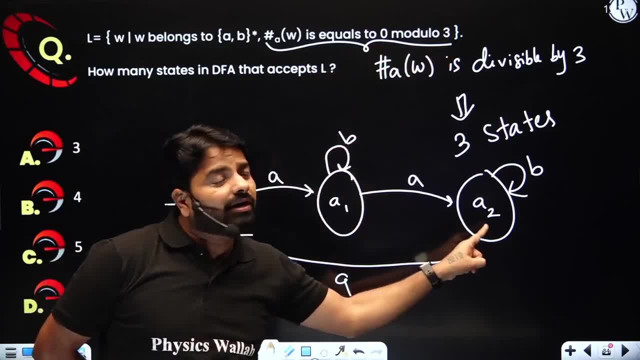 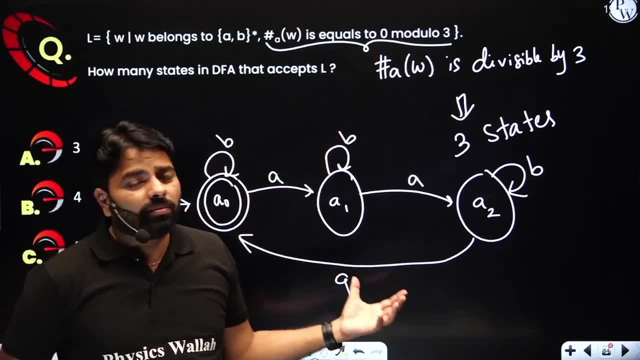 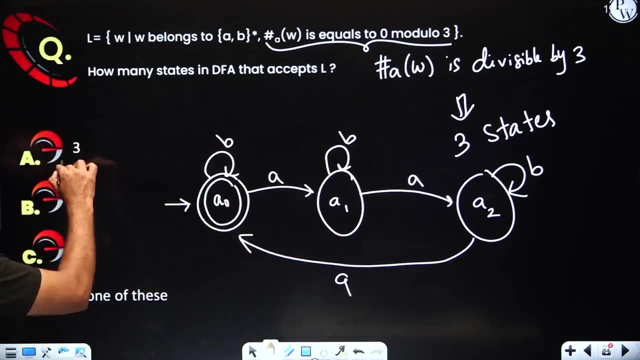 this is equal to one modulo three. if i make only this is the final two modulo three. so all depends on your condition. if you know this machine you can solve lot of problems which are depending on this divisibility. fine, how many states three? of course, this can be answered in two or three seconds. 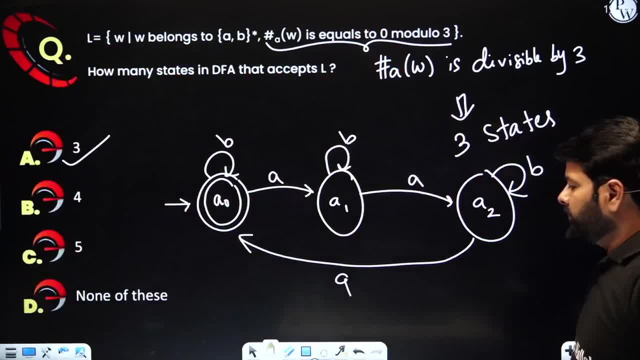 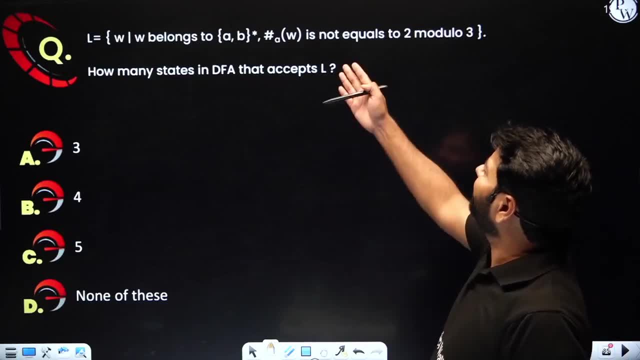 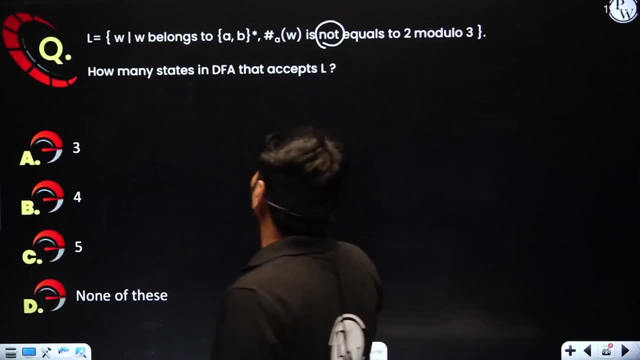 after reading this line: okay, five, five seconds at least. okay, i think, uh, okay, this is uh uh different. not equals to two modulo three. equals to two modulo three. what we'll make a2 as the final. let me design the machine first. okay, we have a0, we have a1. 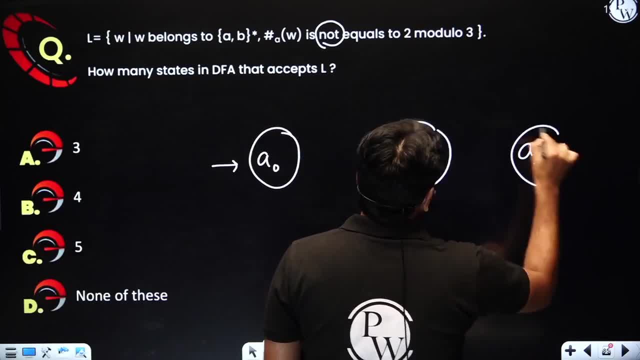 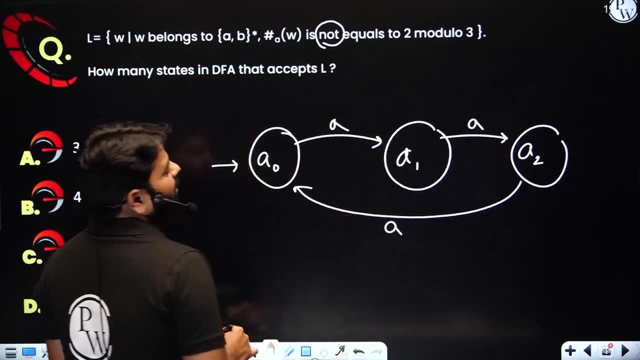 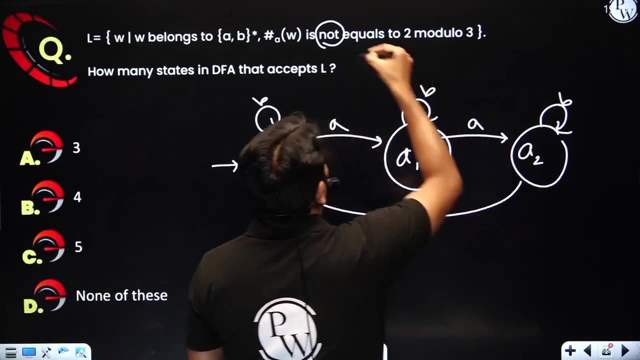 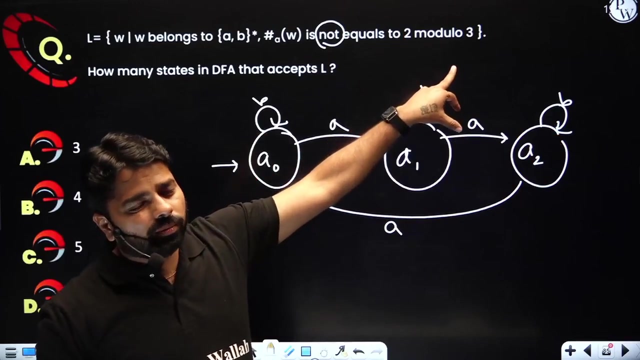 it's about a's only right. we have a2 and every a. you are changing the state to see the multiple of three concept and b's. you put a self loop. now who will be final? as per the question, number of a's equal to two modulo three means this two will be final. not equal to two means other than this two. 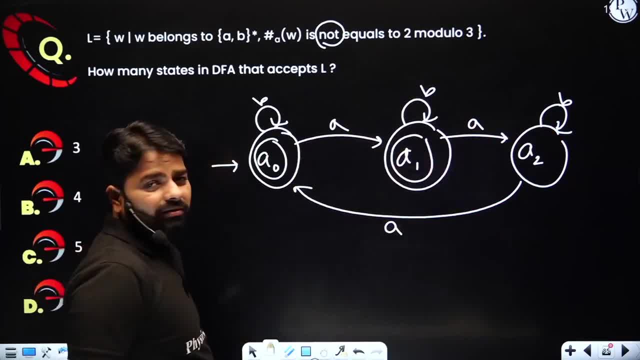 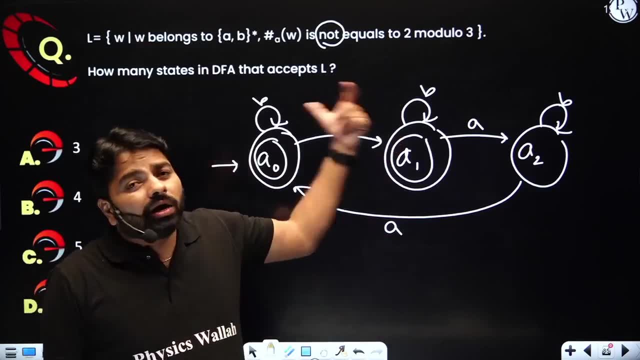 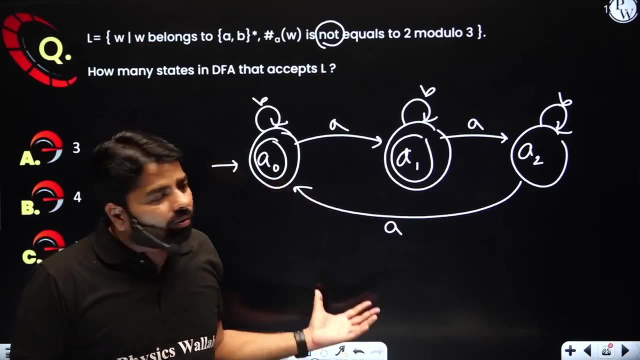 you will make. this. two are final, that's it. but again, the number of states would not vary in the exam. designing dfa is not important. understanding what dfa needed, right, who is final, non-final? you know it may take time, few seconds, but you already know it requires three states. go blindly. 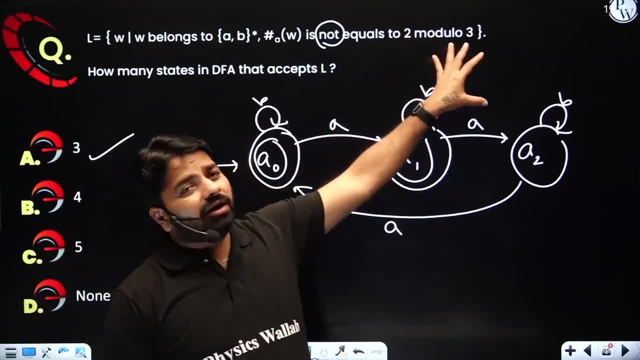 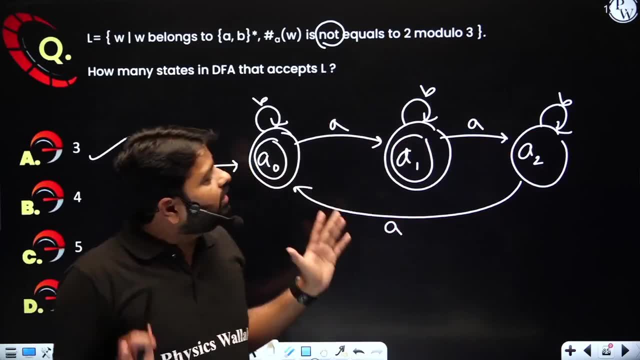 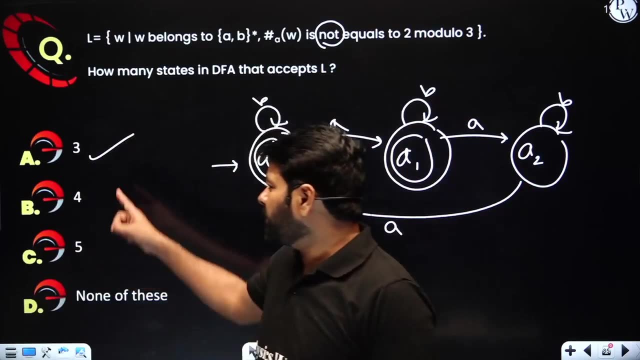 here, okay. so remember, unless you have some trick in the question, you don't need to wait for you know designing a dfa, you already know divisible by three concept, three states doesn't matter, only the finals are different. but whole machine is same. then make three as a number of states. 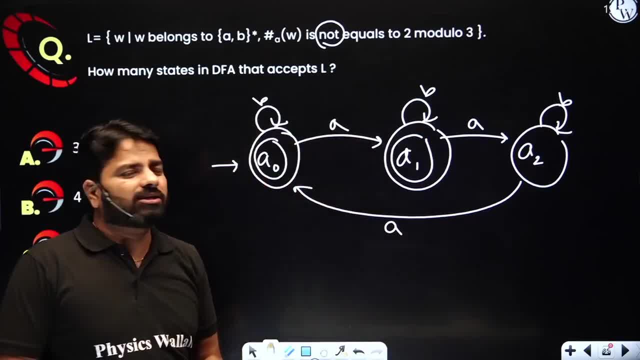 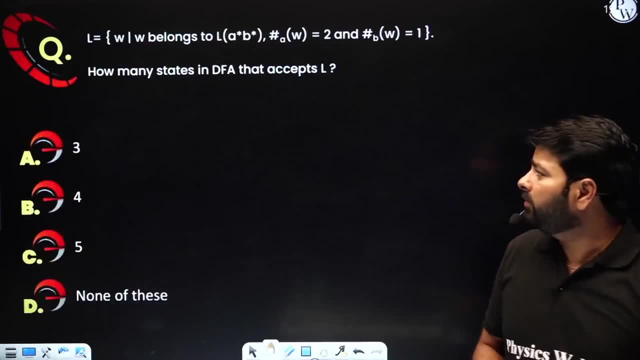 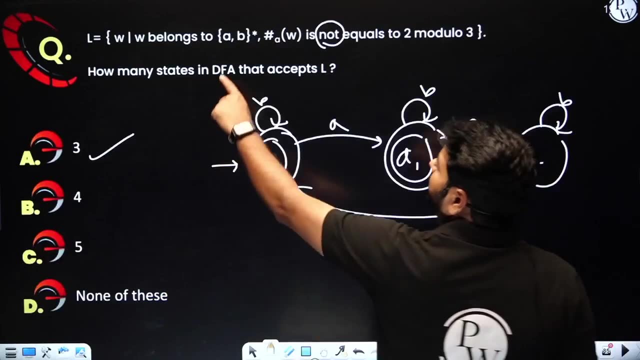 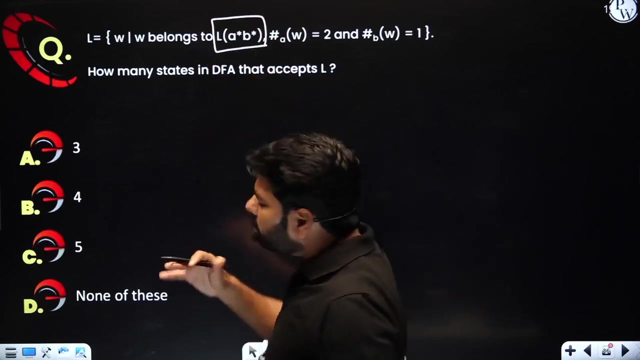 okay, it should take, just as per my knowledge, it will take max, you know, five to ten seconds, if you have solved uh this kind of problems during practice. oh, number of states? oh, this question is: uh see the difference. here you have a comma b whole star, and here you have a star b star. that's all you know you need to observe. w belongs to. 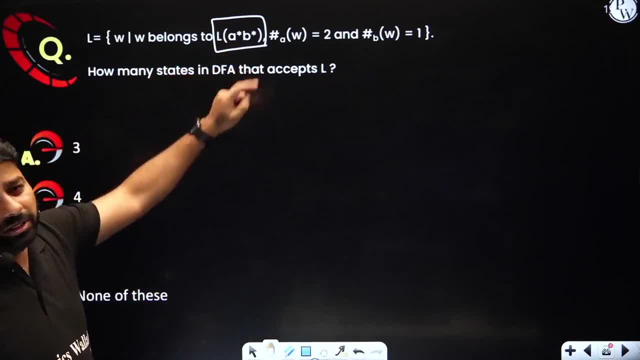 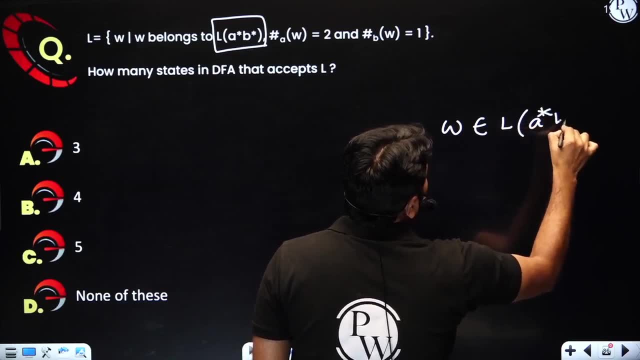 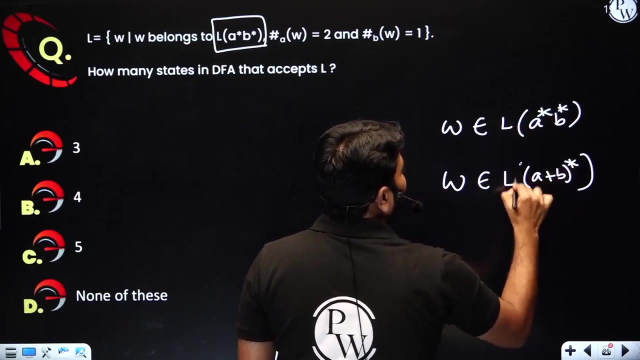 what? here there is a language over a star b star. so w here belongs to the language generated by a star b star, how it is different from w belongs to an a to b star or a really a b star. this symbol, this symbol today, is the language generated by. 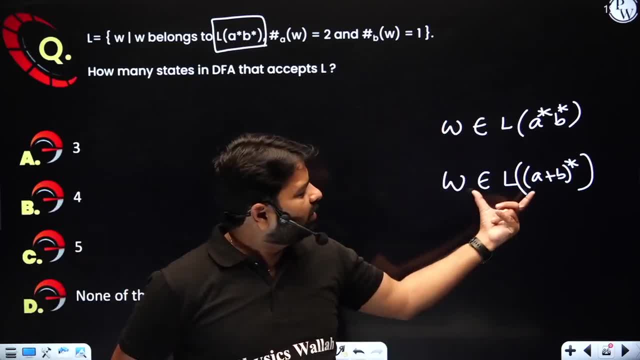 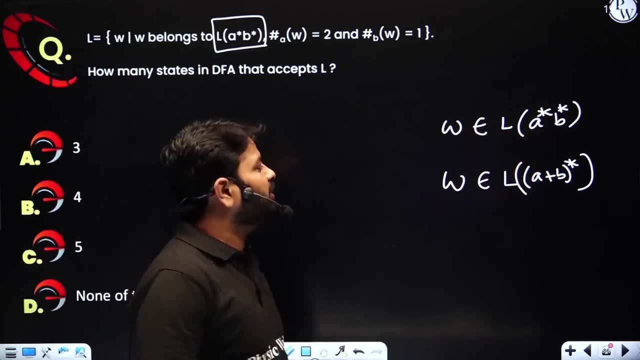 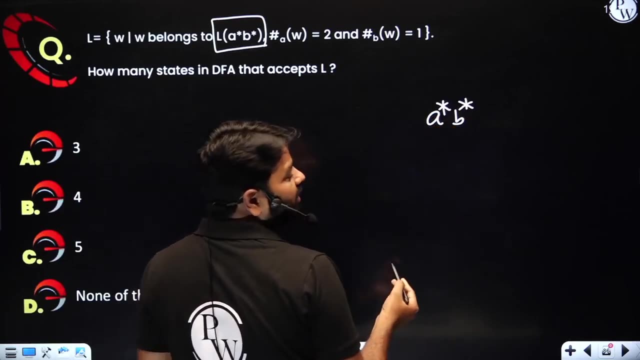 a plus b whole star. okay, this was the previous concept we are solving. w belongs to a comma b whole star. we are, we were always taken from here. but now you need to look at a star b star. what is a star b star? what is a plus b whole star? let's focus on that. a star b star means the strings. 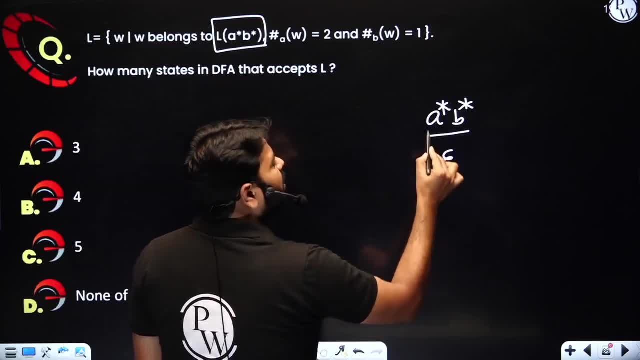 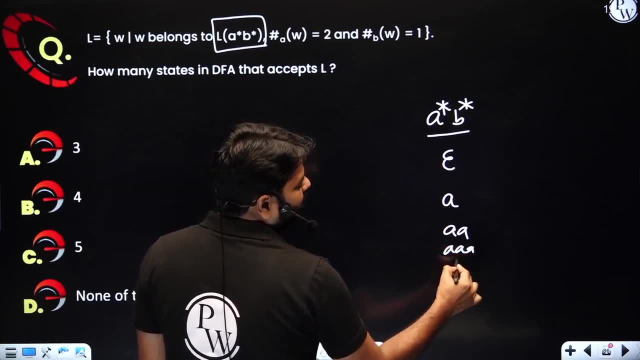 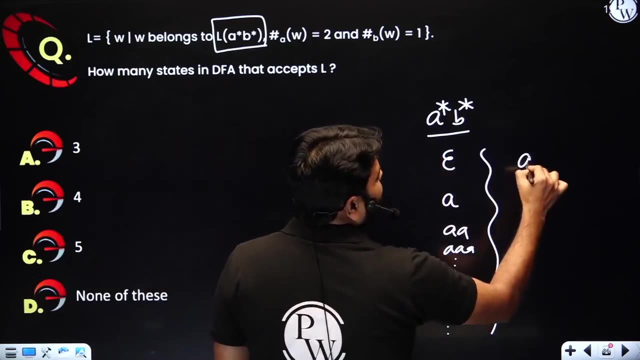 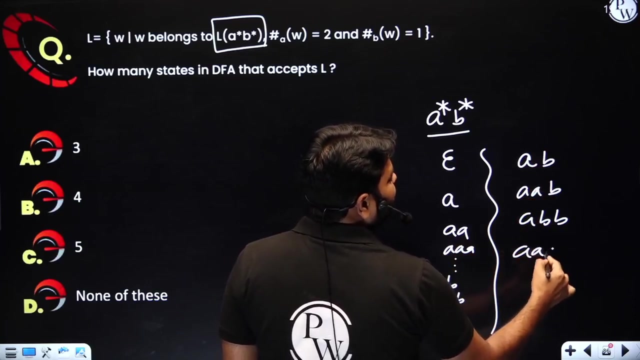 having a particular sequence. a is followed by b's means it may be epsilon or it may be only a pr stages. you have like only a's, a double a, triple a or only b's, or you can have, you can have- a any number of b's, like a b, a a b or a double b, but the sequence is very important. double a. 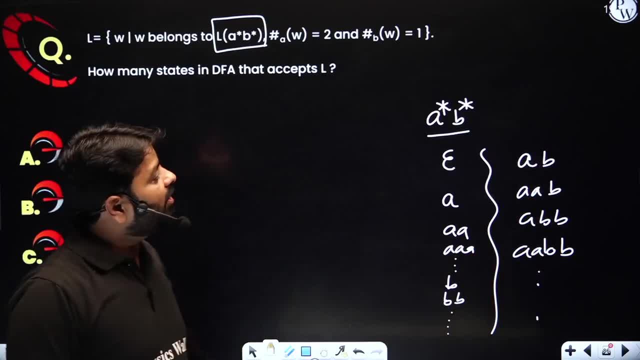 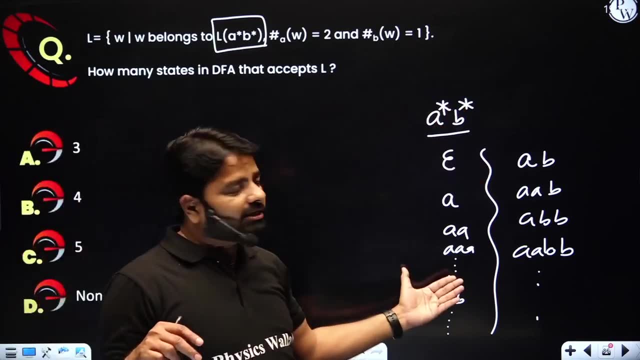 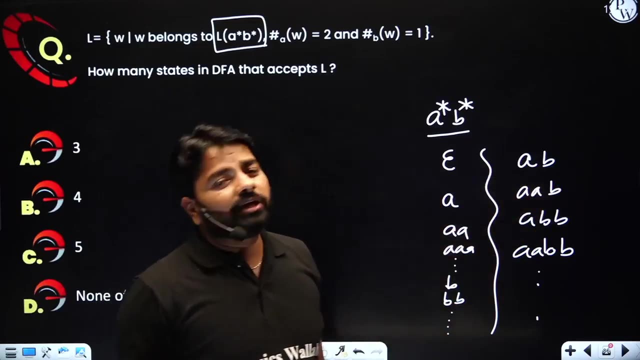 double b, so on, but you will never have after b a. it's very clear. the string will have the a's followed by b's, that's all. a's may be present, or b's may be present, or no a, no b present. if both are present, a's followed by b's. so you have the few things that you observe. epsilon is valid. 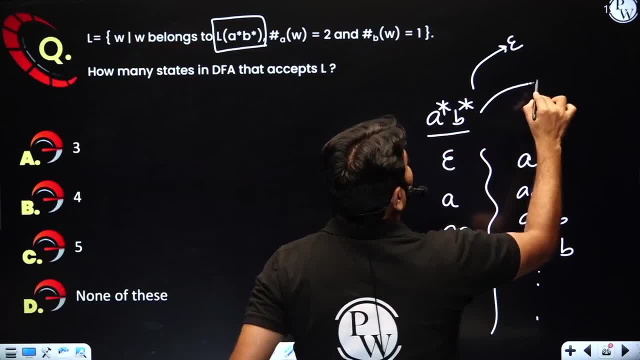 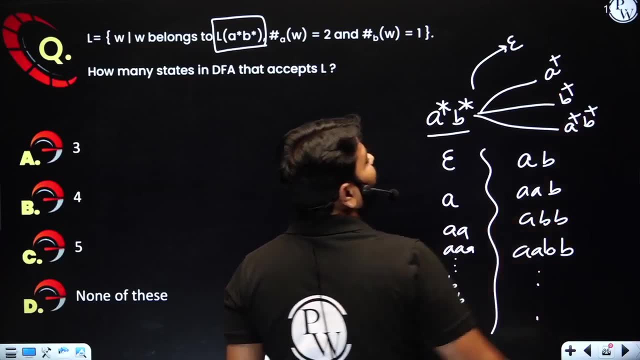 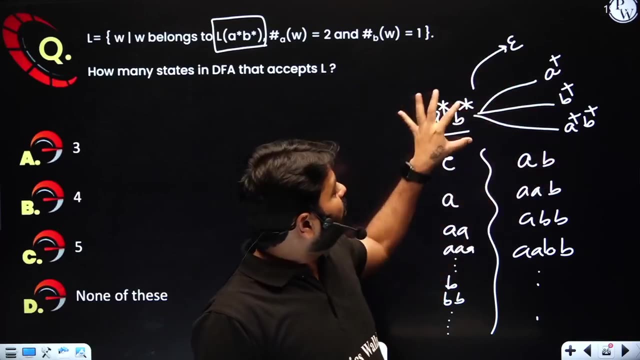 of course, in this only- i'm not talking about this here- only a's valid, only b's valid and both are valid, a's, followed by b's, both when both are present. all the four. when you combine you will get a star, b star. look at what i have done. when nobody. 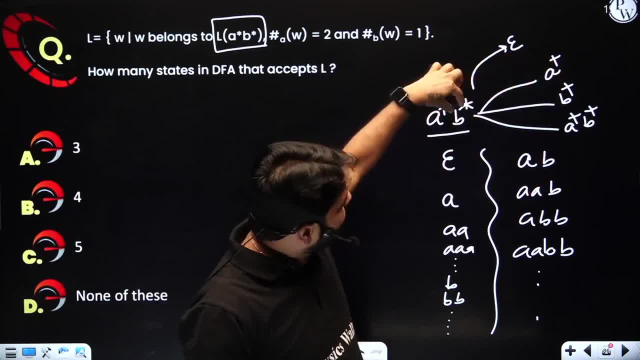 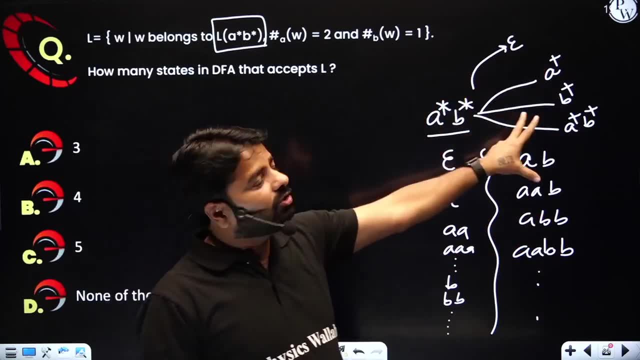 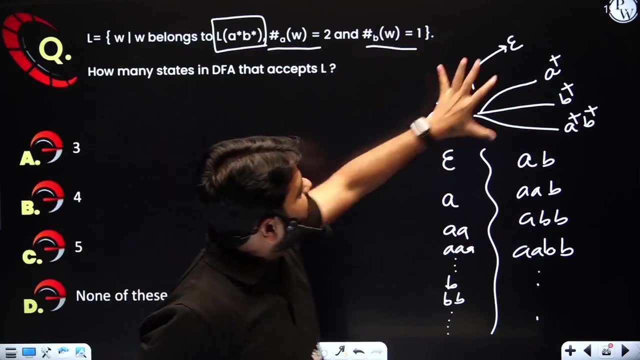 is there epsilon, only a's. are there a plus only b's. are there b plus? when both are there, a plus b plus. so this four combinations are there here. in this we are going to look at our condition that number of a's is equal to two and number of b's equal to one. that means this three will not. 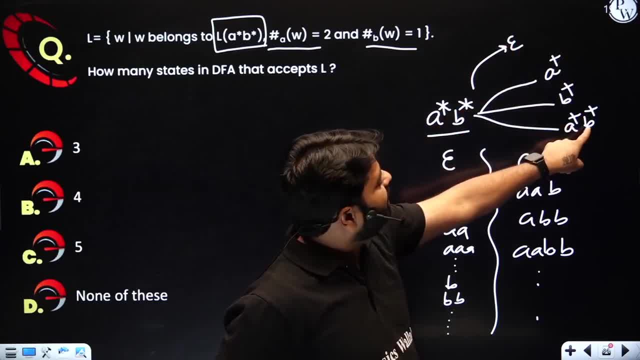 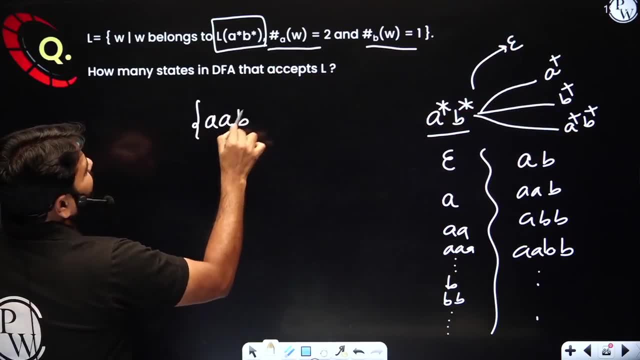 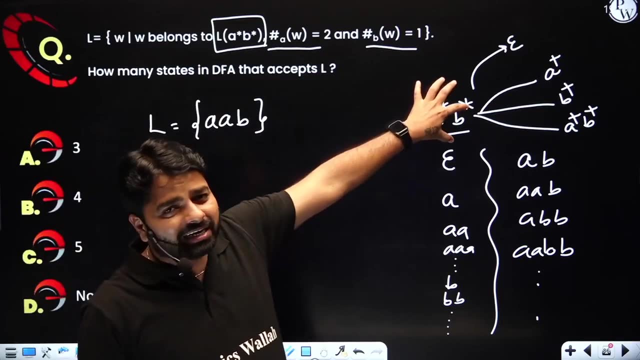 be there only in this, when a is two, when when b is equal to one, that is uh, straightforward, right? just one string, double a, b, that's all. this is your language. one string only. you don't need to think much about right, this is having infinite strings from them, a power to b, power one is your problem. how many strings? one string. 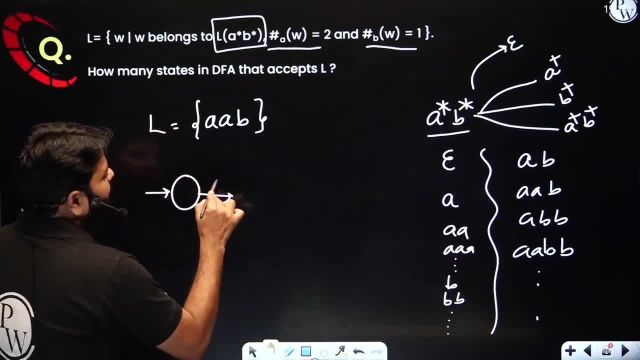 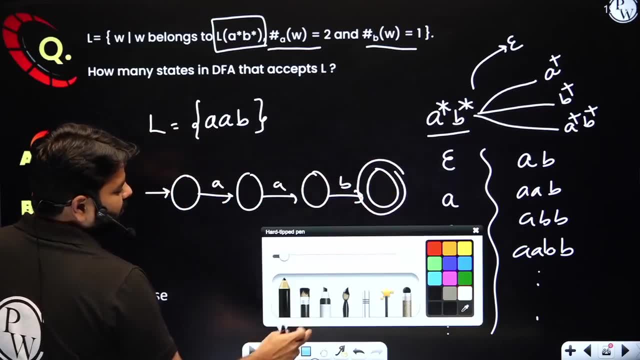 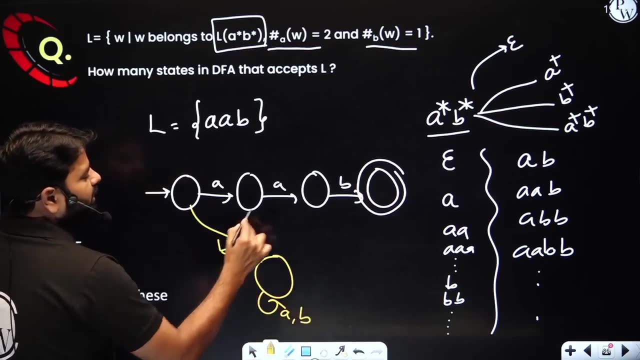 can't be designed: double a followed by b. everything else you go to dead. we don't have any combination other than this one string, so easy to design right. anything you go to what dead state. anything else here? b cannot come here. b cannot come here b is there? a cannot come here. a or b. 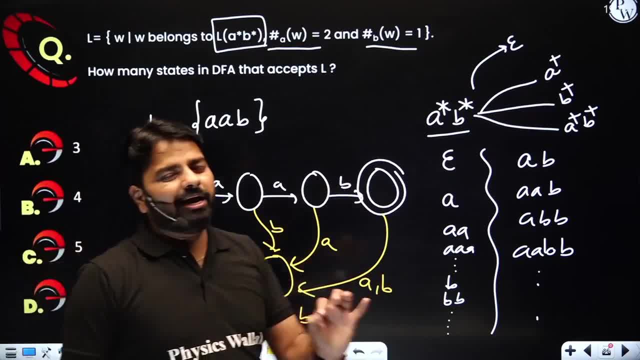 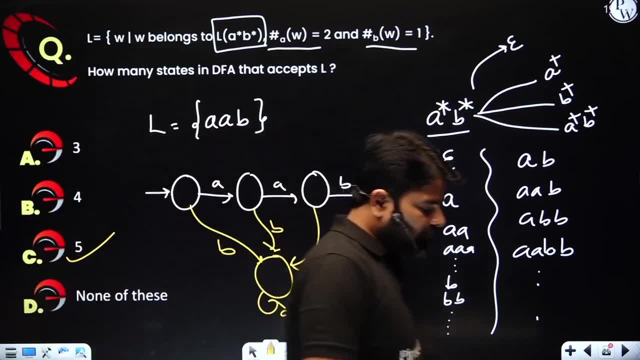 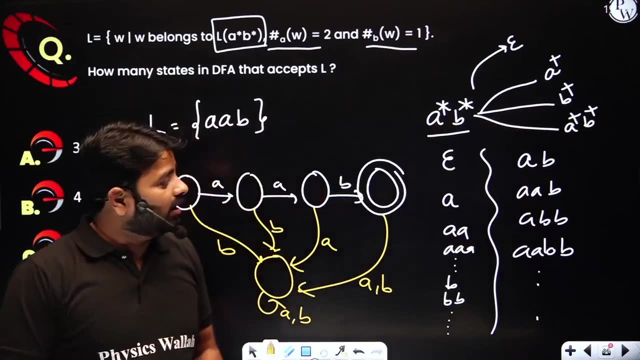 cannot come. as you know, only one string should accept a, a, b, no other string. so how many states required? five states: click answer. fine, okay, similarly, i'll be giving you a lot of homework questions. you can practice and answer it the number of states of the below this video. so let 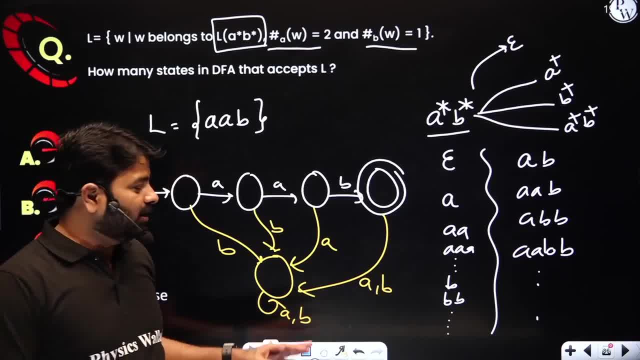 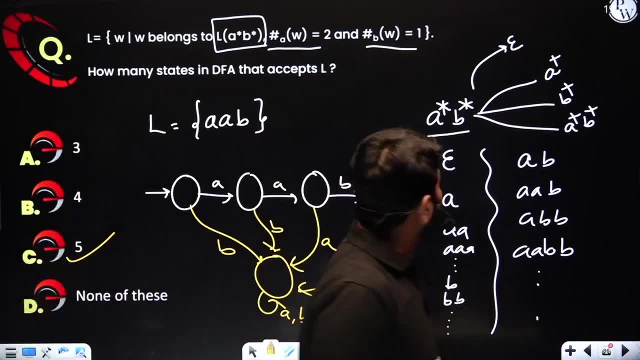 me know in the comment section you should practice at any cost. in case, if you have a doubt, you can post your doubt below this video in comment section. i'll be replying it. so next question is homework for you. how many states in dfa that acts well where the same concept- a, star b, star w- belongs? 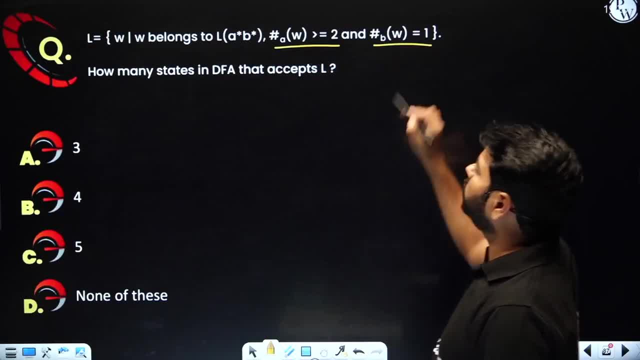 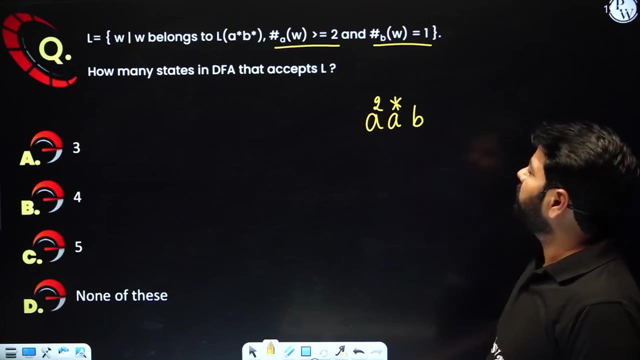 to, but is it is not equal to, b is equal to one, then how do you write it? a, at least two right, a power. so here you. i'm writing here: a power, two, a star, of course together. you can write some other way too. i'm not doing that. and b, that's it. so this is your problem. 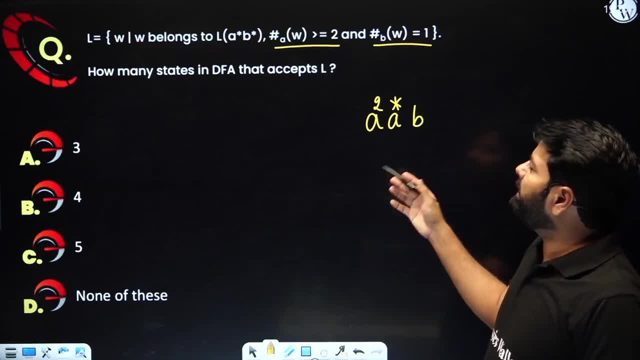 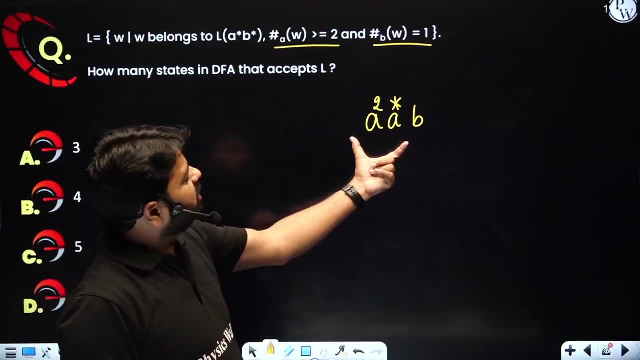 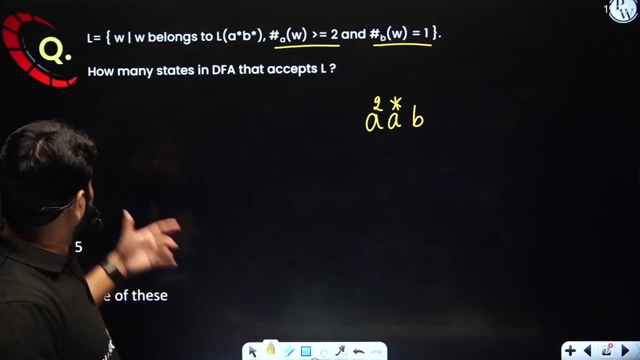 and language will have lot of strings, but minimum single will be double a b. so if you design double a b, then your problem will be simple. so this is your expression, this is your language, and now you try to accept all the strings from this expression and tell me how many number of states. 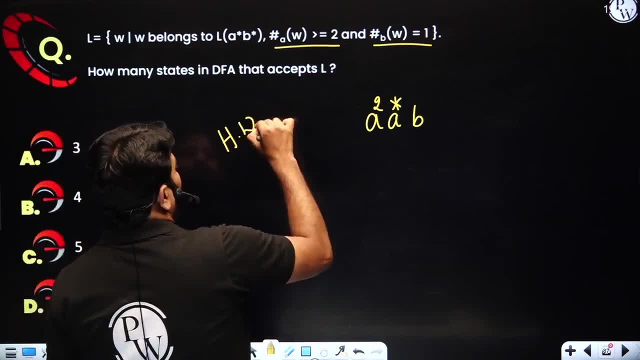 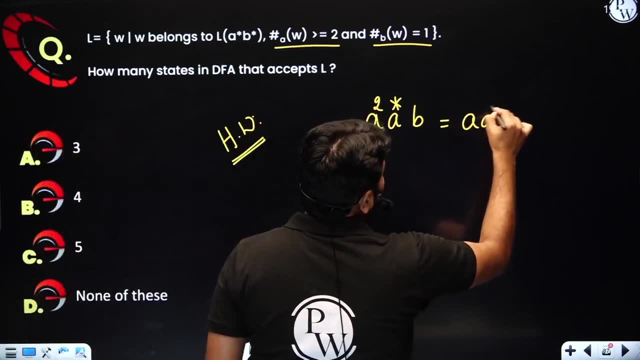 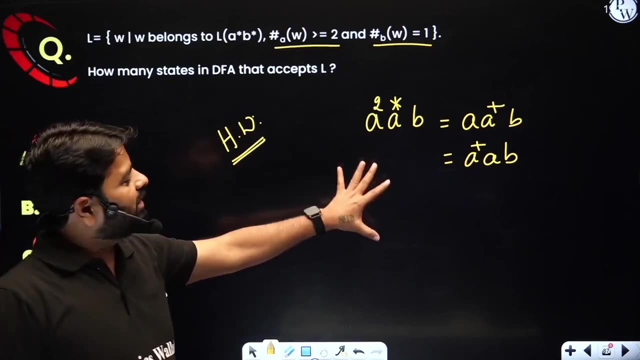 i hope you can do it. please take it as homework and i believe you can answer it very easily. okay, you may represent many other ways, like you know: a a plus b, or a plus a b- i don't care how do you write it, all are same. but you should know how to design the dfa for this. 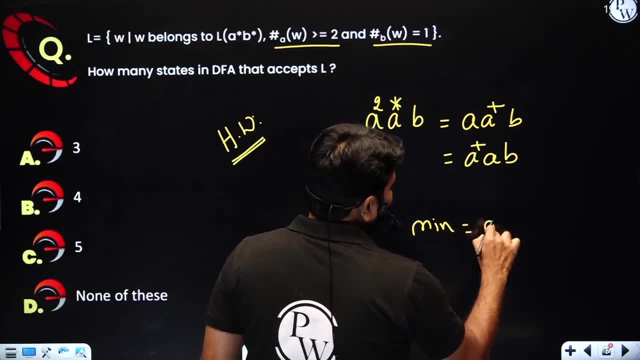 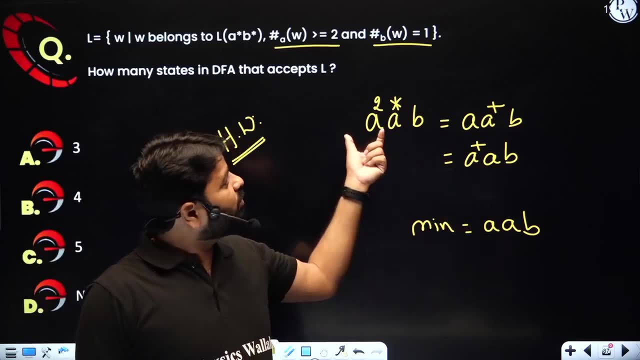 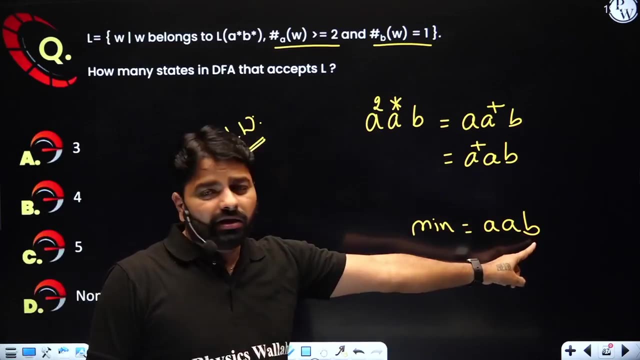 take minimum string. i'm giving hint: double a, b. how do you do that? now? how do you do that? i should have two a's. i should have two a's. must right in this process, beginning b should never come. so if b comes, go to red state. once you have the b, only one b. so after b, either a or b go to. 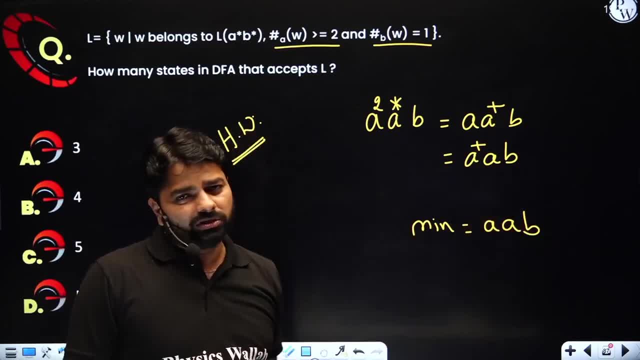 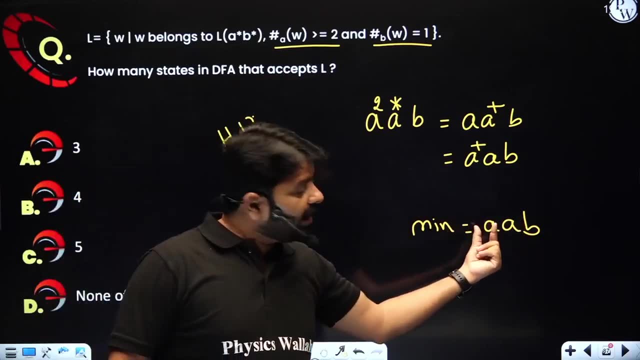 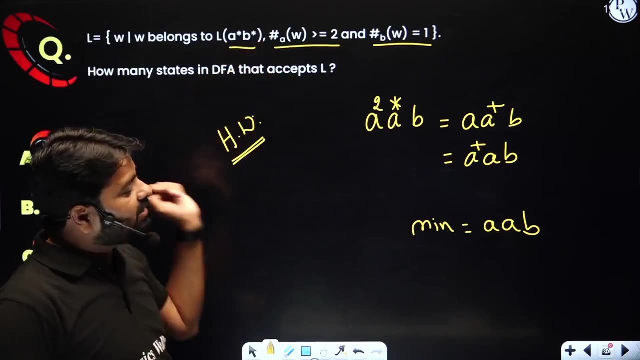 red state because second b never be there and after b a never comes. the sequence has one beauty is here that after b a never comes, before a b never comes. so these points you should remember as you have a sequence right. so when you have a sequence like a's followed by b's, the many things you can easily 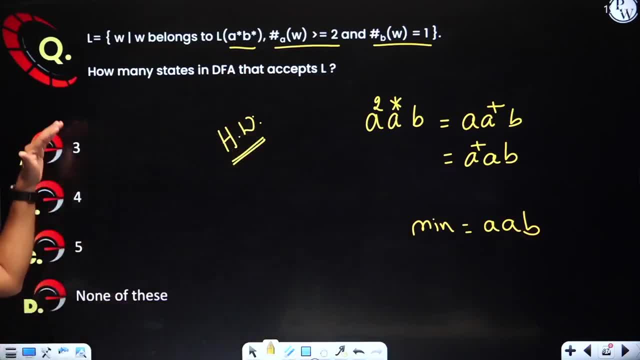 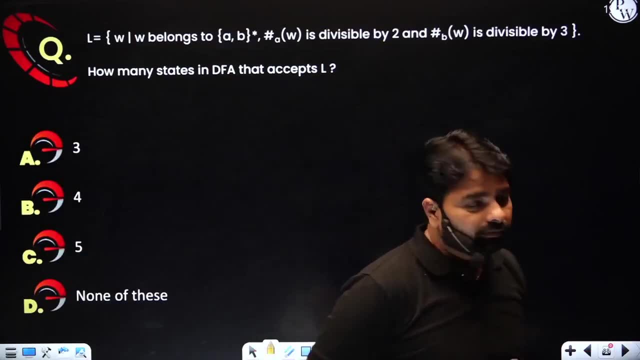 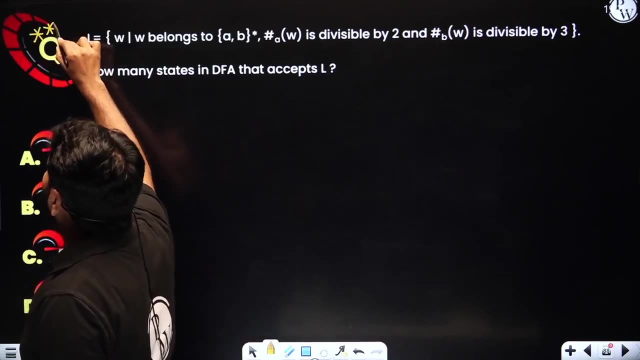 observe. fine, so i believe you may answer something here. so i'll see below this video, your comment whether it's right or wrong. okay, next one, very interesting, and this was a gate: p by q multiple times, not one time again. number of a's is divisible by two and number of b's is divisible by three. so when this 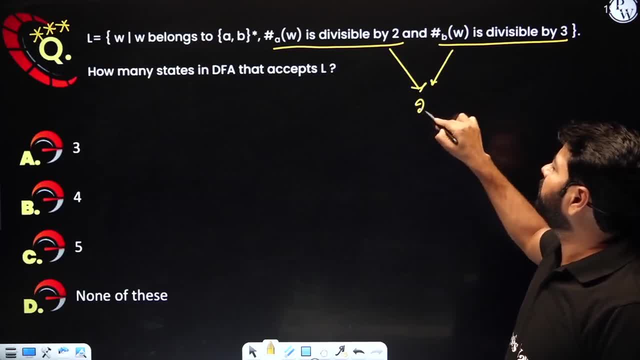 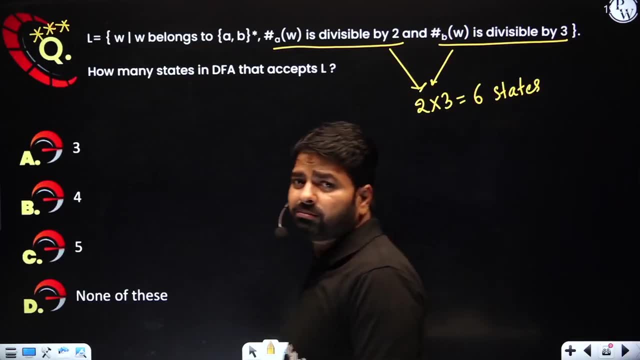 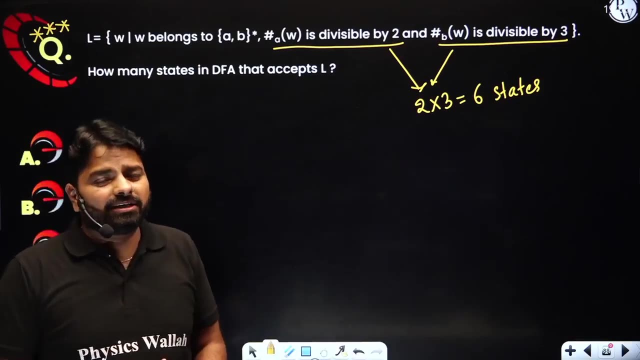 question comes the straight away. the multiplication to multiply with three, six states is an answer, because you should know why the six states comes. but in the exam answer is six. but before the exam, know why it is six. right, you should save your time in the exam, right? you can't design even you know it. 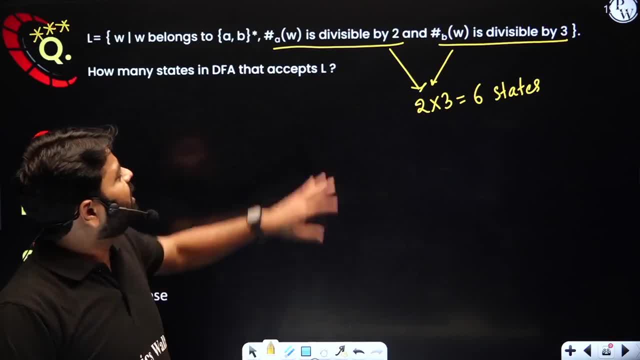 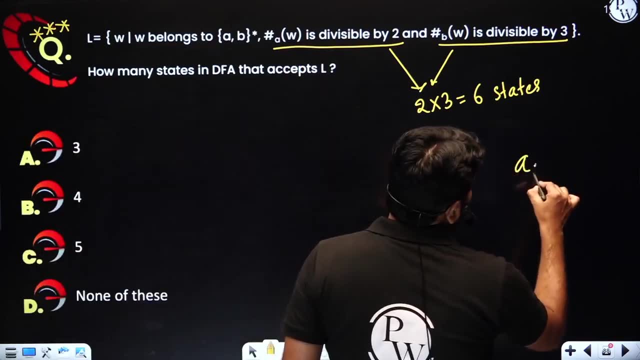 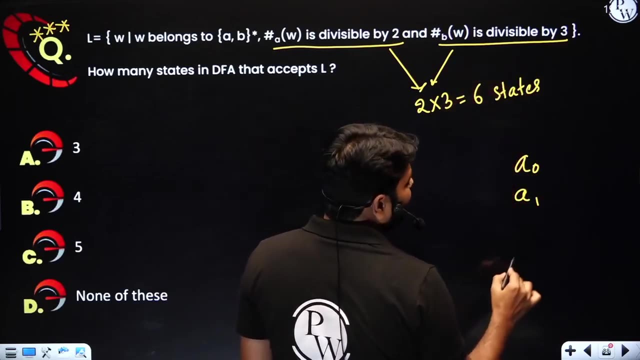 okay now why six states? the reason is number of a's. when you divide with two, you will have two remainders. let's say a0 and a1, two remainders for a's when you divide number of a's with two. when you divide number of b's with three, you will have three remainders. 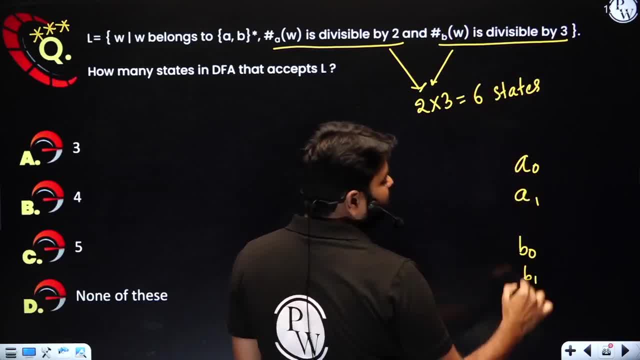 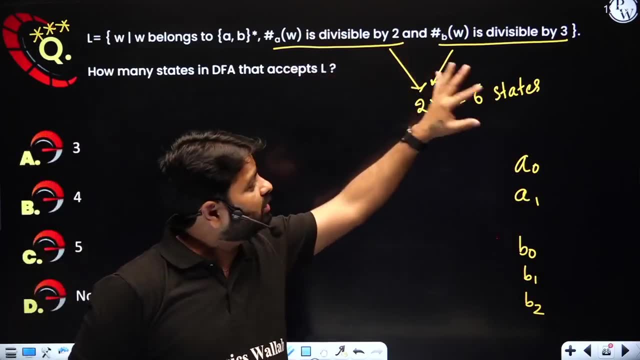 for b0, three remainders for the b's, b0, b1, b2. so overall you may have any combination like a's could be any remainder, b's could be any remainder. so when you look at the cortesian product, two multiply with three you will get all the six combination like you should know. 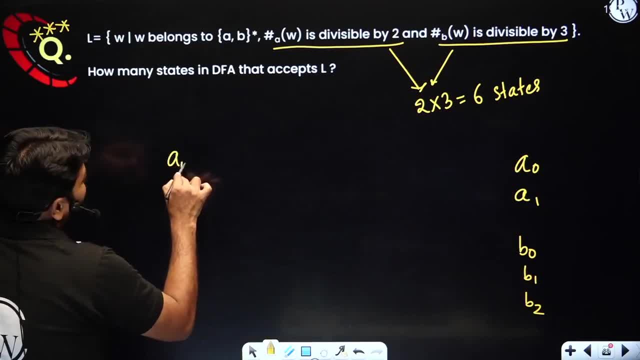 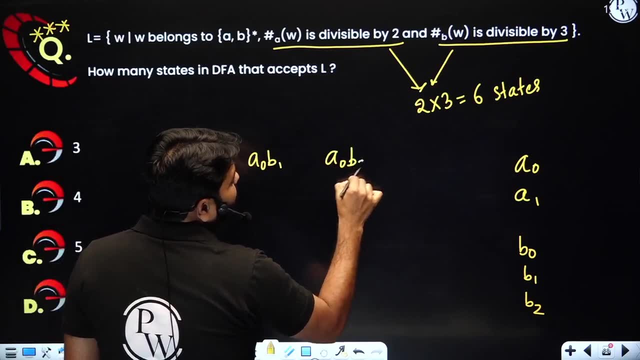 sequence doesn't matter: a0, b0, b0 doesn't matter. like a0, b01, state now a0, b1, another state a0, b2. but don't assume that after a becomes, we are not talking about after, you can write b2, a0 also doesn't matter here, because 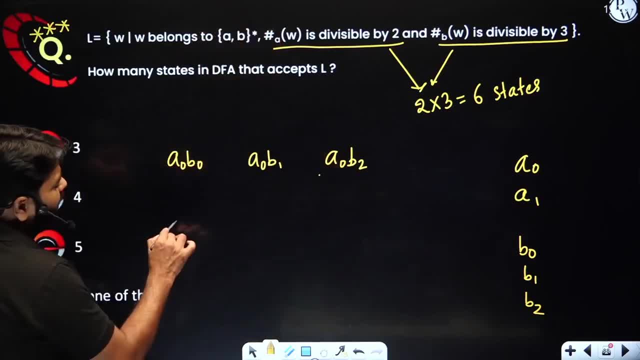 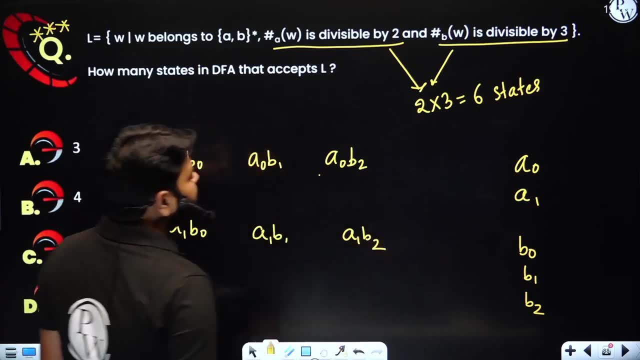 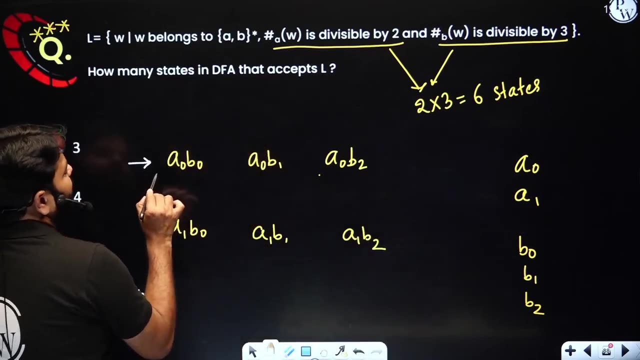 w is over a comma, b, whole star, a1, b0 and a1, b1, combination only. I am talking about a1, b2, so this many states are there. initial state is a0, b0 and the meaning I have written. 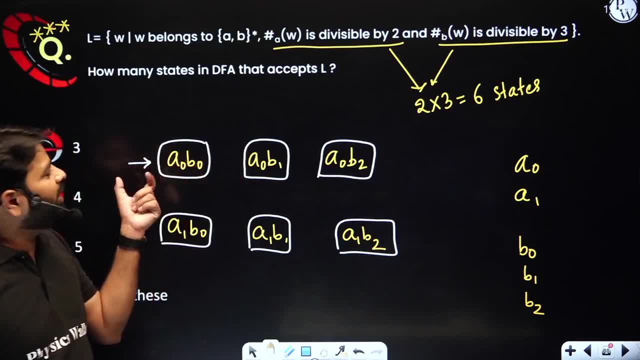 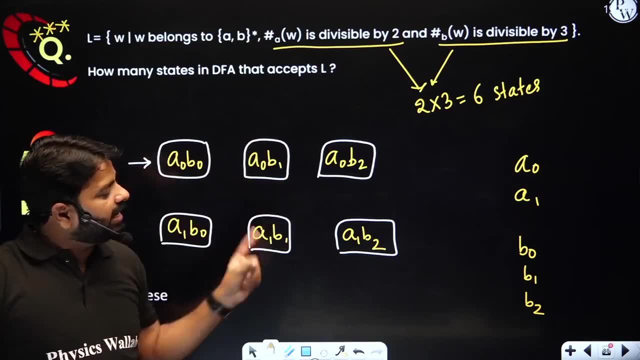 the meaning of every state. when you stay here. it means the number of a's is divisible by 2 and number of b's is divisible by 3, so every state has a meaning if you stay here, if you come here, if you halt here. number of a's. 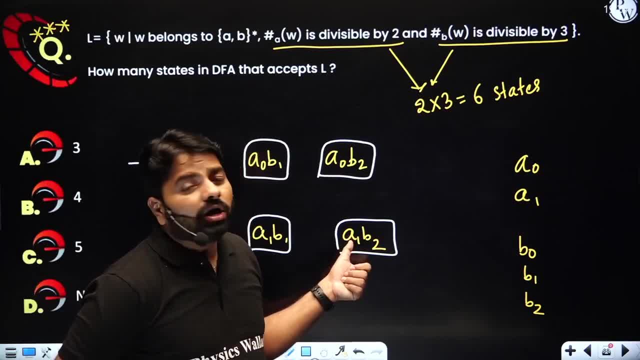 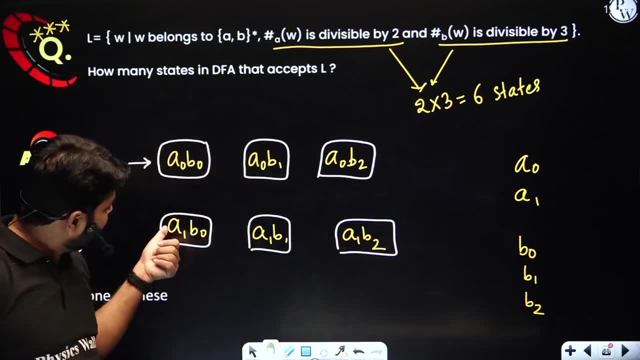 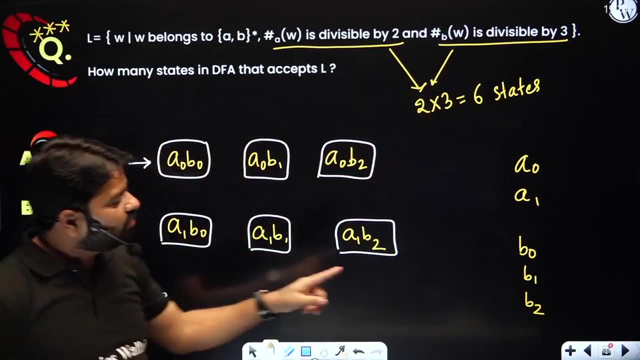 is not divisible by 2,. it means 1 modulo 2, number of b's 2 modulo 3. when you stay here, and when you stay here, number of a's is 1 modulo 2. number of b's is divisible by 3 because b is 0. so whenever you see b 0, b is 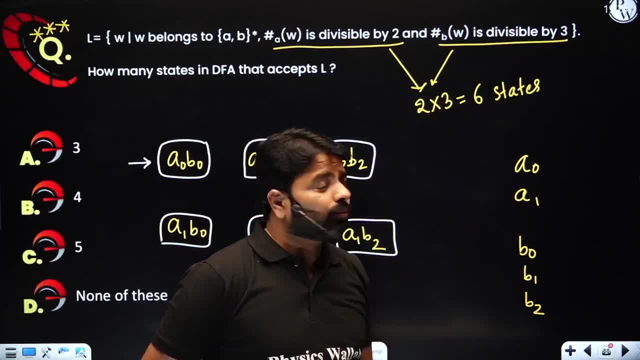 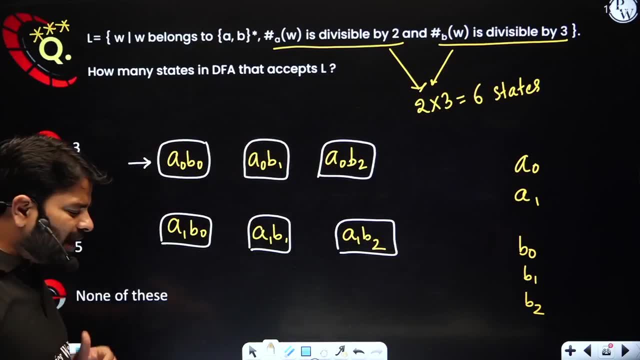 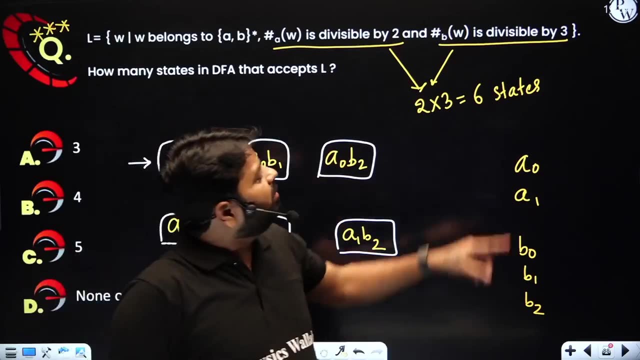 divisible by 3. whenever you see a 0, a is divisible by 2. so 2 for a's, 3 for b's. remember the relation? now, very simple: whenever you have a's, count on a's, always divide with 2. whenever you have, whenever you get the b's, count b's, but always divide with 3, let's do it. 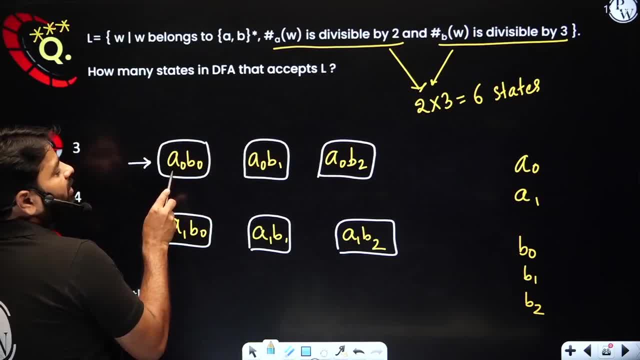 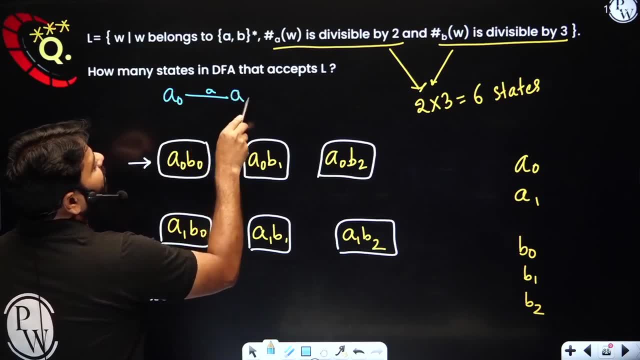 now from this a comes. already a's are 0 here. if one more a comes, the 0 become 1. so look at here: a 0. if one more a comes, it will become a 1, b will be same, b will be same, so you will go there. 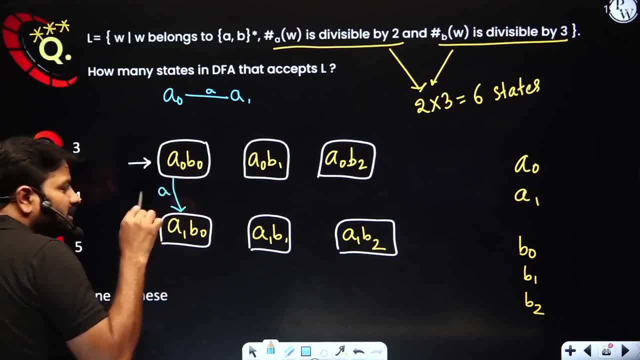 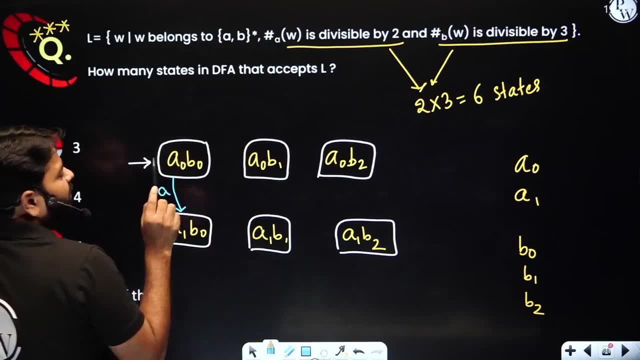 so here, look at on 1: a just increase the number of a's, increase the number of a's. okay. so from every state i'm going to do that: from this state, a covered and from this state b, i will cover if i increase 0 to 1. 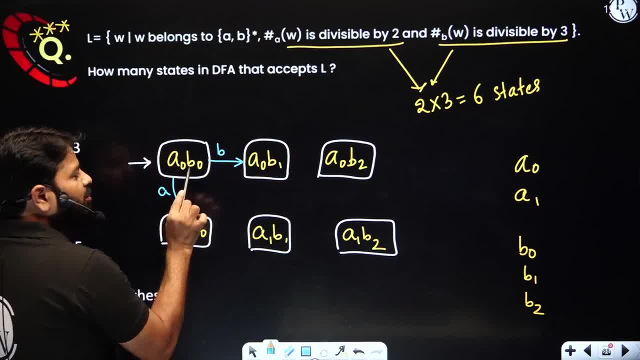 so from this state a covered and from this state b, i will cover if i increase 0 to 1. so from this state a covered and from this state b, i will cover if i increase 0 to 1 because i'm getting a 1 b. do i go here check b 0 become b 1, but a should be same as i'm not. 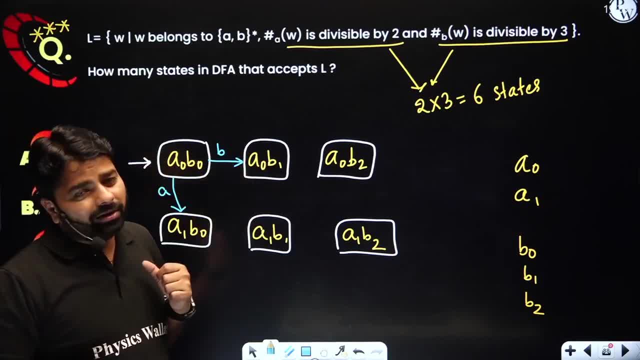 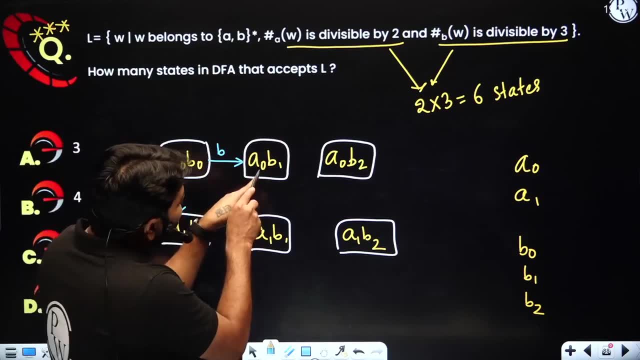 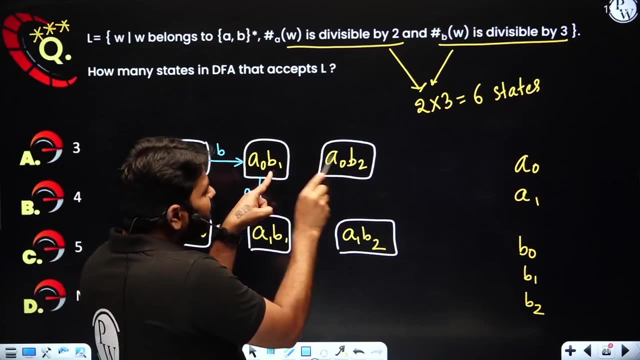 counting a's to move from here to here, because b's are only coming, okay, from this state, a and b covered. similarly, can you do for every state from this state: cover a and b. if you get a, this 0 become 1, so you will get here. b should be same a and if you get a, b, b 1 become b, 2, but a's will. 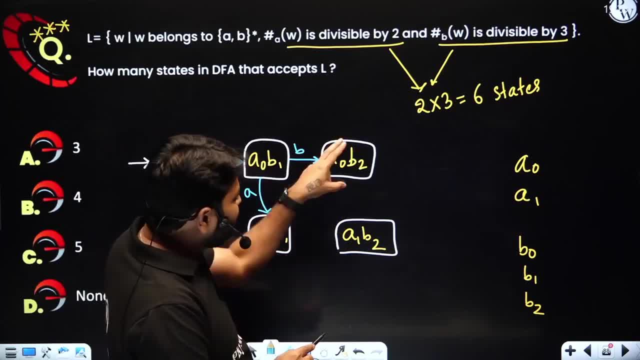 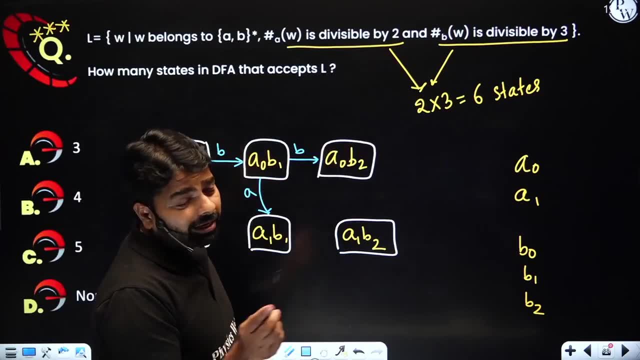 be same. okay, from this state, if a comes 0 to 1, b should be same a. and if you get a, b, b, 1 become 0, become 1. but always remember, when it crosses 1, then you must divide with 2, because remainder. 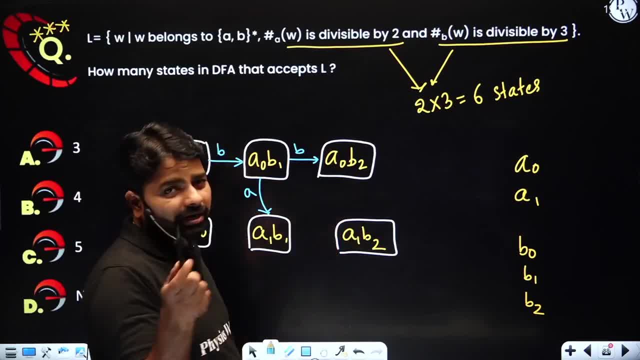 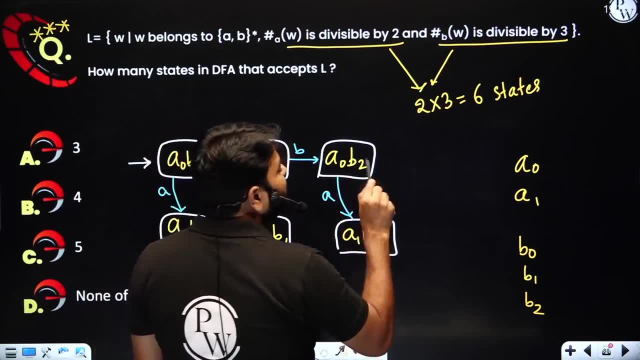 never be 2. it should. when 2 comes, remainder has to be 0. so now, when a comes, 0 become 1, but b's will be same. now look at here: when b comes, b 2 become b 3, but b 3 will not be there. 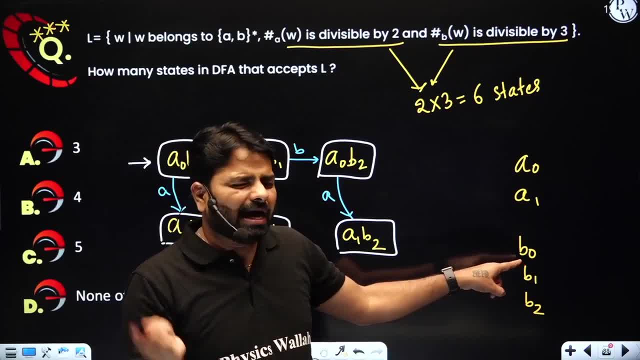 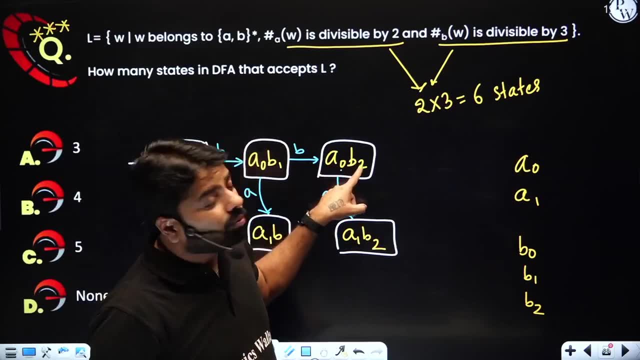 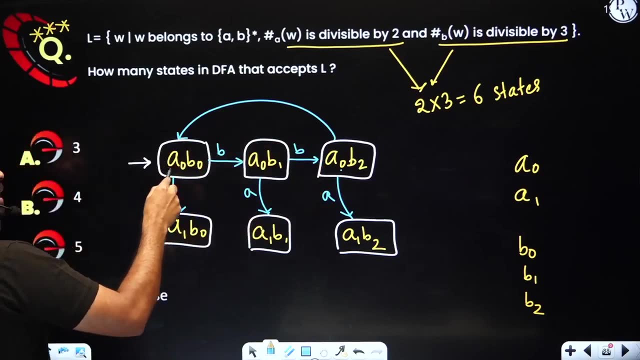 because b 3 means b 0. remainder has to be 0 when 3 b's comes, so a 0. when b 2 become b 3, a 0, b 0 happens here. so when third b comes, the b 2 followed by b will become b 0, as you are. 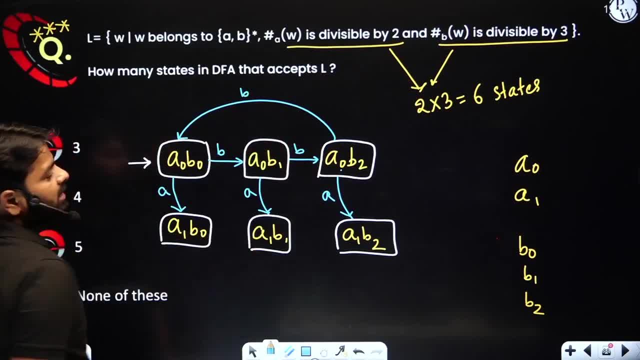 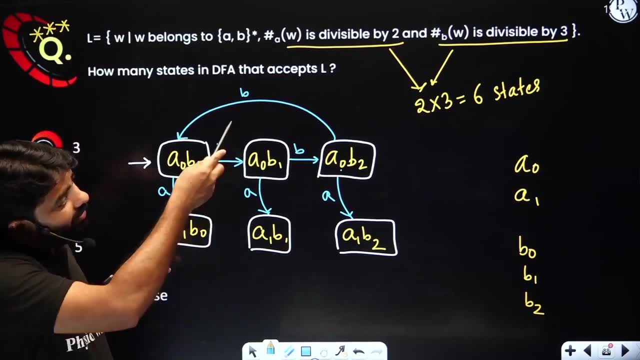 dividing with 3, so which is on b. similarly now here, if one more a comes, it's already 1 a right, one more a comes, it will become a 2, but a 2 divide with 2 that it will become a 0, so we will. 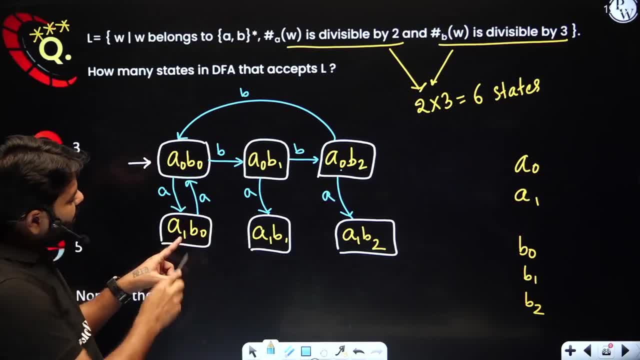 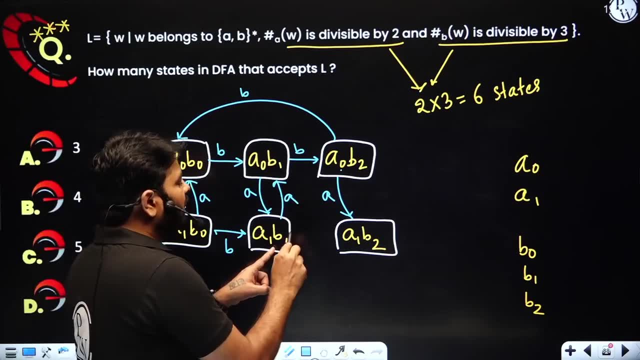 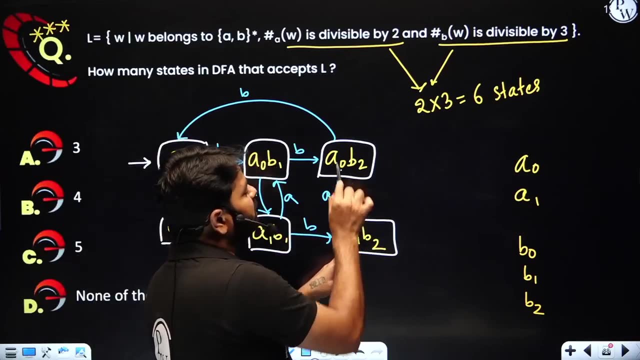 go back here and b b 0 become b 1. i hope you understood. then copy: a 1 become a 0 by adding one more a and b comes will go here, because b 1 become b 2 and a will be same. and here, if a comes, a 1 become a 2, but 2 divided with 2 is 0 remainder. so 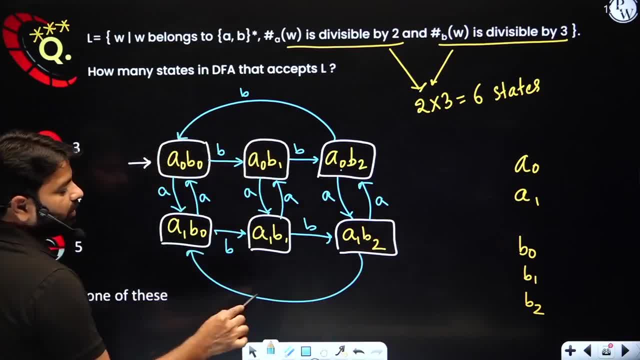 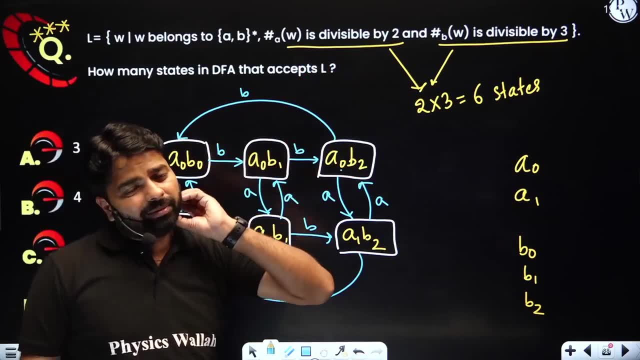 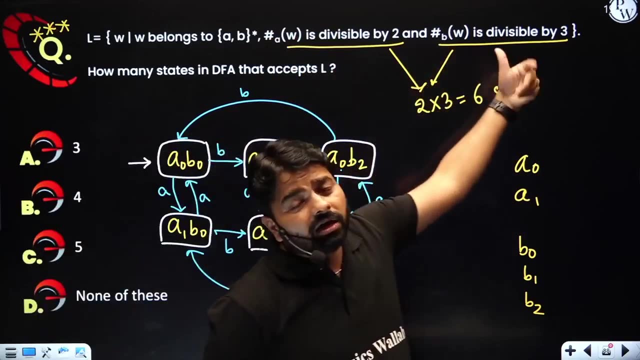 we will go there. b you come back. b 2 will become b 0. fine, so this is the machine where number of a is divisible by 2 and number of b is divisible by 3. each state has a meaning in the exam. they may ask differently. like a is not divisible by 2, b is divisible by 2. 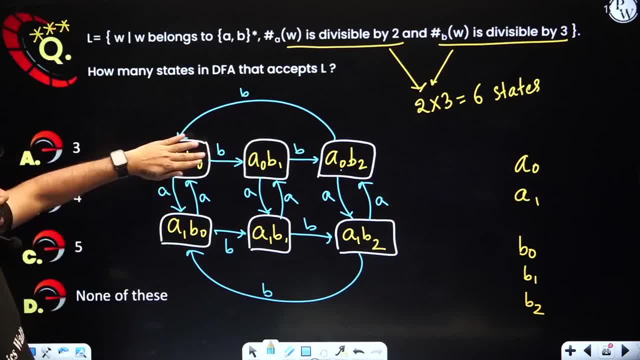 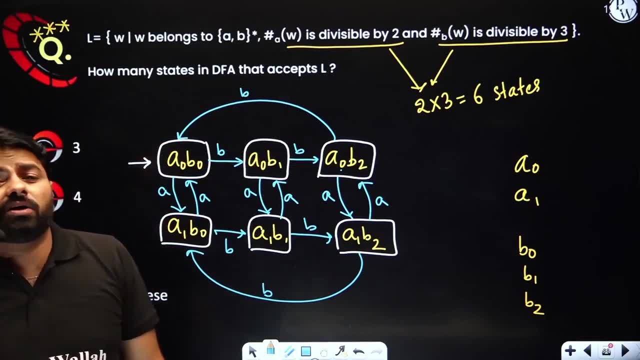 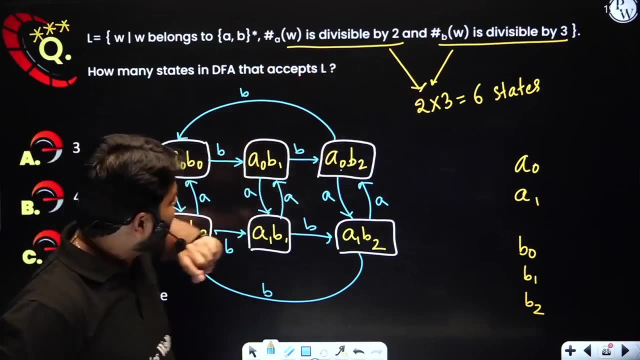 is not divisible by 3. answer is here, no doubt, except this: you make. all these are final. then what do you have? ac is not divisible by 2, as well as b is not divisible by 3. so if you make- oh sorry, which one? i'm very sorry. ac is not divisible by 2 and this is not divisible by 3. 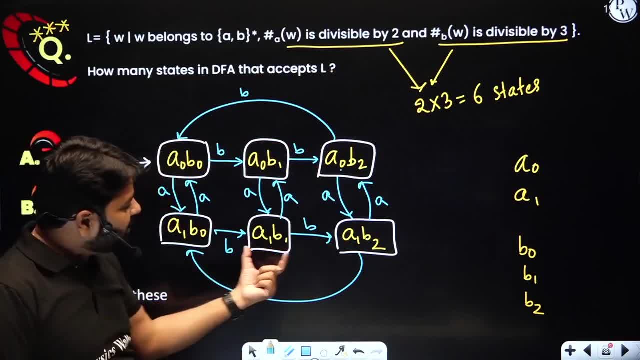 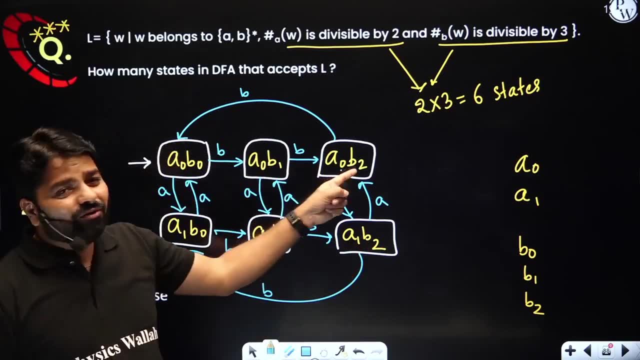 so you should not have 0 this way, especially if you make this two final. in both of them there is no 0. that means both are satisfying, not divisibility. please don't make this. two are these are final? why? because their ac is divisible by 2, is there? 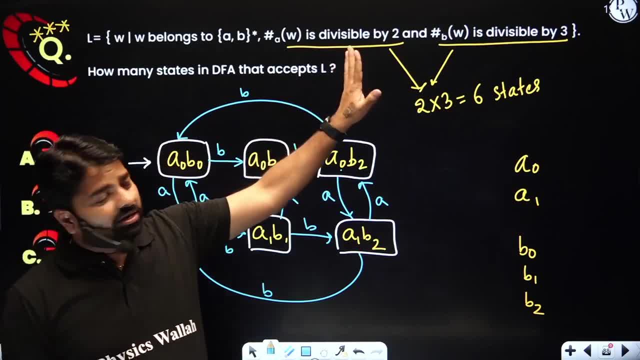 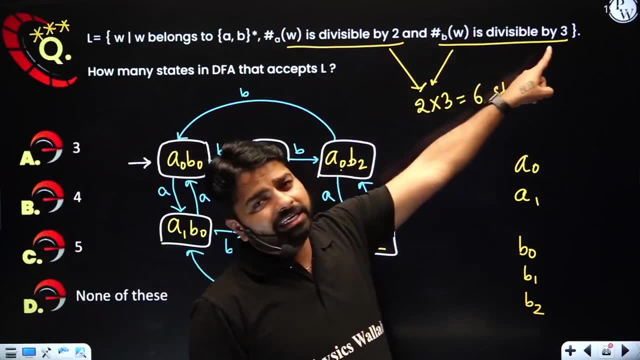 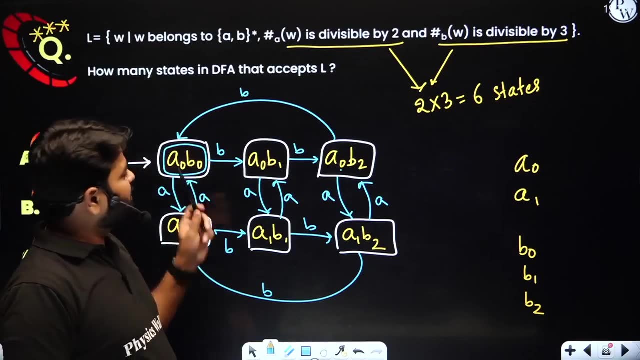 okay, clearly understand what is the question. is here too many combinations? are there so many? okay, according to the question, both should be satisfying divisibility, so both should have the remainder zero. so we will make this as the final. okay, we will make this as the final, in case if 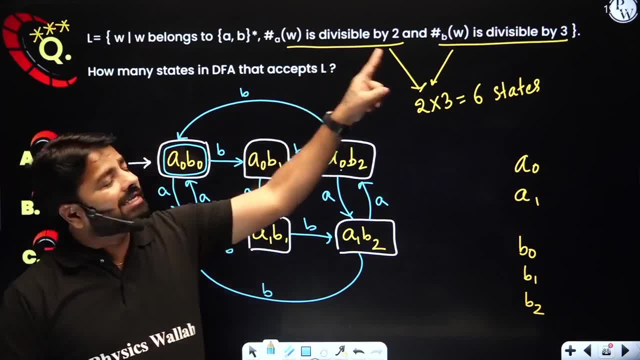 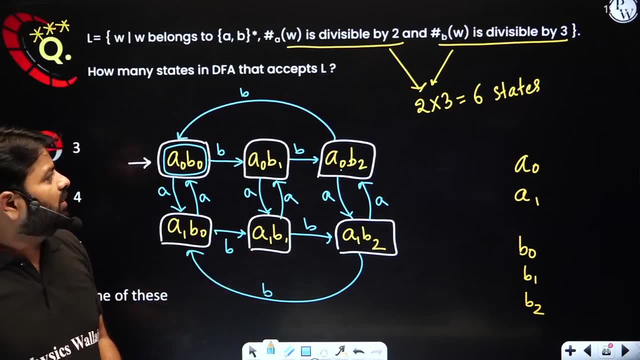 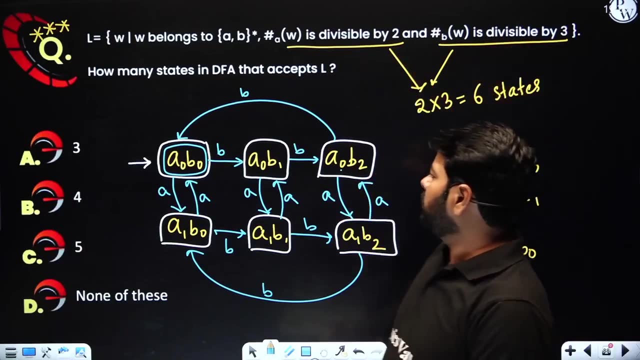 you are making this. two are final. that means both of them are satisfying, not divisibility. okay, so understand the concept to make the final states. i hope this problem will help you in number of problems which are depending on these two conditions. okay, answer is odd: two into three. 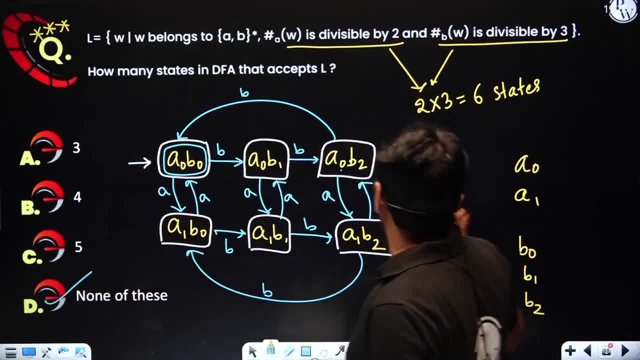 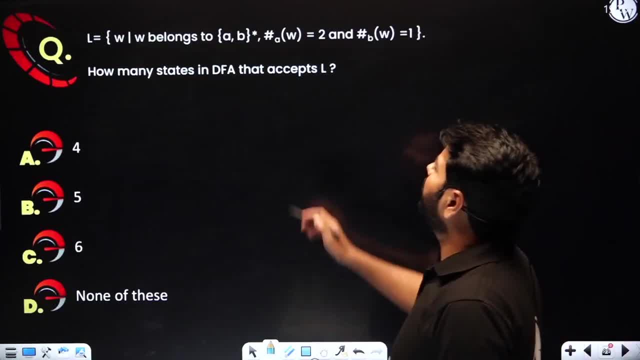 six and there is no option here, so we'll go to none of this. answer will be six states. okay, i hope you can answer it. number of a's is exactly two. number of b's is exactly one. so then, what is the language? okay, i hope you can answer it. number of a's is exactly two. number of b's is exactly one. 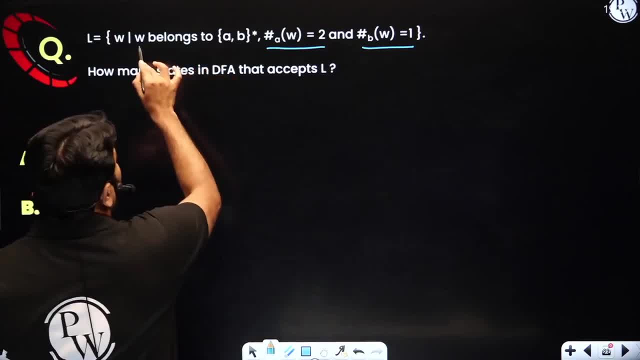 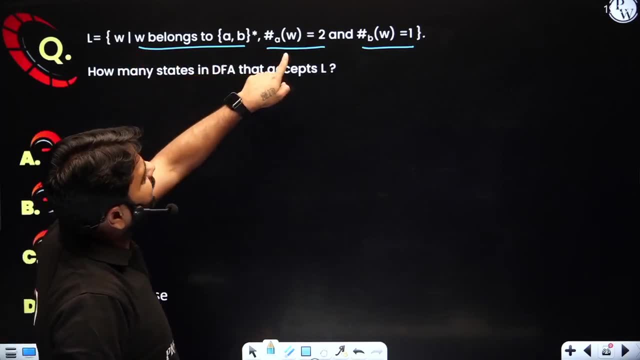 okay, i hope you can answer it. number of a's is exactly two. number of b's is exactly one. it's not a star b star. again, you need to look at each and every con, every condition. clearly w is having any combination over a's and b's, but a's is exactly two, b's is exactly one. what does? 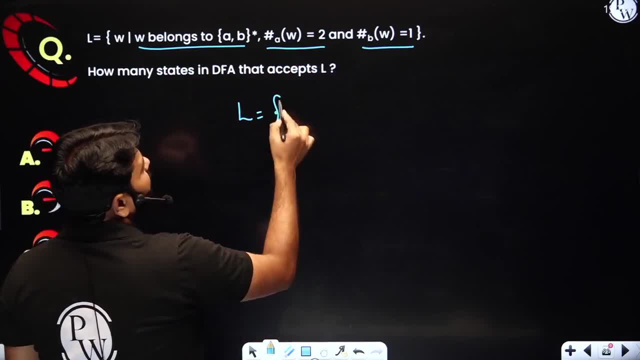 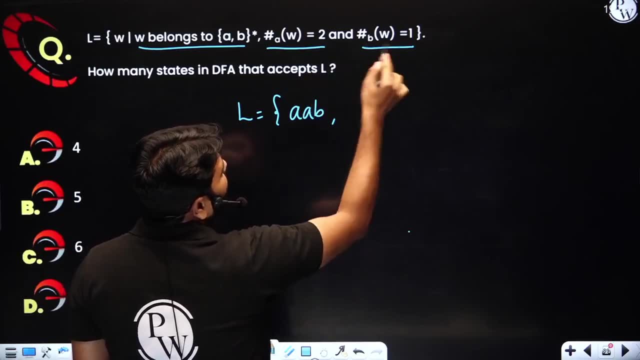 this means the language is having, you know, many possibilities like a a, b, two a's, two a's, one b, two a's, one b. it could be a b, a, or it could be b double a or anything else that i'm missing. just check it. so one b. 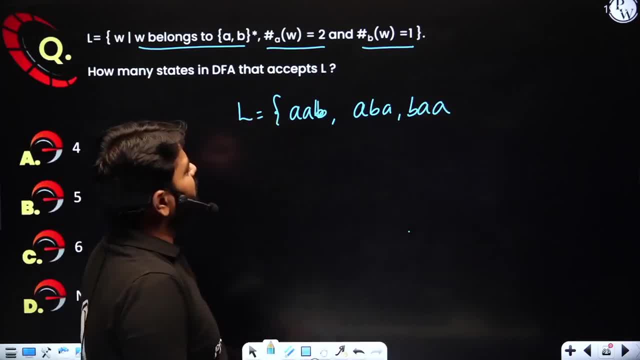 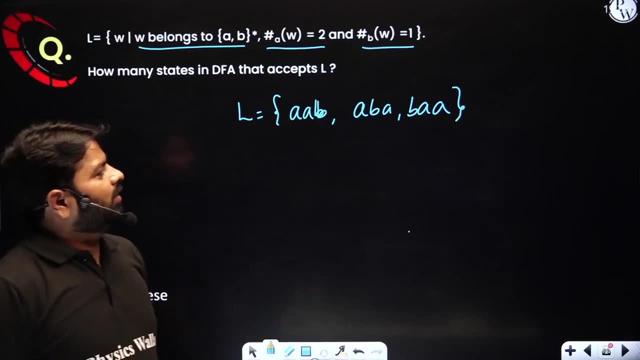 two a's. any order could be there. of course, it's final language now. can you try you out? i'll give some time or pause this video and please try to solve this question here in the string. the order is not important: a after a b may come or after b, a may. 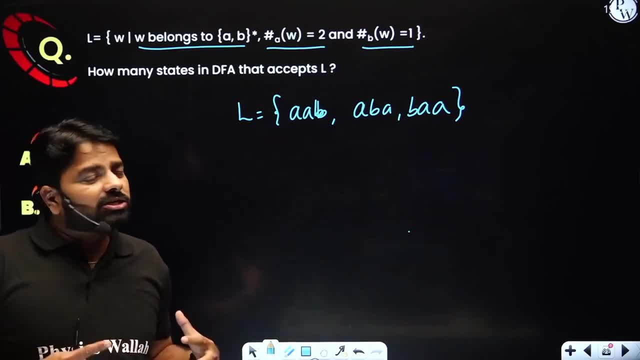 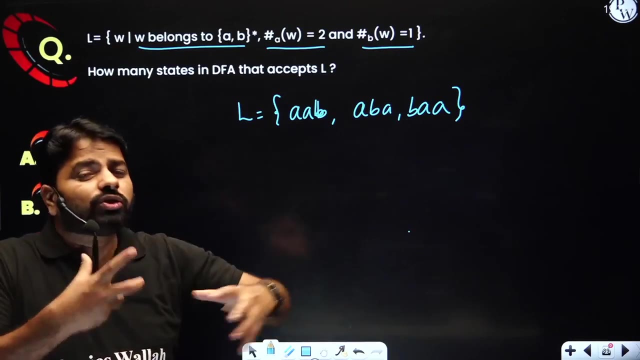 come. but counting is important. so from the beginning, initial state your focus is on when i get two a's and third year i should go to dead state. when i get one b, it's fine. when i get the second b, i should go to dead state because second b never comes. so this count you should remember. 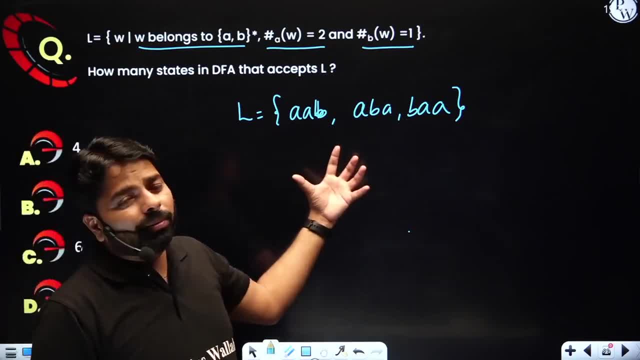 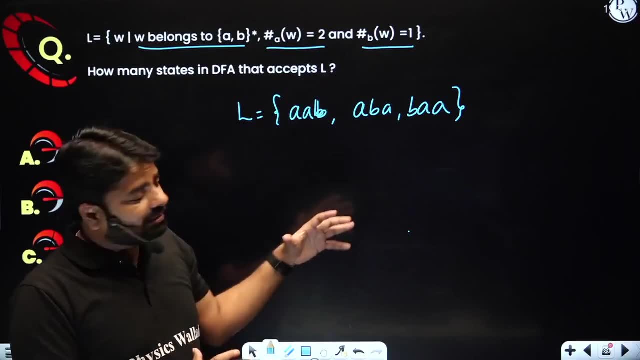 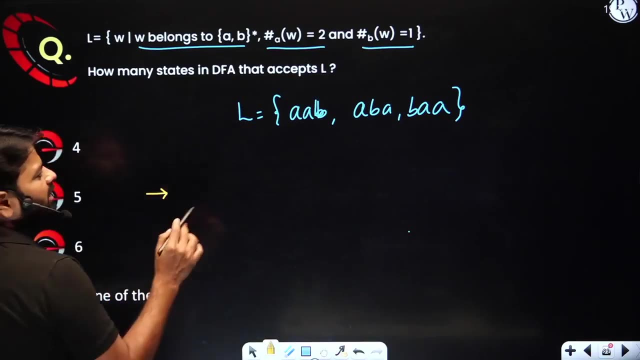 right, you need to keep track of the count: how many a's and how many b's. let's start with the count. any problem that i take in this pattern. you just remember how i follow in designing dfe. the counting is very important initially. what is the count? count is, i may write you know. 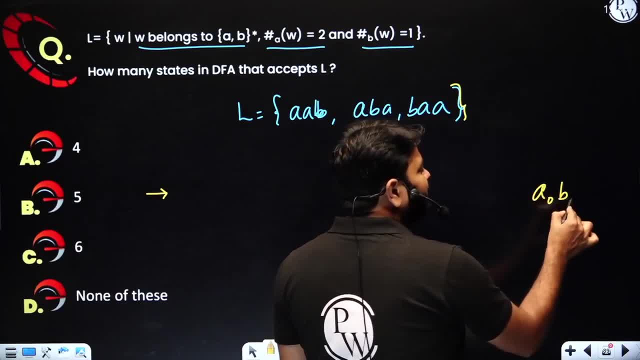 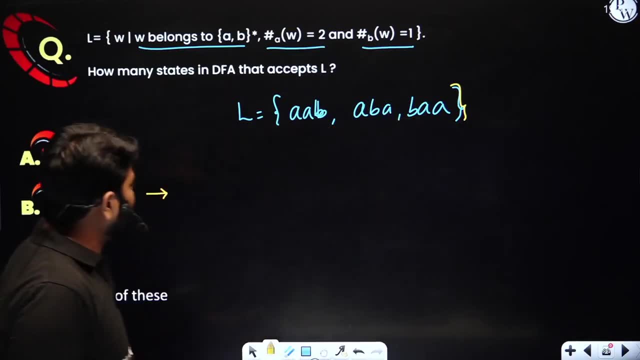 a0- b0. it doesn't mean that after a b comes, it it is. it could be same as even b0- a0, because your order doesn't matter right, count only important. so please note down that i'm writing here a0- b0. it also means b0- a0. okay, remember that point. accepted or not? no, when it will be accepting? 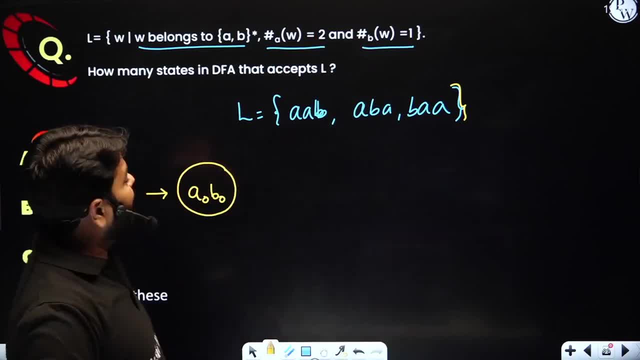 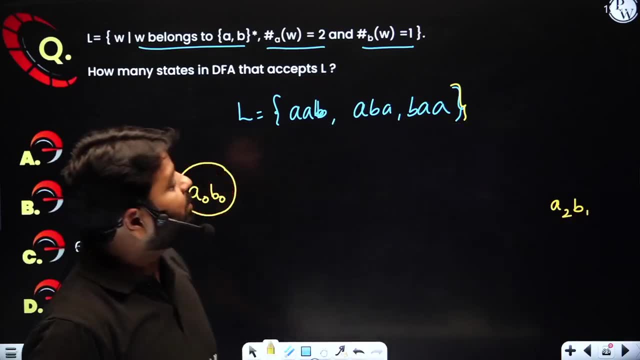 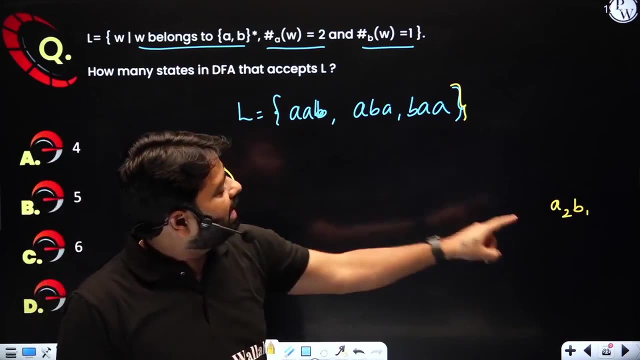 two a's, one b. so that is your target. a to b1 is your target. what is it? a to b1 is your target after two a's and b1. okay, i'm not writing power, i'm writing. subscript means order doesn't matter. remember that way. in all of them we have a to b1. 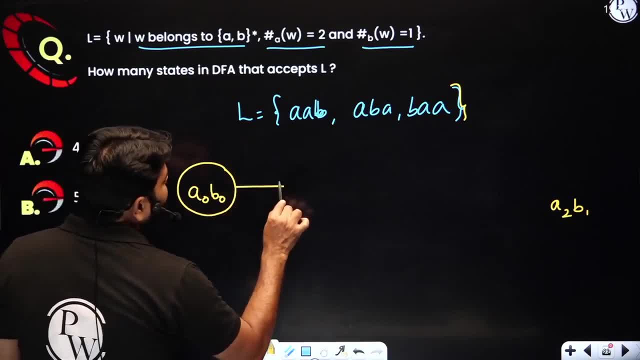 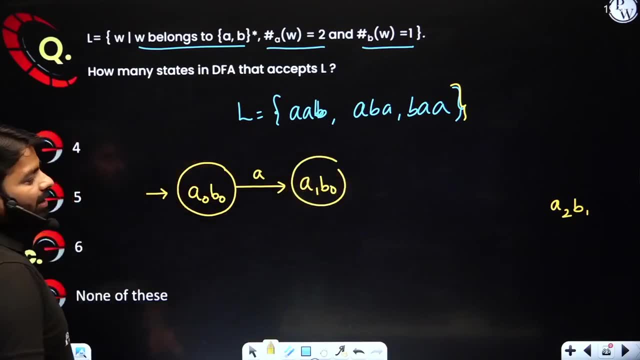 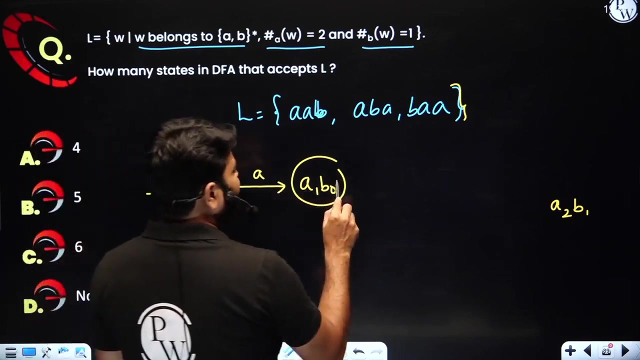 now, if a comes here, what is the count changing? a1, b0, keep track of it. okay. whenever crosses your count, go to dead state. whenever you reach the count, go to final state. and when you get a, b from here, a0, b1- okay, now, from here, if a comes, that's going to be a to b0. 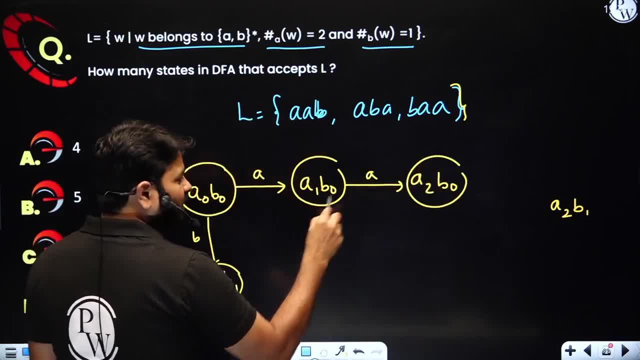 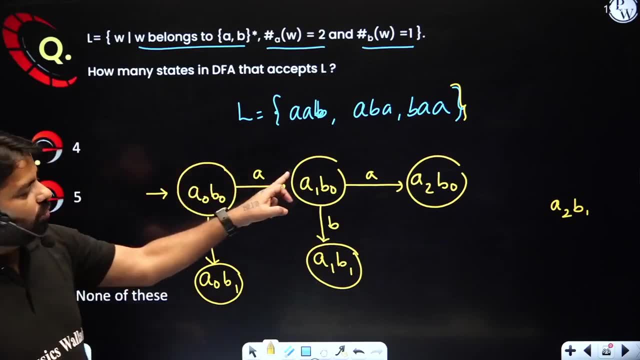 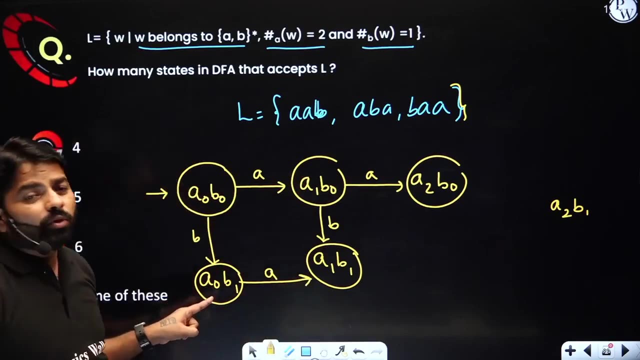 if a comes or a is over, if b comes, here that's a1, b1 and one, two. both are covered. and third one from here a comes, a1, b1 already there. so go there. very simple. but here one more b comes. already one b is. 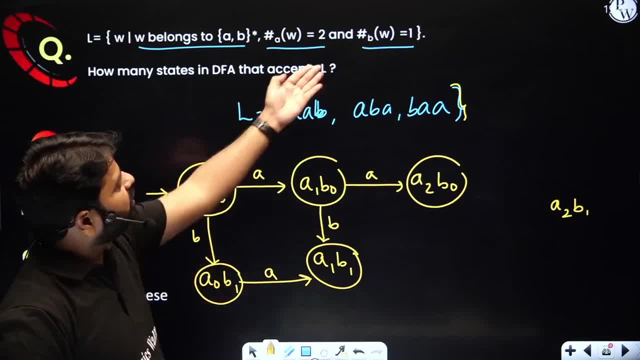 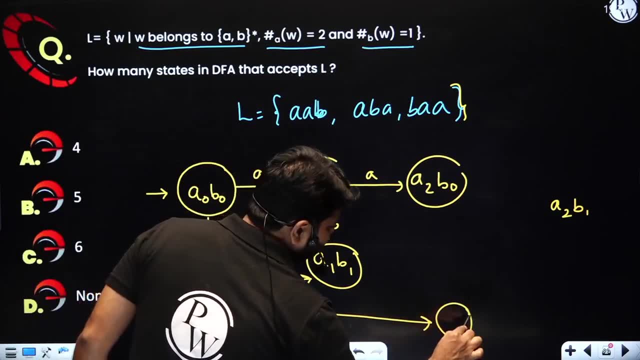 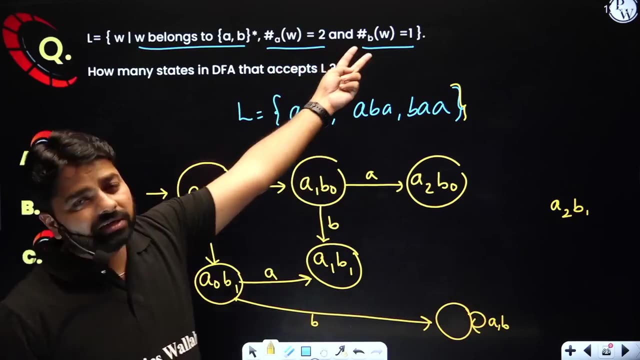 taken now a0, b2, we don't have a two bees possibility, so we'll go to dead state. i'm just taking a dead state here, dead state. it's crossing our limit. our condition is failing because of two b's are coming right after this. b doesn't matter, is a b's, we don't count. 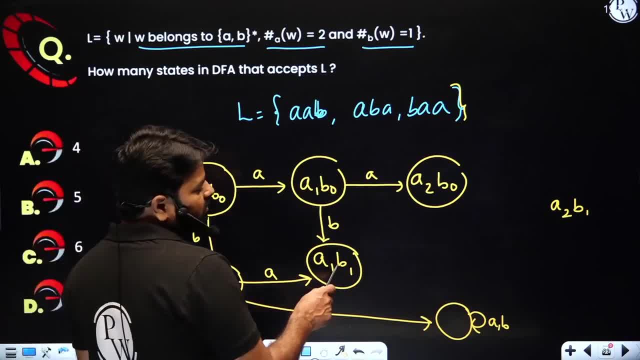 now from this a and b covered. now from this one more a comes, it will be a to b1. so that is our target, right? so i can't do that, so i'm going to go back and i'm going to go back and i'm going to. 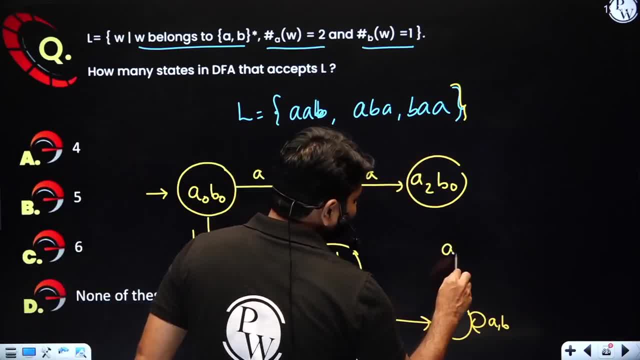 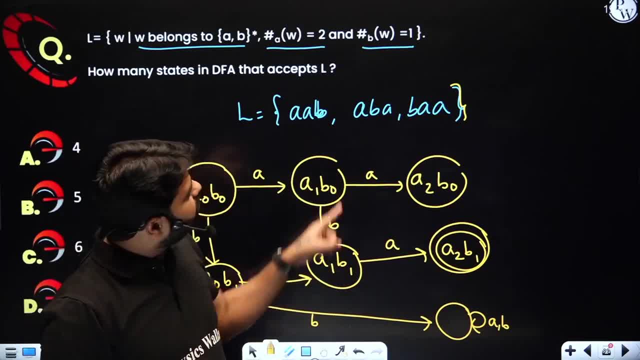 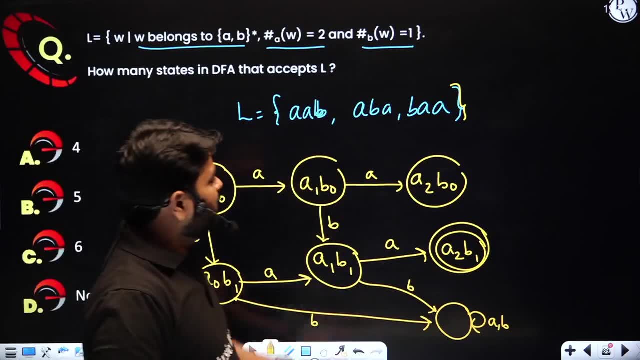 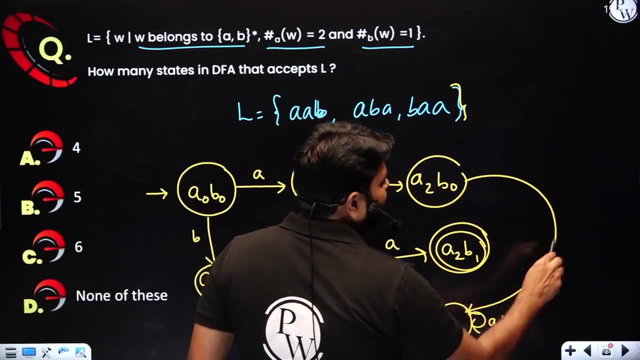 but one more b comes here, the a1, b2, oh, b2, impossible. so we go to dead state. so that counting is important. counting is important. so from this third a, is it possible? impossible. so already a2 is there. if one more a comes, we are crossing the number of a's. 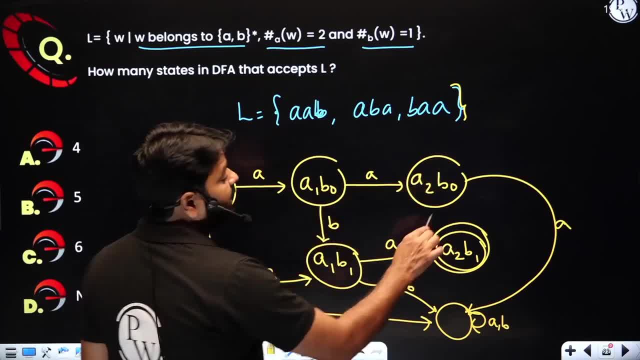 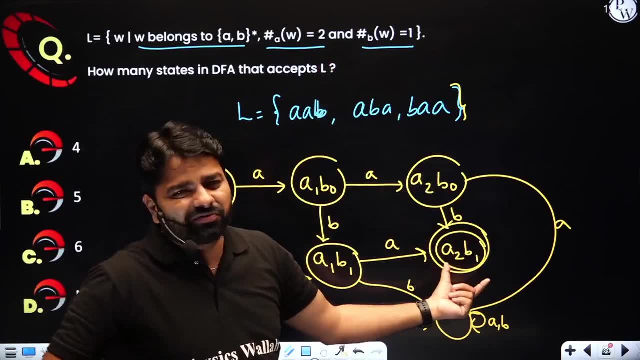 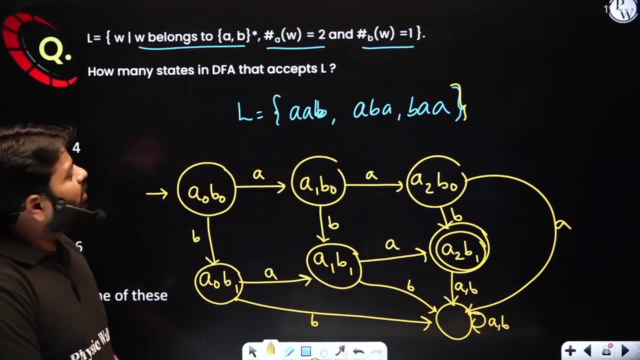 from here b comes a to b0, become b1. oh, that's a valid string. now from a to b1. already the maximum right two a's, b1's. from this a or b you are, will be crossing the limit. now see how easy if you can keep track of counting. 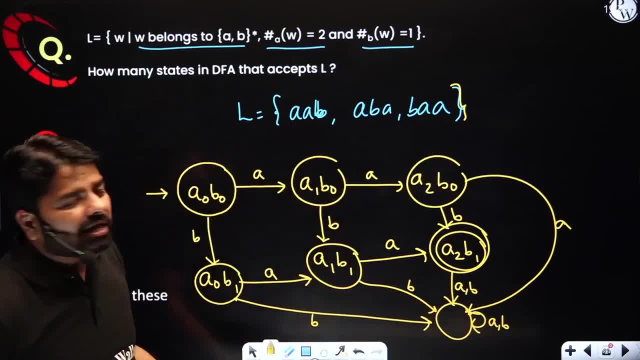 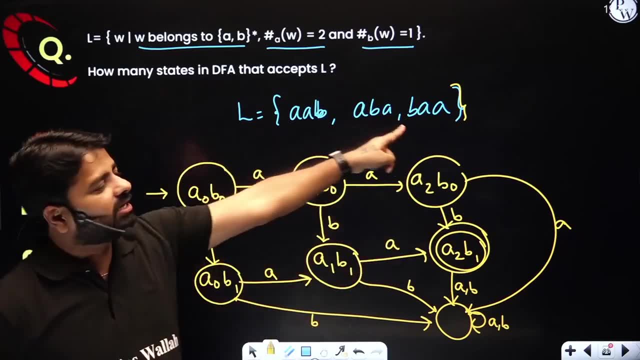 now you may ask, sir, how these three strings are accepted. look at the paths to reach this final one path. second path, third path, that's all three paths are there to accept these three strings. you can check a, b, so where is that a, a, b, a, b a. see that a, b, a. 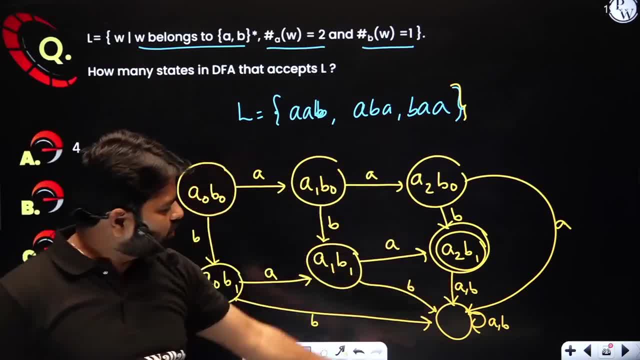 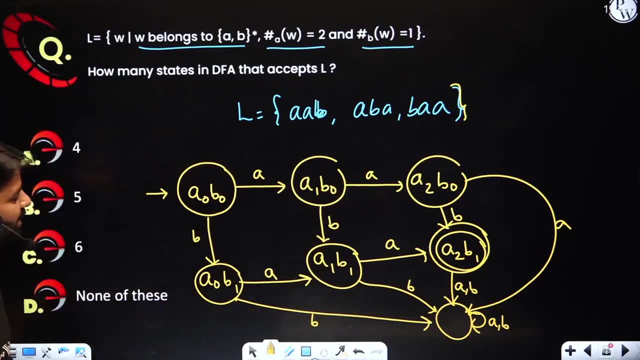 see this: b double a, b double a, that's all. any other string will go to dead state. any other string will go to dead state or will halt it, not final, somewhere. okay, so how many straights are there? one, two, three, four, five, six, seven. so here seven. answer, not there, so we'll. 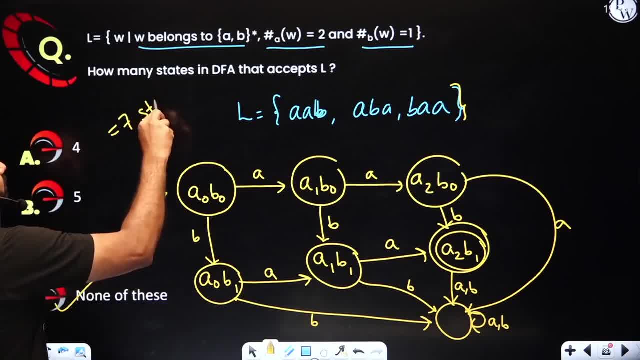 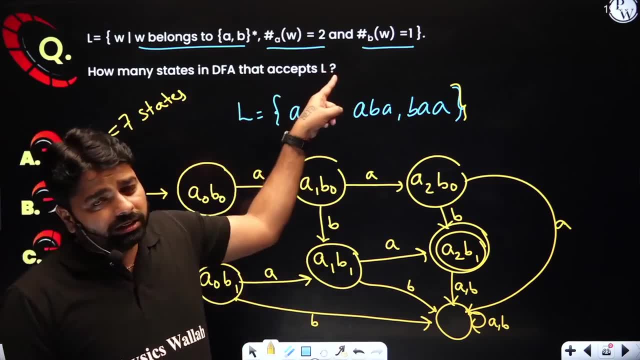 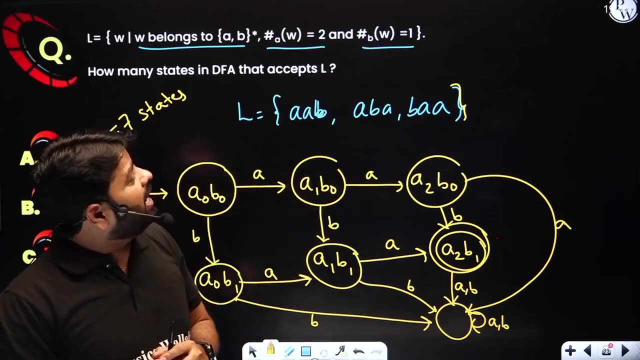 go to none of this. so seven states required for this problem. so i hope similarly you may solve the questions which are depending on this. but here i have said exactly two, exactly one b, right, exactly exactly one b. in case, if you have at least one b, then after one b the second b should not go dead. you. 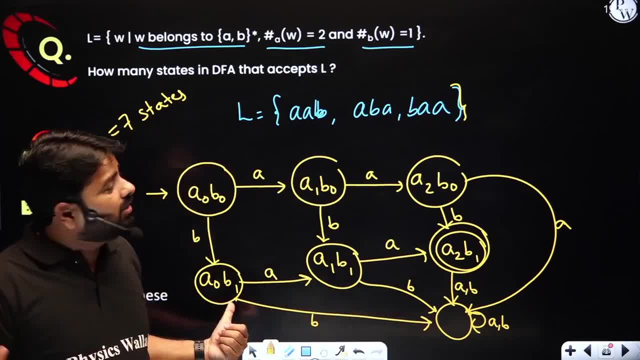 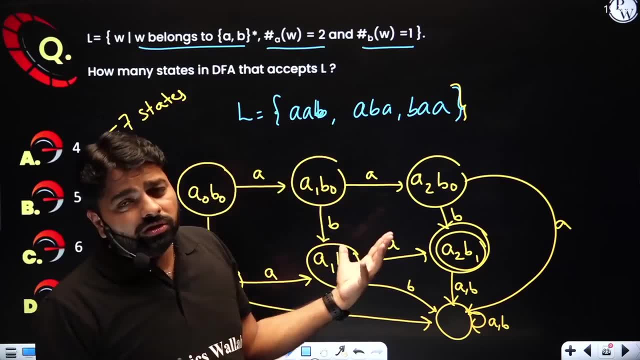 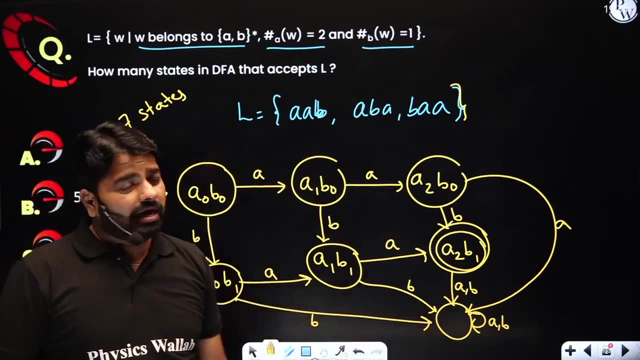 should put a cell flow because, second, we thought before we find right. so when you have at least condition, put a cell flip. once you satisfy the minimum condition, when you have at most, then let's say at most one b, then zero b is fine, one b is fine, then two b, you go to red, okay, and 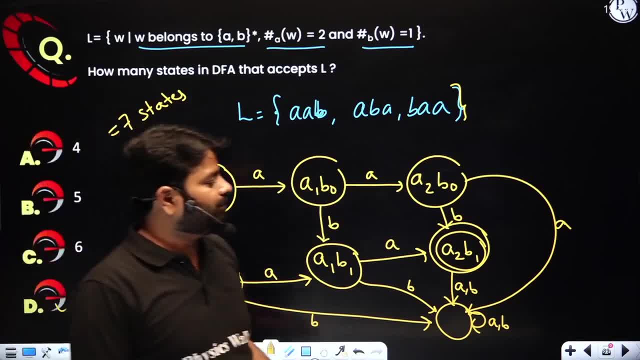 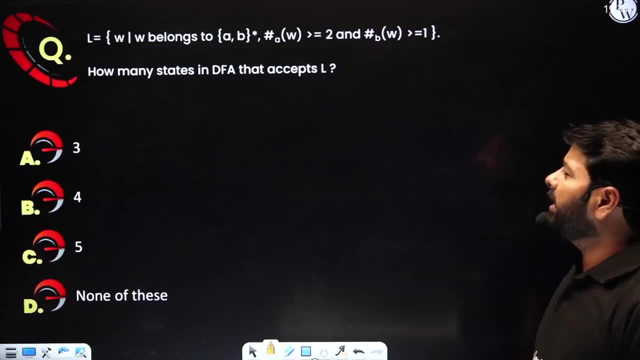 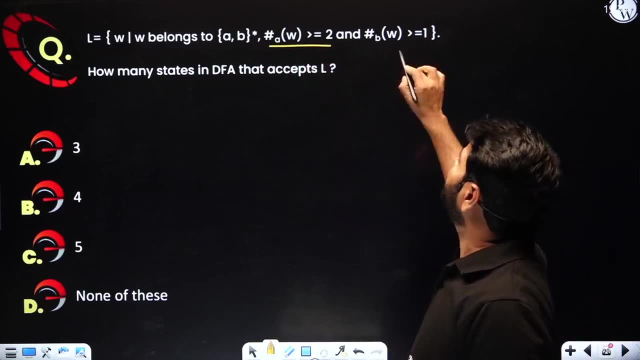 understand the problem and design it appropriately. again, i'm uh giving this homework. i think i should solve this. that next one: you take it as a work, if you have any. this number of a's is greater than or equal to, means at least two a's. this is at least one b. so now, here you don't have dead state why. 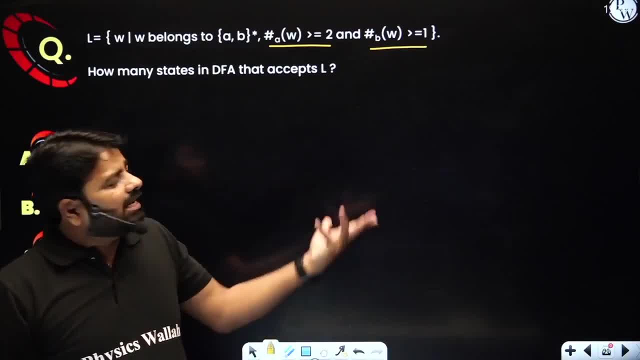 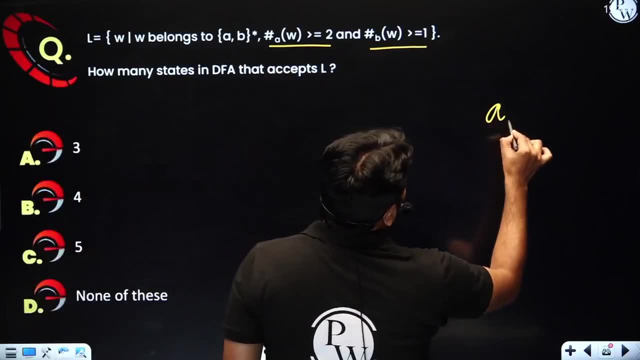 at least is fine, right, it's not at most or exactly in the at least condition. you will go till that condition and then put a cell flow. now keep on counting this one you need to have, you need to reach this one: a greater than or equal to b greater than or equal one. but once you 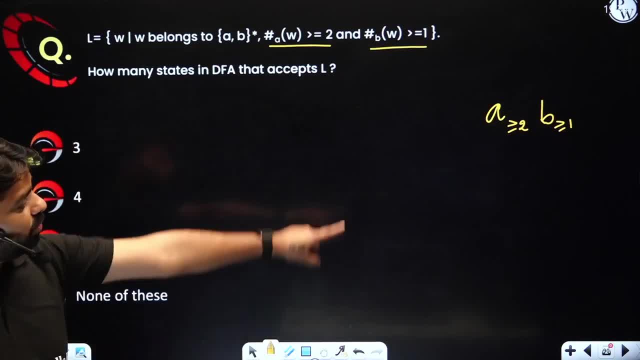 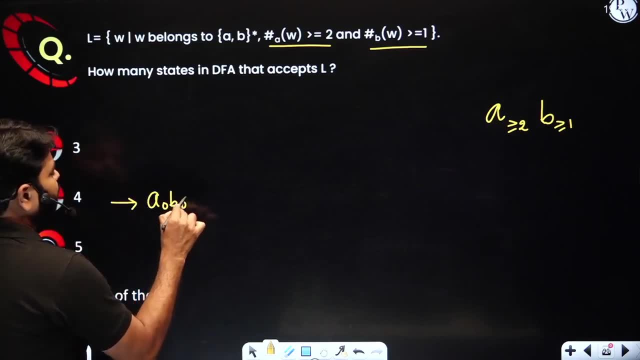 reach the state, stay there. everything is accepted. but to reach that it will take much time. let's do that. initially, a 0 b 0. if 1 a comes, that's a 1 b 0. if 1 b comes, a 0, b- 1. keep doing that. 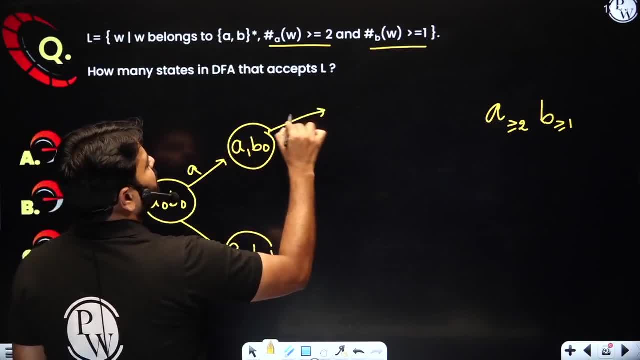 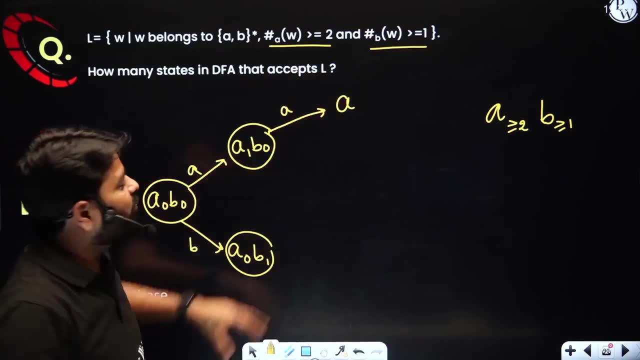 and from here one more a comes, then a 2. whenever you reach a 2, put greater than or equal to, because from there any number of a's put cell flow, so even the two a's. i know it is equal to two, but i don't put. 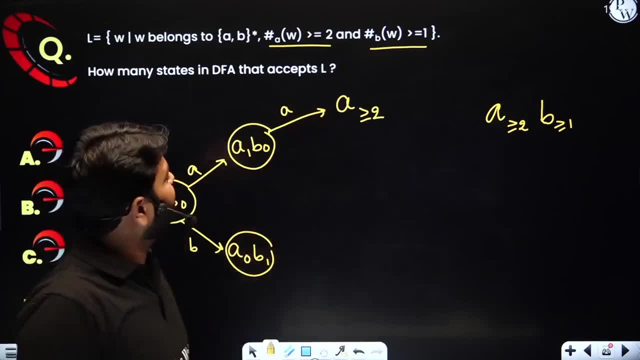 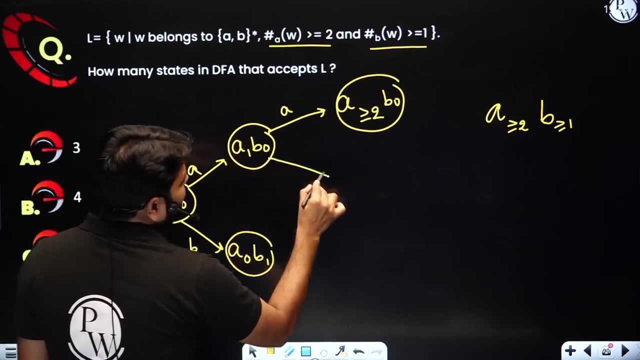 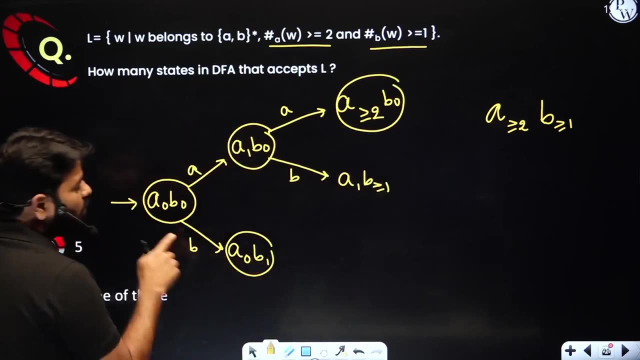 because third, a, fourth, a, i will stay here only and b 0 i will maintain. if b comes here, a 1, b 1 not there anywhere, so i have to maintain b 1. 1 means what greater than or equal to 1, so here also, when there is a 1, b put greater than or equal to 1. 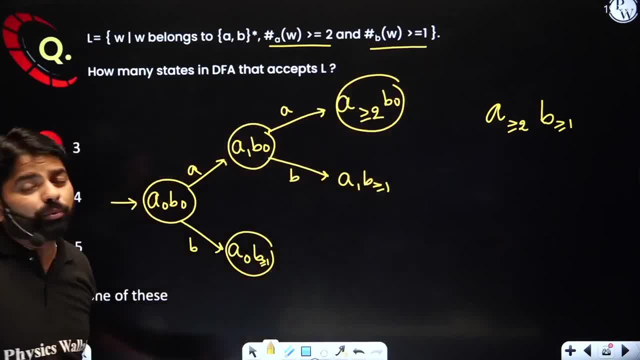 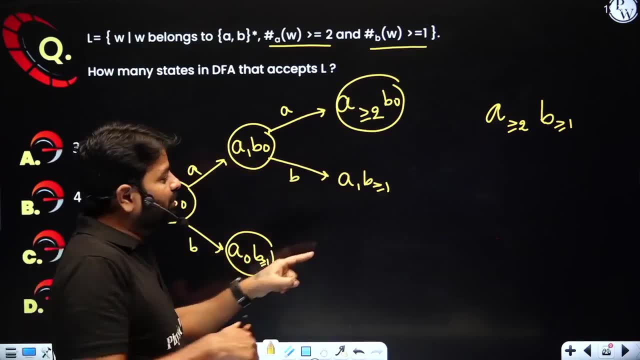 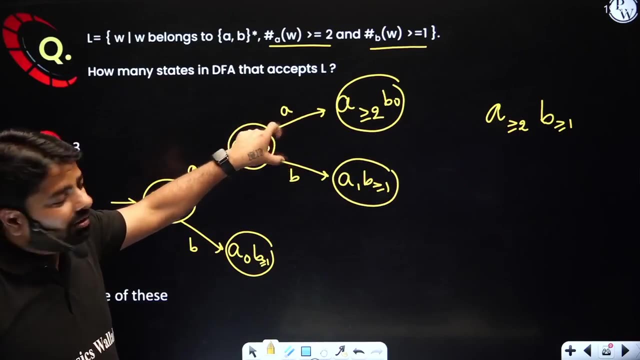 because we satisfied the minimum condition. so it's one of the important key factor: when you satisfy the minimum, put that greater than or equal, because there you can put a self loop for the b's, here you can put the self loop for the b's later now. this state covered a and b. this state covered a and b. 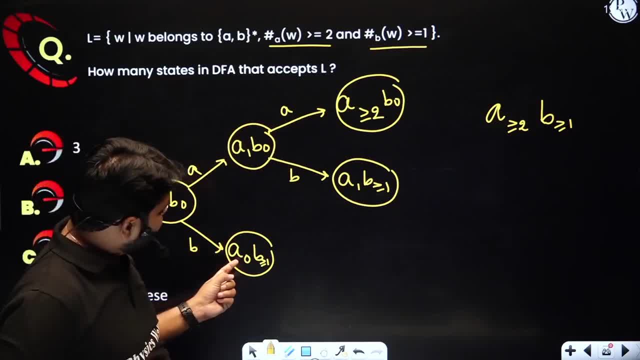 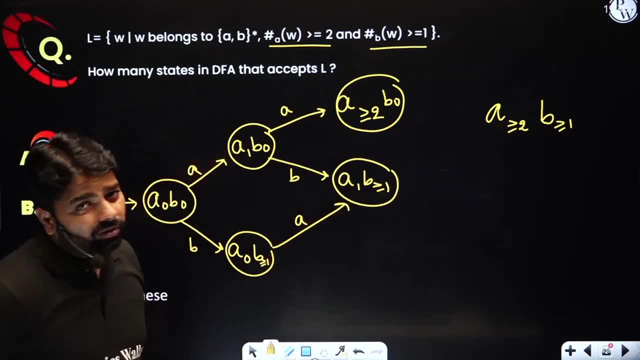 and i'm covering this state now, a and b. first, when you have a here, a 1 b greater than or equal 1, you have here. right, you can go there. see that how easy. if you don't have your design now, when you get a b, what do you do? this is what i'm talking about. 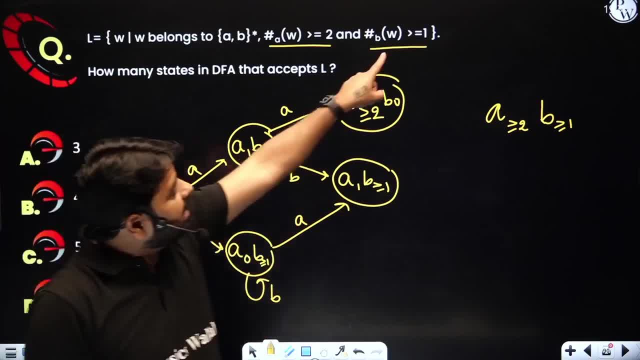 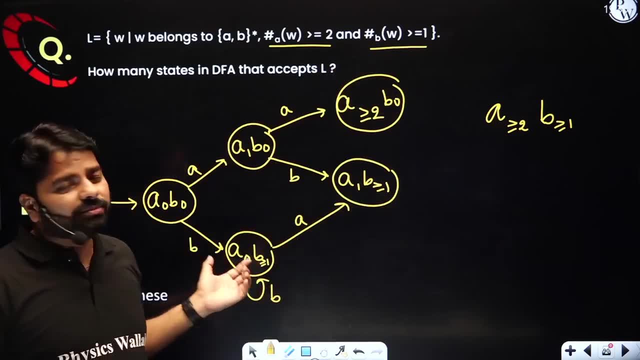 you b, put a b self loop as you don't need to count more, you satisfy. the minimum number of b is 1. when you have a minimum 1 b, that means greater than or equal to 1 b. so either this b or this b stay in same. 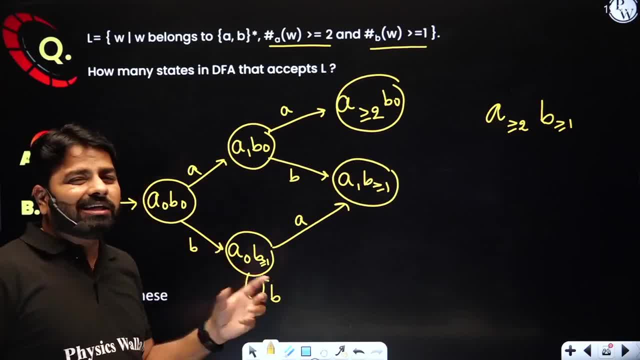 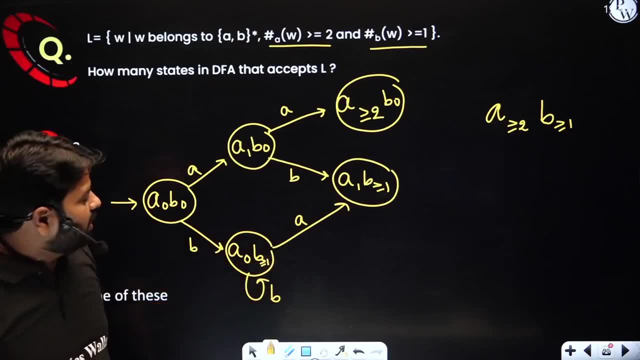 state. that's why equal to 1, greater than 1, i just take one state. i don't need multiple states for that. okay, so that is the advantage of putting greater than or equal 1. and now this state: if you get more, a's already minimum to a satisfied any. 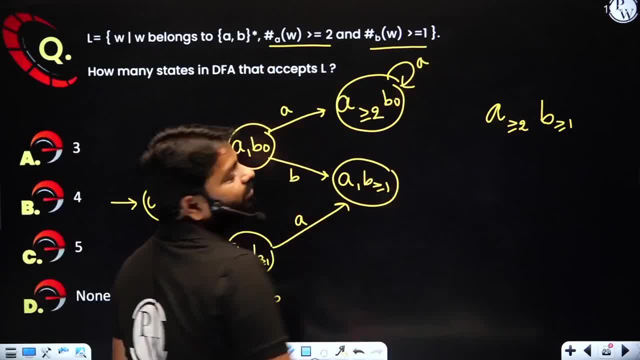 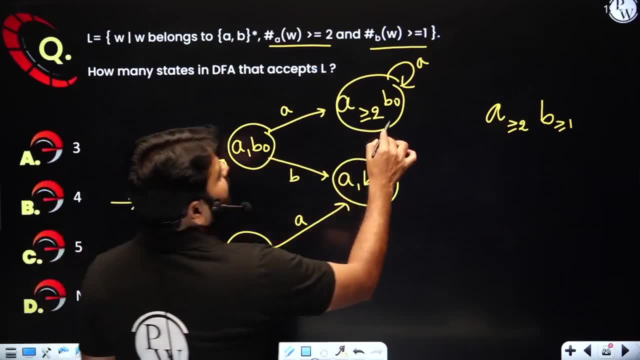 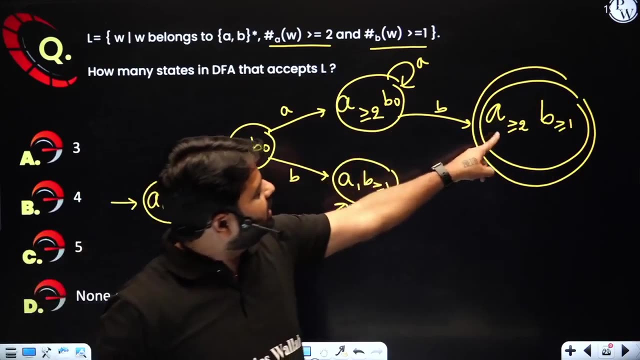 number of a's. just wait there why you are waiting for the b. already a satisfied the condition, the b's you are waiting when you get one more b. that's your string. that's when you get one more b. this is your final state, right? you satisfied already two a's. now you 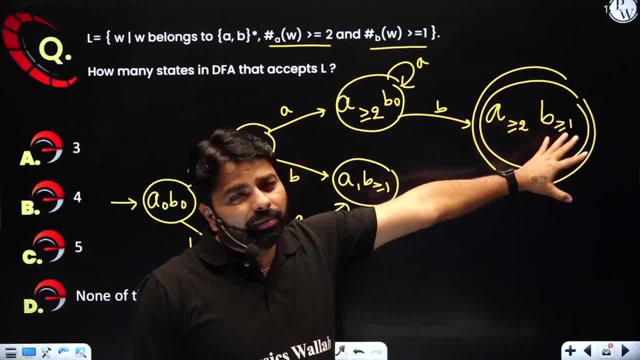 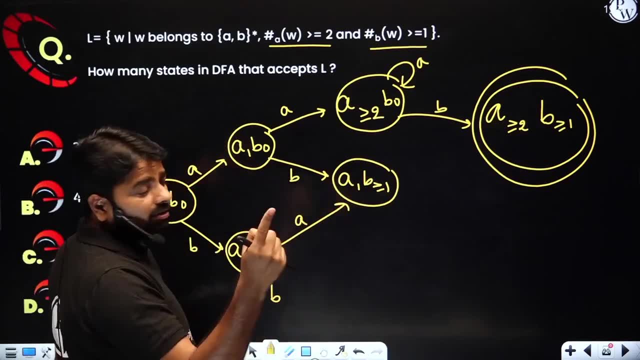 are going to satisfy minimum one b. so minimum one b means greater than or equal one. okay, now this one e a, a 1 become a 2, but 2 means greater than or equal 2. you can go there. satisfied a till now, b, satisfied already. minimum condition a is: 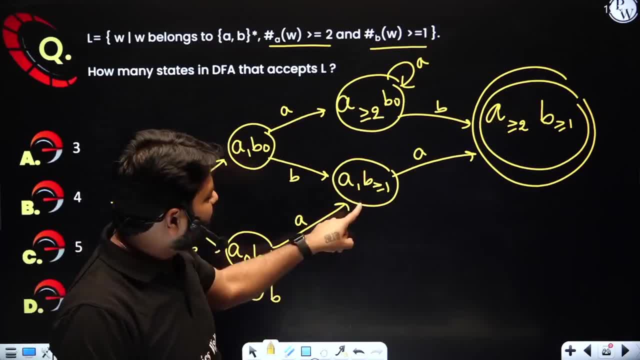 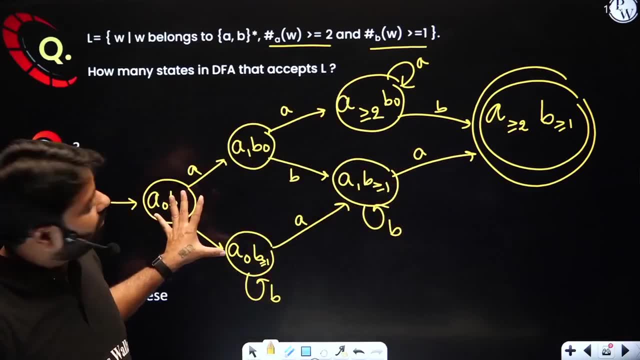 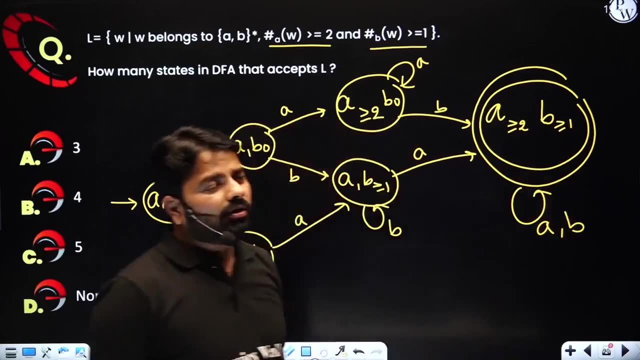 waiting for one more. okay, now b, you can put a self loop because b already satisfied. we are waiting for only a right b self loop. now. all the states are covering, covered for a and b. now this is only left once you satisfied both the minimum, either a or b, doesn't matter, just stay in the self loop. 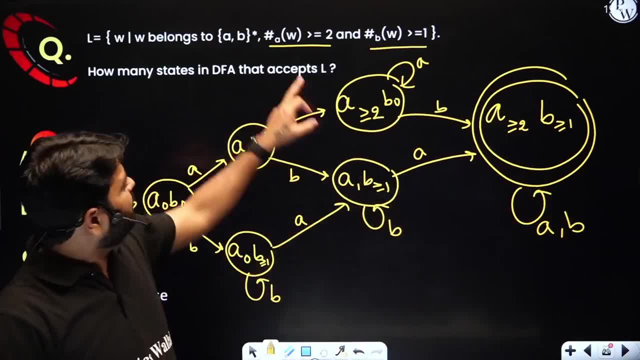 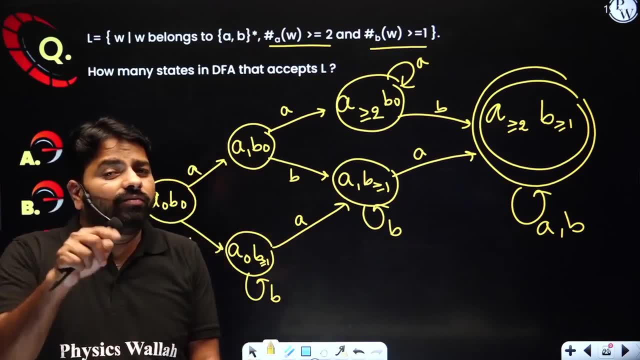 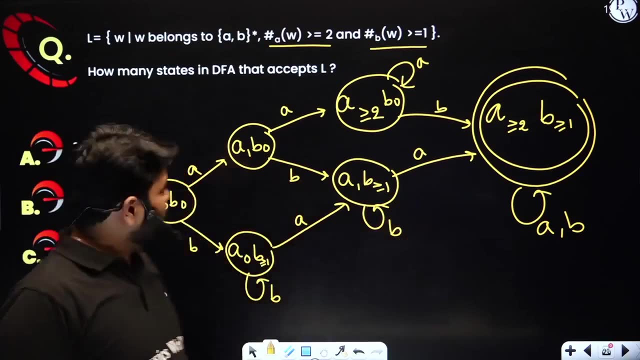 because more than 2 is always accepted. this condition is there. so at least condition do not require that. but when you see exactly or at most, then definitely you will need dead state. i hope you understood this problem. and how many states you have six. so answer will be: none of this again, but here: 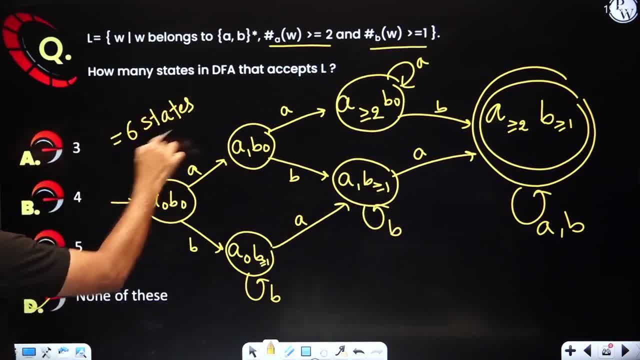 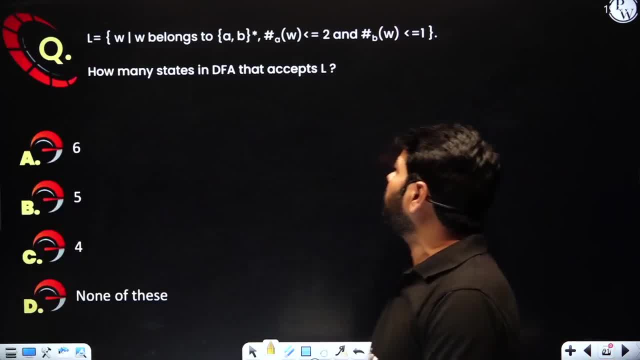 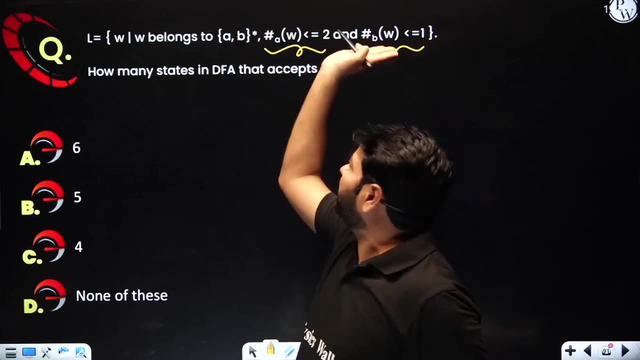 six states is the right answer. the previous one was a seven. there you have a dead state. here you don't have a dead state. okay, anything which is there similar to this, please take it as homework. and yeah, you got it. number of faces: at most two. number of pieces: at most one is almost similar to exactly, to exactly. 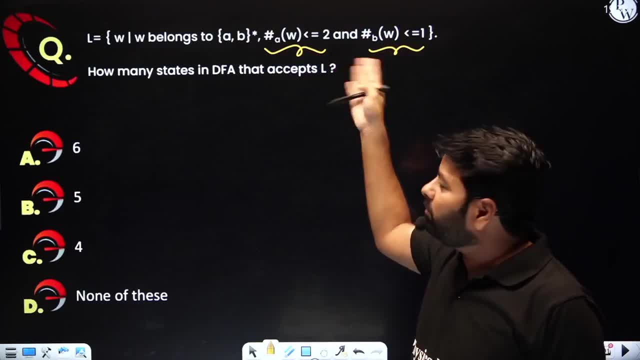 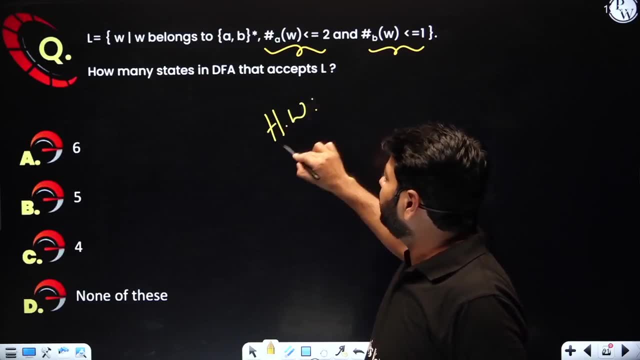 one right, but before this you try to take care of all the combinations which are accepted, so so many finalists might be there here to take care of them. so it is homework. i'm very happy if you can solve and post the answer below this video and let me know how many of you are solving this. 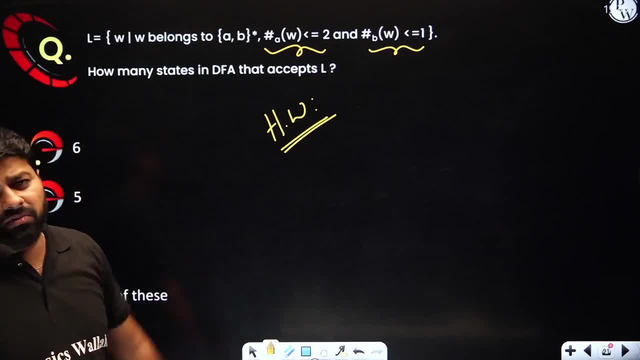 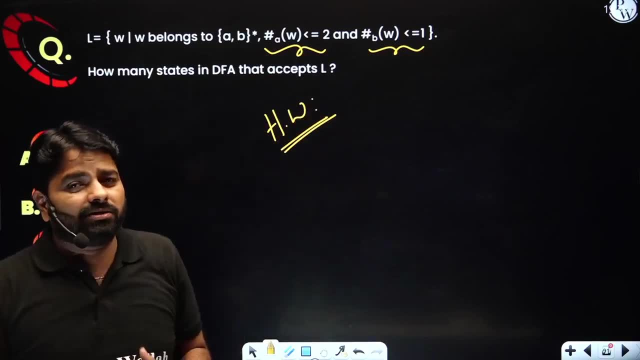 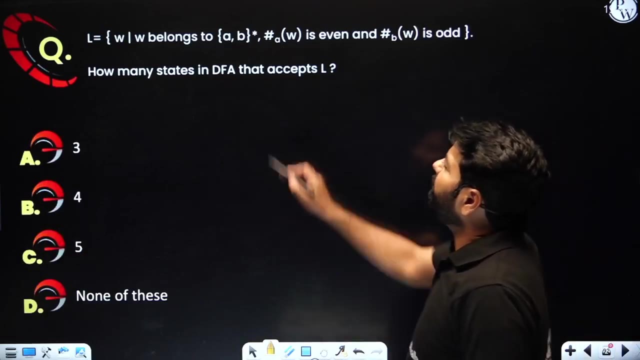 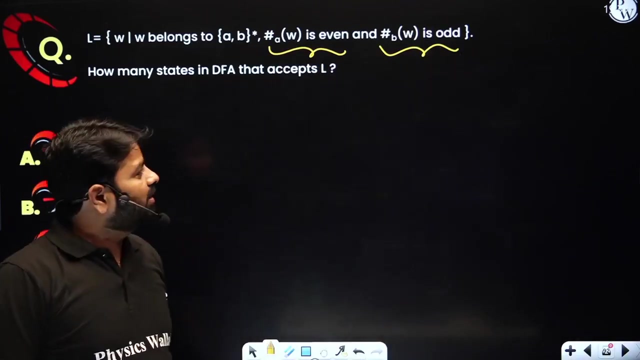 question: okay, the question is clearly: you know almost which is uh, same as the, uh exactly to exactly one only thing is here: you will have many finals, many finals, okay, okay, number of a's is even and number of base is odd. tell me, we have solved this question already. 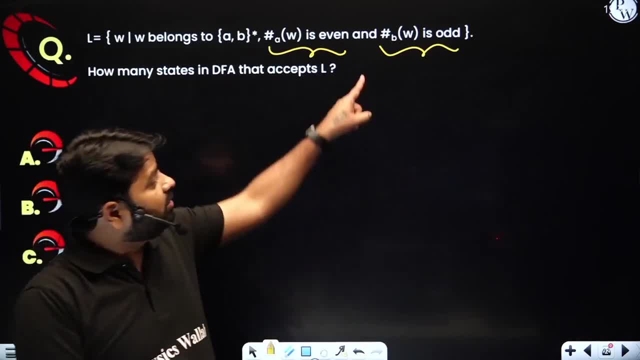 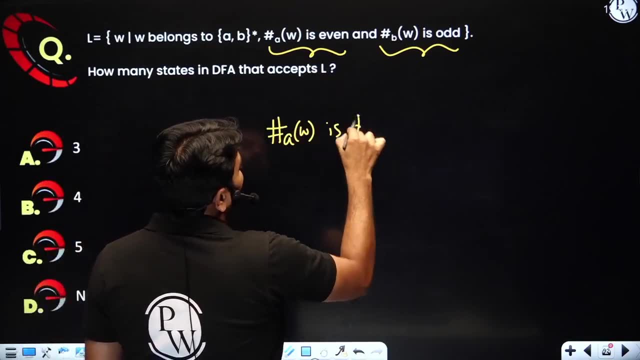 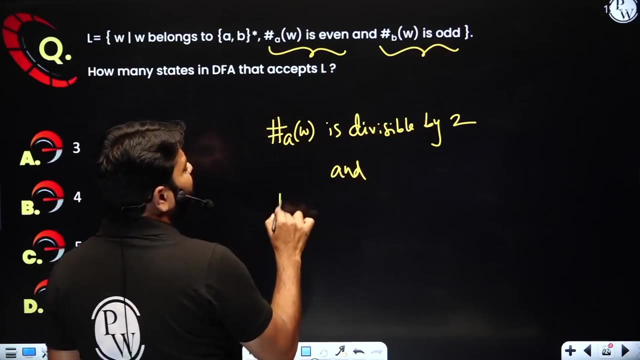 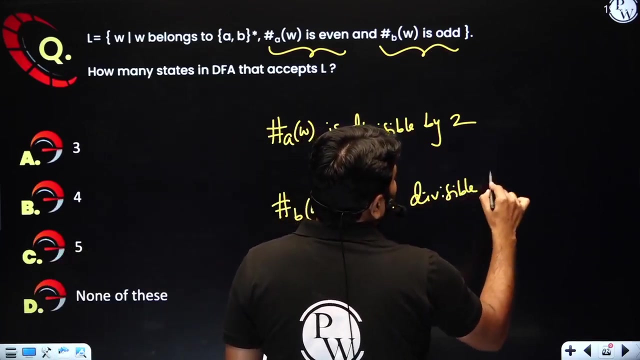 have you remembered that already? what we have solved, which is similar to this, did you remember? even means what number of a's is divisible by two, yes or no? and this one number of b's is odd means is not divisible by two. okay, the question is simple: whether it is divisible by two. 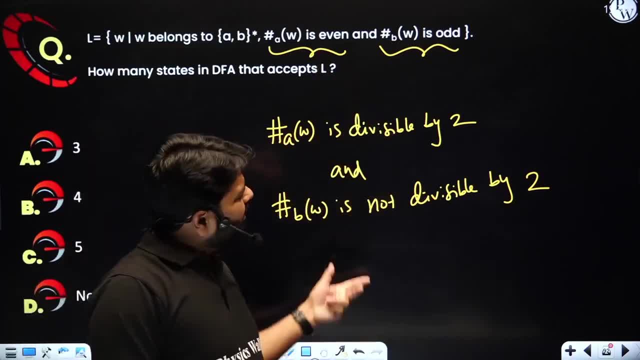 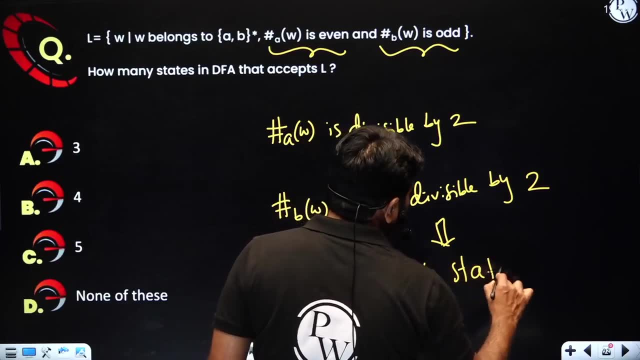 a is divisible by two. b is divisible by three. two into three, six here, not divisible by two. still answer same. two multiply with two will become four states. in case if you want to answer very quickly in the exam, answer will be four states. but if you want to design you, 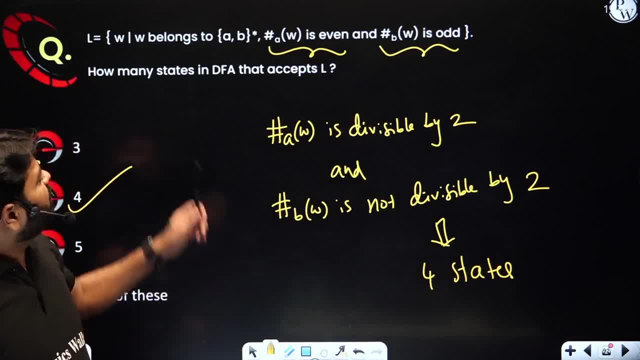 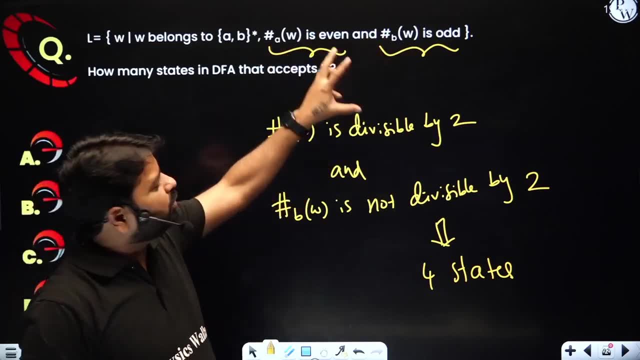 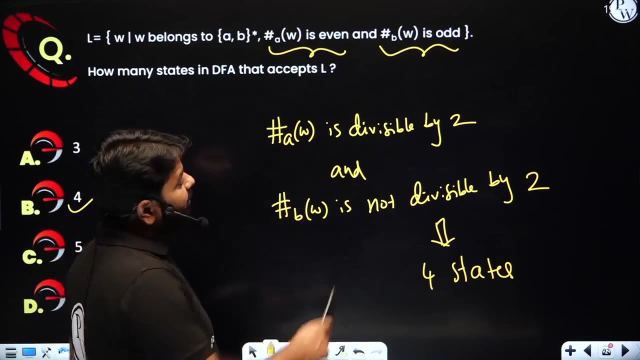 should understand the property or behavior. so let's start designing the machine. okay, in the exam. very simple: if you know the concept or this composition trick, you can apply it. if not, you have to design the machine. okay, which which was solved already. like there you seen, a is divisible by two, b is 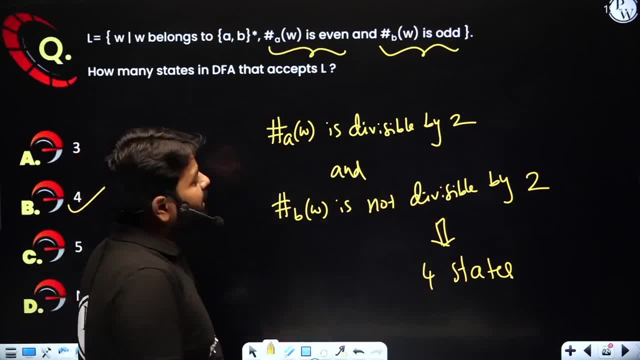 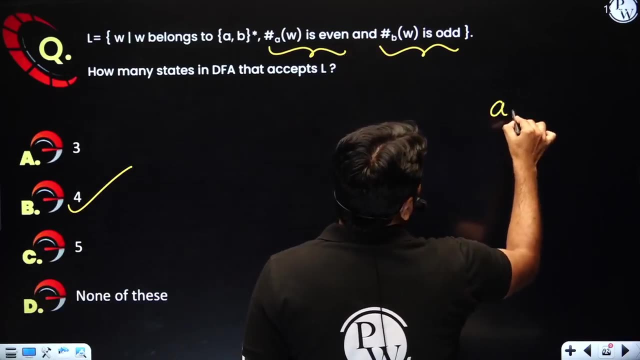 divisible by three. so two multiply with three is six. but here both are concept, both concepts are, are both symbols, depending on divisible by two. so we did do two into two is four. okay, now how to design other way. so this is the first. one other way, so h is even. so we have two reminders: a0, a1. 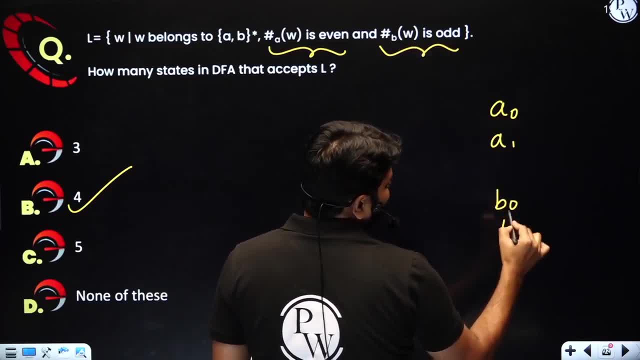 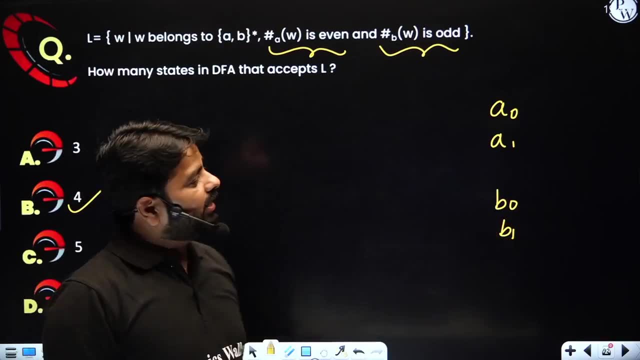 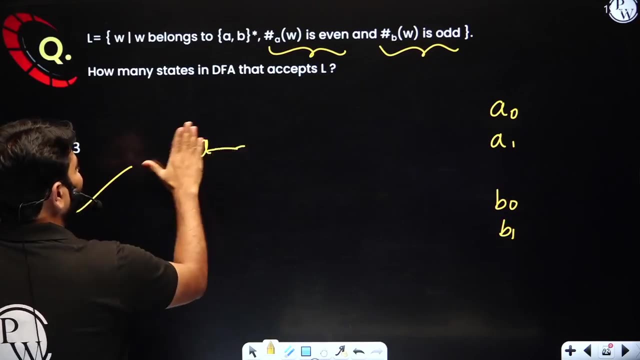 bc is odd. again two remainders, b0, b1. but it is even or order. you will have two remainders. that's why two multiply with two will become four. right now, combinations: a0, a1. sorry, a0, b0. two different symbols. right, you need track both. 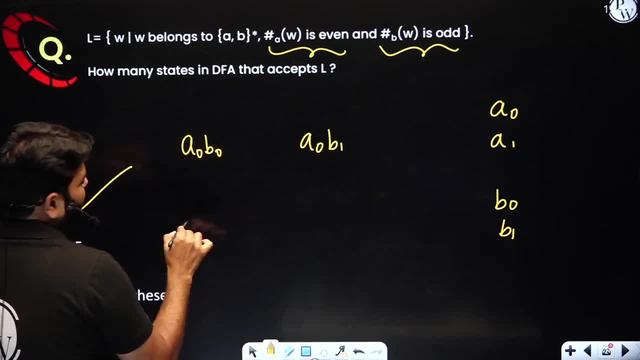 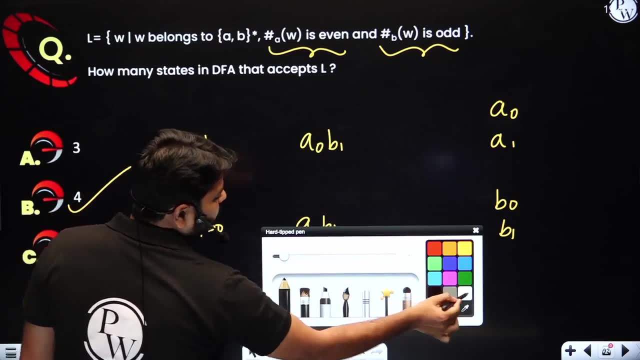 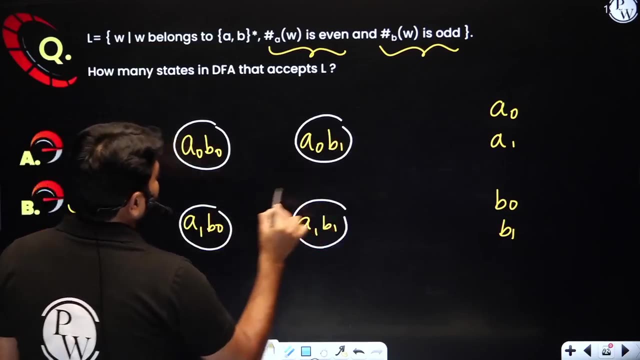 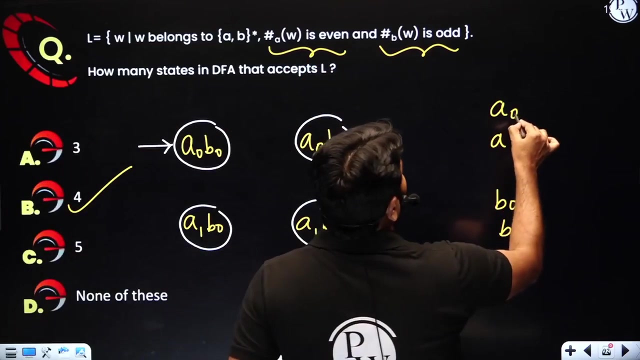 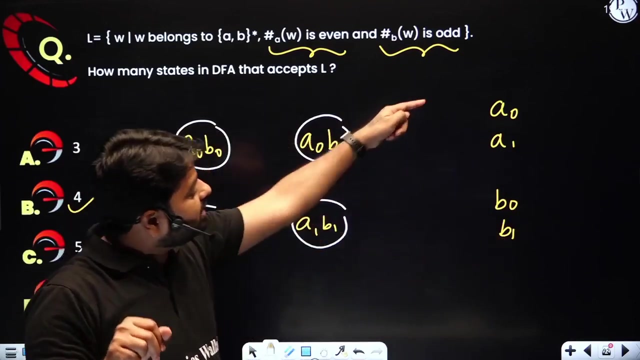 a0, b1 and a1- b1. who is initial state: a naught, b naught. so now the question is: A is even means you need to accept you need to have zero remainder. B is odd, so b should have one reminder: A0, b1 is even, his is even so. this would replace b0- b1. 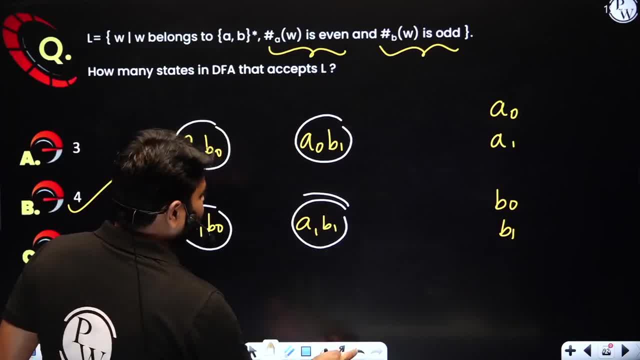 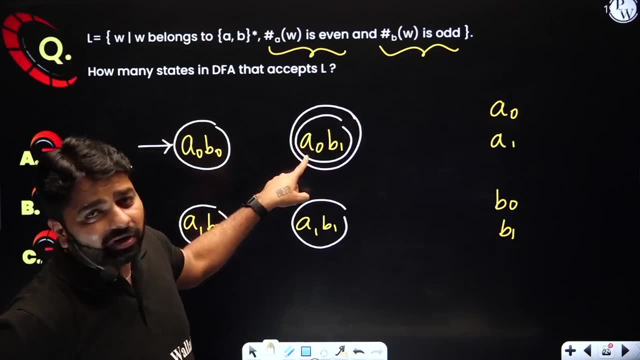 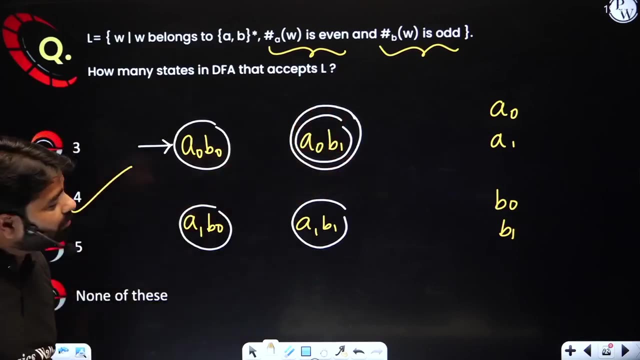 one. this will become final. sorry what i am saying. a zero, b one. where is it here? this one will be final. so a's is even then a is multiple of odd divisible by two and b's is odd means b is not divisible by two. so this is the final and very simple designing the machine. and from here whenever. 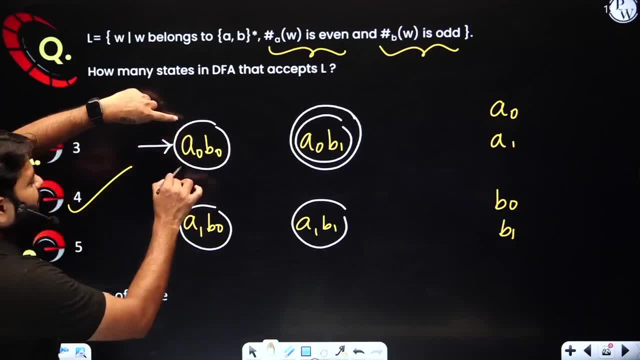 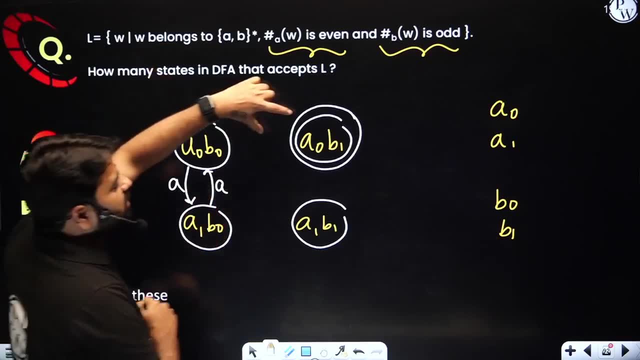 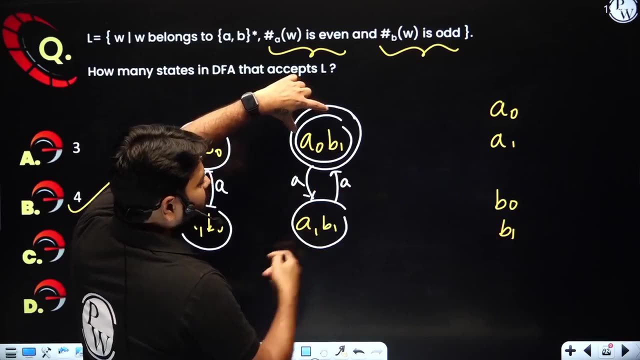 even number of a's comes, you should come back. see here, when one a go there, other a, you come back. that's it from here and here. also same one a you go to a one, but b one will be same. and when you get one more a it will be remainder zero and similarly b b zero will become b one if 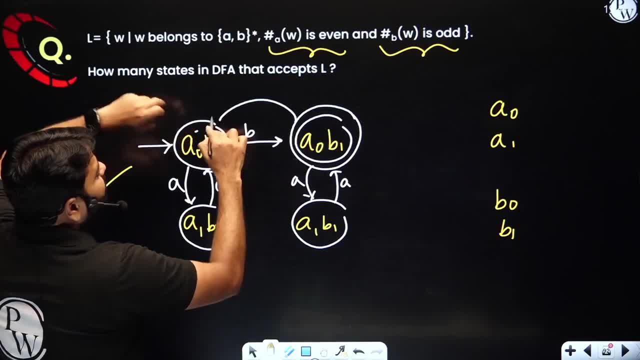 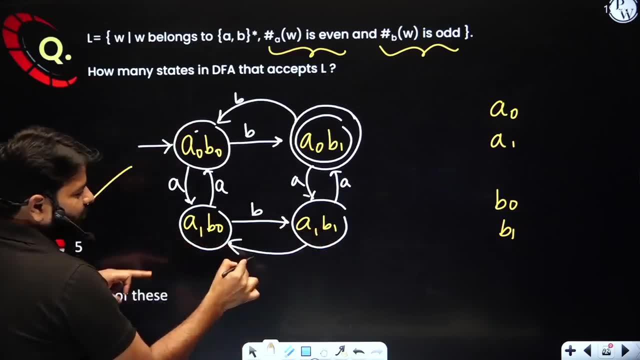 one b comes, one more b comes, that b one will become b zero. similarly, here b zero will become b one. if one b comes, other b comes from. here b one will become b zero, which is designed right. when a is divisible by two, b is divisible by the same concept. 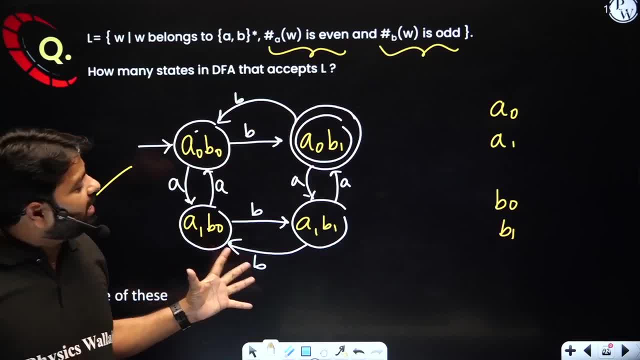 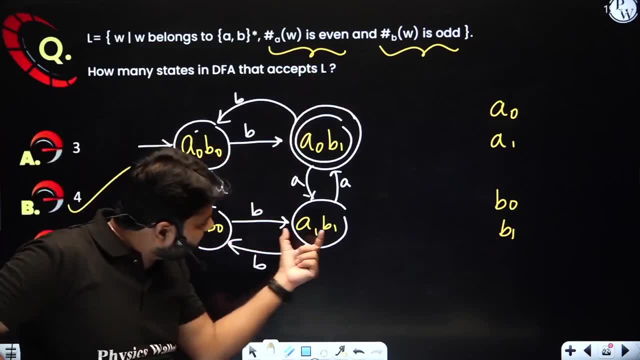 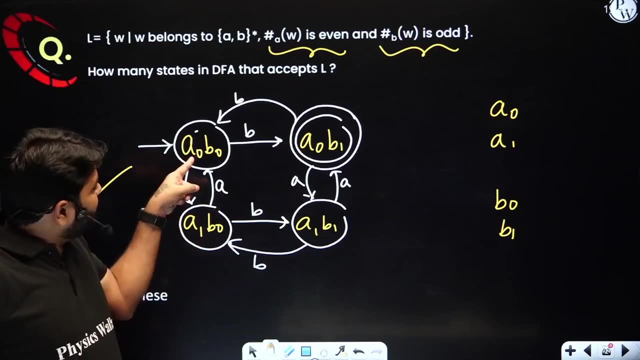 but so easy machine. now look at how many different problems you can solve with the help of this machine. a zero b. one will say a's is even, b's is odd. if i make this, one is the final, that is, a's is odd, b's is odd. if i make this is the final, a's is odd, b's is even. if i make this is the final a's. 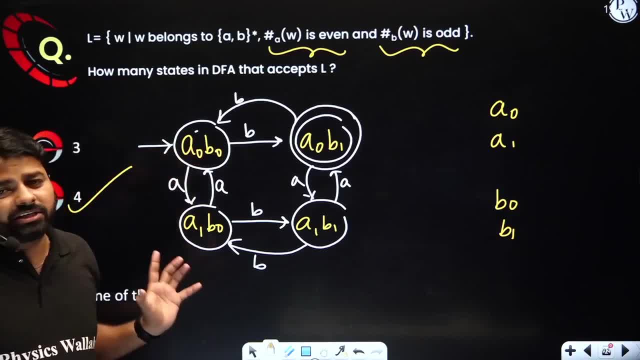 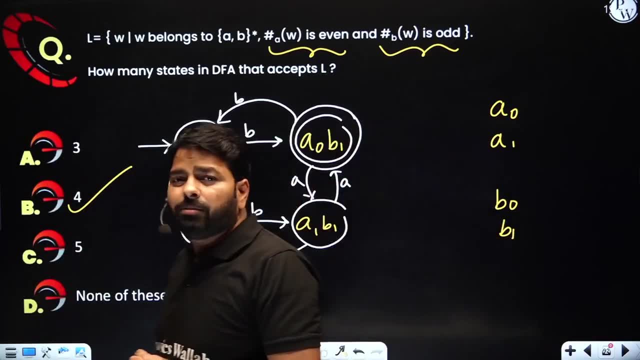 is even b's is even see how many, how many problems exist here. okay, it's a very simple concept. if you want to answer for the gate, right, it could be answered within five seconds. but if you want to understand, it will. likely it will take little time to design the whole machine. fine, you got the four answer, four states: 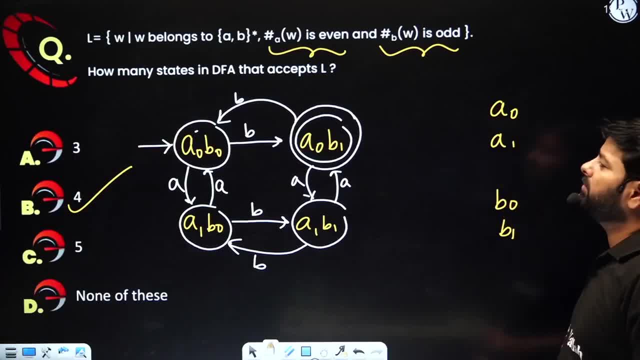 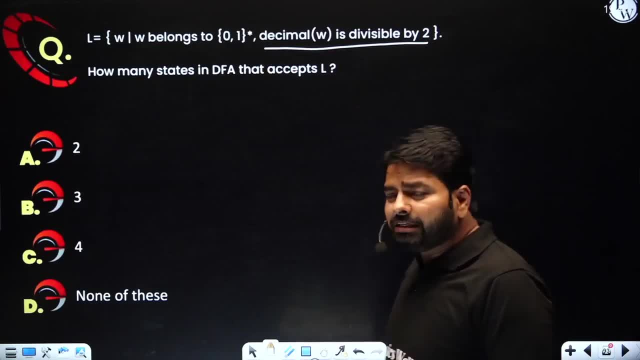 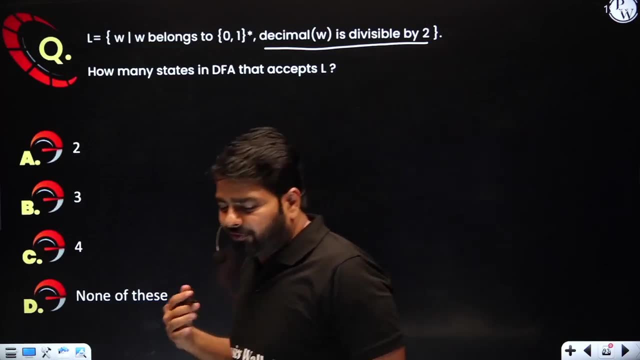 i have shown how to design with the help of reminders. okay, uh yeah, decimal equivalent of w is divisible by two. so it's a very simple again. the number of states will be divisible by two, which will depend on some i know different property. it's not the length, it's not number. 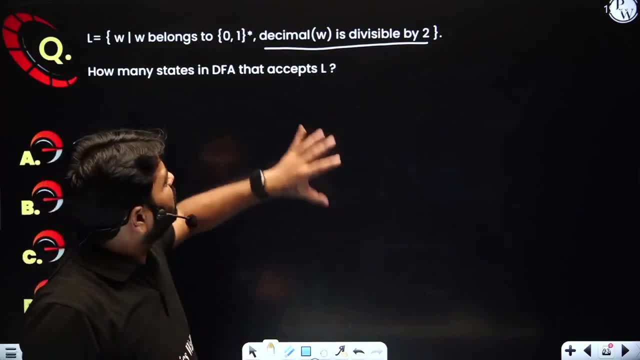 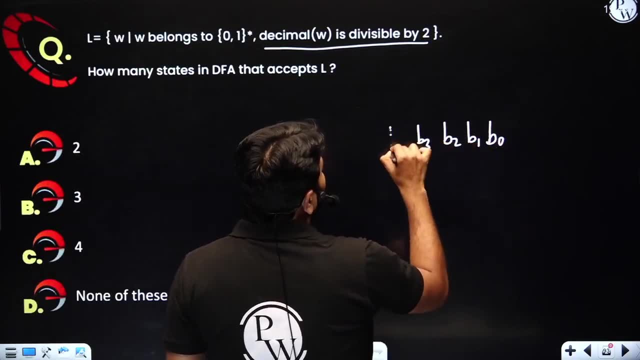 of a's, it's not number of b's, it's decimal equivalent. so what is this decimal equivalent of binary? see, you have a binary concept right: b0, b1, b2, b3. tell me if this binary number is divisible by two. of course decimal equivalent of binary is divisible. 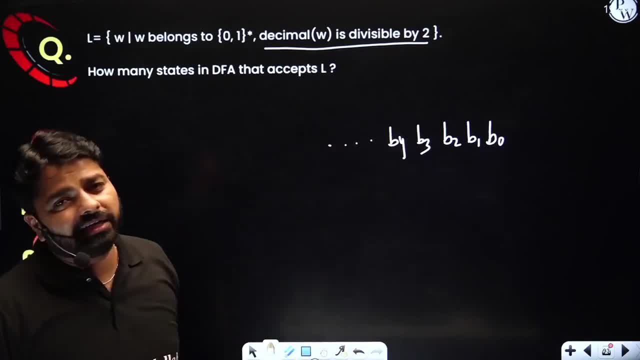 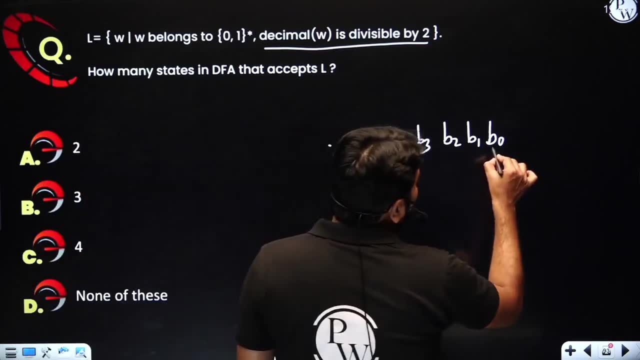 by two. what do you see? what do you see? a speciality in this? you will never see here one, because you know it's even length means ends with zero. so it's you always see here, no one here. it's always zero. here, right ends with zero. it's almost the same concept and you will never see here one. 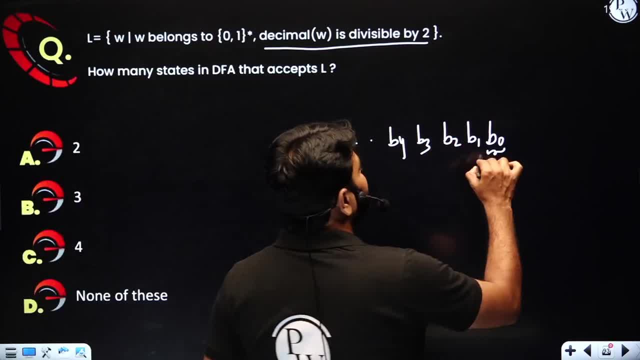 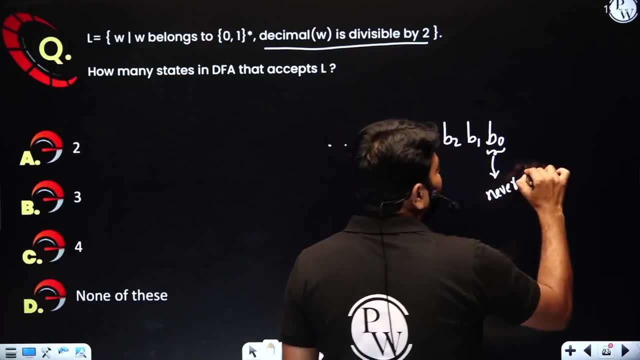 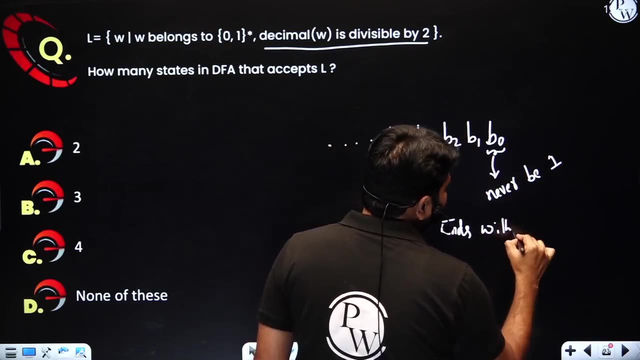 so like ends with zero, right? this is never have a zero. it will never contain zero. sorry, never be one. i'm very sorry, never be one. it's ends with zero concept, right? if any binary number ends with zero, can i say that it's always divisible by two? yes, because 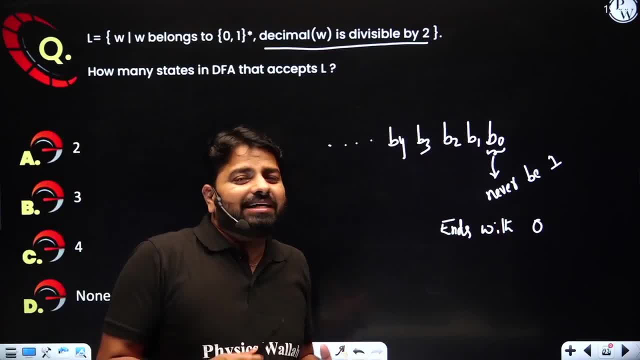 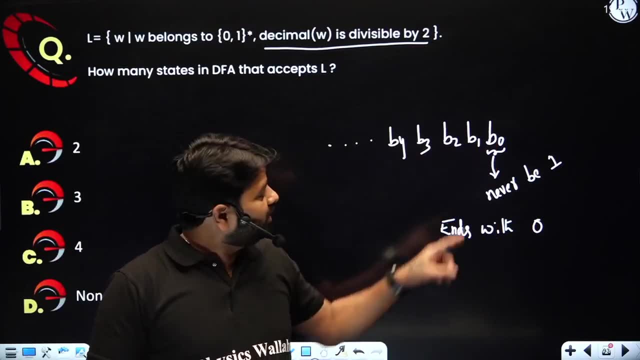 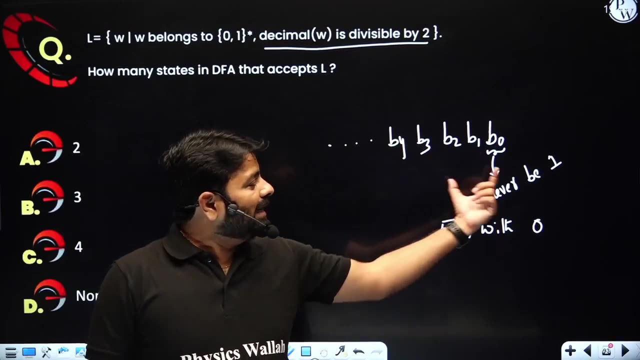 it's even number. what is? even if binary number is having the lsb as zero, it's always multiple, two or even number. when you convert to decimal- right, because this all are two powers, you will get the even number. if you want to become odd, that b0 position has to be one, so that never be. 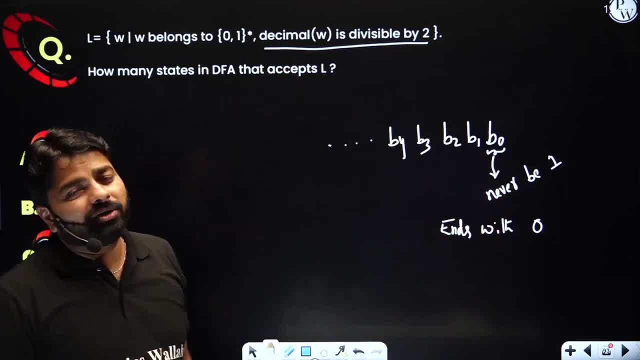 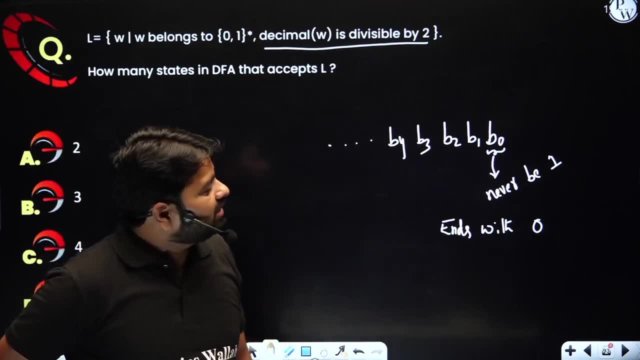 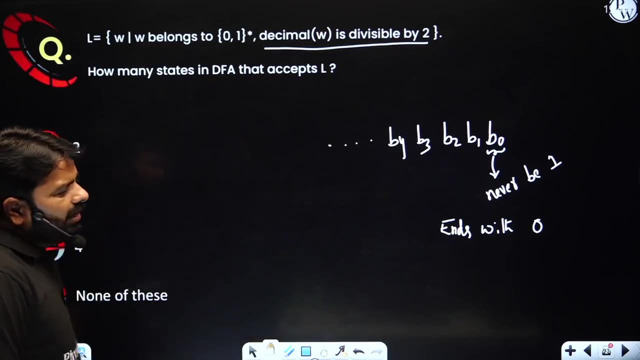 one will guarantee that decimal of w is divisible by two. okay, there are special strings like epsilon. do you want to accept or not single zero? you want to accept or not, that's your choices. but you may keep epsilon or not is your trick. so ends with zero, in case, if you design, ends with zero. 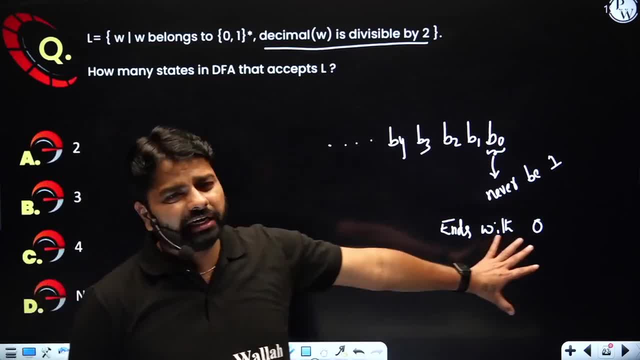 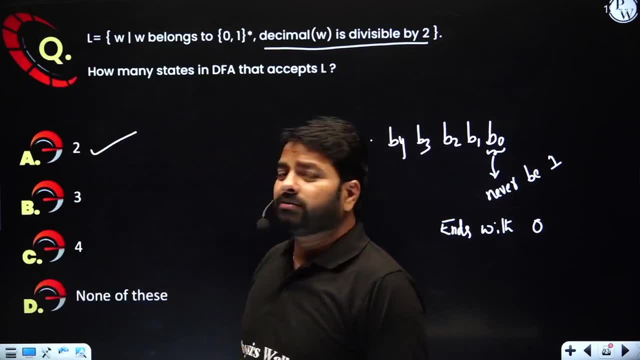 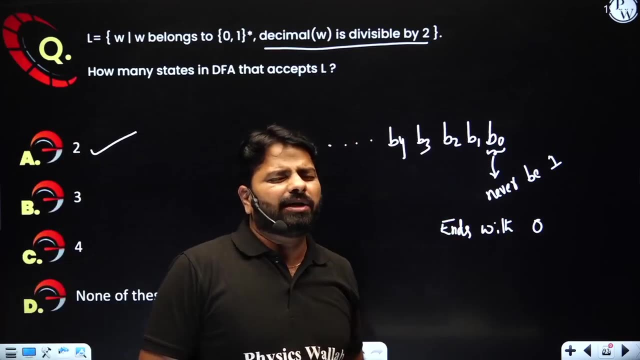 the machine how many states required? it's two states, right. the same motion can be used here as two states, so here the answer is two states. then how did you get this? how did you get this so very simple that you know all the properties? decimal equivalent of binary number will have the 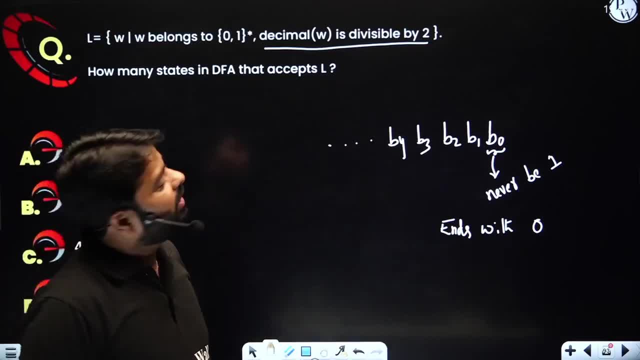 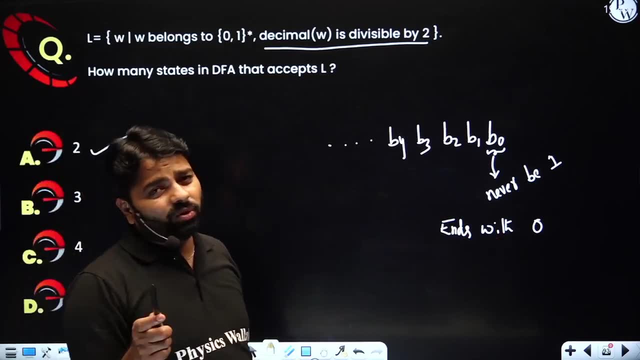 similar property like, instead of divisible by two if you have, let's say, four. so i'm just writing a shortcut. but if you want to design definitely will take time, so i'm just giving the shortcut how to answer it, in case if you see that videos, please follow it. suppose you have divisible by four. 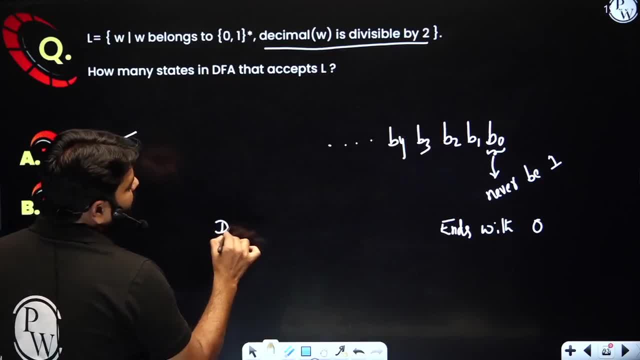 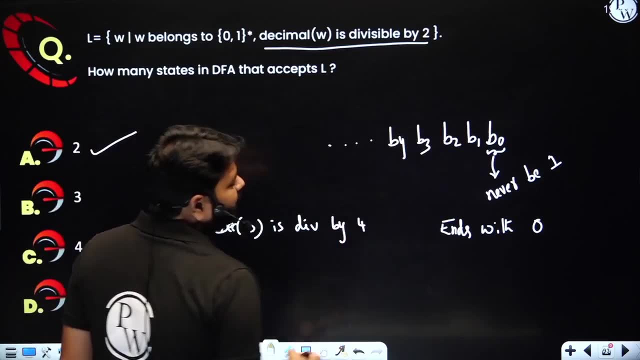 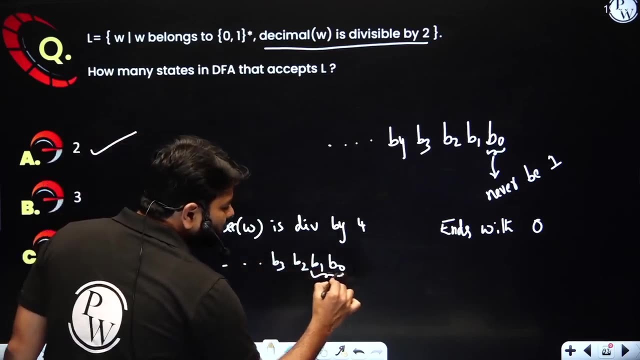 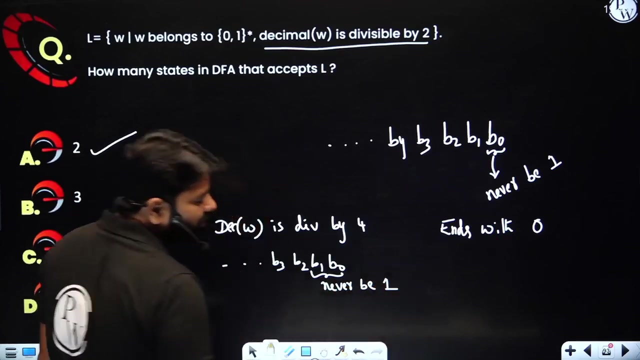 divisible by four. i'm just solving it: decimal of shortcut. i am trying to help you- is divisible by four. then what is the concept you will be having this? last two bits should never have a one right, never be one. b0 and b1 should never be one. then remaining will all. remaining will all have the multiple of four. 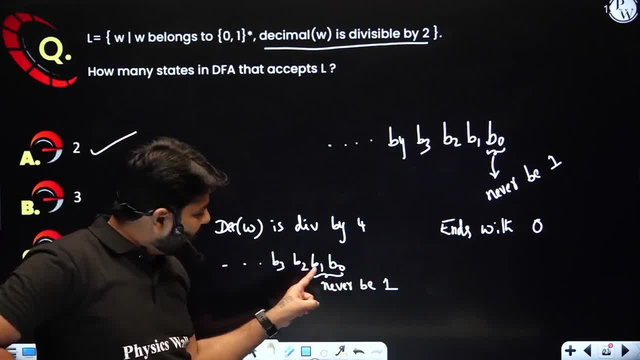 so number will be definitely divisible by four. so if you keep any one here, either b0 or b1, then that number will- uh, that decimal equivalent will never be divisible by four. that is the reason this should never be one. so it's almost equivalent to ends with double zero. 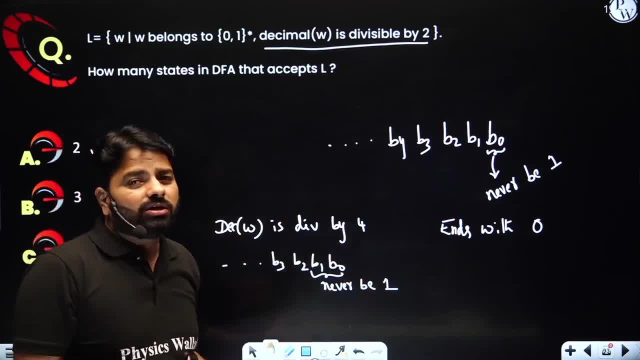 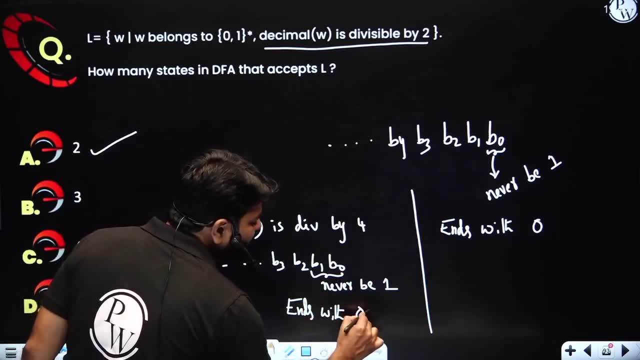 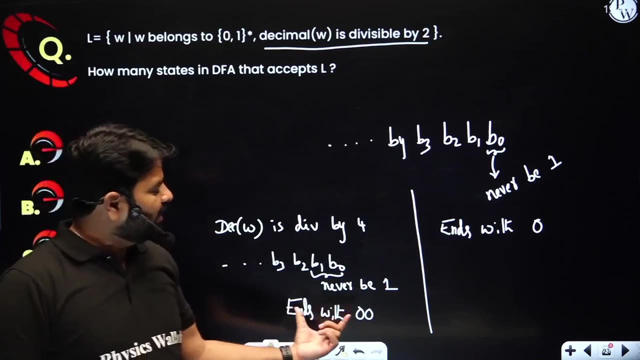 of course, not exactly same, but the same motion will be used somehow. okay, so this will be concept similar to ends with double zero. how many states required for ends with double zero? ends with double zero. if you solve it, it will take just three states. okay, please try that. ends with: 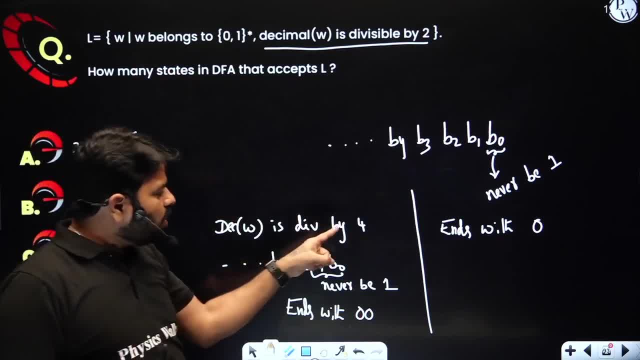 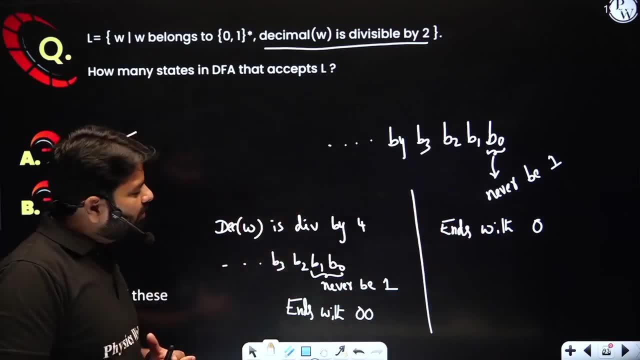 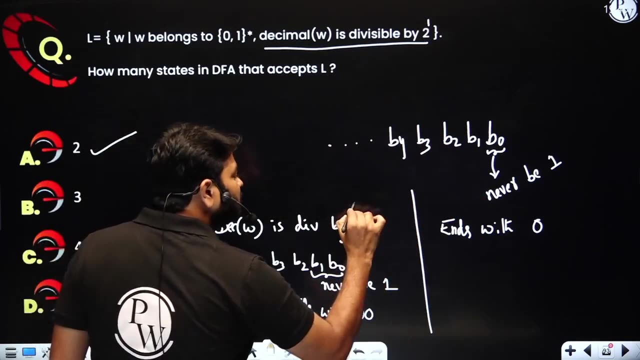 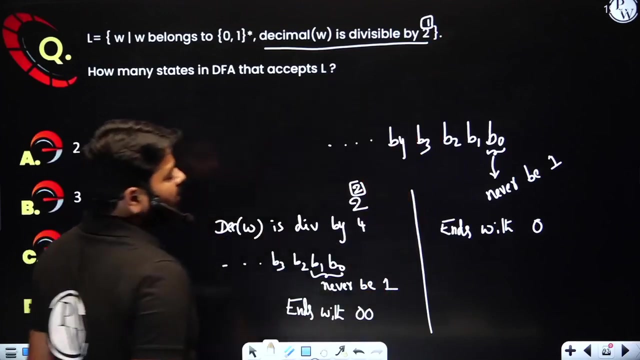 double zero motion, it will take three states. so what is the concept? divisible by four, three states, divisible by two or two states, what is this concept? right? so remember? divisible by two, just assume it is two power one. divisible by four, assume it is two power two. so look at this power. look at this power if it is one. so if i say it's a binary number only, 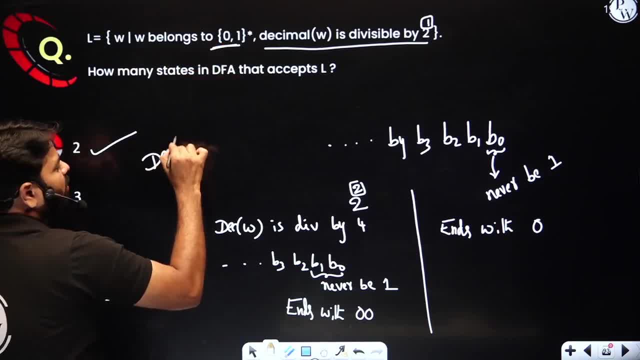 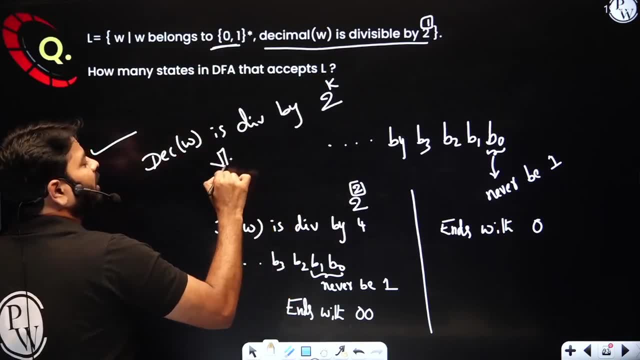 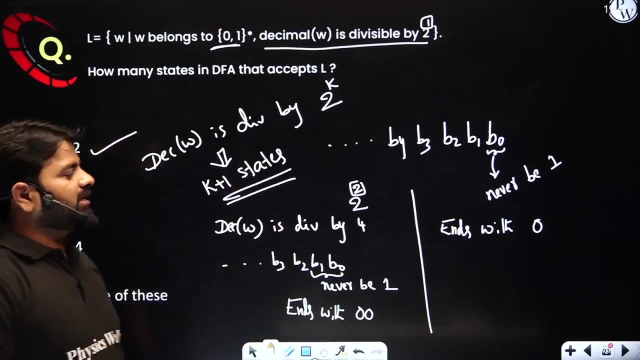 i'm talking about, not ternary or any other. right now, decimal of w is divisible by two power. let's say k, then the straight away you can answer k plus one states. so very easy shortcuts for you to remember. but of course, designing the dfa will definitely take time and i believe that you can try. 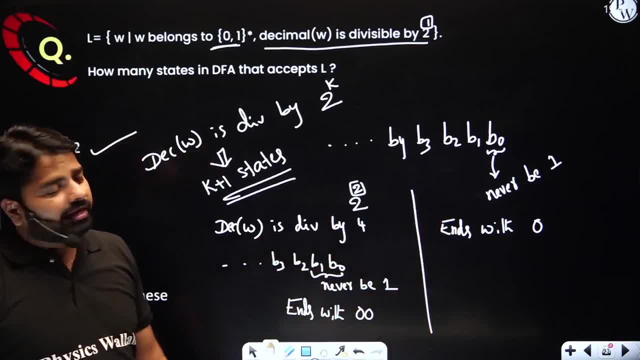 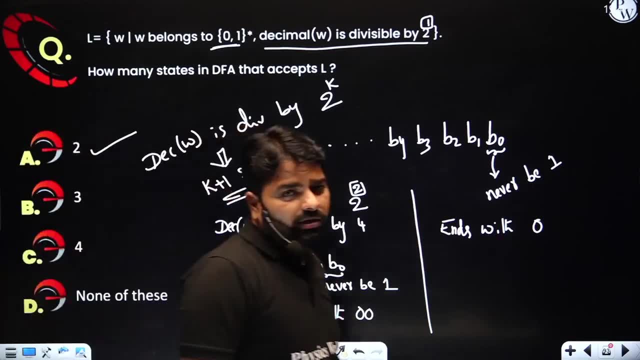 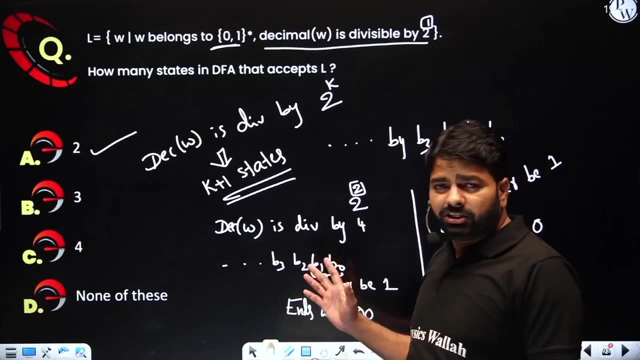 on your own. i have shown the trick how you do that. in case, if you really want it, i can take one problem. i can do it, but work on it or remember the shortcut. that is your choice, fine. so in case you wanted to understand more about it, please, uh, keep on watching the practice sessions that. 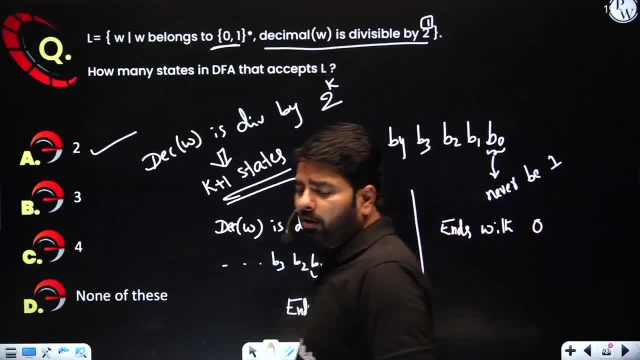 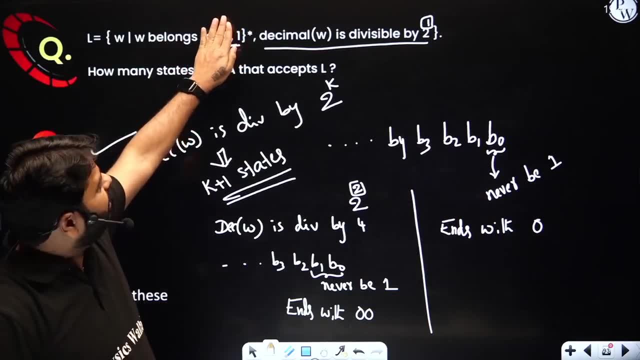 i do at the end. so definitely i'll come up with this one problem and i'll i'll solve for you. fine, so you have a shortcut now. whenever you see binary number here, binary language here, and in the description you can see that every decimal equivalent is divisible by some two power: k. 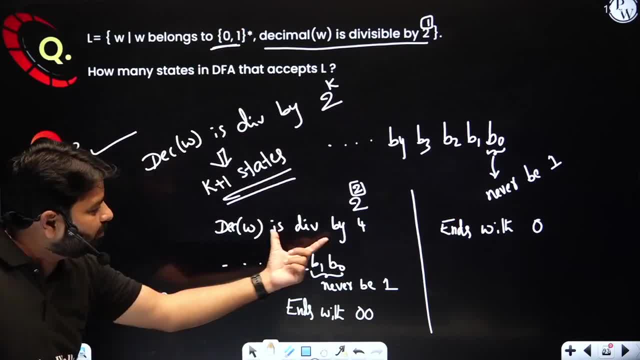 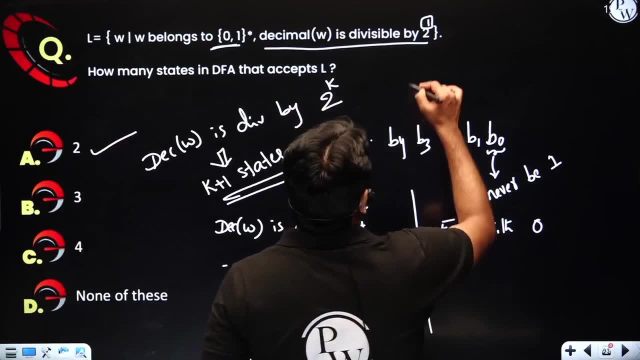 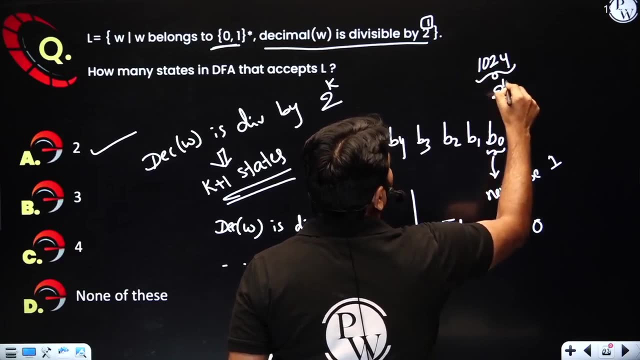 let's just say that k plus one states needed here diesel by four. convert this four into two power k form and k plus one. now i'll tell you: divisible by previous gate question, divisible by 10, 24.. tell me how do you do that? 10: 24 is nothing but 2 power 10.. how many states required 10 plus 1? 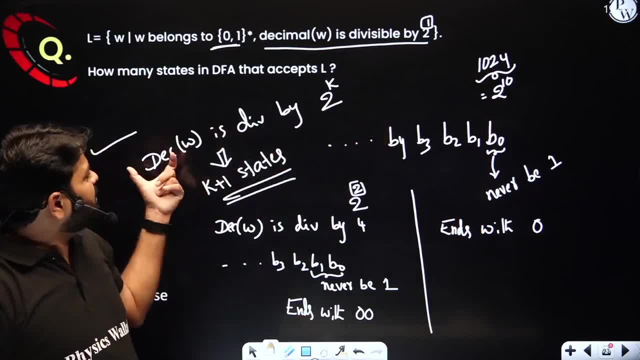 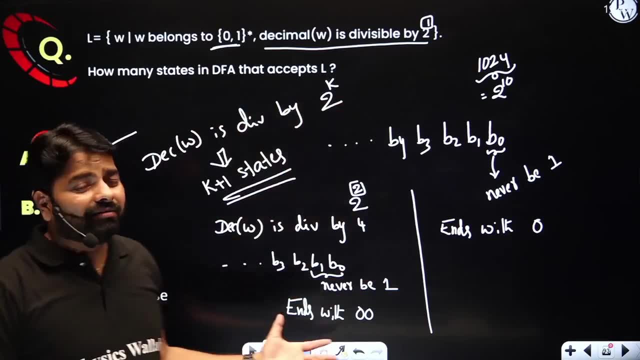 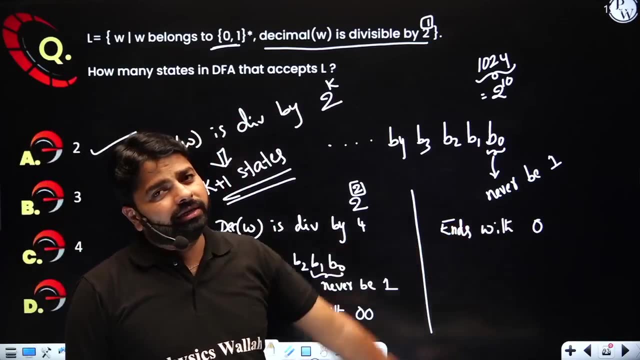 11 states. that's all. that was the gateway by q. so decimal equivalent of binary is divisible by 10, 24.. 11 state: okay, don't show somebody how the 11 states, which is not required, but understand how you get this formula. that is very important. okay, as it is. 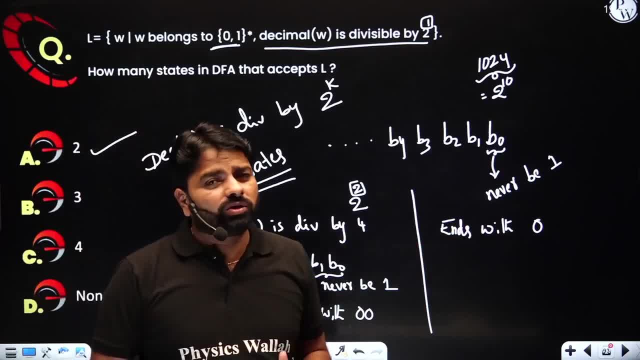 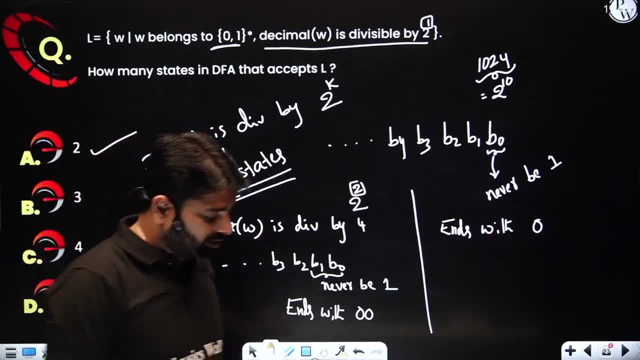 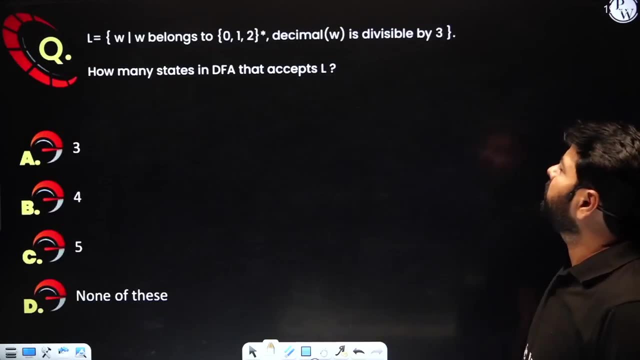 a crash course. so it's important to know how to answer the each question in the gate, rather than knowing you know each and every concept at the end of the um, end of the you know just before the gate exam. fine, you have the homework. now the same question here. it is churnary now in stock b binary right now. 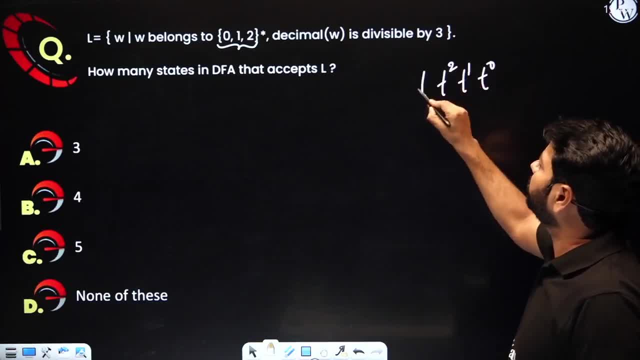 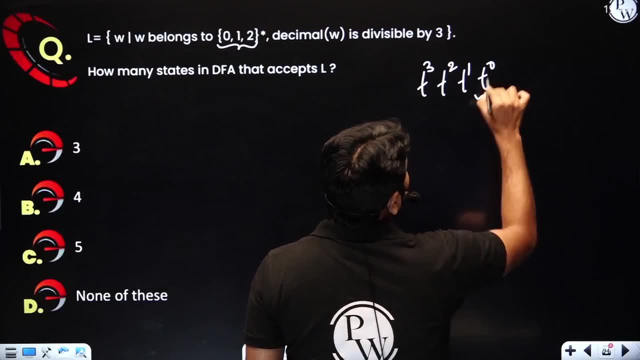 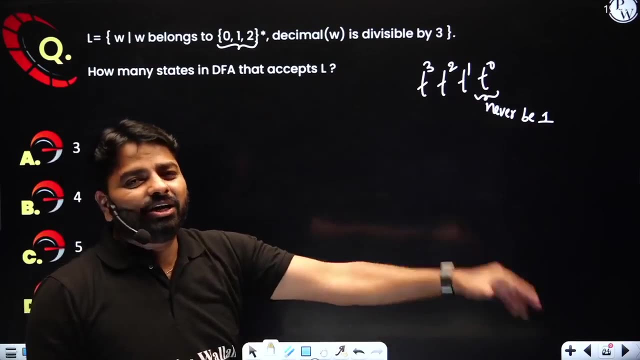 t power 0. churnary number. now: t power 1, t power 2, t power 3. now divisible by 3: same concept. divisible by 3 means three should never be one. this t power zero, it should not be one again ends with zero concept. the answer will be same again: two states will have. so here three powers. it is a turner in a. 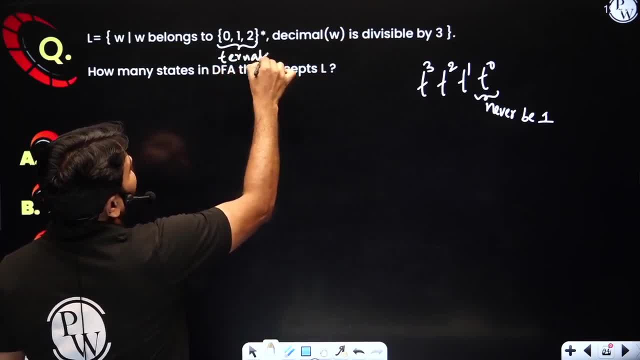 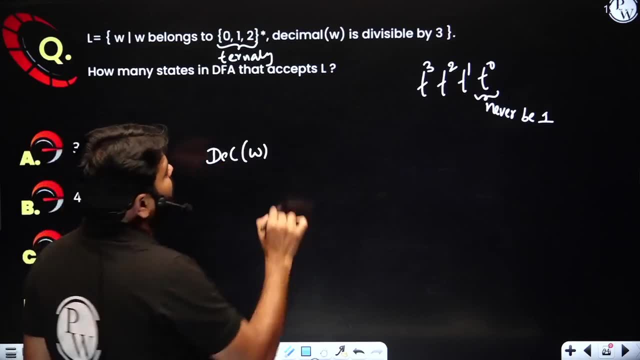 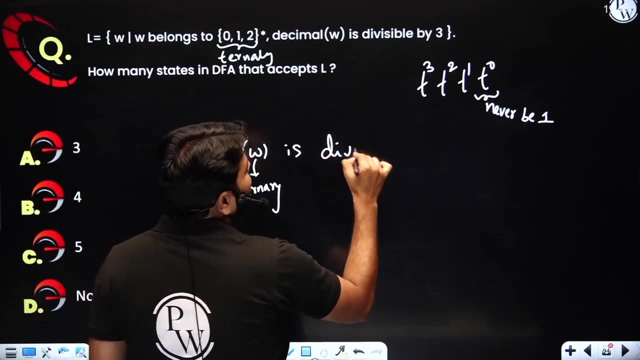 number. this is ternary. remember that. it's ternary concept, right. so here, divisible by decimal of- but don't use this formula, for binary will not work- decimal after this is ternary number. remember that is divisible by 3. power k will definitely require k plus. 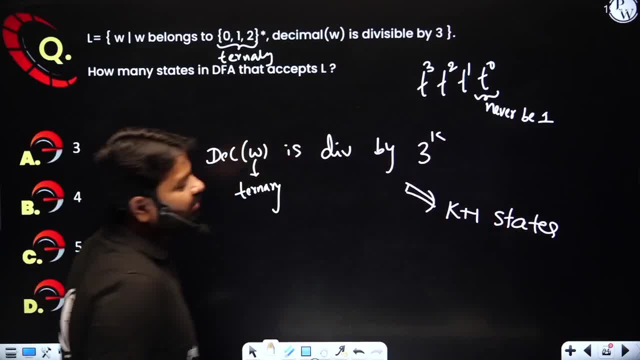 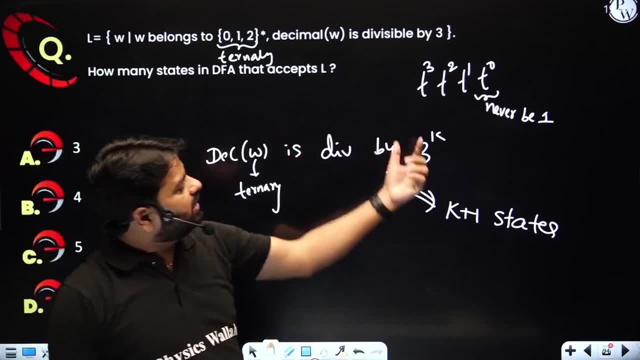 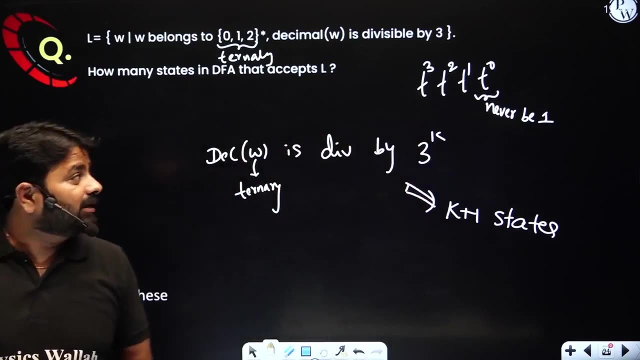 1 states. only the thing is, language over the alphabet is different. okay, this is another shortcut so you may use. now this is the 3 power 1, so definitely 1 plus 1. 2 states here. okay, you can just answer it without you know designing the machine. similarly, i can go for any language. 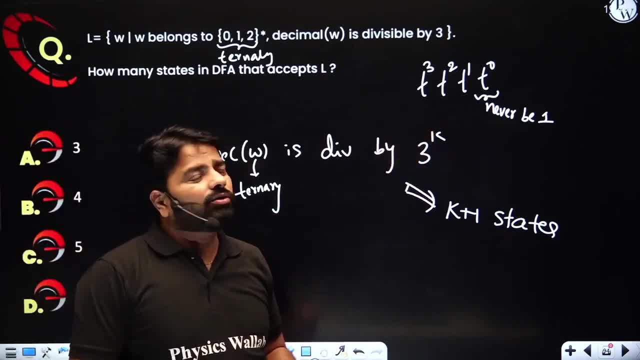 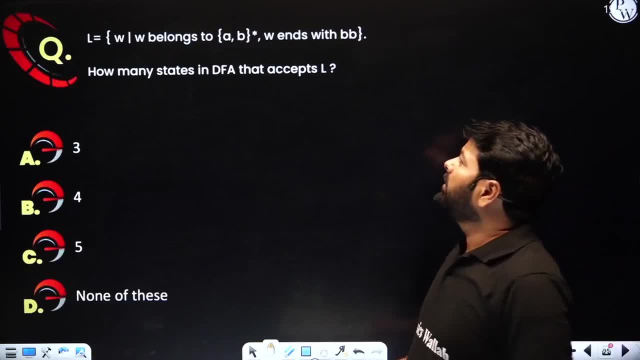 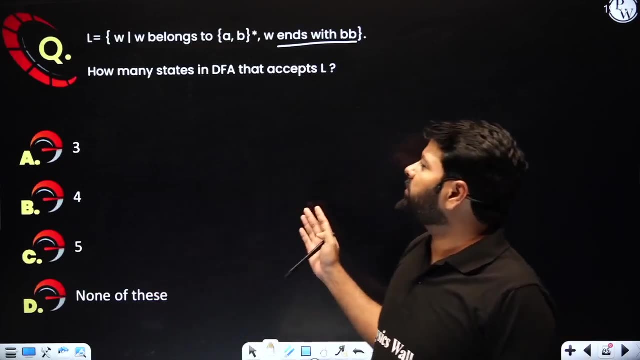 or any alphabet. it could be binary or unary, ternary or any concept. you can solve the similar way. okay, ends with double b. first time i'm solving ends with double b concept, right ends. i have not done it, so i wanted to solve this question for you. ending is one of the important concept in 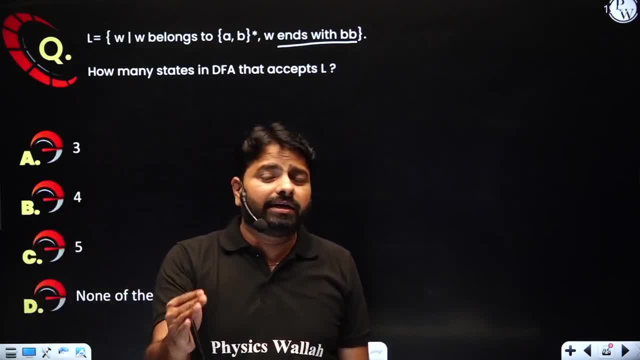 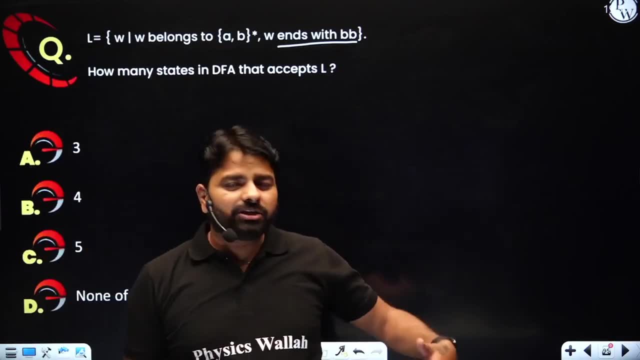 designing dfa. that's why most of the people will fear while designing dfa for ending conditions, because if you never know that the ending when happens, you should wait for that end. starting means you can check and if not, you go to dead state. but will you go to the dead state? 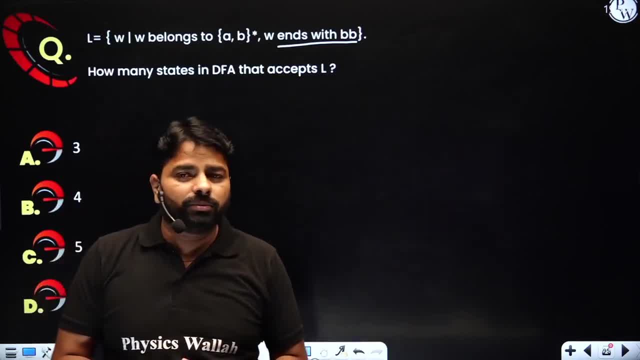 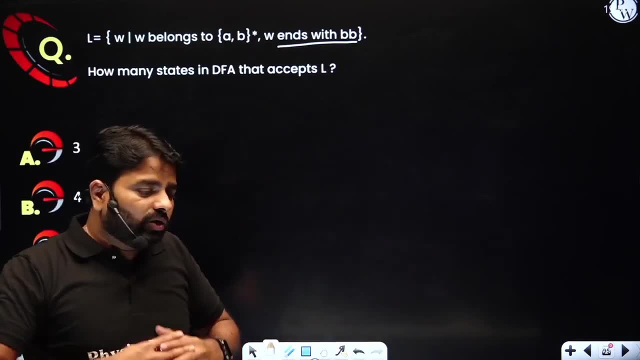 while waiting for the end condition. no, that's not possible. that is the reason you you should design many problems which are having ending conditions, so that you will get to know how dfa helps in understanding the problems or solving the problems which are looking a little bit difficult or different. but come to the point, how many states? 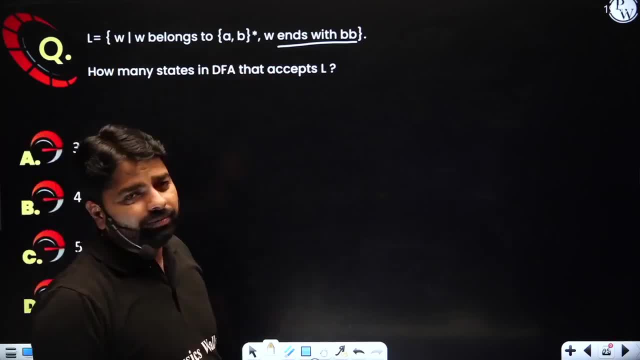 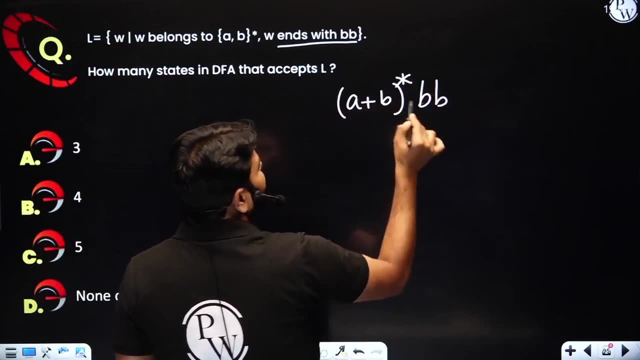 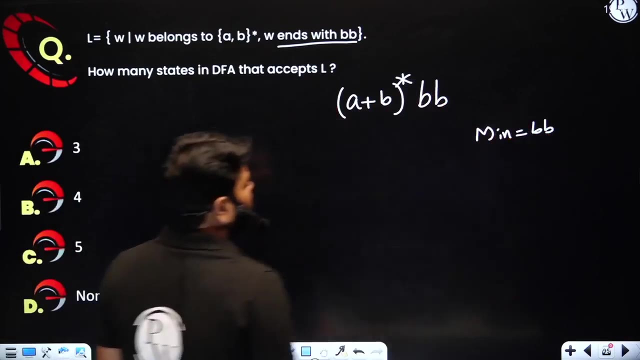 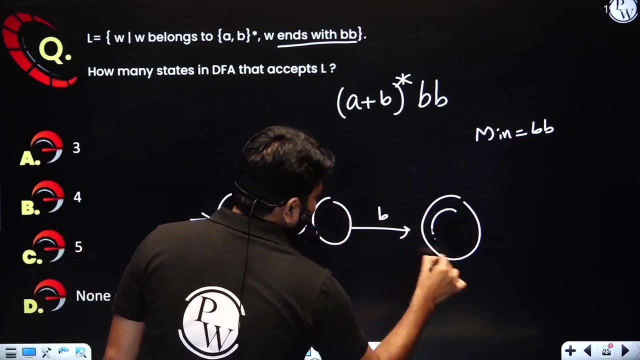 in dfa that accepts l, where the string ending with double b. what is ending with double b? so ending with double b, before that, any number of symbols over a's and b's. this is your expression and what is the minimum string? double b. so how do you design a machine? b followed by b. then you go to final state: okay. 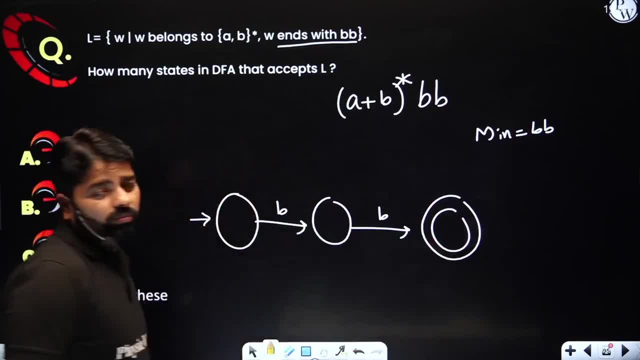 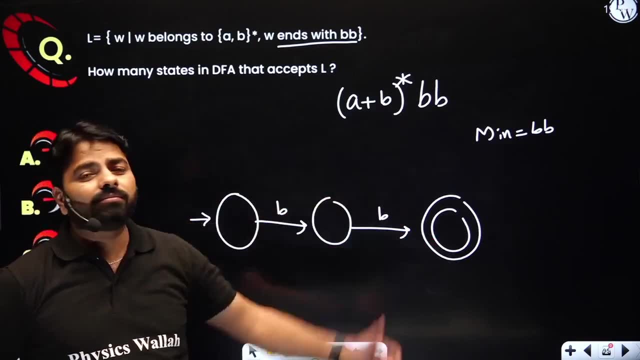 but now, in this process, should never go to dead state. why, if you go to dead after the double b may come, you can't come to the final once you go to dead. that is a difficulty, right? so you should never think about dead state. you should never think about dead state. you should never think about 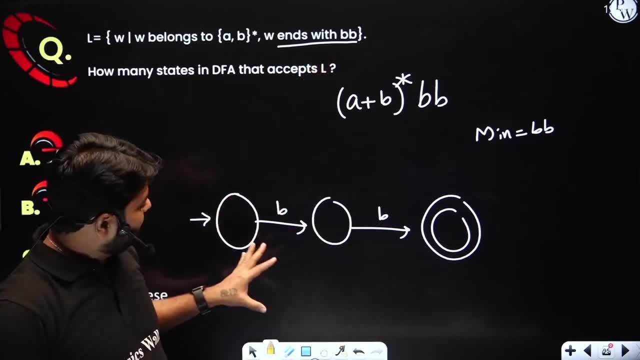 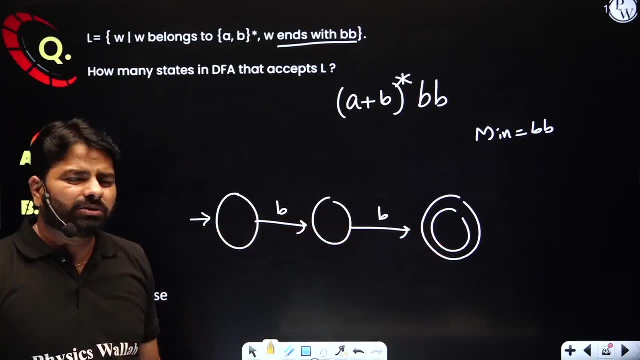 dead state. in this ending condition right now, our target is to stay here when you get double b now, before this b. if a comes, will you wait or will you go to dead? you will wait, so i'll stay here any number of a's, because i don't know when double b comes. so i stay here after b. when a comes, don't. 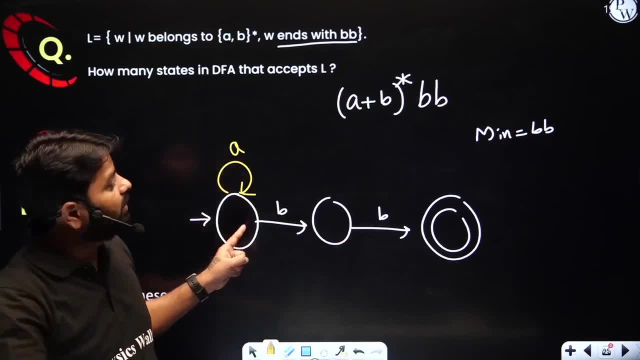 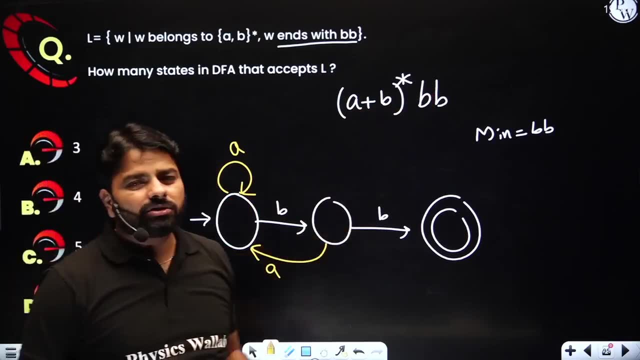 go dead, i'll come back. i'll look for two consecutive b's because i need two consecutive b's at the end. when a comes, i'll come back. right, if this b comes, don't assume your string is over, because after double b you may have something. 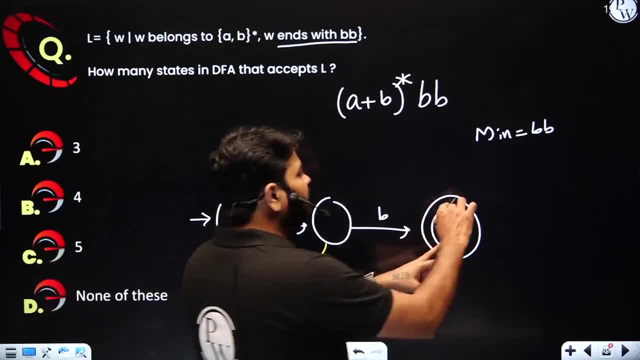 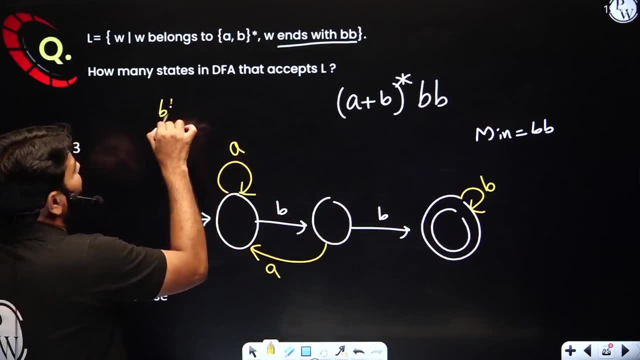 you don't know, right after double b, if b comes, you are safe. why safe? because double b followed by any number of b's, it's still ending with double b only. you see that once you get a double b, any number of b's are coming. still it is ending with double b only. but after this double b or after 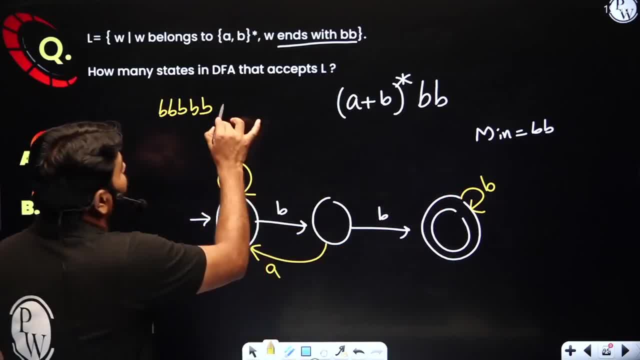 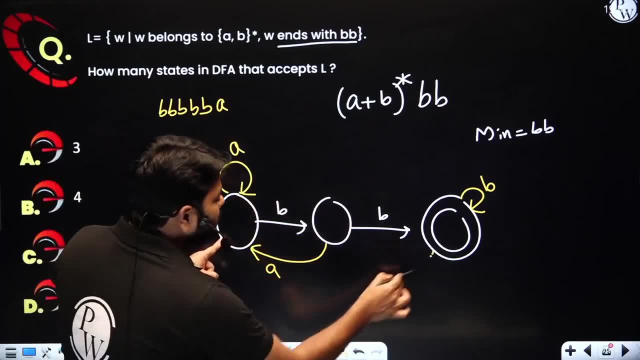 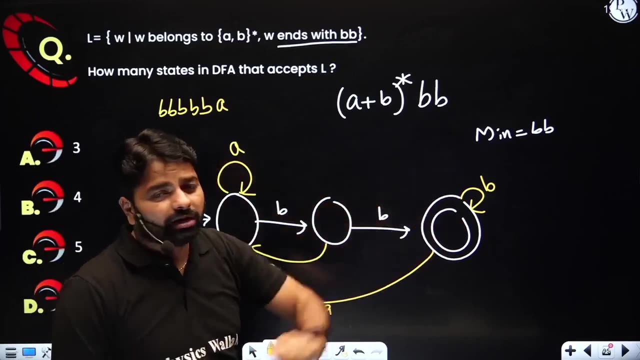 this b. if a comes, then whole sequence is interrupted. now again you have to look for double b. so you should come here to look for double b again. is your machine over? yes, see that. from this a b covered. from this a b covered. from this a, b covered now. 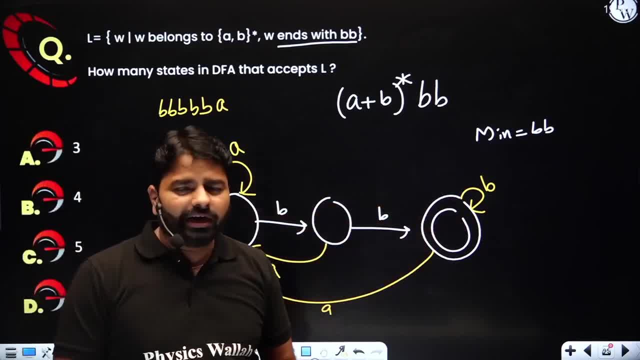 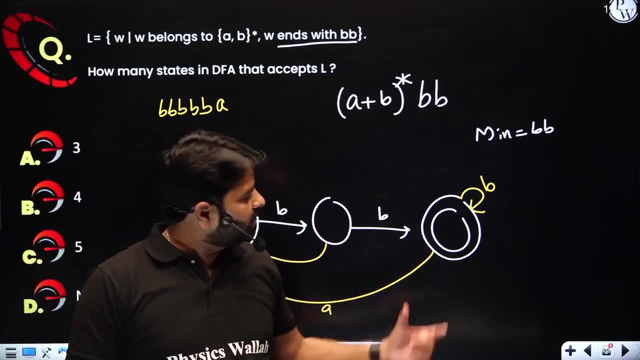 any string which is ending with double b, you will always halt here. if not, ending with double b definitely will halt here. that means whenever the string is halting here, it is invalid. you know the string halts here. it is valid because this state represent ends with double b. how many states? 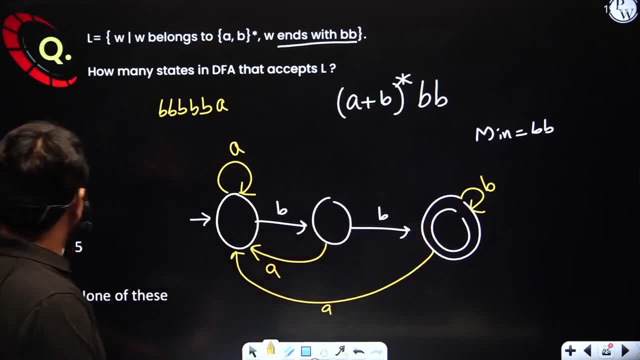 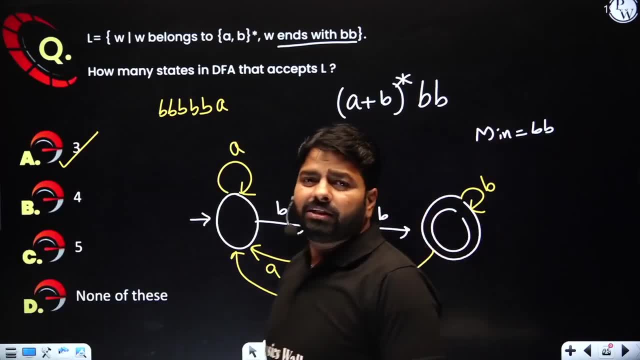 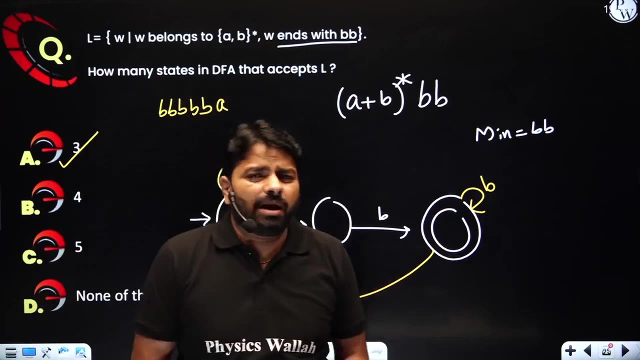 required three states. three states, which is right answer. okay, so this kind of problems are really interesting and in the gate exam ending with two consecutive b's, ending with three consecutive b's are containing three consecutive b's. these questions are happen many times and it may come again in the future. 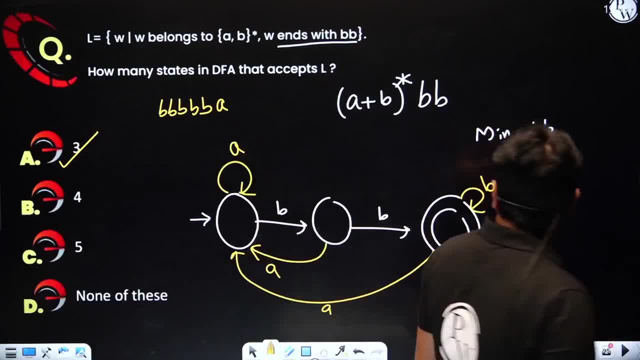 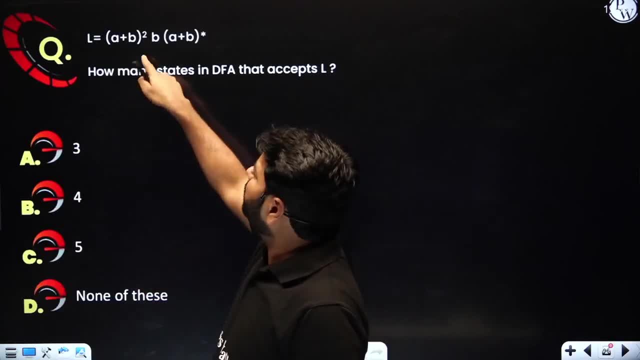 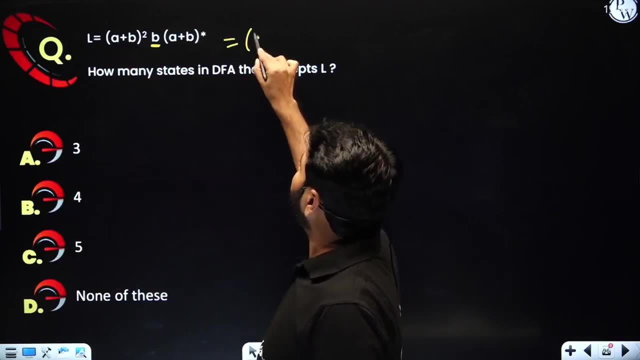 okay, so i hope now onwards you can think about how to solve them like this problem is: the third symbol from the beginning is b, because first two symbols are any, because you can see the same as a plus b, followed by a plus b, followed by b, followed by a. 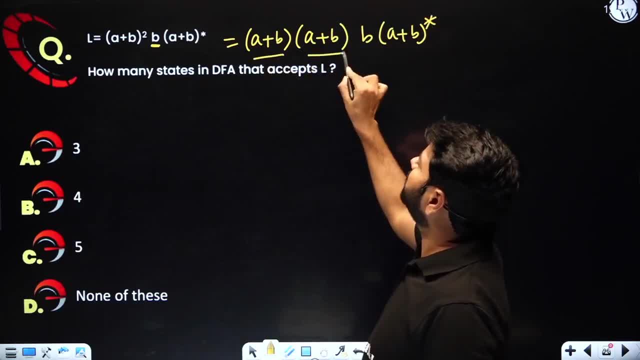 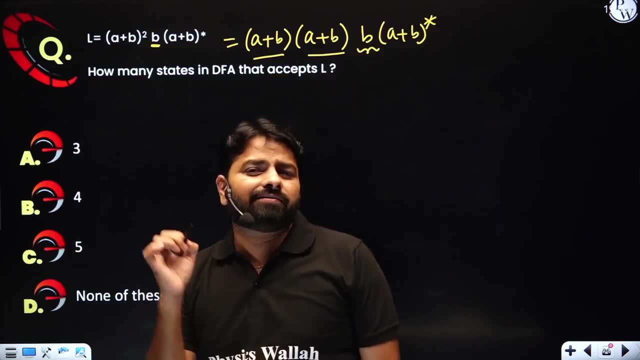 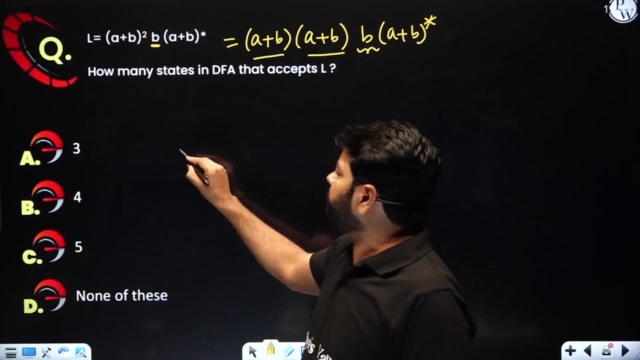 plus b, whole star. it means first two symbols. we don't care anything could happen. but third has to be b. that means minimum string will definitely have three length, right. third position is b. speed away, you design, you will get the answer. first position. i don't care, but somebody should come. 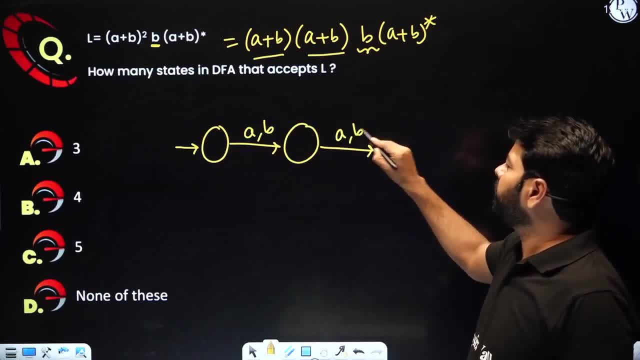 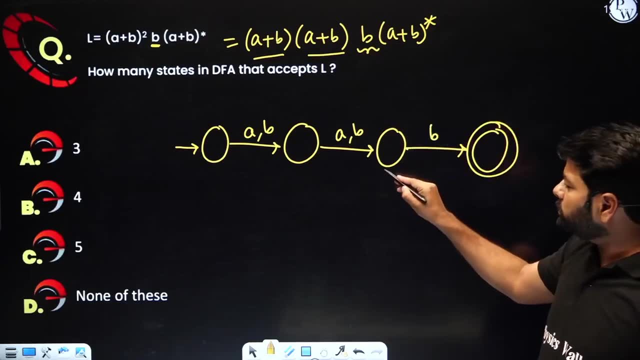 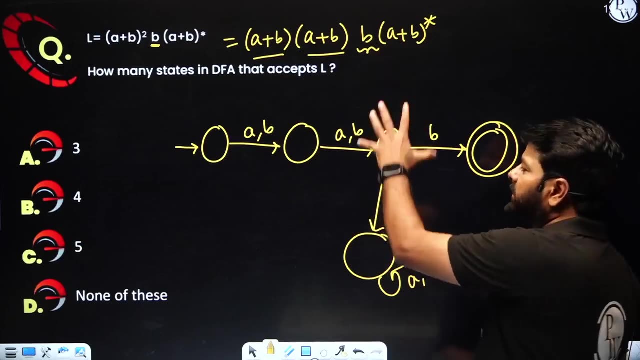 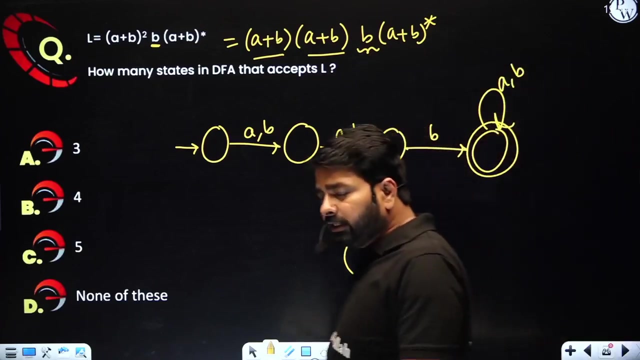 and second position: anybody, that's fine. but third position has to be b. if not b, then go to dead, go to dead. so that would be a and go to dead. the third symbol: never be a. that's guaranteed. once third symbol is b, we don't care, because everything is accepted after that. what do you see in the expression? 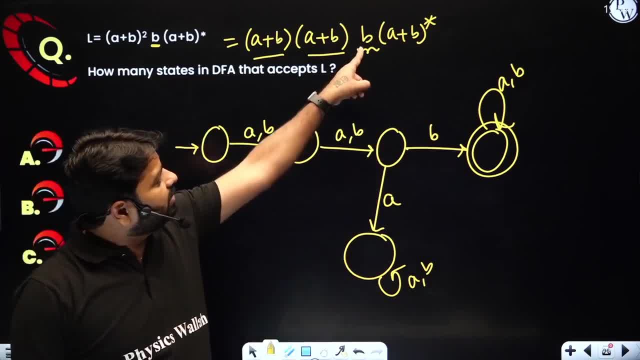 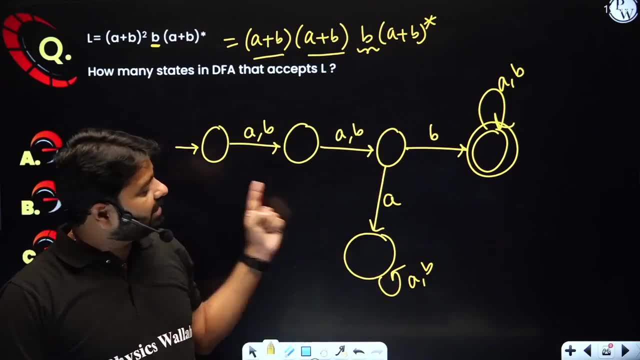 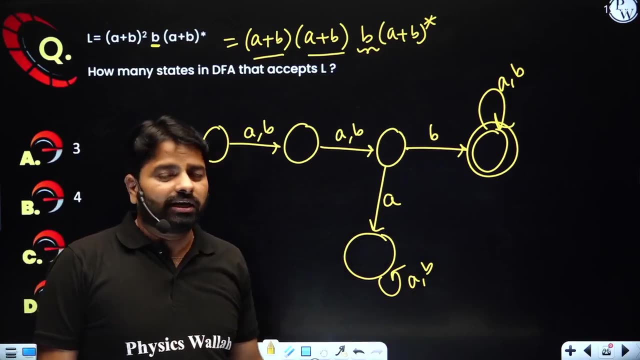 same thing replicated on the machine. but only thing is, when the third symbol is a should go to dead state, because every string in the sigma star will have exactly one path in the dfa right. whether string is accepted or not accepted, dfa will have exactly one path. that is the 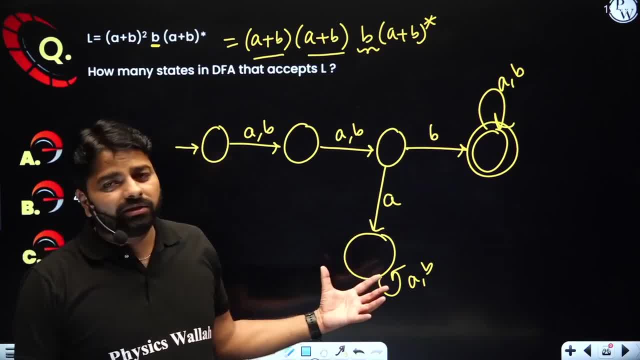 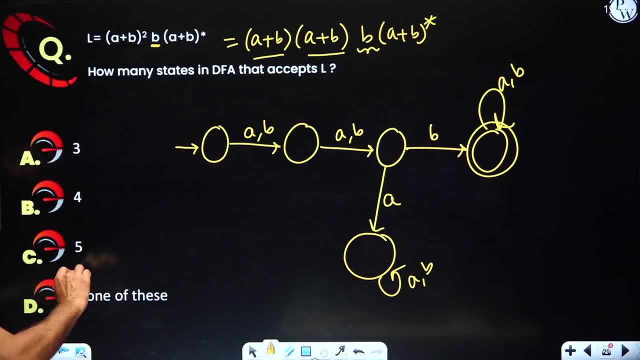 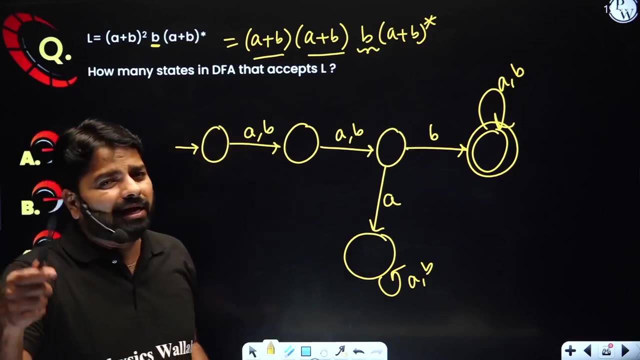 you know, beauty of the dfa. it will show a path, it will hold somewhere in the machine. okay, how many states you have? you will have five states. the third symbol from the beginning is b will have three plus two: five states. in case in the exam the same kind of question comes, like this: 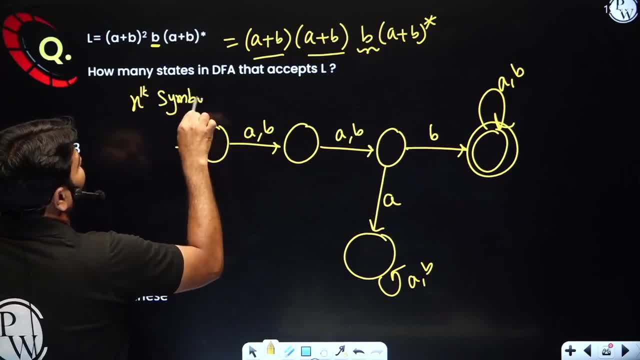 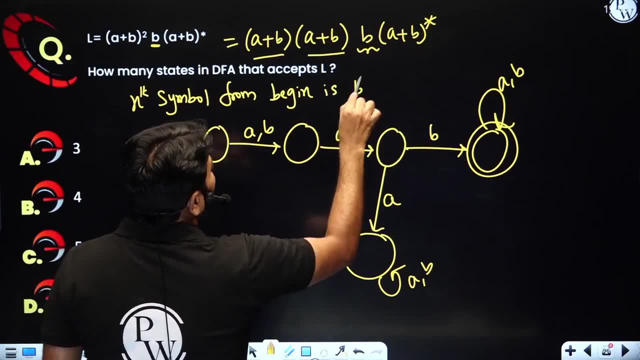 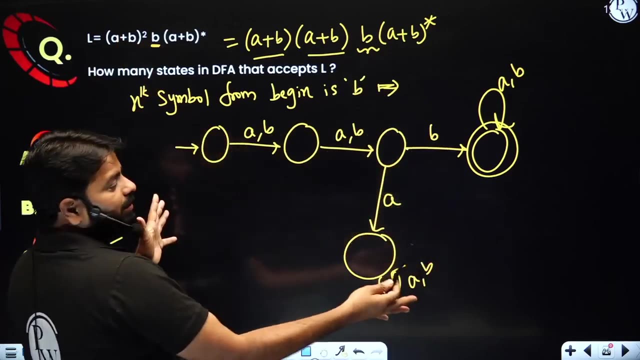 nth symbol. nth symbol from lhs or from begin is b or a, doesn't matter, begin is b. how many states you will take? your third is there. so after two symbols, third symbol, you got total three plus two, and here we'll have n plus two in dfa. 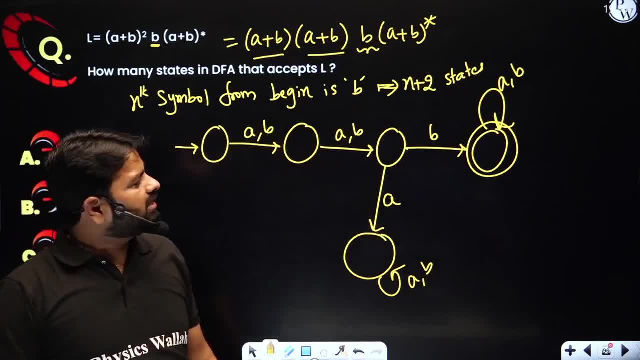 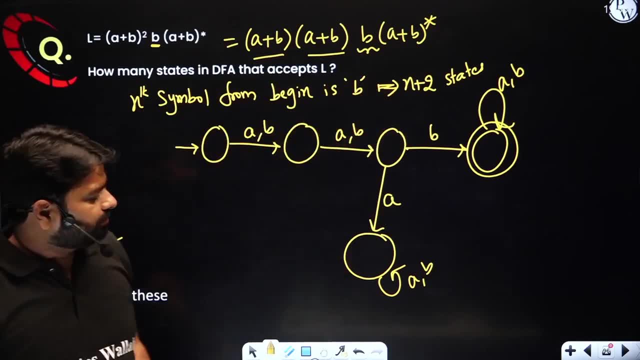 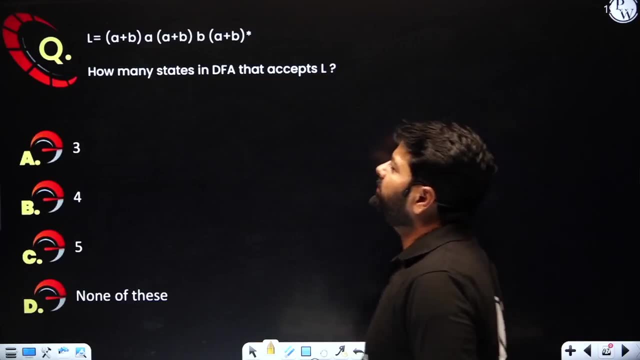 if it is nfa, this state will not be required. there you have n plus one. we'll see later. but nth symbol from begin is b. in dfa you will require n plus two states. fine, okay, uh, can you understand what is the meaning of this one? how many states in dfa for the given? 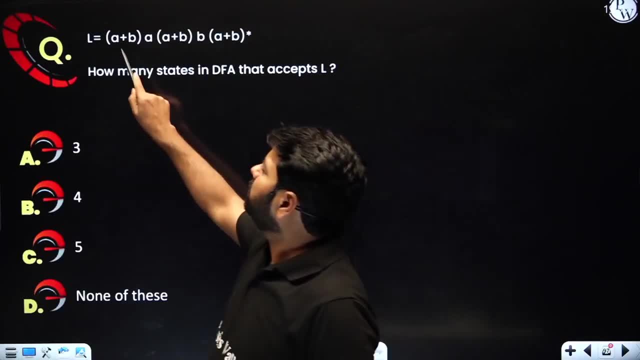 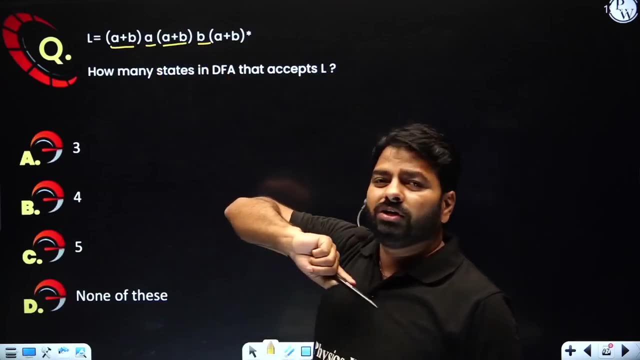 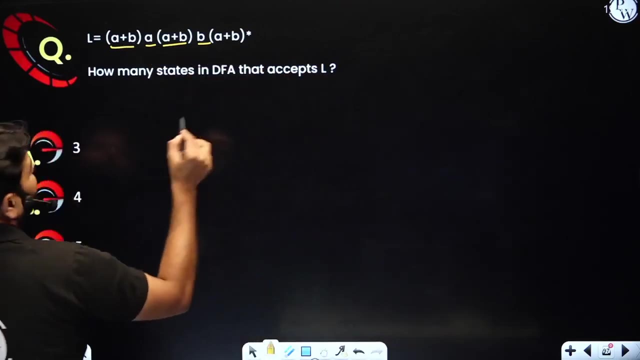 language. but what is the language? so look at the positions. the first is any. second is restricted. so the second symbol is a. third is any. fourth symbol is b. so in the language, second symbol is a and fourth symbol is b. that's your condition. so it's very simple. again, the first is any. any means either. 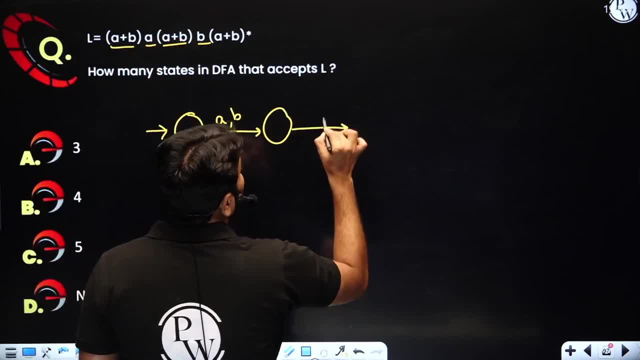 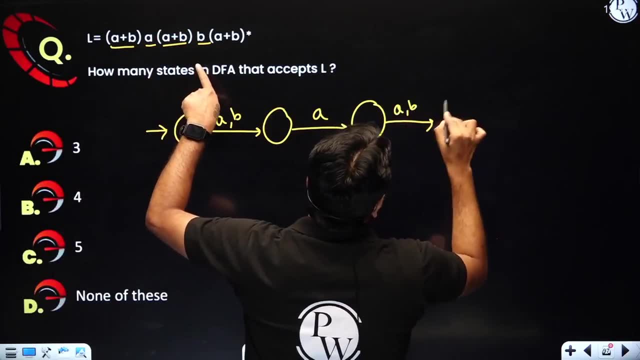 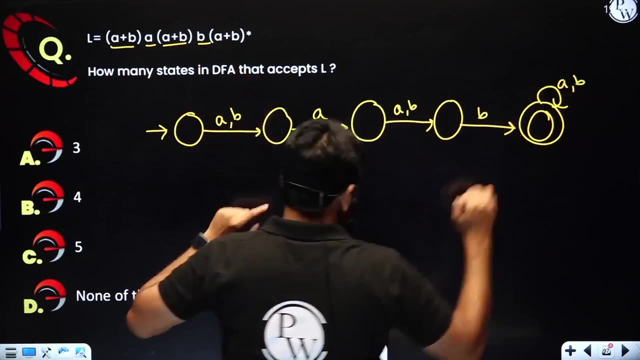 a or b. second symbol is a. if not a, then you must go to dead state. i'll show that. and third symbol is a or b. fourth symbol must be b, otherwise go to dead. anything is fine. now you must remember this. when the second symbol is not a, that should be b. 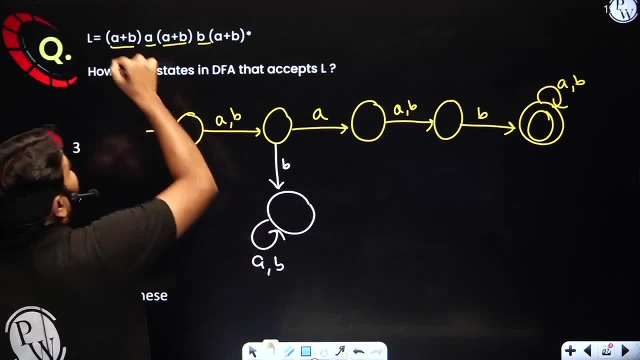 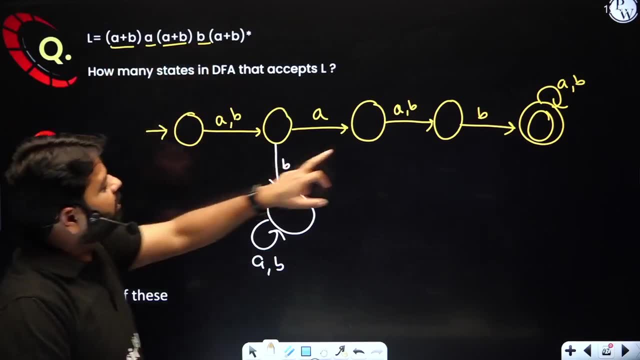 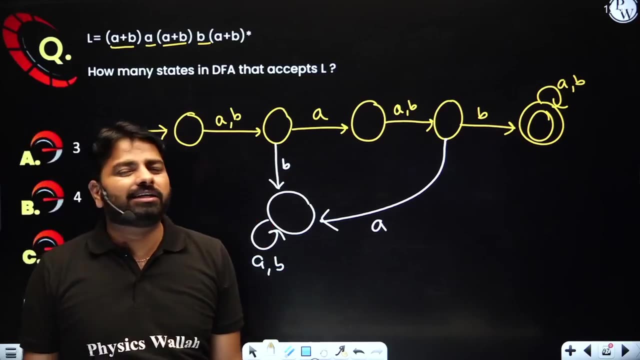 go to dead. state in this sequence: second symbol: never be b right. and third, uh, fourth symbol: never be a if not b, this if not b it will be a only in case the fourth symbol is a. go to dead and say that the string is invalid after reading whole string. 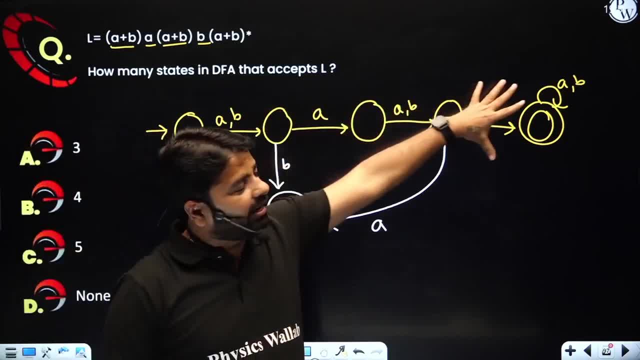 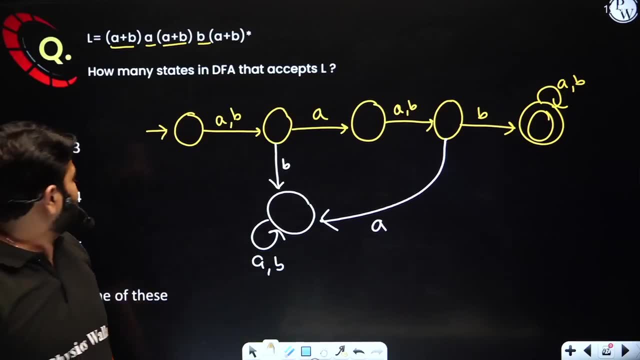 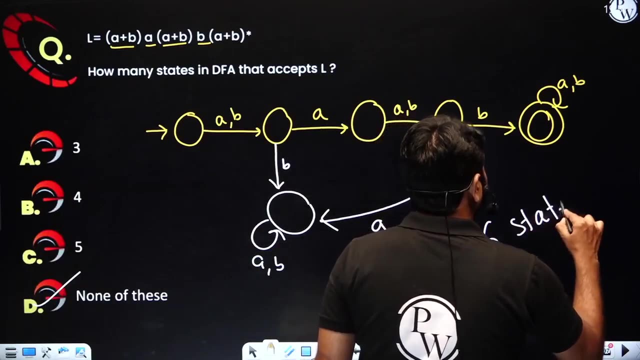 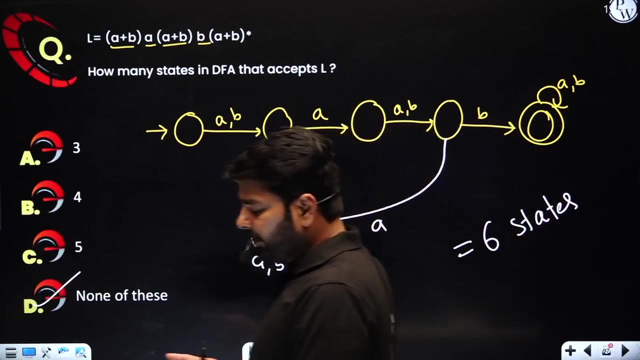 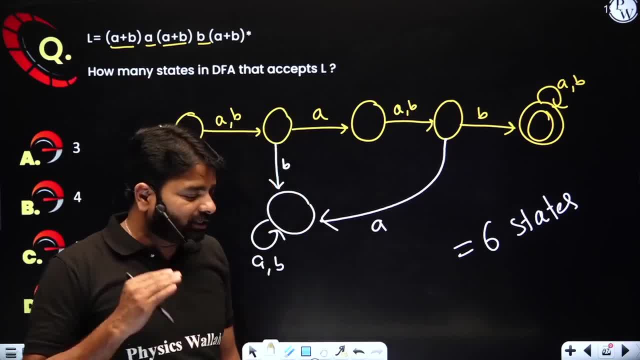 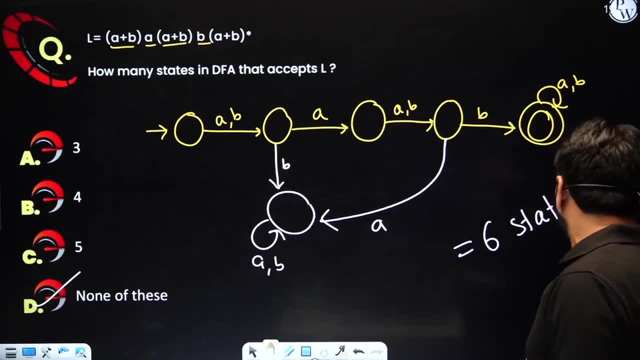 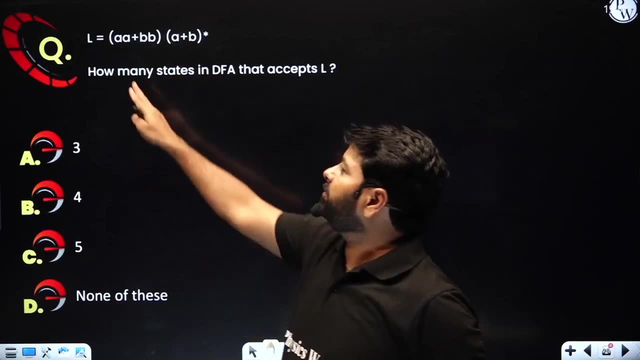 construct them. and in case if you have any doubts, please keep discussing. below this video i'll help you. what is the right answer, how to approach it? okay, so let me give you a lot of homework problems for you. this is starting with w or double b definitely will have a dead state. okay, if you get after a b or after b a, you should go to red state. 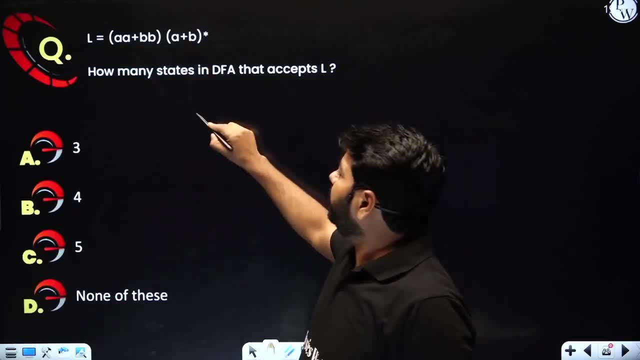 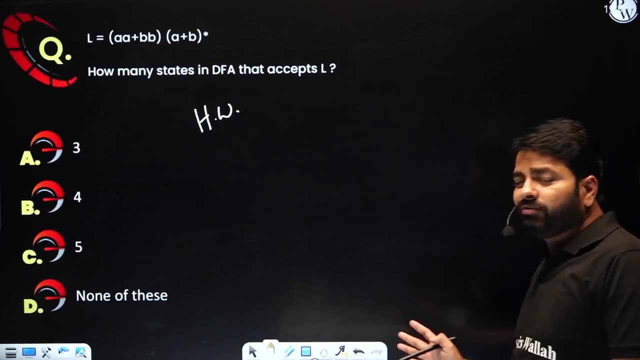 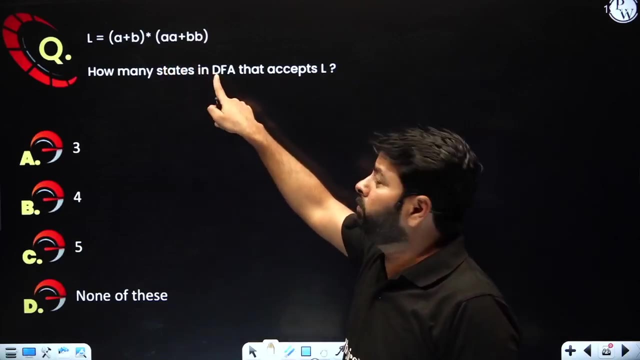 so this is a very interesting problem, and take it as homework. minimum string is w or double b that you should design and just find out how many states we'll have- four or five or six, whatever you want. okay, so this is how you can use this problem. now we are going to use the w or double b. 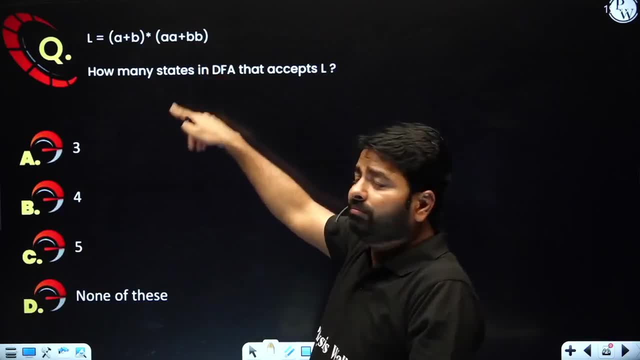 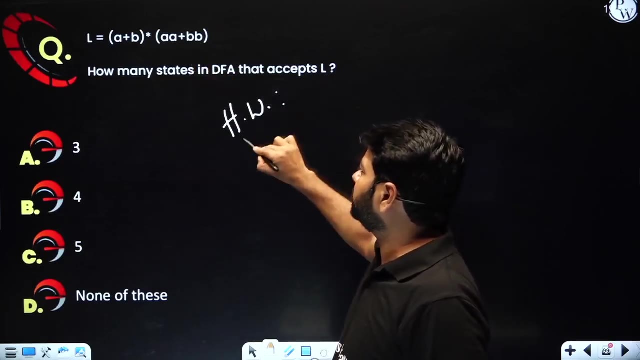 and this problem is ends with w double b. i already help. you- ends with double v. now it's ends with w r double b. you will not have the dead state here, but in the previous problem you may have debts. you will have dead state for starting condition, for ending condition. you will not have this. 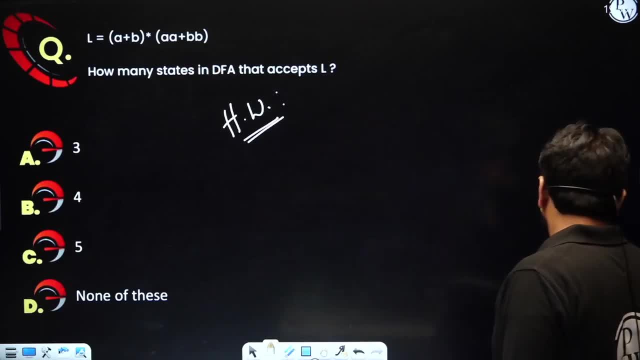 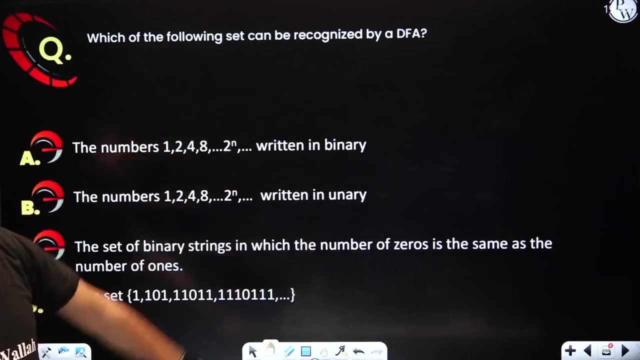 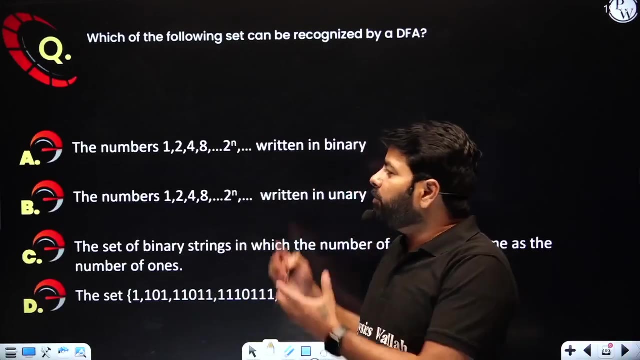 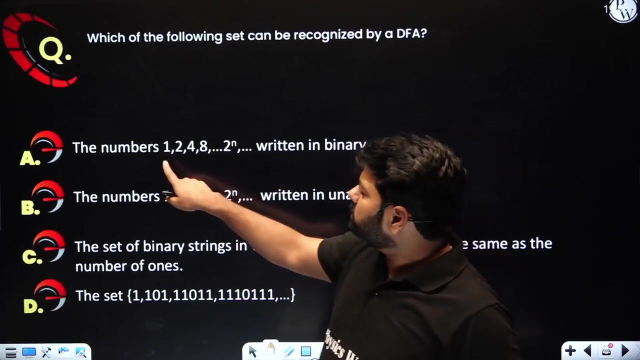 take it as homework and please discuss below this video question in the gate, which is: which of the following language can be recognized by a DFA? that means who is having a DFA, and if you can understand the problem, then only you can tell which one will have a DFA to accept. now look at the numbers 1, 2, 4, 8, 2 power n written in binary: 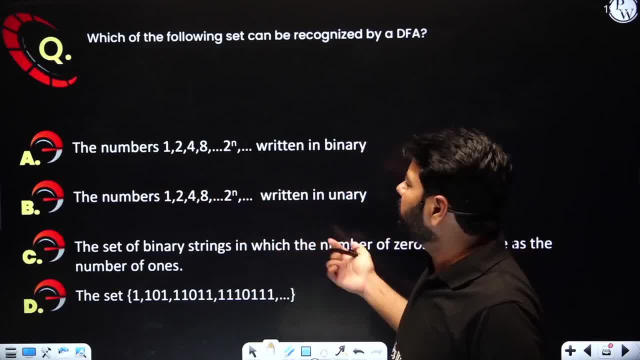 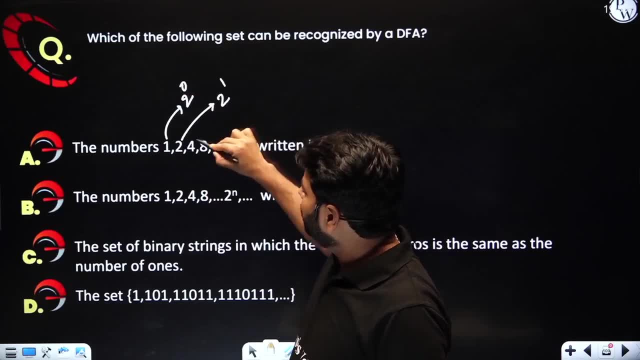 means in terms of the sigma over 0: 1 right. what is the meaning of this? how do you get this: 1, 2 power 0? how do you get this 2, 2 power 1? how do you get this 4, 2 power 2? how do you get this 8? 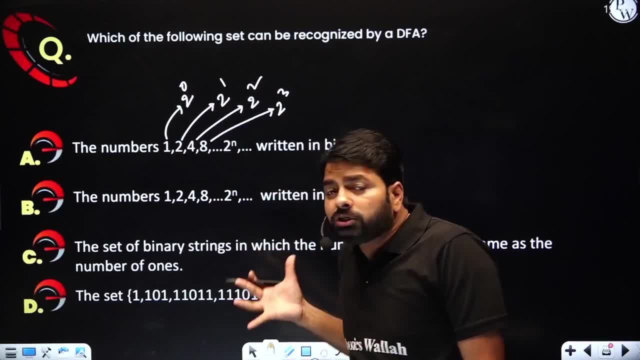 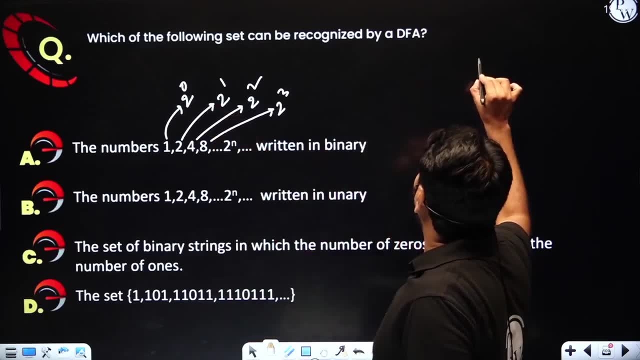 2 power 3 and so on. these numbers you wanted, but that should be written in binary. how do you write this? 2 power 0, 1, 1, right, you know that right. 2 power 0, 2 power 1- binary number. how do you? 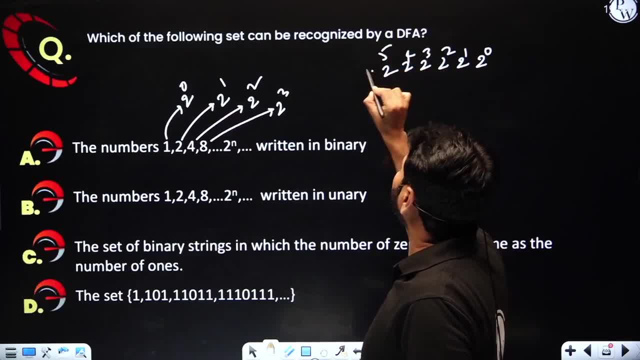 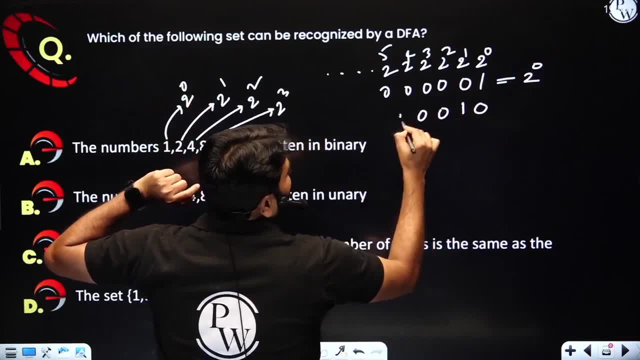 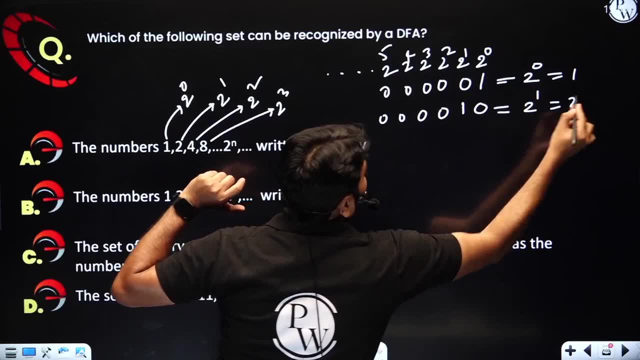 2, power 0. if I keep this 1, remaining all are 0. this is equal to 2, power 1 or 2, you can say: right, this is equal to 1, this is equal to 2, and if I keep this 1, what is that means? it is equal to. 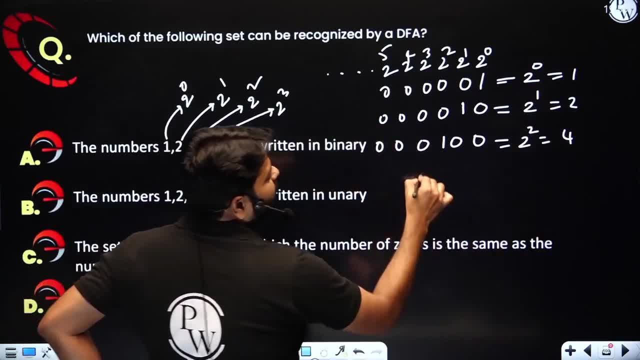 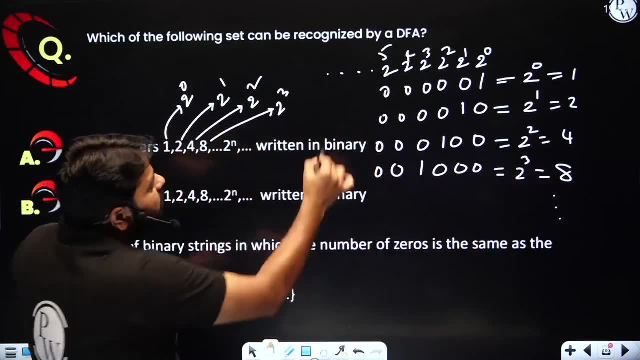 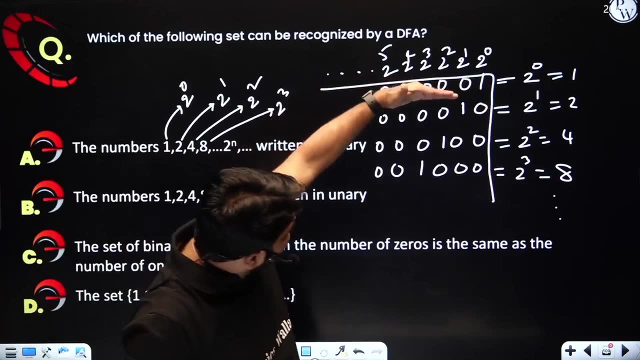 2 square, which is equal to 4, and similarly 1, remaining all are 0, which is equal to 2 power 3, nothing but 8. so now, this is your binary strings. these are your binary strings, and if you are writing in binary, can you form an expression for this? can you see that the one 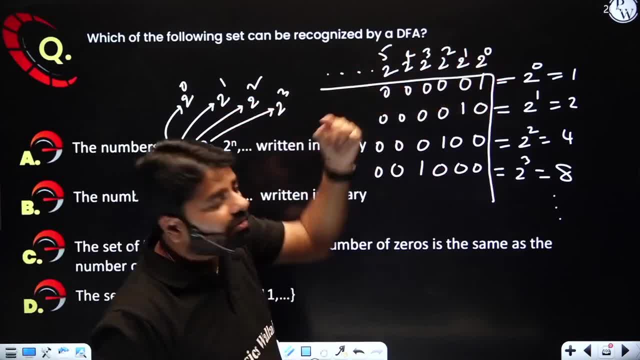 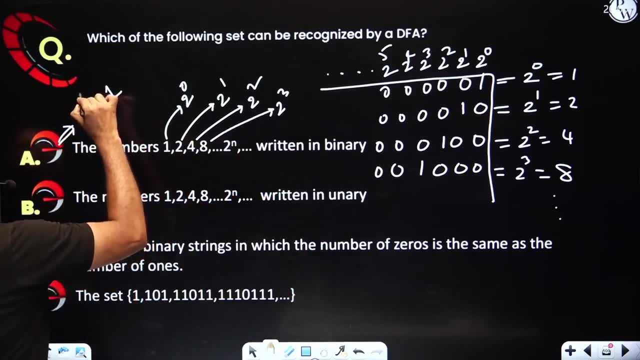 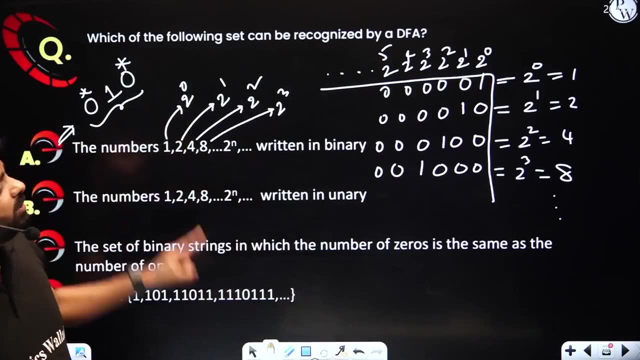 in entire sequence in the string will have only one, 1. that means for this: for this, you have a 1 before, after any number of zeros. is it regular expression or not? yes, you will have a dfa for this. no doubt, because I have written regular expression for it, right, this number will? 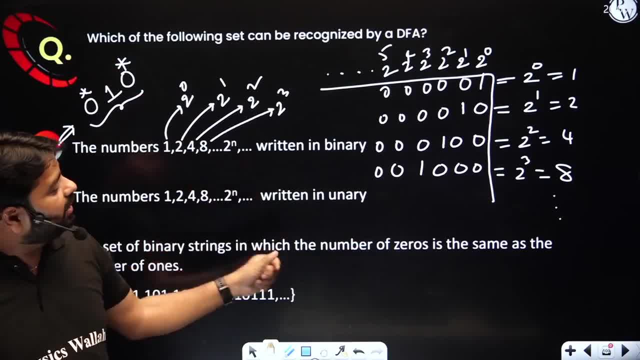 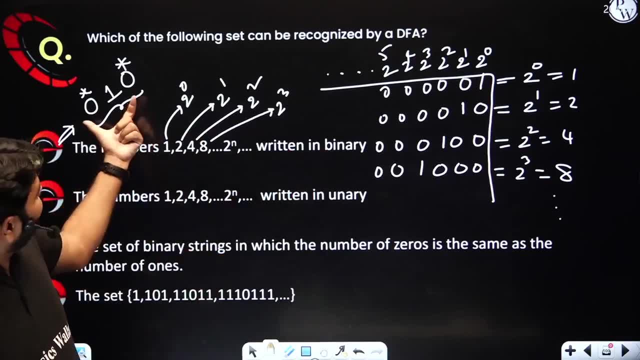 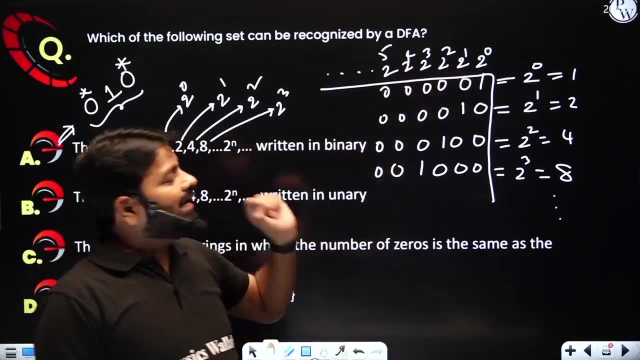 definitely give you these numbers when you convert into decimal of the binary. so when you form, when you convert them into binary- this is your binary string- it will definitely represent one of this 2 power form. okay, so, any one of this digit, only one of this. if you keep one, you will have this 2 power form because your binary number is formed based on. 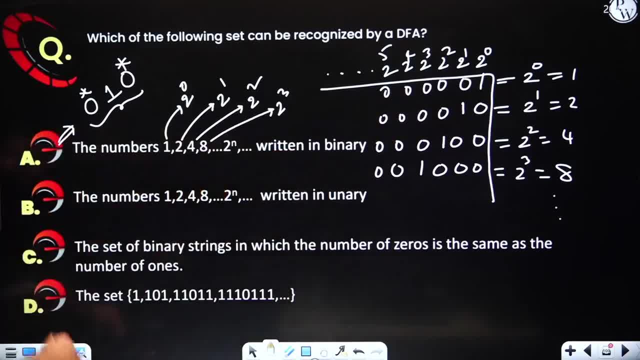 this 2 power sequence. okay, that is the reason the a will have a dfa. it's. it was mcq question, the first option itself. you got an answer, so blindly you can choose it, but you should know what are other things too. anyhow, in the coming topic finding. 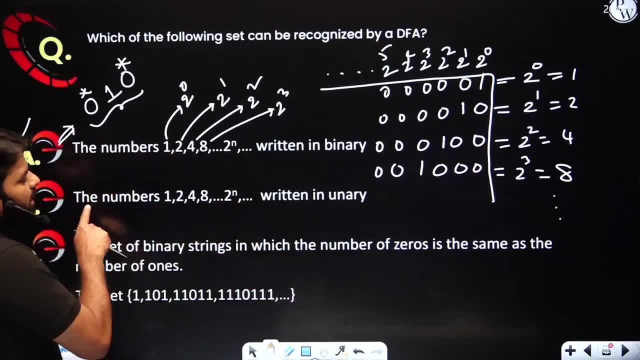 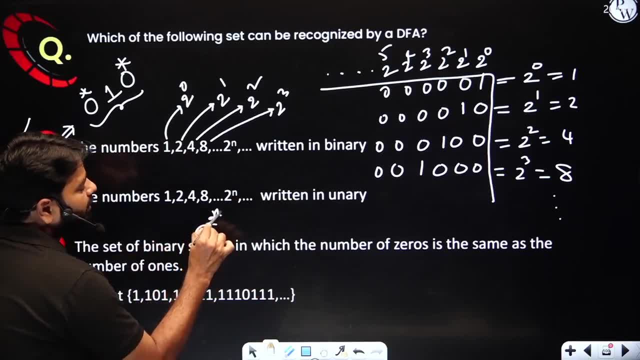 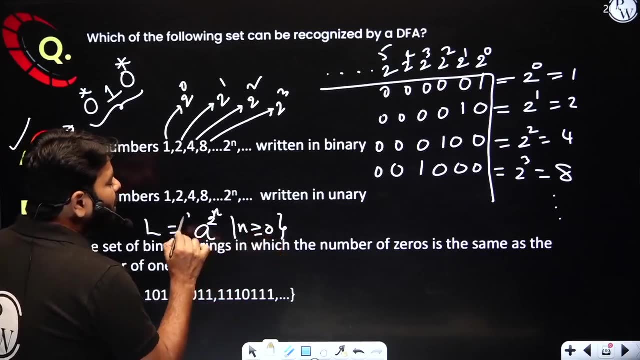 regulars, non-regulars. I'll come up with this too, but I'll explain now the numbers which are written in unary. unary means let's take symbol a, so a power 2 power n. and if the language is a power 2 power n where n is greater than or equal to 0, it will not form automatic progression. I will be. 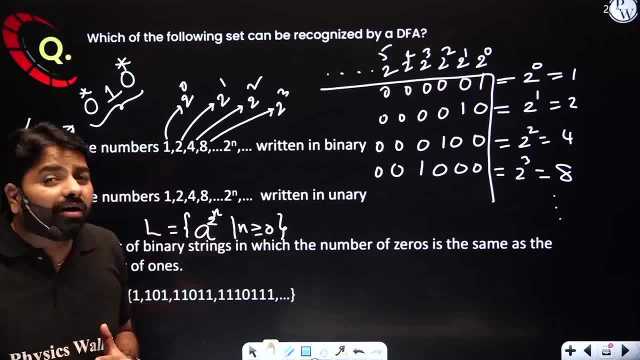 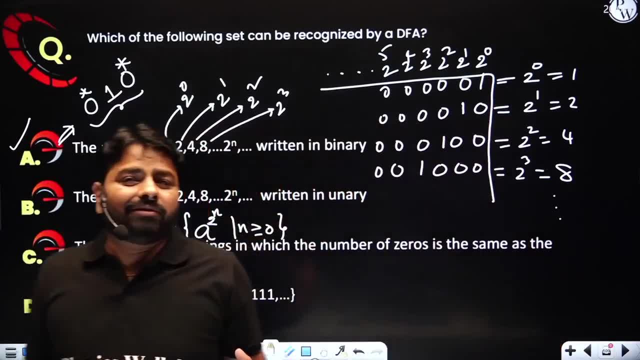 discussing this because right now our knowledge is not enough to say non-regular. I told you we are learning regulars, but non-regulars will take time. as you know, you should know a lot of regular languages and you should know property of non-regulars too. so this one, it is over one symbol. 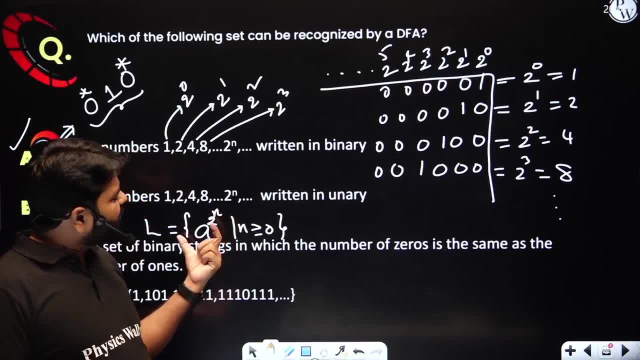 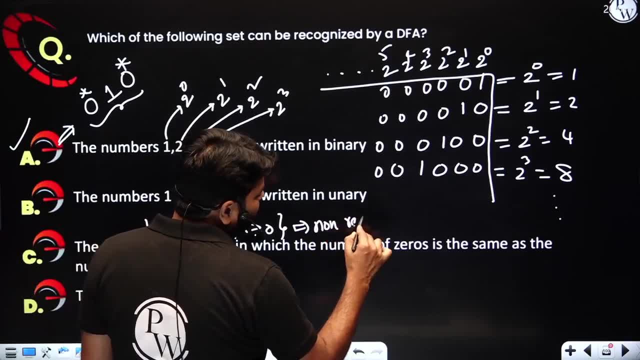 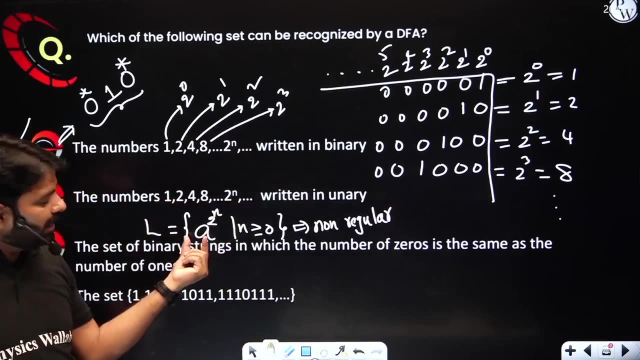 not, will not form automatic progression because 2 power n, which will not give you any cycle when you design dfa. so this is going to be non-regular. I'll show you this later on which languages are non-regular later on. right, so you can represent this. second problem, as a is one symbol, sigma over. 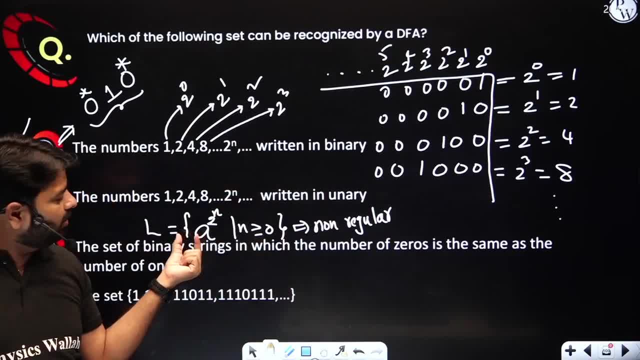 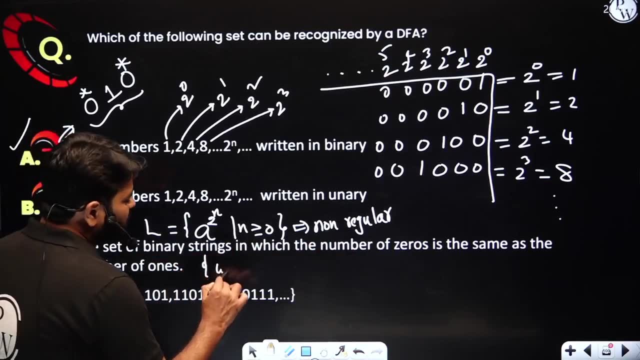 n. written in unary means one symbol. that is one symbol. I have taken a, or you can take zero, or you can take one, doesn't matter, but symbol a. power 2, power n: there is non-regular language and the set of minus strings in which the number of zeros is same as the number of ones. really, that is w such 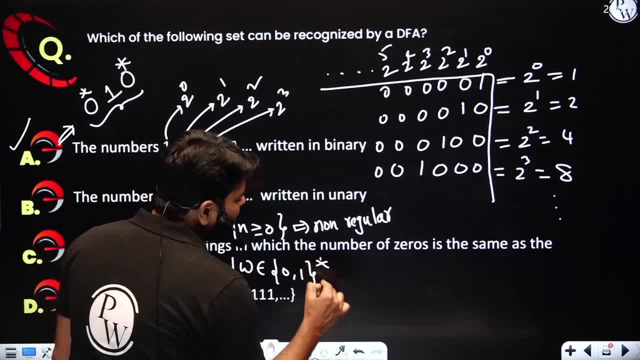 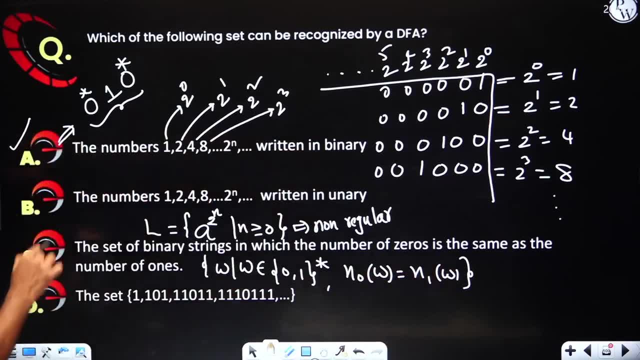 that w belongs to 0 comma 1, whole star, where number of zeros is equal to number of ones. and obviously there is a dependency which is also non-regular. and look at this: you have a 1 here, okay, 1 1 here, and double 1, double 1. there is a dependency again. 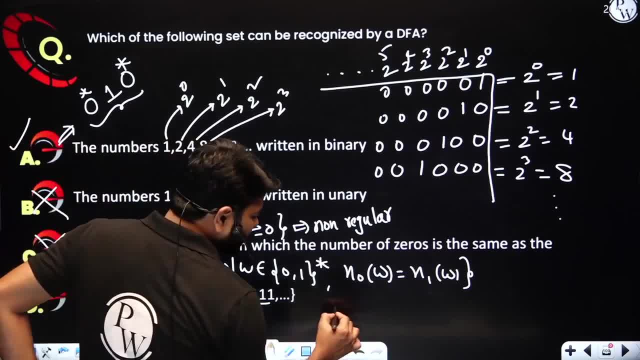 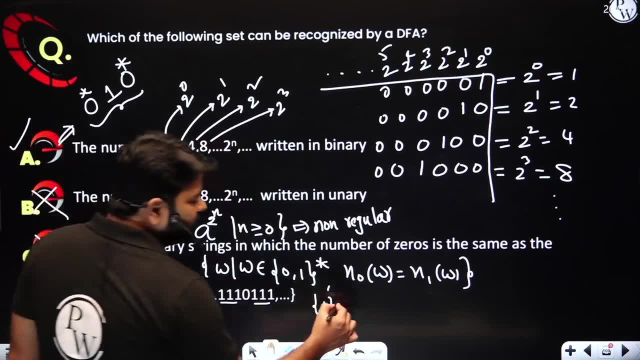 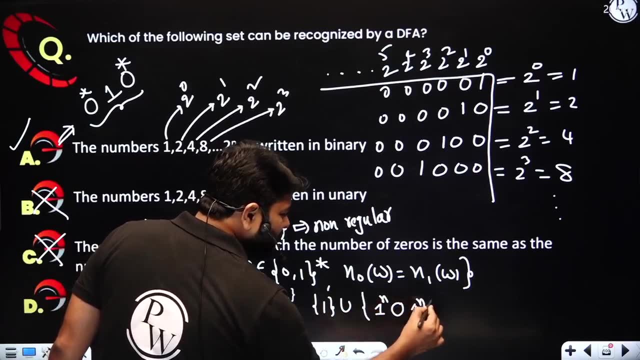 except the first string. except the first string, you see that the language 1, the first one, I have taken one separately. the remaining all, you see, union. there is a 0 and before and after the 1 power is same, yes or no, and when you look at this, of course the n has to be greater than or equal to. 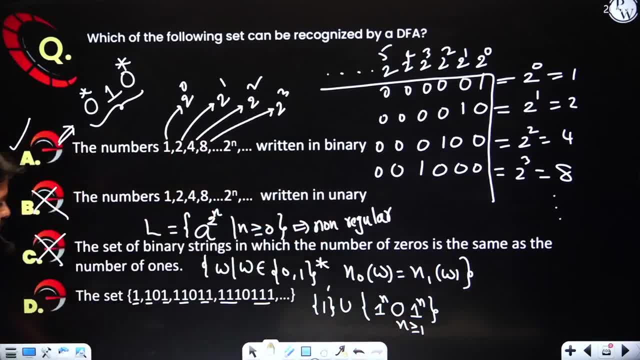 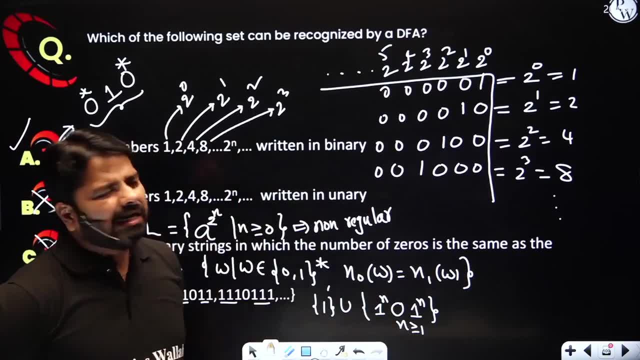 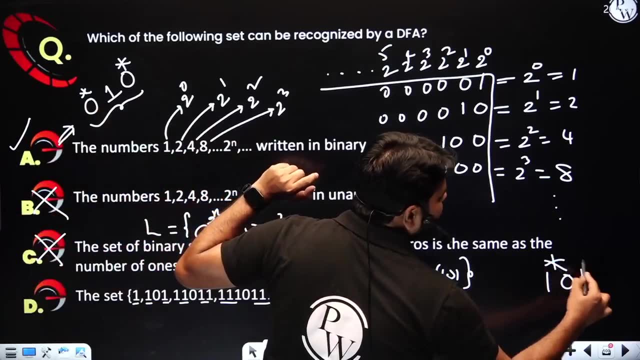 1. n has to be greater than or equal to 1. it's not 0, right. one, zero one. double one, zero, double one. triple one, zero, double one. so before zero, after zero, same number of ones. that dependency is not possible with the DFA. if you have once like this, one star, zero, one star, that's okay, you can do it. 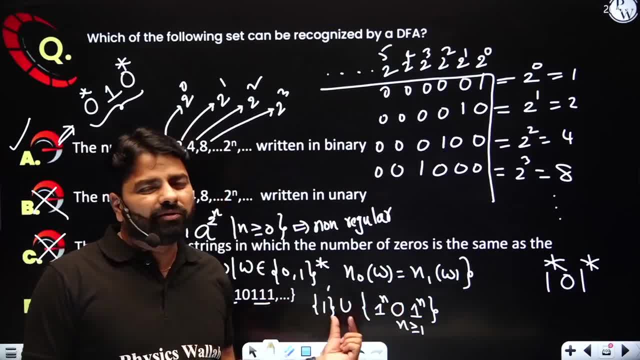 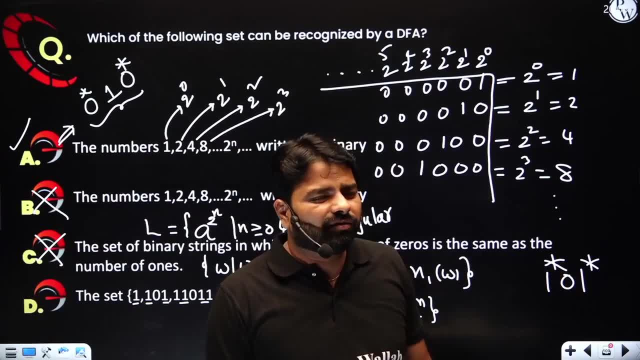 but one power and zero. one power n how do I remember? before zero, after zero, same number of ones. if you don't have any same, then I can put a self-loop before zero, after zero, I can put a self-loop for one. it will work. but you can't keep cell flow because you have a dependency. so the last three. 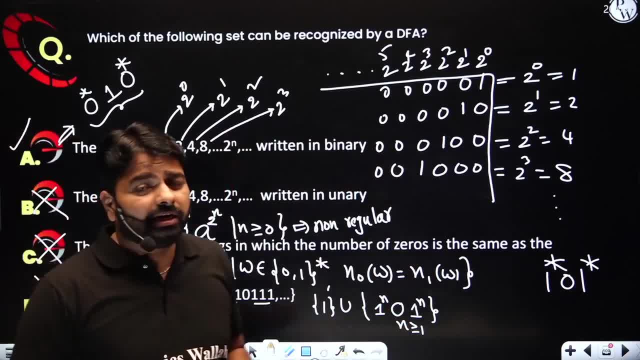 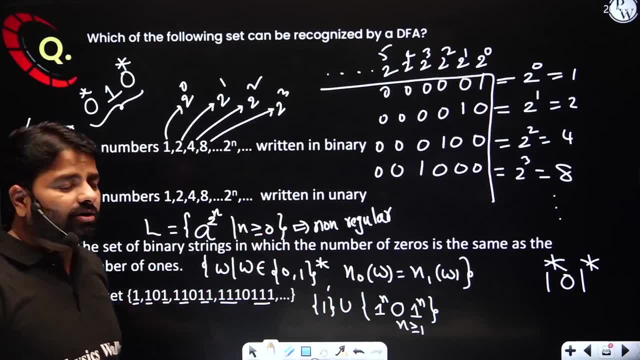 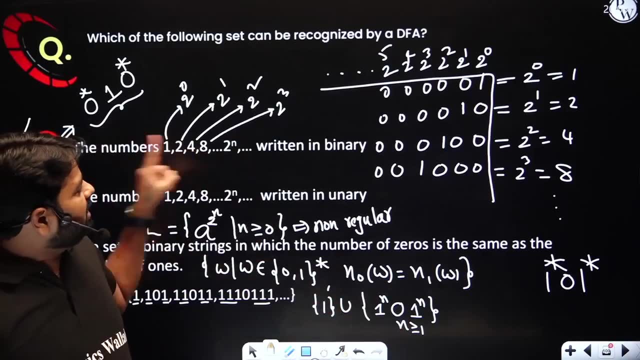 problems, you can't have a dfa and which is which is really important question. but i hope you, this question and this question and this question will be covered again in non-regulars. so there we will practice why these are non-regular again, but right now your knowledge is important, why this is. 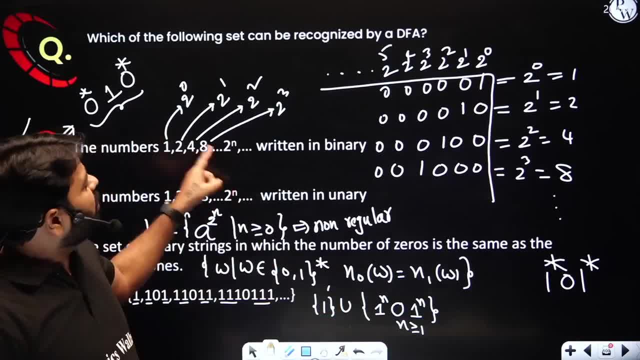 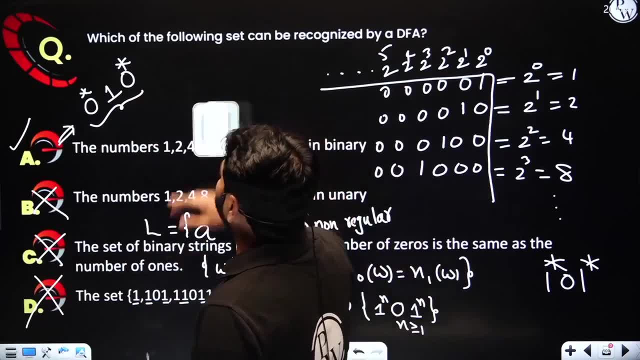 regular, or why this is having dfa? because we can design a dfa for this. can you design dfa for this, yes or no? so let's try this: dfa: 0 star. 1, 0 star minimum. one minimum string is one. what do you do? 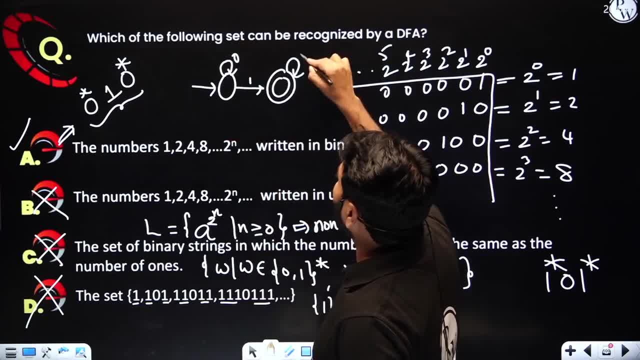 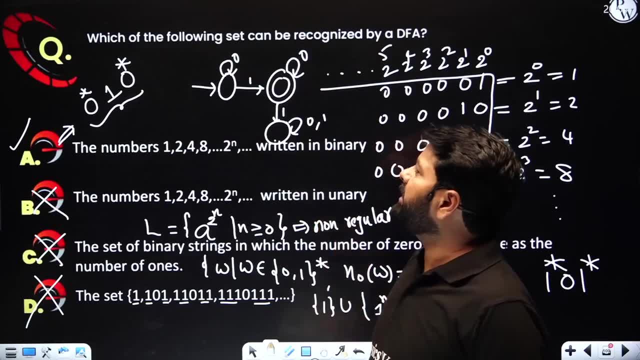 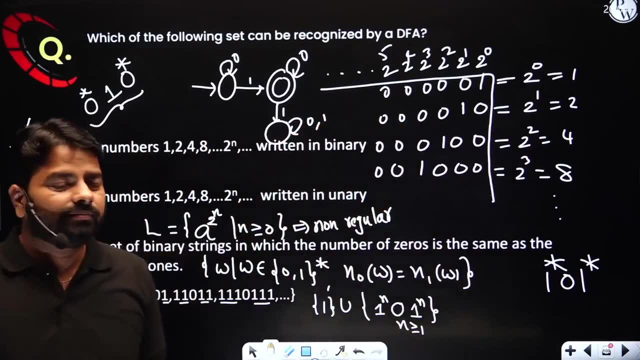 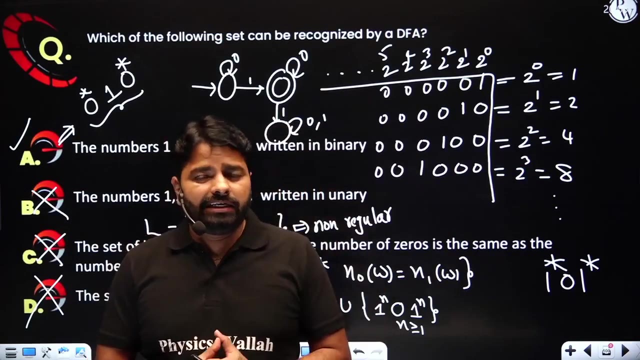 before one, any number of zeros after one, any number of zeros there after this, second one never comes. so you go to dead. that's enough over. if you design this dfa that will accept all the minus strings which are equivalent to this number. similarly, with this we have understood regular expressions and dfa, and what else is missing here is: 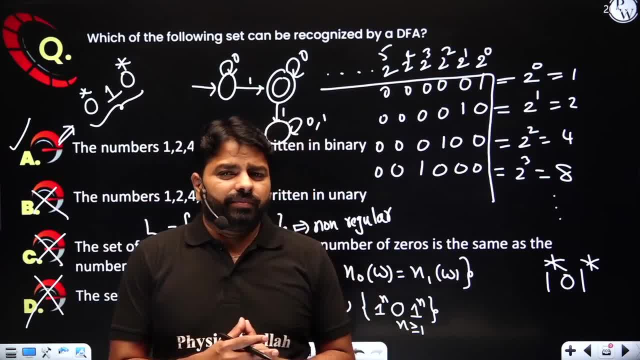 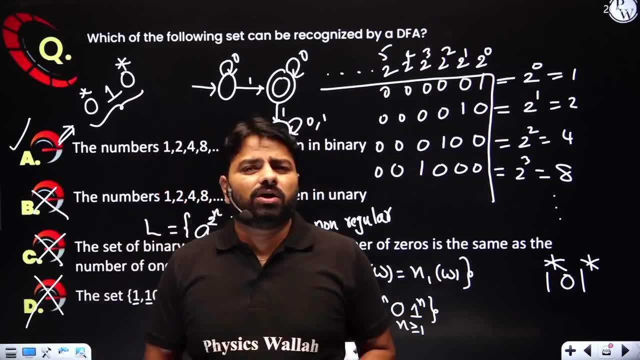 non-deterministic finite automata and some other important points will be covered in another video, but main focus is, like i have, focused on many important topics of dfa and regular expression and definitely i'll be covering in end of this video. so thank you for watching and i'll see you in the next video. 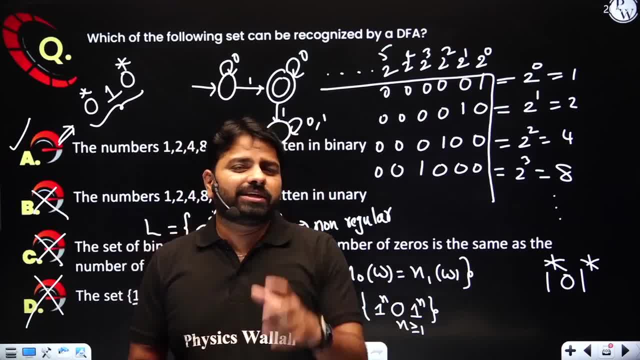 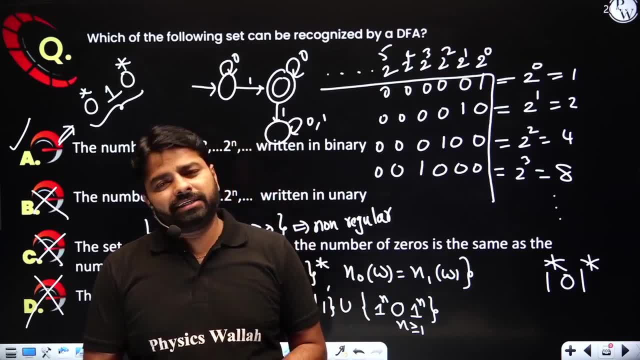 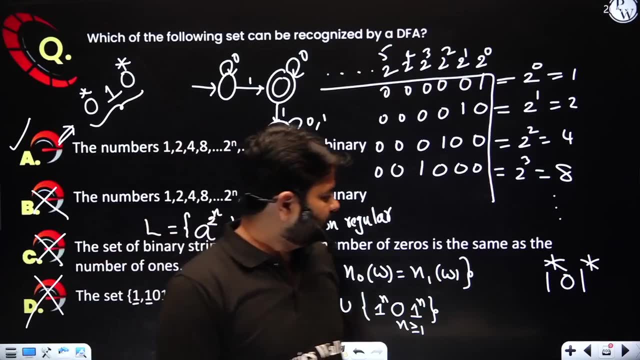 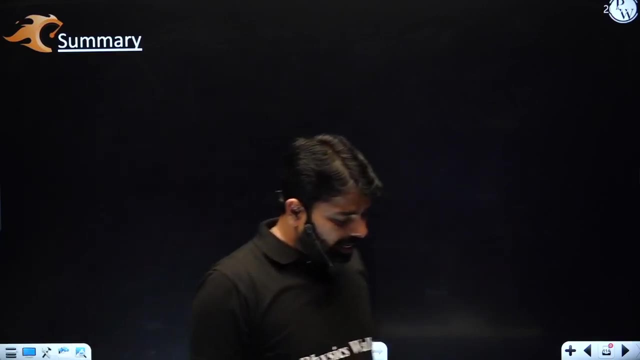 okay, so let's see you in the next video with other topic: regulars and non-regulars. so before concluding today's lecture in this lecture, in this lecture, let me explain what we have done so far. in this video we have learned the first topic: regular languages and non-regulars. 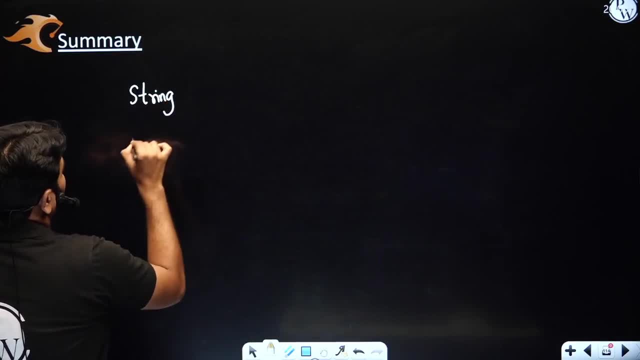 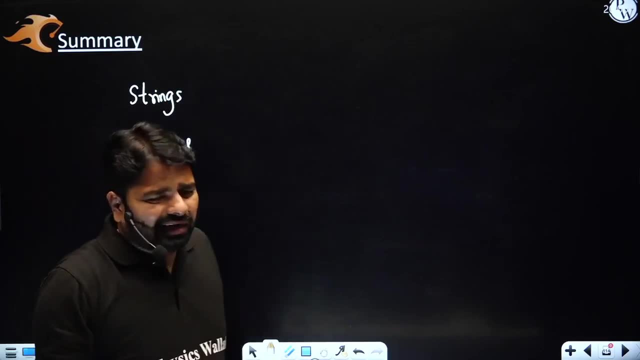 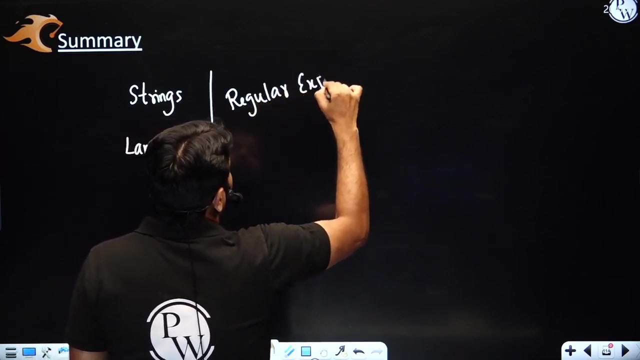 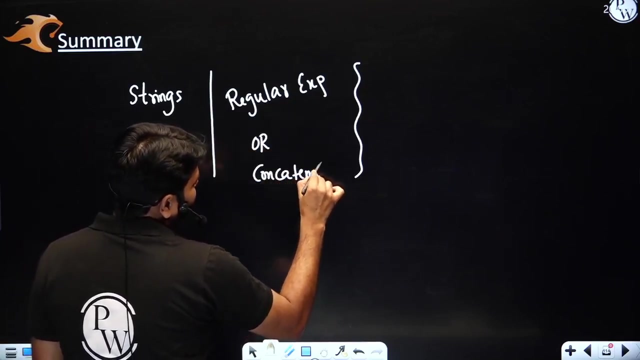 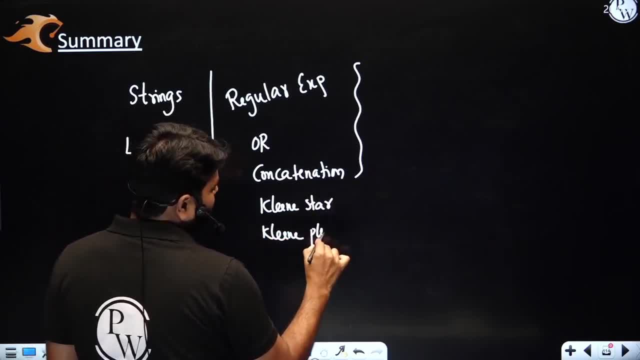 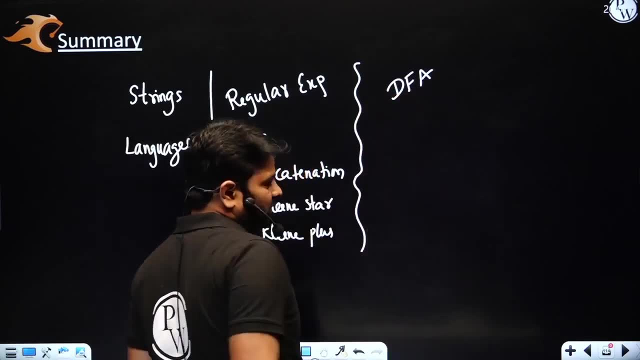 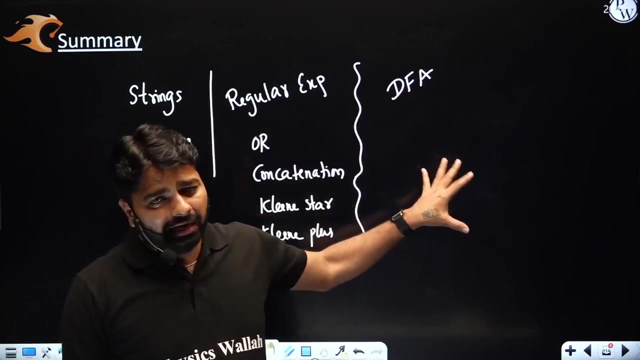 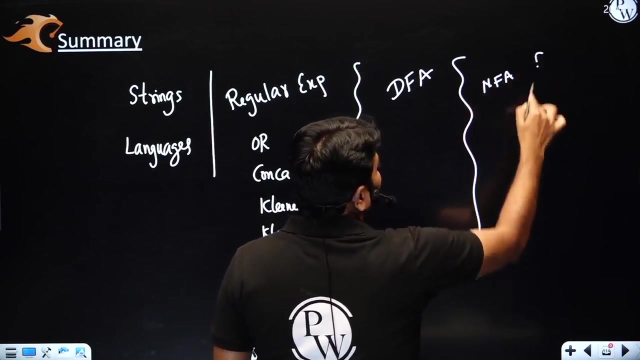 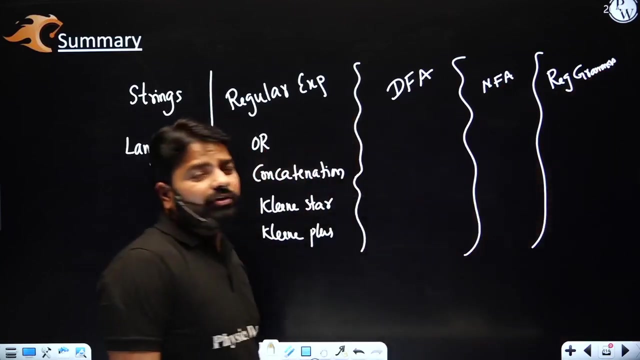 plus two unary and two binary, and then we have mostly focused on dfa to accept the languages okay. and here these two models, or these two, helps us to represent regular language. apart from this, you have other models, like nfa, regular grammars, okay, okay, which are also going to represent regular languages. so in future we will be learning.